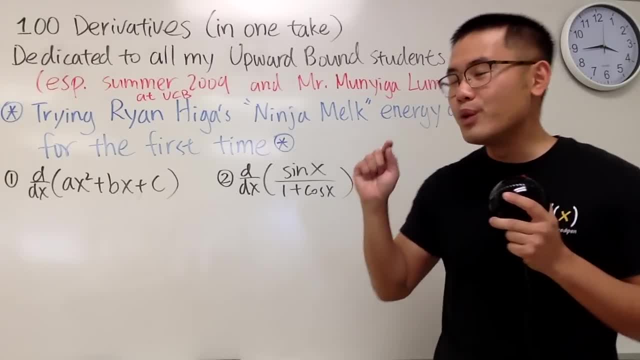 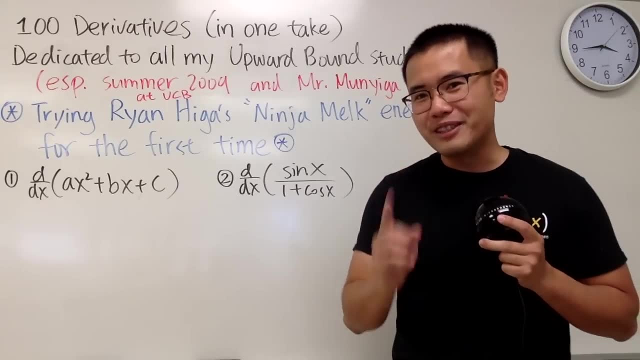 Yes, I am serious. Today, we'll be doing 100 derivatives, and we'll be doing them in one take. However, this is not the first time doing this, though, because I actually did this 10 years ago already, But let me tell you guys this: first, I would like to dedicate this video to all my 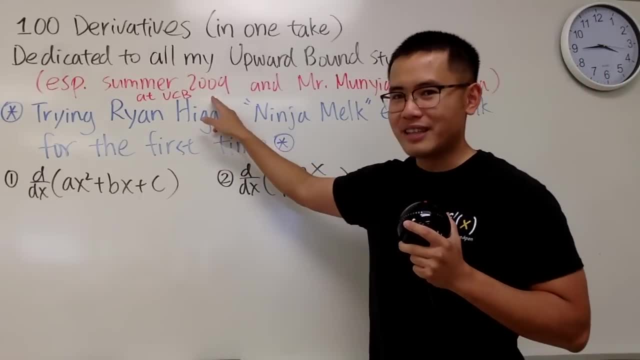 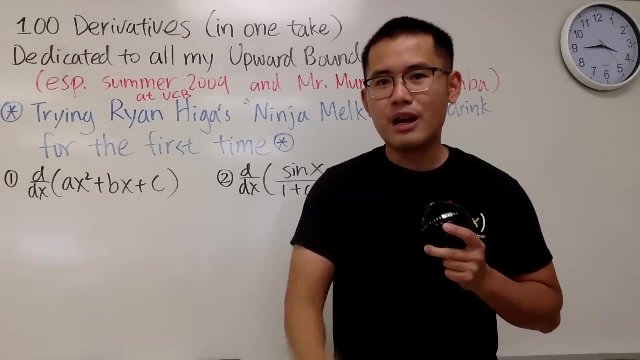 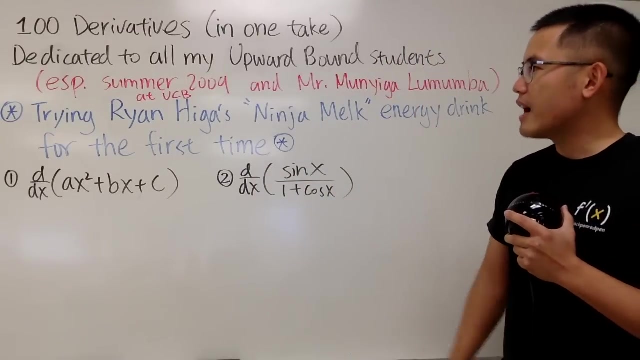 upper bound students, especially the ones in 2009, in the summer at UC Berkeley campus. And let me tell you guys, my upper bound students, I still remember everyone. I still remember you guys. It was such a wonderful experience that we had And that was the second time that I had my own. 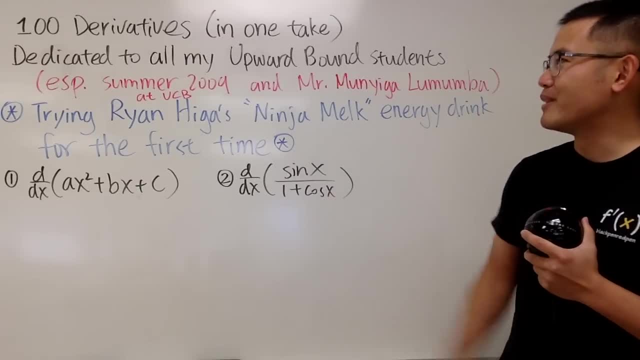 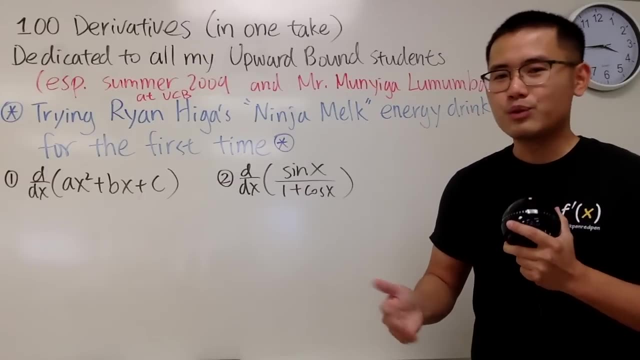 class. I taught my own calculus class during the summer And the upper bound. you know it's a program that helps high school students who are from low-income family, just like myself as well, And I, of course, have to thank my director. 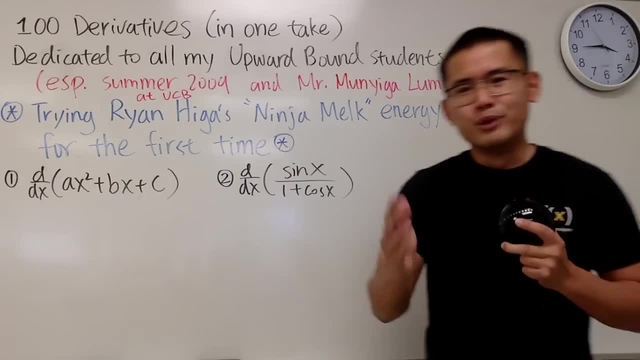 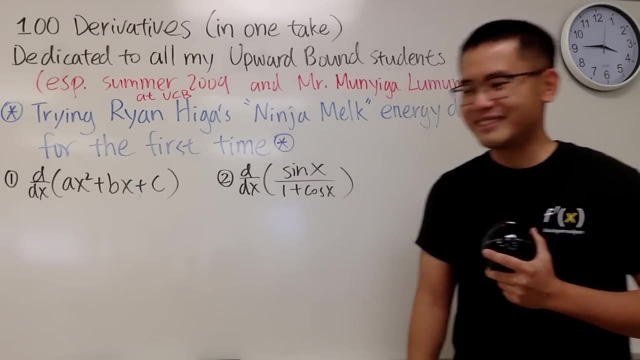 my main man, Mr Muniga Lamumba Mun. thank you so much for believing in me. Thank you so much for giving me so many chances to teach the class. I will tell you. of course, I cannot be who I am. 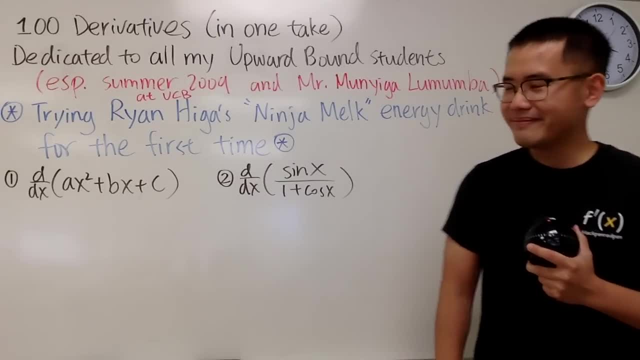 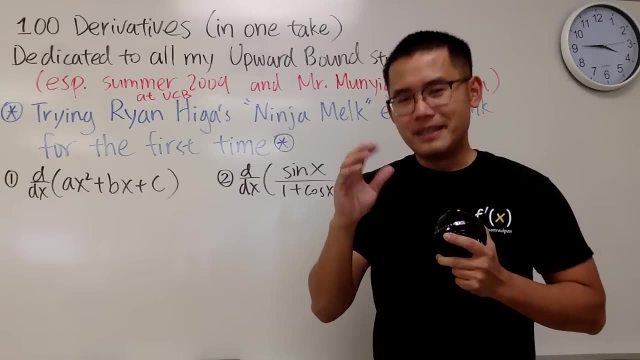 today. I cannot thank you enough. Thank you All right. So 10 years ago I actually did a PDF because I teach my class right And I decided to produce enough examples for my students, And how many examples are enough. 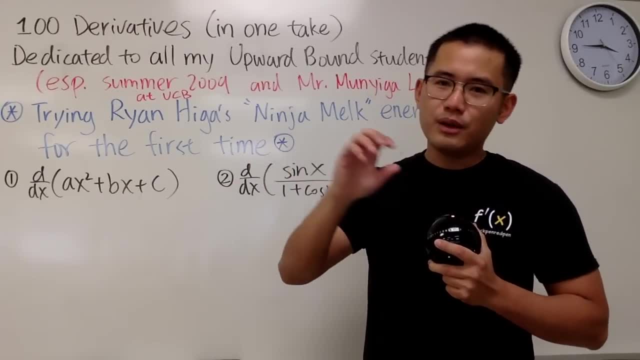 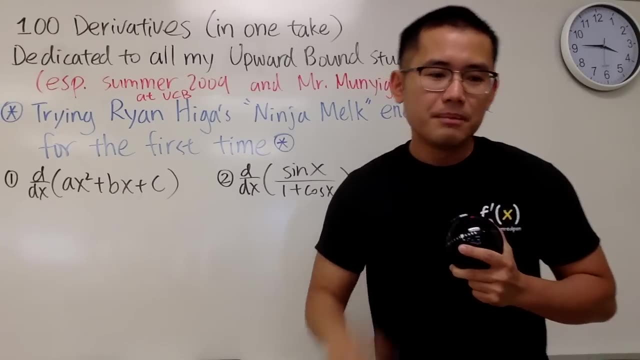 It came out with 100 derivatives, questions and also solutions, And typing them up, you guys can find the link to the PDF. I will have that in the description for you guys, But today, though, we'll be doing something different. I have this right here for you guys. 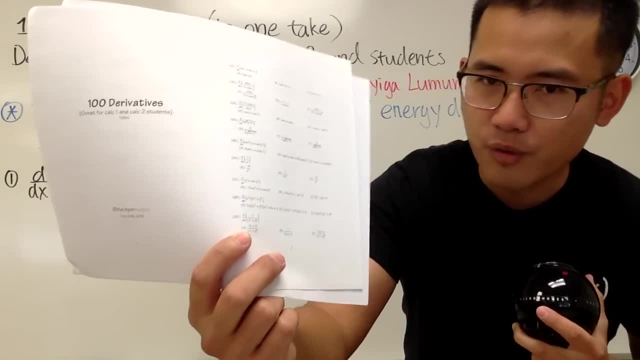 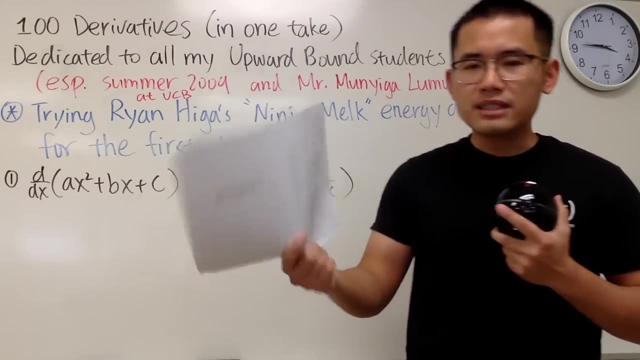 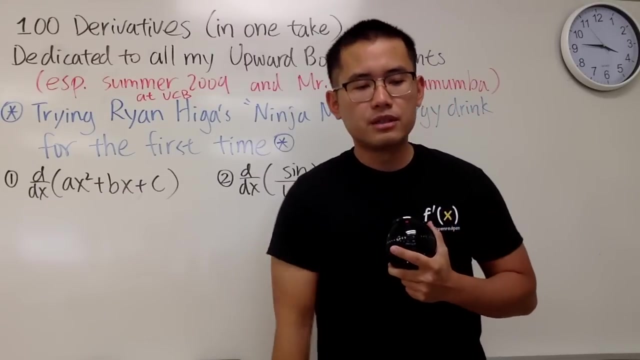 And notice that the questions here they are in a multiple choice format because I believe it's the best when you have derivative questions with multiple choice format, because sometimes you don't know how much more you have to simplify, how much more you have to keep going or when to stop, So multiple choice format is the best. 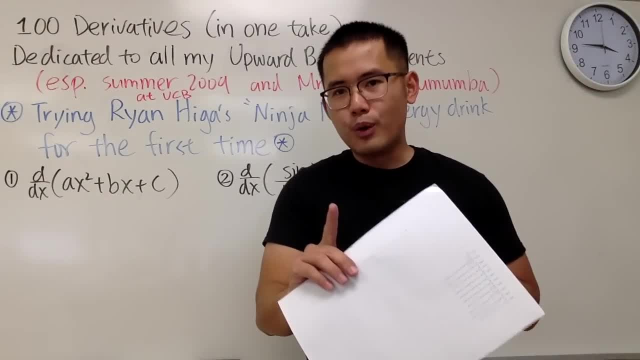 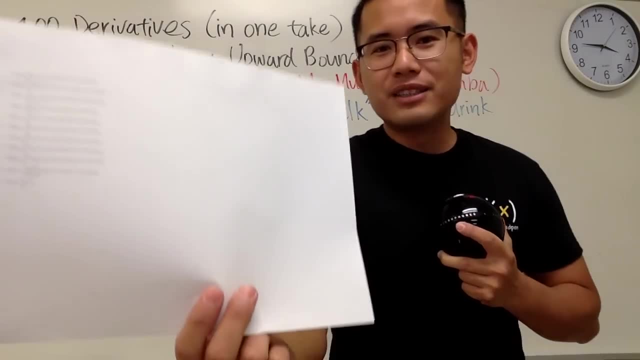 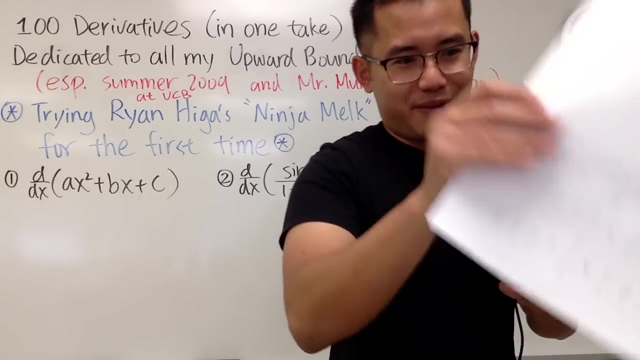 for derivative questions And for the people who would like to know this: yes, of course. how can we have derivatives without the definition, right? So if you guys would like the last 10 questions were solved, yes, derivative by using the definition, But the first 90 question. 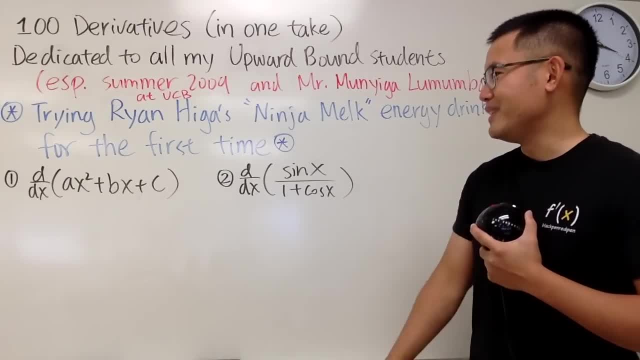 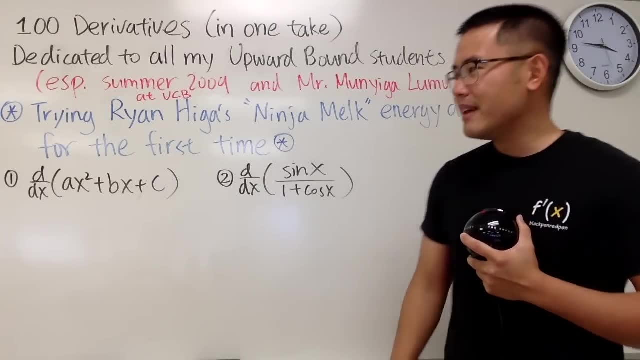 would be: just we use the rules that we have known already. okay, all that. So this is going to be good for Cal 1,, Cal 2, and hopefully you guys all enjoy this, And in fact, today I have something fun. 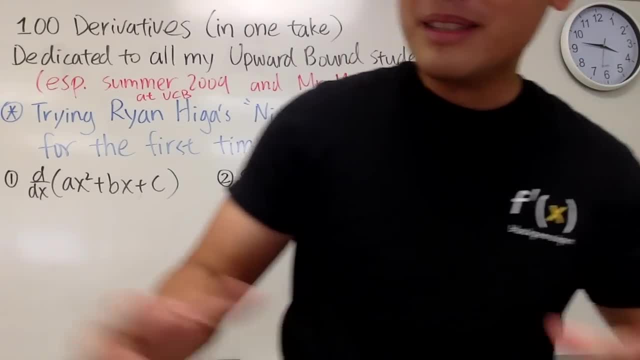 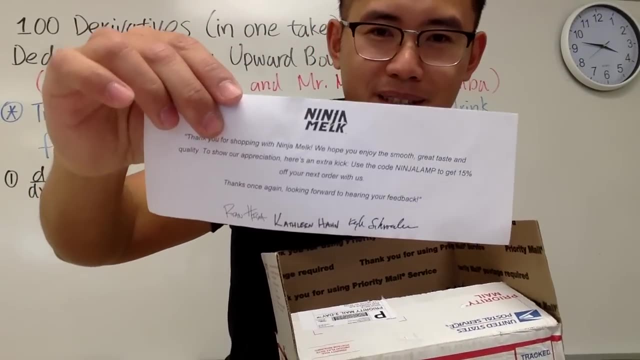 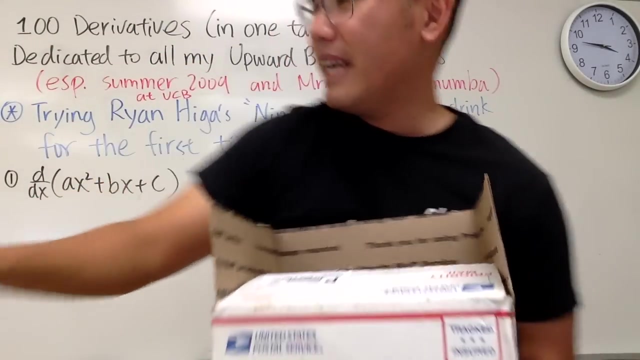 Let me just show you guys this right here. I bought this recently. I bought this recently and I opened it. This is called the Ninja Milk- M-E-L-K- M-E-L-K, so Ninja Milk from Ryan Higa, And I will be trying his energy drink for the first time, So you guys can see. 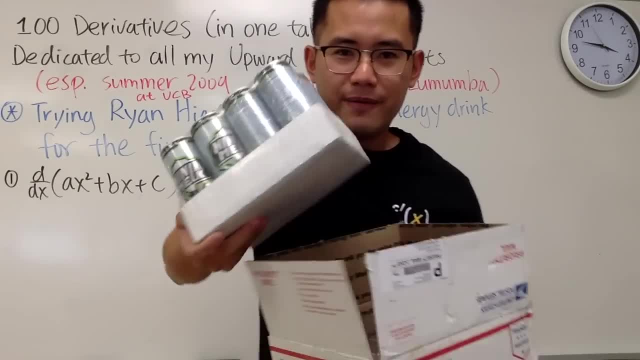 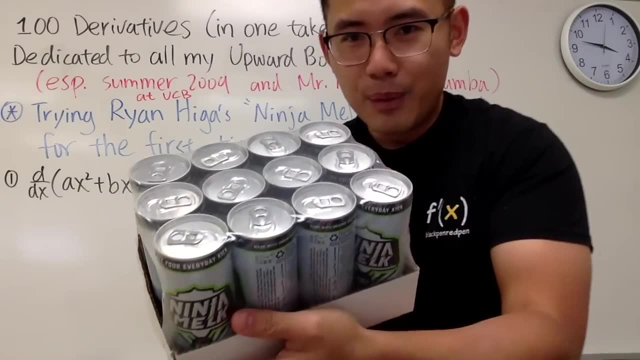 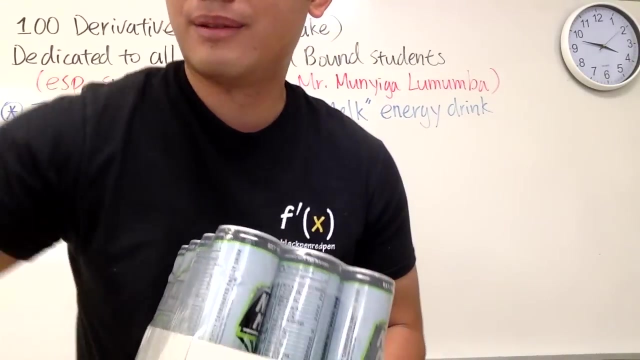 I have this package right here, right? So I haven't opened the package yet. So I will show you guys. I will tell you guys how it tastes, but not now, because right now I have enough energy, so I don't need it yet. I don't know how long this will take me. 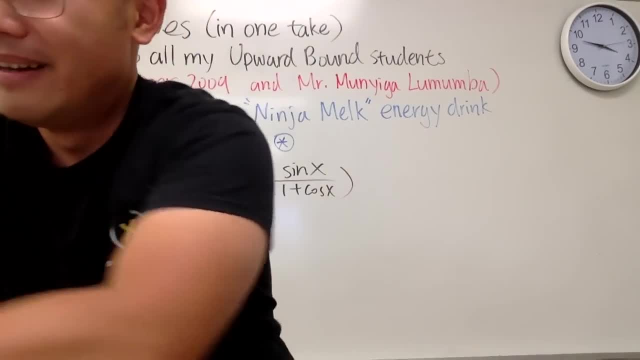 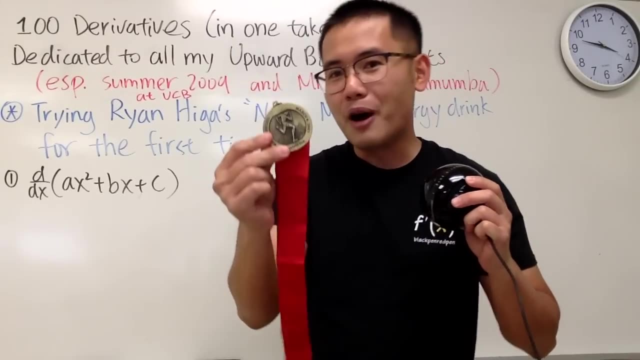 though, so I don't know how many I'll be drinking, so I don't know. And of course, I have my Marathon medal. This is the one from 2007, and in fact, this is the one from 2009.. And you might be wondering why don't I bring the one that's from? 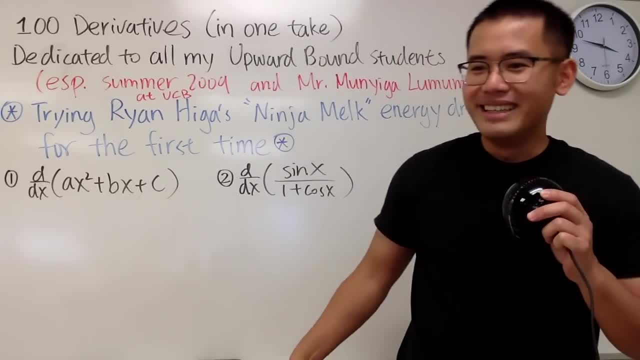 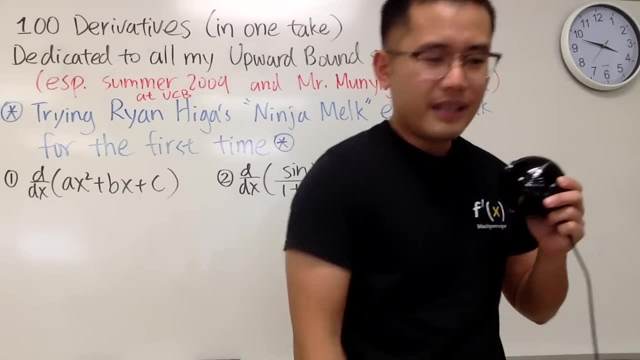 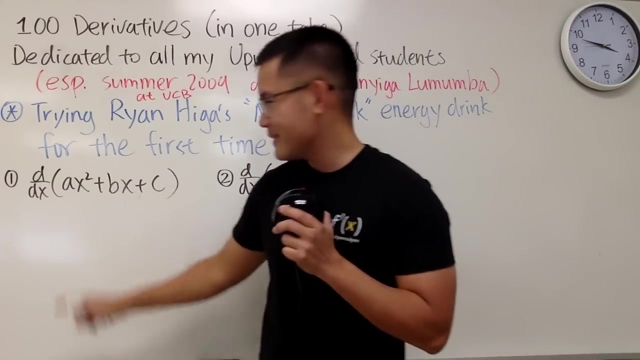 2009?? Unfortunately, I didn't run that one in 2009.. All right, anyway, you guys can find the PDF in the description right here. right? So yeah, All right, here we go. First question: we are going to be differentiating x squared plus bx plus c. Notice that a, b, c are just constants. 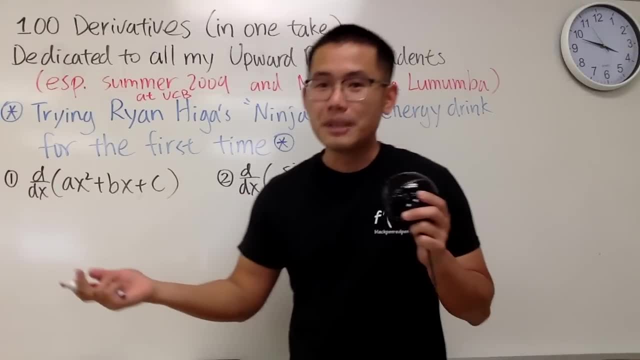 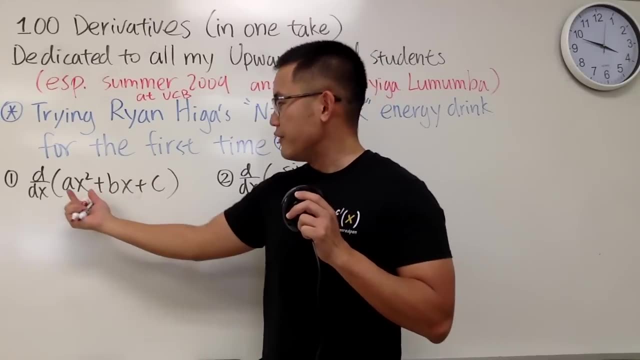 so for the first one, we'll just start something easy. This is just the power rule, and the idea is that whenever you're adding or subtracting- right, but this is just all adding- you can just differentiate the first and then differentiate the second. 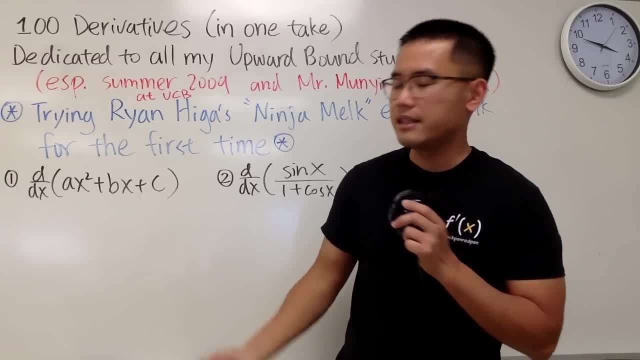 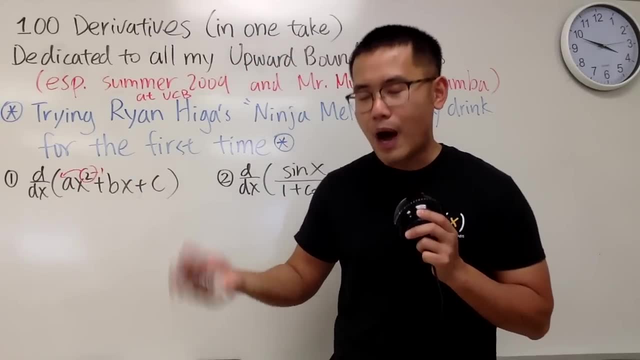 and differentiate the third and then just put the results together. That's it. So for the first one, for this right here, I will just bring the two to the front and then minus one. That's the Google Power rule, right? So the first term we'll get 2a and then x to the first. 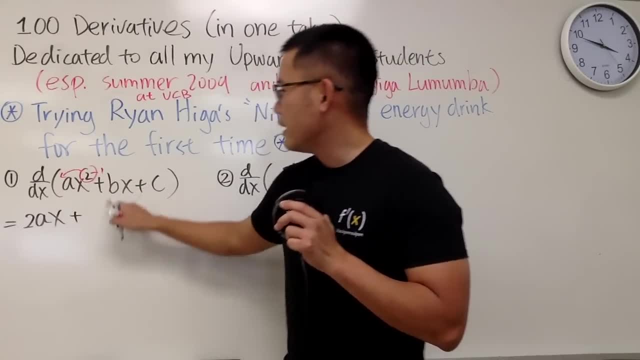 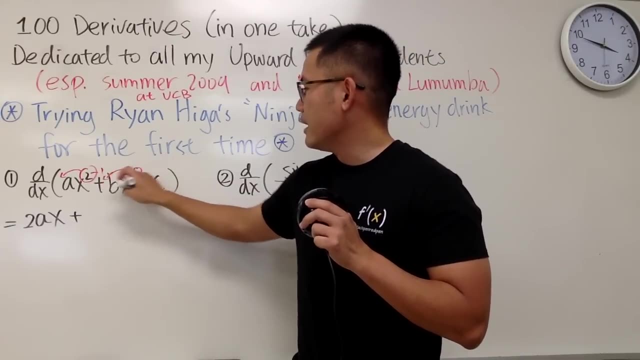 one. You don't have to put on the one And then the next one is plus. When we have b times x to the first power, well, you can put on the one right here, You can bring the one to the front and then. 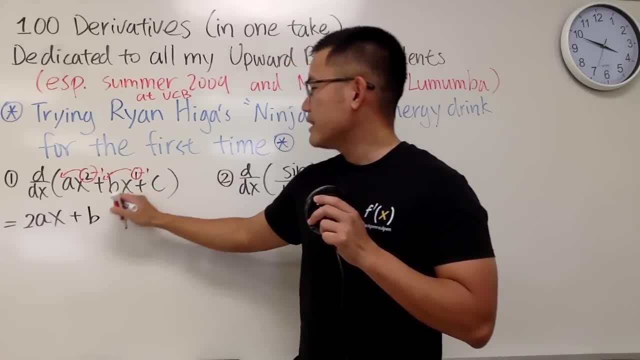 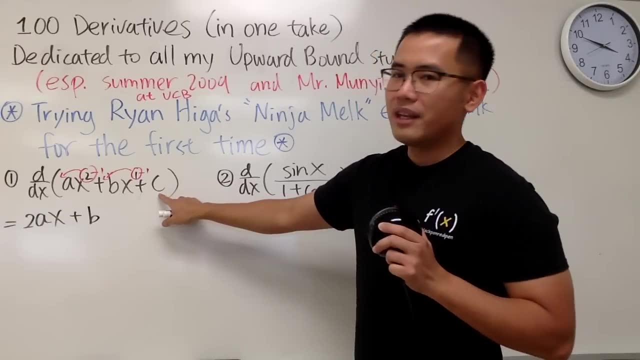 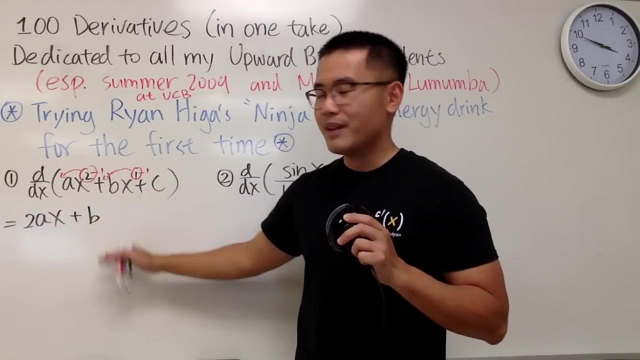 minus one One times b is just b, and x to the zero's power is just one. So it's just b, It's just the coefficient of x. Lastly, this right here is just a constant. So when you differentiate a constant c, when there's no x, the derivative of this is just going to be zero. So you don't even. 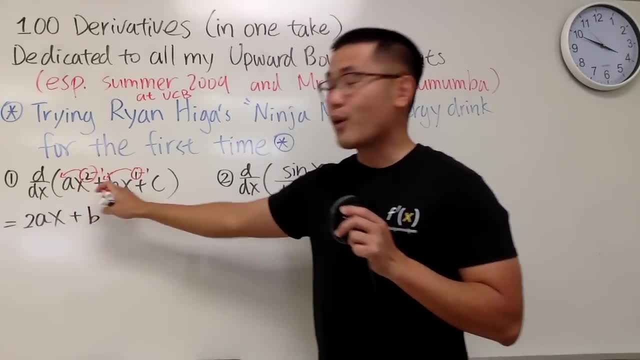 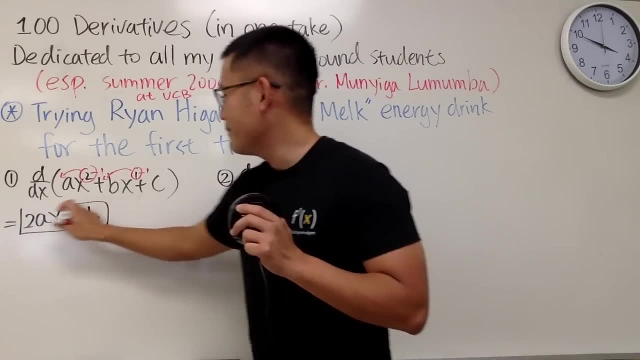 have to put that down. So for the first one, the derivative of a quadratic is just 2ax plus b, and that's it. Start with something easy, right, And I'm not going to give you guys the answer key. Hopefully. 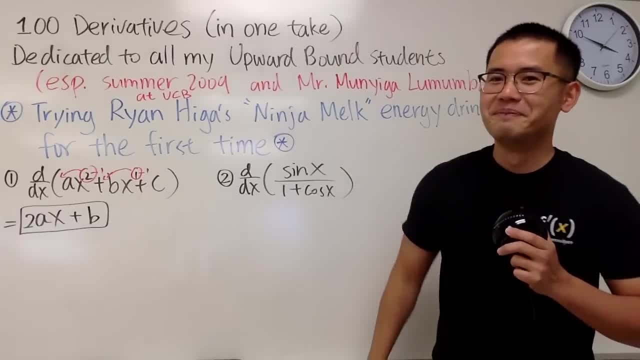 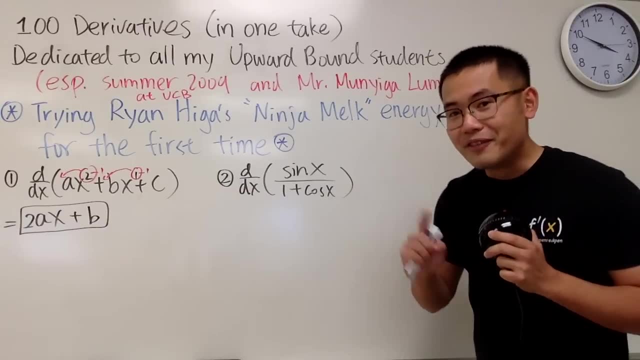 you guys can all figure this out. So there's a nice pattern. You guys can let me know in the comment down below and let me know what the pattern is. Anyway, second one: we'll be differentiating sine x over 1 plus cosine x. Notice that this is a. 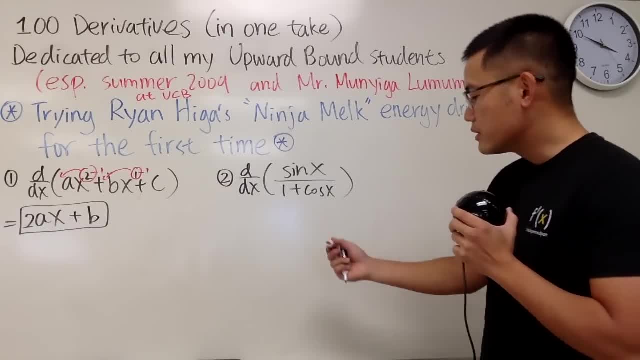 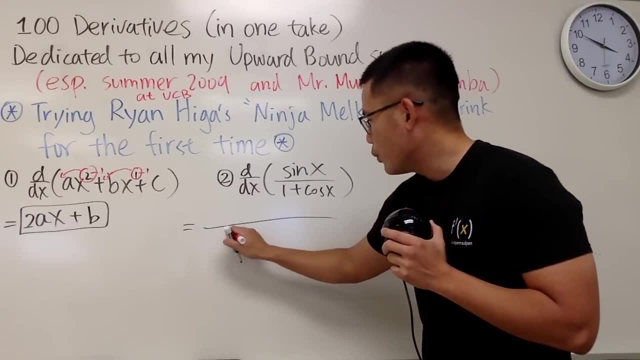 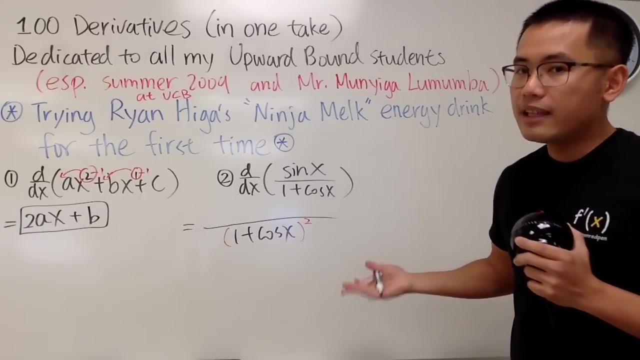 abbreviated equation and we'll be just using the quotient rule for this. So here we go. Before we forget, let's go ahead and square the denominator. So we will have 1 plus cosine x and we will raise that to the second power, And then the quotient rule says we will have: 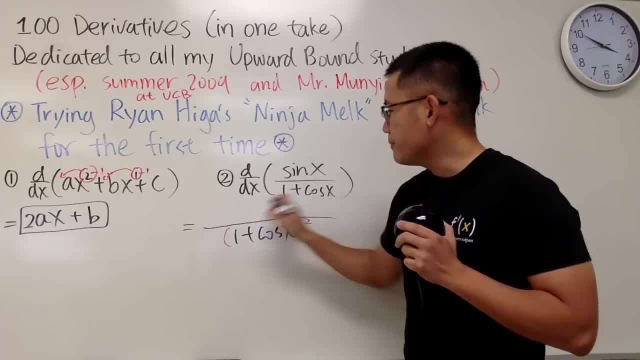 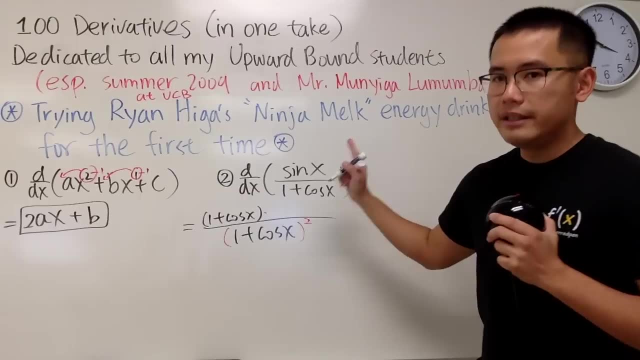 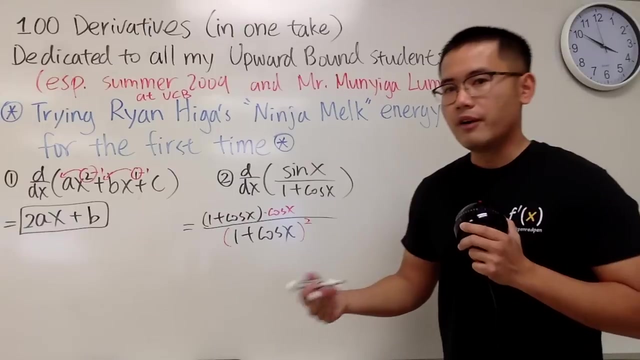 to put the denominator to the top right here. So let me just write down 1 plus cosine x, And then we multiply by the derivative of the top. The derivative of sine x is just going to give us cosine x, And of course you have to know all the derivatives of the functions, right? 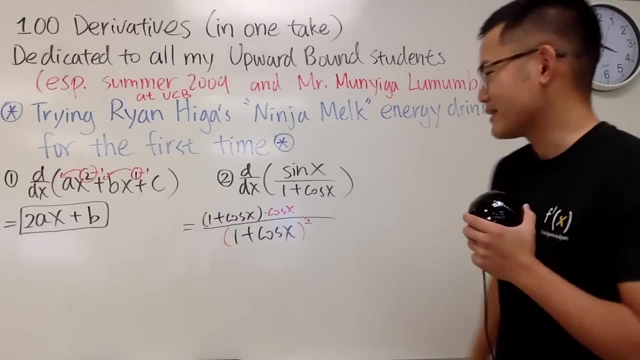 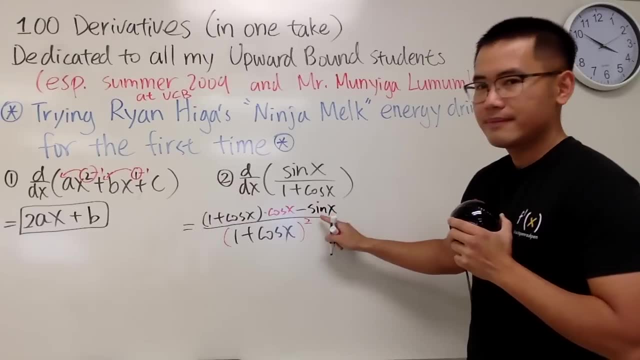 Hmm, Yeah, so you have to know that. Alright, so you have all this, and then you have to subtract the top function, which is sine x, And then multiply by the derivative of the bottom function. The derivative of 1 is 0.. 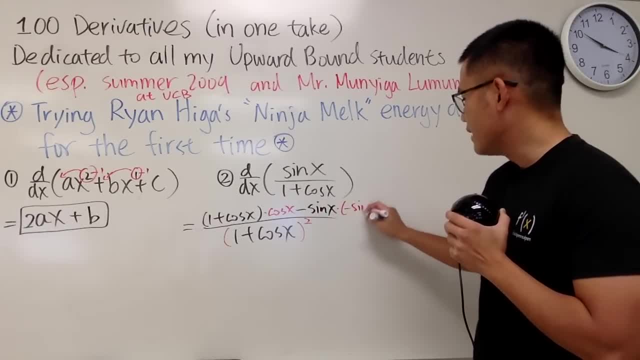 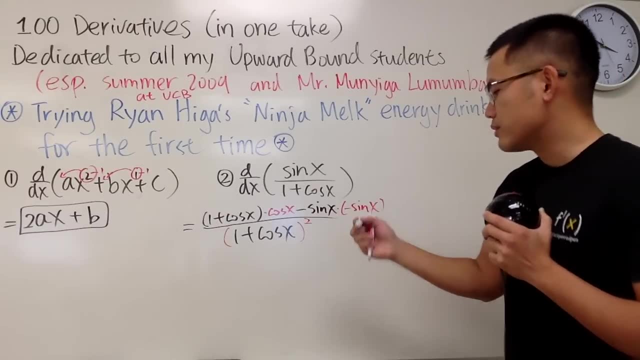 The derivative of cosine x is negative sine. So we have negative sine x right here And now. this is the time that you have to think about how we can simplify all the expressions right here. Well, of course, we can just distribute the top right here. 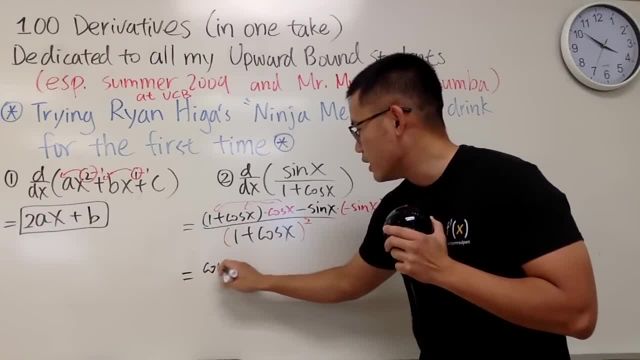 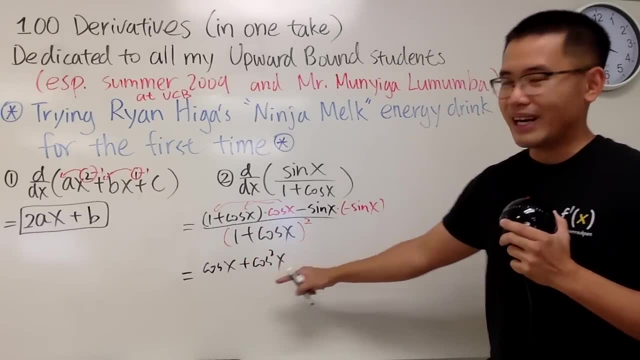 So we'll do that, do that. So cosine times 1 is just cosine x, Cosine times cosine is cosine squared x, And we put the power 2 right here, right, Cosine x, and then squared, And then negative. negative becomes positive. 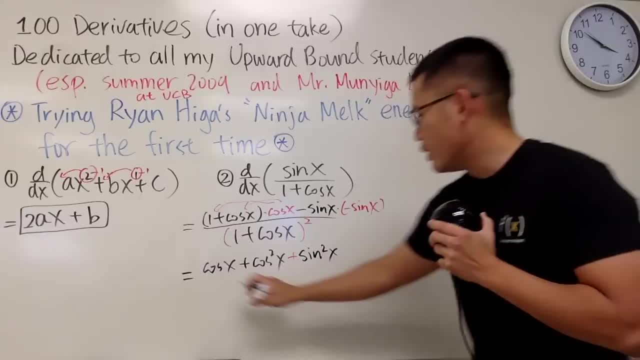 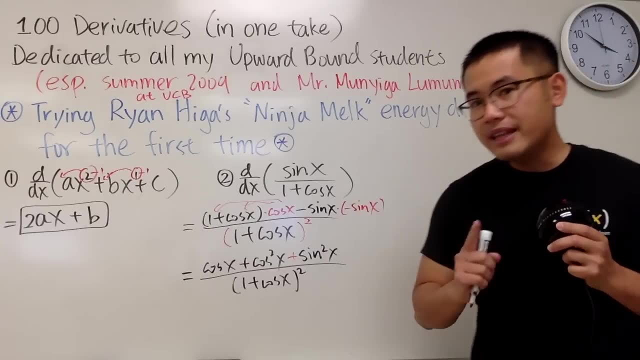 And then sine Times. sine x is of course just sine squared x Over the denominator right here, which is 1 plus cosine x squared. And now check this out: Here we have cosine squared x plus sine squared x. Guess what? 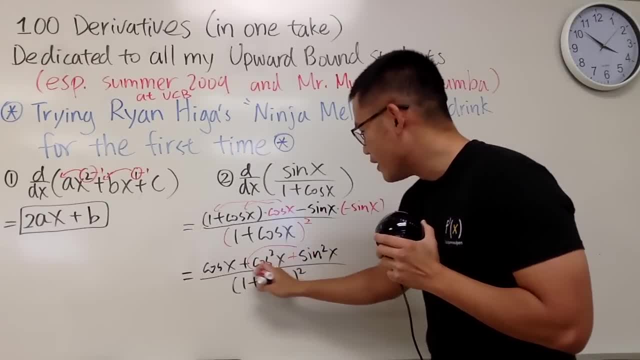 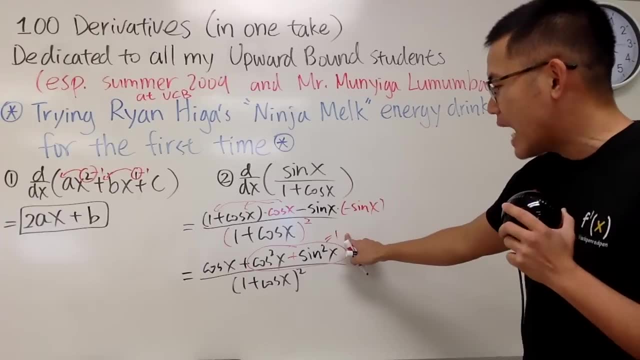 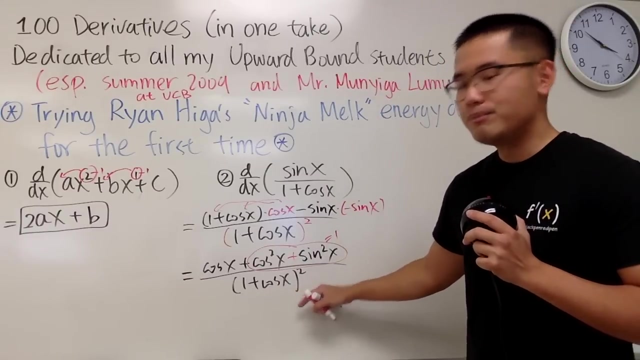 Yes, we can use a nice trig identity for this. This right here is nicely equal to 1.. So we just have a 1 right here. In fact, on the top we have 1 plus cosine x, And then we have 1 plus cosine x squared. 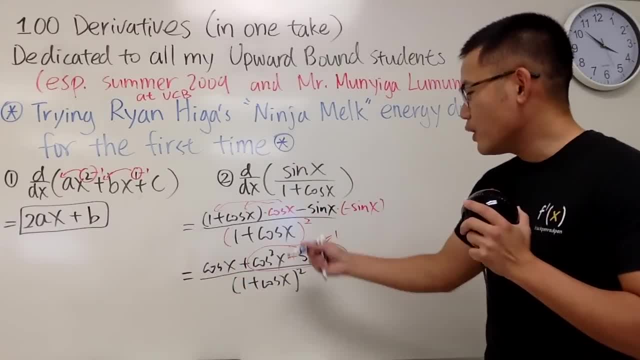 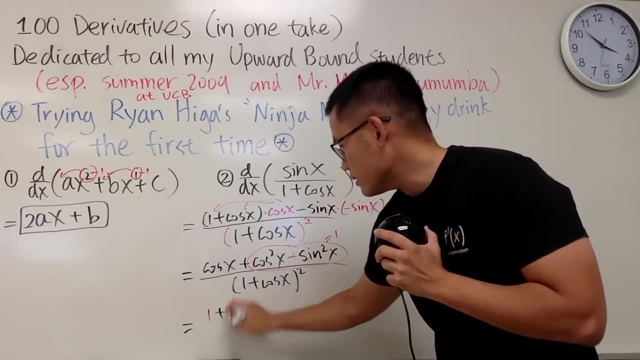 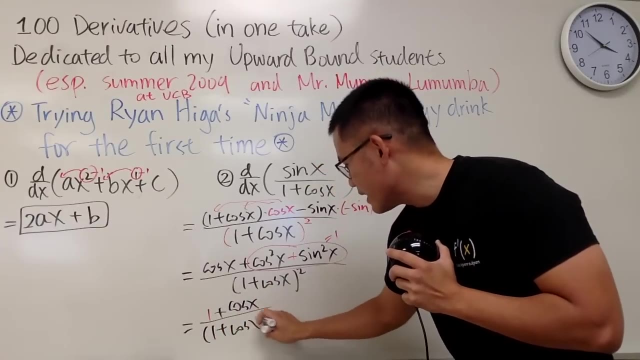 So, therefore, what we can do is we can actually cancel the top. Perhaps I'll just write it down again for you guys to make it clear. This is, like I said, 1 plus cosine x, And then we divide it by. the bottom is parentheses, 1 plus cosine x. and then to the second power. 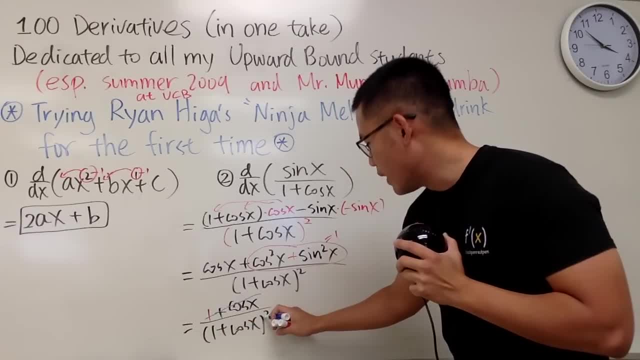 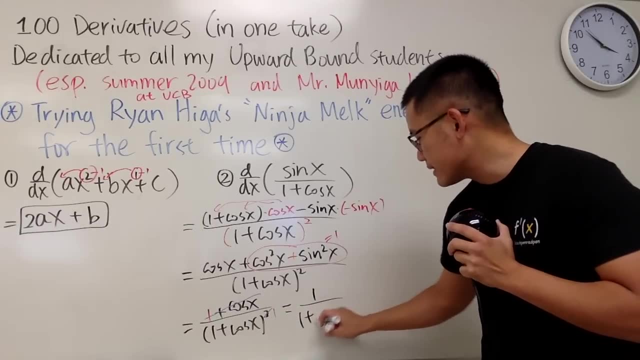 So of course we can cancel this one out with 1 of it on the bottom And therefore, all in all, we have 1 plus cosine x squared. So the answer is just 1 on the top over 1 plus cosine x to the first power, like this: 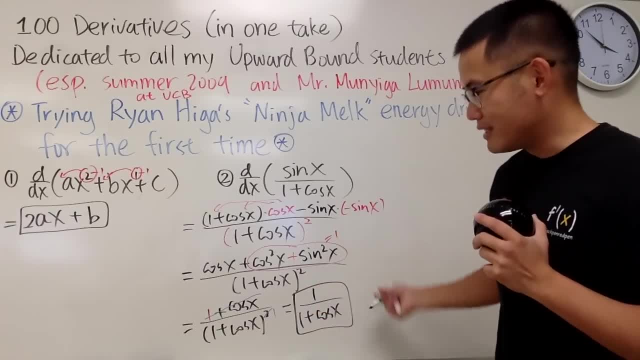 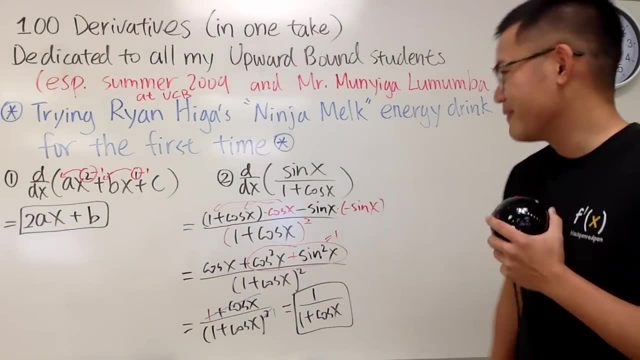 And after that we are done. We don't need to put down the plus c, because this is derivative. This has nothing to do with integration, So find the answer in the answer choices right there. All right, number 3, I will also fit in here, right here? 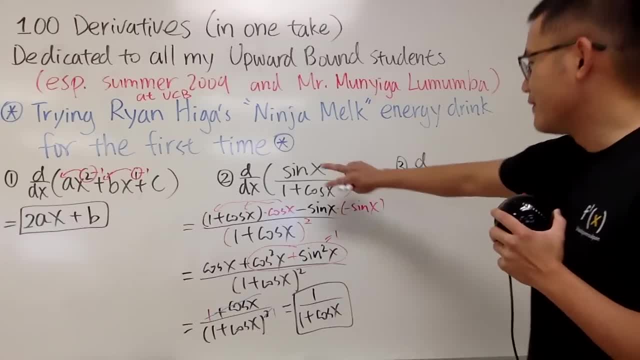 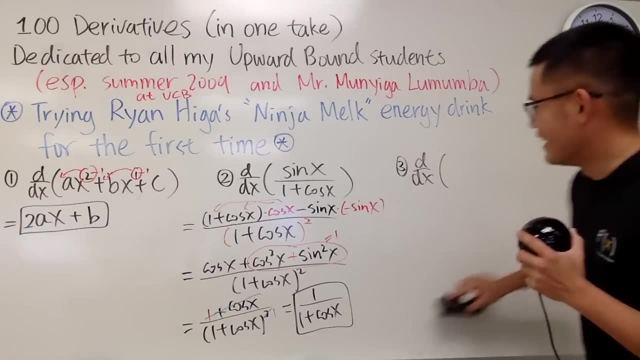 So we will be differentiating. Ah, it's just a flip of this. This: right here we have sine x over- Oops, sorry, Number 3, I should have written this down earlier. Number 3, we have 1 plus cosine x over sine x, like this: 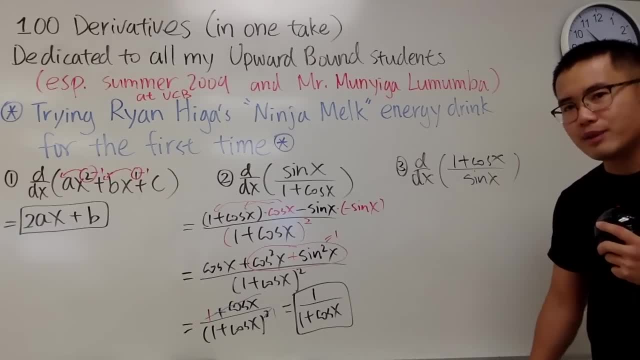 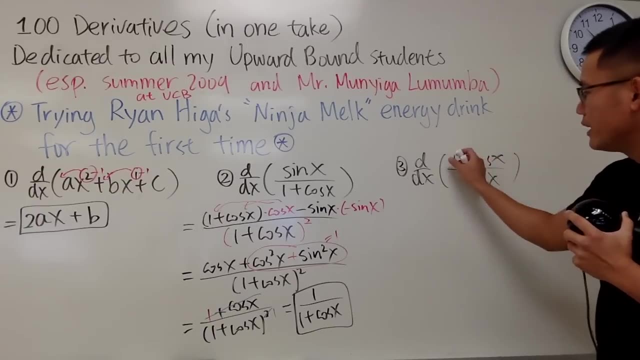 Well, for this question, in fact, we don't have to use the quotient rule, because we only have one thing on the bottom And we have two things on the top right, Two terms. We can just split the fraction. It will be easier this way. 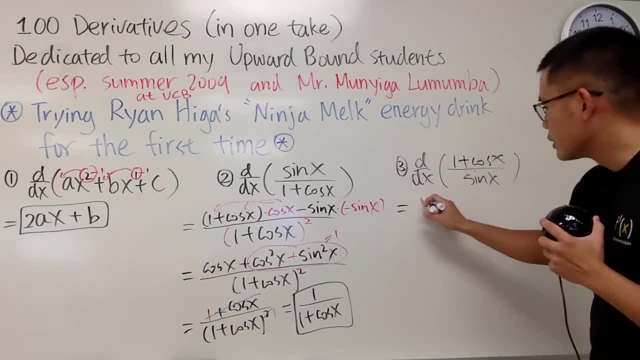 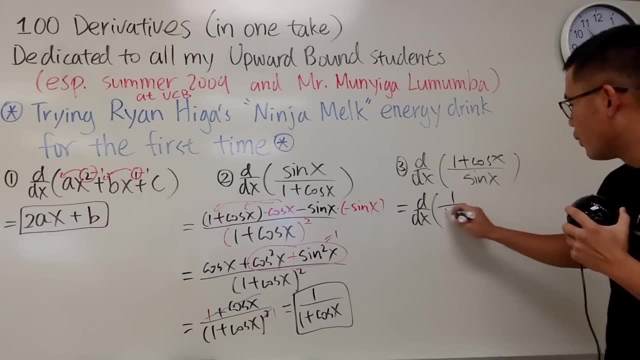 So now check this out. I'm not doing derivatives yet. I will just put down d dx To mean that we will. We'll be taking derivative and we'll split the fractions 1 over this, 1 over sine x. And then the second one is plus cosine x over sine x. 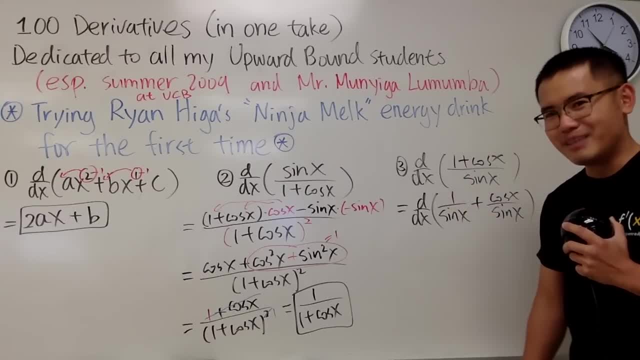 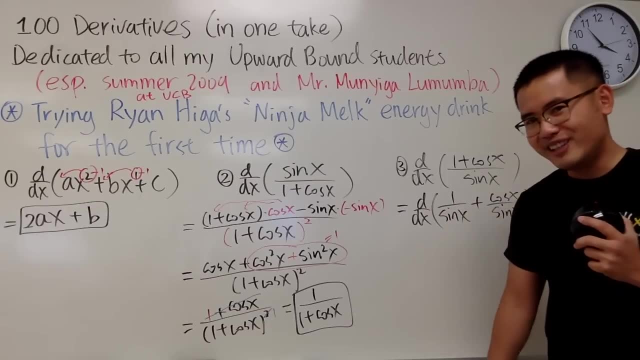 And then, of course, 1 over sine x. Do we know anything about that? This right here: Yes, it's just cosecant x. Likewise, this is just cotangent x. So check this out. This right here is just to differentiate. 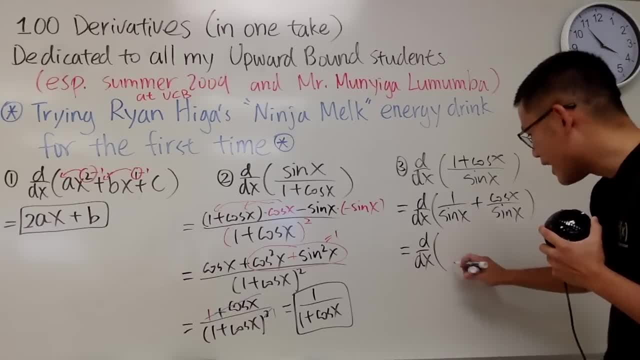 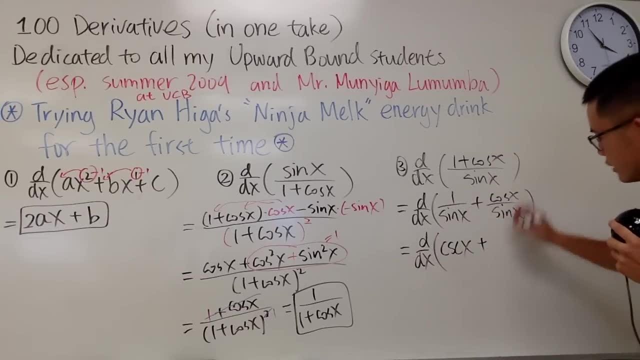 We haven't done that, We haven't done the derivatives yet, So we still have to write this down. We have to differentiate: This is cosecant x And we will have to add the result with This right. here is cotangent x. 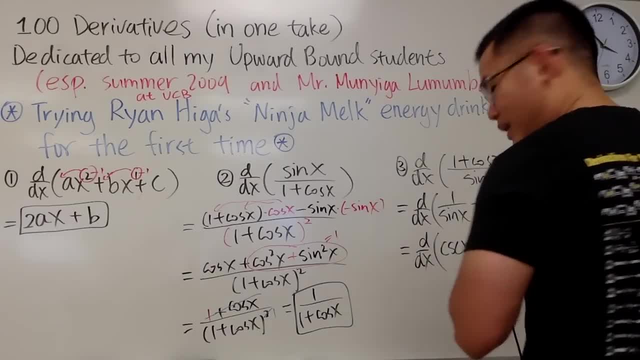 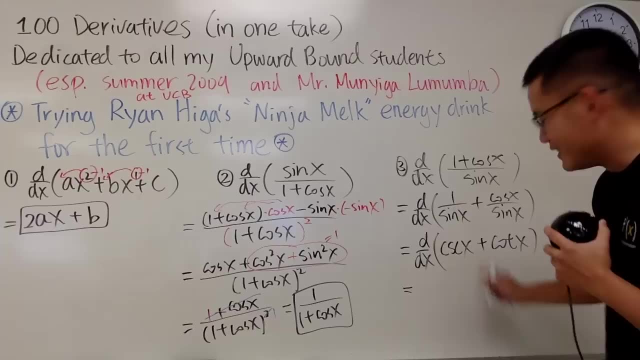 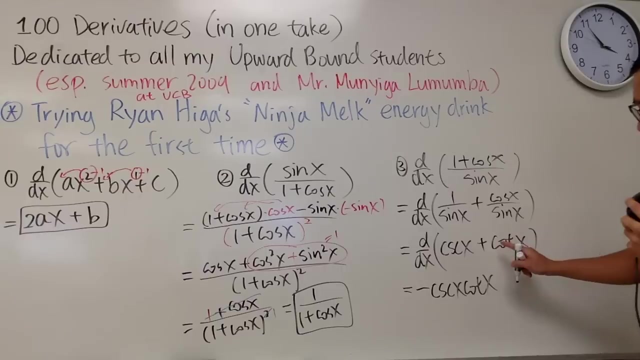 Like this. Oh my goodness, I will have to remember what the derivative of this and this are. Ah, I think I know. The derivative of cosecant x is negative. cosecant x times cotangent x. And then the derivative of: 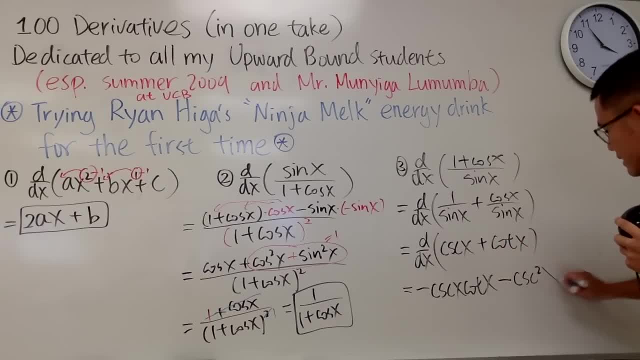 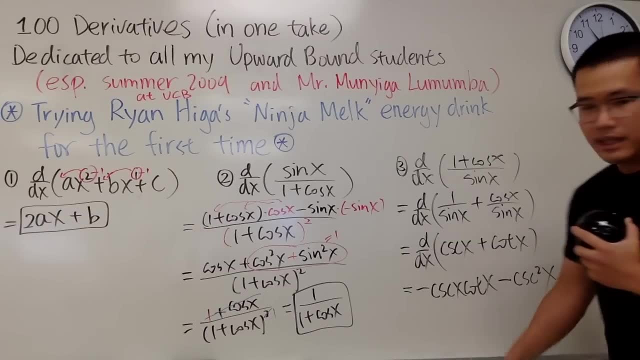 Cotangent x is negative. cosecant x: squared. Well, you put a 2 right here, right And that's it. You don't have to factor out the cosecant x And you can find the answer in the answer choice right over there. 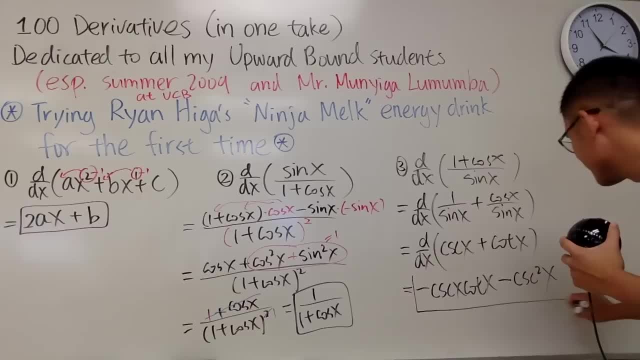 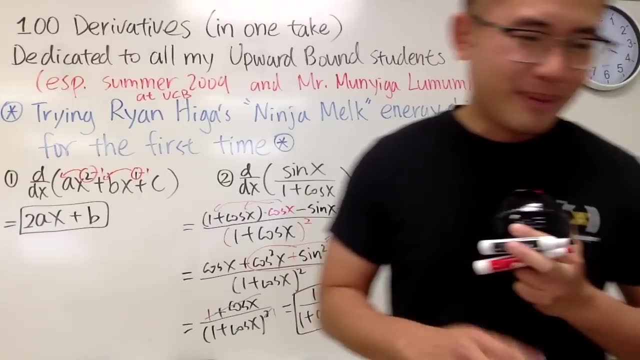 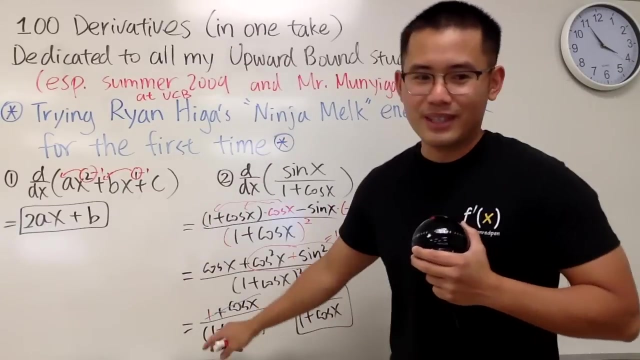 So that would be good. I just realized I make a typo on my answer choice And I'll fix that later. But yeah, So yeah, if you guys saw the answer earlier. but just look at the file in the description. 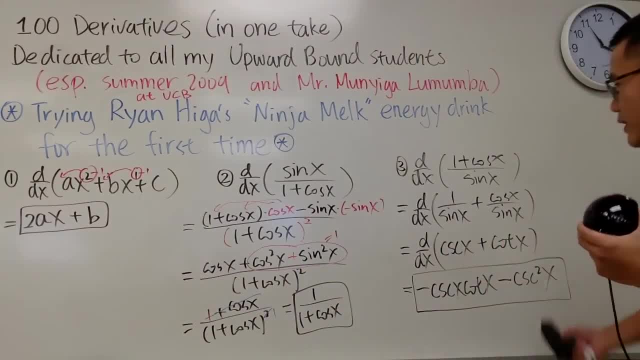 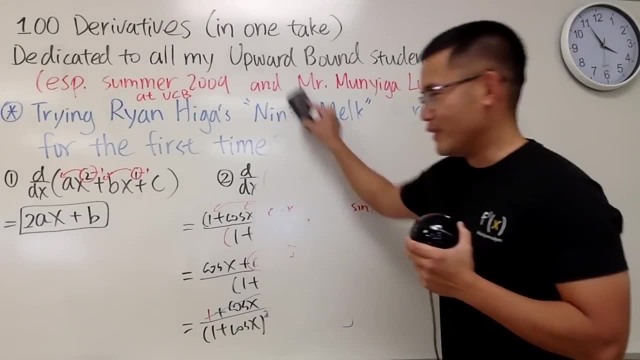 I'll fix that before I post it. So anyway, these are the first two questions. I don't know how long this will take me. Derivatives usually aren't so bad Until we hit the definition Right. When we have to prove the derivative of. 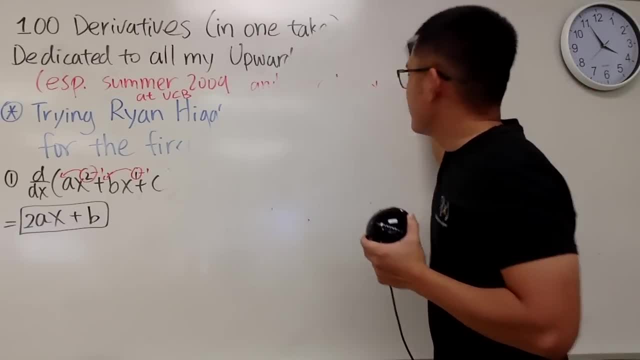 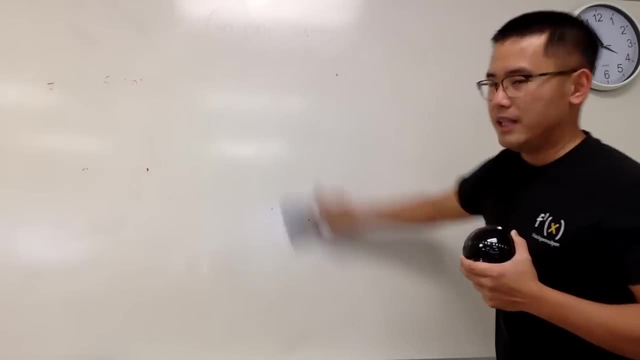 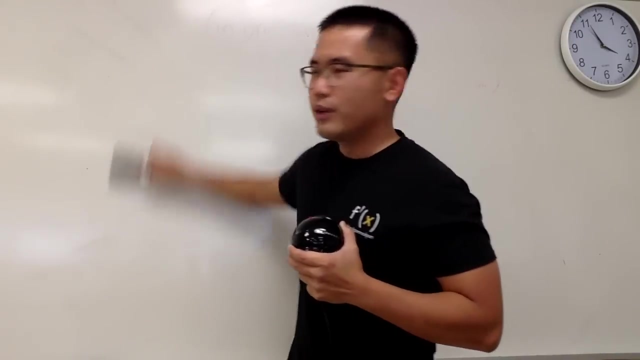 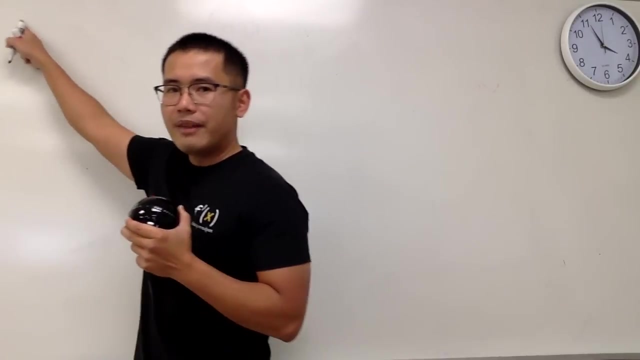 What is the definition of derivatives? Alright, So three questions down And many more to go, And hopefully you guys all find this video to be helpful. Right, Alright, Number 4.. We have the square root Right, So here we have number 4.. 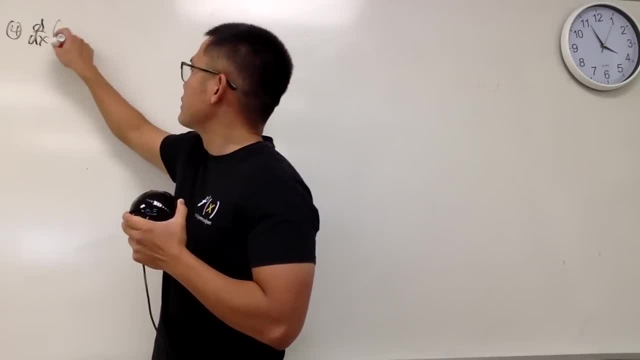 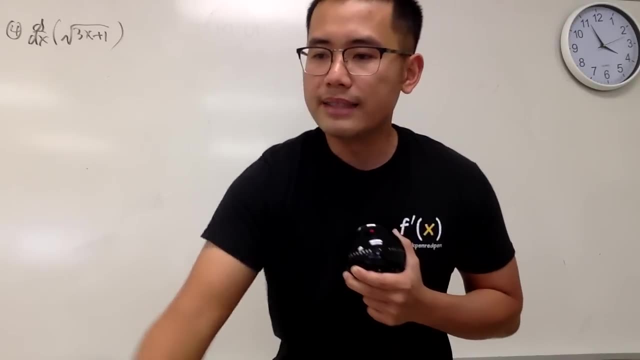 We will have to differentiate the square root of 3x plus 1.. Derivative of square root of 3x plus 1.. Now this is how we can do it. First thing first. You have to know, You have to know. 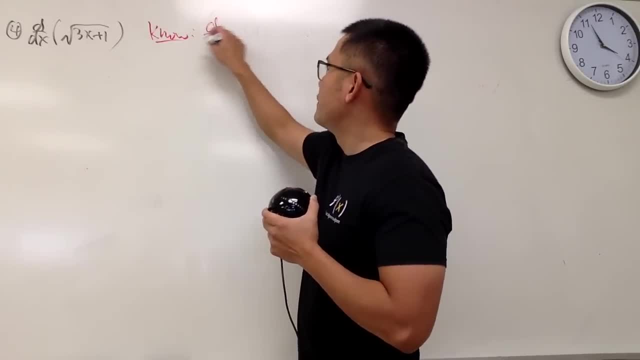 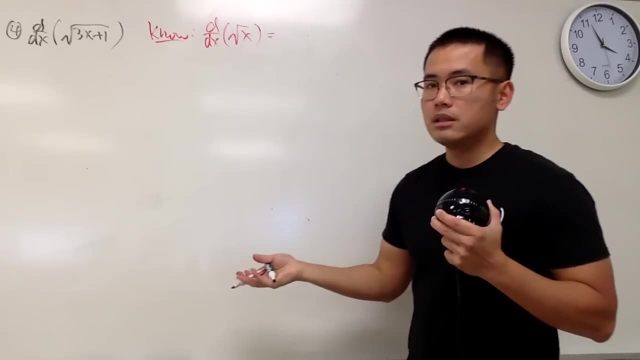 Right. You have to know that the derivative of the square root of x Like this. This right here will happen a lot, So you just might as well remember it. The derivative of square root of x is 1 over 2. square root of x. 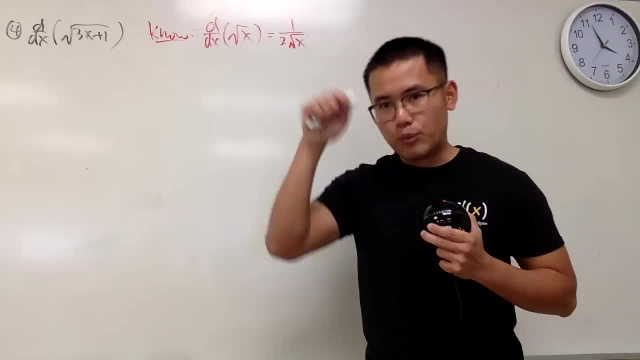 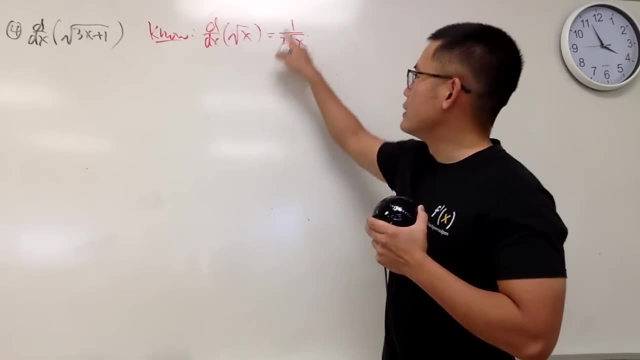 And to do this you will have to write the square root as the 1 half power And you bring the power to the front And then minus 1 from the power. So you end up with 1 half x to the negative 1 half. 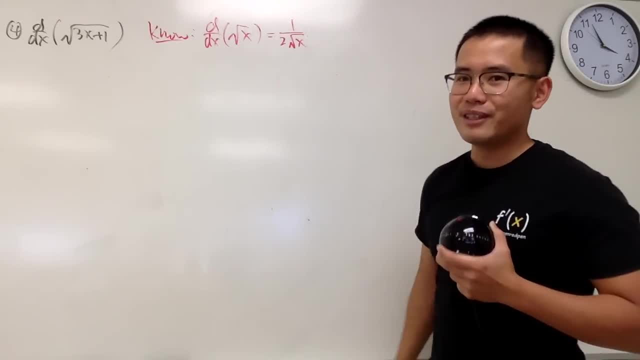 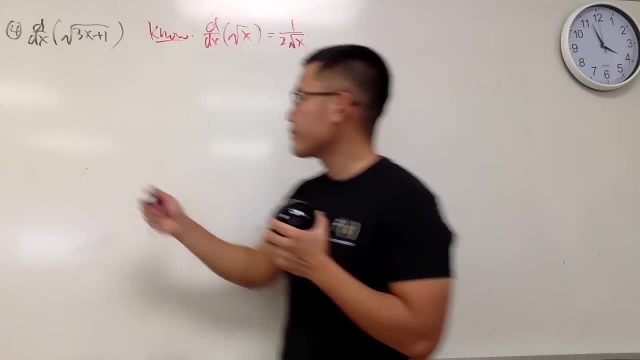 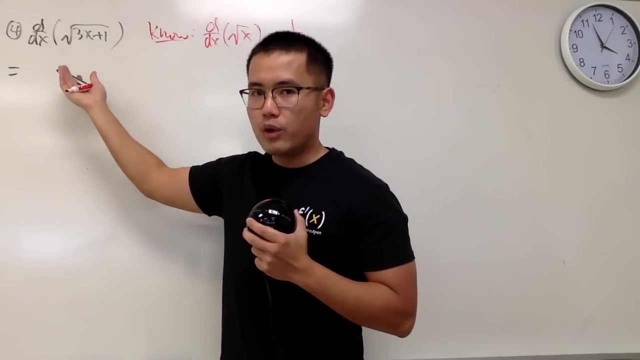 x to the negative 1 half is the same as putting the square root in the denominator, But, as I said, you should just remember this And then use that to do the questions like this. So here we go: To differentiate the square root of 3x plus 1, we will just have to look at the big picture, which is the square root. 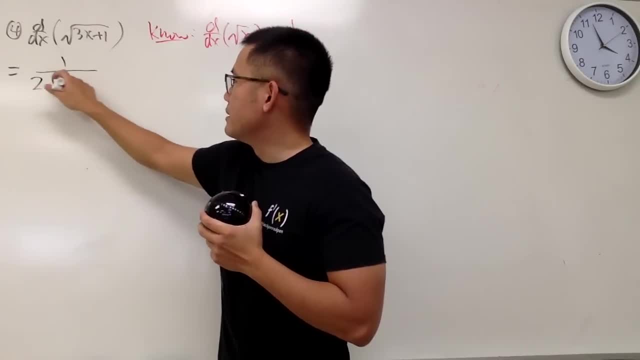 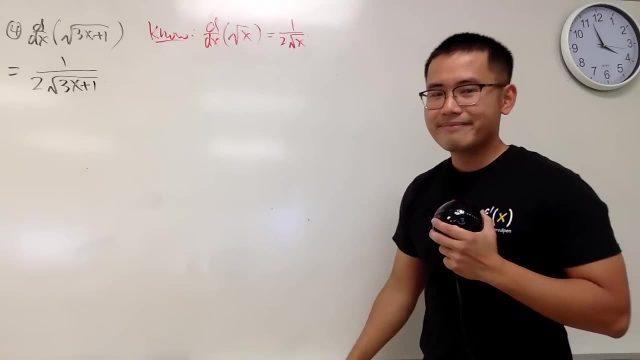 We will have to do 1 over 2 times the square root of the inside, which is 3x plus 1.. Right, You might hear it over there. However, don't forget the chain rule. We have to multiply by the derivative of the inside. 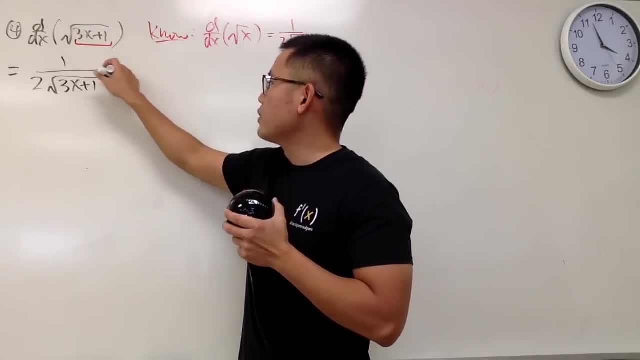 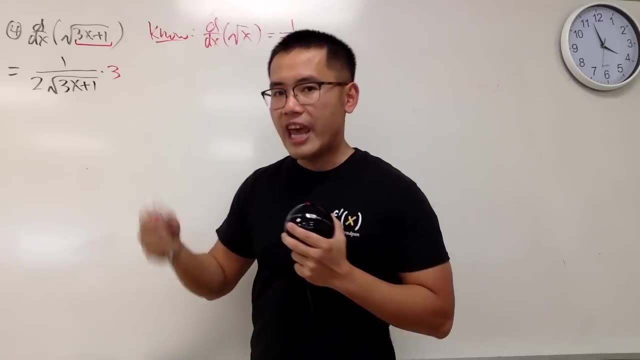 The derivative of 3x plus 1 is just a 3.. So you multiply by 3, right here? Right. So this is the chain rule, And some textbooks they like to call this step the chain rule. So one way or the other they both work pretty nicely. 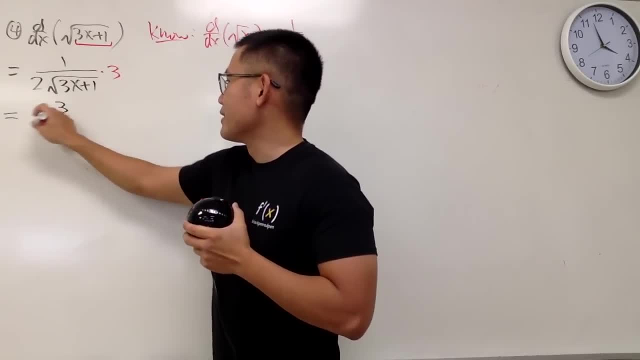 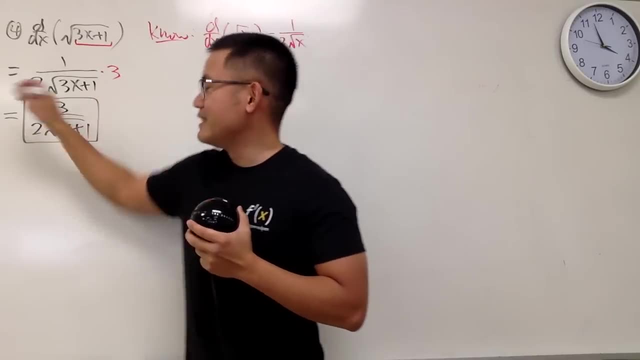 In the end, of course, 1 times 3, you can just put a 3 on the top, So 3 over 2, square root of 3x plus 1.. And guess what We are done? So this right here is it. 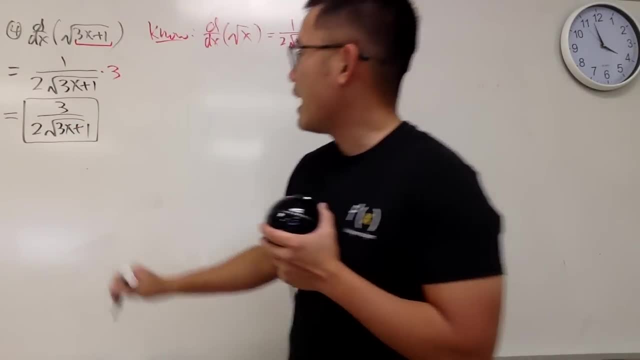 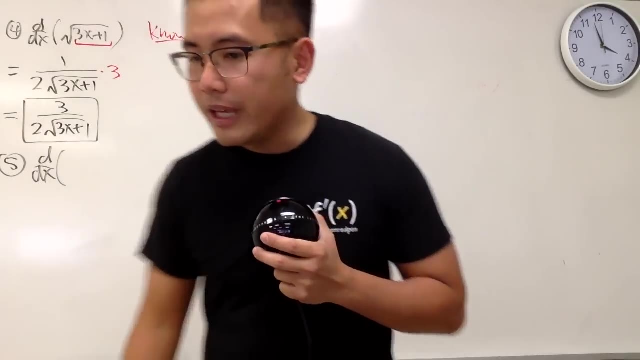 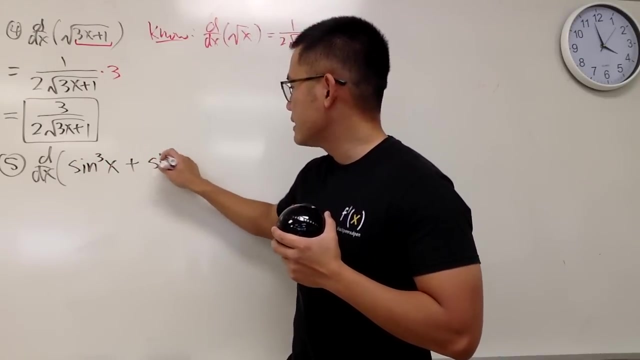 All right, Now number 5.. So here we have d, dx. This again means to take the derivative, And we have these two notations: Sine, and you put a 3 right here of x, And then we add sine x, like this: 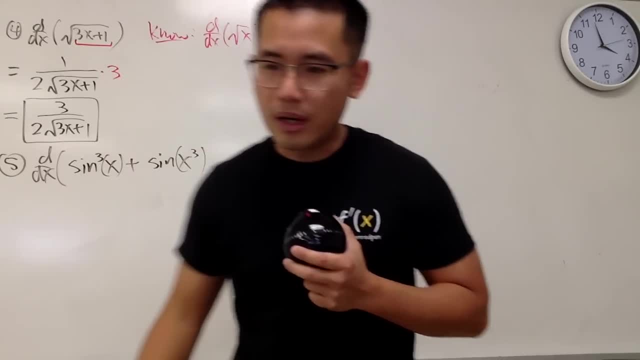 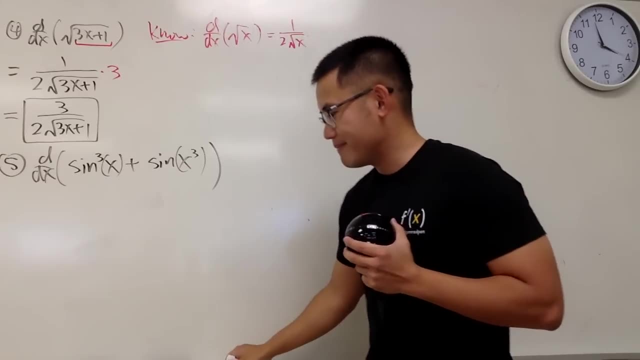 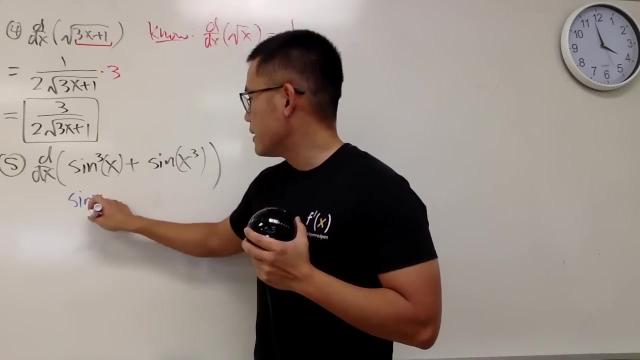 With a 3 right here, parentheses, And technically I also have the parentheses right up there. Here is the DEO: This right here, right, This right here. it means we will have sine x raised to the third power like this: 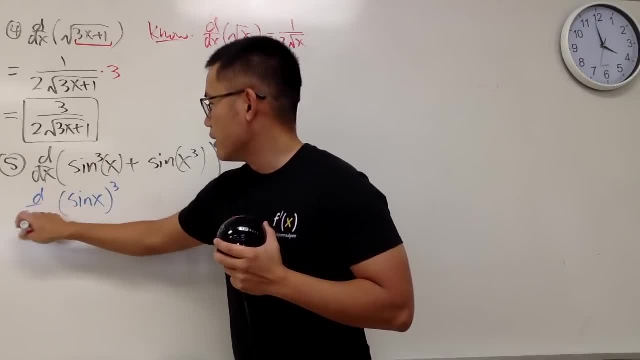 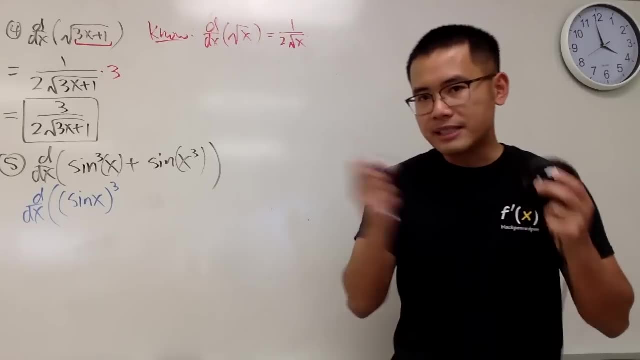 And then of course we will have to differentiate this guy Right. So it's just the notation: Whenever we have the 3 right here, it means we have sine x times sine x times sine x. Of course we write it like this. 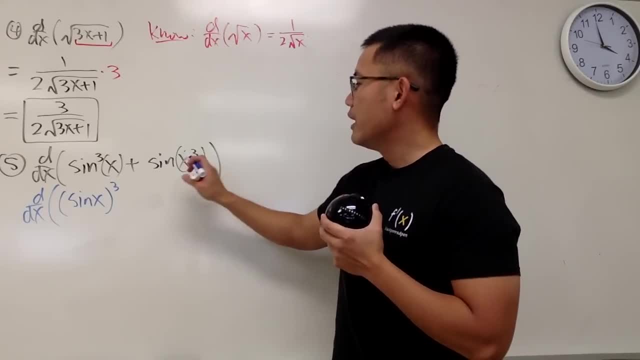 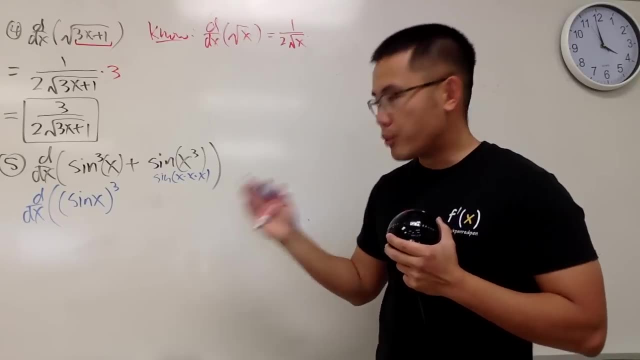 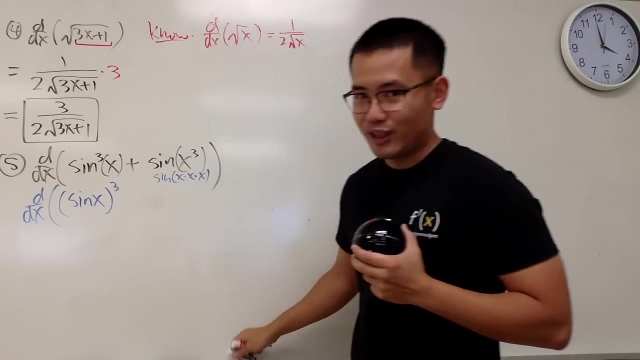 Right. But when we have sine of x raised to the third power, this means we have sine of x times x times x, Like that. Parentheses matters. Parentheses matters. They are totally different. Be sure you are familiar with the notations. 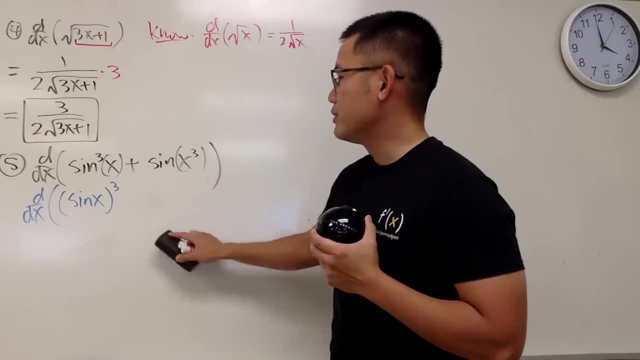 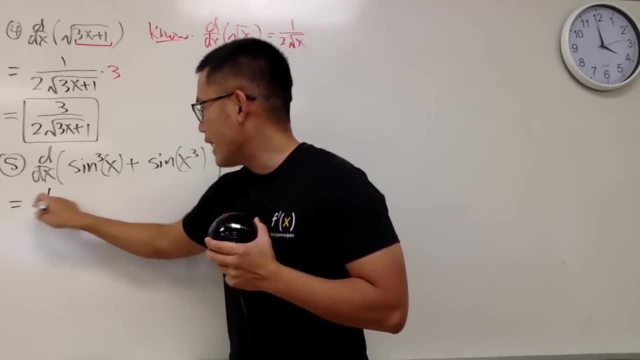 Right. So this is how I would recommend you guys to do these questions. We technically have two questions to do, right? Two parts. All right, Here we go. Let's differentiate. For the first one, let's write it as sine x to the third power. 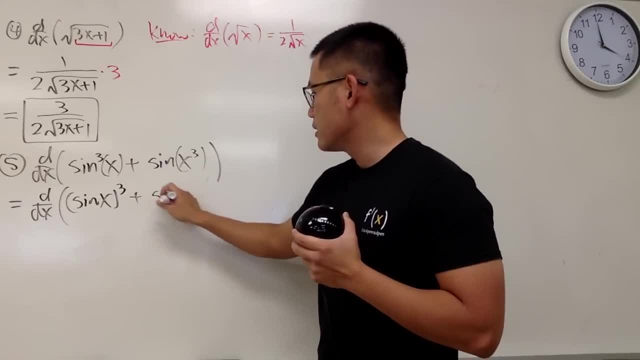 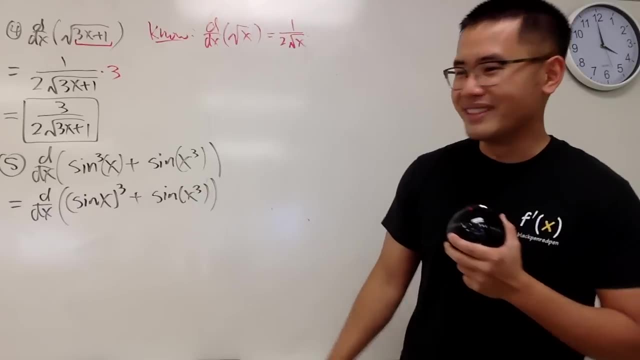 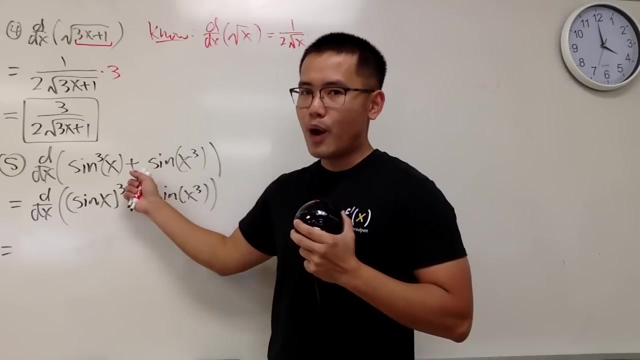 And then for the second one. I'll just keep it like this: Just remember to use the chain loop a few times whenever we need to. Okay, Here we go For the first one. sine x is the input, and then we have this raised to the third power. 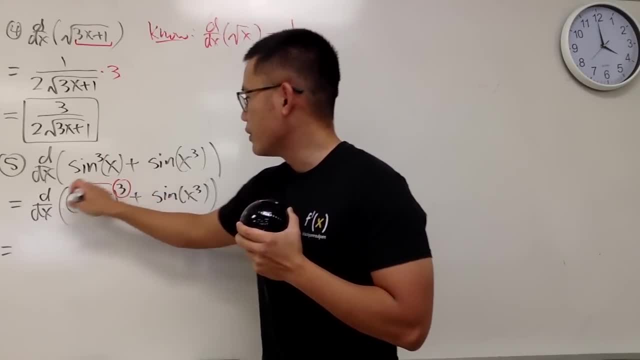 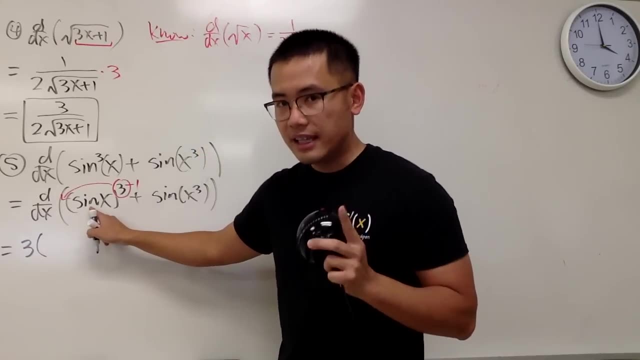 So do the picture. first Bring the power to the front and then minus 1.. So we end up with three parentheses and the inside states the same for now. So just write down sine x and then 3 minus 1.. 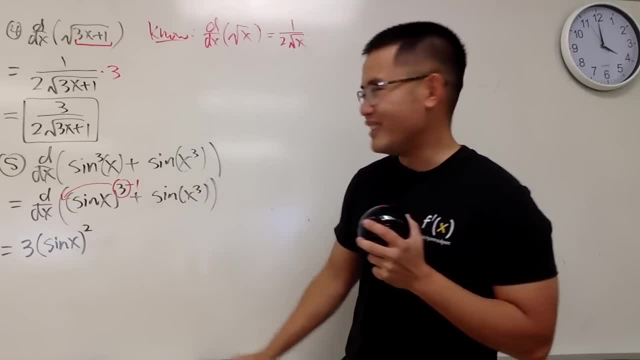 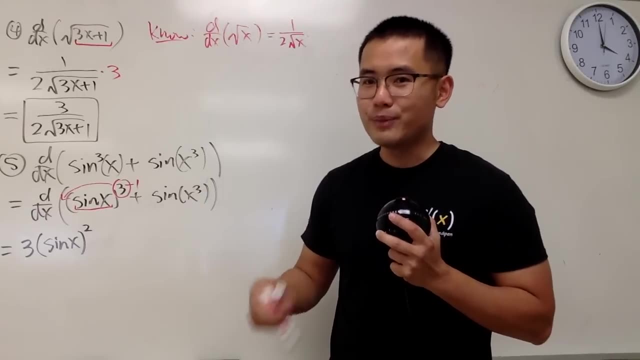 That's the new power, which is 2.. And now it's the time to use the chain loop. You look at the inside, which is sine x, and you ask yourself what's the derivative of sine x, which is just cosine x, right? 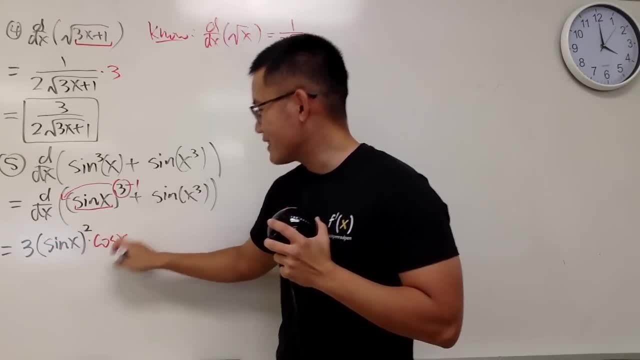 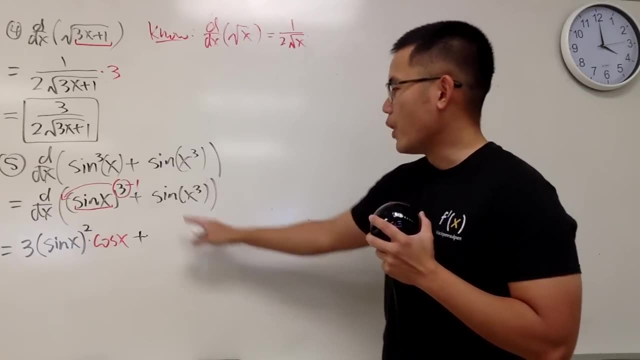 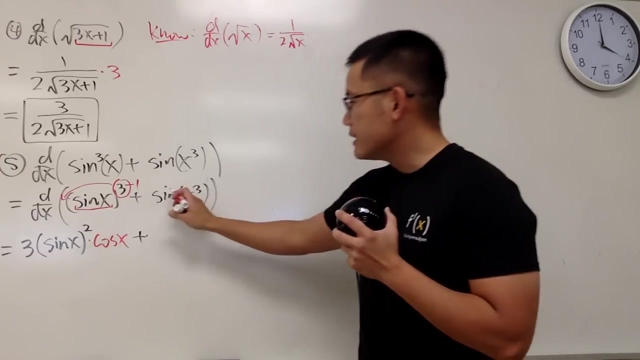 And you multiply this part by cosine x. This is the chain loop, And then, right here, let's go ahead and add for this part. Well, this time though, the big picture is sine of this, So you differentiate sine, which is cosine, and the input is x to the third power. 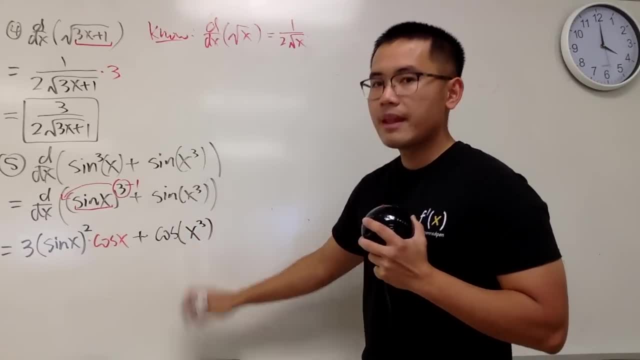 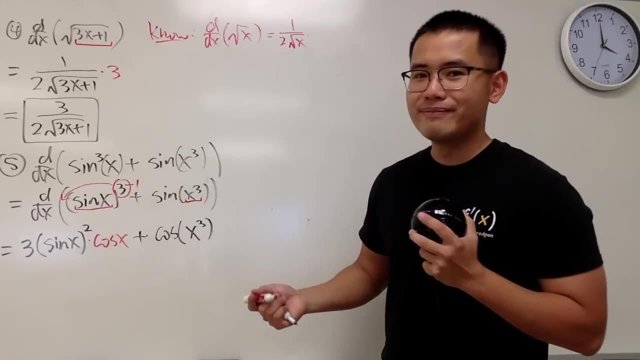 It states the same right here. Okay, And then we look into the parentheses. The derivative of x to the third power is what? Well, it's 3x squared, right? Just use the Power rule So you get 3x squared. 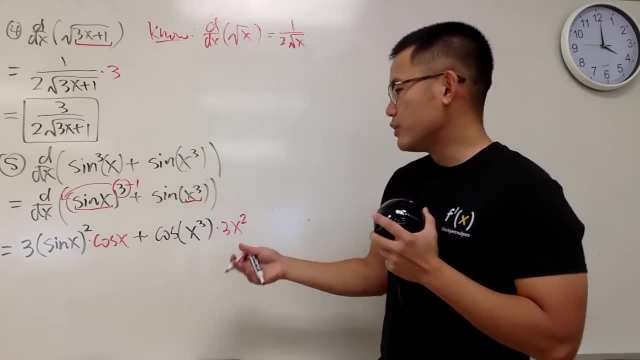 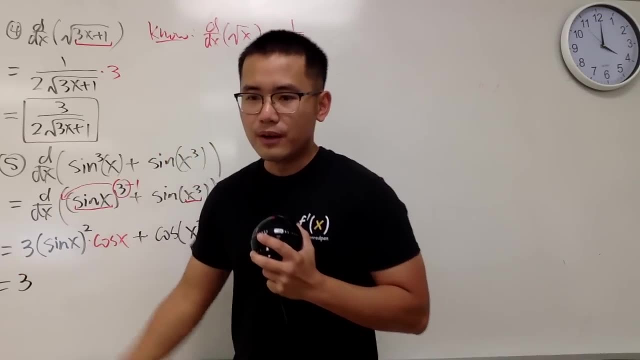 So this is it right, This is it. And finally, we'll just write this down the usual way. So here we go. I will put down the 3 right here and I will put down the cosine first. Did I put that down? 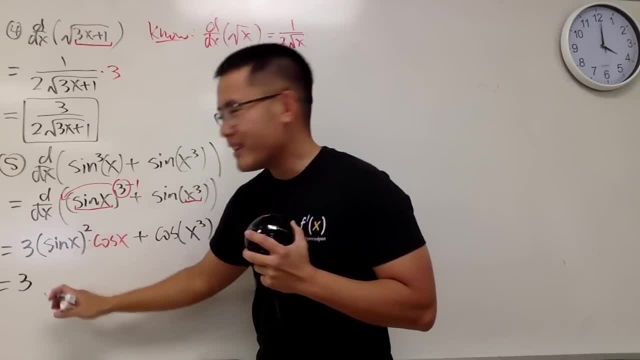 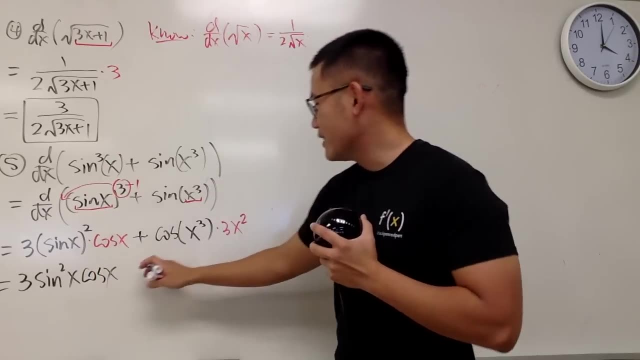 No, I didn't put down the cosine first. I was just writing down this: This right here is the same as saying sine, with a 2, right here, right, And then the cosine x, And for this one usually we put the polynomial part in the front. 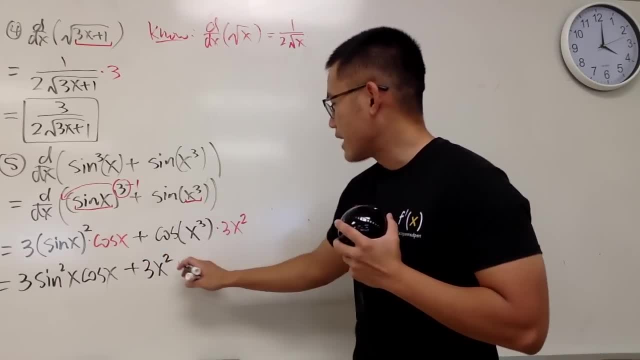 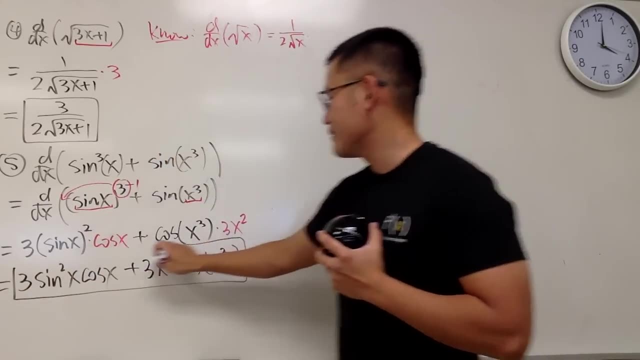 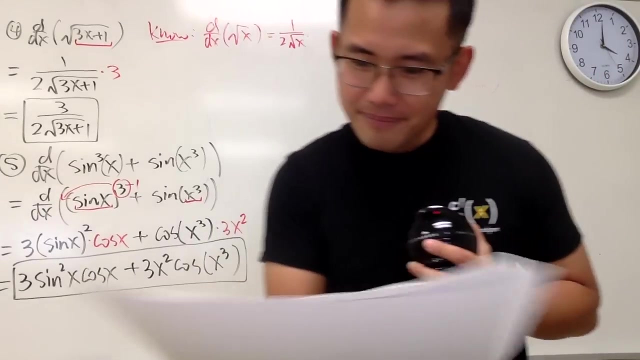 So I will write this down first, which is the 3x squared times cosine of x to the third power like this, And with that we are done. This is going pretty well, unlike the integrals. So this is number 5.. 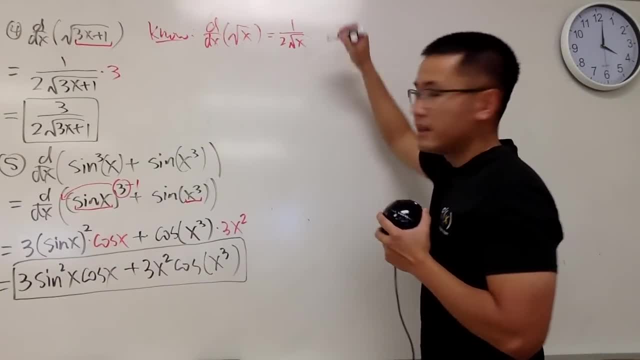 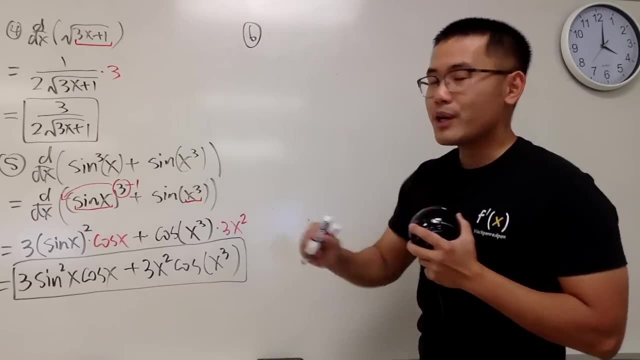 Okay, Number 6.. I will just put it down right here. I will just erase this a little bit, so I can. Number 6.. Here we go. We have to differentiate 1 over x to the fourth power, like this: 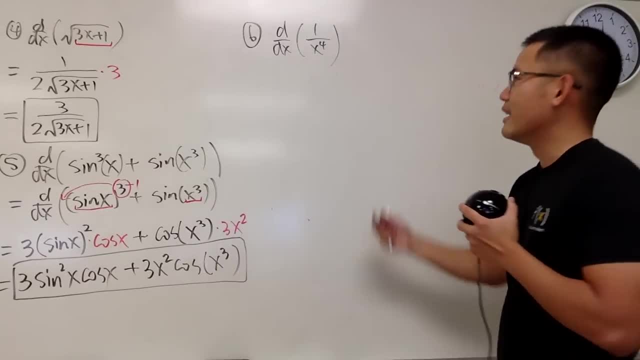 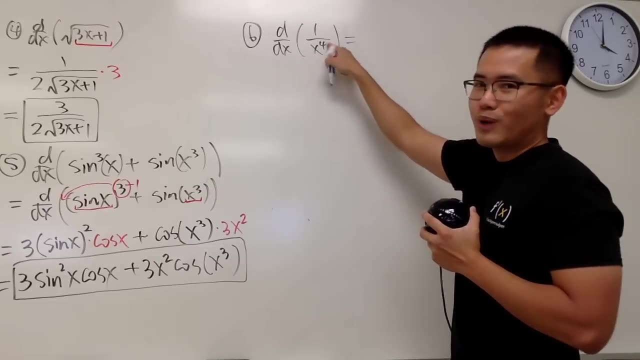 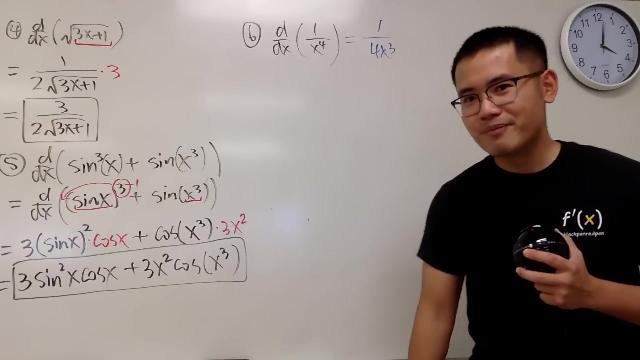 Okay, So x to the fourth power. This is easy, huh. So of course we can just look at x to the fourth power, bring the 4 to the front, which is just 4x, and then minus 1, which is 4x to the third power, and that's in the denominator. just like that, right. 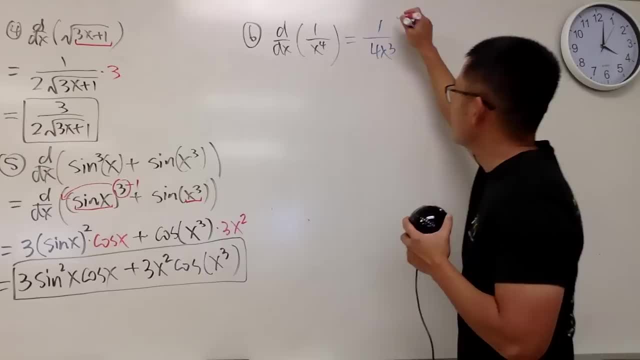 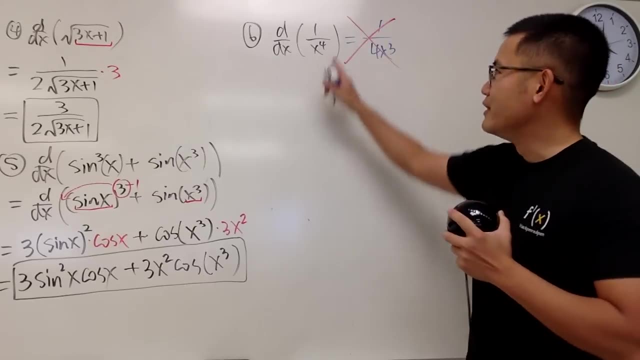 No, Don't do it like this. No, No, no, no, no, no. This is not the answer. Not the answer Why? Because the 4 that you see right here it's not really a 4, because it's in the denominator. 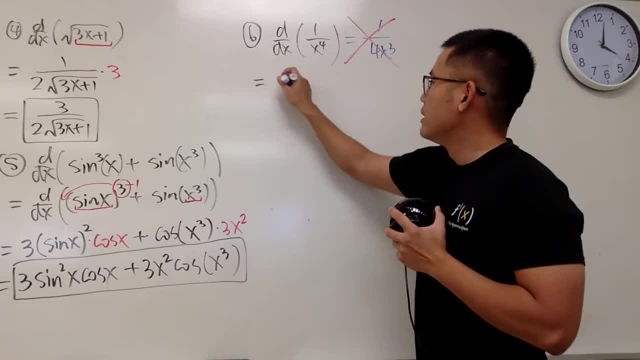 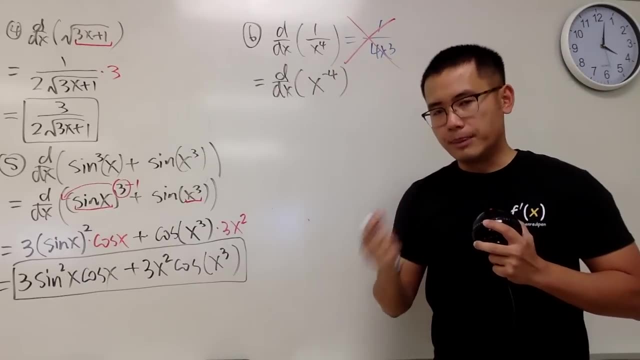 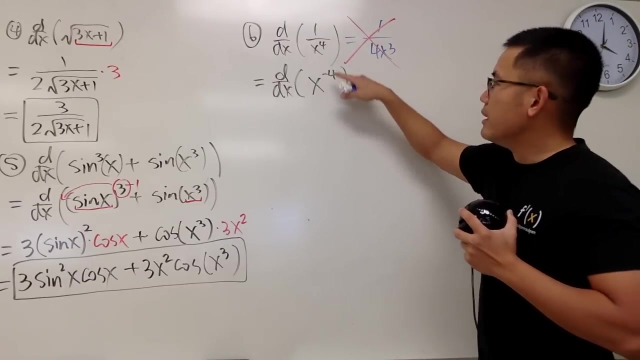 Therefore, this right here, it's really asking to differentiate x to the negative fourth power In order for us to use the power rule. remember, remember, remember, we have to have x to some number, right? Well, 1 over x to the fourth power. 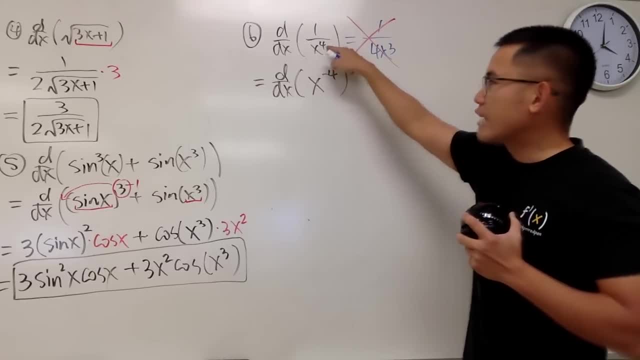 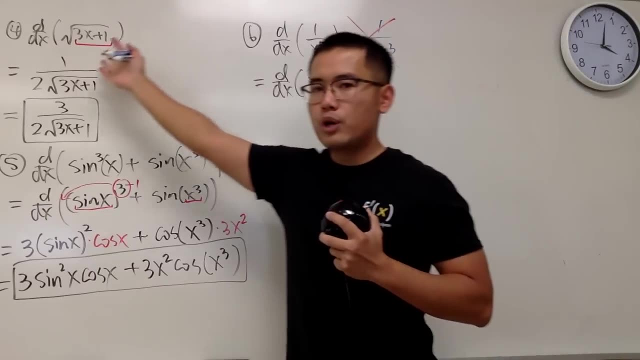 Well, 1 over x to the fourth power. unfortunately, this 4, it's actually a negative fourth power. So you have to know your rule of exponent really well. This is very similar to the square root example. You have to write the square root with 1 half power. 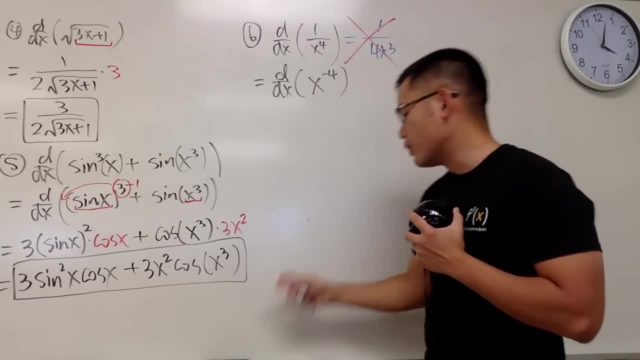 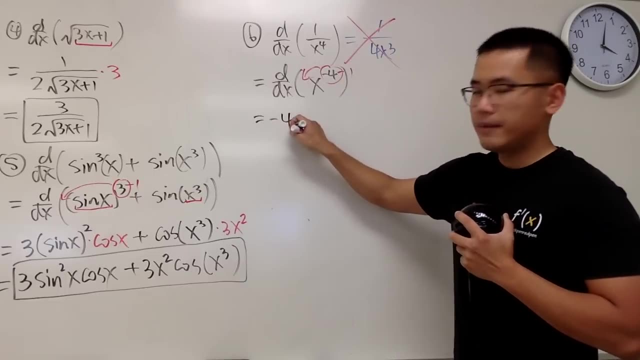 Anyway, look at this right here, and then do the power rule, Bring this to the front, and then minus 1 right here, and we end up with negative 4 times x to the negative 5, and then you subtract them and that's pretty much it. 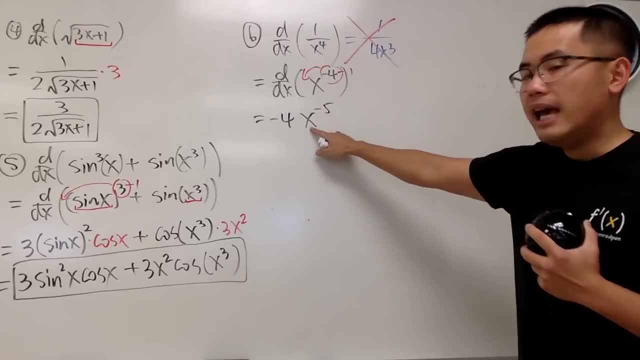 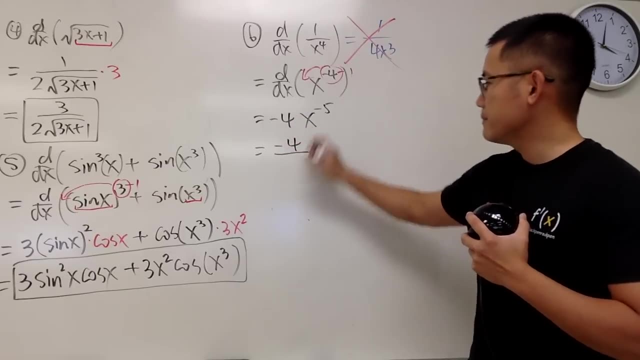 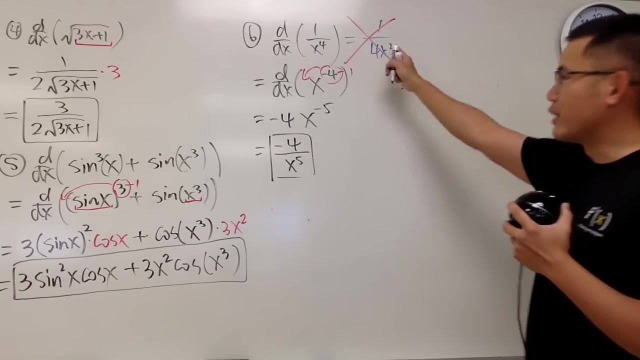 Finally, negative 5, that's the power for the x, So we can bring this down to the denominator. Therefore we end up with negative 4 over x to the positive 5 power like this. So this, right here, it's a correct answer. 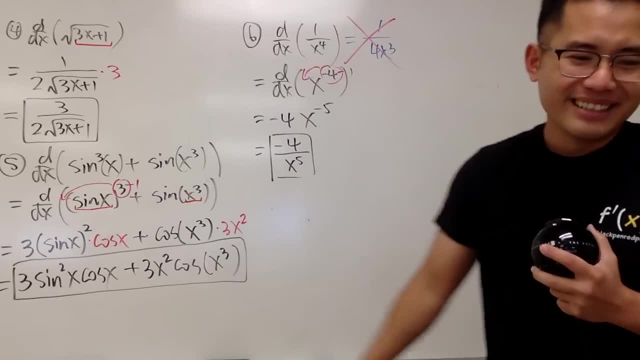 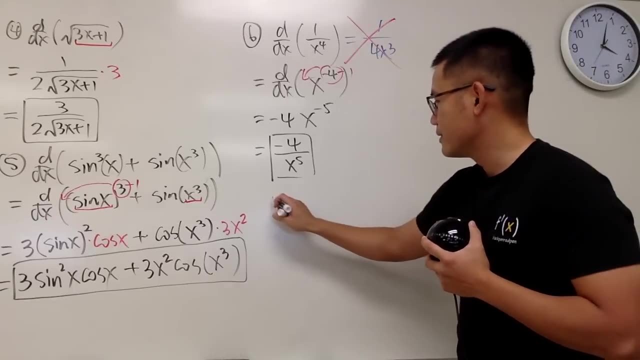 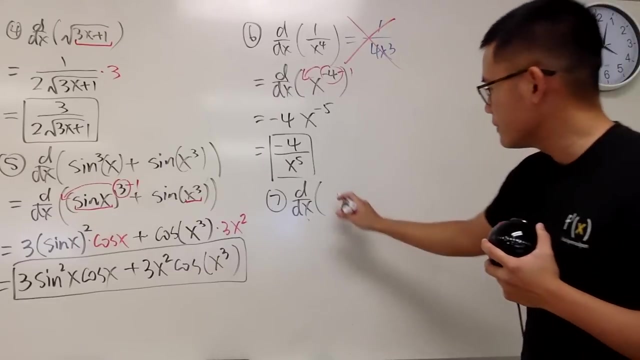 This right here. it's a common mistake. Don't do it like that, right? Don't do it like that, Alright. continue, continue, continue. Number 7, number 7, number 7.. Here we are going to differentiate and we have 1 plus cotangent to the third power. 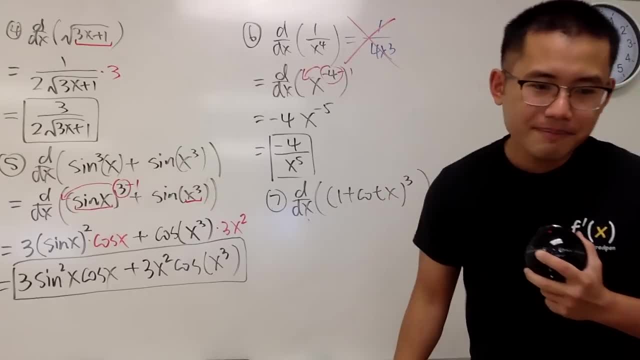 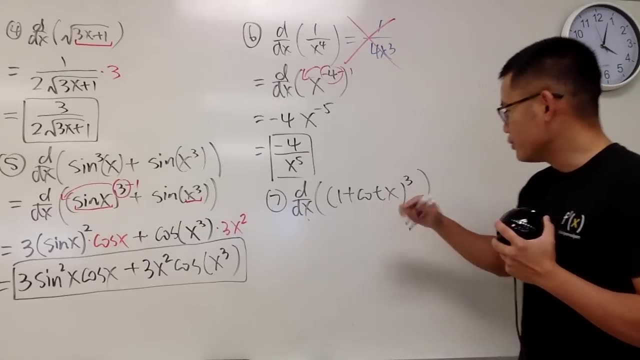 cotangent x and then to the third power, like this right. So here we go. Of course we have the inside and then raise to the third power. So again, we have to do the big picture first, which is the outside power rule right. 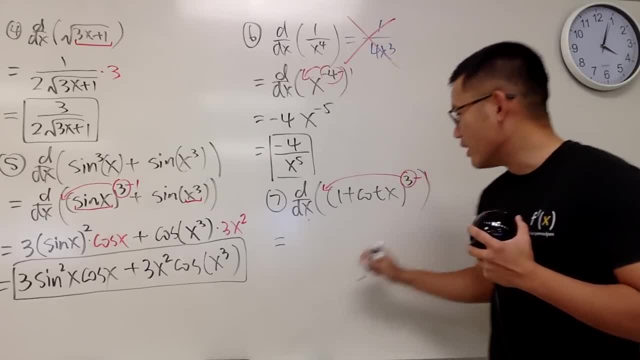 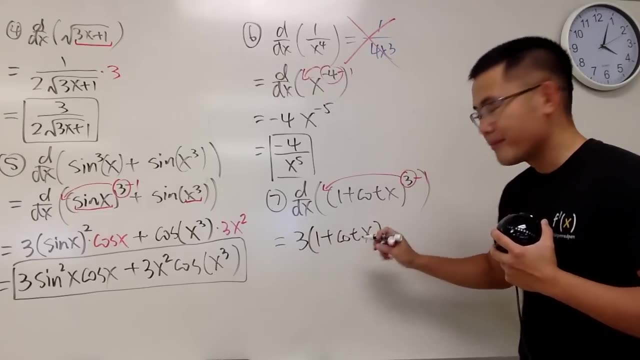 Bring the 3 to the front and then minus 1.. So here we go. Bring the 3 to the front. Inside stays the same. Just write down 1 plus cotangent x And 3 minus 1 is 2, of course. 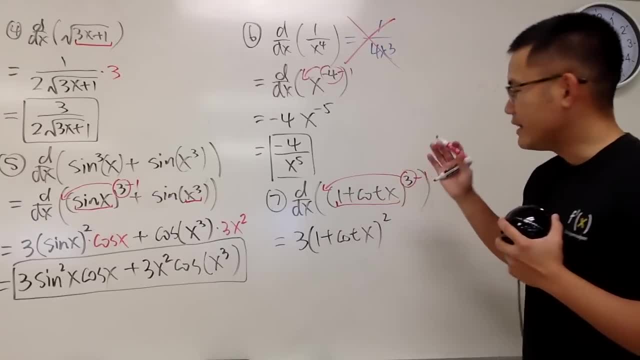 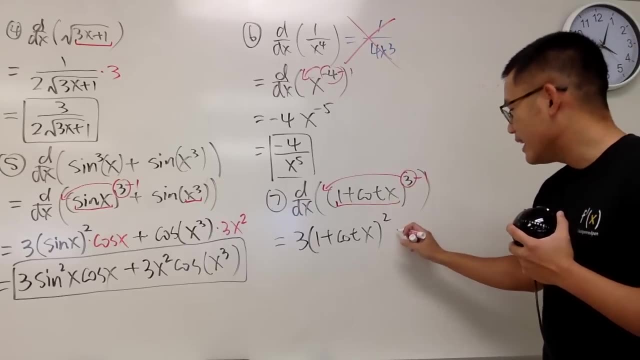 We're not done yet, though. Look at the inside and ask yourself: what's the derivative of 1?, Which is 0.. What's the derivative of cotangent x? Well, that's negative. cosecant squared x. Remember the chain rule right. 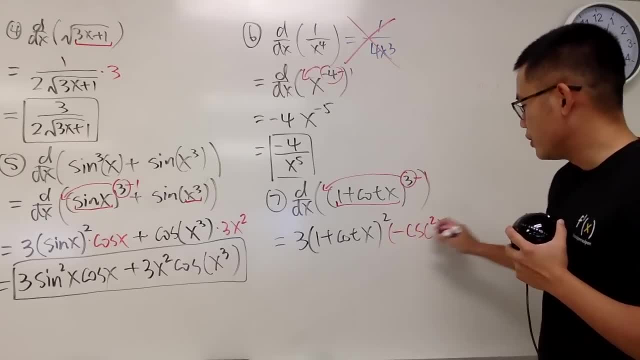 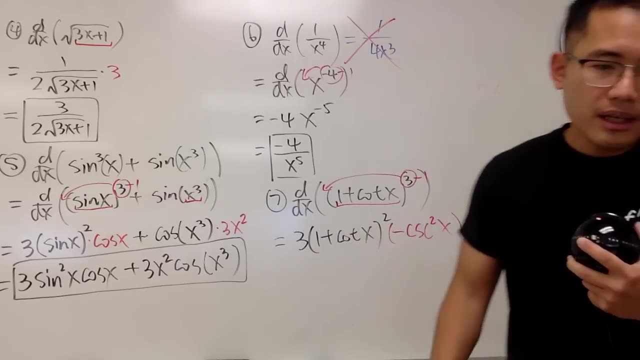 And of course, this right here. it looks like subtraction, So be sure you just put parentheses. This is the derivative from here And we have to multiply this with that. This right here is pretty much it, And in the end we just have to write it down nicely. 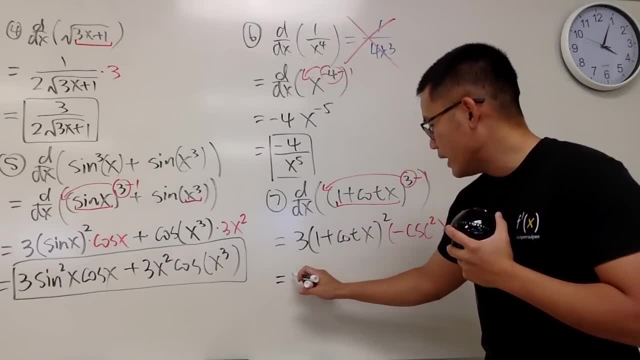 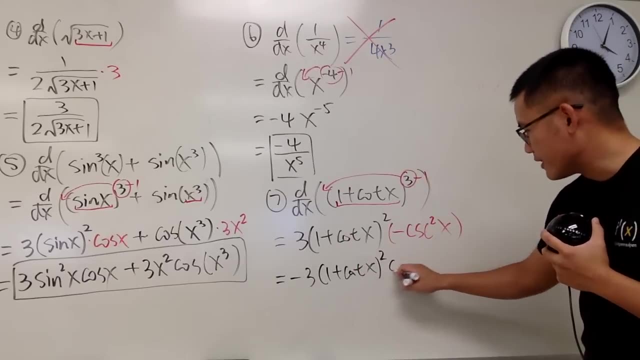 Put the negative all the way in the front, That's all. So finally we have negative 3 times this, which is 1 plus cotangent x, And then square, And then in the end I have the csc squared x, which is the cosecant squared x. 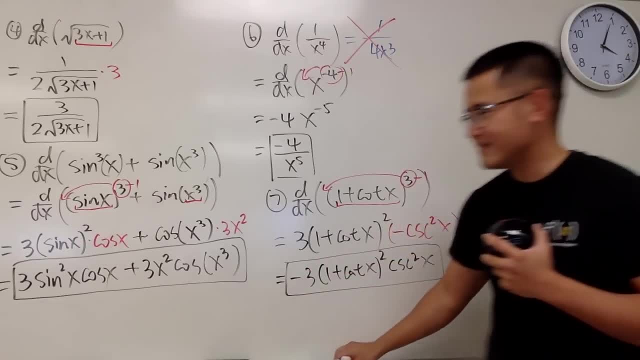 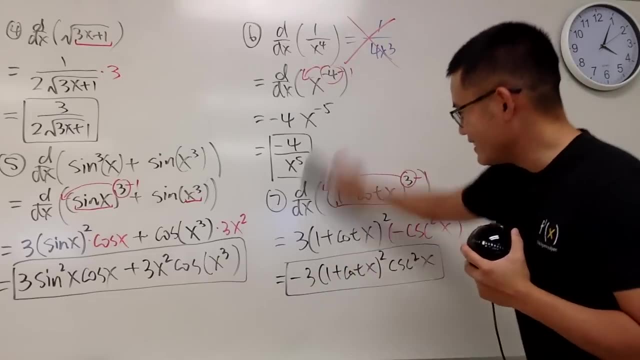 Just like that, And that's it All. right Now, number 8.. I need more space, so I will have to erase this now. So the first couple questions- I think the first 20 questions are more for like warm-up. 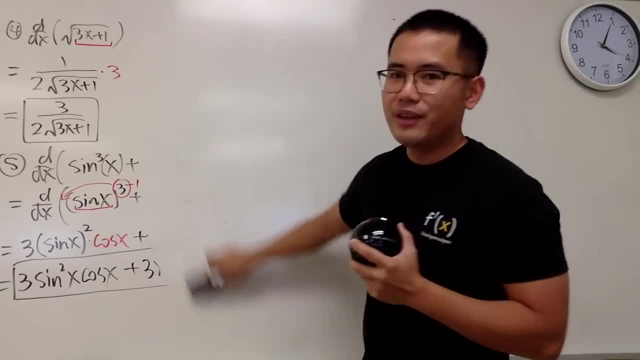 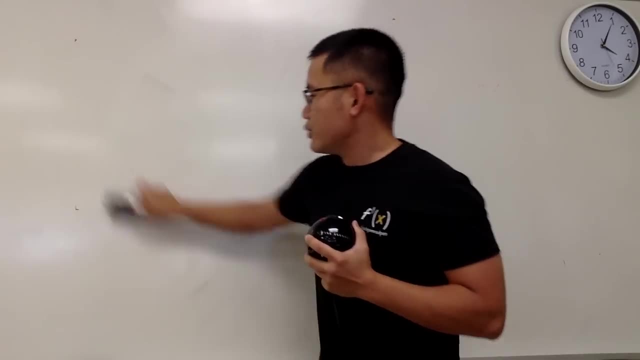 And I put it like according to the difficulty and also the things that you have to know, in the usual order. Later on you'll see the inverse trig functions, natural log, exponential and hyperbolic functions, All that stuff. 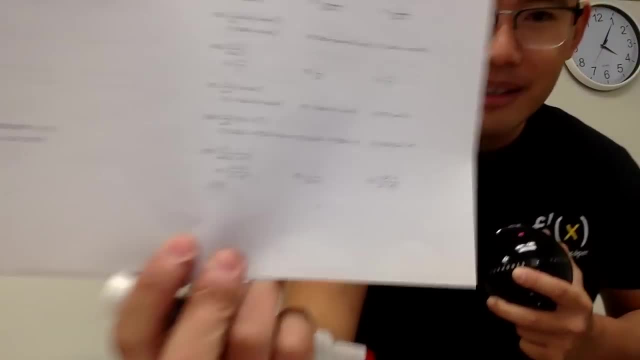 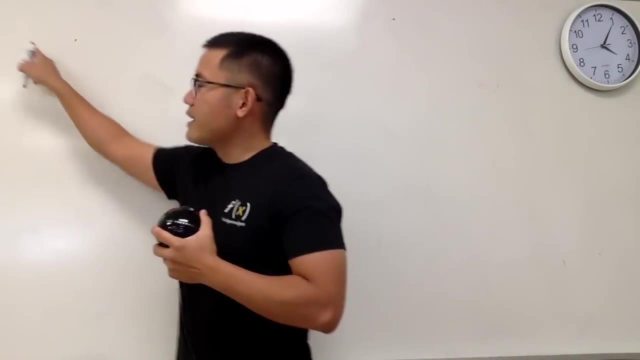 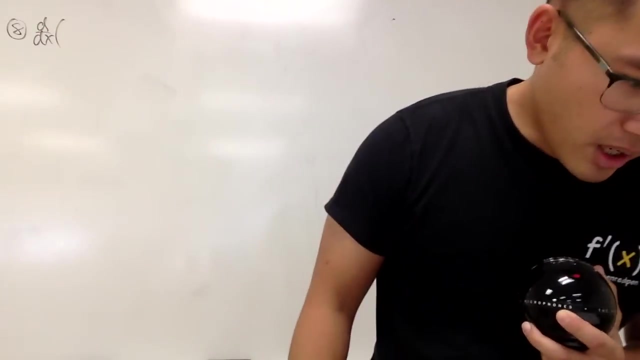 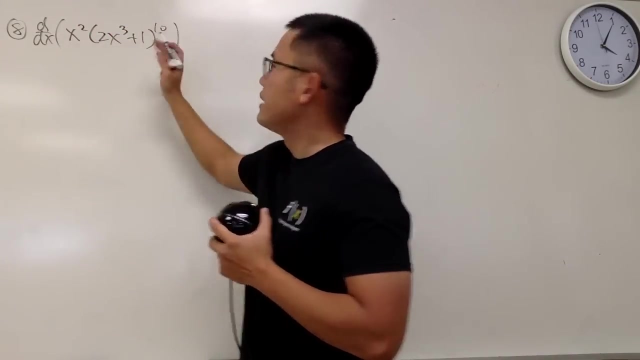 All right, Now things are getting slightly trickier and also slightly more complicated. Anyway, here we go, Number 8. We are going to differentiate. let's see x squared times 2x to the third power plus 1 and raised to the tenth power, like that: 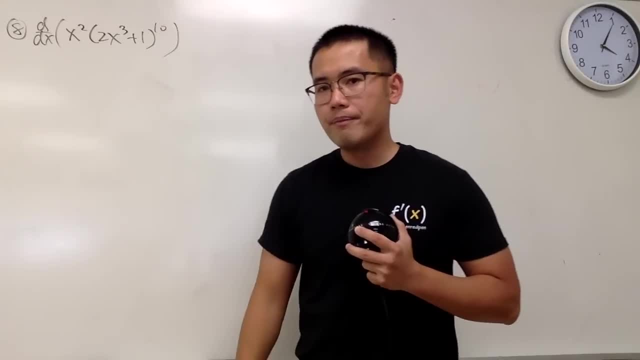 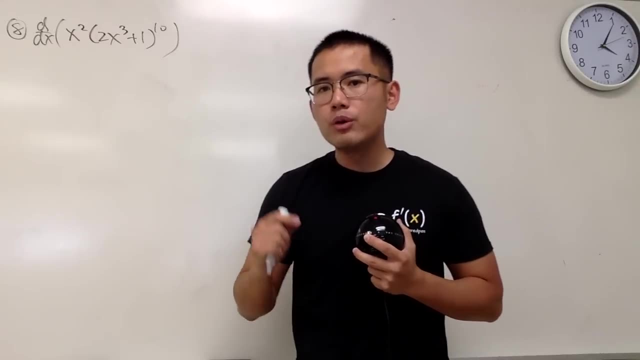 All right, This one compared to the earlier one. well, we have x squared right here. times this quantity to the tenth power. So it's not just a simple chain rule question, Because right here we will actually have to use the product rule. 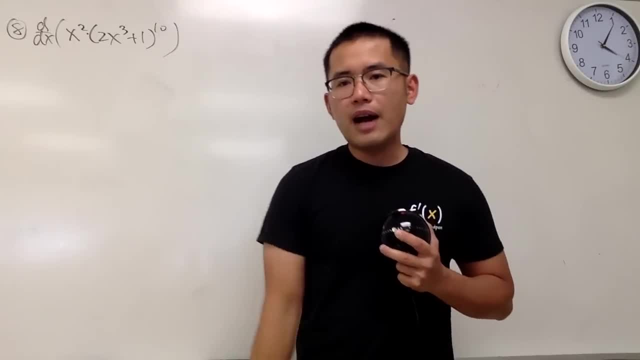 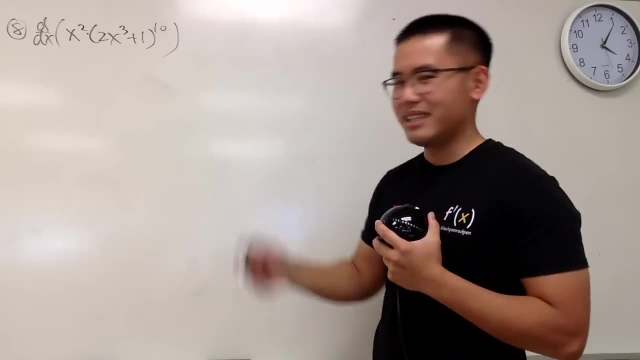 Because we have x squared times. this And this is how I like to set up the power. This is how I like to set up the product rule for my students for the first. I'll show you guys at least one time right here in this video. 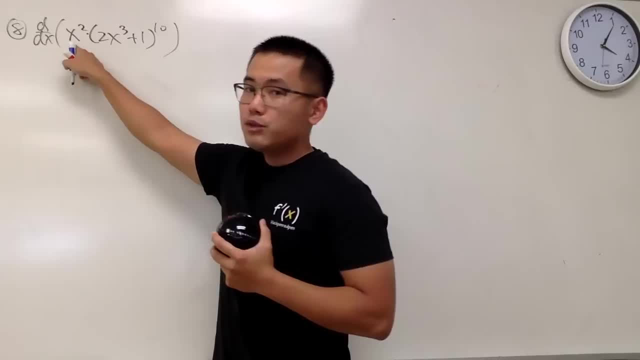 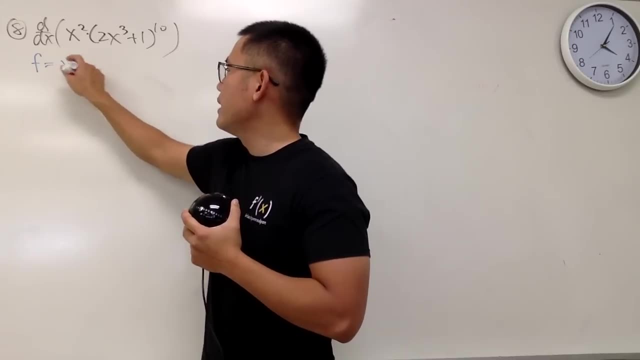 So here we go. Well, this, right here, it's the first function, So I'll just write down x, squared, and I will call that to be f. This is just the first function, x squared like this, And this is the second function. 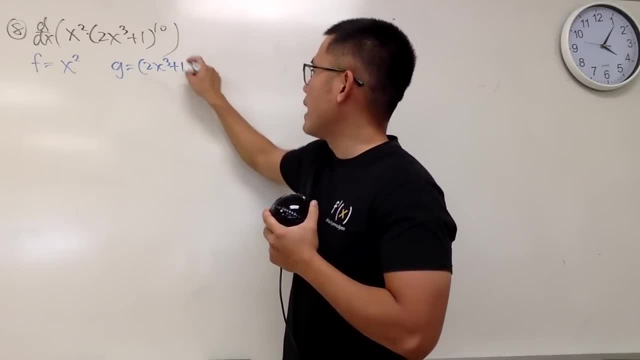 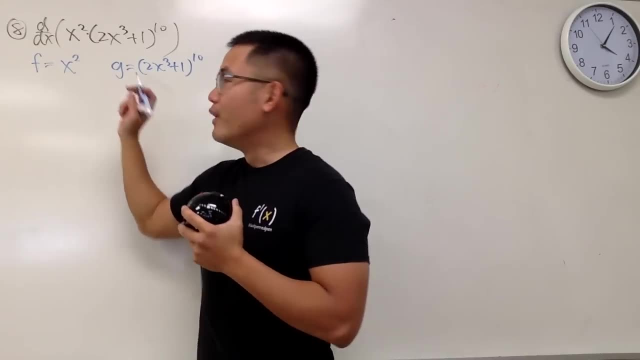 So it's g, which is 2x to the third power plus 1 to the tenth power, like that. Well, separate this and I will differentiate them individually. For the first one, the derivative of this, which is just 2x. 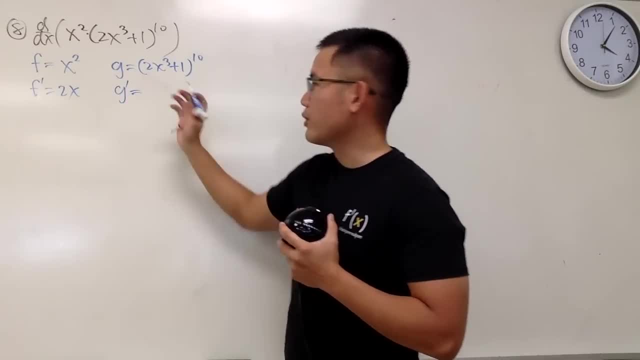 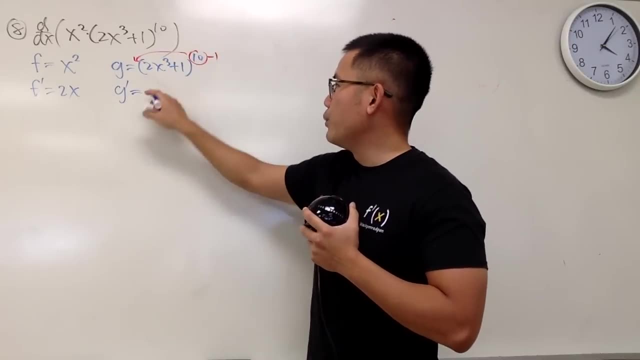 And then the derivative of this. this is g, right, So g prime is going to be the following: The derivative of this: of course, you bring the 10 to the front Minus 1. And we get 10.. 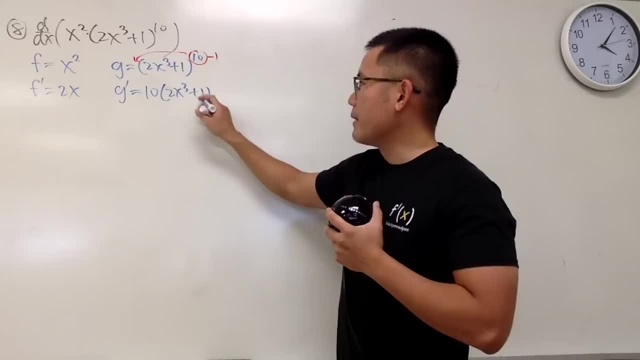 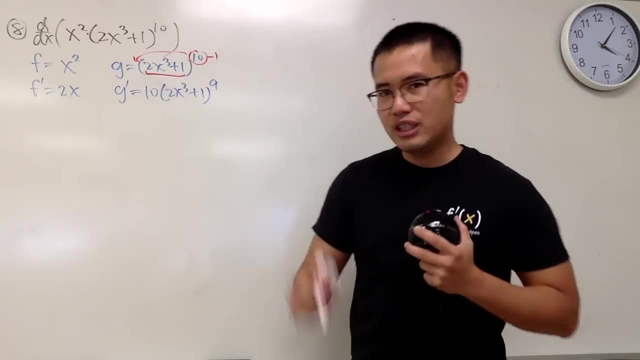 And the inside stays the same: 2x to the third power plus 1 to the ninth power, like that. And then we multiply by the derivative of the inside. because of the chain rule, The derivative of the inside is just pretty much this part. 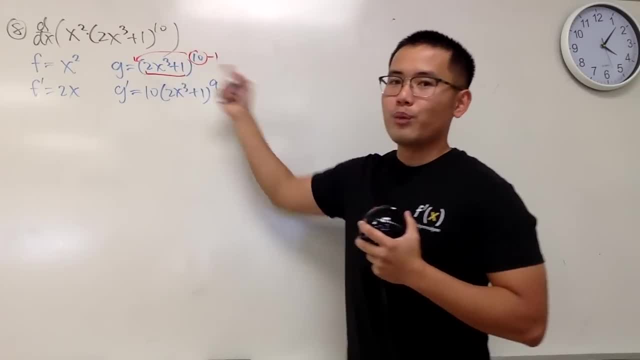 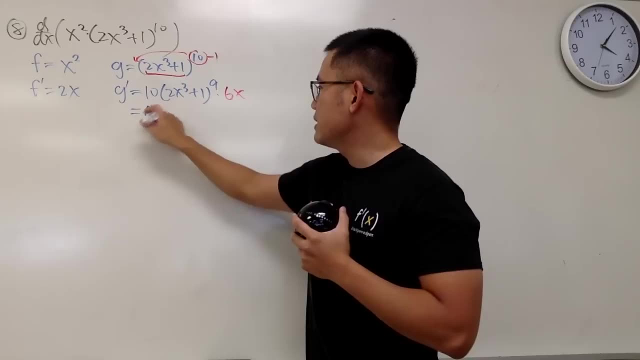 We need the 6x right here, Because the derivative of 1 is just 0. So it's just like that, And of course we can simplify this a little bit: 6x times 10, so it's 6tx. 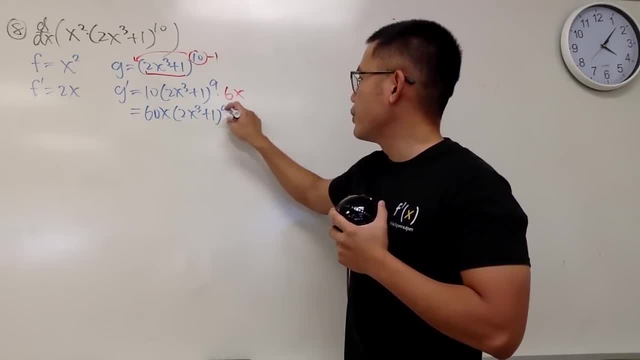 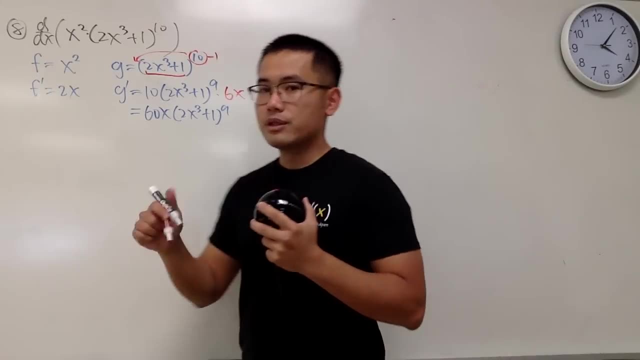 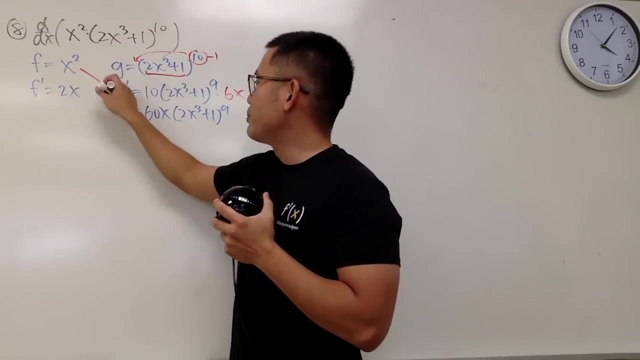 And this is 2x to the third power plus 1 to the ninth power. So you can just set it up like this, And then we just kind of cross multiply to construct our answer. Product rule in action: f times g prime. 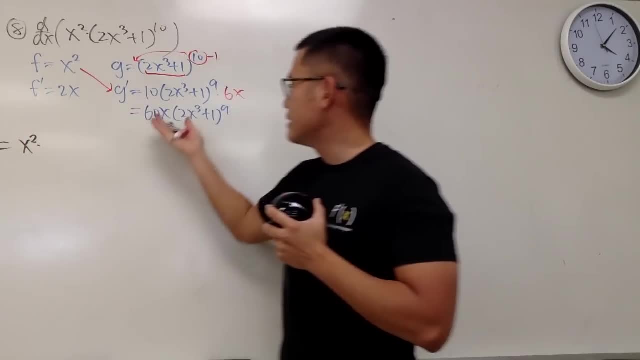 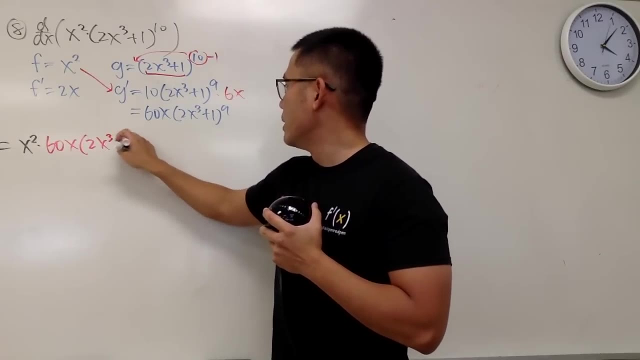 So we will have x squared times this, right. So let me just put this down right here, which is 6tx times 2x to the third power, plus 1 to the ninth power, And then we go the other way, which is this times that: 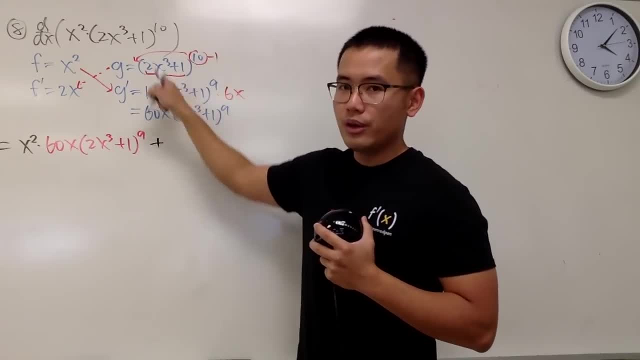 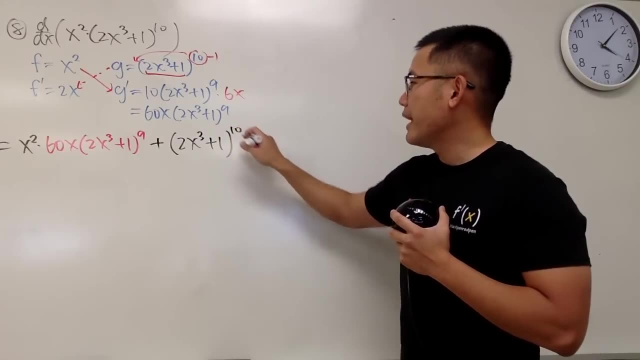 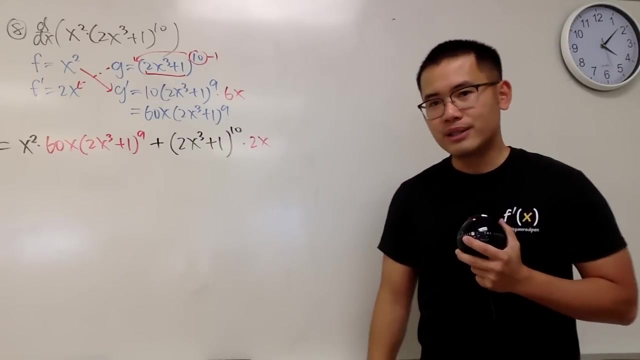 We add this times that which is the original in blue. We have parentheses 2x to the third power plus 1 to the tenth power And we multiply by 2x. So this is the write-out right, By using the product rule and also the chain rule. 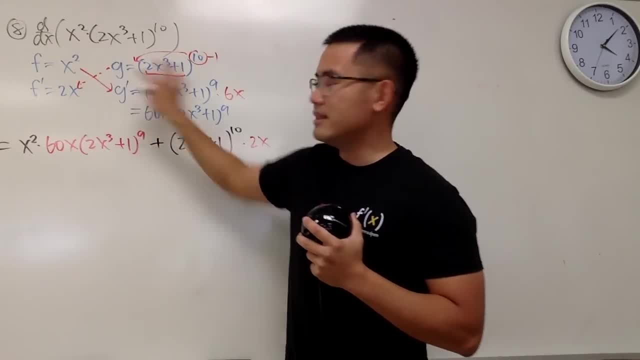 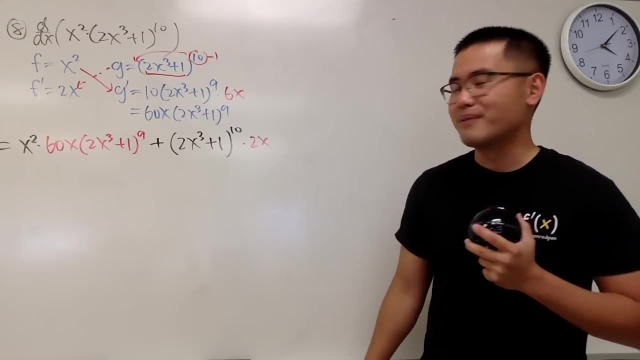 So you just have to do it carefully And later I'll show you guys, without these things right, But I think this is helpful, especially if you're doing derivative effect calculus for the first time. Alright, in the end we just have to simplify this. 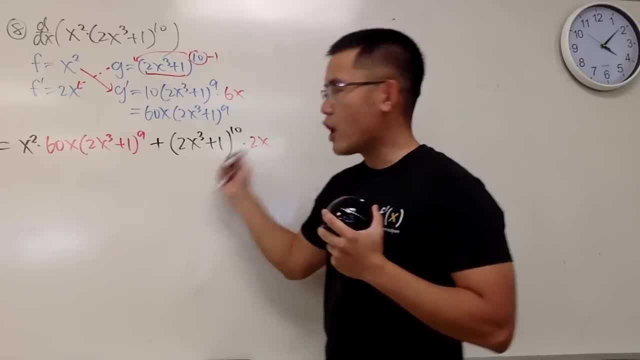 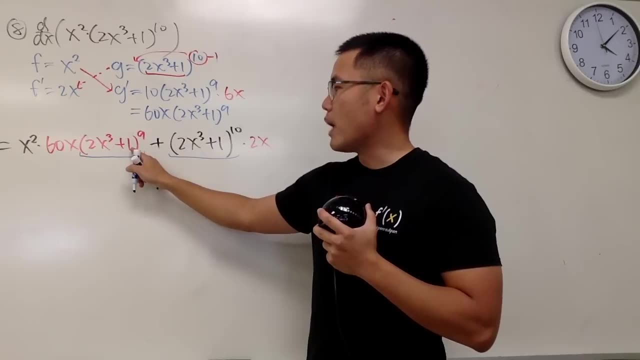 Let's see. First of all, we notice that both terms they have this factor right: 2x to the third power plus 1.. And this is the ninth power and this is the tenth power. So we can factor out the smaller exponent. 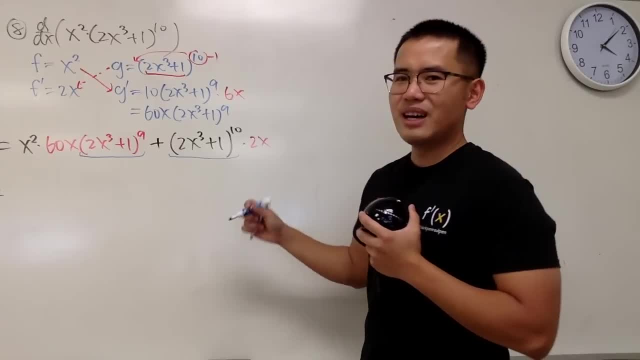 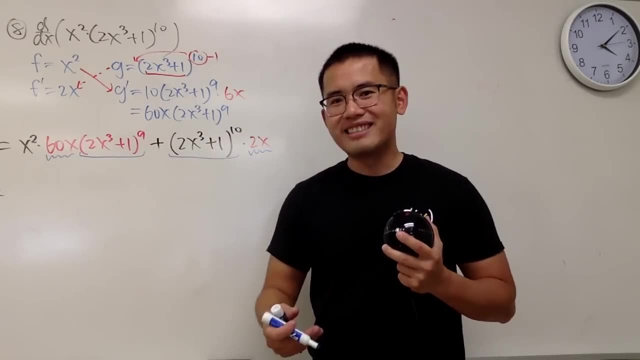 So perhaps let's do that, And in fact we can also factor things out. This right here is 2x And this is 60x. Both of them have x and both of them have a factor 2.. 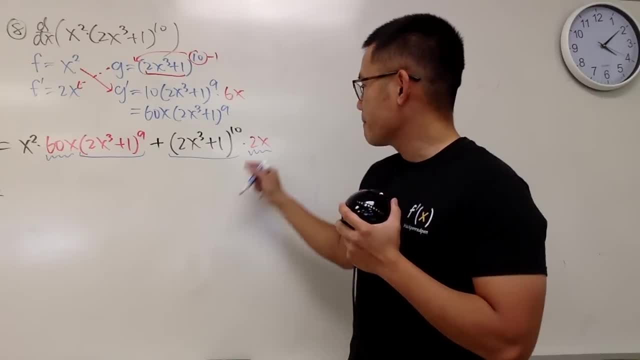 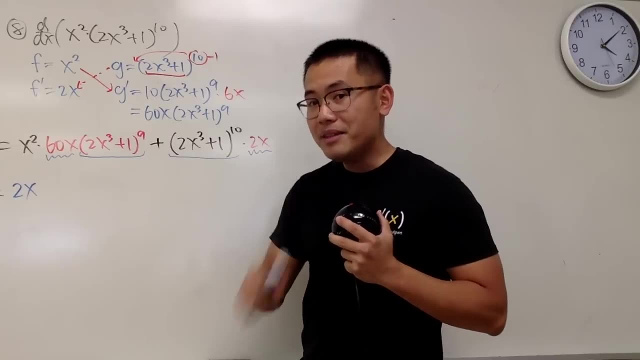 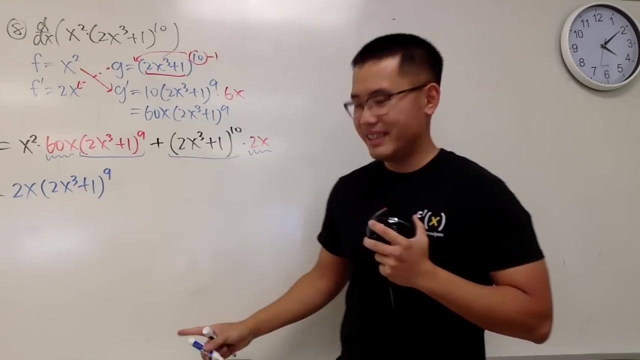 So perhaps let's do this first. Let's put down the factor of this, right? So let's factor out 2x. Alright, let's factor out 2x, Okay. In the meantime, we can also factor this out, which is 2x to the third power plus 1 to the ninth power, like this: 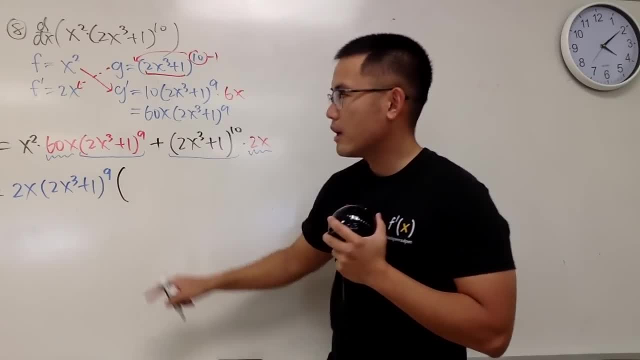 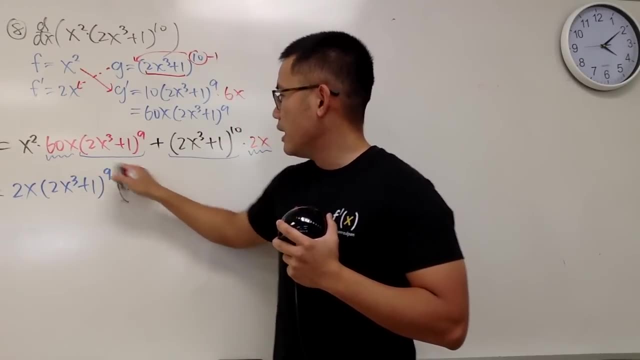 And now let me show you what the leftover is. Well, if you look at this part, we've factored out the 2x. so 60 divided by 2 is 30.. This x is out, but we still have x squared. so we write down x squared right here. 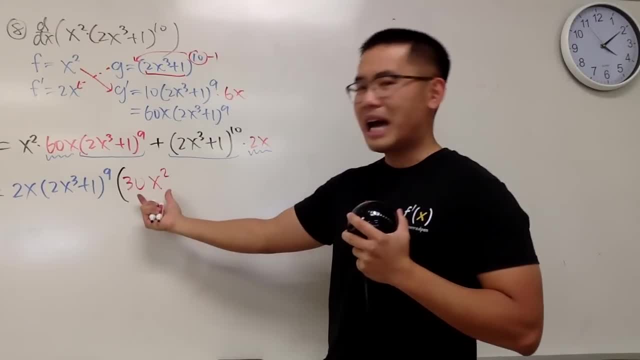 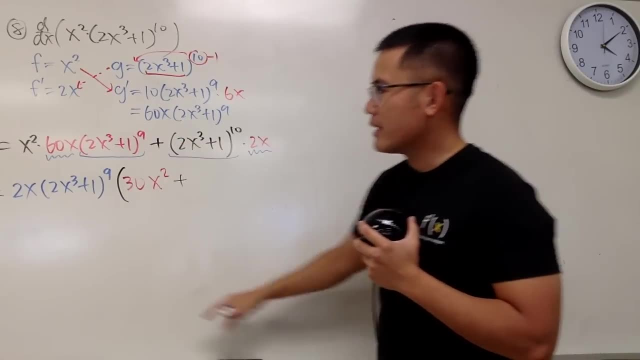 And you see this part. we've factored it out already. so this is all we have, namely 30x squared. Now, if we look at this part first, we have to add: Notice the 2x is in the front already. 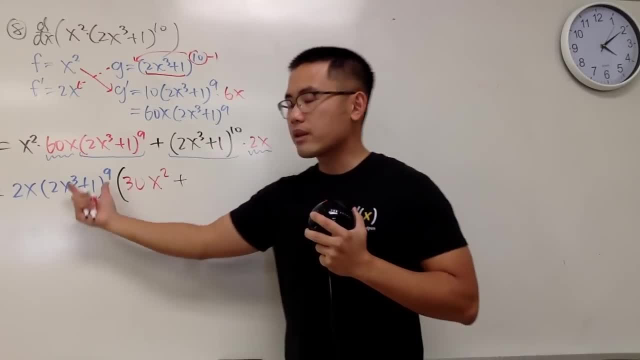 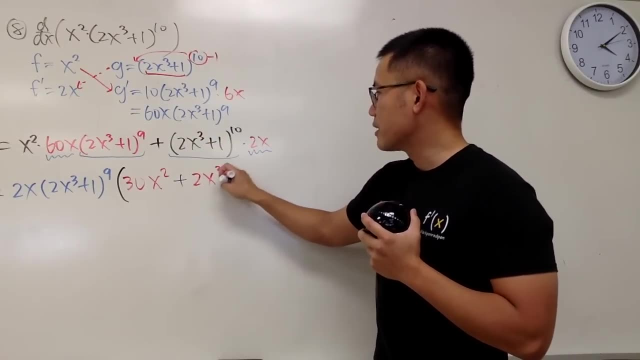 And then, for this part, we see we took out nine of the factors already. That means we have one more. So we just have the inside, which is 2x to the third power plus 1 to the first power, just like that. 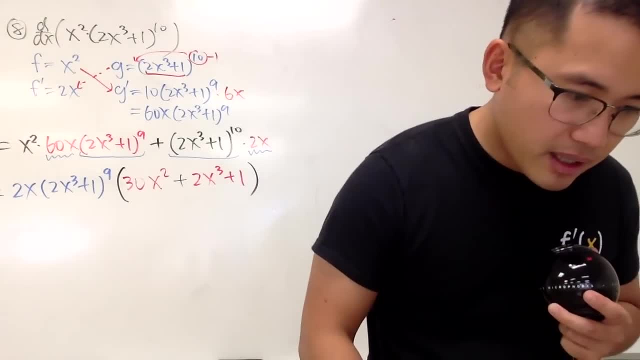 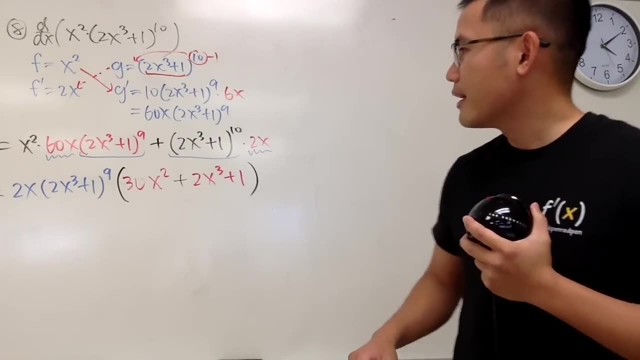 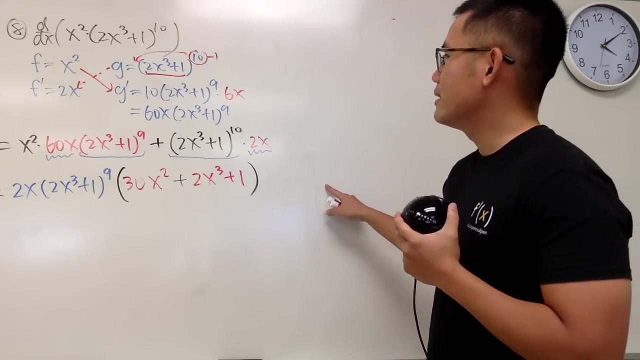 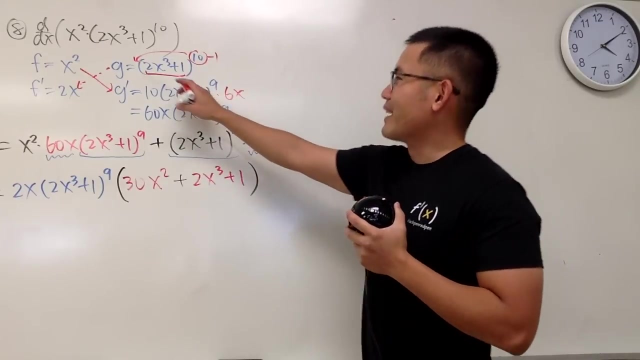 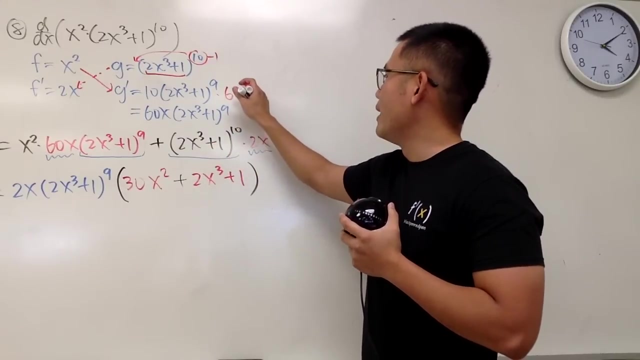 And in the end I just kind of leave it like that. I think, Yeah, I didn't do any. Ah, no, No, I made a small mistake, Man, okay, Okay, okay, okay. 2x to the third power. the derivative of 2x to the third power is 6x squared. 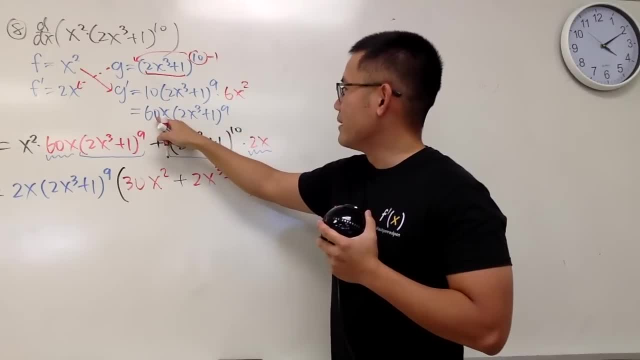 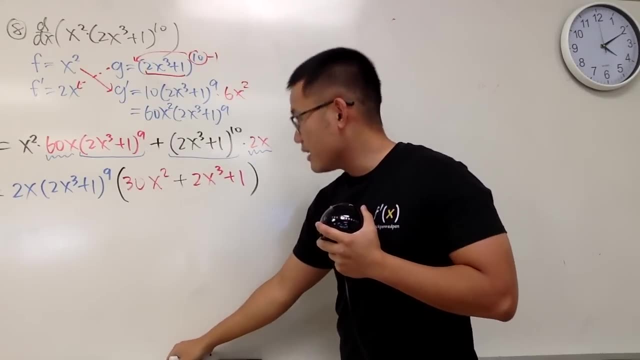 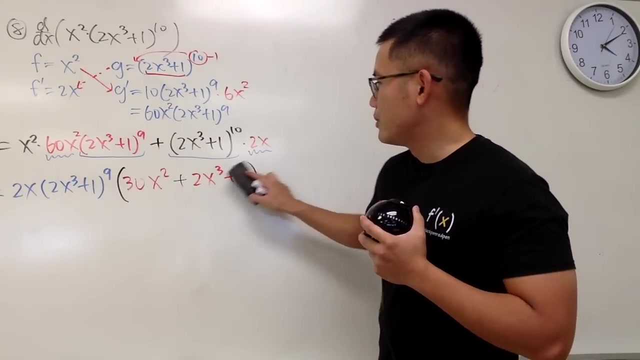 My bad, All right. And then this right here should have been a 60x squared right here, 60x squared right here, And let's see. So this right here should have been 60x squared. And let me just do this part again for you guys. 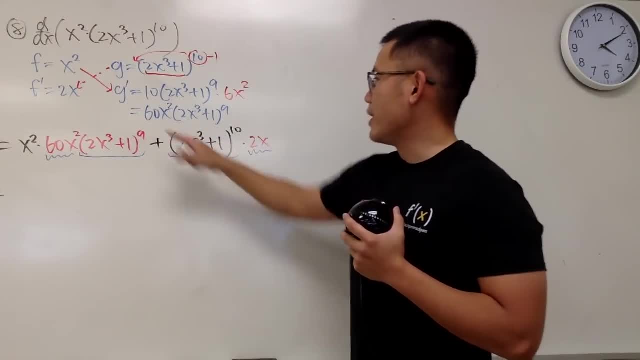 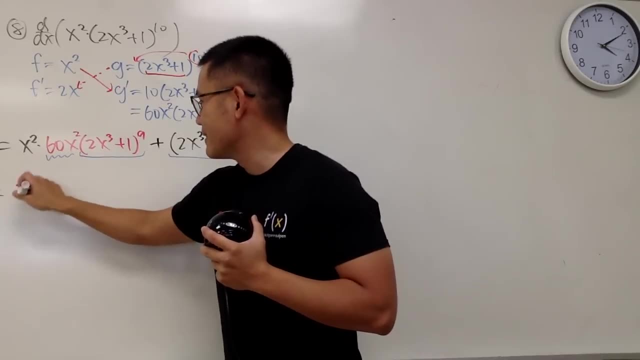 Let me just do this part again for you guys. All right, So 60x squared right here. Again same thing. We can factor out the 2x. right, So we can factor out 2x. Let's do that. 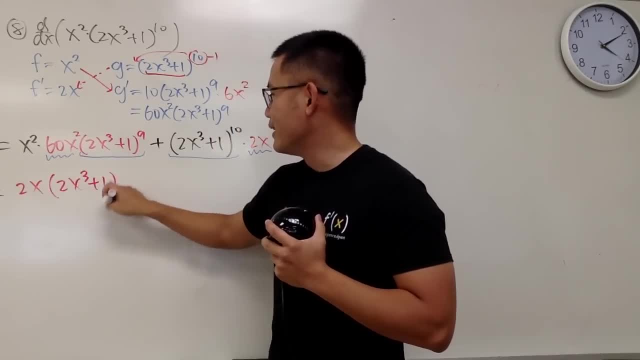 And we can also factor this out- which is 2x to the third power plus 1 to the ninth power. And now, actually, Actually, I put this down in blue earlier, So I'll put it down in blue again. 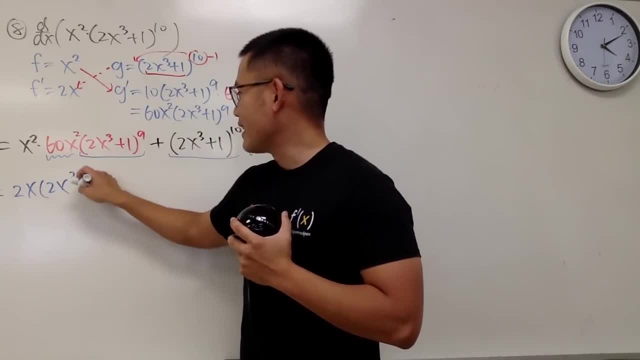 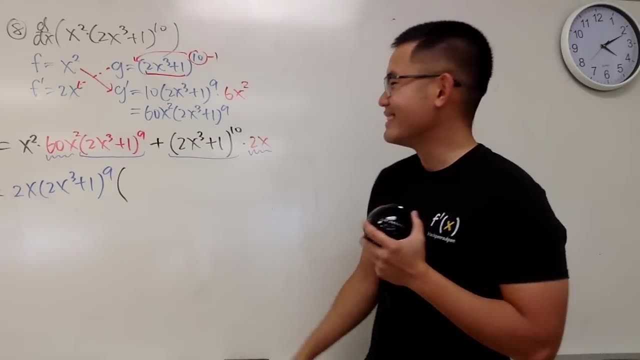 Anyway, 2x, 2x to the third power plus 1, and then to the ninth power And parentheses. you see, I make mistake too. okay, All right, parentheses. okay for this part. again, we took out the 2,, so we have 30. 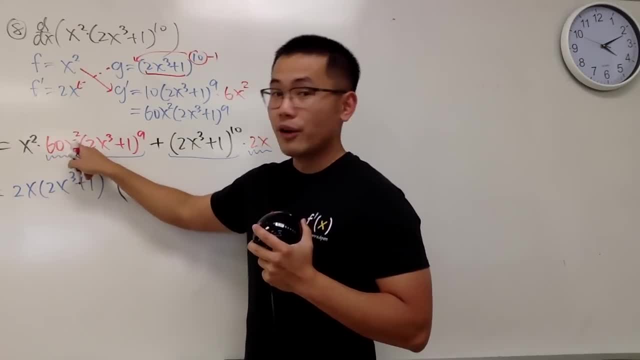 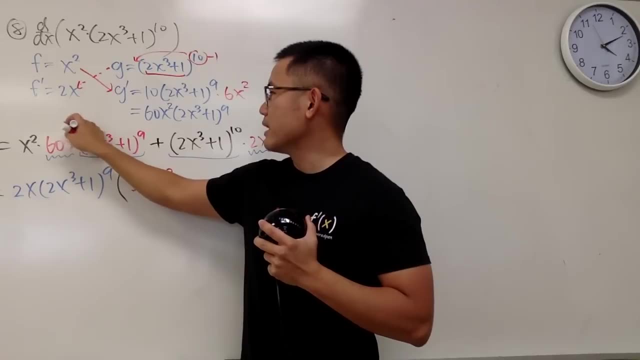 And then we took out an x, So this right here is just x to the first power x times x. squared, though, is x to the third power, Again, because this right here is x squared, so it's x times x. 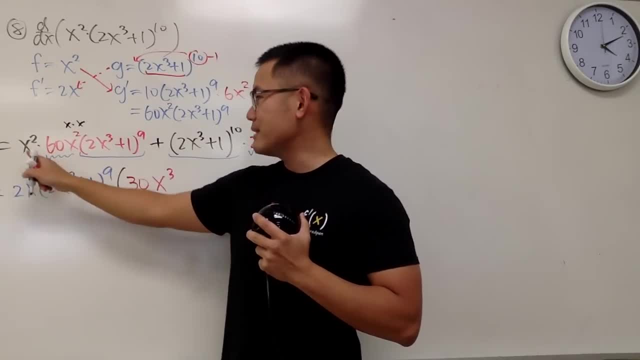 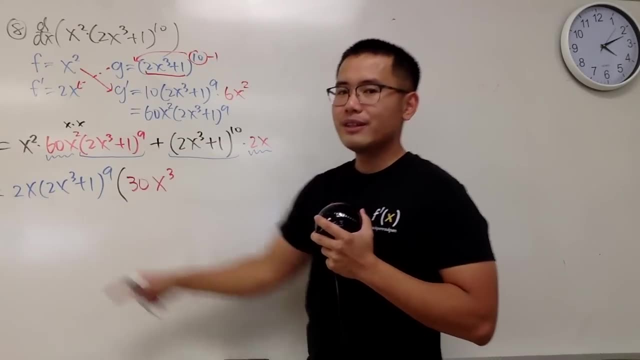 So you took out one of them, you have another x, This x times x to the second power, we get x to the third power. All right, And then that's it for the first part, because this is out. For this part, this is out. 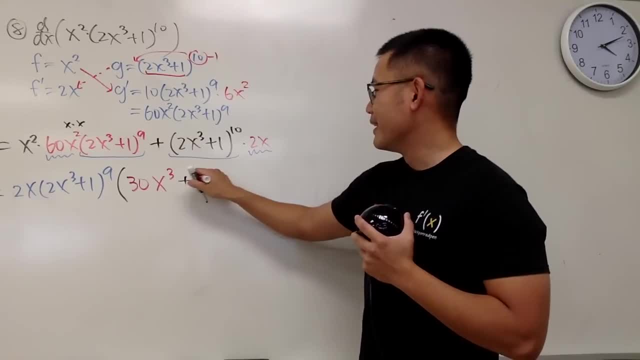 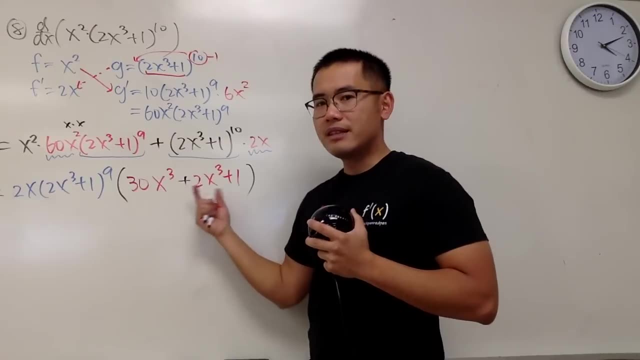 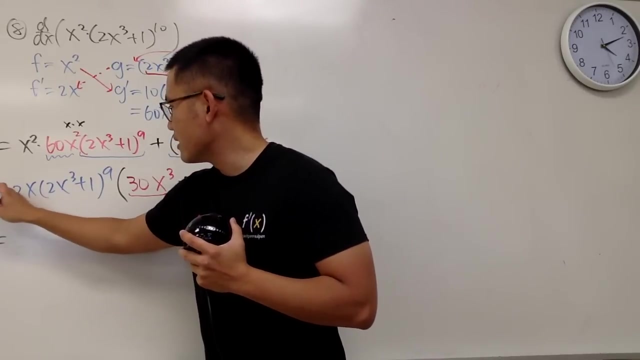 We have this left to the first power, So we add 2x to the third power plus 1 to the first power, like this: In the end we can combine this and that together. So we'll do that And finally we see the answer is: where's my equal sign? 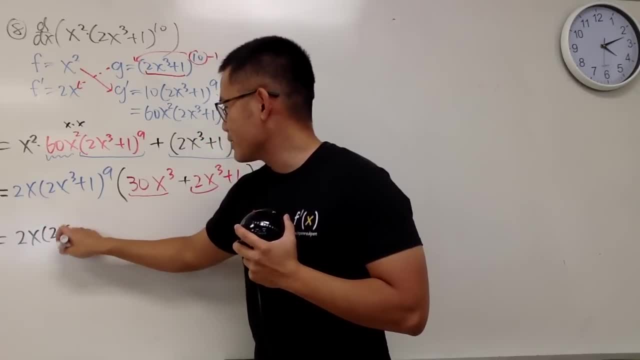 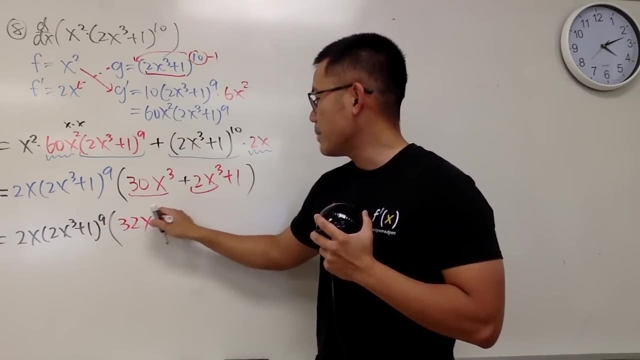 Here we go. The answer is 2x times 2x to the third power, plus 1 to the ninth power. times this plus that, which is 32x to the third power, And in the end we have the plus 1.. 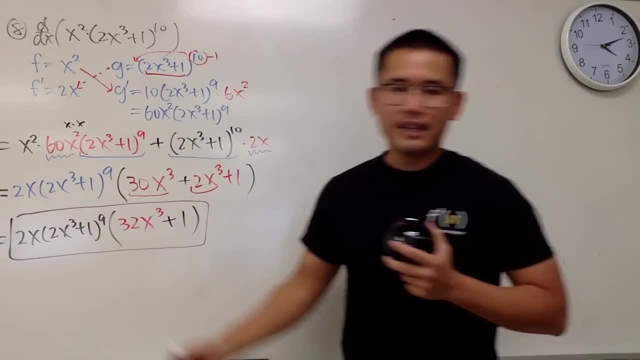 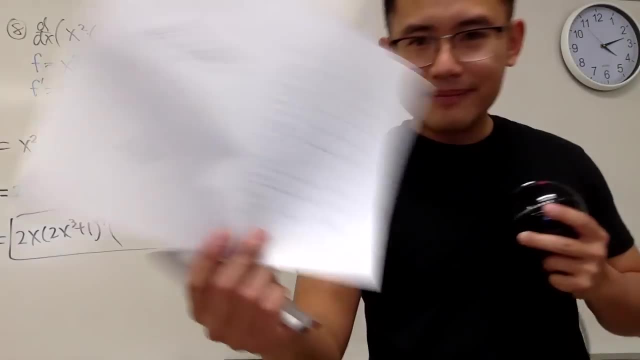 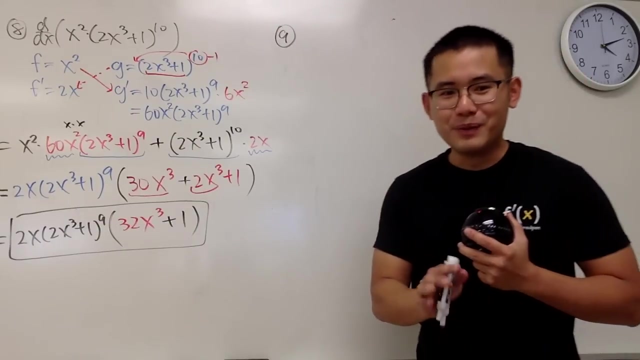 And that's it. So it's simplified pretty nicely, right, And Yeah, All right, Now number 9.. By the way, it took me a lot of time to come up with the answer choices as well, not just the question. 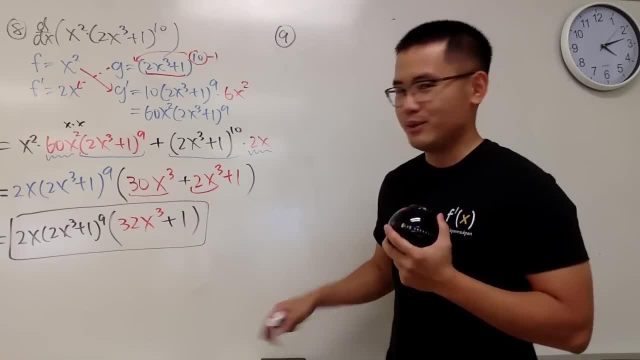 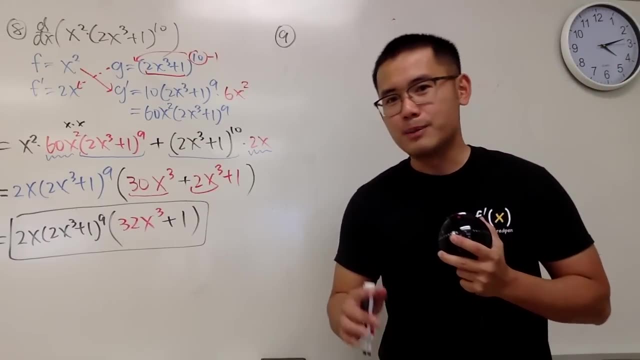 I want to make it rather legitimate. I can just like give it to my students for them to practice And for the actual exams or actual quiz that I give out to my students. I usually have about 5 or 6 answer choices. 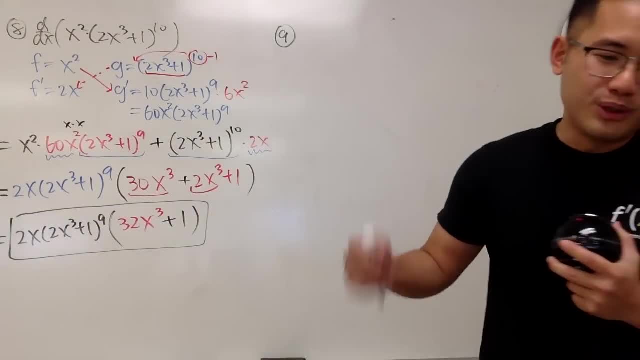 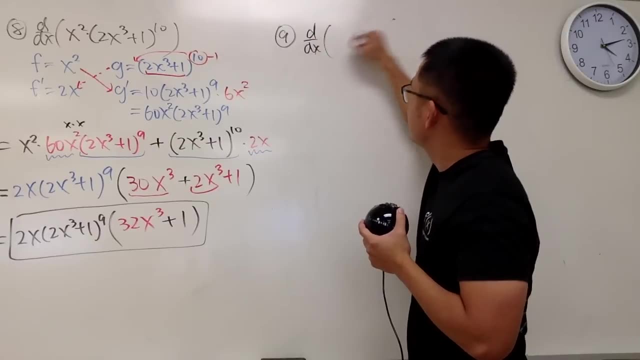 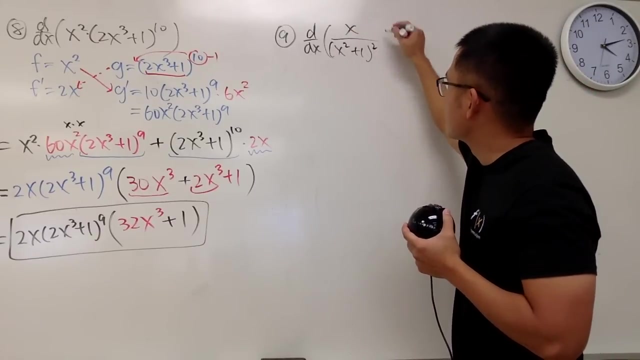 But this is just for practice. That's why I only have 3 choices Anyway. number 9.. Here we go, We have this. We have to differentiate x over, And the bottom here is parentheses: x squared plus 1 to the second power, like that: 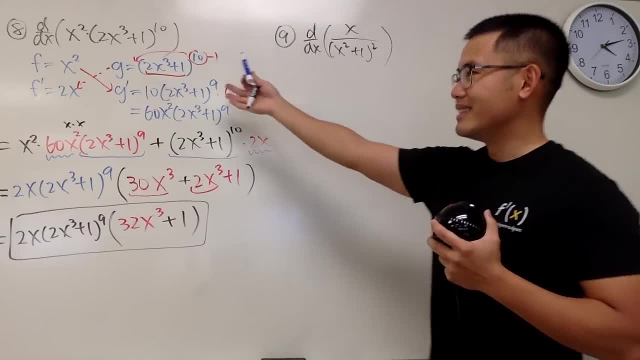 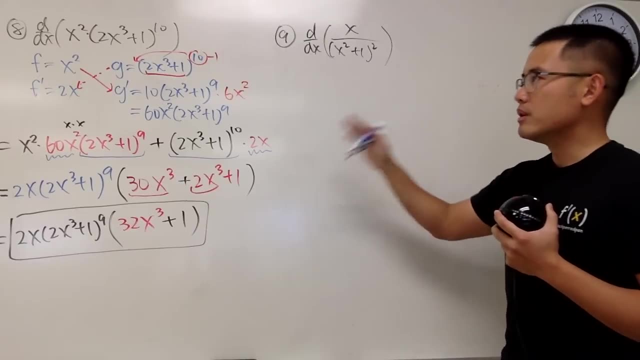 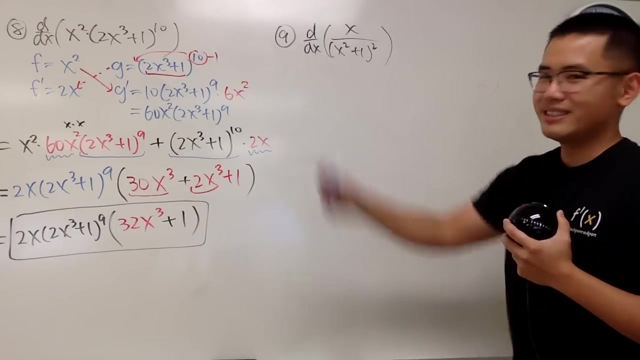 Well, well. Why don't I show you guys this right here as well? I call this the memory device whenever we have to do the product rule, quotient rule and chain rule, and all that Especially if the question is complicated. I like to show my students this. 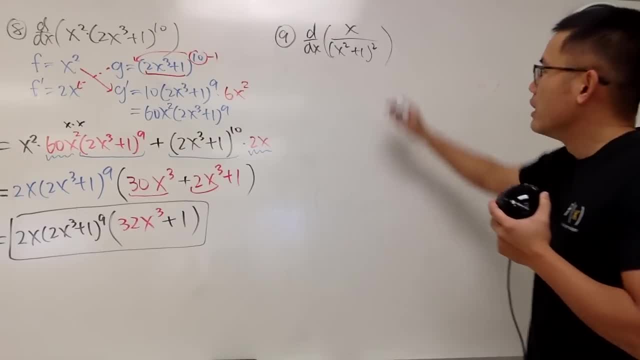 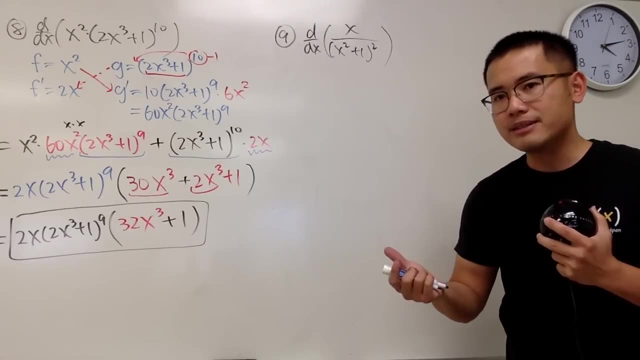 Especially for the first time. Anyway, here we go. This right here is a quotient x over this right. So we have to use the quotient rule And the quotient is just the opposite of the product. So what you do is: on the top is the f function, on the bottom is the g function. 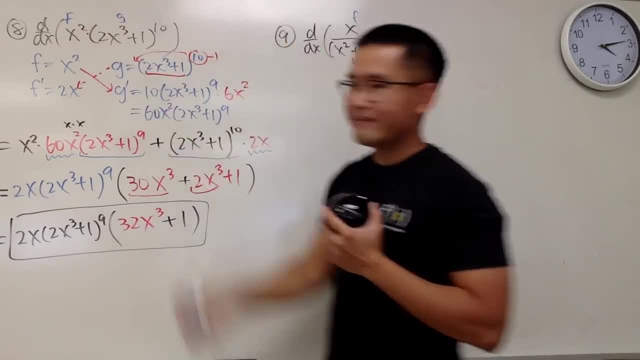 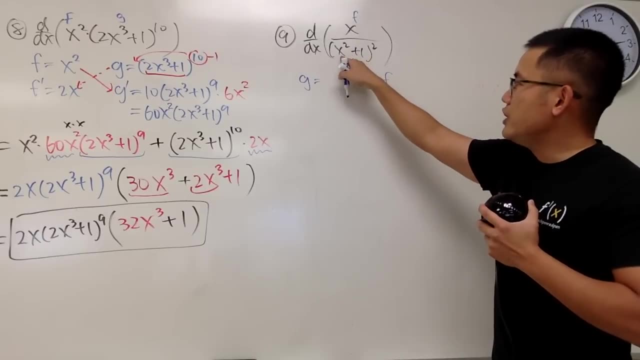 Well earlier. you see, the first one is f, the second one is g. Well, for the quotient rule, we actually write down g first And then f, right here. So the g function is this, which is x squared plus 1 to the second power. 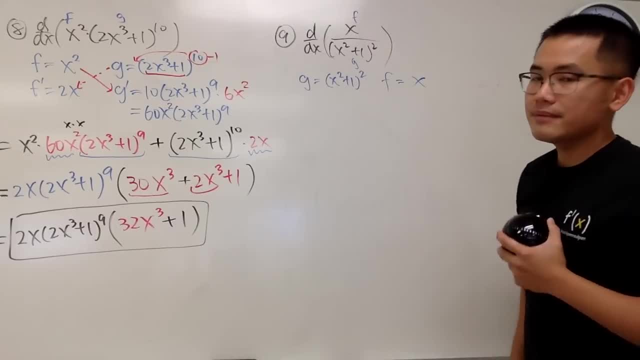 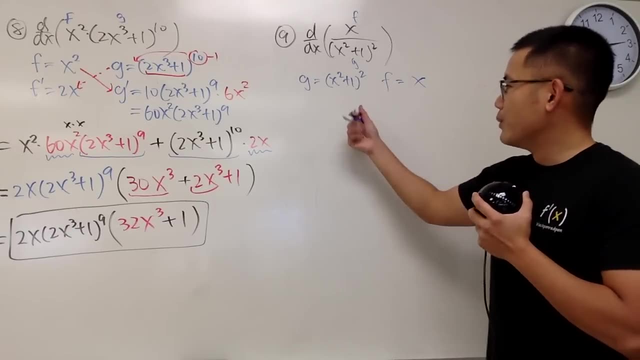 And then the f function is just x on the top. Once we put them down individually, we can just differentiate them individually. For the first one we will just get g prime And this is going to be okay. put the 2 to the front minus 1.. 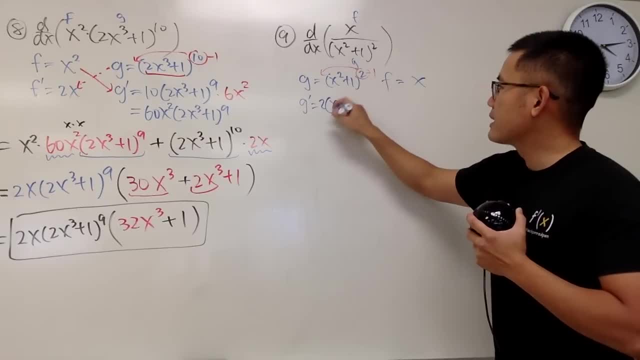 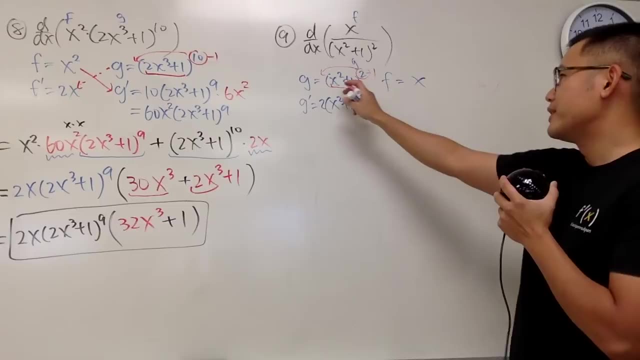 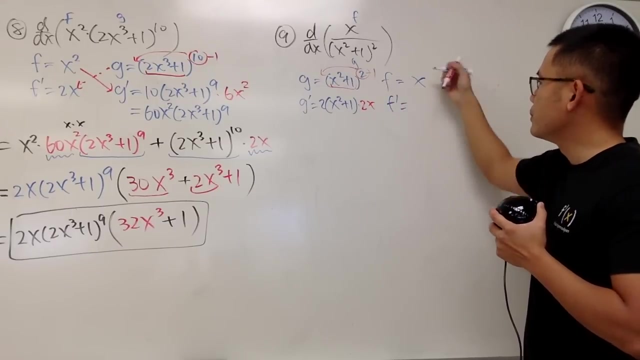 And we will get 2 parentheses, x squared, plus 1 to the first power, And we multiply by the derivative of the inside. Because of the Chengdu, the derivative of this is 2x. So just like that. Well, for this one, of course, differentiate this real quick. we just get 1.. 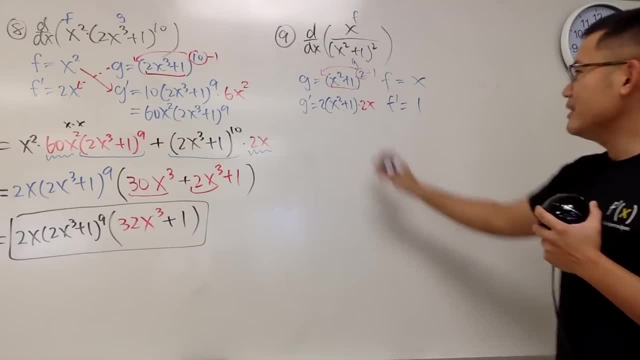 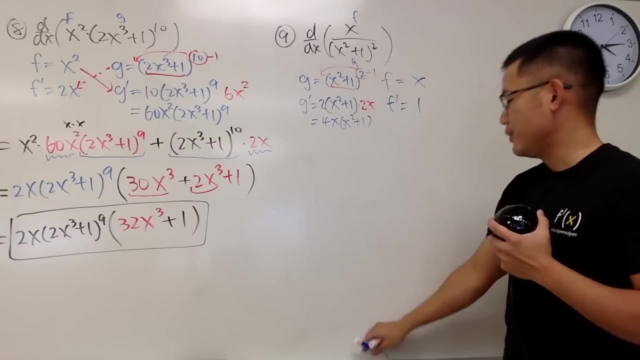 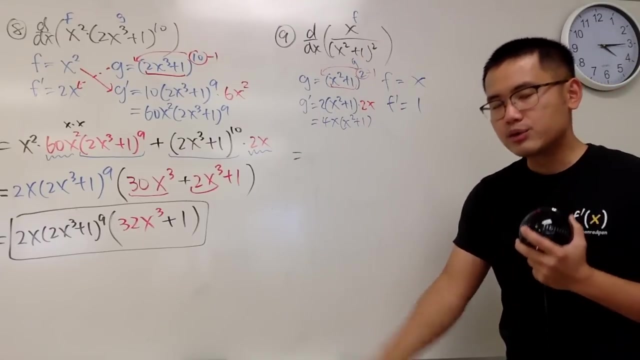 So that's pretty nice, And let's simplify this a little bit. This is just 4x times x squared plus 1,, if you would like, right? So I think we'll just leave it like that. Now, the answer to this: to construct the quotient rule. 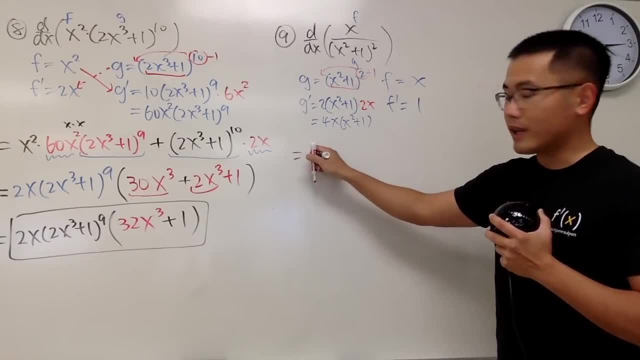 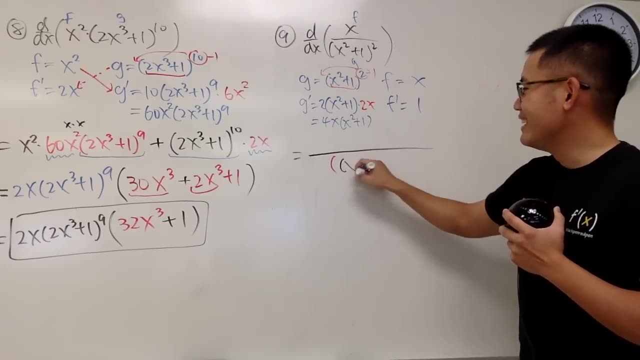 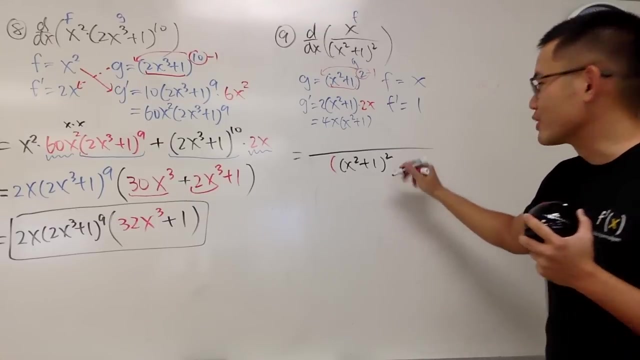 You do this times. that still right. But before we forget, we have to square the denominator right away. So I will put down parentheses with this: inside: x squared plus 1 squared. This had a square. that's the original, But we still have to square it because of the quotient rule, right? 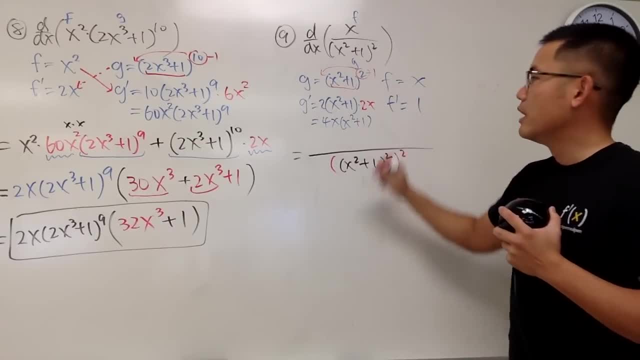 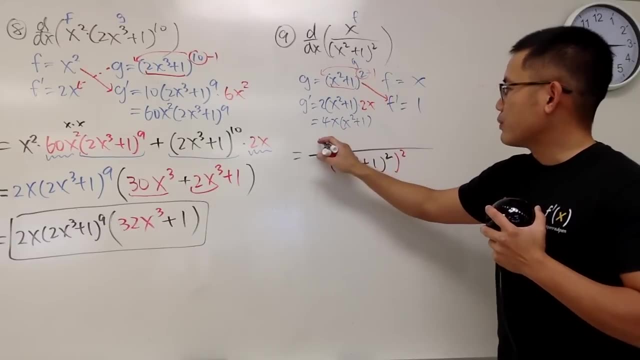 Okay for the top. this is where the top comes in. I'm going to multiply this with that. So this right here is just that which is I'll put in. I'll just put in red. why not? x squared plus 1 to the second? I was just putting black? 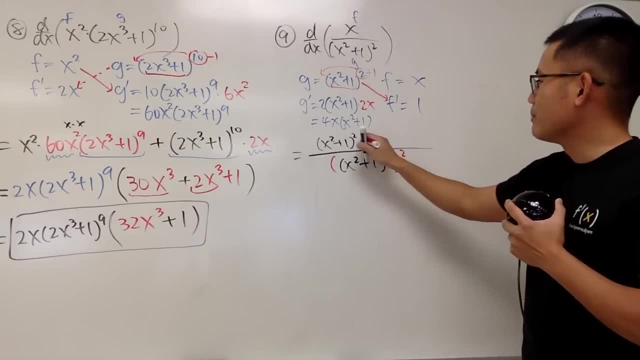 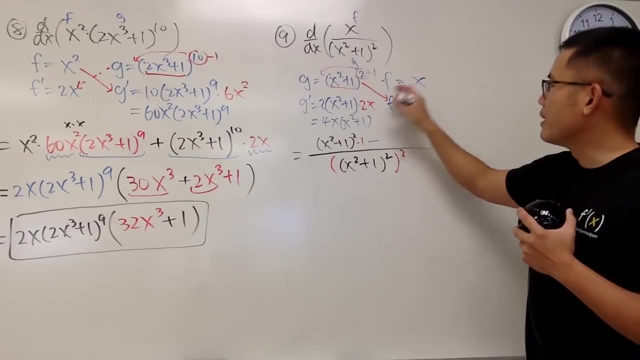 This times that. so x squared plus 1 squared, and we multiply by 1, right here. And then for the quotient rule, remember it's subtraction, So we subtract and we go from here to here. So we subtract this times that. 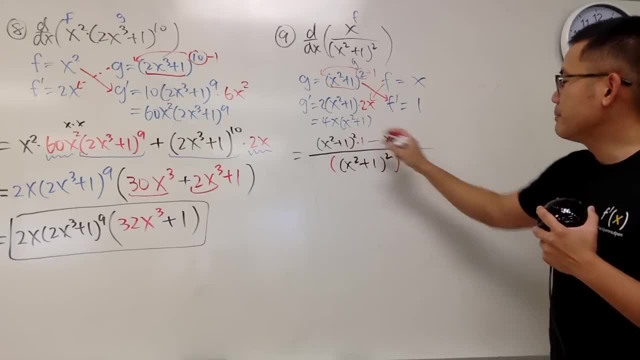 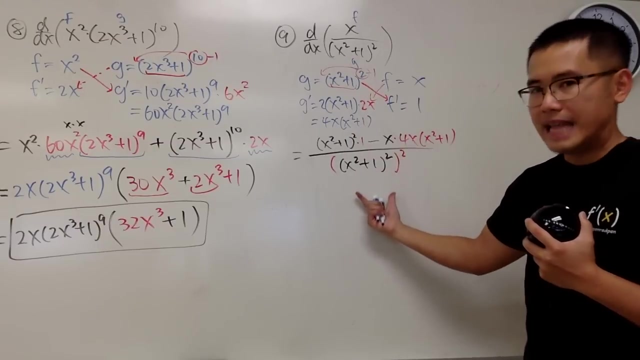 Alright, we have x Times, this part Which is parentheses. let me just put it on the dot Times: 4x times x squared plus 1.. Like this, And of course this is the good way You can just square the denominator. 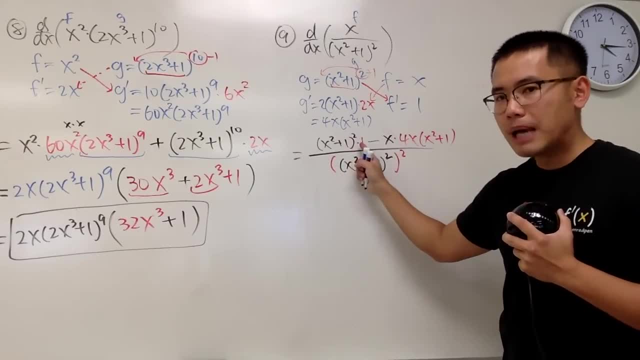 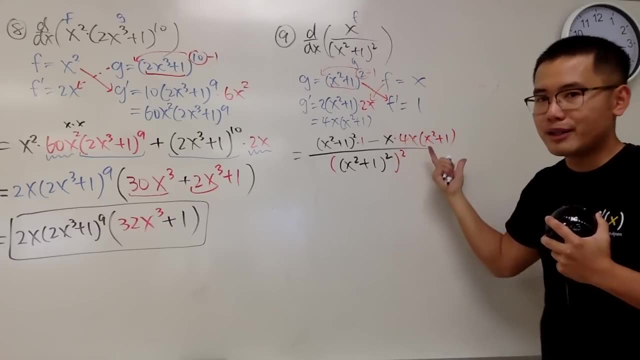 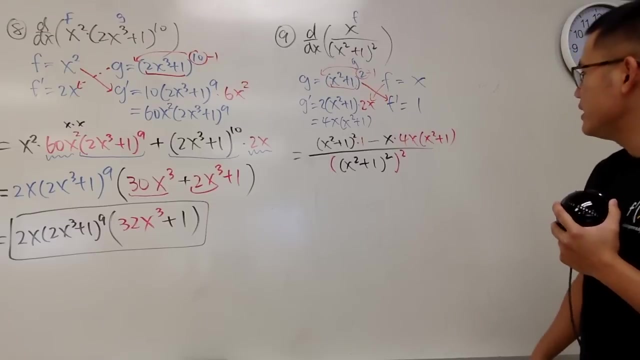 And you put the bottom function right here And you multiply by the derivative of the top And you minus the top function times the derivative of the bottom, And later on I will really just be doing dot steps without showing this right here. Okay, let's see if there's anything we can do to simplify this. 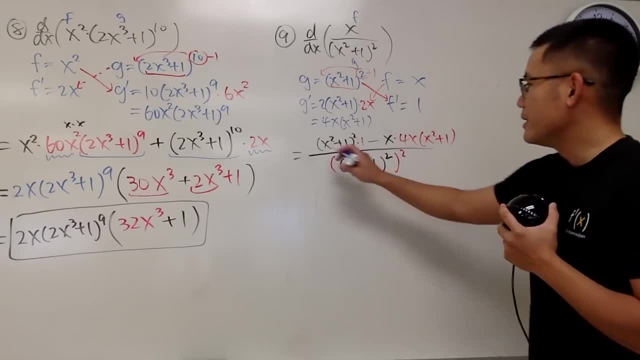 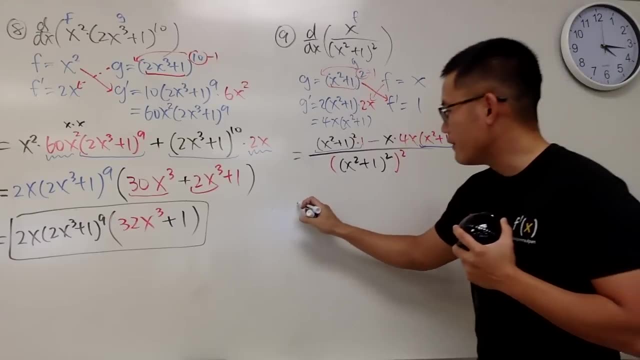 Notice on the top. we can again factor things out, Because here we have x squared plus 1 to the second power, And here we have x squared plus 1 to the first power. So we can factor that out, Parentheses: x squared plus 1.. 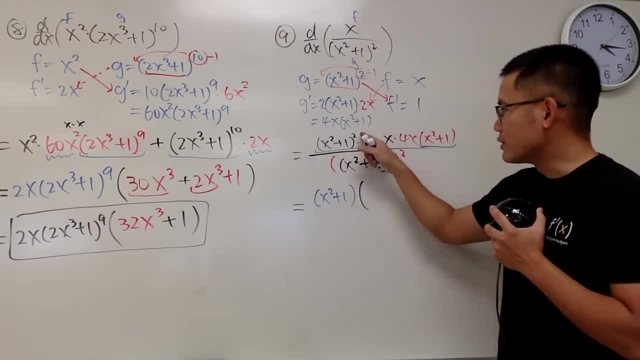 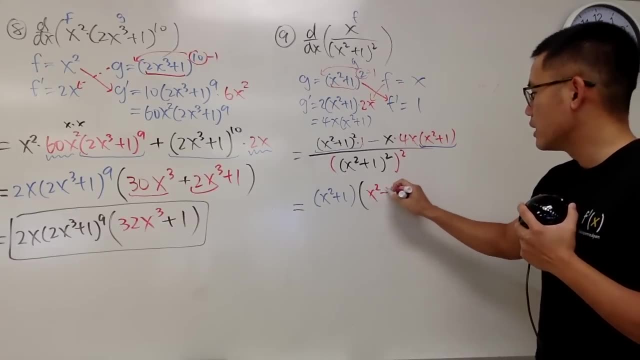 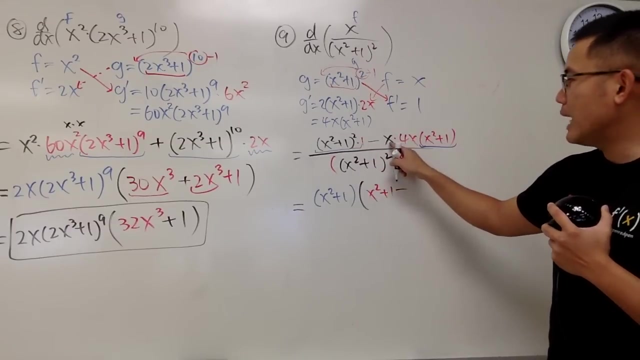 And let's see what we have left. Originally, this was to a second power. We took out one of them, So we still have x squared plus 1. Good, And then we have to minus. Well, this is out, But we still have to have this and that. 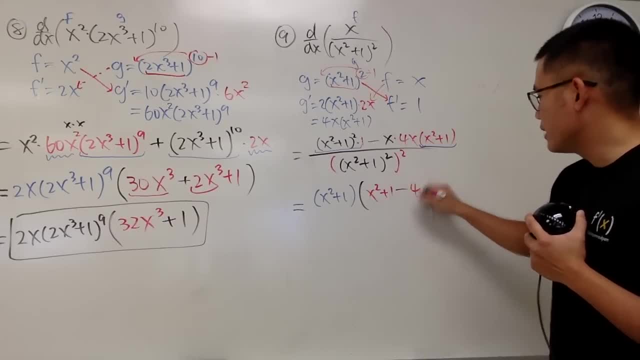 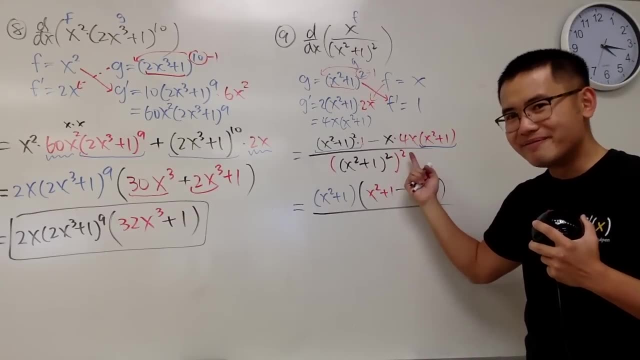 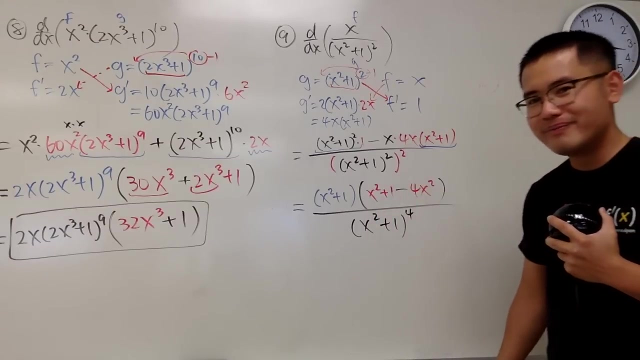 And we multiply them together: 4x squared right here. So we put that down, of course, And then all over, Of course. when we have this square and the square, we multiply the powers. So we end up with x squared plus 1 to the fourth power. 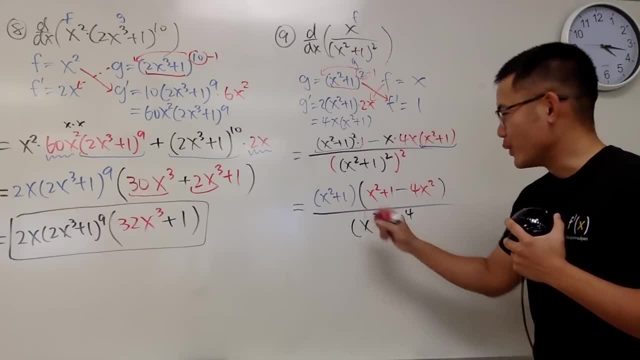 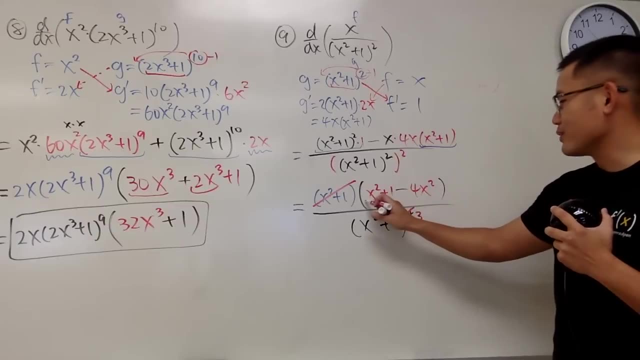 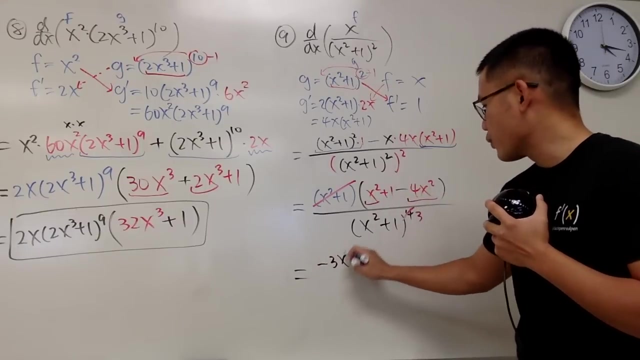 And now check this out: This and that can reduce, So we will cancel this and that out And this becomes the third power, And that's pretty much all we can do. And of course we will also combine this and that. So finally, this minus, that is negative 3x squared. 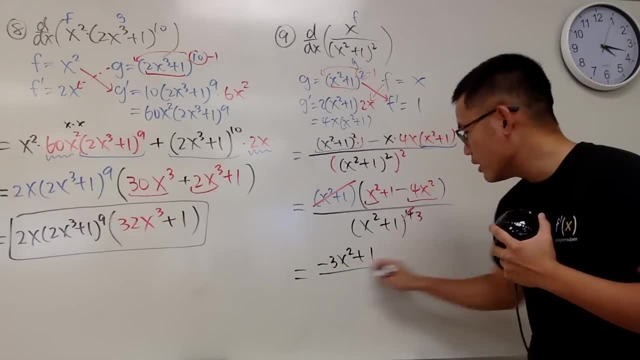 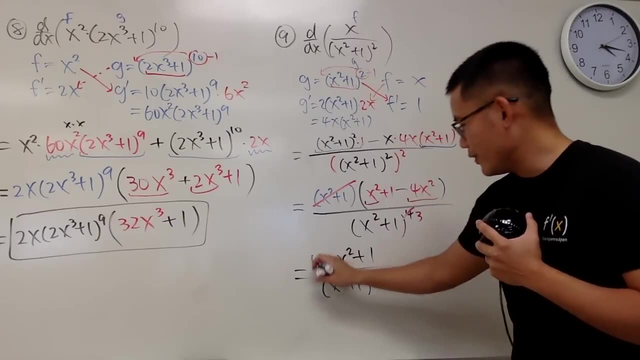 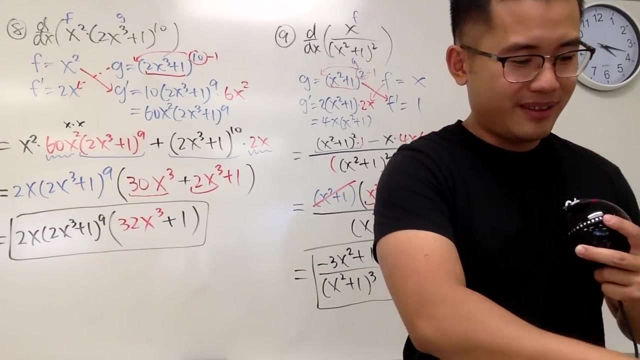 And then we have the plus 1.. Over this to the third power. So x squared plus 1 to the third power, Like this, And with that we are done. That is it, And very nice. We did the first page already. 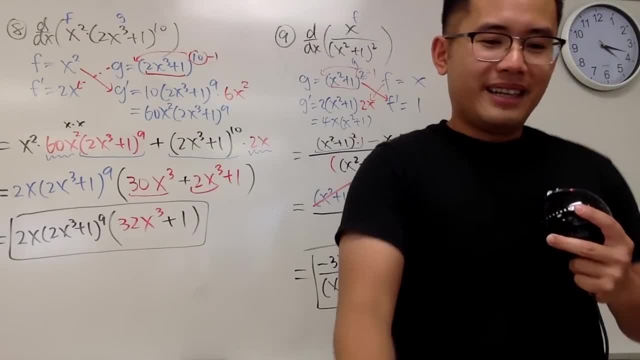 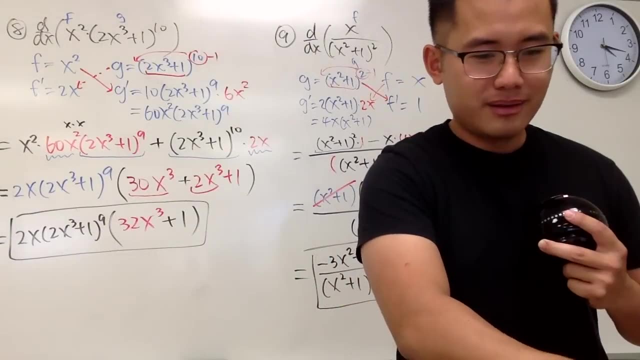 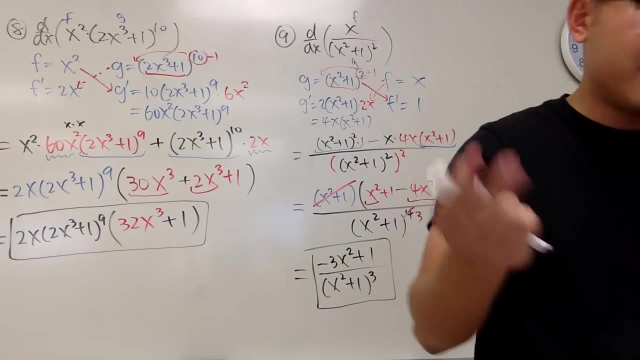 Let me just show you. That was the first page, But the problem is there are 13 pages, So I don't know, man. Anyway, 10 questions took me this long, Five, six hours again. It's OK though. 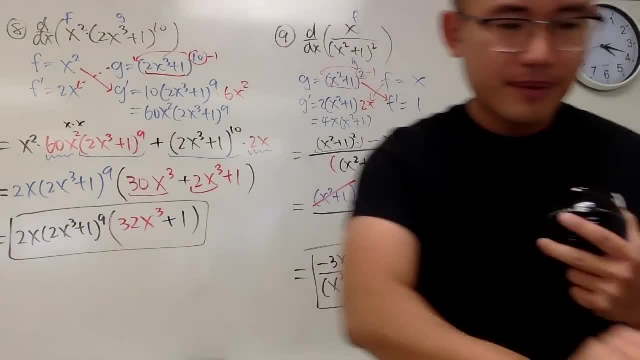 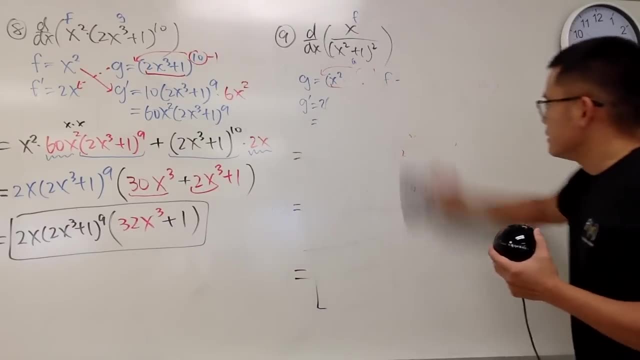 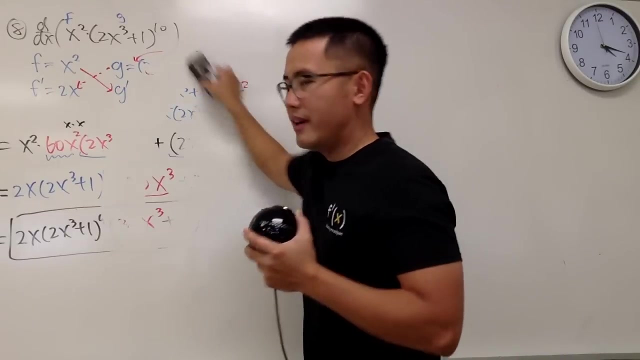 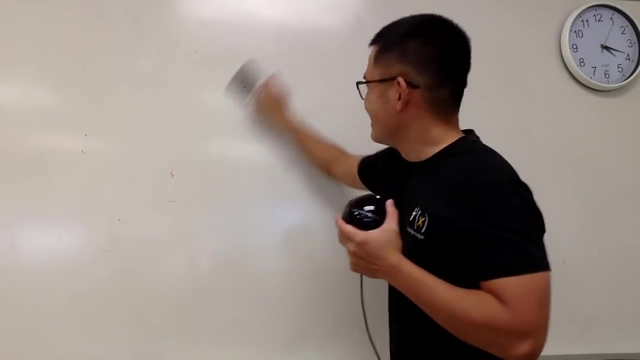 The more we do it, the faster we get, Anyway, number 10.. Right, But I will have to erase this. OK, Maybe I will drink the ninja milk Milk, The ninja milk, Once I reach question number 30.. 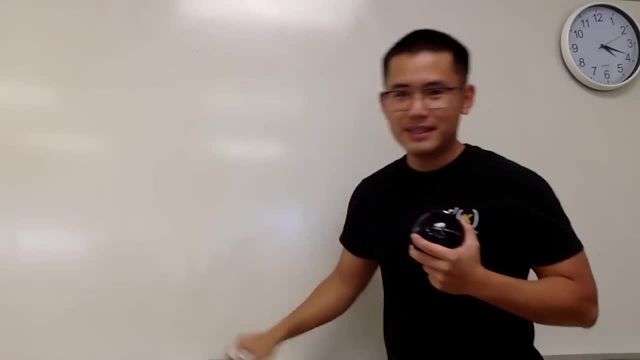 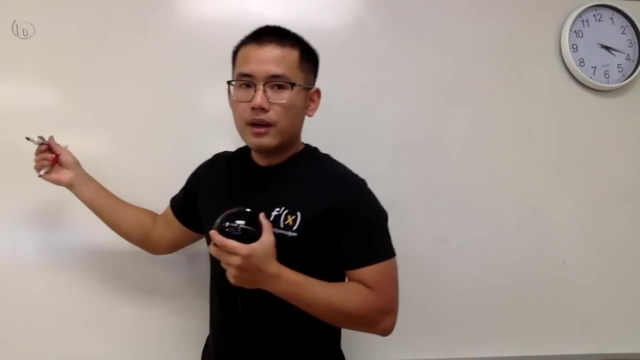 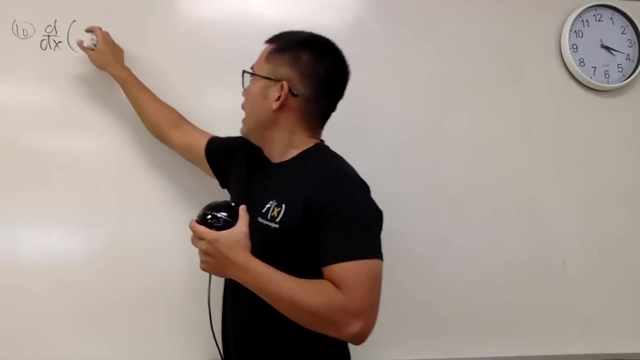 Yeah, I think that's a fair thing for me to do. All right, Number 10. Differentiating the following: So we will be differentiating: On the top we have 20. And on the bottom we have 1 plus 5.. 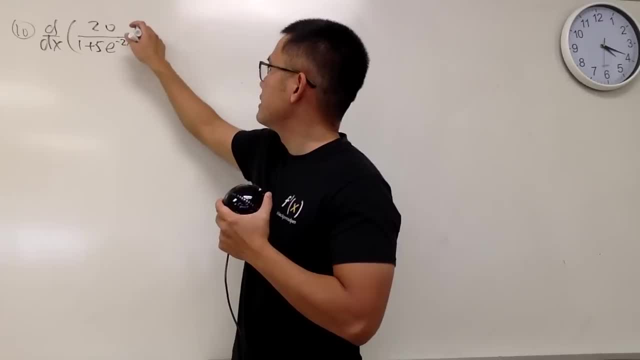 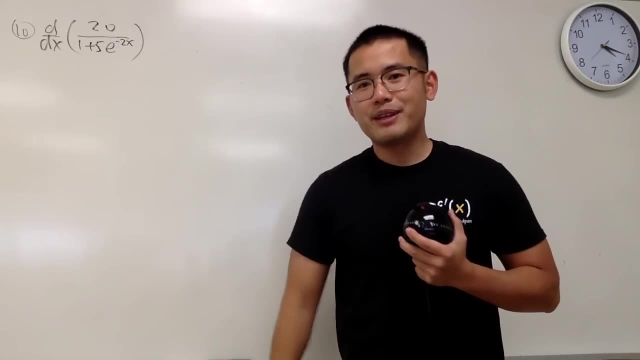 And this is e to the negative 2x. Like this, Right, Like that, All right, Good. Well, let me just tell you guys a little thing. This right here, like this function, right here, you can see it from the logistic growth function. 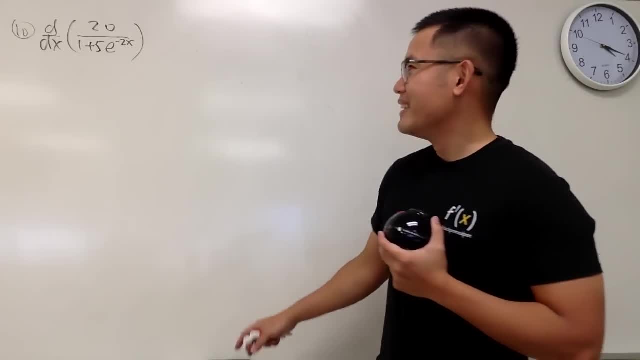 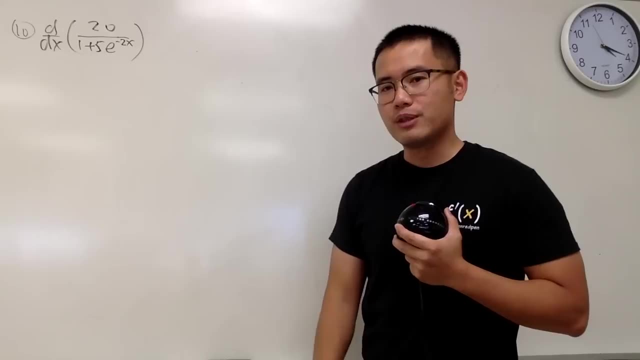 So it's not quite exponential, but it's logistic, So it's really legit, OK. Well, how do we differentiate that, though? You don't necessarily have to use the quotient rule. You can, but you don't have to. 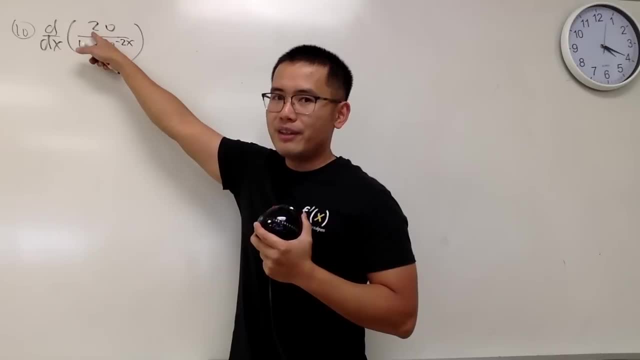 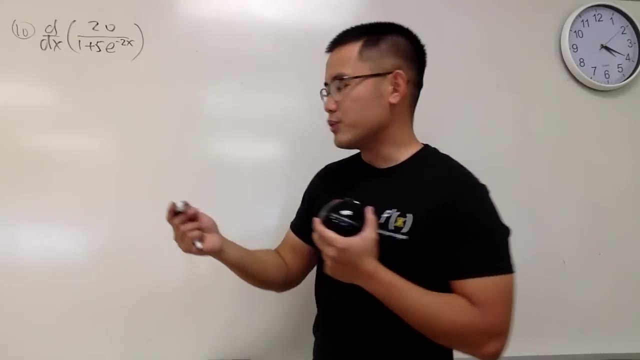 And the reason is because, notice, on the top, we just have 20,, which is just a constant. This is the function part, right here. right, It's easier to do it. this way We can just write the s to take the derivative. 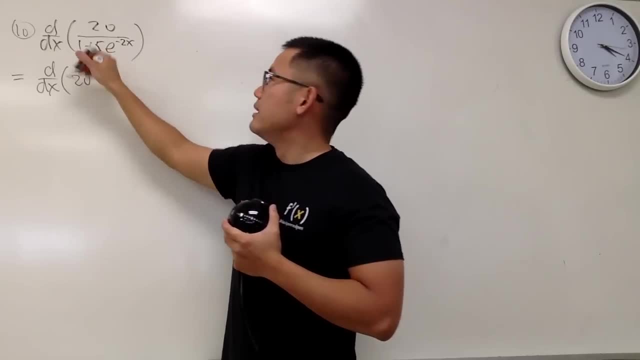 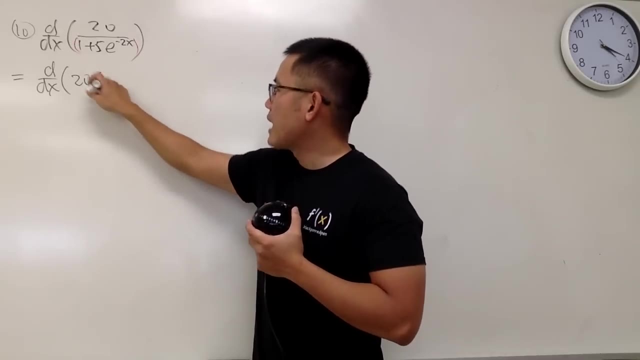 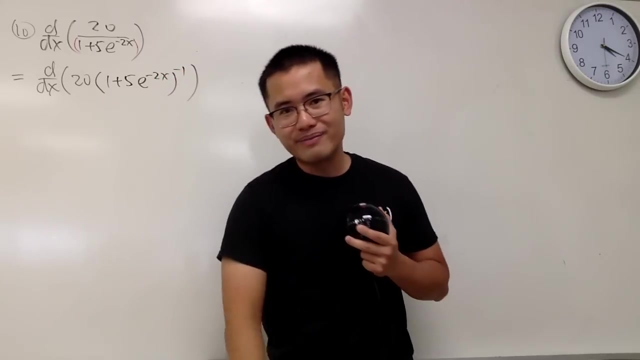 20 is still 20, but we can write this the denominator, bring that up and raise that to the negative 1 power. So 20 times 1 plus 5e negative 2x like this to the negative 1 power. 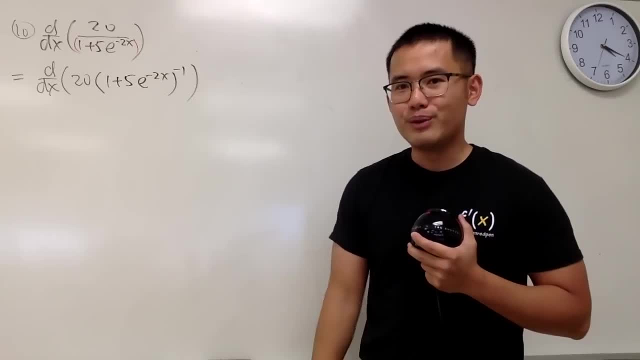 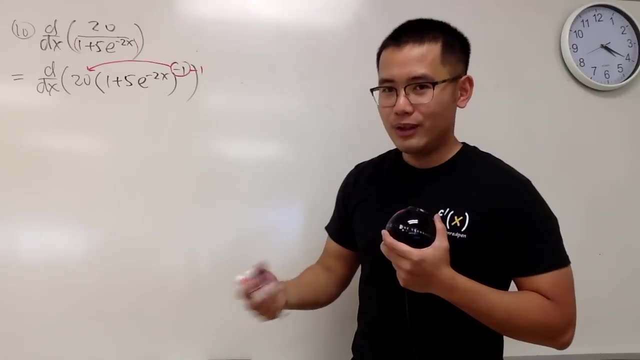 And the reason to do that is because we don't have to use the quotient rule. this way, We can just bring the negative 1 to the front And then minus 1 to the power And do the chain rule after that. All right, 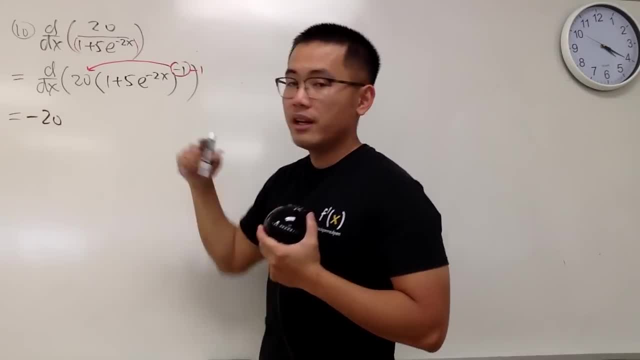 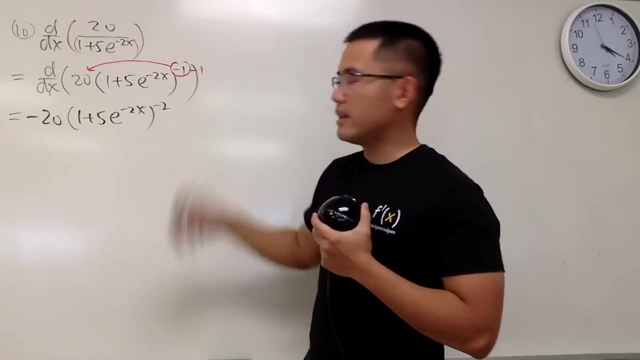 20 times negative 1, we have negative 20. And this right here again states the same: 1 plus 5e negative 2x Negative 1, negative 1. So altogether you get negative 2.. 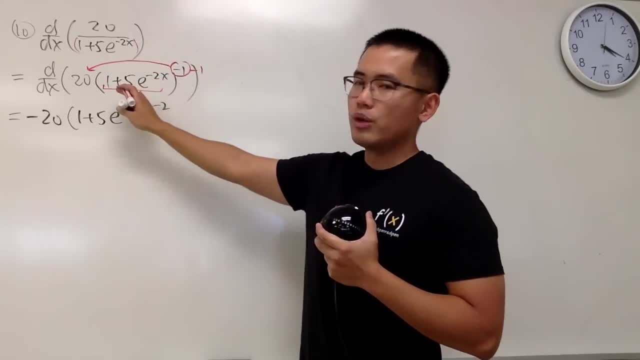 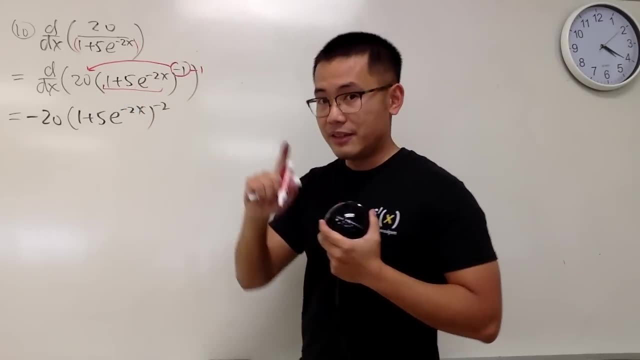 But not done yet. Use the chain rule: Multiply by the derivative of the inside. Derivative of 1 is 0.. Derivative of 5e to the negative 2x is the following: Whenever we have e to the 5th, this part just repeats itself first. 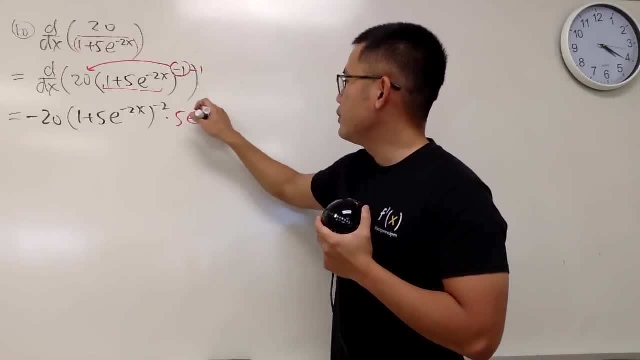 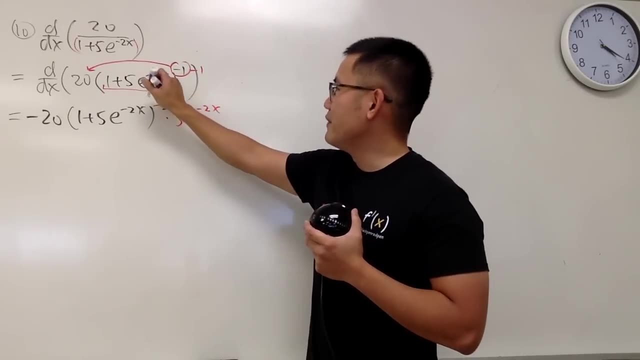 So we multiply by 5e to the negative 2x. But we're not done yet Because we have to look at the derivative of the inside of the inside, which is this part. The derivative of negative 2x is negative 2.. 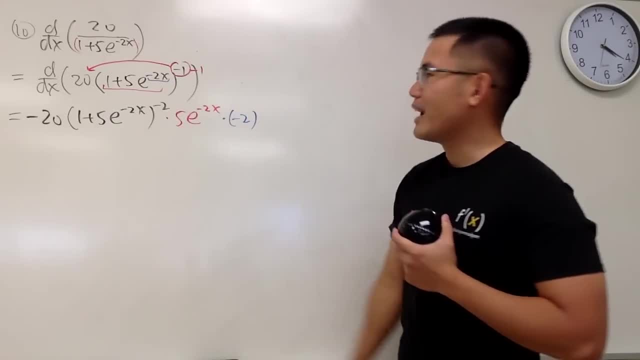 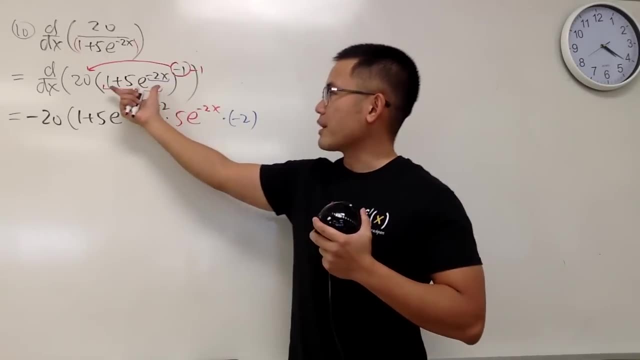 So we have to multiply by negative 2, right here. So we have to use the chain rule twice for this part. All right, So this is from here, And then, to differentiate this part, we have to multiply by the derivative of negative 2x. 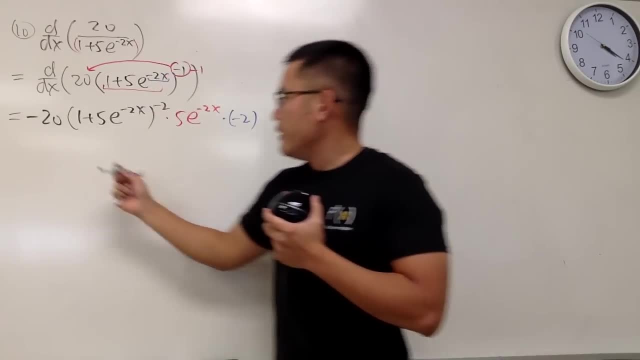 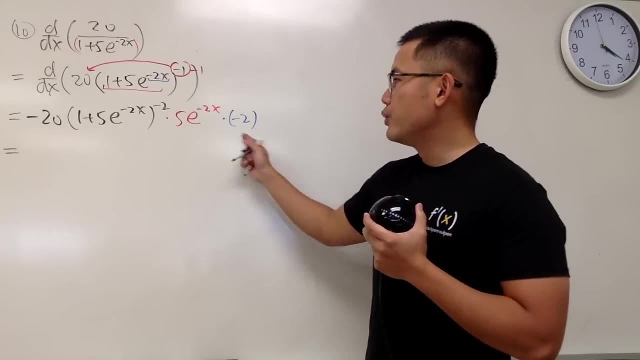 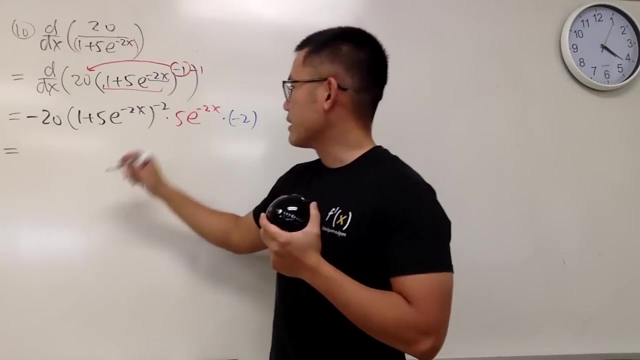 which is the negative 2 right here. Okay, Now we will just put everything together. Let's see Negative negative, we get positive. 2 times 5 is 10.. Times 20 is 200.. And I will just leave this on the top as well. 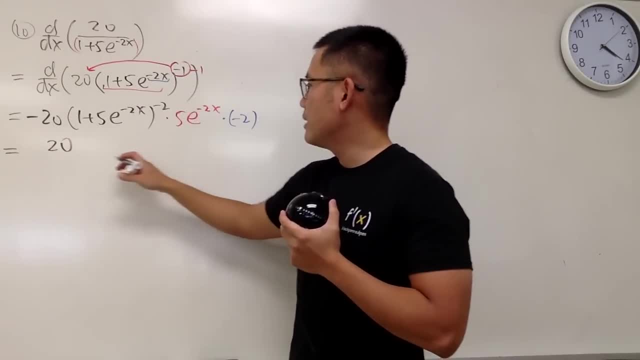 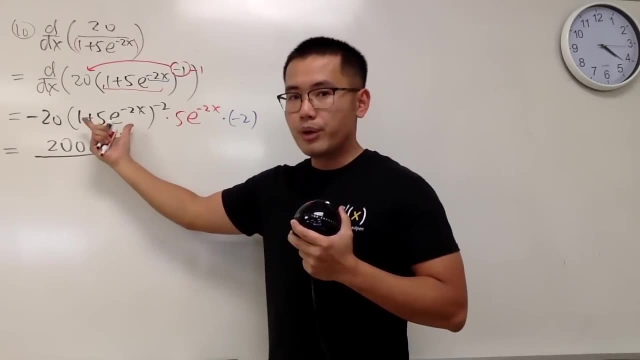 So we have 20.. Oh, I mean 200. And we have e to the negative 2x, like this. And then I have this all over. We can bring this down to the denominator, which is 1 plus 5e to the negative 2x. 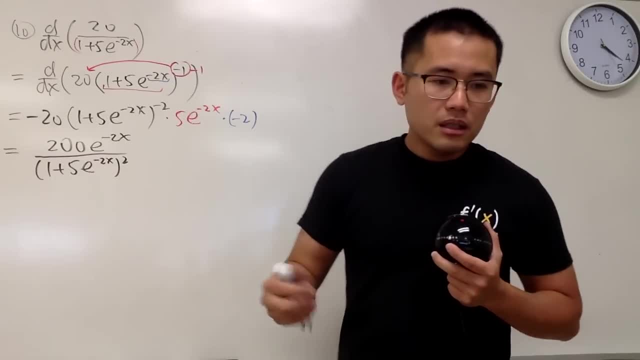 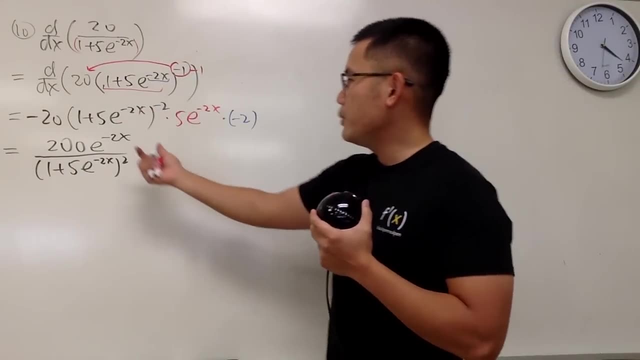 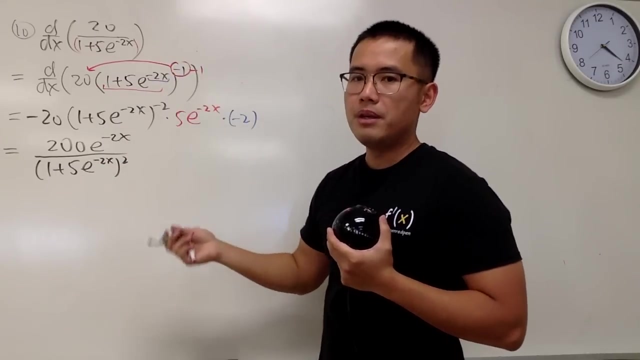 This negative 2 is the second power, like that, And that's the answer choice right here, And I just stop it right here. Sometimes maybe we will write this down here, But it depends. I think this is more clear. I'm using this method, or maybe using the quotient rule. 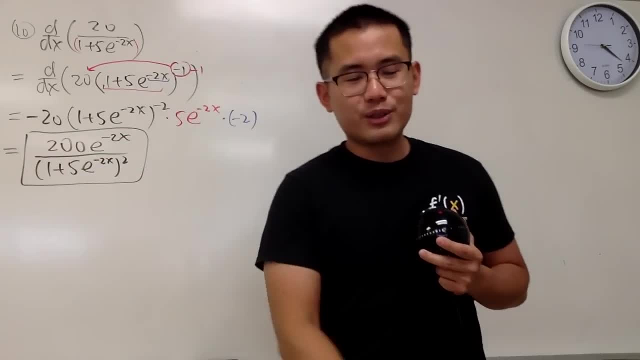 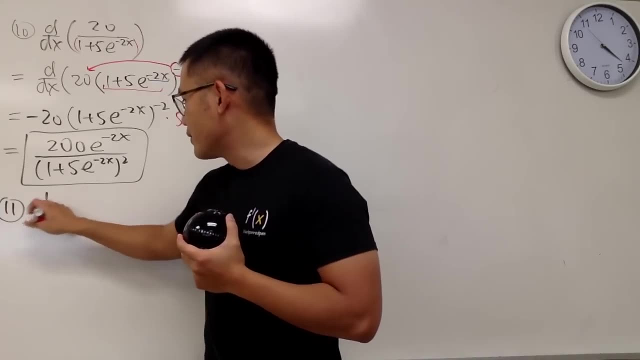 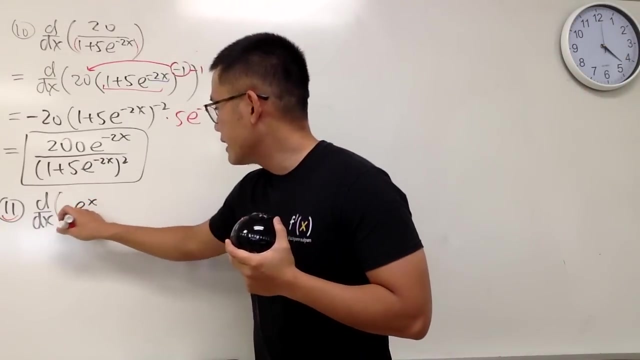 But, as I said, whenever you have a multiple choice question, of course we choose the best answer. So that will be it. Now, number 11, we have to differentiate Here. we have e to the x in the square root, And then for the second one. 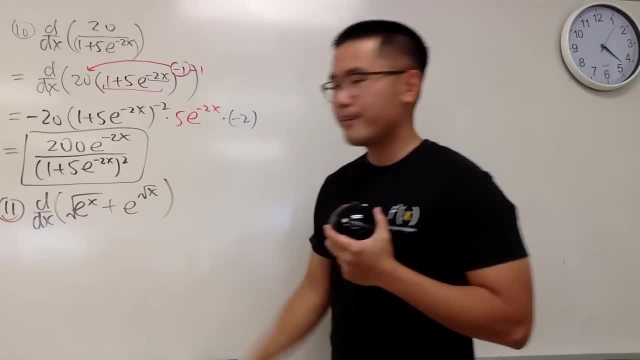 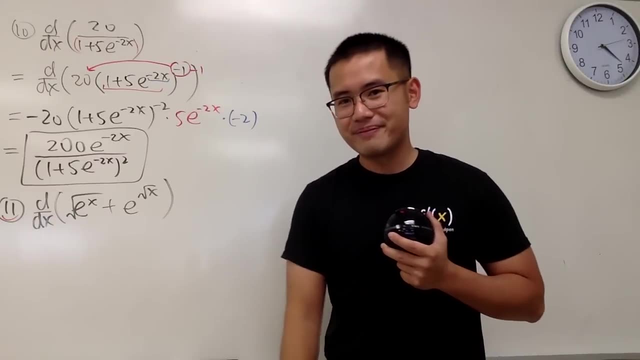 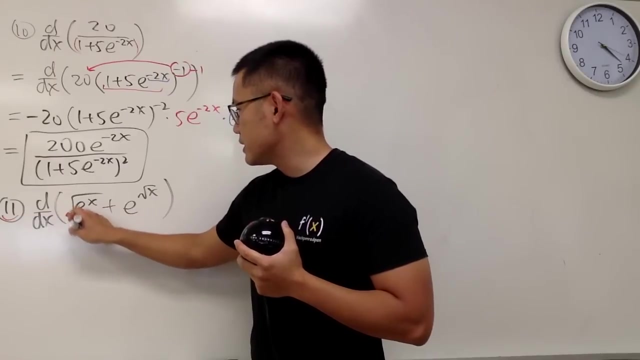 we have to add e to the square root of x. We are not using the product rule right here. This is just a teaching. So we differentiate the first and then differentiate the second. Well, check this out Whenever we have square roots in calculus. 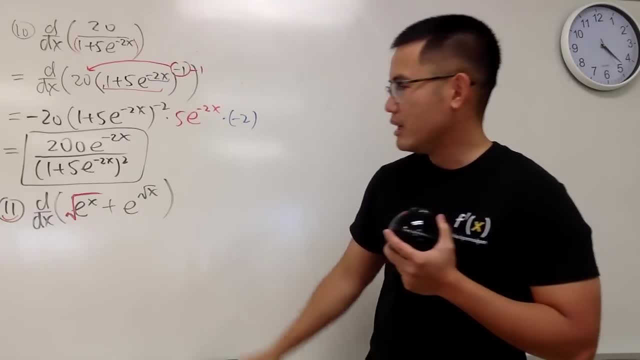 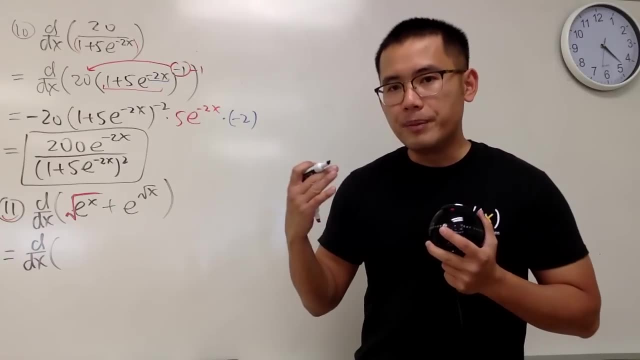 we almost always look at square roots as 1 half power. So in fact, for the first one, we can look at this And we're just doing algebra. So the idea is that we should be doing algebra first before we do calculus. 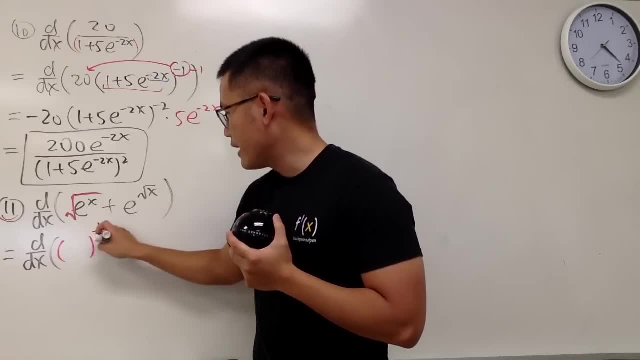 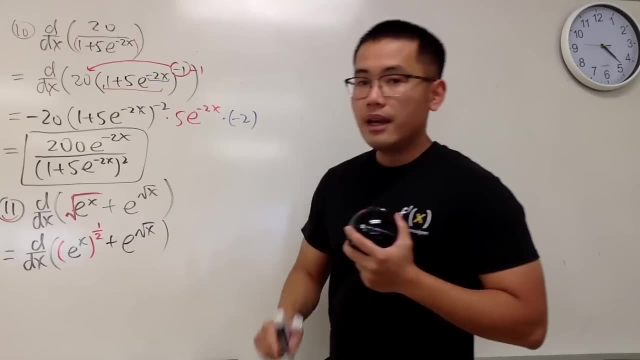 So if you look at this part- we just look at this to the 1 half power and this is e to the x. inside This part states how it is, And the reason I want to point this out is because this right here we can just do x times 1 half. 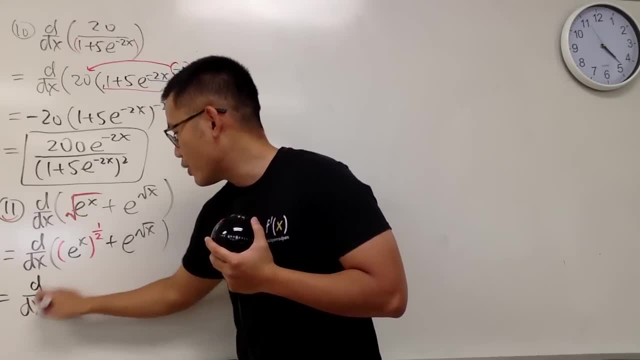 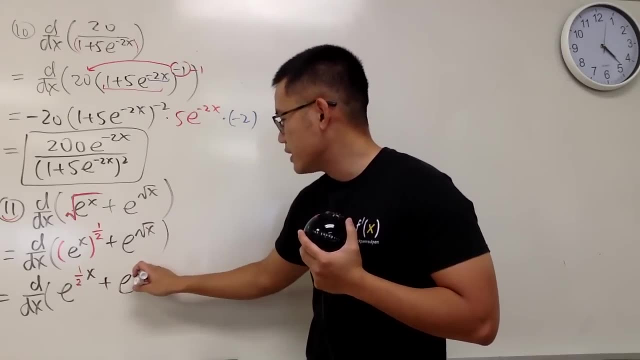 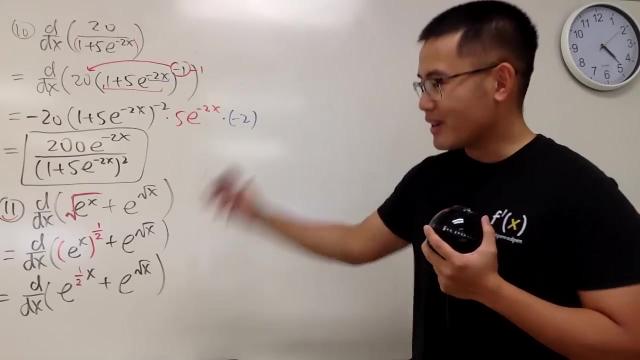 and we can rewrite this as to take the derivative of e to the 1 half x plus e to the square root of x. like that, Do algebra first before you do calculus, And then right here we can just do the calculus. 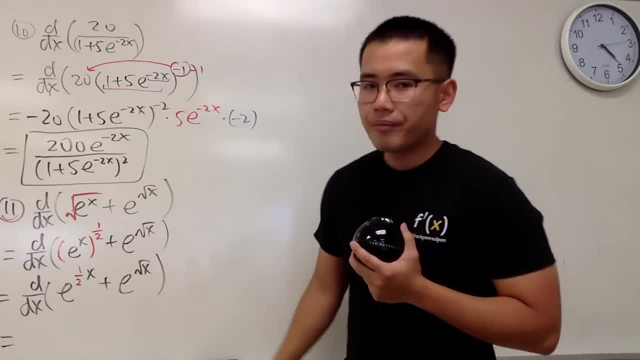 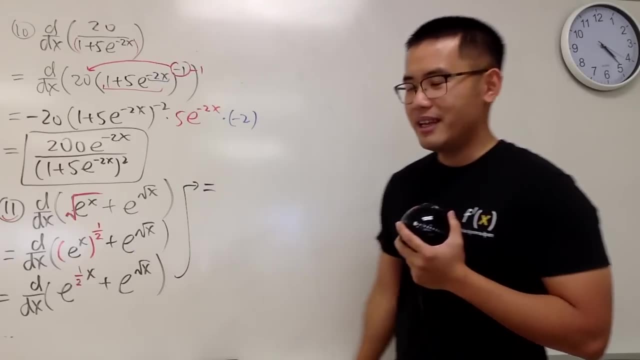 Okay, here we go. Let me actually just probably put it here like that: This is not integration, so this is just an arrow, right? Anyway, here we go, Differentiating e to the something we first. just repeat the whole thing. 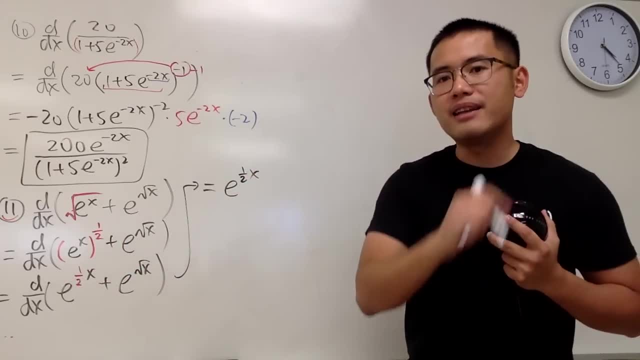 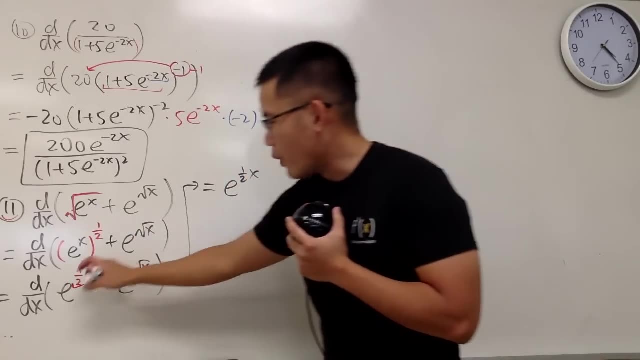 namely e to the 1 half x. And then we do the Chengdu. Look at the exponent right here and ask yourself what's the derivative of 1 half x? And the answer to that is just 1 half Good. 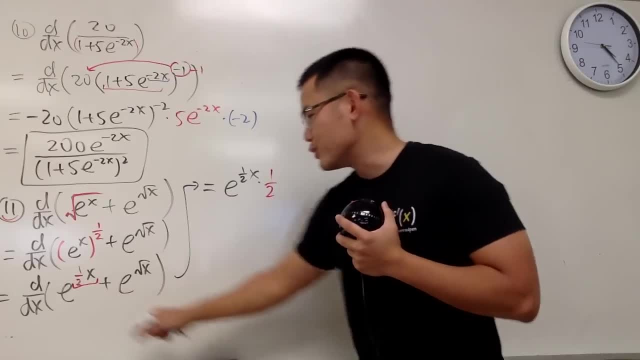 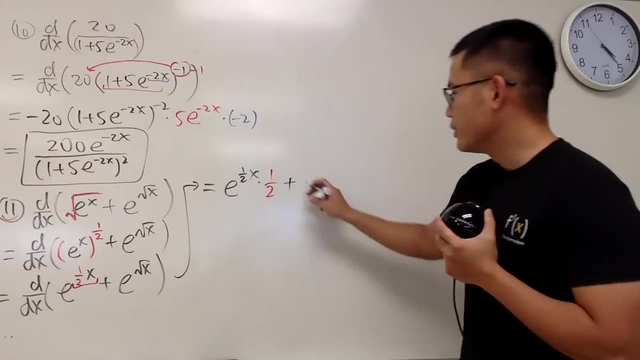 Now we do the second part And notice again, we're just adding. so we just have to add the result for the second. We are not doing. the product rule right. The derivative of e to the square root of x. 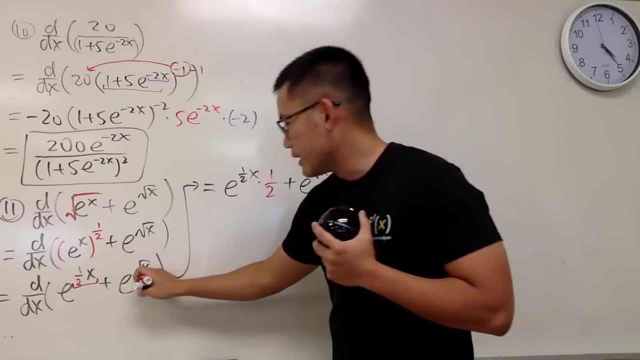 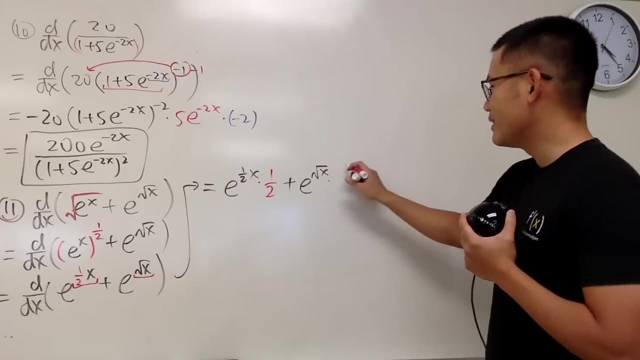 we can just first repeat that And then again I look at this right here and ask myself: what's the derivative of square root of x? We talked about this earlier, so that's why I didn't, you know, write that as the 1 half power. 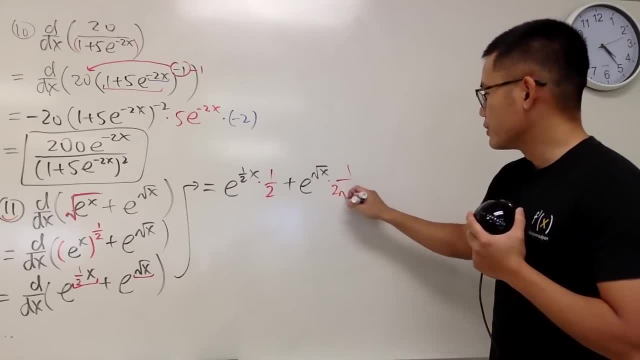 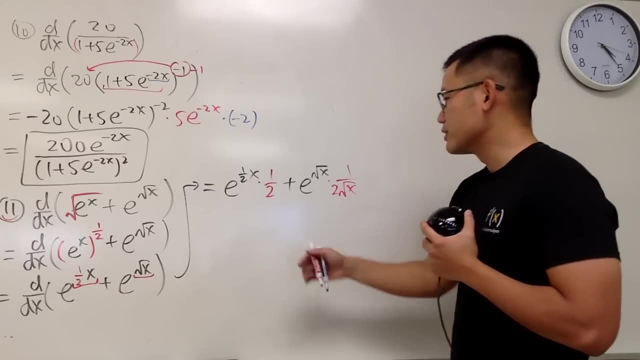 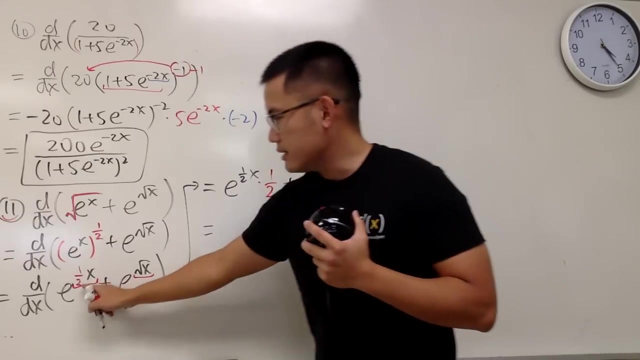 Derivative of square root of x is just 1 over 2 square root of x, like that, And that's pretty much it In the end. perhaps we'll just write this down nicely. Check this out: e to the 1 half x. this part is this: 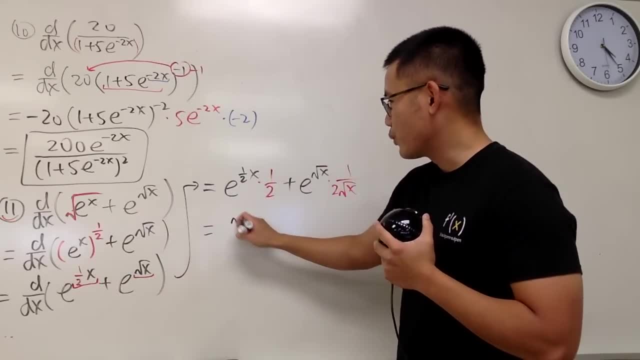 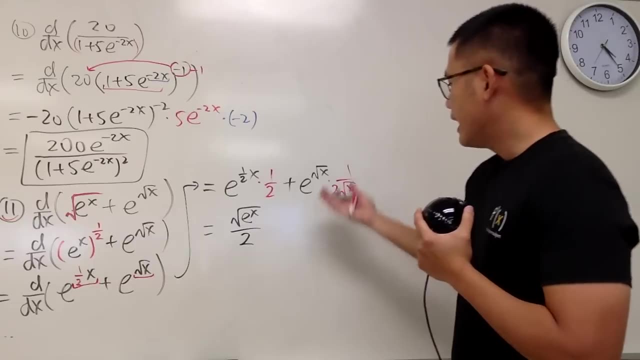 which is that. which is that. So this part is just the square root of e to the x inside over 2.. So I'll put down the over 2 right here And then for this part, I can just put this on the top. 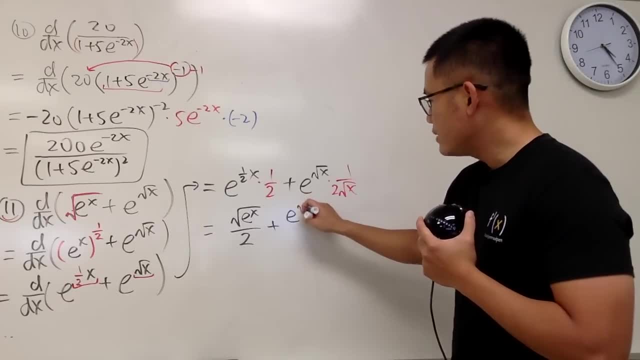 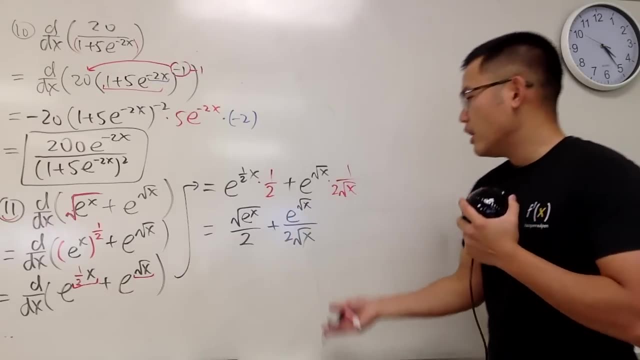 this times 1.. So we put down plus e raised to the square root of x, power divided by 2 square root of x, like this: Of course you might want to get the common denominator if you want, and all that, but 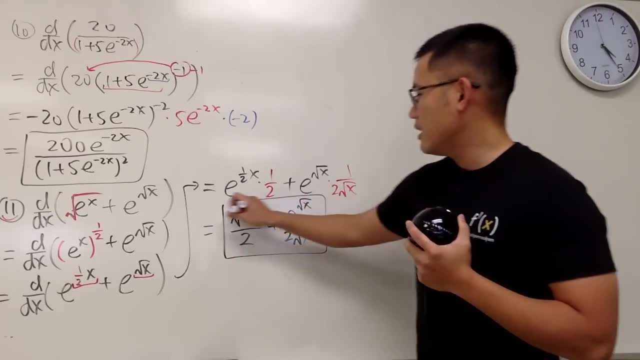 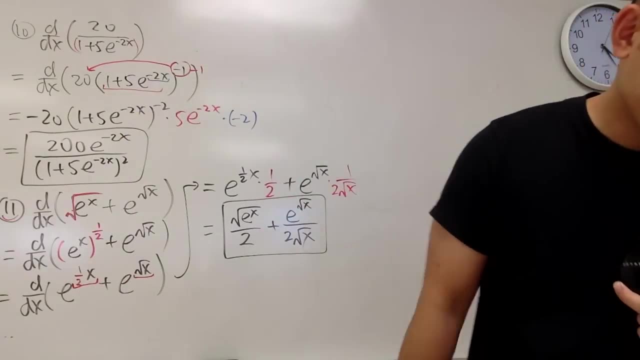 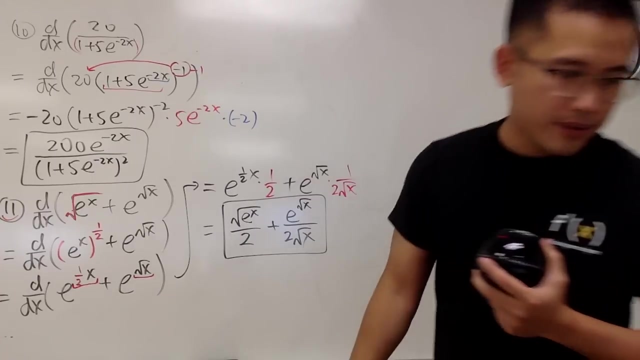 again. I left the answer like this in the answer choice. so that's it for the question. So that's yeah. Okay, now number 12.. What do I need to do? Oh, this is a good one, number 12.. 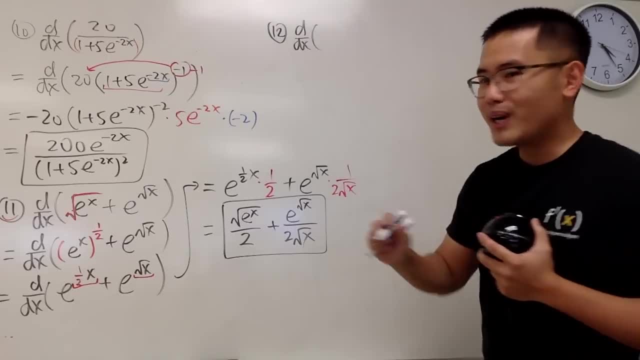 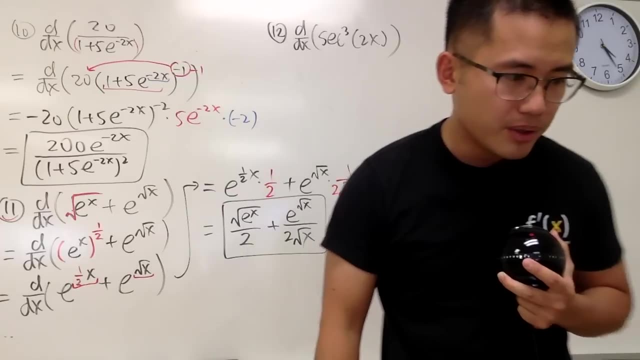 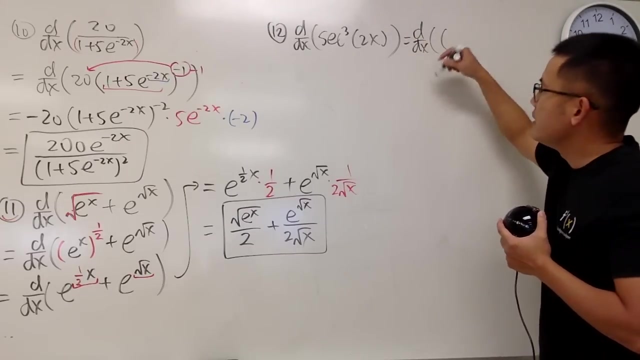 Differentiating. Here we are going to differentiate: secant to the third power of 2x. Secant to the third power of 2x. Well, it's a good idea to look at this as to take the derivative of parentheses. 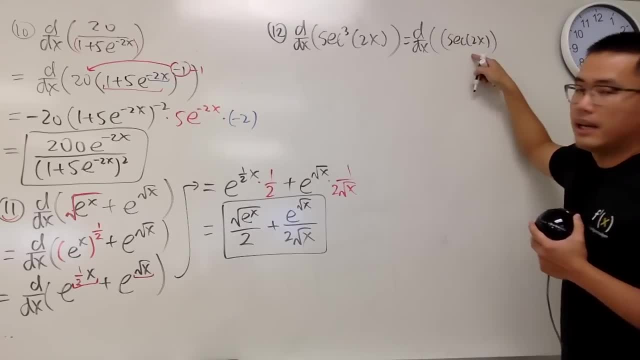 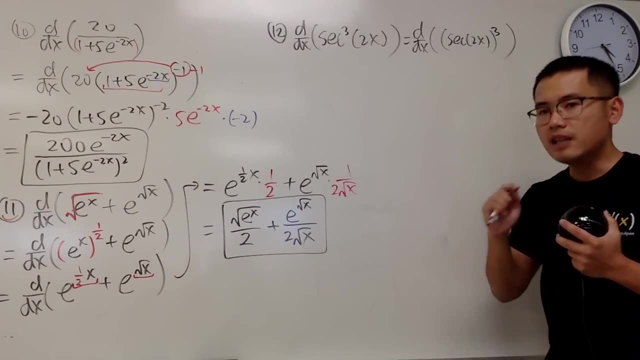 secant of 2x inside, like this: and then to the third power. Especially if this is the first time that we are doing derivatives, it's always a good idea to put the power right here, And don't forget to use the big parentheses. 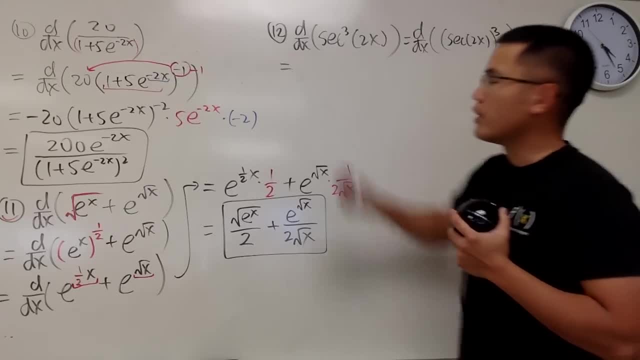 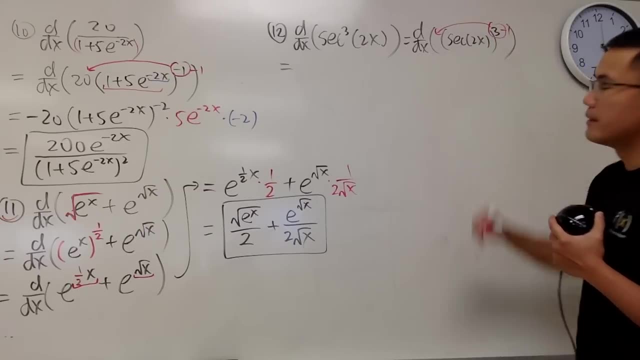 to group the expressions. All right, here we go. We have to look at this- to the third power, so we can just put down the power to the front and then minus 1.. So the first part, we have 3, and then we have this right here. 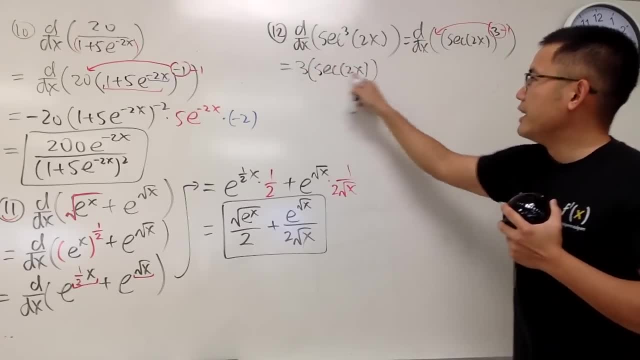 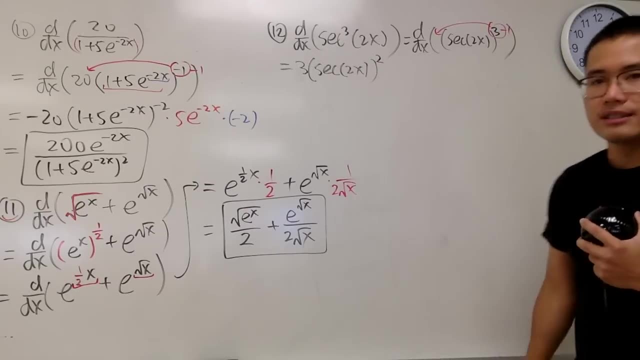 which is parentheses secant of 2x. The inside states the same for now right. It states the same right here: And 3 minus 1 is 2.. That's a new power And we do the Chandu. 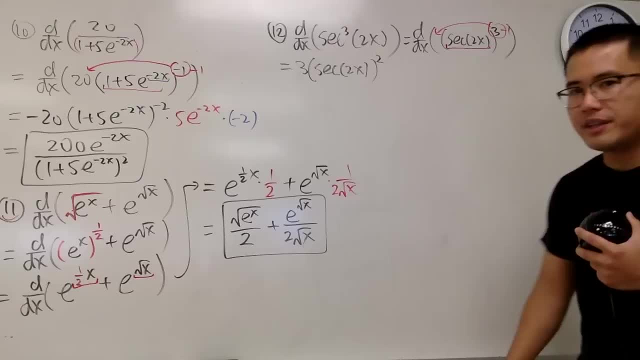 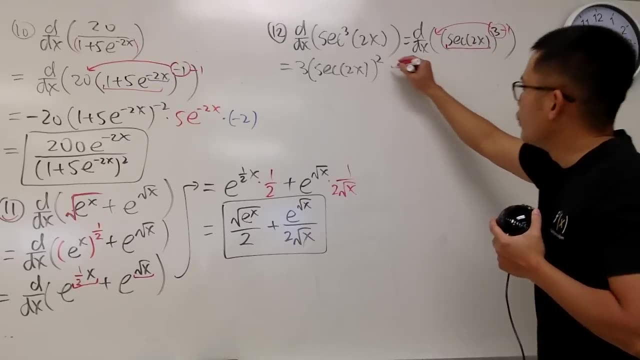 Look at the inside. This is the time that we have to do the derivative inside. Derivative secant is secant of the inside times, tangent of the inside right, So we will have secant of 2x. again, the inside states the same. 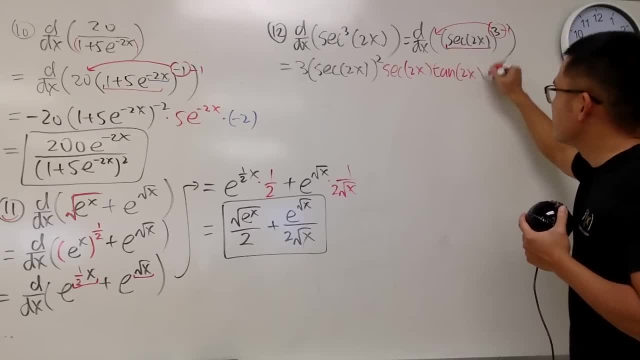 And we also have to have the tangent of 2x, like this: But what's the inside of the inside? It was a 2x, isn't it? Well, we have to do the Chandu again. What's the derivative of 2x? 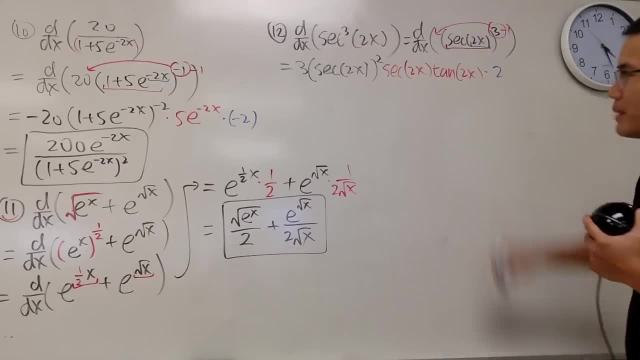 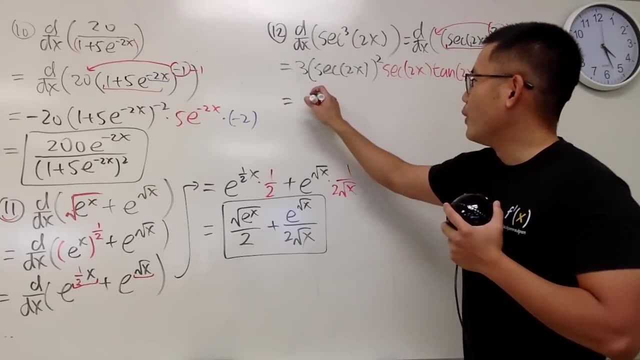 Just a 2.. Very nice, Multiply by 2.- Now we'll just put everything together- 3 times 2 is of course 6.. So altogether we have 6.. Here we have 6.. And check this out. 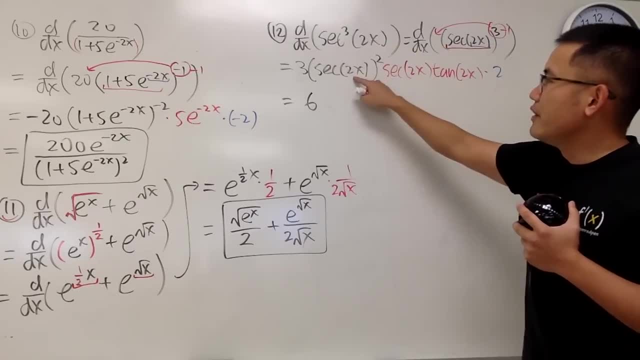 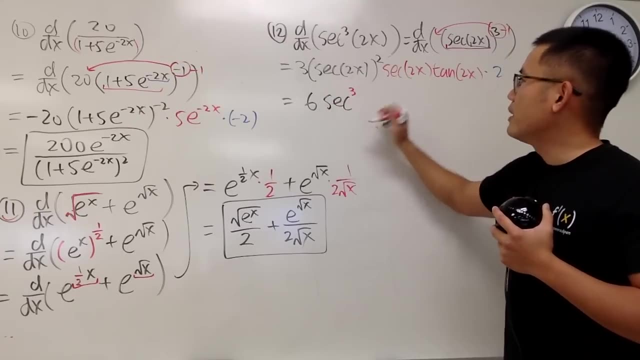 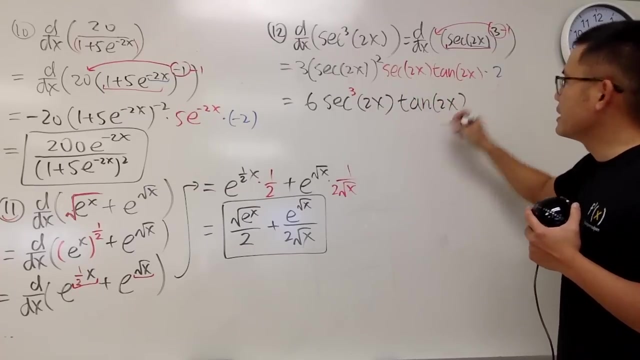 This is secant to the second power and secant to the first power. They have the same input. right This times that together we can write it as secant to the third power and the input stays the same, And we multiply that with tangent of 2x. 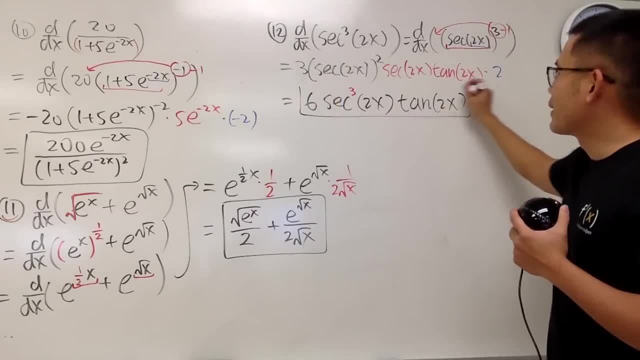 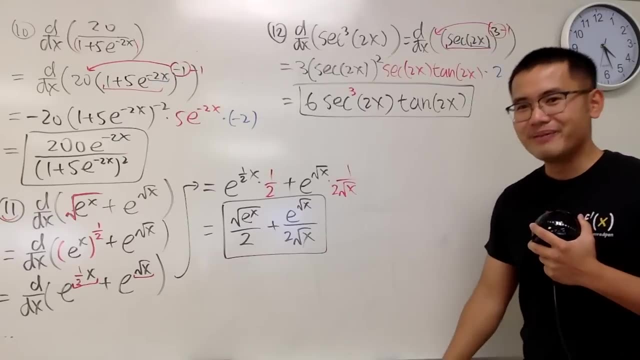 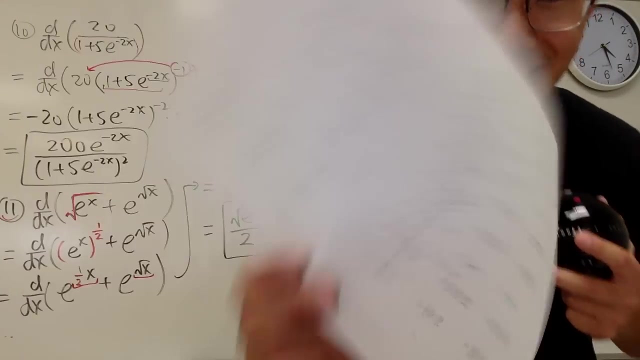 Just like this. So this right here is the answer. Second power: power. together we have the third power and we put the power right there for the final answer. Just like that. Okay, Number 13.. It's one of my favorite ones. 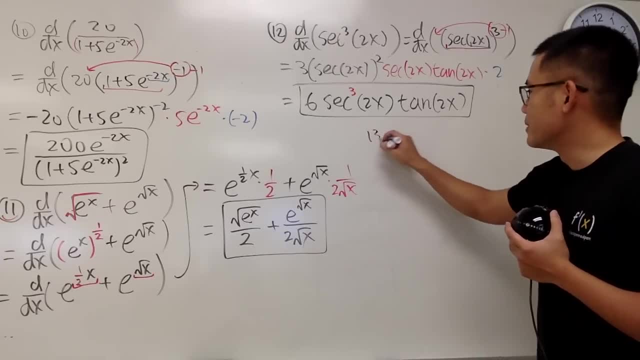 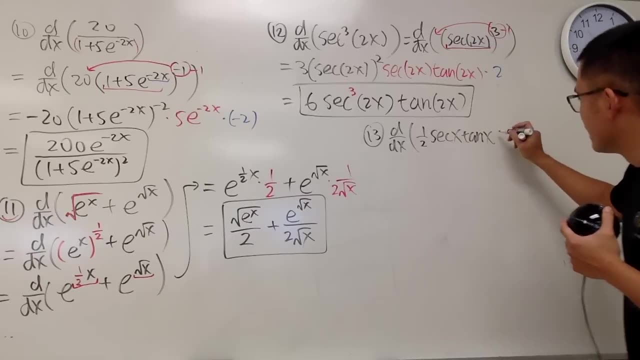 You'll see why. So number 13,, number 13,, number 13.. We will be differentiating 1 half secant x, tangent x plus, and this is the first time that we have the natural log. So I'll talk about the natural log function. 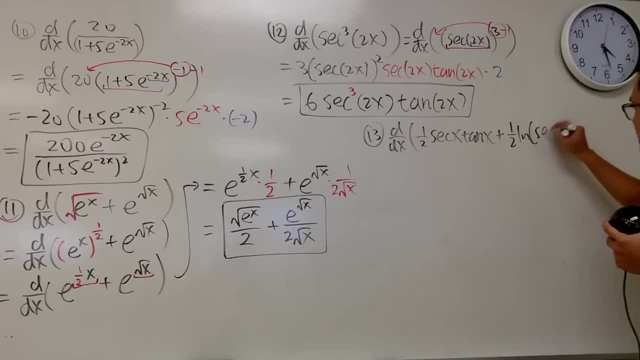 1 half natural log of secant x plus tangent x, like this. So parentheses and another parentheses for that. Alright, Here we go. There's nothing that we can do to rewrite, Unfortunately. yeah, this is instead of the natural law. 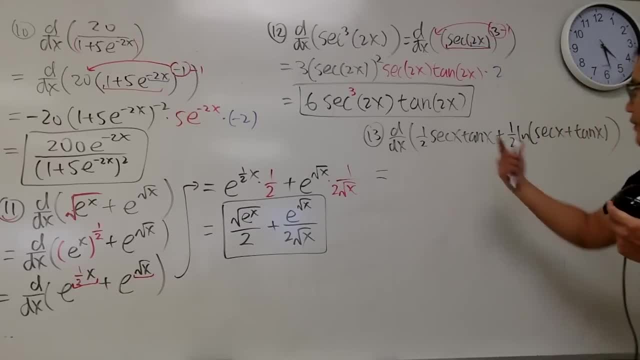 so we have to just deal with these two parts individually. For the first part, we have to use the product rule, because the first function times the second function. So let's get this part done first. Well, product rule in action. We have to keep the first function. 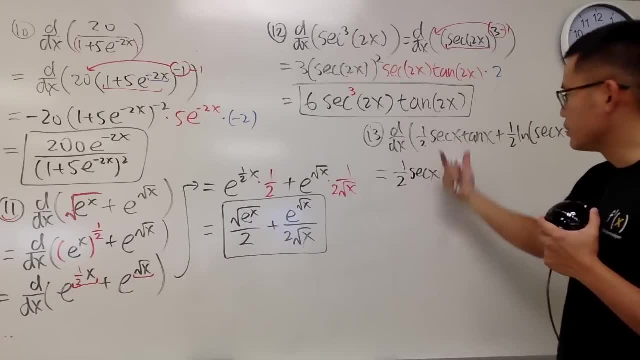 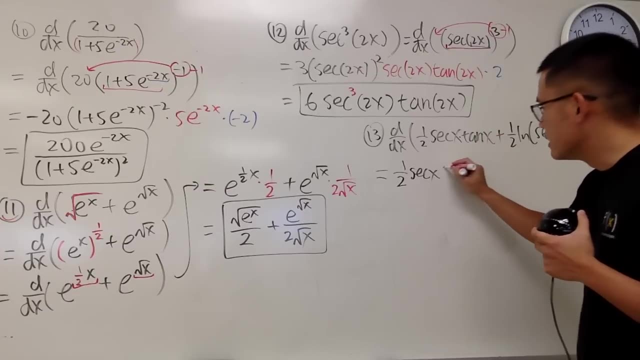 which is 1 half, and we have secant x. This is just the first function times. the derivative of the second, The derivative of second derivative of tangent x, is secant square x. And again, you have to know your derivative 3D really well. 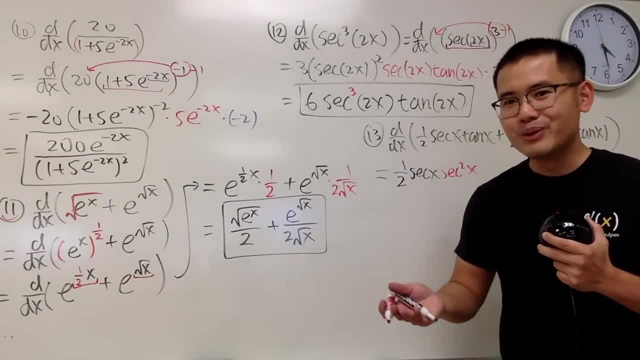 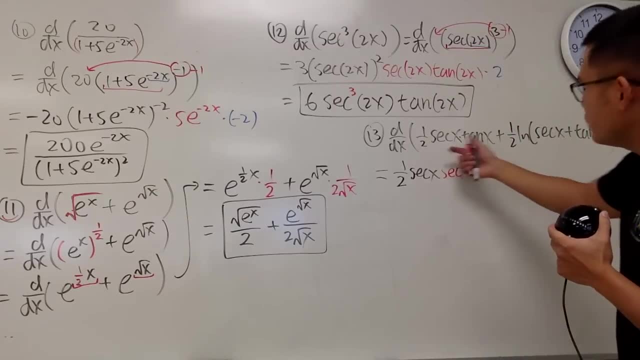 for all these kind of questions And later on in Cal 2, maybe when you're doing integrations in Calc 1, you have to know the derivatives backwards. Anyway, first, one times the derivative of second, plus the second function which is tangent. 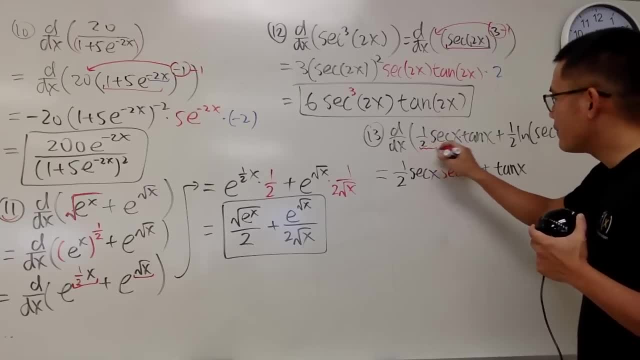 times the derivative of the first And notice I have the 1 half secant x as my first function, so I need to have the 1 half. Whenever we have a constant multiple, just go ahead and put it down And then you focus on differentiating. 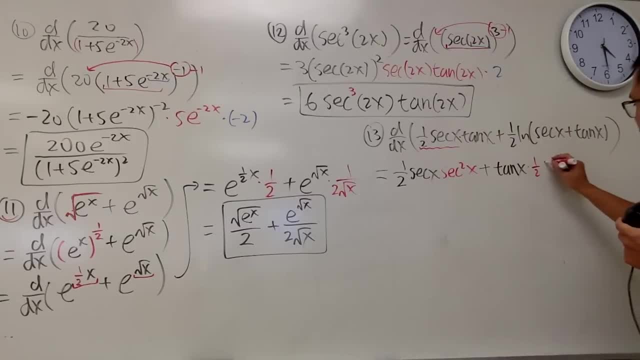 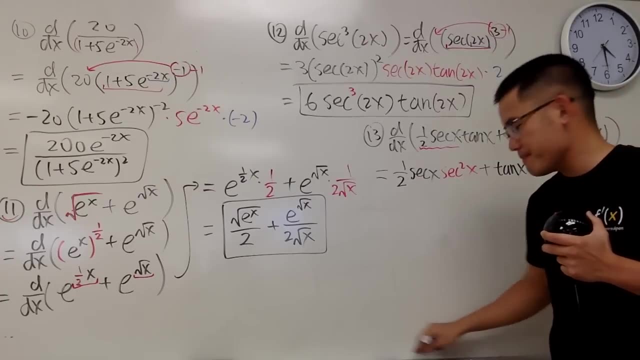 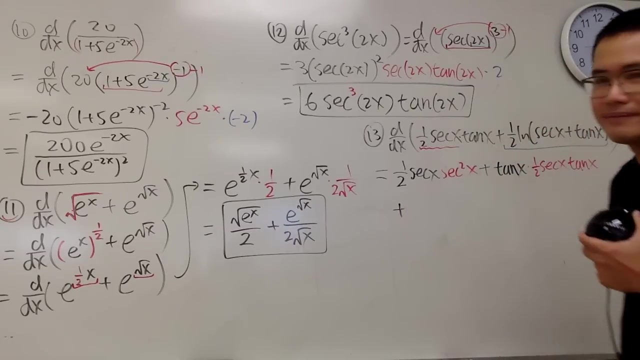 the secant x, which will give us secant x times tangent x. So this, right here, is the first part. Okay, Now I will do the second part. right here in blue. We will have to add: well, again, 1 half times this thing. 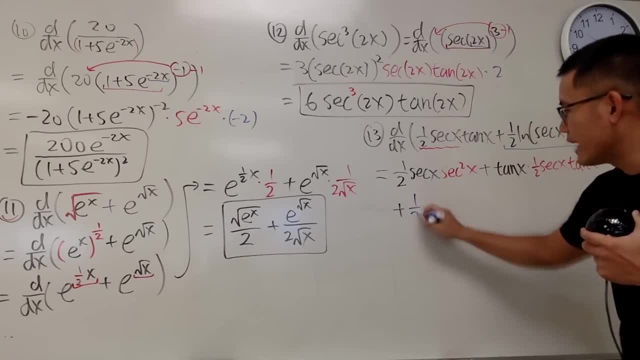 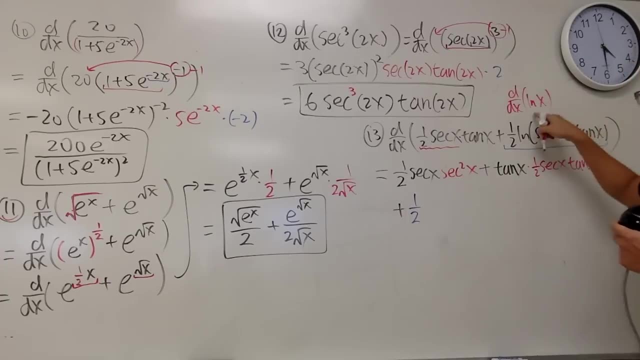 so we will have to just maintain the 1 half as 1 half, And this right here as a reminder: whenever we differentiate natural log of x, natural log of the inside, we just get 1 over the inside, like this: 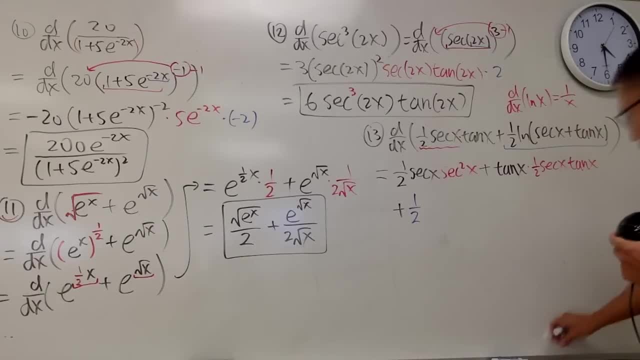 And, of course, we will have to use the chain rule, right? Okay, so we have the natural log of this, so we do 1 over this thing, which is secant x plus tangent x. Well, well, chain rule, right here. 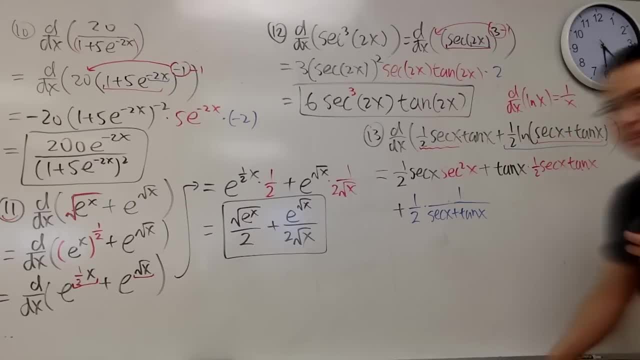 isn't it? We have to multiply by the derivative of the inside right. Okay, this right here is a plus, so you just do the derivative of the first and you add the derivative of the second. You have two things, so be sure you put the parentheses. 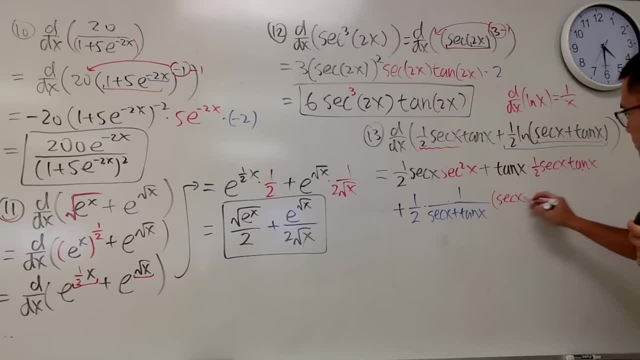 The derivative of the first is secant x times tangent x. The derivative of secant x is this: And then you just need to add the derivative of secant x. sorry, the derivative of tangent x is secant square x, like this: 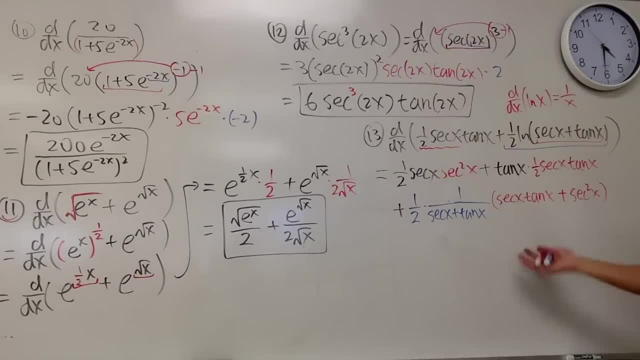 Wow, such a long expression, isn't it? So again, the derivative of secant x is that we add it with the derivative of tangent x, is that? So this is what we have, But do not leave this as the answer. 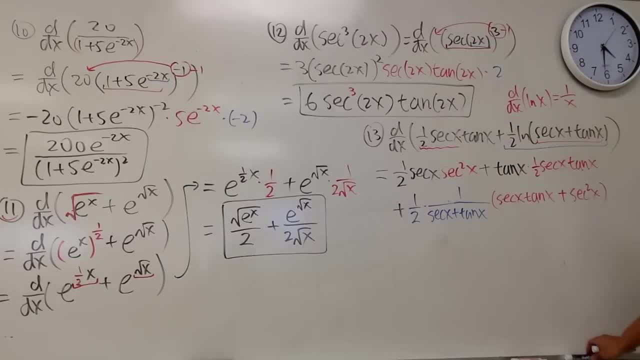 because we can do better than this. Check this out to see what we can do. Hmm, this is kind of weird. I'll show you. Check this out. Here we have secant, secant square, so we can factor our secant. 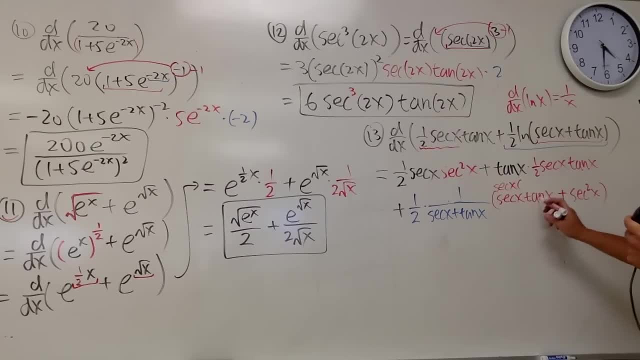 isn't it? So we can factor our secant x And then we will have tangent x plus secant x. right, We can factor it out. Hey, look at that. Here we have secant x plus tangent x. Here we have. 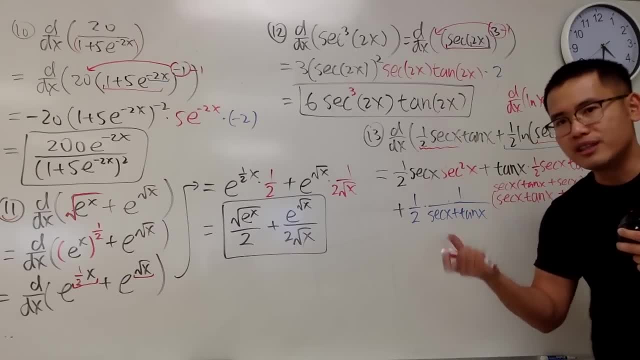 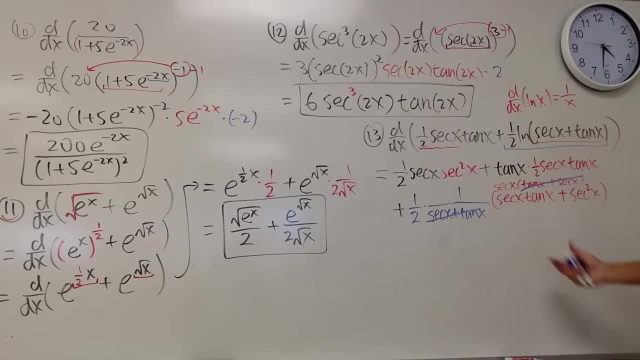 tangent x plus secant x And of course the order of addition doesn't matter. Therefore we can legitimately cancel this and that out. So for the second part, we actually just end up with one-half secant x for the derivative. 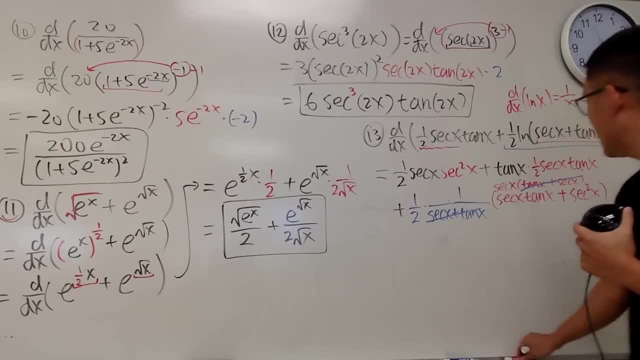 That's very nice, And perhaps let's look at this first part as well. Hmm, we have okay for this part. we will just write this down in blue. okay, I will just put this down right here. We add: 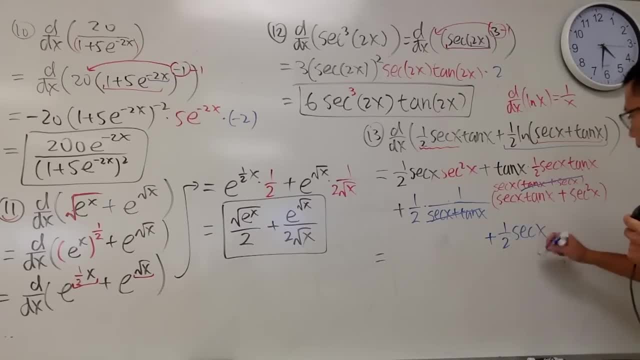 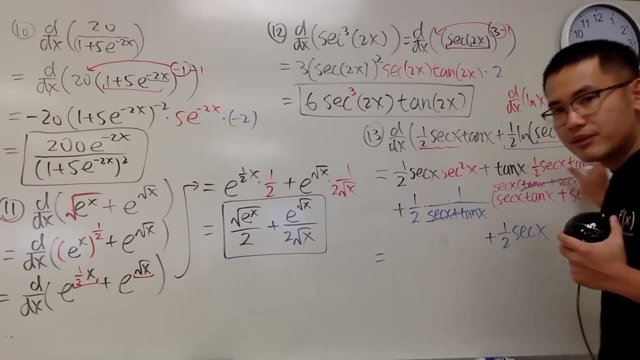 one-half secant, x Again. that's just the first, that's just the second part, And now we still have to take care of this part. We just have to take. we still have to take care of this part, And. 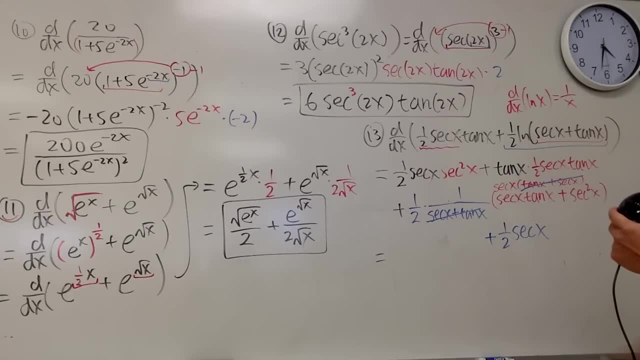 it seems like we can also factor things out, huh, Because this right here has one-half x. well, one-half secant x, and this is also one-half secant x. So let's factor it out and see what happens: One-half. 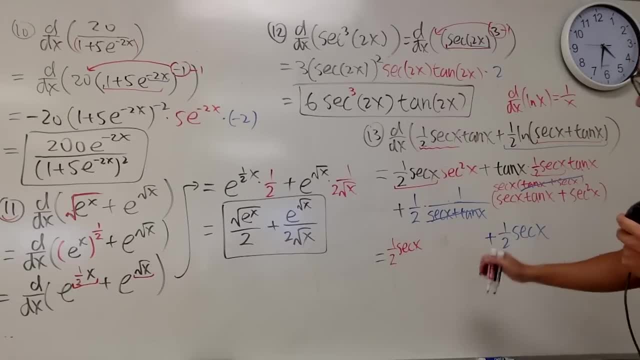 secant x, right? In fact we can also factor this out, but let's do that later because it's kind of slightly too confusing. a little bit Left over here we have secant squared x plus left over tangent, tangent. So we have. 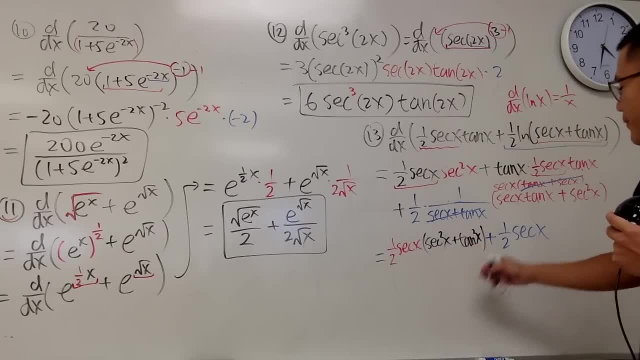 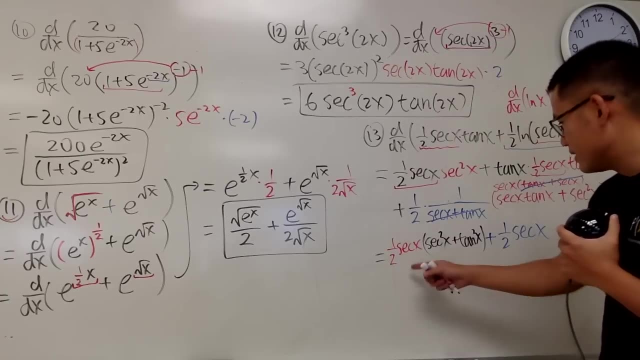 tangent squared x. That's it. okay, So that's pretty much the factorings that we have at the moment, And now, of course, we can factor this out together. So we see this and that can be factored in. 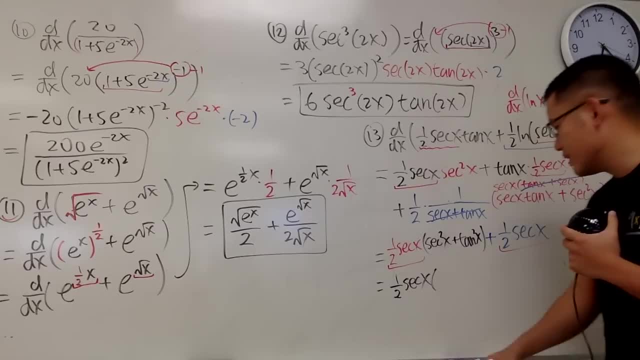 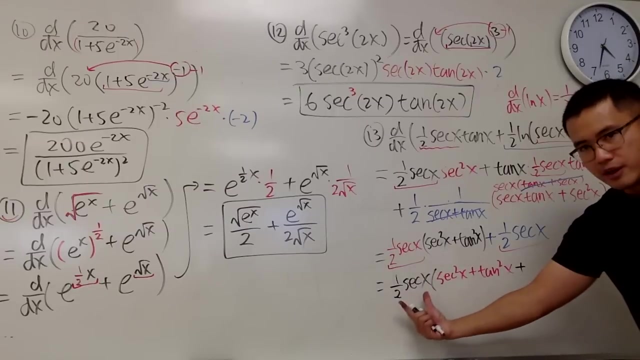 Put it outside right, Put it outside. Multiply with the left over. Here we have secant squared x and this is plus tangent squared x And we have to add. well, we factored this out in the front already. So for this, 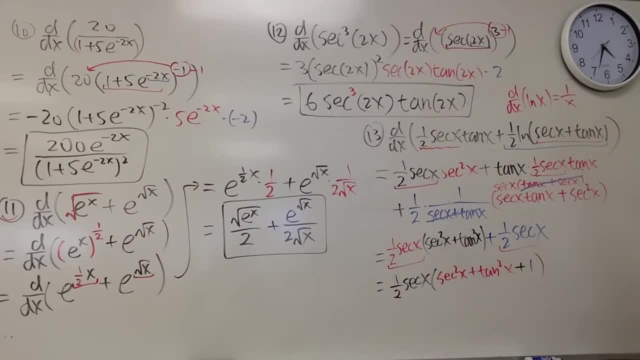 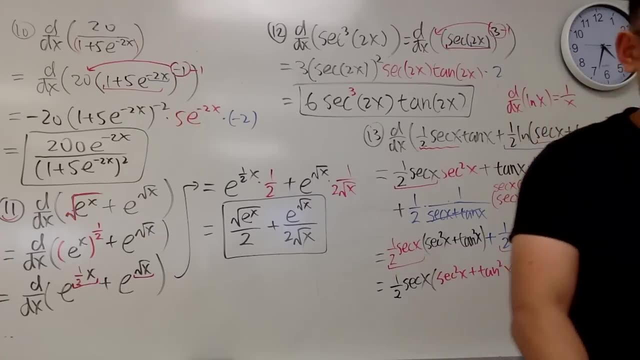 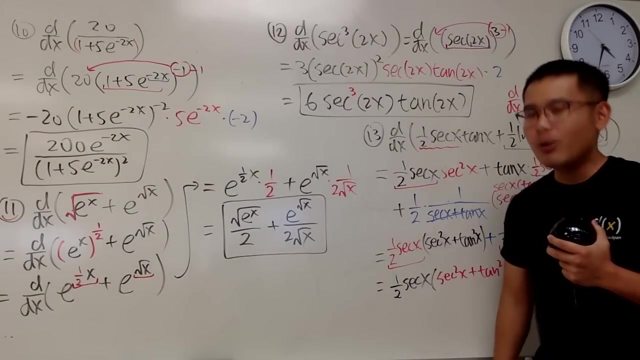 we have a one left, So that's what we have. But now, is there anything else that we can do? In fact, this is not one of the answer in the answer choices. This is the time that we have to know our trig identities. 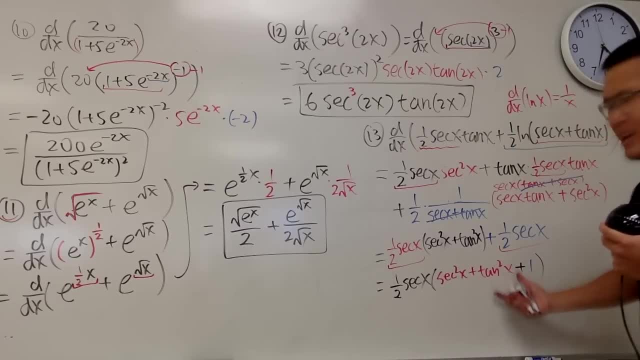 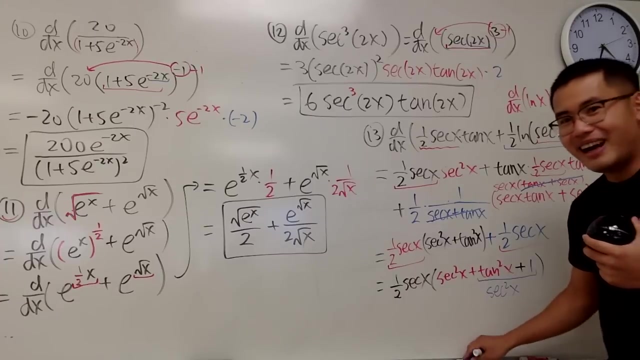 Unfortunately, secant squared x plus tangent squared x, we cannot combine them nicely. But we can actually combine tangent squared x plus one nicely, Because this right here gives us nicely secant squared x as well. I'm serious This add up to be: 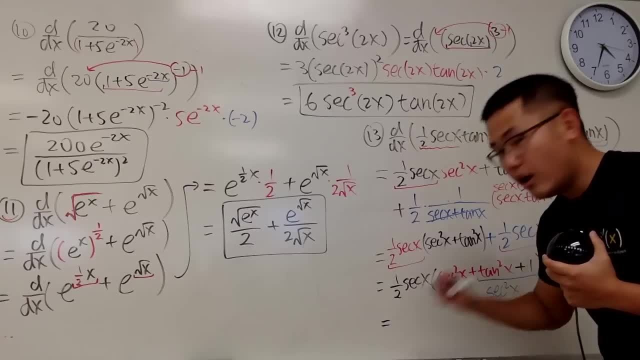 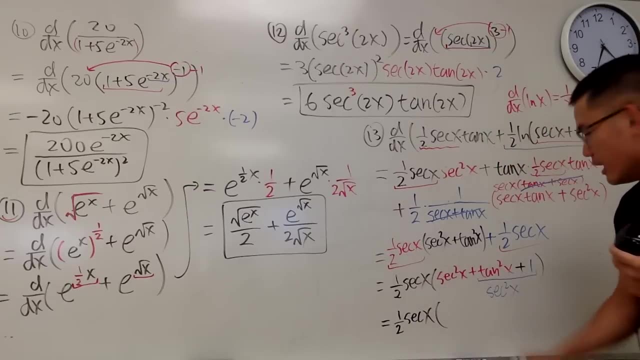 secant squared x. So check this out. All in all, we have one half secant squared. we have one half secant x in the front, all right, And for the inside we have secant squared plus another secant squared. 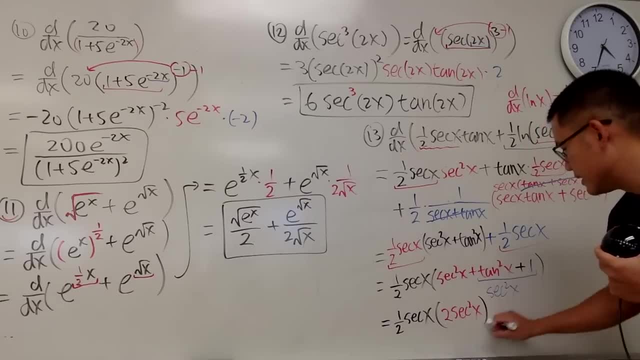 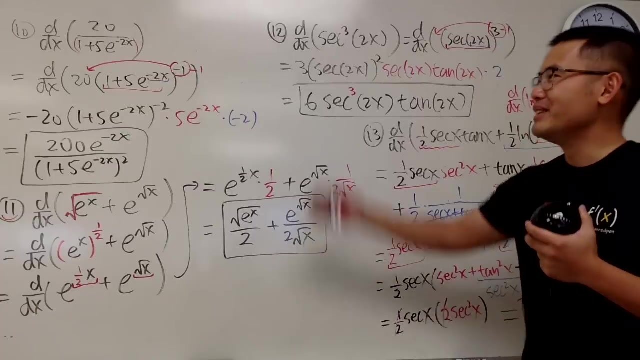 So we have two secant squared x, like that, Again, this plus that. Finally, you see one half times two. Well, of course they cancel. And lastly, we have one half squared squared x plus one squared squared squared. 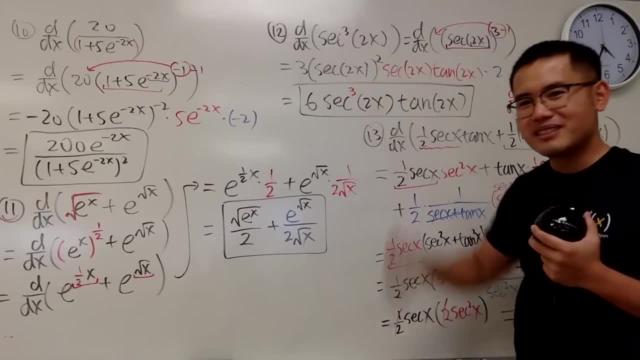 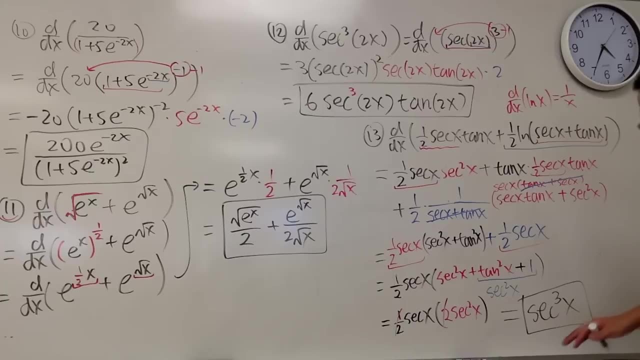 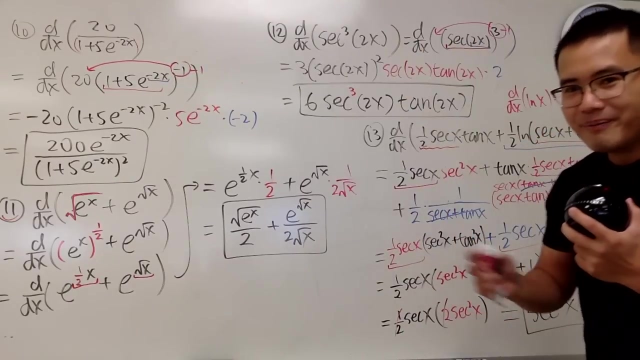 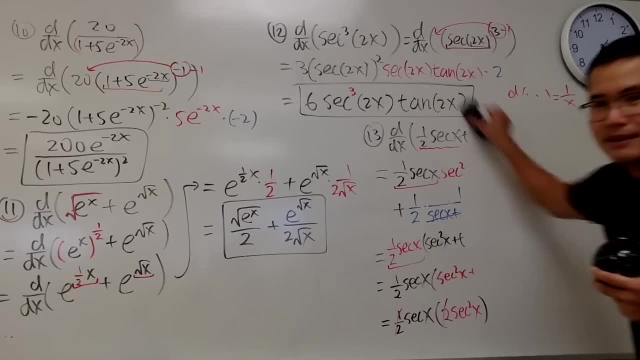 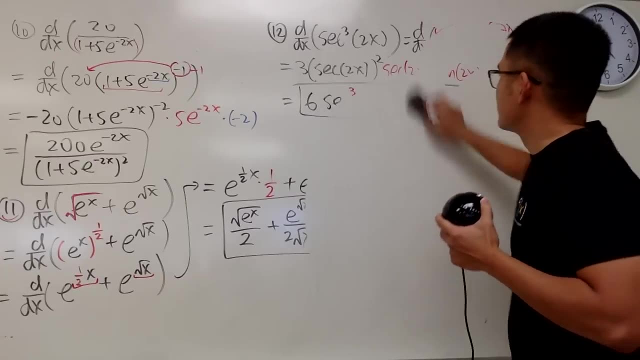 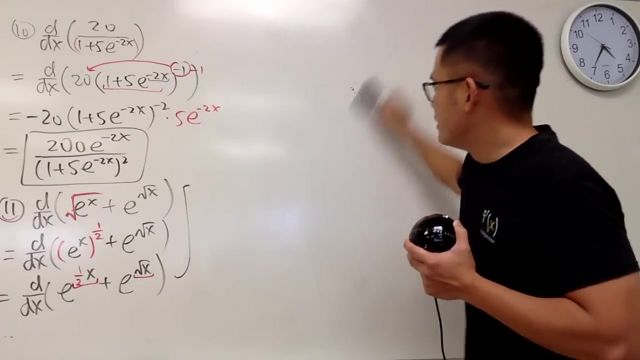 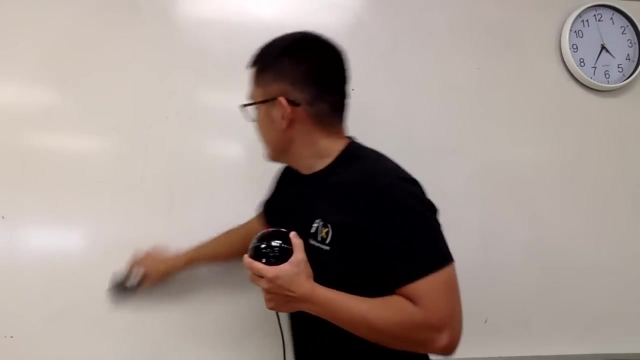 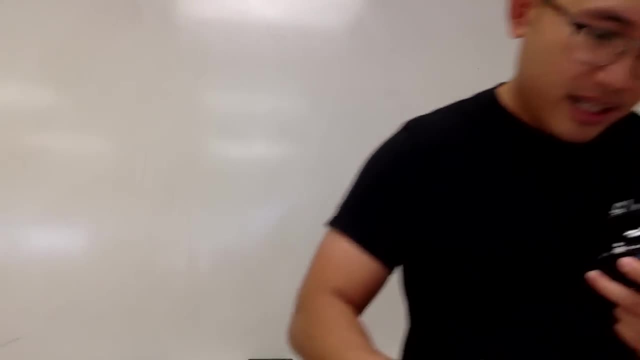 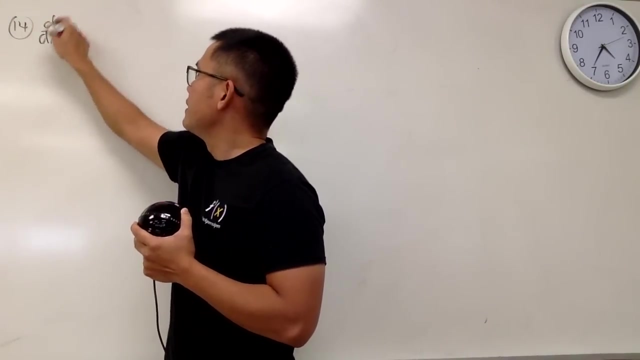 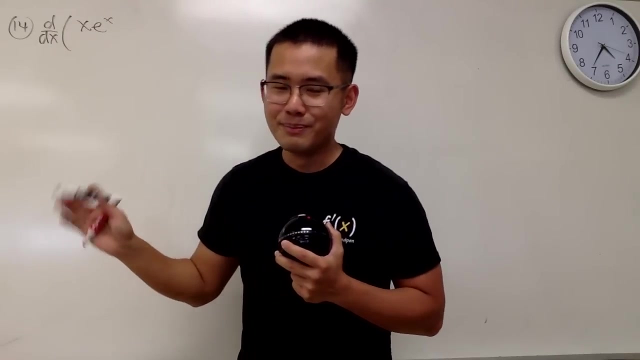 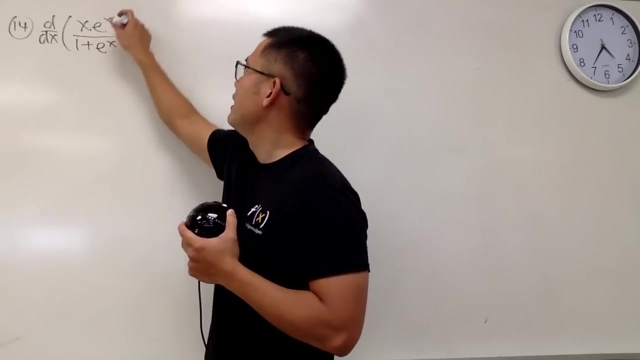 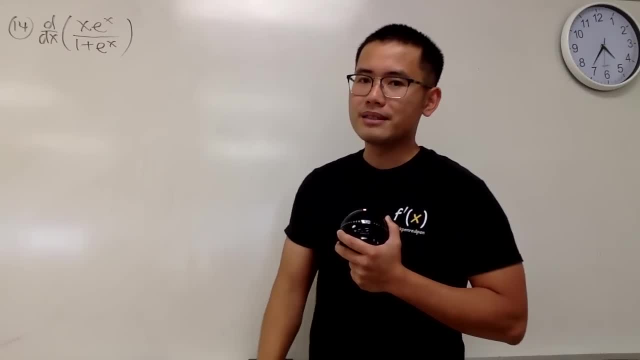 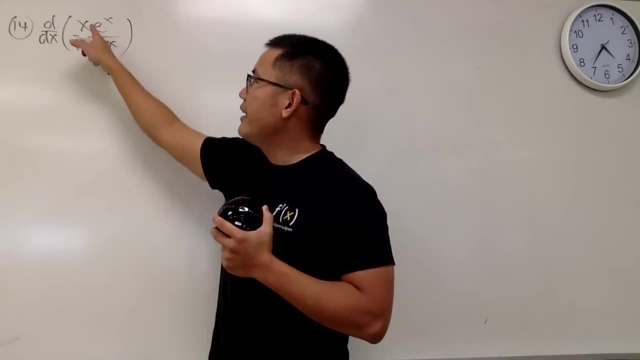 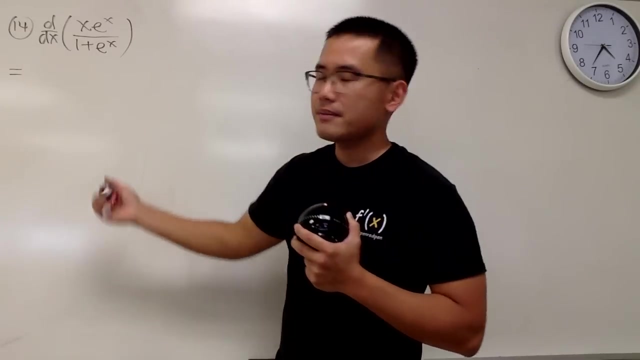 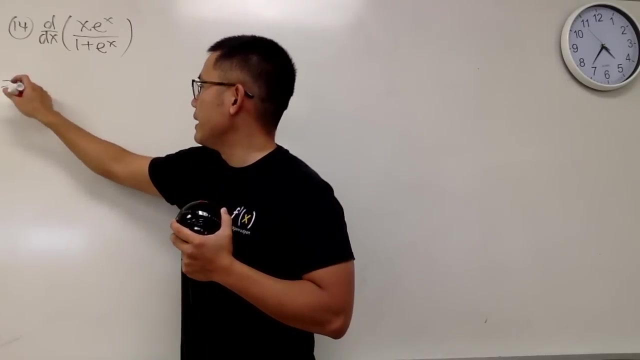 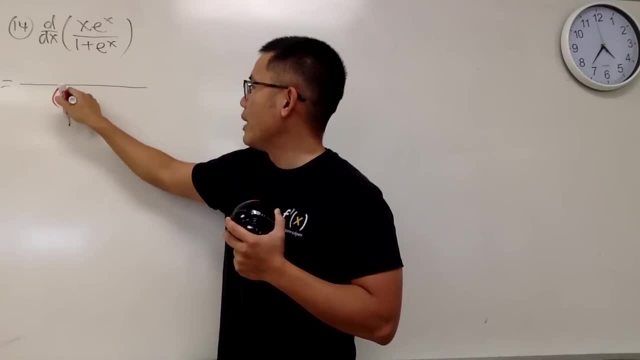 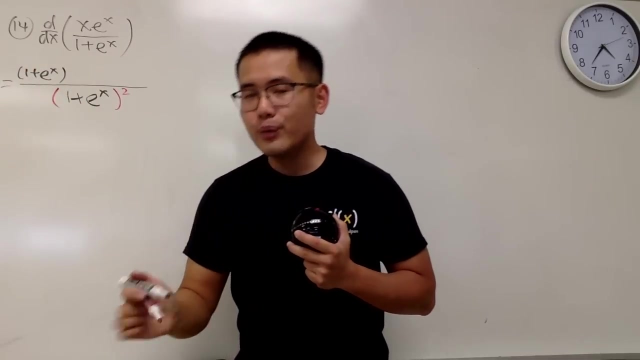 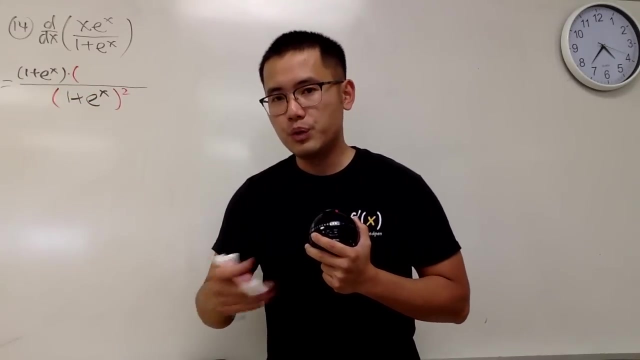 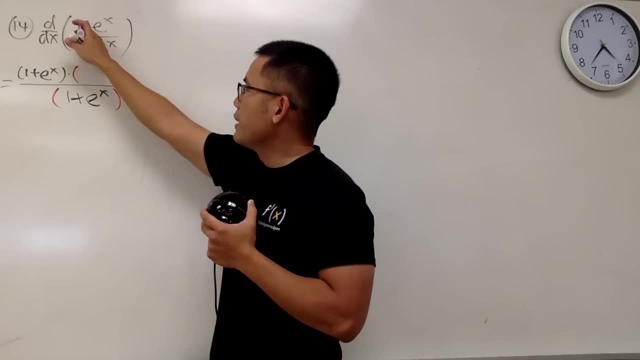 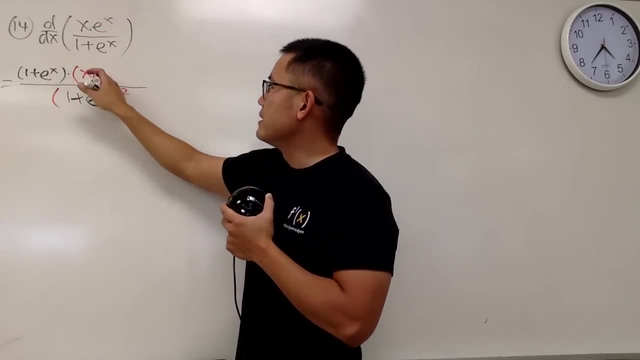 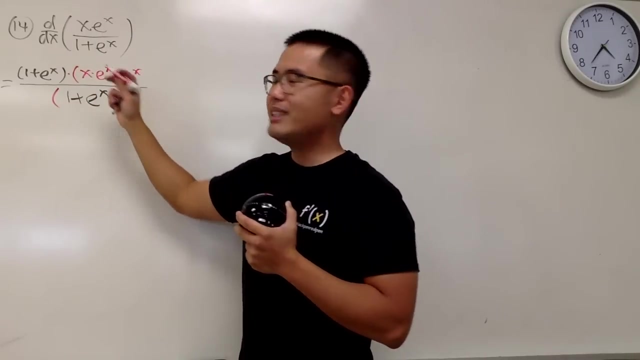 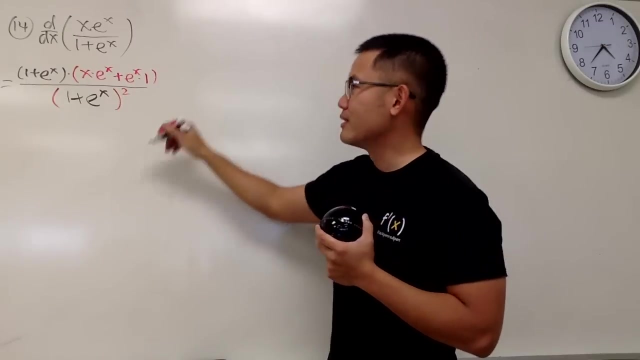 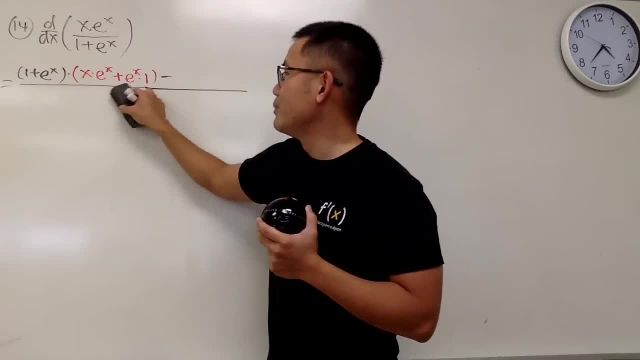 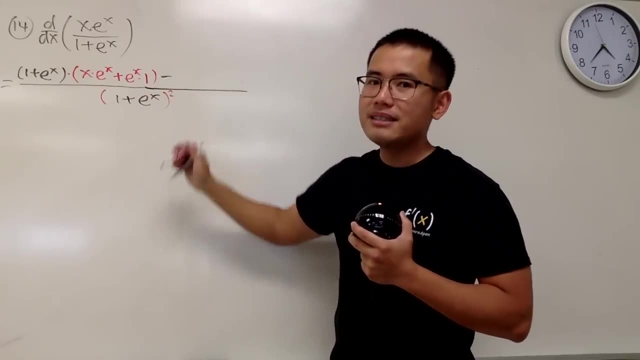 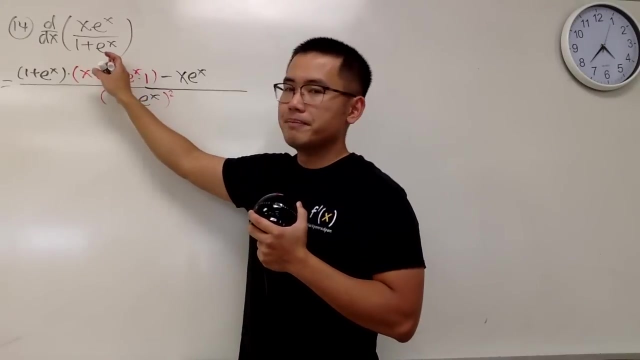 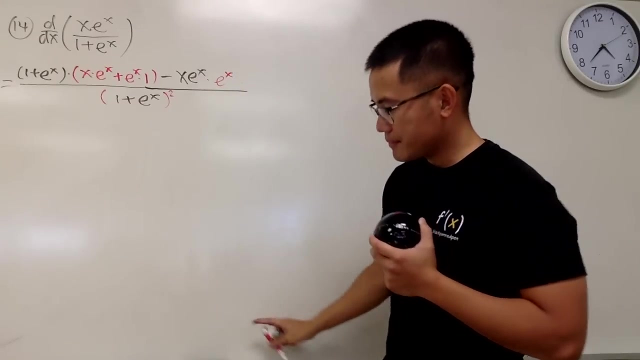 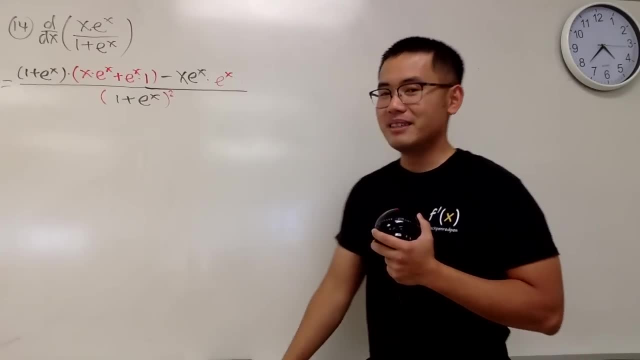 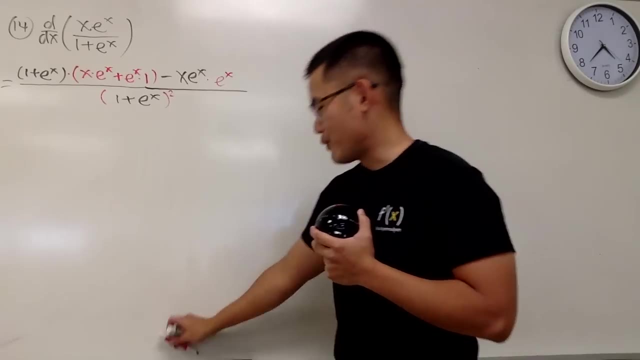 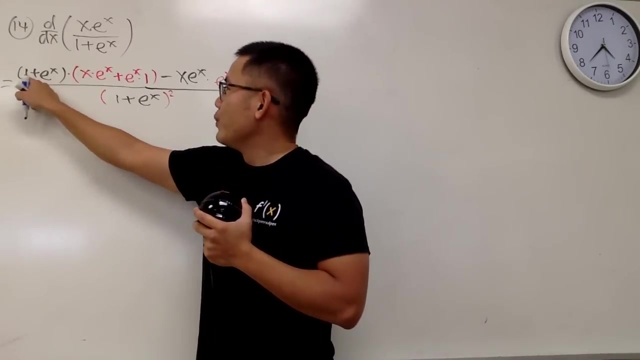 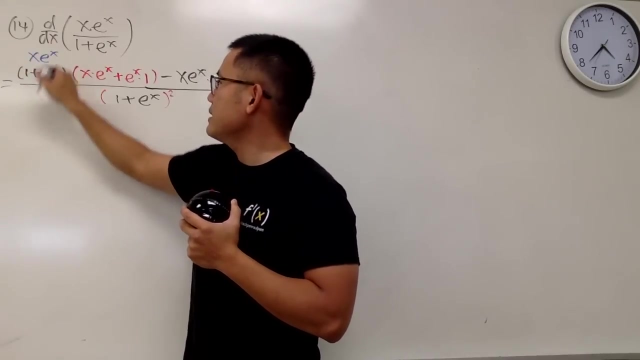 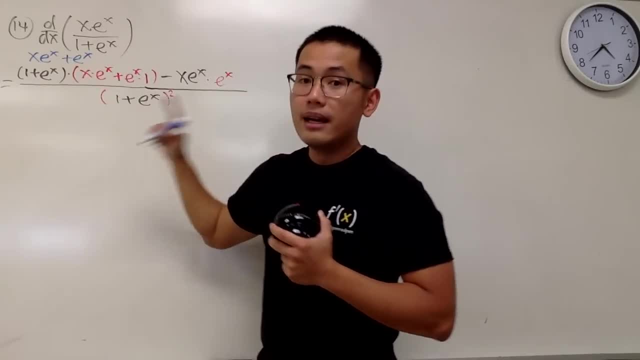 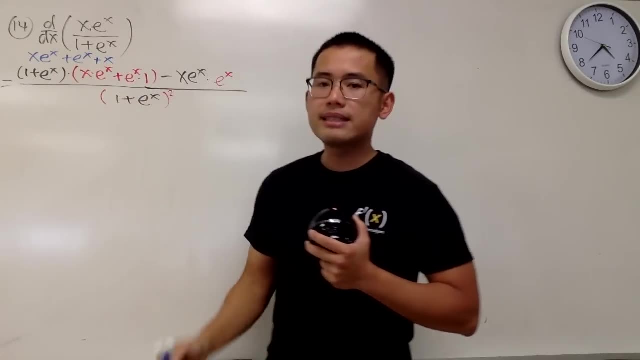 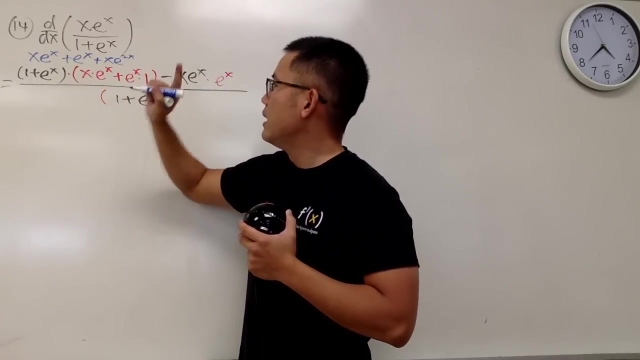 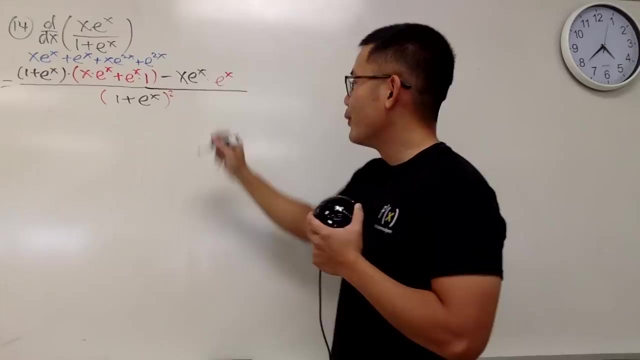 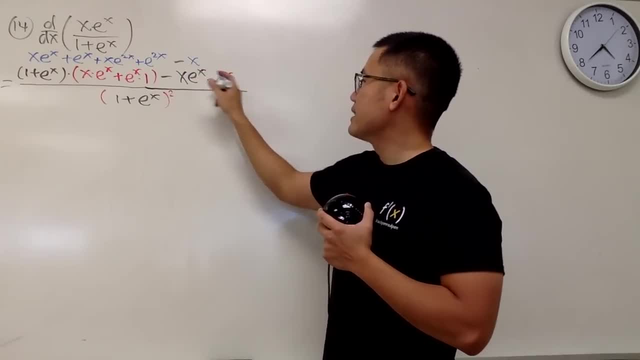 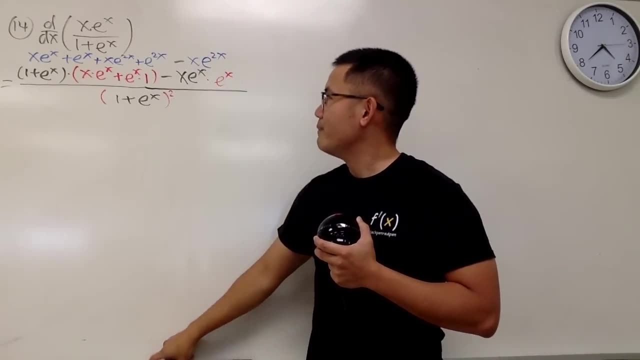 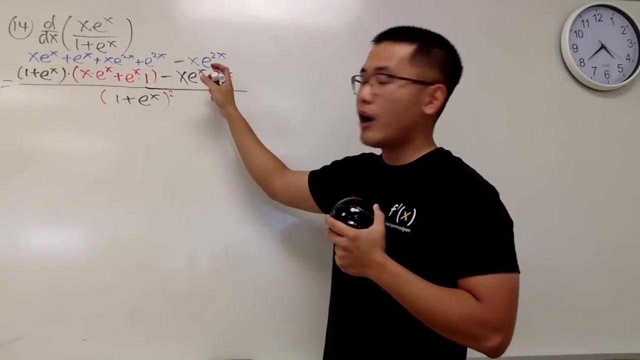 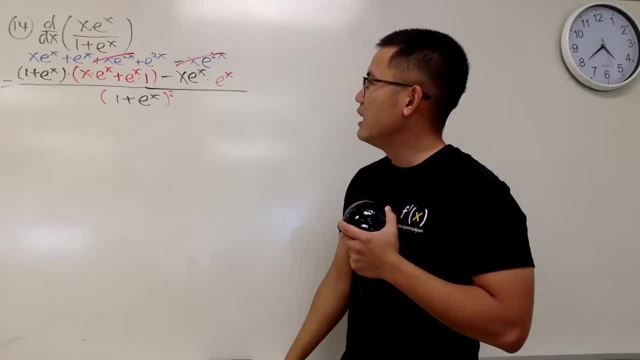 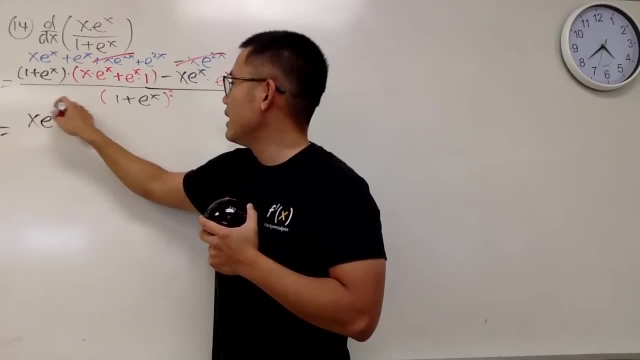 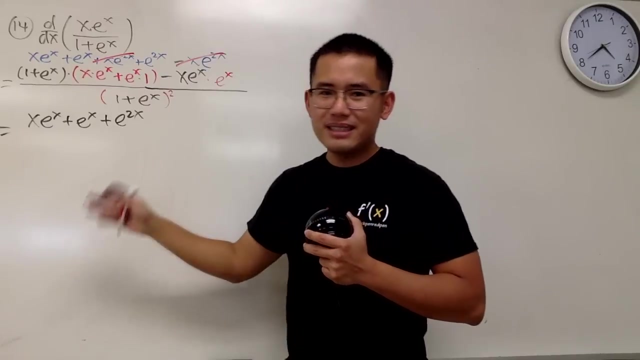 So we can cancel them out, And that's it. So that's pretty much on the top. So in the end we have x e to the x, plus e to the x plus e to the 2x. We can factor things out, but the answer is just in this form, so we'll leave it. 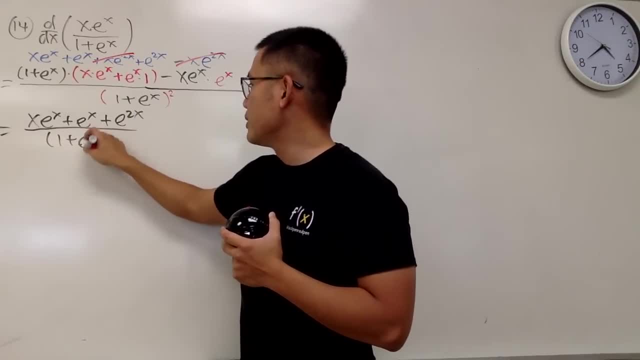 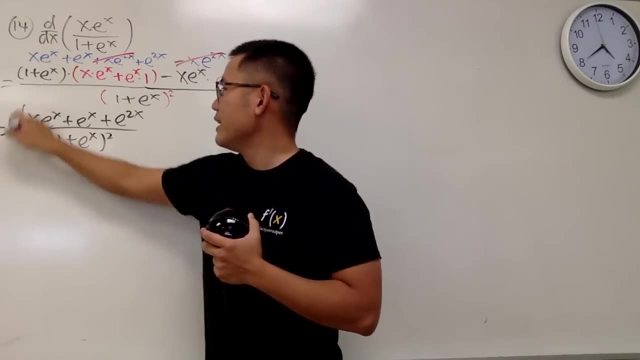 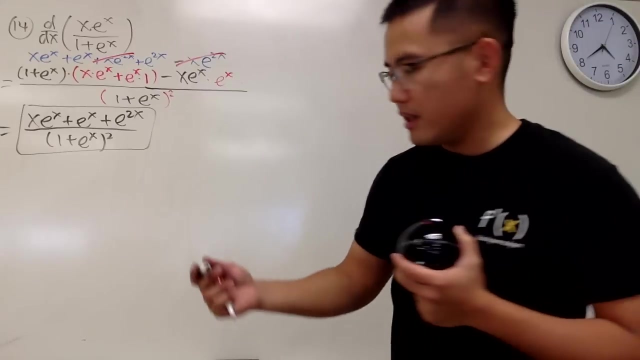 On the bottom, just that. 1 plus e to the 2x, sorry, 1 plus e to the x raised to the second power. Just the bottom, And with that we are done. All right, Number 15.. 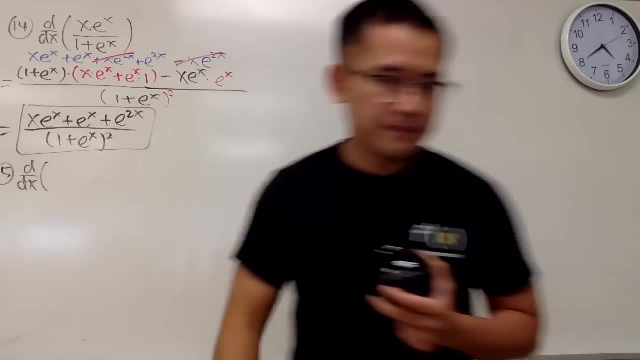 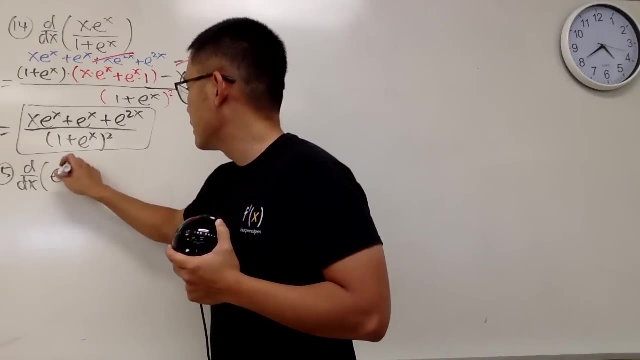 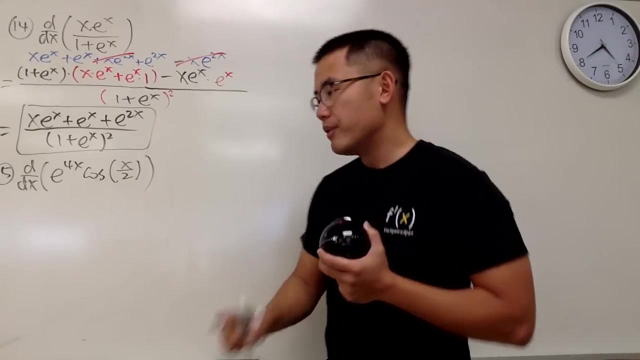 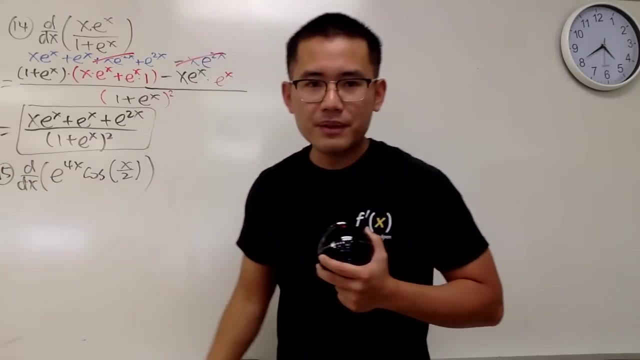 d, dx, We will have to differentiate e to the 4x times cosine of x over 2.. Right, So notice that this is a multiplication. so be sure, we use the product rule, And this is number 15.. Number 15,, you guess? 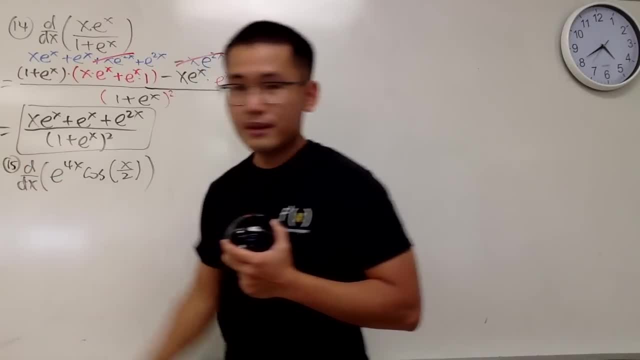 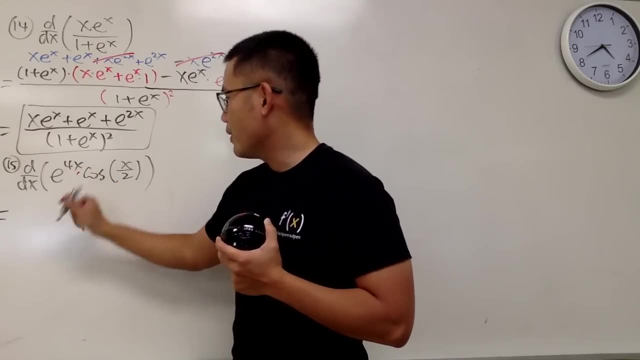 Number 15,, okay, Number 15.. Number 15 is not number 5.. There we go. Okay, Here we go. This is just going to be a product rule example. Well, we of course keep the first function, which is e, to the 4x. 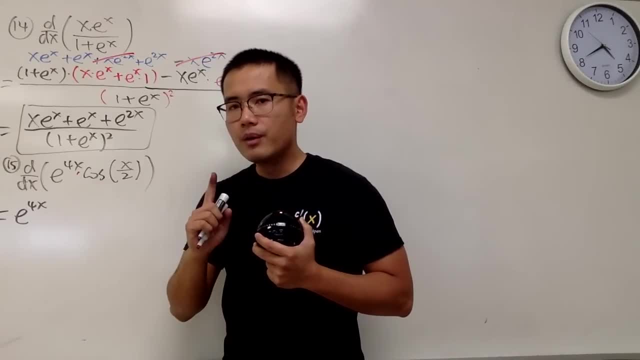 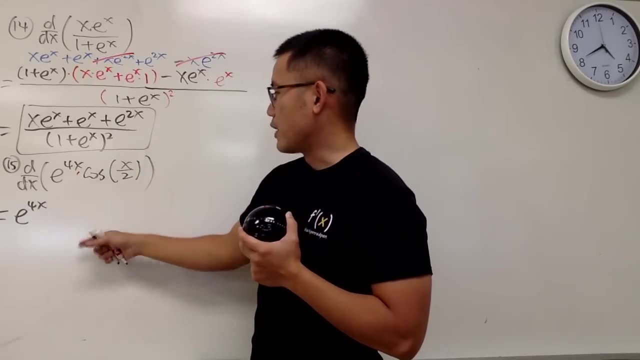 And we multiply by the derivative of the second. Well, we have to use the chain rule right here as well, so don't just be careful with that. Anyway, the derivative of the second function, derivative of cosine, is negative sine. so we multiply by parentheses: negative sine. 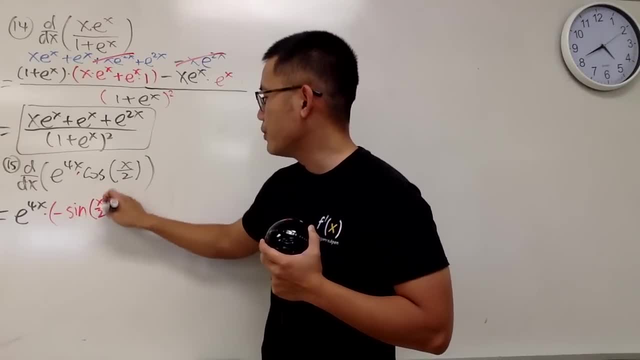 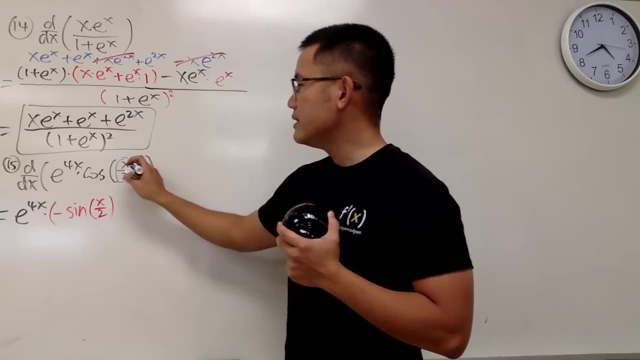 And the input stays the same. So x over 2, right here. But we will have to multiply by the derivative of the inside. What's the derivative of x over 2? It's just 1 half Good, Why. 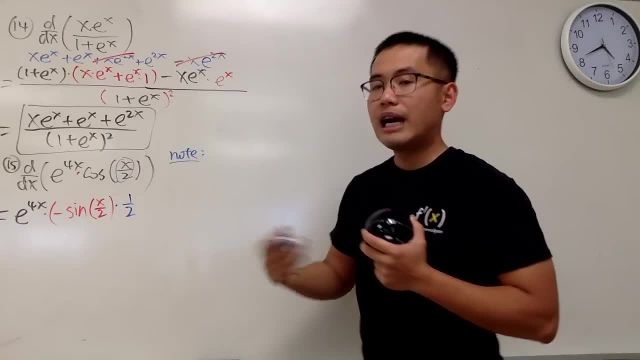 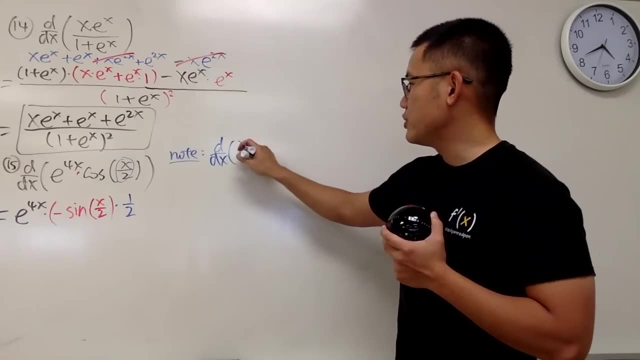 This is just a small note, okay, Because I have experienced some students. they would like to just use the quotient rule right here. You don't do the quotient rule for that, Because when you have to differentiate x over 2, you have two ways to do it. 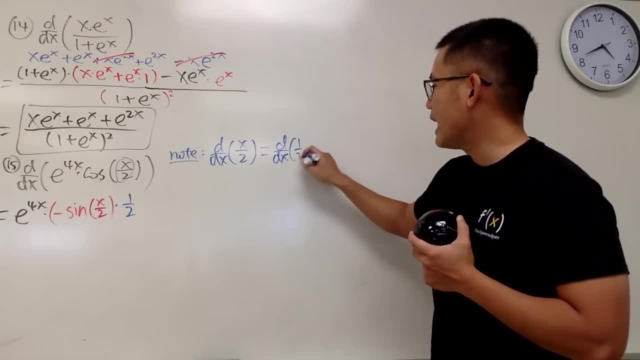 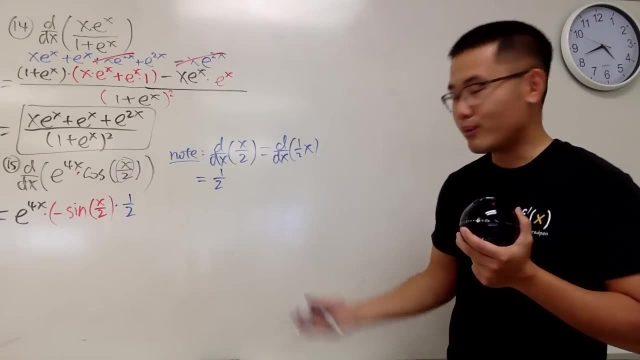 You can just look at it and you can do this as to differentiate 1 half x, right, 1 half times x, And of course you'll just end up with 1 half like that. So differentiating this is just 1 half. 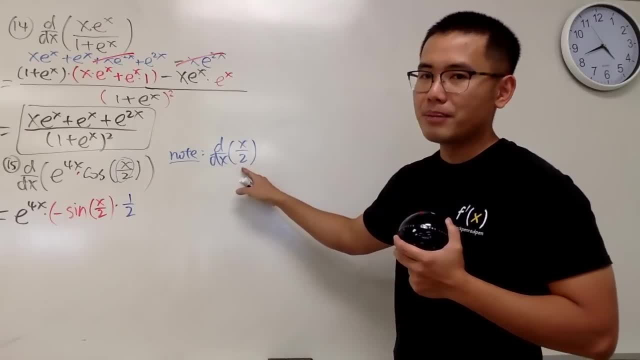 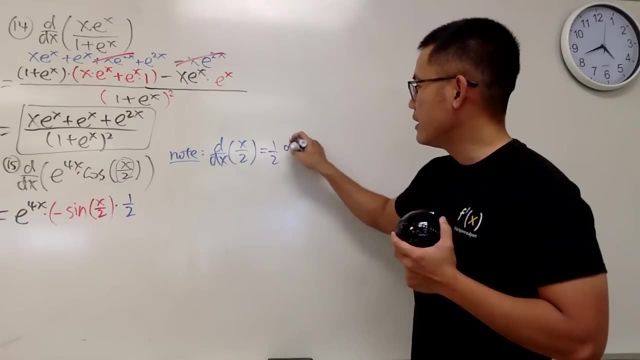 Do not do quotient rule. Whenever you have a number on the bottom, just focus on the number. One other thing you can do is bring the fraction 1 half in the front and then differentiate whatever function is left, Just like that. 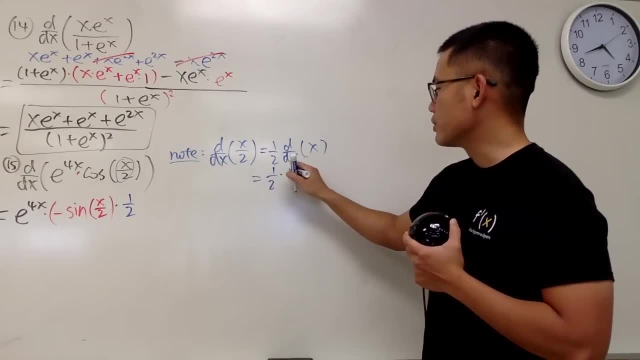 And you see this is 1 half times x. This is 1 half times the derivative of x, It's just 1.. So it's just 1 half times 1, which is just 1 half. Just all that stuff. 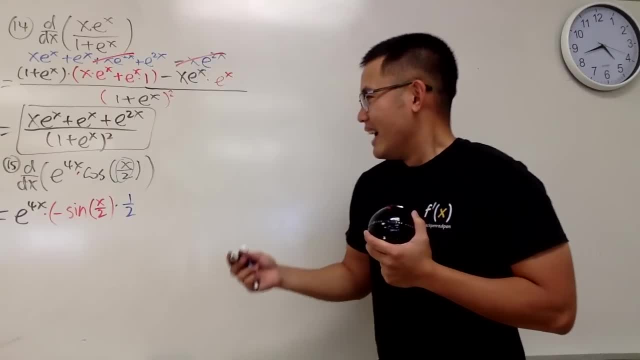 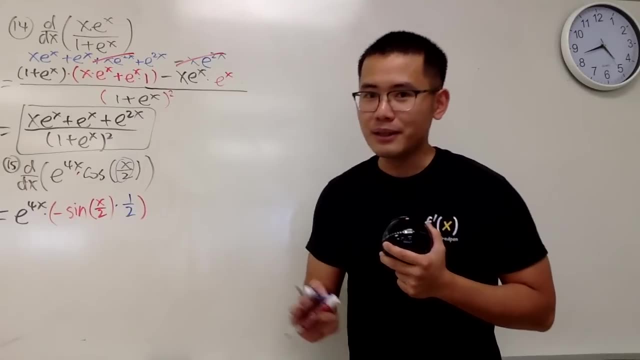 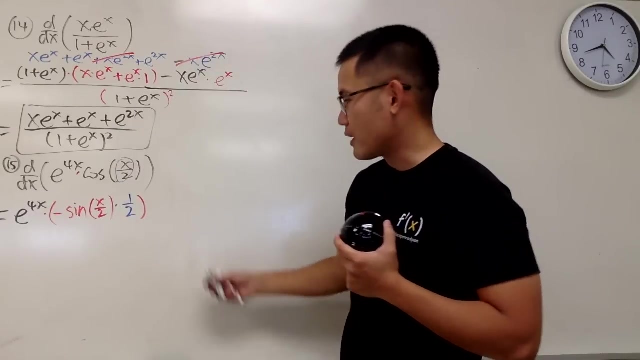 Yeah, So yeah, All right, I have to close the parentheses Right here. Not done yet, Not done yet. This is just the first function times the derivative of the second, And then we add a second function, So we put on plus. 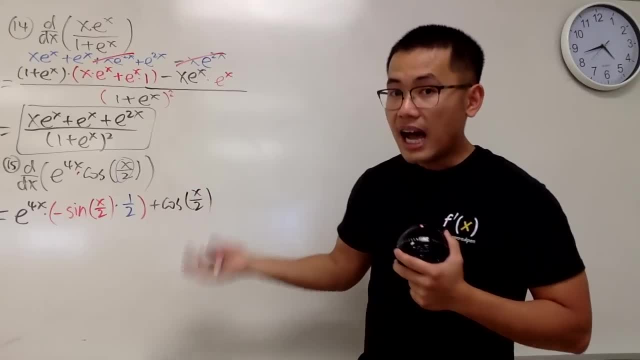 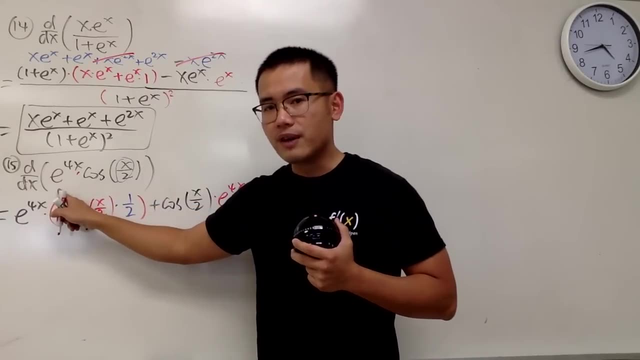 And the second function is cosine of x over 2.. Cosine of x over 2 times the derivative of the first function. So we multiply by e to the 4x right, Because the derivative of the first function derivative e to the 4x. we first write it down. 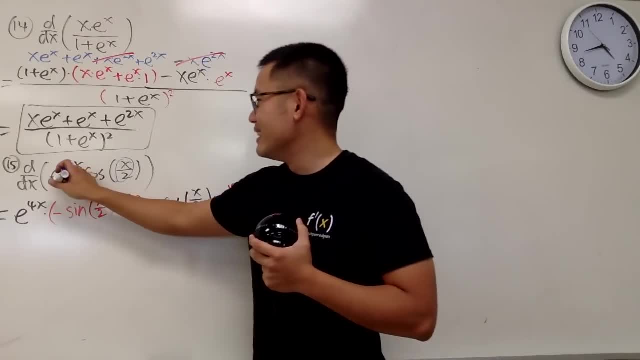 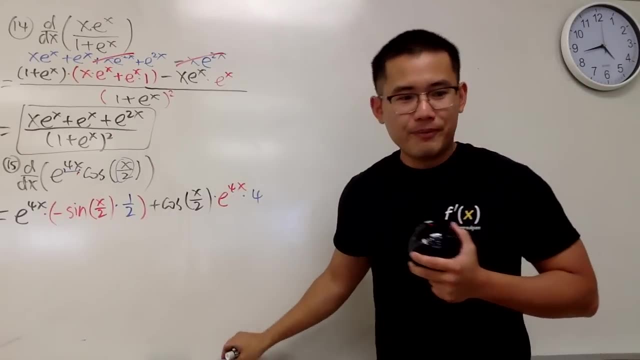 And then we multiply by the derivative of 4x, which is just a 4. So this right here is the Chen-Lu part. So this right here is pretty good And there's nothing too much we can do to simplify. 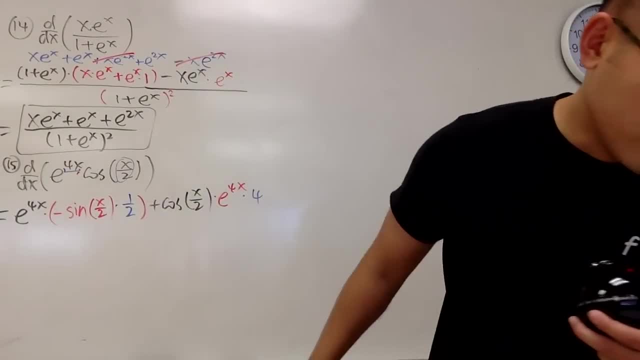 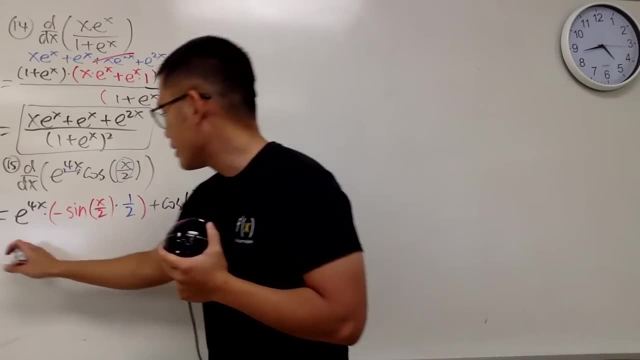 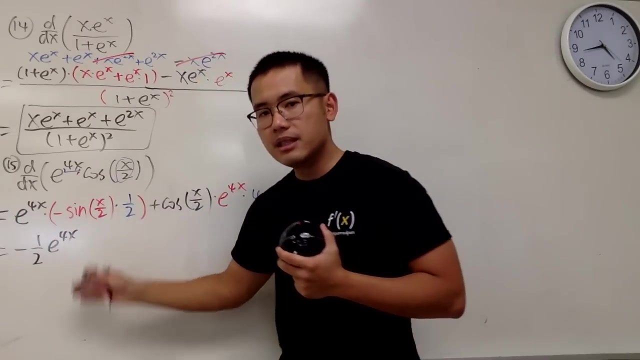 And I didn't factor out e to the whatever, So I will just pretty much write down the results. That's how it is. So finally, the answer right here is negative 1 half e to the 4x times sine of x over 2.. 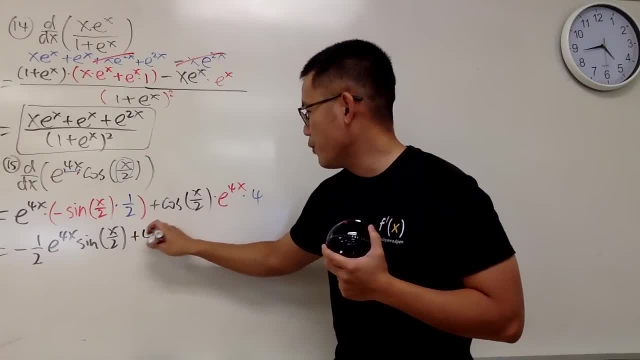 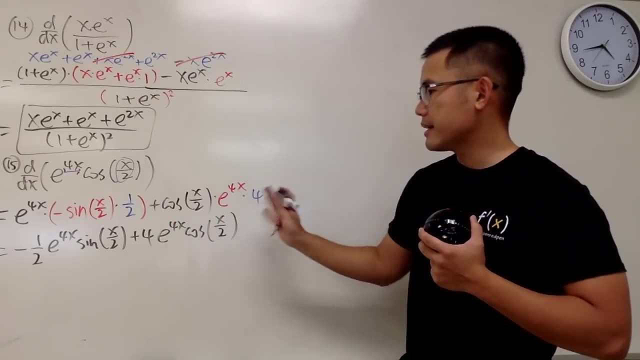 And then 4 all the way in the front, So plus 4. And then let me put on e to the 4x And cosine of x over 2. Like that? So this right here is the answer for that derivative. 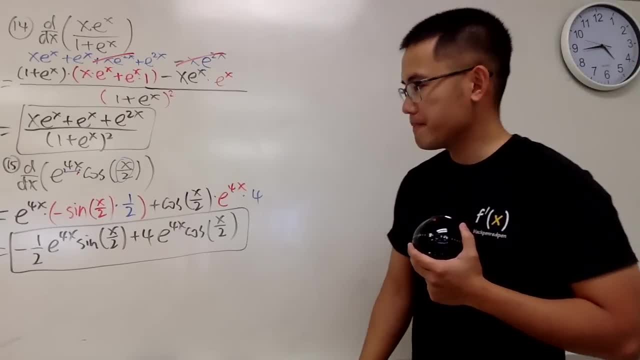 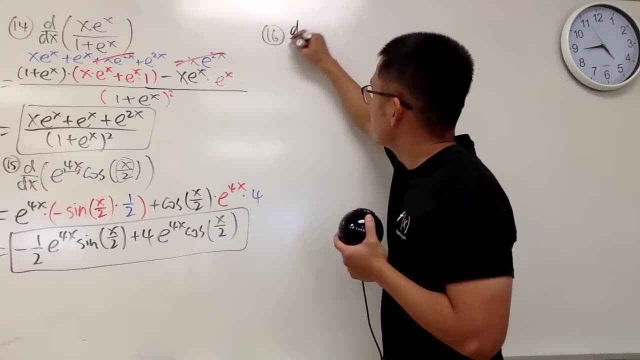 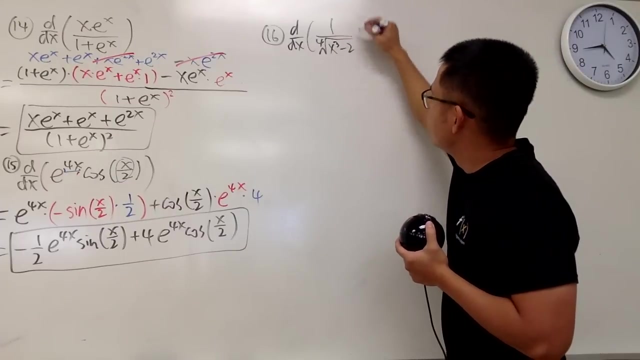 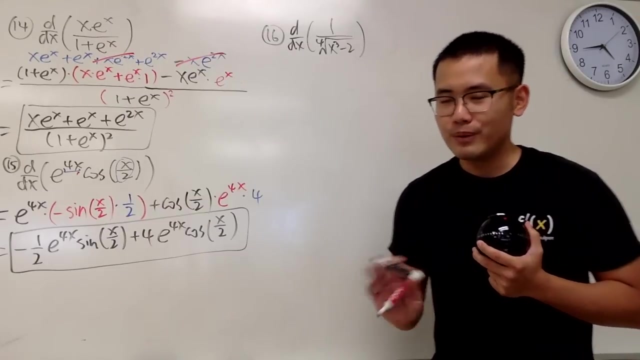 All right, Number 16.. I will just write it down here, Number 16.. Here we are going to differentiate 1 over the fourth root of x to the third power minus 2.. Like that, Should we use the quotient rule? 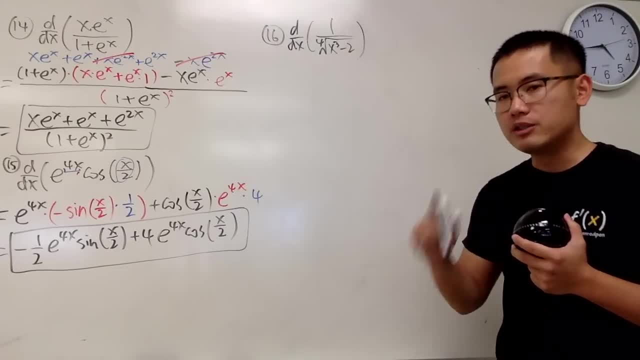 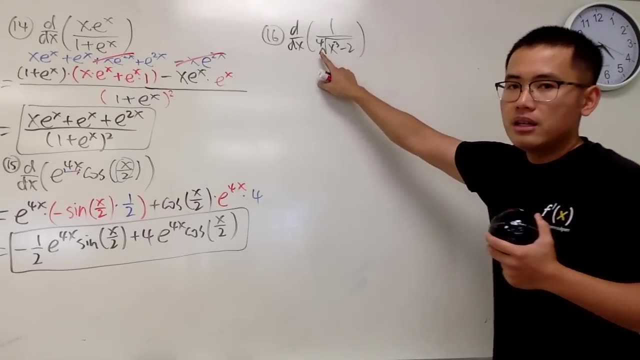 No, Because on the top again, it's just a number, It's just a 1, right. So it's a much better idea to write this as a negative power, And this right here is like the same as a 1 over 4 power. 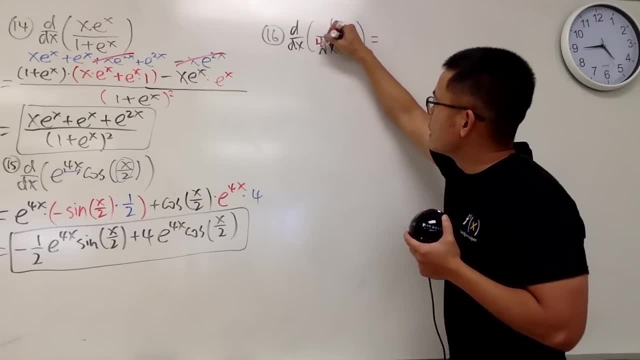 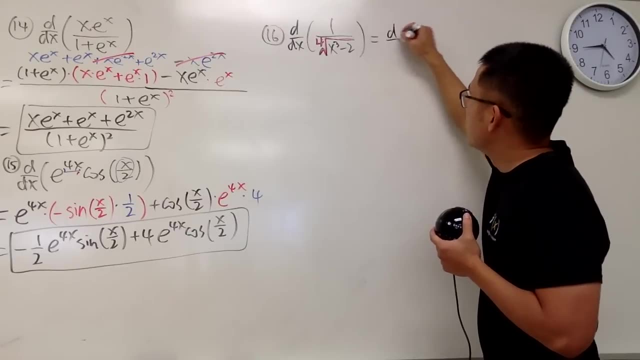 So here we go. This is the fourth root. It's like 1 over 4 power, but it's in the denominator, So when you write it on the top we will just write it as parentheses, with x to the third power minus 2 inside. 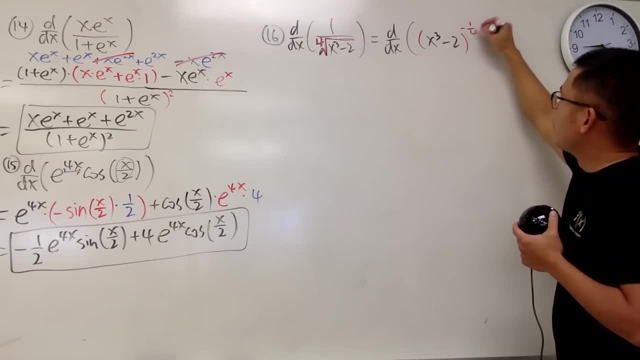 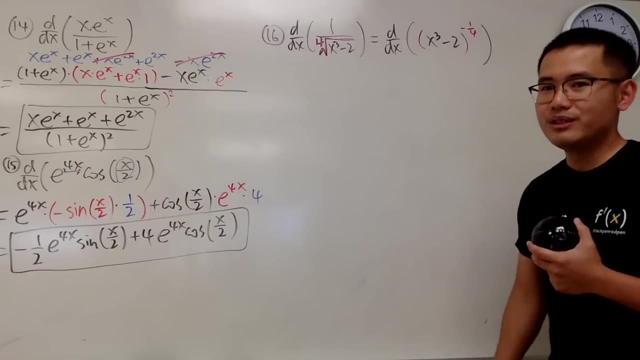 And then we raise this to a negative 1 over fourth power, Like that, And when we are looking at the expression this way, we can just use the power rule and also the Chandu, And we will do that, of course. 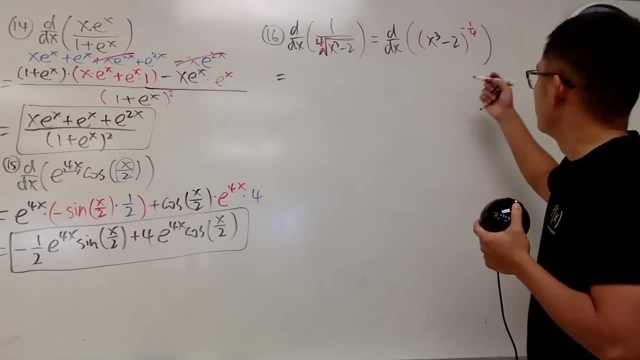 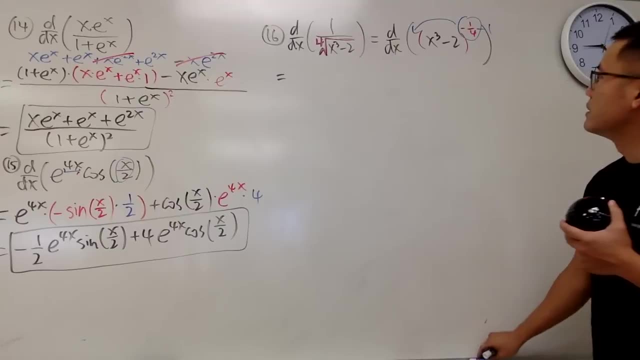 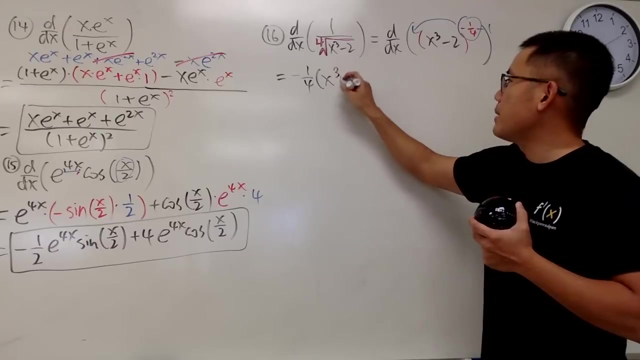 So here we go. I'll just put this down: All right Power rule in action first. So we have the negative 1 over 4 over the window front Inside states the same. So x to the third power minus 2.. 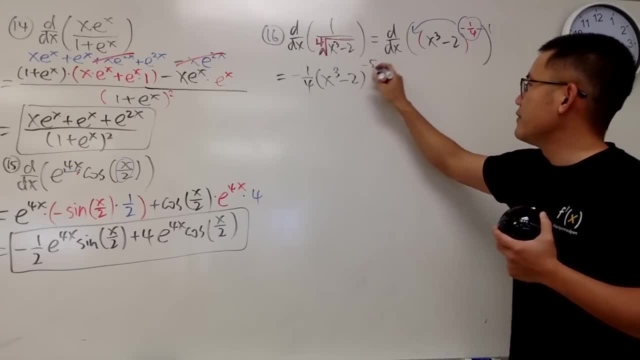 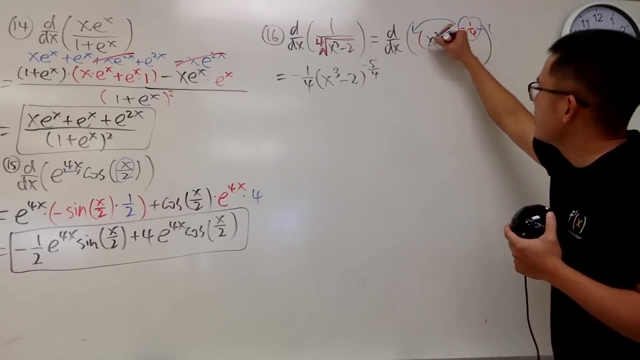 Negative 1 over 4 minus 1.. Just do your fraction. You end up with negative 5 over 4.. And we do our Chandu. The derivative of the inside, The derivative of x to the third power, is 3x squared. 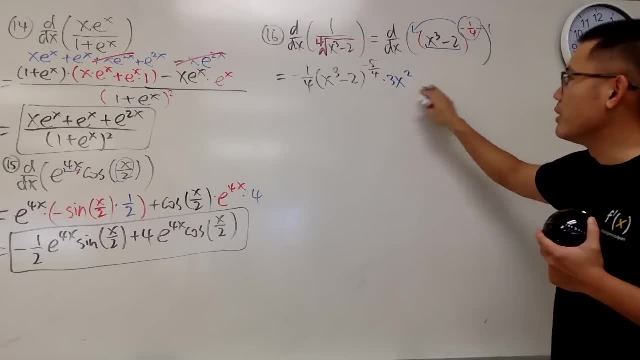 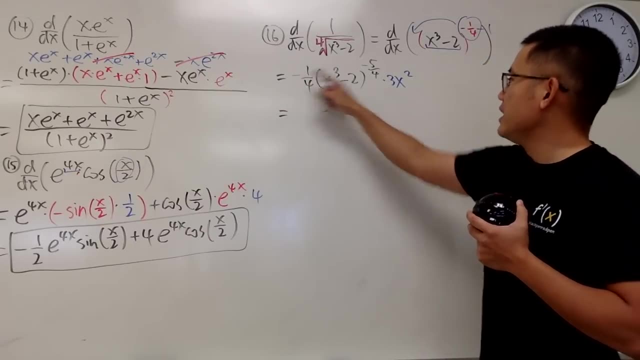 And just one term, Because the derivative of negative 2 is just 0.. So this is all we need. Lastly, we put things down together: Negative, And this is on the top, So let me write it down as negative 3x squared over. 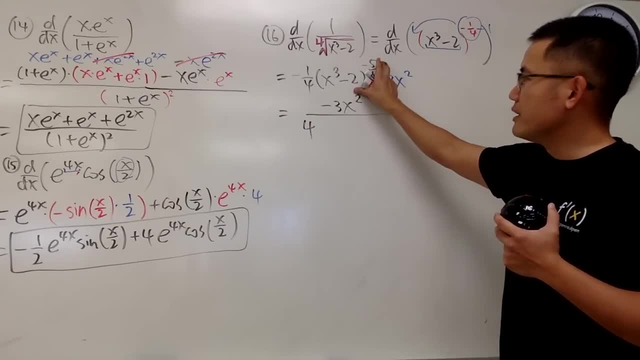 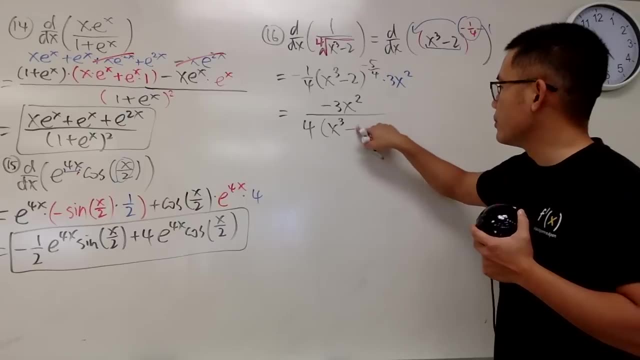 We have this 4 right here. I'm going to bring this down to the denominator And because that's a negative power, right, So we will just write it as x to the third power minus 2 times 2. And then raised to the 5 over fourth power. 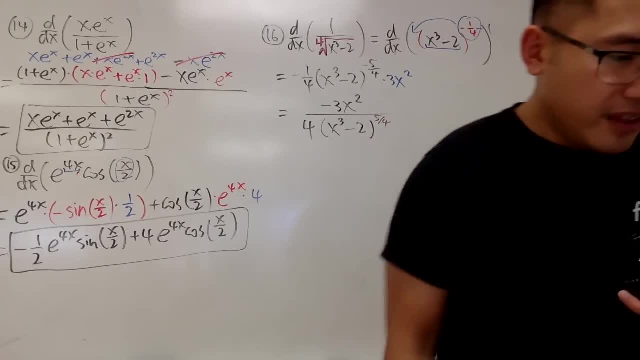 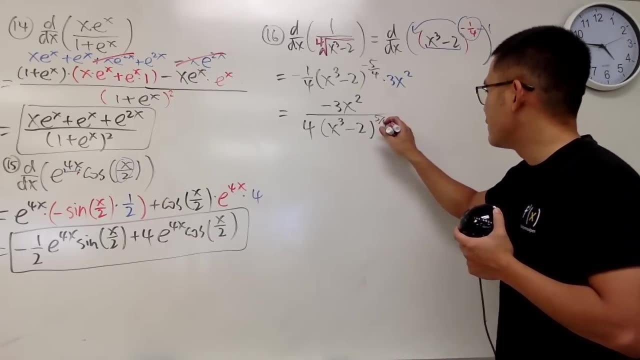 And that's a positive 5 over 4.. Well, I didn't leave the answer like that. I changed the answer to the radical form. So remember, whenever we have a fourth, like if the power has an over 4,. 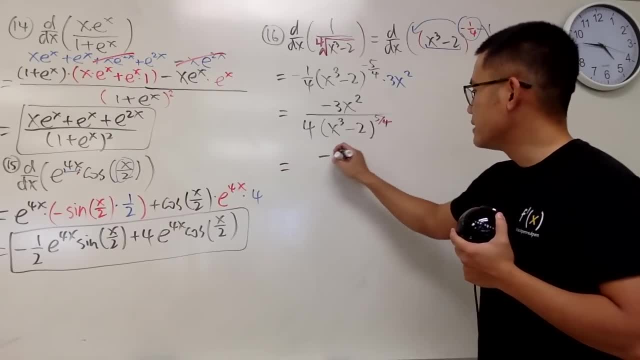 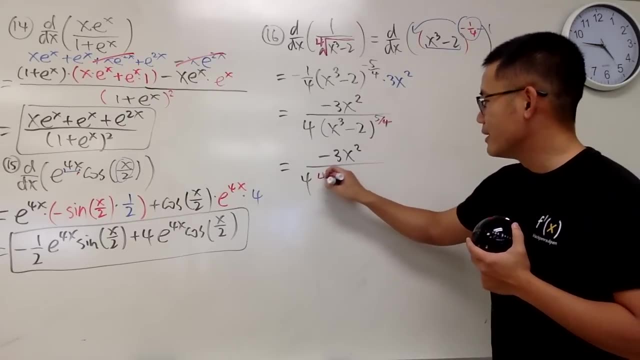 that turns out to be a fourth root. So on the top is negative 3x squared over. This is 4.. This little fractional denominator is the fourth root, And then we just write it inside as x to the third power minus 2. 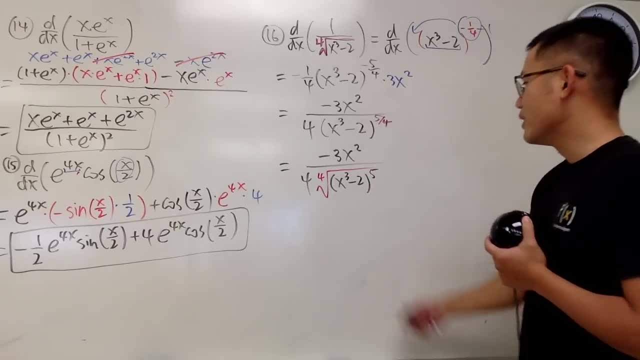 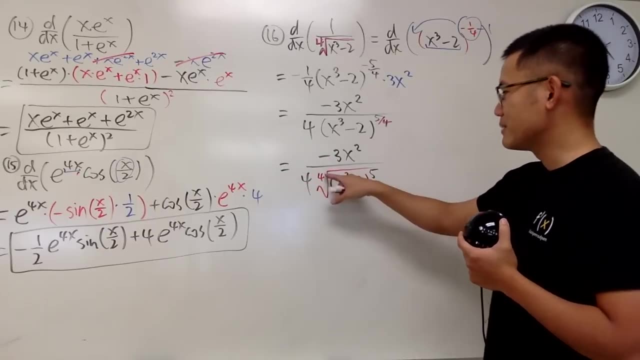 and raised to the fifth power. And some people might be wondering: should I factor out, should I take out x to the third power minus 2 to the first power, and then times Doesn't matter. This is the answer already, okay. 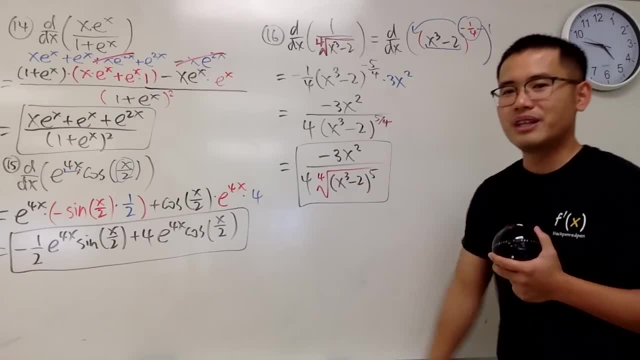 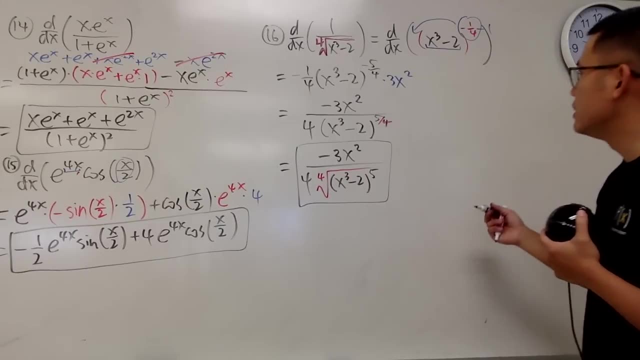 You can simplify the radical if necessary, But in calculus this right here is totally acceptable. All right, Number 17.. I will do it here, maybe. Let's see. Let me just write it down right here. I don't know why I want to do this. 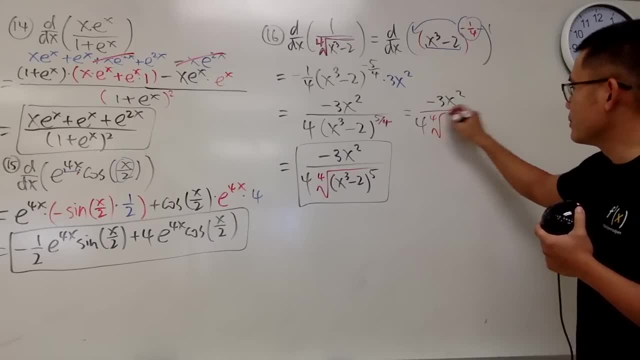 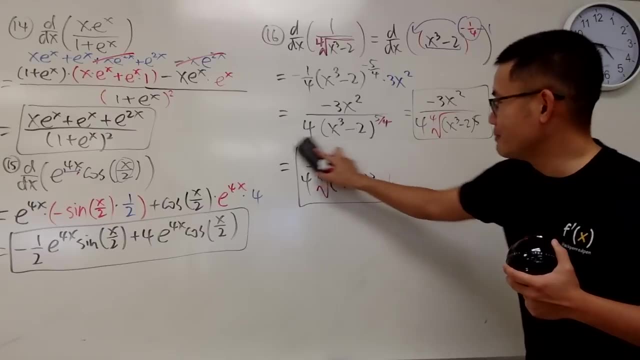 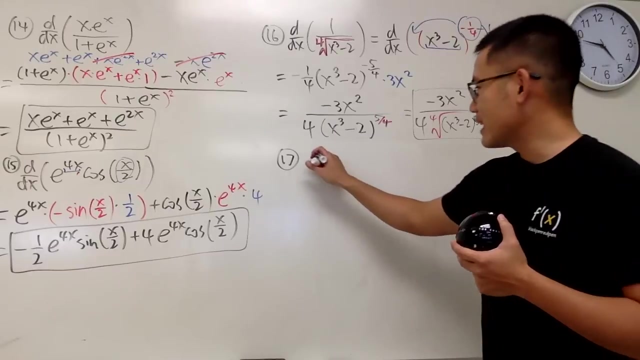 but I think I can fit in number 17 right here before I erase. So let me just do that I will erase this part and then I'll put in number 17 right here And now. I just feel really satisfying if I can fit a lot of. 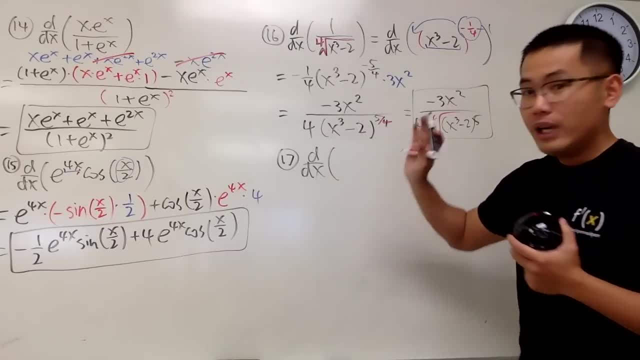 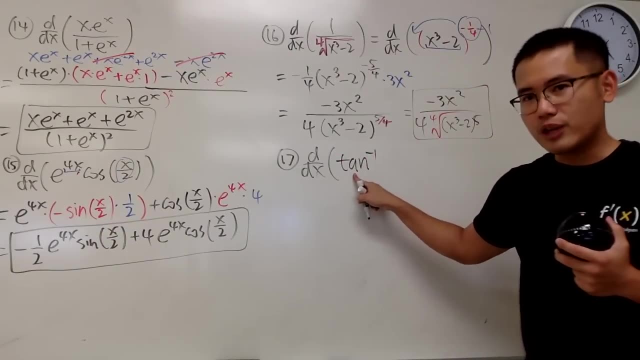 math on one board, you know. Anyway, we are going to be differentiating. This is the first time that we are doing the inverse tangent. So we have the inverse tangent And this notation- I know it's one of the most disliked notation in math. 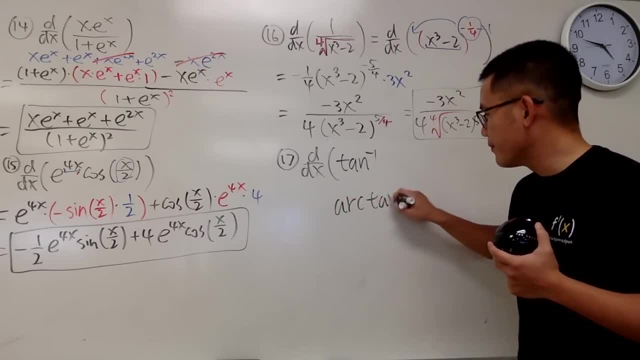 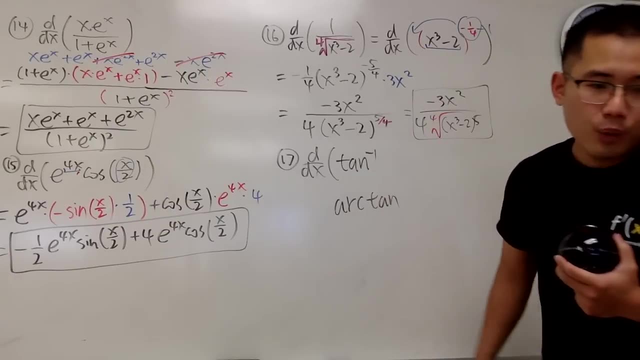 Some people like to write it as the arc tangent, but it's the same thing, right? So just get used to it. This doesn't mean 1 over tangent, so just keep that in mind. Anyway, we have the inverse tangent. 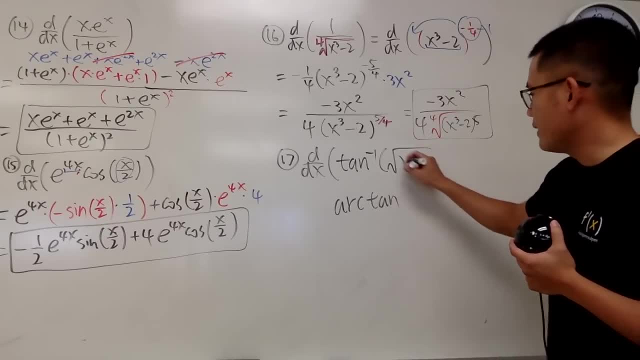 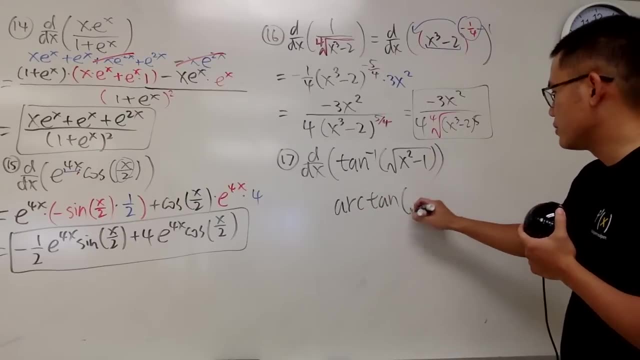 and the input is square root of x squared minus 1.. Like that. And, of course, if you write it as the arc tangent, you just write arc tangent of square root of x squared minus 1, like that, right? Anyway, first of all, 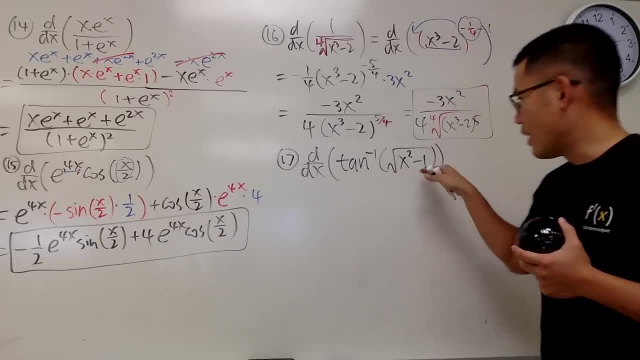 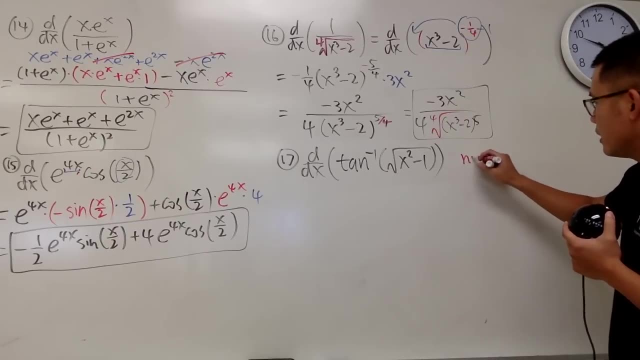 this right here is not 1 over tangent of whatever You don't do the power rule for this, You just have to know the derivative for inverse tangent. So I will put down a quick note right here for you guys. Today, if we differentiate inverse tangent of x, 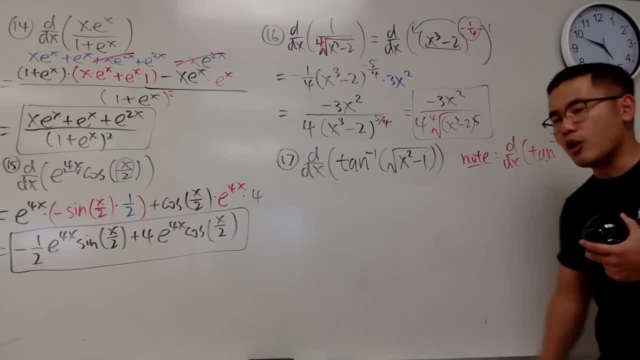 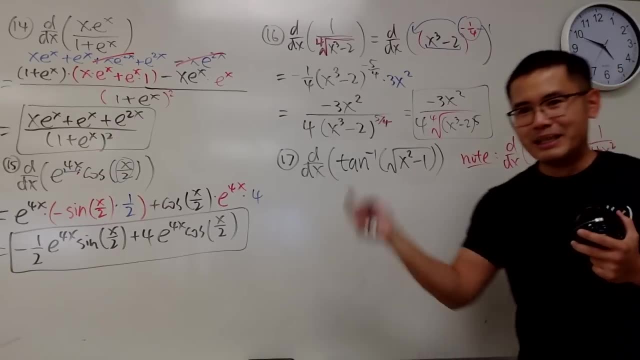 this is the one that you definitely have to know really well. You get 1 over 1 plus x, squared right. Well, how do we prove it? You'll see by the end of the video Number. I don't remember. 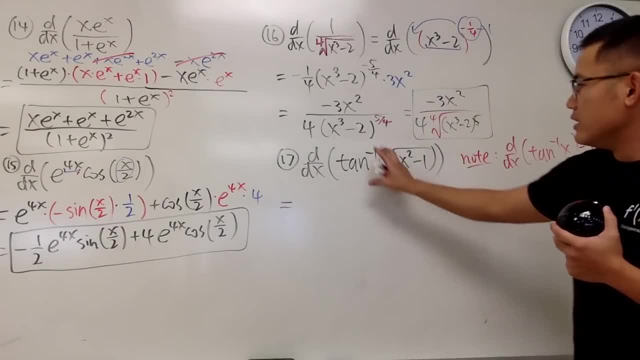 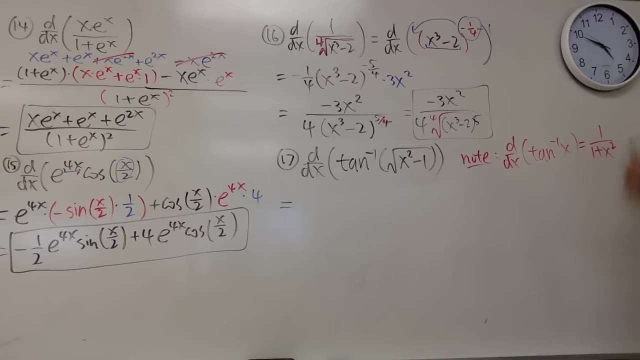 Anyway, here we go. So whenever we're differentiating inverse tangent of the input, you see that we will do 1 over 1, plus the input being squared. So we'll do that Right here: we do 1 over 1 plus. 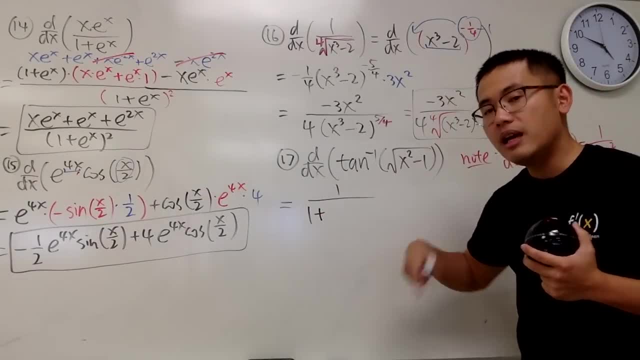 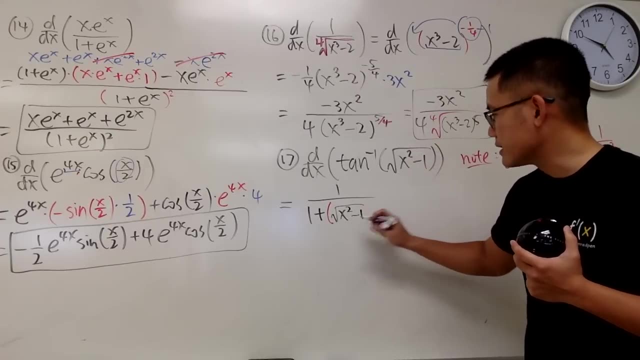 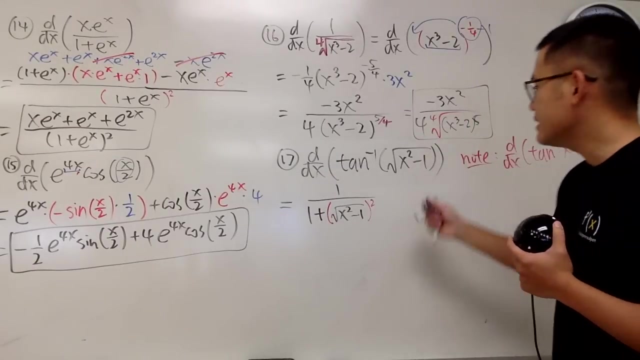 we put it inside right here and we square that. So I will put down parentheses with square root of x squared minus 1 inside and I will square that Right. So that's the general form for the inverse tangent derivative. But again we will have to do the chain rule. 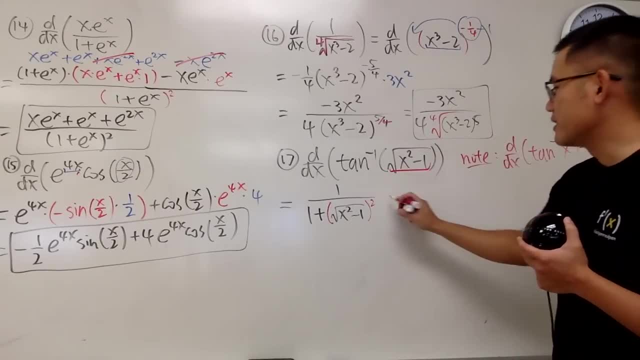 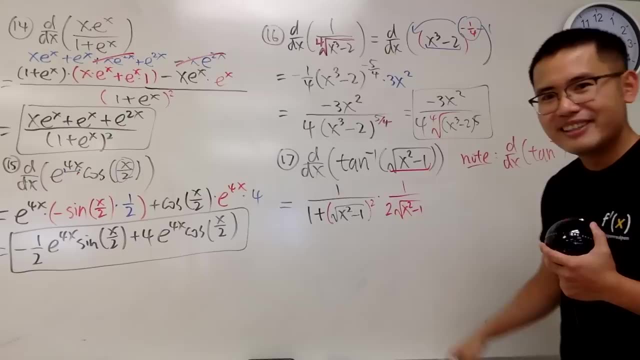 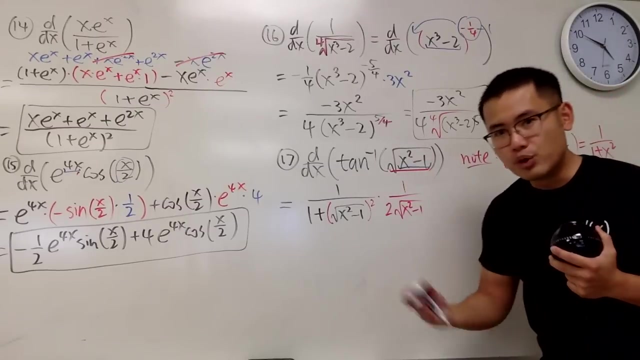 Here we go. The derivative of square root of something is 1 over 2 square root of the inside. you keep it again. right, Just keep it. But we do the chain rule again, because the derivative of the inside, derivative of x squared minus 1, is 2x. 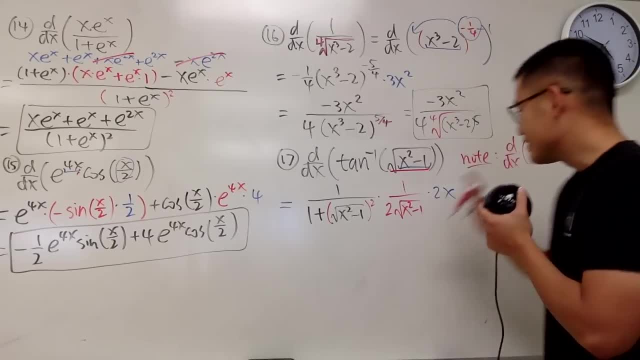 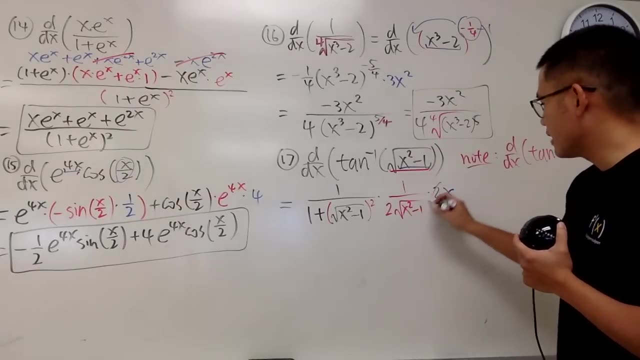 So we multiply by 2x, like this: Alright, so this is the idea, This is pretty much it, And now we just simplify. I notice that we have the 2 over 2, so we can cancel them out. That's very nice. 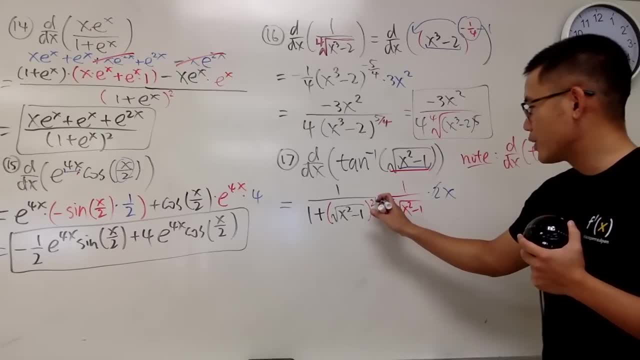 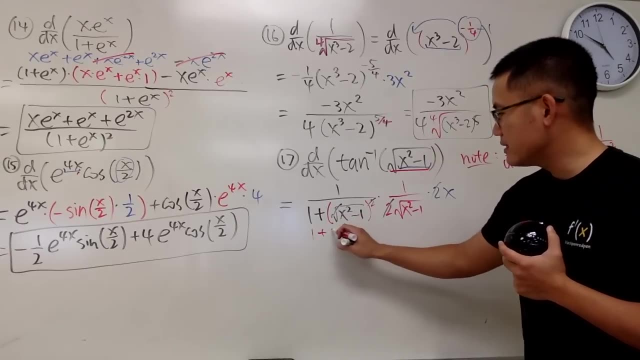 And we also see that this square and the square root cancel each other. That's also very nice. When we cancel this out, we get 1 plus. this is just x squared minus 1.. 1 minus 1.. Cancel it out. 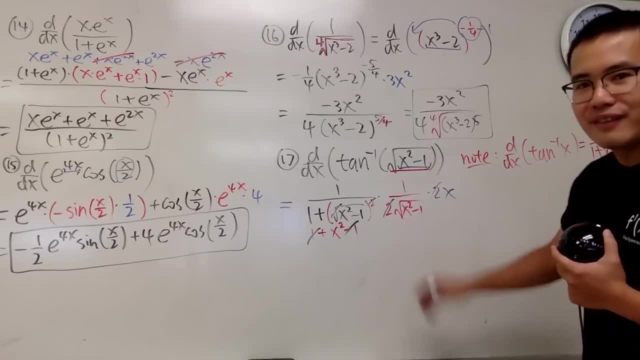 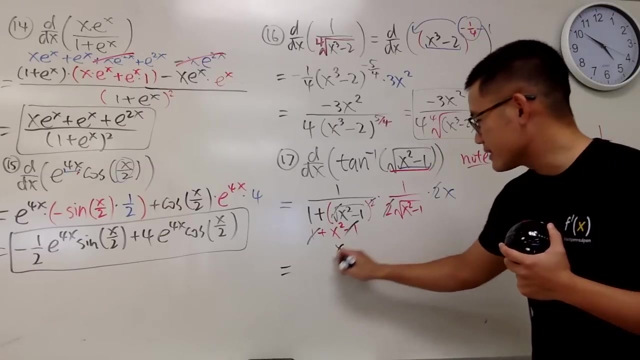 That's pretty nice. So that's what we have. Is there anything else that we can cancel out? Yes, Because we see that this is just x over x squared, Right. So let me just write it down nicely for you: x over this right here is x squared. 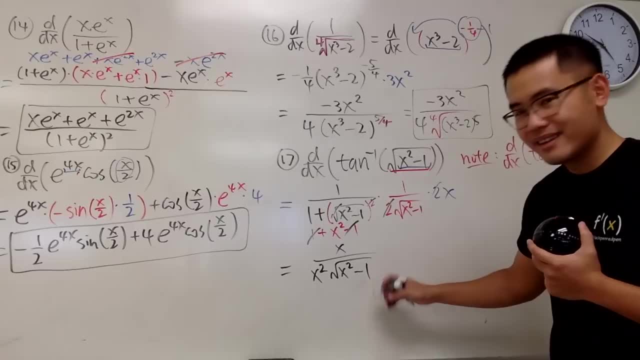 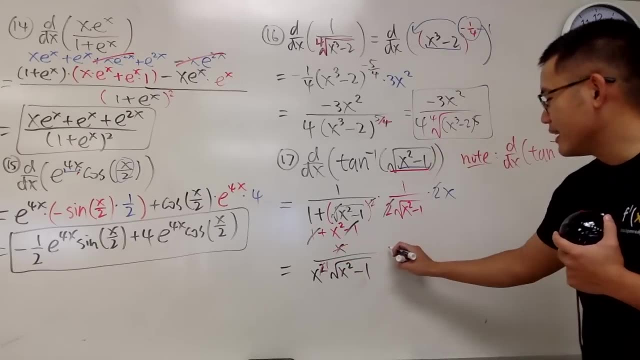 and we keep it square root of x squared minus 1.. This and that we can cancel them out, We'll just get 1, and this becomes the first power. So finally, the answer is 1 over only x to the first power in the front. 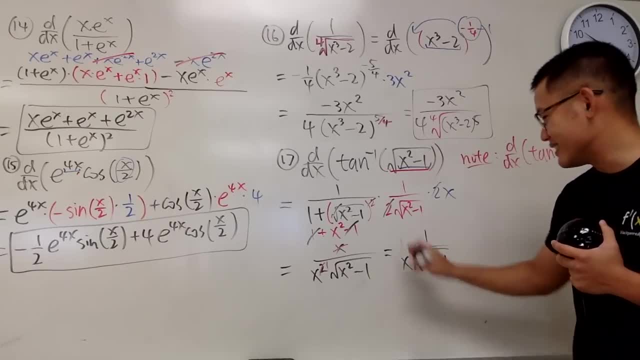 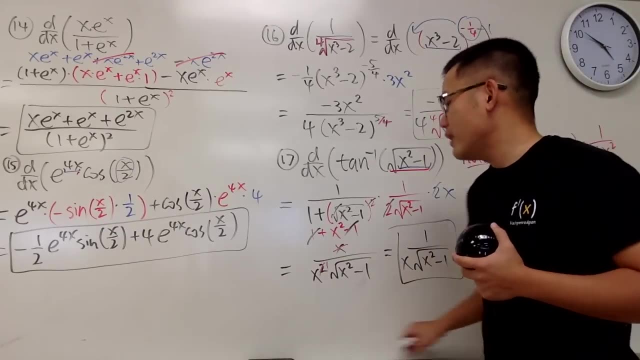 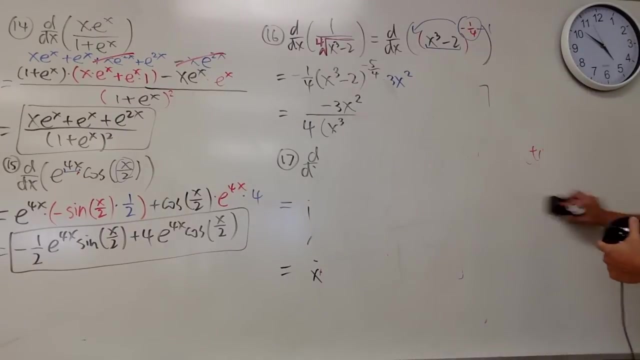 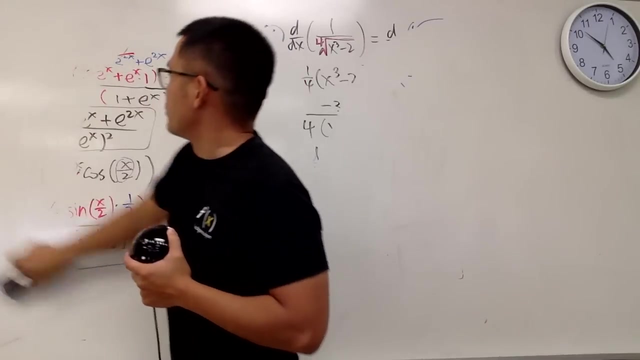 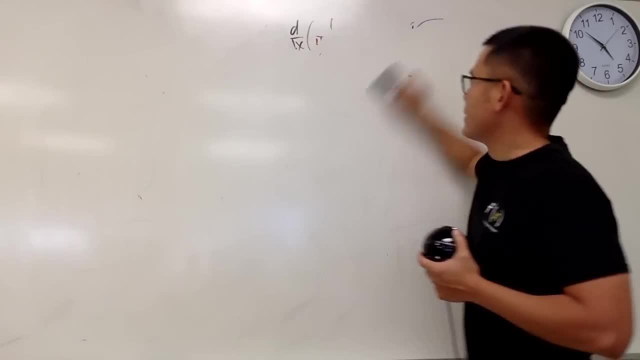 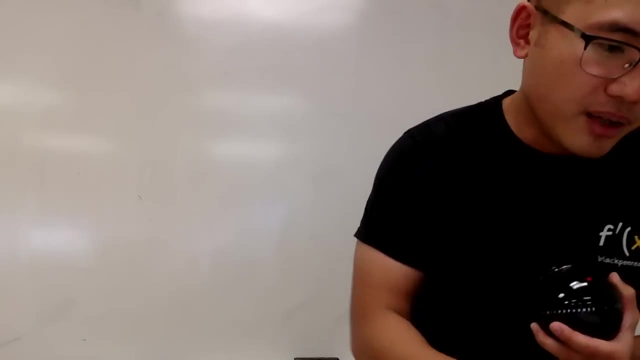 Hopefully at some point I can do like a. I can speed up the process. But, as I said, the first 20 questions were so I just want to make sure I give that detailed explanation and all that. Anyway, number 18.. 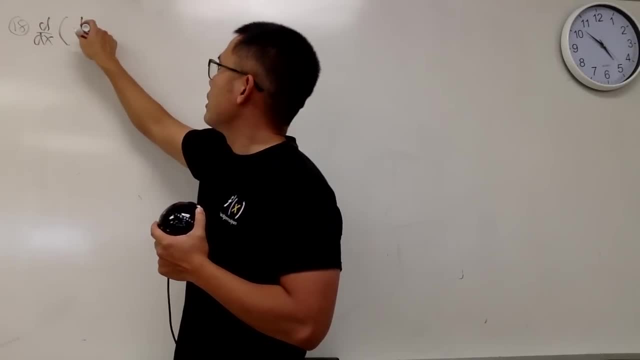 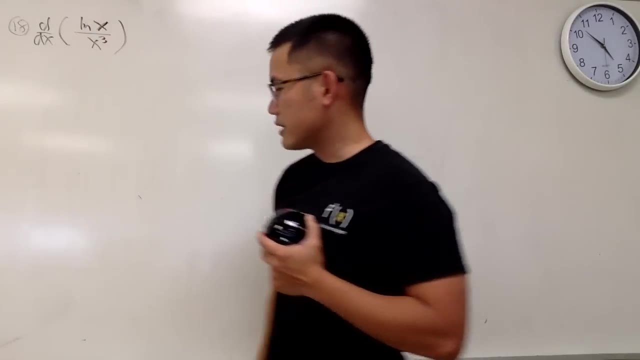 Here we have to differentiate. We have natural log of x over x to the third power, Like that. All right, Here we go: The x to the third power in the denominator and the natural log of x on the top. We have to use the quotient rule. 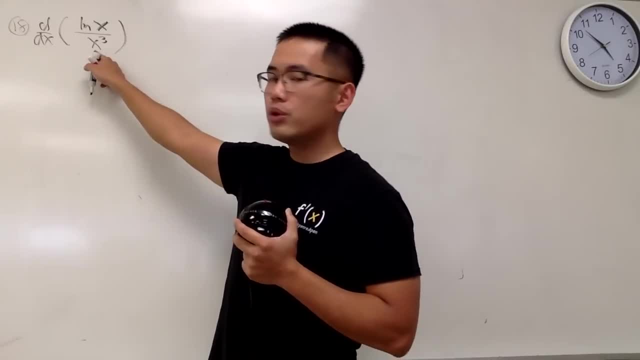 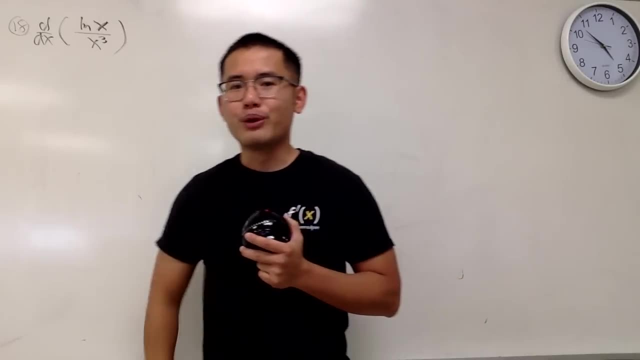 Two functions, dividing quotient rule. Some people will tell you to write this as x to the negative 3 power times natural log of x and do the product rule. That's fine, Up to you, though. I'll just do the quotient rule, Why not? 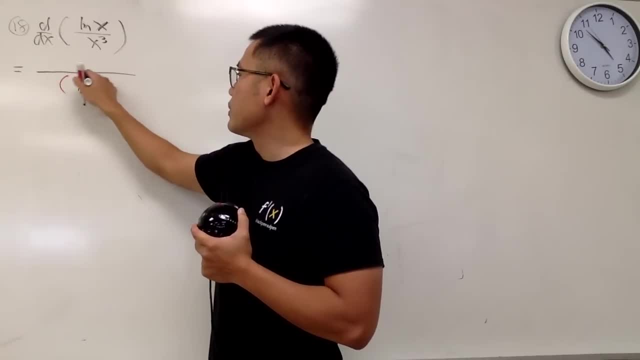 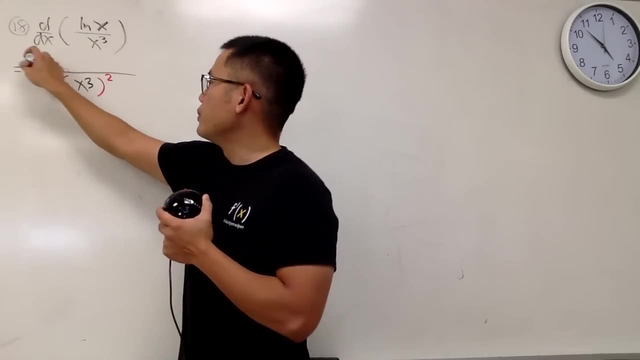 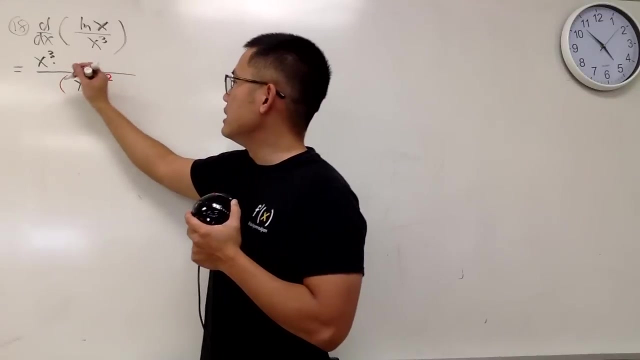 So let's go ahead and square the denominator. So we have x to the third power and we square that On the top. we keep the bottom function, which is x to the third power, and we multiply by the derivative of the top. The derivative of natural log of x is 1 over x. 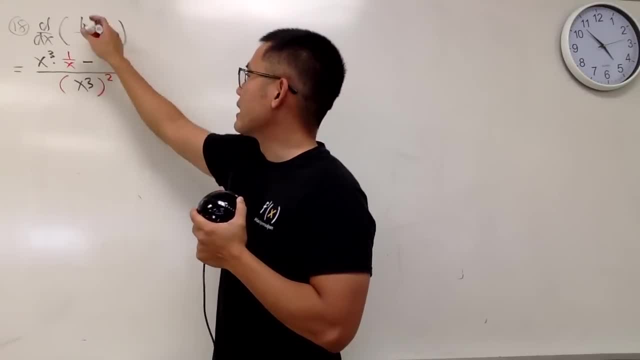 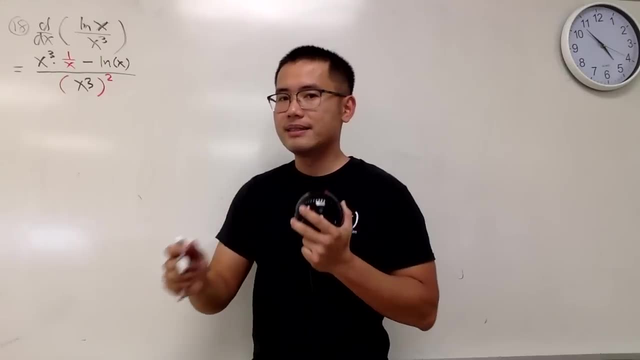 Good. And then we minus the top function, which is natural log of x. I would like to use the parentheses right here- Natural log with the input x, Because I will have to multiply by the derivative of the inside, The derivative of. 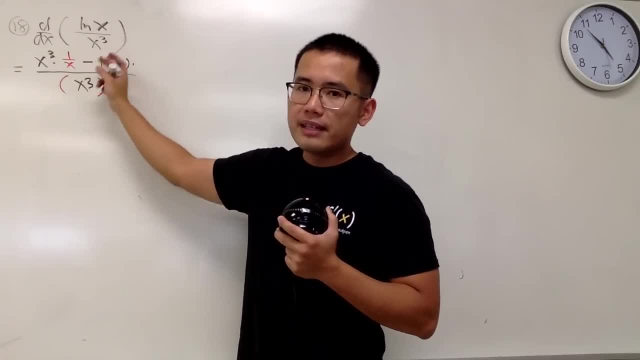 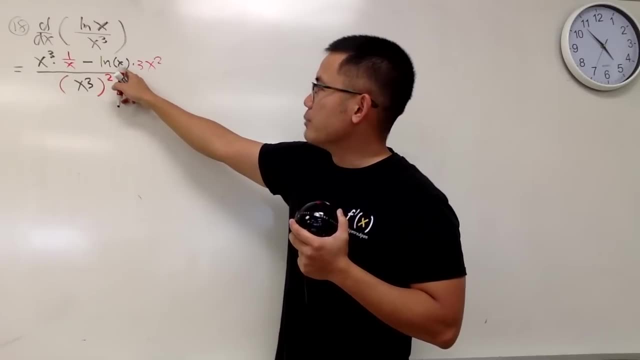 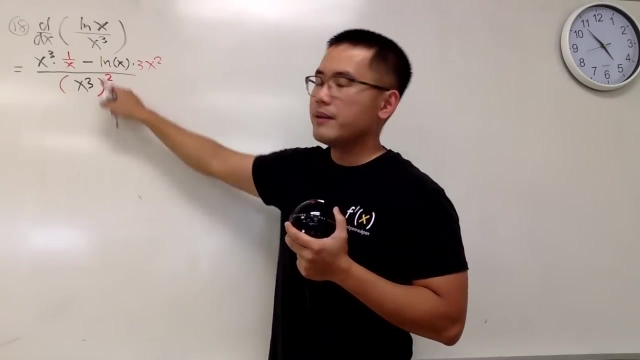 sorry, the derivative of the bottom, The derivative of x to the third power, is 3x squared. Without the parentheses, it seems like you can just multiply the x and 3x squared together, But no, This x is an input for the natural log. 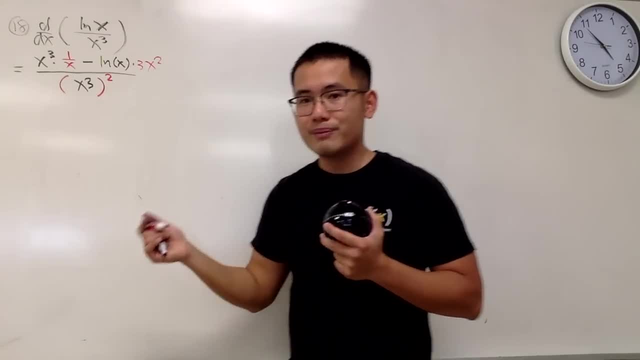 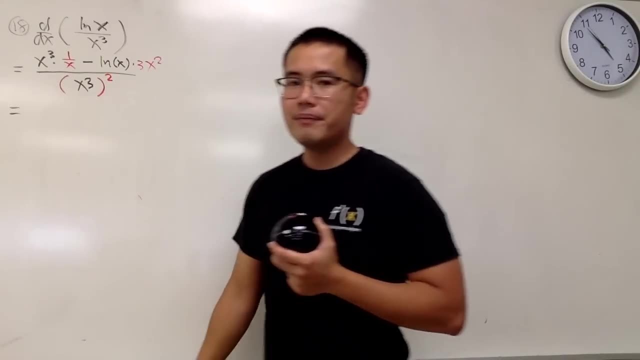 This is just like 3x squared being multiplied with the whole function. You cannot multiply the x and the x squared right here, No Right? Anyway, this is pretty much it for the derivative. Now simplify this. x to the third. power over x. 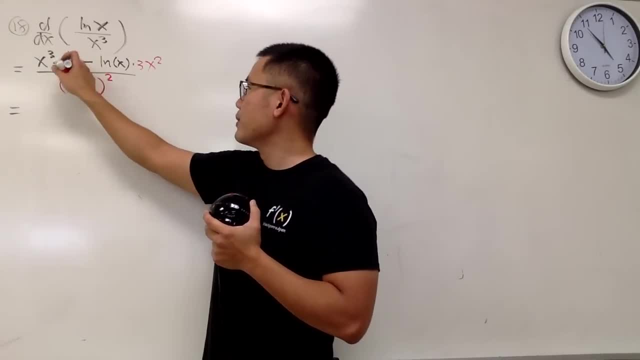 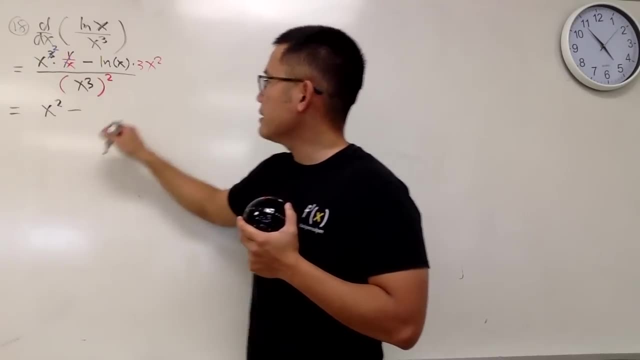 We get x to the second power. Let me just cancel things out for you guys. This right here: cancel out. So we get x squared And this is minus, And perhaps I'll just bring that to the front- 3x squared. 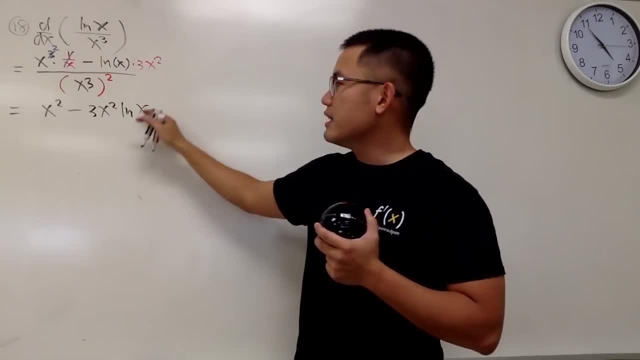 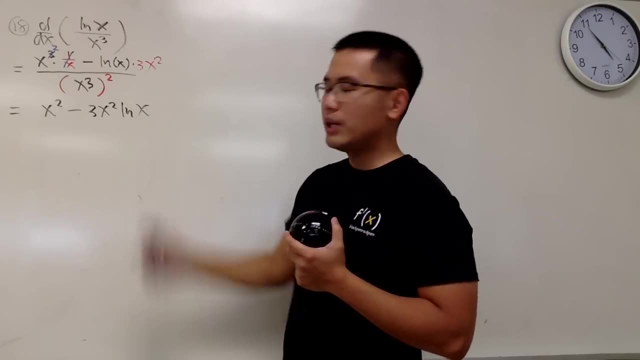 And then we have natural log of x. Whenever there's nothing after the natural log and there's only one input for the x. for the natural log you don't necessarily have to put down the parentheses. So this is okay On the bottom. 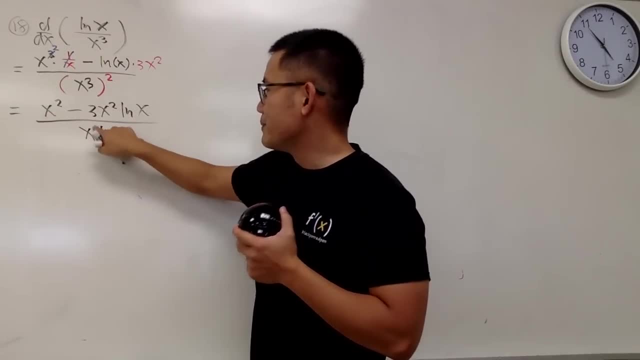 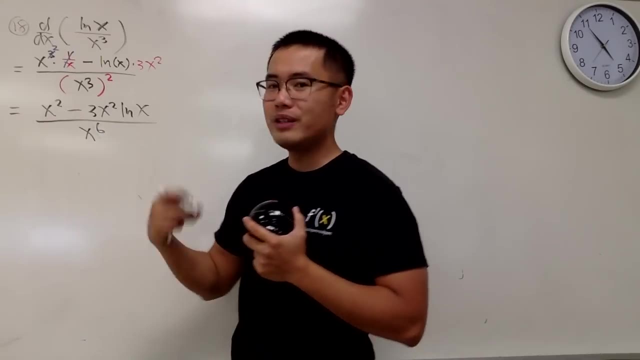 x to the third. power squared, we get x to the sixth. That's the answer, you'll see: x to the sixth. Well, we can do more, Because notice that we can factor out the x squared and then cancel things out, right? 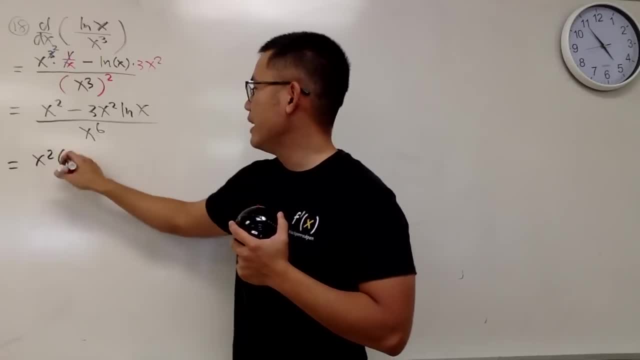 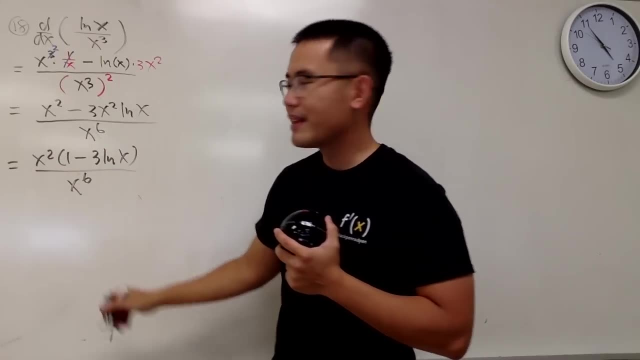 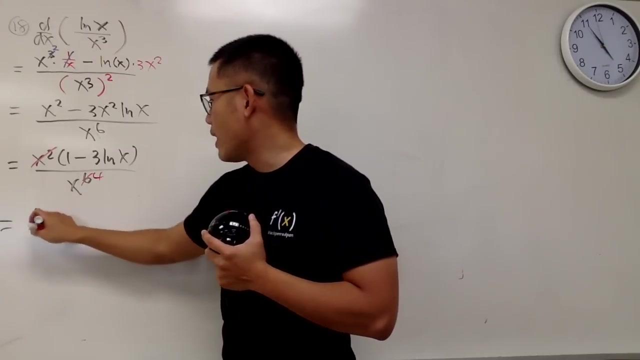 So we will do that. We have the x squared in the front And then 1 minus 3 natural log of x over x to the sixth power We can reduce. That's how I know this is a 4.. Anyway, finally we get 1 minus 3 natural log of x. 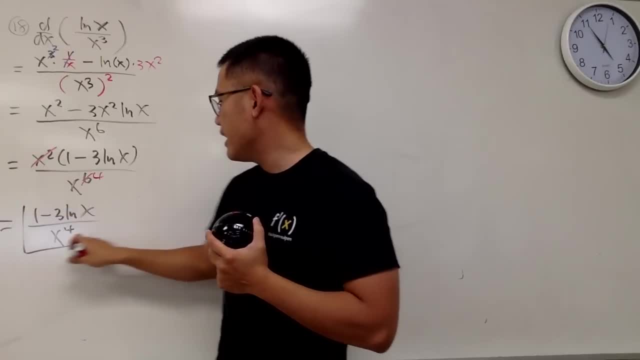 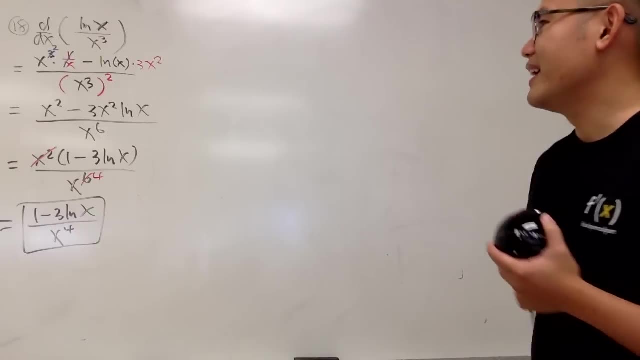 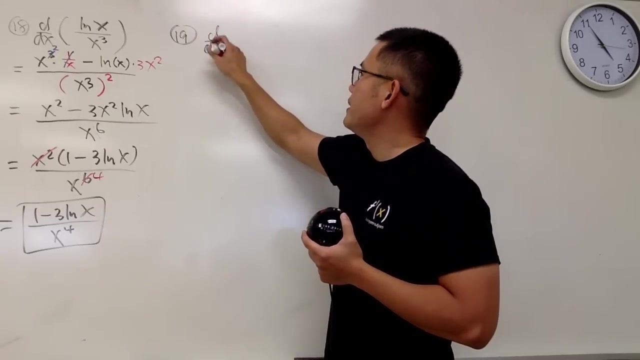 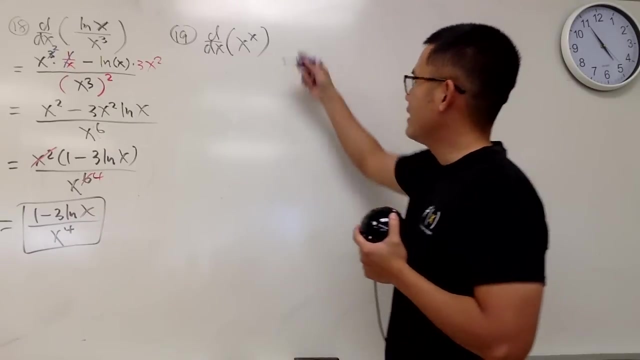 over x to the fourth power. And we are done. That is it? Okay, Number 19.. We are going to be differentiating x to the x power. I see x to x power. Does it have the power? I can just bring the power to the front. 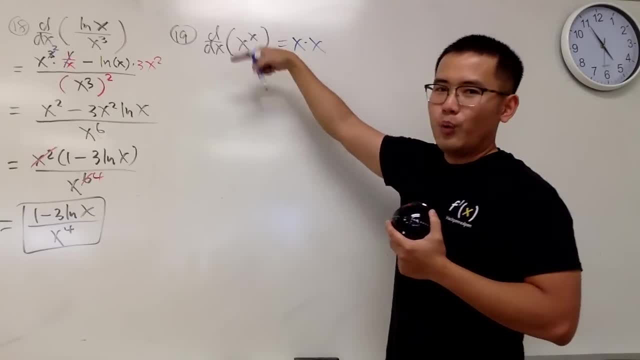 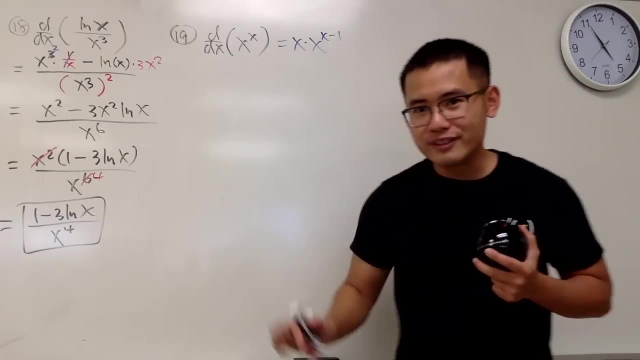 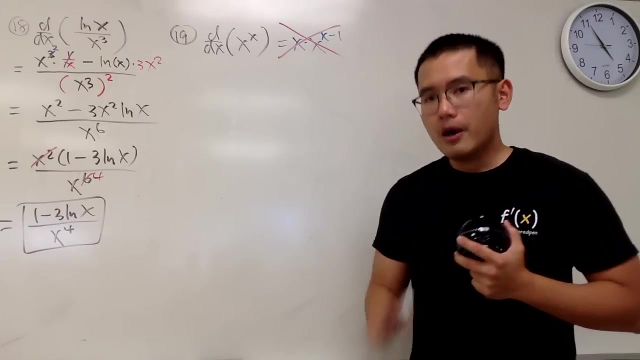 And then this is x, And then 1 minus 1 for the power of x minus 1, like this, Of course not. You know it, You know it. You know it. Otherwise, I have to change that to blue, All right. 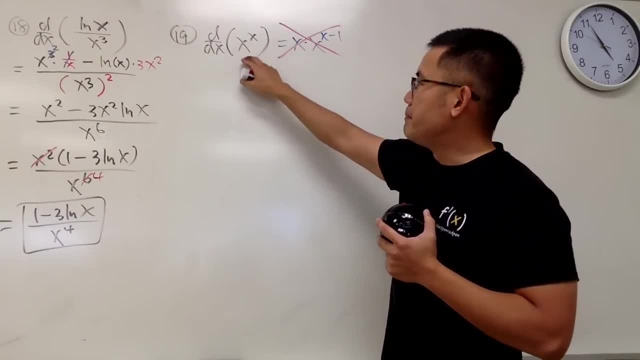 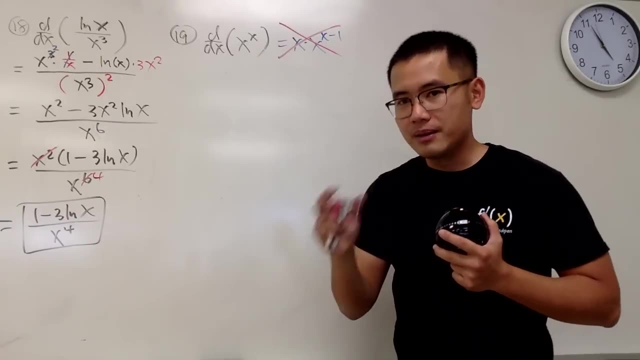 Here is the deal, This right here. it's not a power function. It's also not an exponential function. It's kind of like both, Because you have x for the base and you also have x for the exponent Right. So it's like both. 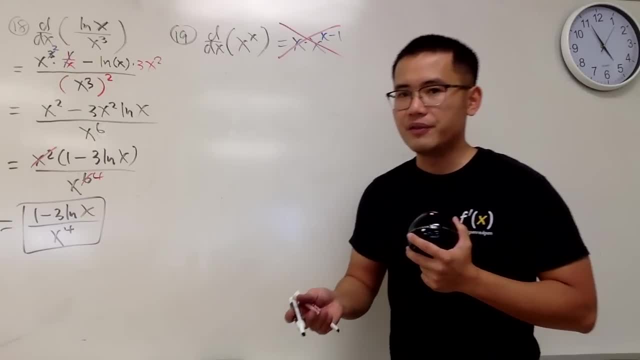 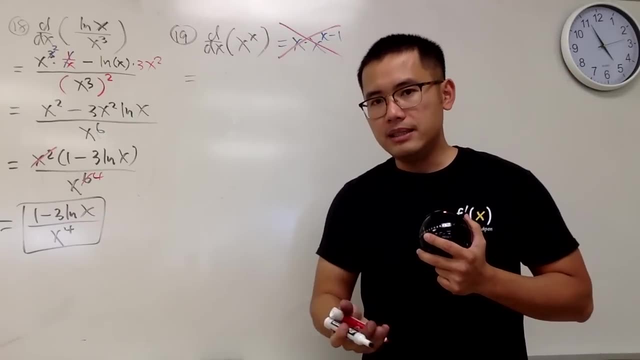 I will show you guys how you can take out this without doing the implicit differentiation. This is the deal. The idea is that you want to work with space, E Right Whenever you have an exponential function. But this is not really an exponential function yet. 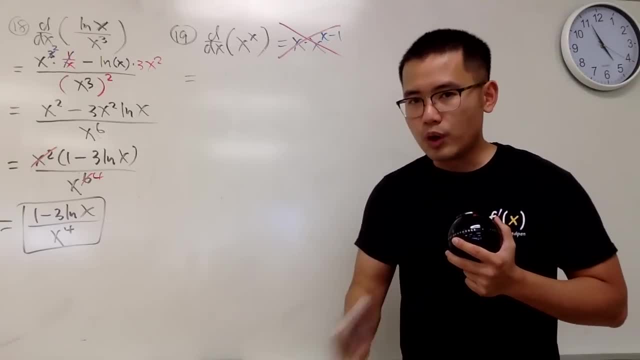 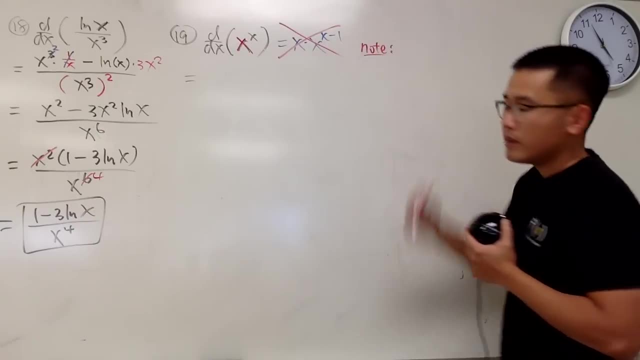 Because, again, the base is x. You don't want to work with space x. This is how you can do it. Look at x And I'll put down a note right here for you guys. What we can do is we can write x as E. 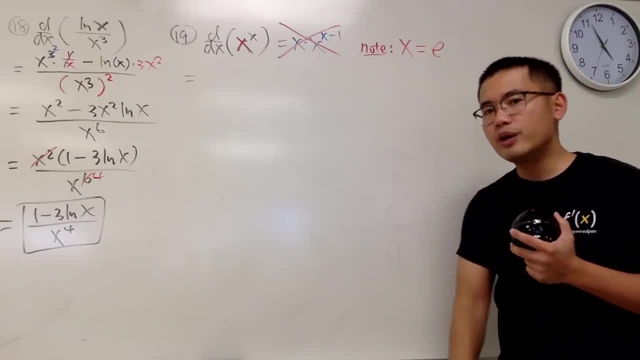 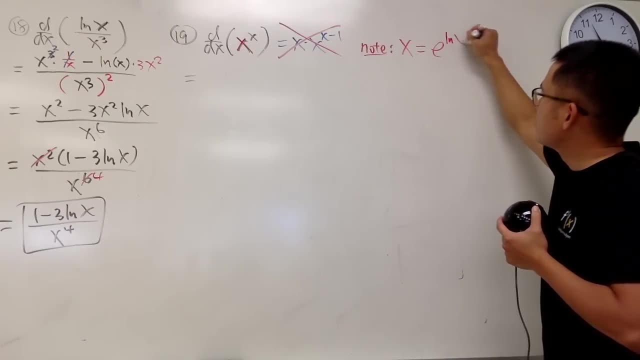 as I said, because we like to work with space E rather than any other base. And well, if I want to get back to x, I can just put E to the natural log of x power, because they cancel. You just get x back. 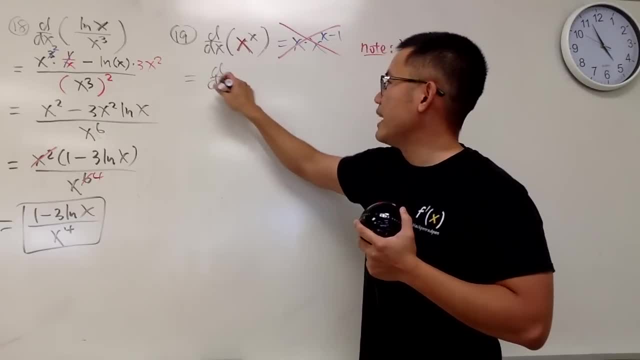 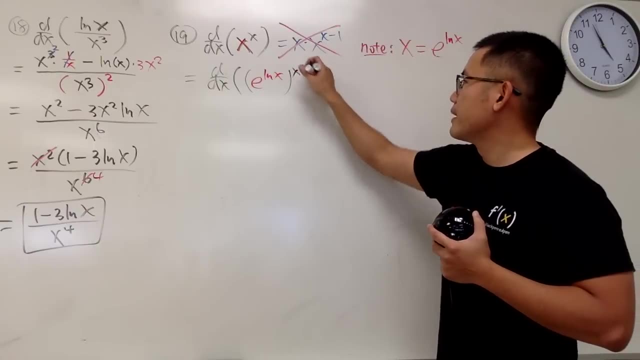 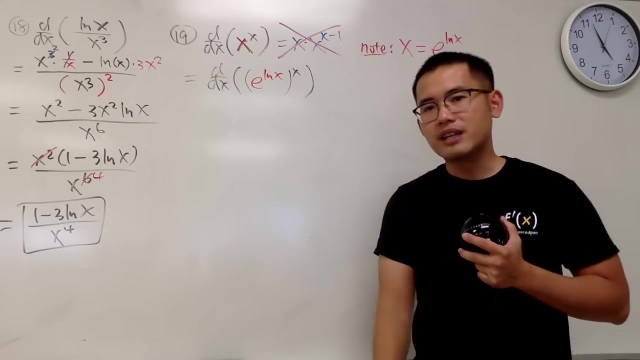 Now we'll just change this. We will be looking at E to the natural log of x and then raised to the x power, Right? Well, however, you see that this to the x power. we can just multiply the powers together. 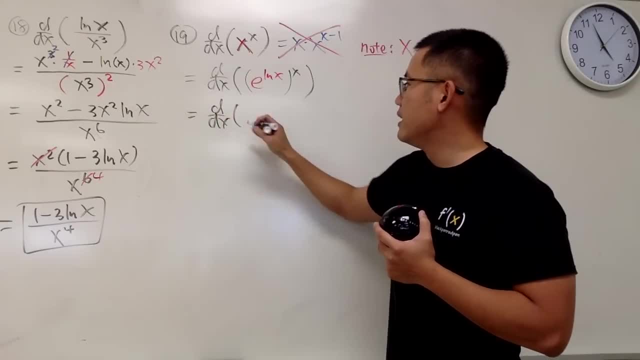 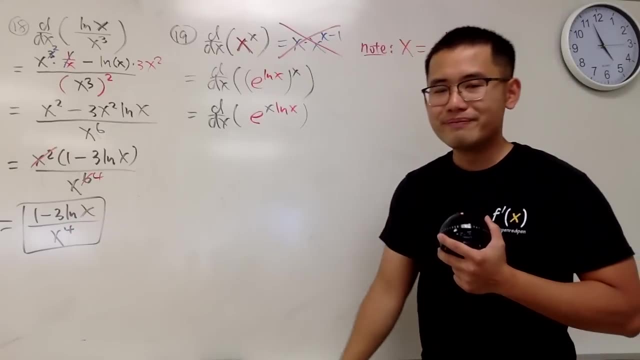 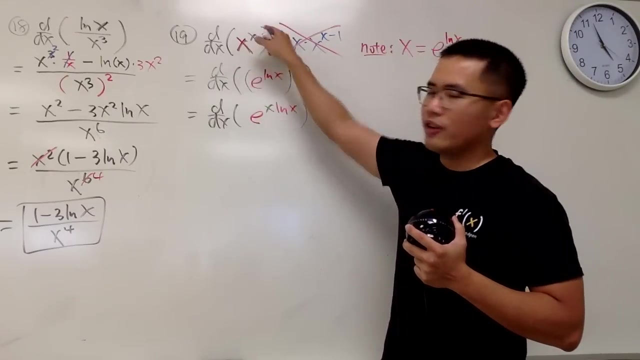 So we just have to differentiate E for the base, x times natural log of x for the power. So this is the idea. You want to work with space E whenever you have a function to a function power. This is one of the ways to do it. 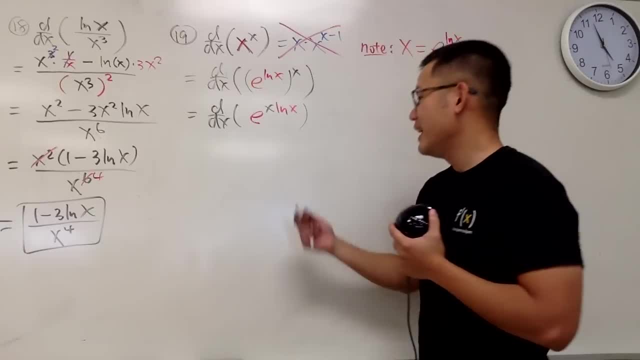 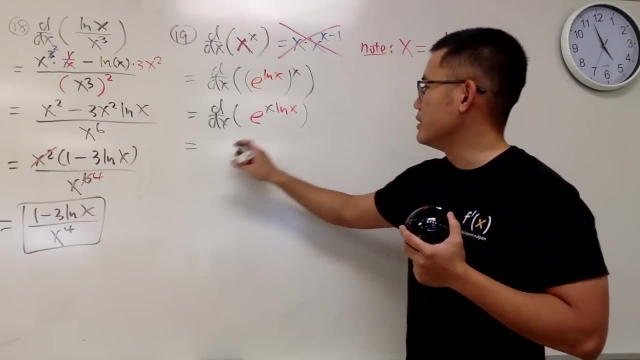 I will show you, guys, the implicit differentiation once we get to that part. Anyway, here we go To differentiate E to the something. first of all, just repeat that which is just E to the same thing: x. natural log of x. 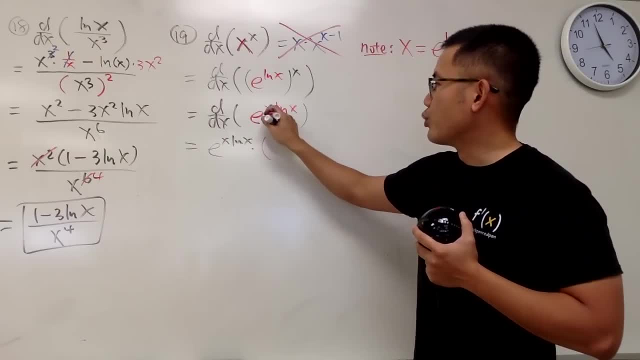 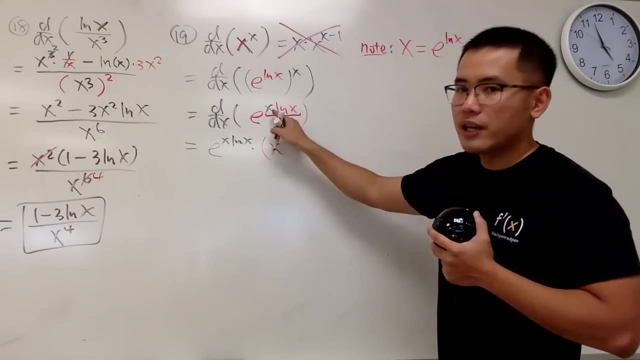 And then you multiply by the derivative of the input. because of the Chengdu right, The derivative of this. I will keep the x, keep the first function, and we multiply by the derivative of the second, The derivative of natural log of x. 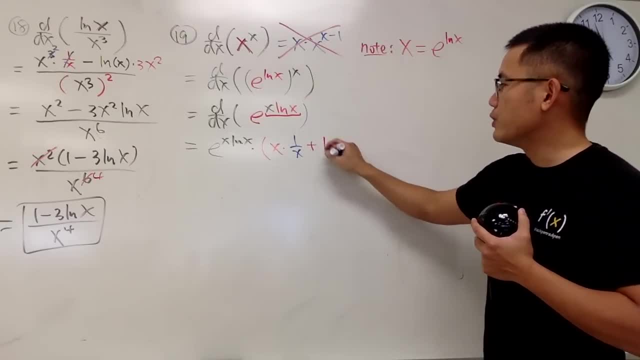 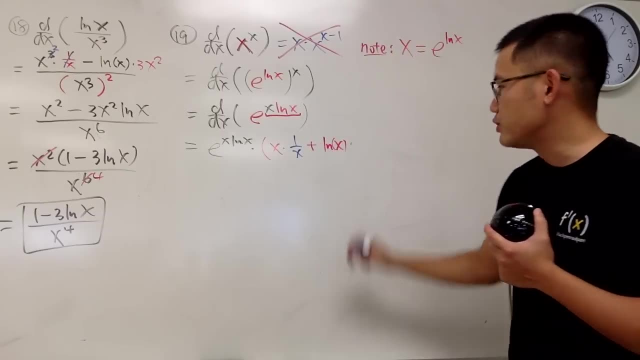 is just 1 of x. And then we add the second function, which is natural log of x times the derivative of the first. The derivative of x is just 1.. So we multiply by 1, like that. So that's pretty much the idea. 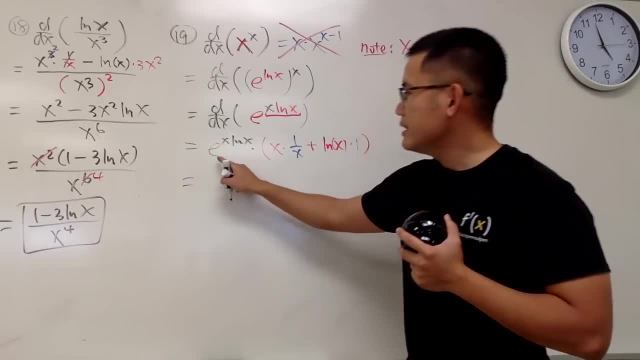 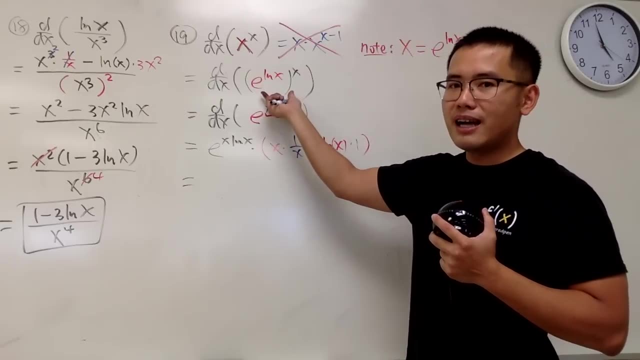 And now check this out: What's E to the x, to the natural log of x power? This is the same as that. yeah, Which is the same as that, Which is the same as x to the x. So all the way in the front. 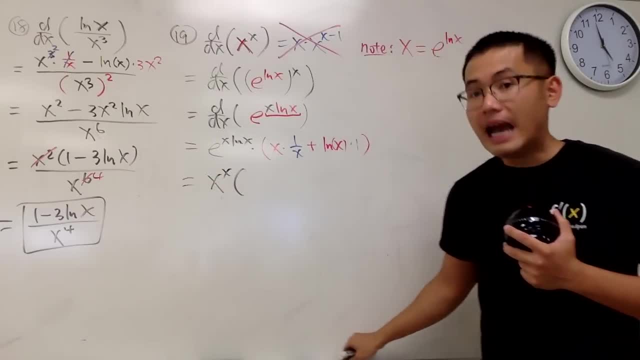 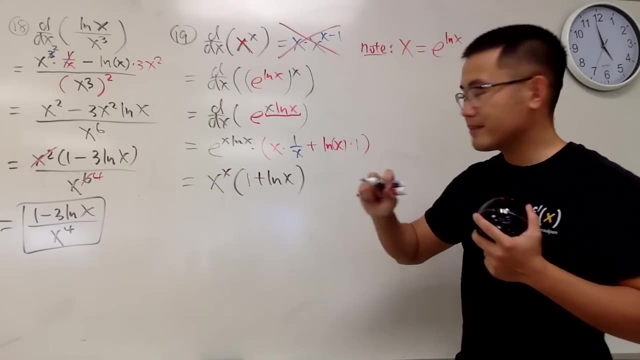 we have x to the x power And then x times 1 over. x, of course, is just 1.. And this right here is just natural log of x And we're done. That's it: x to the x times 1 plus. 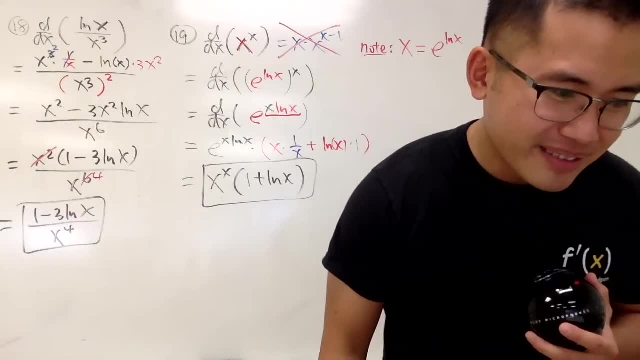 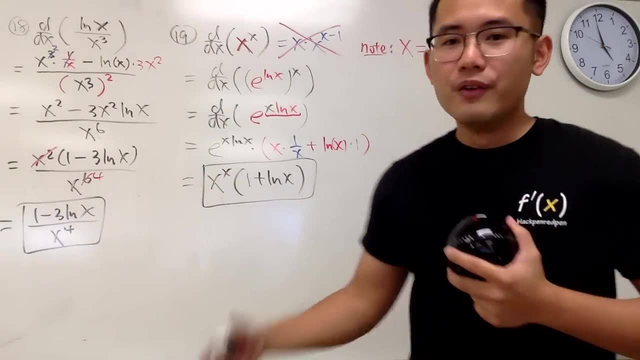 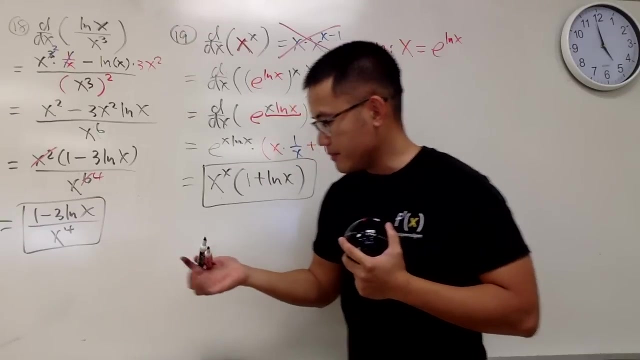 natural log of x. That is the answer. Pretty good, huh. And now, as I said, we are getting to the implicit differentiation part for question number 20 to 29.. I believe that's my setup for that. I know my hands are really dirty. 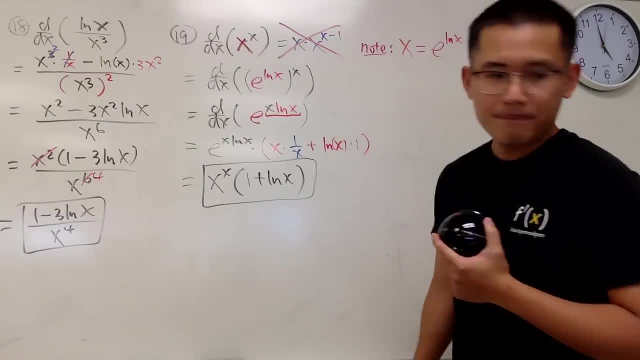 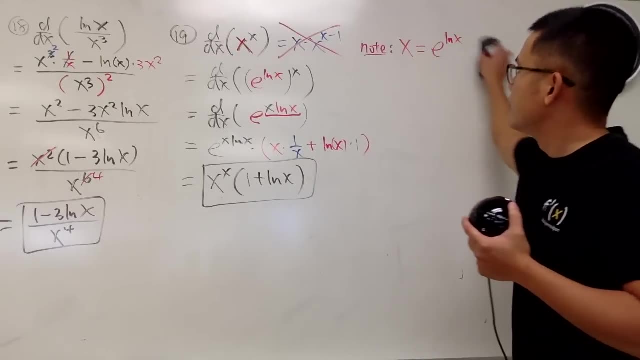 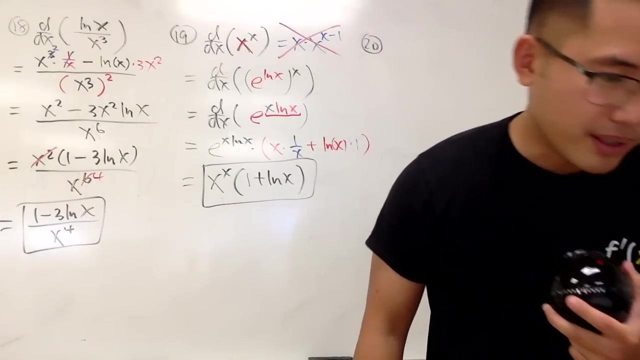 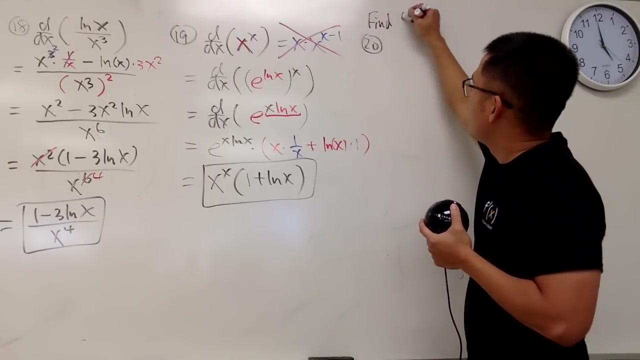 because all this is pretty dirty. So yeah, Let's see I shall be able to do it here, All right, Question number 20.. Okay, We have to find dy dx, right? So our goal is to find dy dx. 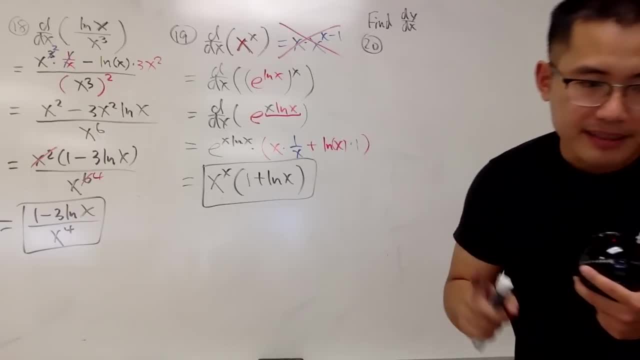 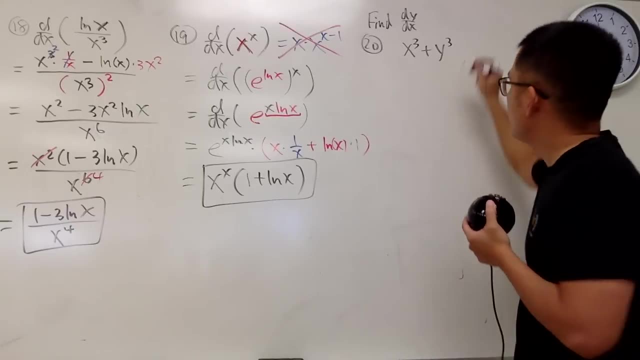 which is the derivative. But the problem is that the y is not by itself. We will have the equation x to the third power plus y to the third power And we have that equals. we have that equal to 6 times x times y. 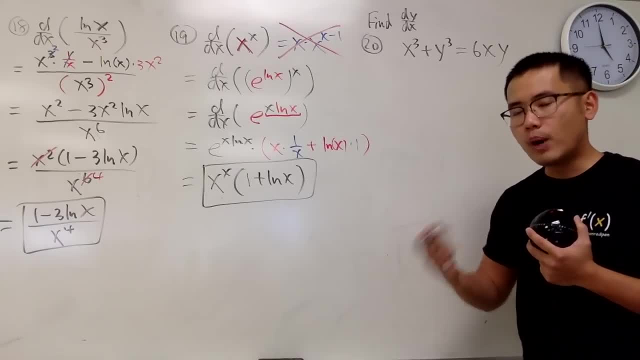 All right. So we are given this equation. The y is not by itself, But it's okay. This is how we can do it. Let me just put down d dx all the way in the front to tell people that we are differentiating. 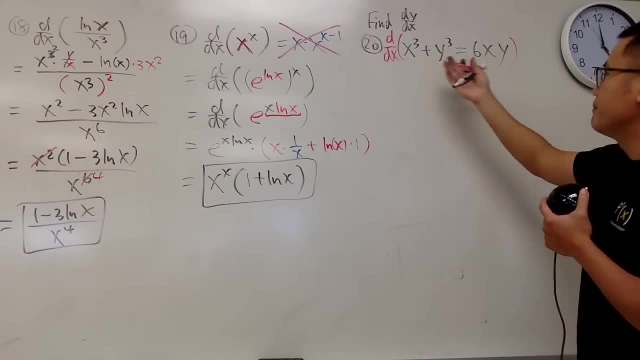 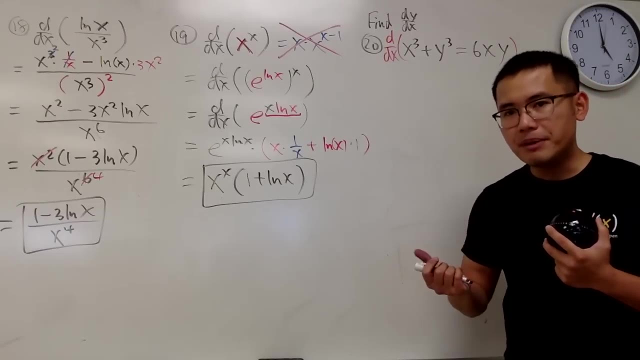 with respect to x. Right, And with that being said, that means y is a function of x And you have to do the following carefully. Anyway, here we go, Differentiating x to the third power. we get x to the third power. 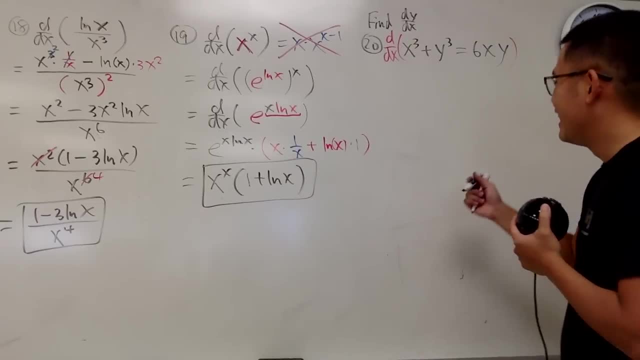 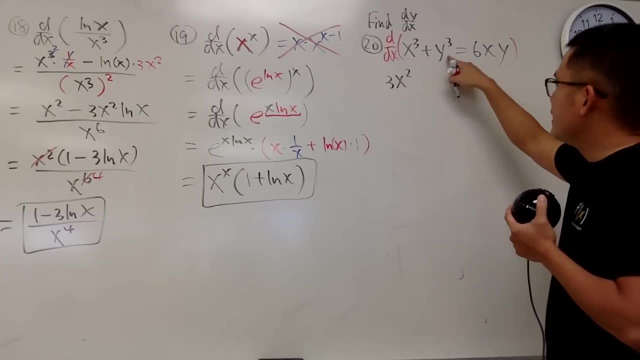 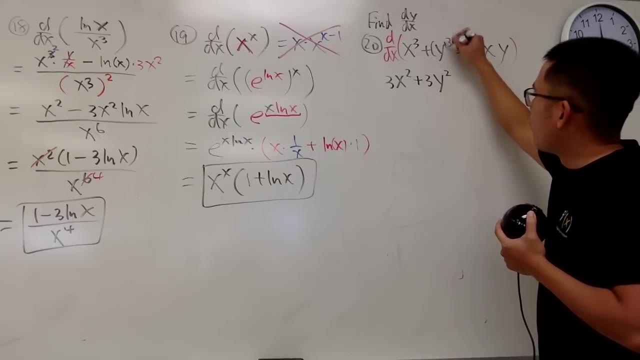 plus y to the third power, and that's it. Differentiating y to the third power, we get plus 3y square. But you know this is I say y to the third power. So we have this, And then 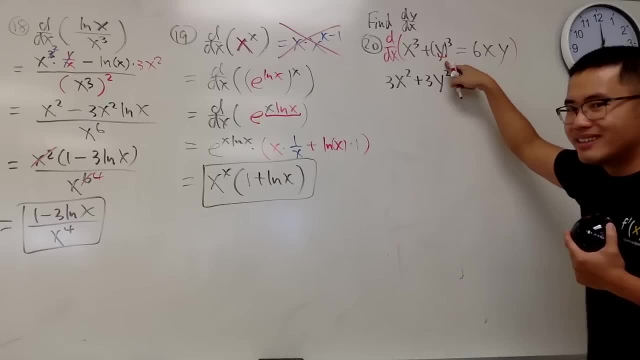 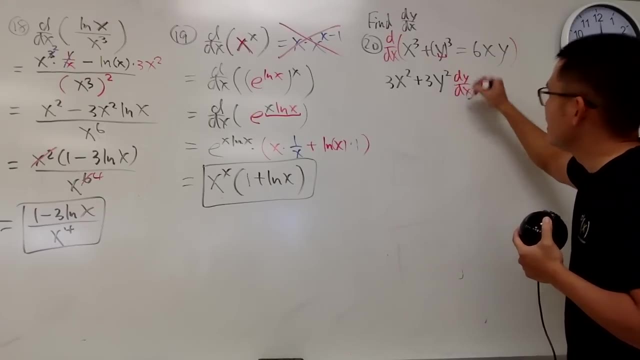 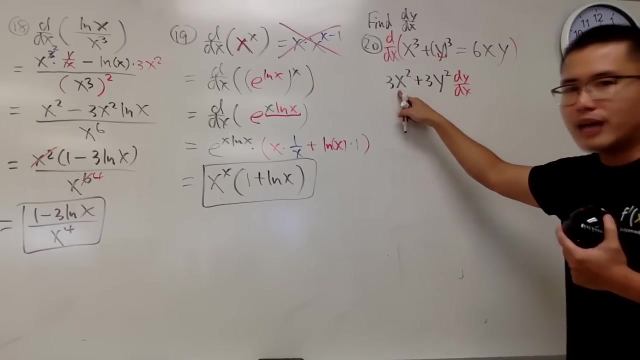 you look at inside, the derivative of y to the third power was 3y square. But since y is a function of x, we will have to multiply by dy dx. the derivative inside The derivative of y is dy dx And you might be wondering how come we didn't do that. 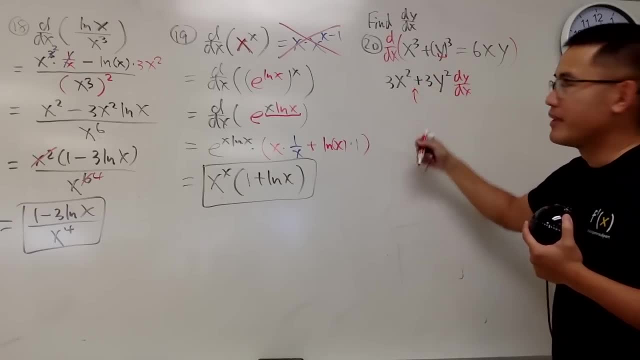 Well, if you would like, you can just think about it like this: x to the third power, so you have 3x squared and you should multiply by dx, dx, huh, Isn't it? Well, what's dx over dx? 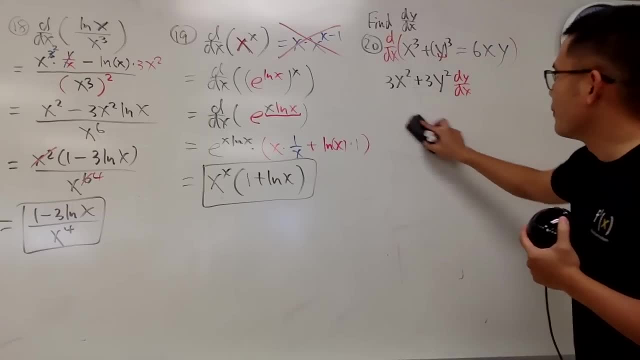 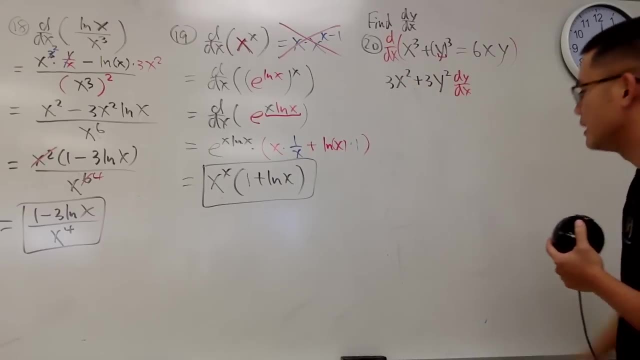 Just 1.. So you don't have to do that. So be really careful with this idea. So this is just that, but this will give you this right here, Right Now. for the right-hand side, this is 6x times y. 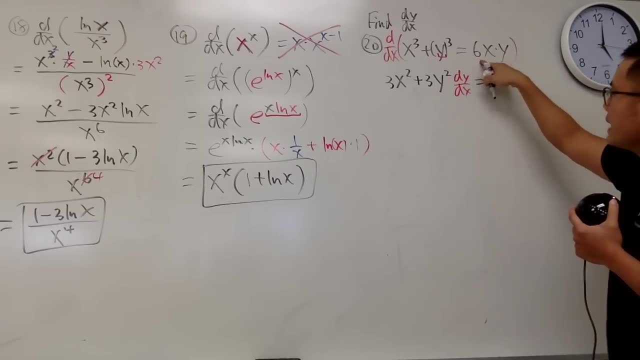 so let me just say this is the first function, that's the second Product rule in action. keep the first function, which is 6x, and multiply by the derivative of the second. The derivative of y is just dy, dx, And then we add the second function, which is y. 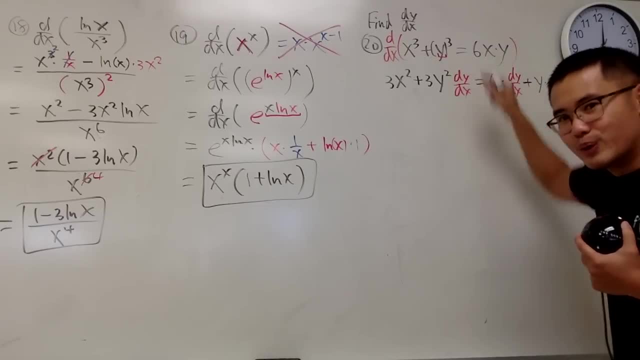 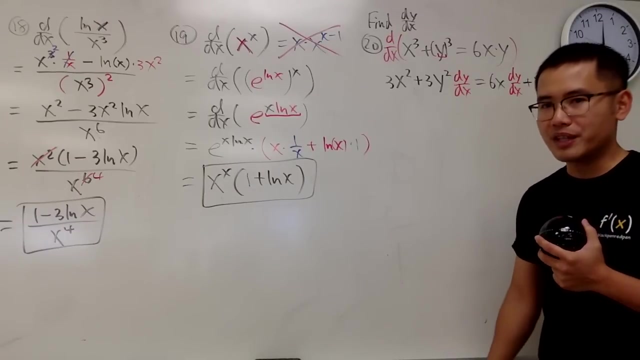 and we multiply by the derivative of 6x, which is just a 6.. Whew, My god. This, right here, is a write-off for the implicit differentiation. And now we have to isolate dy dx, because that is the derivative. 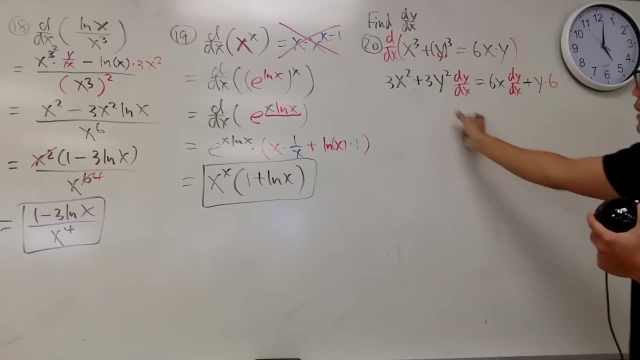 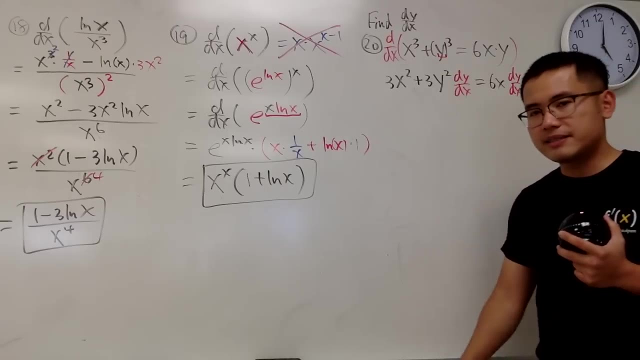 And to do so, well, I'm going to move this to the other side. I'm going to move this to the other side, right, Because I want to collect all the terms that have the dy dx, so we can factor out the dy dx. 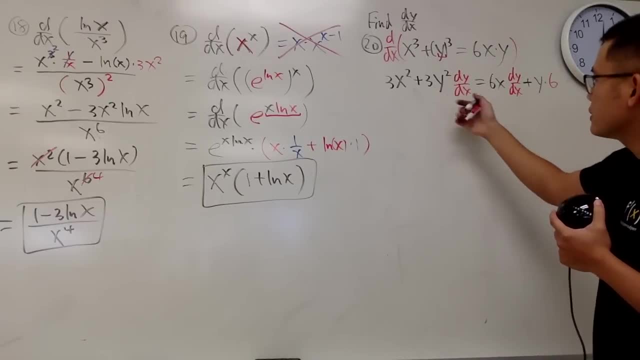 and then we can isolate that. Well, let me just write this down for you guys. I'm going to move this to the other side, but I will also factor the dy dx in the meantime, And when I factor it out, I would like to put the dy dx at the end. 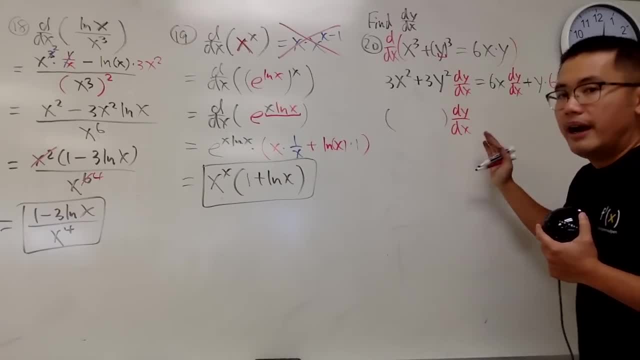 and then open the parentheses in the front. And the reason I want to put the dy dx at the end is that this right here, it's the object, it's the derivative. It looks similar to d dx, but d dx means to take the derivative right. 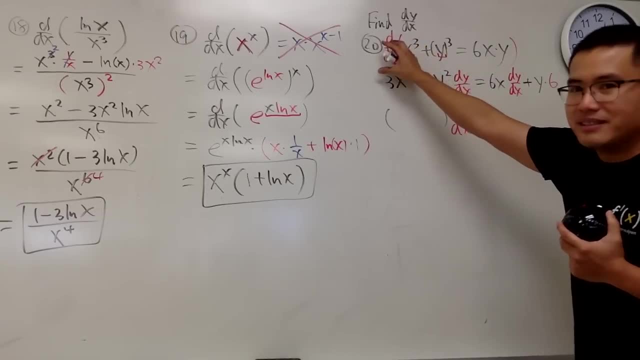 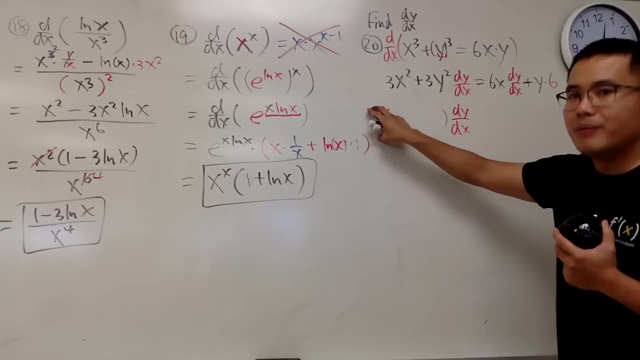 This is what we are trying to find already. this is the things that you have to do, the operator. So I prefer to have this at the end of the parentheses rather than in the front, because otherwise it might look like we still have to differentiate, which is not correct. 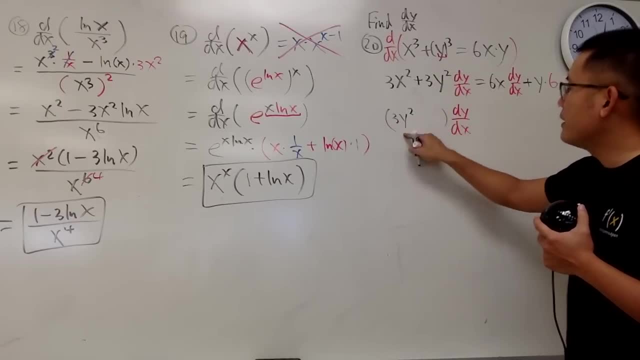 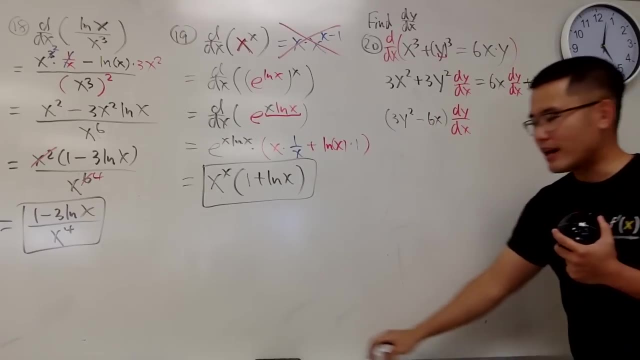 Anyway, this right here was positive: 3y squared. I brought this to the other side so it would be negative with a 6x And we factor out the dy dx at the end. right there. already This is equal to 6y. 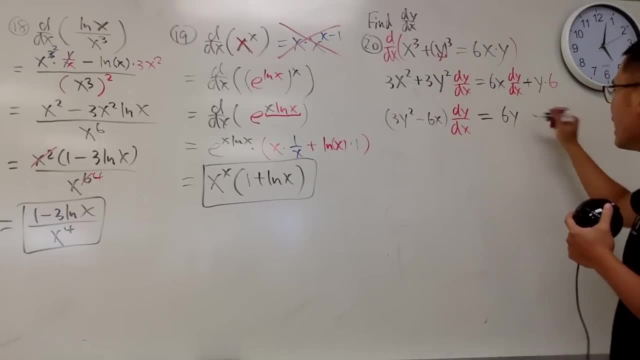 so let's keep the positive first, and then we bring this to the other side becomes negative 3x squared Like that. So that's pretty much it, huh. And then of course we can divide. So we see that dy dx equals. 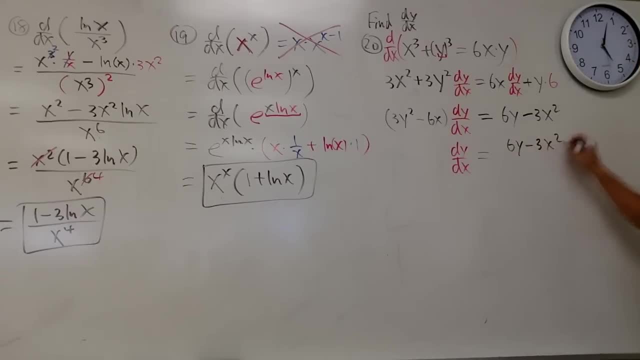 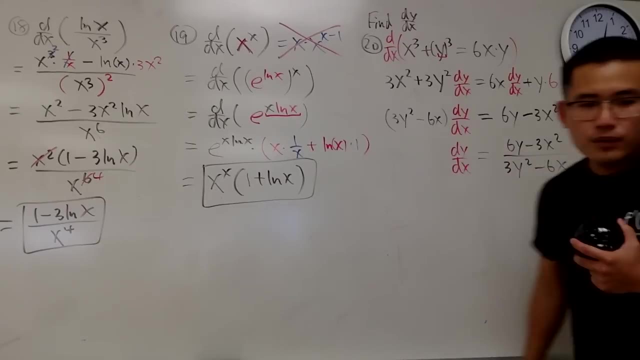 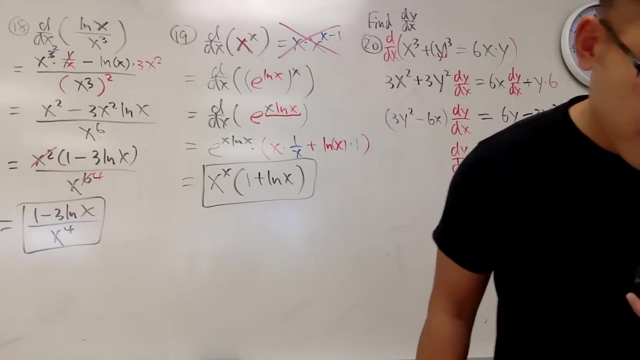 here we have 6y minus 3x squared and over right here we have 3y squared minus 6x. Well, we can actually read this: as we reduce this a little bit- and I'm just checking that- my answer key is the jet. 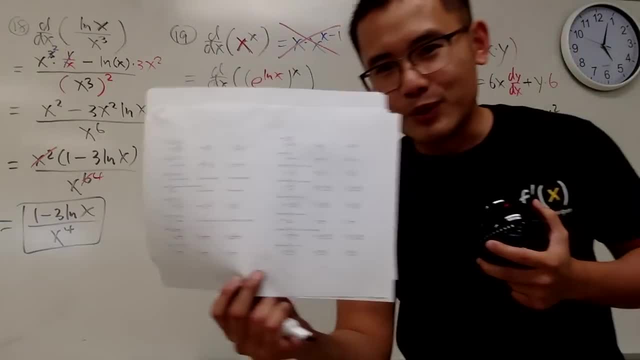 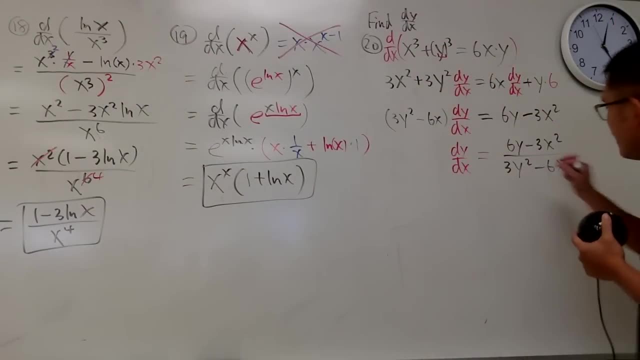 Yes, it's good. my answer key is good Because, as I said, I come up with all the answer key. no, I come up with all the answer choices myself. I just want to make sure that I didn't mistype anything, or so. 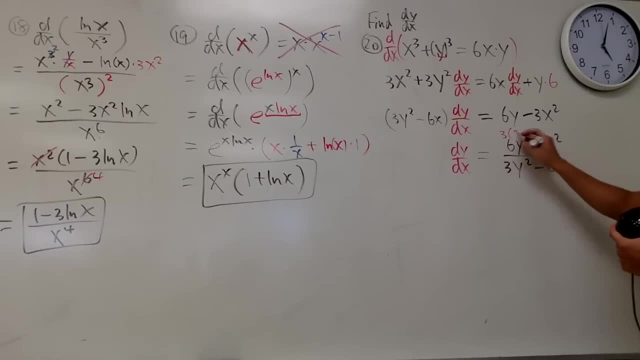 Anyway, we can factor out our 3 on the top. So here we have 2y minus x squared, and we can factor out our 3 on the bottom as well. so this is y squared minus 2x. Cancel, cancel and in the end, 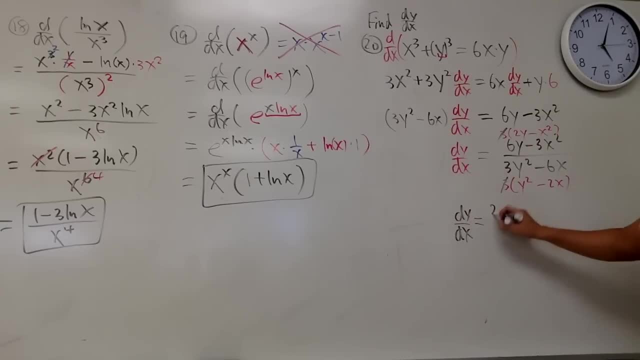 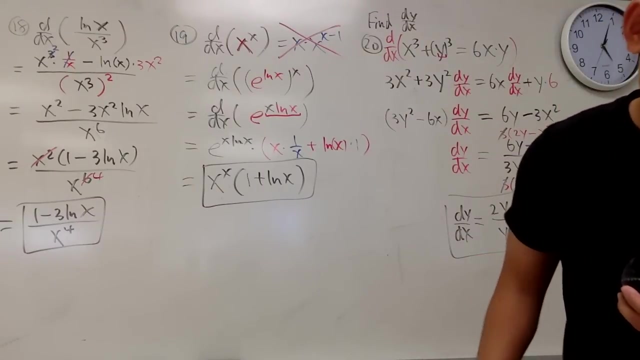 dy dx equals 2y minus x squared over y squared minus 2x. I just noticed: if you differentiate this, you get that. if you differentiate that, you get this. I don't know coincidence. Yeah, that's it. Oh, interesting enough. 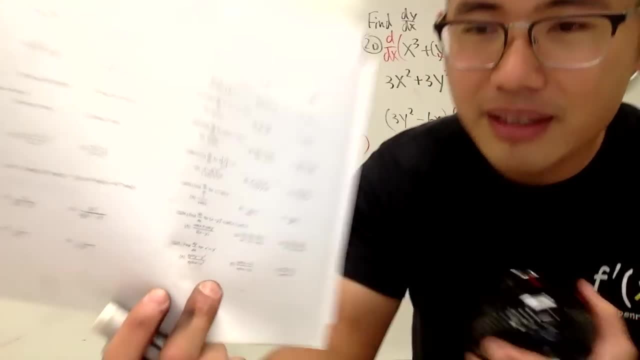 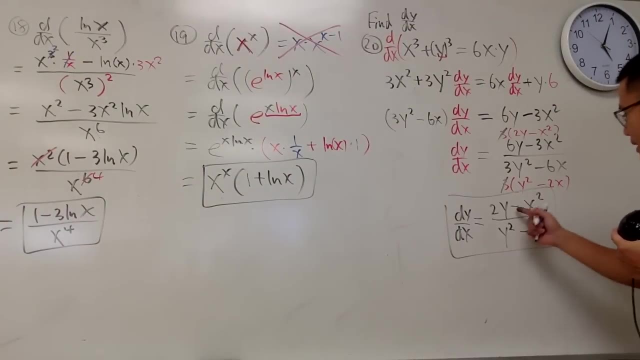 I actually have this right here, right number 20, you can see it right here. I have the answer key backwards On the answer key, the reason I did this. I just put the x first and then factor it out. So in fact, this right here is the same as saying: 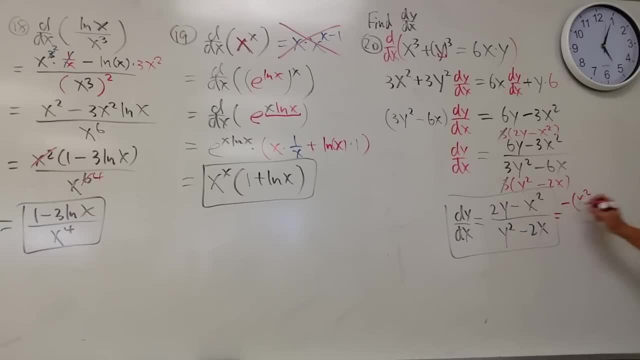 we can factor out negative and then put the x squared minus 2y and then over negative, and we'll put this first, Which is 2x minus y squared, And cancel the negative. And it depends how you move the things around. 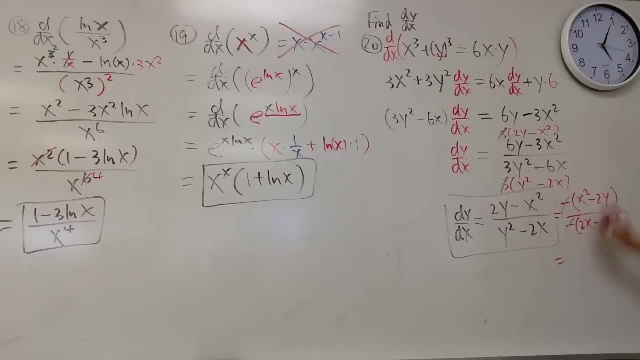 So it's either this one or this one, And you should be able to see that the answers are equivalent. So that's just algebra part that you have to know. So this and that are the same Right? So yeah. 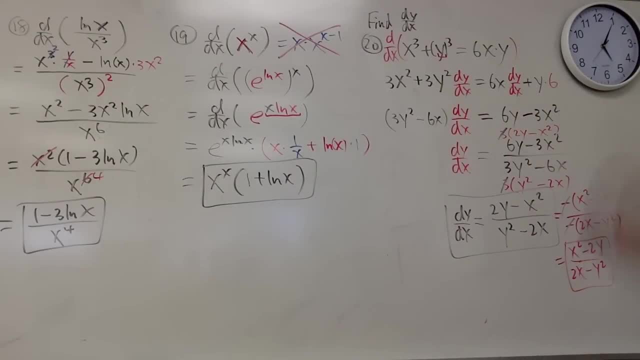 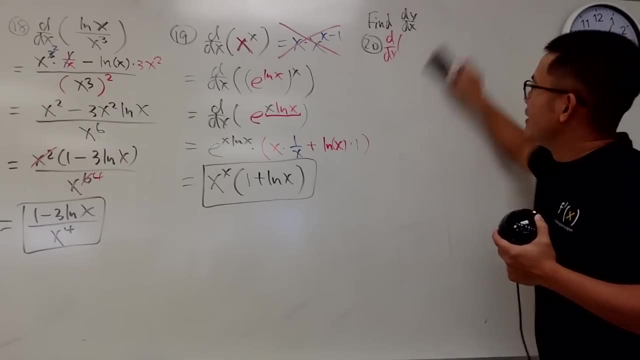 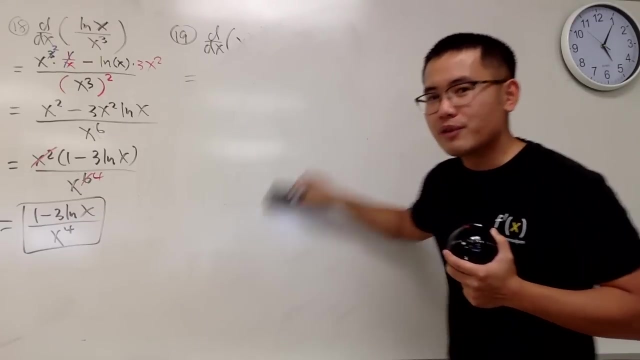 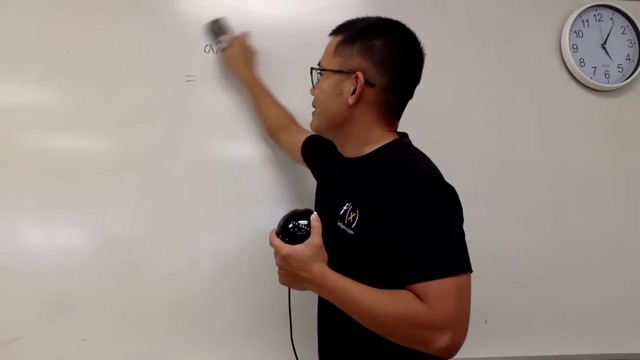 Just like this. So take a look, take a look, take a look. All right, I was expecting to, I think, to do 100 derivatives will take longer to do compared to 100 integrals, Because it's just like so many things I have to go through. 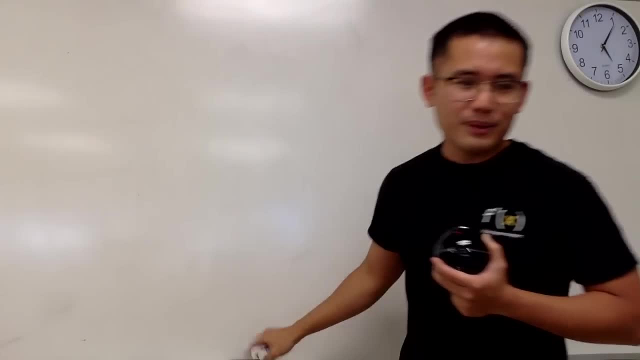 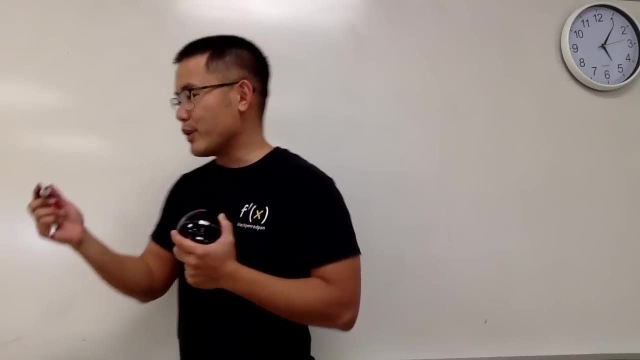 I don't know, man, I don't know which one will take me longer, I don't know. Anyway, Next one, Another implicit differentiation. I will just write down the equation for you guys, though. So here we have number 21.. 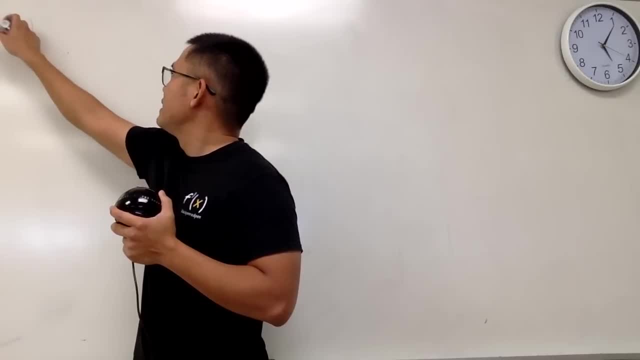 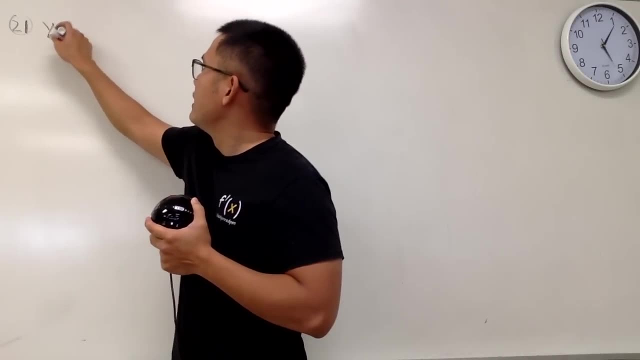 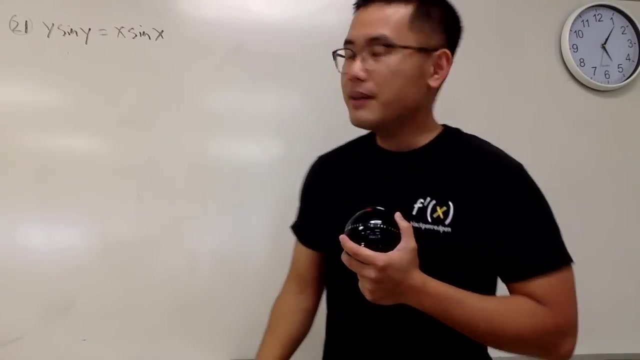 Should I retire this marker? I hope not. Good job, You can still work. Okay, We have y sine y equals x Sine x. All right, Okay, Why it's not isolated And in fact you cannot isolate it? 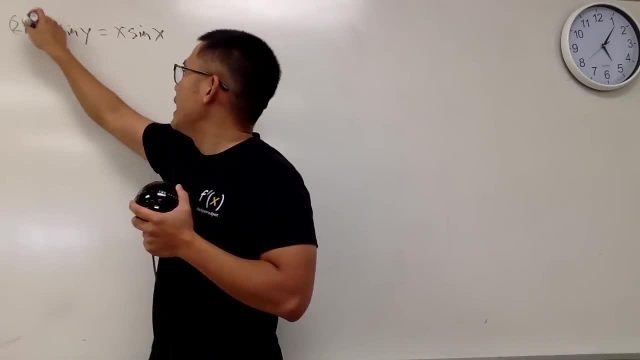 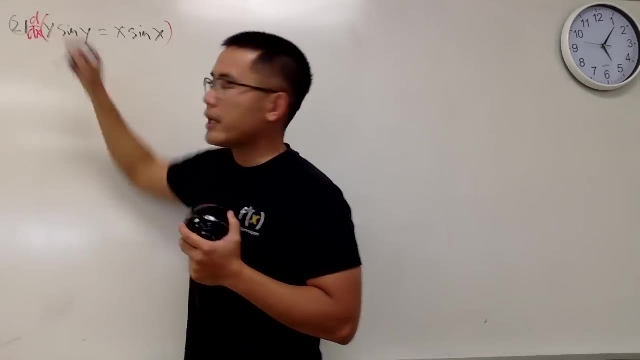 In fact, you cannot isolate y in this situation. It's okay, Just go ahead, Do d dx. Implicit differentiation. Here we go. This, right here, requires the product rule, So I will keep the first function Times d derivative to the second. 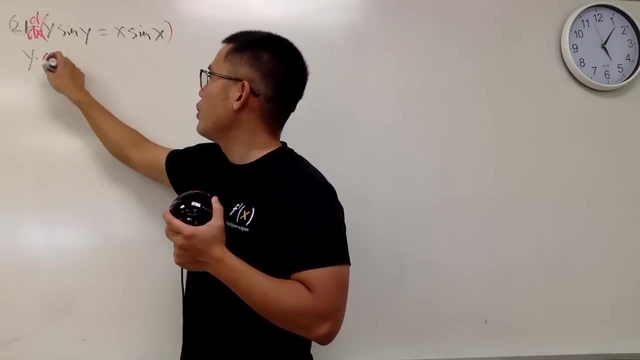 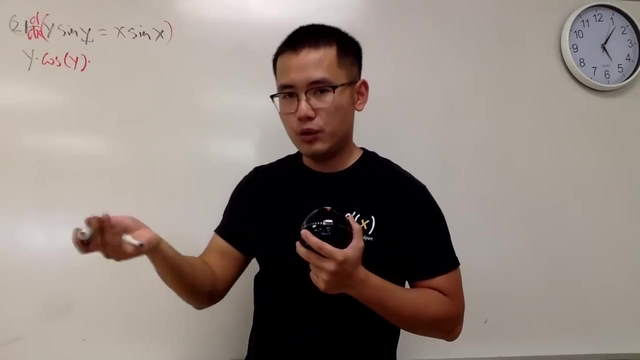 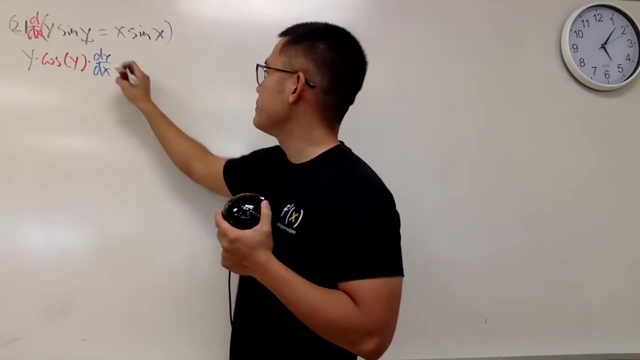 Derivative of sine of something is cosine of the input, And then the input is y. So we have to multiply by dy, dx, Because that's the derivative of y And this is the chain rule. And then we have to add the second function, which is sine y. 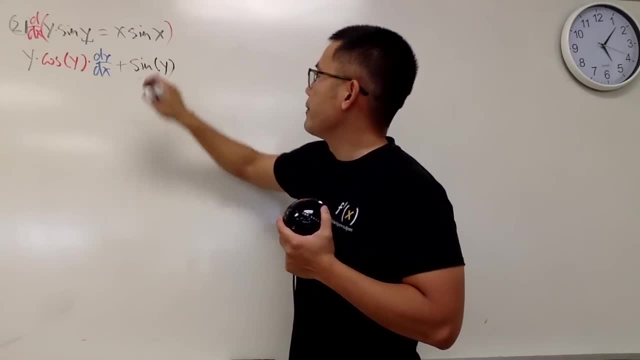 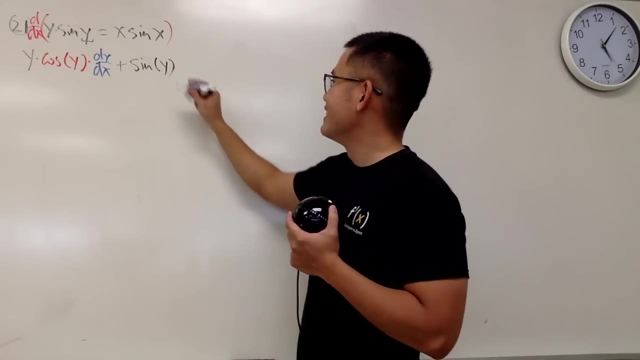 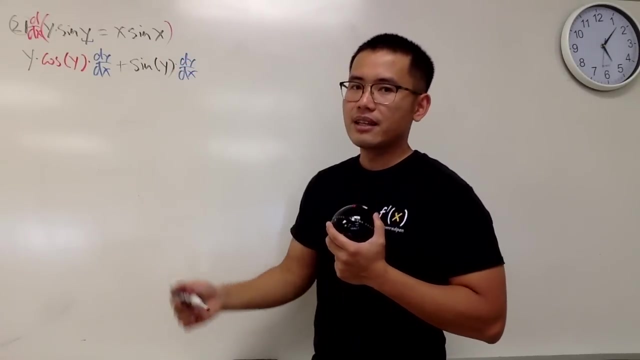 All right. Second function is sine y. So I just put down sine of y And we multiply by d derivative of the first d derivative of y is dy dx. So we multiply by dy dx, like that. So this is the left-hand side. 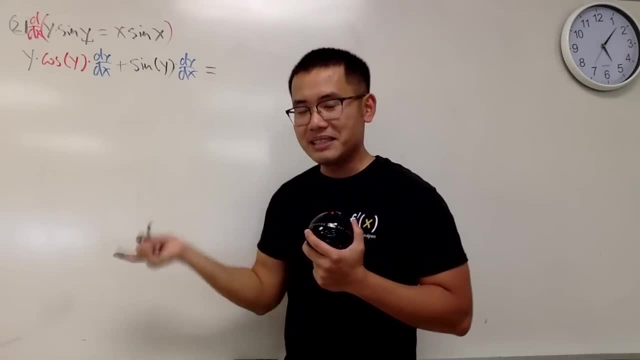 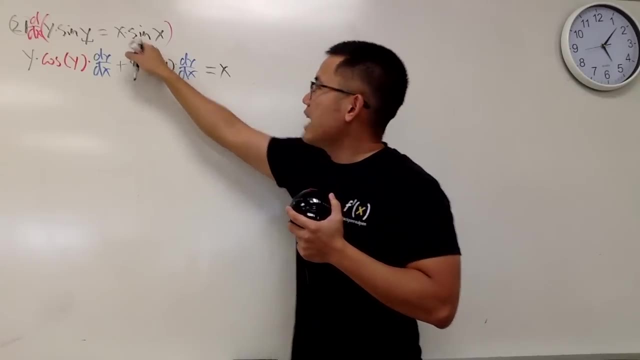 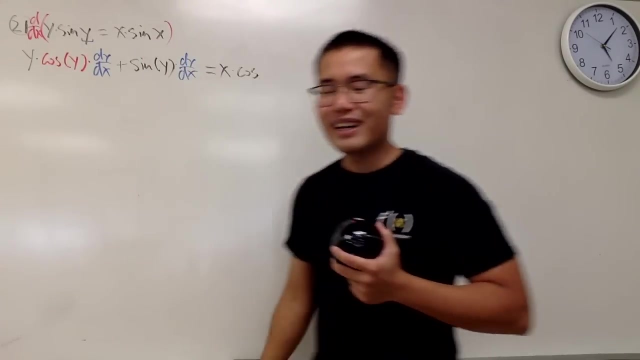 Now for the right-hand side. same thing, But with x instead of y. Product rule again: Keep the first function Times d derivative of the second Derivative of sine is just cosine And notice that the input is x And we have to differentiate that with respect to x. 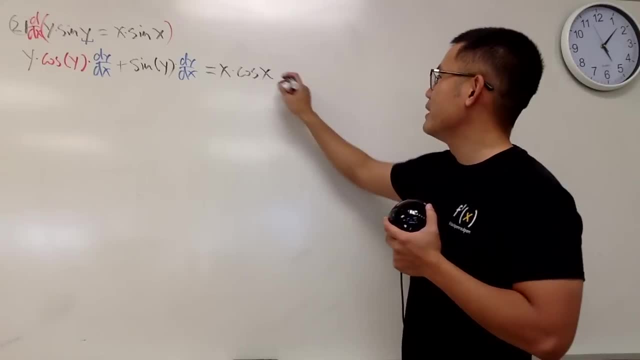 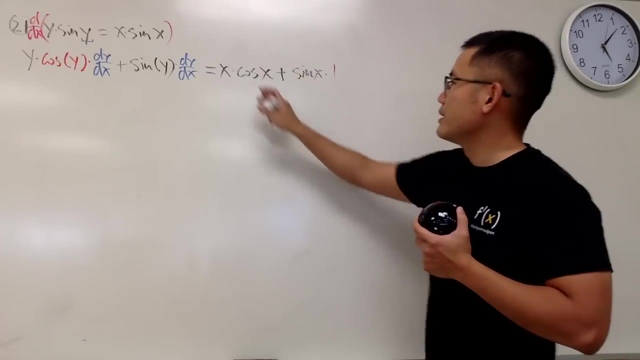 So it's just cosine x like this And we're done for that. Okay, And then we add the second function, which is sine x, And we multiply by d derivative of the first, which is 1.. So I should also put down the cosine x in red. 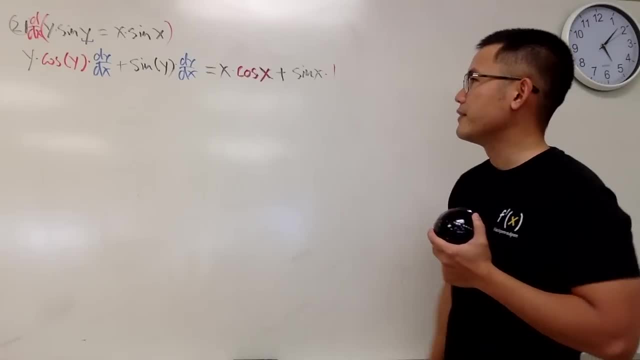 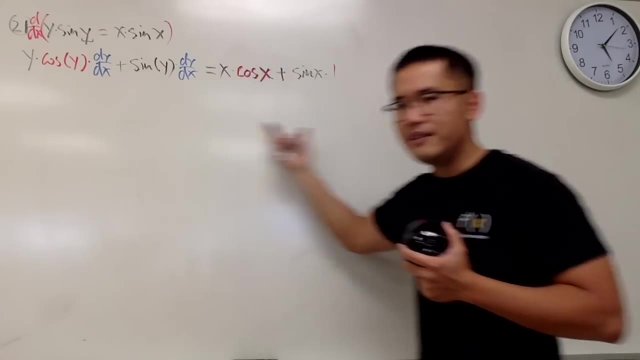 First times the derivative of the second plus the second times the derivative of the first. This is it, And now we can just factor out the dy dx on the left-hand side and then divide it. That's pretty much it, right, So we'll do it in one step. 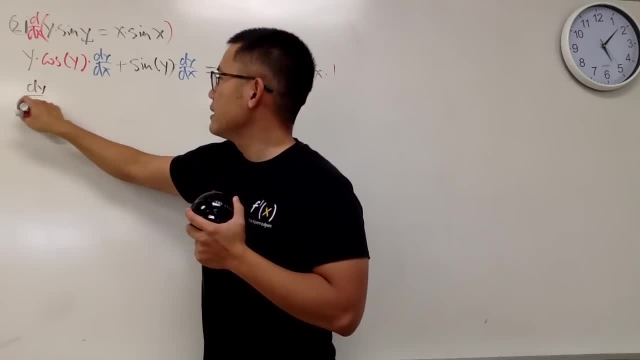 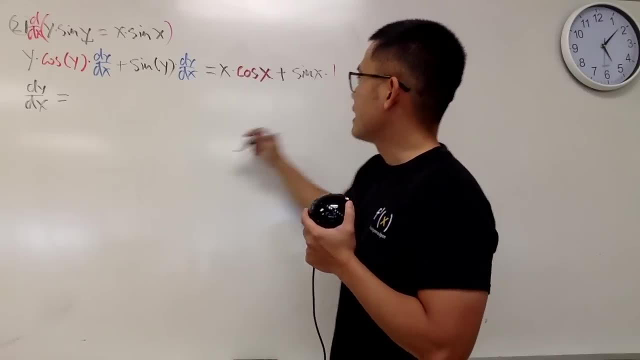 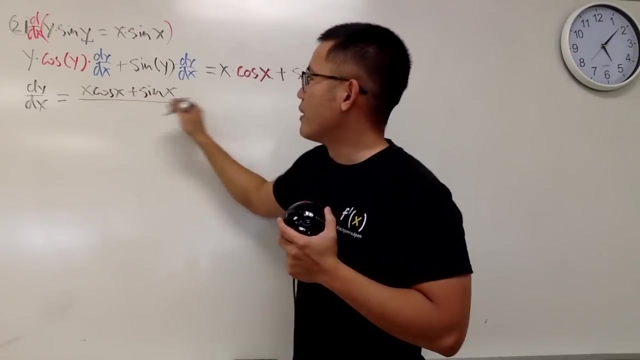 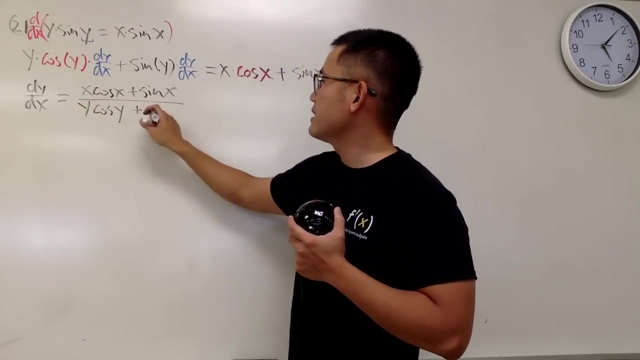 Because we see that this is just dy dx. we can just have this and that being factored in the parentheses. This is the right-hand side, So we have x- cosine x plus sine x over this and that in the denominator Namely y- cosine y plus sine y. 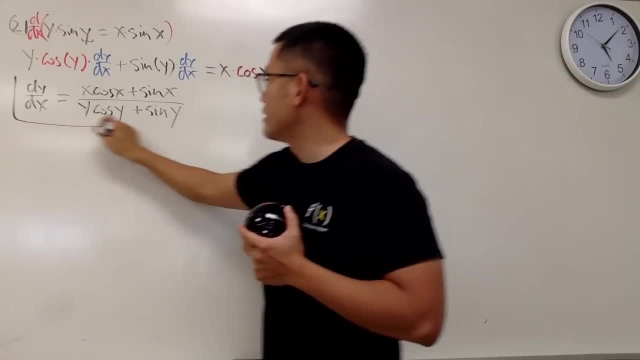 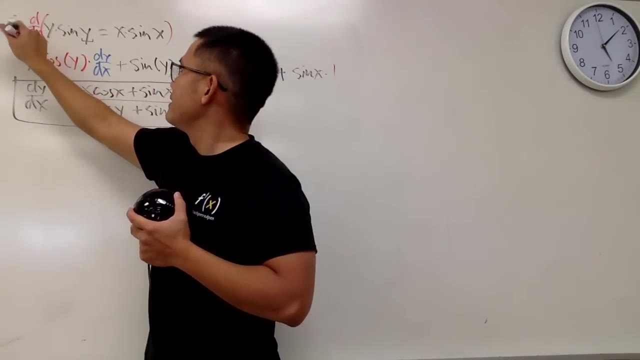 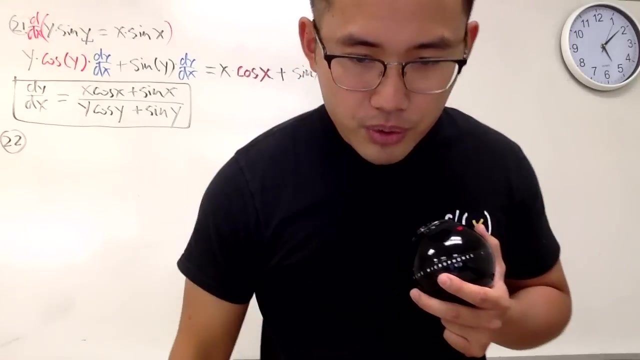 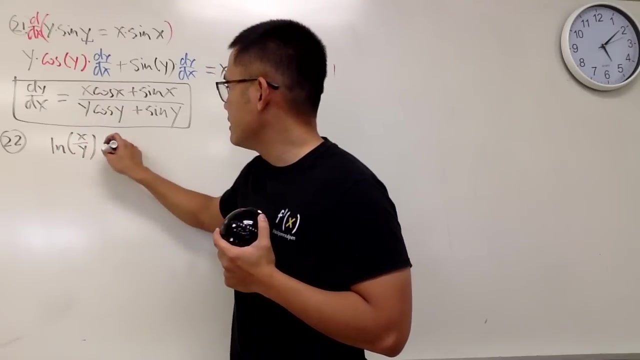 And we are done This right. here is the answer, And that was number 21.. And this is number 21.. All right, Number 22.. Here we are going to differentiate natural log of x over y, And this is equal to e to the x, y to the third power. 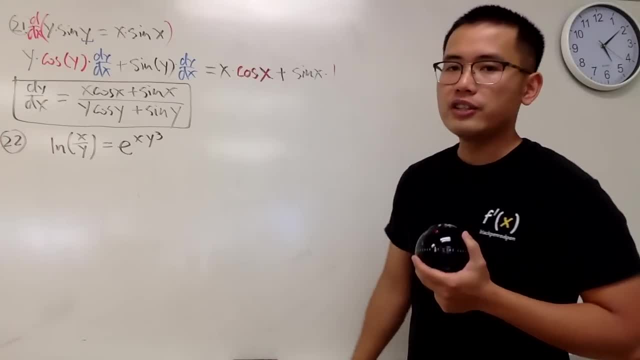 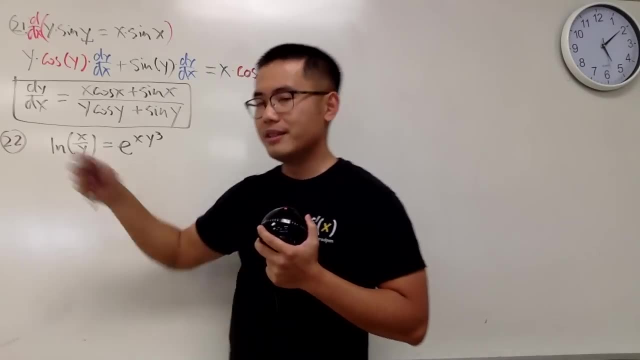 Like that. Okay, So implicit differentiation. But before we do anything like that, notice that we have a natural log of x over y. The truth is, we can break this down. We can write this as natural log of x minus natural log of y. 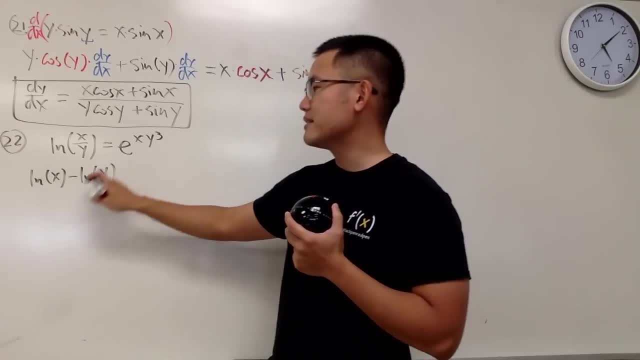 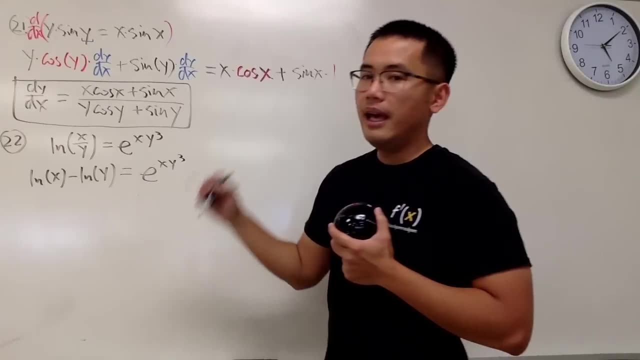 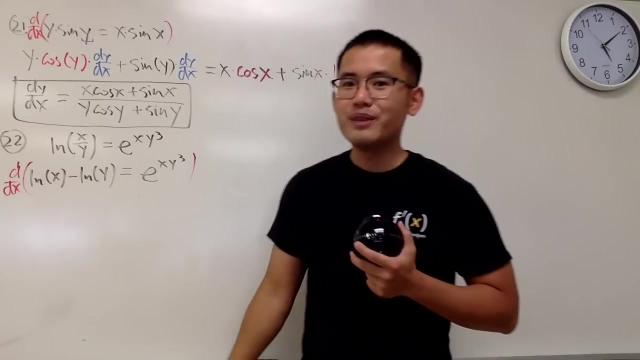 So that we can just differentiate the first and then minus the derivative of the second. All right, And of course this is just the algebra. We'll just write down the rest. And here we will just put down d, dx, to simplify, to signify that we are differentiating with respect to x. 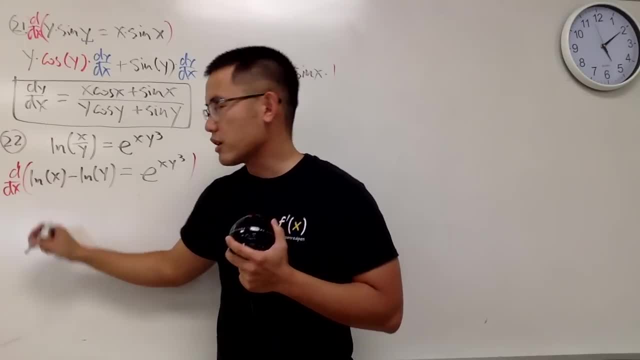 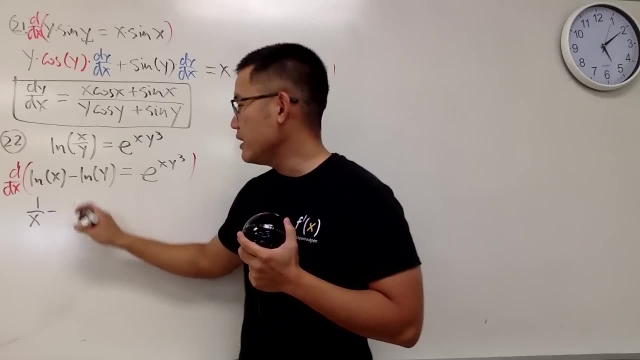 Here we go. Derivative of natural log of x is just 1 over y. It's just 1 over x. That's it Minus. the derivative of natural log of y is 1 over y, But the inside is y. 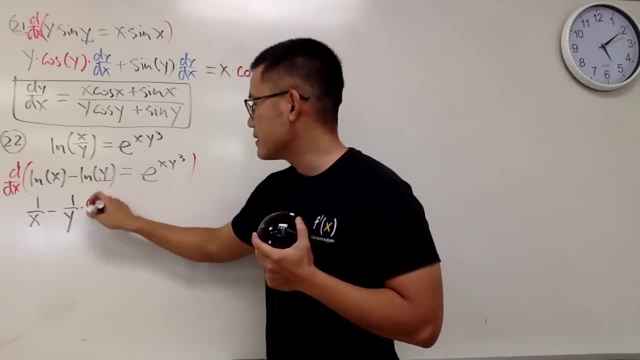 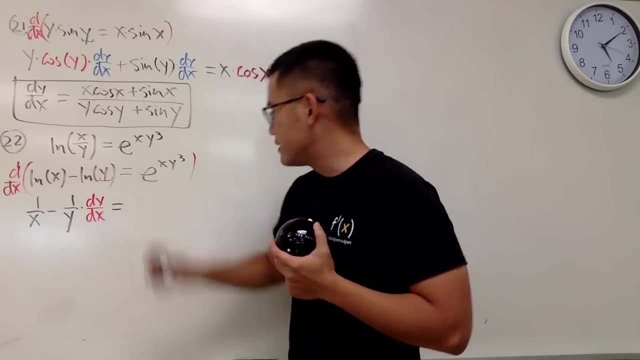 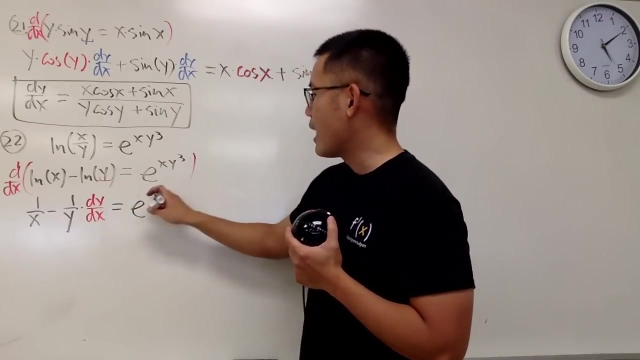 The derivative of y with respect to x is dy dx. This is how we squeeze out the dy dx Equals. here we have the derivative of this. Well, e to the whatever. you just repeat e to that whatever, xy to the third power. 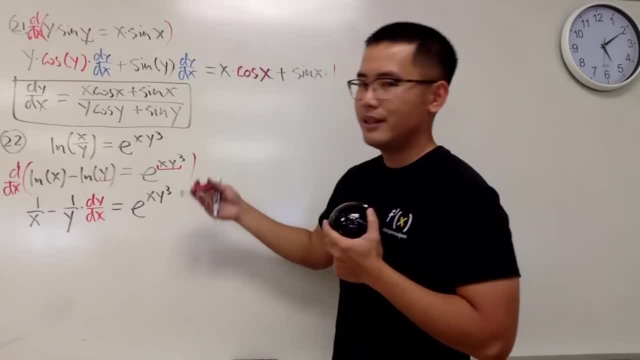 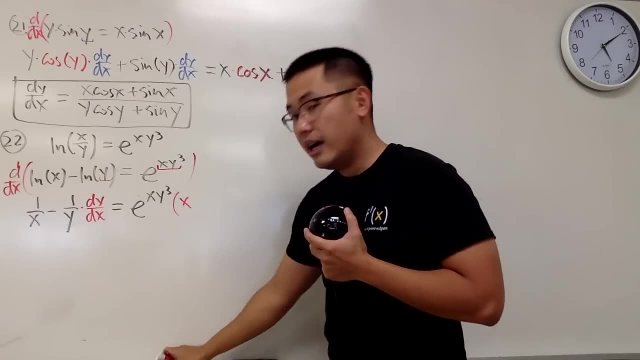 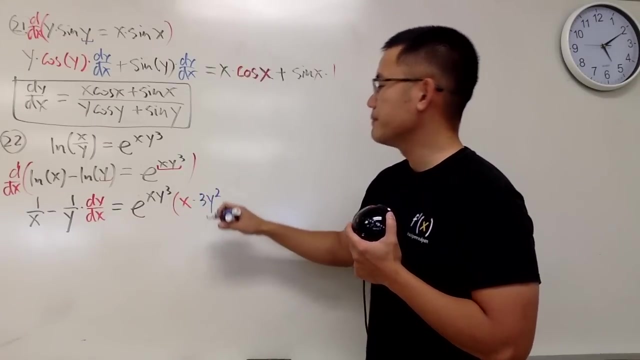 And now we differentiate the power. Yes, we do the product rule. This is x times that, Right. So the first function is x And we multiply by the derivative of the second Derivative of y to the third power, we get 3y squared. 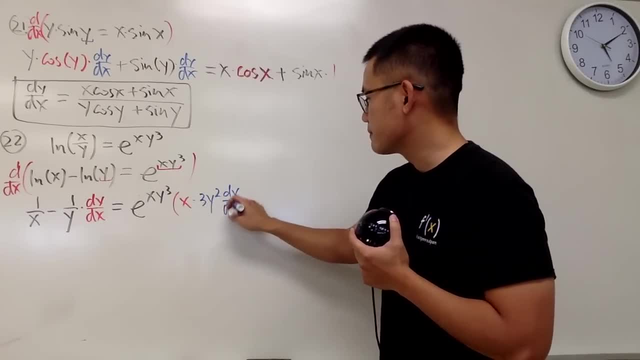 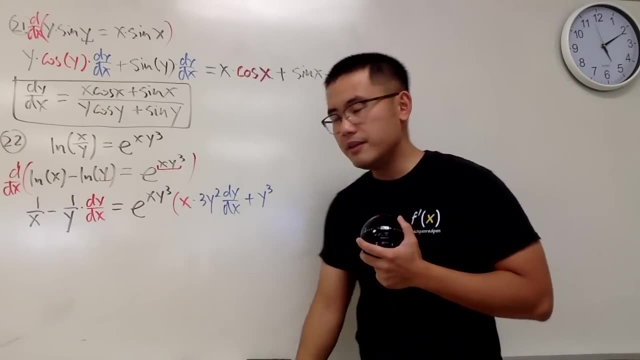 And you know the DO. We have to have the dy, dx, And then we add the second function, which is y, to the third power. Times the derivative of y to the third power, We get the derivative of dx, which is just 1.. 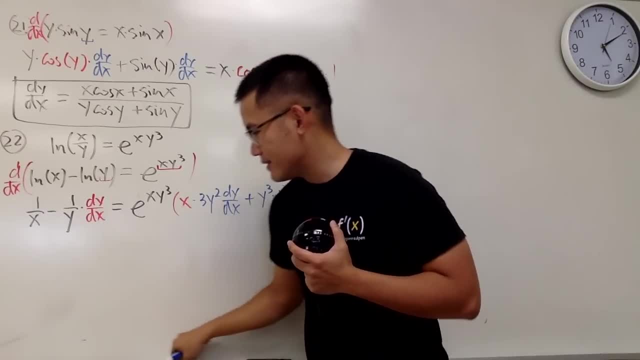 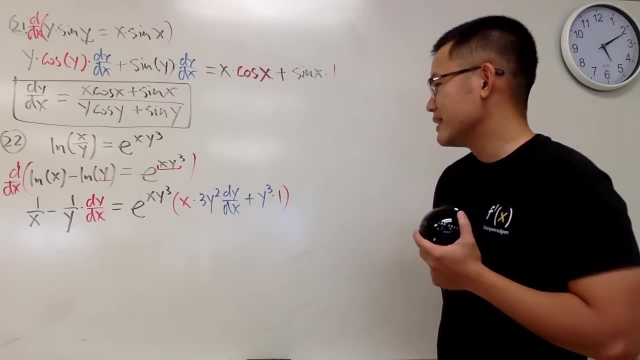 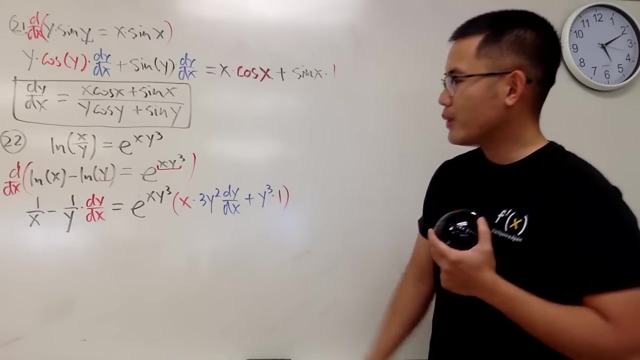 So this, right here, is what we have, Well. well, let's see what we can do with all that. This is not. this is man. I want to simplify this. Well, we have a fraction with x and y, The x here and y here for the denominators. 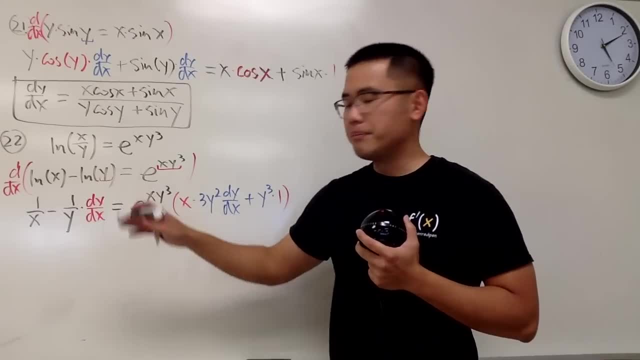 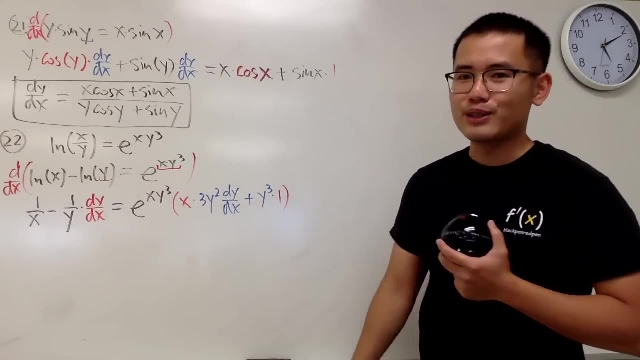 I think it's a good idea to just multiply out Everything by x, y, so that we don't have to deal with the complex fractions later on. So we'll do that And perhaps I'll just put down this in blue. Okay. 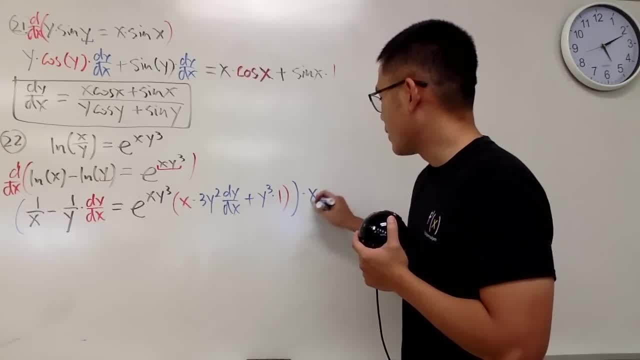 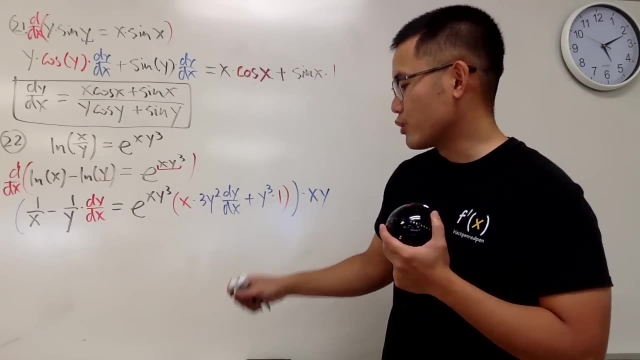 So we are going to multiply everybody by x- y. So again, the point is so that we don't need to worry about the common denominator, We don't need to worry about the complex fractions later on. All right, x y times 1 over x. 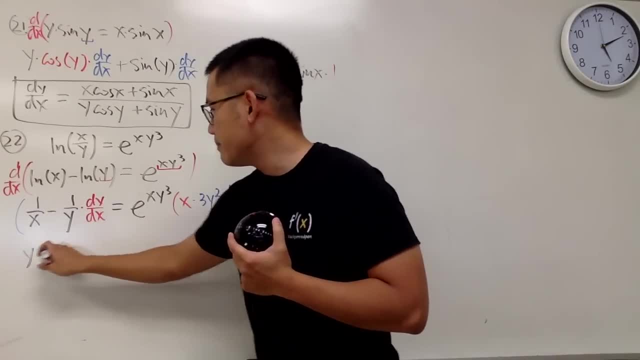 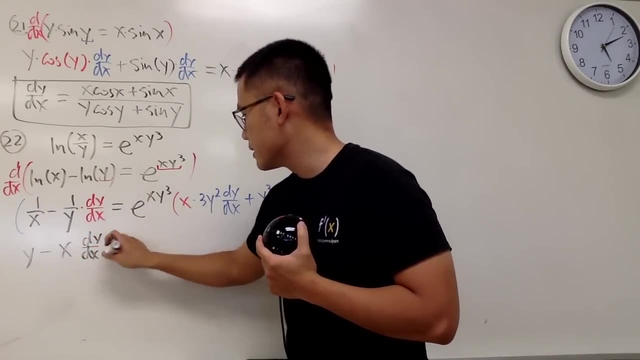 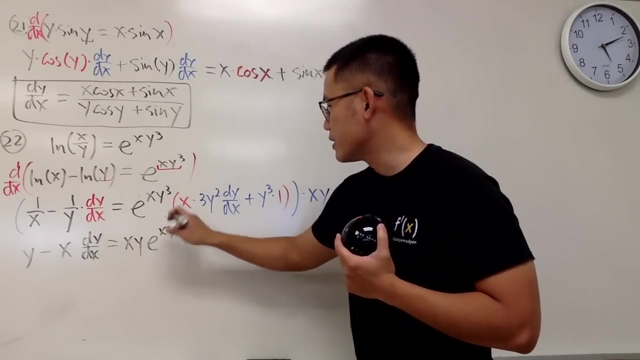 We get y, And then minus x, y times 1 over y, We get x. And this is still dy dx, And perhaps I'll just put down x, y right here. So we have x, y, e to the x, y to the third power. 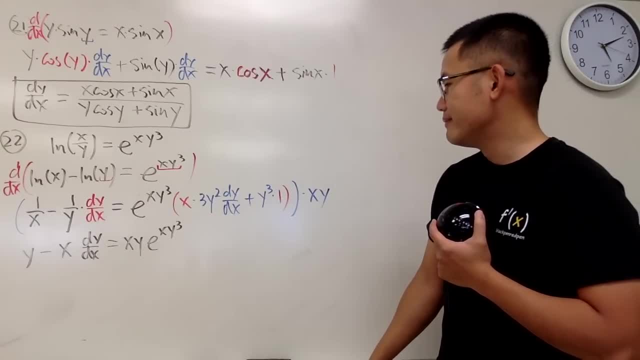 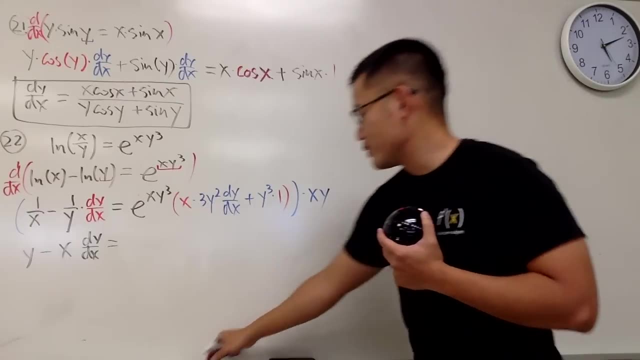 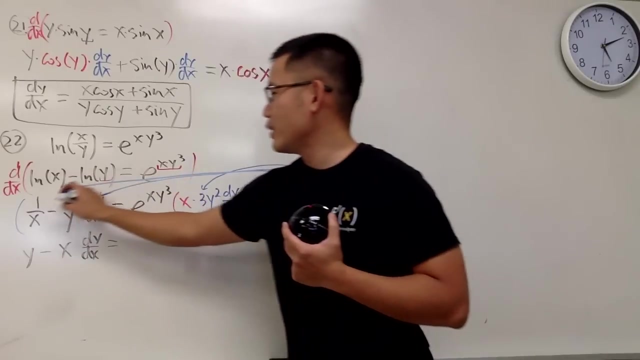 And then let's also multiply everything out right here. So check this out. Okay, Let's just do this thing backwards. So it's this times that We did this times this already. Man draw the arrows is kind of fun. We did this part already. 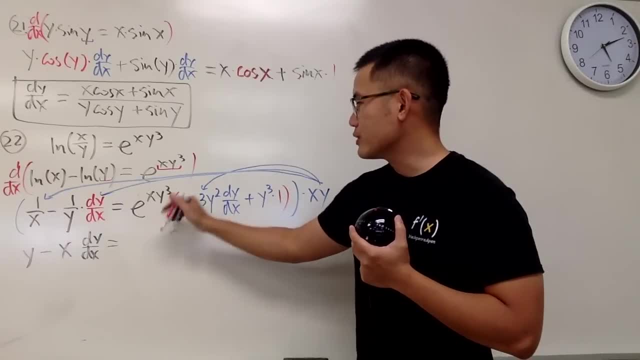 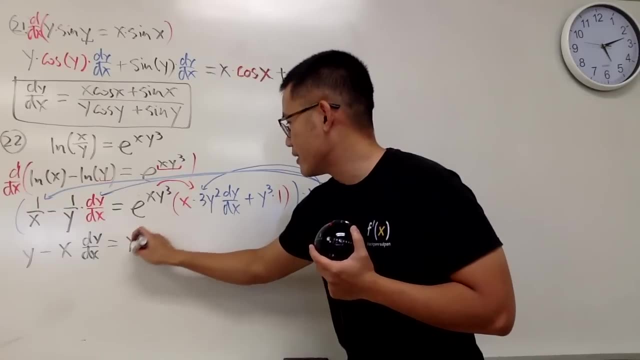 Now we have to do this times that. But also this right here has to be multiplied inside, Okay, So here we go. x times x is x squared, y times 3y squared, So we have this 3 right here, And then y squared times y is y cubed. 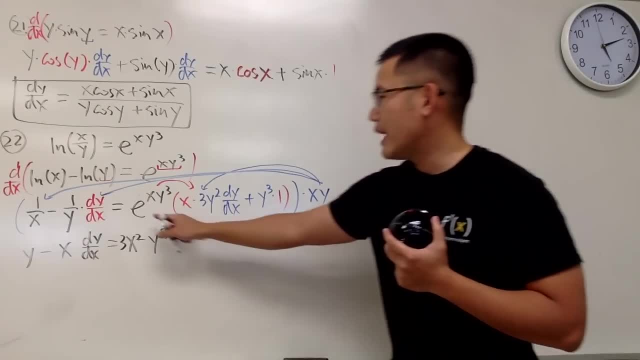 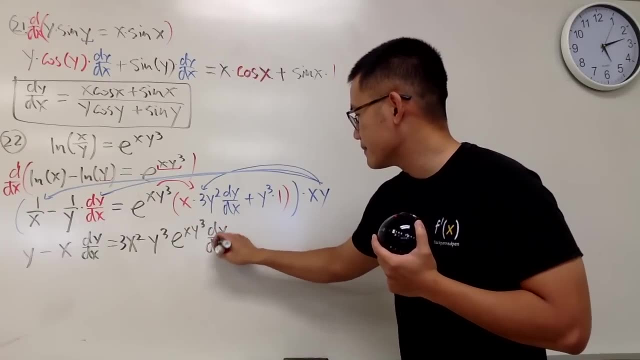 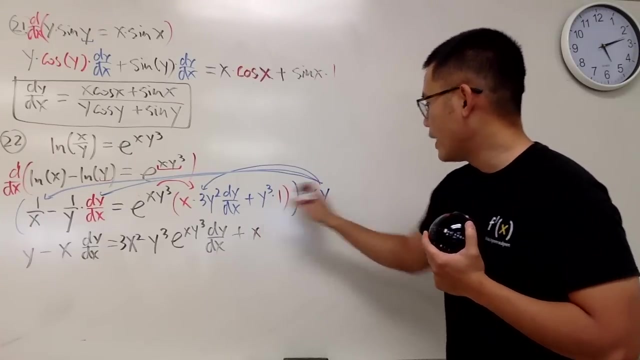 Right, Yes, And then I will put this down, which is e to the x, y cubed, And I will put down the dy, dx, Good, Next, we do this times that. So we put down plus We have x, y to the fourth power. 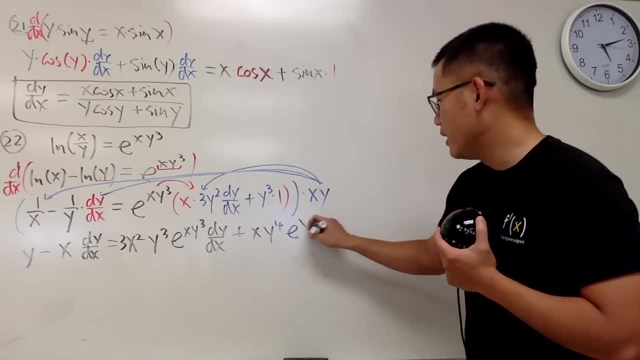 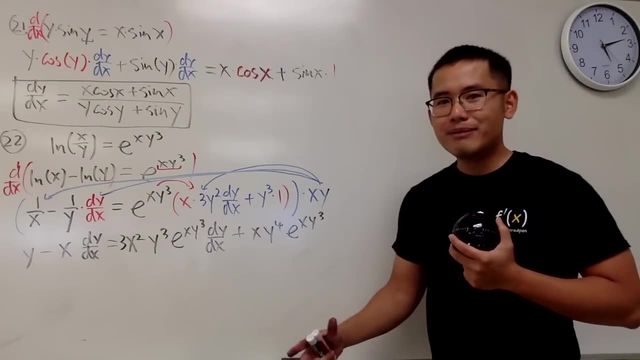 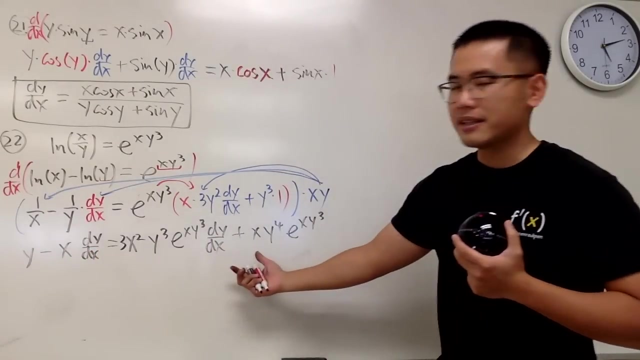 And multiply by that, So it's e to the x, y cubed, Just like that. Very good, huh, All right, So now we have to do what we did before. I am going to keep this on the right-hand side because I would like to add this to the other side. 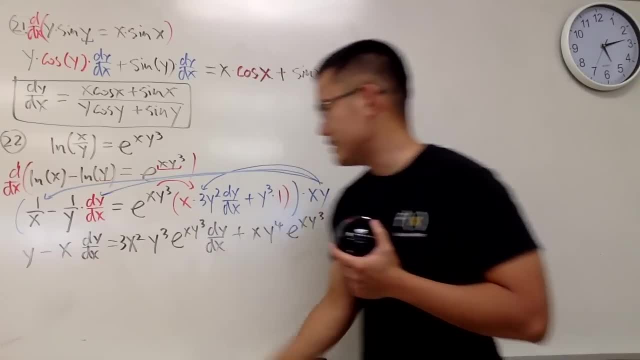 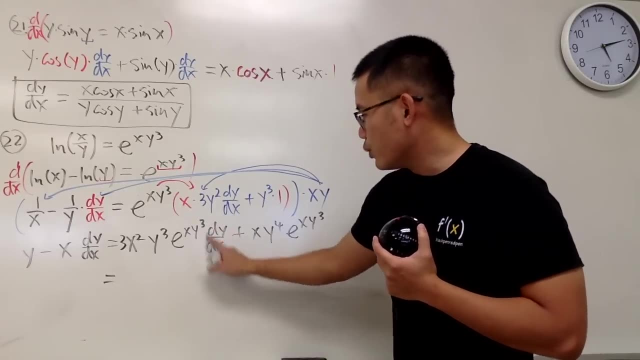 I want to keep everything positive right And now bring this to the other side. It's easier this way. So when we do that, let's see On the right-hand side again. we will factor this out, We will put it at the end. 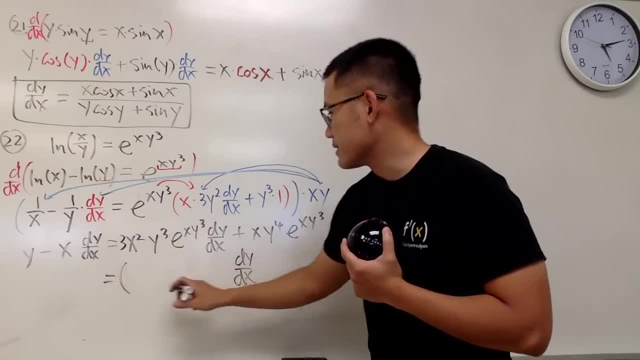 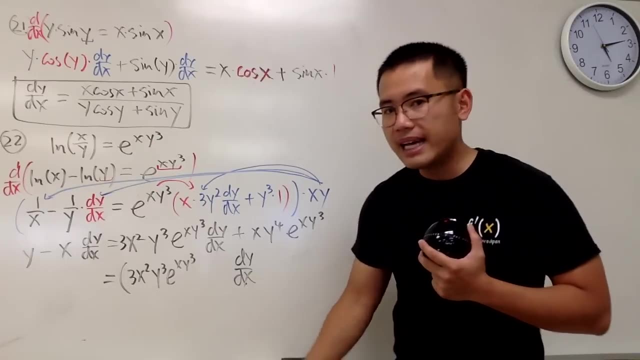 So we have the dy dx. Well, this was positive. So we just write down: 3x squared, y to the third power, e to the x, y to the third power, And when we bring this to the other side, it becomes a plus x. 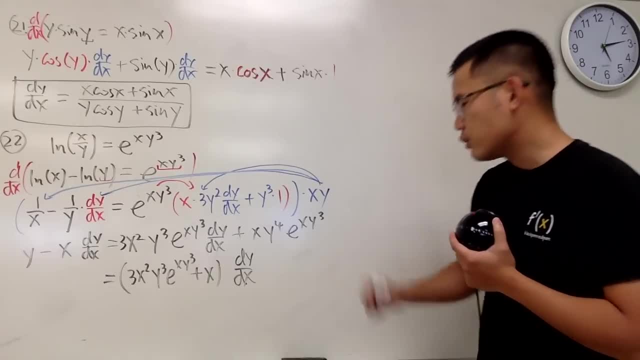 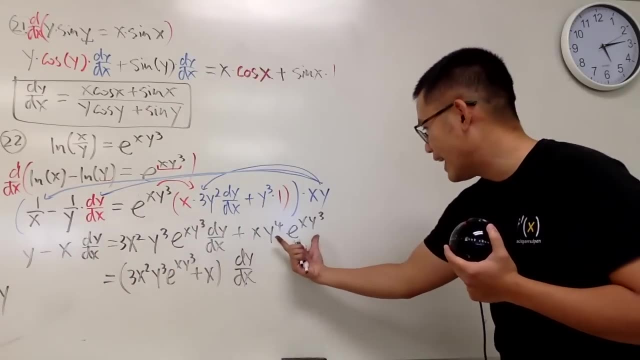 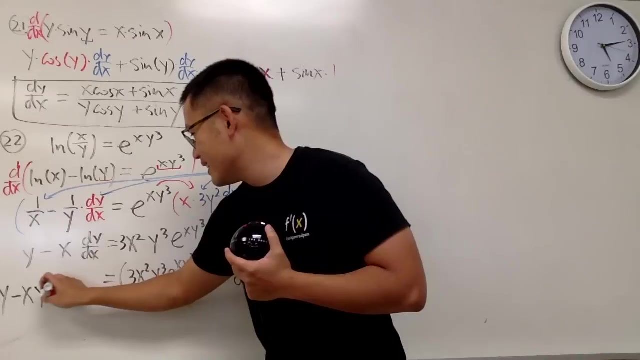 And this is being factored out right here already. So that's what we have, And for the left-hand side, this y is still chilling right here, But we will have to move this to the other side. So we minus x y to the fourth power. 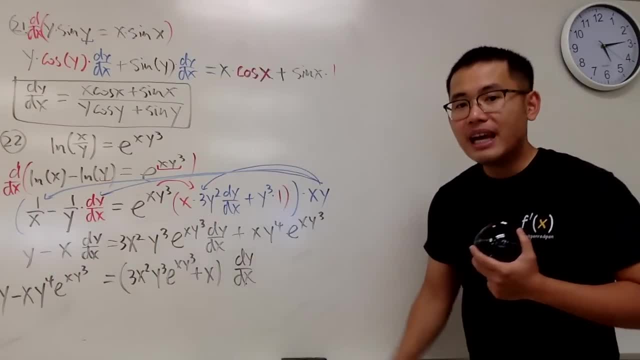 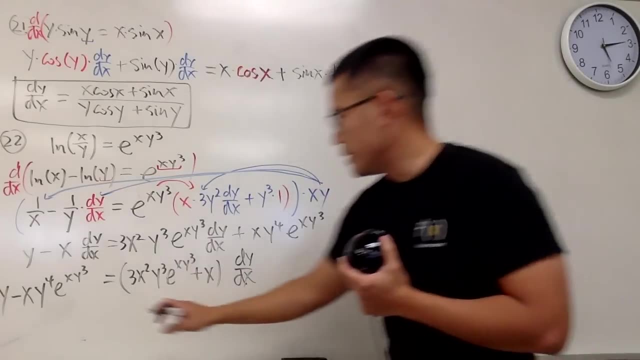 And then e to the x, y cubed Like that. In the end we just need to divide this on both sides and we'll be done. So perhaps I will. I should be able to fit in here. So dy dx equals. 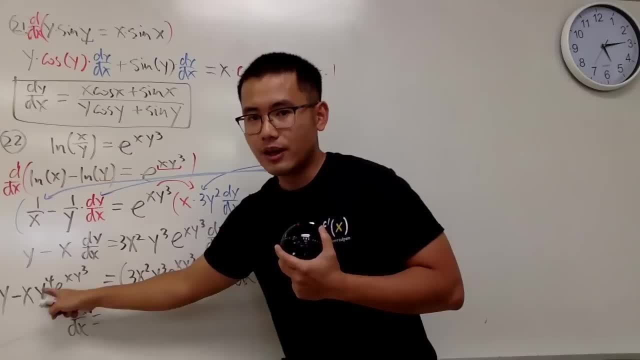 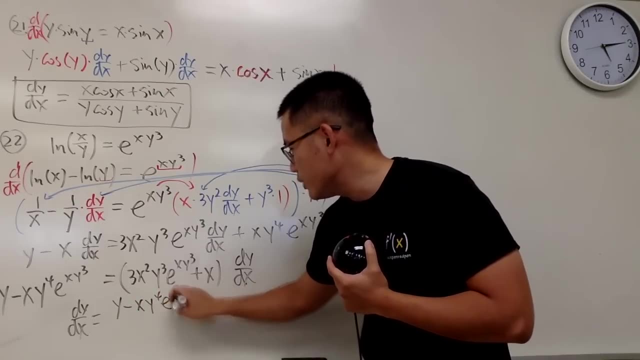 This right here will be divided here. So this is on the top. So I will just write it right here: y minus x, y to the fourth power, e to the x, y to the third power, And then divide it by: 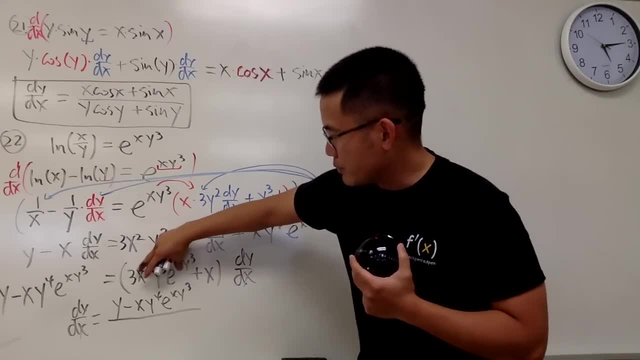 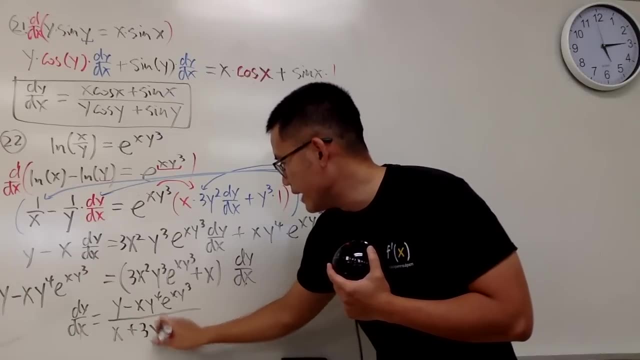 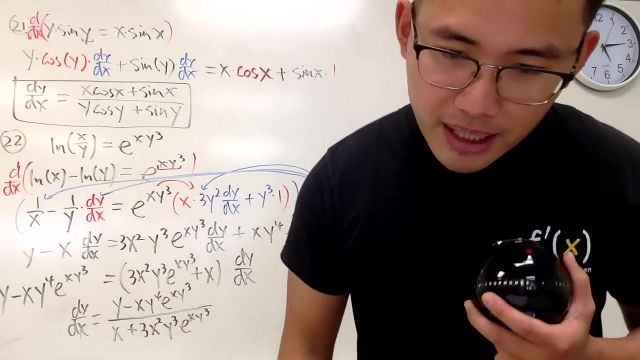 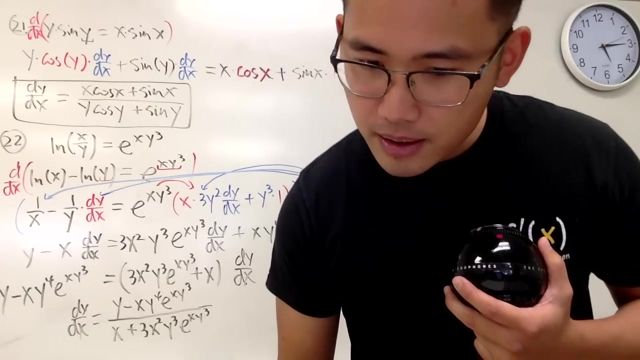 Well, perhaps we'll put this at the end, Just put the x right here, So we have x plus this part. 3x squared y cubed e to the x, y cubed Like that, And let me just make sure I didn't do anything wrong. 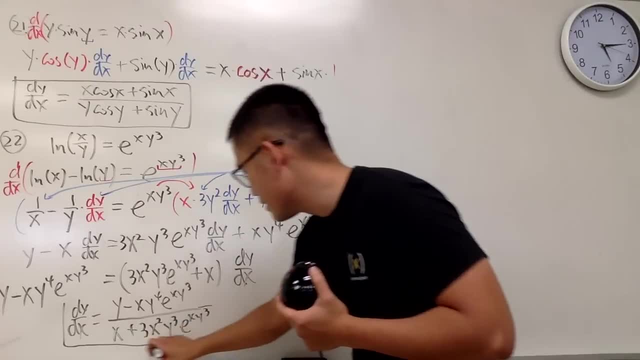 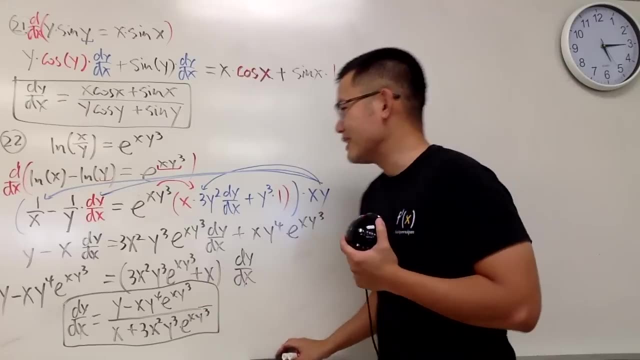 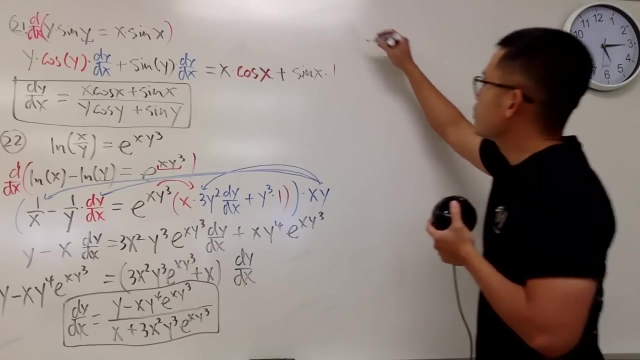 I didn't do anything wrong because I see the answer on my answer key. Good, So a slightly longer one, but it's not that bad. So take a look right here. All right, Question number 23.. Question number 23.. 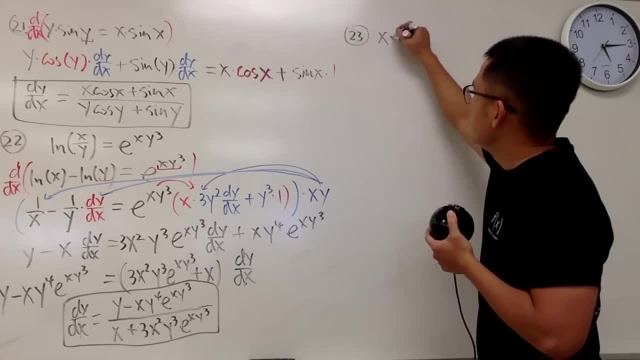 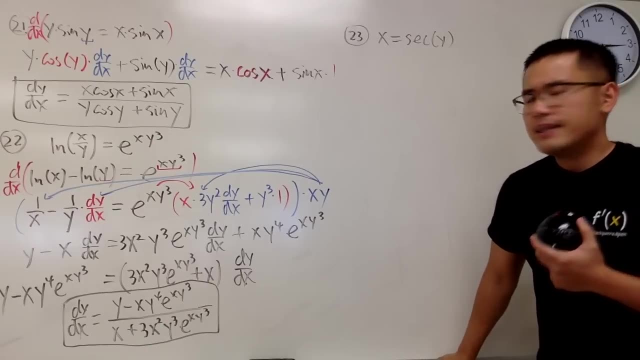 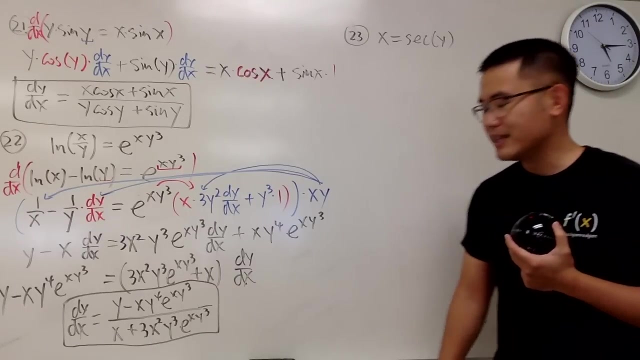 This right here is a weird one. We have x equals secant of y, Like that. And now you might be wondering: okay, can we just isolate the y right away by taking the inverse secant on both sides? Yes, We can do that. 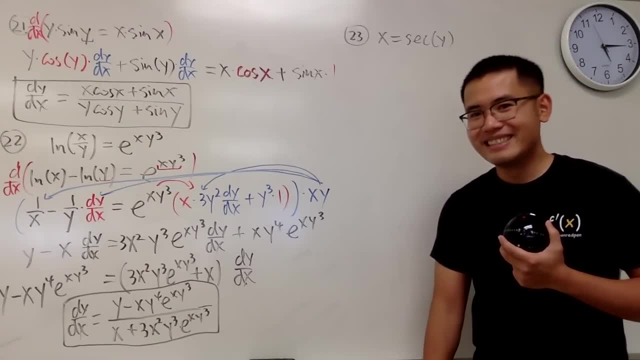 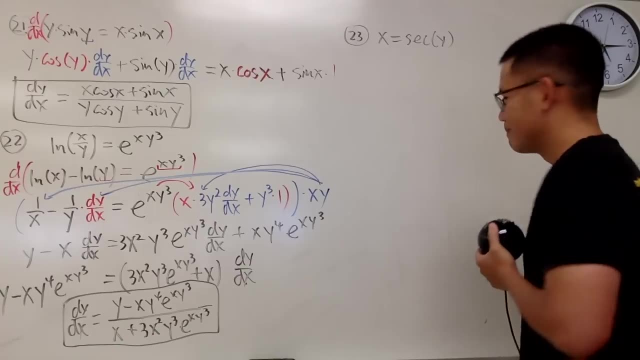 But what's the derivative of the inverse secant? Well, if you remember it, it's okay, You can just put down the answer. I'll just tell you guys that I do know the answer. I'll just put it down right here. 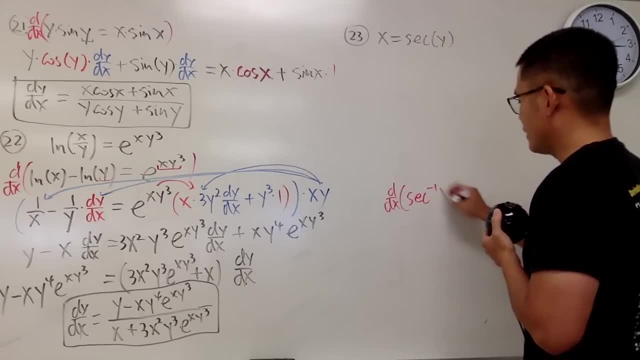 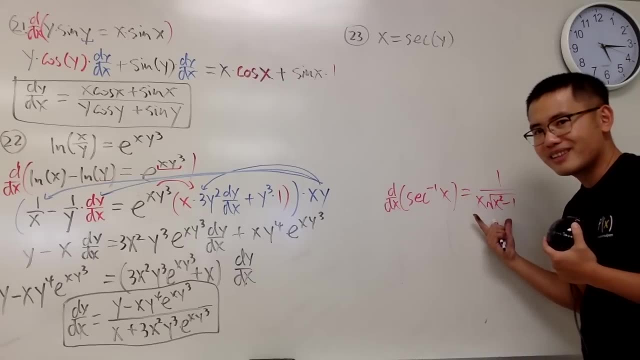 Derivative of the inverse secant of x. This right here is 1 over x squared, root of x squared minus 1.. And does this look familiar to you guys? No, I'm not trying to show you guys my back. I am trying to show you guys my back. 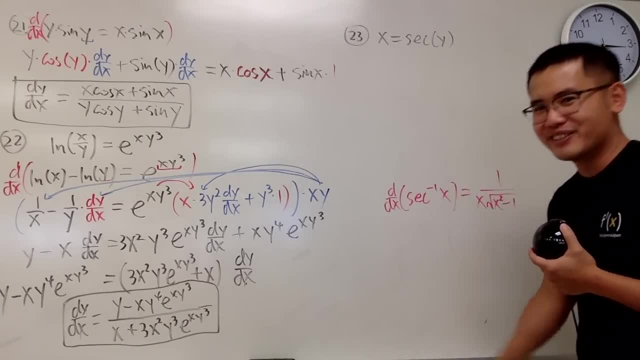 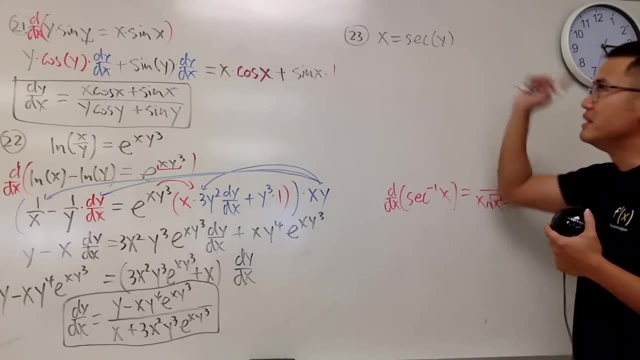 but this is actually one of the answers that we got earlier from one of the questions. right, You can let me know which question it was. Anyway, if you remember this good, But if you don't, this is how you can prove it. 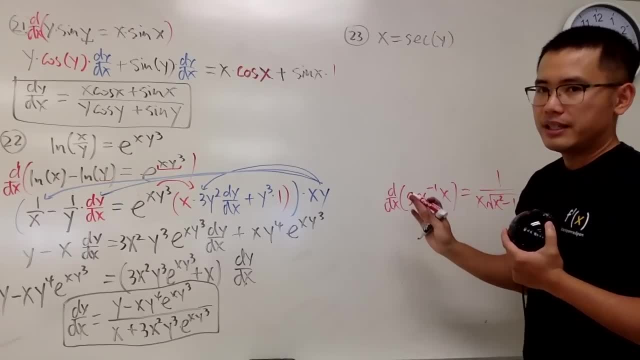 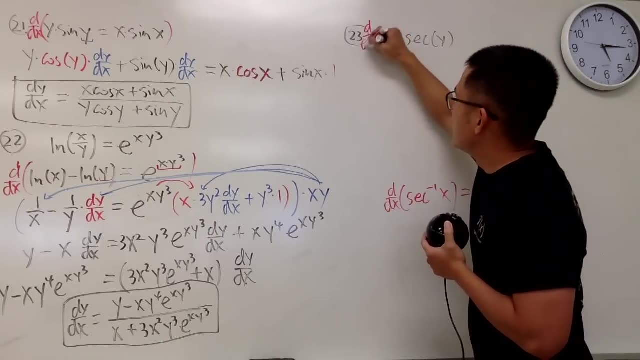 I will show you Right here. the y is not isolated. This is slightly more preferred because we do know the derivative of secant x, Secant y in this case actually, So we can handle the original secant. This is how. 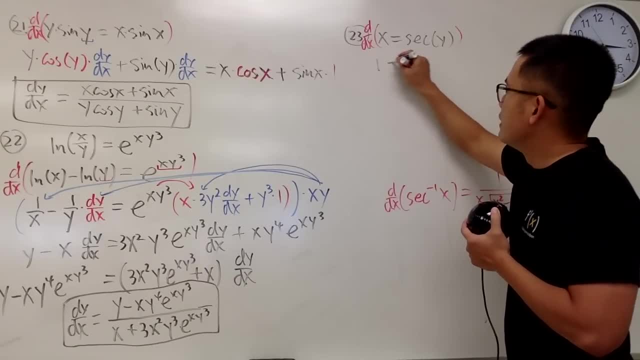 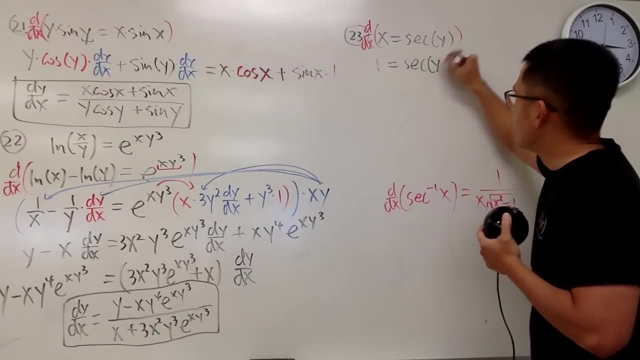 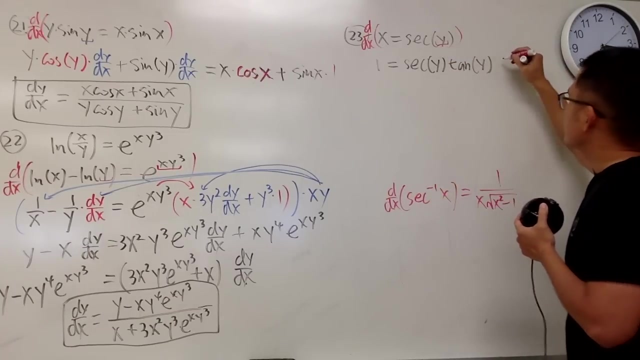 Okay, taking the derivative of x is just 1.. Well, derivative of secant. this is the original. We just have secant of the input times, tangent of the input and the derivative of the input. Thanks to the Chandu, we have to multiply by dy, dx. 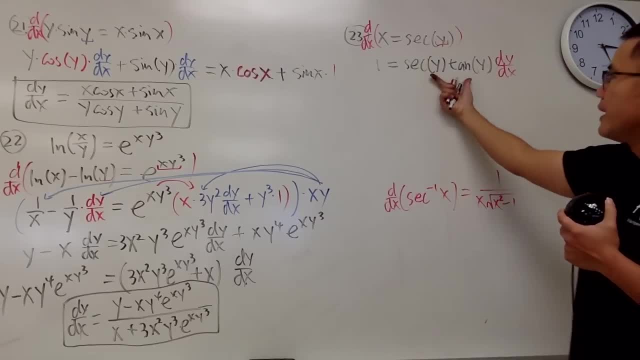 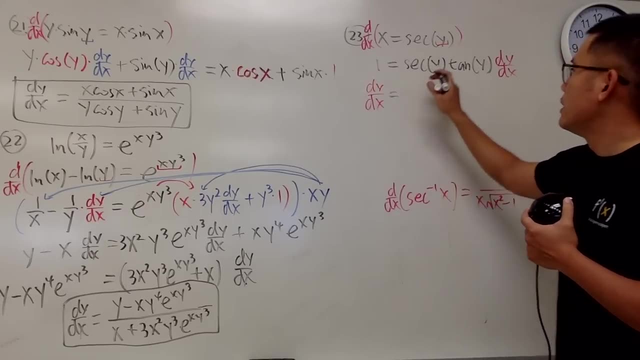 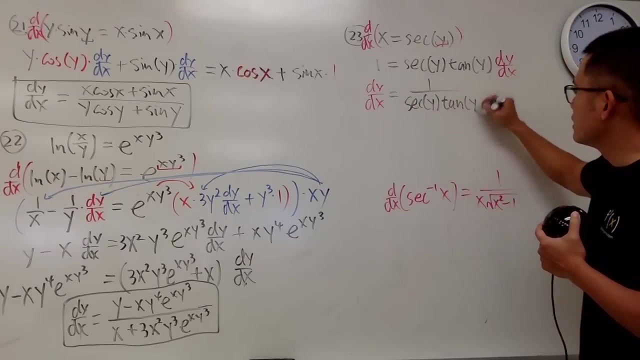 And now we can just keep this right here and divide both sides by this. So we get dy dx being equal to 1 over secant y times, tangent y Right, and you might be thinking this is not that bad at all. 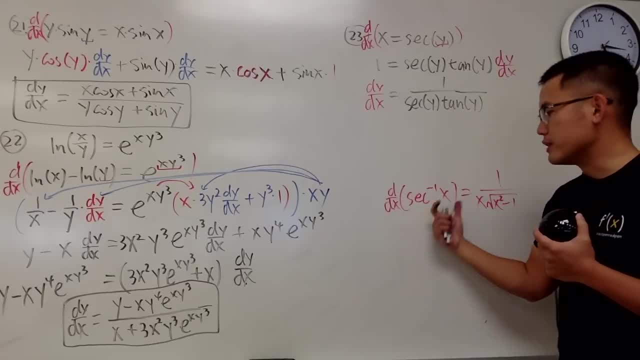 But here's the trouble. If you want to figure out the derivative of inverse secant x, well, if you want to just take the inverse secant x on both sides, the idea is that when you take the derivative of inverse secant of x, 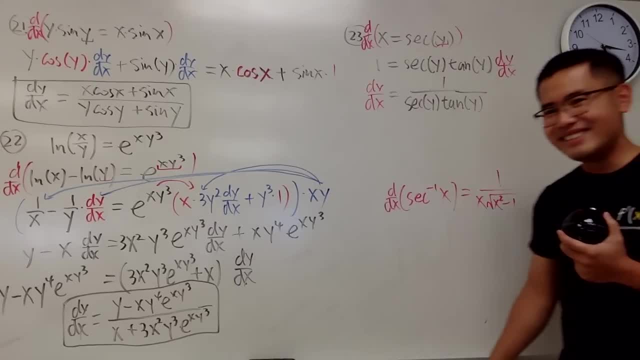 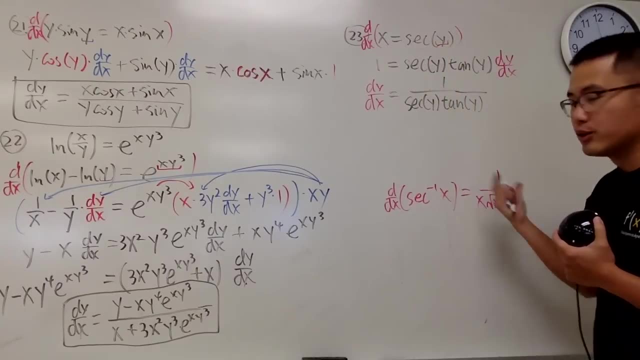 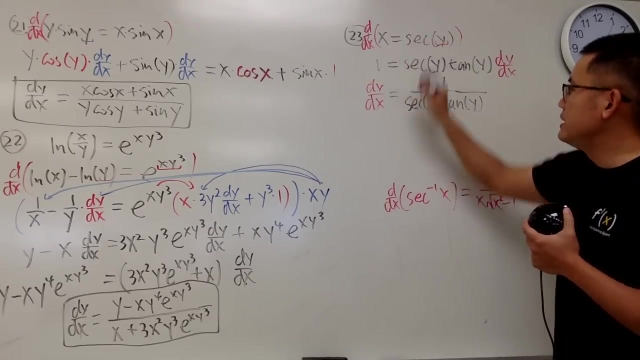 your answer should be in terms of x as well, isn't it? So now, this is how you get back to x Again. this question right here, is to show you guys how to prove this right here. right, Alright, so to handle this, well, we do know. secant y is equal to x. 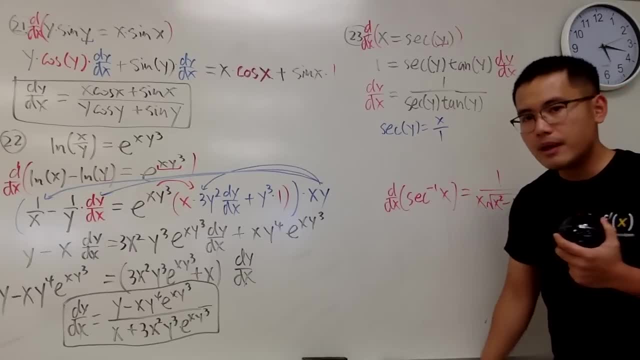 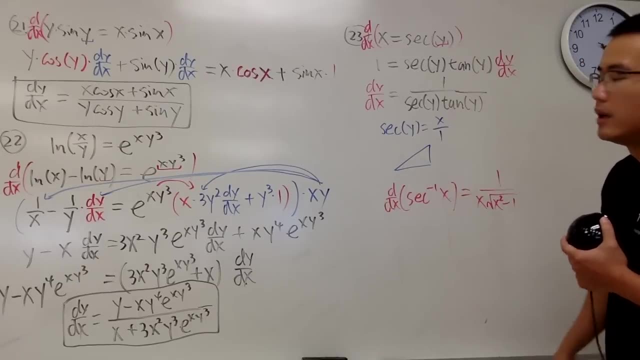 which is the same as saying x over 1. And by looking at this right here we can come up with a right triangle. So I will put down the right triangle right here, And the reason to do so is because we can put the angle here, that's y. 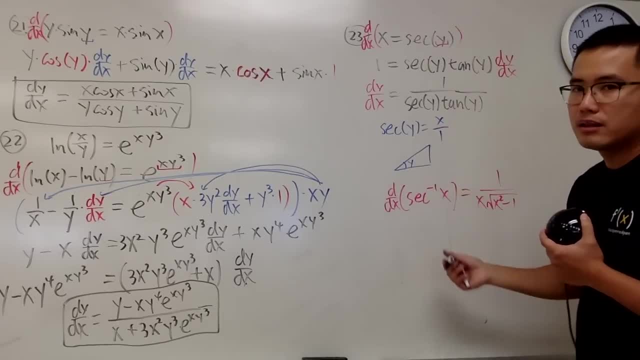 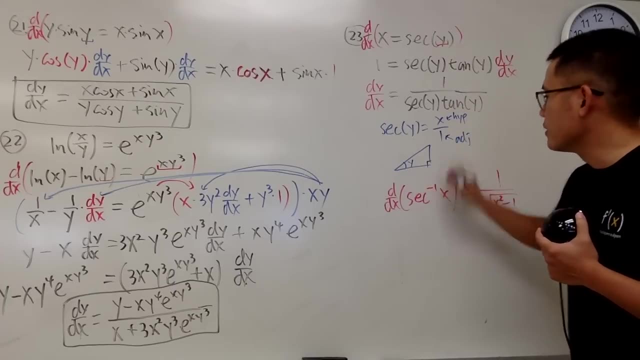 and we can label the sides And remember secant is what Secant is, hypotenuse over adjacent when you are talking about right triangle. So that means x is right here and y is right here And now for the other side. that's missing. 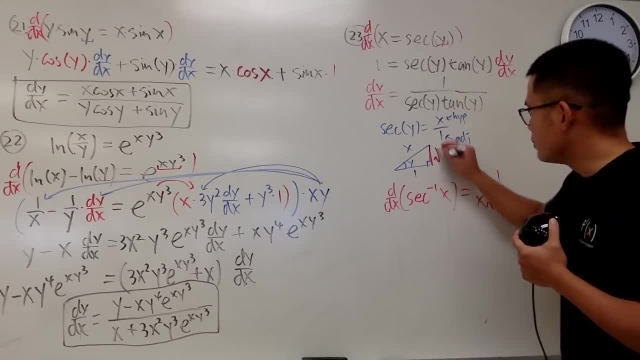 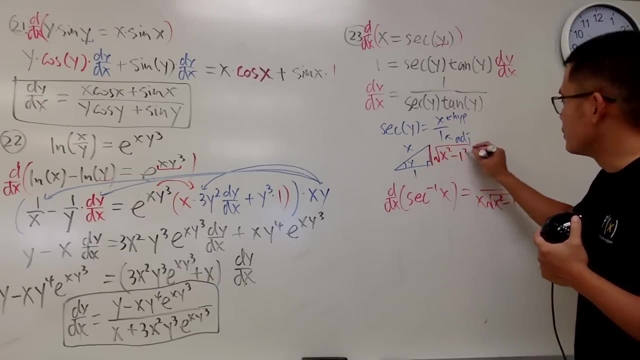 well, the easier way to find this out is just: you open the square root and you square the hypotenuse, which is x squared, and you minus the square of this side, which is 1 squared. By looking at this triangle, you can figure out whatever you want. 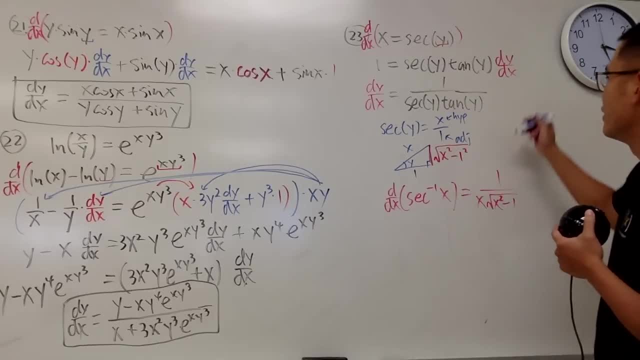 Of course, for tangent as well. Here is the deal In the end. you will see we have a 1 on the top over secant. y is just x over 1, which is just x, That's good. And tangent of y of tangent. this picture here is just the opposite, which is this: 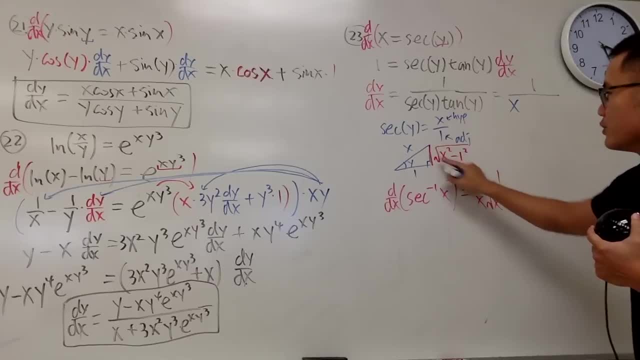 Over the adjacent, Over 1, doesn't matter, so it's just that. So we can just put down: square root of x squared, and then minus 1 squared, which is the same as just minus 1.. That's it. That's it. 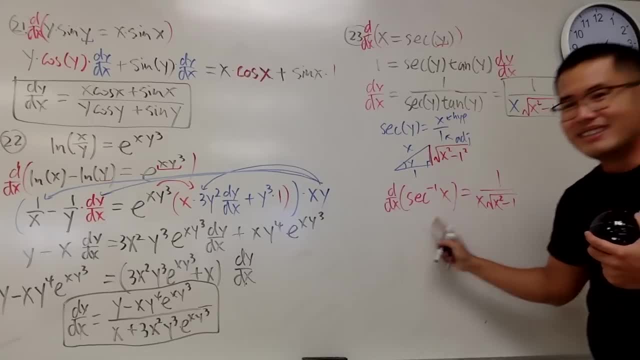 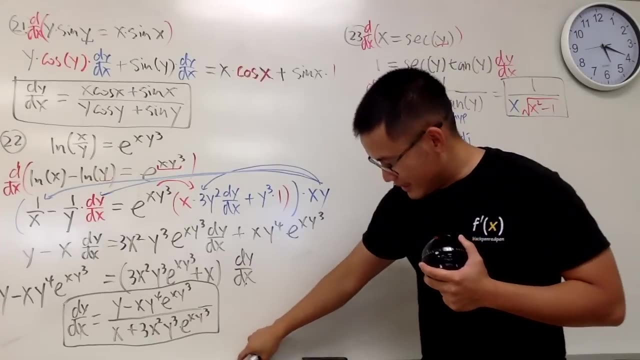 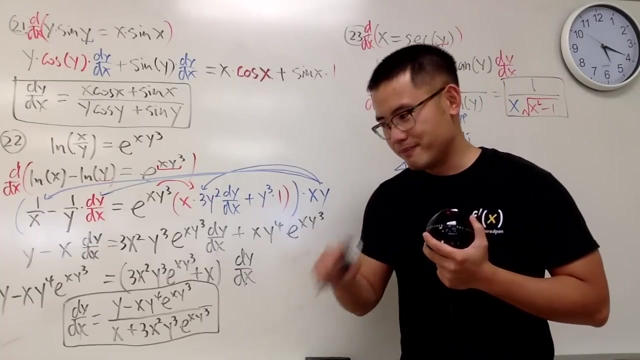 So this right here is how you prove the inverse secant has the derivative being that Right. So this is one of the ways to prove it. I will show you guys how to prove the inverse tangent derivative by using the definition once we get here. 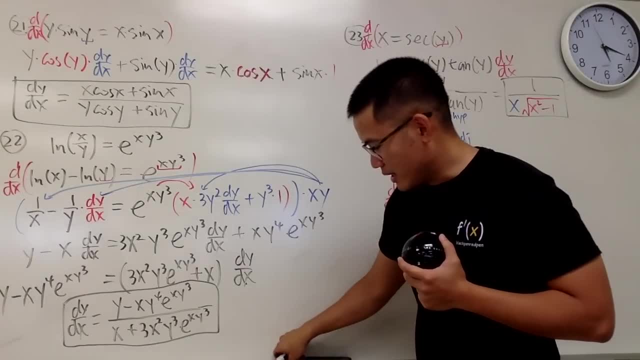 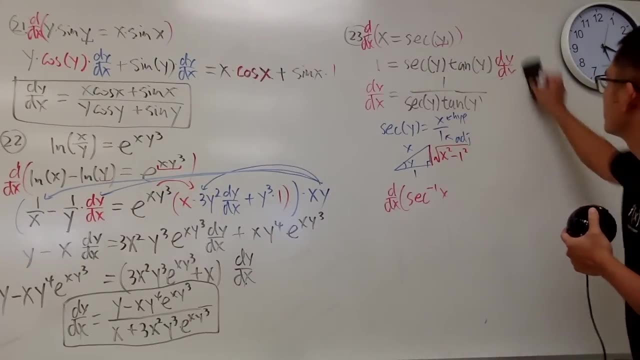 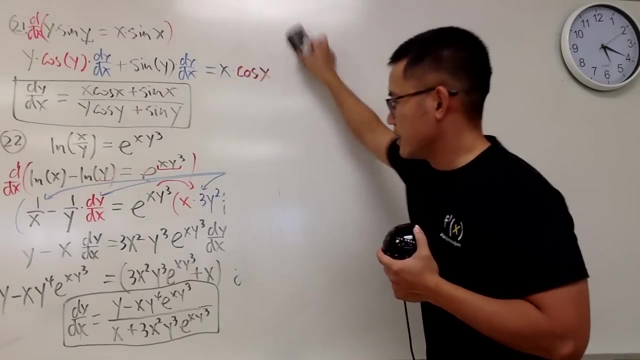 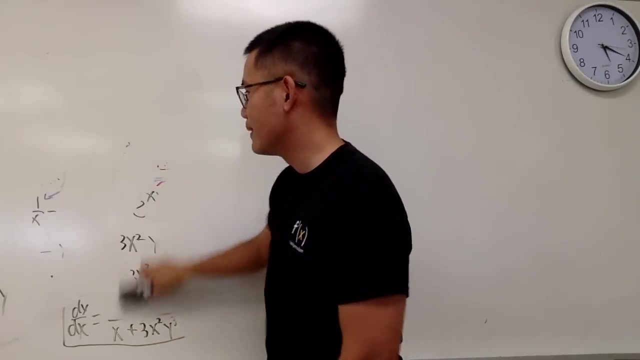 Alright, number 23.. That was question number 23.. Man, when can I drink the ninja milk? I don't know. So I'd like to tell you guys this: right here is seriously just running a marathon. So this is like halfway, almost halfway done. 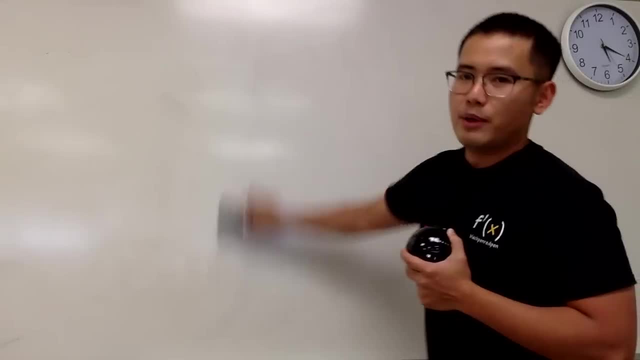 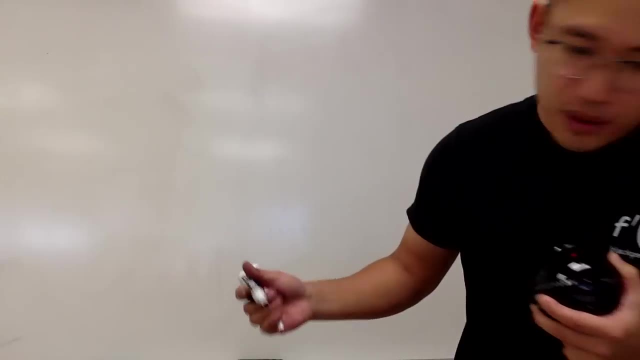 So minus 6 each. Alright, That was question number 23.. And now moving on to question number 24,, of course, 24.. And we have parentheses: x minus 1,, minus 1,, minus 1,. 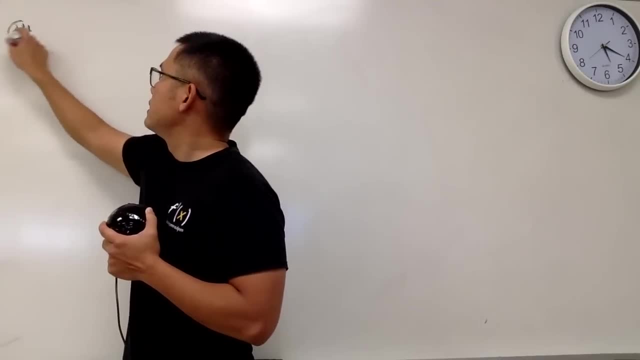 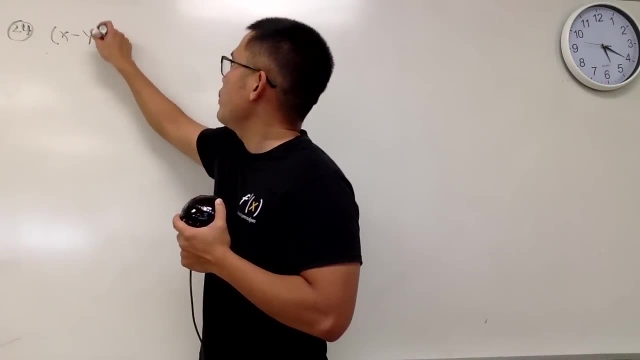 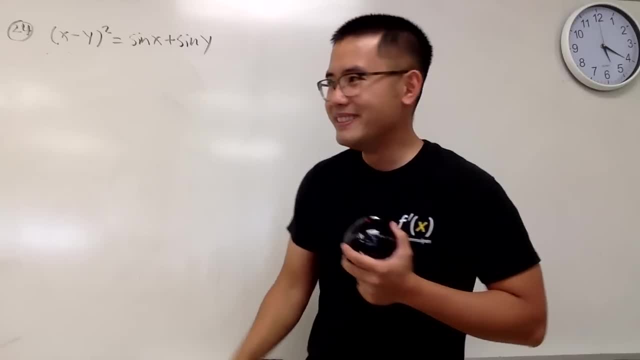 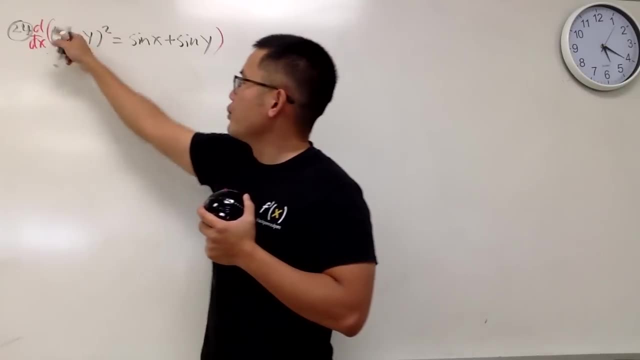 Like that. Alright, implicit differential action in action. so D, D and x, Here we go Right here. bring the 2 to the front because you have to look at the big picture. So power root first, right. 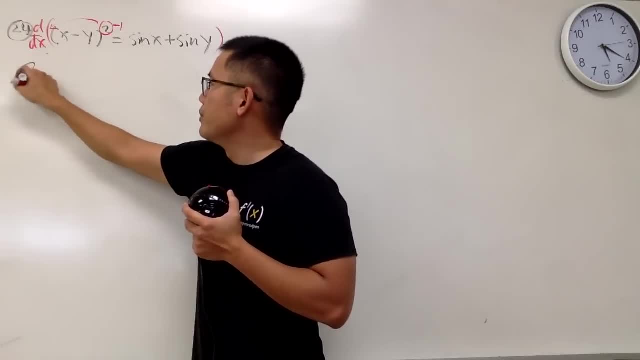 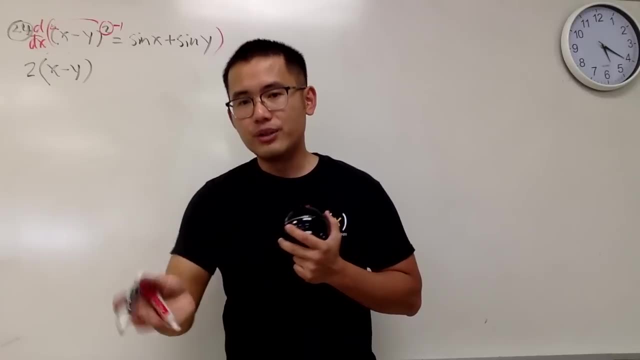 Bring the 2 to the front and the minus 1.. So here we have 2.. Open the parentheses and then the inside states the same x minus y and do the Chandu. Look at the inside and ask yourself what the derivative is. 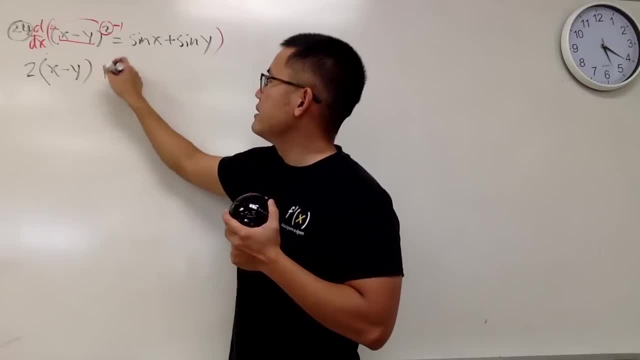 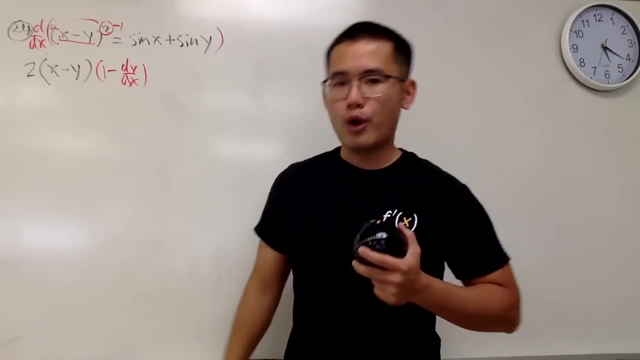 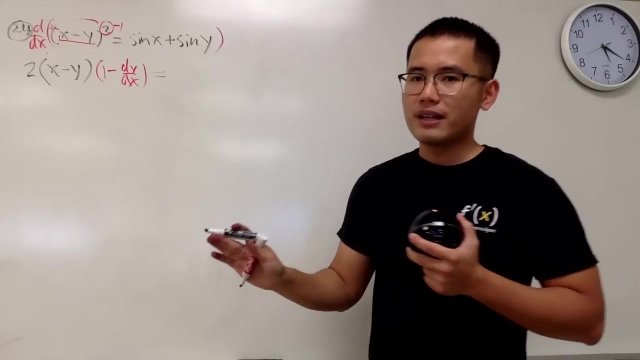 Derivative of x is 1, minus. the derivative of y is dy, dx. And notice that it has two terms. so you have to put up parentheses. That's it for the left-hand side. and now for the right-hand side. This right here, you don't need to do the product rule. 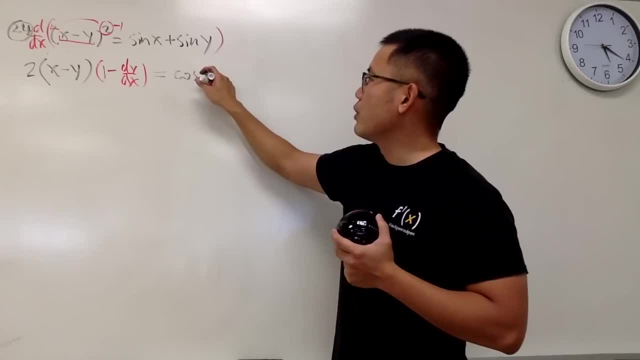 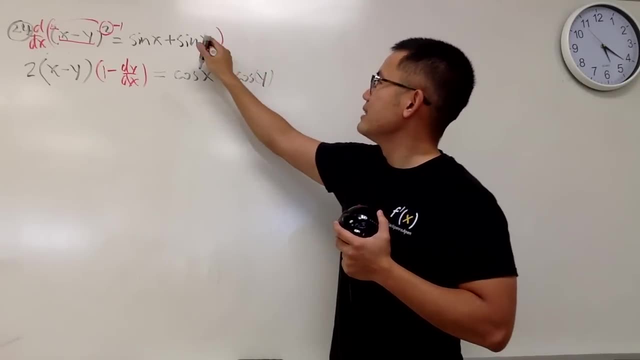 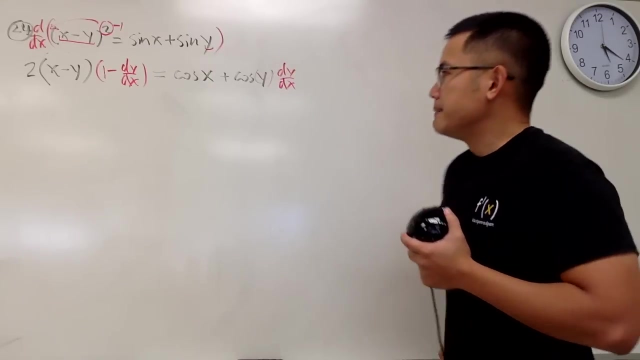 just differentiate the first, which is going to give us cosine x, and differentiate the second, we get plus cosine y. but the derivative of y is dy dx. So don't forget the dy dx right here, Just like that. Hmm, Well, we have to multiply this out. 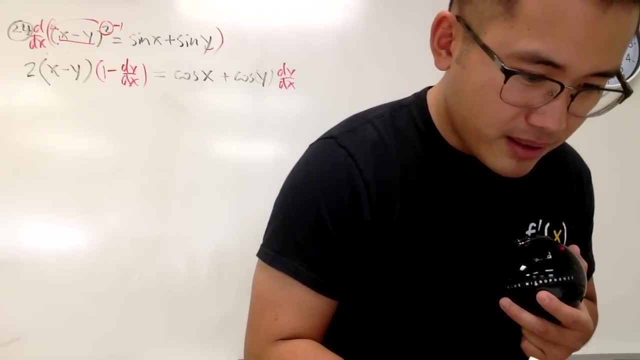 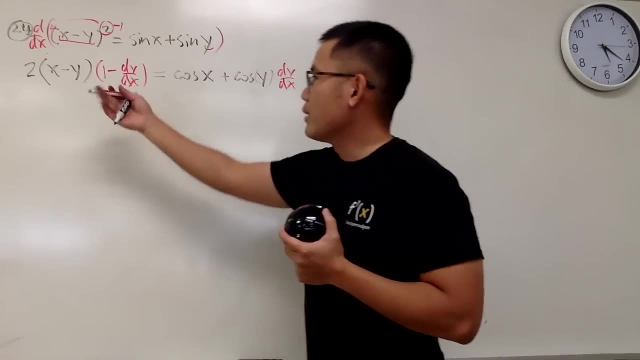 and based on how I come up with the: Yeah, just multiply this out. Anyway, I think I will multiply this out as well. so I will just multiply. Oh, I'll do this for you guys, this and that first. So I'll multiply this out this way for you guys. 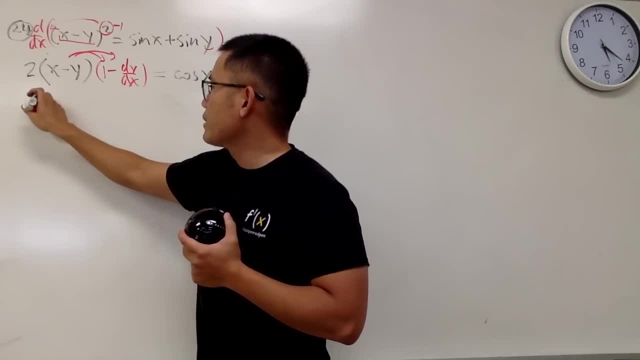 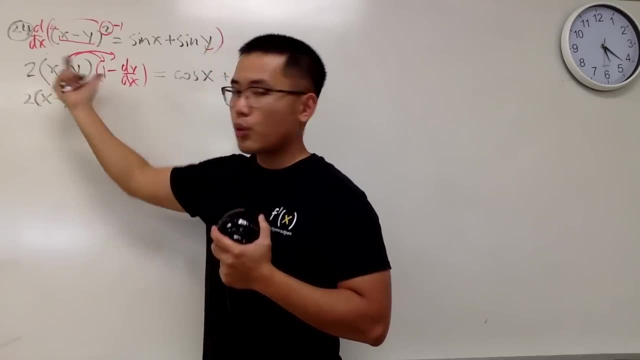 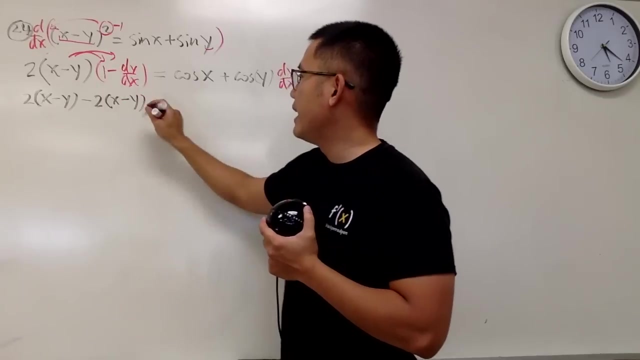 When we do that, I will keep the 2xy, 2 times x minus y. I'll take this quantity times 1, which is still that, and then minus 2 times x minus y and we have the dy dx. 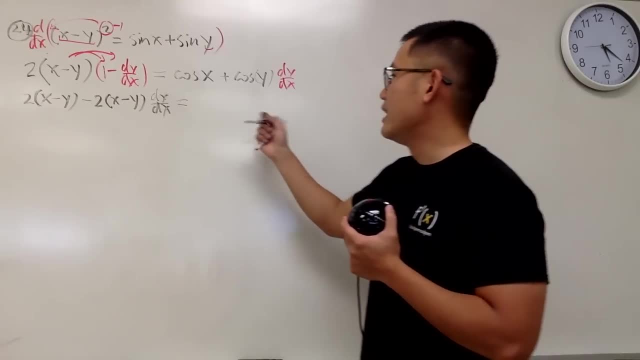 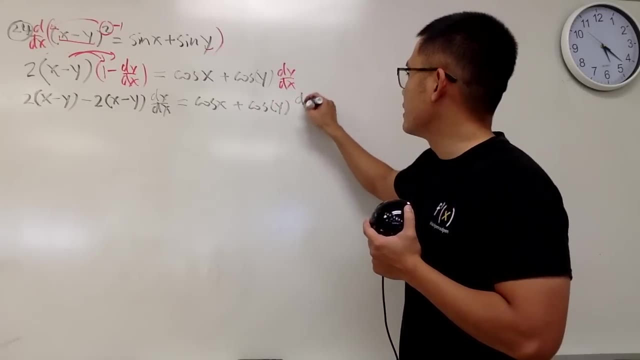 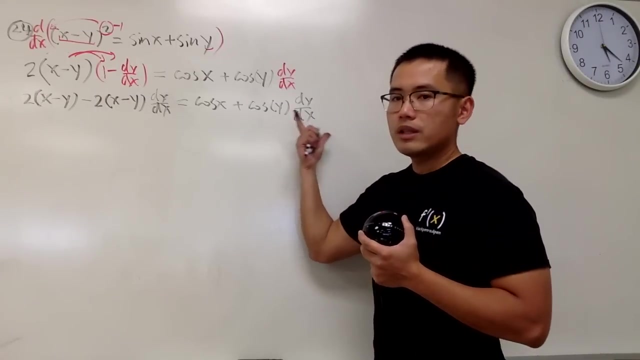 Right, And that is equal to the right-hand side, which the right-hand side didn't do a thing, so I'll just write it down: Cosine x plus cosine y and again the dy dx right here. Okay, I would like to keep the dy dx on the right-hand side. 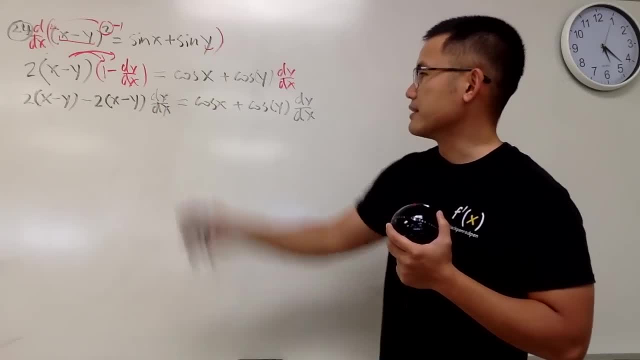 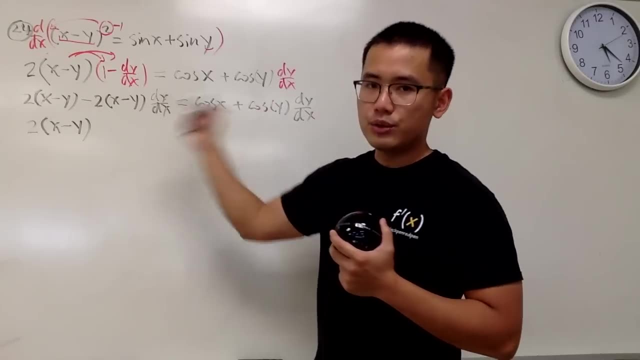 so that I can make that positive and I'll bring that to the other side. So perhaps I'll just write it down right here first. This right here stays. so it's 2 times x minus y. Bring this to the other side. 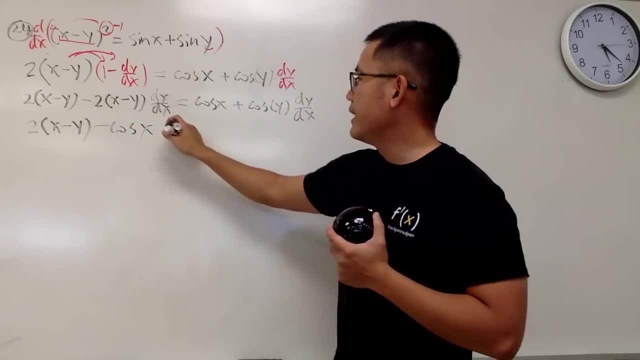 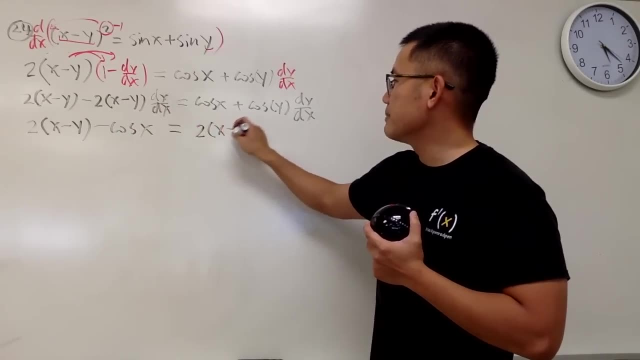 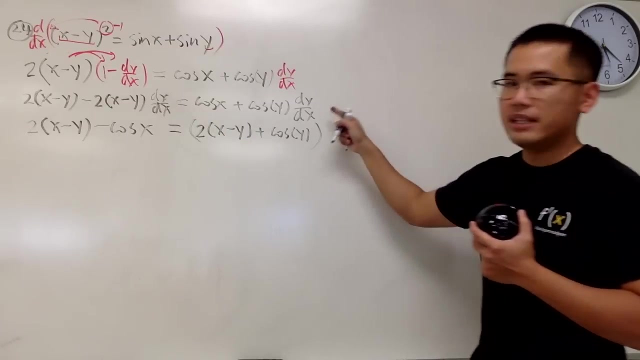 which is minus cosine x, and that's equal to well. bring this to the other side: it becomes positive 2, parentheses x minus y, and we add this with cosine of y, and then both of them have the dy dx. 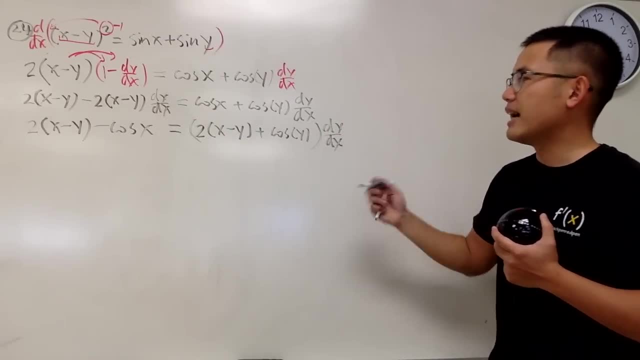 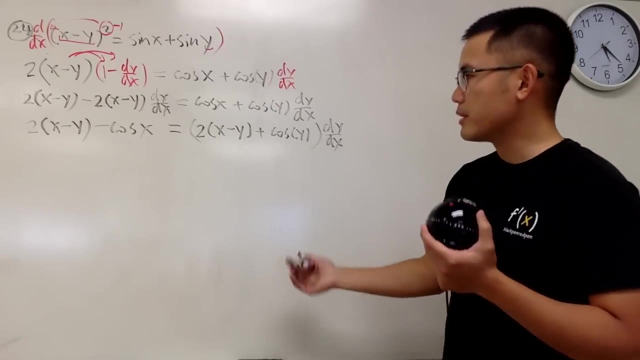 so factor the out, put it at the end Like that, Right, And in the end, of course, we can just bring this to the other side by dividing, and that's pretty much it. So we'll do that. Finally, dy dx. 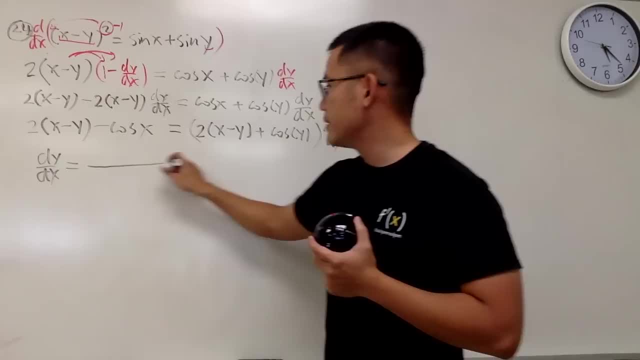 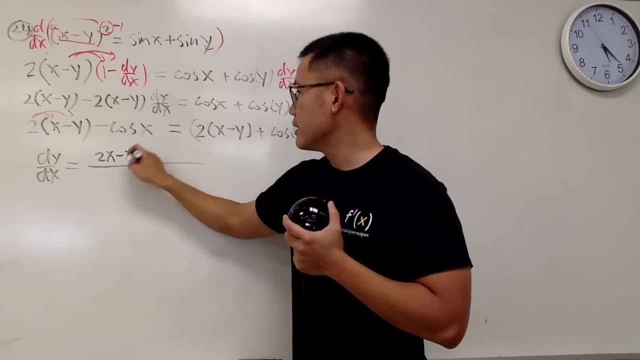 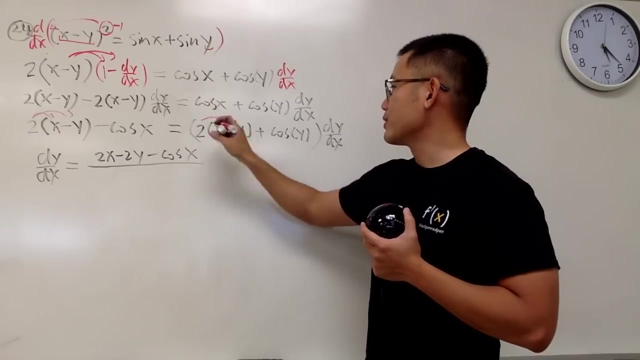 The answer to that is this on the top, But of course now it's the time to distribute. So we have 2x minus 2y and then minus cosine x and bring this to the other side, right? So I'll also divide that. 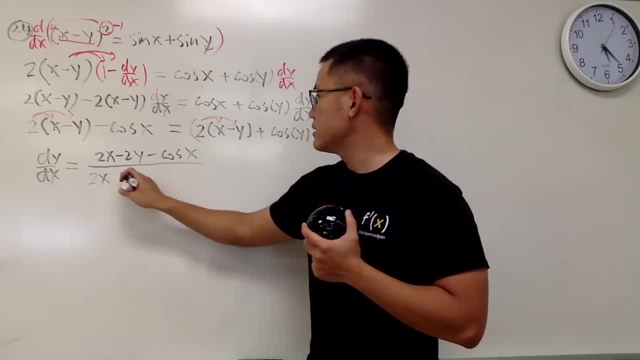 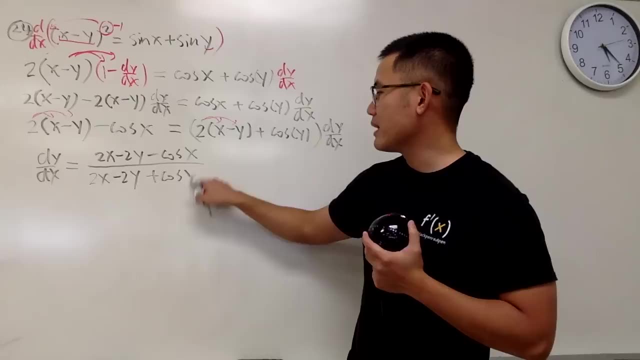 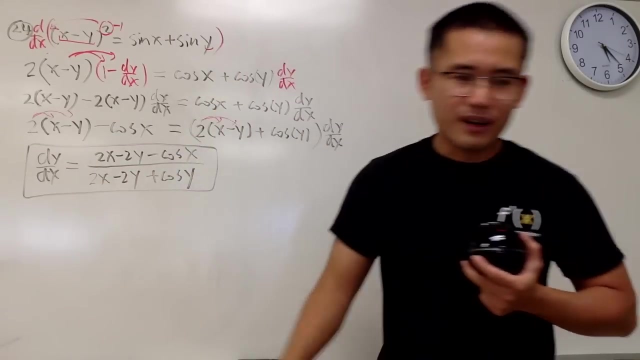 This will be on the bottom, 2x minus 2y plus cosine y. So this right here is a plus, Right. This right here is a plus. That's it Right. This right here is the answer. That was question number 24.. 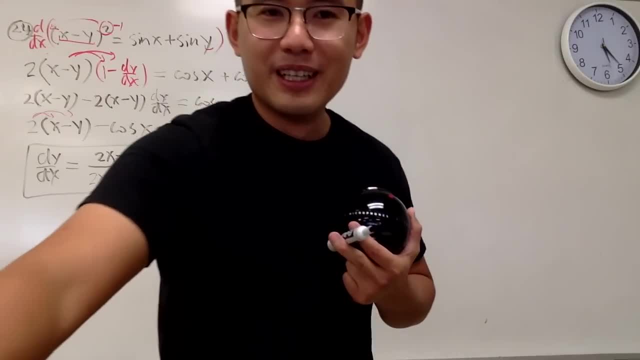 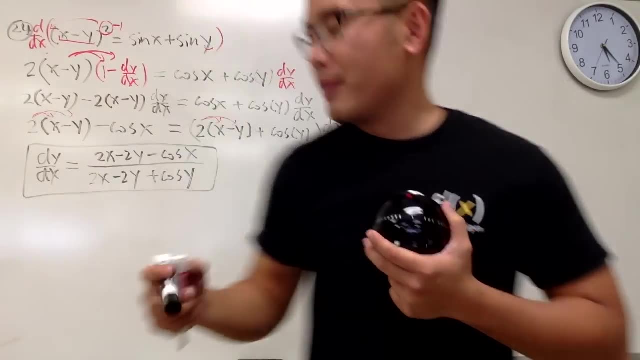 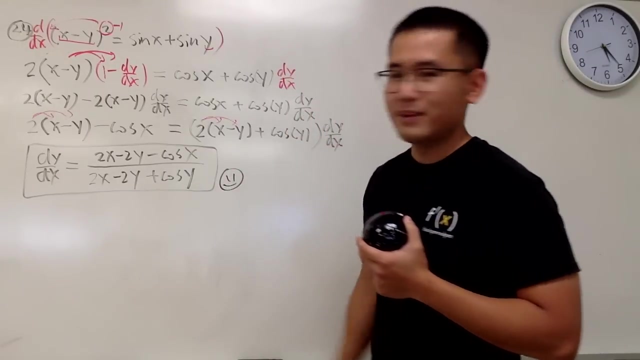 And I think it's a fair time for me to change the marker This time. unfortunately, I cannot do 100 derivatives with one marker. I don't have a fresh marker. Hopefully this one will work well. Ah, much better. 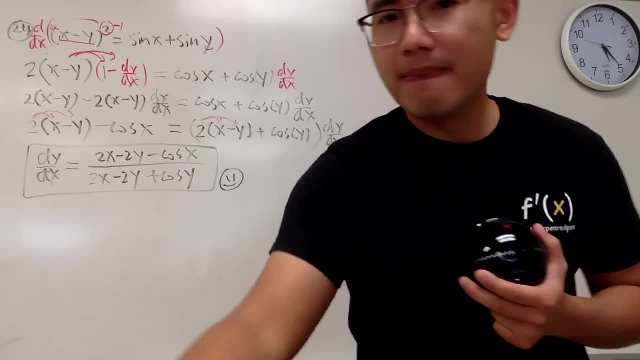 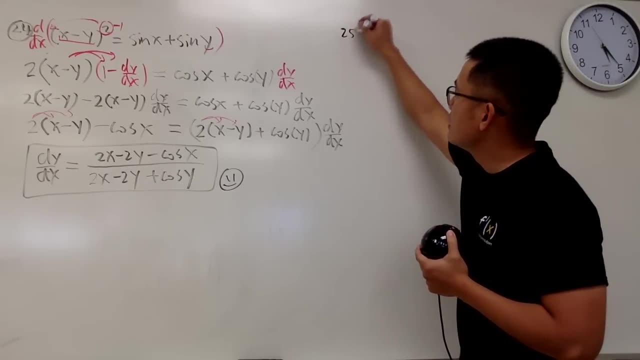 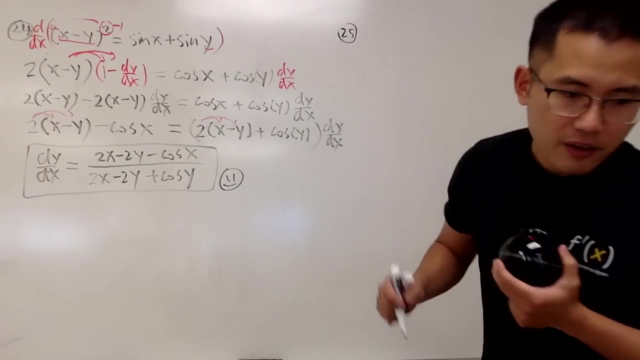 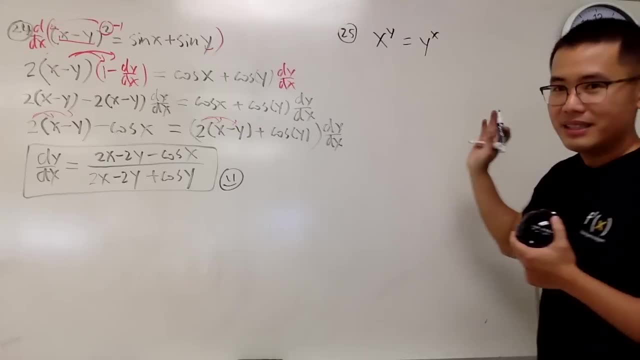 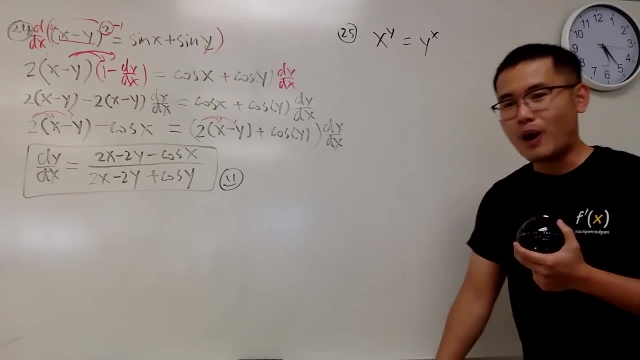 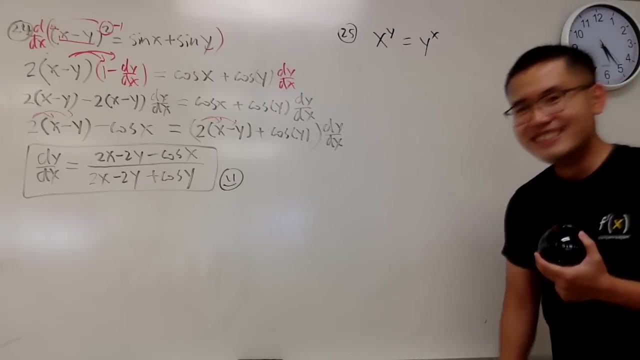 equals y to the x-th power. This is actually one of the really really famous questions. I mean the equation-wise. Why? Because I have a thesis on this equation: how to solve for x and y. that satisfies this equation and it has a lot of use. 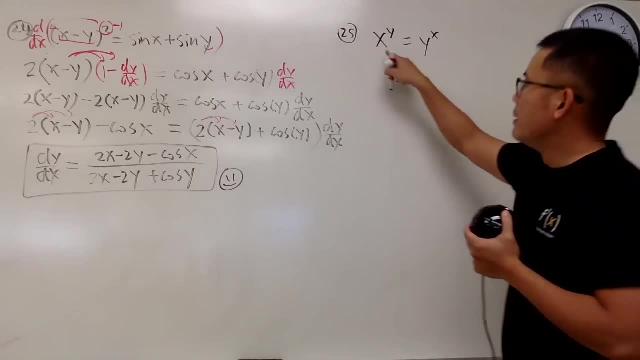 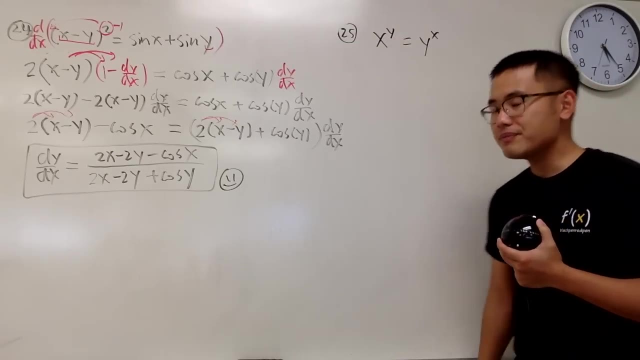 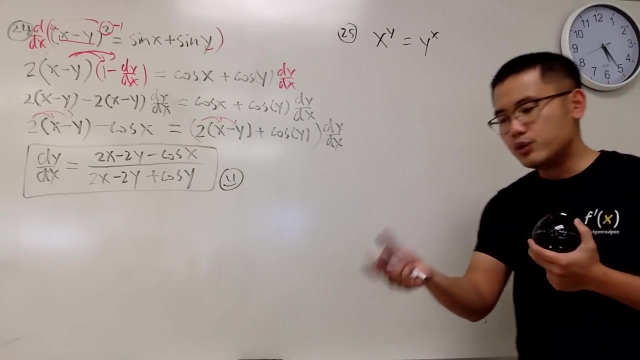 Anyway, we are going to find the derivative right here. Well, this is the function. Why it's also a function, So we cannot just do anything in a moment. Earlier we did x to the x and then we wrote the base x as e to the natural log of x. 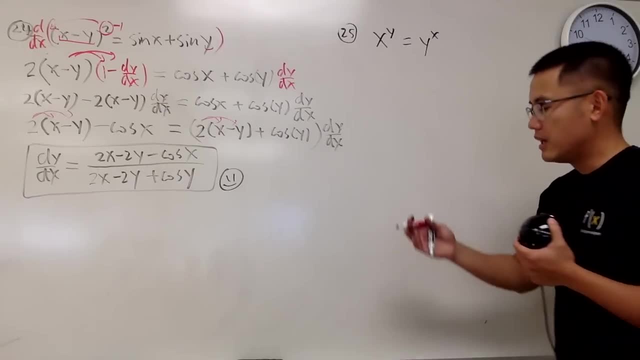 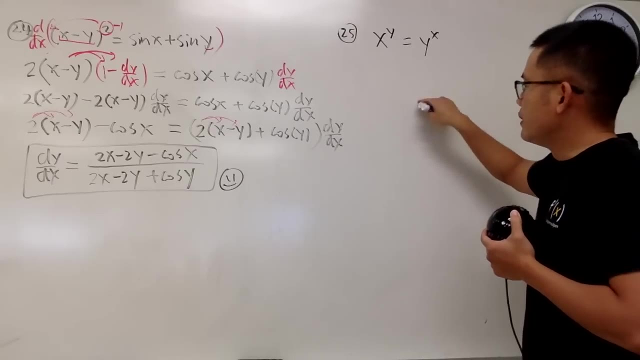 That will show you guys this way, right here We can do that. We can write x as e to the natural log of x, raised to the y, and then we can write y as e to the natural log of y and then raised to the x. 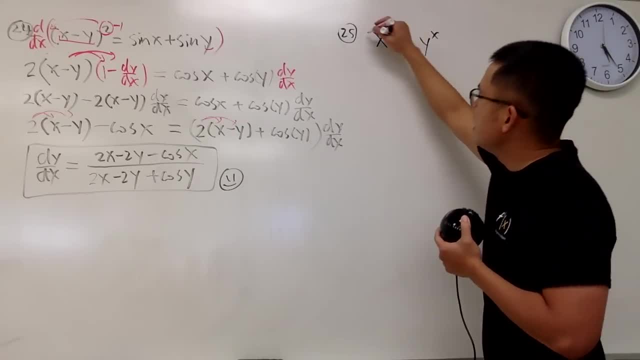 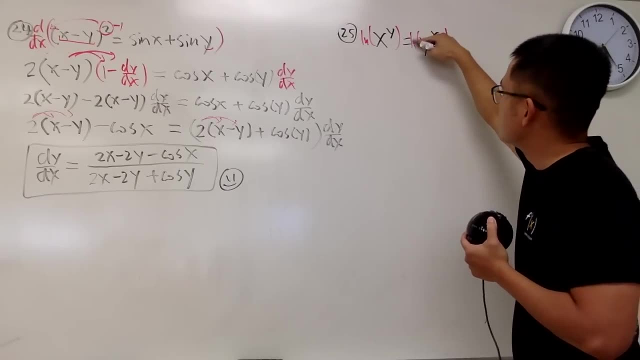 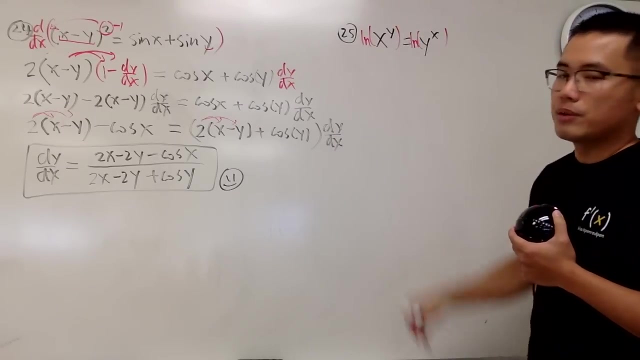 We can still do that, But in this case it might be easier if we just take the natural log on both sides. to begin with, We would like to do some algebra first, And this is also a pretty good strategy whenever you have a function to a function power. 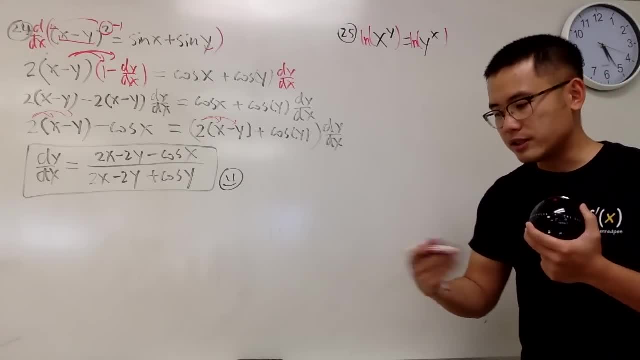 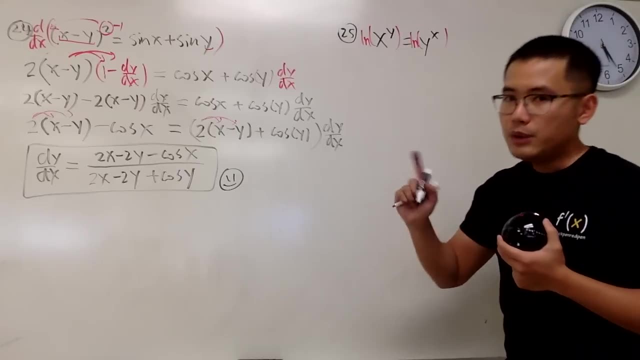 Or maybe, when you have a lot of functions multiplying together or dividing, you can take the natural log on both sides. You can use the natural log properties to bring things down. Anyway, enough talking, Here's the deal. This is y as a power. 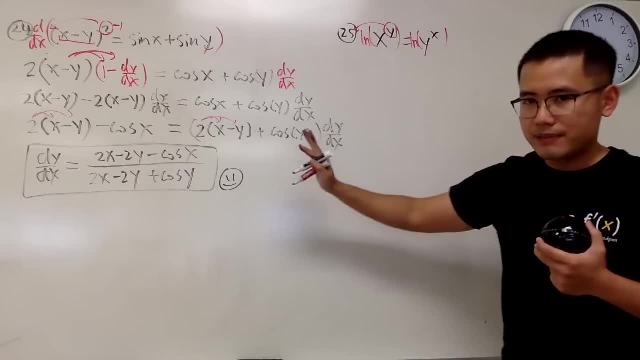 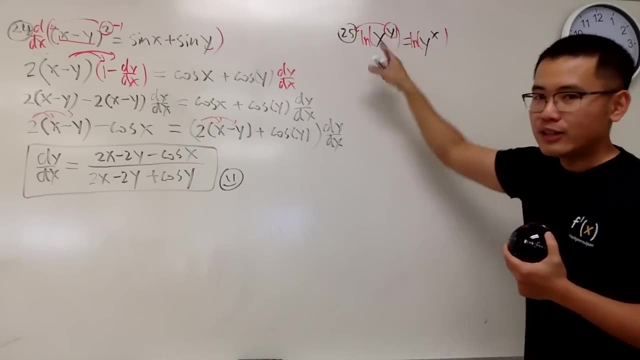 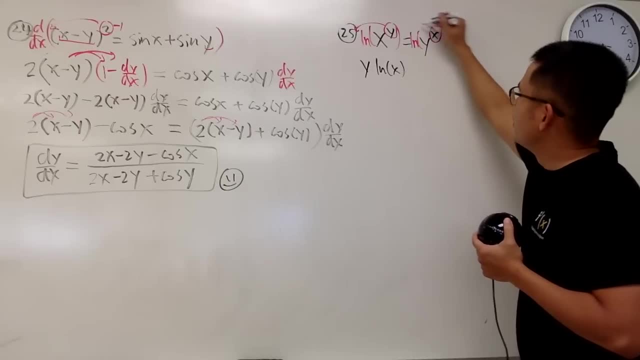 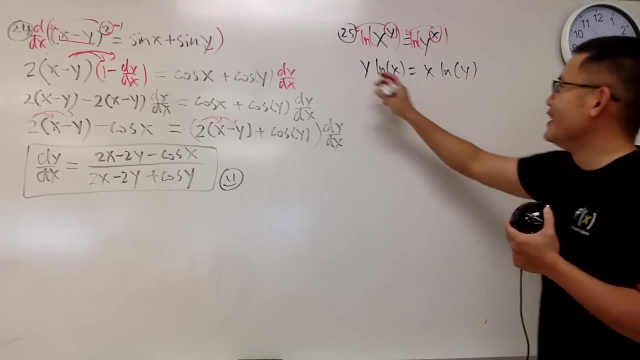 Like this: Okay. And then, similarly, we bring this to the front. we have x times natural log of y. Seriously, just like that. Okay, Now we are going to differentiate, So put the d? dx right here. It doesn't have any weird situations. 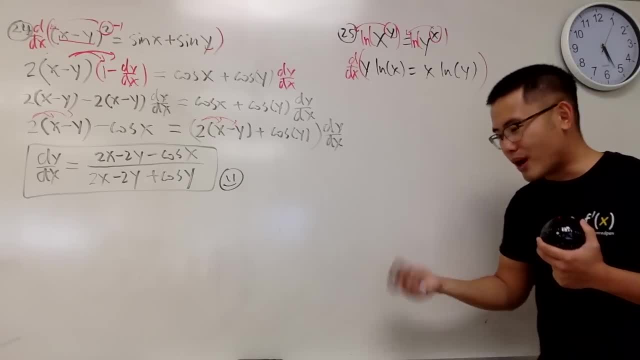 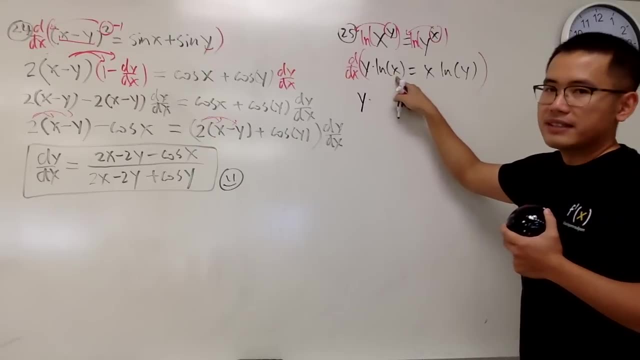 This is just an innocent case. You can just use the product rule now. So here we go. Product rule in action. We keep the first function, which is y times the derivative of the second Derivative of natural log of x is just 1 over x. 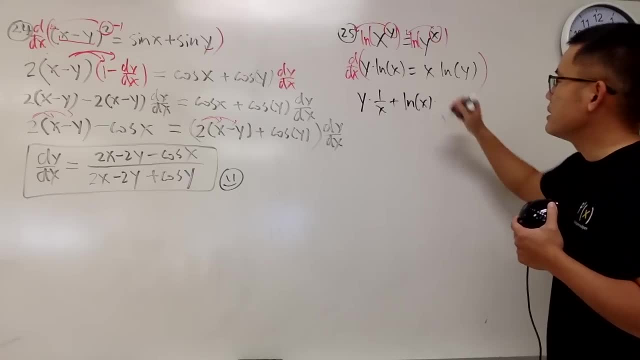 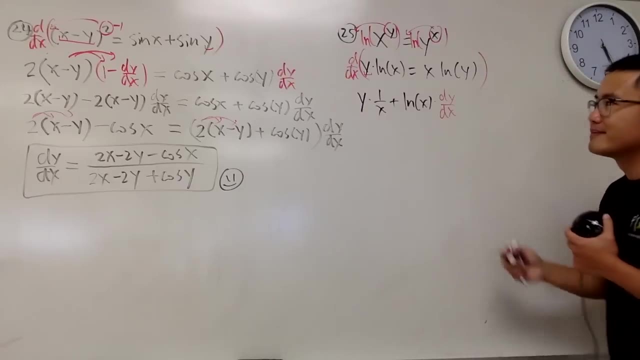 And then we add the second function, natural log of x times the derivative of the first Derivative of y is dy dx. Here is the dy dx. Aha, Then we add: I mean we have this equal to, then we have this equal to. 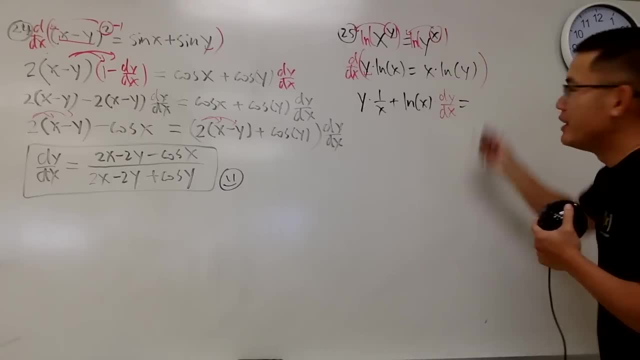 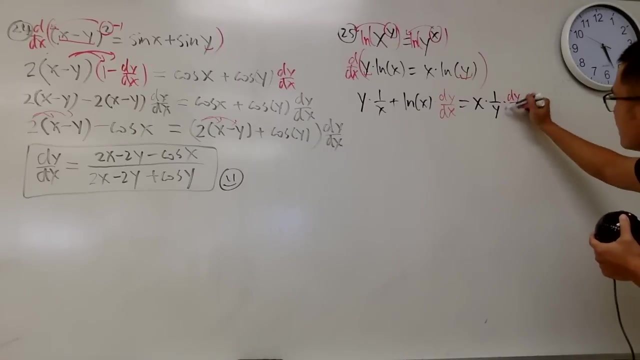 here we have the product situation again. Keep the first function, which is x times the derivative of the second Derivative of natural log of y is 1 over y times the derivative of y. thanks to Chen Lu, Here is the dy dx again. 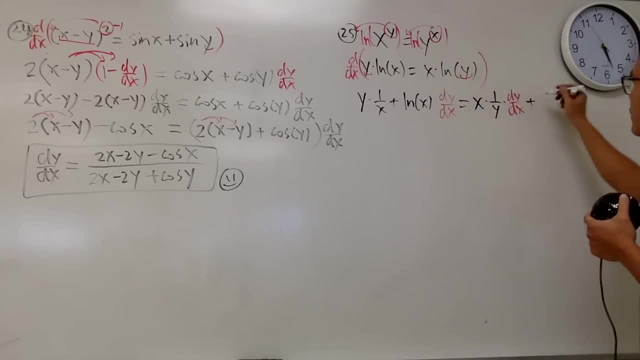 Right. And lastly, we have to add the second function, which is natural log of y times the derivative of the first, which is just a nice 1, right there? Okay, so that's the idea, Well, well, right here. 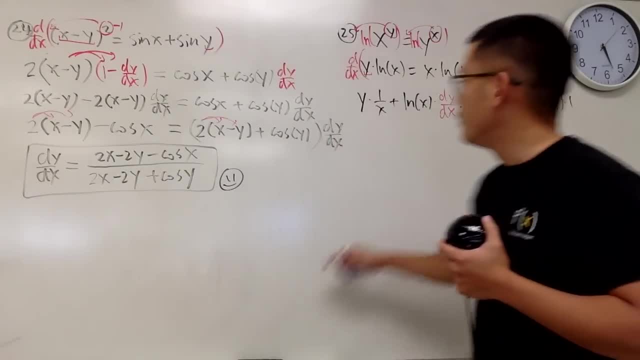 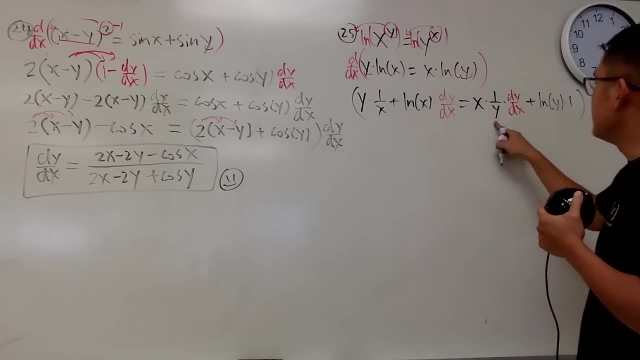 again, we see that we have an equation with fractions, so we have the x and y. So perhaps let's multiply everybody by this denominator and that denominator. Let's put down the x, y all the way at the end. Okay, so you guys can still see this one. 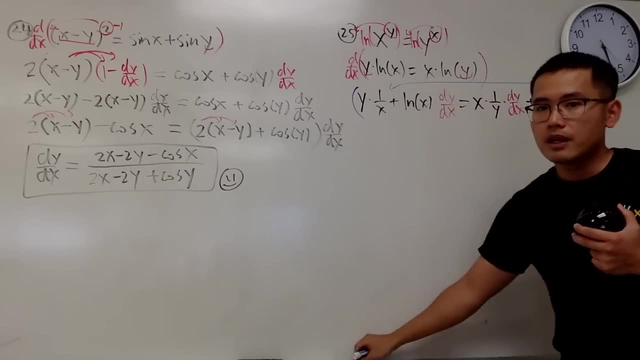 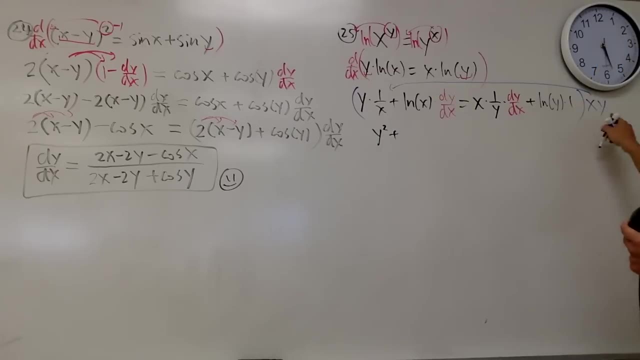 Anyway, here we go, Just draw arrows for you guys. x cancelled by y and y becomes y squared Plus this times that. so it's x, y and then natural log of x and then dy, dx, This times that. 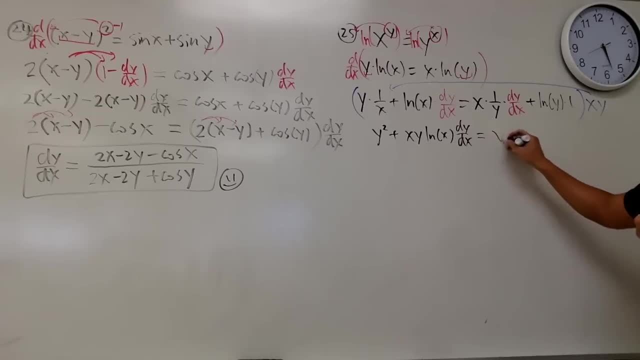 the y cancels. so we have x squared, so this is equal to x squared and this is dy dx and this is x y. oops, x y. natural log of y, Like that You know back here. 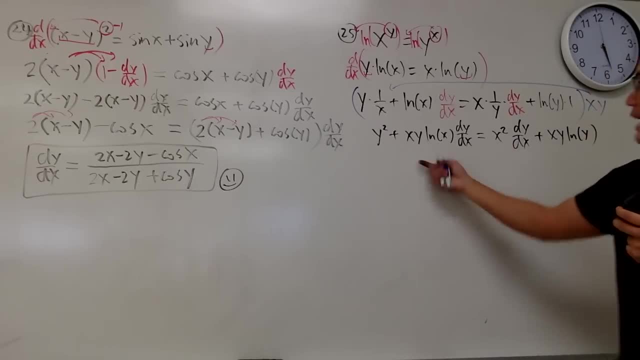 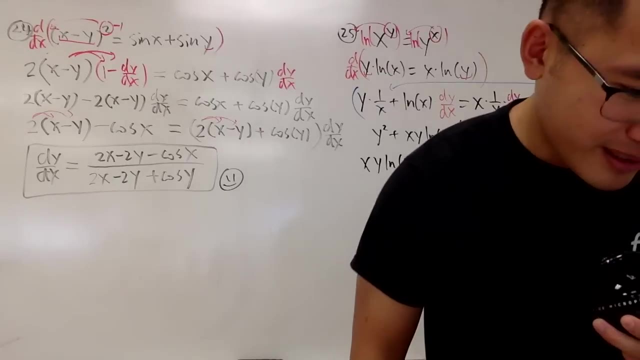 Now move this to the other side, move that to the other side. so we have this right here. Okay, I can just keep it. x y natural log of x. Hold on, let me see how I subtract, Yeah. 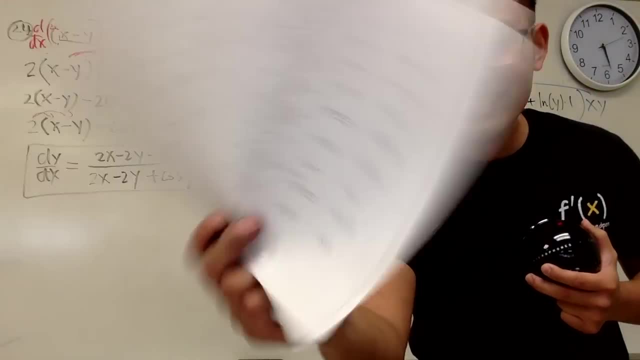 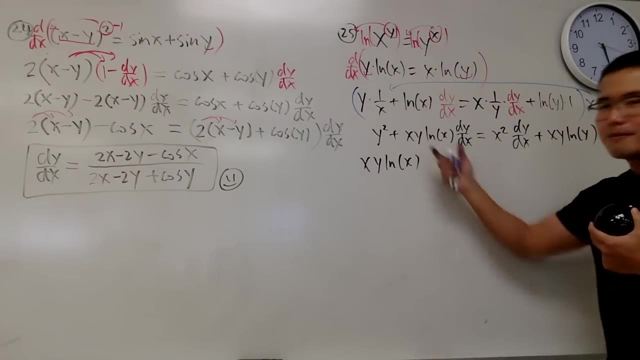 I did it this way because that's what I put down for the answer choices. Of course, if you subtract the other way, that's okay too, and then you'll just get the backwards version and then it's actually equivalent, so that doesn't matter. 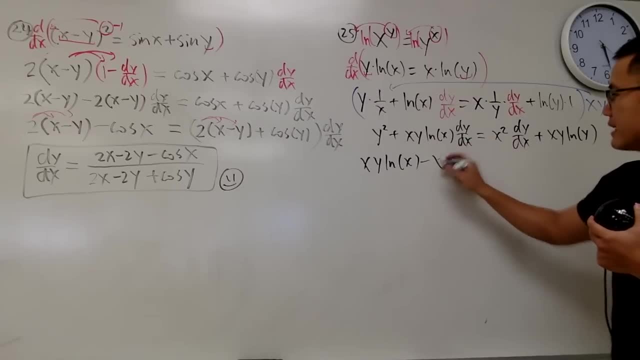 Anyway, I will move this to the other side. so we have minus x squared and we will of course factor out the dy, dx, put it at the end and this is equal to. we have this right here first, which is x, y. natural log of y. 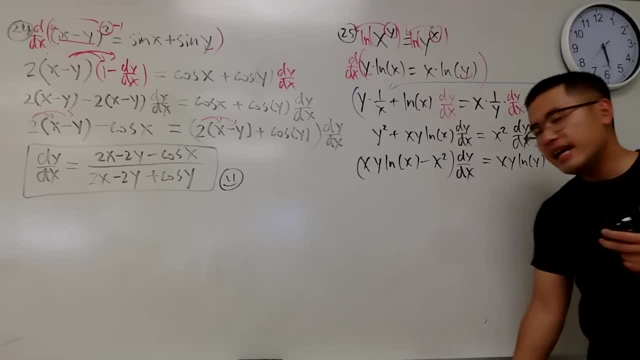 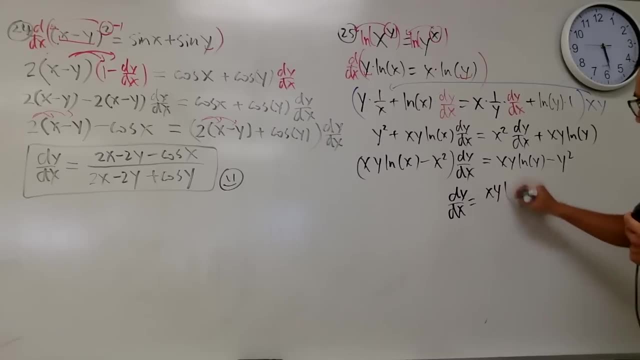 and then minus y, squared like that In the end. divide this on both sides and we'll be done. So finally, dy dx equals x y natural log of y, minus y squared all over x y natural log of x. 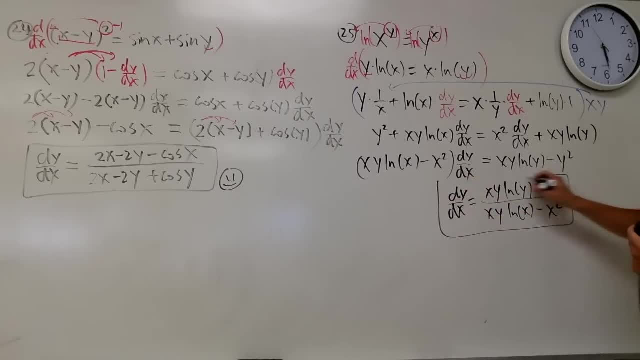 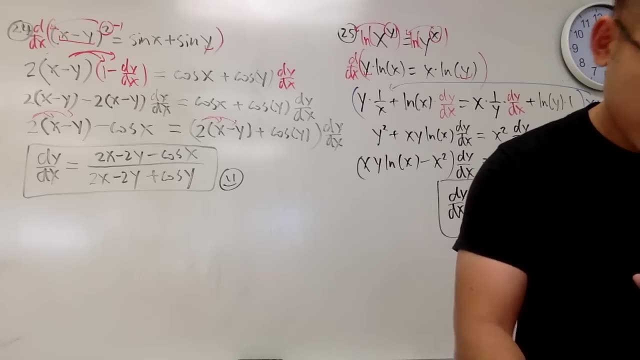 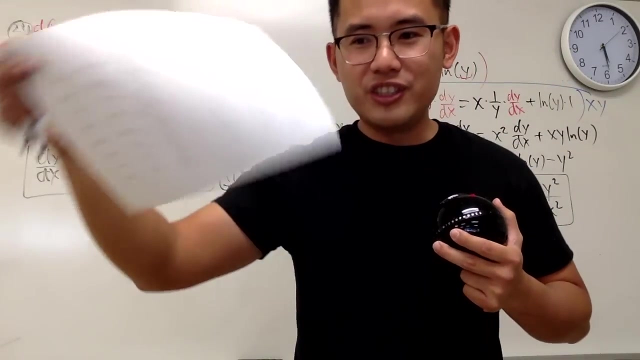 minus x squared, It has a pretty nice symmetry in my opinion. just like that. Very, very nice, Isn't it? Yeah, First pitch done. look at that, look at that, look at that. So page four actually. 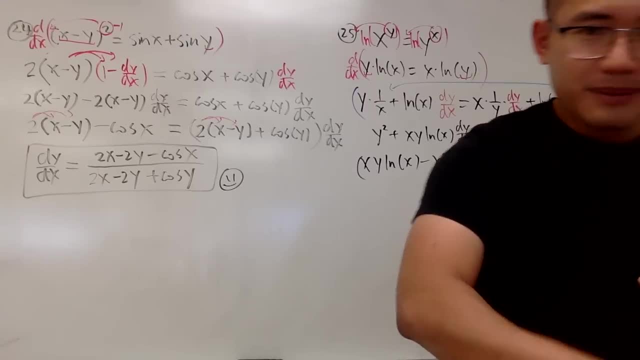 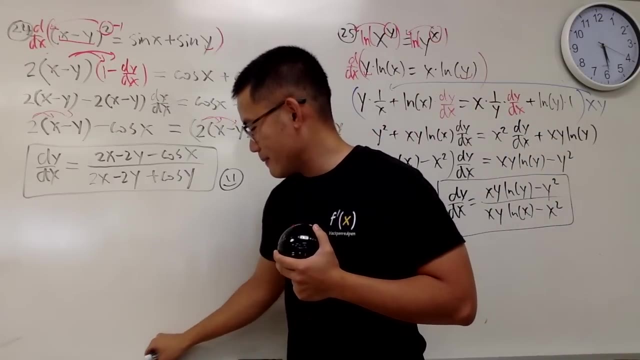 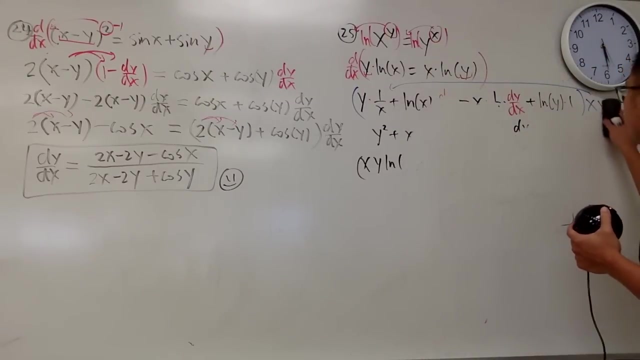 by the first sheet done. Man, I'm afraid, man, this has a lot. It's okay, It's like, seriously, for the first one, for the first integral of 100 integrals. I didn't know if I was able to do it or not. 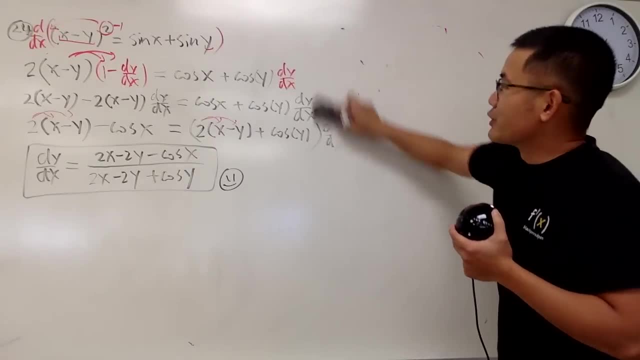 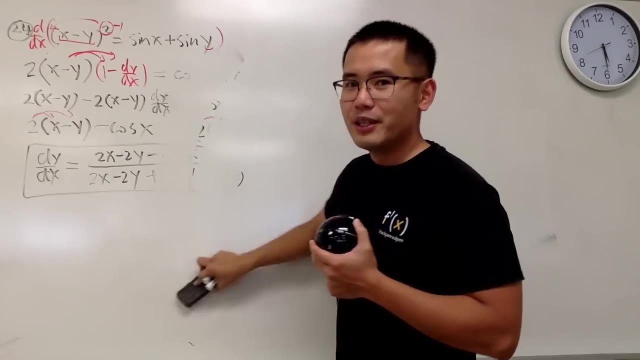 Just like my first ever marathon. I was not sure if I was able to finish it or not, But I did Just like I did: finish the 100 integrals right, And after I finished that, it's like man, I just want to do more. 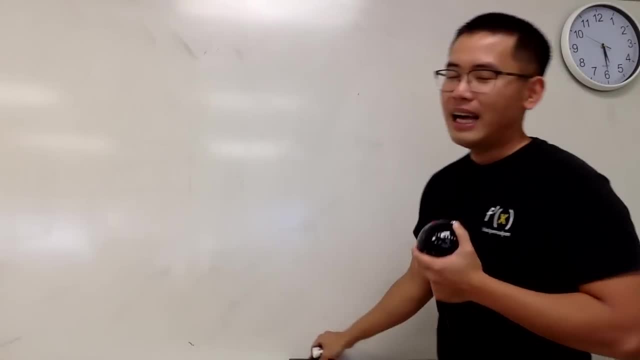 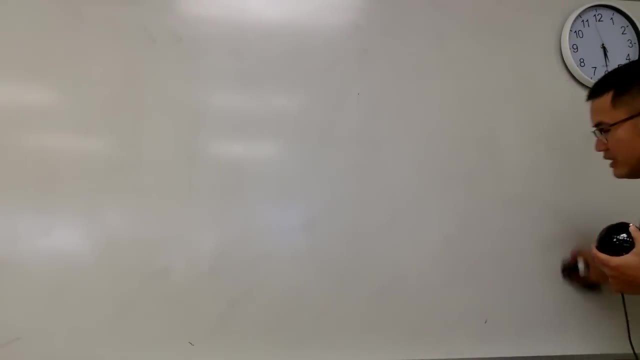 and more and more. It's just like I've been running about. I have done nine marathons in my life already. It's not a lot compared to the elite runners, but it's a lot for me seriously, because I'm not a good athlete in the first place. 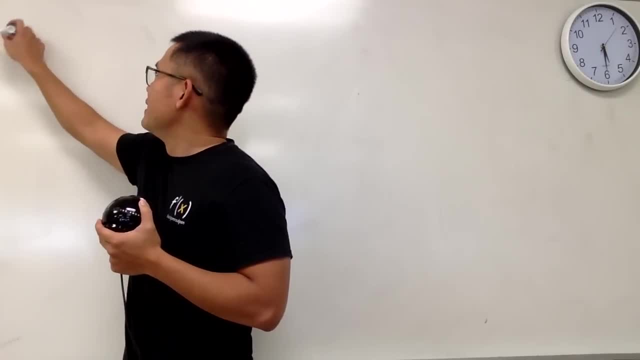 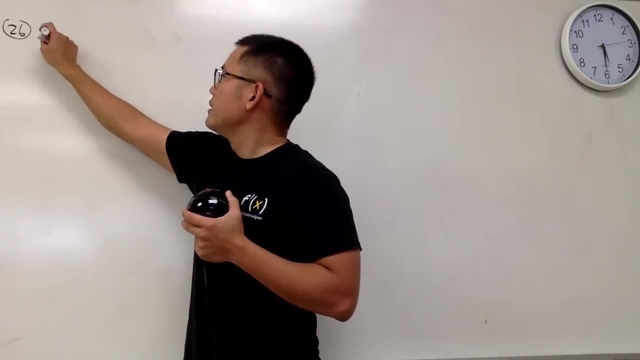 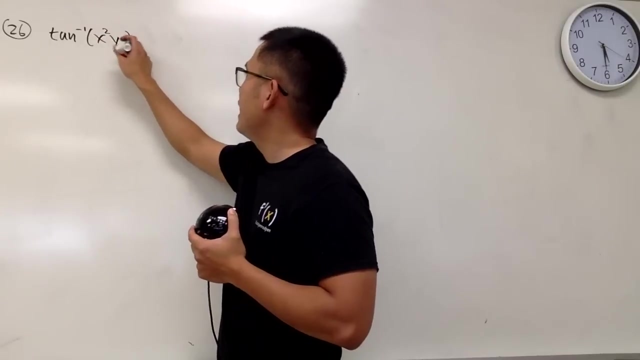 So I'm enjoying it a lot. Anyway. number 26. We are going to find the derivative for inverse tangent and the input is x times y, x squared times y, and that's equal to x plus y to the third power. 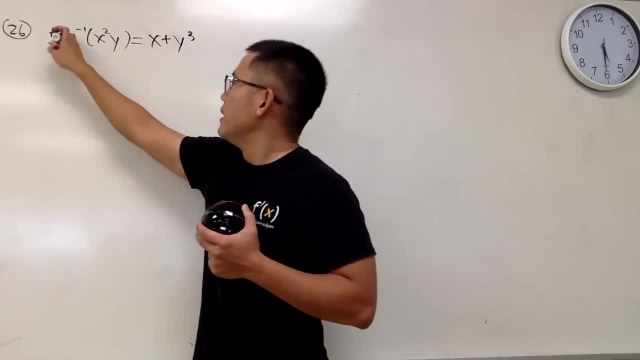 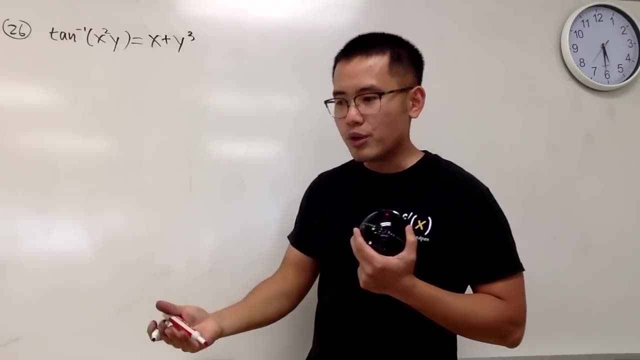 Alright, so this right here is not so bad. I don't recommend you guys to take the original tangent on both sides, though We'll just keep this right here, because the derivative in the end will be more algebraic rather than you'll see the inverse tangent whatsoever. 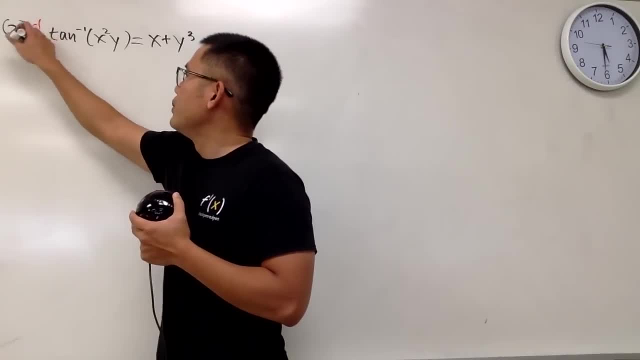 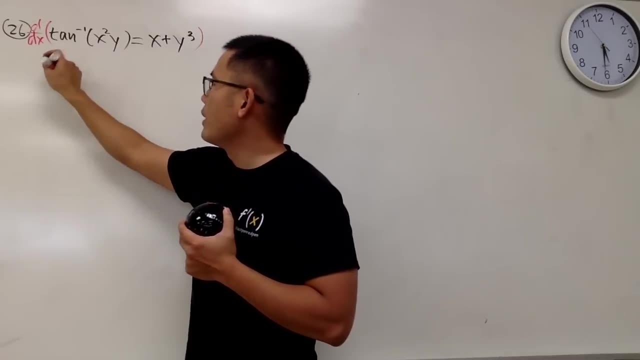 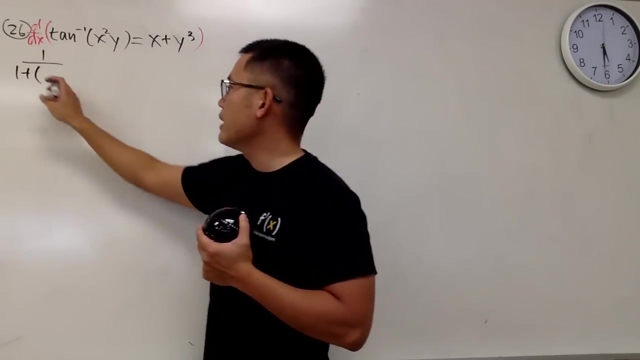 I mean, you know what I mean. Anyway, go ahead and do the derivative. Here's the deal. Inverse tangent: right here we get 1 over 1 plus parentheses. you put the input right here and you square that all the time. 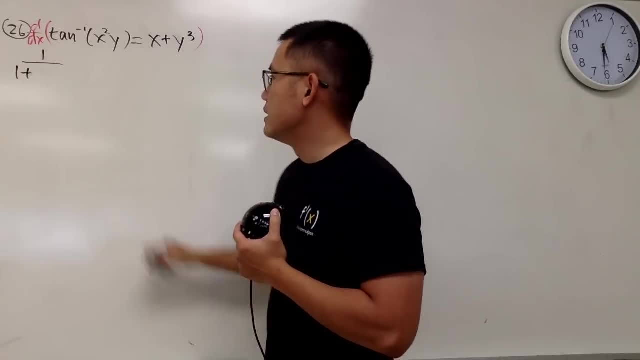 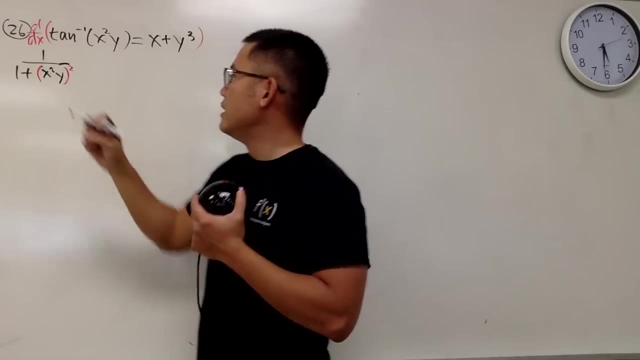 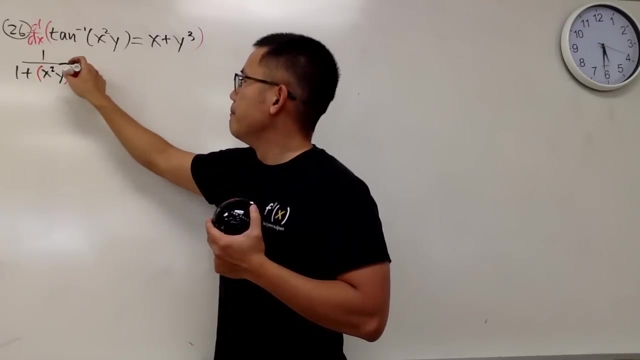 So you have 1 over 1, plus parentheses, x, squared times y, and we have to square that. This is just the general form for inverse tangent when you take the derivative of that. But we have to do the Chengdu. 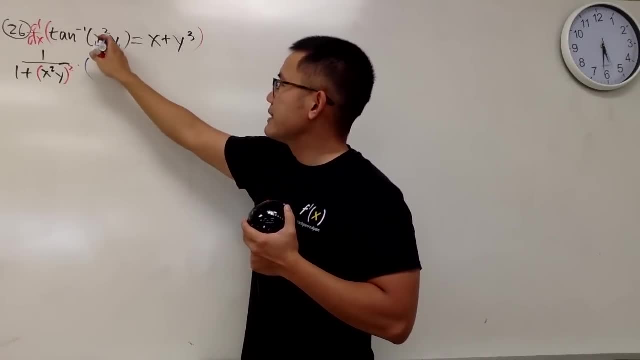 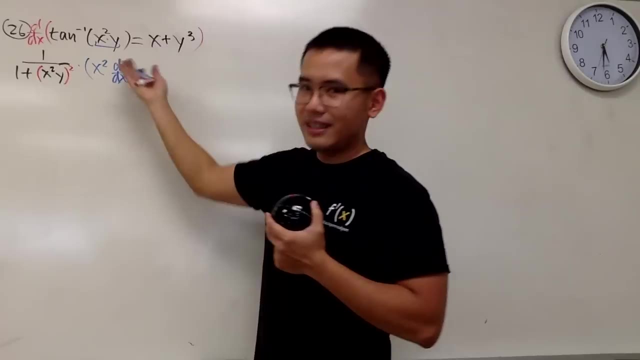 the derivative inside. So here we go: Derivative of x times y, so x squared. you keep it and then you differentiate the second, so that will be dy, dx. That's the derivative of y And we add the second function. 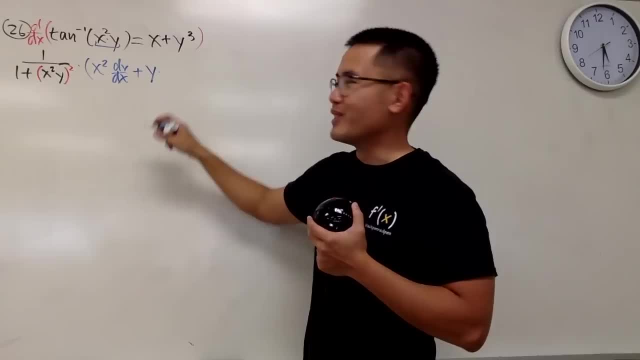 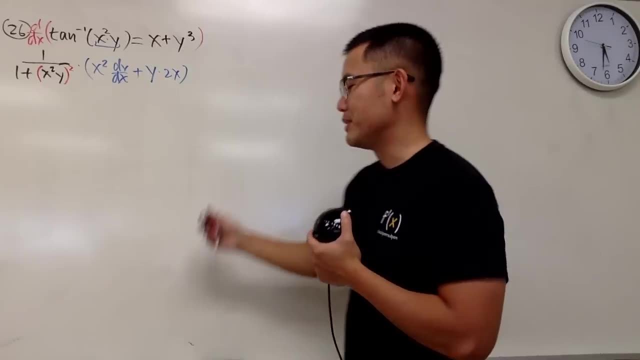 which is y times the derivative of the first, which is just 2x. Whew, just like that, Not so bad, huh? Now on the right hand side, that's the even better news, because it's not so bad. 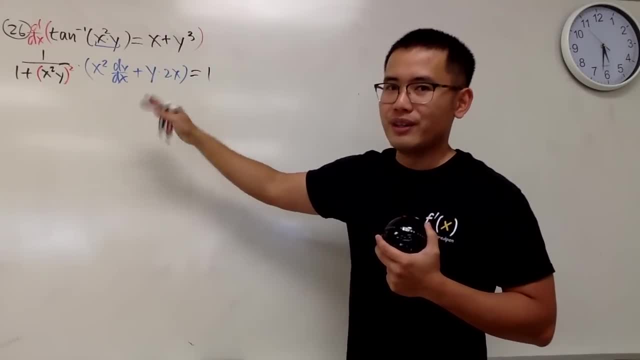 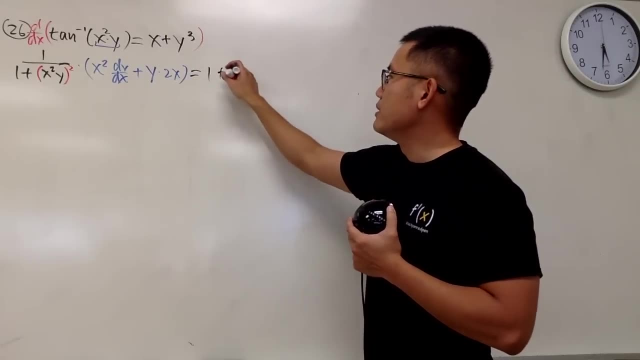 Derivative of x is 1, and you don't do product root here, it's just a sum. So you just do the derivative of x, which is 1, and you add derivative of y to the third power is 3y squared. 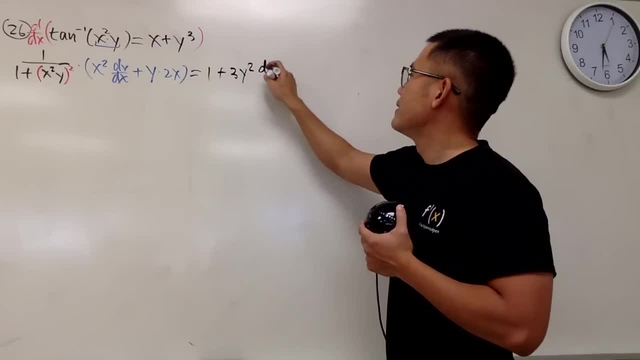 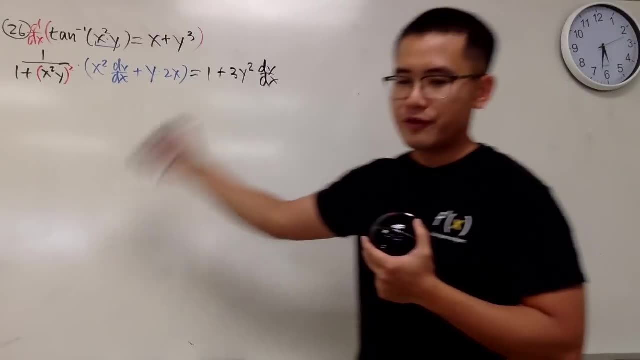 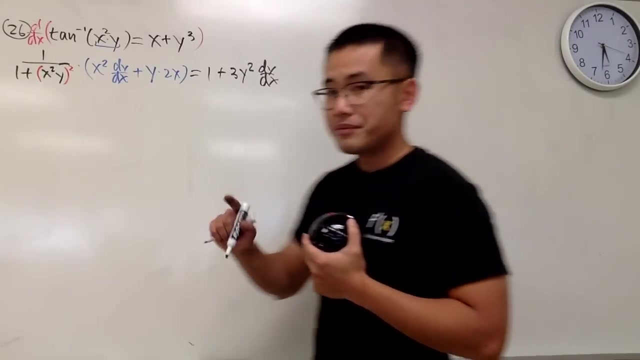 dy, dx, Just like that. Okay, Again, we have equation with fraction and I did clear the fraction before I go, so we'll see This right here. if you look at and just work this out, this is 1 plus. 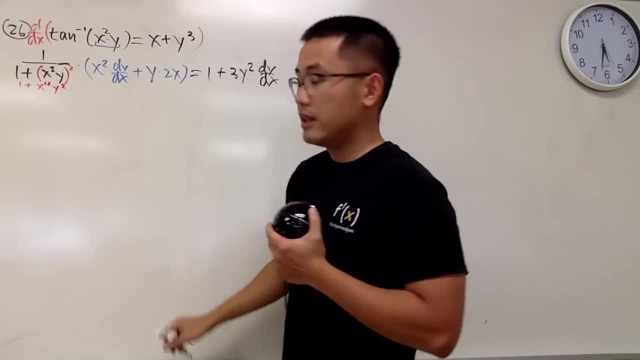 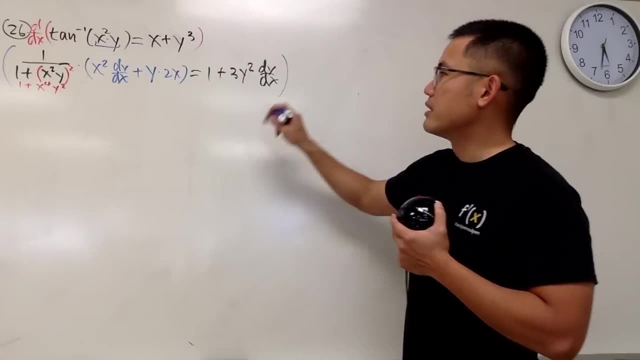 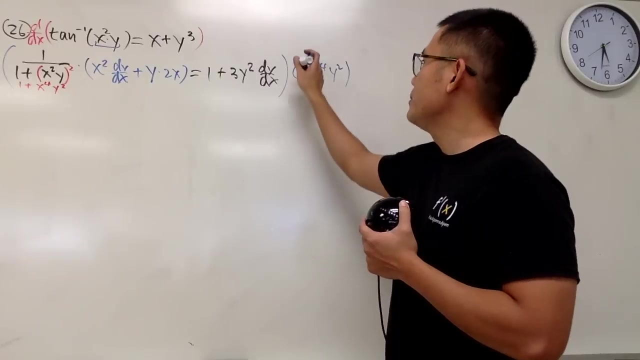 x to the fourth power, y to the second power, right? So I would prefer to just multiply everybody right here by that denominator, which is 1 plus x to the fourth power, y squared. Okay, And again, let me just show you guys. 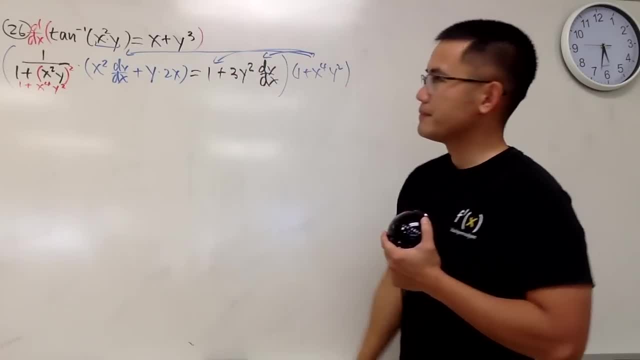 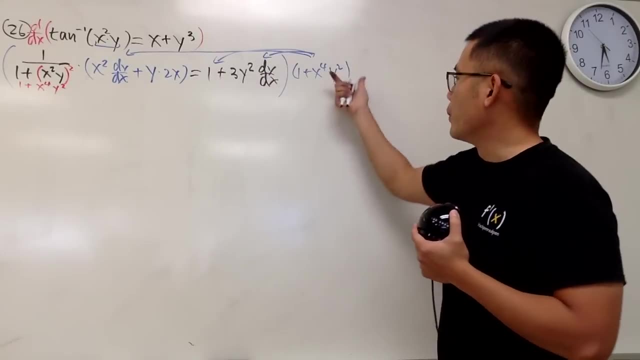 we multiply this right there and this right here and this right here. I only draw three arrows, because this quantity is being multiplied by that. When we do this, times that this and that cancel, So we just have this. 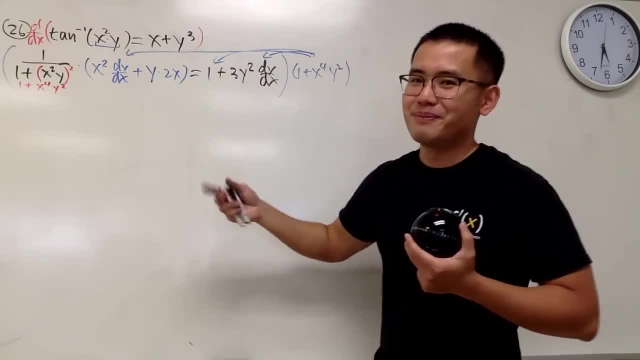 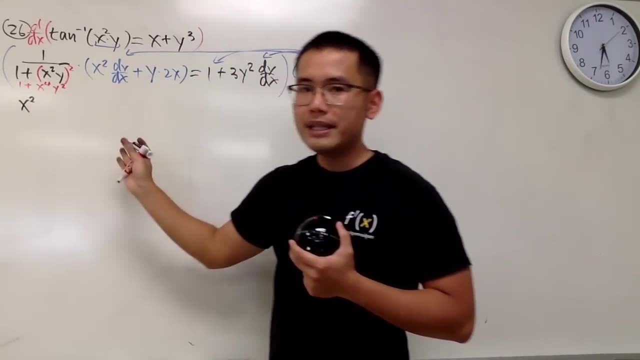 So over another series you can just think about multiplying this on both sides. Yeah, Anyway. so on the left-hand side we get x squared, dy, dx and then 2xy. So let's just put that down. 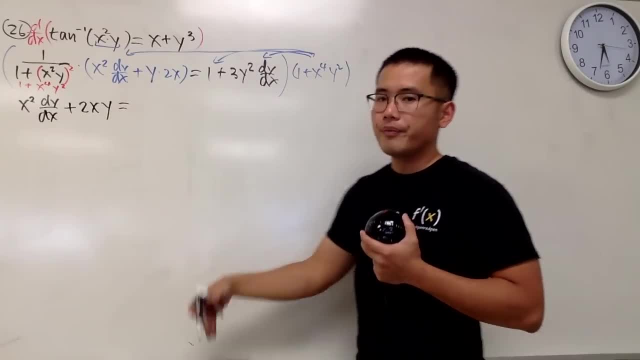 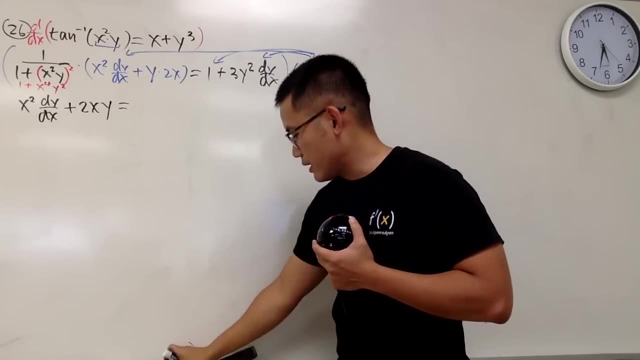 plus 2xy, And that's equal to- I will do this times 1,, which is just 1 plus. let me just put it down like this: in blue: 1 times that, so we can just have 1 plus 4x. 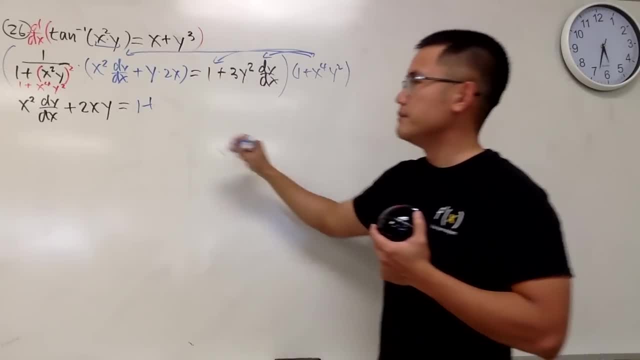 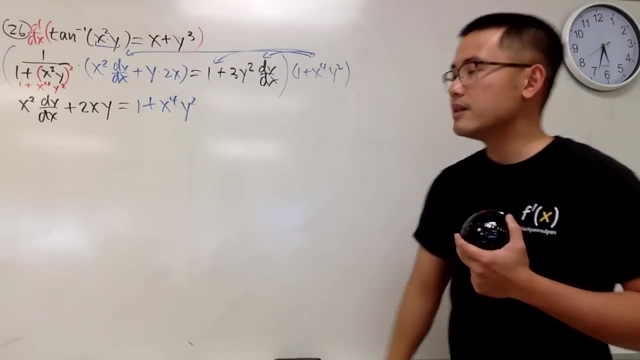 sorry, 1 plus x4, x to the fourth y squared right, 1 times that. Then what we do next is we do this times that. but it has the dy dx, So I'm not going to multiply the y yet. 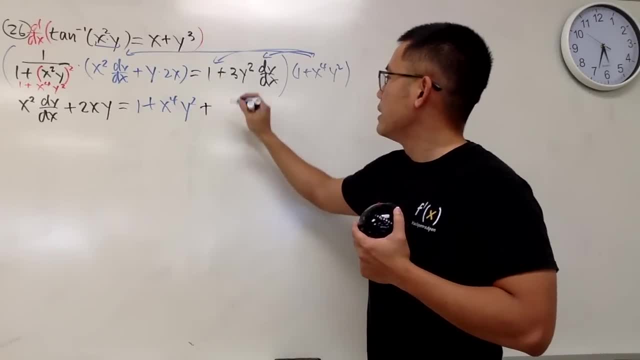 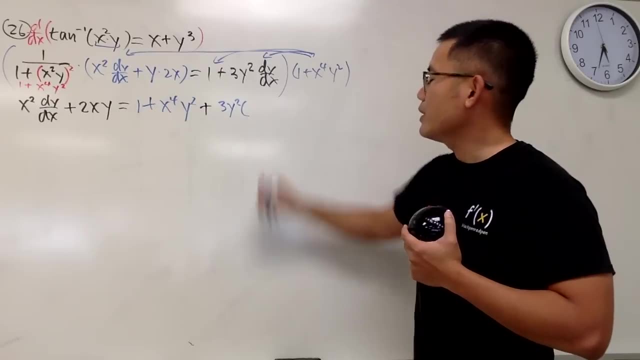 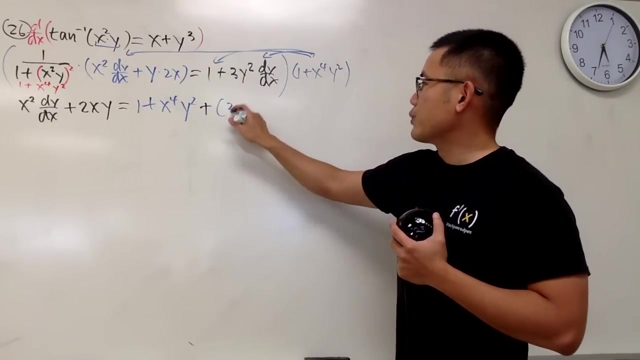 I will just keep it as plus. this is 3y square times. this thing, Actually, that's this: 3y squared times: 1 is 3y squared, And then 3y squared times, that is plus 3,. 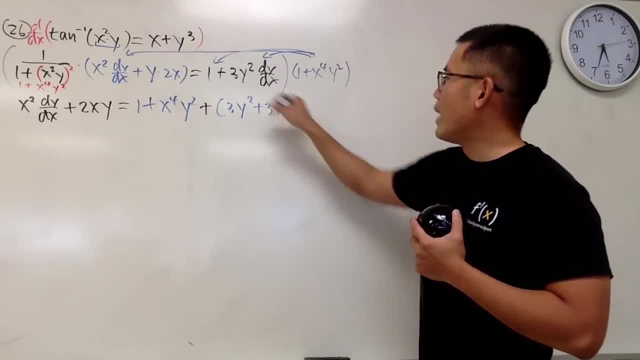 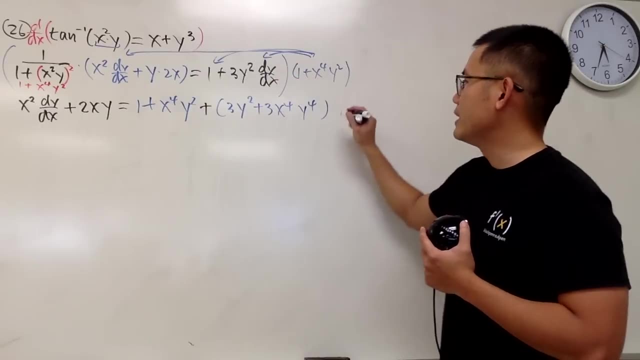 and we have the x to the fourth power, y to the fourth power, like this: Right, We'll take this and multiply by that, And then we have the dy dx. We have the dy dx all the way at the end. 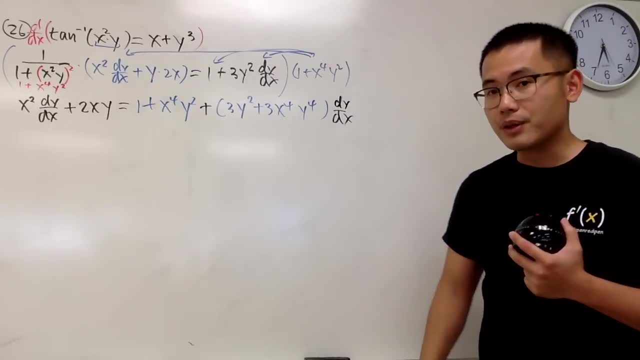 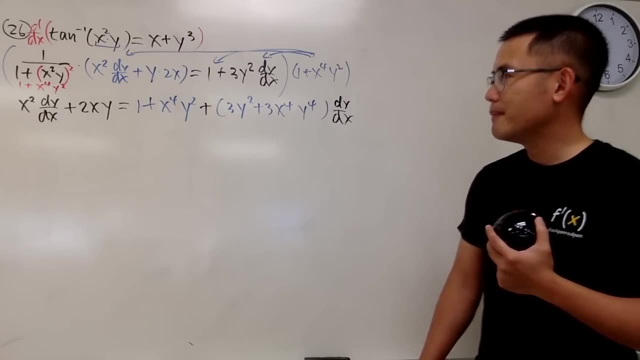 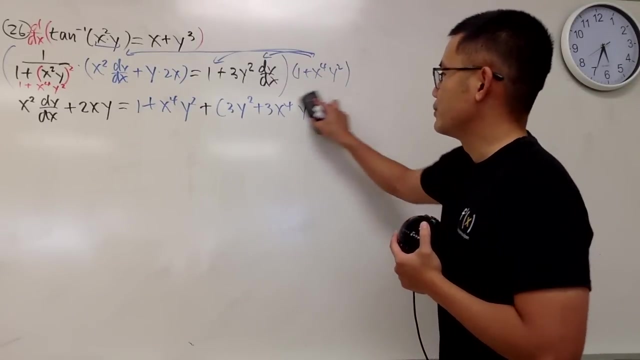 And notice I didn't distribute the dy dx. okay, for a good reason. You can do it, but it doesn't really matter. Let me see It's actually a good idea, It's? let's just do that. Let's just do that. 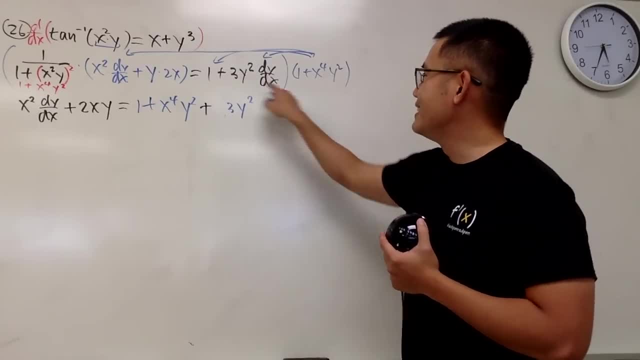 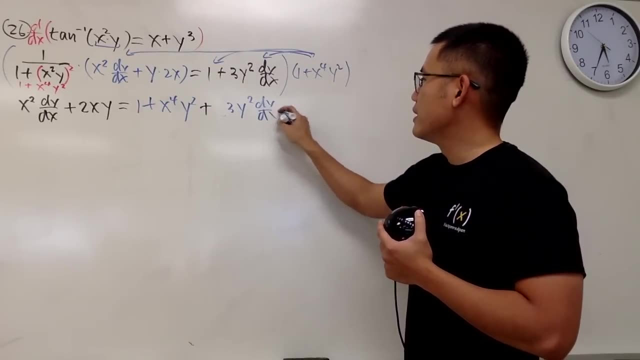 Why not? All right. So multiply this and that, so we have 3y squared dy dx times 1, so it's 3y squared, and perhaps I'll just put down the dy dx right here And then. 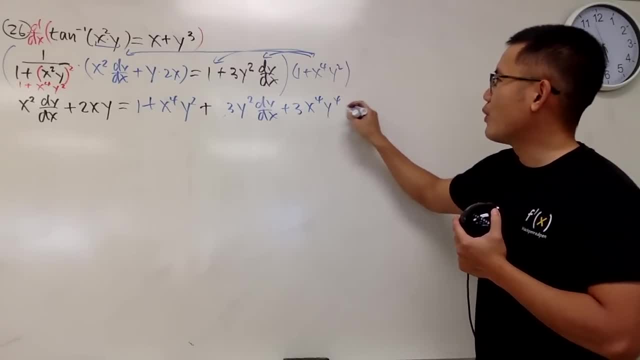 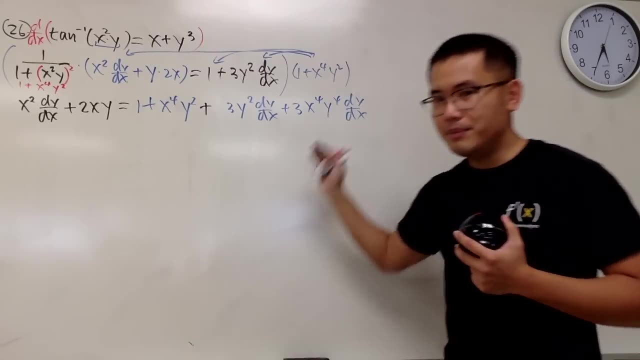 this times that we have plus 3x4y to the fourth, dy, dx. All right, so this is what we have. All right, And let's. this is it for the, for the calculus, and now, this is just the algebra part. 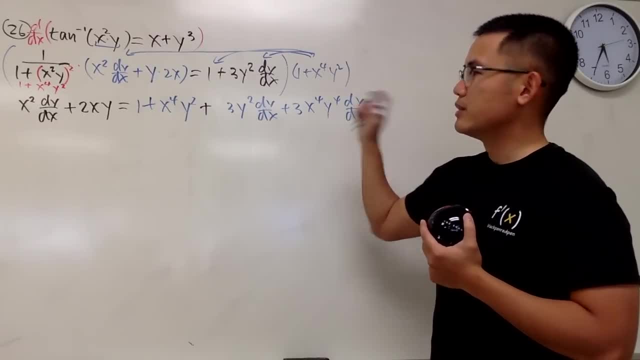 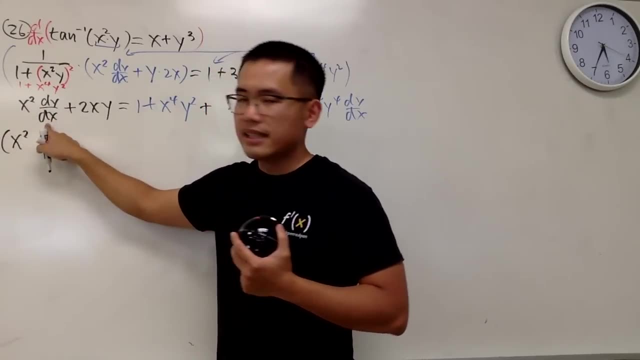 Anyway, I am going to move this, this to the other side. Factor it out: the dy dx. So you see here, right here is x squared. It has the dy dx. I will factor it out and put it at the end. 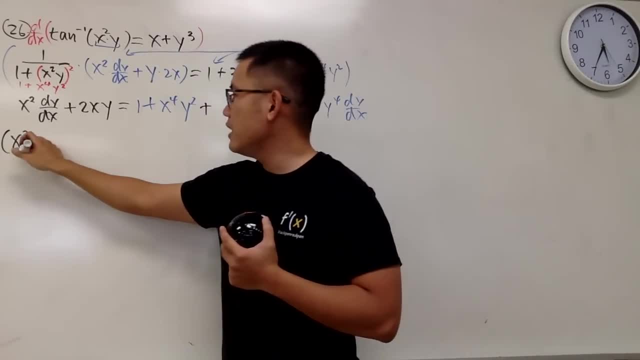 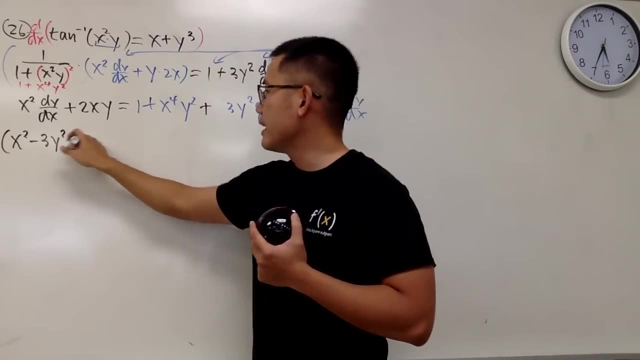 I will move this to the other side so it becomes negative 3y squared and the dy dx will be happening at the end And I will also put this to the other side. that will be minus and we will have 3x to the fourth power. 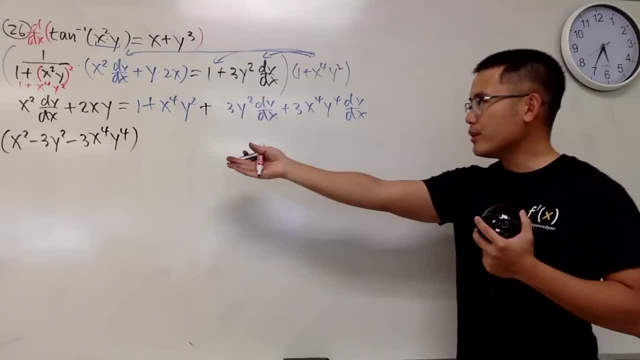 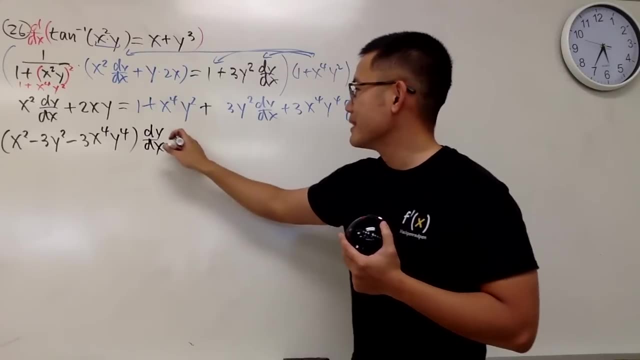 y to the fourth power. All, all in all, everybody will have the dy dx. so we just put down the dy dx at the end like this: And then we have this, this and that. so we just put 1 plus x to the fourth. 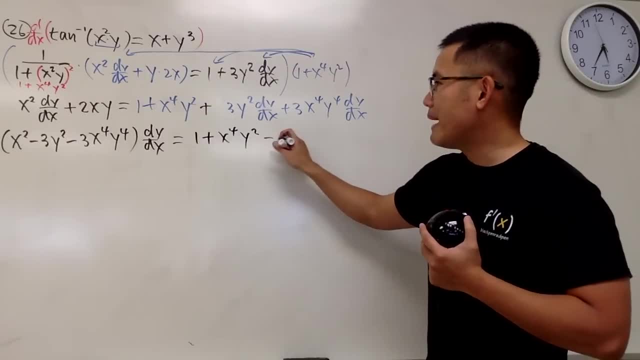 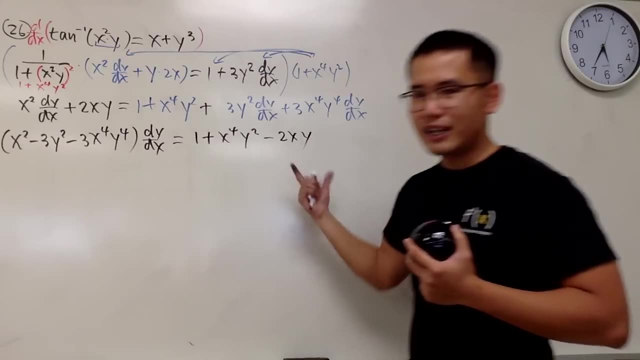 y to the second. bring this to the other side, it becomes minus 2xy. Yeah, that's pretty much it. And then divide this to the other side and we are done. So finally, dy dx equals 1 plus x to the fourth power. 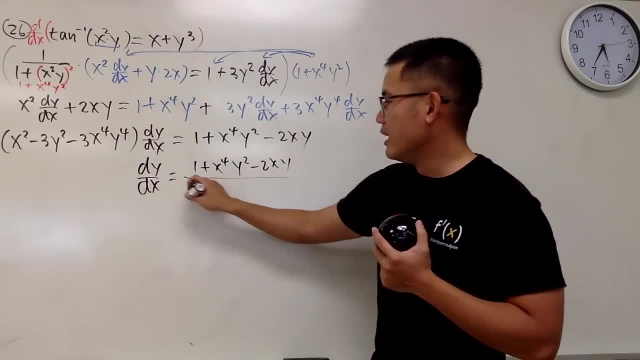 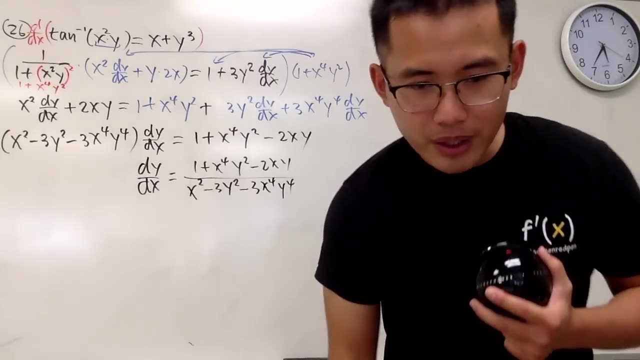 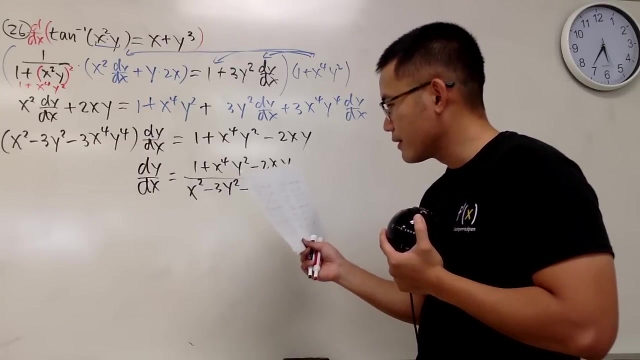 y squared minus 2xy or over that guy, x squared minus 3y squared minus 3x. y to the fourth like this, And I would like to check my answer choice to see if I can find it. 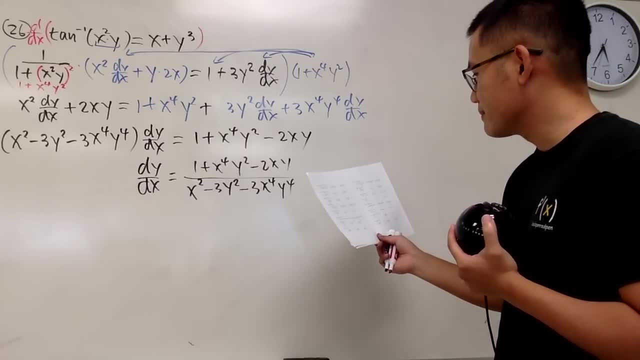 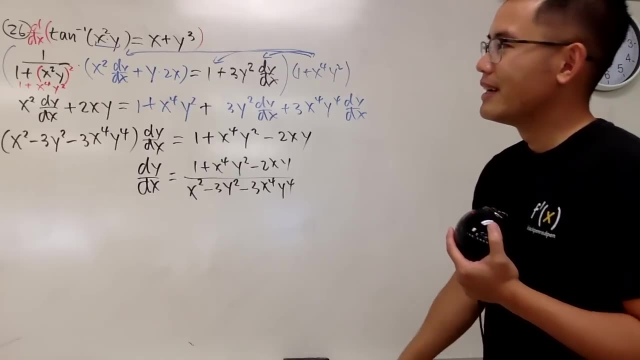 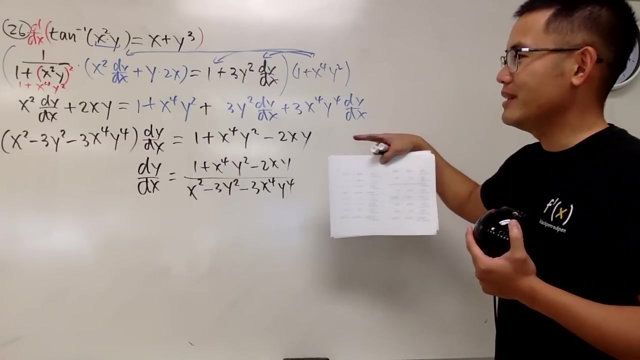 Ah, I have the other order again. So this is the travel like depends on how you want to. no, the way I did it is I moved this to the other side, so that's why you see, the answer key is: 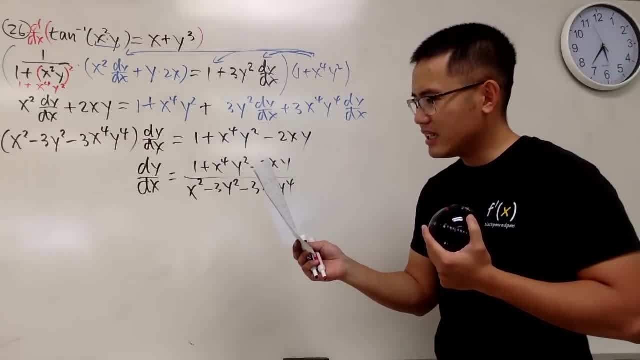 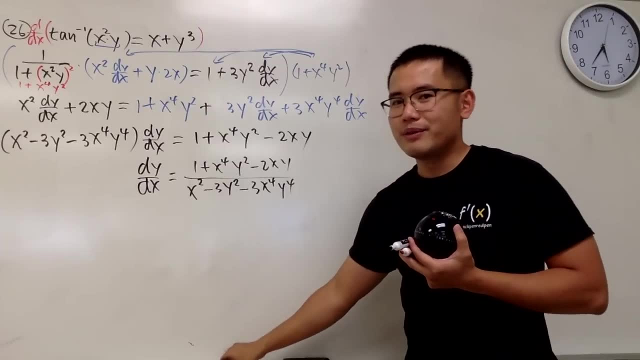 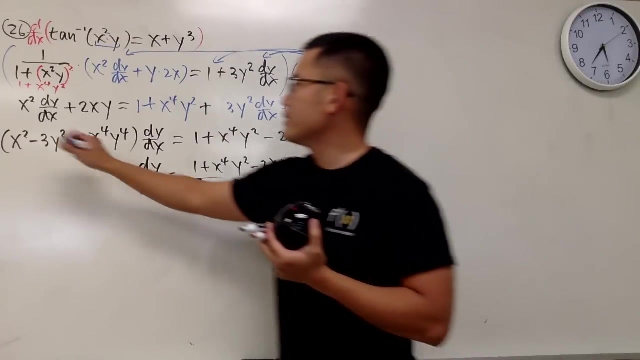 that's why you see the answer choice has the x squared being negative. Anyway, this is the part that you just have to kind of work out the ah sign on your own. The way I did it is, I put this: 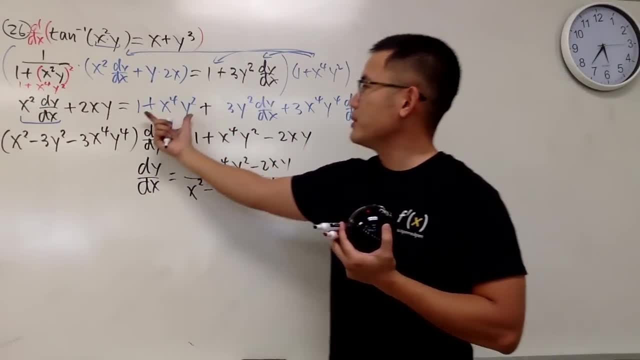 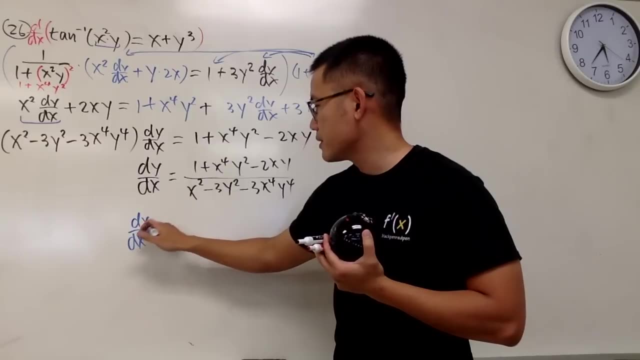 to the other side and I put this: ah on the other side. So the answer key: okay, or you can just write this down: dy dx, Let's try to see if we can do this in our head. Um. 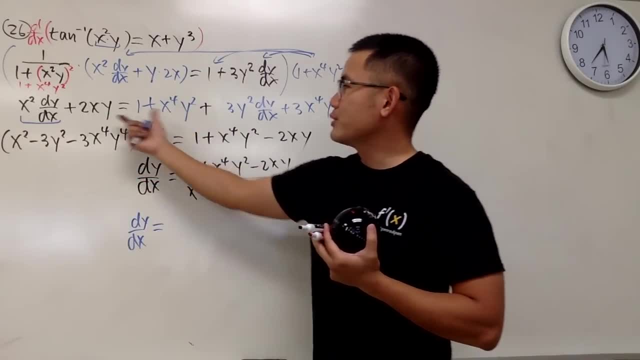 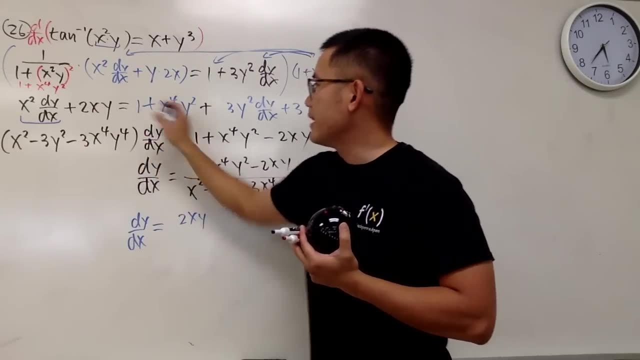 I maintain this. ah no, oh, I bring this to the other side. so I have 2xy being negative And 2x- what being sorry- 2xy being positive. I move this and that to the other side. 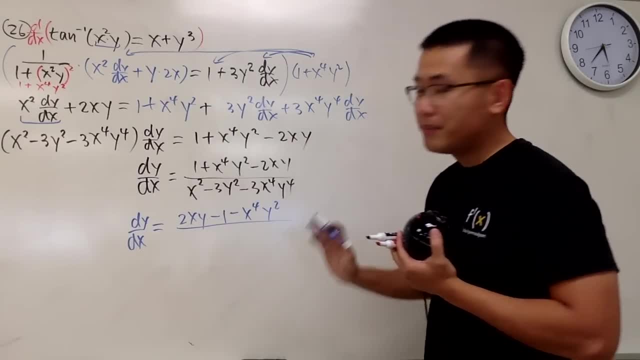 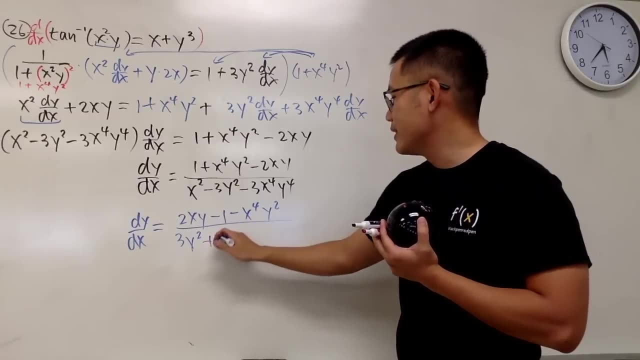 so I have minus 1, and then minus x squared, y to the second, and then divide it by: okay, I kept this and that positive, so we have 3x squared and plus 3x4, y to the fourth. 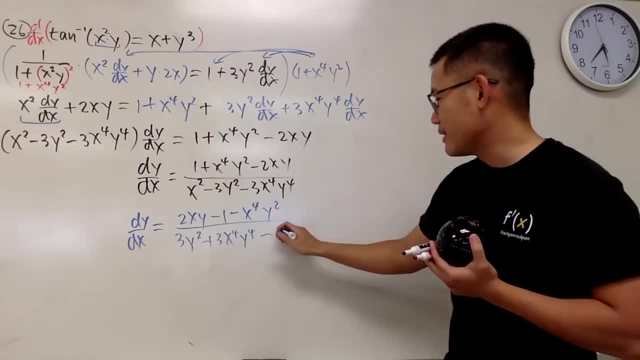 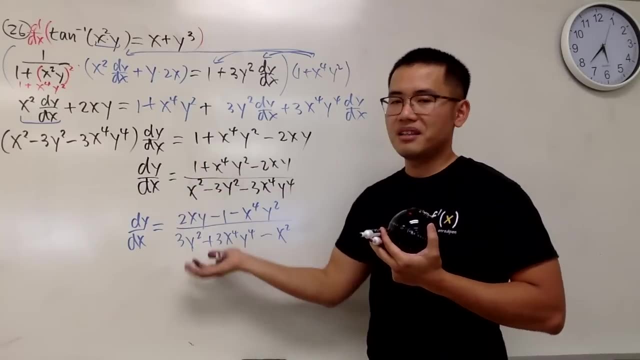 and then minus. I'll bring that to the other side. so that's minus x to the second power. So that's pretty much it. It's the same as that, but that's just all. by just multiply negative, negative. 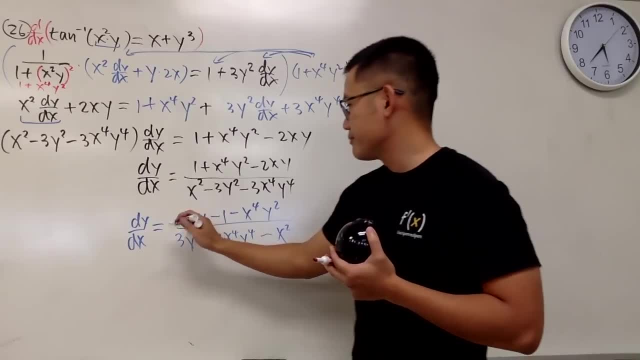 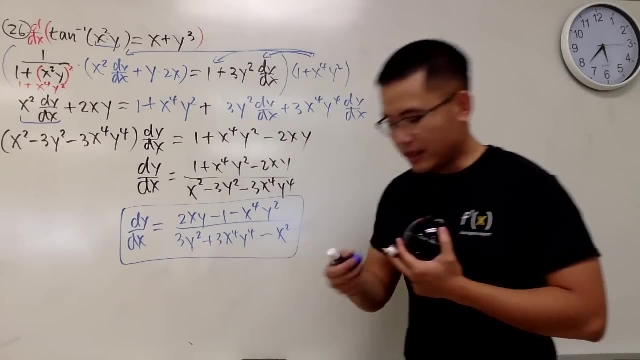 You get that. So it depends on how you- ah, how you- move things around. So I'll box this, because that's the one that I have on the answer key. On the answer choices, I have to say: Anyway, let's see. 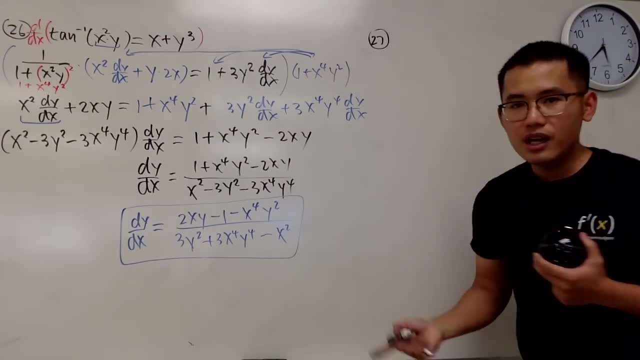 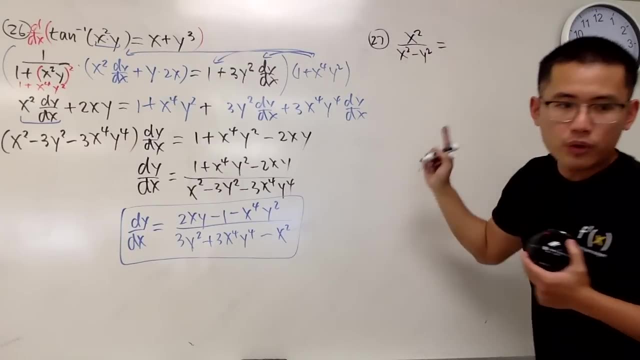 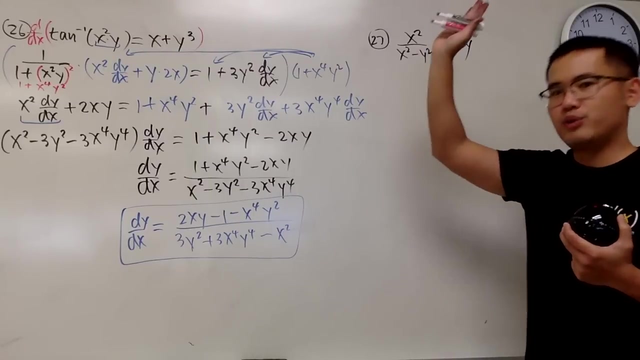 Alright, number 27.. Here we have x squared divided by x squared, minus y squared, and that's equal to 3y. How many of you guys ready to do the quotient rule on the left hand side Raise your hand. 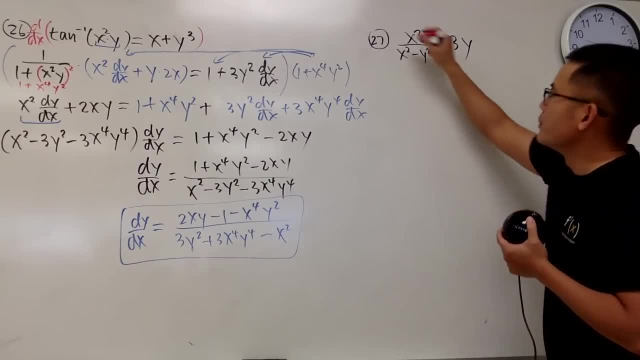 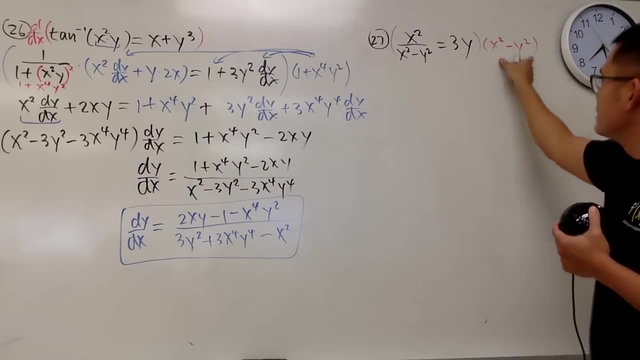 Good, Nobody, because I don't like it neither. This is what we do. Multiply both sides by this denominator: x squared minus y squared. Why? This times that will be gone. we will get x squared and that will be equal to. 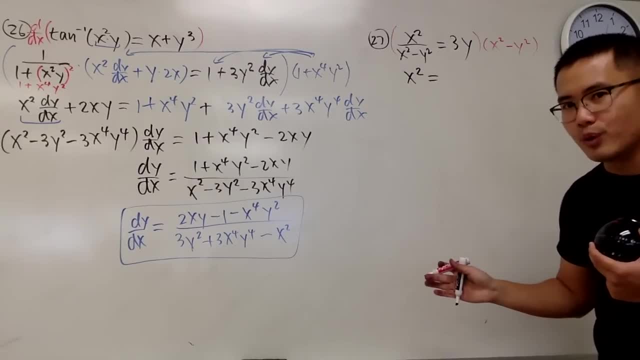 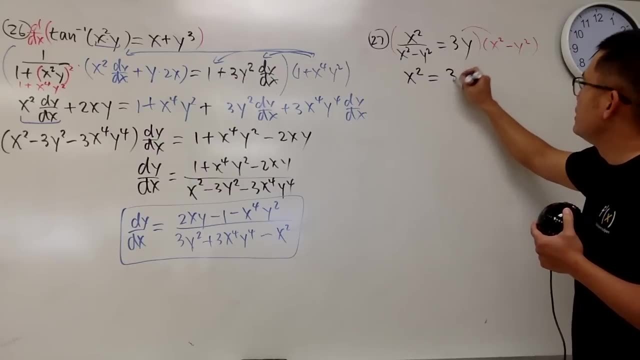 this times that Just multiply it out. We don't have to do the quotient rule if we don't need to. So when we do that, you'll see this and that together we will get 3x squared y. 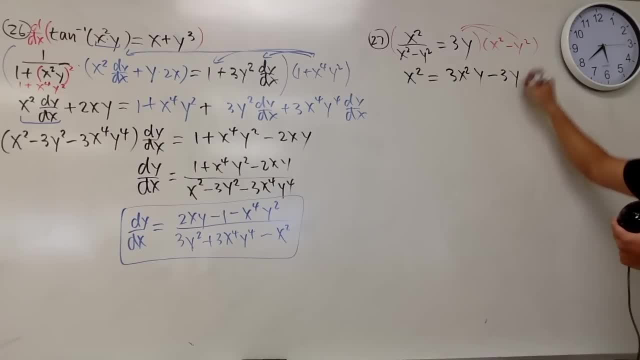 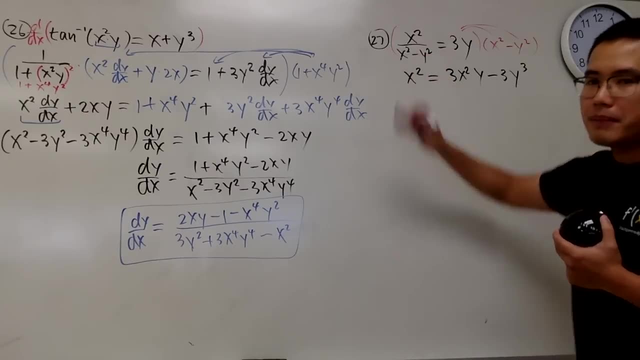 and this and that together will give us minus 3y to the third power. This equation and that equation are the same. Well, of course you have to worry about the domain. but derivative, right here, just focus on the derivative. 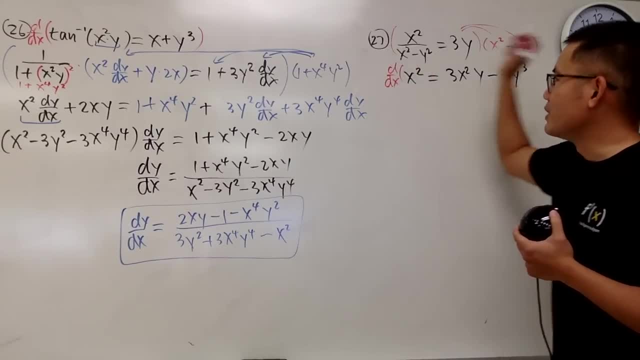 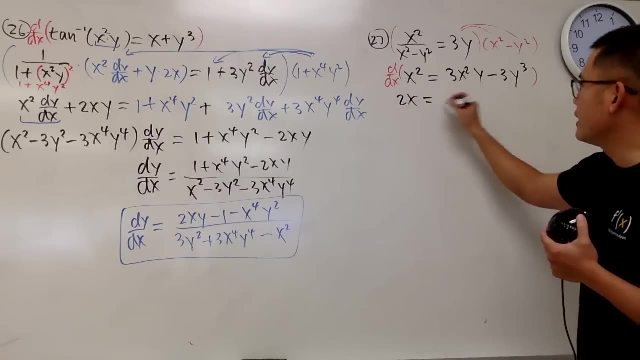 Anyway, right here we differentiate it. So d dx in action On the left hand side. this is everybody's favorite derivative equation: it's just 2x On the right hand side. okay, here we go. Product rule in action. 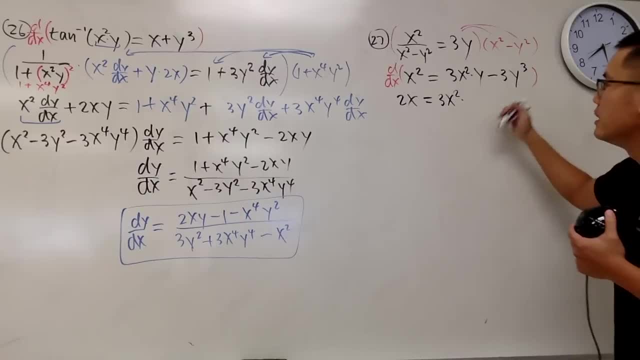 First function, keep it Multiply by the derivative of the second Derivative of y is dy dx, So just put that down. Plus the second function, which is y, times the derivative of the first, Which is: 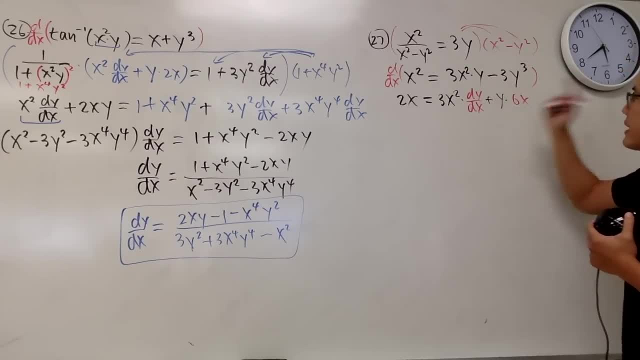 6x. Like that Right 6x. Well, right, here we have to bring the 3 to the front, minus 1. And we have minus 9, y squared and remember y is. 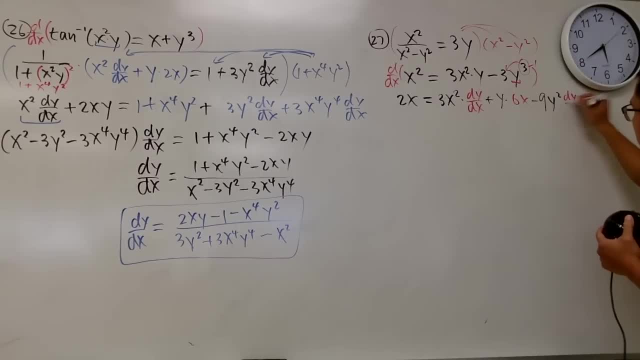 a function of x, So we have to multiply by dy, dx, Like that. Okay, so this part. I will just, of course, keep this and that on the left hand, on the right hand side. Move this to the other side. 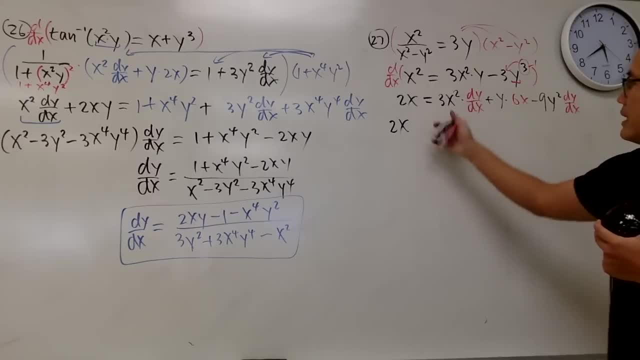 So we get 2x. this to the other side becomes minus 6xy And this right here is equal to: I can factor out the dy dx. I will write down: 3x squared. 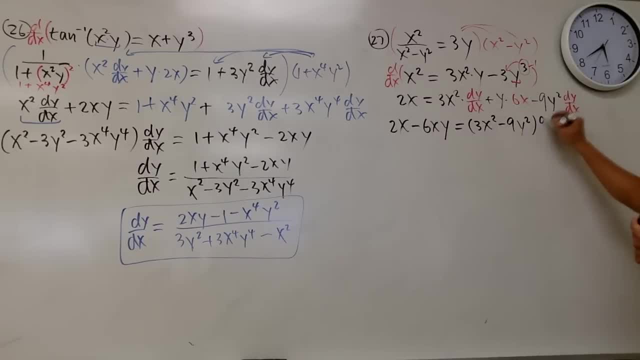 minus 9y squared and dy dx. Okay, Alright, divide this to the other side, So we get dy dx. Keep in mind, this is on the top. This is right here. 2x. 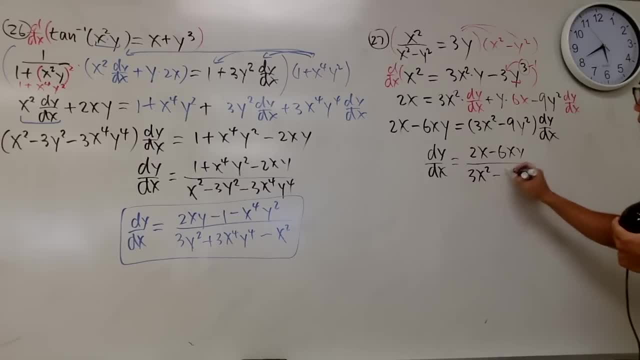 minus 6xy all over this right here: 3x squared minus 9y to the second power. Can we simplify? Uh, I think so. or did I not do it? No, we cannot simplify. 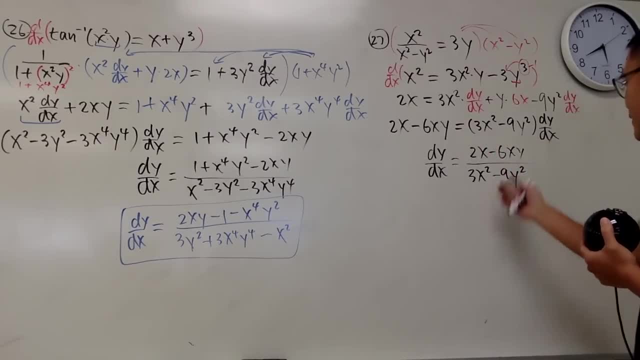 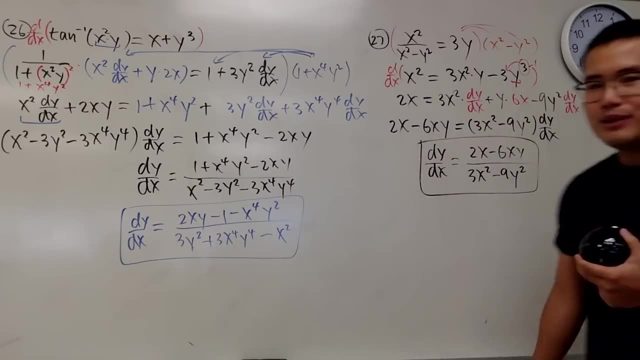 Uh, on the top we can factor out 2,, but it doesn't do us any good. I didn't even. yeah, just leave it like that, Because if you factor it out, we cannot cancel, so why bother? 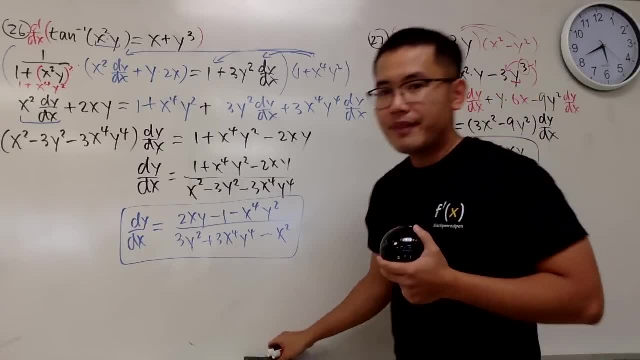 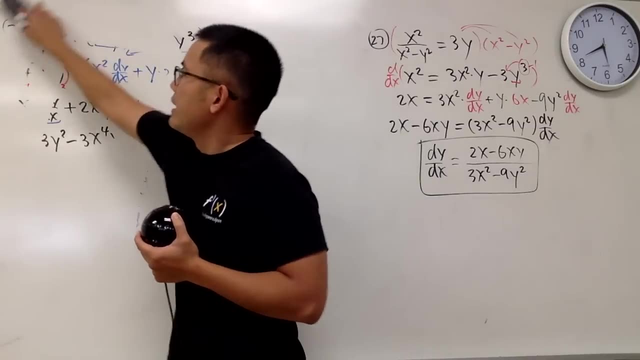 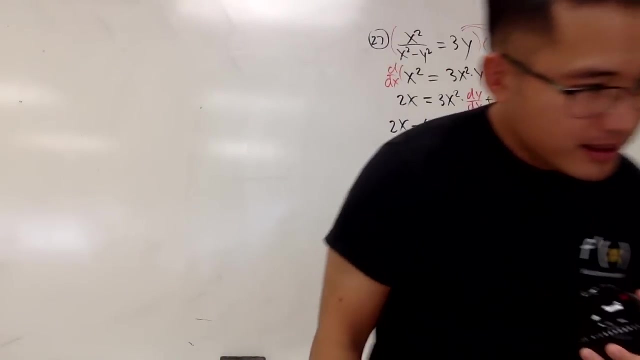 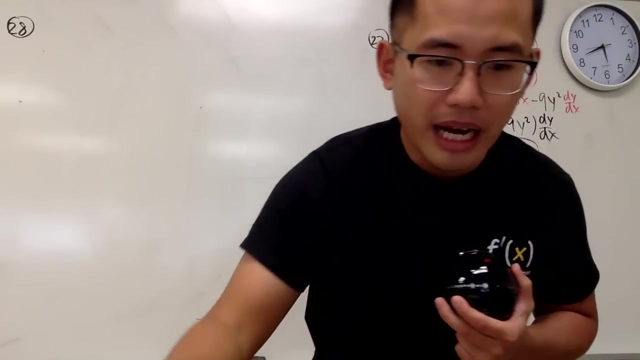 right. So that's it Alright. now I would like to do number 28.. Side by side with number 27,. you will see why. Okay, here we go, Number 28,. we have e to the 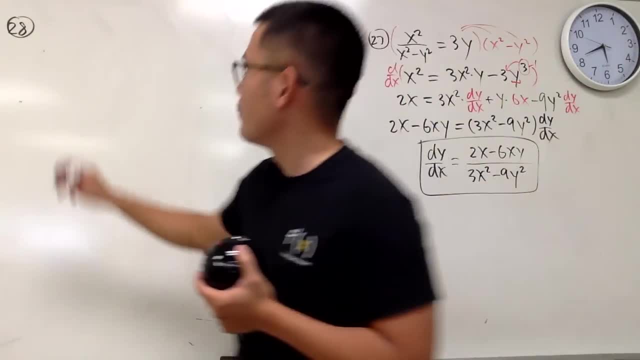 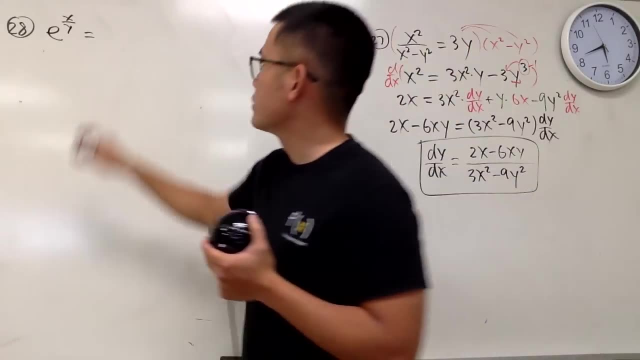 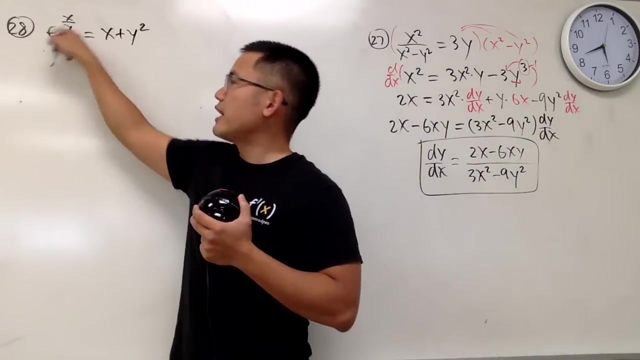 natural log of x minus, sorry e to the x over y and that's equal to x plus y squared. Alright, first thing. first, you can take the natural log of both sides and get rid of the e. 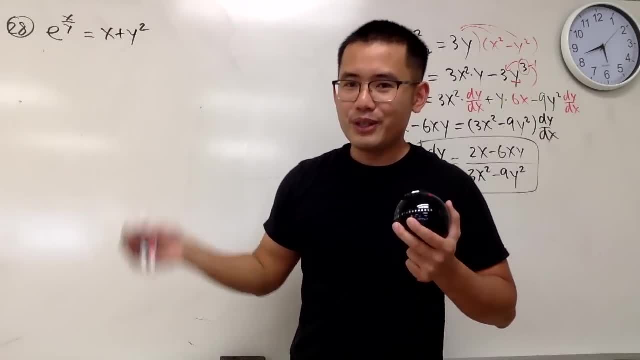 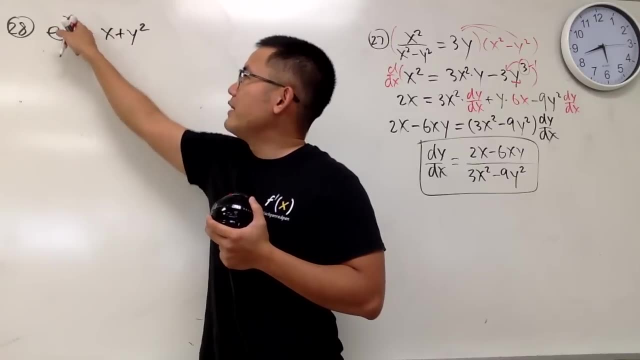 that's fine, But it doesn't really matter. you can just deal with the e, that's. that's just as fine. you just like to do the equation as how it is. Notice that we have x over y. 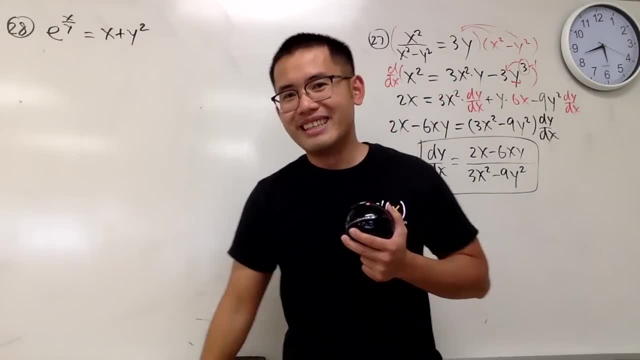 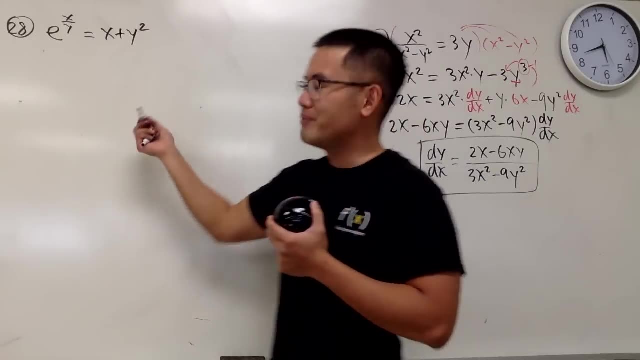 With that, we have to just use the quotient rule. If you take the natural log of both sides, you can multiply by y, and let me know how that goes. You have to use the chain rule a lot, So I think that's a trade off. 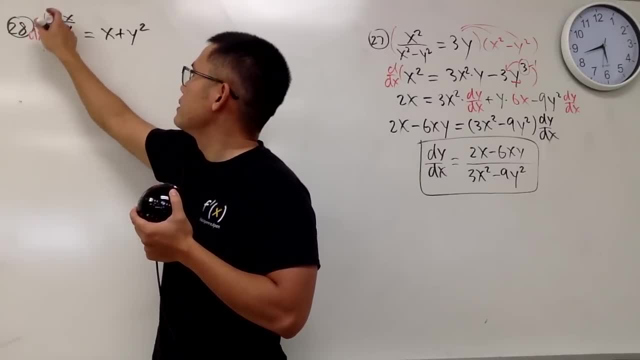 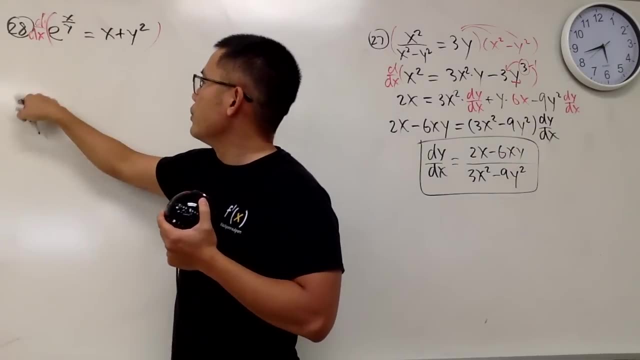 But after you. Anyway, here d dx all the way across Left hand side, e to the x, y, the derivative of that which is e to the x over y, And then multiply by the. 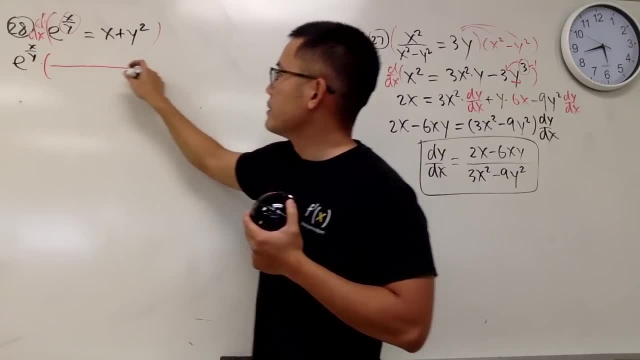 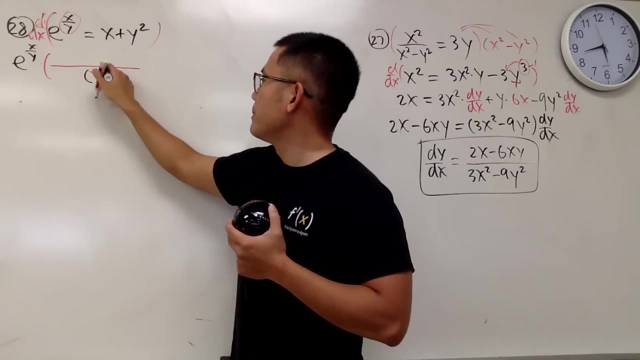 derivative of the inside And we have to use the quotient rule Here we go: Square the bottom function, which is y squared like this. So square the bottom function And then we bring down the. we break down the bottom function. 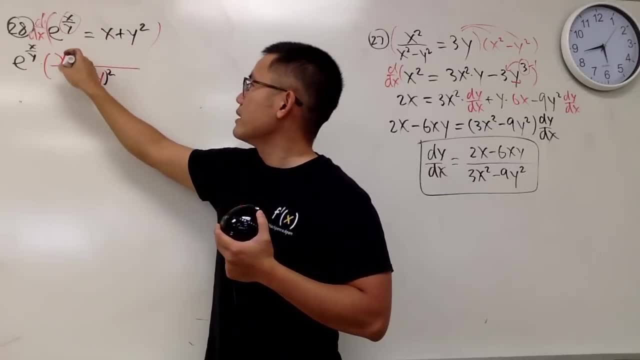 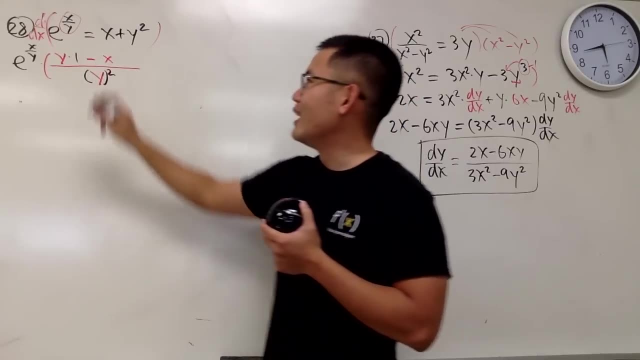 times the derivative of the top Derivative of x is one, And then we minus the top function, which is x, And we multiply by the derivative of the bottom function Derivative of y is dy, dx. 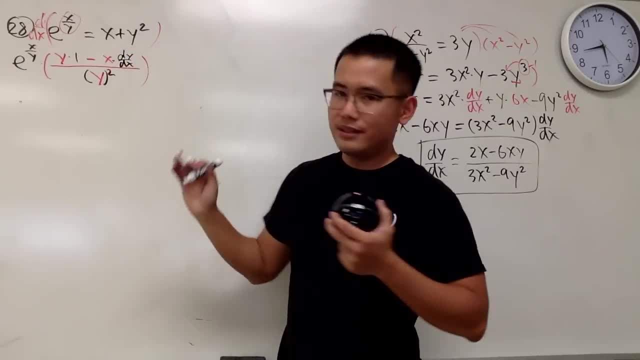 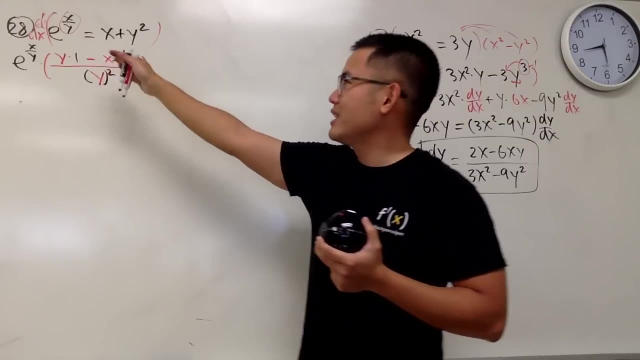 So it's like that, Done for the left hand side And then for the right hand side. this is nice if you are willing to just keep the natural, keep the e to the whatever on the left hand side. right. 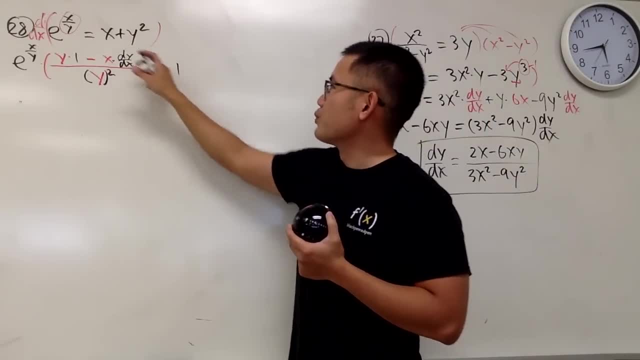 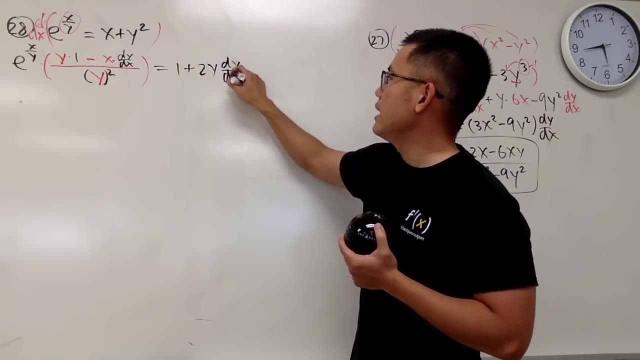 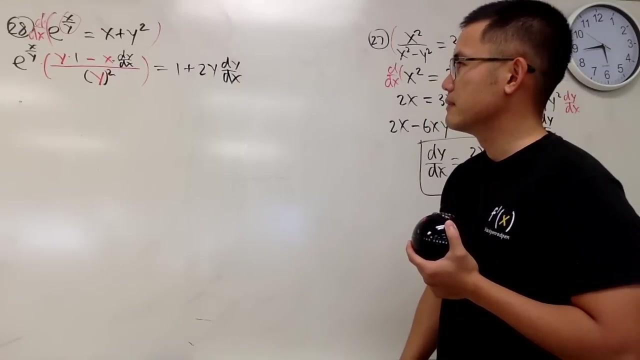 If you don't do the natural. So here derivative of x is one and derivative of y to the second power is two, y and the dy dx, Like that. Okay, Now let's do the following. 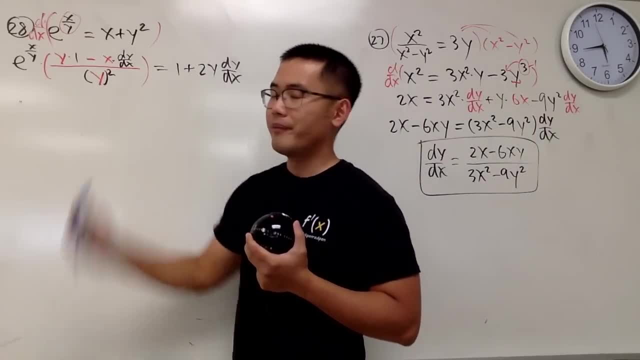 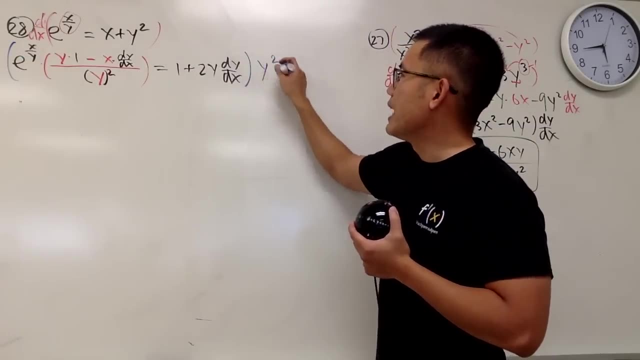 Because again, we have an equation with fraction right here, So it's a better idea to just clear out the fractions right now. Let's multiply everybody by the denominator, which is just a y square, So I will multiply this with: 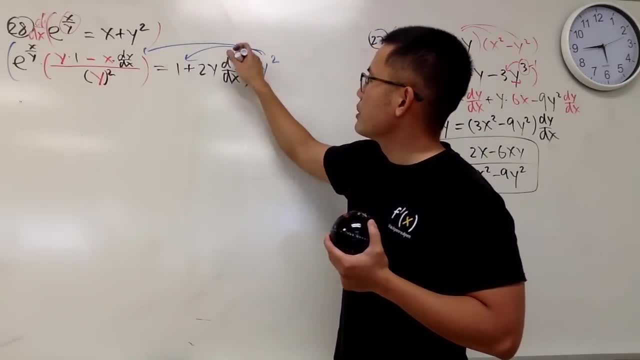 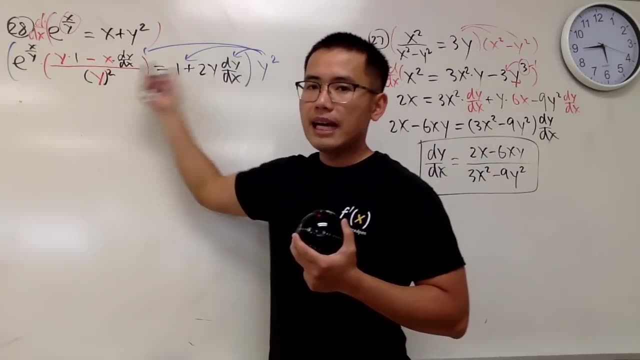 the whole thing here And then multiply and multiply. Yeah, just like that. Okay, so if you look at this part this times, that will cancel out, but we'll still have e to the x over y. 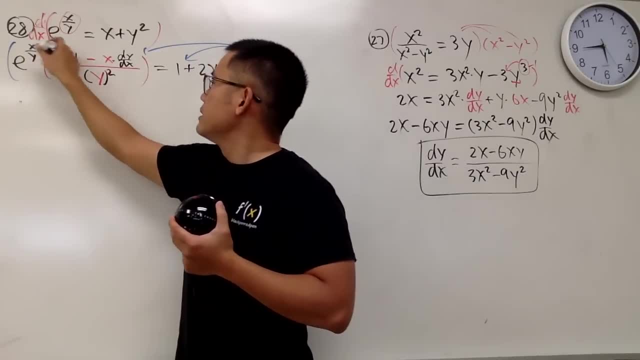 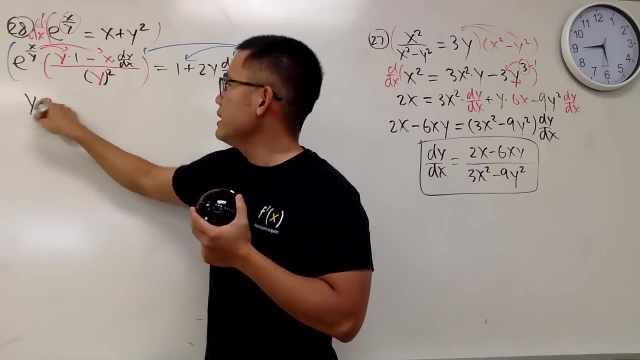 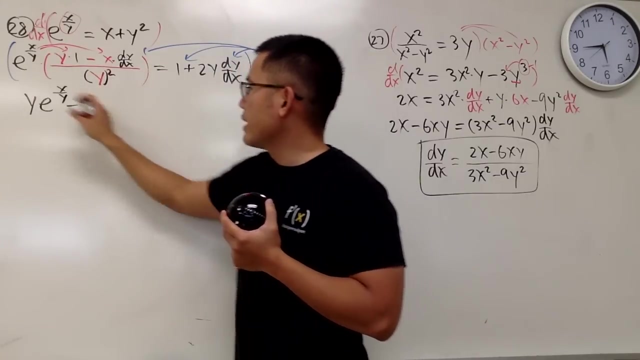 times this and that. Let's distribute this into here, this into here. So first we will have y times e to the x over y right, And then we have minus x, And then let's write that down first. 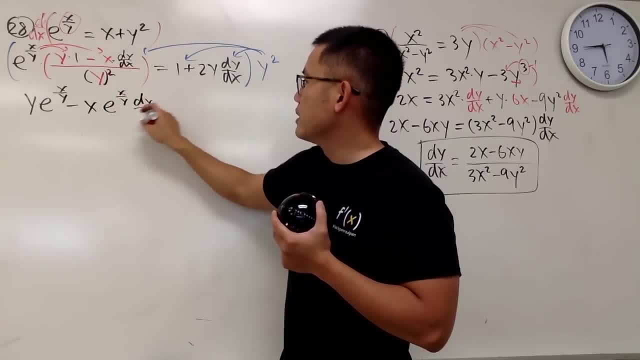 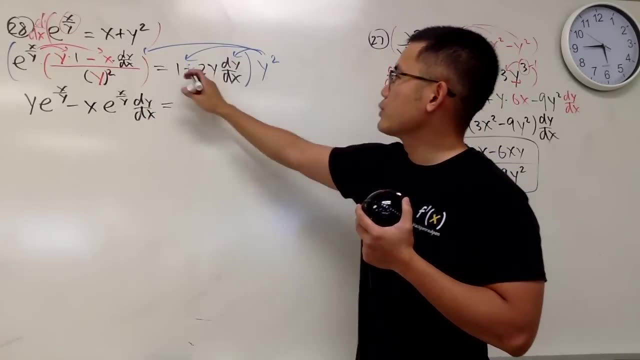 e to the x over y, and then let's put down the dy dx. You should have the dy dx all the way at the end. That's a good idea. Okay, that's it. And then on the right hand side, 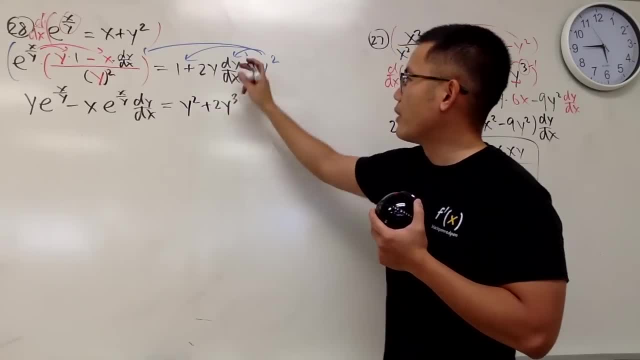 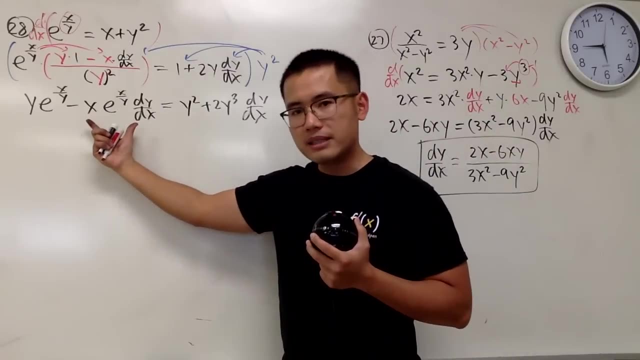 y square times. that is y square, y square times. that is plus 2y third power, And then the dy dx. Okay, to make things positive, let's bring this to the other side. Let's bring this: 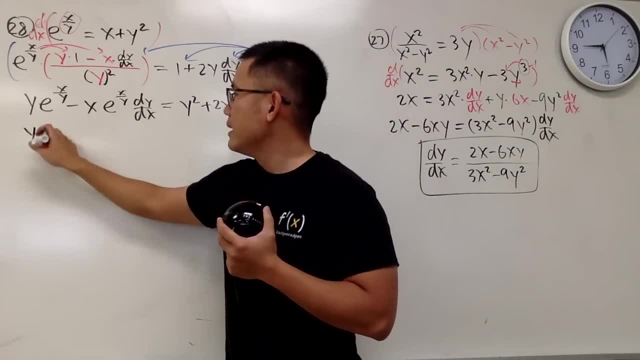 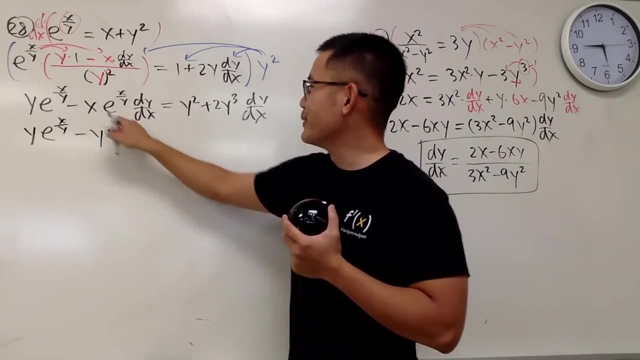 to the other side. So we get y, e to the x over y minus y square and this is equal to okay. I will put this down first. Parentheses 2y to the third power. 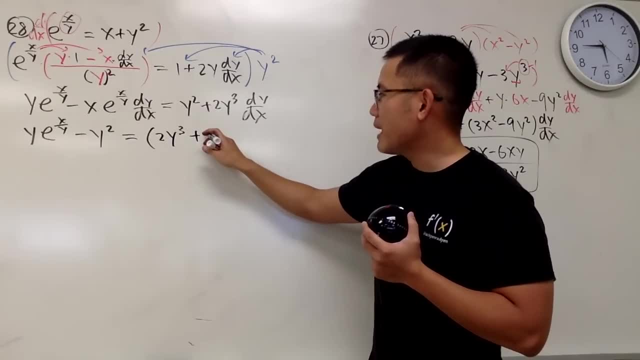 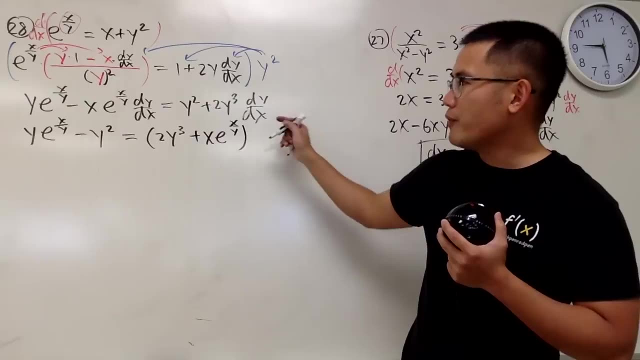 Bring this down, becomes positive right to the other side, Positive x, e to the x over y, And then both of them have x. both of them have dy dx, So I just put the dy dx. 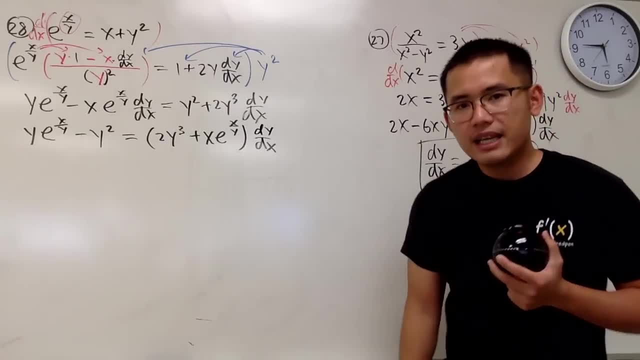 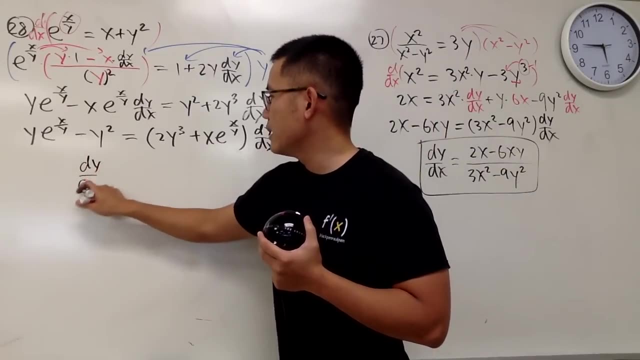 all the way at the end like that: Okay, Now divide this guy on both sides and it will be done. So we will have the dy dx equal to here. we have the y e. 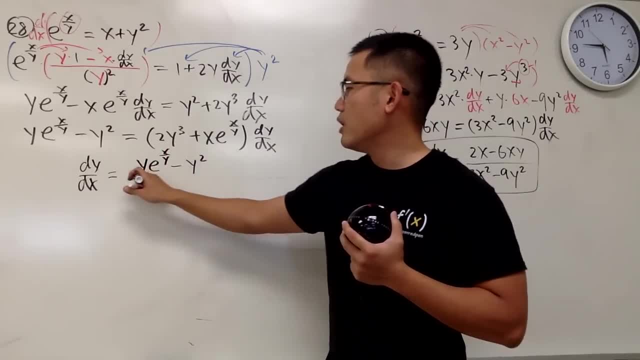 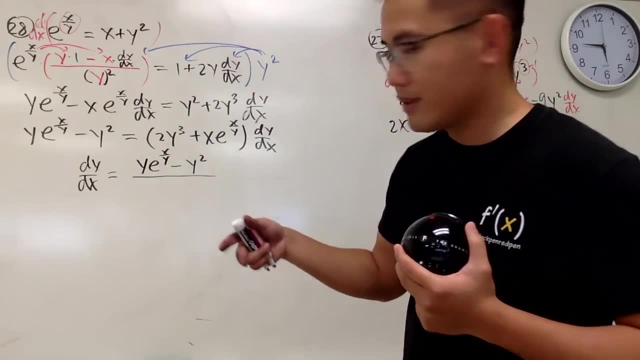 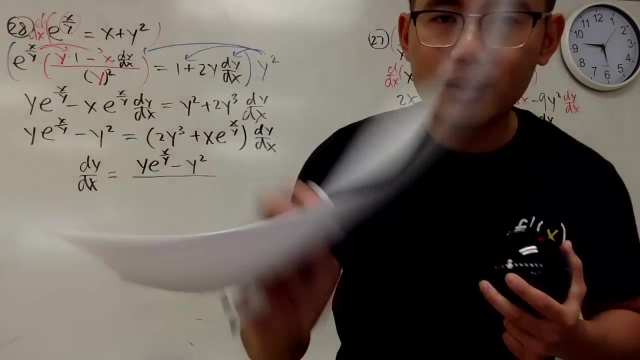 x over y, power minus y, square over. well, I think I like to put a similar term in the front right, So I did have this right here. go first. Now just let me show you guys. 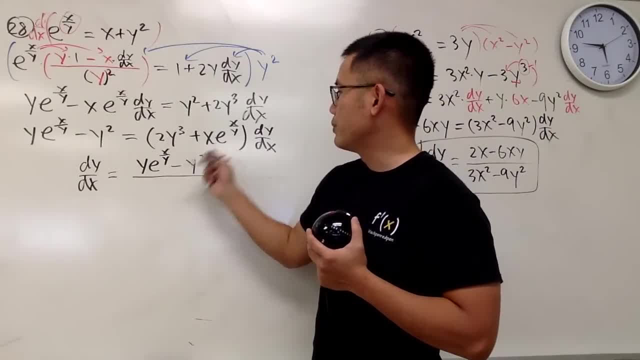 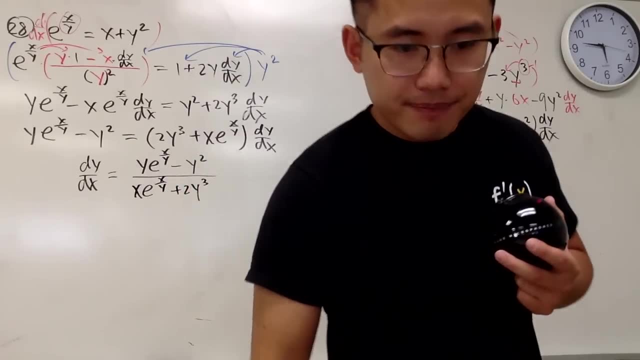 how I have the answer. I have this first, So I will just put this down: x, e to the x over y plus 2y to the third power, like that. Okay, And of course, if you switch the word on the bottom, 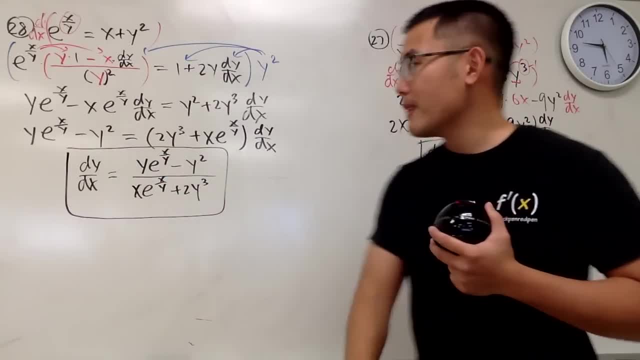 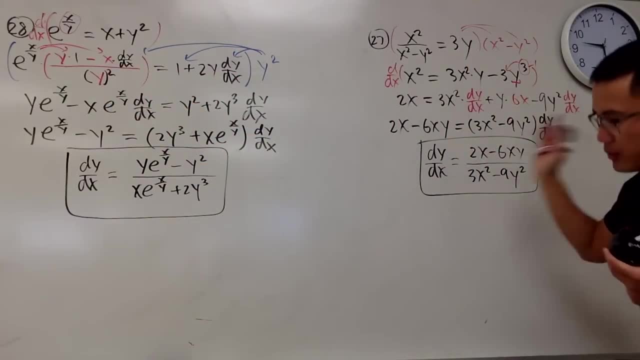 nobody will get mad at you, Just kind of pick the best answer on the answer choices So that one is the implicit differentiation with quotient rule. This right here you should not do the quotient rule, Okay, So. 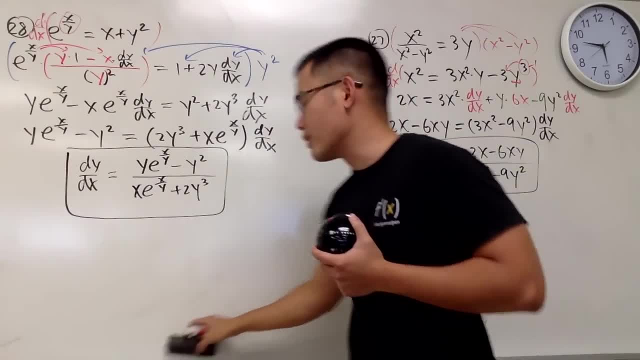 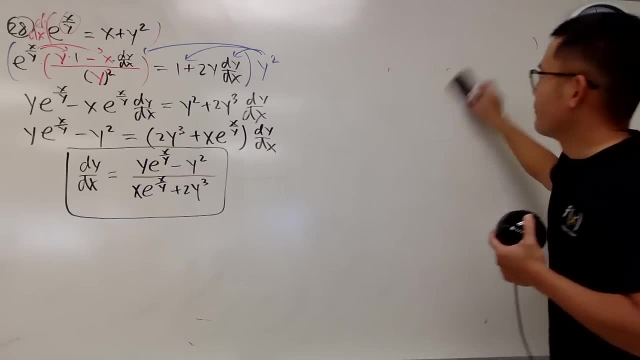 that was twenty eight and two more. I can drink my ming cha milk milk. When I first saw his video that he said he had a energy drink, I thought he was joking, because he always does that right. 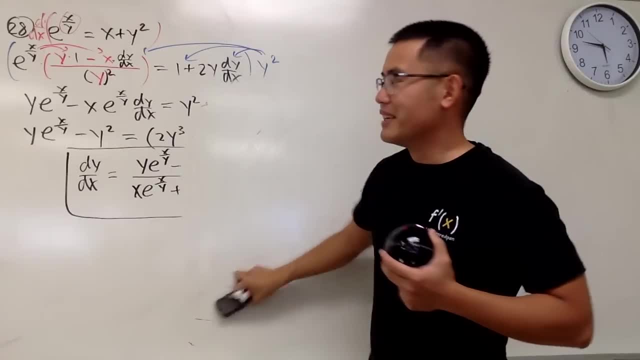 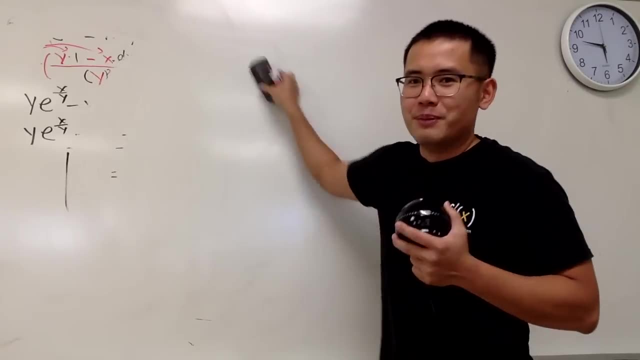 But then I watched the whole thing so, oh my god, it was legit. So I worded it right away, Because you know I used to watch him a lot when I was probably your age, Yeah. 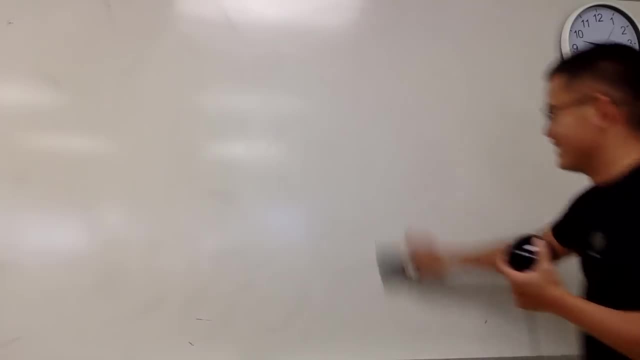 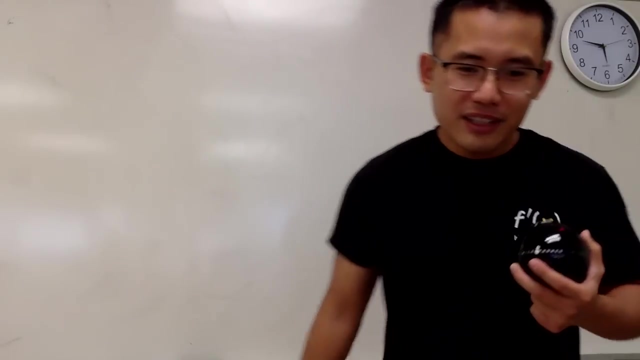 Okay, So subscribe to Nigahiga. That's his channel's name. N-I-G-A um H-I-G-A. I'll have the link in the description, why not? Okay, number twenty-nine, Number twenty-nine. 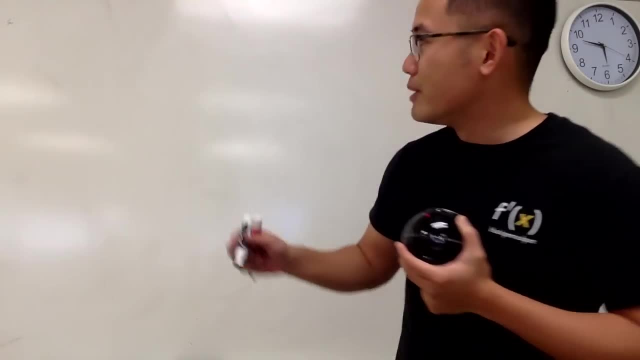 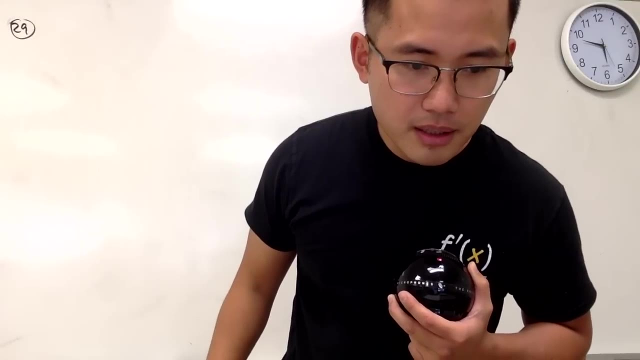 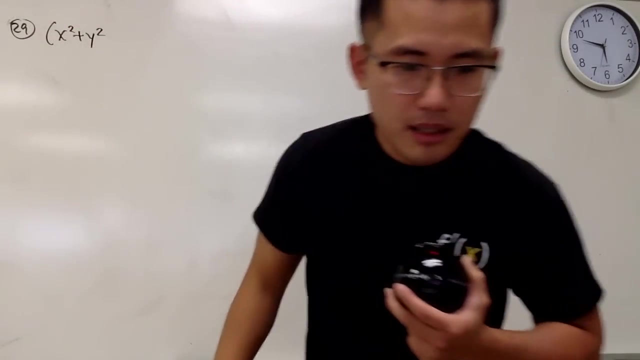 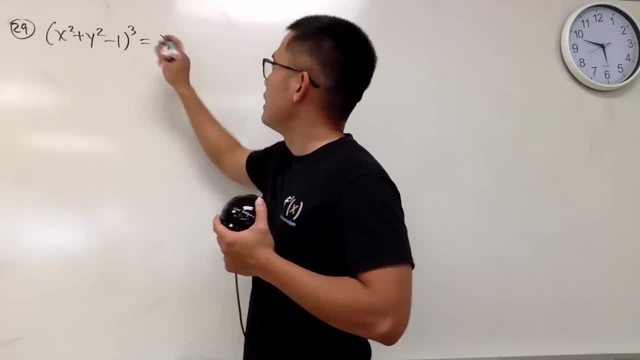 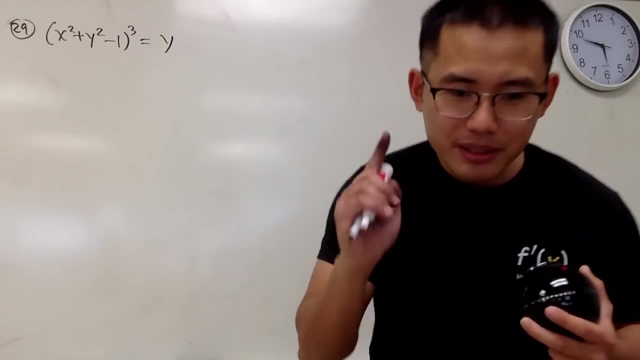 Like this: Okay, so let's just deal with this, And the good thing is that I didn't multiply out anything for the answer key. You will see what I mean by that, So let's go ahead. 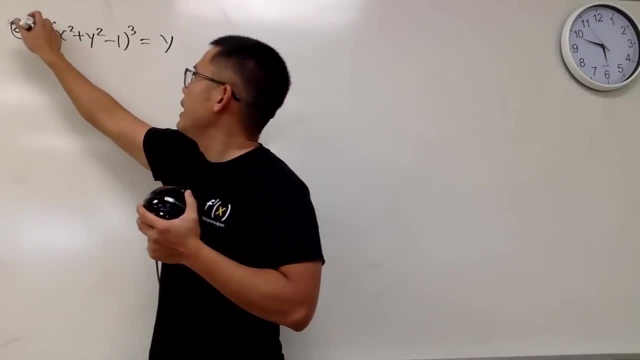 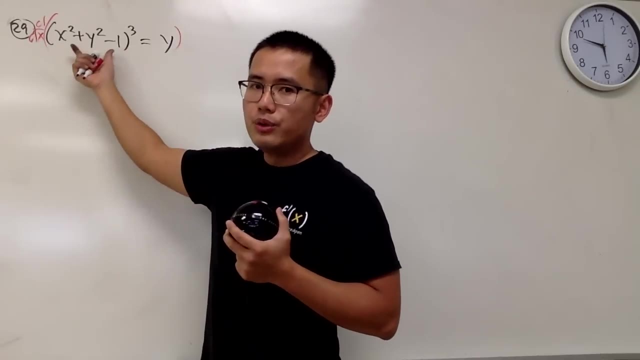 and differentiate on both sides. Okay, here we go On the left-hand side. look at this: to the third power. So bring the square, so bring the three to the front and then minus one. 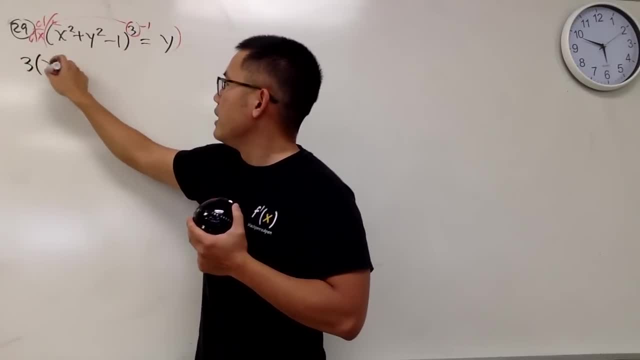 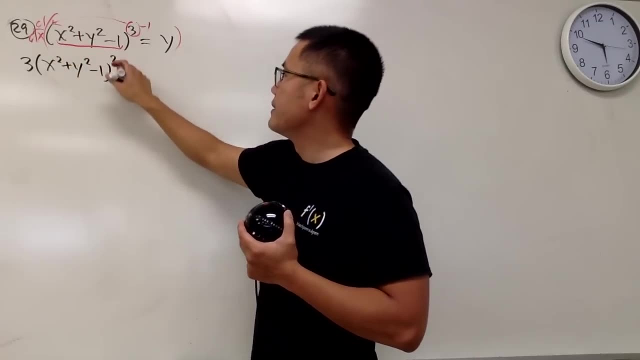 So here we go. We have three parentheses, the inside stays the same- X square plus Y square minus one to the second power, and then we multiply by the derivative of the inside. Open the parentheses. 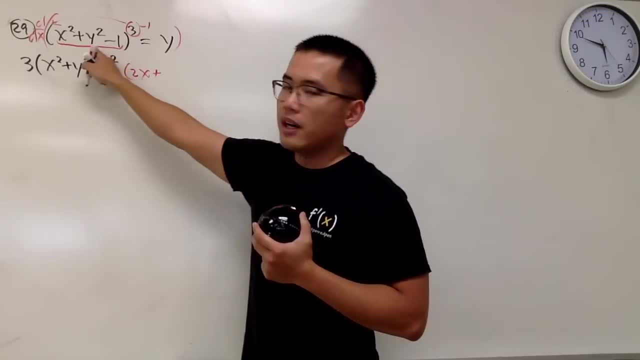 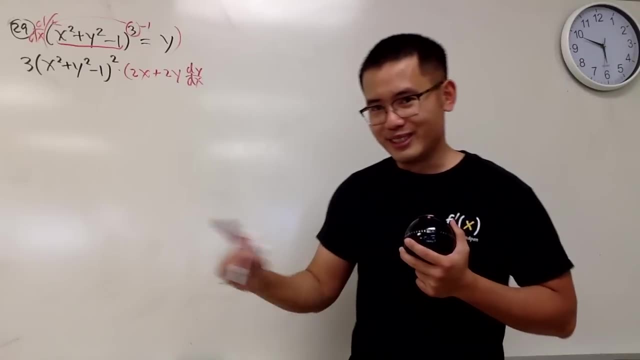 because we have more terms coming. Okay, derivative of X square is two X plus. the derivative of Y square is two Y minus one is just zero. So we are done. Yeah, that's it. 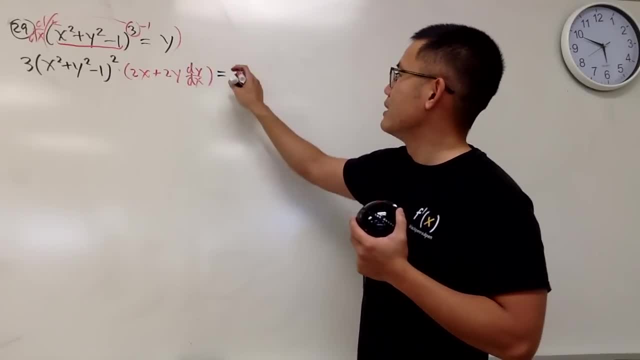 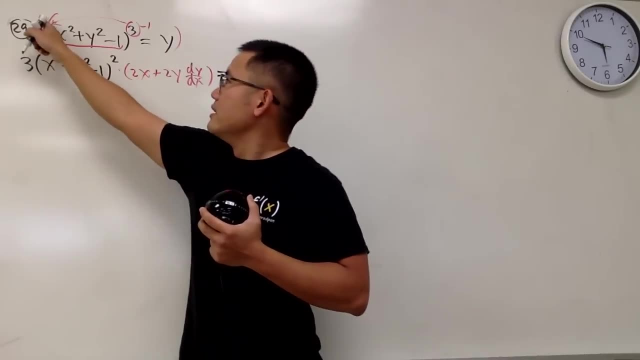 On the right-hand side we have this: the derivative of Y with respect to X is just dy dx. And you see, hopefully the notation makes sense: d? dx of Y is just dy dx. Okay, 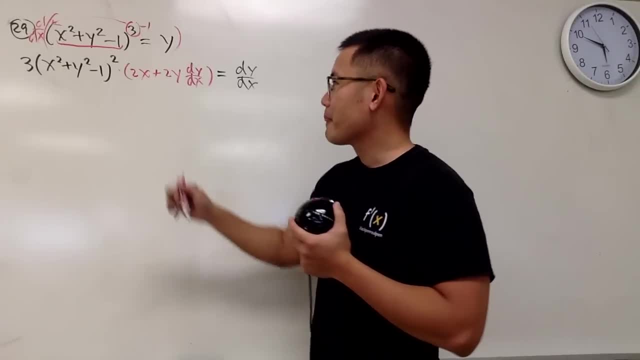 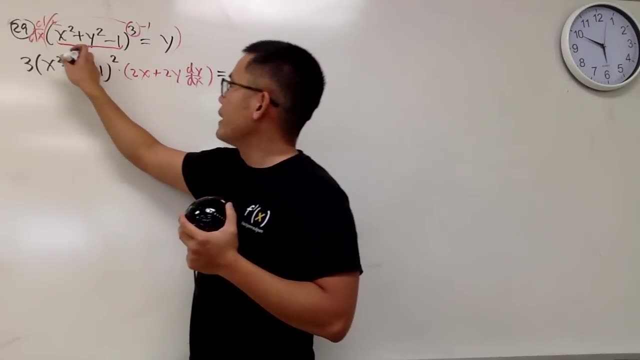 now simplify this guy. This is what I mean. I didn't multiply this out or just keep this. Okay. So to clean things up, we will take this as the whole thing. multiply with this, multiply with that. 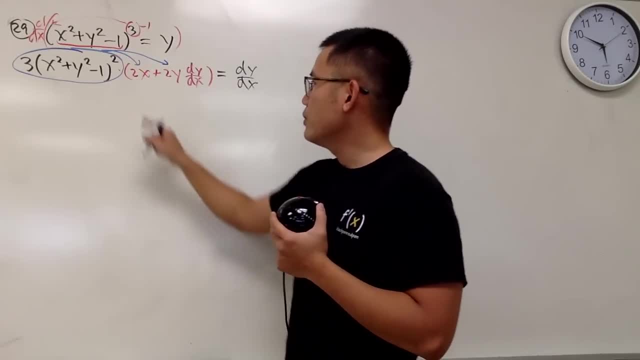 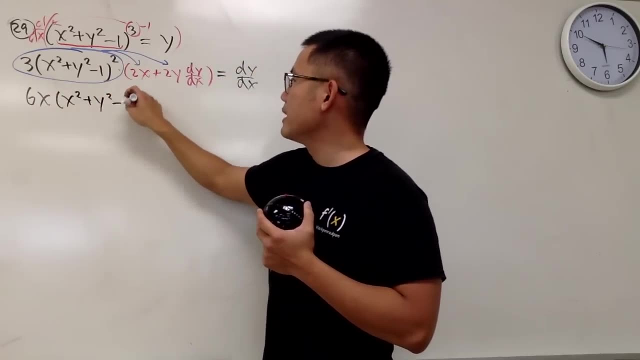 So let's distribute it first. So two X times three is six X, And then we have all that which is X square plus Y square minus one square, Yeah, And then three times two Y. 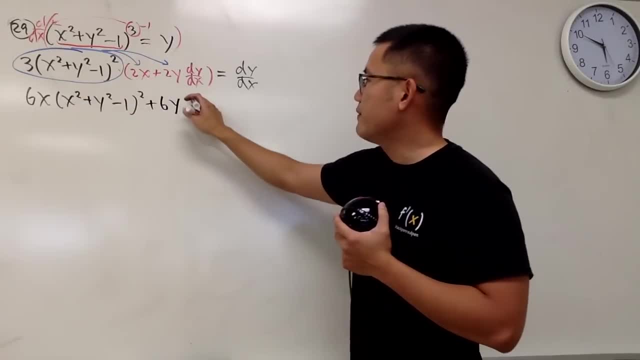 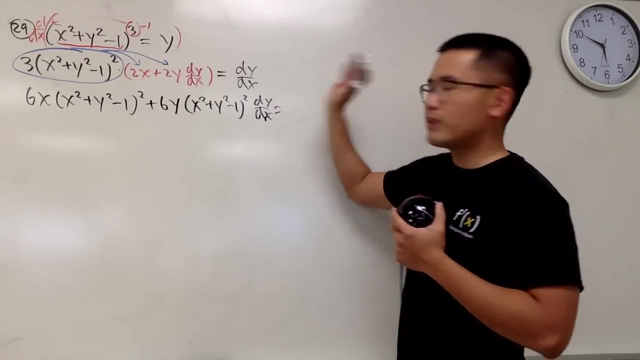 is plus six Y, And then of course, we write that down first before the dy dx Right here and dy dx And right hand side. we still have the dy dx as well. Okay, Okay. 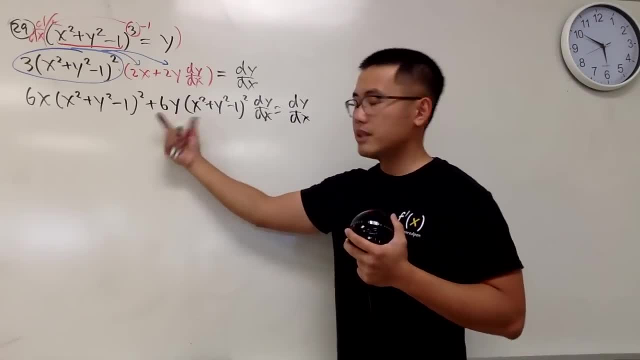 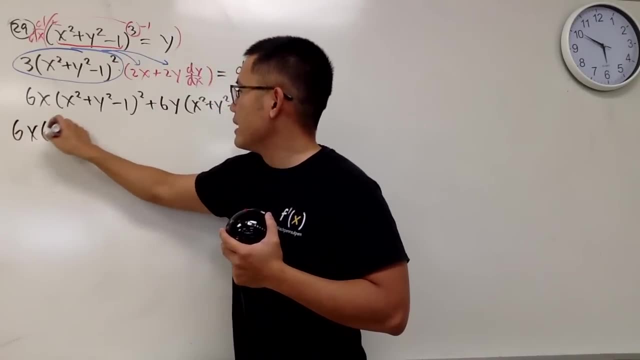 you know the deal: Bring this to the other side, So you have one and all that. surprise. I'll show you guys more work. Six X X square. I know some of you guys can do this in your head. 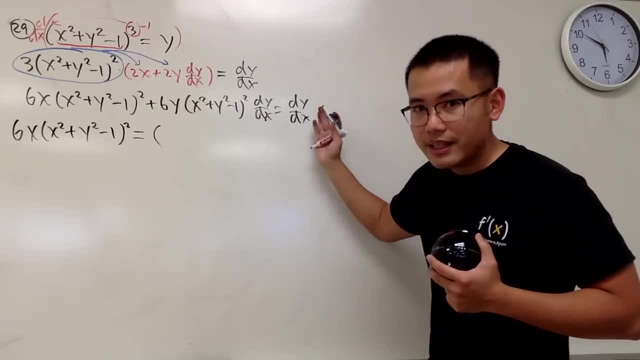 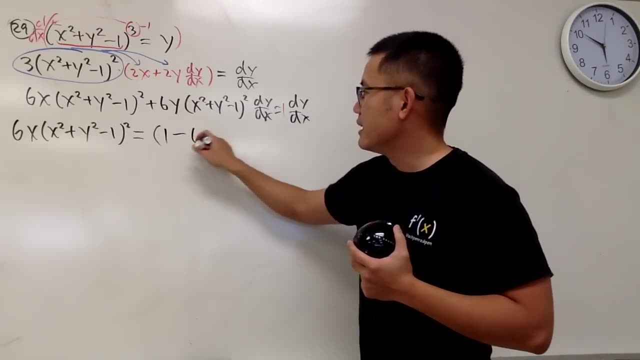 but I'll just show you guys all the work Here. right hand side this is. I think we have a one, And then this on the other side becomes minus six: Y parentheses, X square. 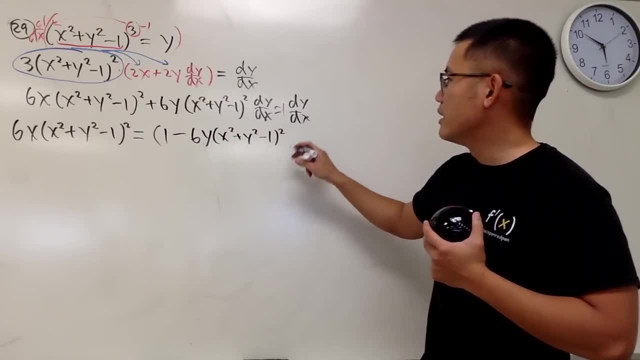 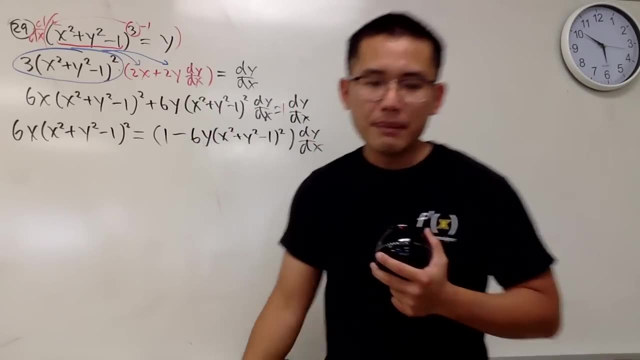 plus Y square minus one square, And then everybody had a dy dx right here, So I cut it out. Now bring this to the other side by dividing, and that's it So. 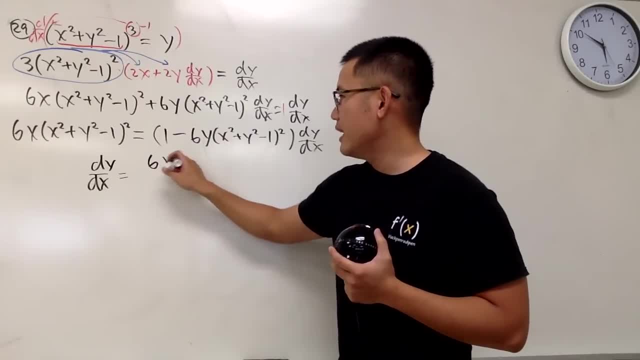 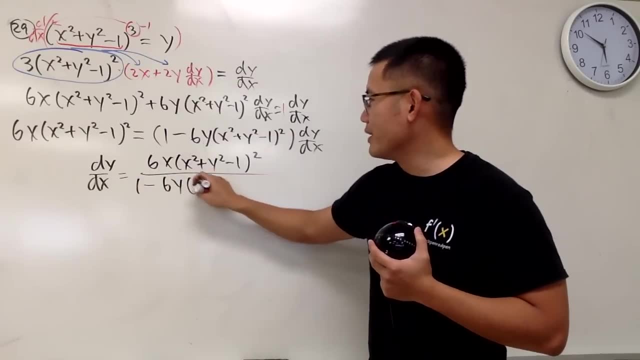 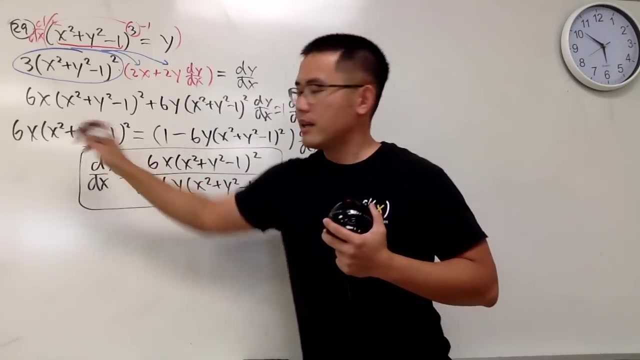 dy, dx equals. that's on the top. So X square plus Y square minus one square, all over one minus six Y parentheses: X square plus Y square minus one square, like this: 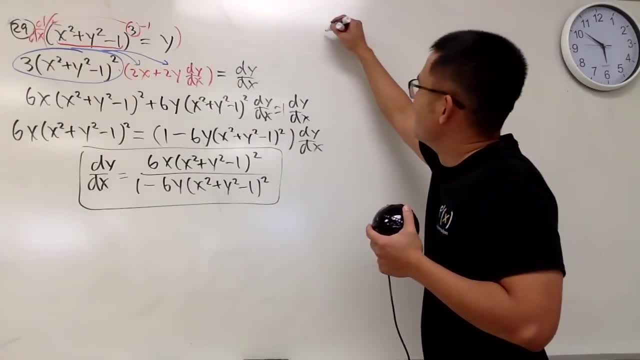 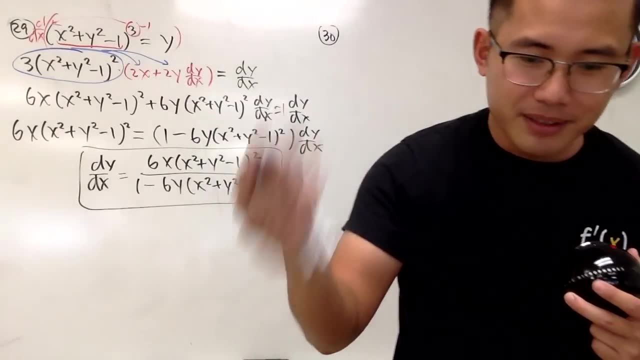 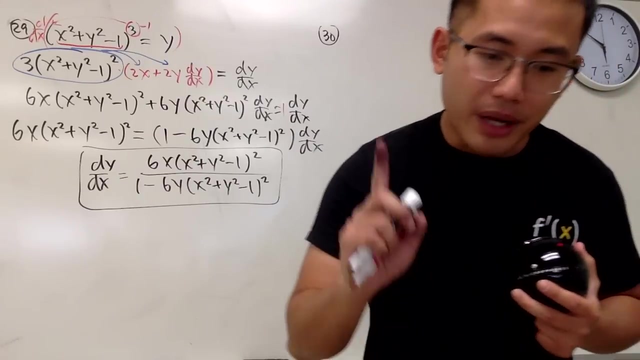 Done, Okay, good, Number thirty, my god, Finally, But it's not any easier. Why? Because we are doing second derivative From number thirty to number thirty nine. Why, Anyway, this right here? 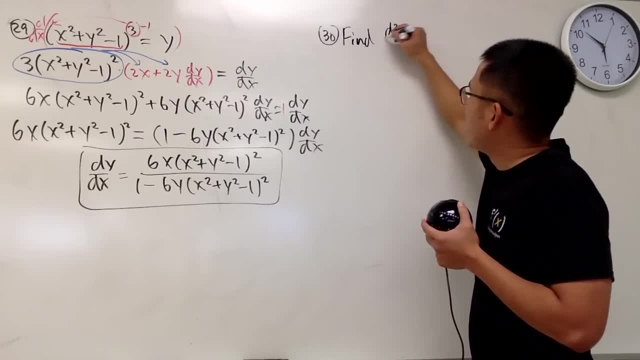 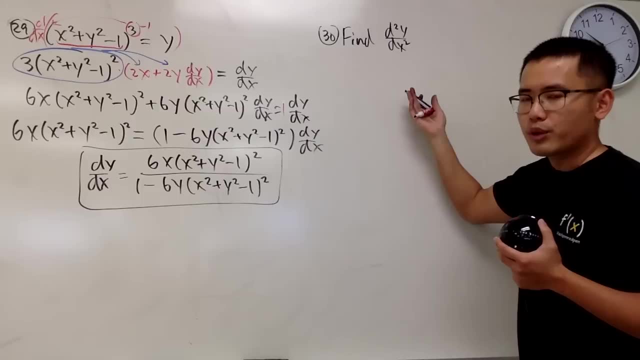 I will have to write down the equation for you guys. We are going to find d two, Y, dx two, And if you look at this right here, this is the second derivative notation. The idea is because, well, to get the second derivative, 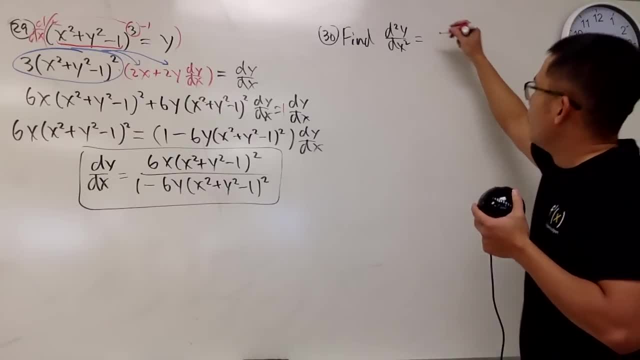 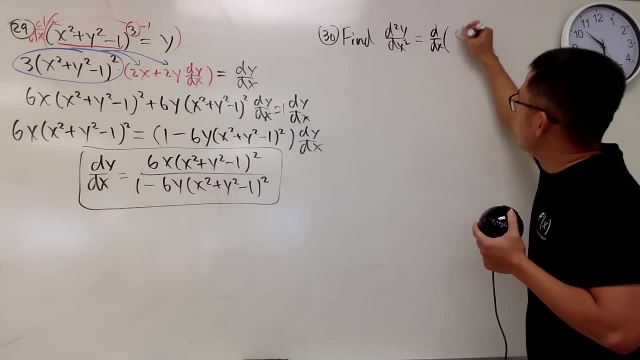 you just have to differentiate the first derivative, right? Well, as I said, we have to differentiate. this is the notation for differentiating. We have to differentiate the first derivative, oops, d, y, d, x. We have to differentiate. 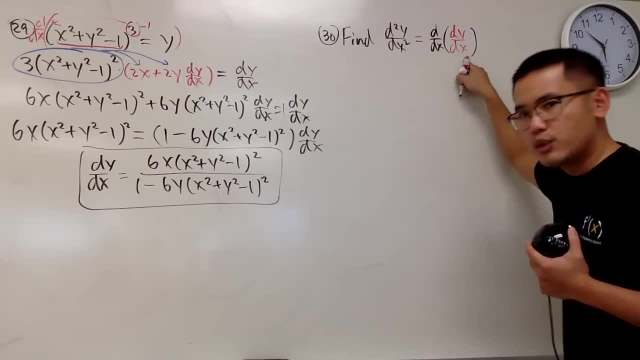 the first derivative. And now you see we have d and d, so that's d square. That's just a notation. it's not really like d square, but we put on d two y, That's how you say it. 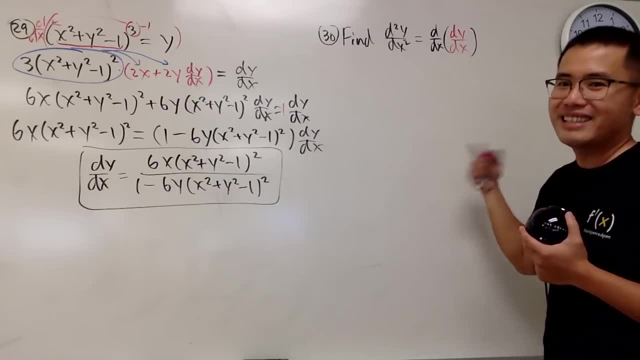 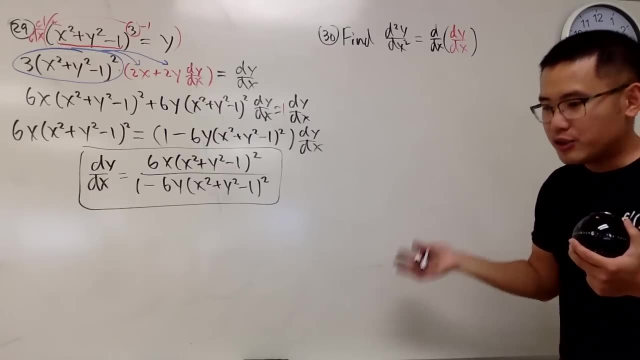 d two y, And on the bottom you see you have d x and d x happening twice, So we have d x two. That's the notation for derivative, for the second derivative. okay, Alright, now we are going to. 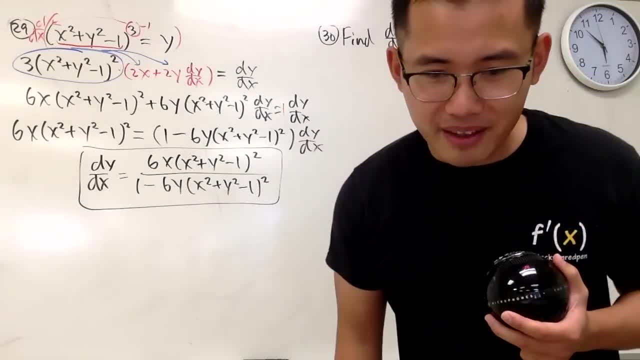 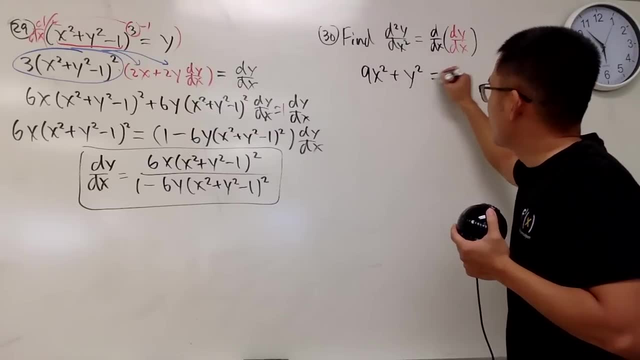 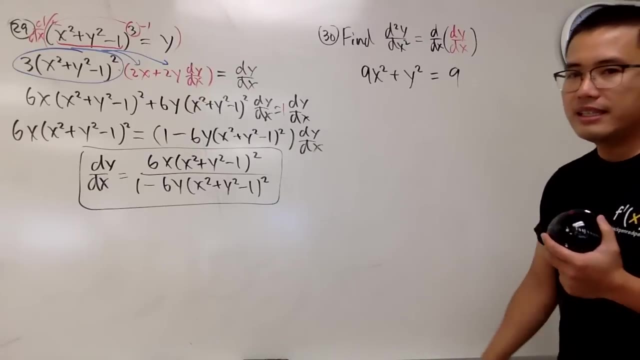 differentiate. Alright. what's the equation? That's the main thing. huh, We have nine. x square plus y square equals nine. Okay, here we go. We have to differentiate this twice. Why it's not isolated. 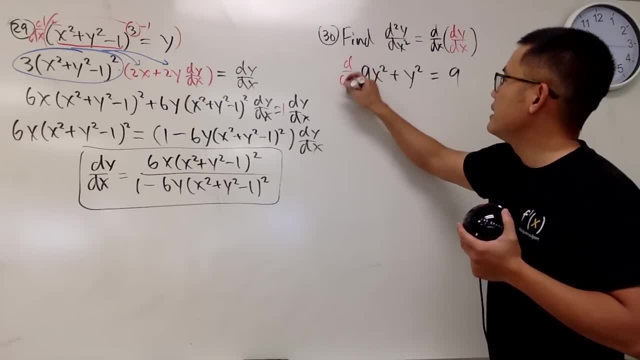 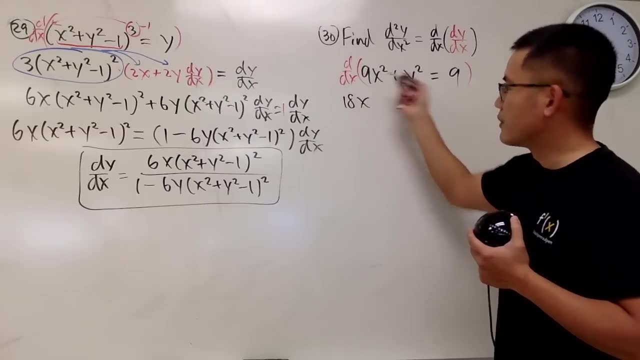 It's okay, just do implicit differentiation. Go ahead, d dx that. Now, on the left hand side, this is 18, right 18 x to the first power, 18 x and the derivative of that is: 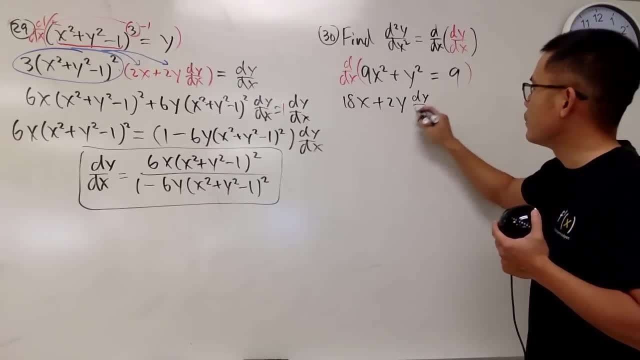 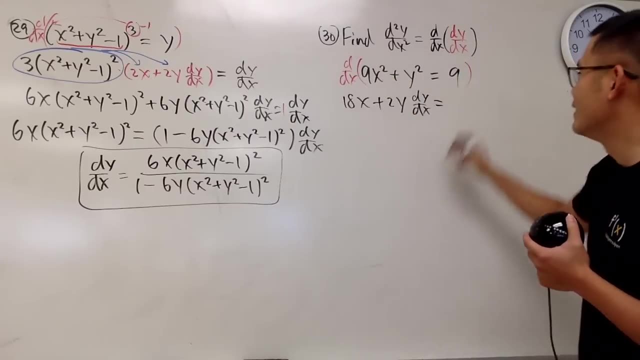 plus two, y. y is a function of x, so we have the d y, d, x like that. Well, the derivative of nine with respect to x is zero, So this is equal to zero. Good Now. 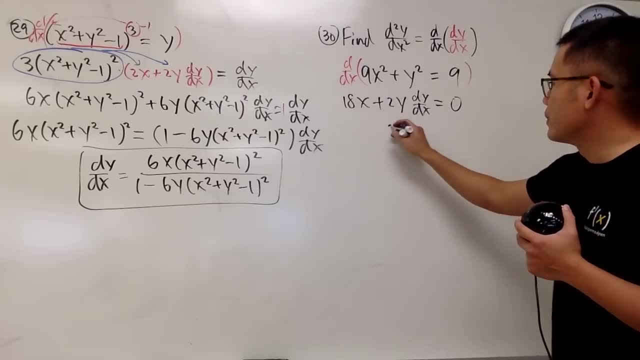 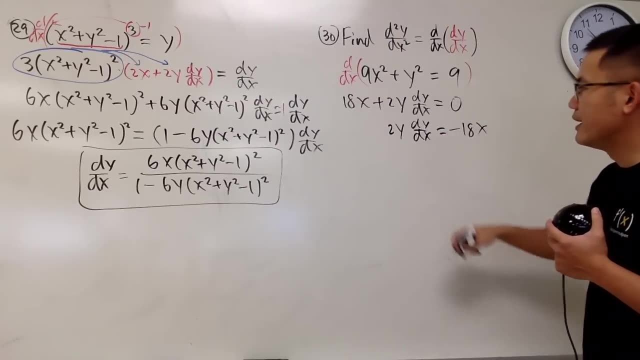 check this out, I will have to move this to the other side. So we have two: y d, y, d, x and that's equal to this to the other side becomes negative 18 x And we will just divide. 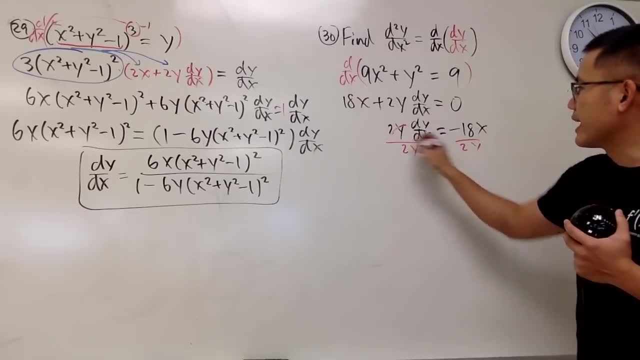 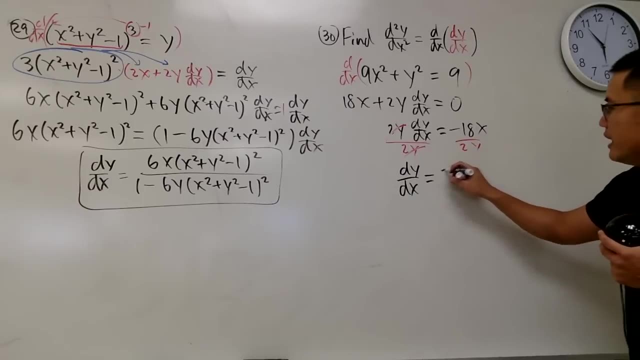 the two y on both sides. So they cancel and you just get d, y, d x equals. reduce that, you get negative x on the top, nine x on the top right, Nine x on the top. 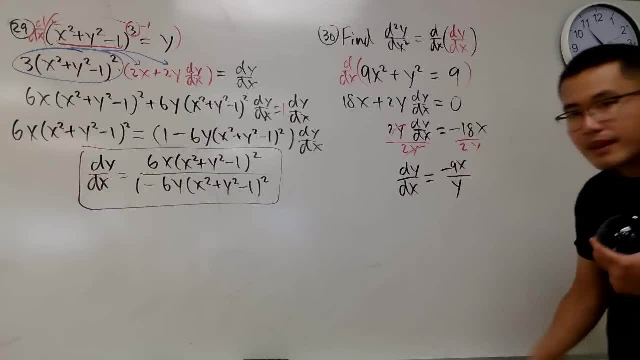 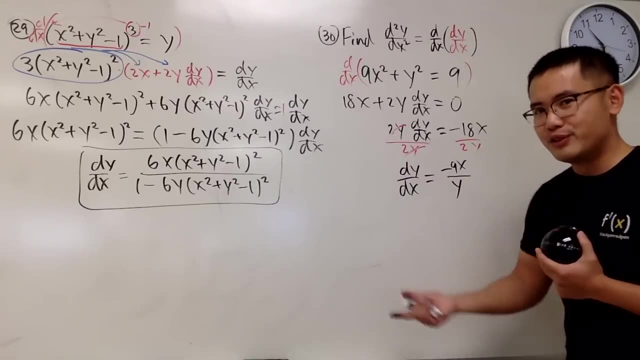 over y. So negative nine x over y. And you see this right. here is the first derivative. We just have to look at this expression and differentiate that again so we can get d two y, d x two. 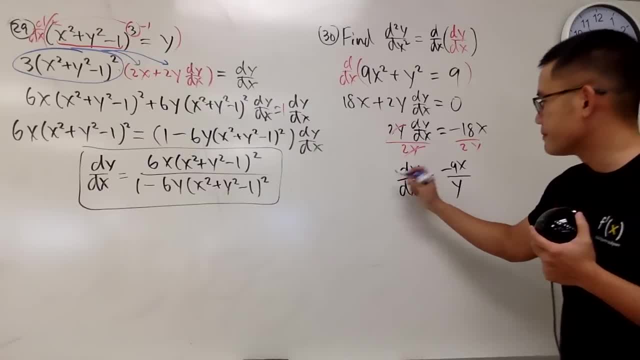 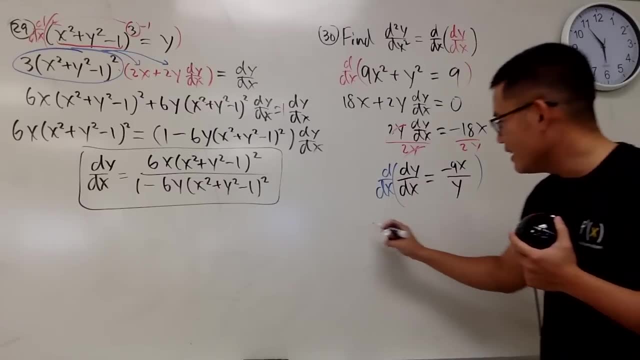 So we got right here. let's just emphasize that: right d d x this right here, right d d x this right here. So we see, right here we get d two y d x two. 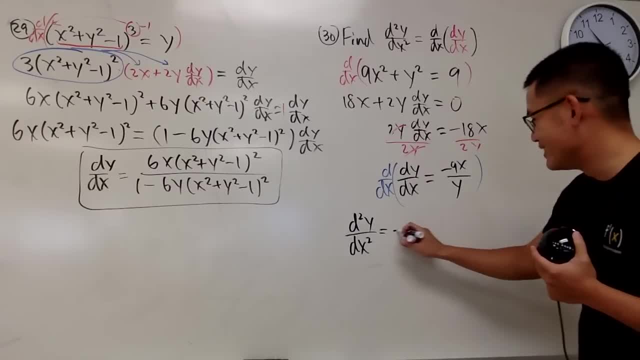 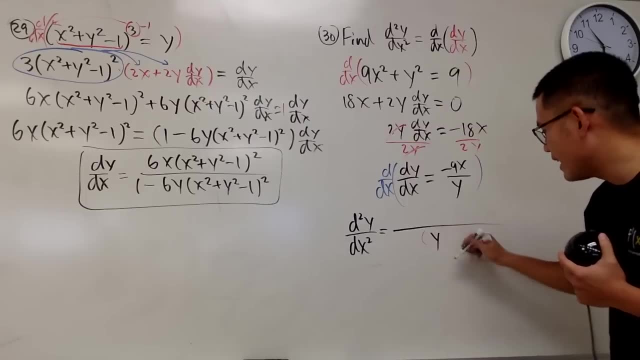 On the right hand side. we have to do the quotient rule again, just like the example that we did number 28,, I believe, Square the denominator, so parentheses: y: square that, square that, Okay, the. 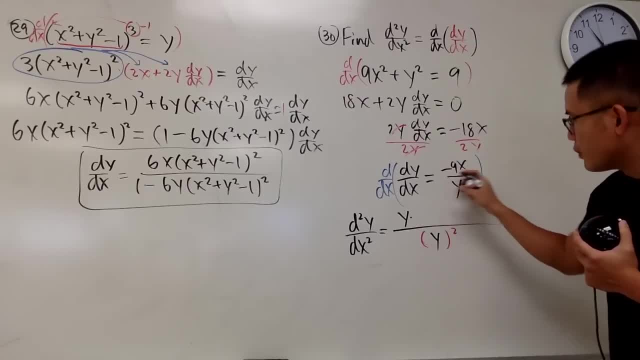 bottom function is y times the derivative of the top, The derivative negative nine. x is just negative nine. so this is the derivative of the top Minus the top function, which is negative nine. x top function. 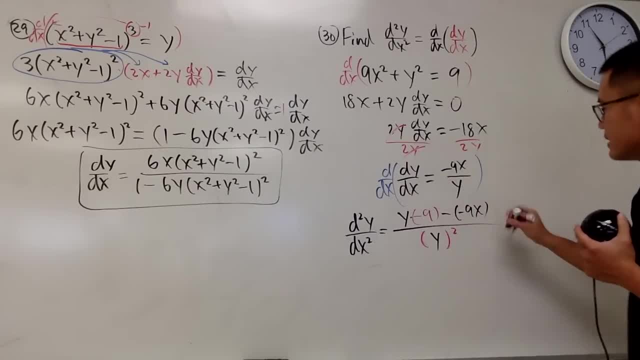 just write it down: Times the derivative of the bottom, The derivative of y, is what d, y, d, x, isn't it? I'll put this down. Okay, so now the derivative of y is d- y. 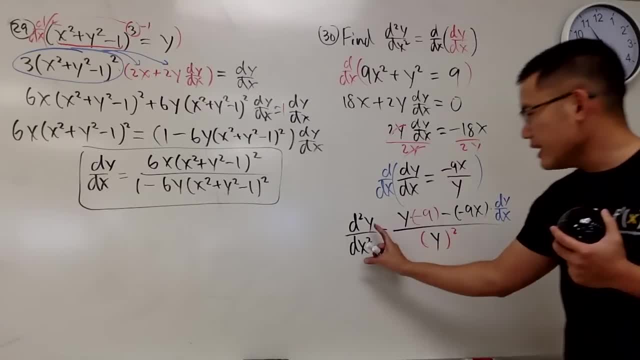 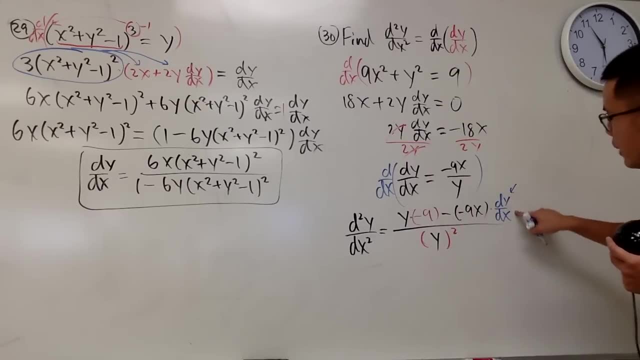 d x. Okay, so you see that the second derivative is based on the first derivative and other stuff, right, But the truth is, if you look back, d y, d x, look back right here. 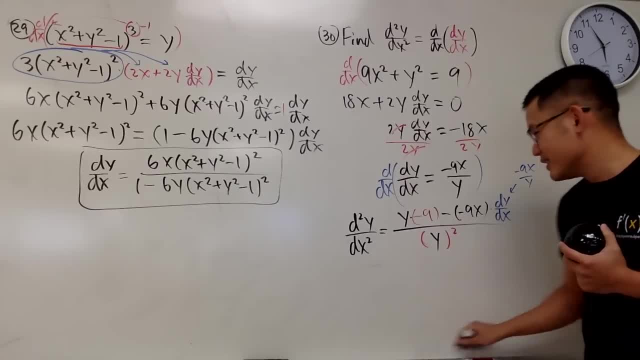 this right here is just negative. nine x over y, So we can replace this right here real quick. So we see for the second derivative we will end up let's see negative, negative without any further explanation. 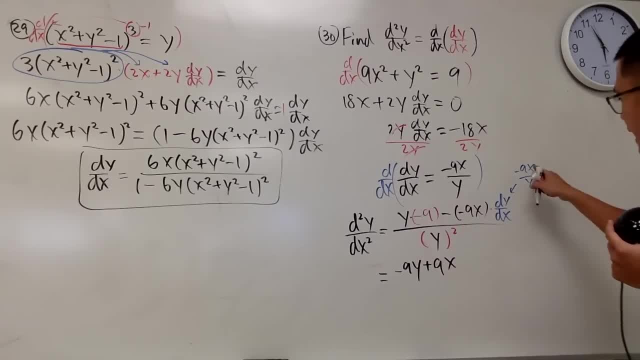 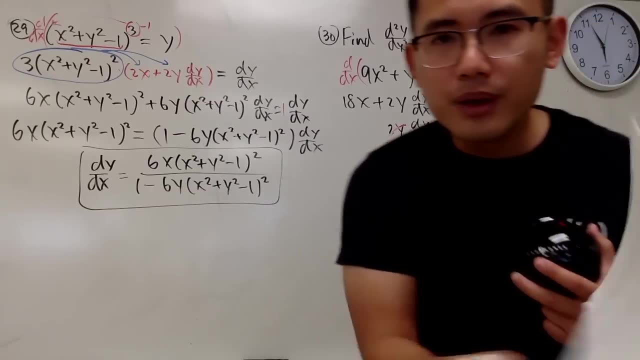 it's just positive nine x right here and we can replace that. we can replace the d y, d x with this, So I will do that real quick. Wait, I thought turn this thing off already. It's the. 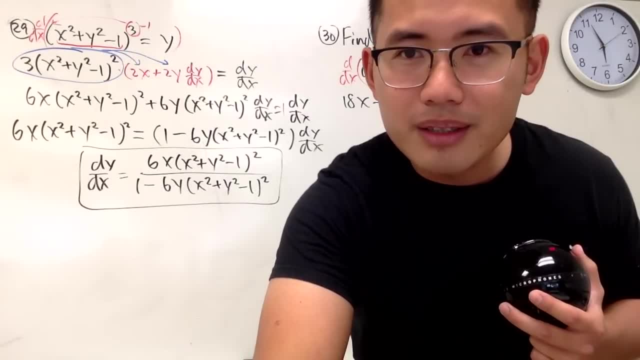 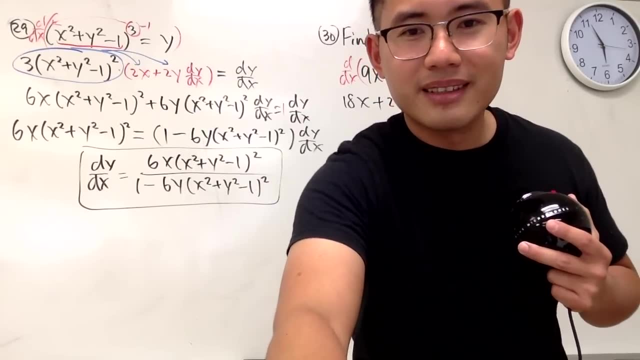 wifi that want me to connect. No, I don't want that. See, The wifi is telling me to update. Okay, anyway, this right here. we will just put it down right here. which is negative: nine x over y. 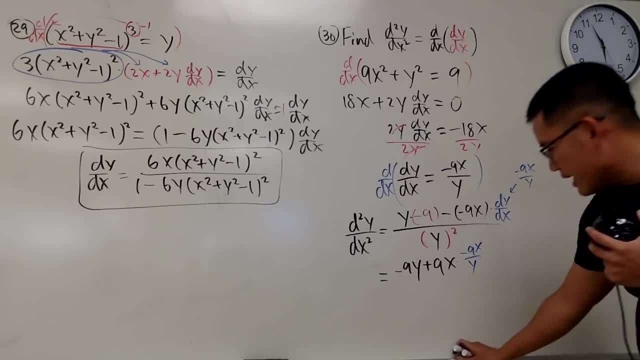 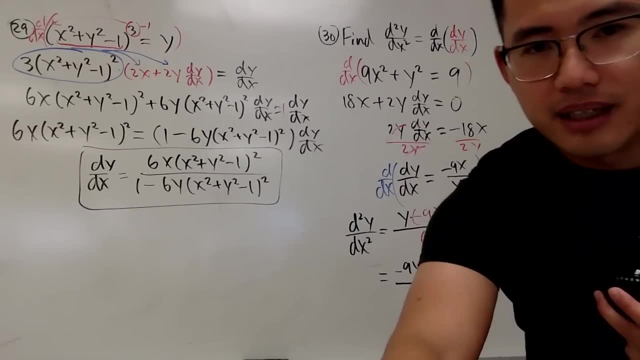 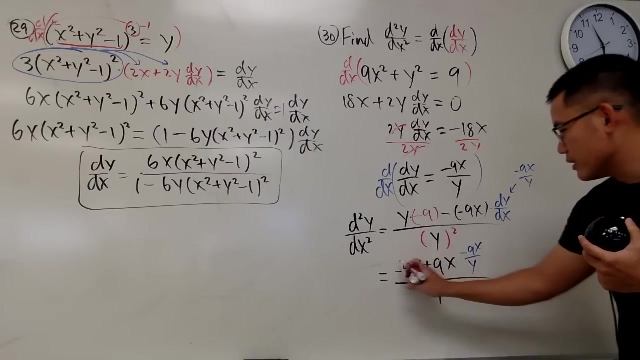 Okay And we divide this by y square like this: So far, so good, right? Hopefully that's the case And, of course, again this right here we had a complex fraction, so perhaps 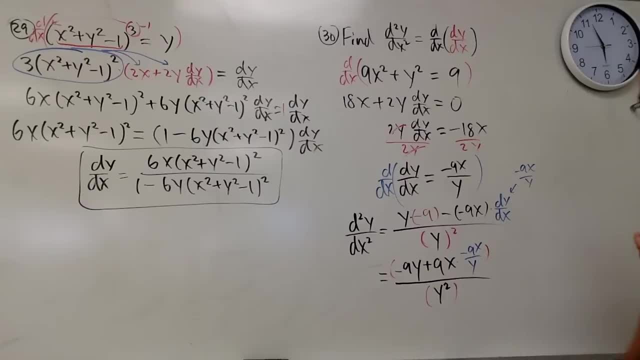 we do the following, So the rest is just some kind of a simplification. Okay, here we go, Because so that I can get rid of the complex fraction situation And let's see, I should be able to fit in here. 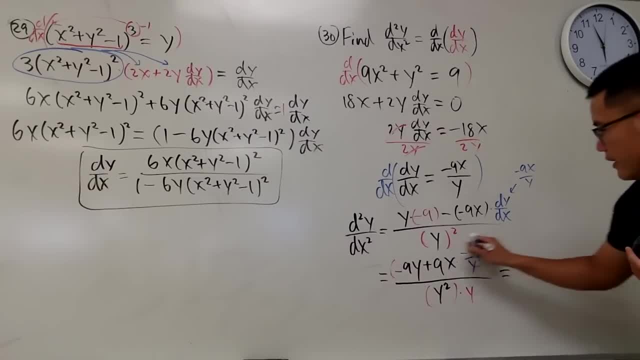 let's see, This is going to give us negative nine y square And this is going to give us y and y cancel out, But nine times negative. nine is negative 81. And we have the x square. 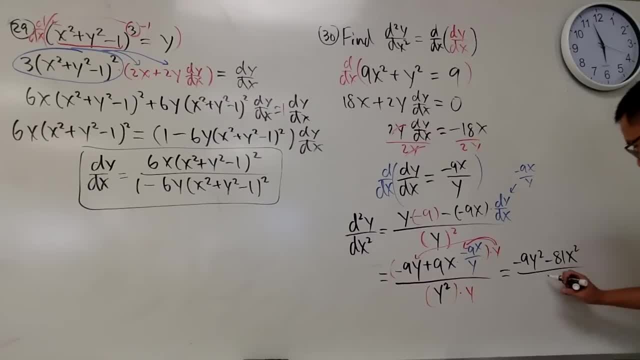 Yeah, Over this. right here is y to the third power, Like this: Okay, And the moment that you think, hey, we are done, but we are not Because, in fact, we can factor something out. 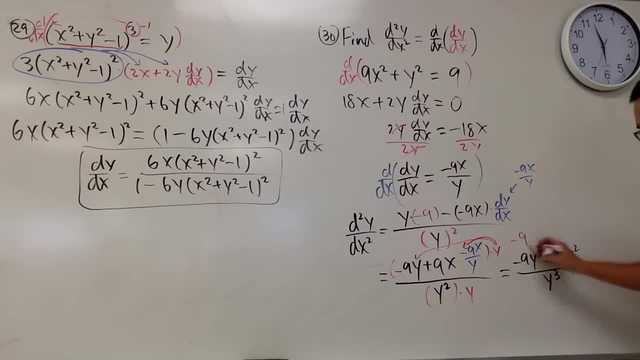 on the top And things will work out pretty nicely. On the top we can factor out negative nine. And you see, if we do that, here we get y square, And we add, And here we get nine. 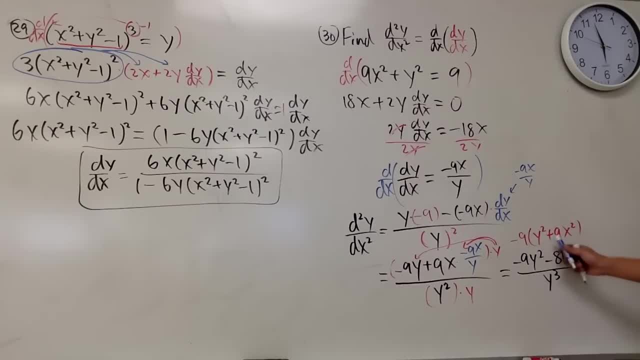 x square Look familiar. Nine x square plus y square. Check this out: Nine x square plus y square- This right here is just equal to nine. So all this right here is just equal to nine. 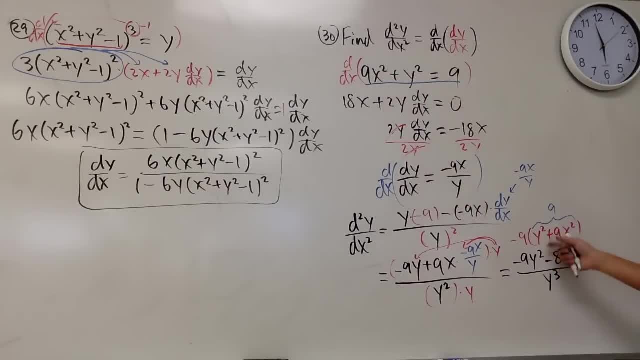 This right here, is equal to nine. Of course, the order doesn't matter of the adding, So this is just equal to nine. Therefore, finally, we can simplify the expression to negative eighty one over y. to the third power. 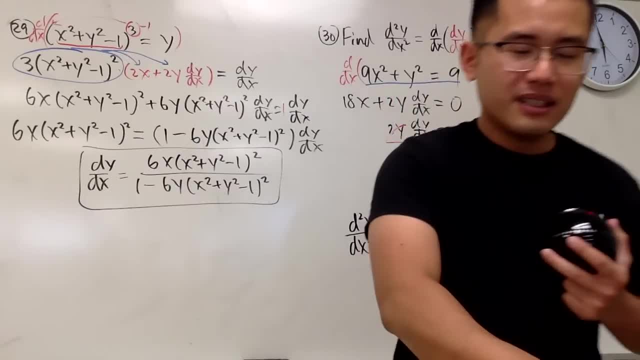 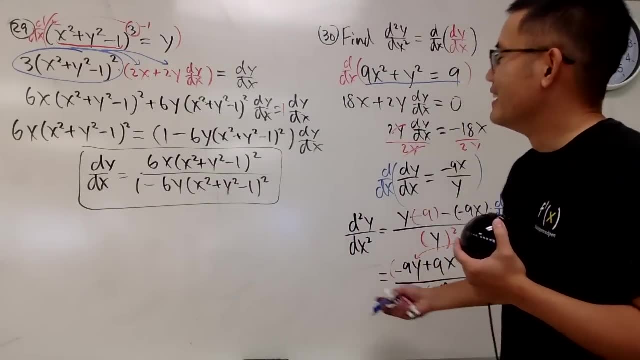 And this right here is it. Okay, This right here is it. Oh man, This is number thirty, So that means I have three more to go. This is going to take more than six hours. 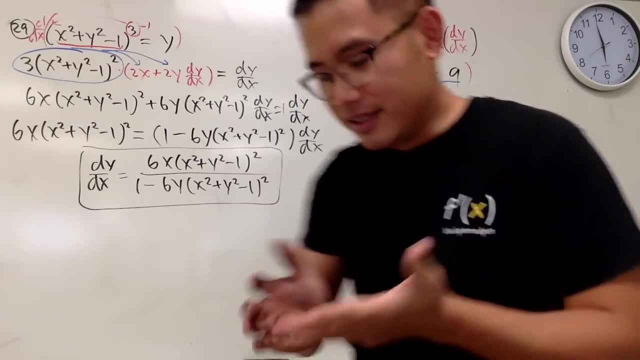 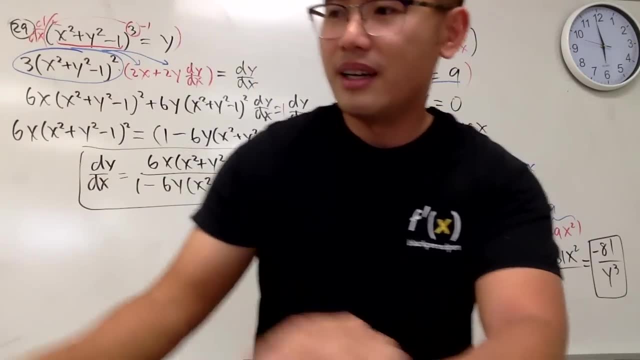 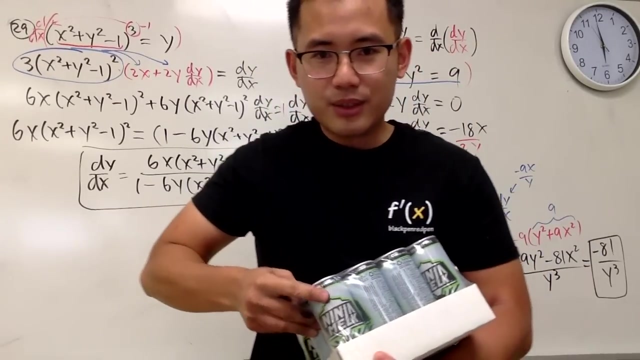 for sure. Why did I do do this to myself? This is going to be more than six hours, for sure. Anyway, let me have, ah, the ninja milk, Eh, Ninja milk. So this is two hour. 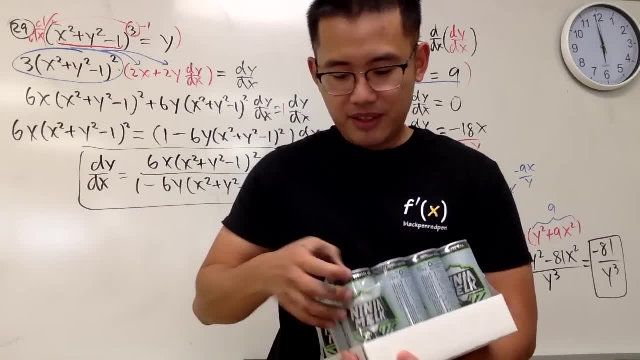 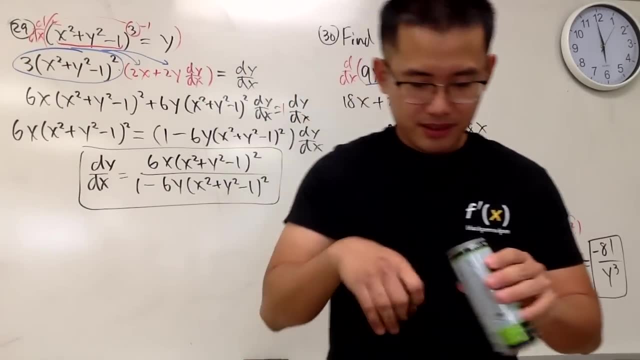 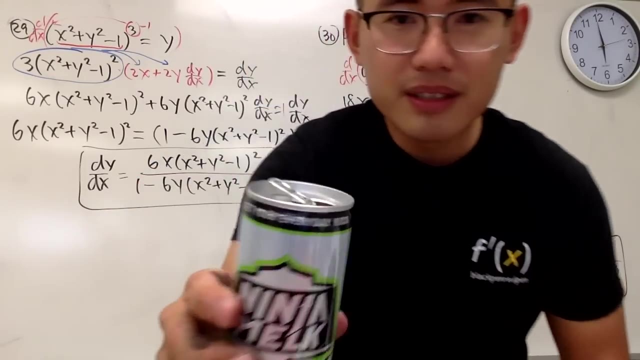 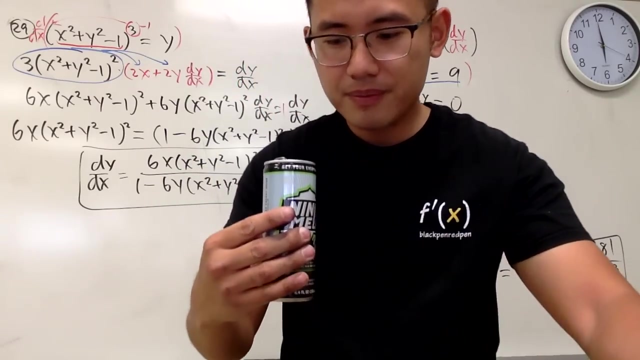 and fourteen minutes. Ah, give this a time stamp Right here, Man. Oh, so this is how it looks like. So it's like Calpico, like the, the Japanese drink, and it's sparkling. 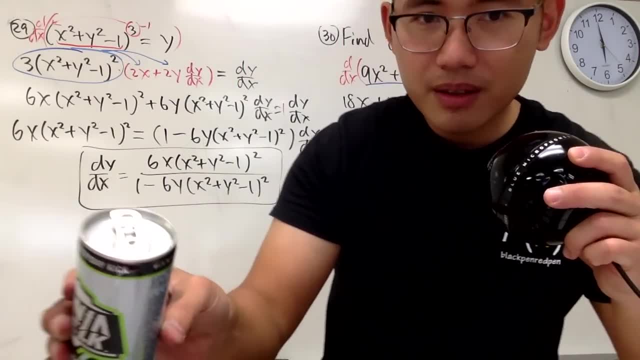 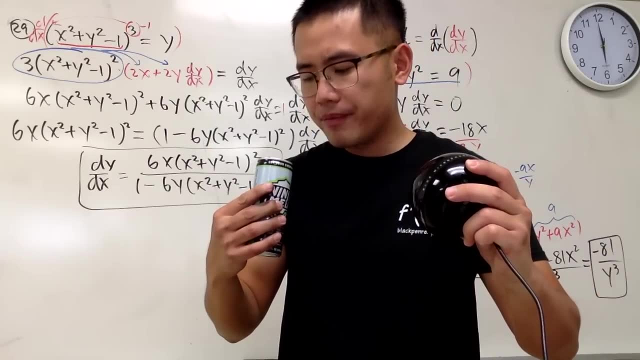 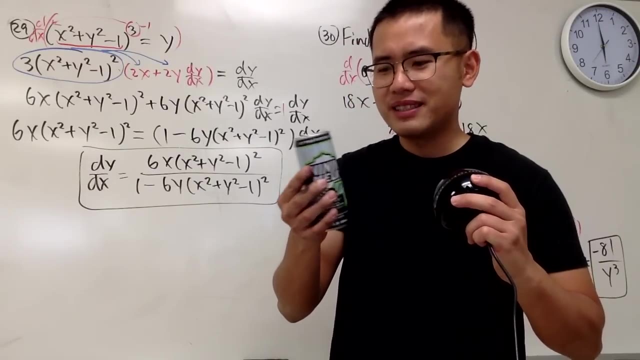 This is like sparkling, Can you guys see? Hey, it's pretty good. actually It tastes like Calpico- I think that's how you say it- um the Japanese drink, And this is sparkling. 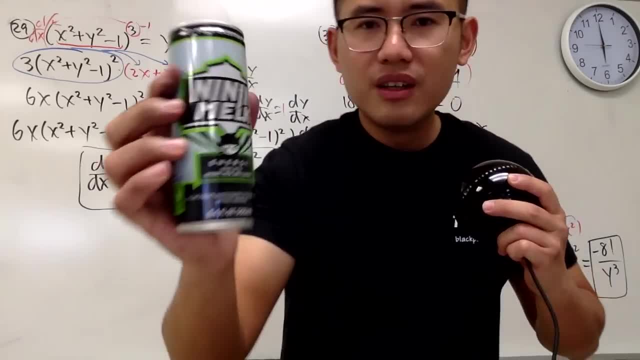 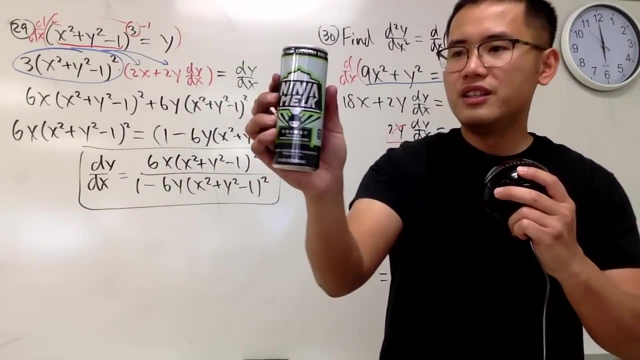 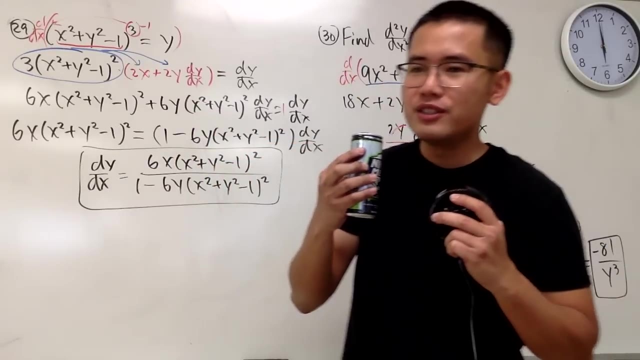 And this is, uh, organic milk with flavor. So take a look right here. Okay, Ryan Higa's, okay Ni Nika Higa's, um ninja milk energy drink. I don't know if this will really give me the energy. 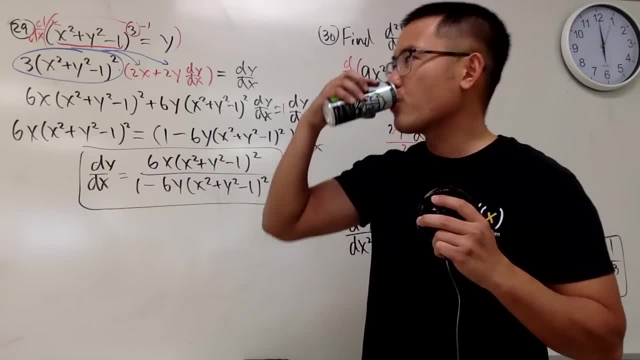 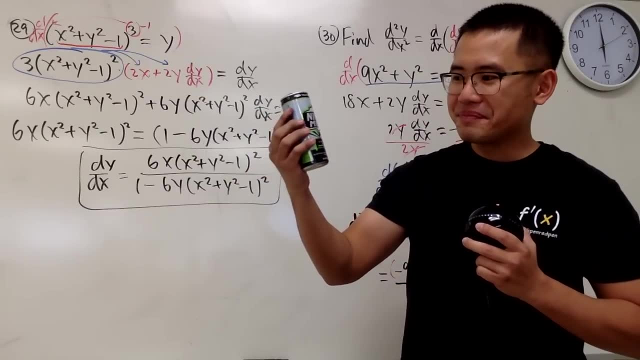 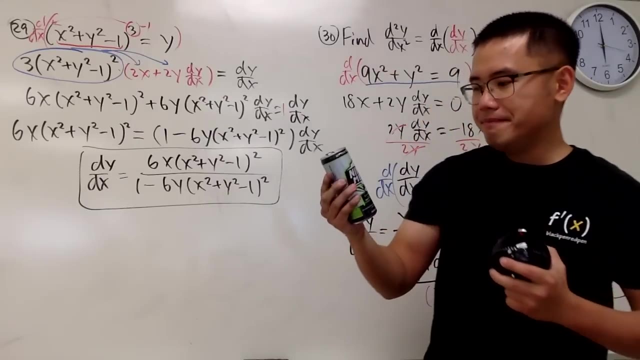 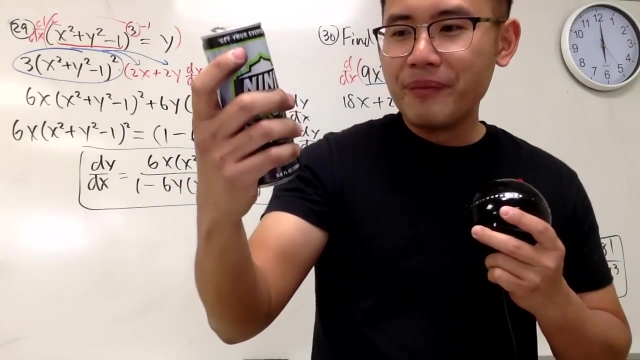 to last for another, I don't know how many hours. Really good, Wow, Tastes really good. actually, 112, calories per can, Right. So for the people, if you care about nutrition here, this is. 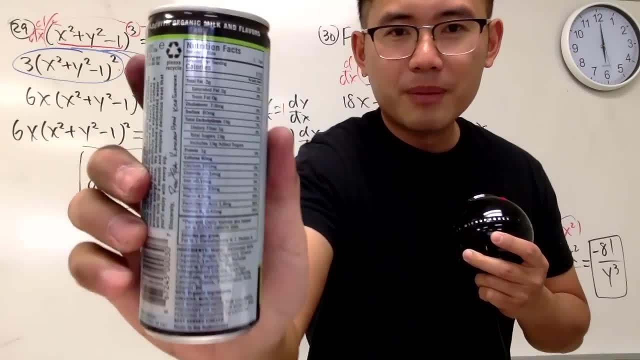 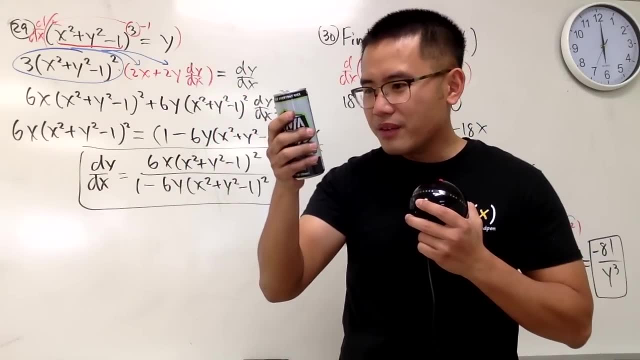 uh, the nutrition label. I'll drink more. How many caffeine do I have? I don't have any caffeine. huh, Oh, caffeine is 80, milligram. Can you guys see right here? Okay, So this is. 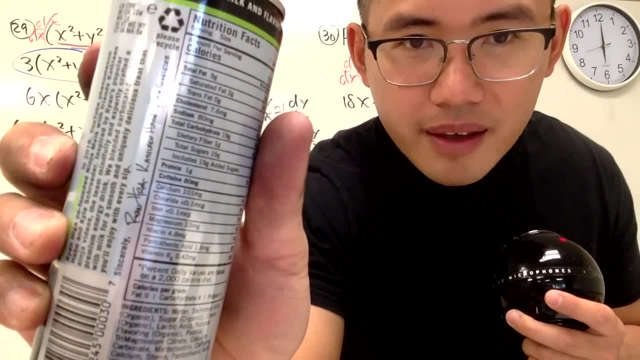 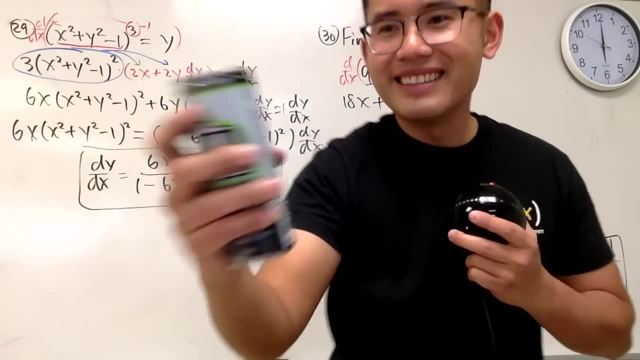 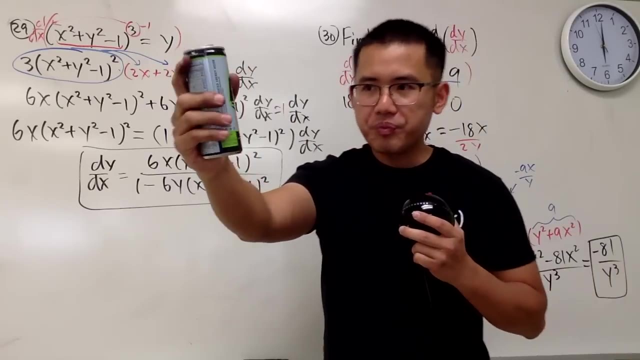 this is uh. caffeine is 80, milligram right here, yeah, And I get one gram of protein. Look at that. Oh man, I feel good. Wow, Tastes really good, Whoa, Okay. 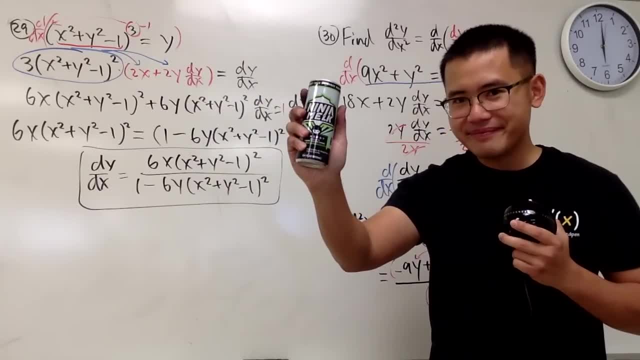 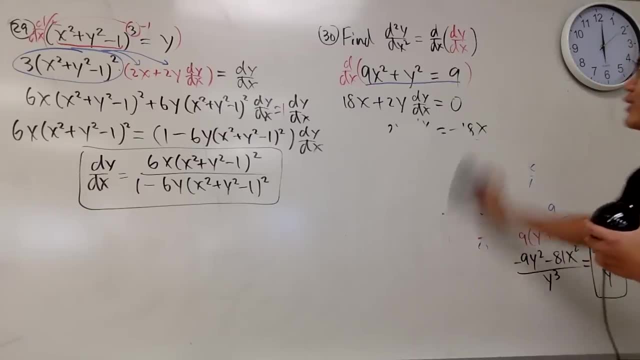 No time to rest, though That was just, uh, as I said, question number 30.. And now I'll drink the, the, the, the, the, the, the uh. ninja, milk Tastes good. 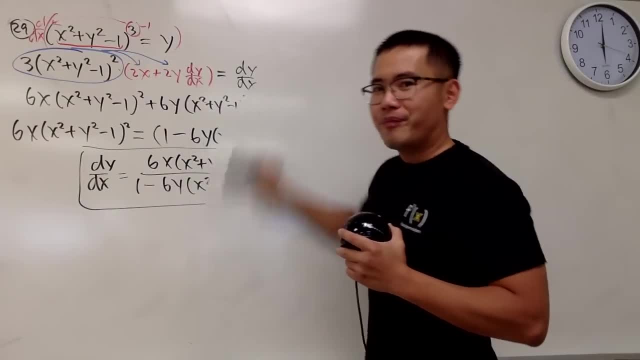 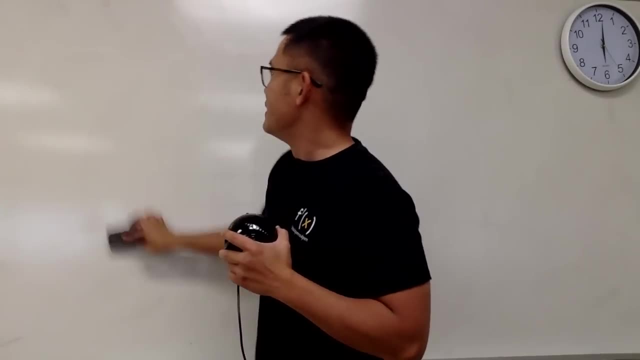 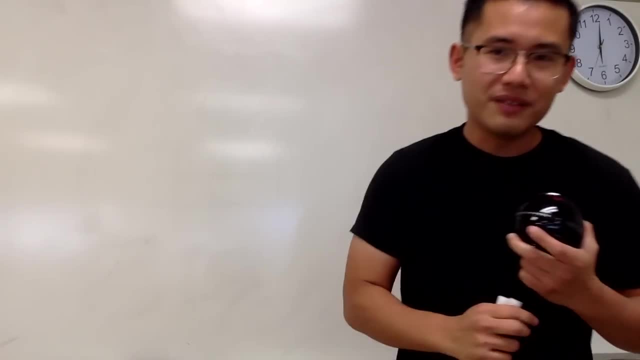 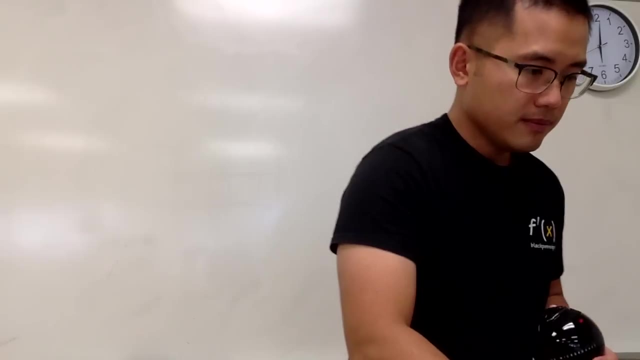 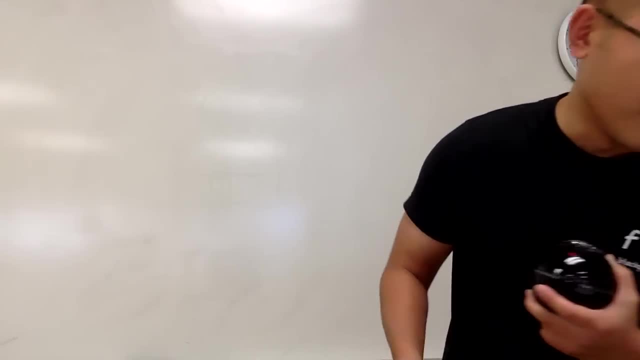 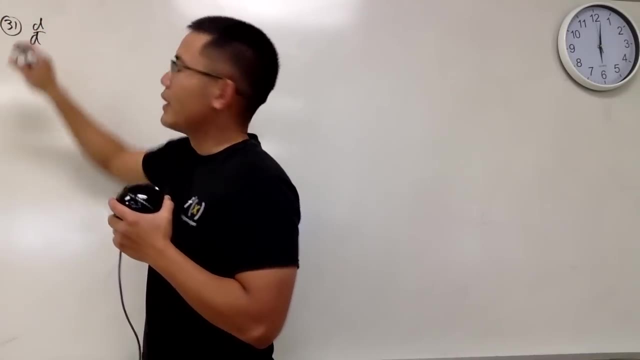 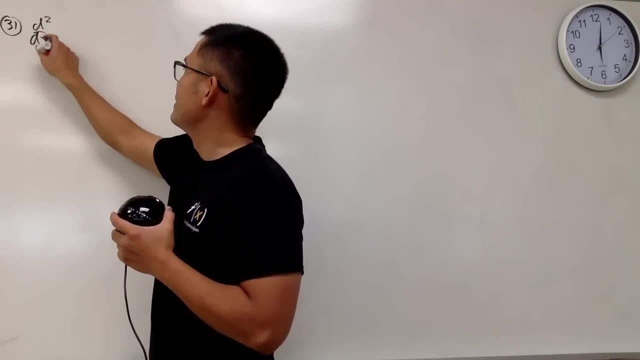 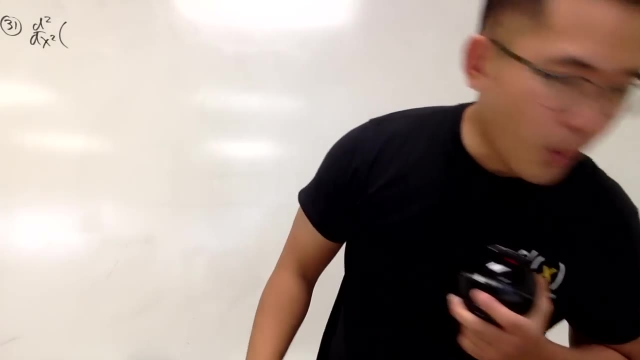 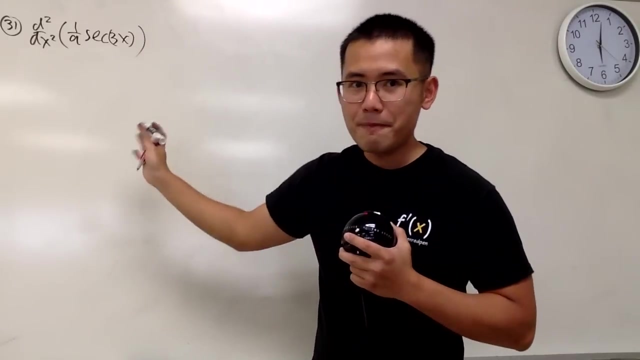 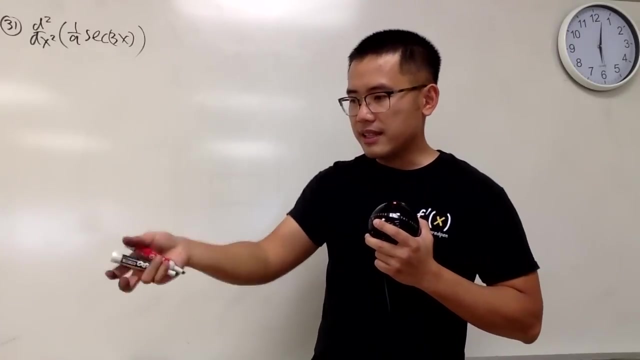 this is. this is this is x2, differentiating whatever is inside twice. here we have 1 over 9 secant to the no secant of 3x, just like that. okay, so here is the DO d2. dx2 means dx, sorry, ddx, ddx, okay. 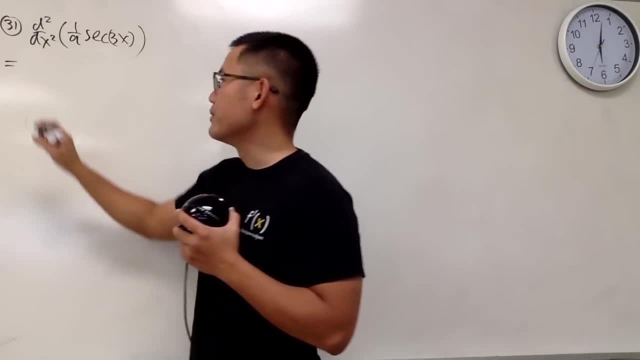 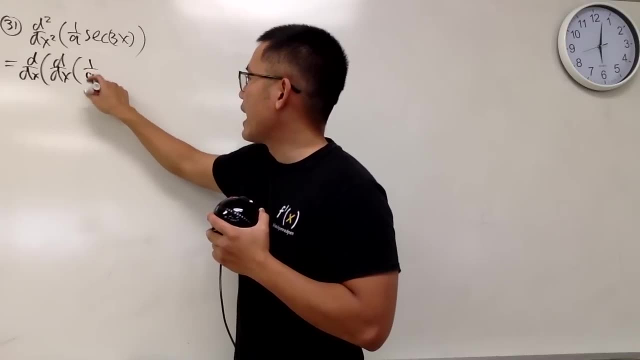 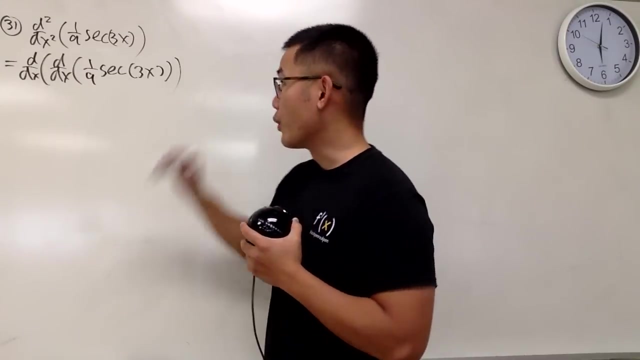 so I will do this one right here, just to show you guys what we have to do. we have to differentiate of differentiating like this, and then 1 over 9 secant of 3x. so we look at this, do it inside out. so here we go, and perhaps for the inside we'll just 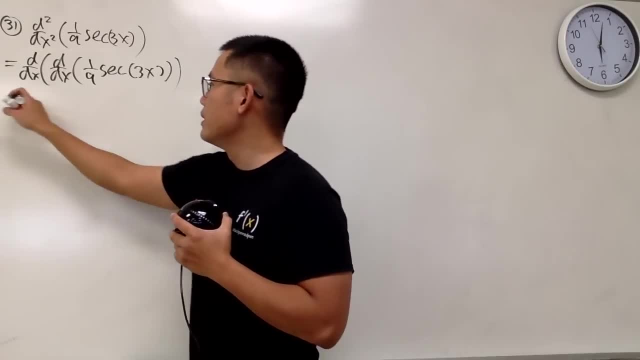 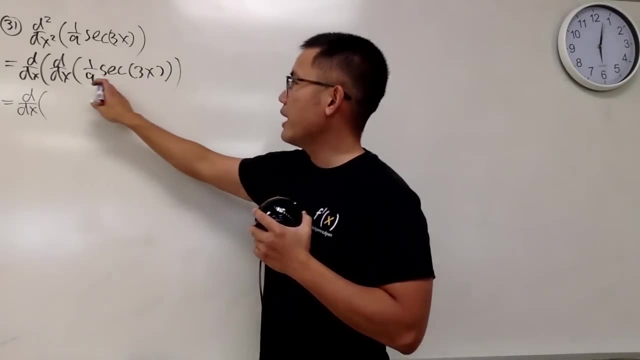 do the end, do the part in black- I mean in blue- and then the final answer: I will end it with black. okay, so differentiate this part. okay, this is not so bad. we have 1 over 9, it's just a constant multiple. 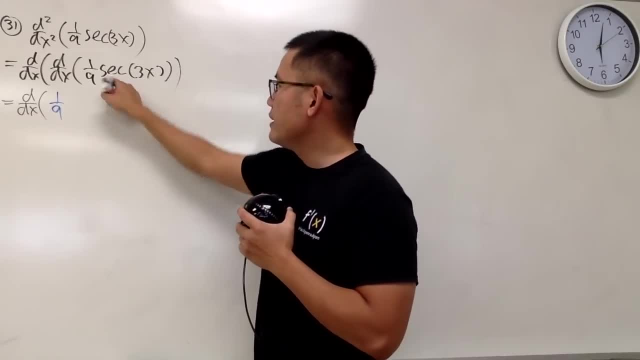 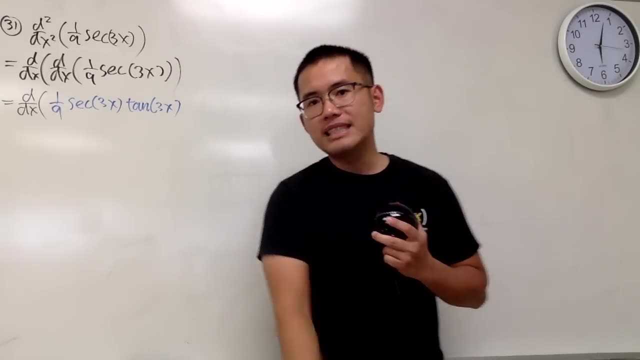 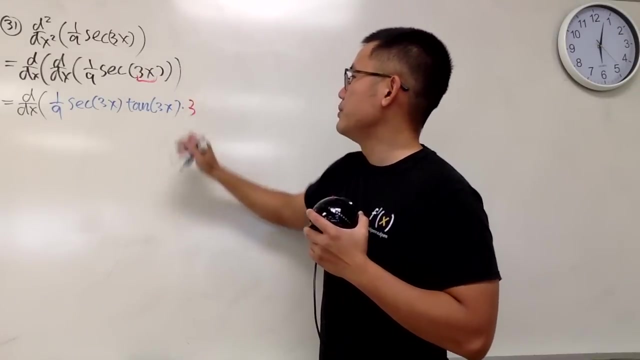 Write it down. write it down. write it down now. differentiating secant of whatever. you put down secant of that whatever times tangent of the same whatever. but we have to multiply by the derivative of that, whatever Chen Lu said, so not me- multiply by 3, so that's. 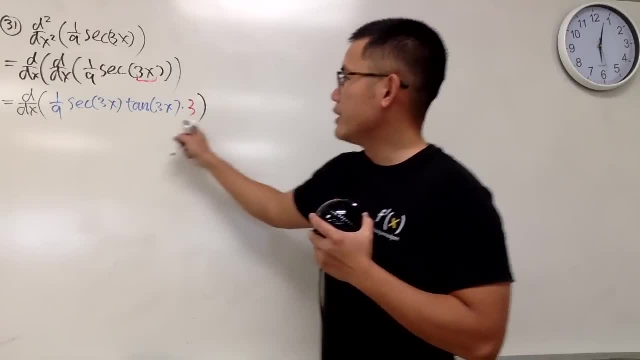 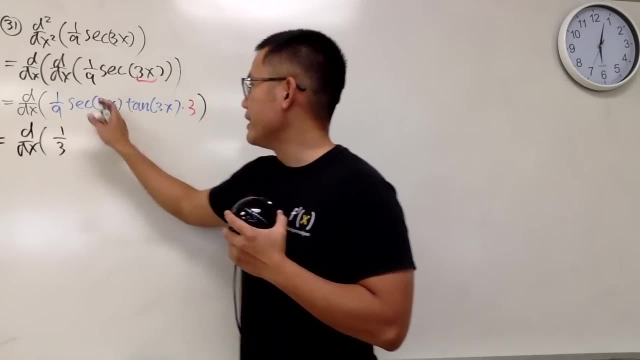 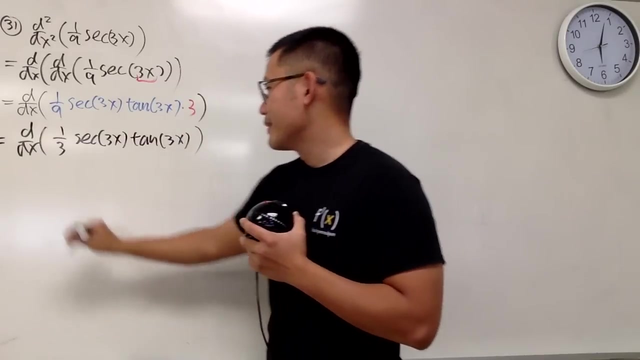 pretty much the idea. well, we can reduce this. that's just 1 over 3, so we will. this is going to be differentiating 1 over 3.. Okay, and here we have secant of 3x times tangent of 3x, now differentiating this. 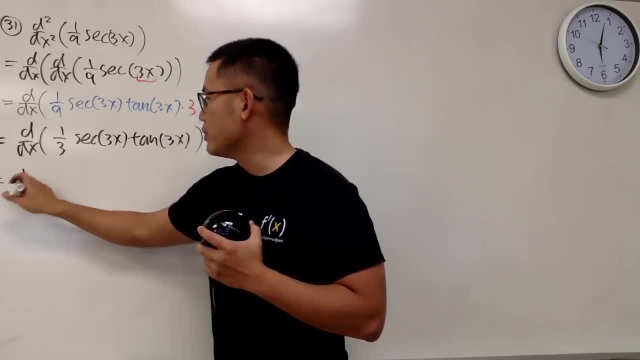 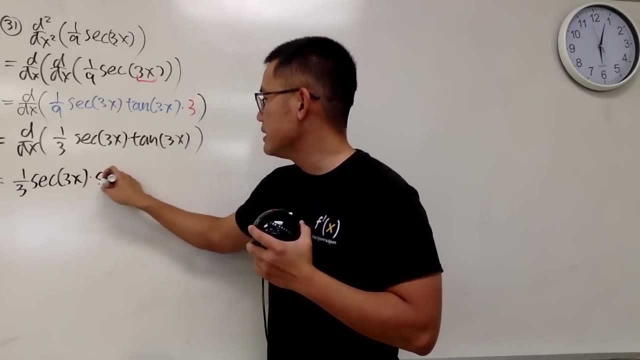 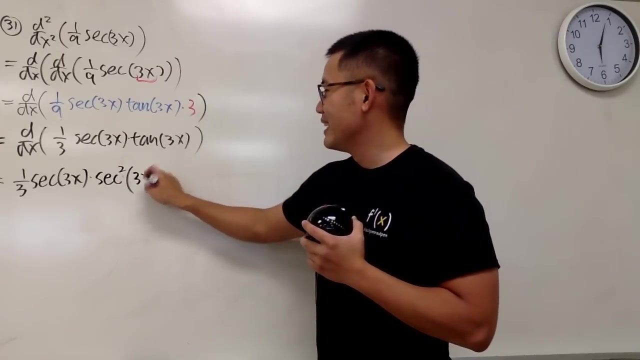 product rule in action. this will be my first function. I'll keep it, which is 1 over 3, secant of 3x times the derivative of the second derivative tangent is secant to the second power and the input is 3x times 3x. 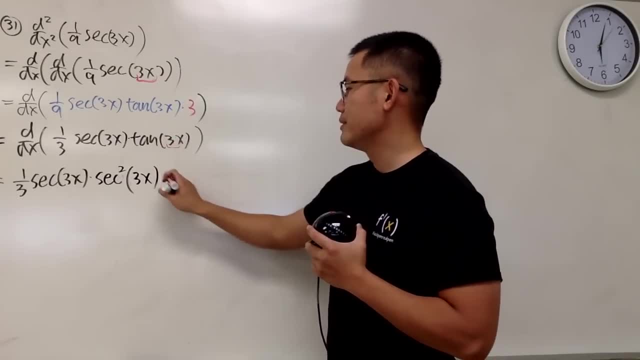 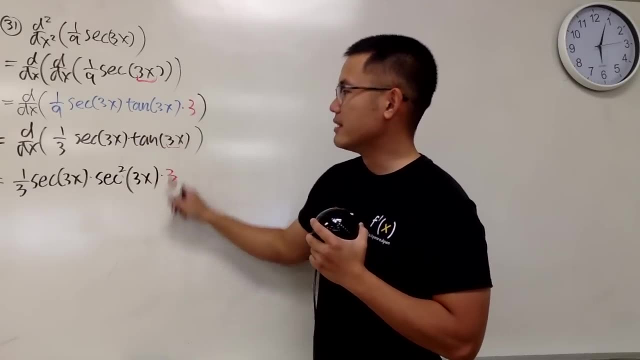 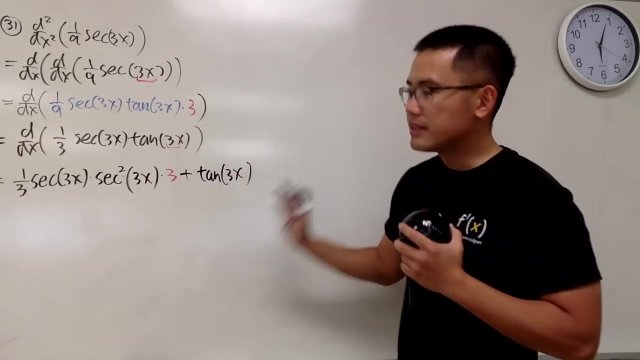 Okay, Okay, The derivative of 3, the derivative of 3x, which is 3, because of the Chen Lu said so. okay, So this is the derivative of tangent of 3x. Now we have to add the second function, which is tangent of 3x times the derivative of. 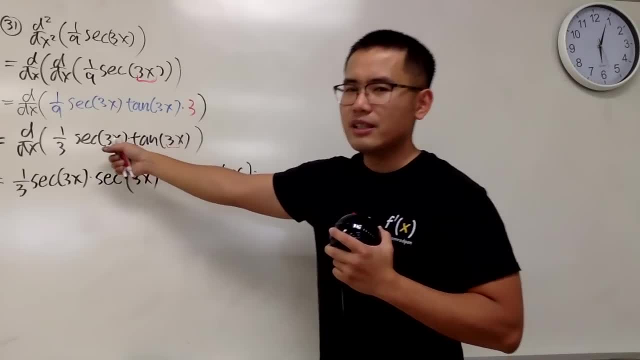 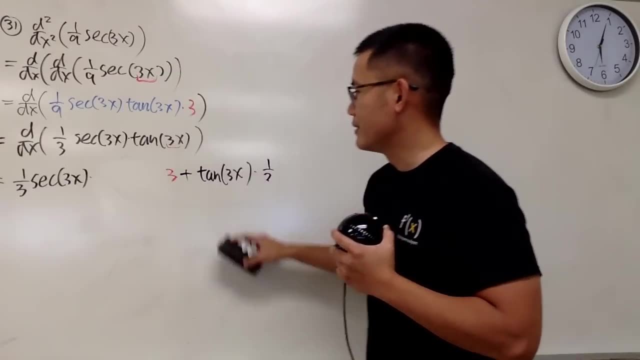 the first derivative of 1 third of secant to the secant of 3x. you write down 1 third secant actually. oh, I messed up with the column. Sorry, Let me do it again. I messed up with the column. 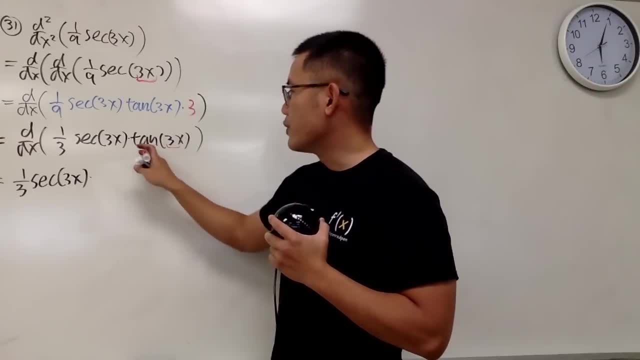 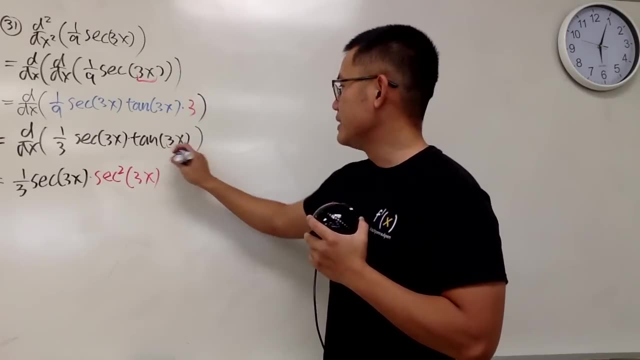 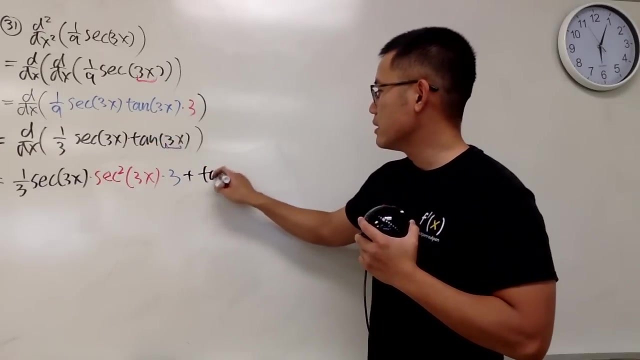 Okay, First function times. the derivative of the second derivative secant derivative tangent is secant to the second power of 3x. but we multiply by the derivative of the inside, which is the 3,. right here Now we add the second function, which is tangent, of 3x, then we multiply by the derivative. 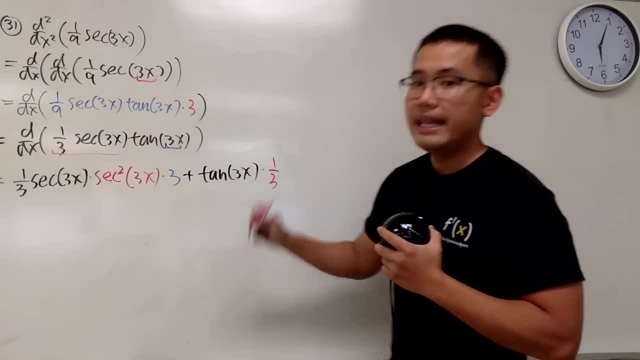 of the first, which is the 1 third, And the derivative secant is secant to the second power of 3x. So it's the second function right here, And the third function we multiply by the derivative of the input, which is the secant. 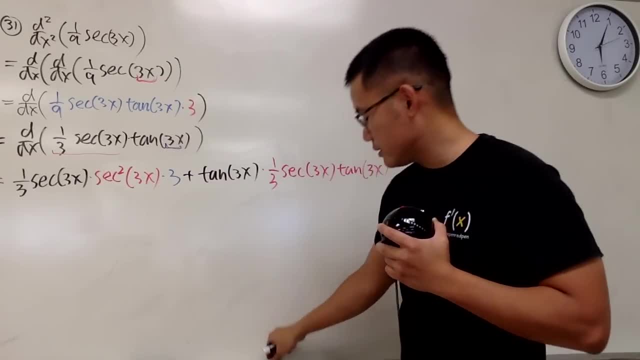 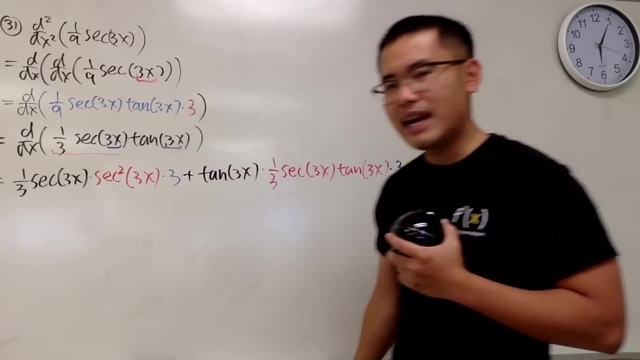 of the input times tangent of that input And the derivative of that input. So you multiply by 3, right here. So that's pretty much it, and now you see that 1- third and 3 cancel for the first part. 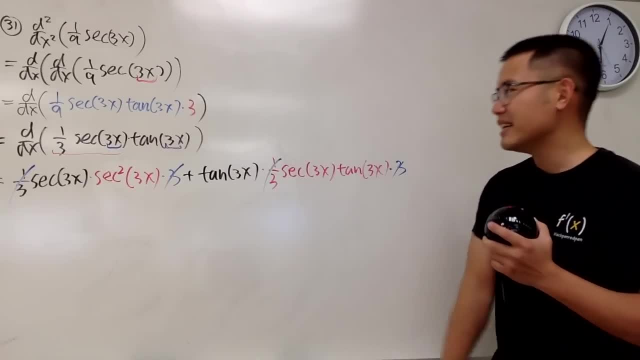 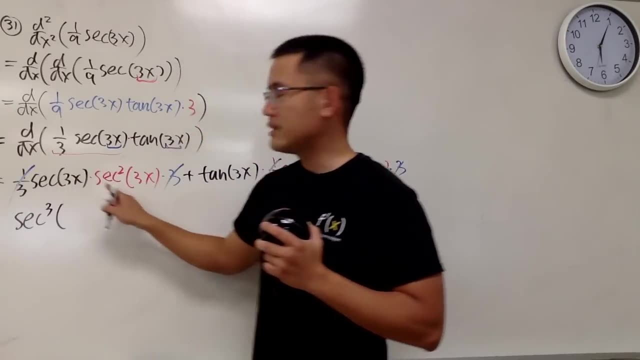 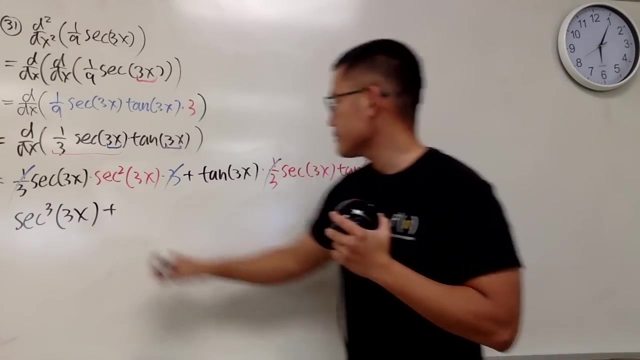 and this 1 third and this 3 cancel for the second part And we just put things together. Finally, the answer is secant to the third power, right this times that first power, second power, third power, and here we have the 3x, like this and we add: this is secant. let's just write down. 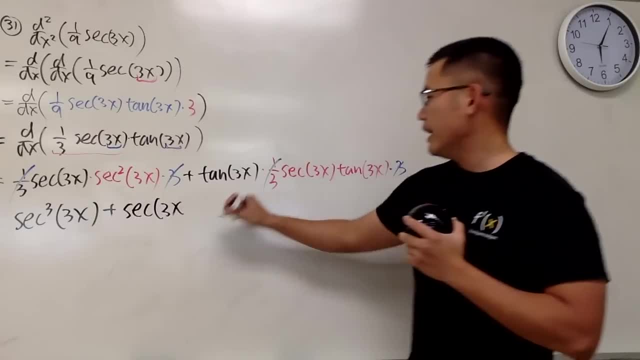 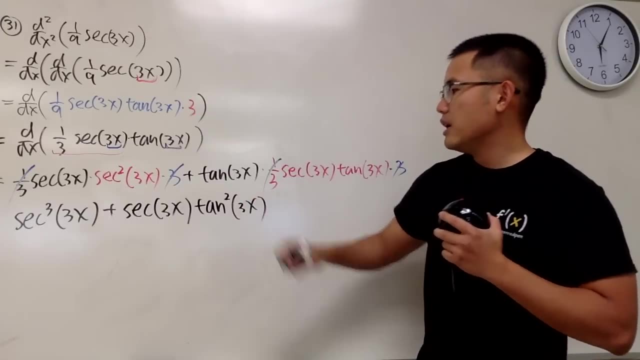 the secant first, secant 3x and tangent tangent. so that's tangent second power right, second power 3x, and again you can perhaps factor out the secant of 3x, but secant squared plus tangent. 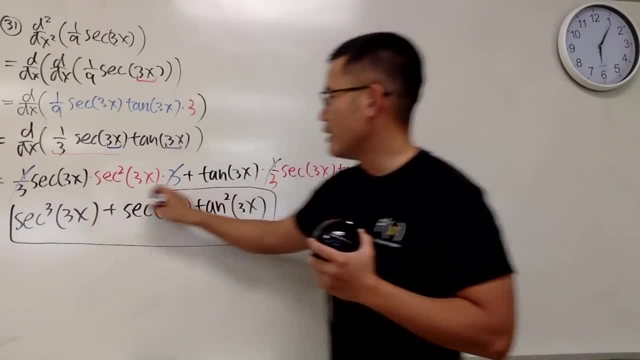 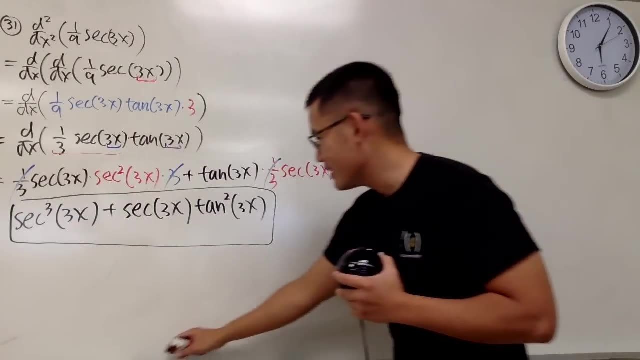 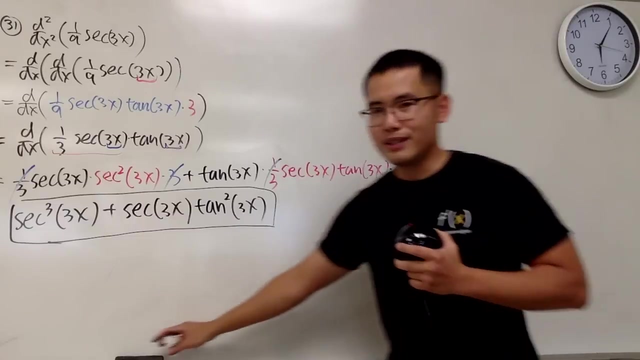 squared, not so much you can do with it, so just leave it like that. in fact, that's what I did as well. that's the answer. okay, this right here is the answer for it. All right. what's after 31?? Of course 32,, but it's just another derivative. 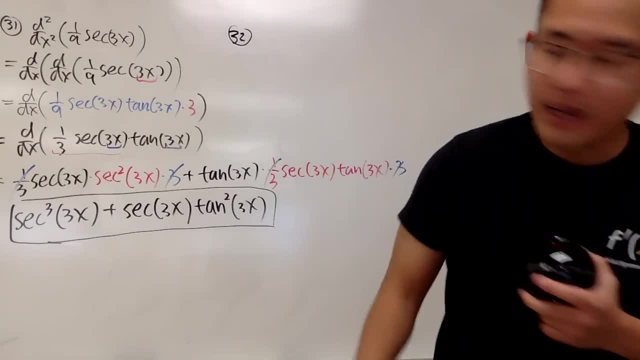 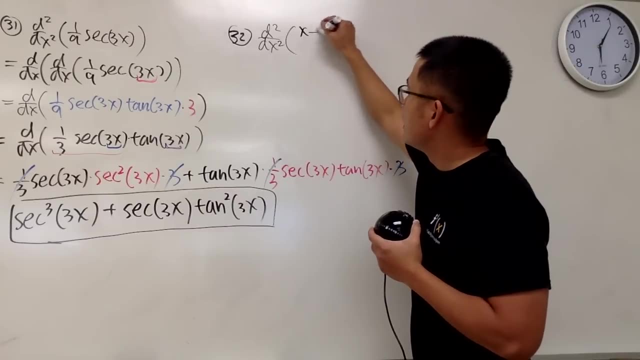 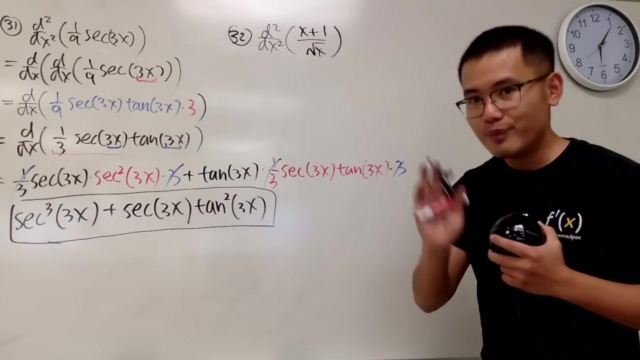 second derivative number 32, okay, d2, dx2 of. we have x plus 1 over square root of x. Okay, do we need to use quotient rule? No, we don't, because thankfully the bottom is just half one term, so that means we can split. 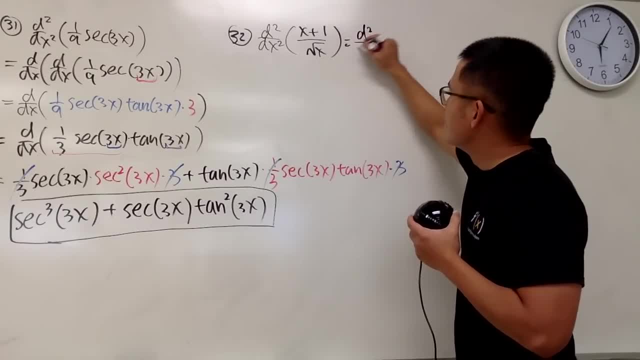 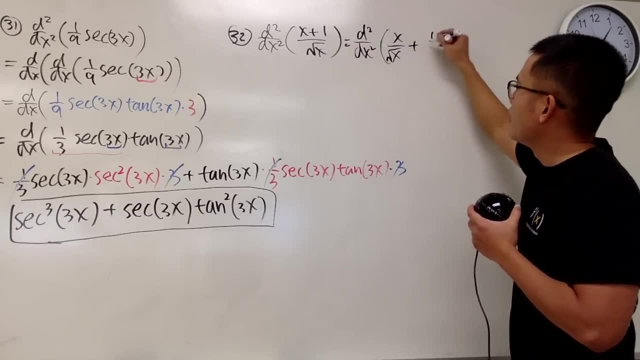 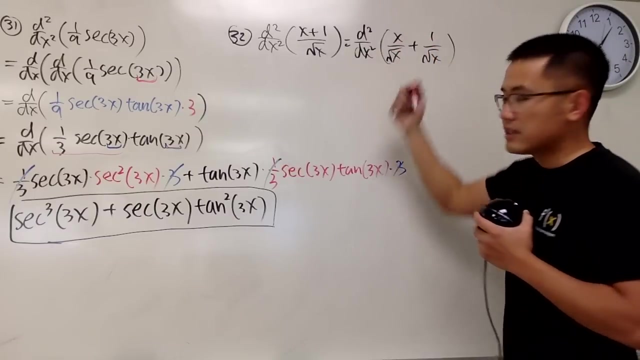 the fraction nicely. so we will just have to differentiate like the secant derivative: okay, x over square root of x and then plus 1 over square root of x. Remember, remember, remember. the square root is like the same as what One half power. so perhaps I should. 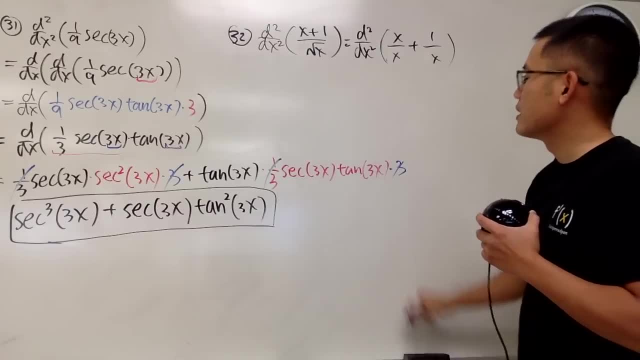 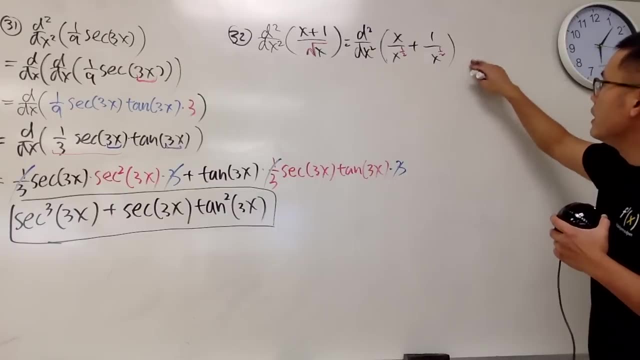 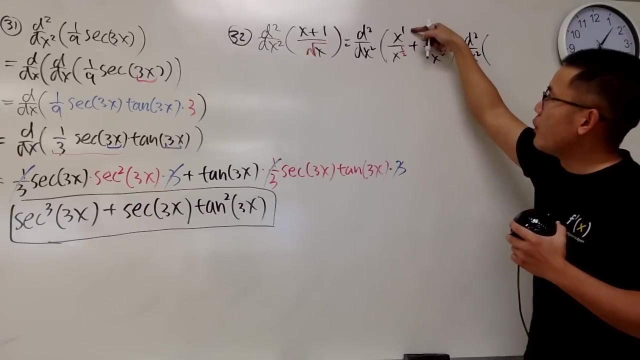 have write this as the. I should have written this down as the one half power. so right here, let's put a one half, put a one half, if you would like. well. well, that means what? Differentiating this twice, this is the same x to the first power over x to the second power. so subtract the powers. 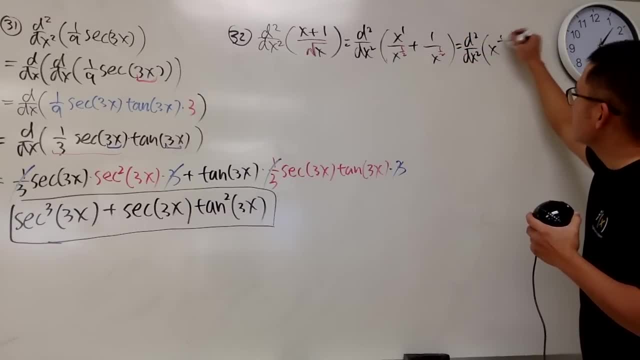 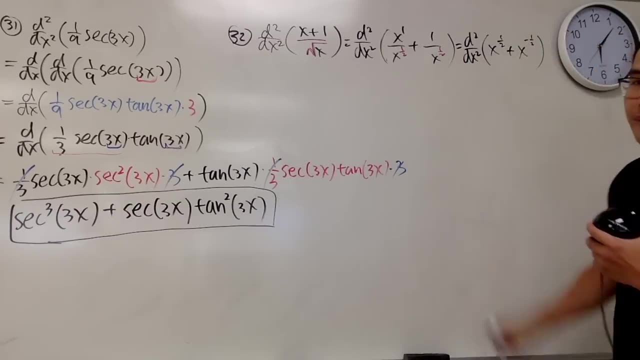 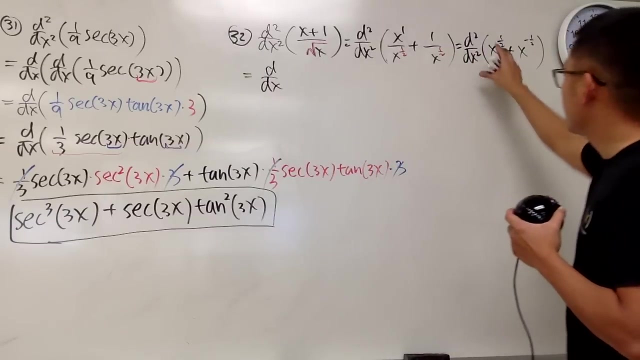 we get just one half. so we have x, x to the positive one, half power for the first one. for the second one, we have x to the negative one: half. okay, and now here we go. Notice, I just put on d dx because I'm going to do the first. 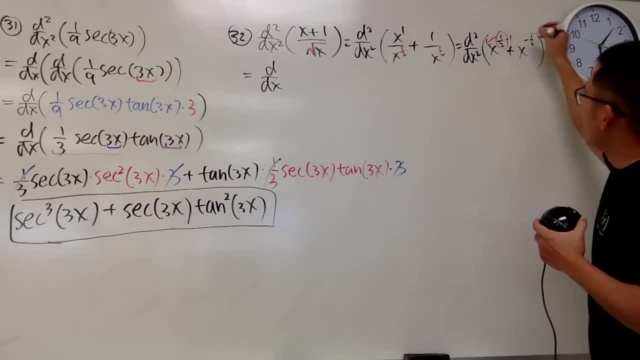 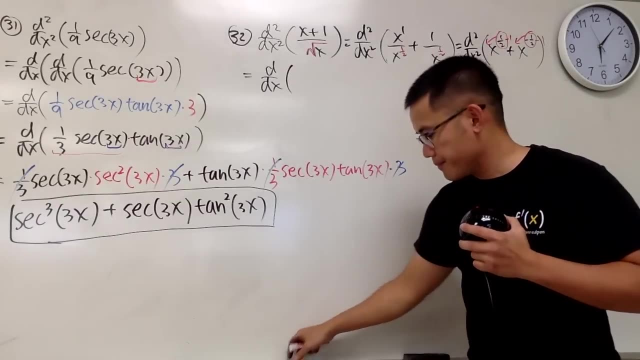 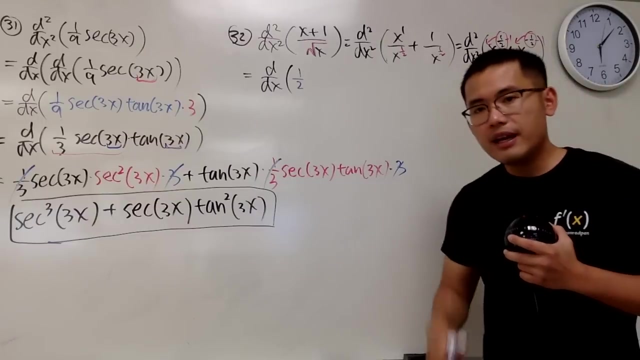 derivative right here already. Let's bring the power to the front minus one. bring the power to the front and minus one. So for the inside- here you'll see the first answer. here is one half and you have x to the negative, one half, and let's just write it down as a power because we have to. 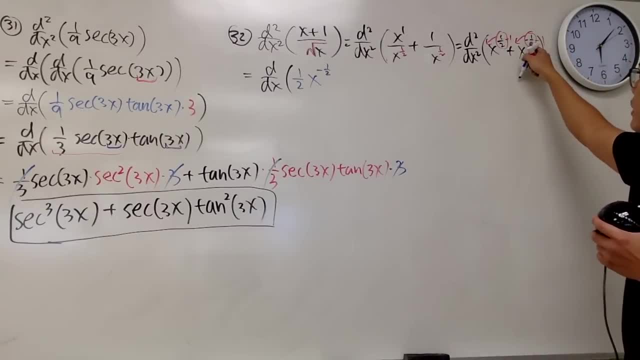 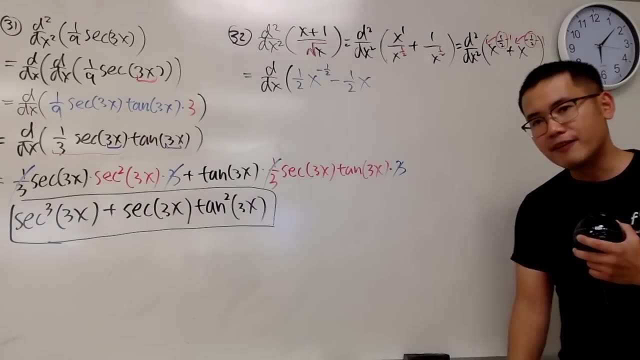 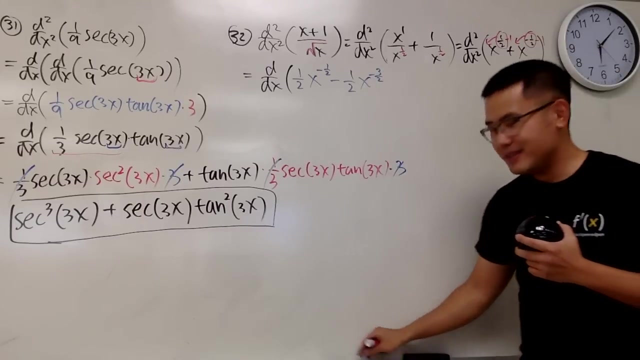 do the derivative again. Similarly for the second one, we have negative, though negative one half, and then x to the negative one. half minus one is negative three half. Ooh, I don't know why I did that, but whatever. 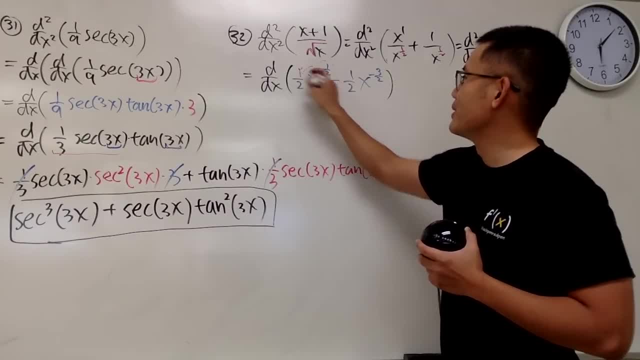 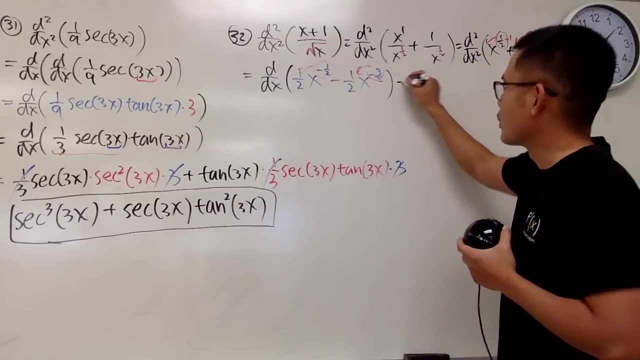 And then, finally, you bring this to the front and do the derivative again. Alright, I don't know why. I thought it was a good idea to just show you guys a lot of derivatives, like even the second derivative. so I'm actually doing like 120 derivatives right here. 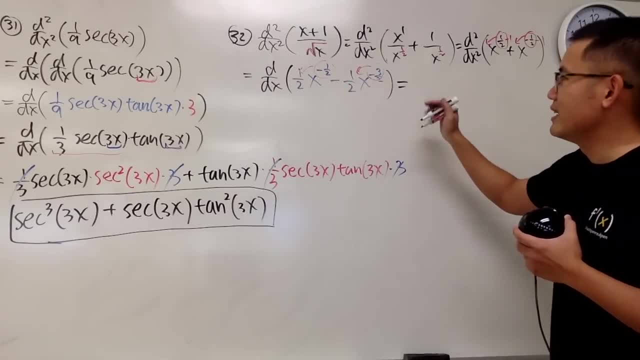 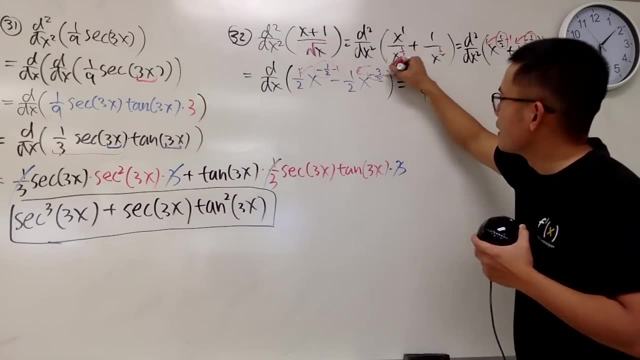 Anyway, this times that no more d, dx, whatever, just the answer, this times that is negative one over four, and this times that Don't forget minus one, don't forget minus one. so we get x to the negative three half. 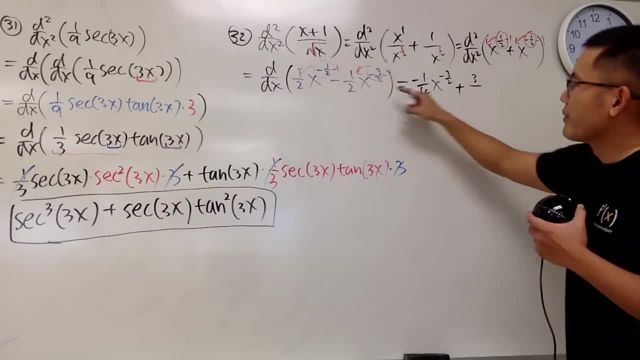 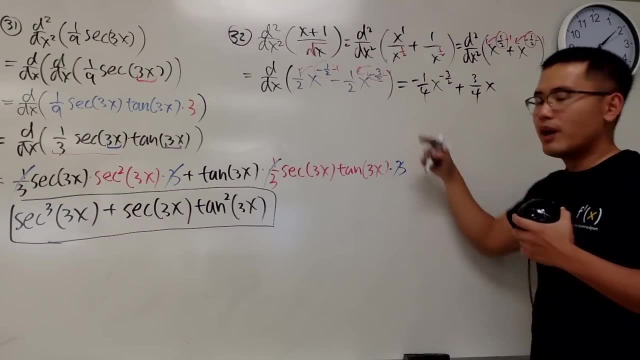 negative becomes plus 3 over 2 times 2 on the bottom, so we have over 4, and then this is x negative, 3, half minus 1 is negative, 5 over 2, like that. Okay, you think you are. 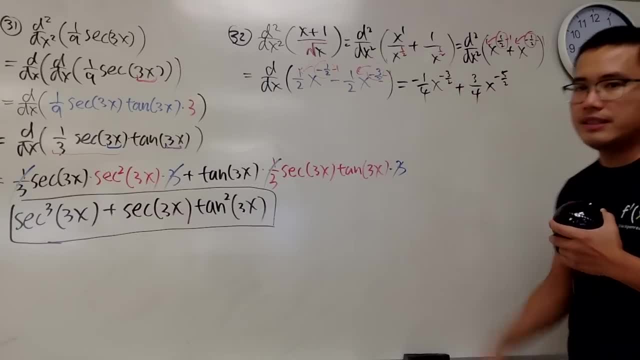 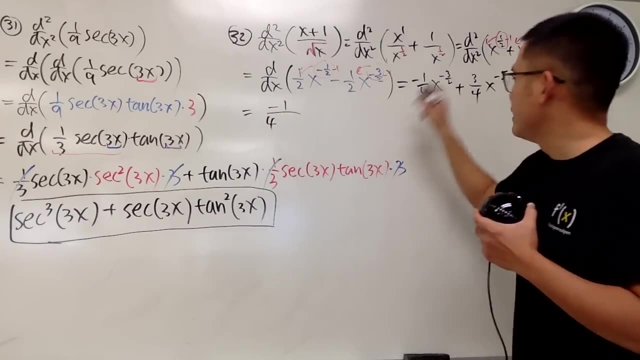 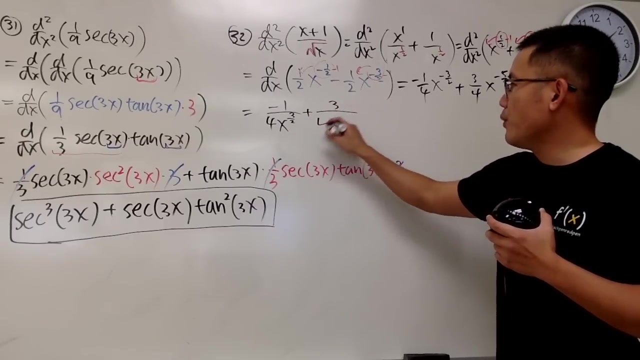 done, but, no, not yet. Bring the x down to the denominator and then work out the simplification So you get negative 1 over 4, and this is x to the 3 over 2 power and plus 3 over 4,. 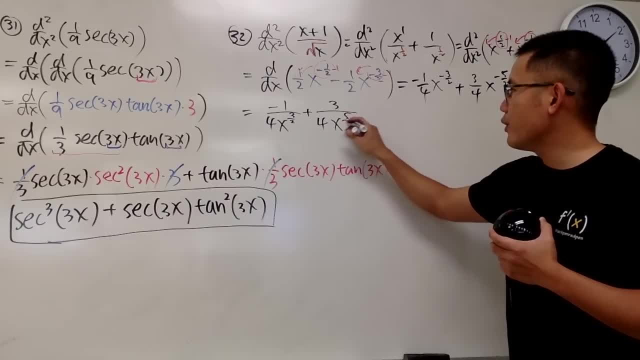 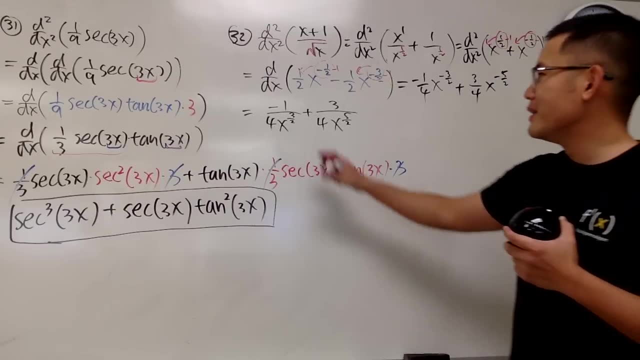 and this is x to the 5 over 2 power. Can we get some common denominator and clean things up? Yeah Well, this is 3 half, If I can get 5 half. this is the same as saying x to the. 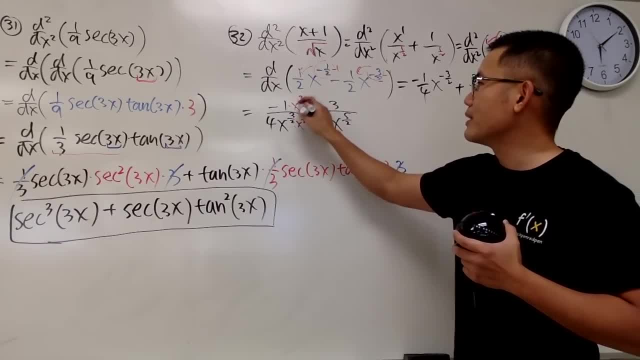 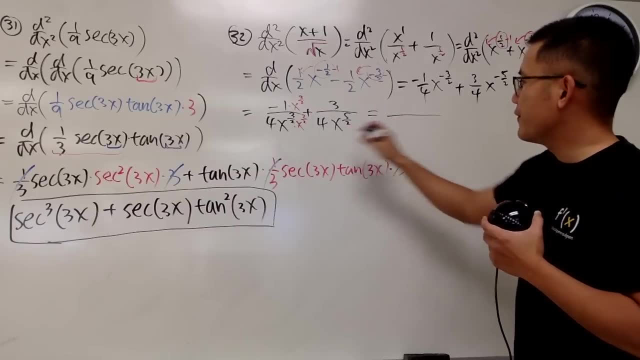 2 over 2.. Which is just x to the first power, but I'll put it out as x to the 2 over 2.. That's all we need, right? Well, all in all, you get 4x to the 5 half, and I didn't write it as. 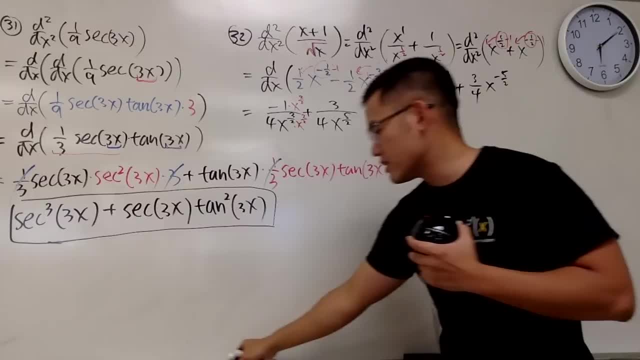 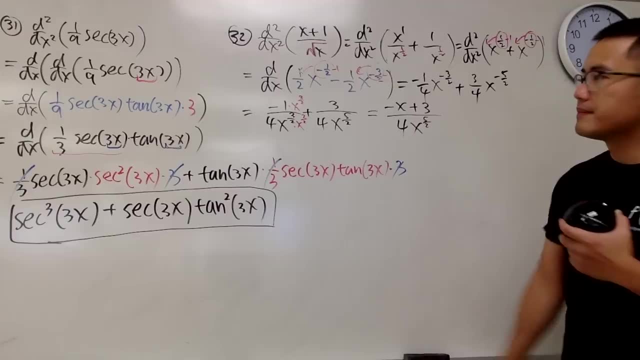 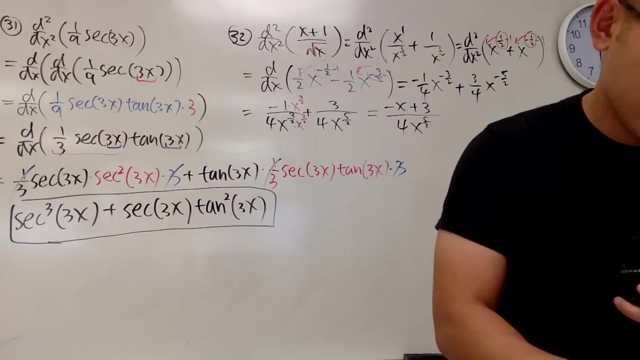 a radical for the answer choices. we'll just keep the answer like this, and this right here is negative x plus 3, and I believe that is it, And I even have the. I have the right order. Well, I didn't have the right order, but I'll put out 3 minus x, which is 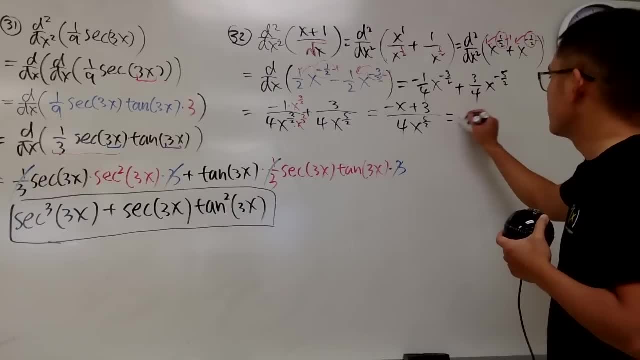 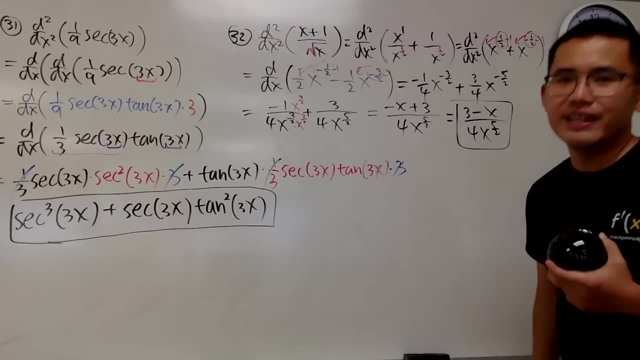 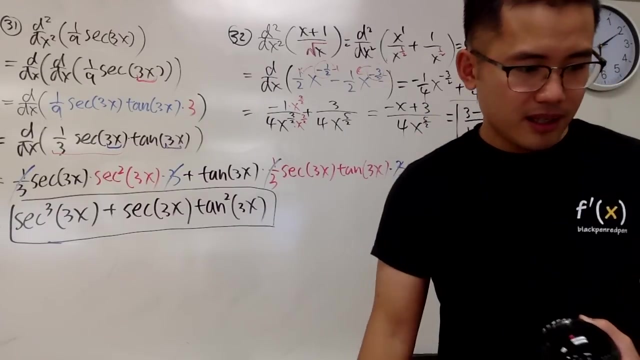 the same thing. Okay, So of course, perhaps this is right. yes, 3 minus x over 4x, 5 over 2 power. Like this Good Man, this is so computational. like for the derivatives, they. 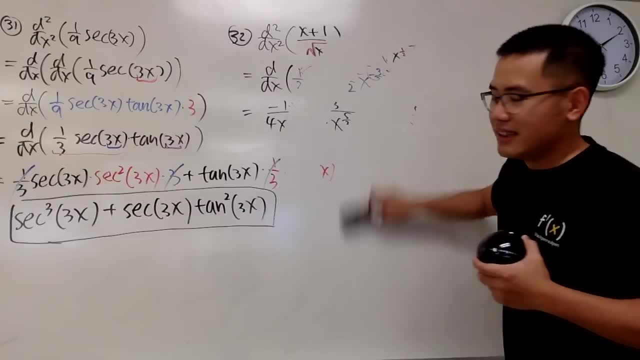 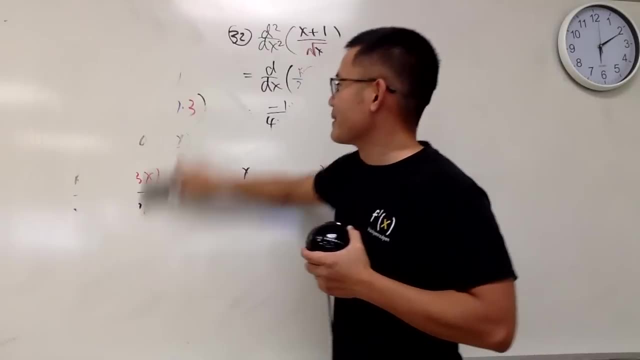 are just so computational. You have to do a lot, a lot of algebra, And I don't know why I- like I was trying to come with the questions right, I was like, huh, maybe the question is too easy, so I make. 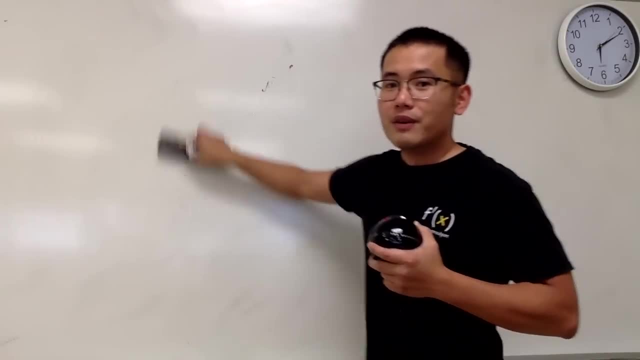 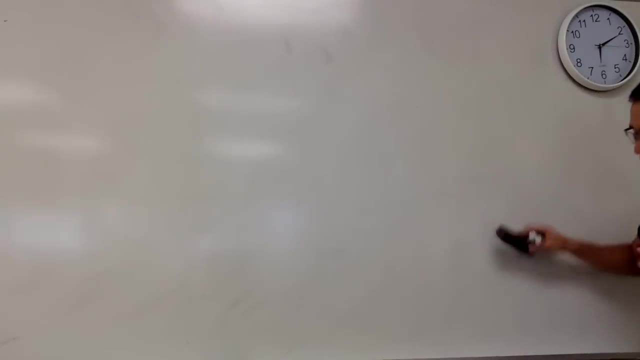 it harder. So I was just having like 100 first derivative. So let me make it harder. Let me put in some implicit differentiation- I did. Let me put in some second derivative, I did. Let me put in some definition of derivative- I did. 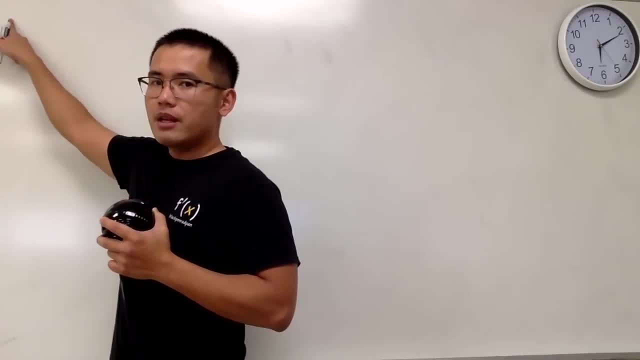 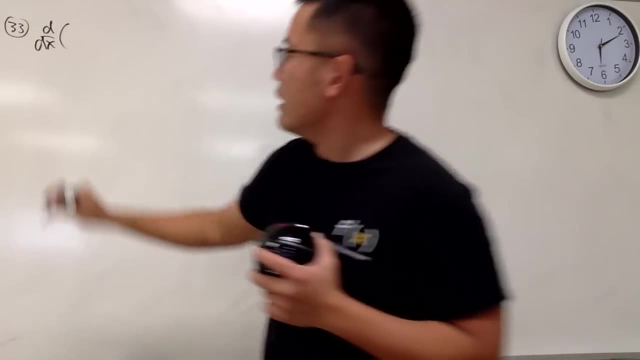 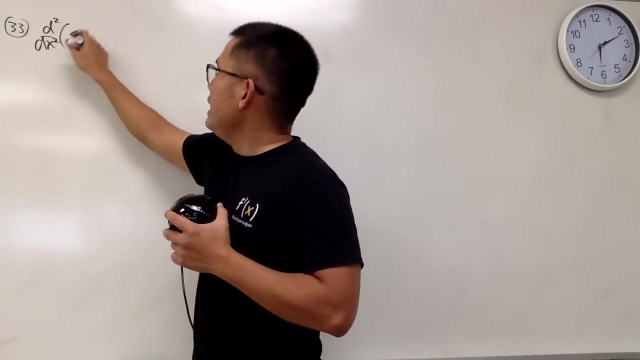 Man, okay, number 33.. Here we go, d dx And we are going to have- well, sorry, in my dream- d2 over dx2, right Here we have inverse sine of x squared, Oh my goodness, Inverse sine of. 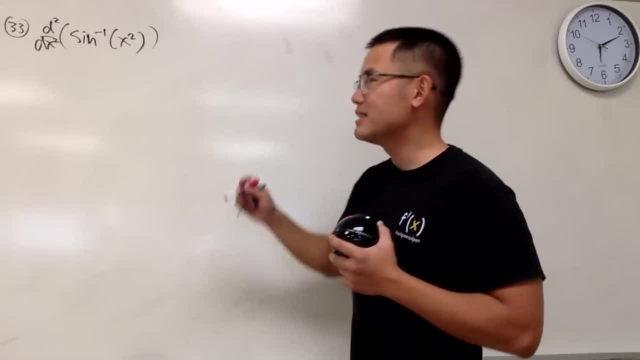 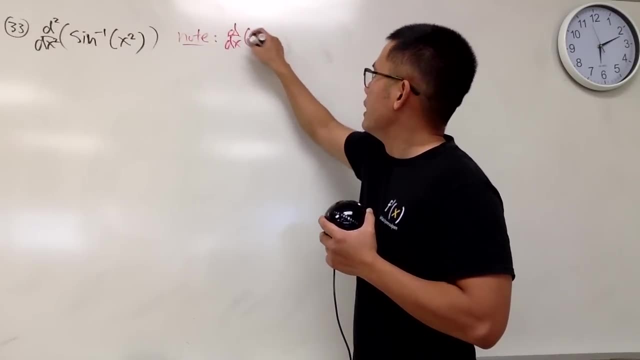 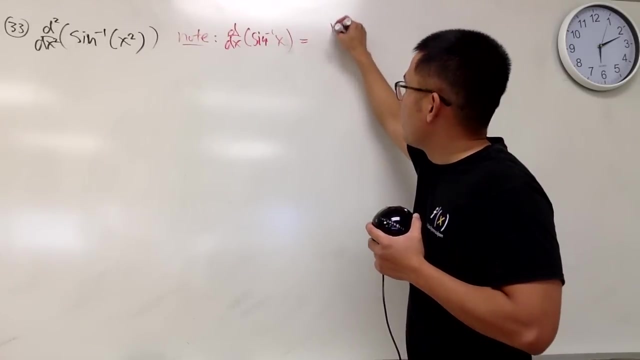 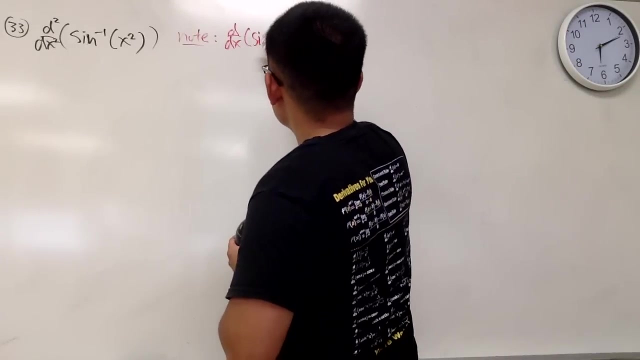 x squared. Of course, here is everybody's note Right, Everybody's favorite note: Okay, To differentiate inverse sine x, This right here is 1 over square root of 1 minus x squared, And maybe you guys can use the chance to kind of Google it to see if I did it right or not. 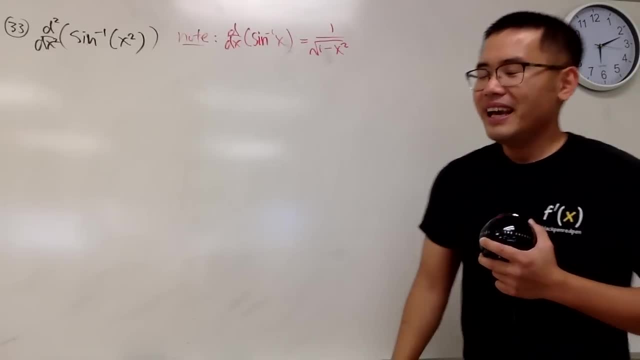 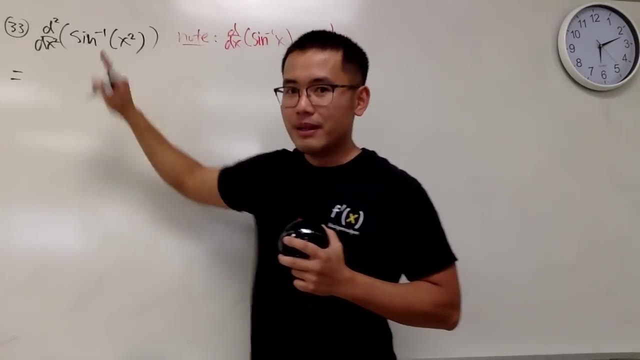 But just help me out if you can tell me if it's right or not. Anyway, it's not funny, I know. Okay, here we go. So here is the input. But you see, I will actually just write down d dx. 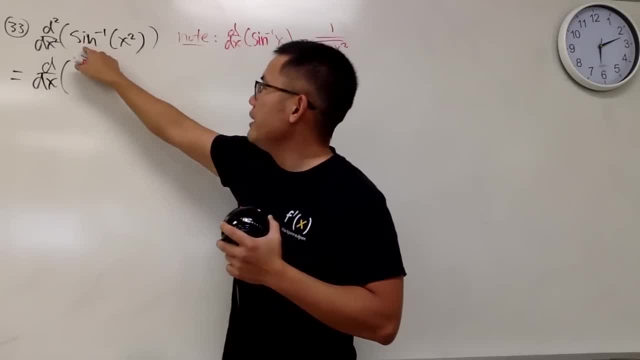 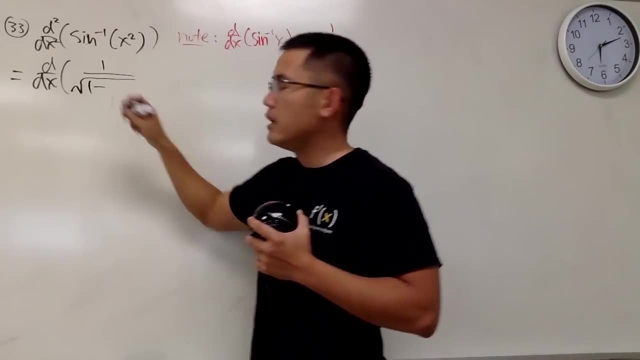 Okay, because I am doing one derivative already: Inverse sine. I get 1 over, open the square root, Open the square root and then the 1 minus the input and you square. The input is x squared, but you have to square this again. 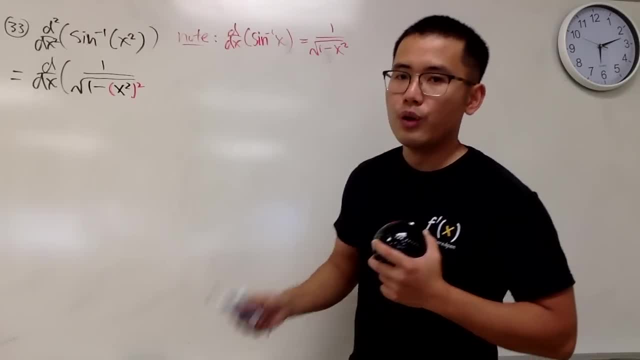 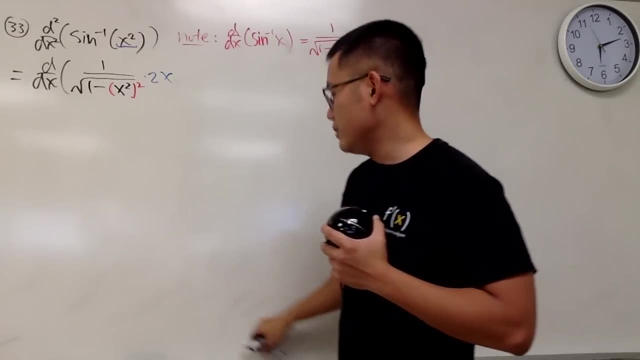 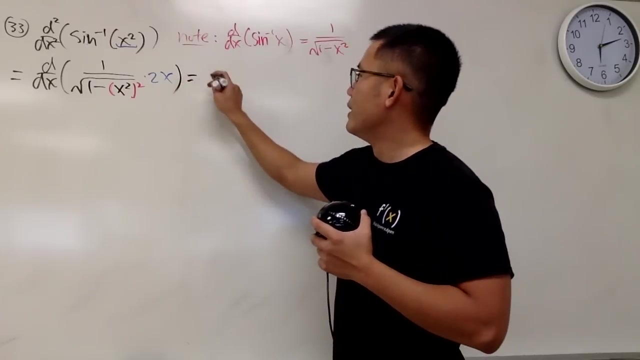 Like that, Are we done? No, we still have to use the channel Multiply by the derivative inside. The derivative of x squared is 2x. So that's what we have. Okay, Man, we have to differentiate. what now? 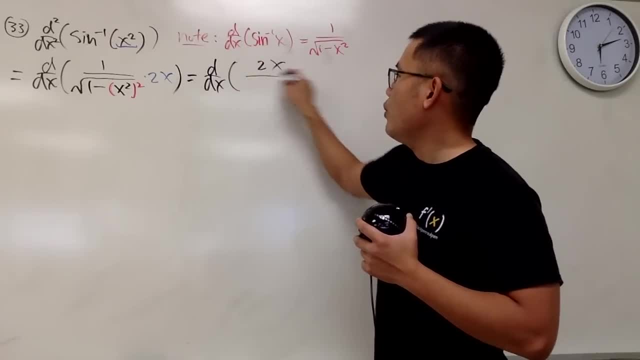 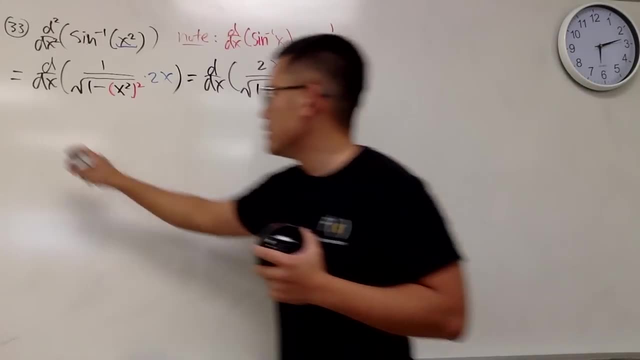 Differentiating 2x over square root of 1 minus x to the fourth power. Oh man, Quotient rule, Put down the denominator Square that. So we have square root of 1 minus x to the fourth power. 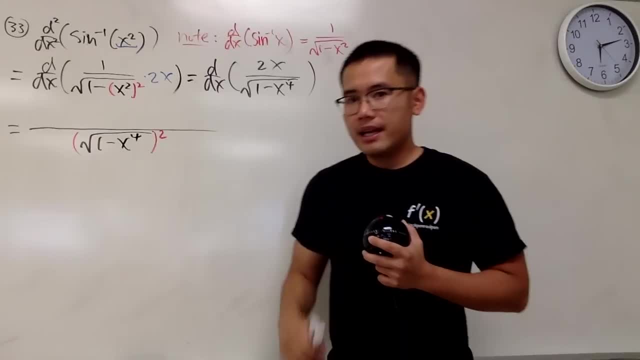 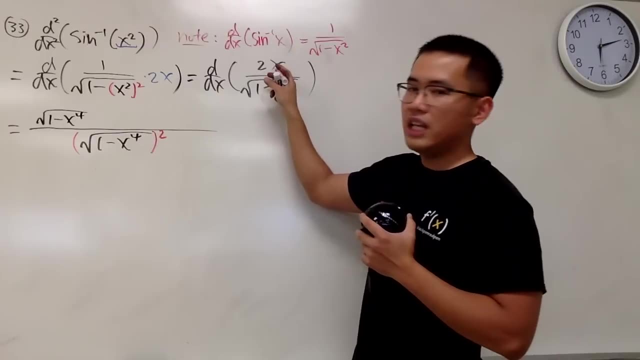 And we square that Bottom function, put it on the top, which is square root, of 1 minus x, to the fourth power Times, the derivative of the top, The derivative of 2x, is just a 2.. And then we minus the top function, which is 2x. 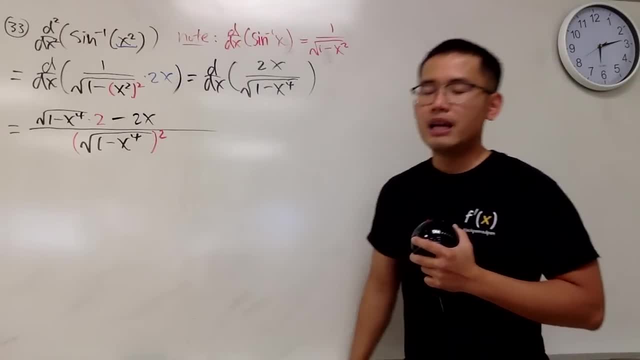 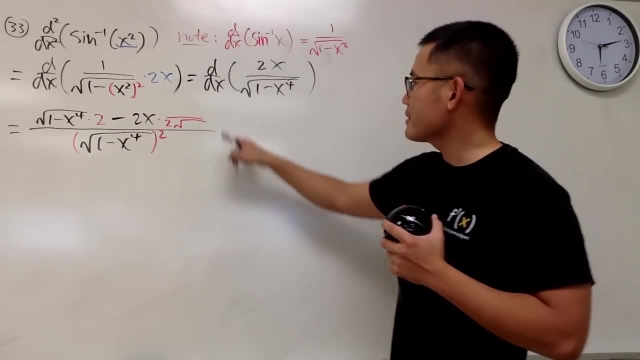 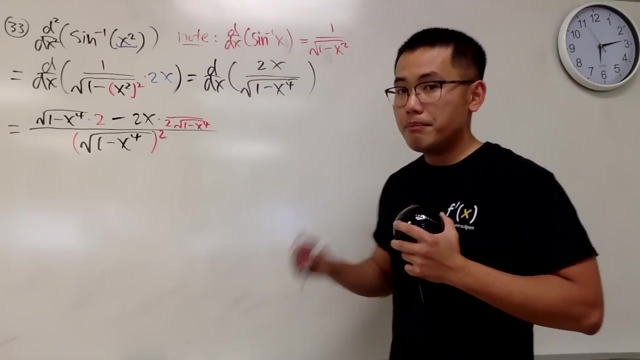 And we multiply by the derivative of the bottom, It's a square root. So we first have 1 over 2 square root. I have a 1.. Keep that in mind. 1 over 2.. Okay, 2 square root of the inside, which is 1 minus x to the fourth power. 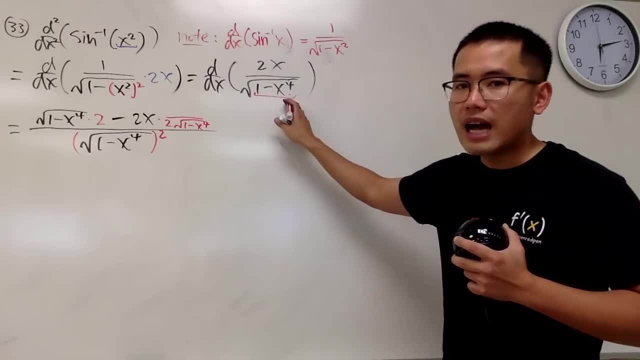 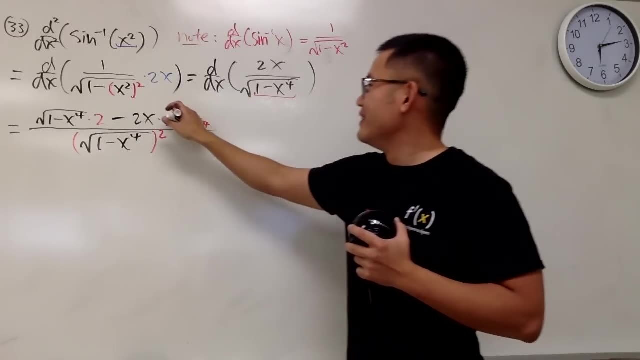 But don't forget, the chain rule says we have to multiply by the derivative of the inside Derivative of negative 1 minus x to the fourth power. we get negative 4x to the third power. like this, Okay, Just like that. 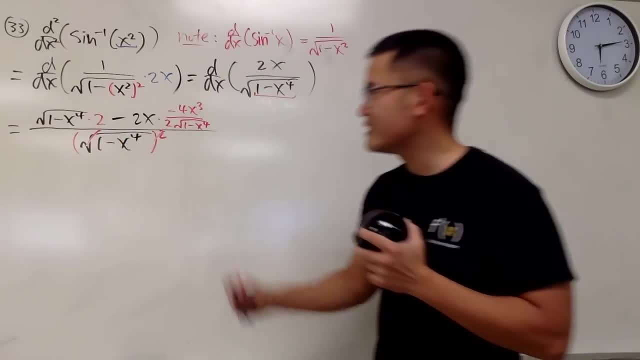 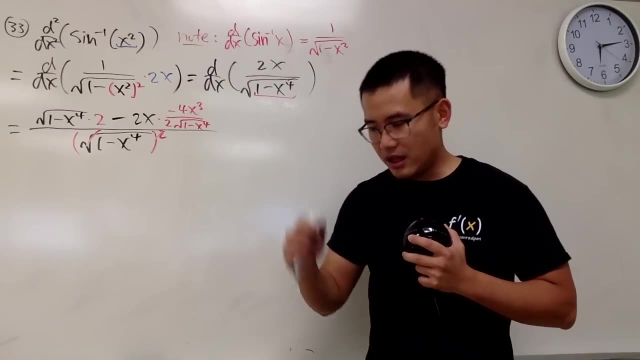 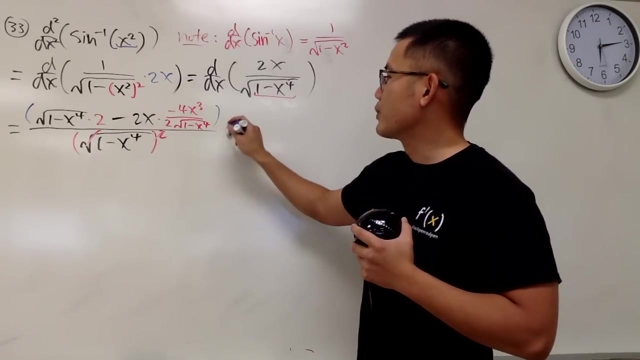 Okay, Cancel, cancel. Yes, But complex fraction. We have this guy in the denominator on the top. No good. So let's multiply the top and bottom by the square root of 1 minus x. to the fourth power: Okay. 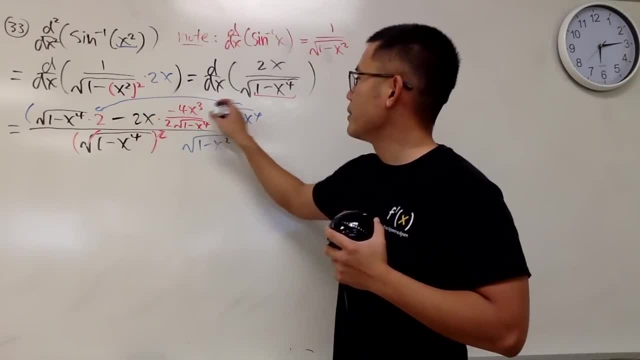 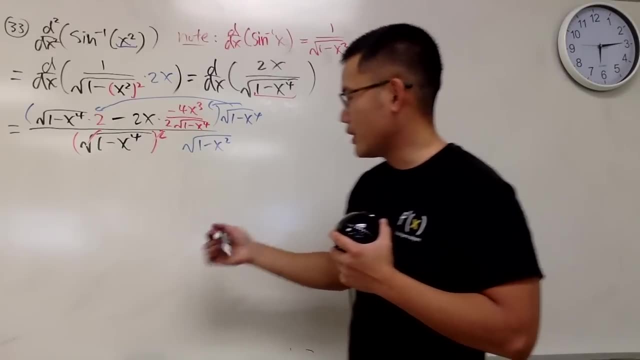 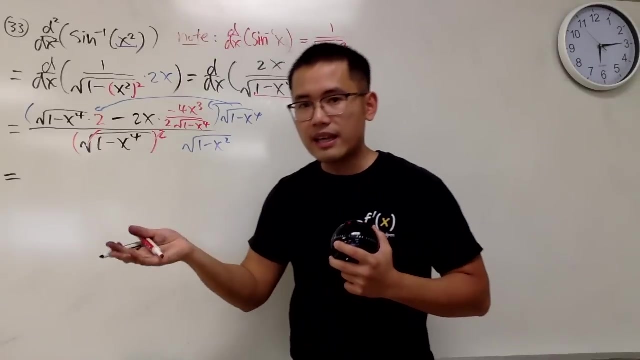 Yeah, Alright. So multiply, multiply, And these are gone already, the square and the square root. So they are gone already. So let's see what we have. Okay, Square root, square root. they cancel when they multiply. 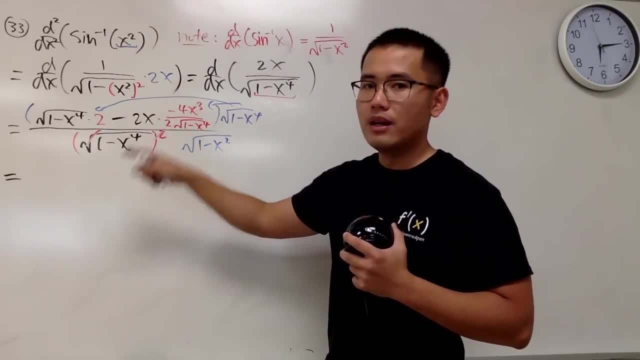 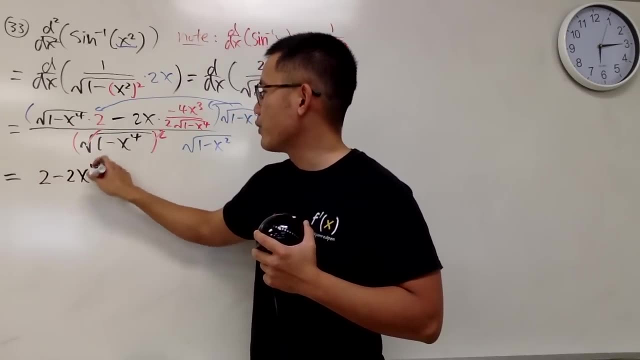 So you have 1 minus x to the fourth power, But you have to multiply by 2.. So you actually get 2 times the inside, which is 2.. 2 times that is minus 2x to the fourth power. 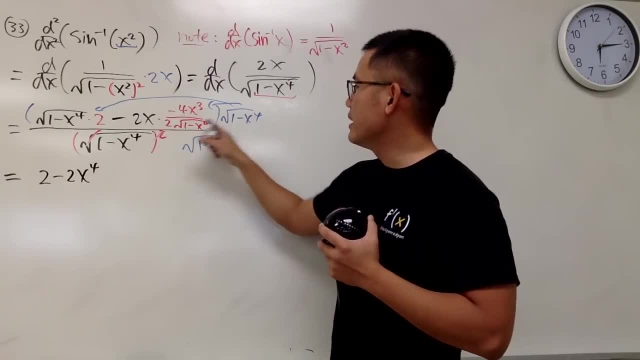 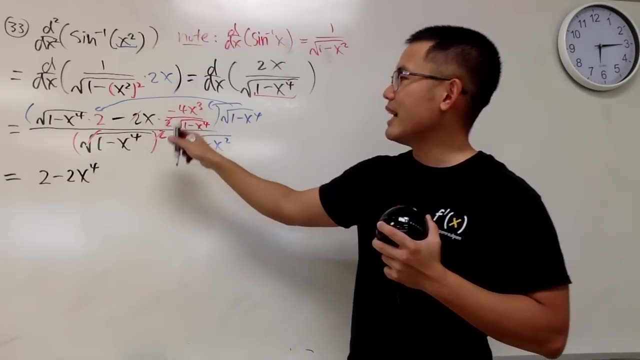 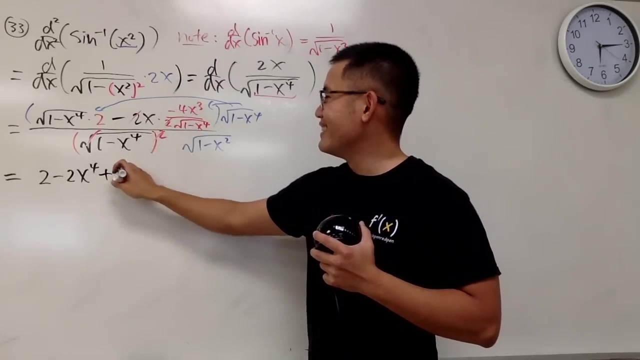 Okay, And then let's see This and that cancel out as well. Okay, 2 cancels out with this, 2.. Yeah, And So negative e times negative, e is positive 4 and x to the fourth power. 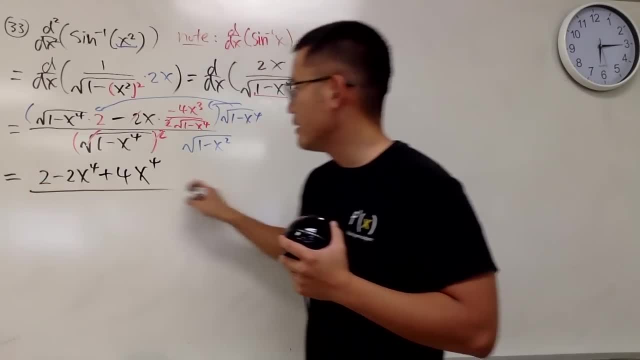 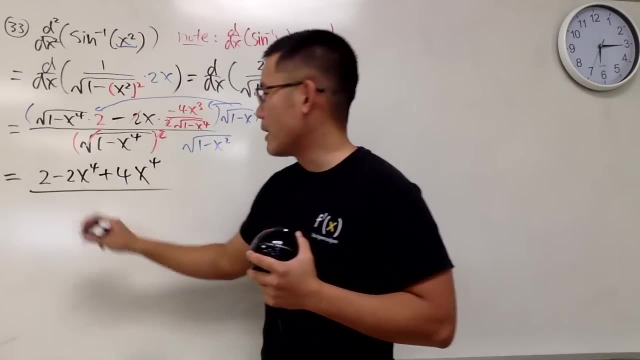 Yes Over. How do I write the answer key? Okay, I have the third power. Okay, Okay, Okay, So this, right here, I put it as the first power. So I write it: 1 minus x to the fourth power. to the first power. 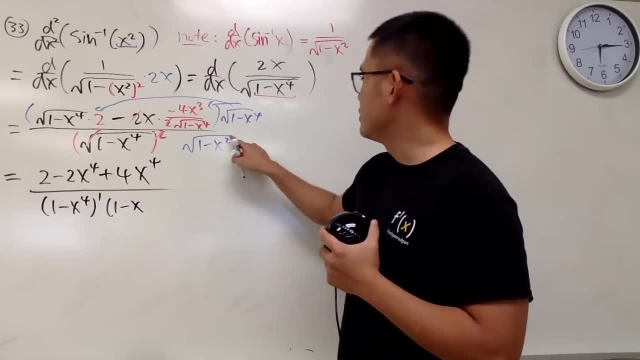 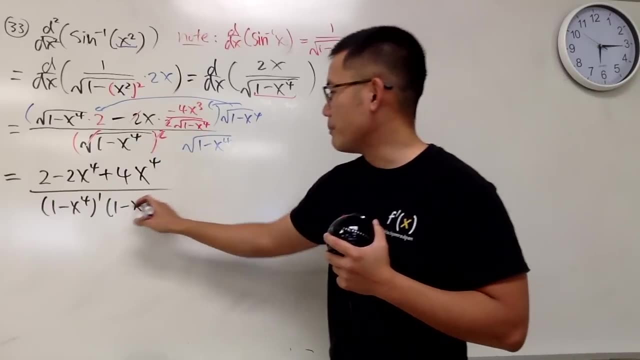 This right here. I wrote it as 1 minus x to the. Sorry, This should have been a 4. And that should be the same. So 1 minus x to the fourth power in the square root. So this right here is 1 minus x to the fourth power, to the one-half power. 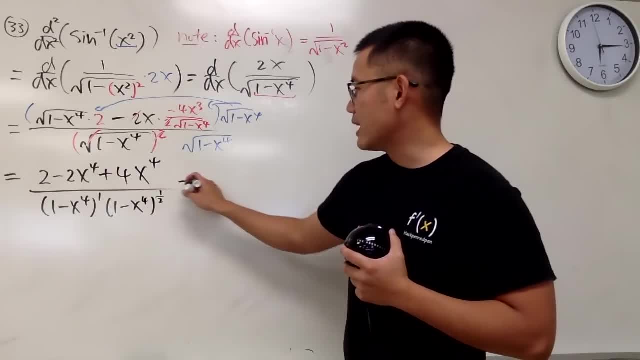 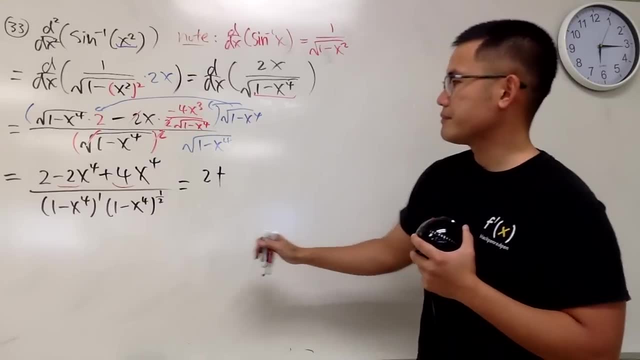 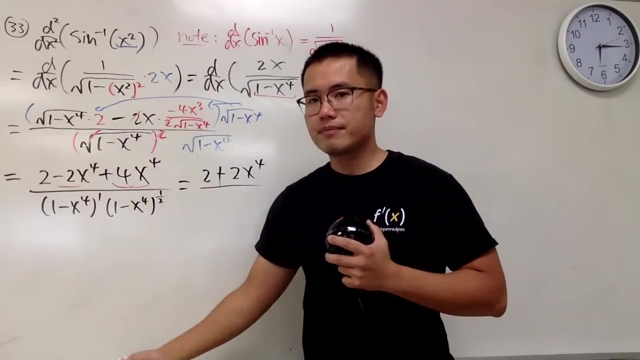 Okay, On the top we can reduce that 2 minus No, plus This and that together We can get 2x to the fourth power over. Now for the bottom, they have the same base, Just add an exponent. 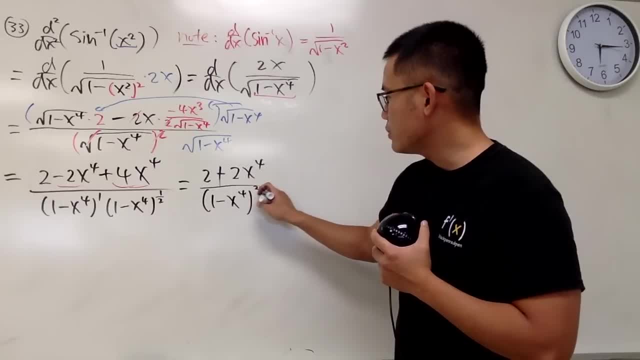 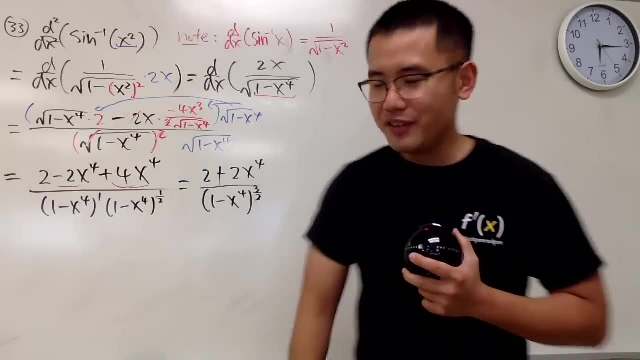 So we get 1 minus x to the fourth power, to the three-half power. But I change that to a square root form, So I will just give you guys the square root answer which is right. here You have the over 2.. 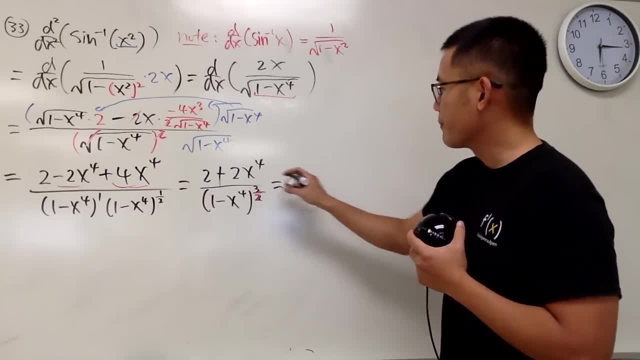 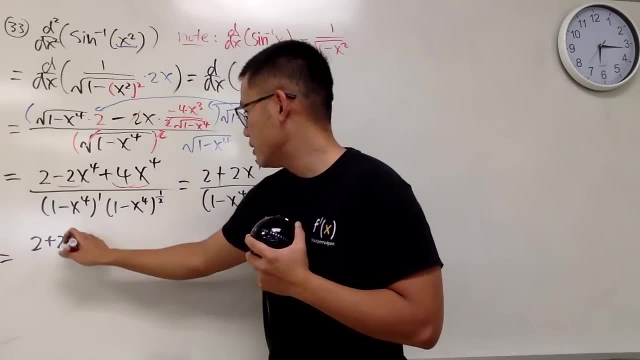 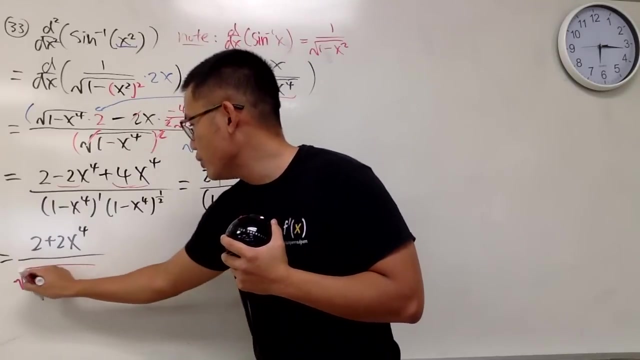 That becomes the radical, the square root. So in the end, In the end, In the end, 2x to the fourth power over This right here will give us the square root And we have 1 minus x to the fourth power. 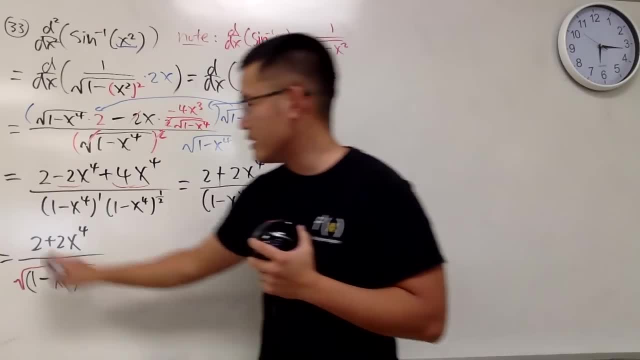 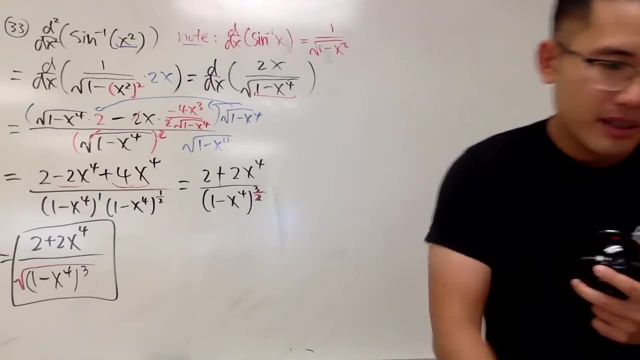 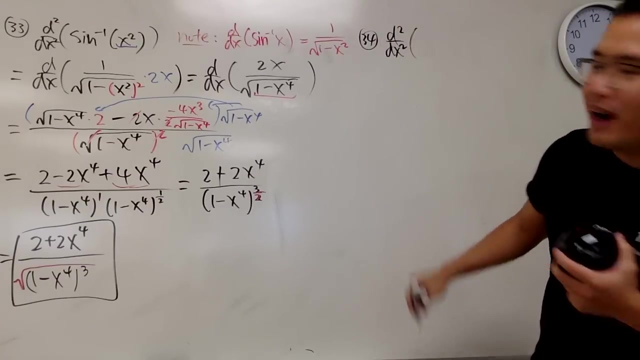 Parentheses that and raise that to the third power. That's the answer. This is the answer. That's it, Number 34. d2, dx2 of 1 over 1 plus cosine x, Like this Quotient rule or not? 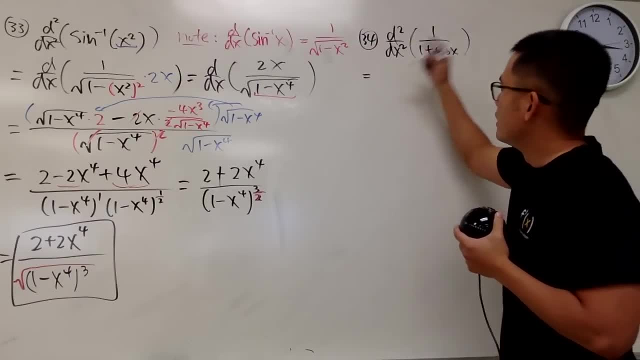 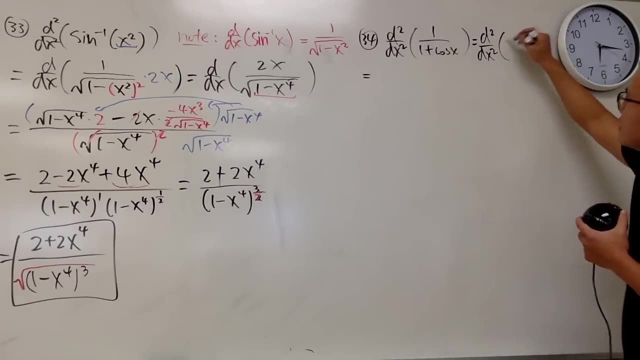 No quotient rule. No quotient rule. Good, Okay, Let's rewrite this as a negative power. first, Let's put it here: d2, dx2.. We can write it as 1 plus cosine x to the negative 1 power, Like this: 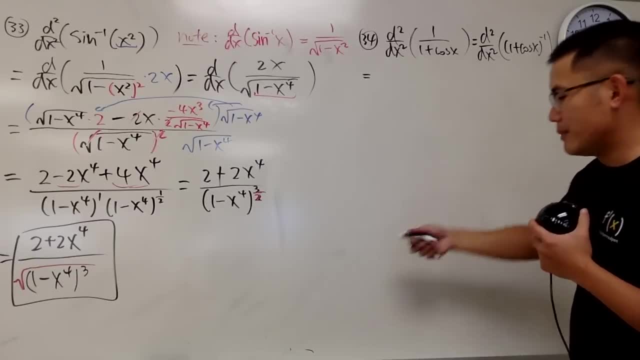 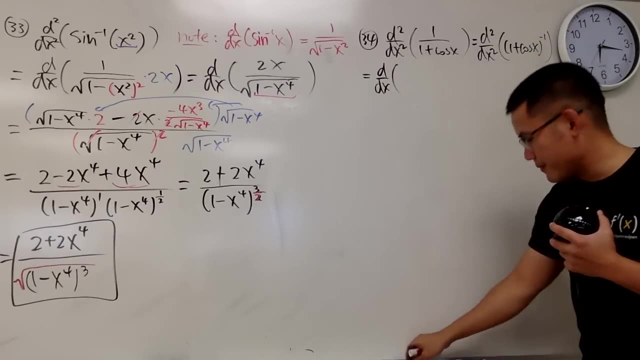 So let's do the first derivative. Oh man, I forgot to do the first derivative in blue over there. I'm sorry, But you know it's okay, I'll do the first derivative in blue right here. The inside here will be the first derivative. 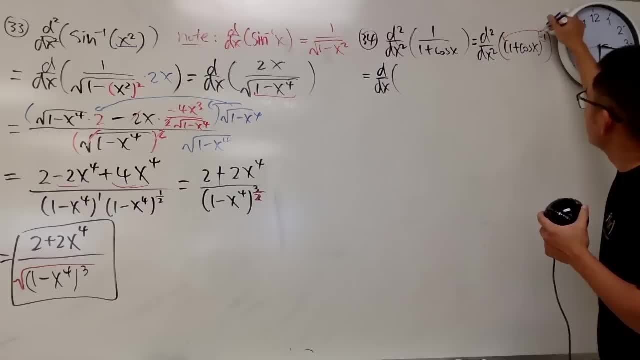 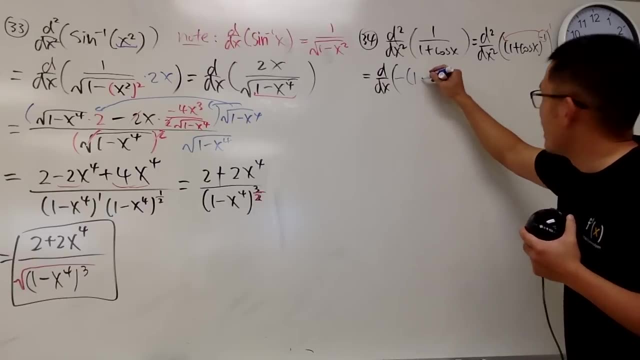 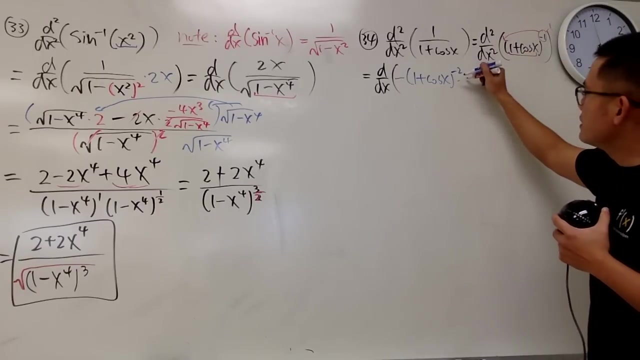 I will first bring the negative 1 to the front and then minus 1.. So we get negative parentheses. The inside states the same, which is 1 plus cosine x, to the negative 2 power, And then we multiply by the derivative inside, which is negative sine x. 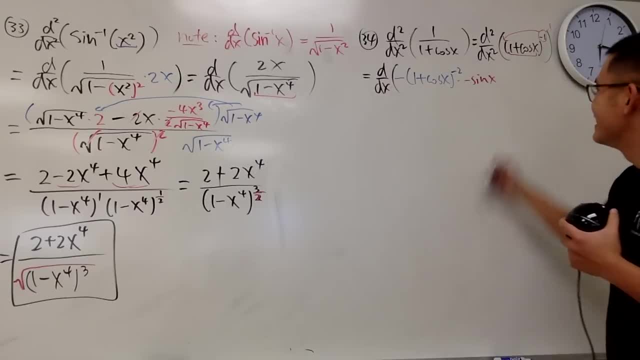 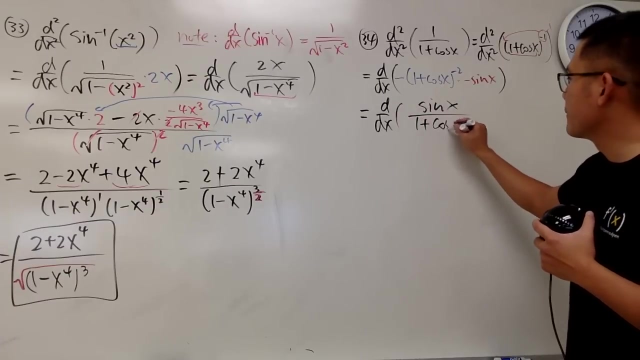 That's the derivative of the inside. Like that, Right, Can we clean things up? Yes, We have d dx Negative. negative becomes positive Positive sine of x Over 1 plus cosine x raised to the second power, Like this: 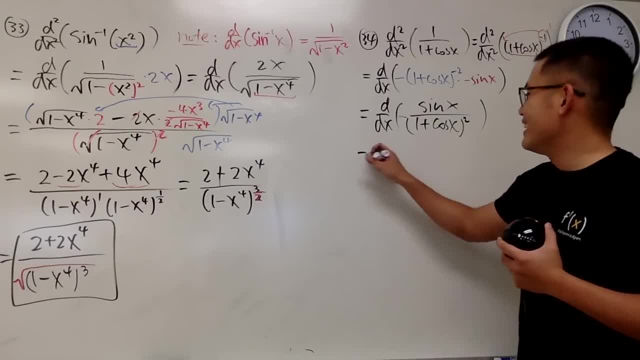 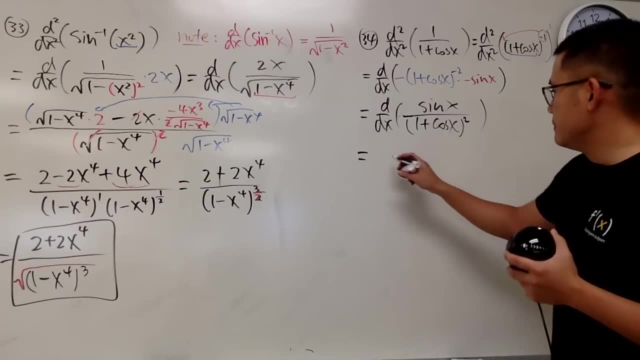 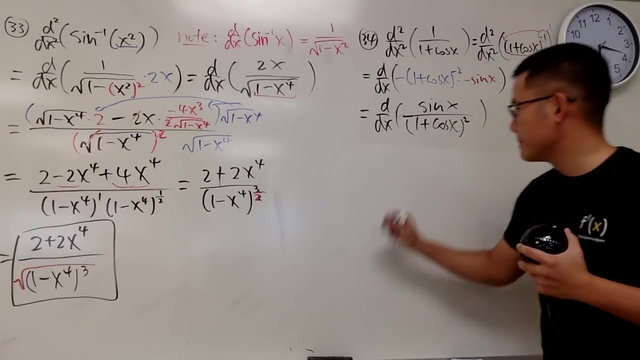 Now we really have to do the quotient rule. You might want to do the product rule right here, but it depends, It depends. So here we go. I will just give myself more space: Square, the denominator. So let me put this down. 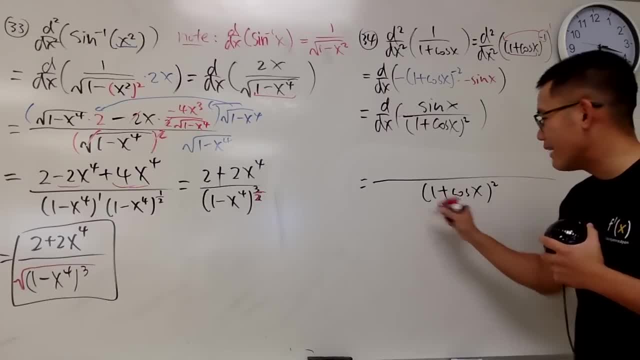 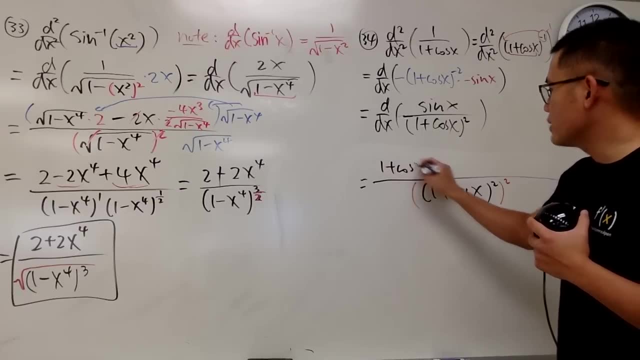 1 plus cosine x squared. But we will have to raise that to the second power. Put down the denominator right here, which is 1 plus cosine x squared. Don't forget, it's a square Times, the derivative of the top. 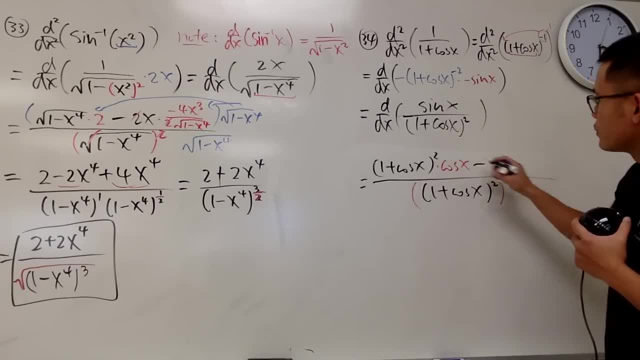 The derivative of sine is cosine, And then minus the top function, which is sine, x Times the derivative of the bottom. This right here Bring the power to the front. So we multiply by 2, parentheses, 1 plus cosine x to the first power. 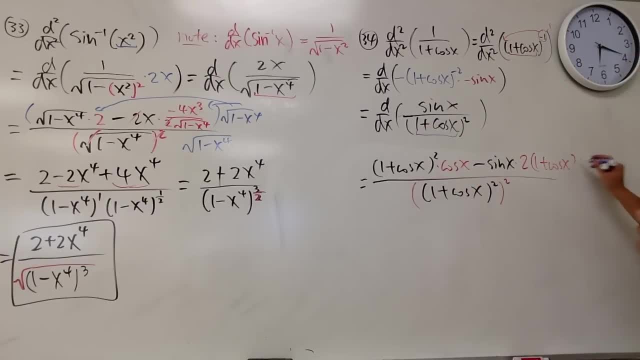 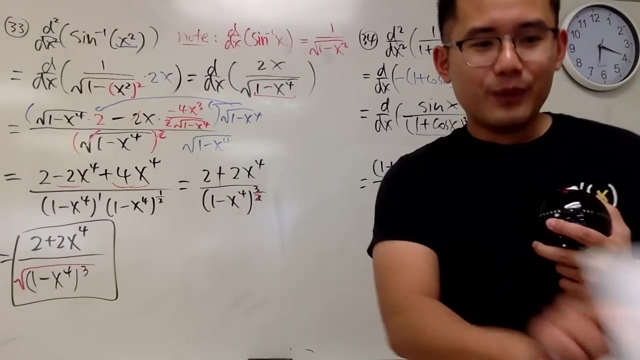 And then multiply by the derivative inside, Which will give us negative sine x, Like that. Oh man, Let's see, Let's see, how did I simplify that? I did simplify the top, So we have to simplify the top. 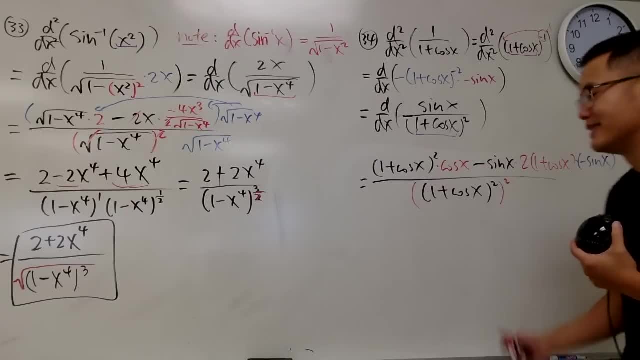 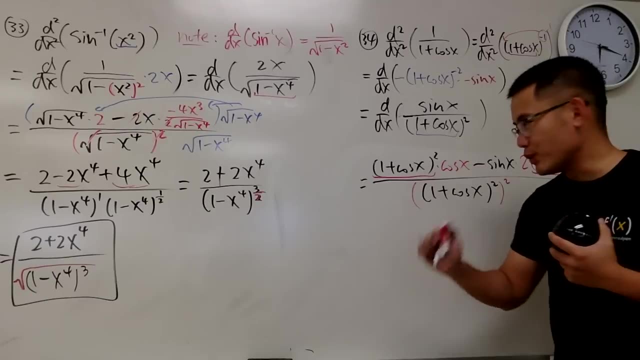 Oh, actually I see how to simplify the top Here. You don't have to really multiply these things out, Because we see this and that can be factored out. So we'll do that first. Can you see the factor tonight? 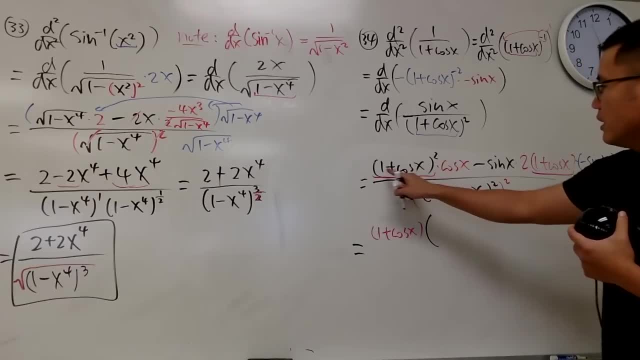 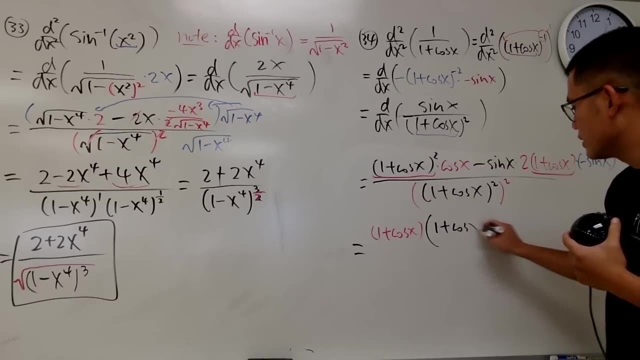 Can you see the factor tonight? Okay, right, here we have the first power. Right, So we have 1 plus cosine x. But don't forget, we still have this cosine x. Good, This is out. Negative times: negative is positive. 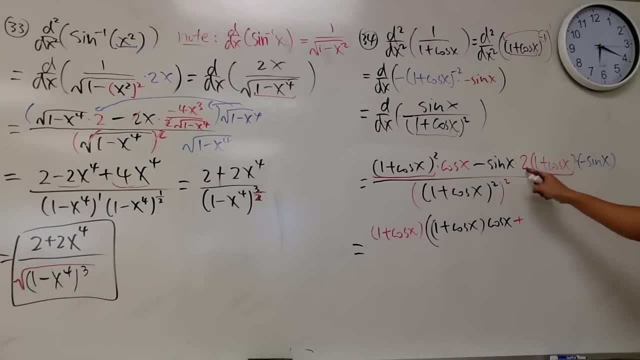 So plus, Just emphasize Plus, You have the 2. And then you have the sine square x, Like that. Yes, Good Over, This guy is 1 plus cosine x to the first power. only Now this, and that can be canceled. 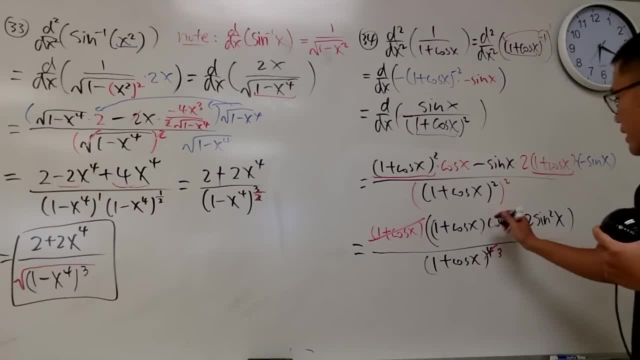 We have 3 more left And let's play And that's pretty much it On the top. we just distribute this And that's cosine square And this is 2 sine square, So we cannot combine anything. 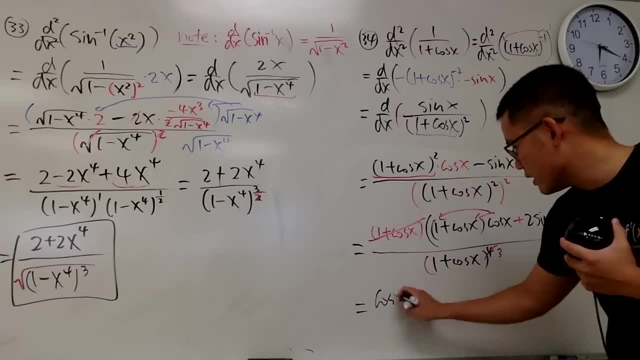 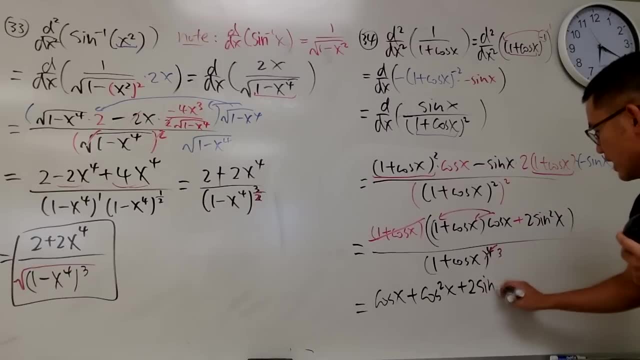 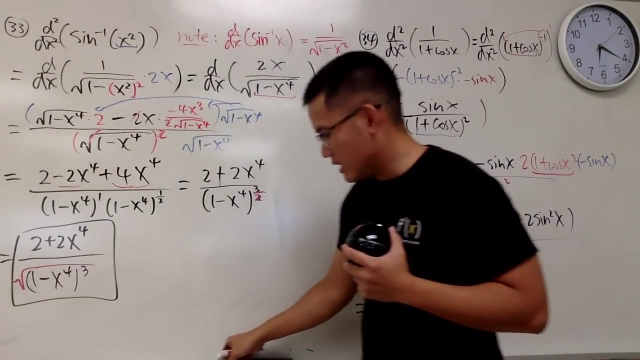 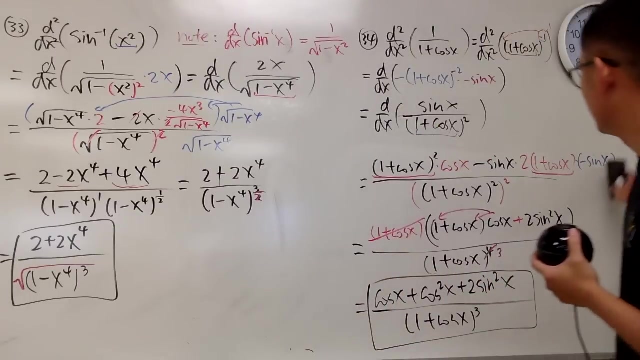 So finally, cosine x plus cosine square x plus 2 sine square x, All over this guy, which is 1 plus cosine x to the third power. And then we are done. This right here is the answer. Answer. Why did I make the question so hard? 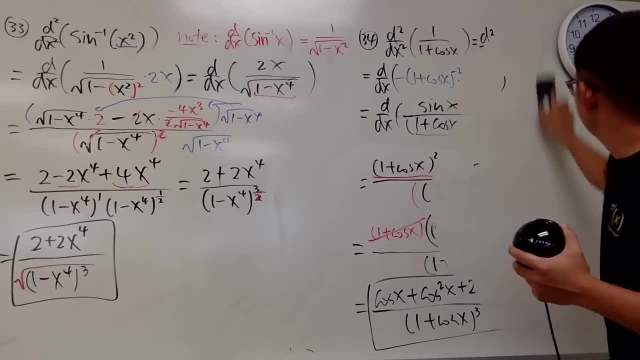 All right, That's 34.. All right, That's 34.. All right, So now we're going to do that, We're going to do that, We're going to do that. So let's do this. 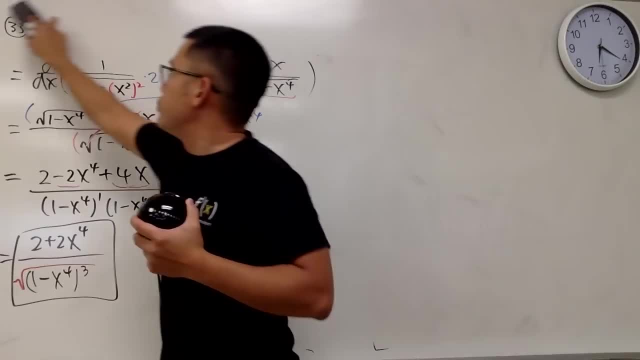 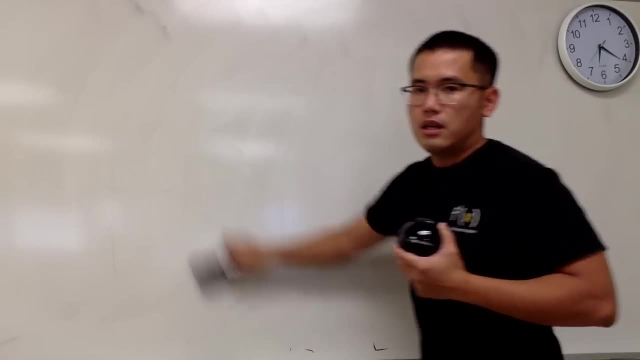 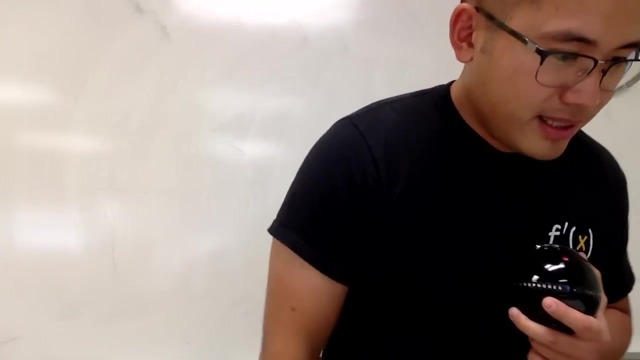 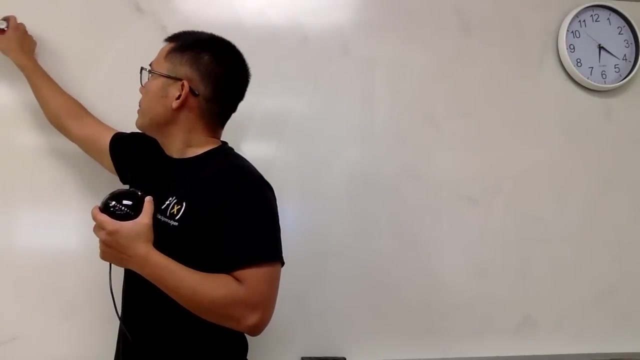 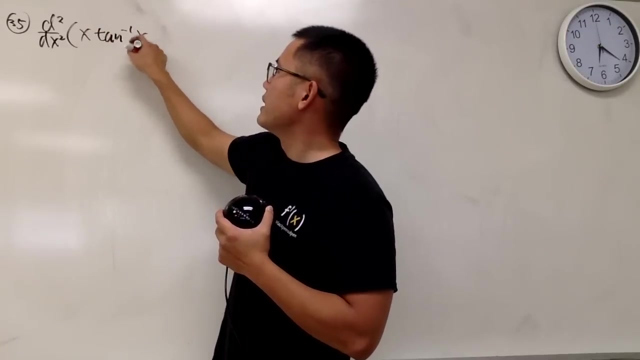 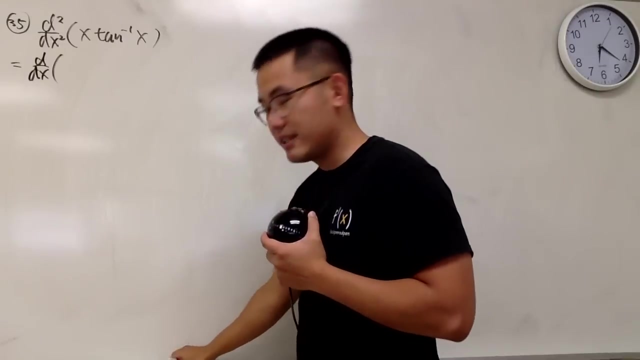 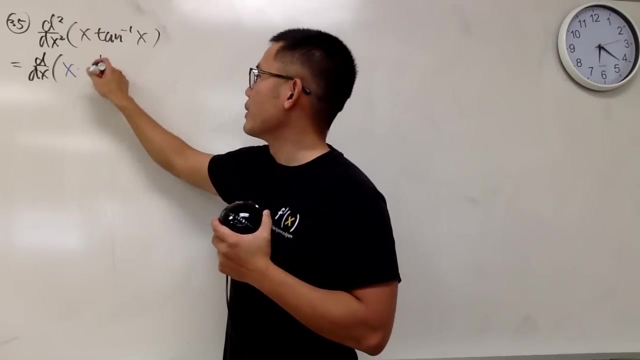 This is the answer. Answer, Answer, Answer, Answer. Answer. question number 35: second derivative: X times the inverse tangent of X. go ahead and do it. d, dx. put this down in blue though: first function, which is X times the derivative, the second, that will give us 1 over 1 plus X square, and we add the. 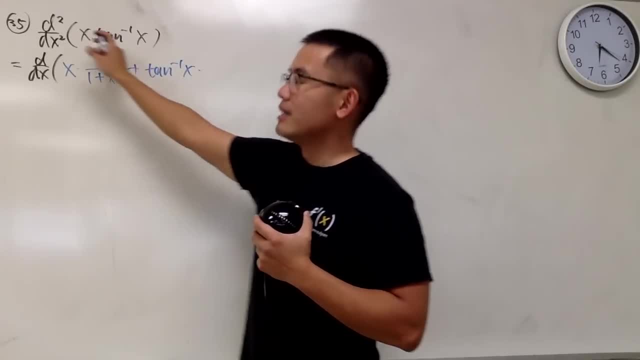 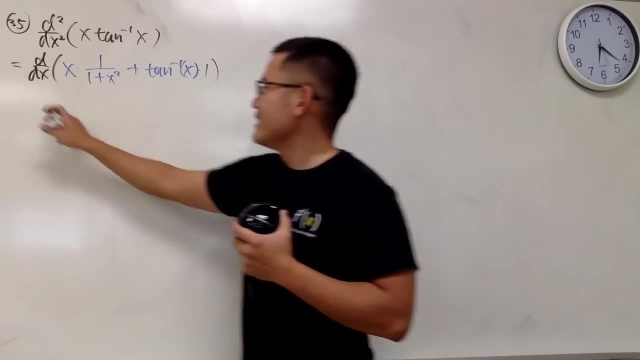 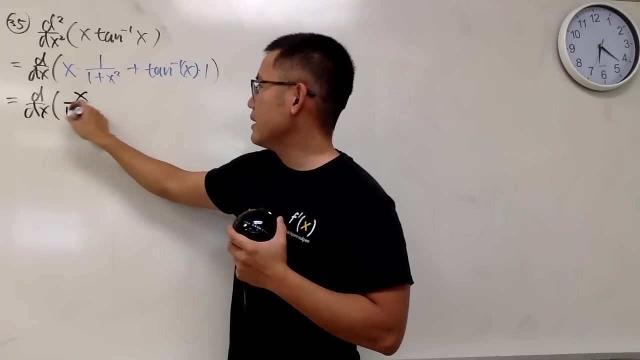 second function, which is inverse, tangent times the derivative of the first, which is just a 1. so that's what we have, nothing too special. all right now we have to differentiate this right here. well, we can just put the X on the top, but we haven't took that. we haven't taken that. 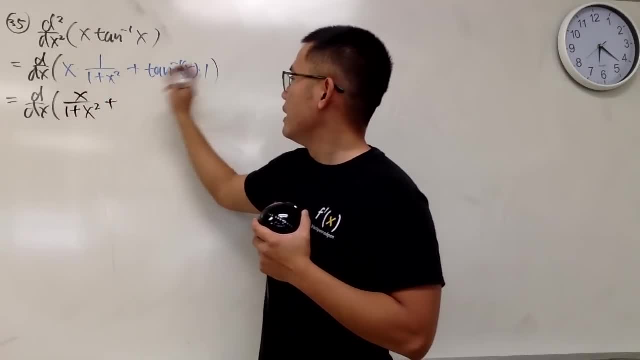 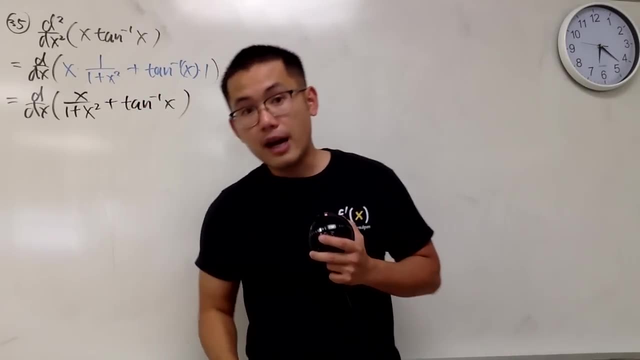 already for the for another time. so we'll just put the eggs on the top and then this is just the inverse tangent of X. we'll just clean up. so this is the first derivative. now just do it for the first one. let's use the quotient rule. so 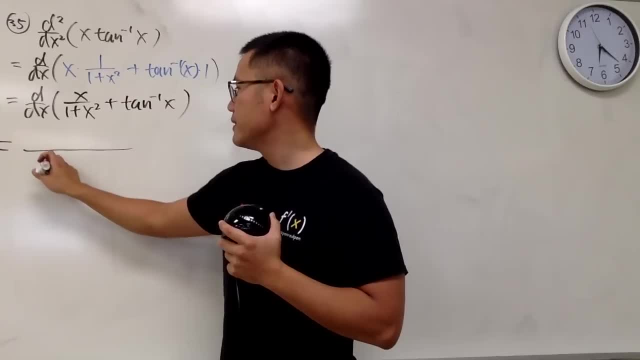 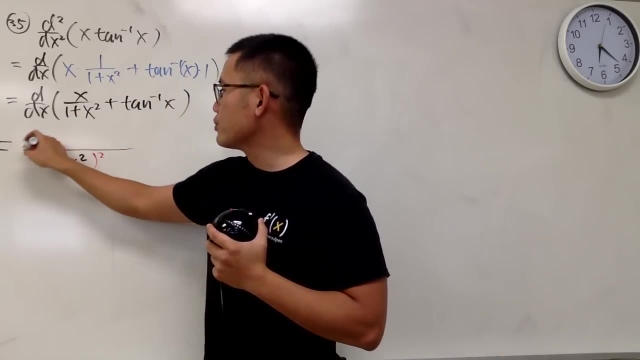 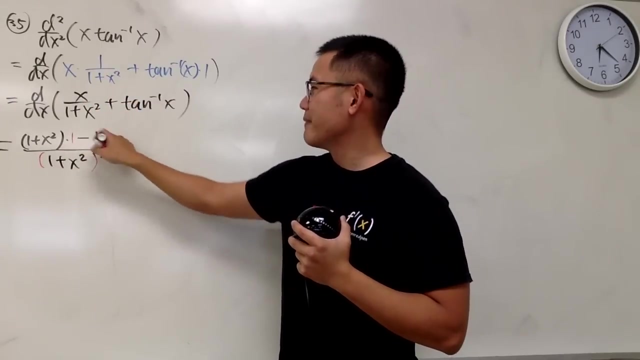 square the bottom, so we will have 1 plus X square and we square that then. Then the bottom function goes to the top, 1 plus x squared times the derivative of the top, and then minus the top function, which is x times the derivative of the bottom. 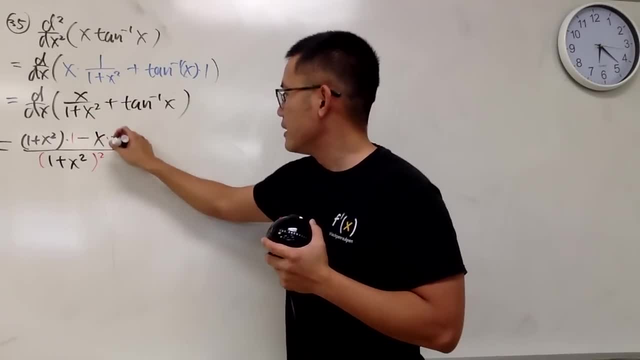 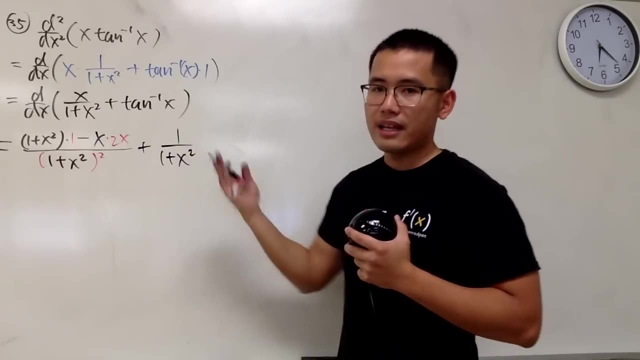 which is going to give us 2x, And then we add the derivative of inverse tangent, which is 1 over 1 plus x, squared like this. Now we are going to do some like little engineering, that kind of thing. 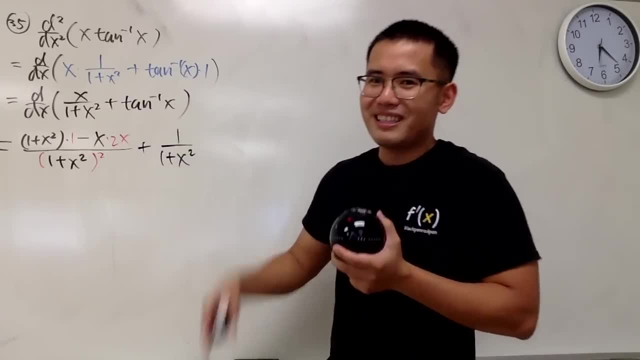 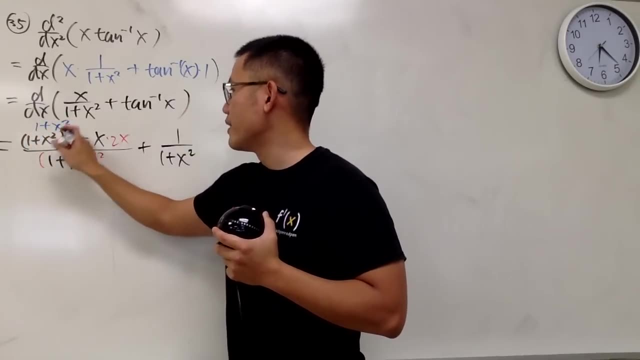 Not so much, though. it's just like: look at this part, look at that part, come right like this: Okay, I see that This right here is just 1 plus x squared times 1, just that minus this times, that is just 2x squared. that's good. 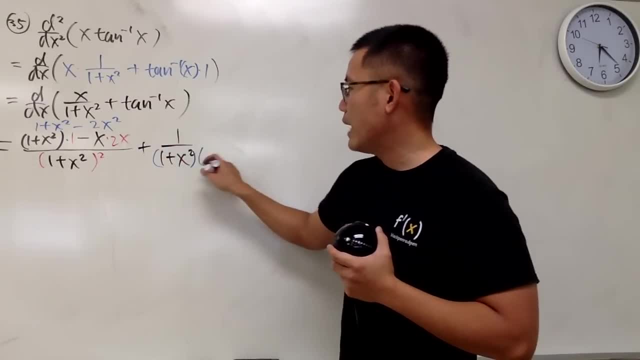 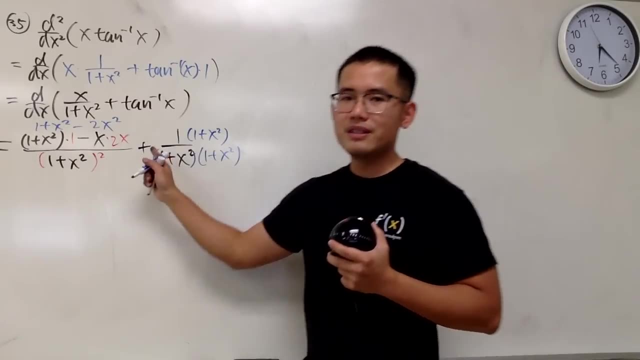 But perhaps let's get some common denominator. So I will multiply this by 1 plus x squared, and also 1 plus x squared. Well, thankfully this is just plus, so we can just add everybody on the top. So this is just u plus 1 times. this is just 1.. 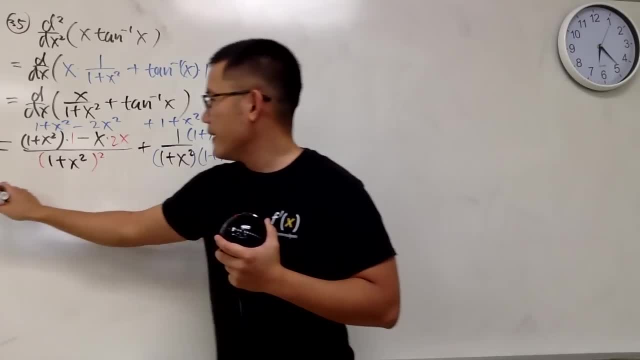 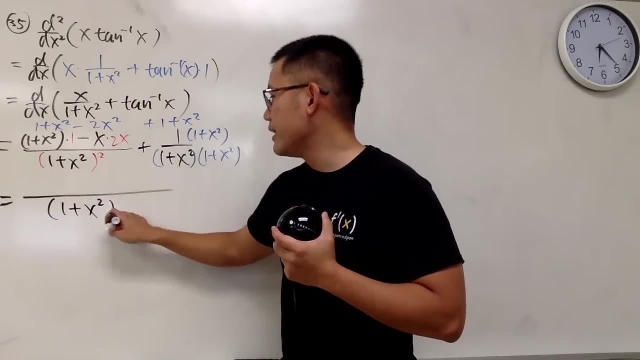 1, just all that. So that's pretty nice, Let's see, let's see. let's see what we get at the end: Parentheses: 1 plus x squared, and then square that for the bottom. Hmm, 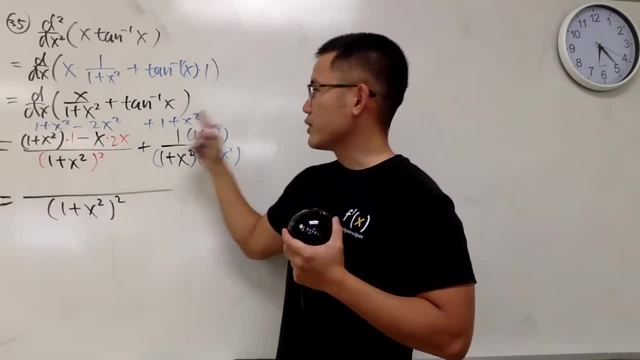 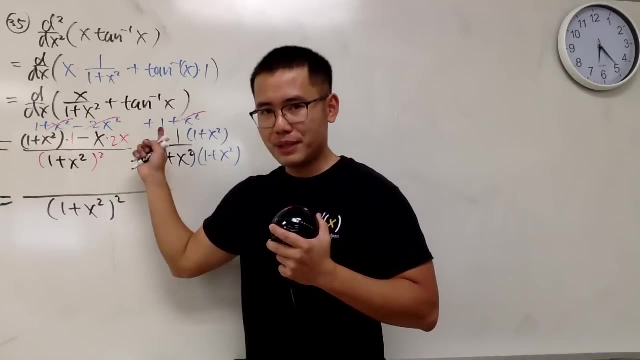 Check this out: x squared, x squared, 2x squared and then minus 2x squared. Oh my God, Cancel this out. And on the top, we just have to do 1 plus 1.. I think it's 2.. 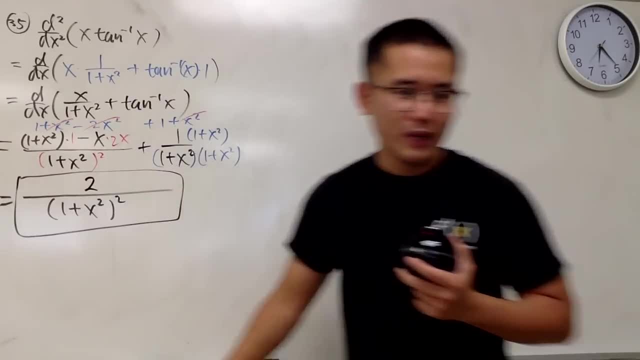 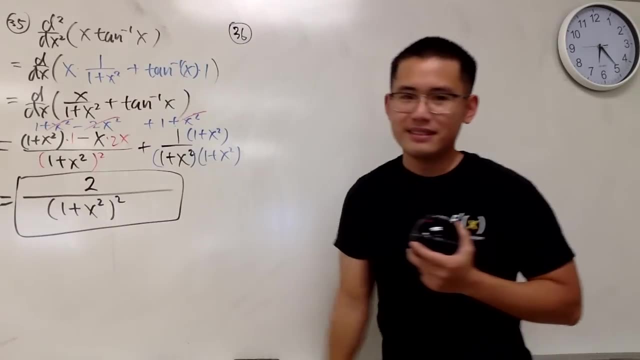 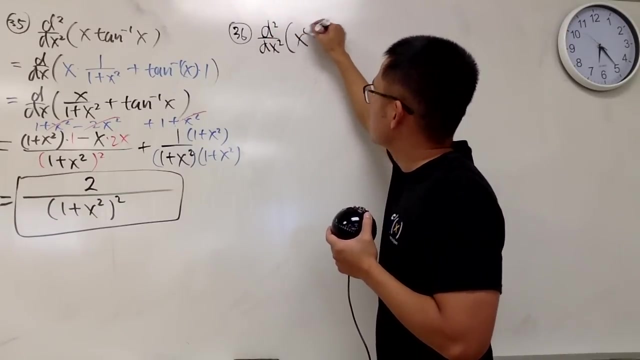 Yeah, So that's the answer, I believe. Let me know if I get this right or not. So, oh my God, that simplifies pretty nicely. huh, Number 36.. Number 36. We have second derivative of x to the fourth power natural log of x. 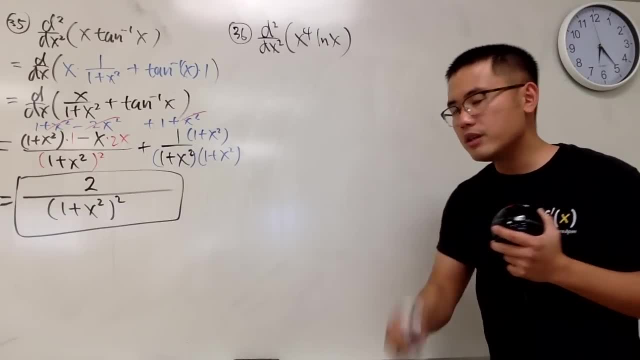 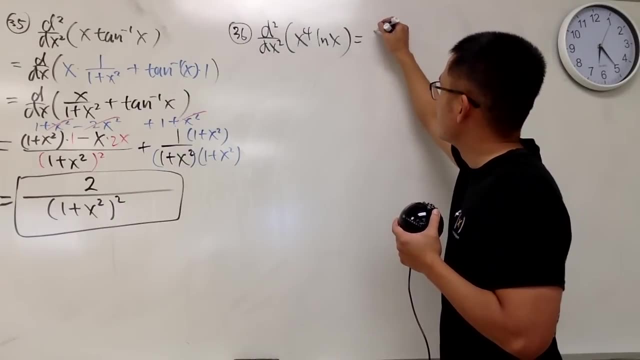 Just like this. Here we go. Okay, For the first one we have to use. Here's the product rule, right? So perhaps it's already done here. D dx- Parentheses- product rule in action. Keep the first function. 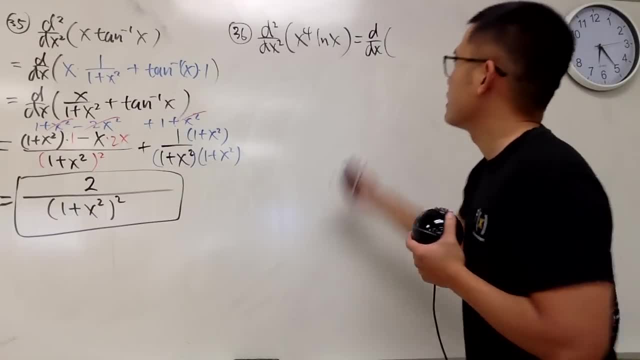 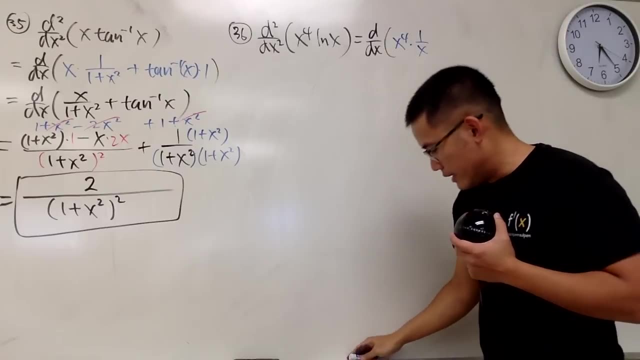 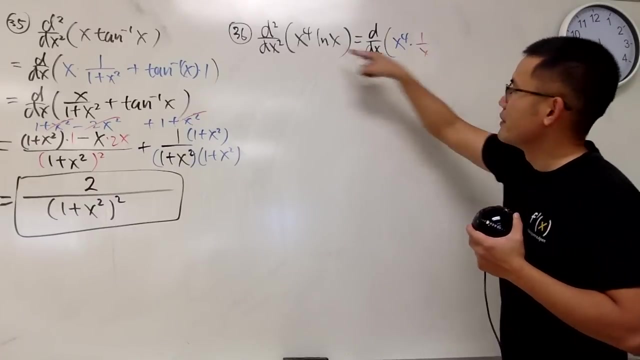 Let me see what's the next one. Yeah, that's just the first. function x4 times the derivative of the second, which is 1 over x And um Derivative of the second. I'm not editing this video, Steve. 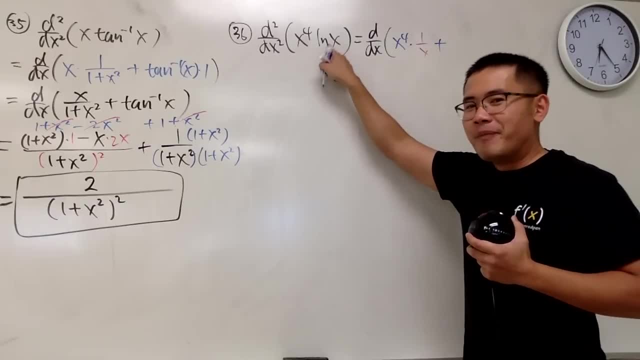 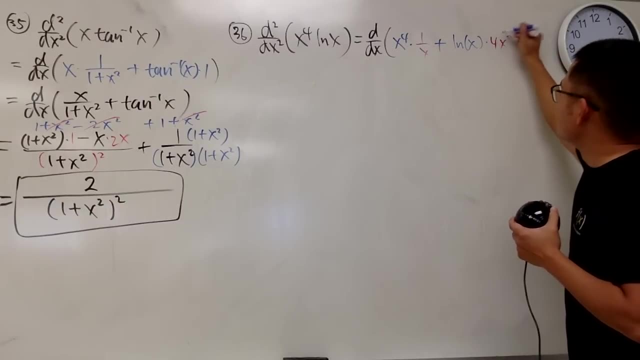 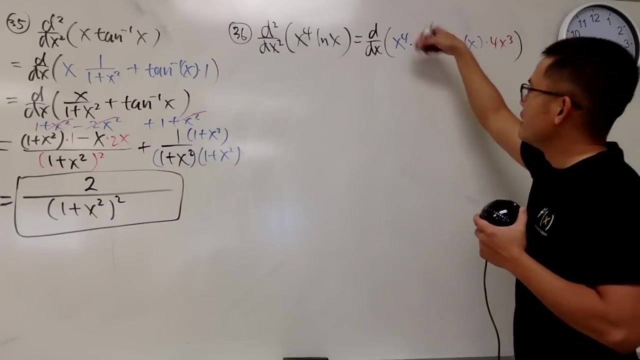 Okay, Pl-pl-plus um natural log of x times the derivative of the first, which is 4x to the third power, like this: x4 times the derivative of the second. Okay, Good, Now of course, this right here is just 3x to the third power, right. 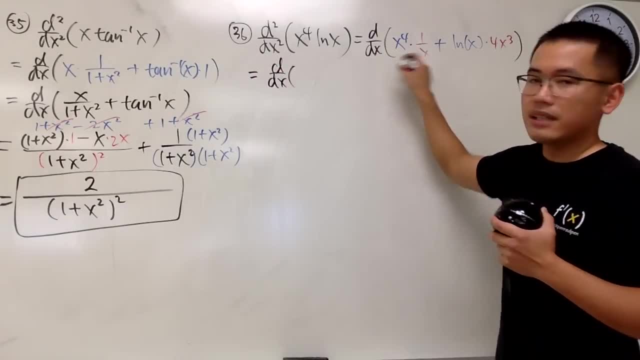 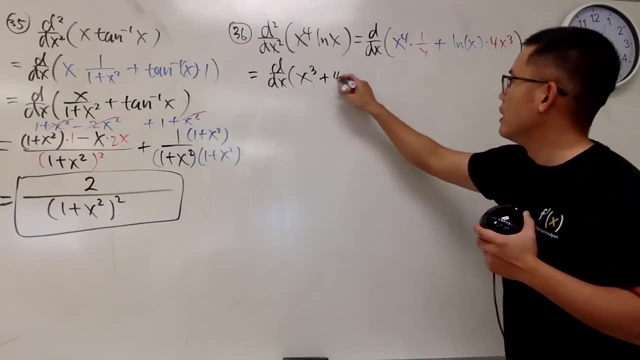 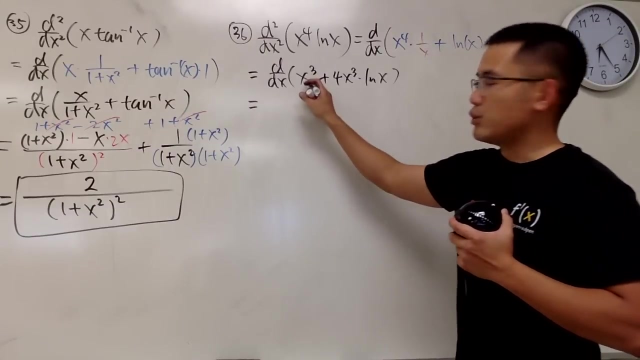 So, all in all we are looking at to differentiate this guy together will be simple of i: d to x to the third power, x to the third power, x to the third power, my god plus 4x cubed times. natural log of x, Derivative again. Why not Derivative this? 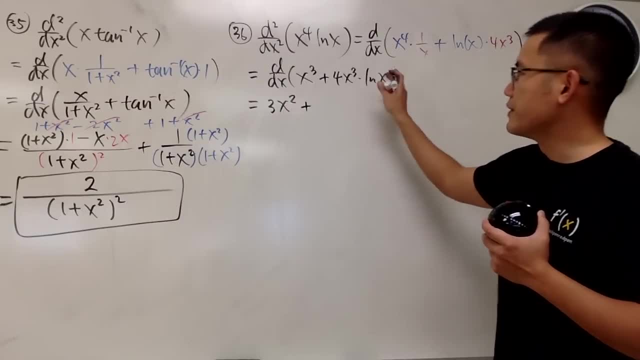 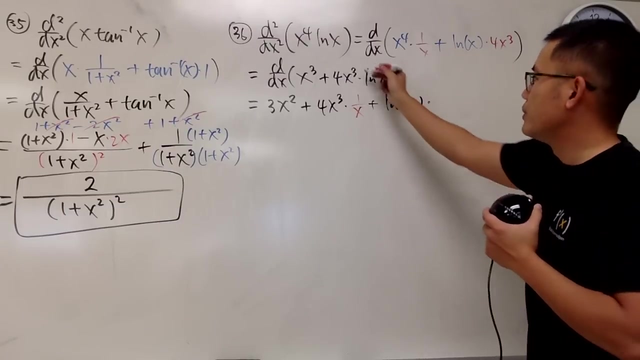 guy is 3x squared and we add the derivative of this guy. This is the first function. 4x to the third power times the derivative of this right 1 over x Plus the second function, which is natural log of x times the derivative of this guy, which is 12x squared, like this: 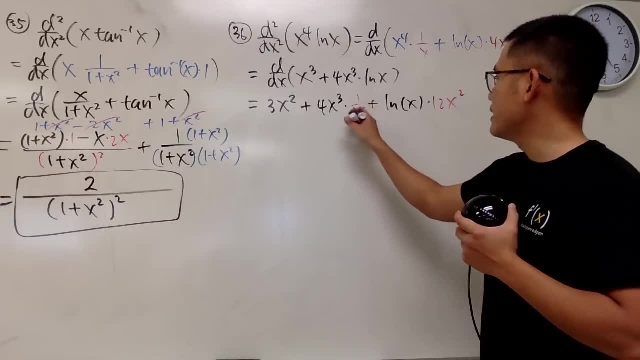 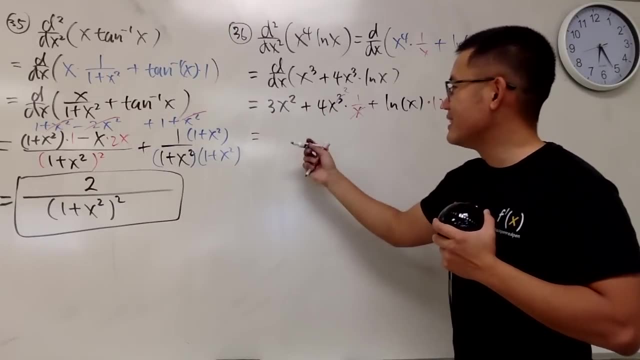 Okay, of course, this part again. we can nicely simplify it, So it's just 2.. 3 plus 4 is 7, and x squared right. So this is 7x squared. Put the 12x squared first, so 12x. 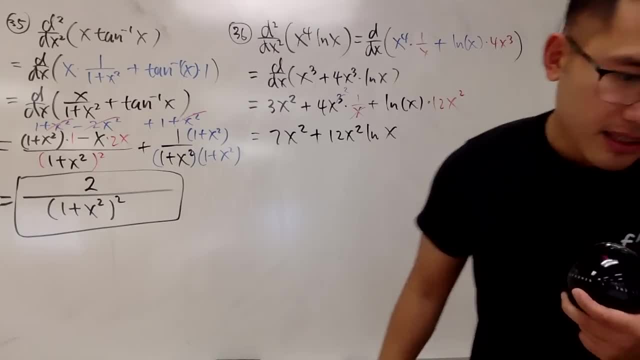 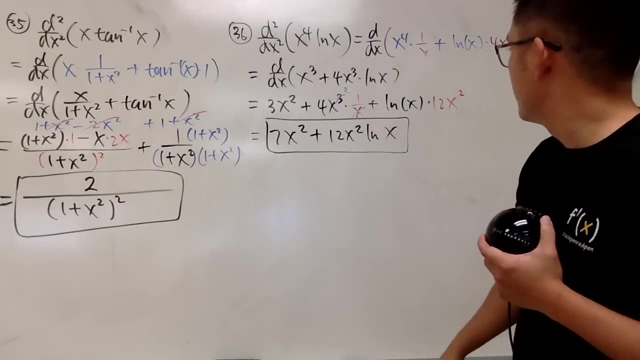 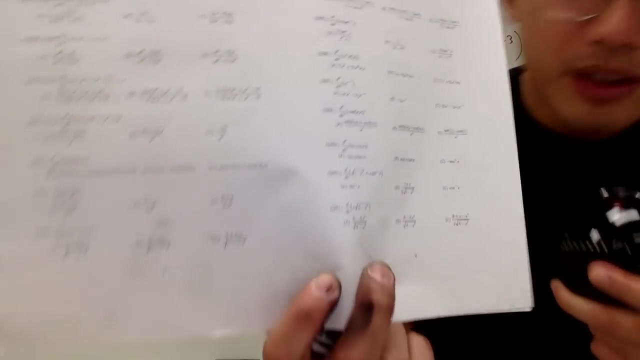 squared, and then we have the natural log of x, And that's it, Nothing else. Yes, Nothing else, Nothing else. Yeah, Be really careful, though, if you need to get my equation number 36.. There's no typo, but I just make a small change for the answer. 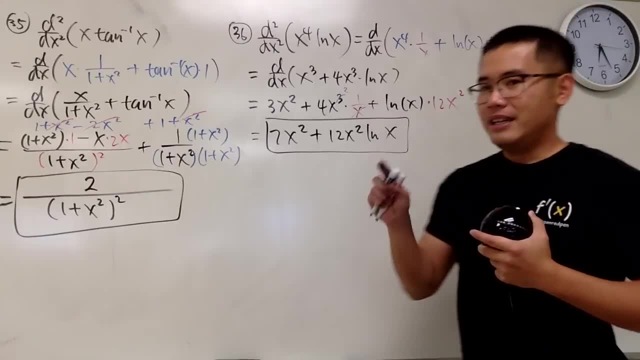 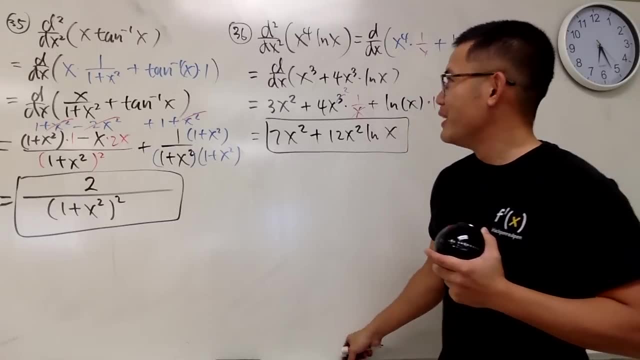 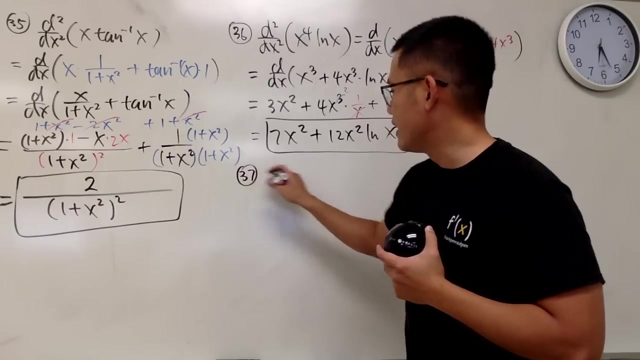 key. So, haha, If you are taking AP test, let me know You know how the AP test, the multiple choice questions, are. They are really tricky. because they are really tricky. Look at this, Because the answer choices are very, very similar. Okay, 37. d2, dx2- e raised. 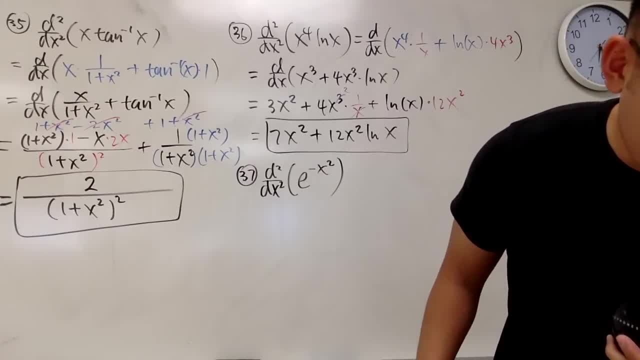 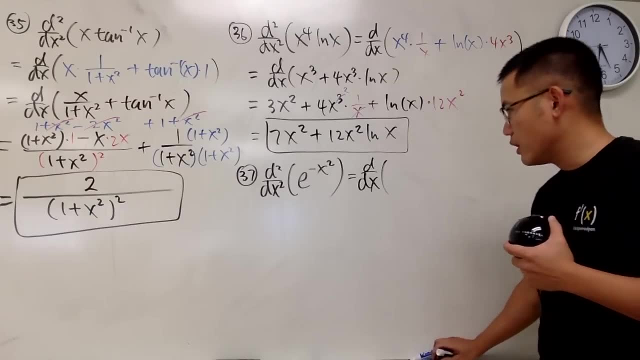 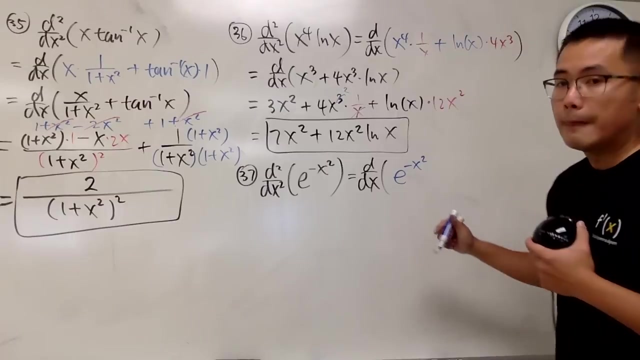 to the negative x squared power, One of my favorite functions. Here we go. We have to differentiate the first derivative And for the first derivative we have this right here stays, which is just e to the negative x squared. But Chengdu says we have to multiply by the derivative inside The derivative of that. 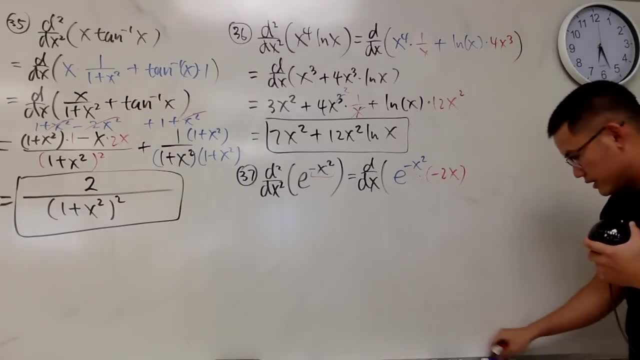 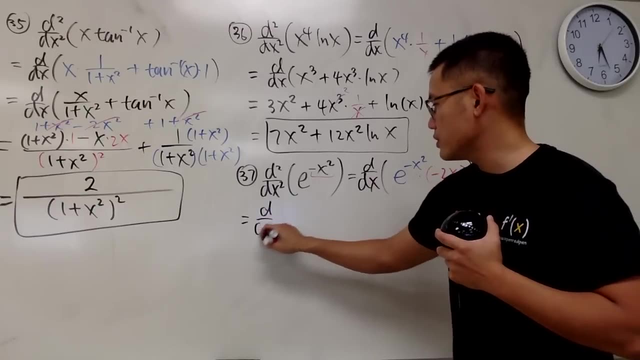 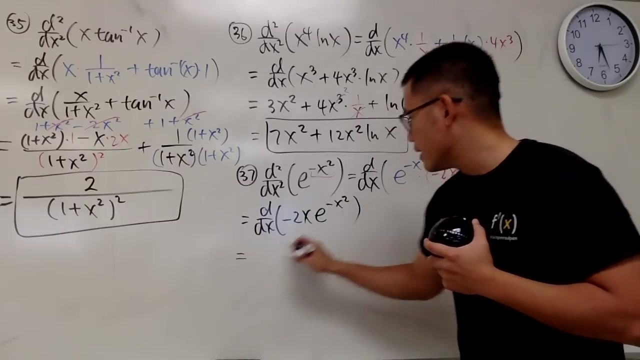 is negative 2x, Like this, Right, So own all. we just have to differentiate. Let me just write it down again: We just have to differentiate negative 2x times e to the negative x squared. So let's do it. First function: we keep it. Times the derivative of the second. The derivative. 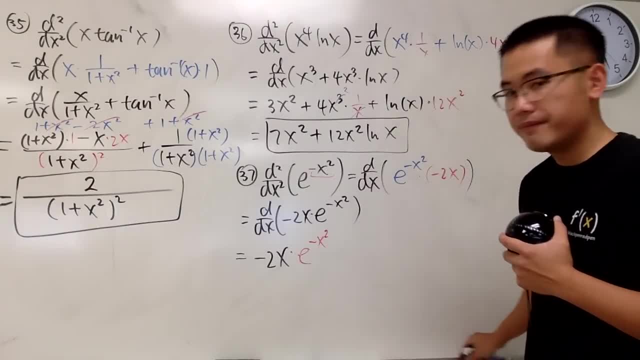 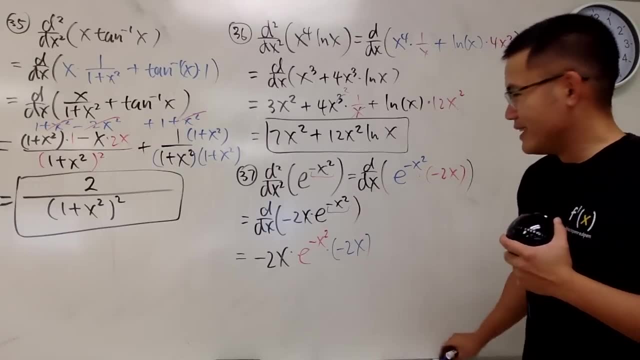 of this is e to the negative x, squared square, and we multiply by the derivative of that because of the Chengdu. So the derivative of that is negative 2x. I don't even know if I'm saying derivative correctly, not by heart. 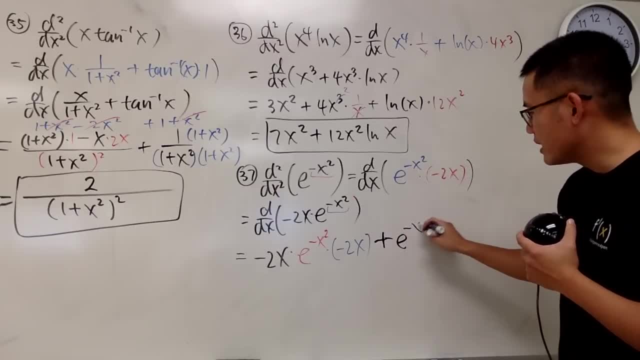 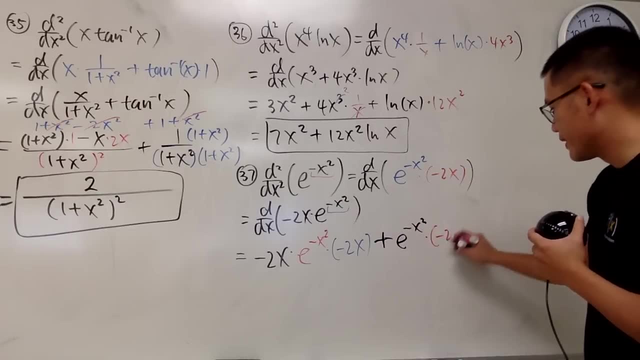 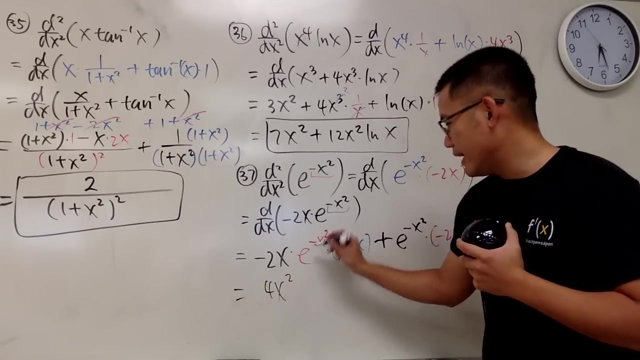 Anyway, we add the second function, which is e to the negative x square times the derivative of the first, which is negative 2.. Alright, finally we clean things up. This and that give us 4x square, and e to the negative x square, and this is minus 2,. 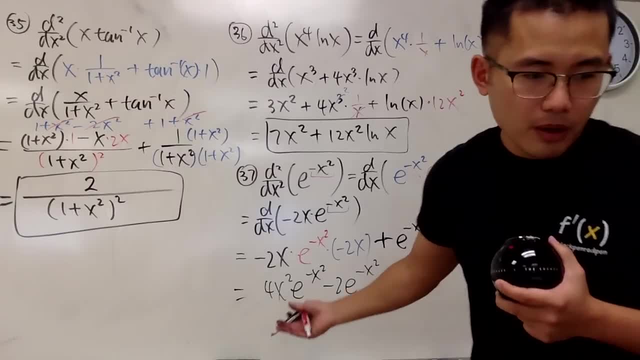 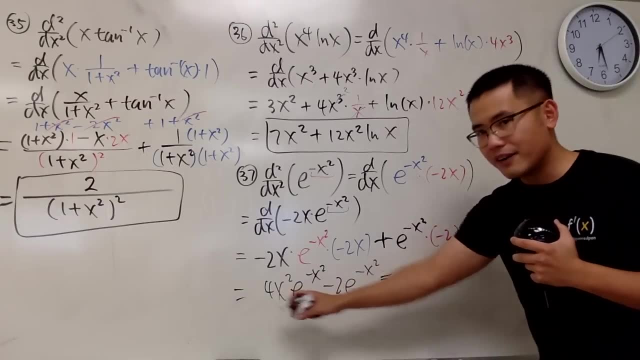 e to the negative x square, And some people may want me to factor out- actually I did factor that myself too, so I will factor it out, because this right here can be factored in. so we will have parentheses: 4x square minus 2, and e to the negative x square. 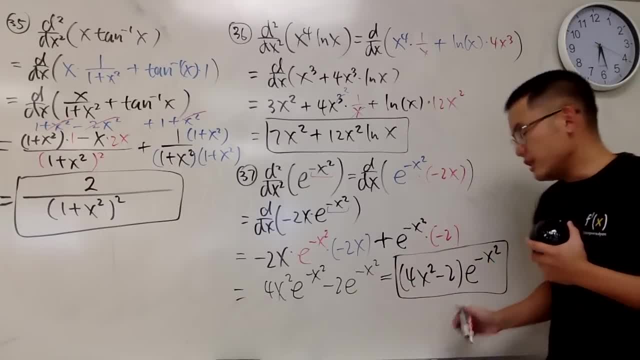 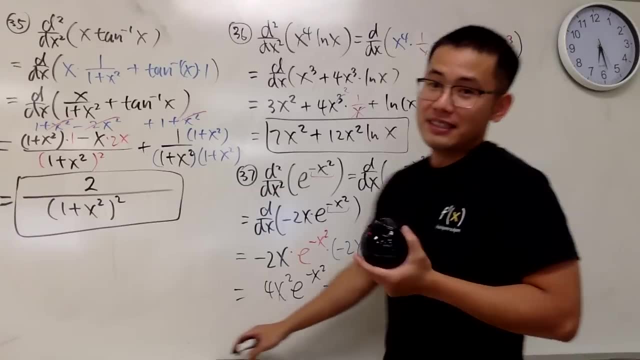 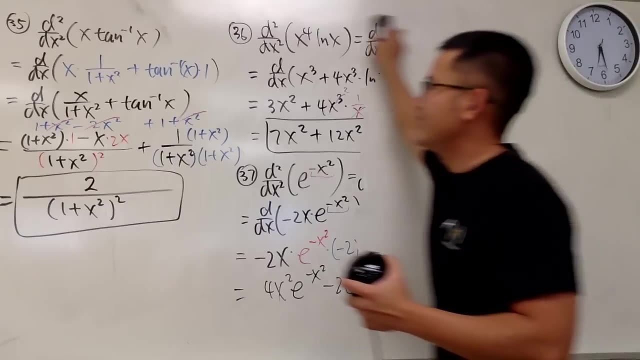 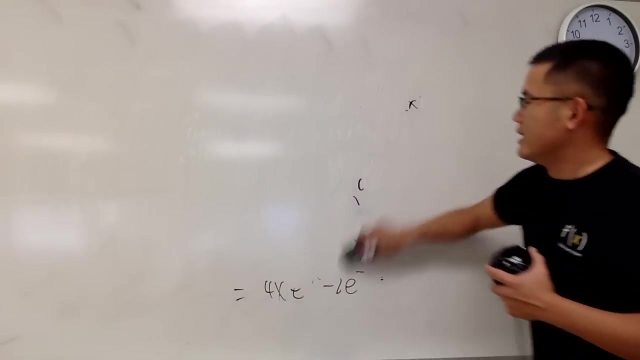 Like this. This is preferred if you need to set this equal to 0, and find the critical numbers. So, oh man, I cannot say this is it. but this is it for number 37.. Man, this is Whew. 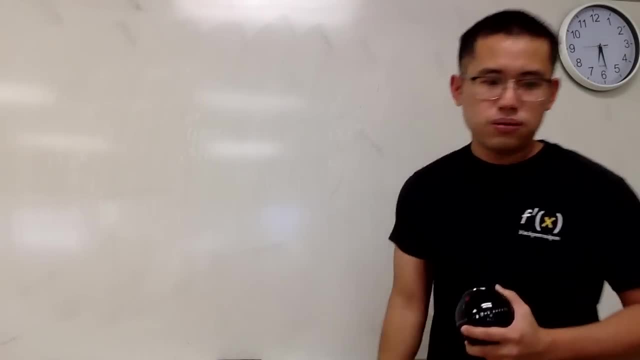 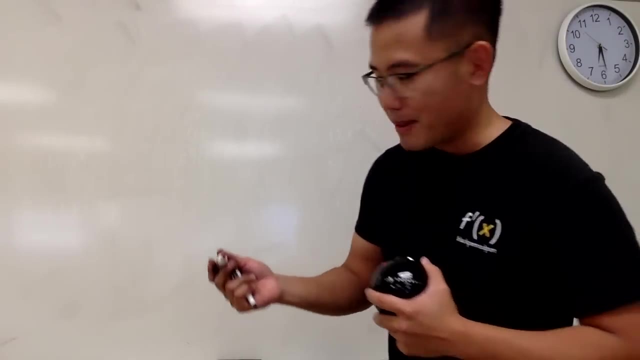 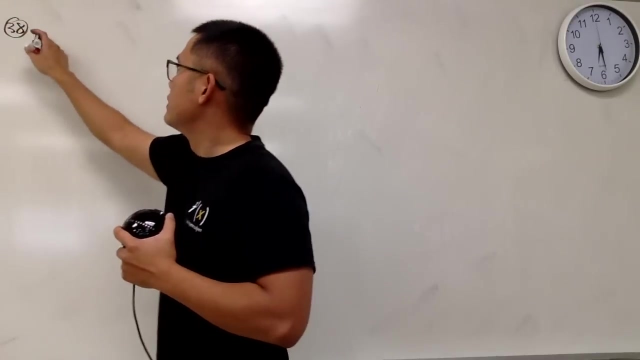 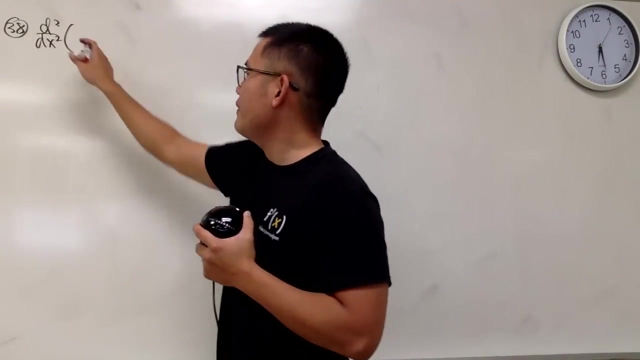 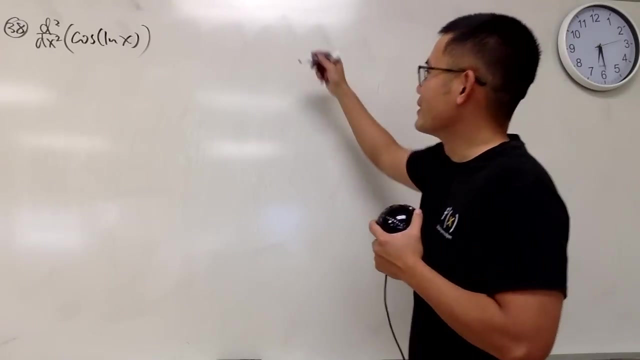 Okay, Okay. Okay, number 38 and 39, I will do them side by side. So here is number 38.. So d2, dx2.. For the first one, we have cosine of natural log of x And in fact you can do the integral of this. you can also do the integral of that, not. 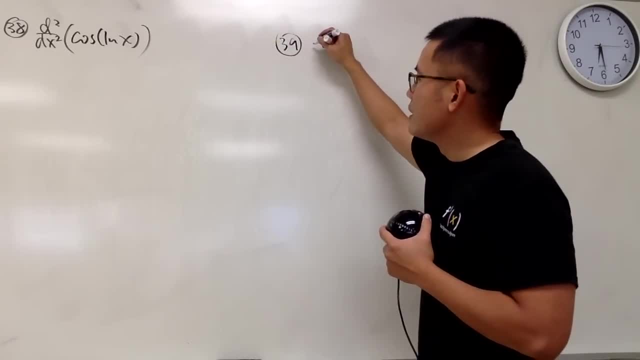 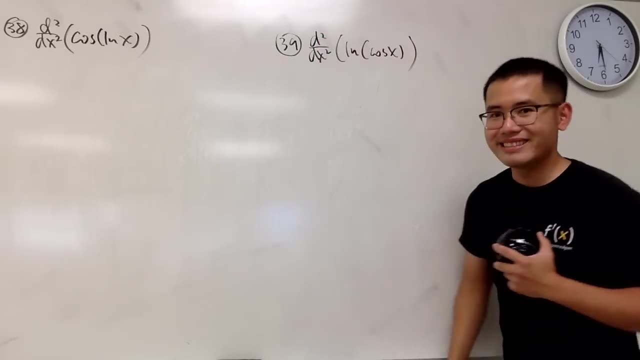 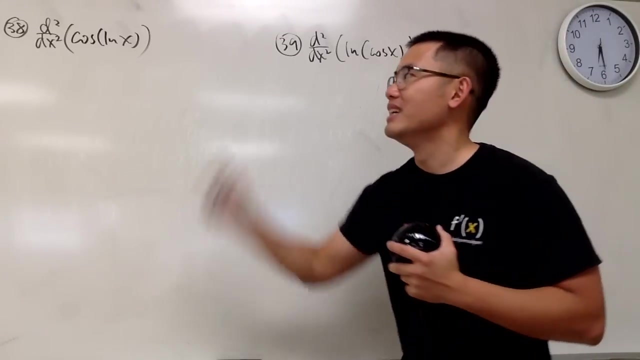 just the derivative, and then I will do the 39 on the side. This is d2 over dx2, natural log of cosine of x, Like this: Okay, we have two derivative equations on the spot. They look similar, but of course they are also very different. 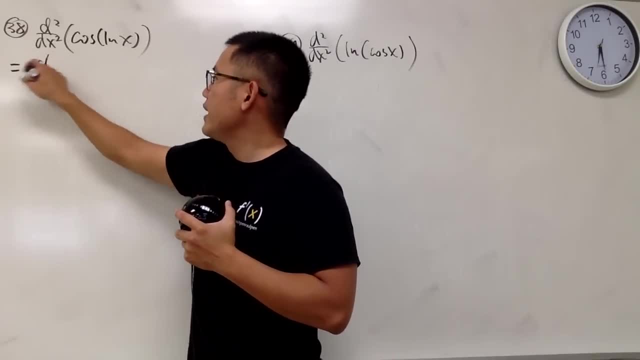 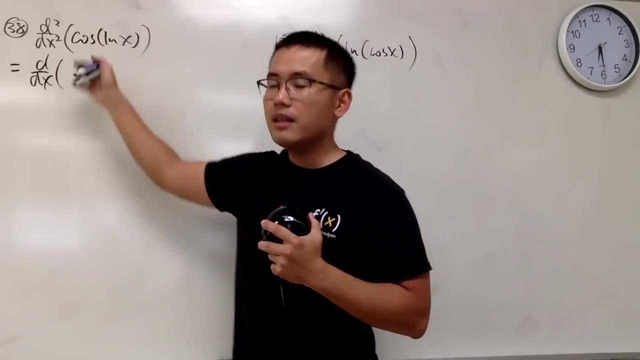 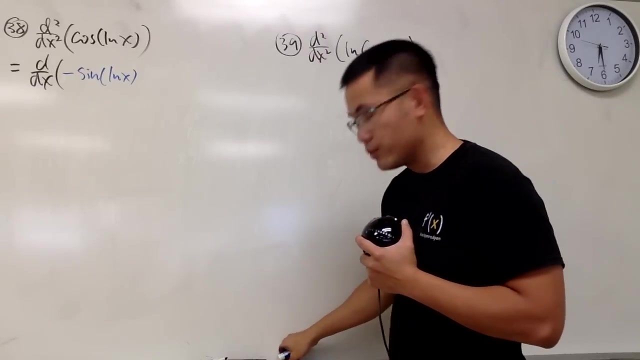 Let's look at this one first. Okay, differentiating. well, we have to get the first derivative right here, Derivative of cosine, of something. first we get negative sine and the input stays the same. And then what We have to do? the channel, the derivative of the inside, which is 1 over x. 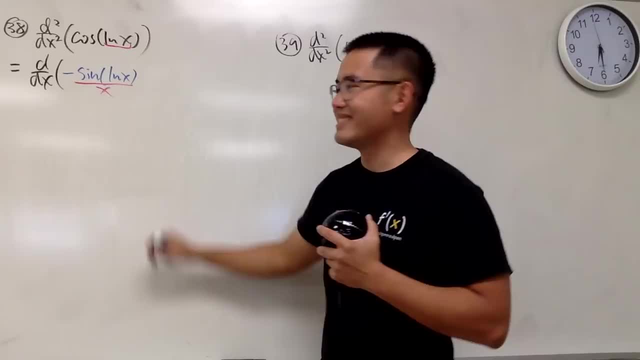 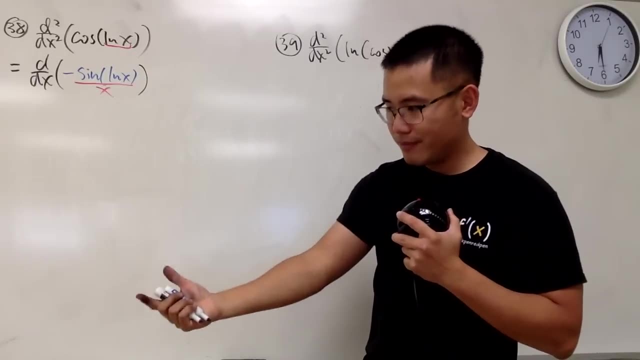 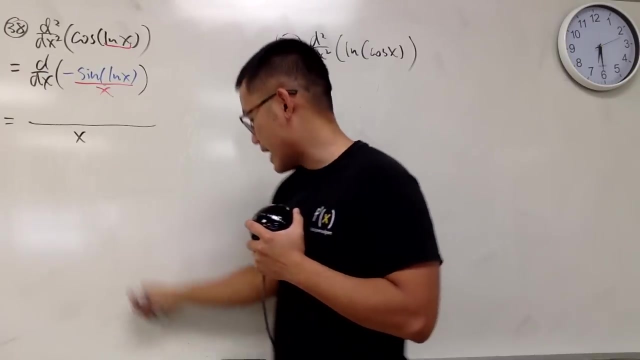 So I'll put on the over x like this: yeah, Over x. Now differentiate that guy. Caused rule. Okay, here we go, Square the bottom, which is x, and we square that X, and then we square that. 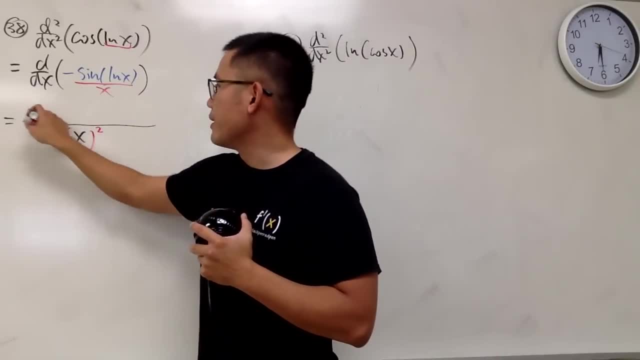 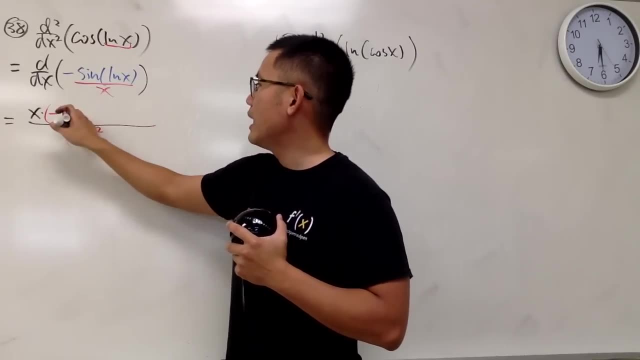 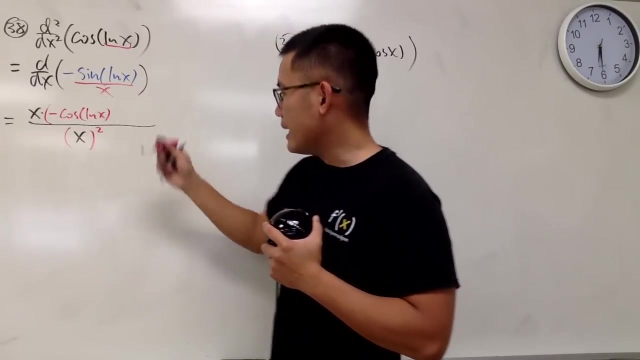 Okay, And I will put on the bottom function right here: times the derivative of the top. This is negative, so I will just keep that as negative. and then we have the derivative of sine. Do that, you get cosine and the input stays the same again. but we have to multiply by. 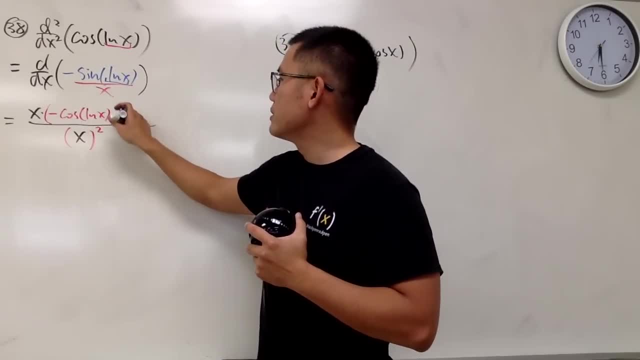 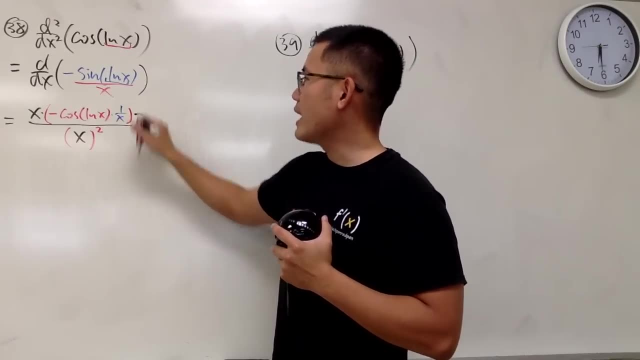 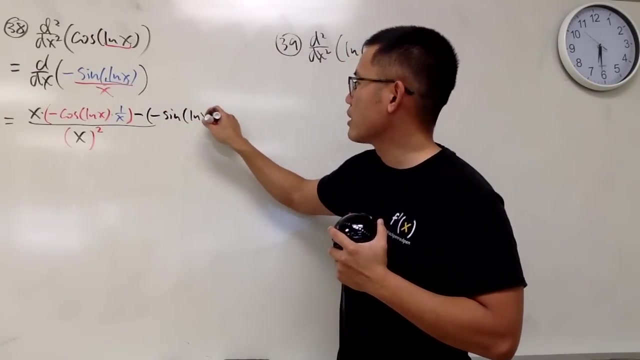 the derivative of the inside right here, which is going to give us 1 over x. So that's it for the first part. Then we subtract the top function And the top function has negative. so you write down negative sine of natural log of. 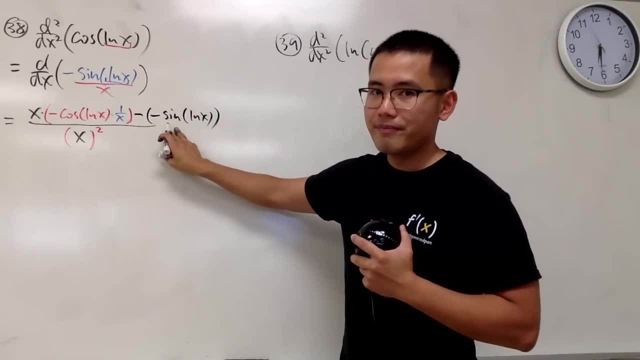 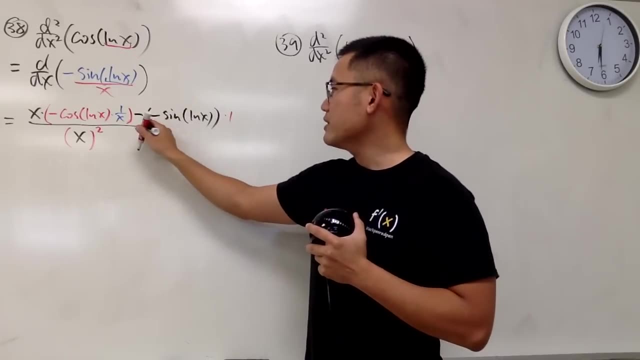 x. Okay, This is the top function, And then we multiply by the derivative of the bottom, and the derivative of x is just 1.. So that's what we have, And check this out: X, And then this is over: x. 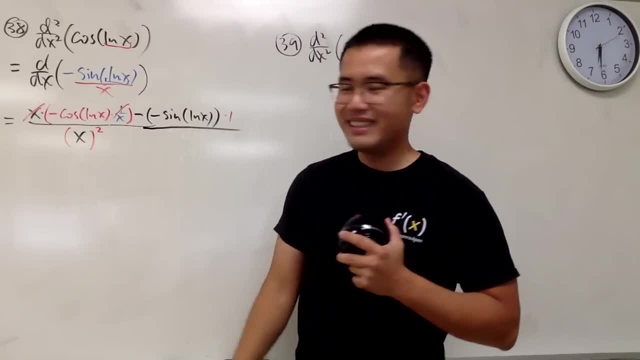 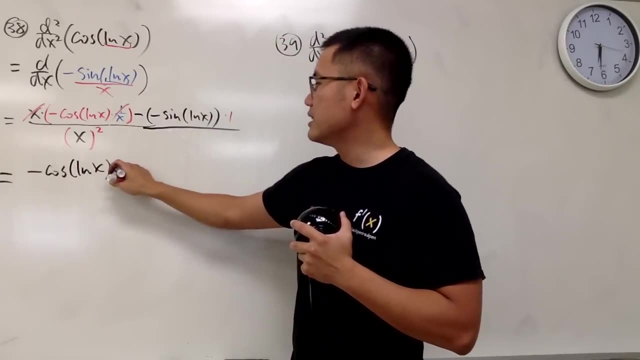 So this and that cancel out very nicely And you will see that this is negative cosine of natural log of x. So this is the top function, And then we multiply by the derivative of the bottom. So that's the second part. So this is the top function. 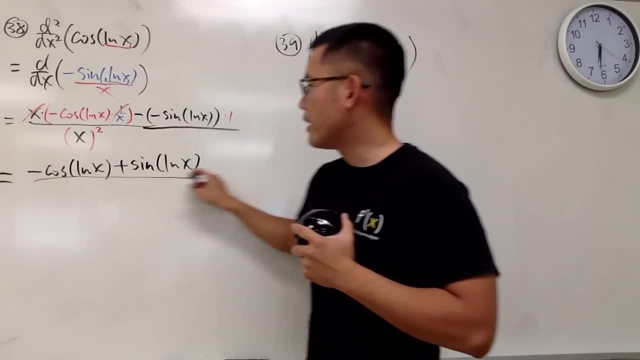 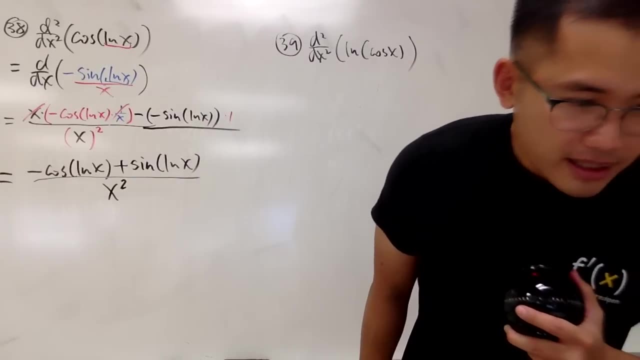 So we have negative sine of natural log of x and negative times. negative is positive sine of natural log of x, All over x squared, All over x squared. And on the answer key I put down the sine first, because I put down the sine over there. 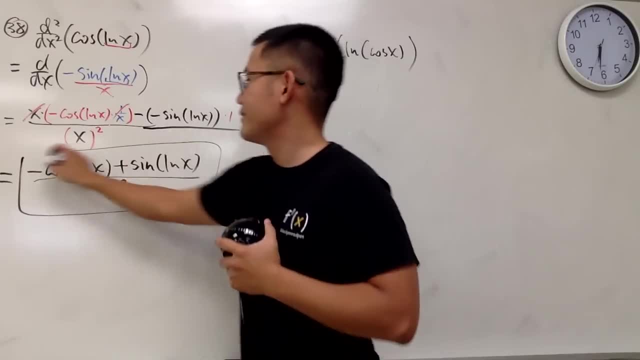 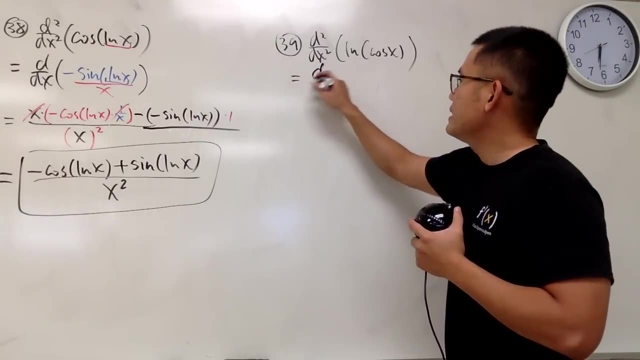 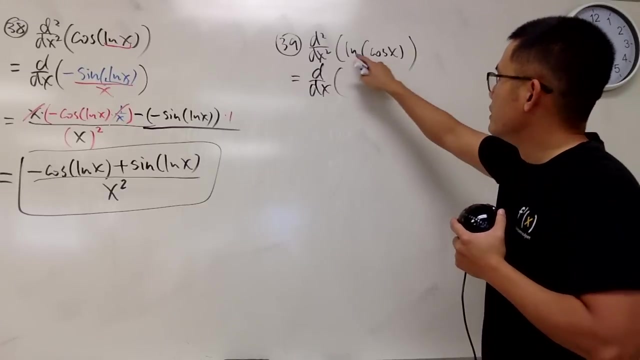 but I will leave that to you guys. Okay, so just do that Now for this one, here we go. Let's get the first derivative right here Inside blue. This time, though, you have to remember, when you differentiate natural log, you first do 1 over. 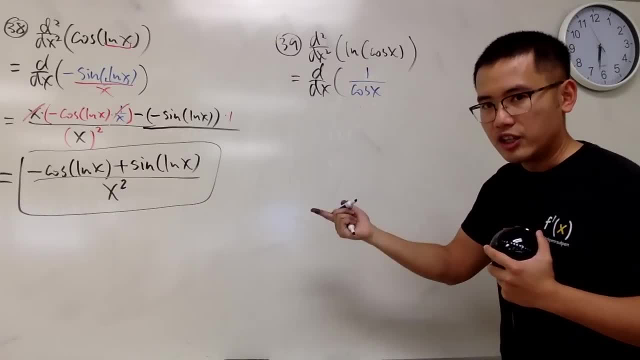 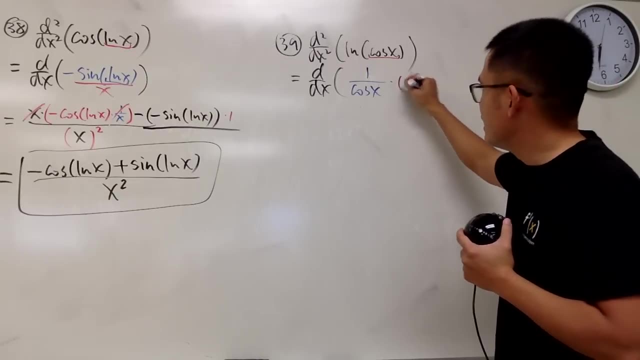 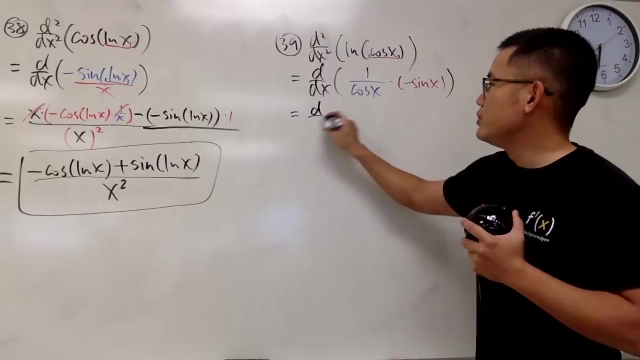 whatever this is, which is cosine x, And then the channel says: multiply by the derivative of the inside Derivative of cosine x is what? Yes, negative sine x Like this. Good, So check this out. This is going to be just to take the derivative. 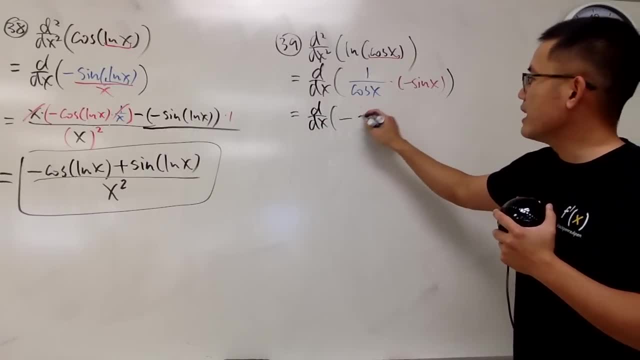 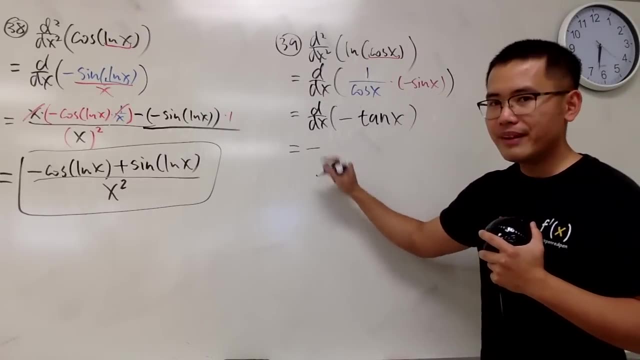 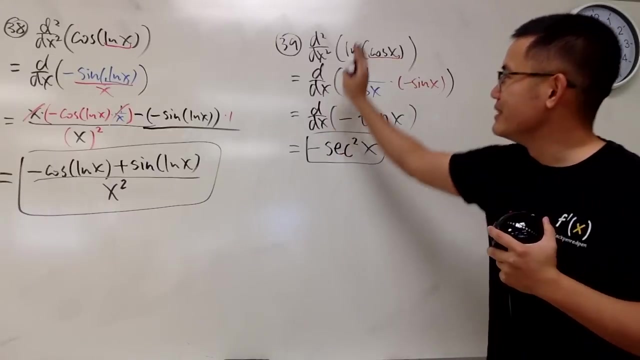 of negative sine x over cosine x. This right here is nicely equal to tangent x. Well, the derivative of negative tangent x is negative. You have secant squared x. That's it. Which one did you guys like more? You see, you just switched the order of the input and the. 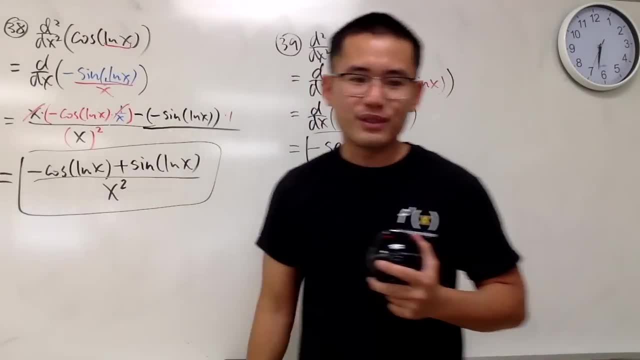 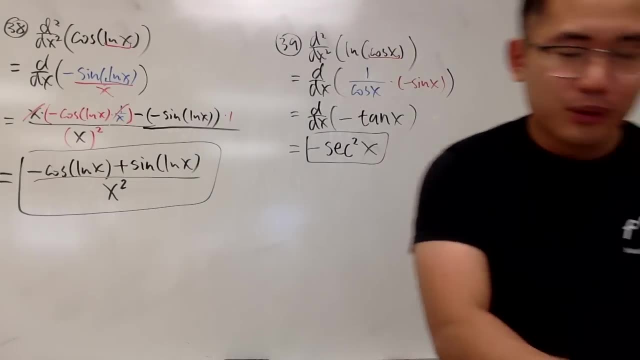 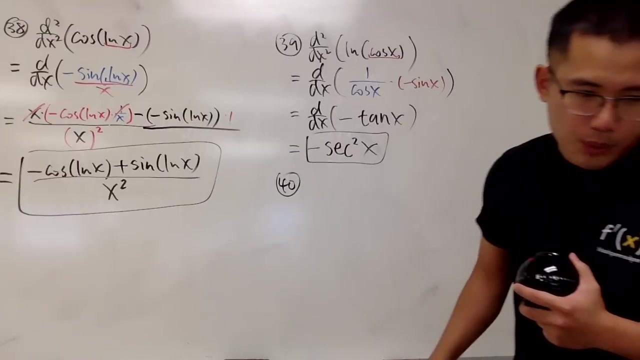 input, and well, the inner function and the outer function. That's it. Oh my god, that was number 16.. Number 39. I don't have to do like two derivative for one question again, Man good. Number 40. Here we go. 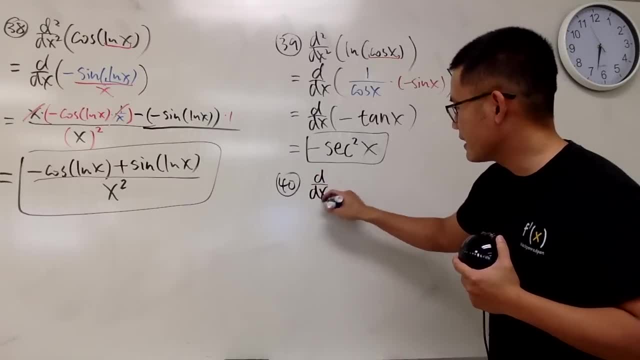 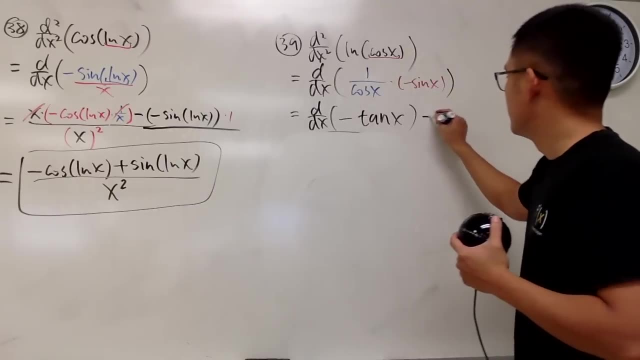 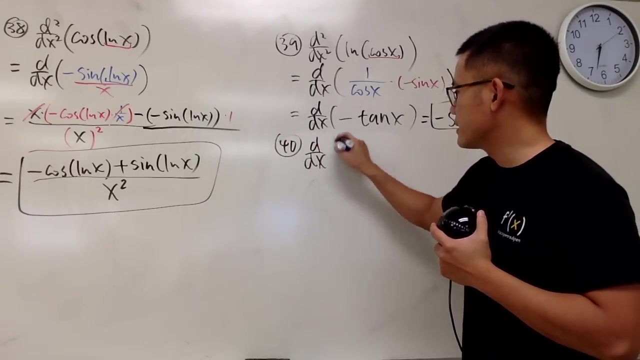 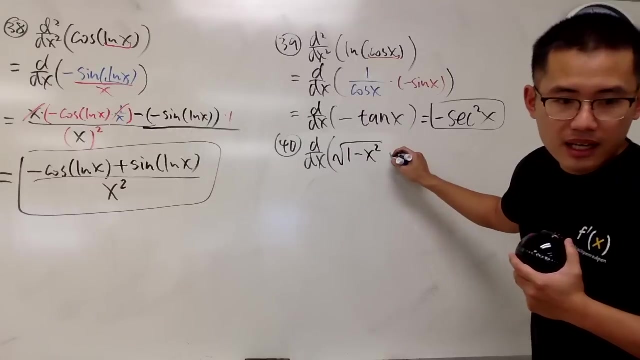 Ah, this is a very good one. d dx. I need more space. Negative secant squared x Number 40.. d dx- d dx is just one derivative, okay, Square root of 1 minus x squared and we add x times. 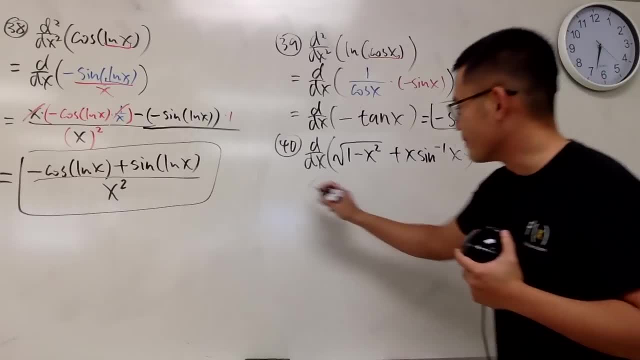 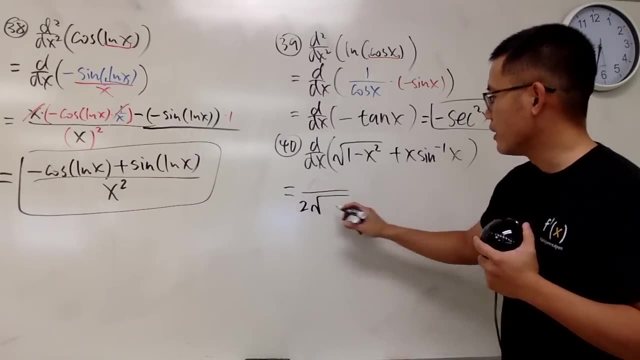 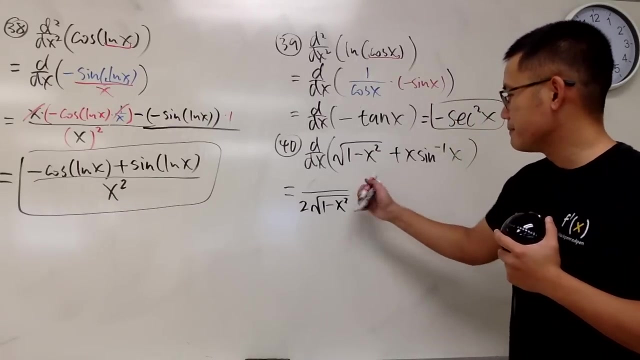 inverse sine of x. Here we go. Just one derivative of the square root. we get 1 over 2 square root of the bottom of the inside, like this On the bottom, like that right, And we multiply by the derivative of the inside. so we multiply by. 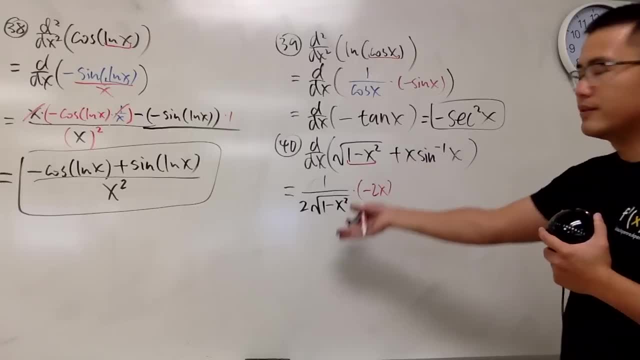 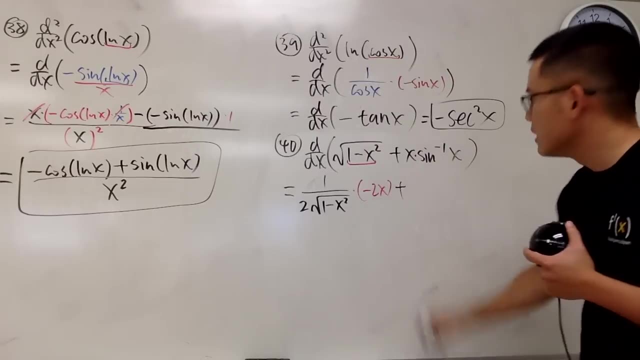 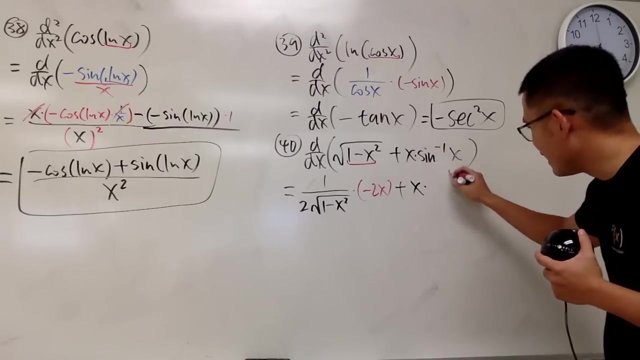 by negative 2x. That's it for the first derivative for this part. And then we add: this part requires the product rule. That's why I have the dot. Keep the first function times. the derivative of the second Derivative, inverse sine, is 1 over square root of 1 minus f squared Similar. 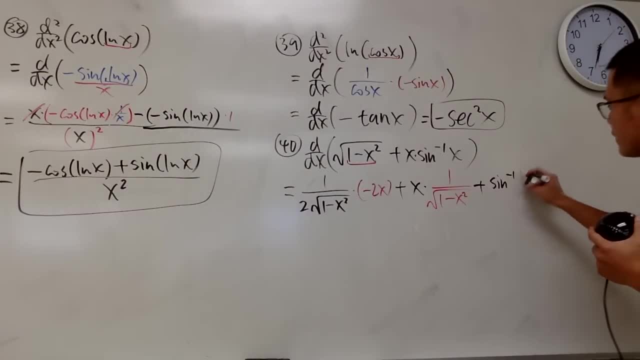 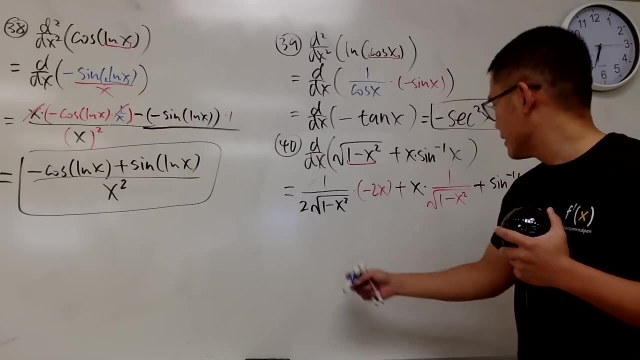 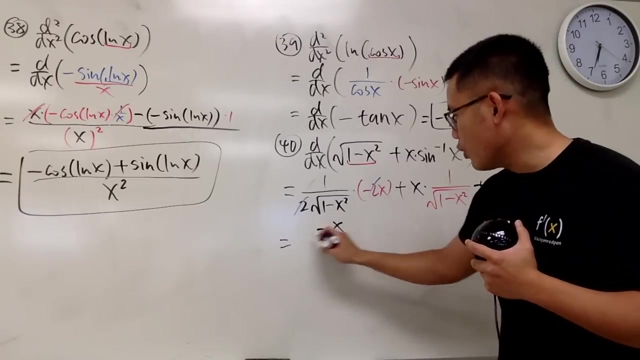 And then we add the second function, which is inverse sine of x times the derivative of x, the first function. Now check this out: Cancel, cancel. So if you write this down again, you will see this is negative x over. this is square root of 1 minus x squared. 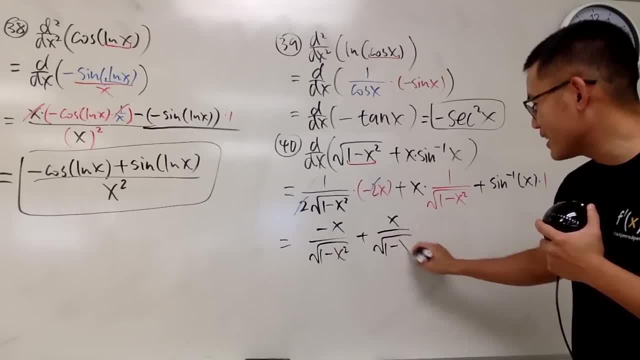 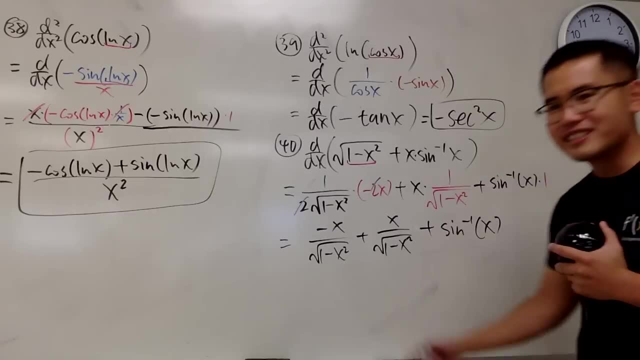 But here is plus x over square root of 1, minus x squared. And of course, don't forget, lastly, you have that inverse friend, inverse sine of x, like that, Of course, this and that can be nicely canceled out. 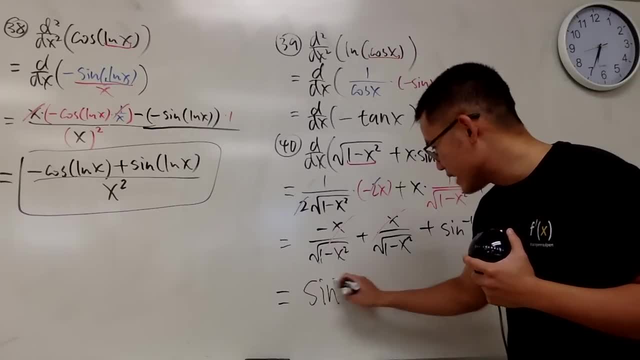 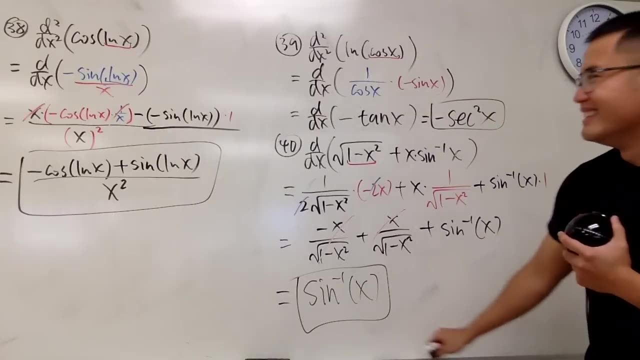 Finally, you just have your inverse friend, inverse sine of x like this plus z. No, you don't have to. This is it In Calc 2, you guys will have to know how to do this backwards Derivative. 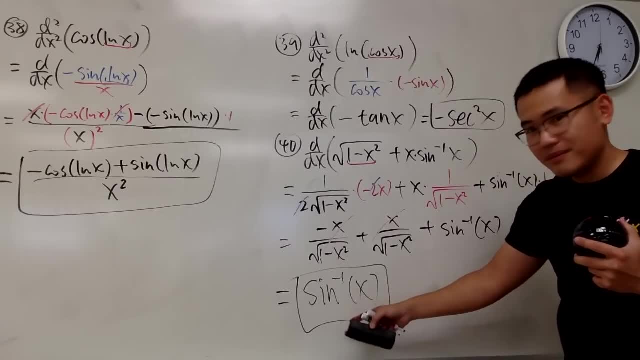 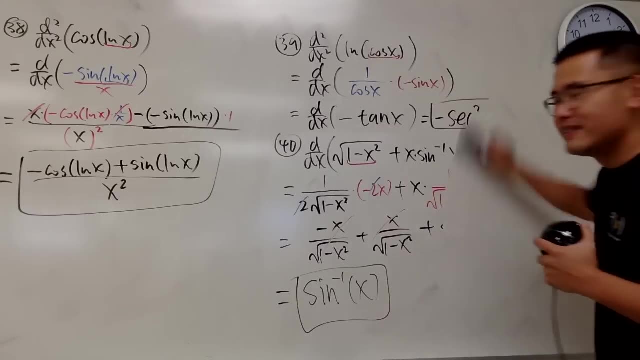 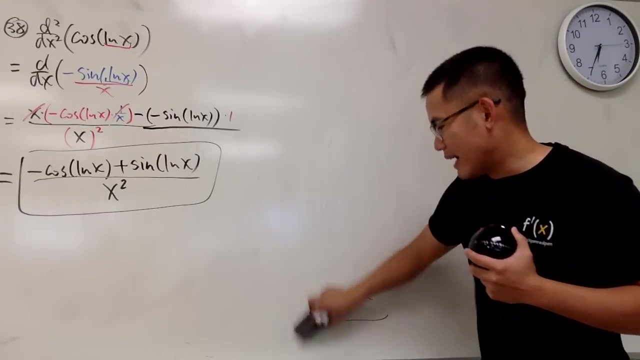 what will give you inverse sine? I'm not asking you what's the derivative inverse sine? I'm asking you: derivative, what which is this will give you inverse sine? Integration by parts. I don't know who are watching the videos. My intention is, of course, for the students. 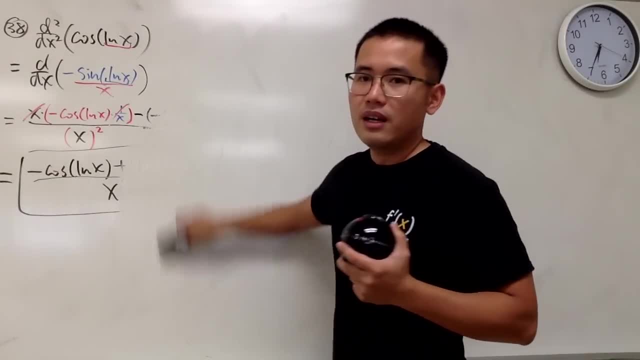 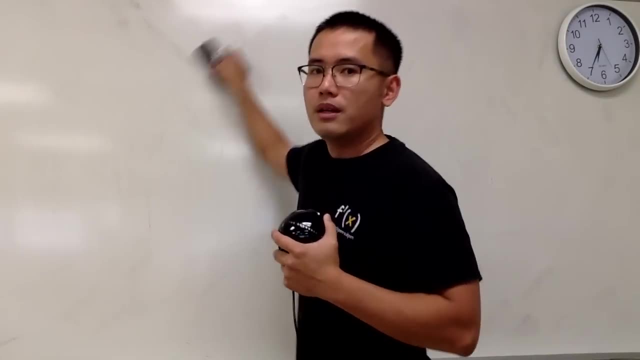 who are in Calc 1 and Calc 2, especially for the very last few questions. Or maybe you haven't done calculus for a while and you are going to do like Calc 3, maybe Especially in the summer- if you just want to practice, you should do this. Maybe you are AP Calc. 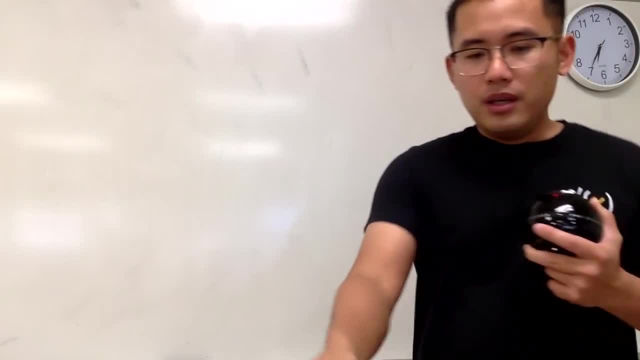 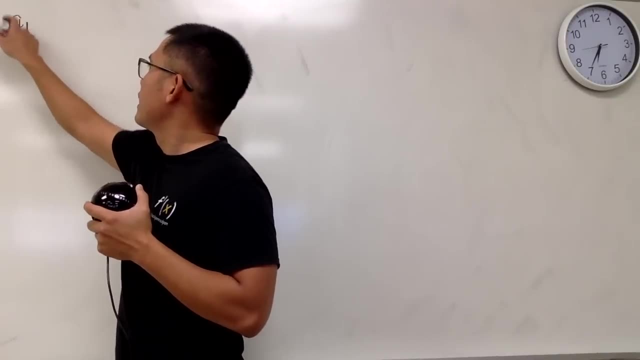 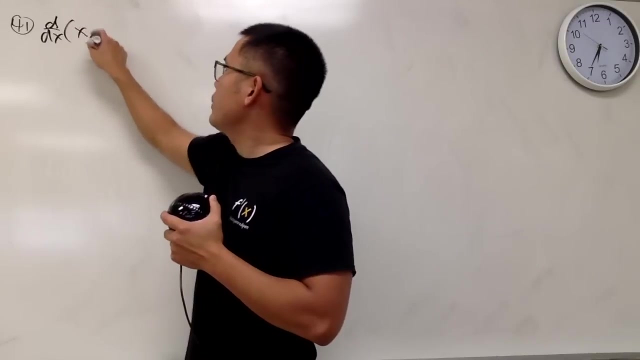 students Just do it, Or maybe you're just like me, who just like derivative calculus and all that. So, as you've seen, the derivative is the derivative of this. Yeah, number 41.. Okay, just one derivative. We're going to differentiate x squared root of 4 minus x. 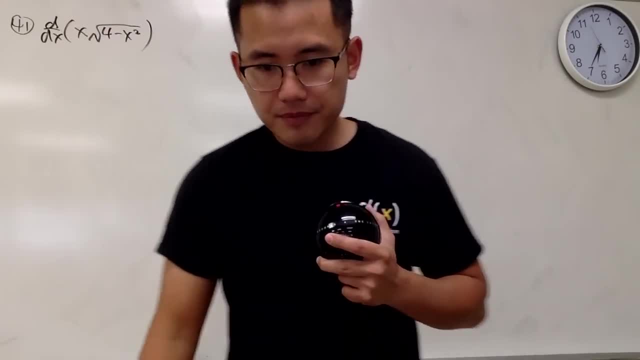 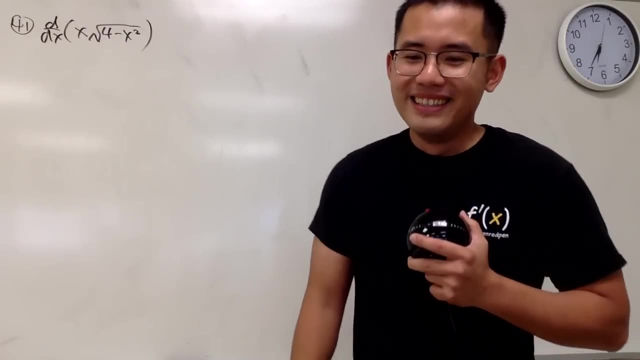 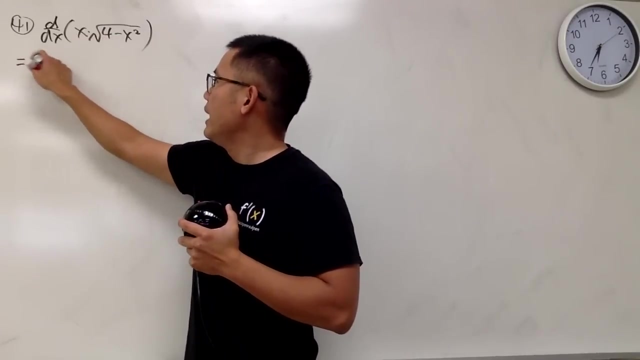 squared. Okay, No, just kidding. I'm not like getting DC. Alright, Product rule in action. This is x times, So here we go: x times x, x times x, So you'll times square root function. so we get 1 over. well, let's just do it. 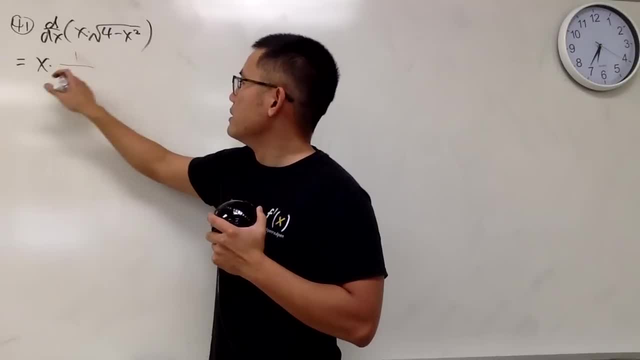 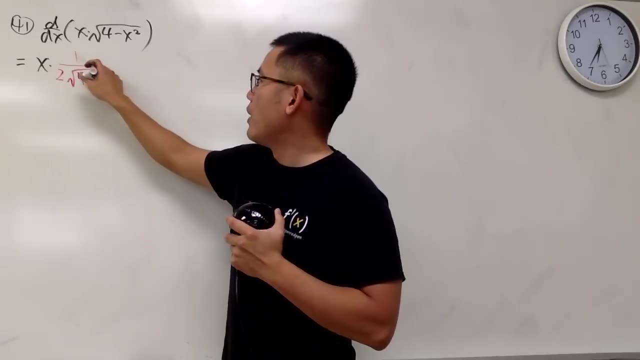 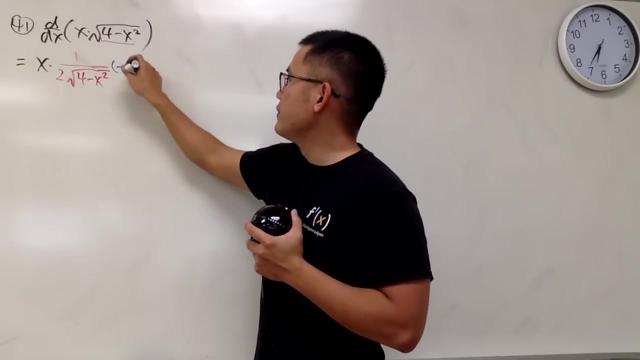 The derivative of this right here. I'll put it in red: 1 over 2, square root of 4 minus x squared. However, use the chain loop, multiply by the derivative of the inside, and that will give us negative 2x. 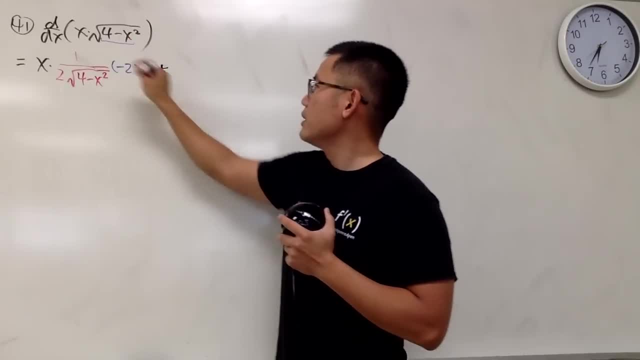 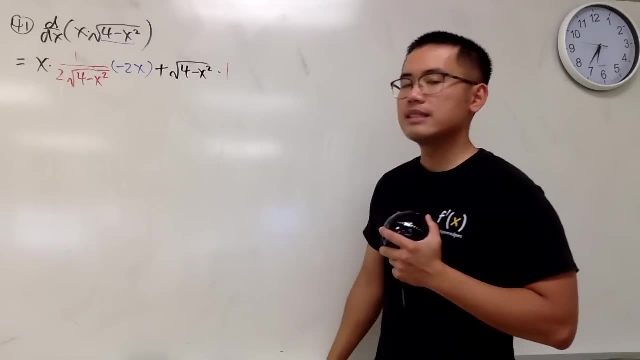 That's the first part. Then we add the second function, which is square root of 4 minus x, squared times the derivative of the first, which is just a nice 1.. Well, well, this 2 and that 2 can be cancelled. 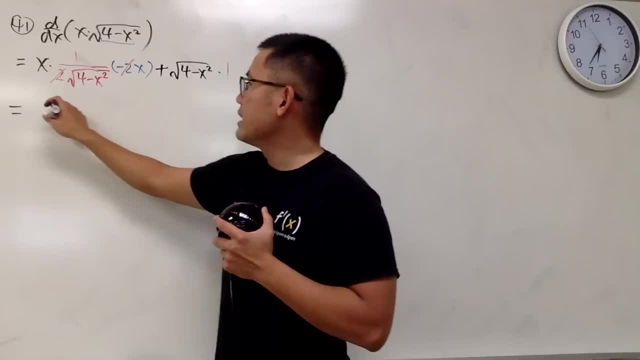 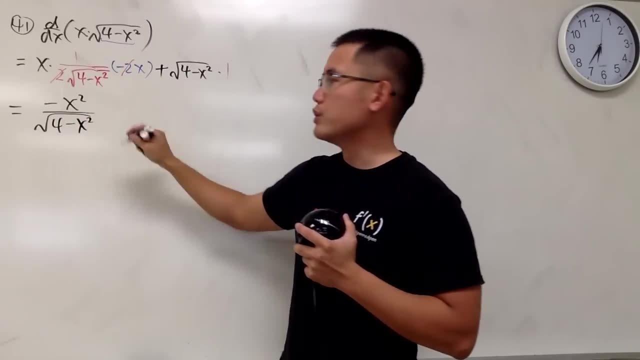 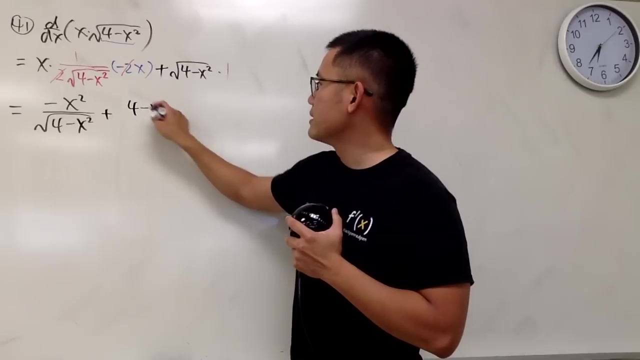 That's good, and we see that x times negative x, that's negative x squared over. this is square root of 4 minus x squared, and we have this part which is plus 4 minus 4 minus. let me do it on this: 4 minus x squared in the square root, right. 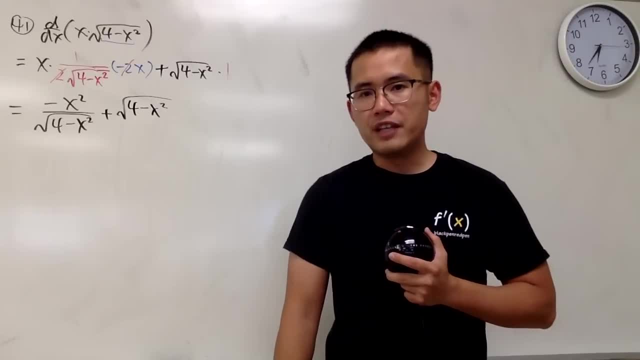 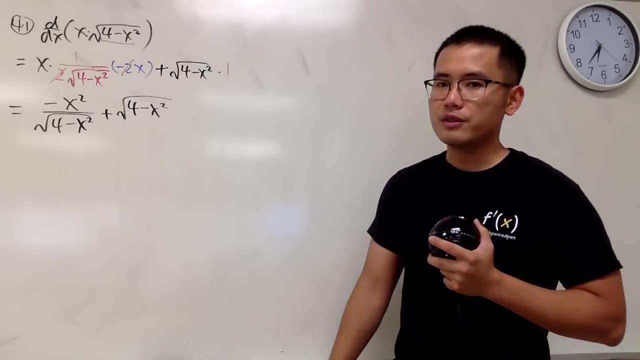 Okay, imagine that you had to find the derivative and you had to set the derivative equal to 0, so you can find the critical numbers. Well, this is not what you preferred. If you need to find if the function is increasing or decreasing or not, 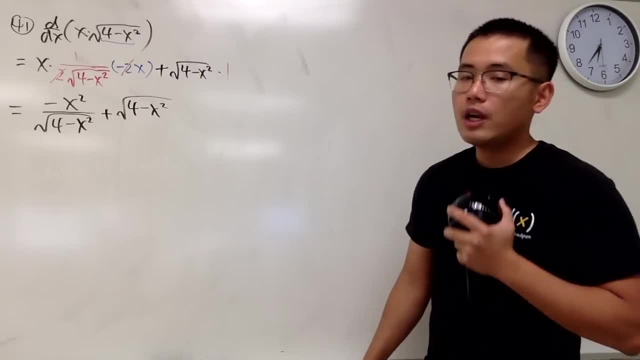 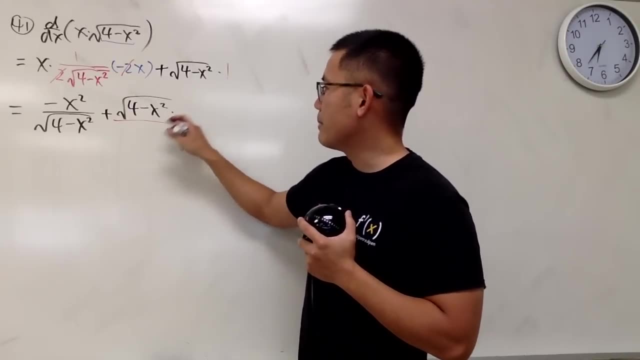 this is not the function you prefer. You want to add them together. With that said, we have to get a common denominator, so let me just multiply this. I'm going to multiply the second one by that which is square root of 4 minus x squared on the bottom. 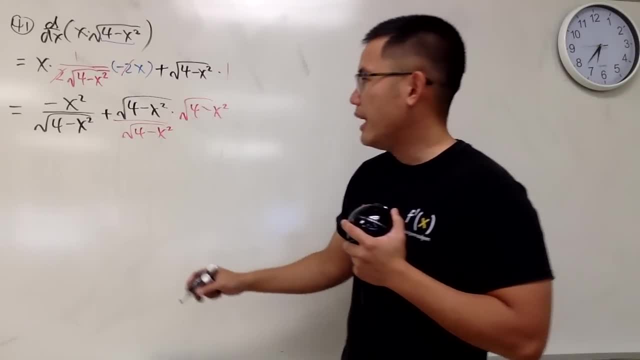 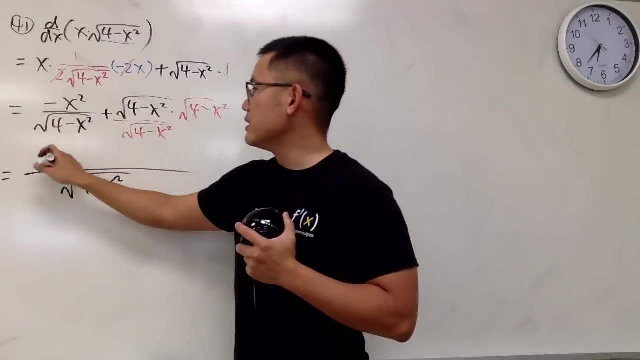 and also on the top like this. And when we do that, you will see on the bottom it's just square root of 4 minus x squared. On the top, here is negative x squared and this times that is just plus. 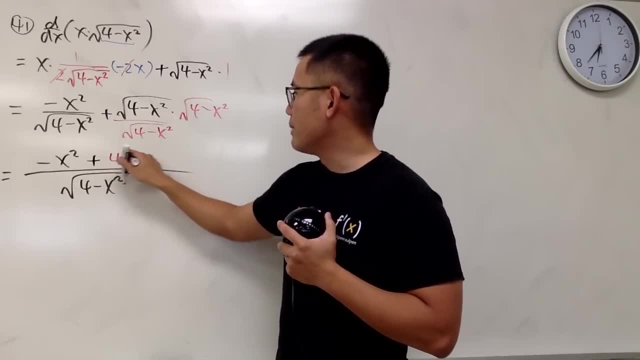 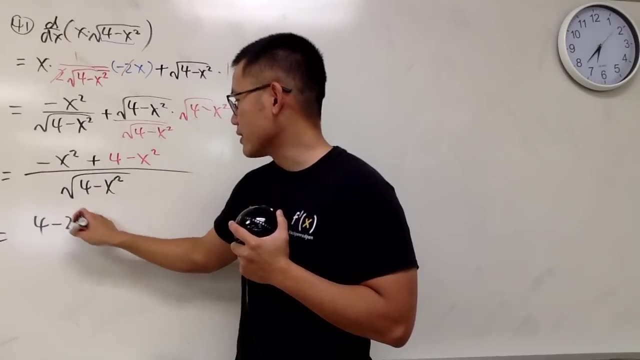 and the square root is just gone. We have 4 minus x squared like this. So all in all you get 4 right here, Minus x squared, minus x squared, Square minus x squared. So that's minus 2x squared over square root of 4 minus x squared. 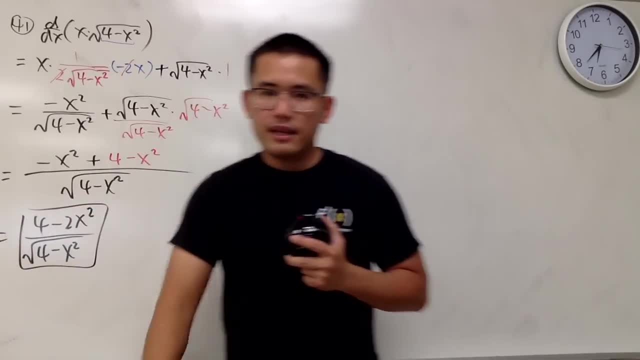 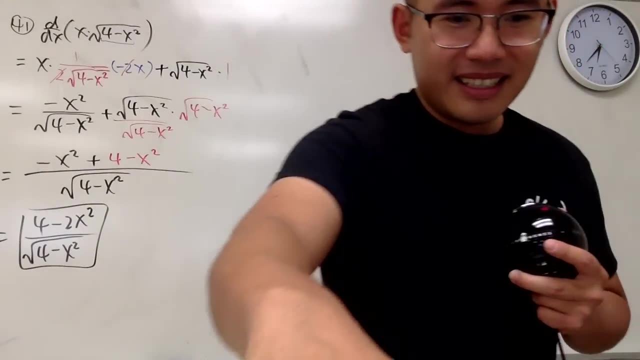 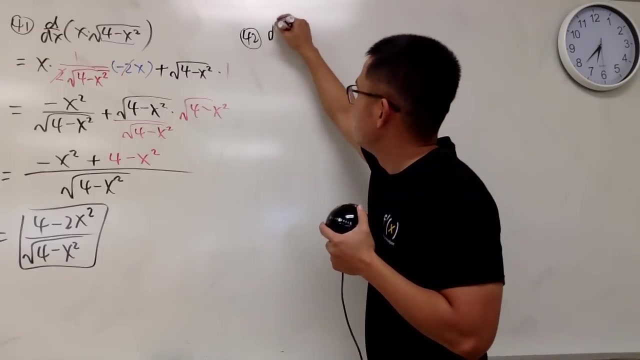 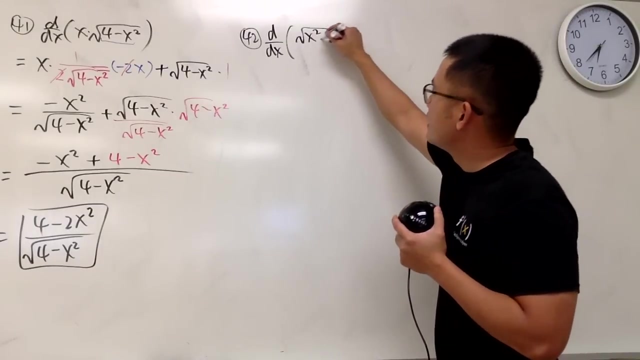 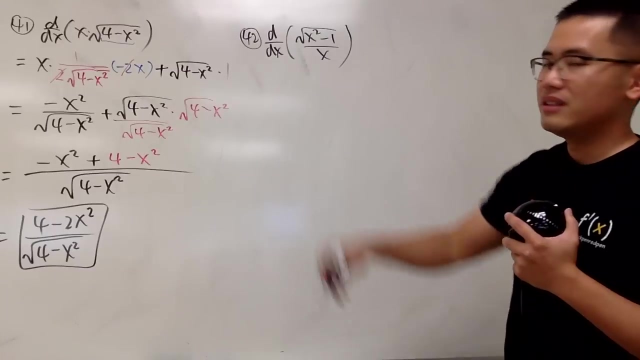 Like that: Good, Nice and cute. huh, Another Done, 42.. Okay, another square root, Differentiating square root of x squared minus 1 and over x. Here we will be using the quotient rule, so it's kind of like the other opposite. 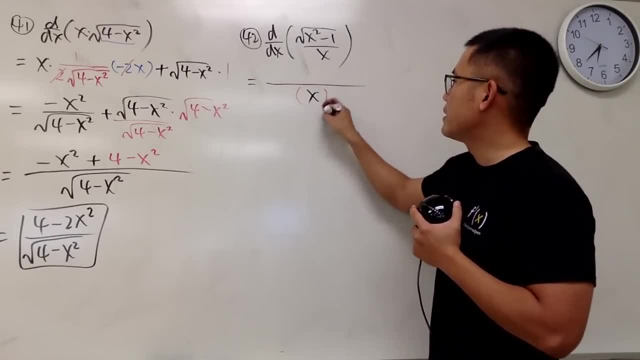 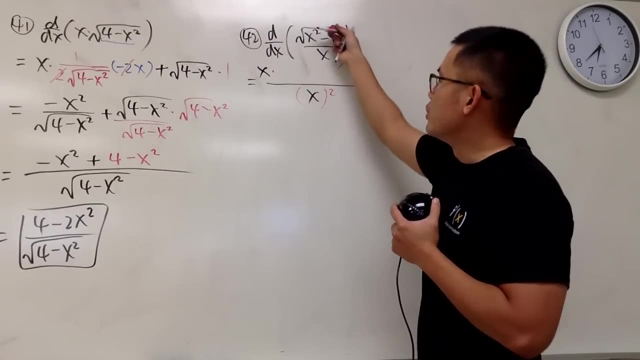 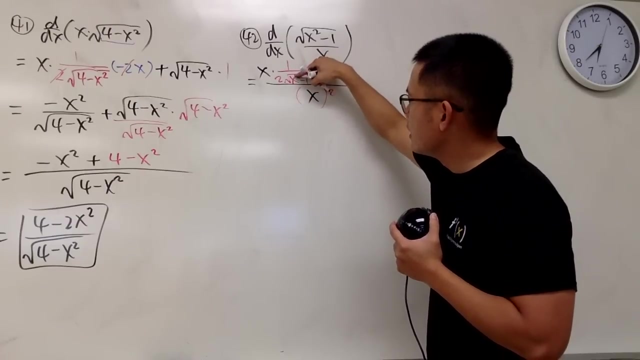 Anyway, go ahead and square the denominator and put down the bottom function right here. Multiply by the derivative of the top. The derivative of the top is going to be 1 over 2 square root of x squared minus 1.. x squared minus 1.. 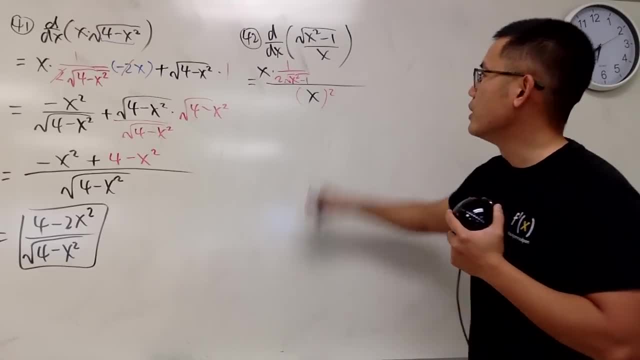 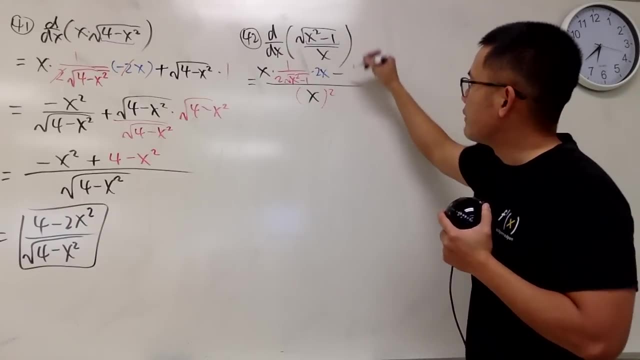 And then don't forget the chain rule. Use the chain rule: Multiply by the derivative inside, which is 2x, And then minus the top function, which is square root of x, squared minus 1, times the derivative of the bottom. 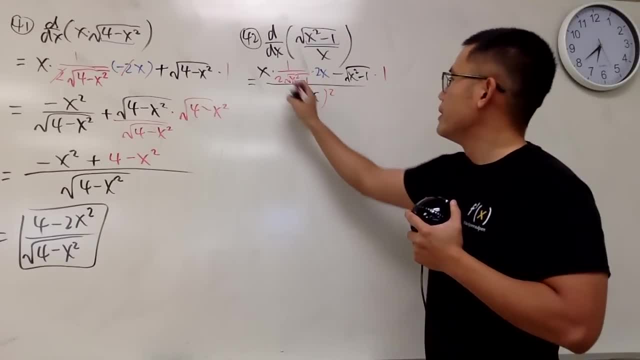 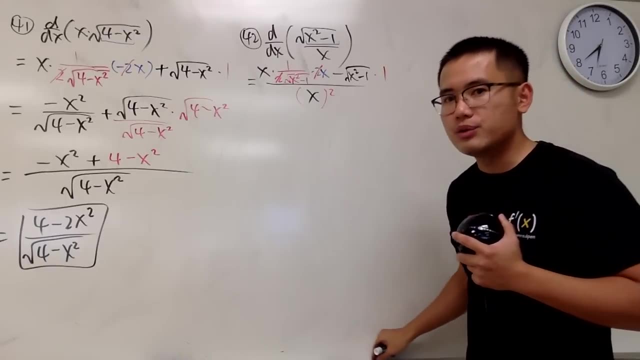 So that's what we have On the top, though again, 2 and 2 cancel out nicely and we have x squared, But we have a complex fraction in this situation. So to handle that, let's multiply the top and bottom. 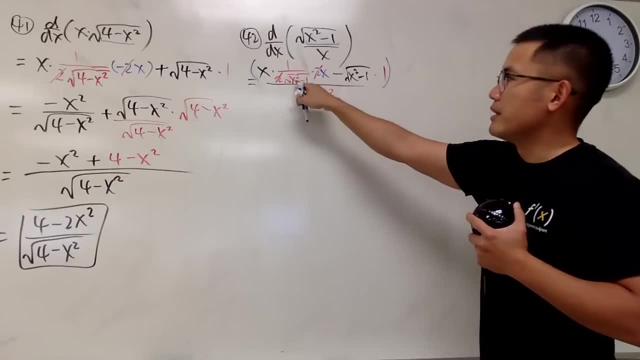 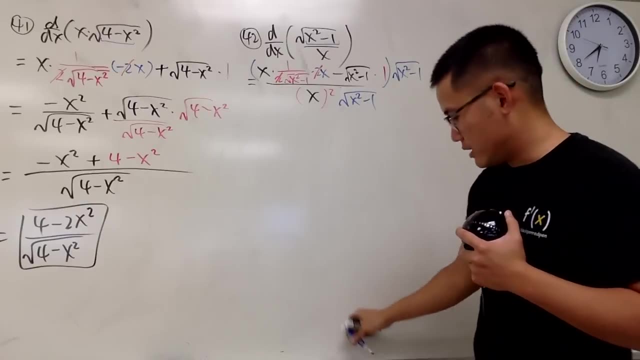 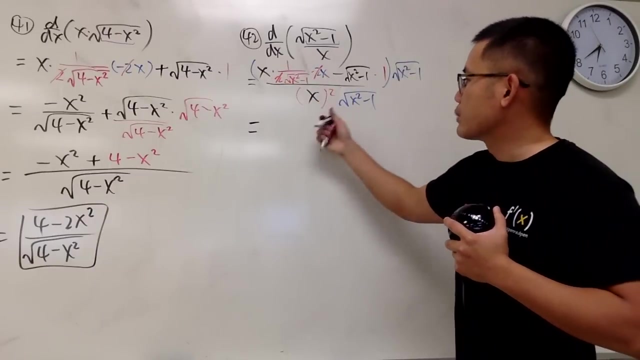 by the common denominator, which is just this. So multiply by square root of x squared minus 1, square root of x squared minus 1.. And then when we do that on the top, this and that will cancel. So we have x times x. 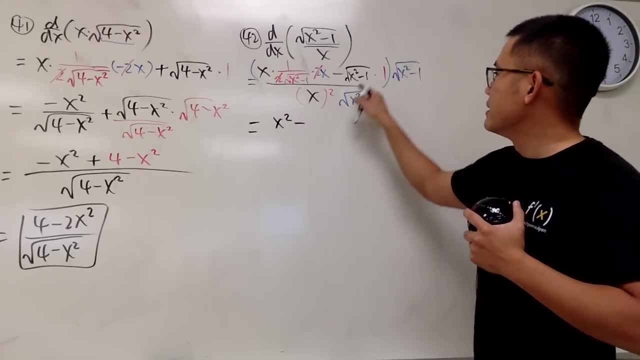 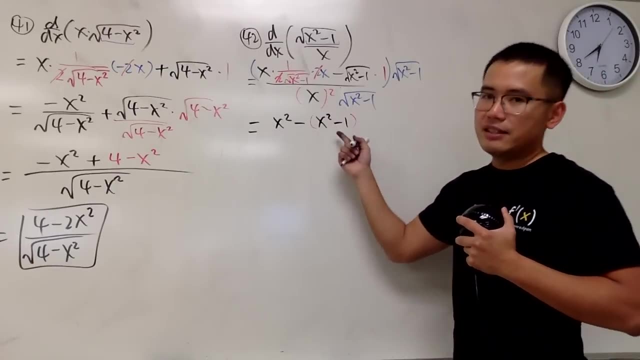 which is x squared, And then this is going to be minus This and that the square root will be out. So you just have a parenthesis and you will have x squared minus 1, like that. I haven't distributed, so yeah. 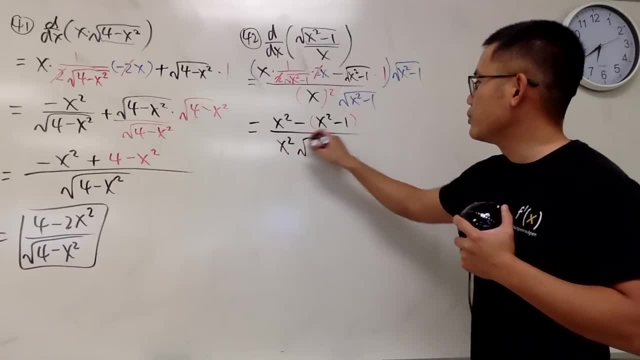 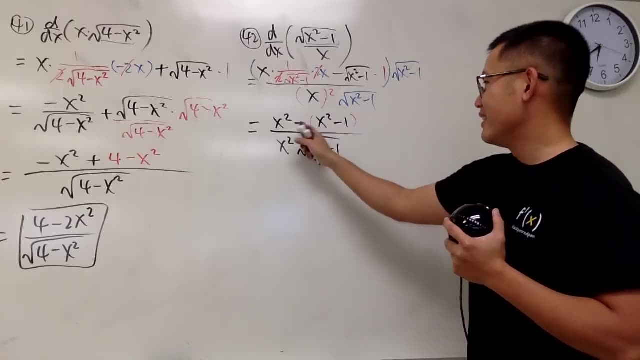 And over here we have x squared and you have the square root of x squared minus 1.. Now, x squared minus x squared is just bye-bye. Negative, negative is just positive 1.. So we have 1 over this guy. 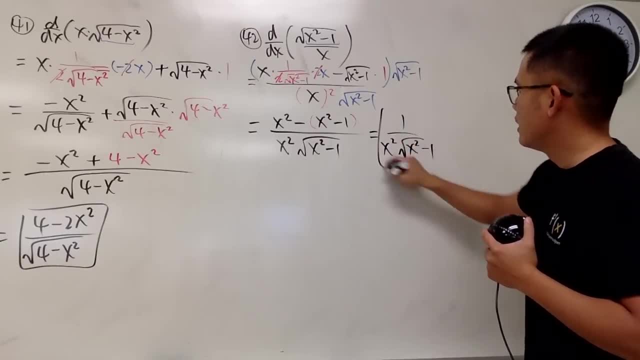 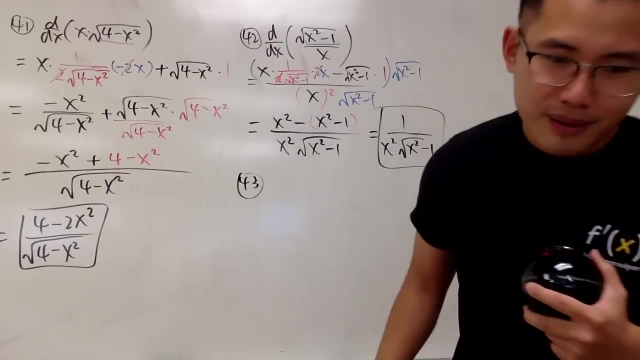 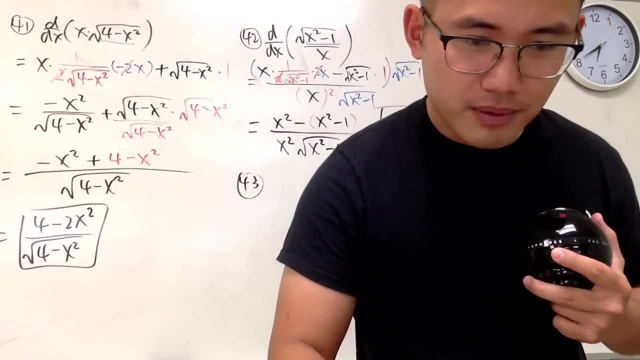 x squared, square root of x squared minus 1.. Like this: Okay, I'm going to fit number 43 right here. I switched the order. Why did I do that? That's interesting. I just switched the order of the x over that. 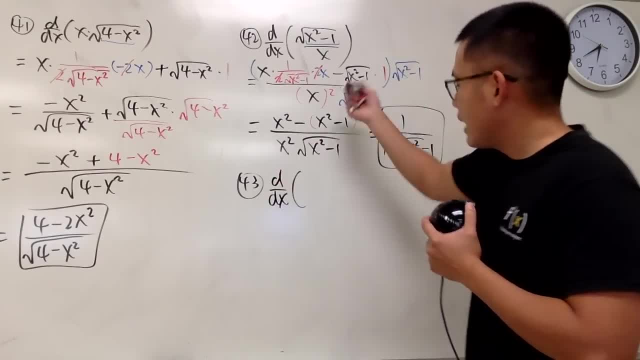 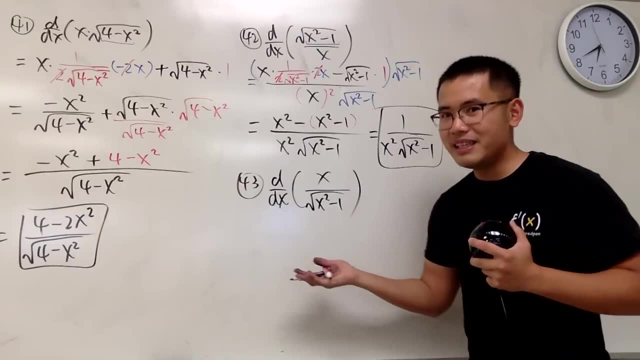 So okay, okay, okay, dx. So this one, I have x on the top instead over square root of x, squared minus 1.. Let's see how the answer will turn out to be okay, Okay. quotient root in action. 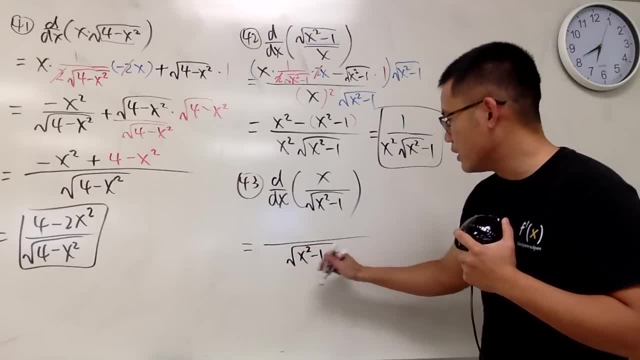 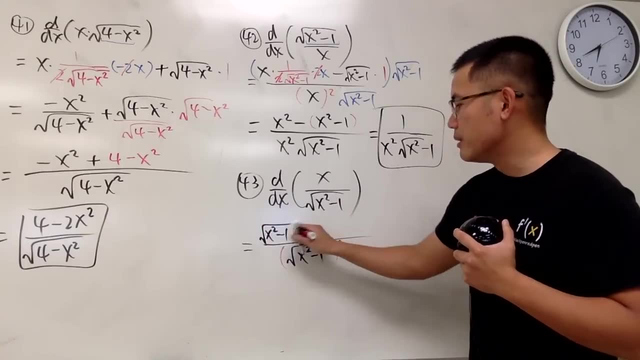 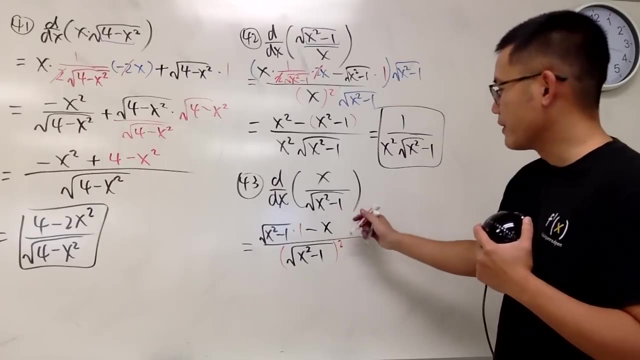 So here we will have to square the denominator. We'll choose this one now. So put that denominator on the top right here. first, Multiply by the derivative of the top, which is 1,, minus the top function times the derivative of the bottom. 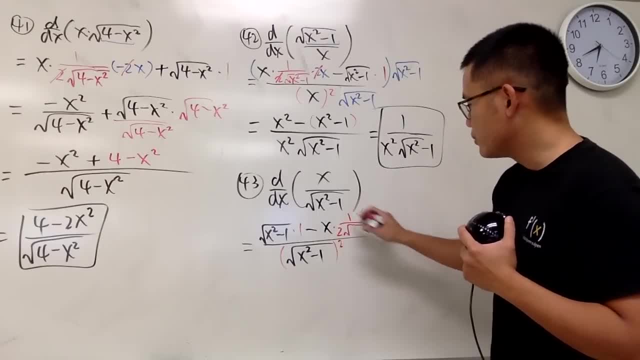 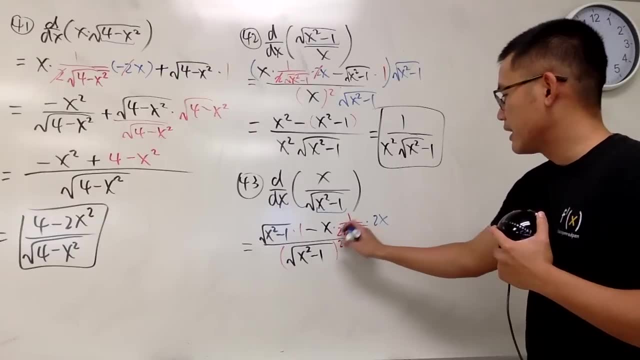 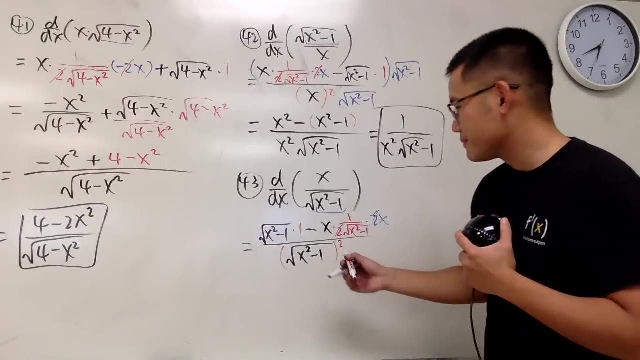 And the derivative of the bottom is 1, over 2 square root of x, squared minus 1, and change to multiply by 2x. Cancel, cancel, right, That's canceled. That's out already Good. However, this time though, 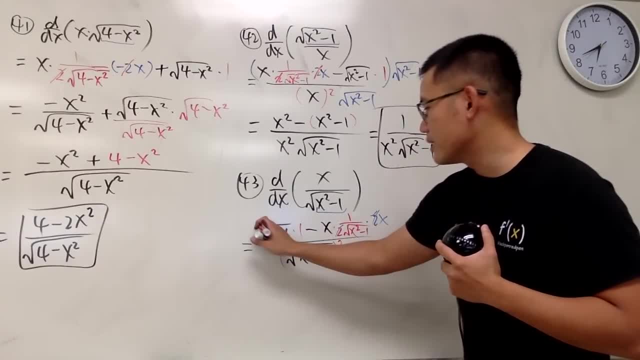 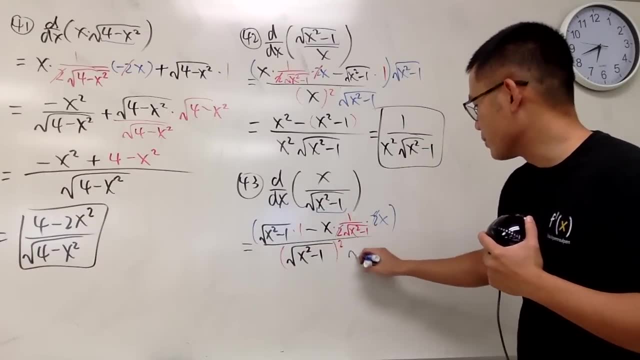 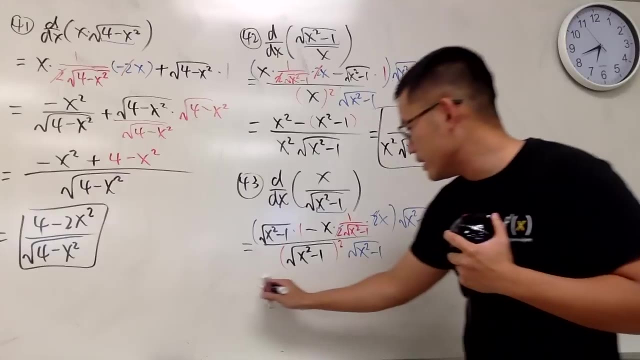 again. get a common denominator, Get a. get a. multiply this guy. Get rid of the complex fraction. So multiply the top and bottom by square root of x squared minus 1.. Let's see what this will give us This, times that we'll just have that. 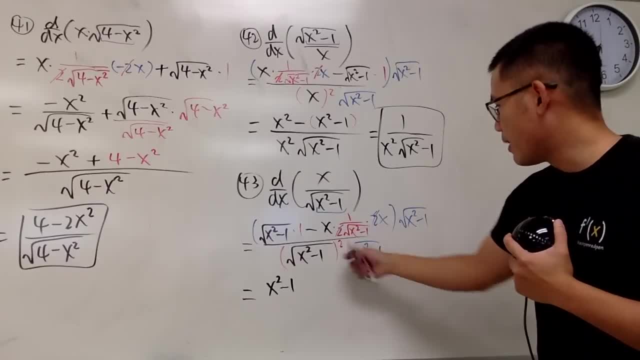 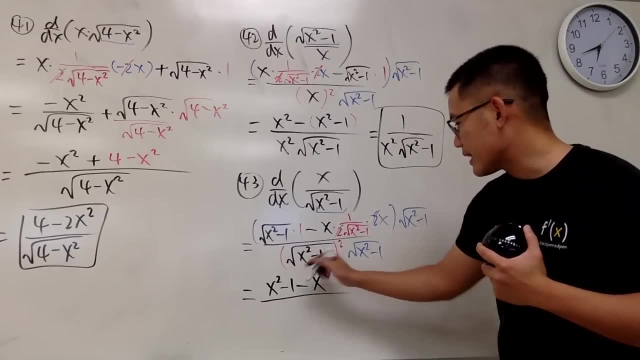 Namely x squared minus 1.. This times, this part, this and that cancel, we have minus x squared over here. this and that cancel, which is that's saying x squared minus 1 to the first power. 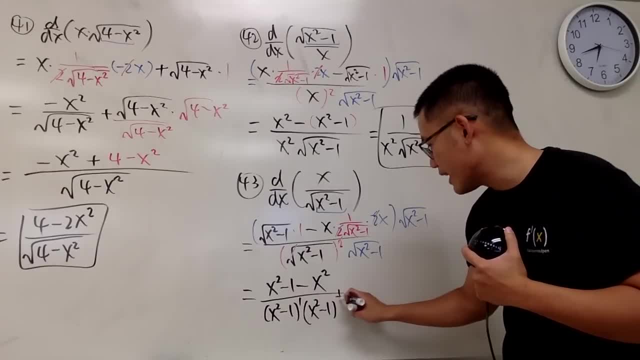 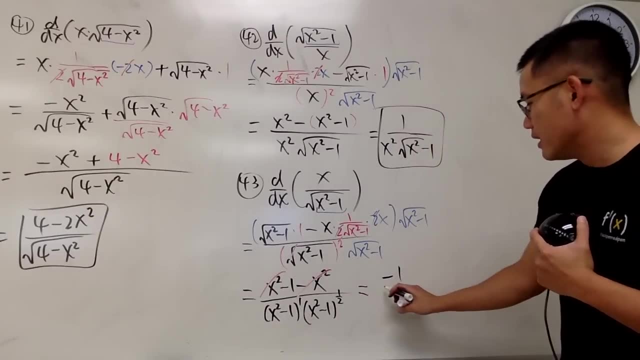 This right here. that's saying x squared minus 1 to the one-half power. This and that cancel On the top we have negative 1, right Over this. right here, I believe, by putting the radical form for the answer. 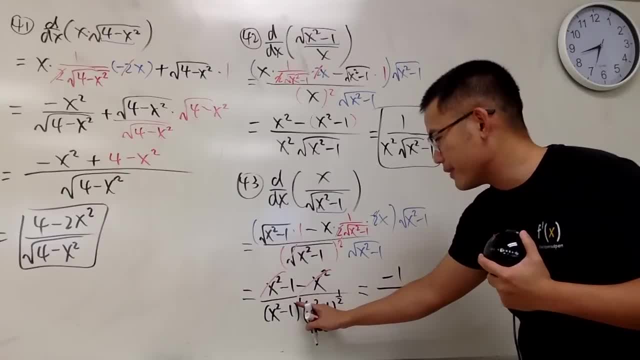 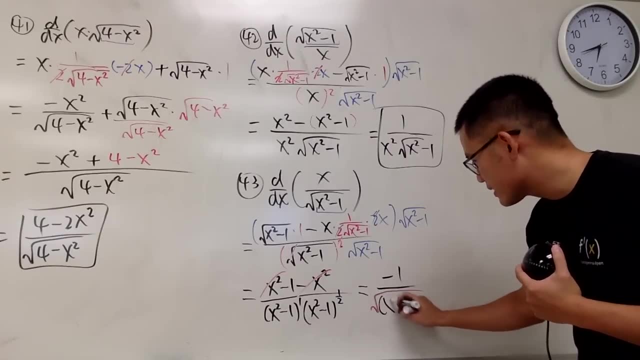 and I did So. let's do this in our head: 1 plus 1-half is 3-half, So the half is the square root And the inside x squared minus 1 to the third power, like this: 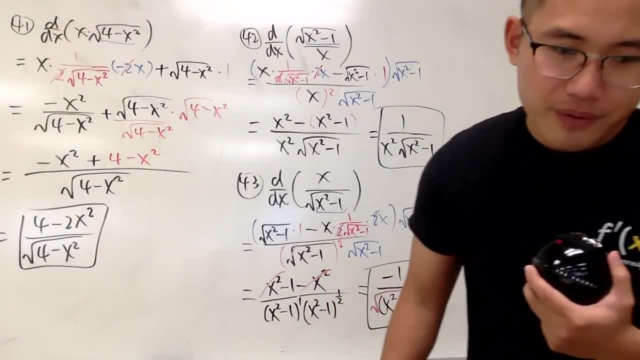 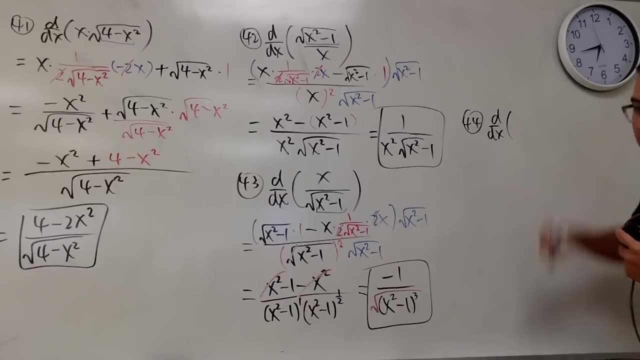 That's it, Number 44.. I'm going to see the number 44 right here as well. Let's see We are going to be differentiating. This one is a fun one. We have cosine of inverse sine x. 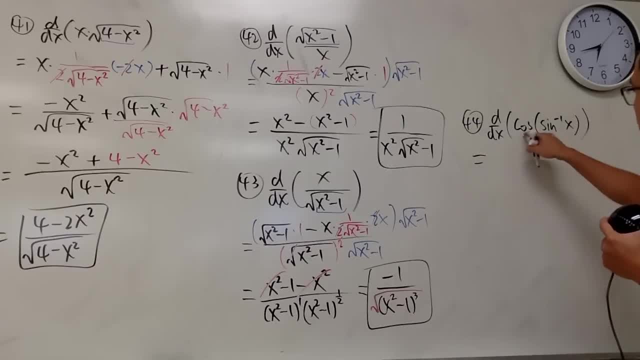 Like that. Okay, here we go. What's the derivative of cosine? Well, it's just negative sine, isn't it? And the input states the same, so you just write it inverse sine of x like this, However: 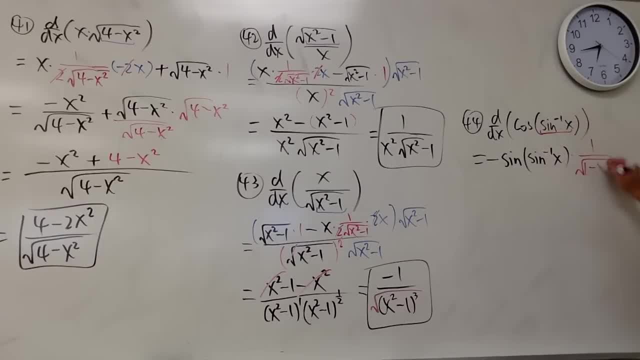 chain rule: right: Multiply by the derivative inside, which is 1 over square root of 1 minus x squared, just like that. Well, well, Sine of inverse sine, they pretty much cancel. You can just put it down like this: 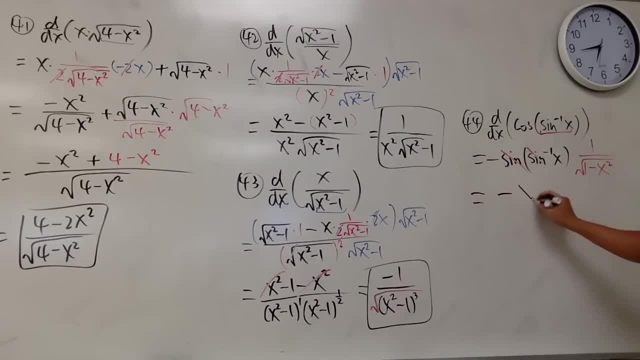 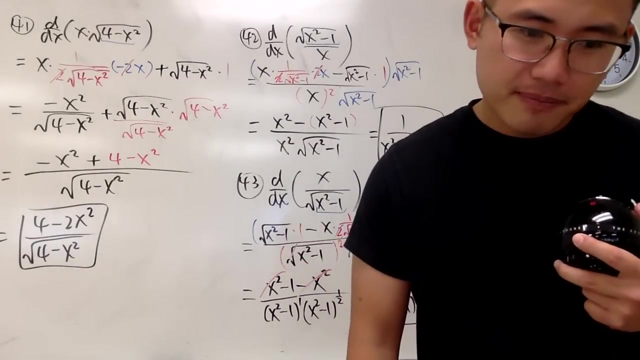 So you have negative x, negative x over this for the denominator. Wow, All the answers look kind of similar to each other, all the square root and all that stuff. Very nice, Very nice, Very nice. Okay, And I'm also going to fit in 45 here. 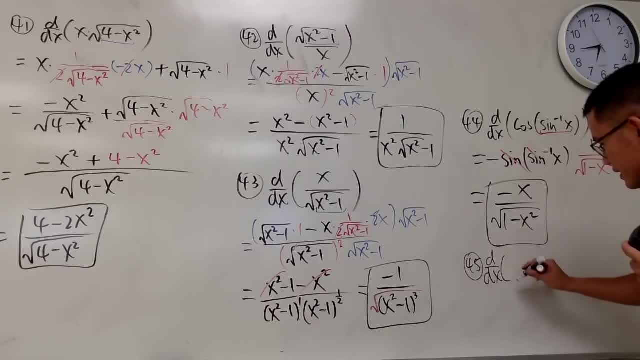 because this one is not bad at all. d, dx, natural log of x squared plus 3x plus 5.. So this is the input and we have natural log right on the outside. So remember it's 1 over the input. 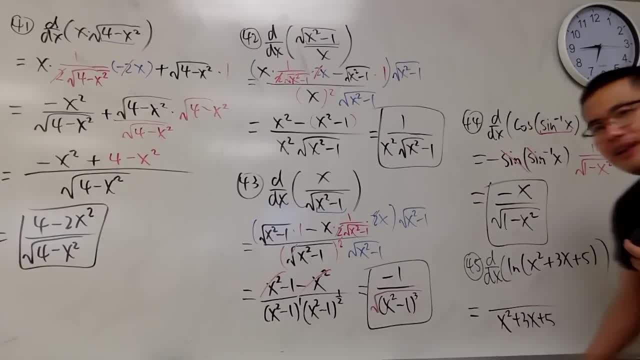 which is x squared plus 3x plus 5.. And the chain rule says what Multiply by the derivative of the inside. Keep in mind it's 1 over that times the derivative inside. We can just put the derivative on the top. 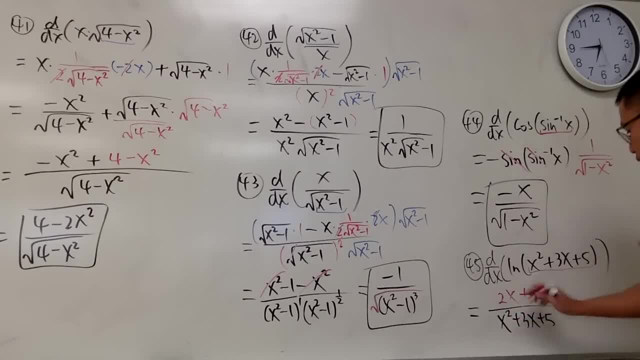 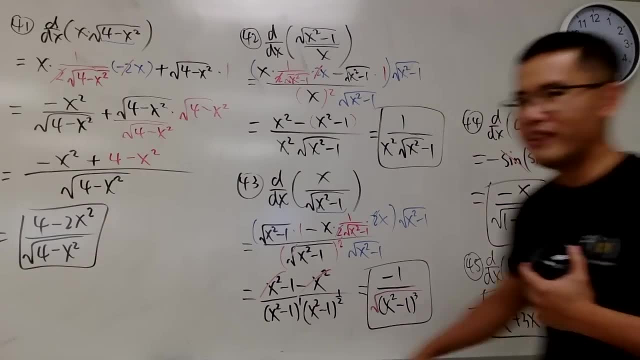 So here we get 2x plus 3x plus 3.. Done, Done Man. I can do the natural log derivative like this all day long. Give me 1,000 of them, I will do it for you in 5 hours. 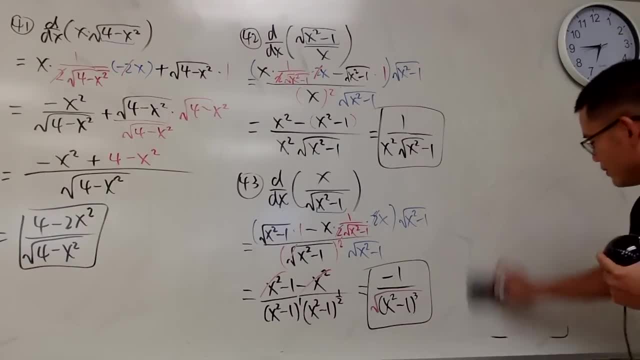 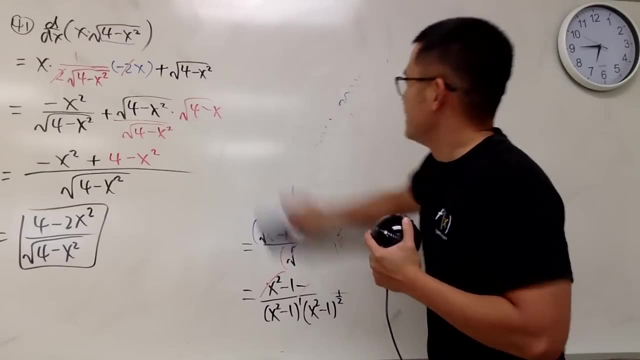 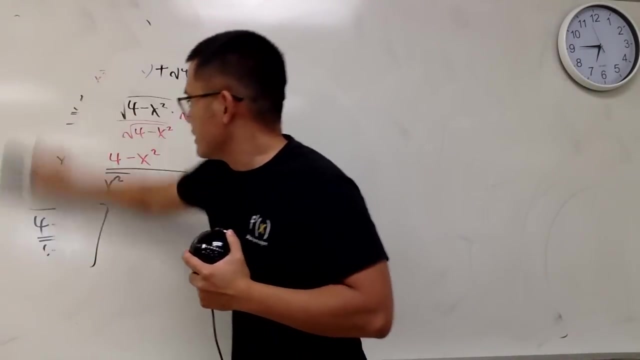 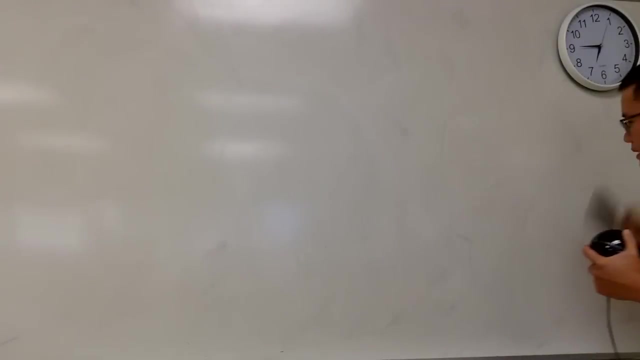 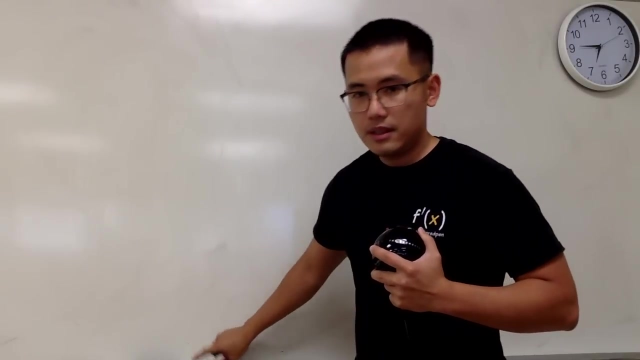 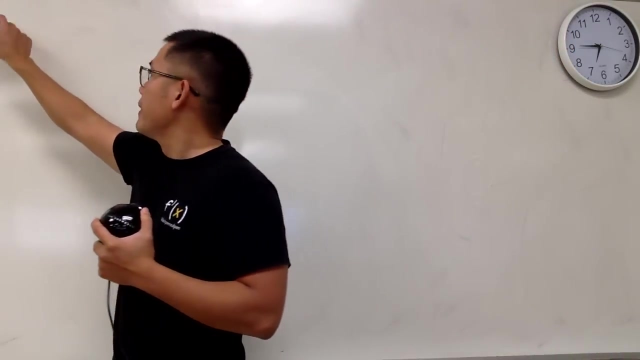 No, Don't do it, Don't give me 1,000.. No, No, Don't take it too seriously. That was me being saying whatever I don't know. Okay, What was that? Number 46 now. 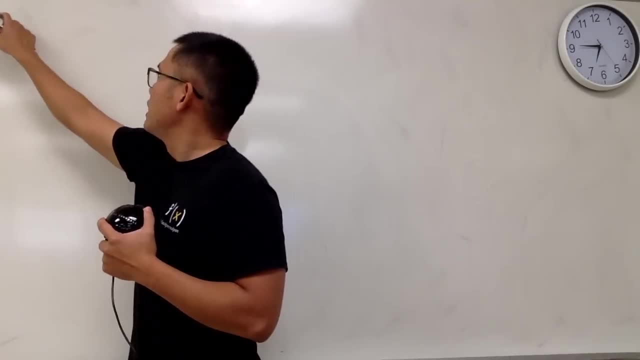 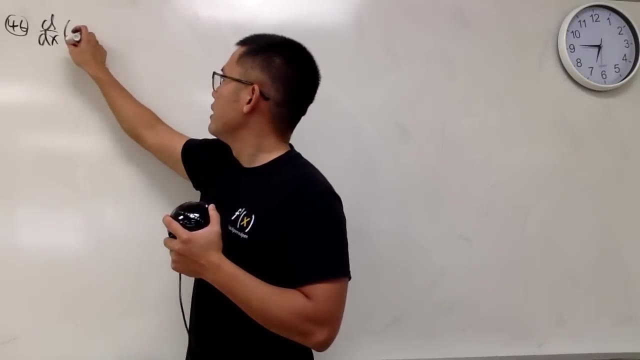 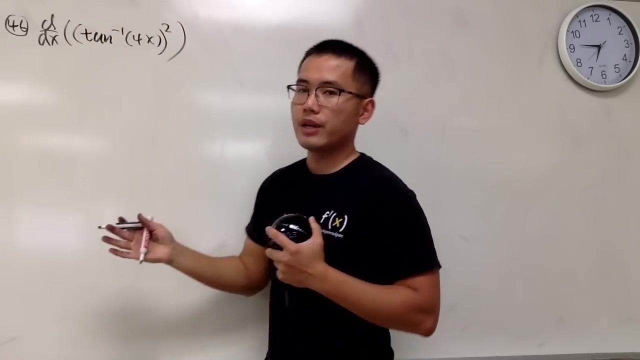 That doesn't look like a 6. D dx. This one is a tricky one. Inverse tangent of 4x. But we raise that to the second power like this: Okay, Here is the deal. Do not multiply this and say: 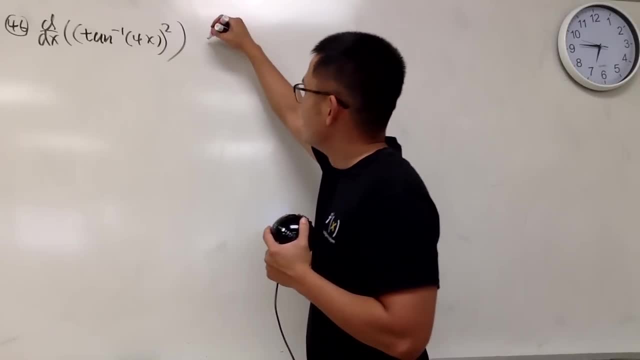 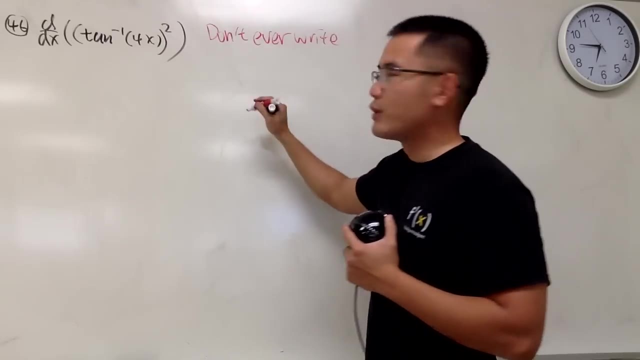 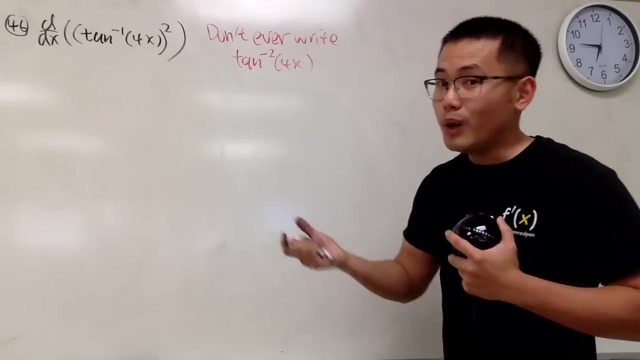 that's tangent negative 2.. Okay, I would just say: don't ever write seriously, don't ever write things like tangent negative 2 right here, 4x like this. Don't If you want to say: 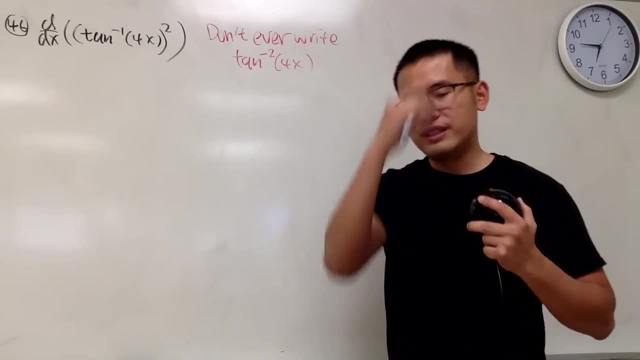 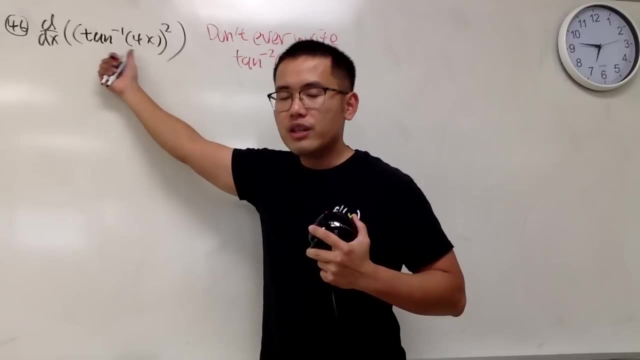 tangent, the regular one tangent, and then raise to the negative 2 power. put that to the outside of the parentheses. Okay, This means you have the inverse tangent of 4x and then you square that Okay. 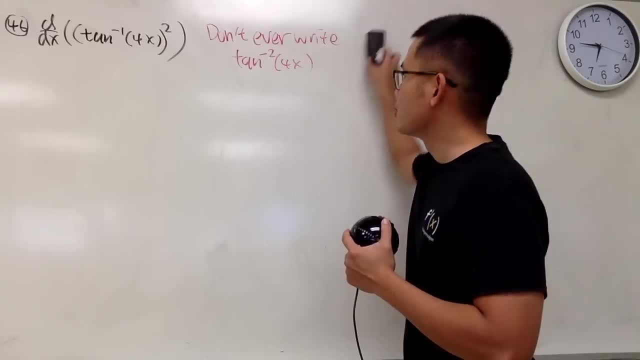 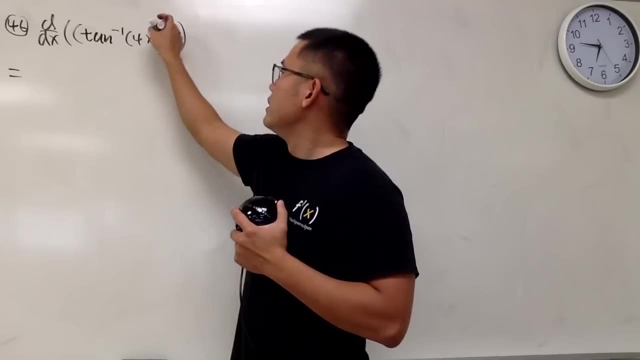 Don't ever write this Seriously, just don't. I have a video on that. You guys can go check that out. That's like the the worst notation. Anyway, here we go. What we do is do the outside. 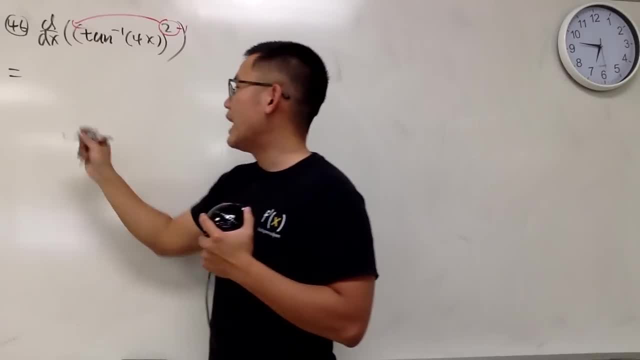 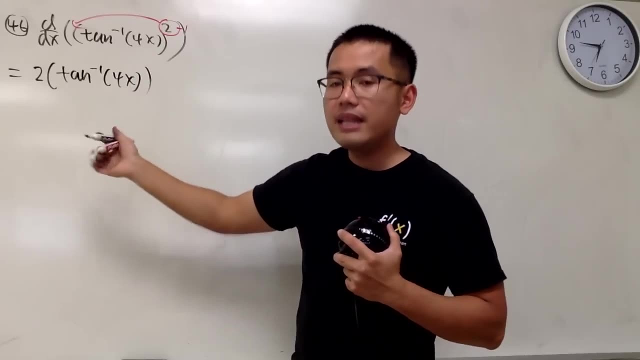 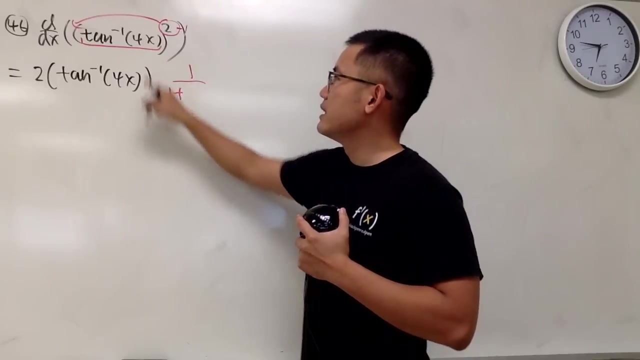 which is the power situation. Here we have 2, parentheses, the inside stays to the first power and then multiply by the derivative of the inside. Derivative of inverse tangent is 1 over 1 plus. 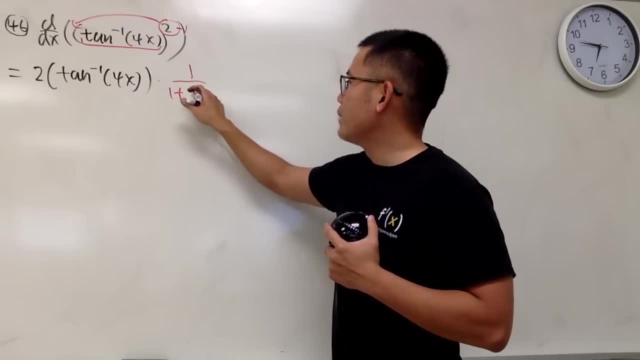 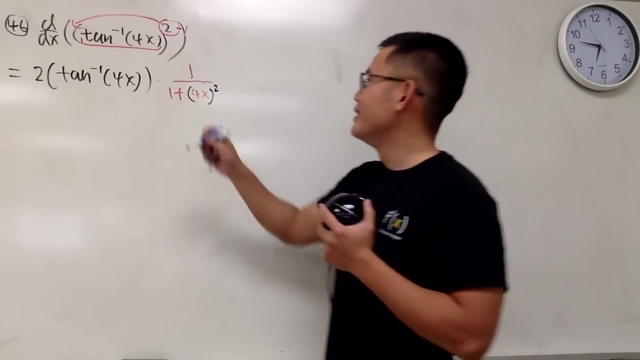 the input square right here, right? So we have to have the 4x here. but don't forget, we square that, Are we done? No, Then do multiply by the derivative of this, which is multiplied by 4,. 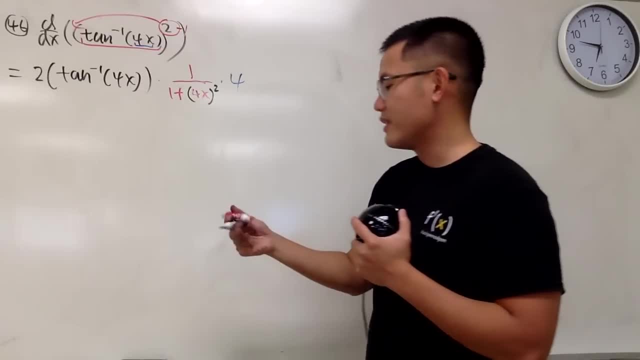 right there. Now put the answers together: All in all, 2 times 1 times 4,, which is 8, and then this is also on the top. so we have the inverse tangent. Do not bring that down to the denominator. 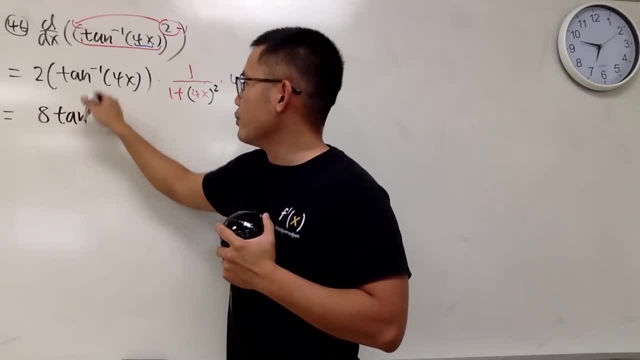 This is the arc tangent, the inverse tangent. So you just write it down like this: All over this right here is 1 plus 4 squared is 16, and then you have the x squared. This is like a really cool expression. 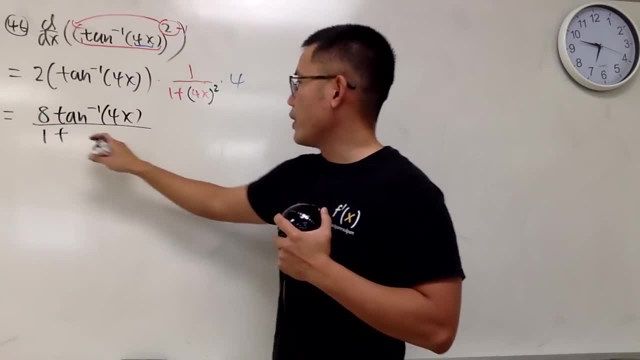 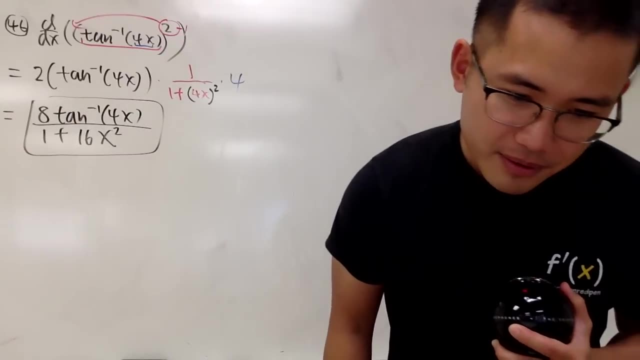 huh. So you just write it down like this All over this right here is 1 plus 4 squared is 16, and then you have the x squared. This is like a really cool expression, huh. Okay, All right. 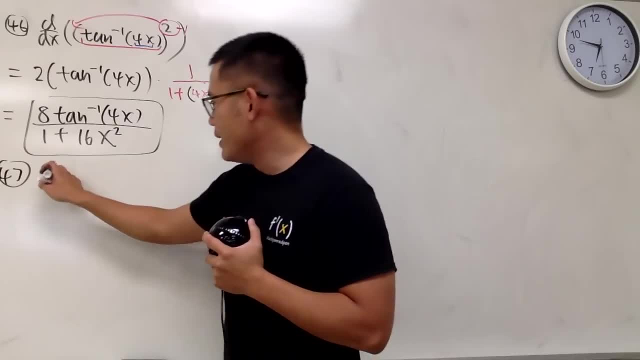 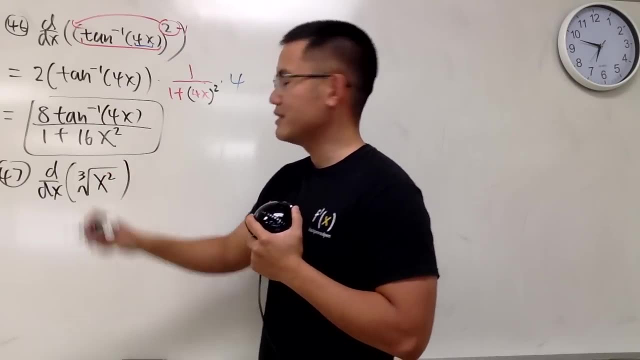 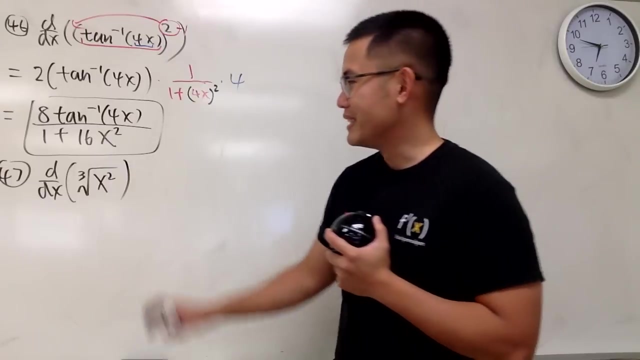 number 47. We are going to be differentiating- Oops, here we have a cube root function By the cube root of x to the second power. like this: Do we do any chain rules? You don't have to. Here is how you do it. 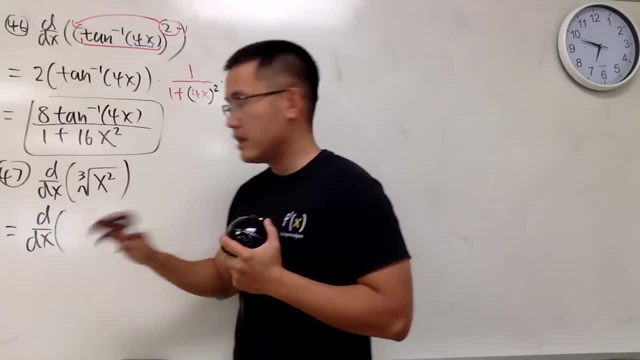 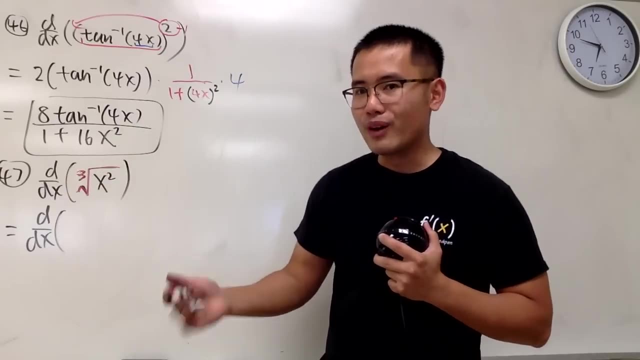 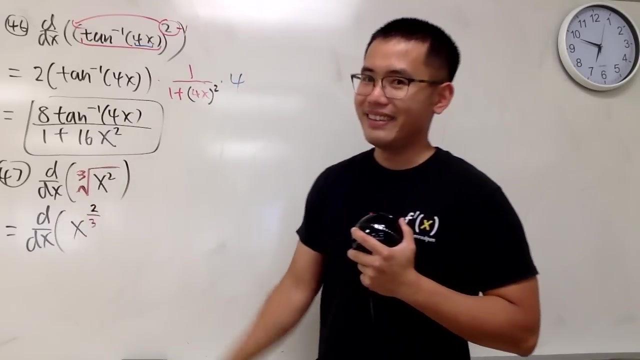 You just have to differentiate. Remember, whenever you have the index here for the radicals, You can write that as a power. So you actually get x. This 2 is right here and then over 3 for the. for the seriously. 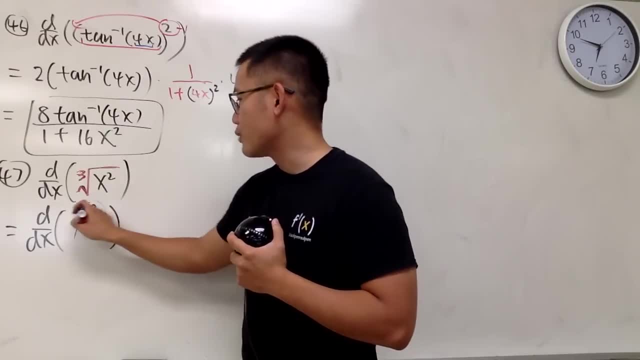 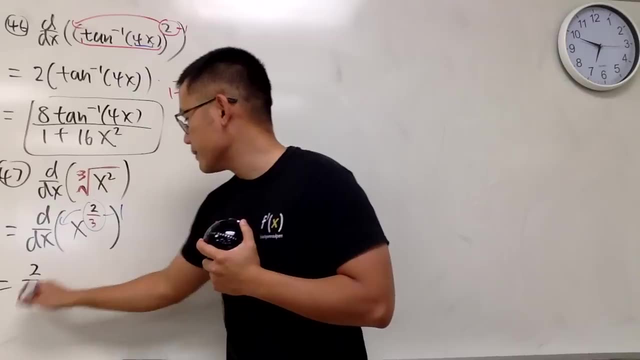 Then we can use the power rule or the power rule, Power rule, I don't know. Anyway, here we go. We get 2: 3rd x. 2 3rd minus 1 is negative 1: 3rd, like this: 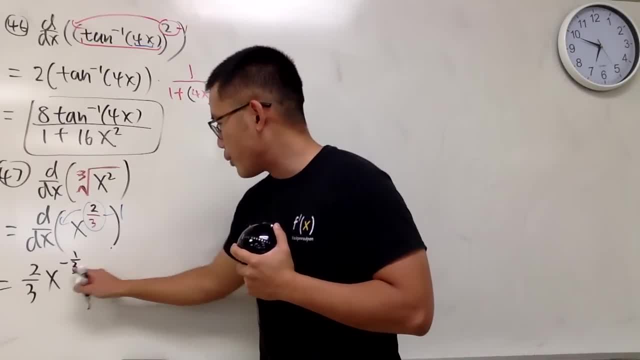 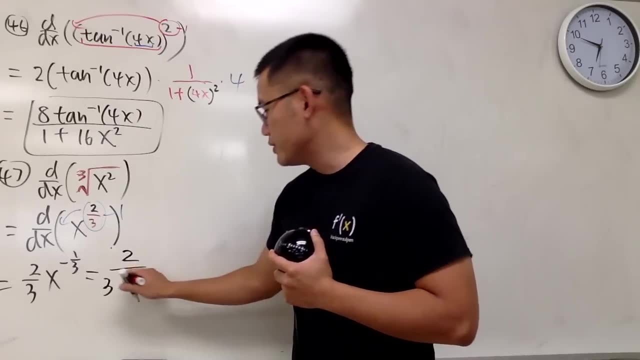 And I rewrite it. I brought this down to the denominator, so we get 2 over 3. x to the 1 3rd, which is the same as cube root of x. x to the 1 3rd, just like that. 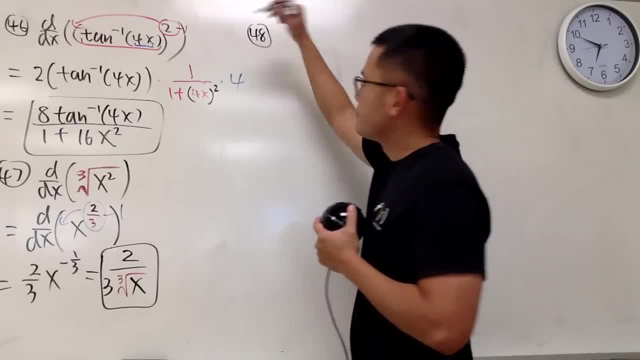 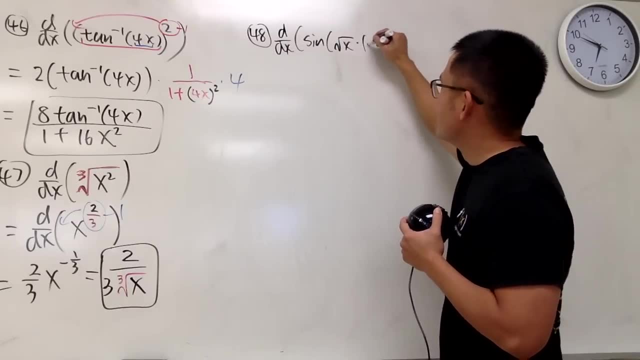 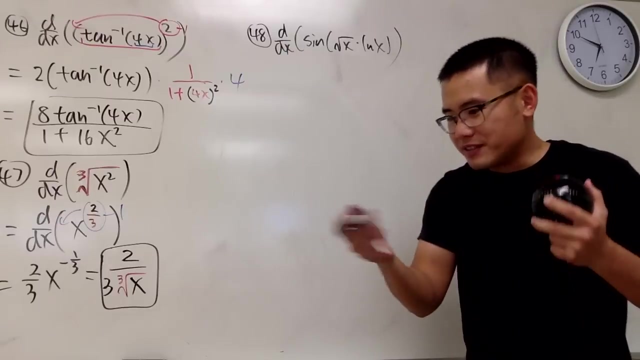 Good, All right, number 48.. Another interesting one: d, dx. Here we have sine of square root of x times natural log of x. Whoo hoo. My question is: can we find the derivative of some function that will give us this for the answer? 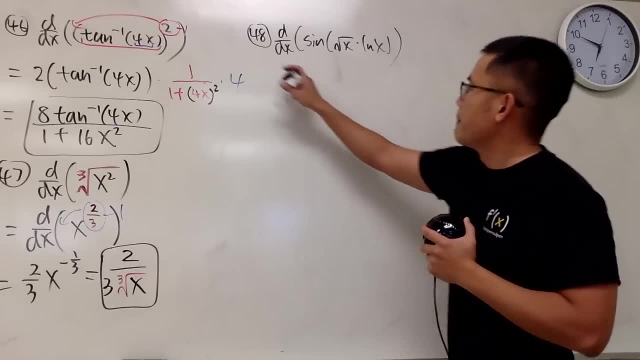 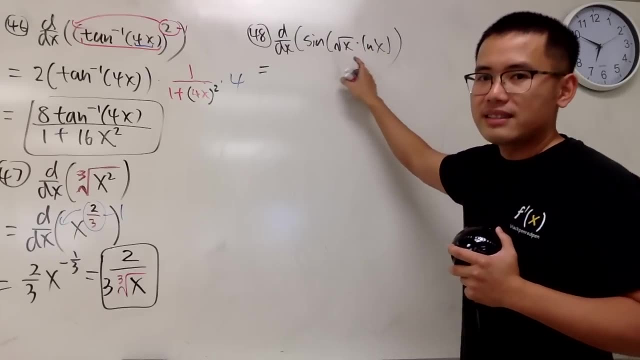 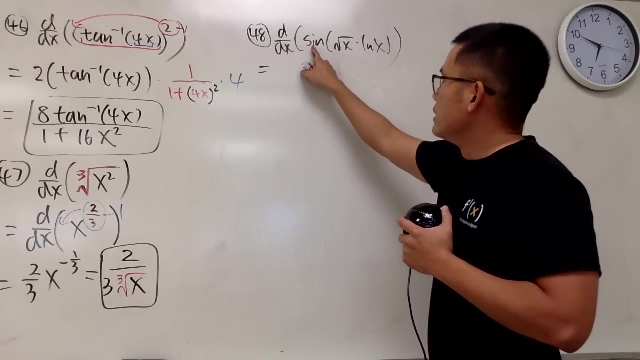 Maybe find the integral for that, I don't know. Anyway, here we go. Sine is the outside function, Both of them are inside. It's not sine: x times square root of x times natural log of x. no, Sine is the outside function, times this thing, this 2, inside. So what we do is differentiating cos this, this, that's the answer: differentiate sine. 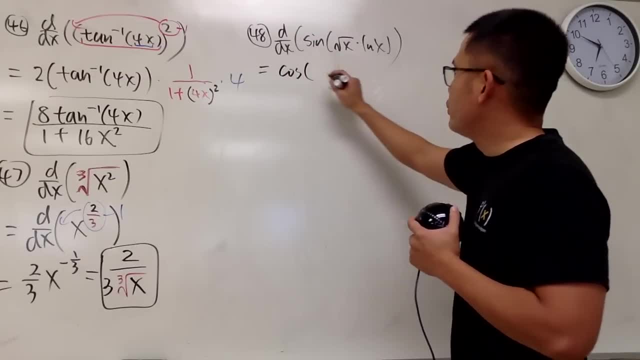 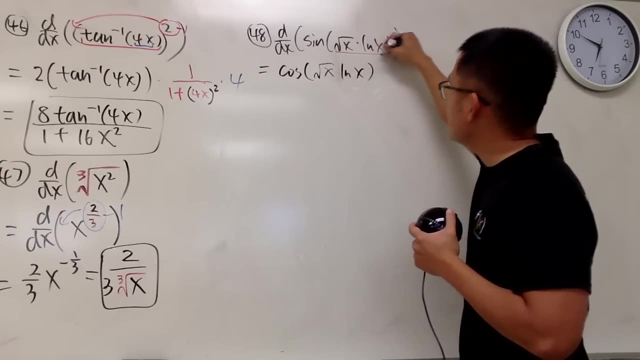 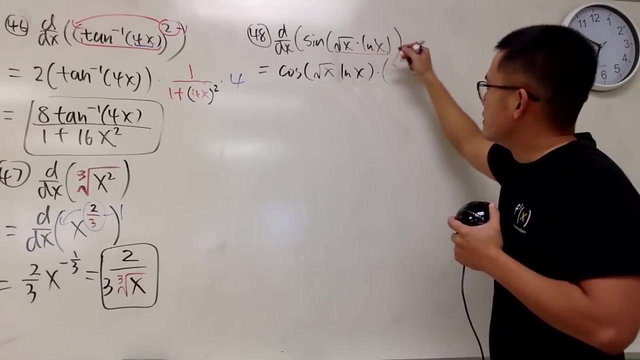 first, which will get cosine and the input states the same square root of x times natural log of x, like this, and then multiply by the derivative of the inside. Okay, we need a product rule in action, so we will do that Derivative of the inside, we'll keep the first. 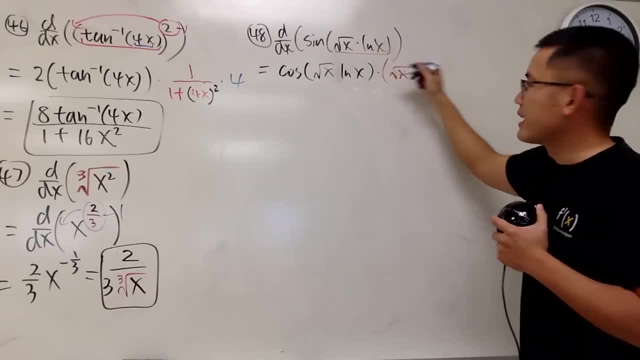 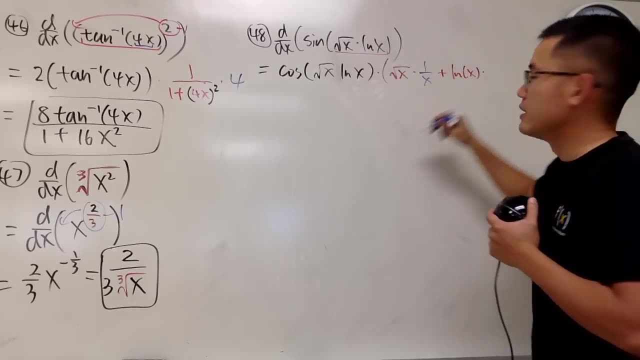 function, which is square root of x, times the derivative of the second, which is 1, of x, plus the second function, which is natural log of x times the derivative of the first, Which is 1 over 2, square root of x, like that. And now we just have to simplify this. 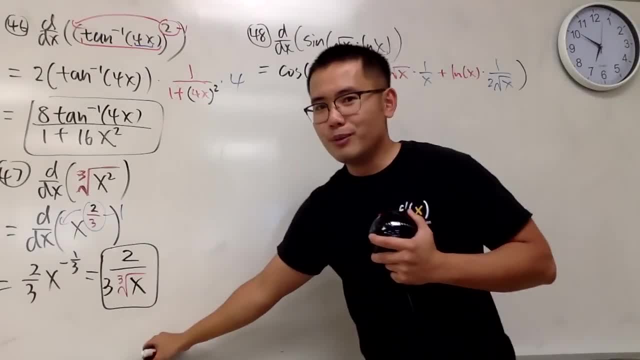 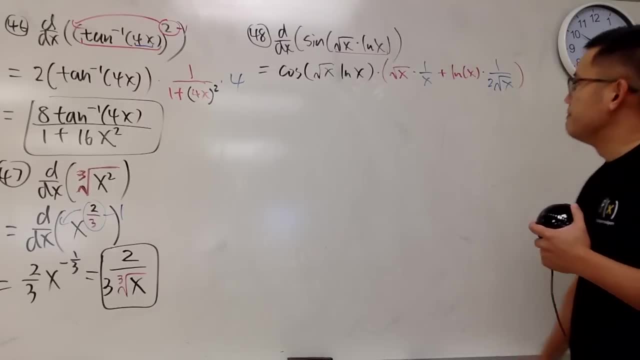 expression. I almost didn't want you to say Shopify, but like that doesn't even make sense Anyway, hmm, let's see. Well, square root of x over x. we can simplify that to be just square root of x in the denominator. 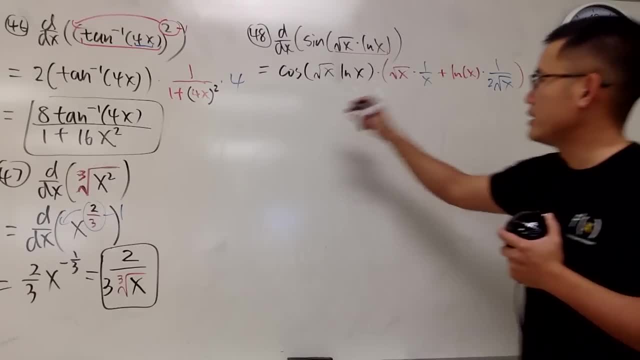 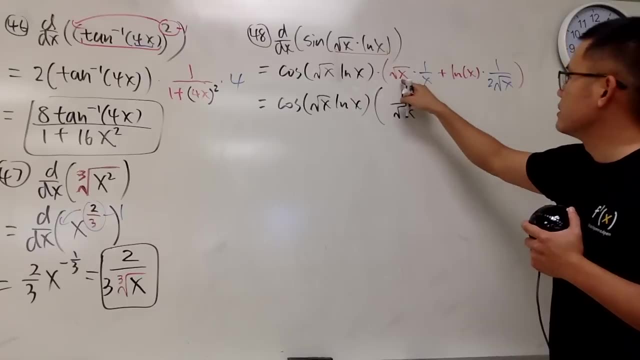 So I think I will just write this down again: Cosine of square root of x by natural log of x. Again, this is just 1 over square root of x, right, Yeah, You can do whatever you want to simplify that. This is x to the 1 half power over x to the first power: 1 half. 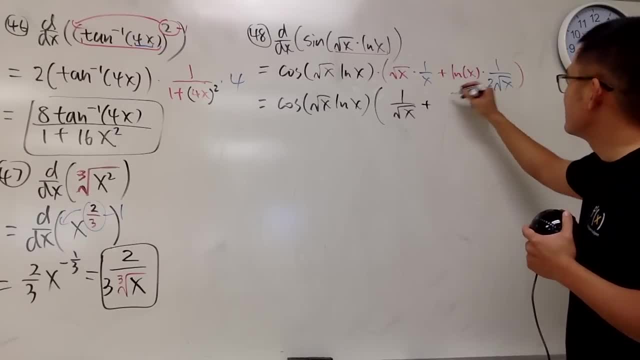 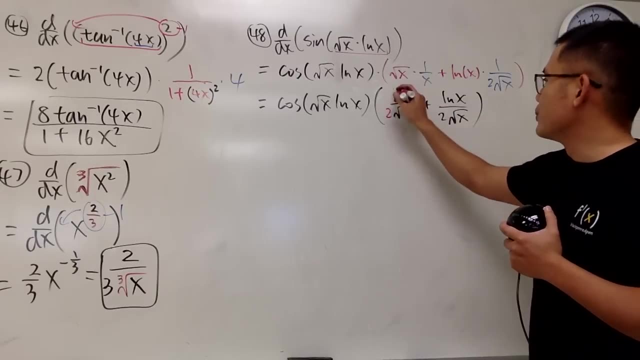 minus 1 is negative 1 half. so you have this, okay, Plus natural log of x over that to square root of x. Ah, so this is So. it's clear. now We just need a 2 right here, Multiply, multiply, So finally the. 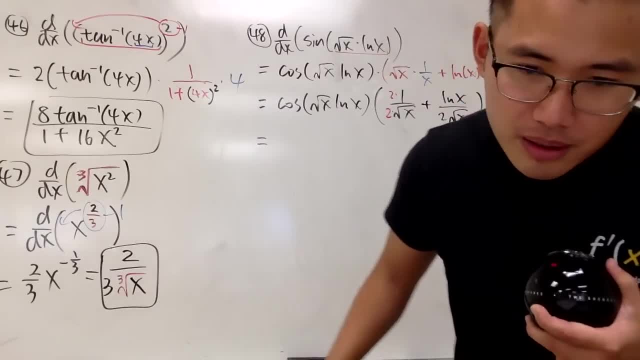 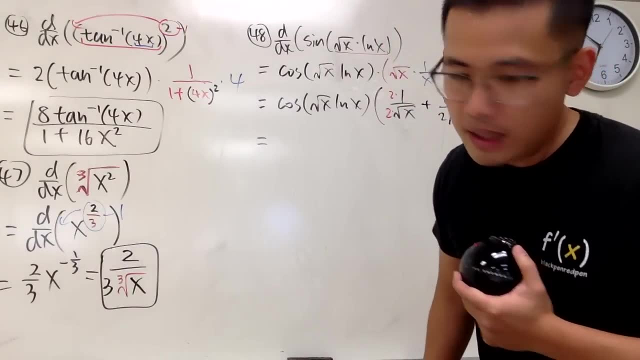 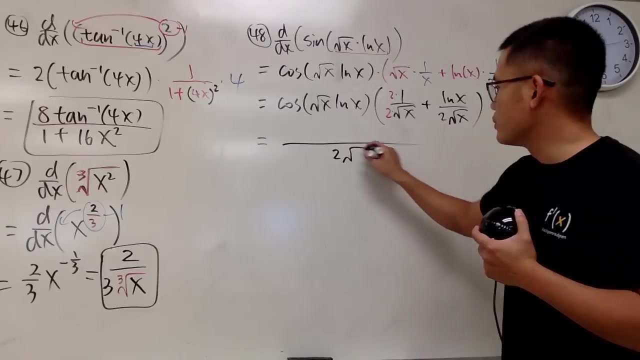 answer is: did I put that on the top as well? I certainly did, And I will do that as well. I put on this first, though The denominator is this, which is 2 square root of x, And for some reason I put on this first, I think, because I just want to tell you guys this. 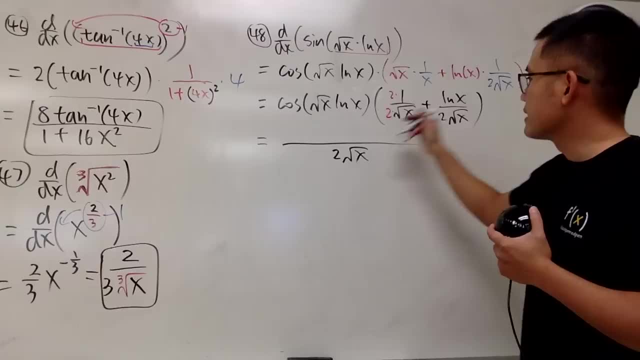 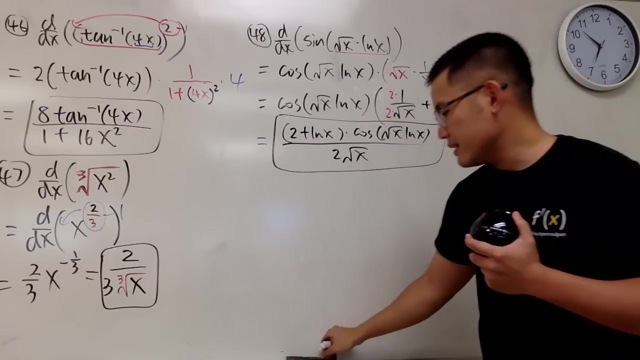 is the only thing inside of the cosine. So let me emphasize that by putting 2 plus natural log of x, first times cosine of square root of x, natural log of x like that. So this is the input for cosine, In fact, in 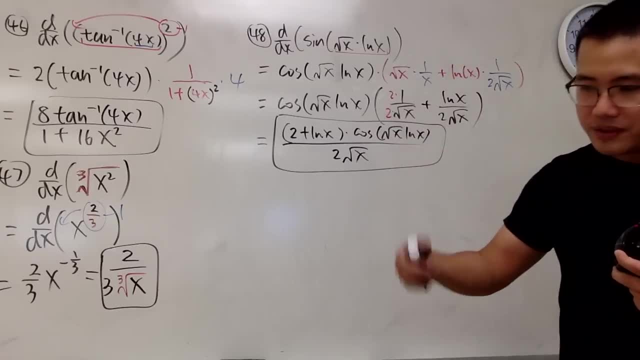 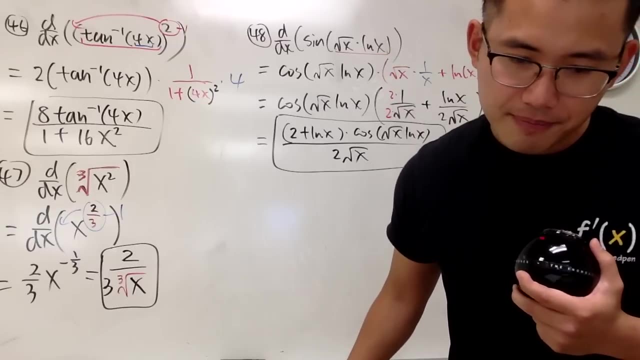 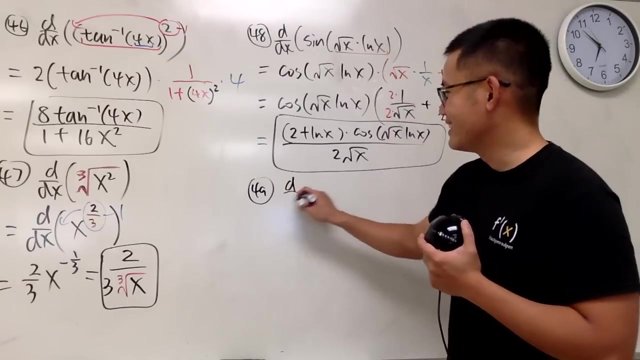 differential equation, you will see this kind of function: cosine of square root of x times natural log of x, all that stuff Okay, So that's good. Number 49.. All right, Number 49.. An easy one. ddx or csc? not really, though, but like you just have to do it carefully, it will be easy. 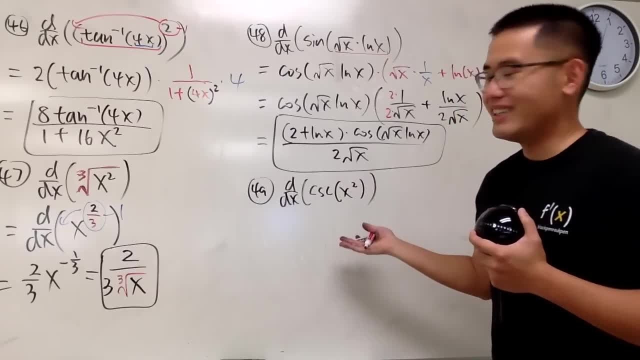 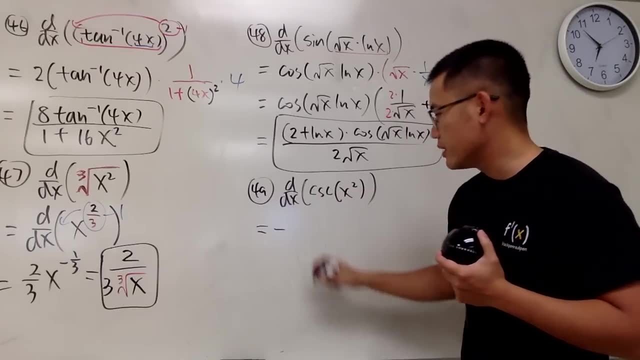 It's actually pretty easy actually: Csc, cosecant of x squared. so there we go. Differentiating cosecant, we get negative cosecant cotangent, so csc. but don't forget the input has to stay the same cotangent. 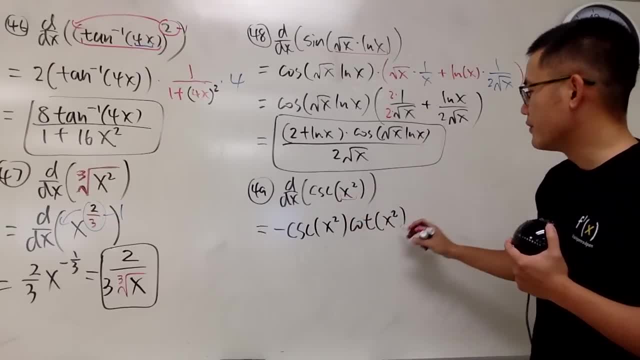 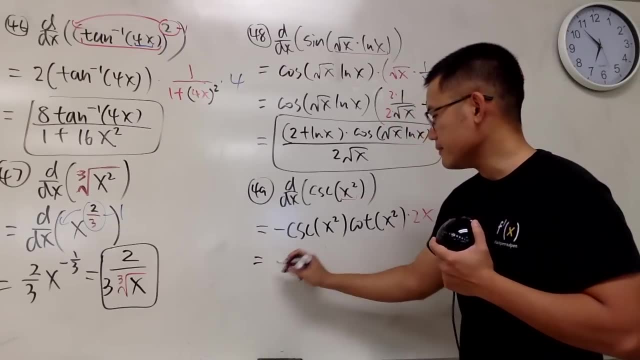 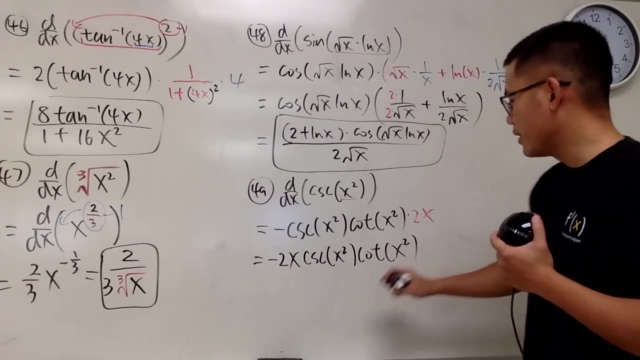 And then do what? Well, channel the derivative of the inside 2x. in the end, put the 2x all the way in the front. Negative 2x times all that: csc x squared, cot x squared. 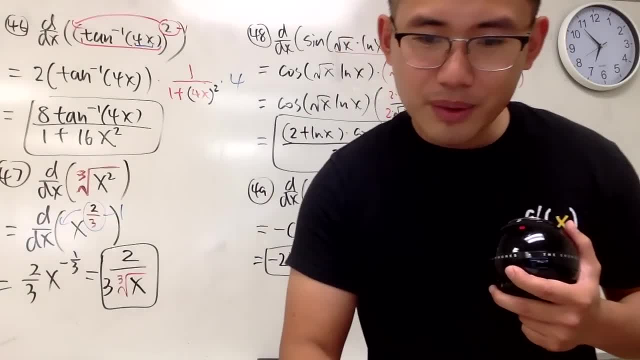 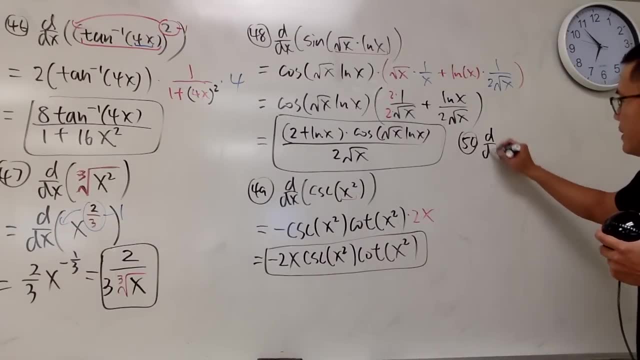 Done. Whoa, look at that, How easy that was. right Number 50, can I fit in number 50?? I will fit in number 50 right here. As I said, I like to fit in a lot of. 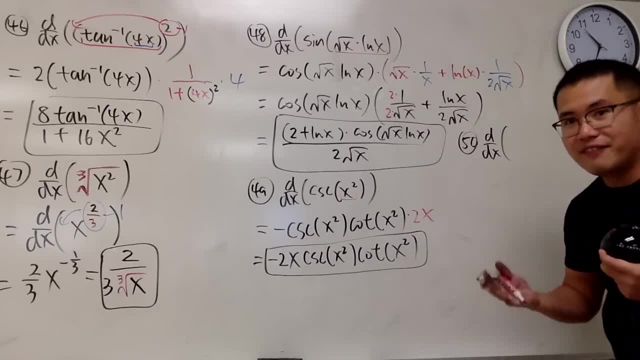 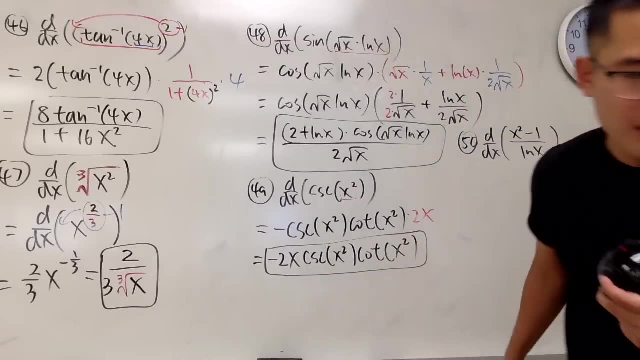 things onto one board, one scratch of paper, and that feeling is really good. okay, That feeling is just really really good. It makes me really satisfied. I know some of you guys are like me too. I think so. Anyway, here we go. quotient rule. 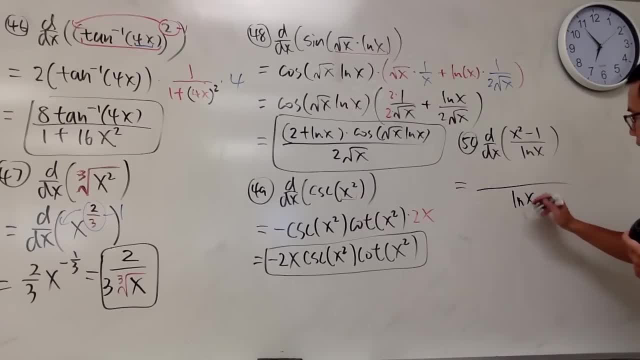 So, square the bottom function, natural log of x. square that guy bottom function is natural log of x times the derivative of the top, The derivative of the top. So the top is 2x and then minus the top function, which is x squared minus 1,. 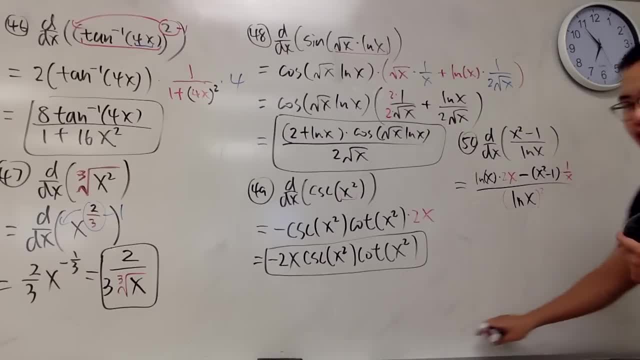 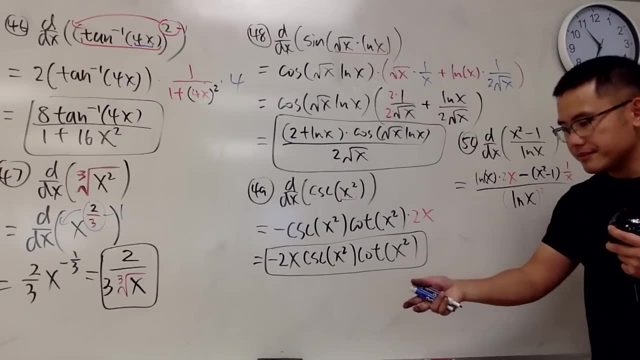 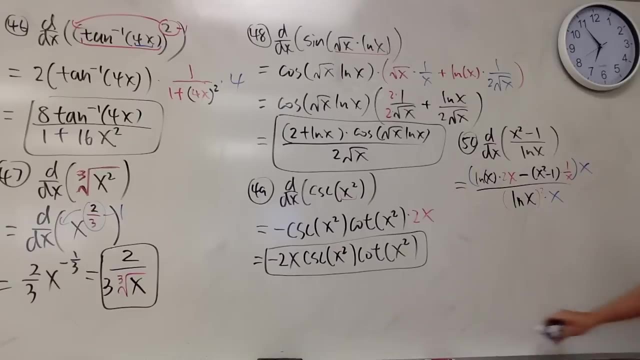 times the derivative of the bottom, which is 1 of x, just like that. Well, you can distribute, but you are going to get complex fractions. so let's just multiply the top and bottom by x, so we can reduce that right. 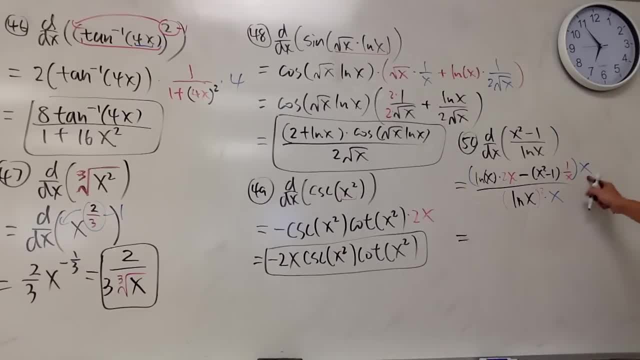 We can simplify that a little bit. In the end, x times this, x times this guy, of course we will get 2x squared and then we have the natural log of x, like that, And then this and that cancel, so you can just distribute the negative nicely. 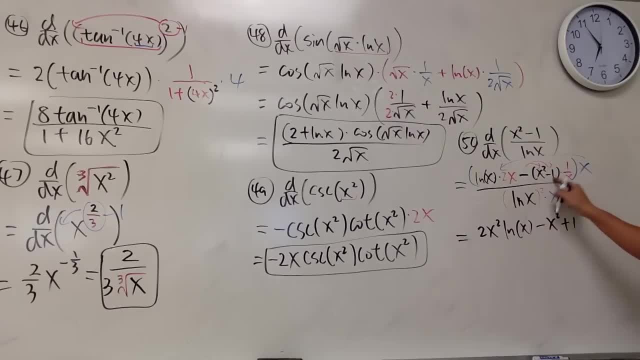 so we have minus x squared and plus 1, okay, Plus 1.. All over x parentheses. natural log of x squared Done, Okay. Oh, by the way, for the people who don't know, I work from Alpha. 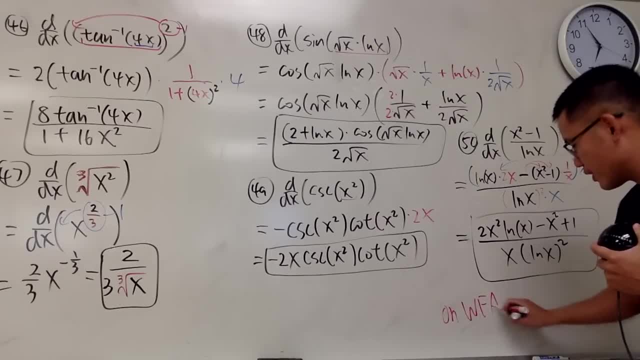 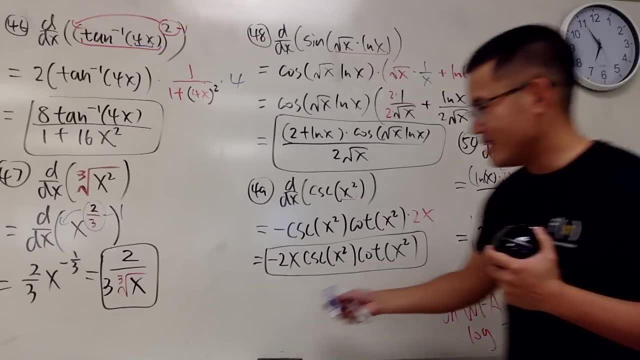 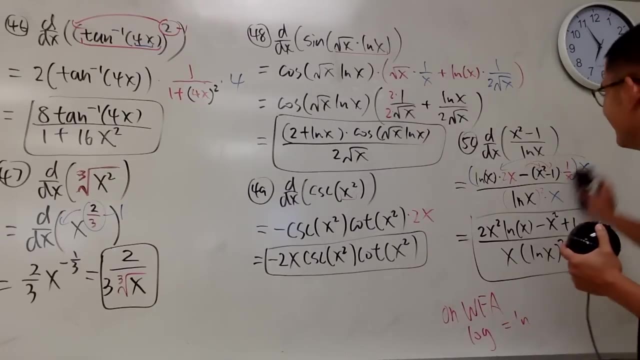 When they say okay, Wufang alpha, When they use log okay, they mean natural log, okay. So if you are doing your calculus problems on Wufang alpha, get used to this notation. Anyway, that was number 50.. Oh my god, halfway done, So it's going to take. 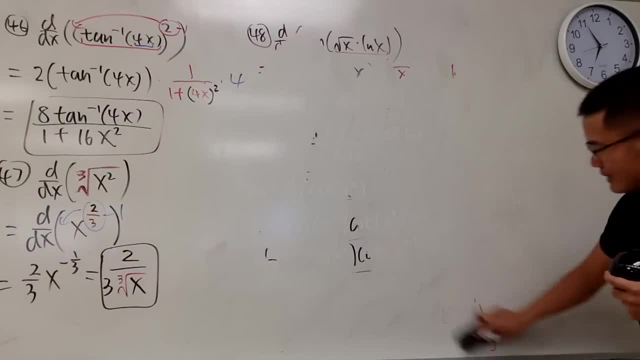 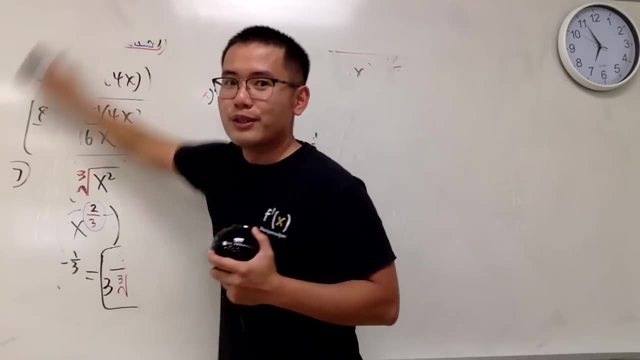 me about six hours or something, and I'm afraid of the last ten questions because, to be honest, they were. they are the definition questions, so I don't know how long it will take. God man, this is taking longer than I. 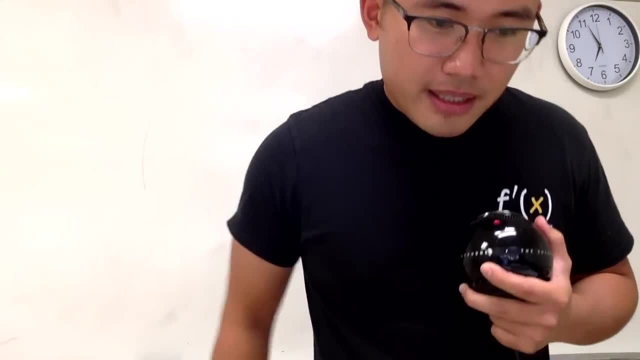 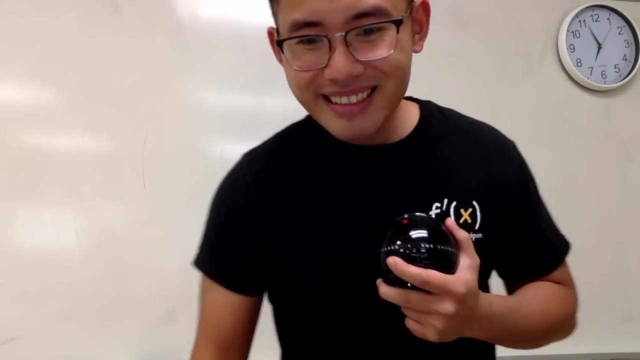 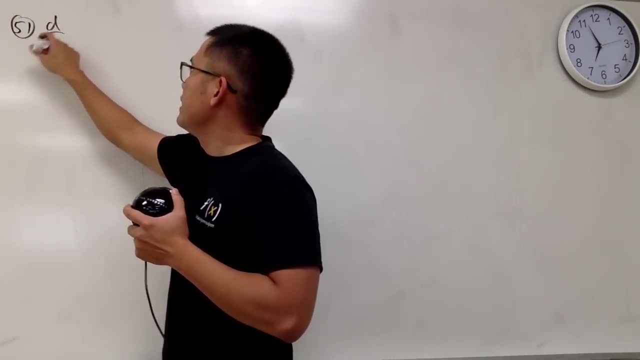 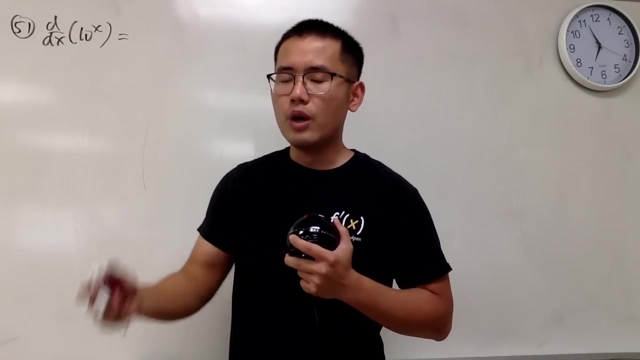 expected. I don't know. Hopefully I have some easy questions coming up. Yes, I am having some nice questions coming up. Number 51. Differentiating 10 to the x. Now you have two ways to do it. One way is just know how to differentiate. 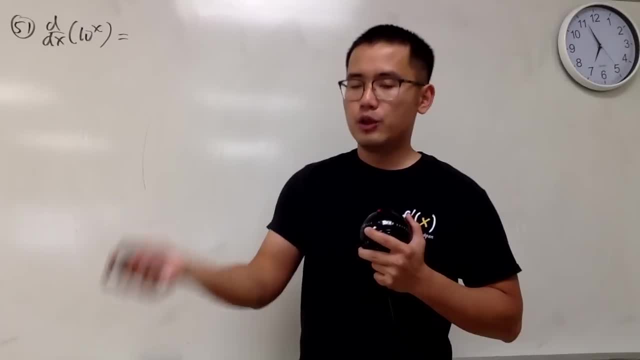 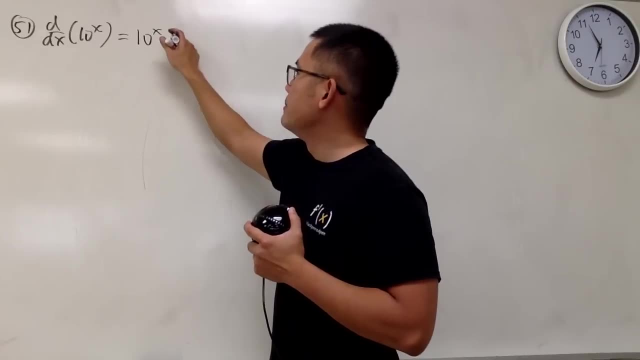 any number, any number, okay for the base raised to the x power. In that case, if you remember that, it's just 10x: 10 to the x power, 10 to the x power. times natural log. 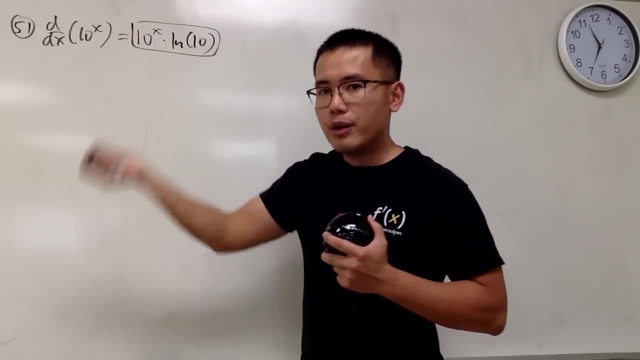 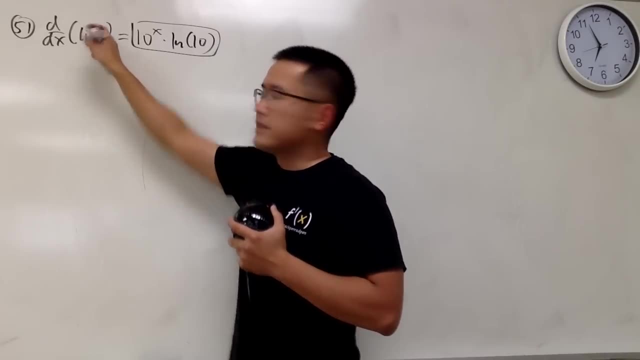 of 10.. It's just always the number to the x power times natural log of the base. And of course you can check the chain. the derivative of x is just 1, so multiply by 1.. It's the same thing. This is the idea And the reason why this is true. it's because 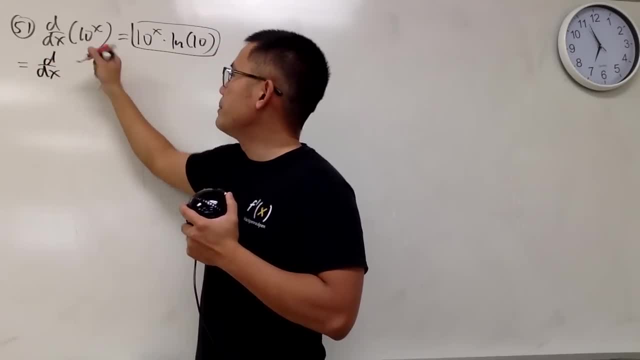 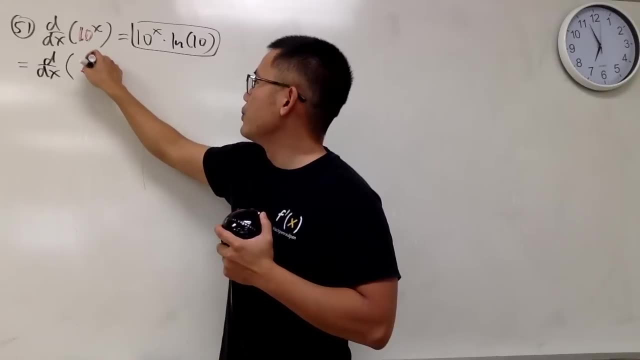 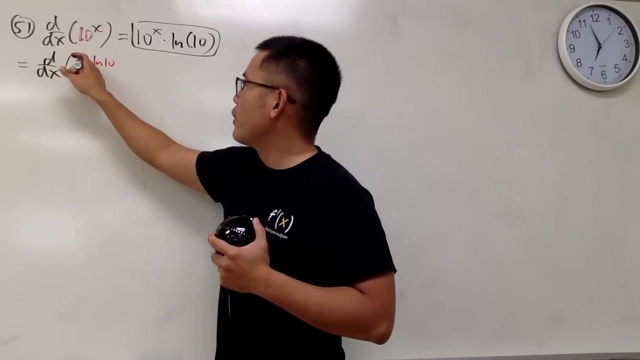 we can look at the 10 as the follow: Remember, ideally speaking, we like to work with space e, So we can look at the 10 as e to the base, I mean e to the ln 10.. This is 10, okay, And, of course, 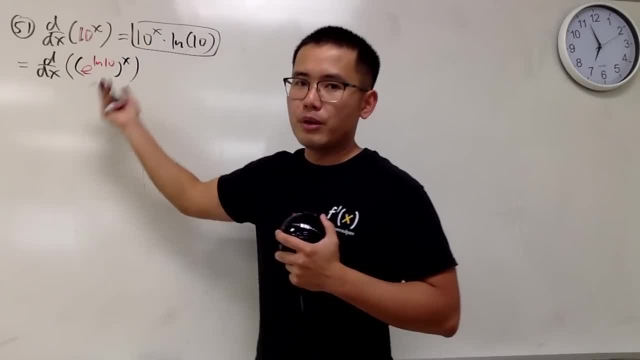 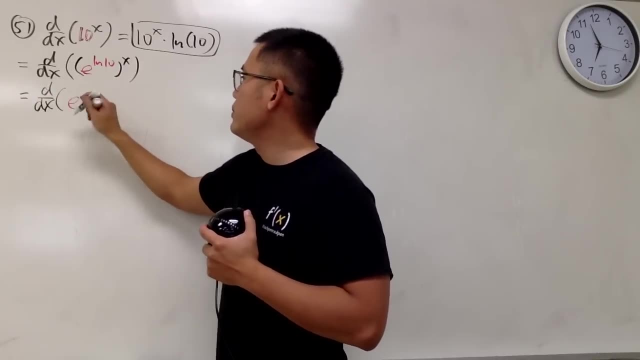 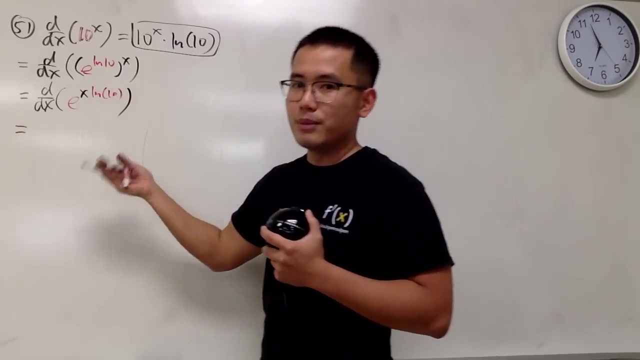 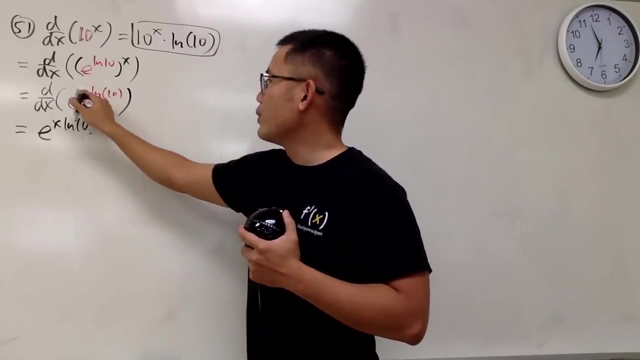 this right here: multiply, well, raised to the x power, and you can multiply the powers and you will get d, dx. This is e to the x times natural log of 10, like this, And this is very similar to the equation we did this right here: You just get e to the x ln, 10, times. now we have. 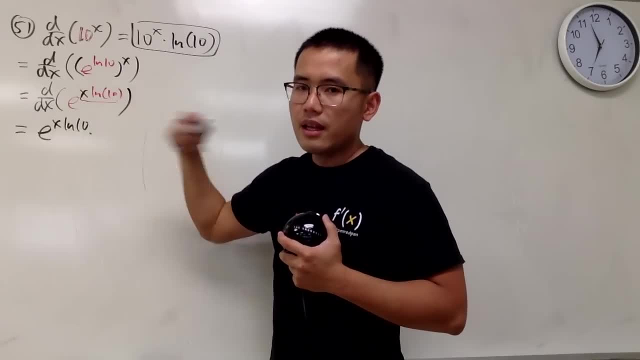 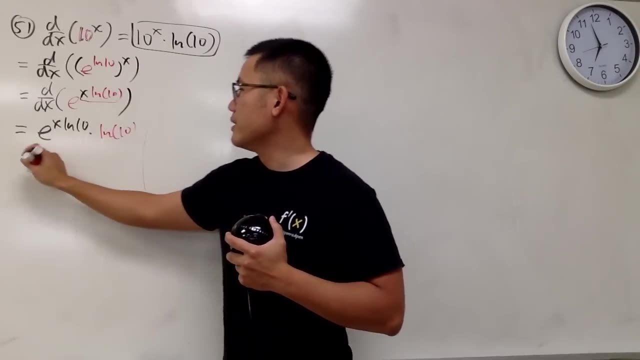 to do the chain loop. The derivative of x, ln 10, ln 10 is a number times x, so you just multiply by ln 10, like this, And this right here is just 10 to the X power. that's how you get the L and 10.. 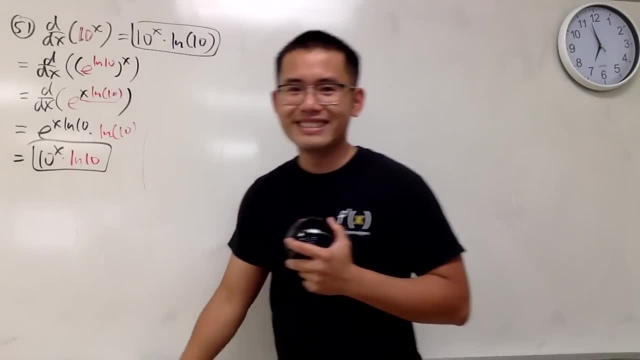 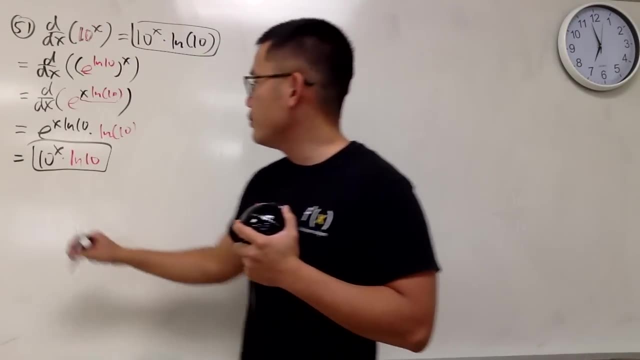 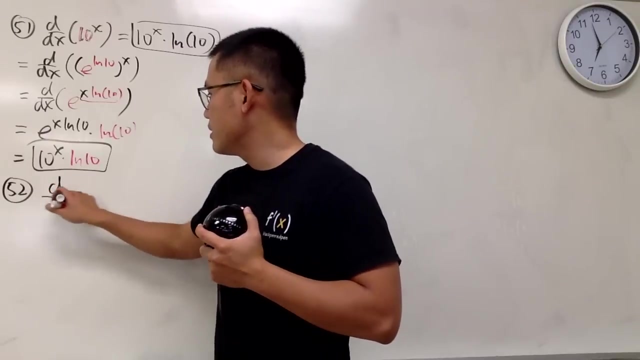 Okay, like that. Okay, number 52.. Number 52.. Number 52,. your order is ready. Please come to the window and pick up your order. I don't know why I'm saying things like that, but whatever, I just did. 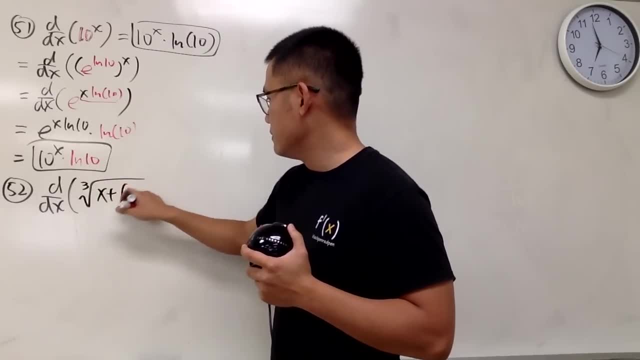 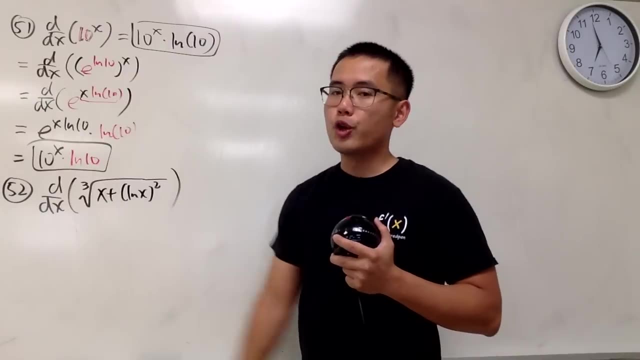 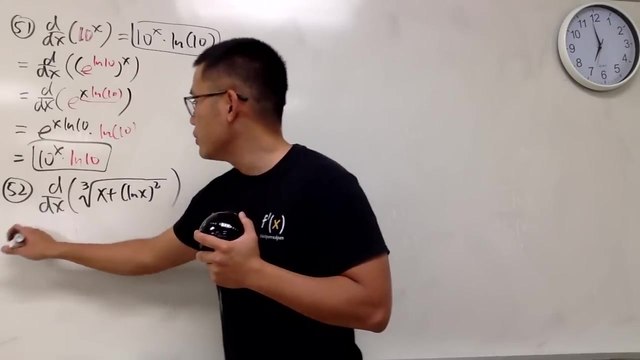 So we have this. Okay, so this right here, it's a cube root. Maybe we are not familiar with a cube root, but, okay, we can write that as the one-third power, So we will do that. Therefore, we are just going to differentiate. 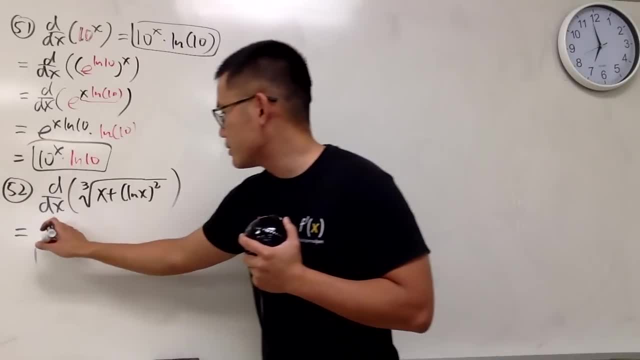 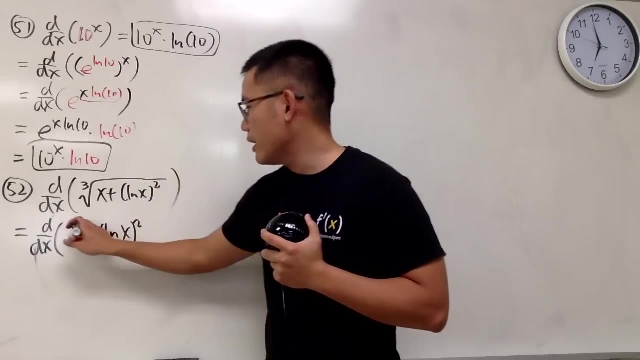 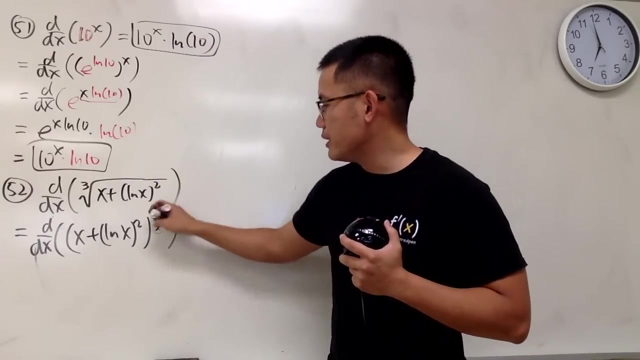 Actually I will. Yeah, I'll just do it here. We'll differentiate: Inside is X plus natural log of X to the second power, and then we raise this guy to the one-third power. Well, power rule in action: put this all the way in the front and then minus 1.. 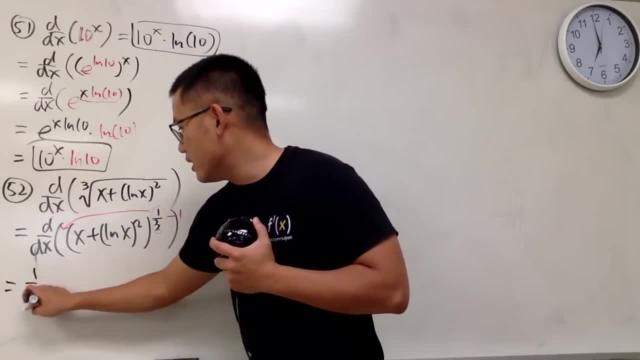 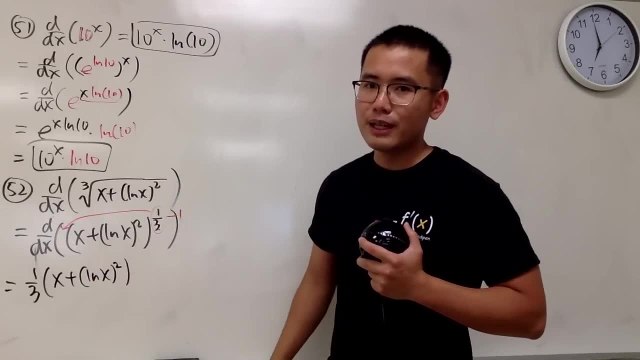 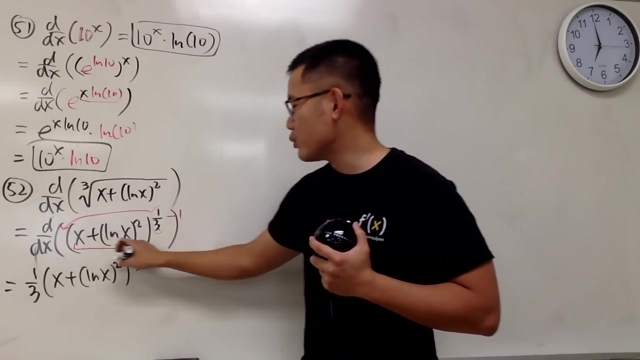 So we see this is going to give us one-third parentheses. inside states the same X plus natural log of X squared. What's one-third minus 1? Negative 2-thirds. So you just have negative 2-thirds here and you multiply by the derivative inside. 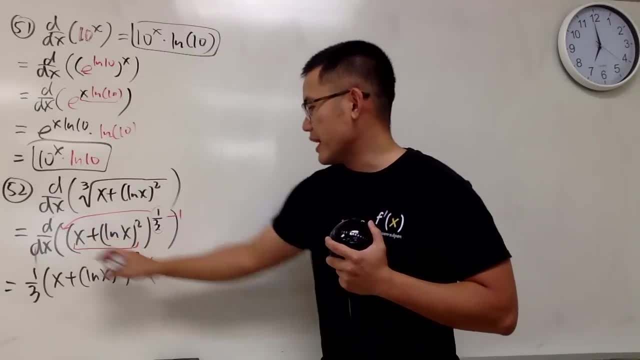 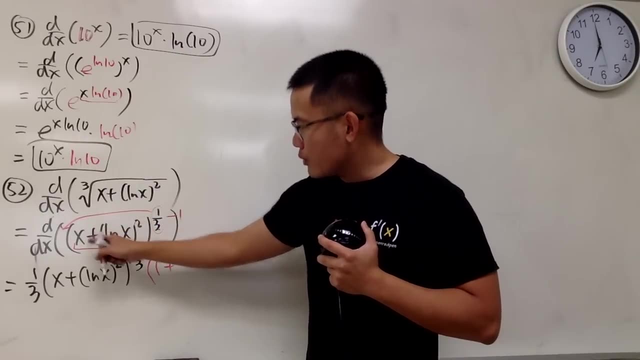 Okay, yes, two things. so be sure you open the parentheses. derivative X is 1 plus the derivative of this. Well, we need to use the power rule again. bring the power to the front, which is 2, inside states the same. 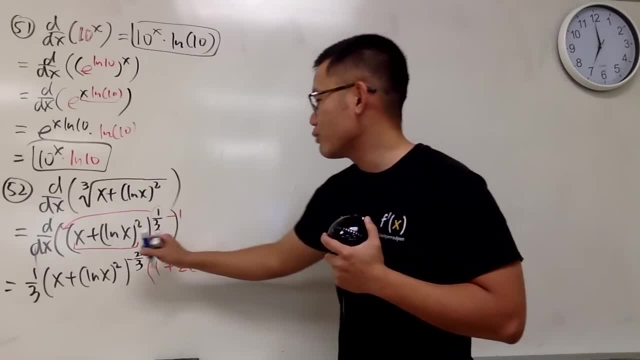 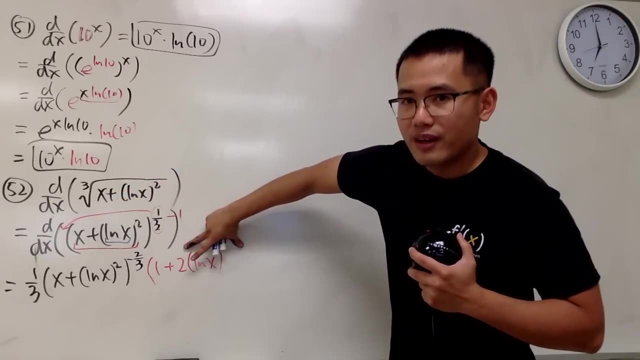 2 minus 1 is 1, but Chengdu says we have to multiply by the derivative of this guy. just to this, though, Because this guy has the derivative right here. So do not close the parentheses. do not multiply 1 over X with the whole thing. 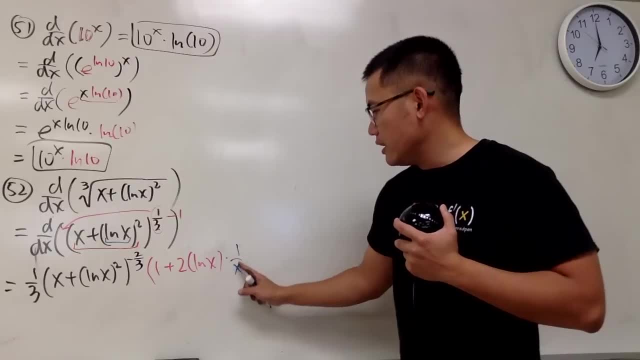 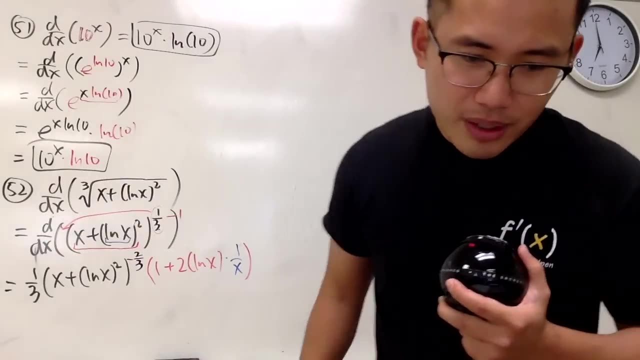 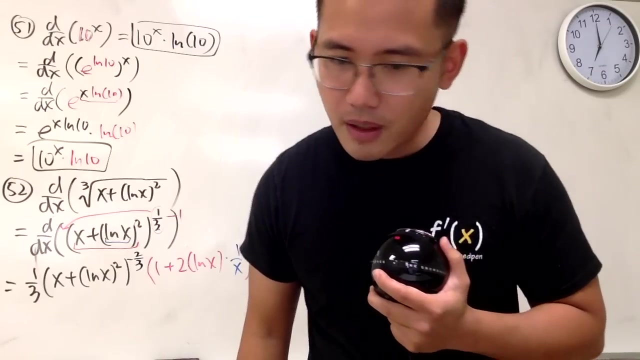 The 1 over X, which is the derivative of natural log of X. it's only for this part, So you have to close the parentheses like this, right? And how do you write the answer? This is not, Oh, okay. 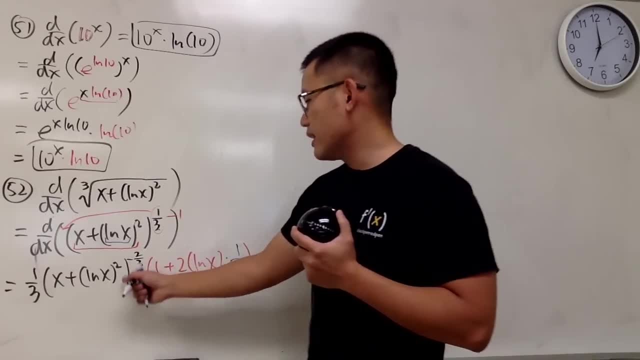 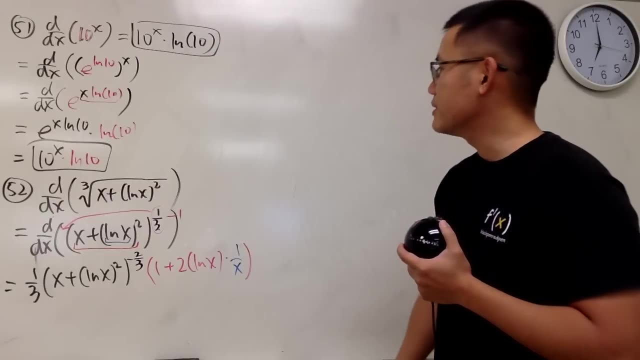 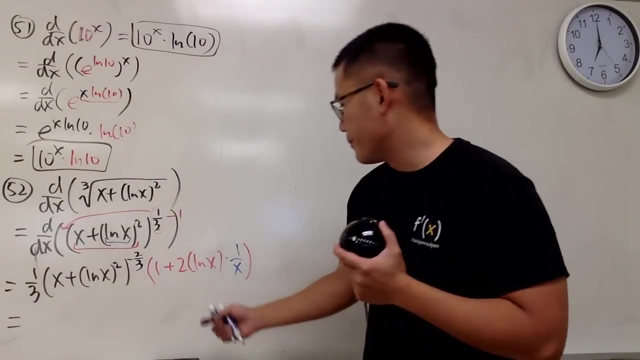 Hmm, we have to Bring this down to the denominator and just do the usual clean-up, because we'll end up with a complex fraction, And I will. I should have more space here. Okay, here we go. This right here is on the top, so I will put it on the top. 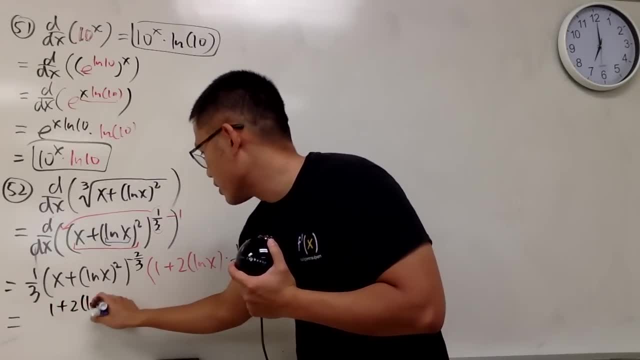 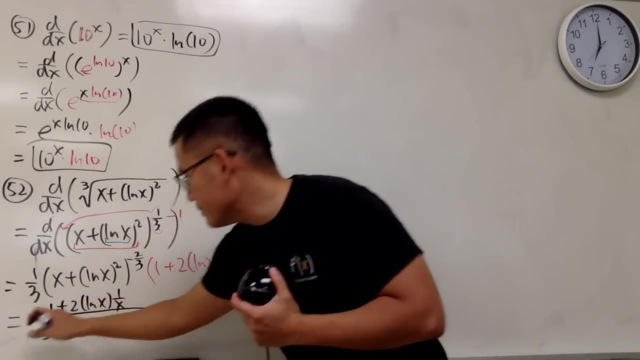 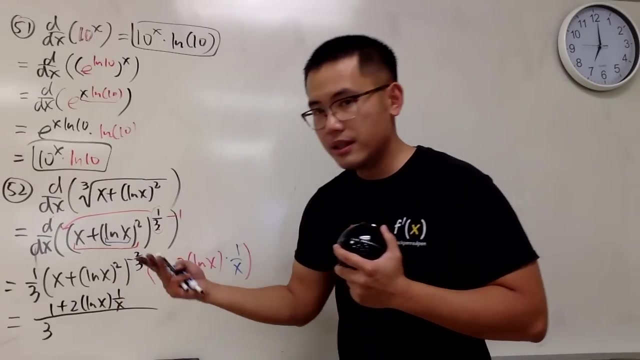 1 plus 2. natural log of X times 1 over X right. Just bear with me right here for now. Over 3 on the bottom. This guy is also on the bottom Negative right, The 3, it's the cube root. 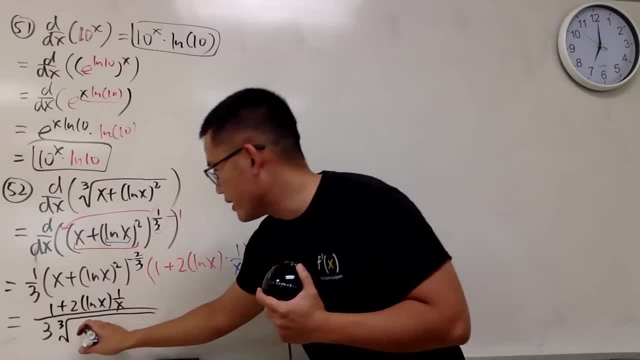 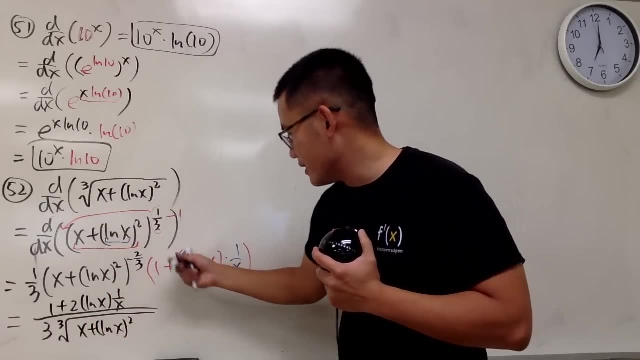 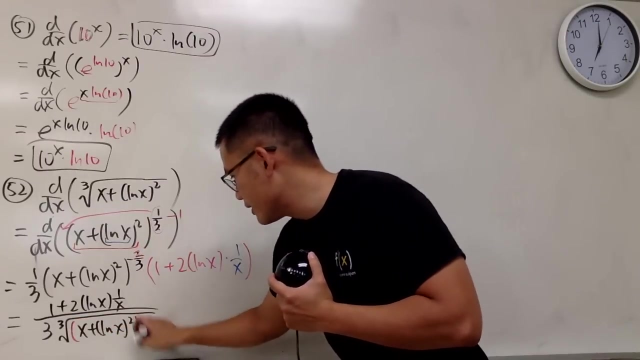 So we have the cube root Open that And this right here, X plus natural log of X. This right here has a square, But don't forget, we still have this square here. So perhaps I will make this 2 red and I will square this guy red like this. 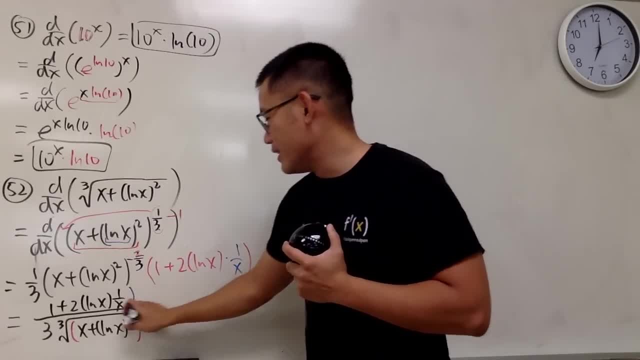 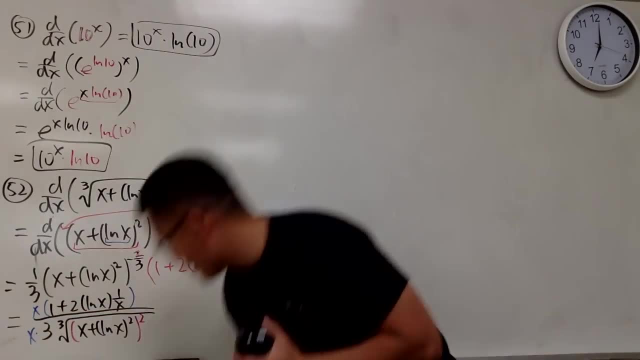 Well, well, As I said, we have the 1 over X here. Let me multiply by the X in the front this time, Because if I put it at the end, it looks like it's itself a square root. I mean the cube root. 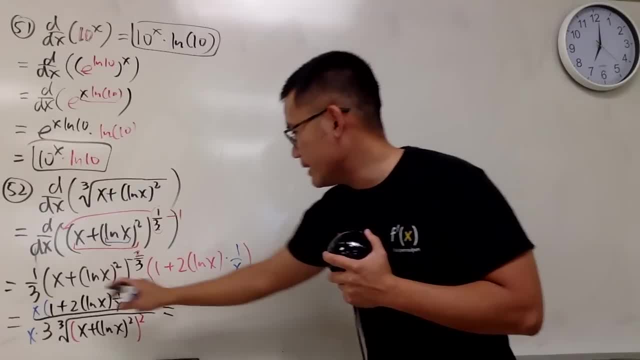 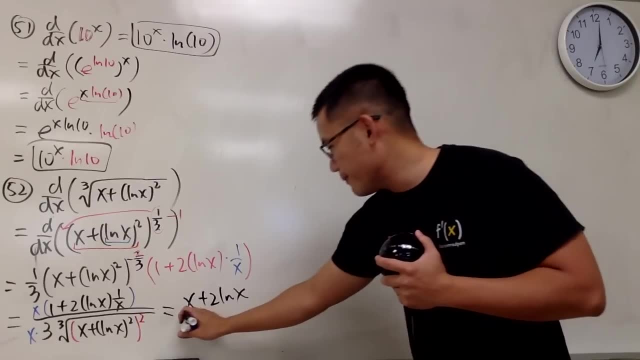 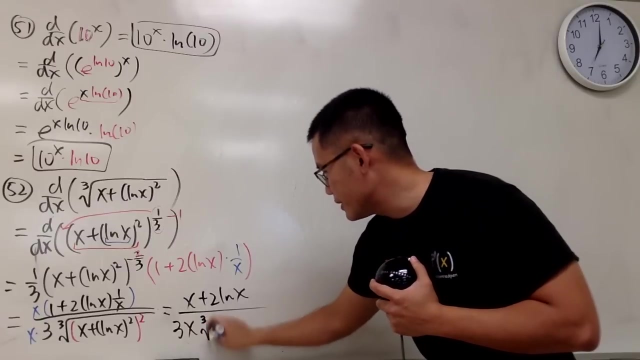 But it's not. Anyway, multiplying in we get X. That cancels. so we just get plus 2 natural log of X, right, And 3X. I'm seeing you guys are okay, huh, 3X and then the cube root of X plus natural log of X. 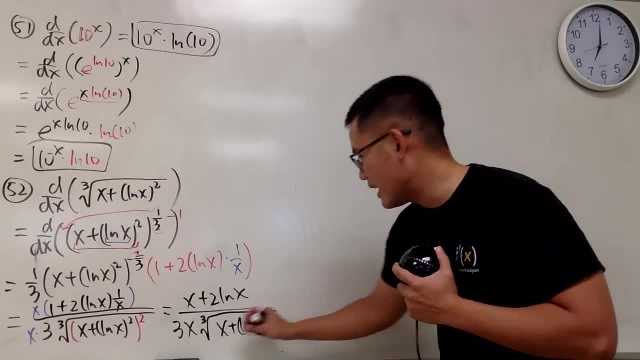 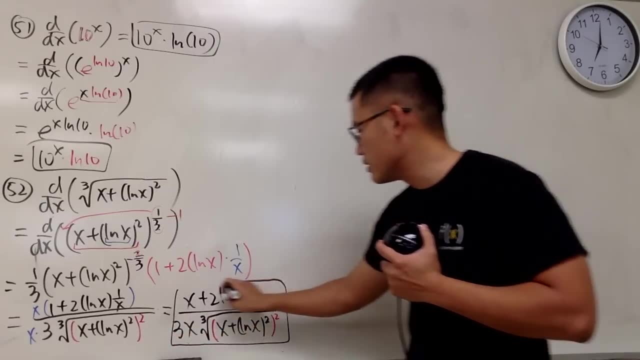 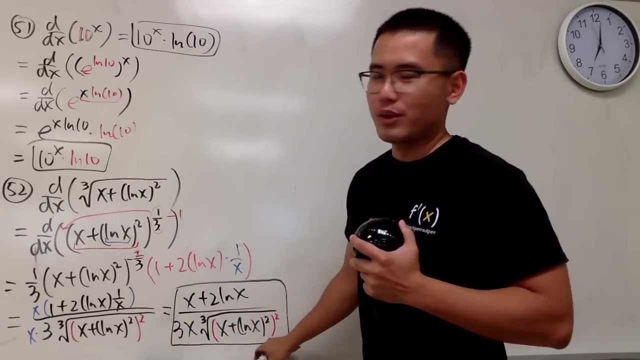 Okay, So this guy's square, and then this guy, the inside guy, is square as well. So this right here is the answer for that. Okay, pretty good, pretty good, pretty good, As long as it's not like second derivative. 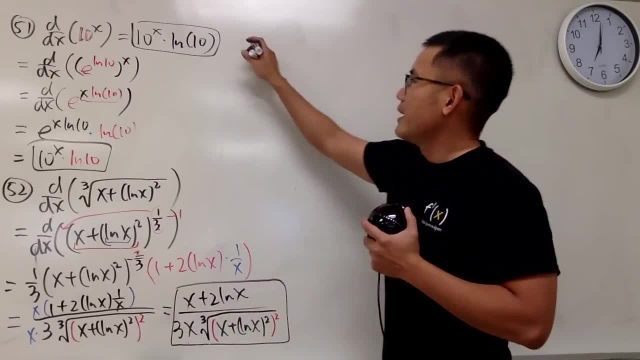 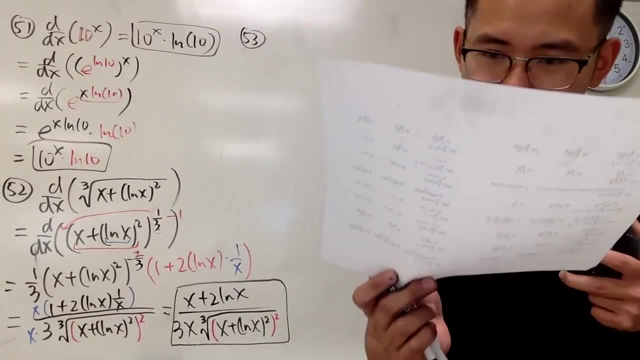 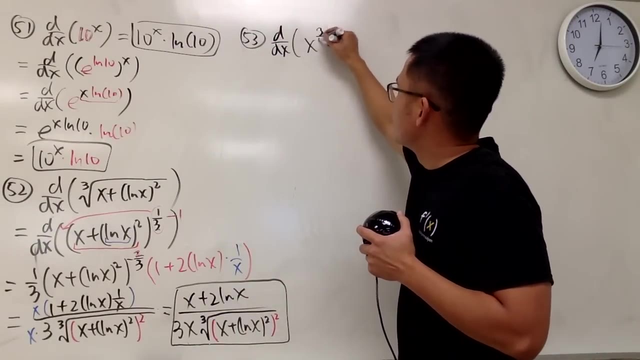 Man, now I don't know why I did that. Okay, number 53.. Ooh, very nice, Just some little power function. Okay, power functions. So we have DDX X to the 3 over 4 power minus. 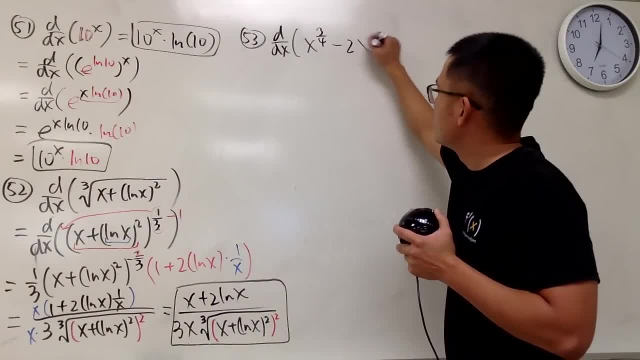 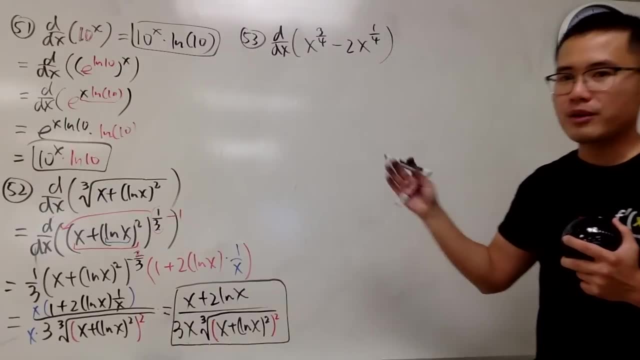 2X to the 1 over 4 power. This right here is actually pretty common if you have to talk about how to sketch a curve, Because you actually get some sharp turn and all that stuff. So you know how to differentiate this. 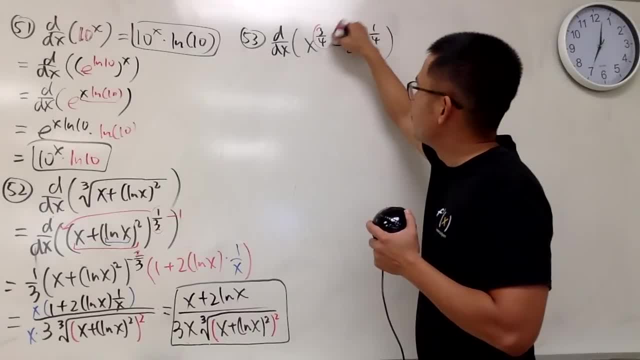 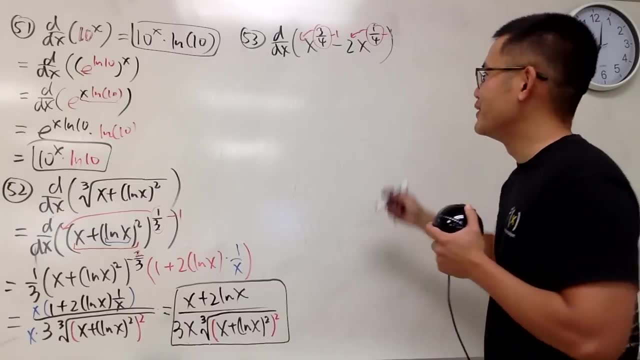 how to find a critical number for this. Anyway, go ahead, bring this to the front. bring this to the front. minus 1, minus 1.. Okay, We have done this question very similar. We have done the question very similar to this one. 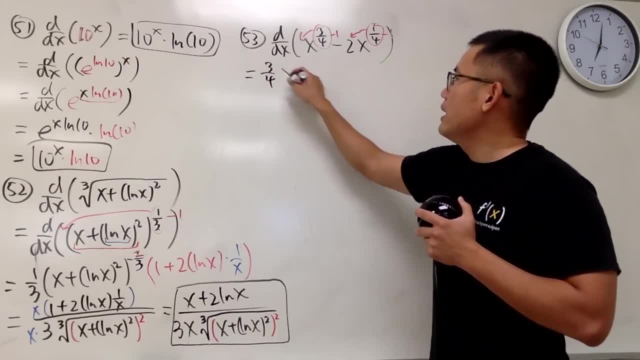 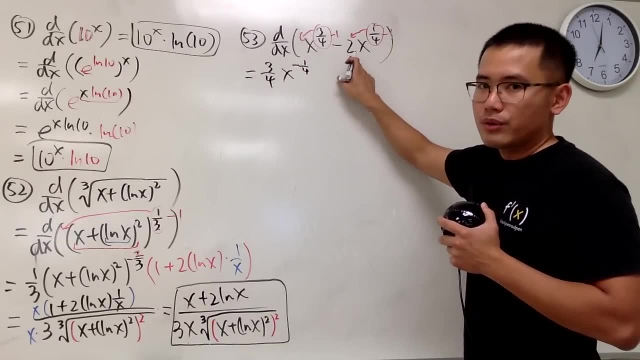 So anyway, we get 3 over 4. X to the 3 over 4 minus 1 is negative 1 over 4.. Okay, negative 2 times 1 over 4, we get negative 1 half, And then 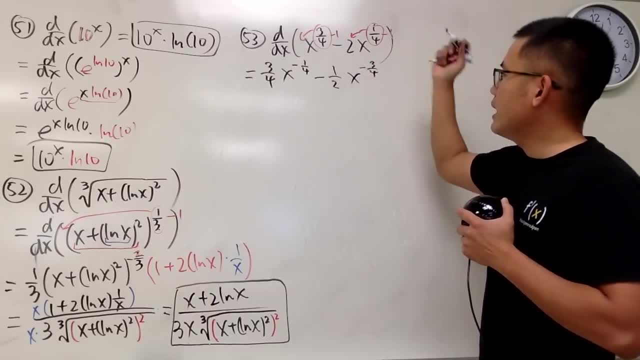 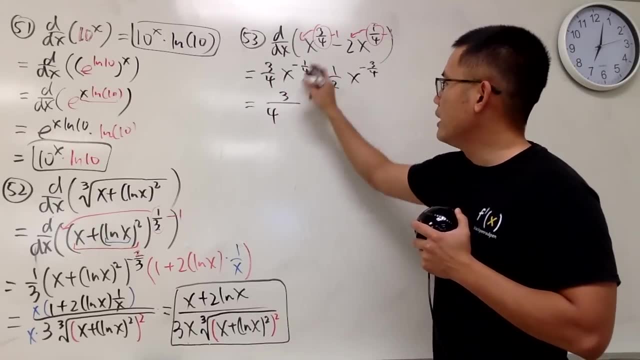 X to the subtract, you get negative 3 over 4, like this: Okay, bring things down to the denominator. So here we have 3 over 4, and this is X to the positive 1 over 4 power. 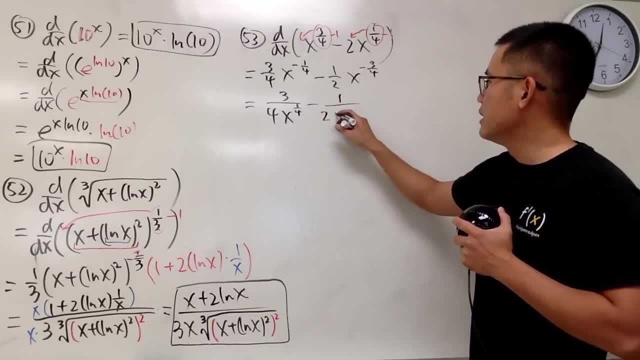 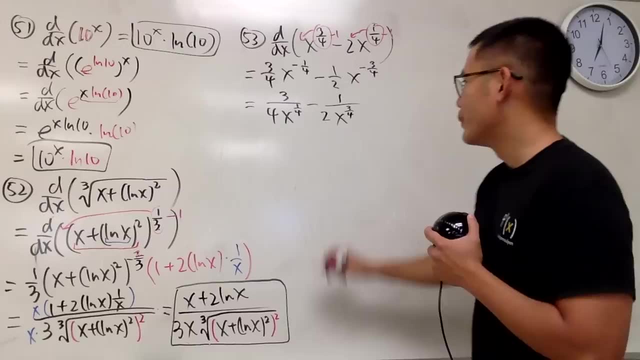 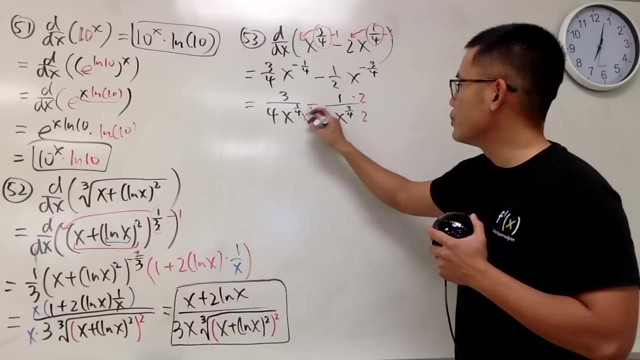 minus 1 over 2, and this is X to the 3 over 4 power. How can we get a common denominator? Well, here I need to multiply by 2, so I can get a 4.. But here I need to multiply by X to the 2 over 4.. 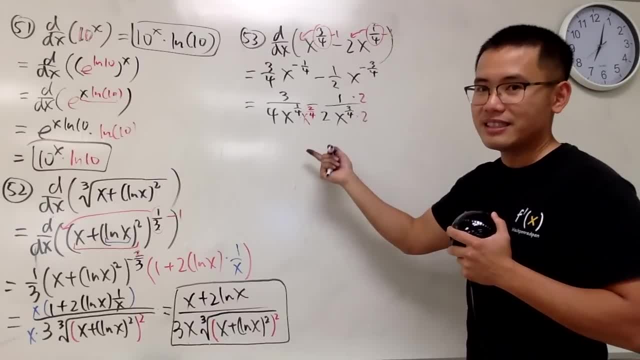 So I can get X to the 3 over 4.. I know that's the same as X to the 1 half. So you know, don't worry, I will fix that. I think it's better this way though. 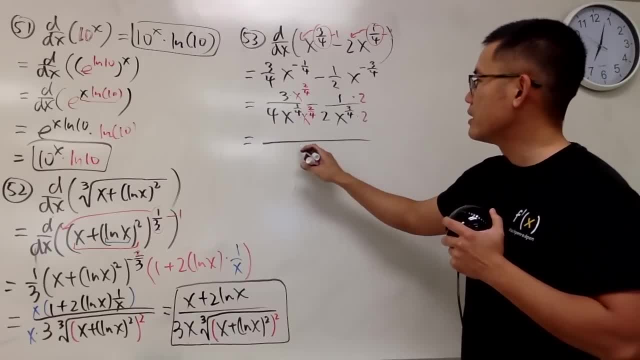 Anyway, when you do that, the bottom has the denominator being just 4, X to the 3 over 4, and then for the top, this is 3.. This guy, it's X to the 1 half Name, the square root of X. 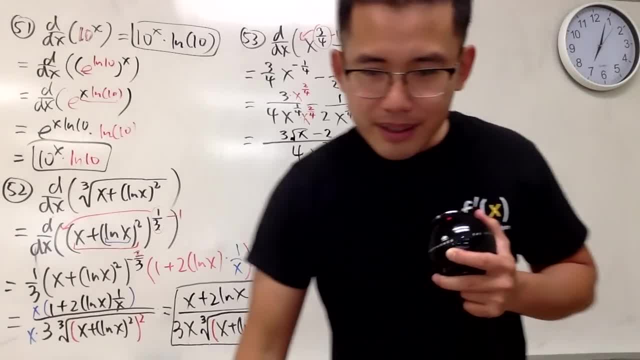 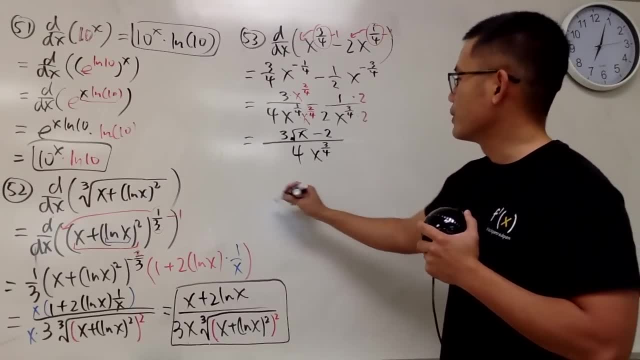 Okay, And then minus 2, like that. And of course I put down the the bottom as a radical as well, So I'll just write it: 3 square root of 2.. Why am I keep using my finger to read this? 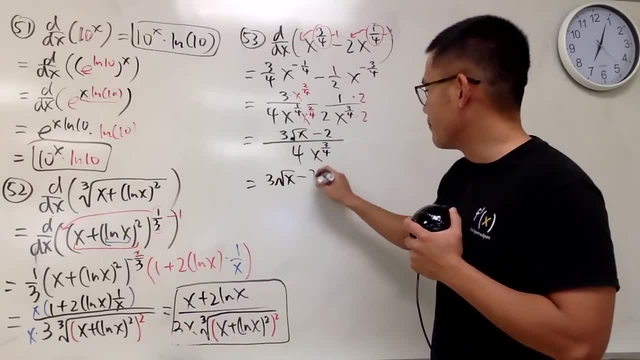 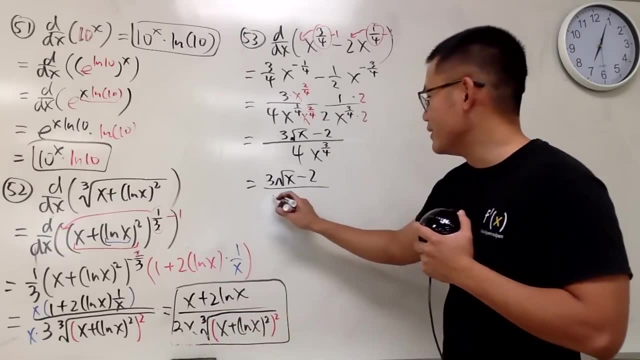 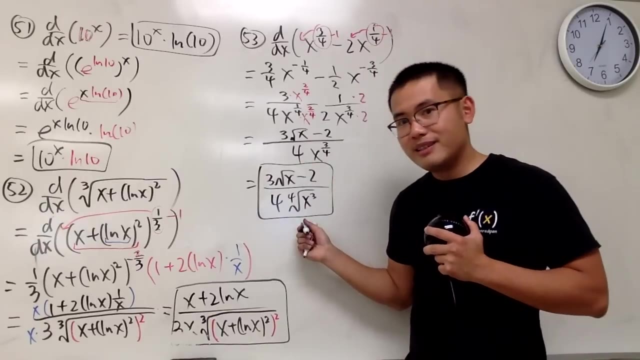 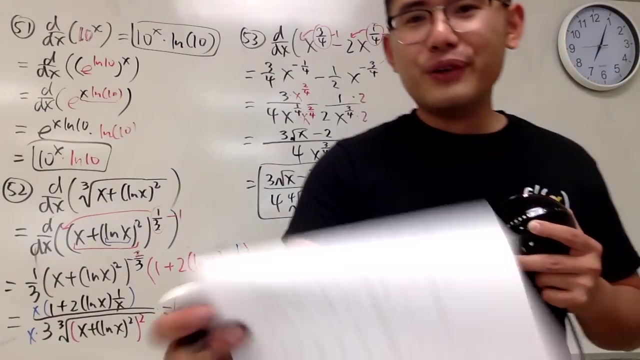 Okay, 3 square root of X minus 2 over 4. X to the 4 over 3 power, which is the fourth root of X to the third power, like that Derivative for this part. Oh, log base 2 for the next one. 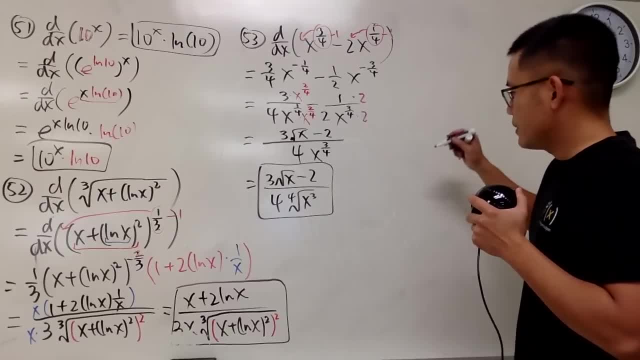 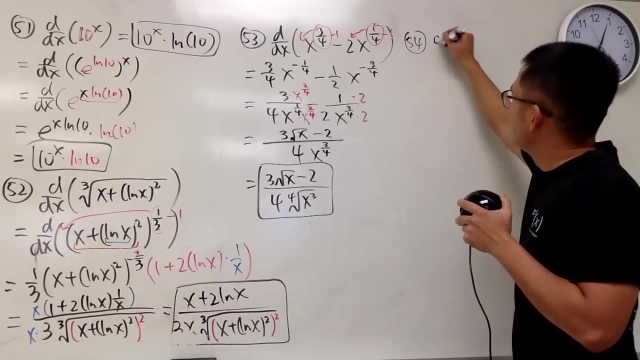 Log base 2, log base 2, log base 2.. Okay, shouldn't be so bad, because we know our log properties. Anyway, here we are going to differentiate. Here is the log base 2.. And we have X times. 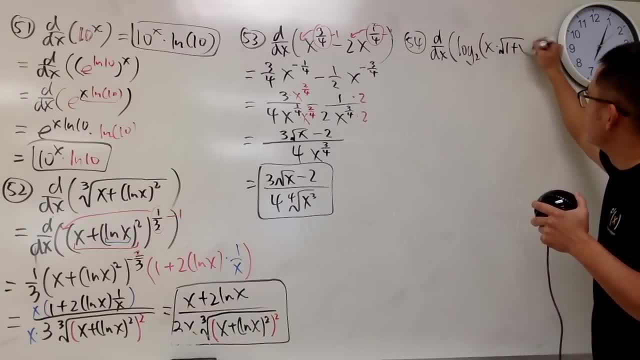 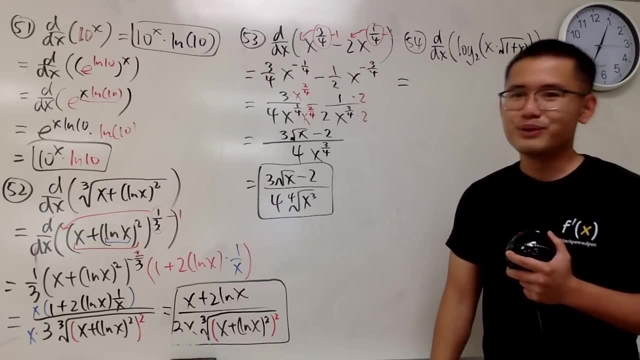 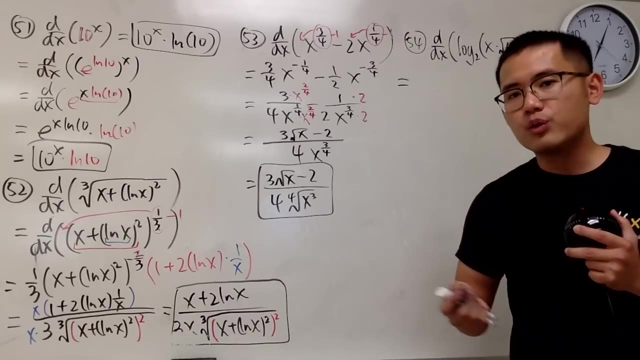 square root of 1 plus X, squared like that. Huh, but I don't know how to take the log base 2 derivative. It's okay, it's similar to this. We can use log properties to take up that. In the log world we like to work with natural log, namely ln. 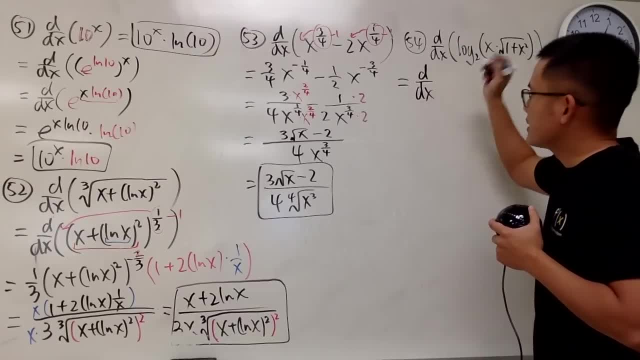 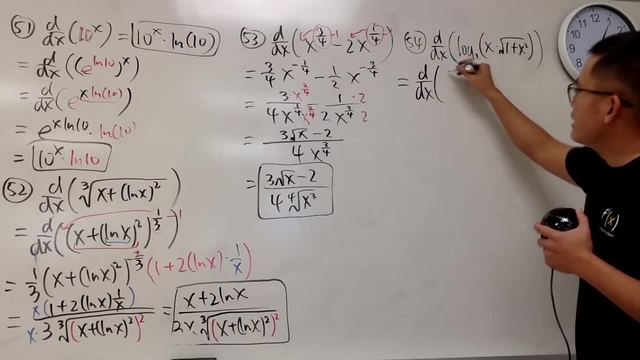 So here is how we can do it. We have ddx, okay, For log base 2, what we can do is just go ahead and do log. so just change this to ln, just change this to ln, and then here we have the inside states like this: 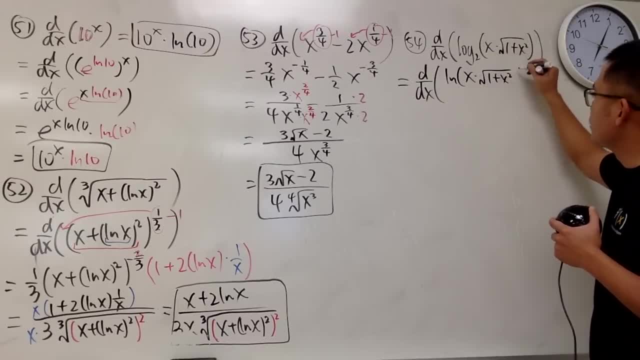 x squared root of. and this is the multiplication: 1 plus x, squared like that. But you see, this is the little 2.. That means you just have to divide it by natural log of 2, like this: okay, So again, natural log of whatever divided by natural log of this number. 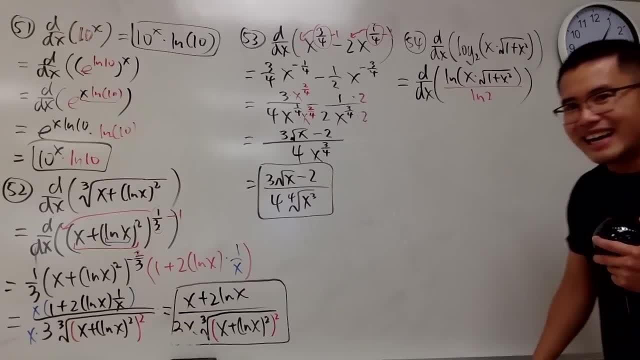 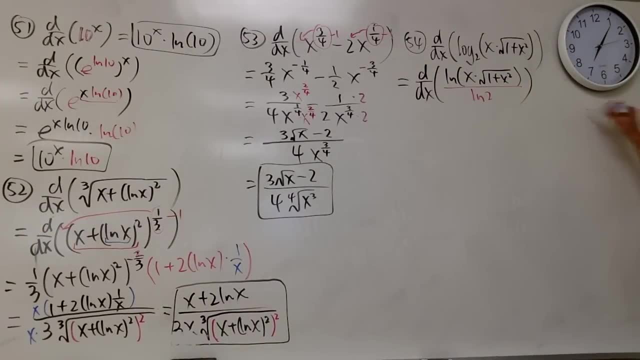 is log of base of this number of the input, like that. okay, So log properties. let me just put it down under the clock. This is log base b of x. okay, This is equal to log of x. Well, any log works, but we're talking about natural log of x. 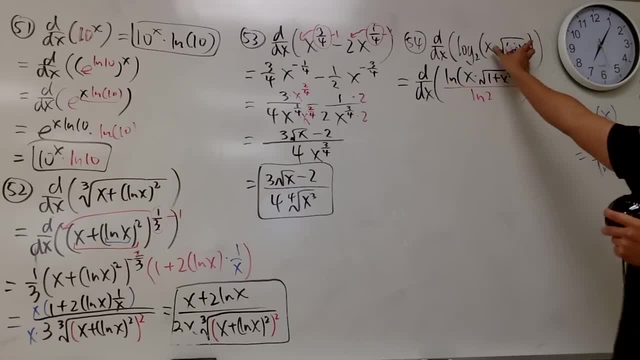 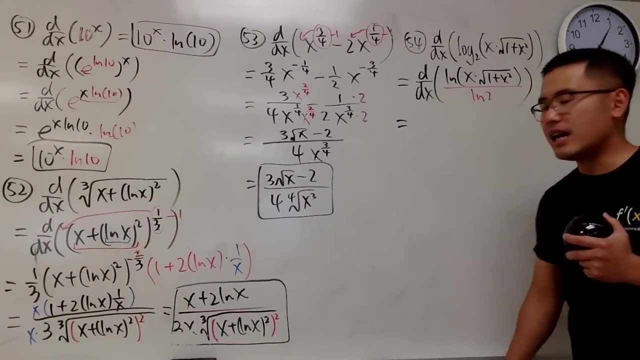 over natural log of b, And it's just. the input is right here. It's slightly more complicated, but get used to it. Okay, now let's do this down. Now let's put this down right. here We have natural log of 2.. 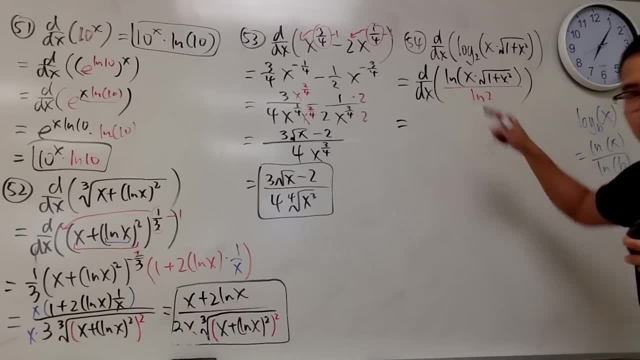 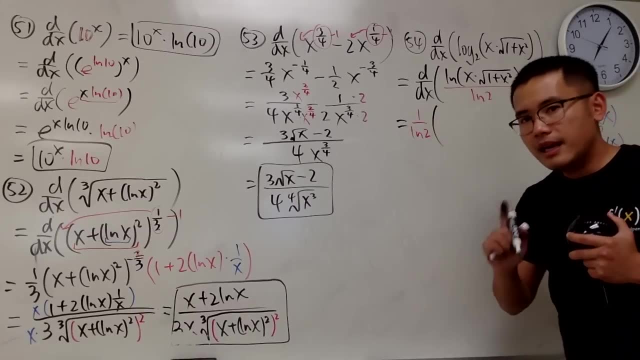 It's just a number and don't let this bother us too much, So let me bring that all the way in the front. That's 1 over natural log of 2, like this: okay, And we are going to differentiate. 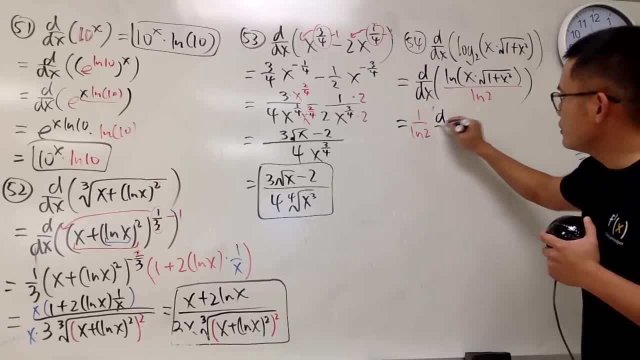 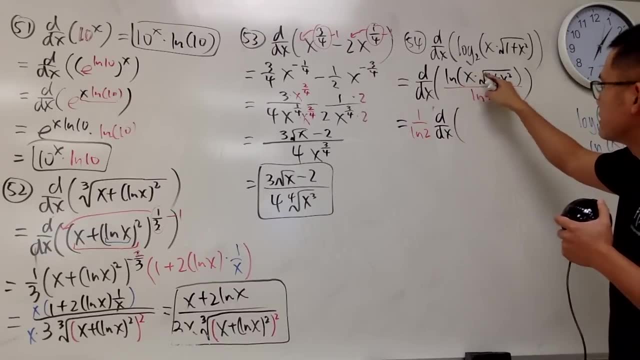 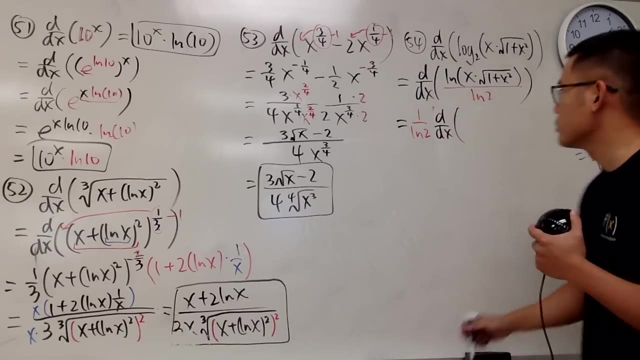 We're going to differentiate Well here. if you look at the part in black, we have natural log of x times natural log of square root. right Product itself is natural log. You can break them apart. It becomes a sum of natural log. 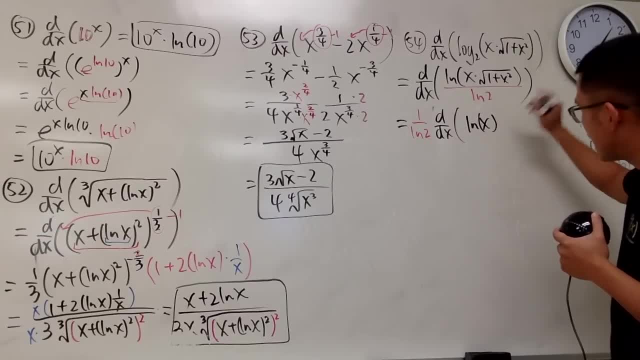 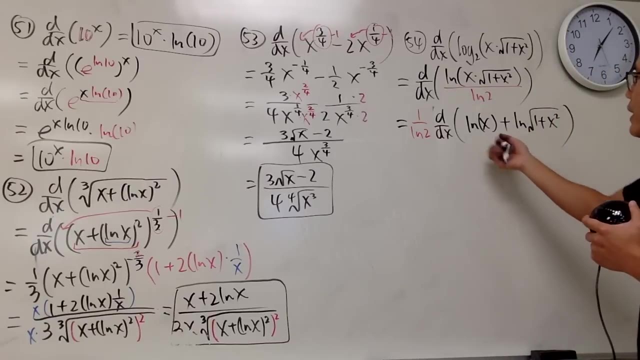 So we can write this as natural log of x. stop, close that and then plus the other natural log and this part, square root of 1 plus x, squared like this: okay, And of course the reason to do so is because this way: 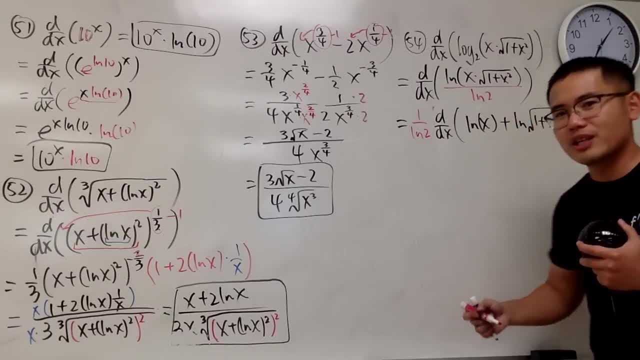 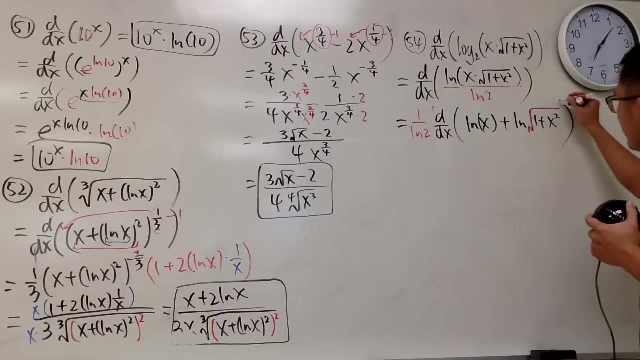 you don't have to use the product rule, And that's how we can actually prove the product rule as well, thanks to the logarithm. Even better, though, when you have the square root. again, this is the same as saying: okay, this is the same as saying: 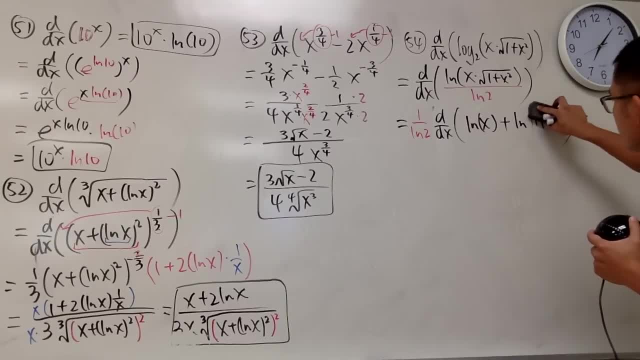 okay, the one-half power, isn't it? So let me just change that. okay, Again, look at the square root right here. We look at it as the one-half power. We can bring the power to the front whenever we have a natural log. 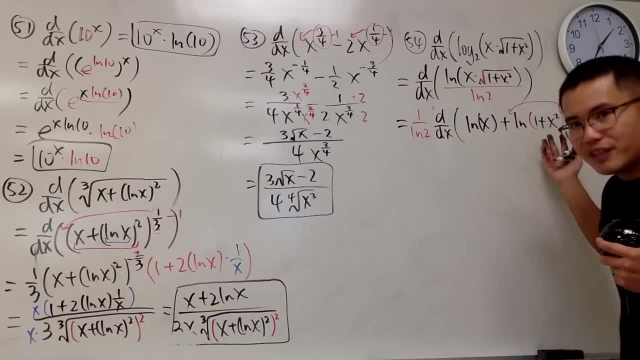 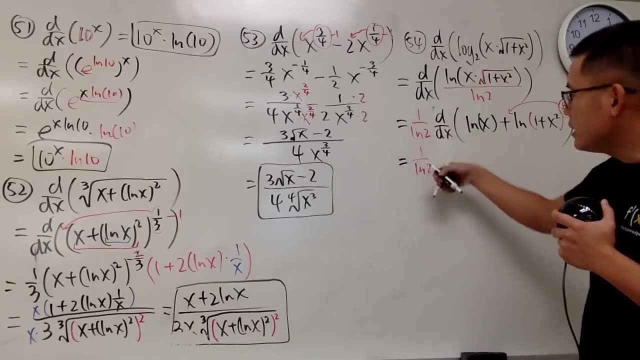 but do not minus 1.. This right here has nothing to do with derivative. This right here is just a natural log property. So, all in all, we will have to differentiate- Here is the natural log in the front And then differentiate. 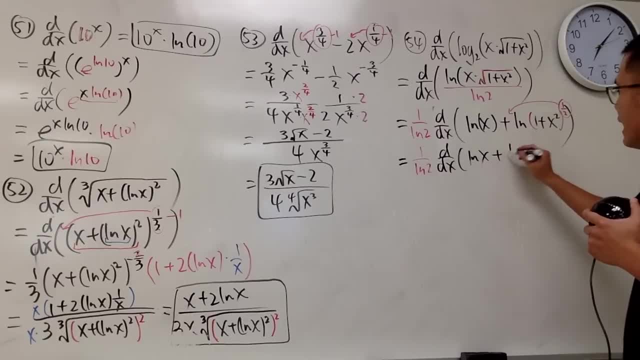 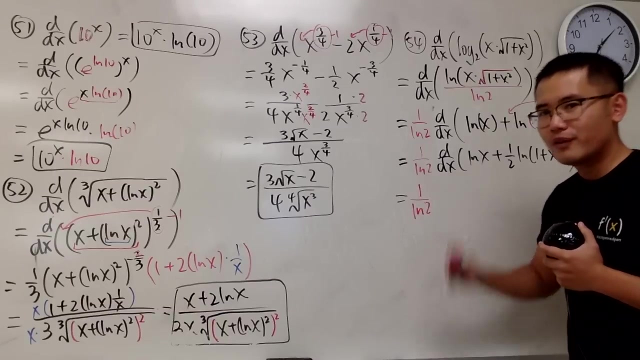 Natural log of x and the one-half in the front and the natural log of 1 plus x squared like this. Enough algebra. Here comes the derivative: 1 over natural log of x, 1 over natural log of 2.. Sorry, 1 over ln 2.. 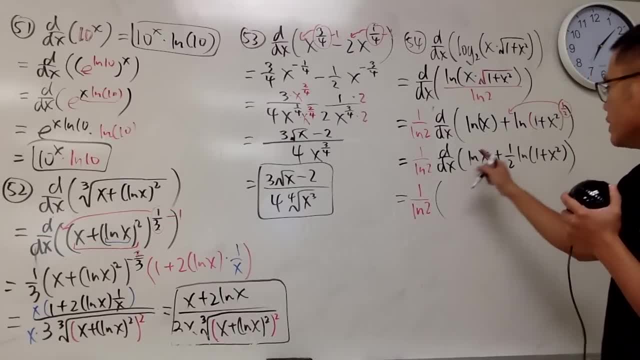 Let's put down parentheses for the result of the differentiation. The derivative of natural log of x is 1 over x Done For this part Plus one-half. It's a constant multiple. Just keep it And then differentiate this part. 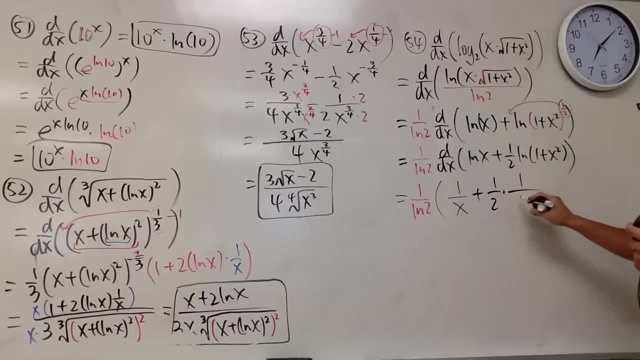 So we have 1 over the inside, which is 1 plus x squared right inside. But the Chengdu says: multiply by the derivative right here, which is 2x, And that's it. We can cancel this out. 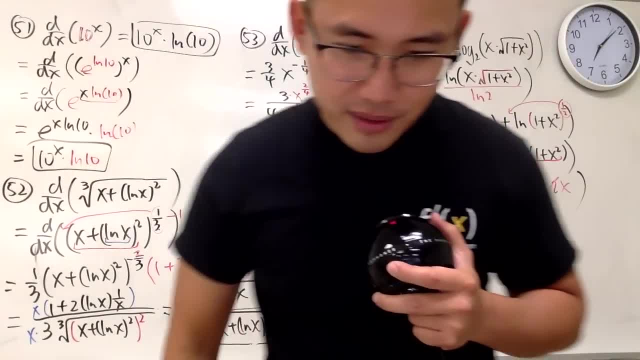 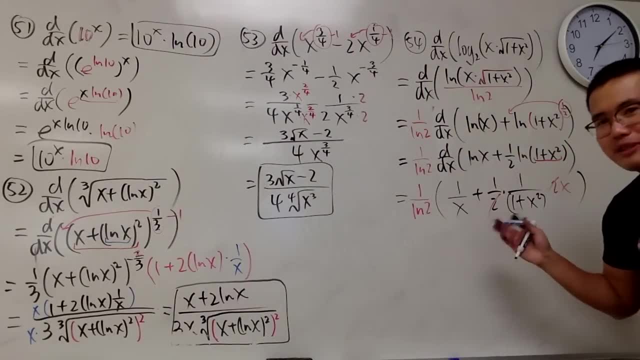 So that's pretty good, But I think I combined the fractions. I did, So take a look right here. This is pretty much it, But I just combined the fractions And to do so, of course, we can just multiply this right here by this denominator 1 plus. 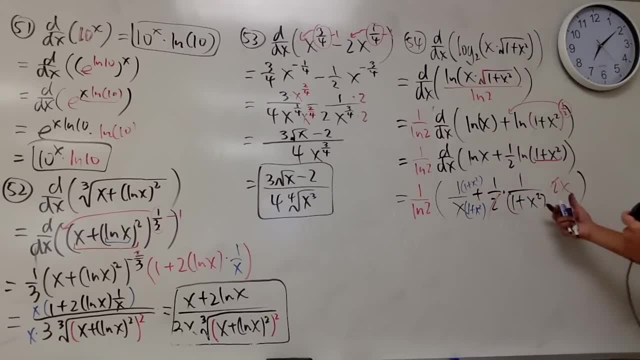 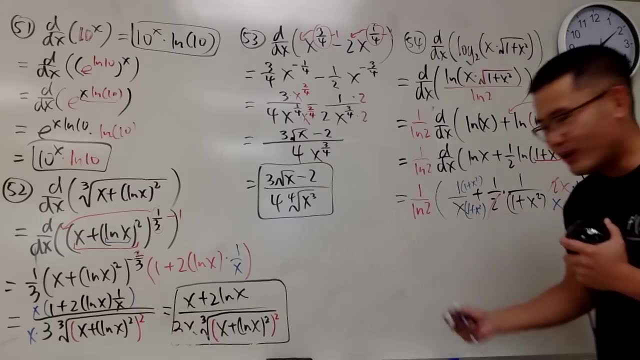 x squared And of course do it on the top as well, And for this one we need the x on the bottom as well. So we multiply the bottom by x, the top by x as well. So all in all, you will see the bottom. 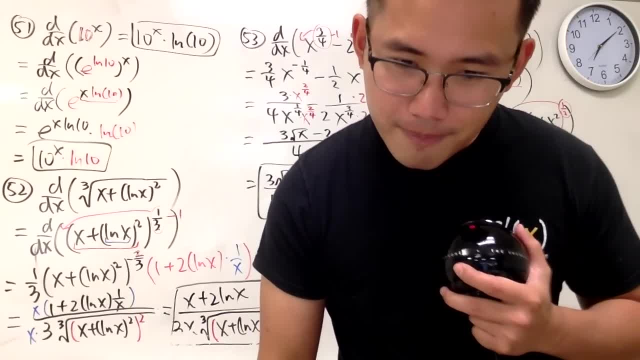 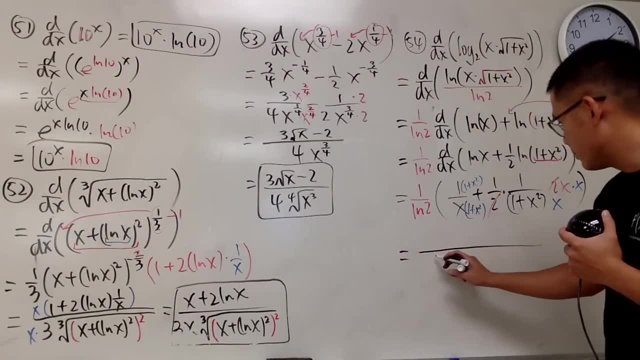 How did I write the answer? I forgot. I put the natural log of 2 all the way at the end, right. So I put natural log of 2 at the end. I put down x first, So I put down x. 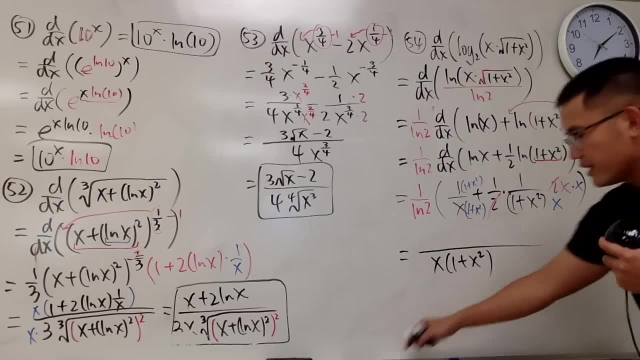 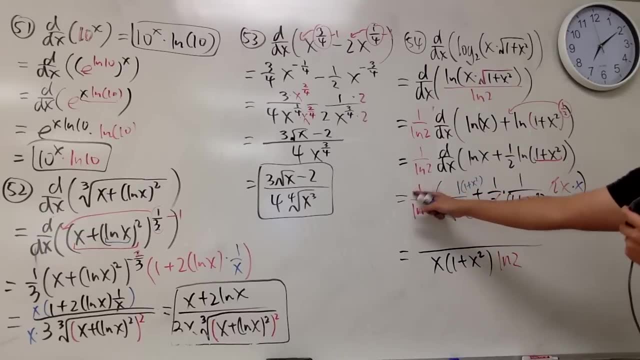 And then 1 plus x squared, And then here is the natural log of 2.. OK, And then we just have to work on the top 1 times. this is just the inside. This is just 1 plus x squared plus x squared. 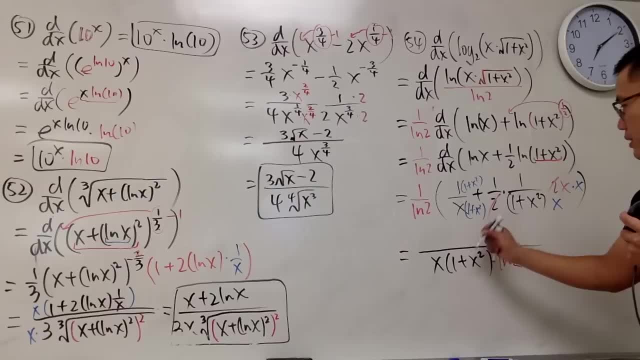 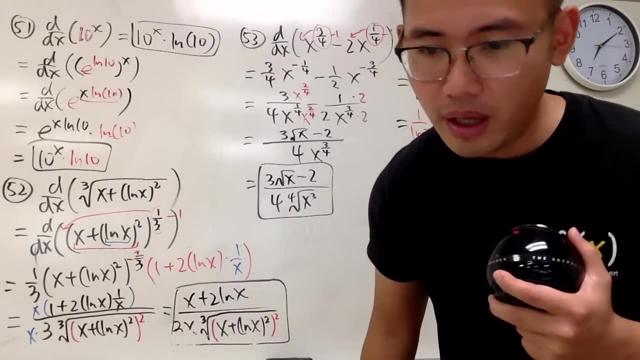 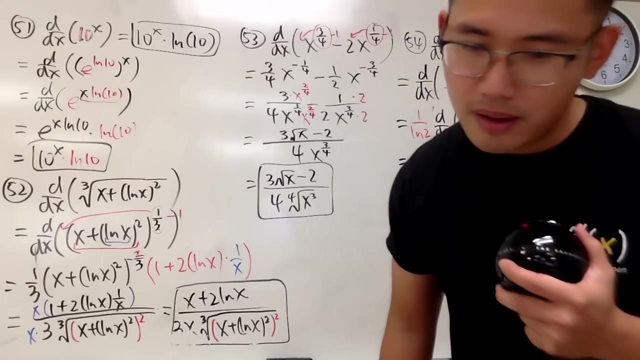 So we have 1 plus 2x squared. 1 plus 2x squared, That's it: 1 plus 2x squared. Yeah, I see the answer on the answer key, So I'm good with my work. 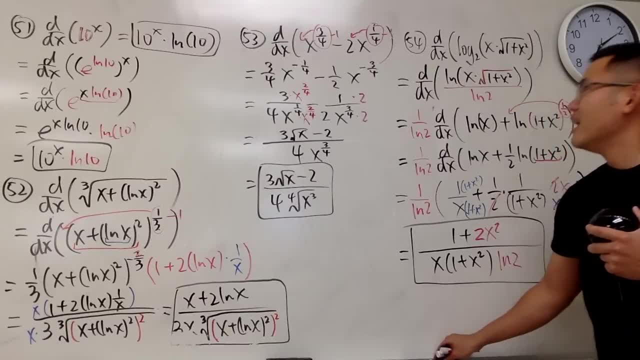 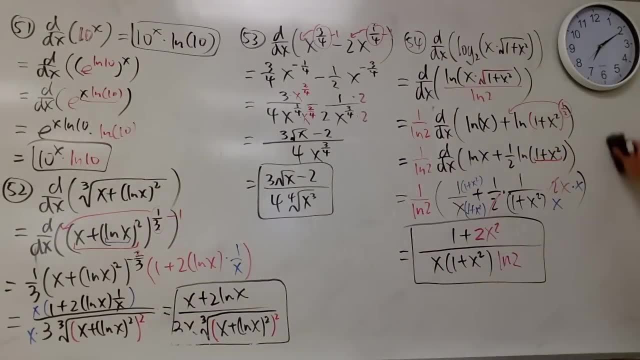 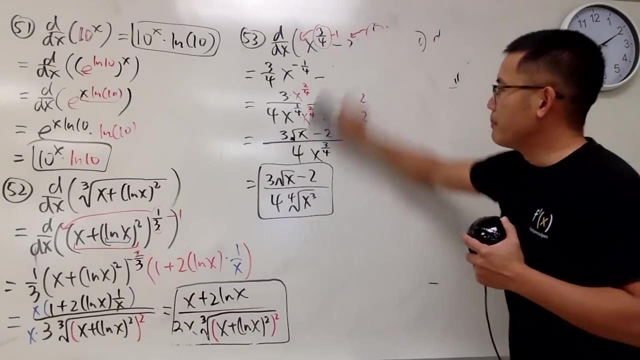 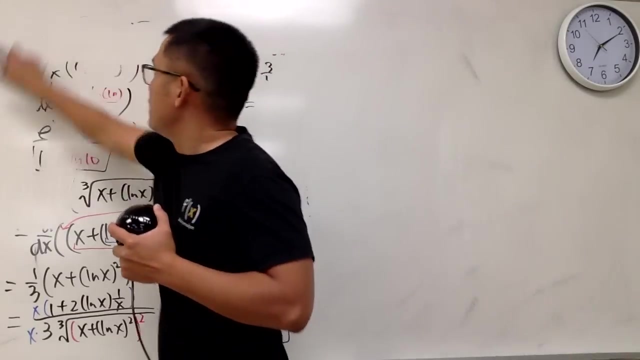 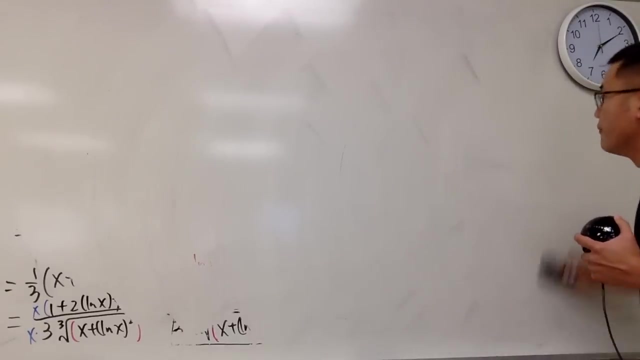 And I'm also good with the answer key. Pretty good, Take a look, Take a look. Take a look. I feel like I write bigger when I'm doing derivative than integrals. I don't know If you guys find my videos helpful. let me know. 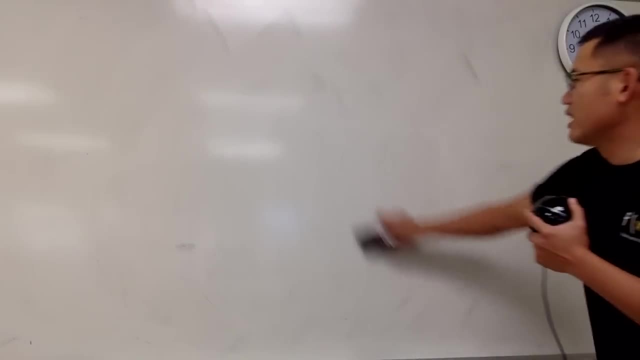 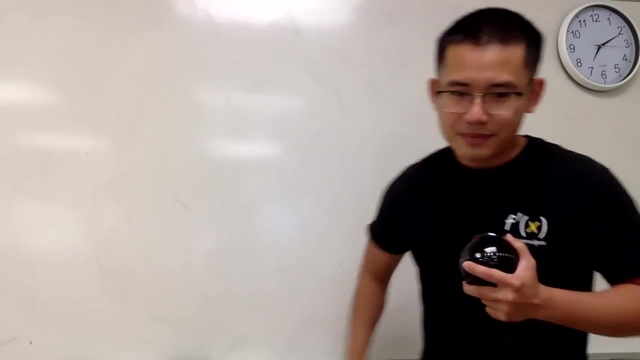 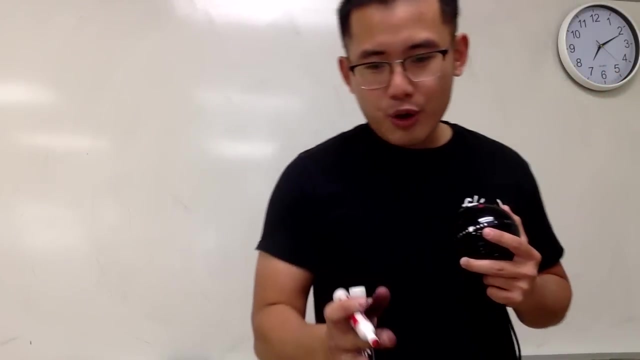 Thank you. I appreciate that You can simply let me know by press the Like button. That would really help the video. Thank you so much, though. Yeah, I'm having fun to do this as well And, most importantly, hopefully you guys do this on your own first. 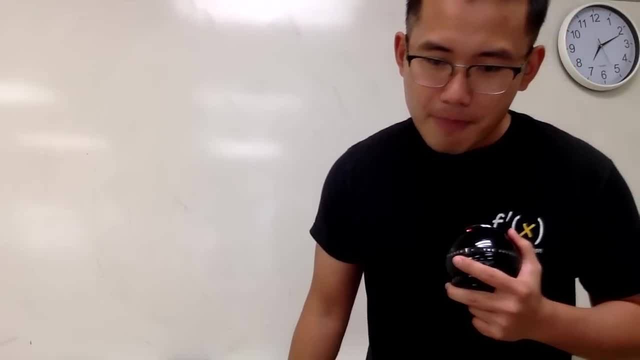 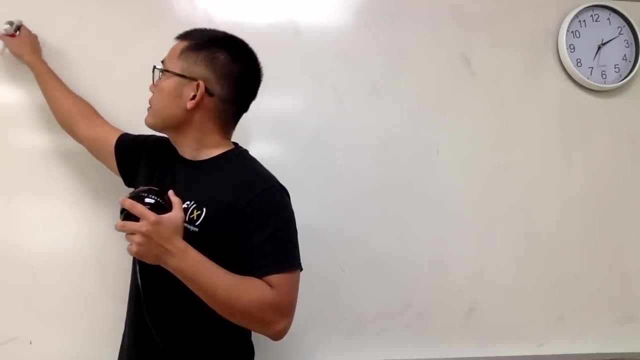 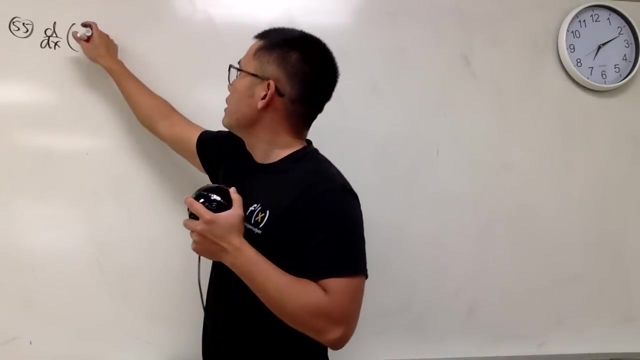 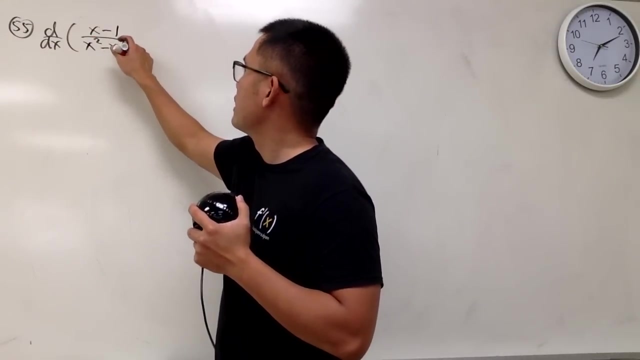 and then check out the video. That's the main part. all right, OK, Number 55, right here Differentiating: Here on the top we have x minus 1 over x squared minus x plus 1.. Three terms on the bottom, but this is OK. 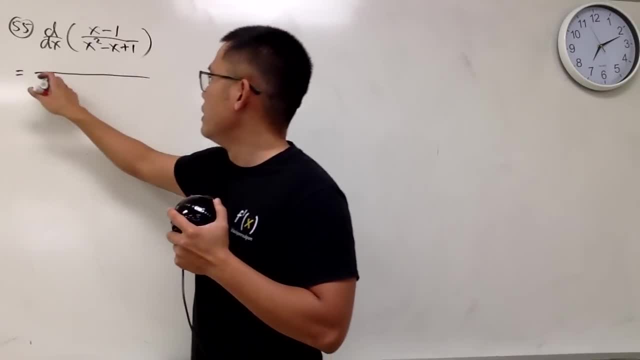 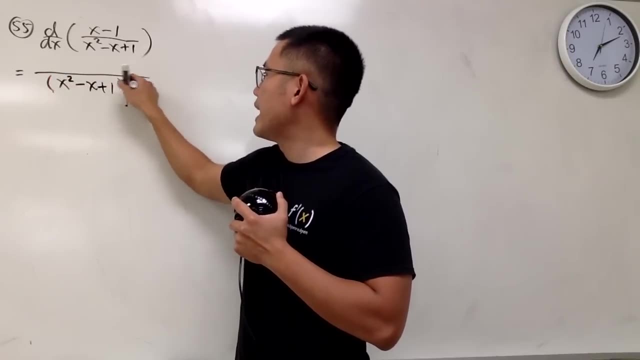 This is still a quotient rule situation. So go ahead, Do the quotient rule. Parentheses. square the denominator x squared minus x plus 1.. Square that, And then on the top Man. Oh my god, I have to. 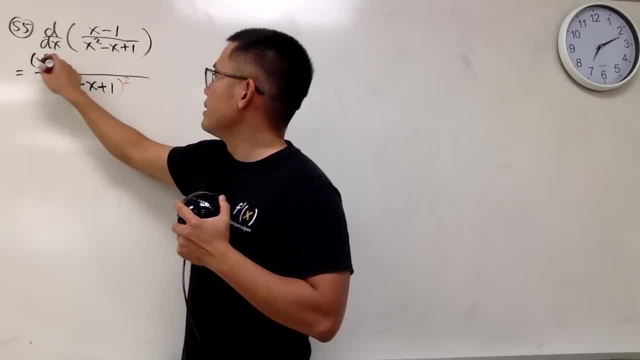 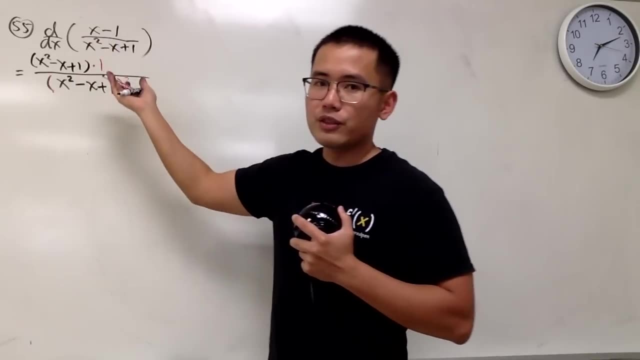 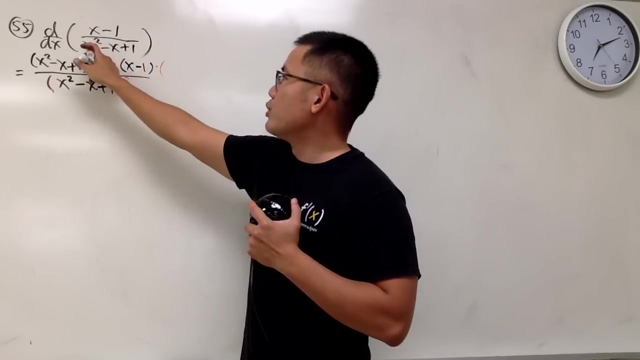 I hope it's not so bad On the top. we have to just keep the denominator and multiply by the function the derivative of the top function, And then minus the top function, which is x minus 1, times the derivative of the bottom. 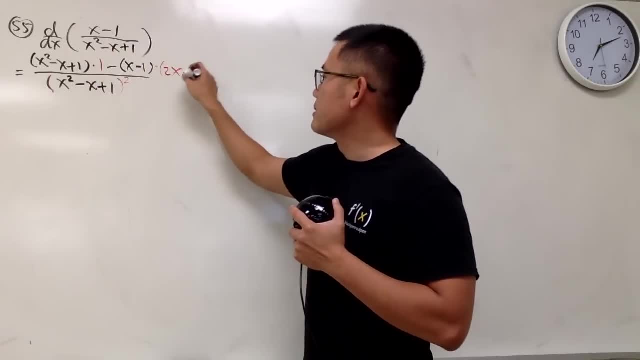 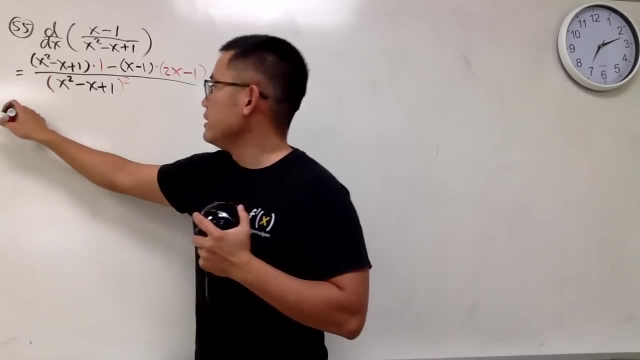 The derivative of x squared is 2x. The derivative of minus x is minus 1.. The derivative of plus 1 is 0.. So that's what we have Now. Let's see On the bottom. we have this: 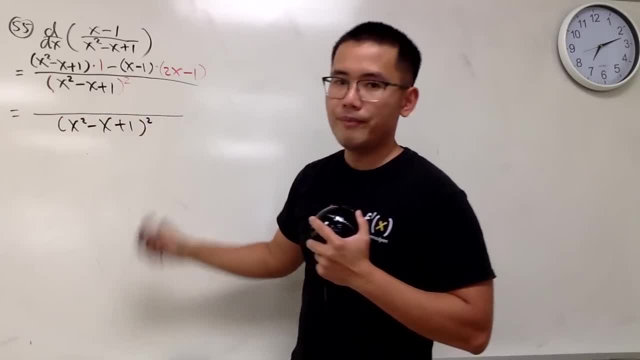 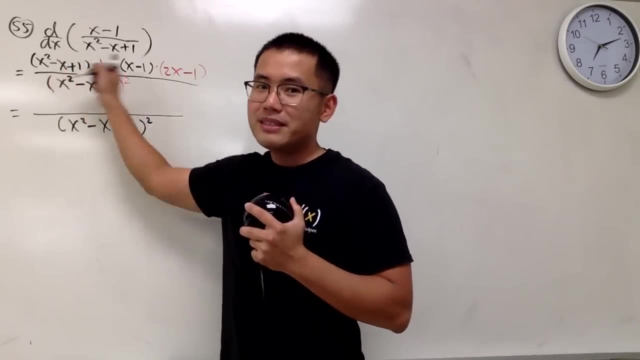 x squared minus x plus 1 squared. I think. I'm still writing, OK, I don't know. Anyway, on the top you have this times that which is just x squared minus x plus 1.. But we have to FOIL this out. 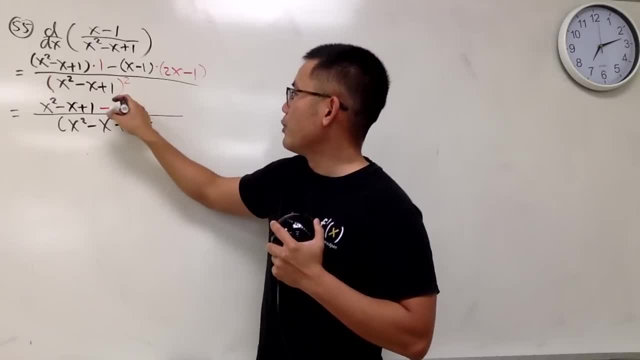 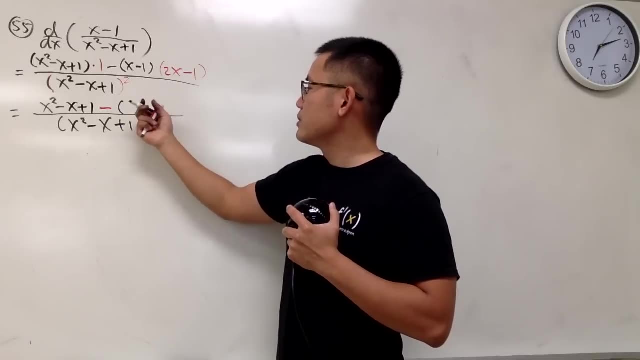 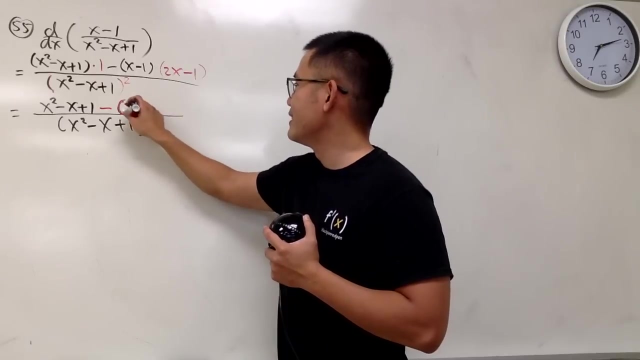 So let me just keep the minus in red right here, And then I'll open the parentheses. x times: this is x times. this is x times 2x is 2x squared, And then this is minus x, And then this is minus 2x. 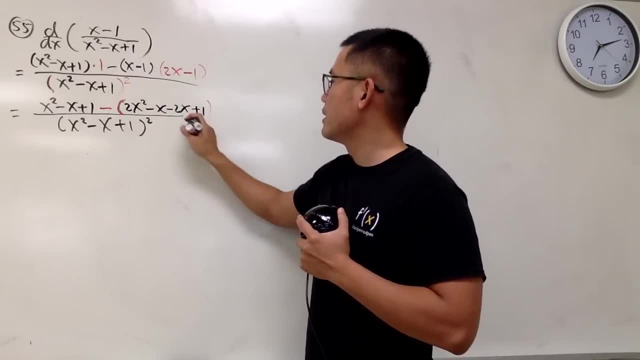 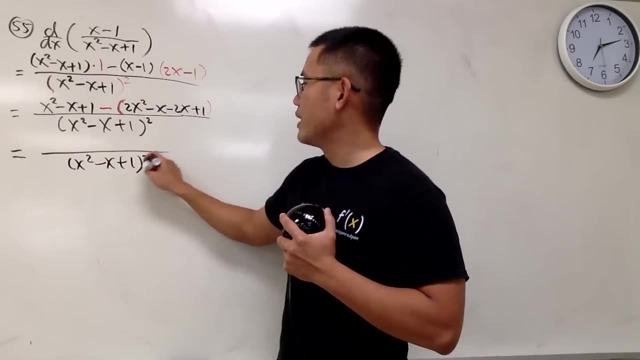 And this is plus 1.. OK, And again, let's see, And we are going to finish this right now, I'll do the computations in our head. Well, actually, I'll still write things down for you guys. Bye. 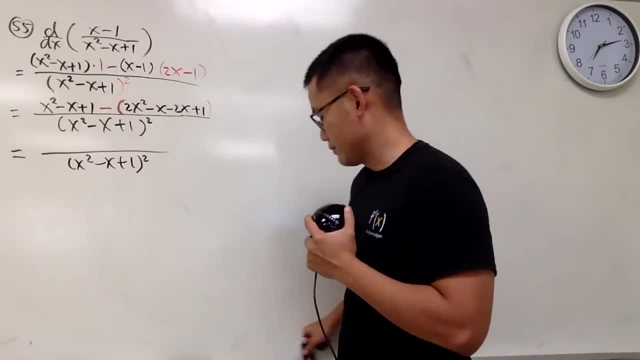 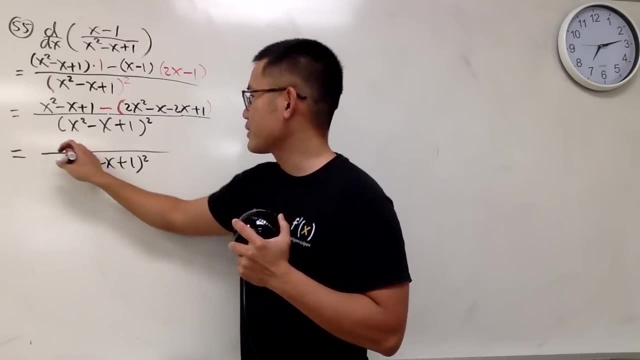 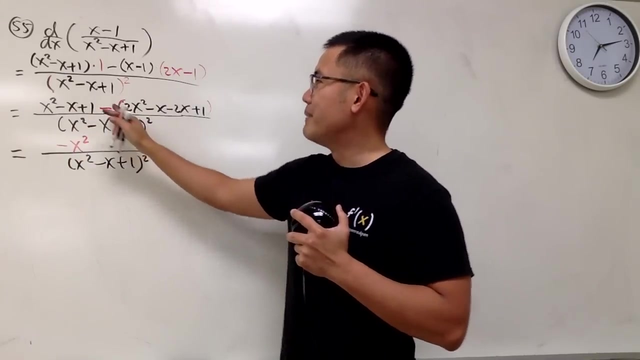 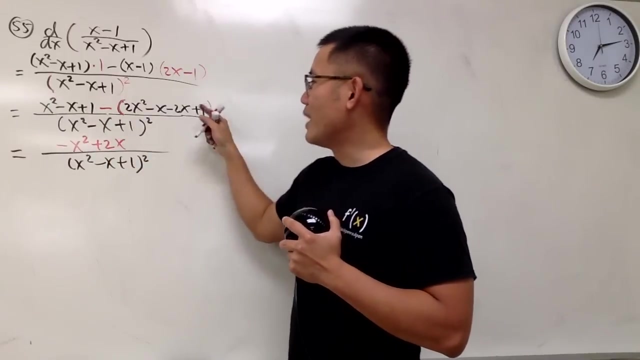 So, alright, okay, let's do it. x squared minus 2x squared is negative x squared- Okay. Next, negative x plus x is 0, but negative, negative 2x is plus 2x. Alright, Lastly, 1 minus 1 is 0, so well done. 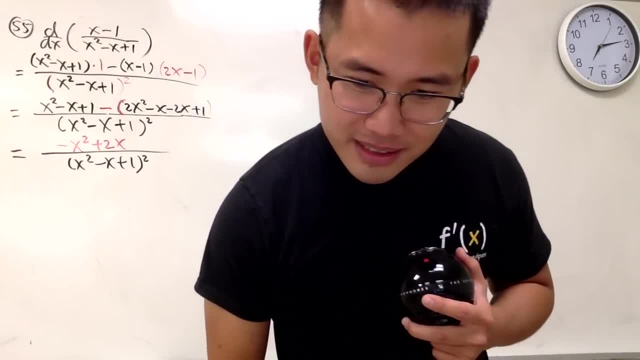 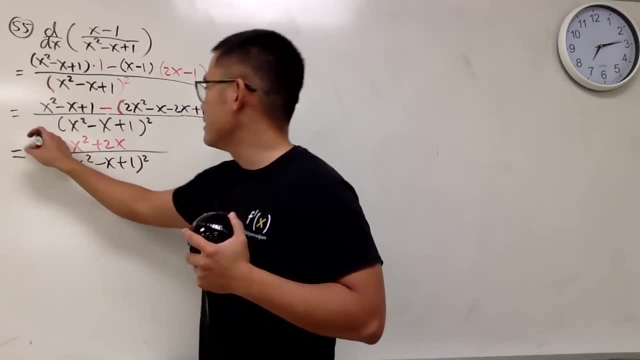 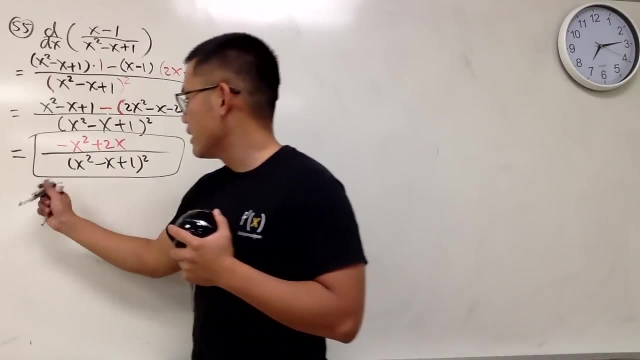 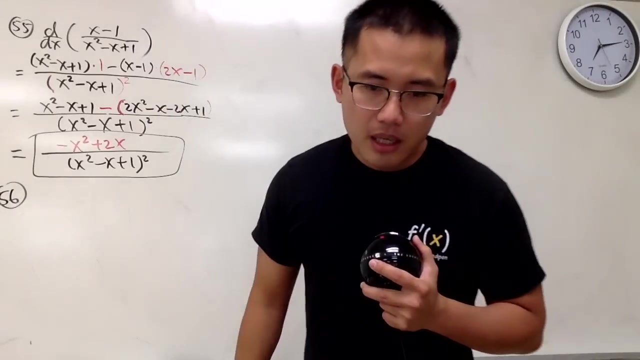 So that's it, I believe. Yeah, that's it for the answer and I left it like this and the answer choices as well. So that's it. Ooh, number 56.. We have to well not integrate, we have to differentiate. 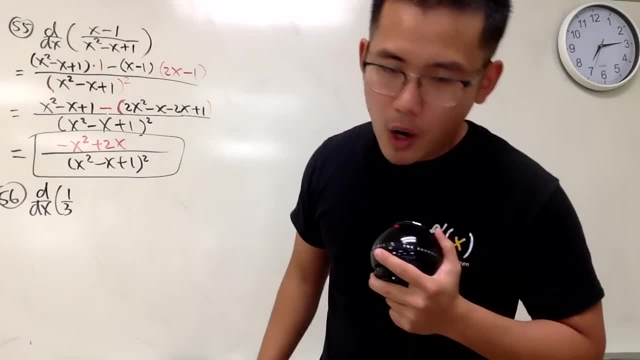 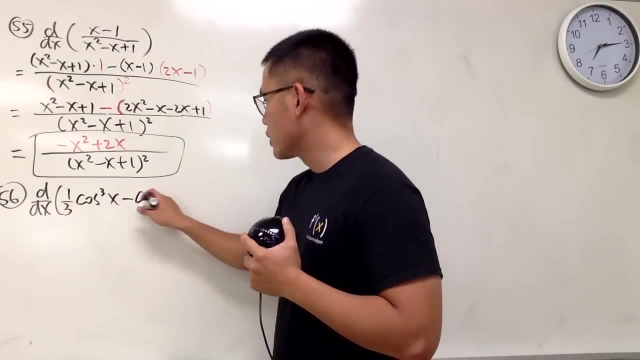 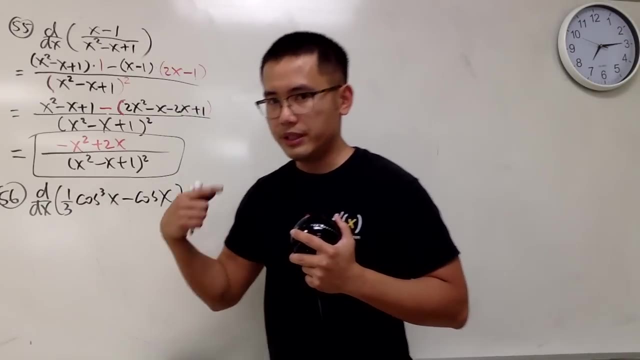 one third, and we have cosine to the third power, x and minus cosine x, like that. Well, well, keep in mind this: right here is cosine x to the third power, right Cosine x and then to the third power. 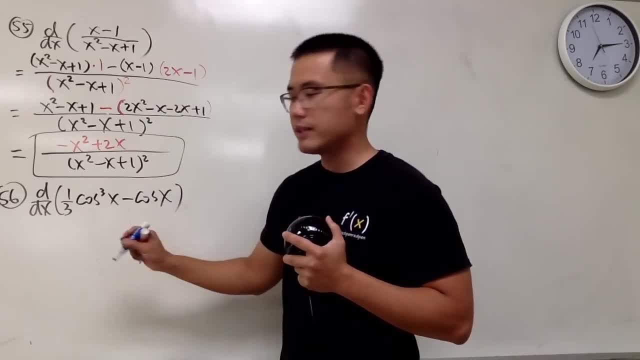 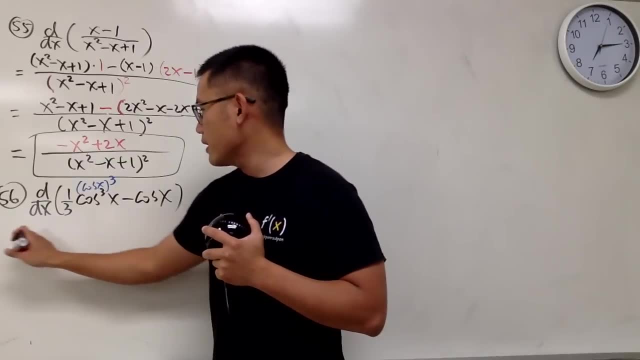 So perhaps I will just make it clear for you guys right here: We will look at this as cosine x to the third power, right here? okay, So here we go, Differentiating this. you bring the 3 to the front and then minus 1.. 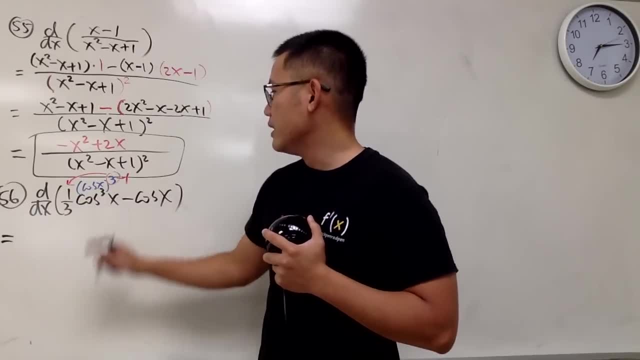 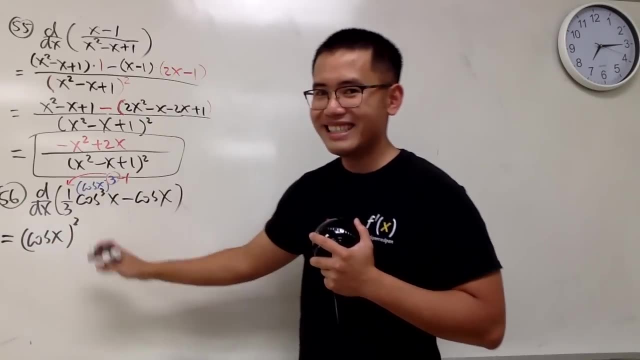 3 times, one third is gone, It's just 1, actually. So we have the inside, which is cosine x, But this times to the second power, And multiply by the derivative inside, which is going to give us negative sine x. 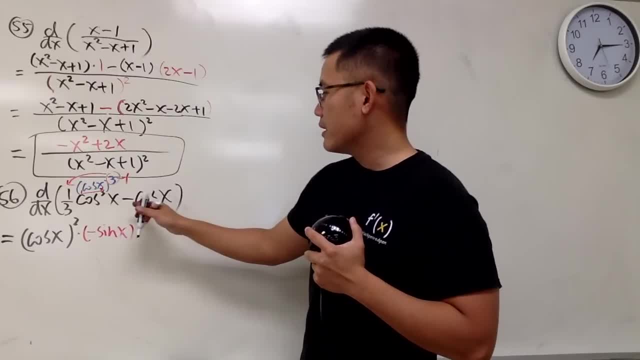 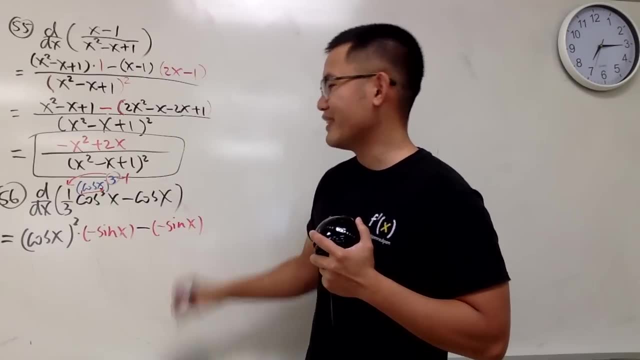 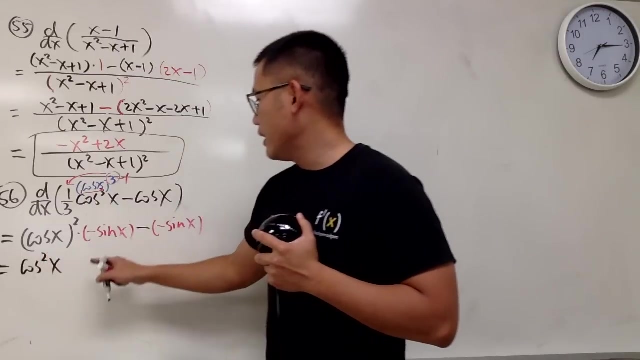 And we are done for the first part. Okay, And then here we have minus the derivative of cosine x. But cosine x is negative sine x. So that's what we have. And now check this out. Here we have cosine, and let's put on the square right here. 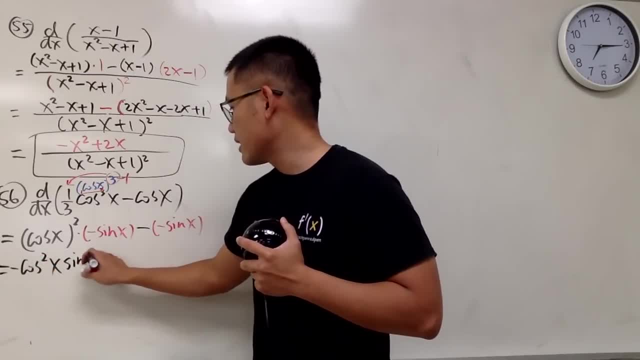 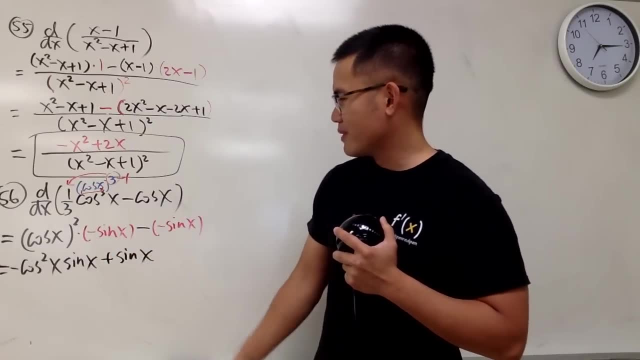 And this is negative sine x, like that right Negative sine x. And then we have the plus sine x, like this: Hmm, Let's factor out the sine x to see what happens. When we do that, we have sine x right. 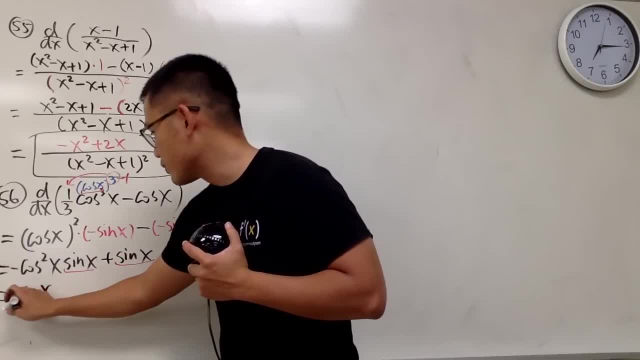 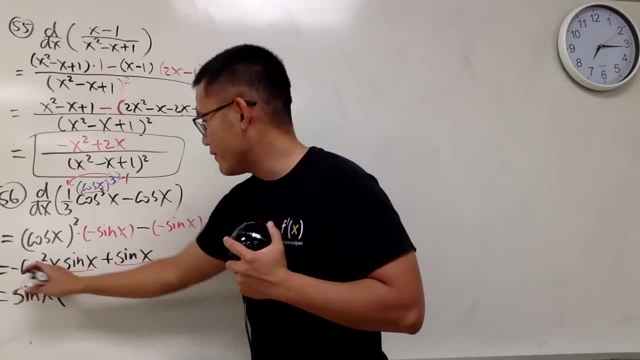 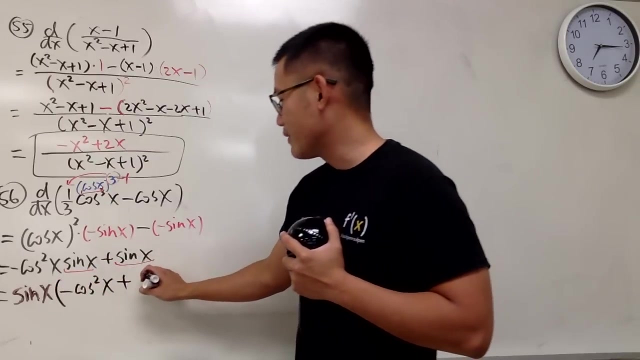 This and that we factor it out to the front. So we have the sine x all the way in the front. Well, well, here we have negative cosine squared x plus. This is out. But don't forget, we still have the 1 right here. 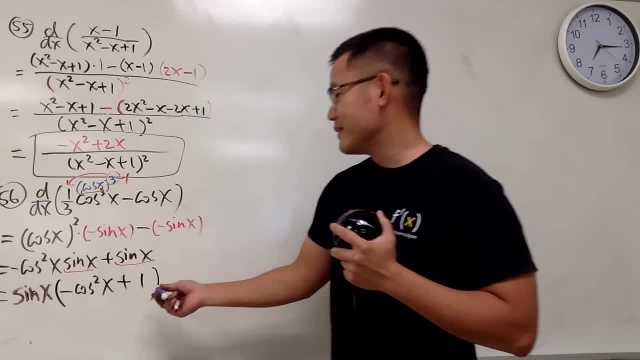 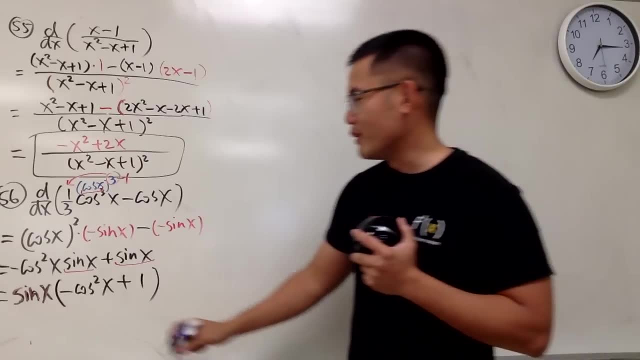 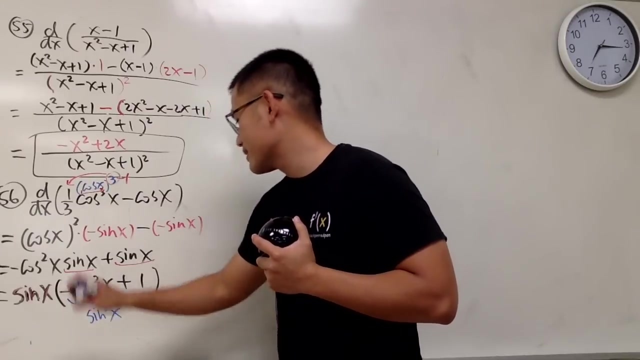 Everybody knows. Well, actually, Oh yeah, Everybody knows. 1 minus cosine squared x is equal to sine squared x. But I know negative cosine squared x plus 1 will give you sine squared x as well: 1 minus cosine squared. 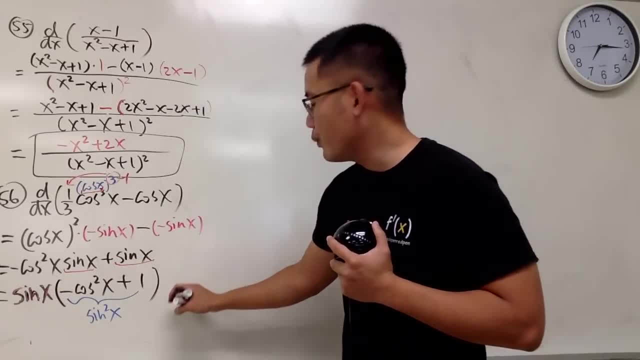 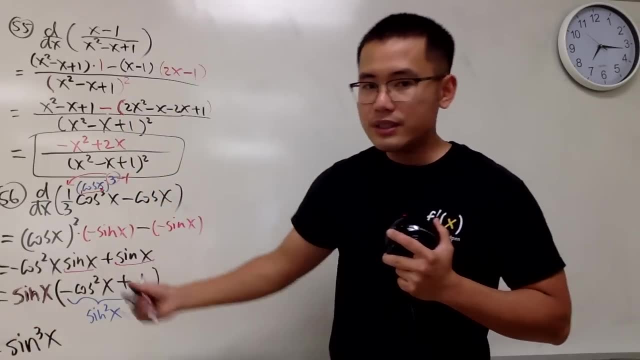 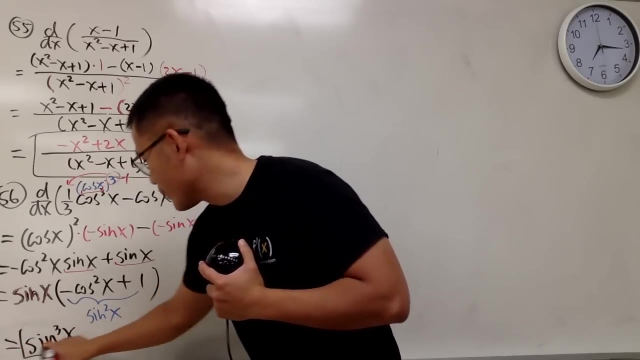 So therefore, sine x times sine squared x, all in all we end up with sine to the third power, x, And with that we are done. But you guys don't see the equal sign, So let me write it down. This is better for you guys. 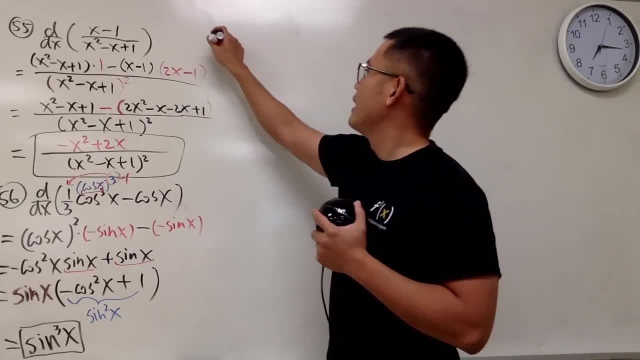 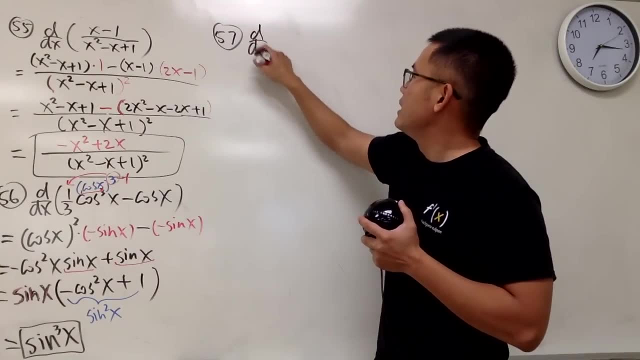 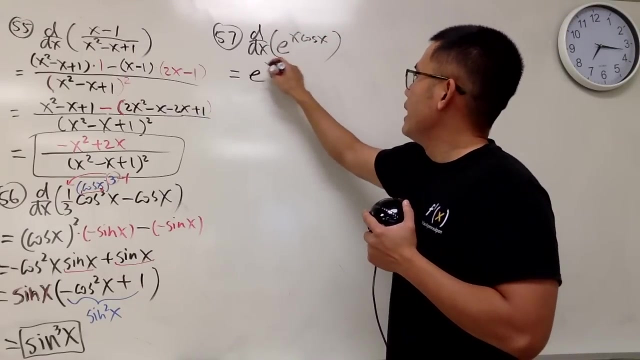 Okay, You see the equal sign, I'm happier. Okay, 56.. No 57.. Ooh, Okay. E to the x times cosine x. Right, Here we go. E to the x, cosine x. Again, you just keep it. 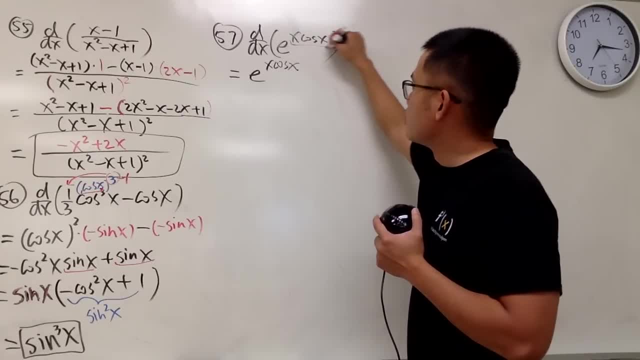 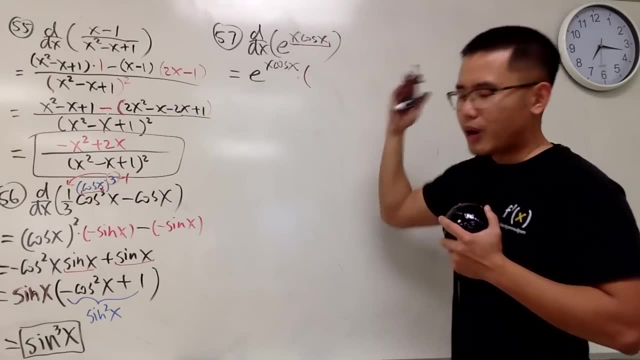 You just keep the e to the whatever, Then you multiply by the derivative of the inside. Pretty much it's this part Like this, This exponent part: Multiply. Here we go. Power Product rules are part Product rule in action. 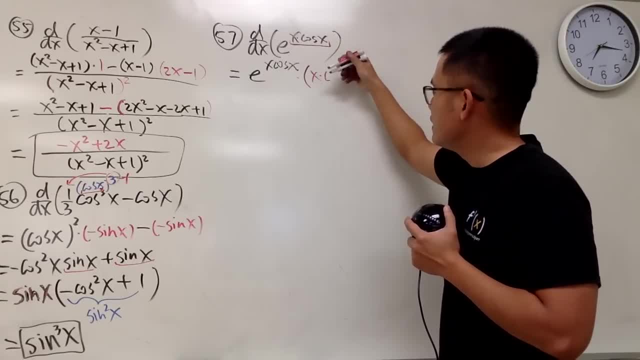 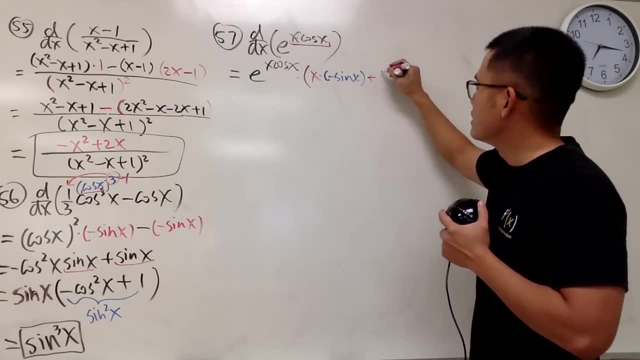 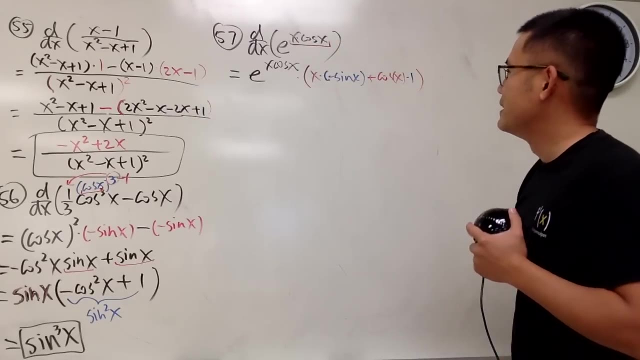 First function, x. Multiply by the derivative of the second, which is negative sine x. Multiply by negative sine x. Add the second function, which is cosine x times the derivative of the first, which is 1.. I put down the answer before I tell you guys. 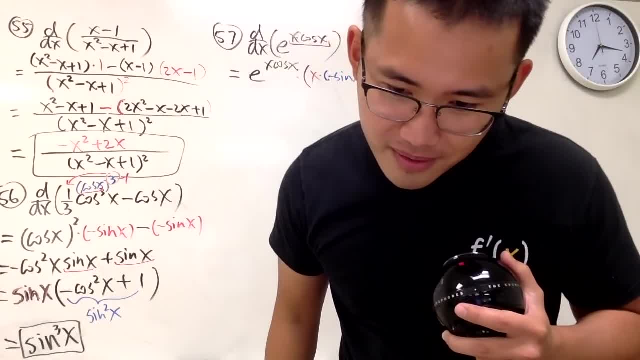 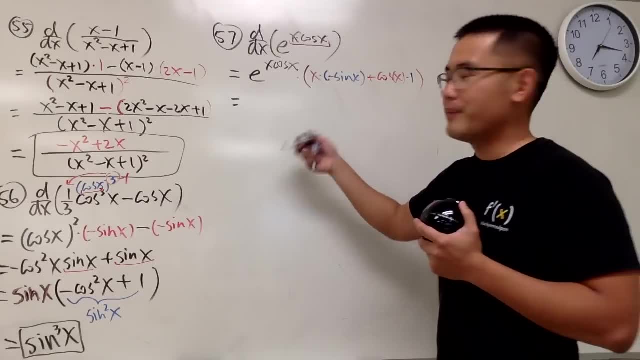 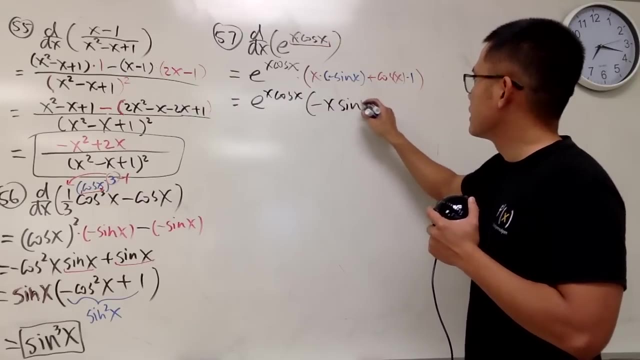 That's pretty much it. What else did I do? That's pretty much it. Nothing too much we can do. So this right here: you just have to know how to write down the derivatives. And this right here is negative x, sine x. 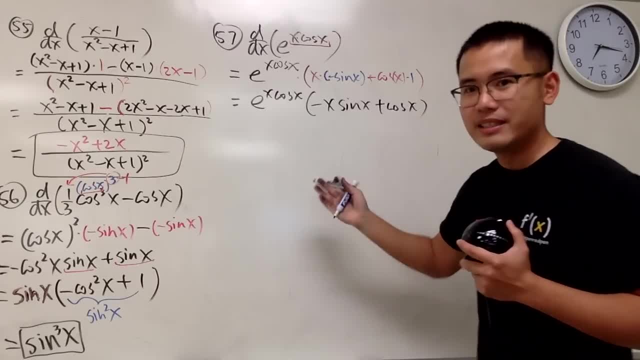 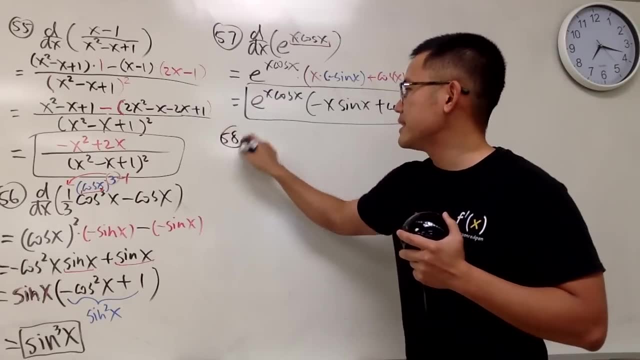 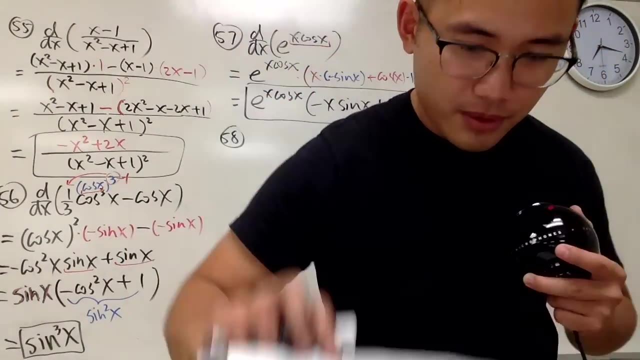 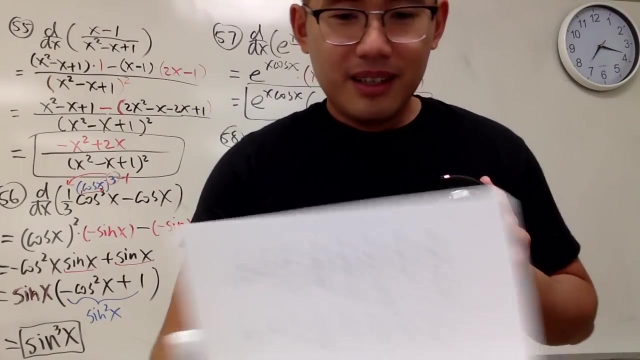 And plus cosine x, Like this, And with that we are done. Okay 58.. This is done already. Number 58.. Oh my god, This sheet is done. actually, This sheet is done. Two more sheets, But like this is the part I'm afraid of, okay. 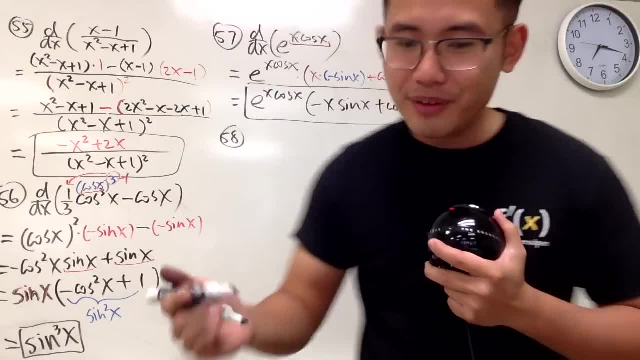 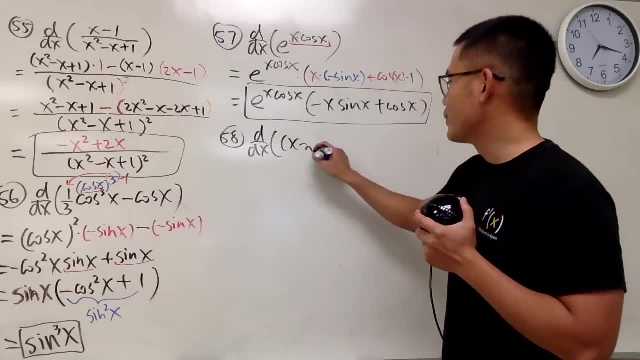 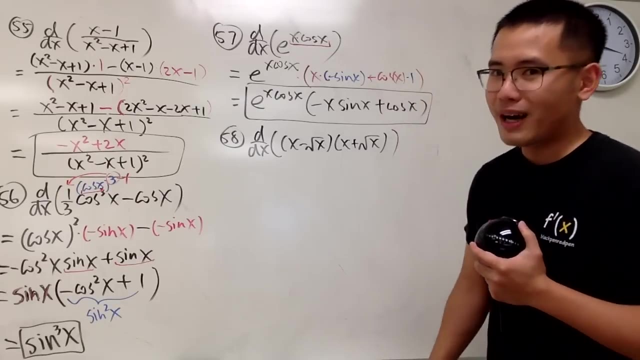 This is the part I'm afraid of, to be honest with you guys. Number 58.. Anyway, d dx of x And we have minus square root of x, Times x plus square root of x, Like that. Well, do we need to use the product rule? 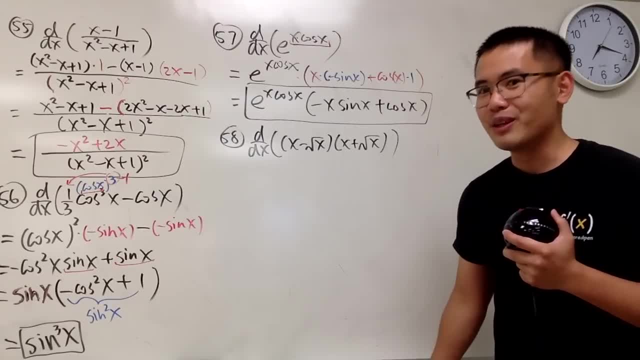 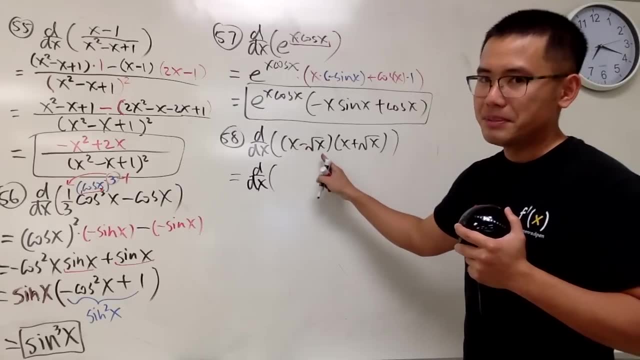 No, Because you can do the algebra. You can multiply this out yourself first. And, better yet, check this out This right here: This is a minus b times a plus b In that form right. So the result is just a squared minus b squared. 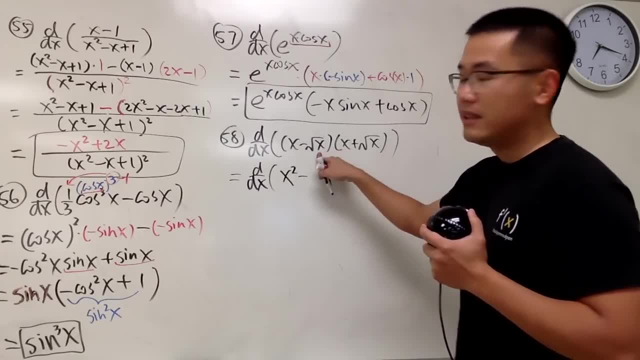 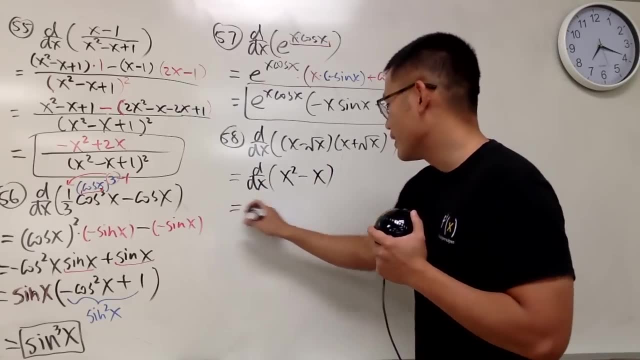 Namely, we'll get x squared minus square root of x squared, which is just x. So we just have to differentiate this instead. In another word, we can just say the answer is 2x minus 1.. Done, Okay. 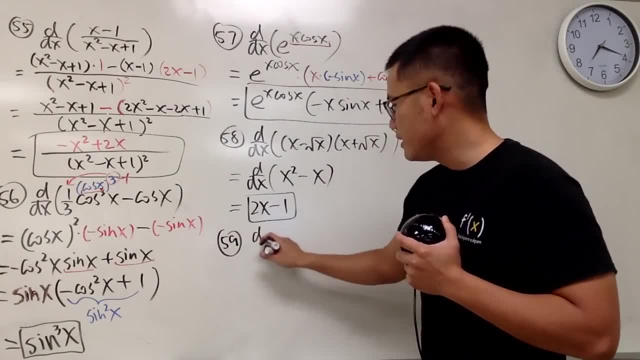 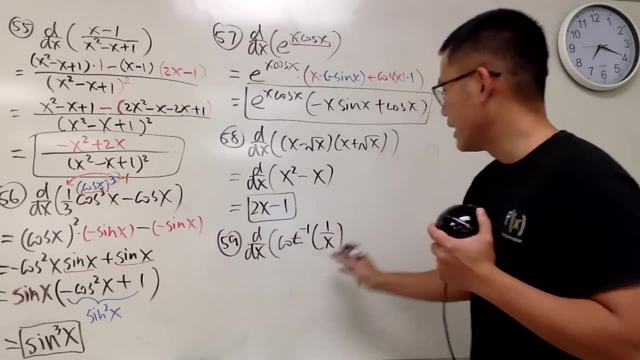 Next one, 59. We are going to be differentiating inverse cotangent, right Inverse cotangent of 1 over x, Like this: Ah man, I'm going to just see. I have to think about how to save space. 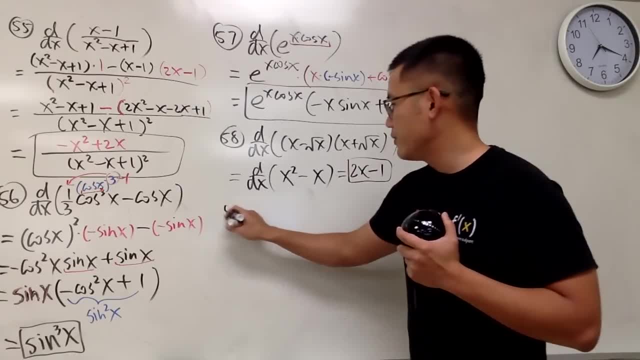 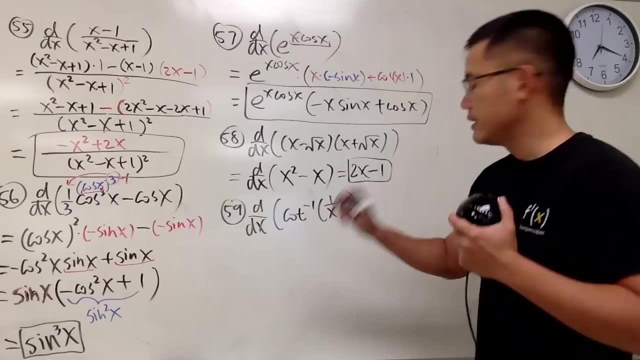 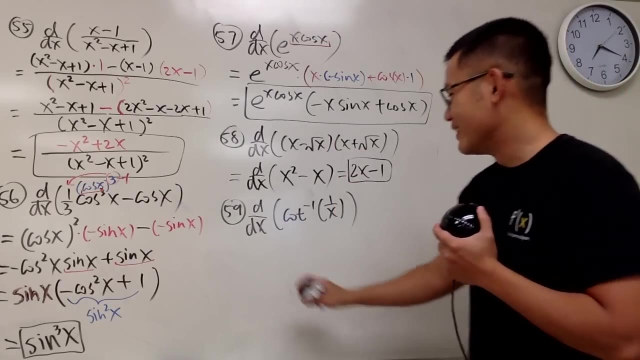 59, differentiating inverse cotangent of 1 over x, Like that. Oh my god, What's the derivative of inverse cotangent? Don't worry, It's just negative. 1 over 1 plus x. squared Right, But you have to be careful of the input. 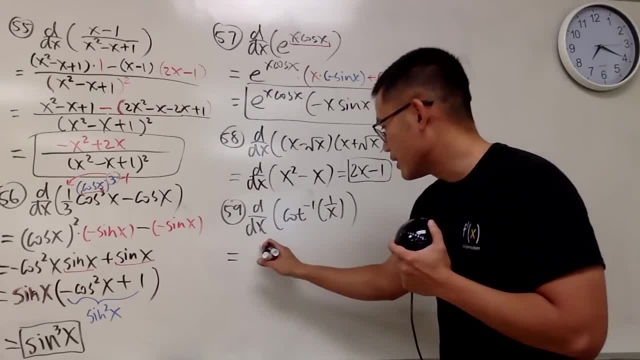 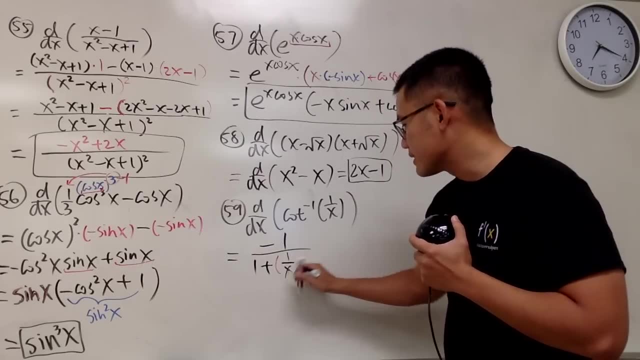 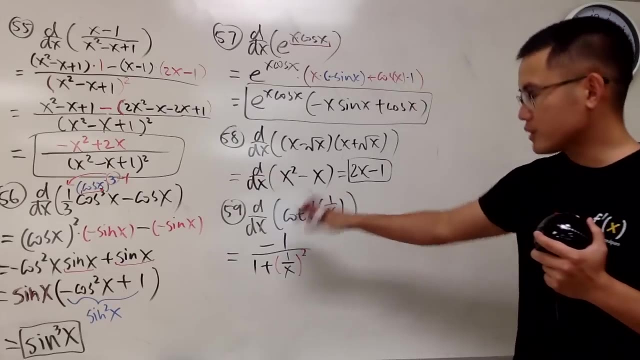 Here we go. Derivative of inverse cotangent. You'll get negative 1 over 1 plus the input being squared. So here, 1 over x And you square that. It's very similar to the inverse tangent. For the inverse cotangent it's a negative, right here. 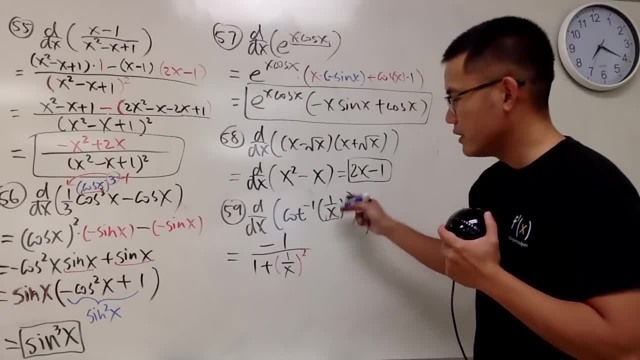 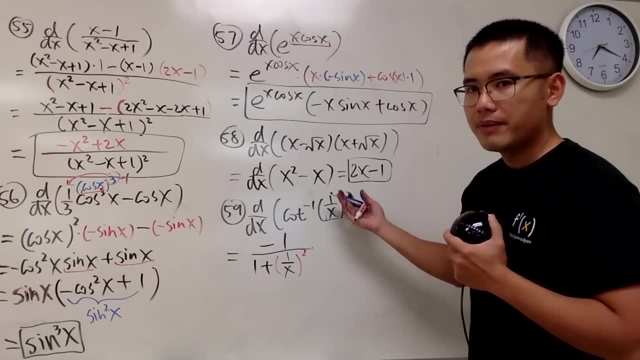 But don't forget we have to multiply by the derivative of the inside Derivative of 1 over x. Well, it's like saying x to the negative 1.. Bring the negative 1 to the front, You have negative 1.. 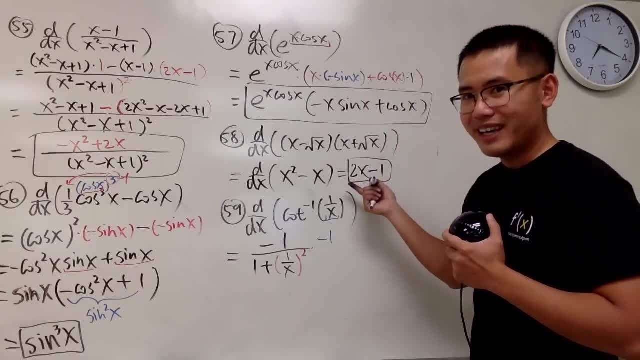 And Negative 1 minus 1 is negative 2.. For the exponent x to the negative 2 is the same as saying over x squared Like that, And in fact this also happens a lot. You should remember it. Derivative of 1 over x is this: 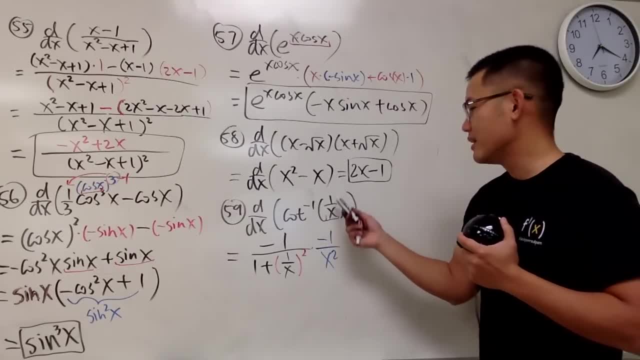 You can put that down right away. That's pretty much it. We'll simplify. Shall we Negative times? negative is positive. This right here. Tending condition: Put down parentheses. Here we get 1 plus. This is 1 over x squared. 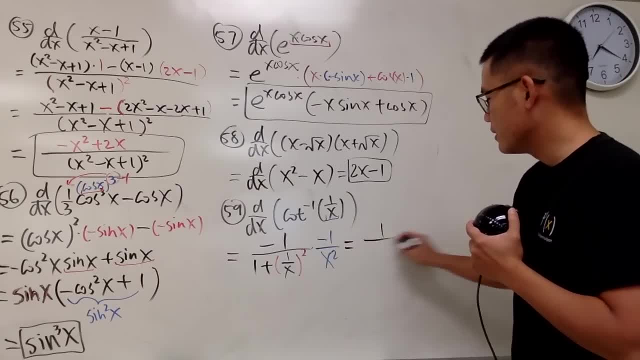 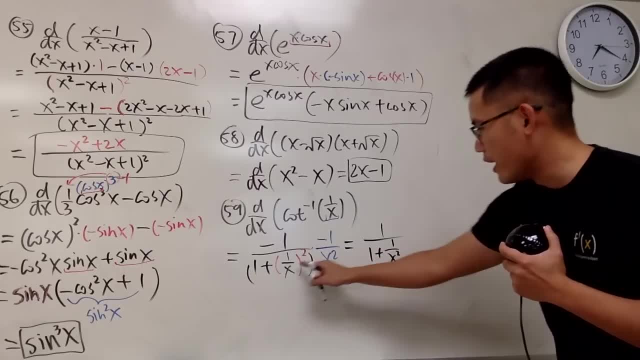 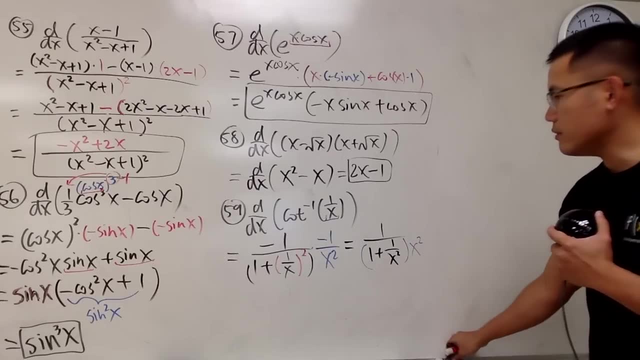 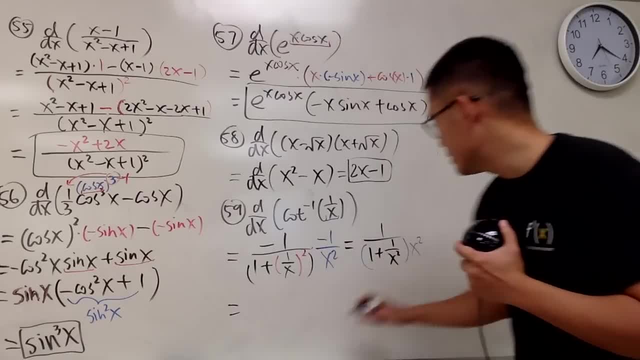 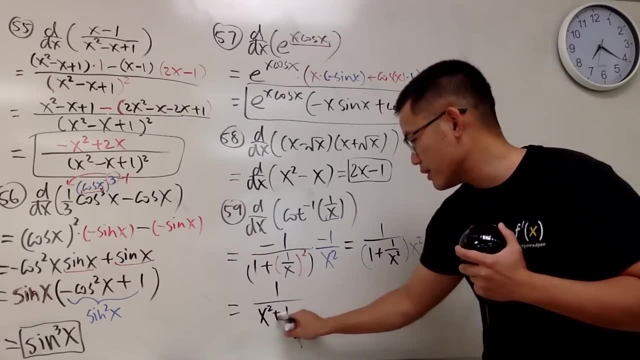 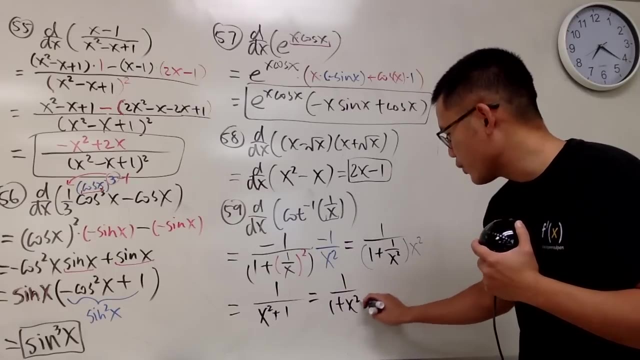 So, all in all, you actually just end up with 1 over. this times, that is x squared plus this times, that is, of course, just plus 1.. Hey, does this look familiar? Of course This is the same as saying 1 over 1 plus x squared. 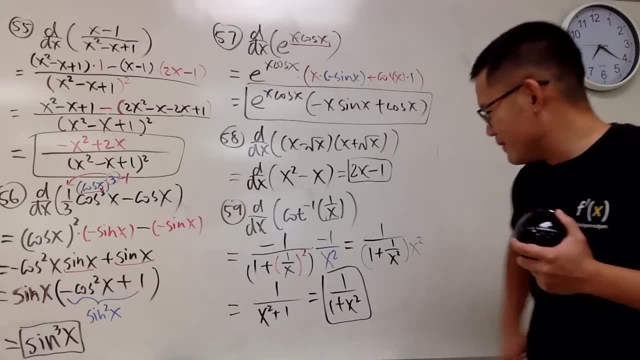 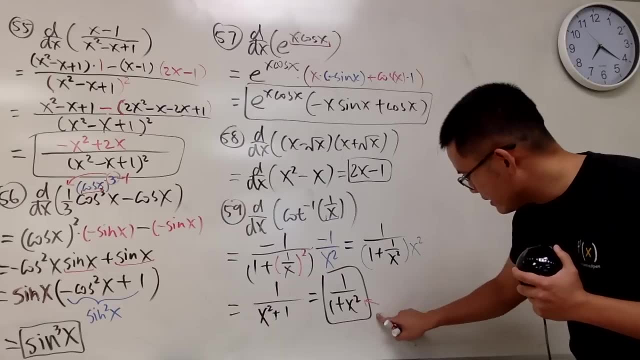 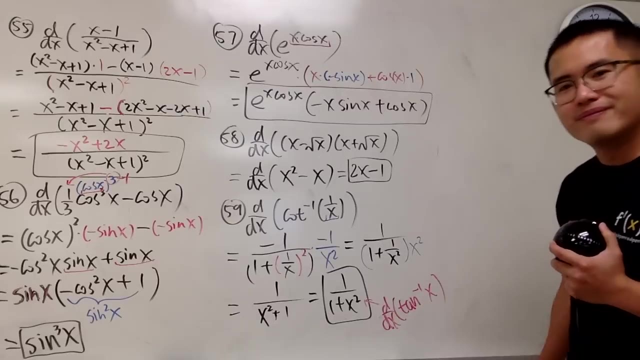 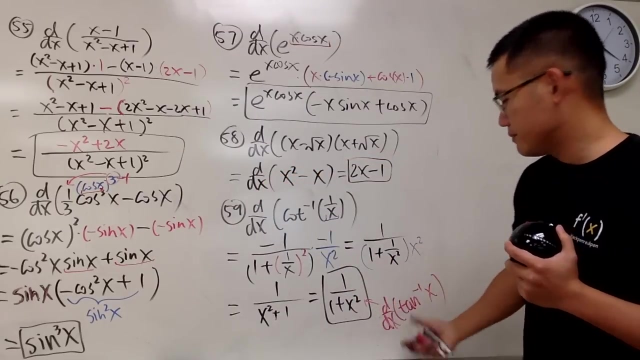 But didn't I say this is the derivative of 3? Sounds like inverse tangent. huh, Yes, In fact, this right here is the derivative of inverse tangent of x. Well, here's a question for you: When the derivative of a function is equal to the derivative of another function, does 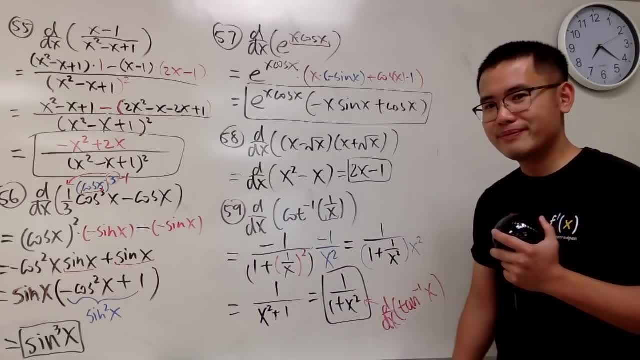 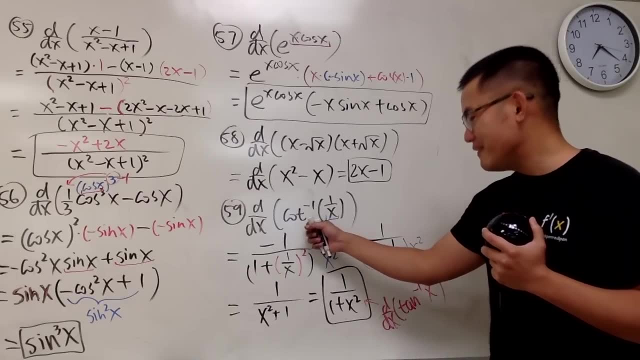 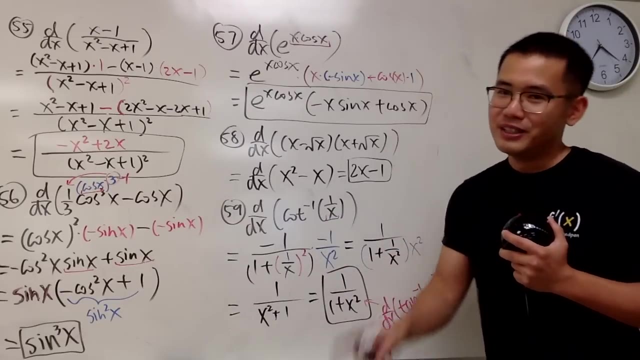 that mean that the functions are equal to each other. In this particular case, this is in fact the same as that, But in many cases the functions might be off by a constant. Check out my other video for more detailed explanation, right? 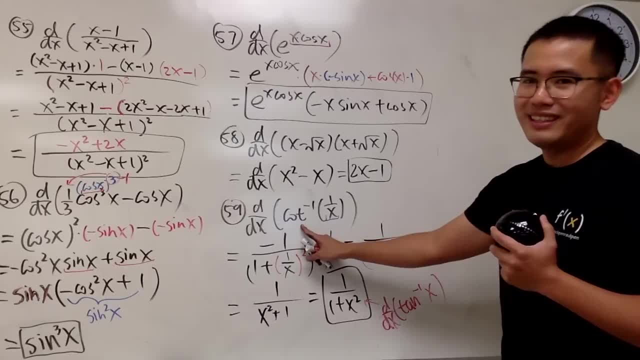 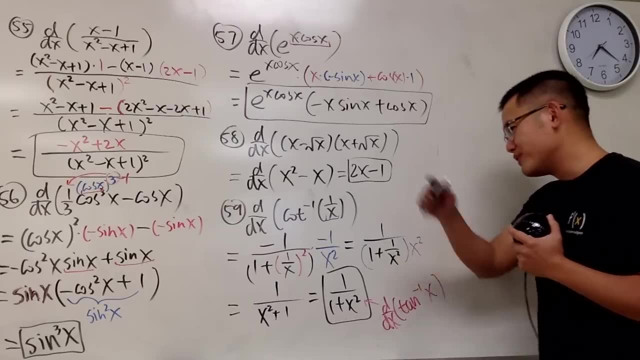 But in this particular case inverse tangent of x. in fact, you can write it as cotangent, Inverse cotangent of. You can write this as inverse cotangent of 1 over x. I'll prove this for you guys another time, waiting for my 100 trick identity, or maybe. 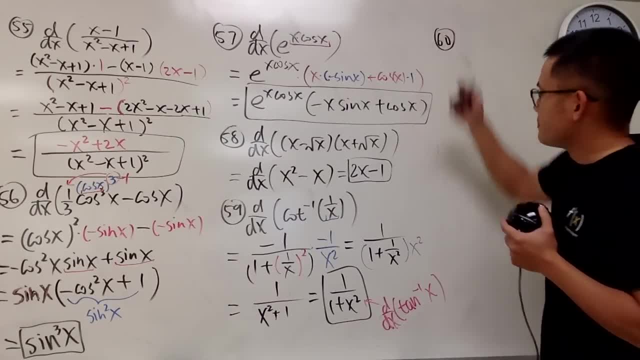 trick problems that you have to solve. Anyway, number 60. So, anyway, number 60. Okay, Okay, okay, okay, I don't know if I can fit it here. Let's see, This is a long one. 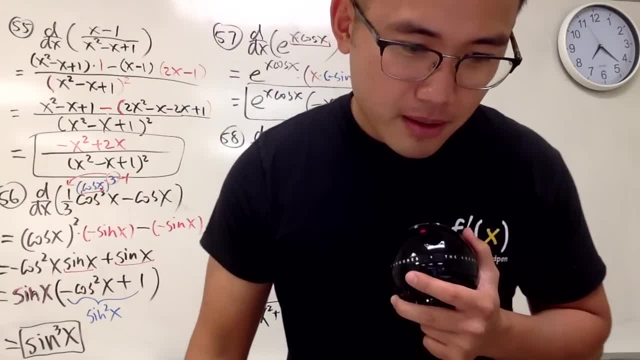 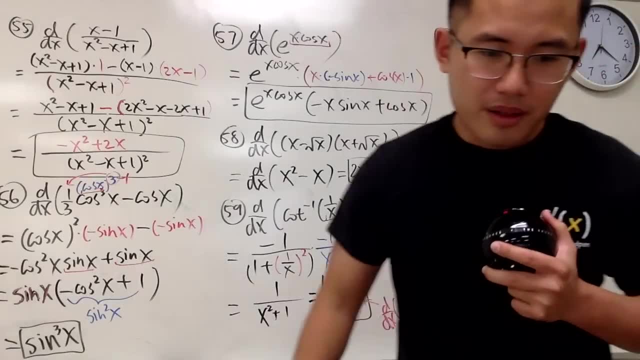 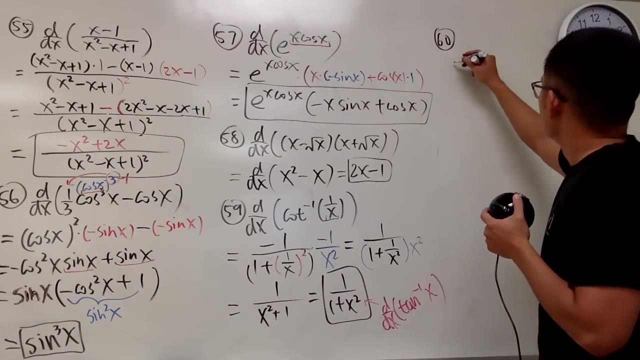 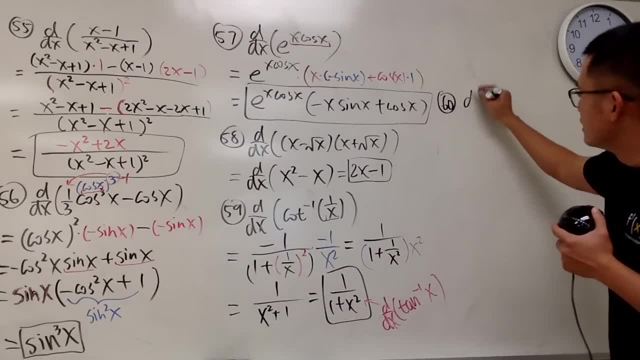 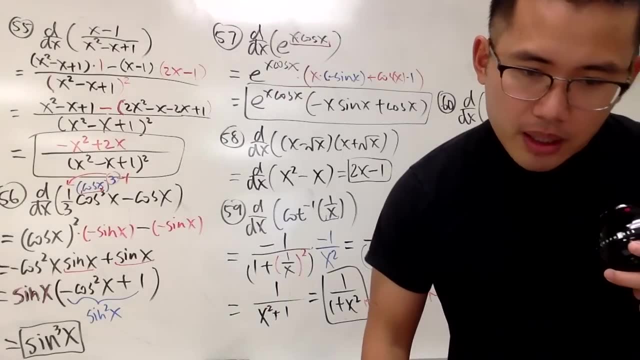 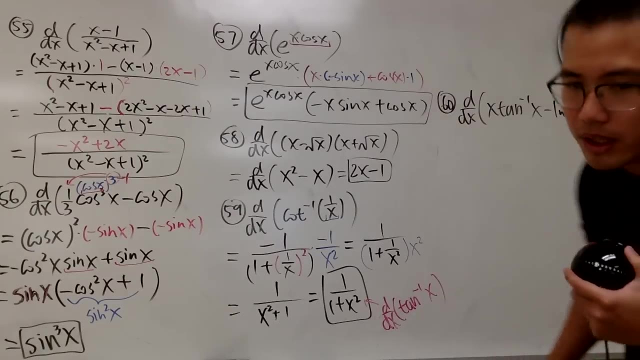 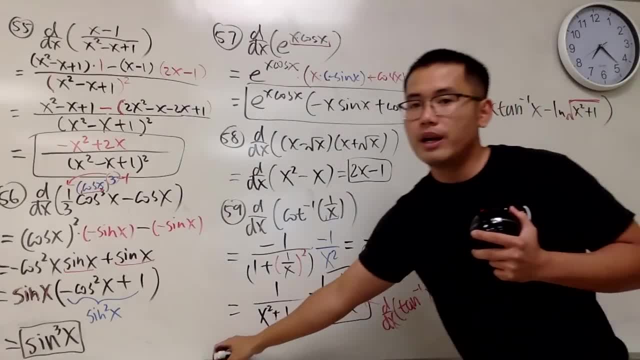 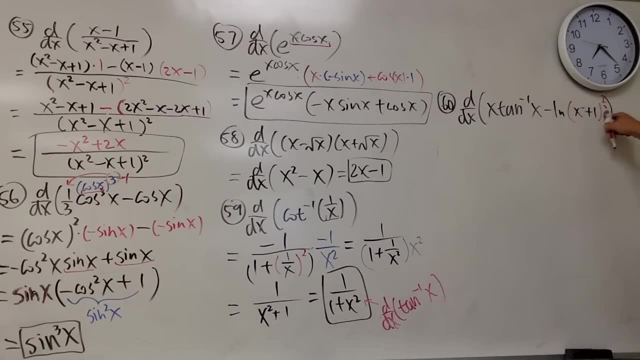 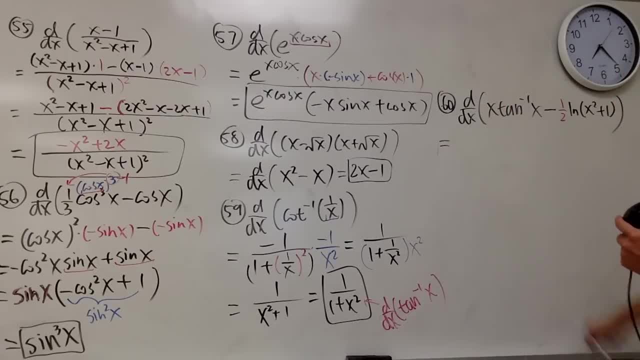 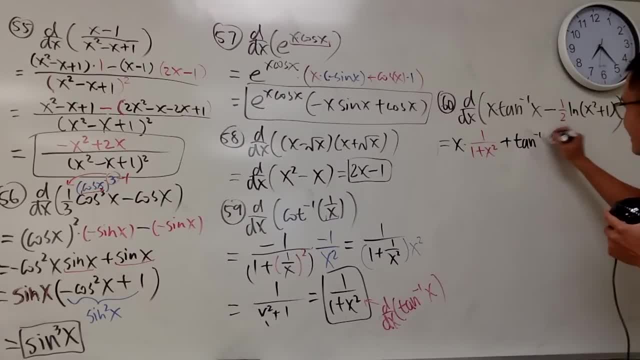 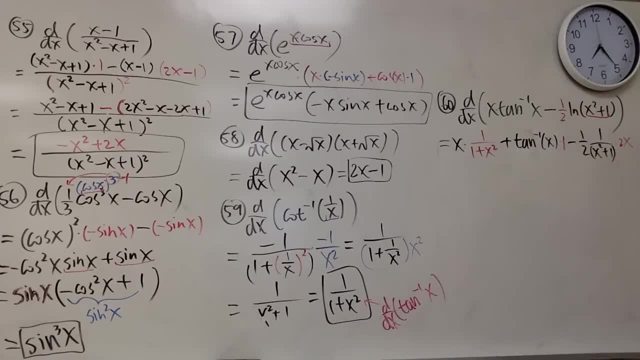 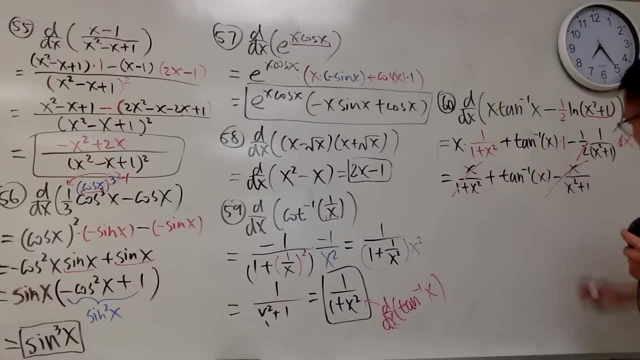 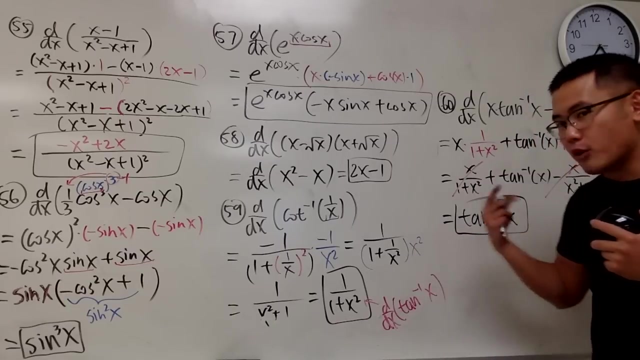 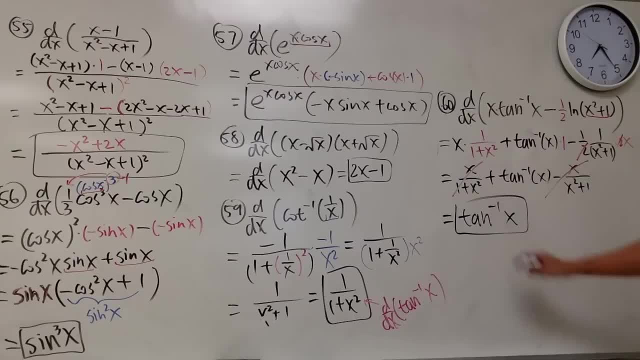 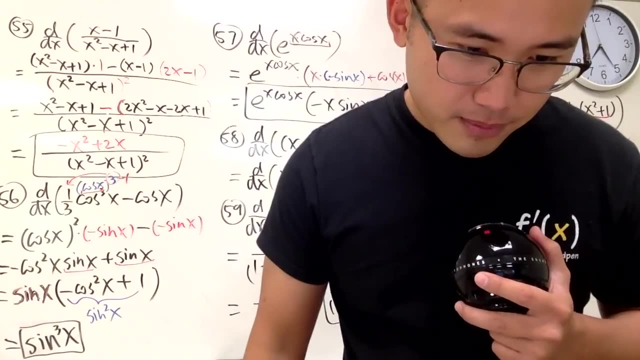 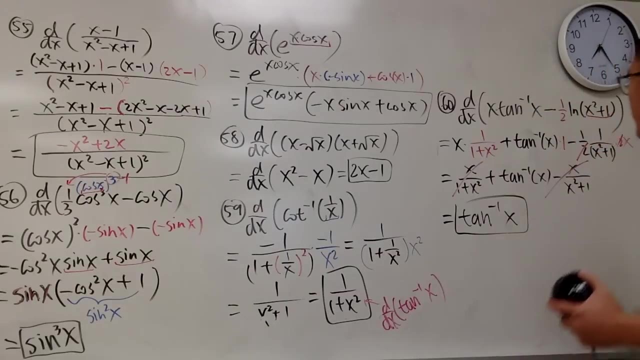 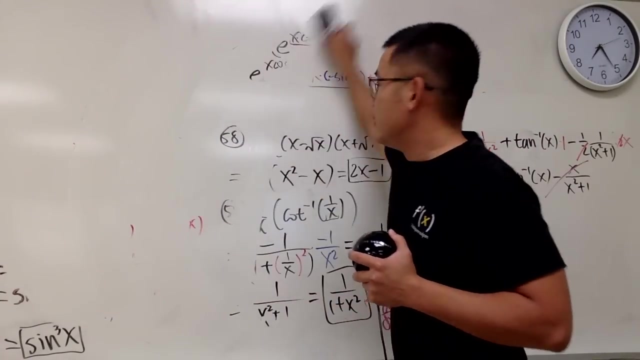 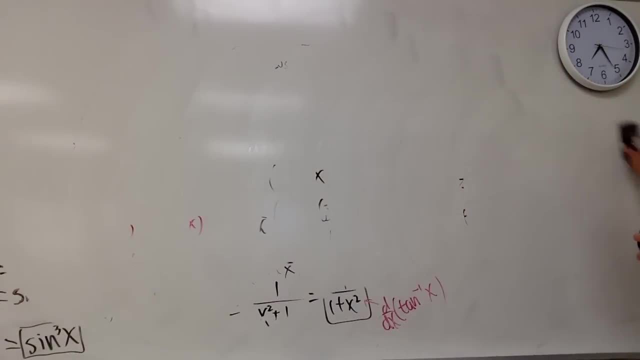 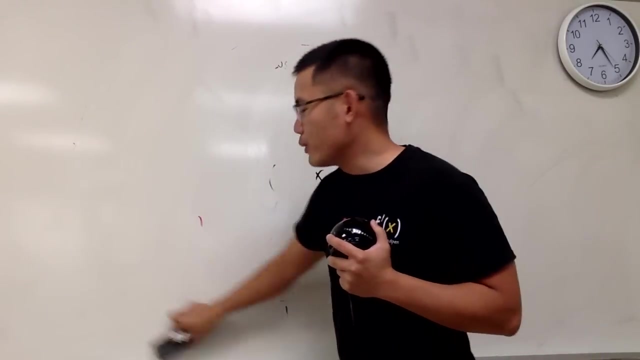 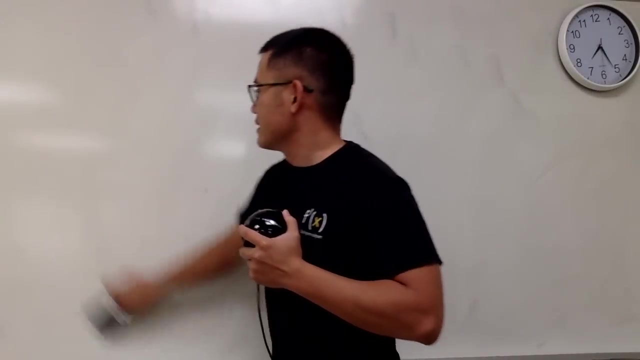 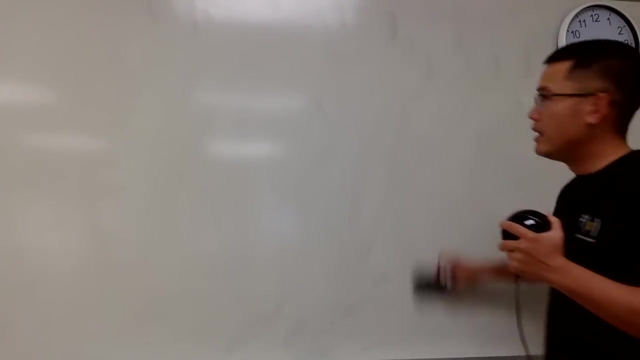 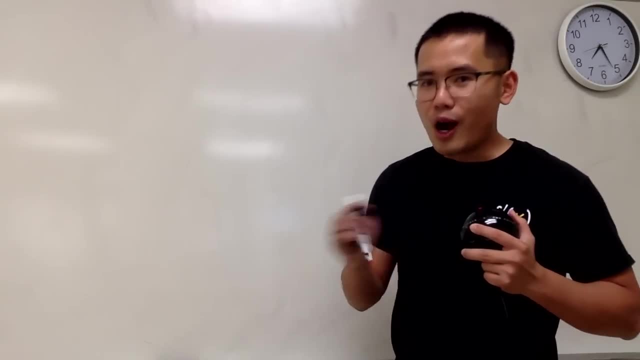 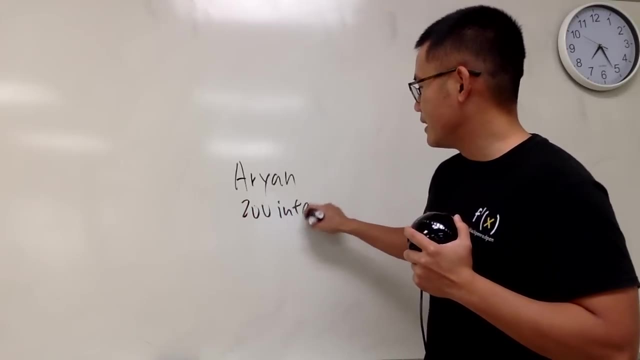 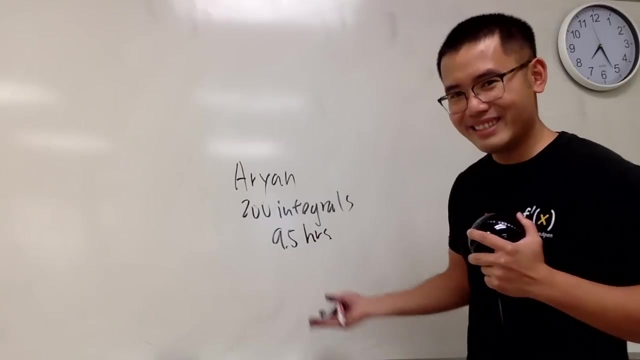 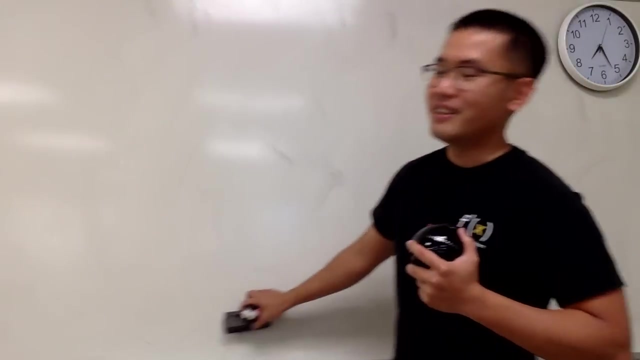 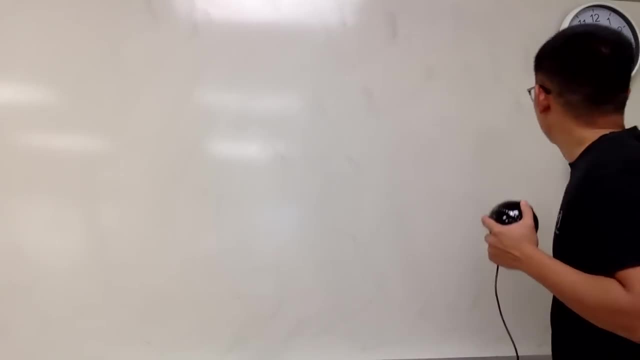 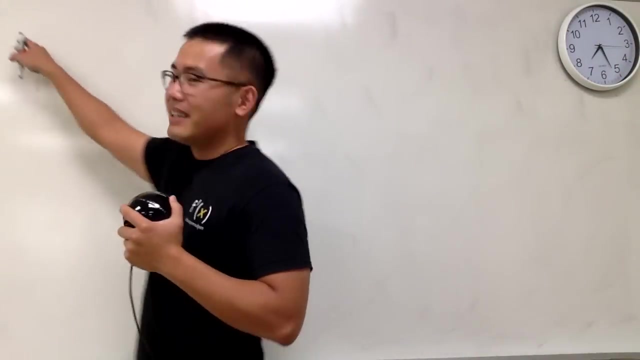 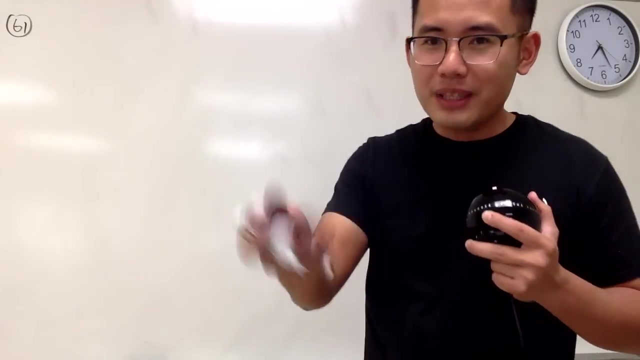 Okay, I don't know. Wow, I'm speechless. OK Yeah, I enjoyed that video a lot, though, because that video gave me that, made me feel like how you guys are feeling right now, like when you watch me doing. 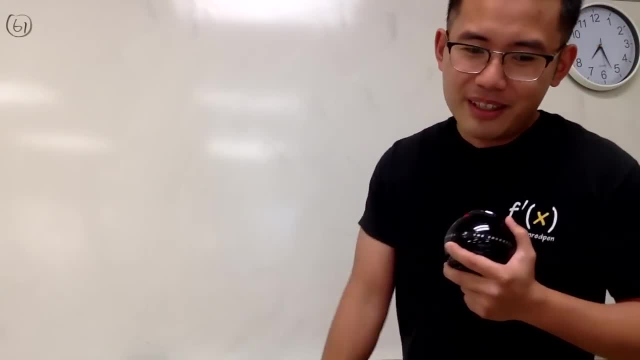 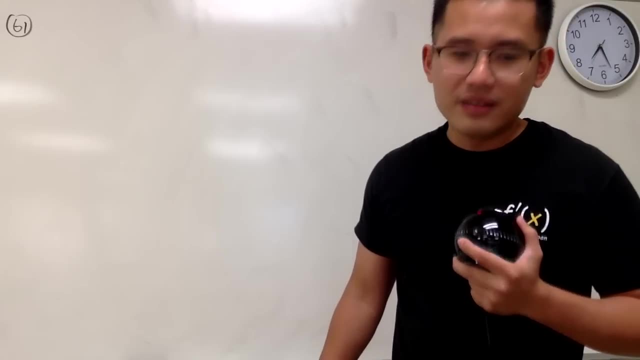 that 100 integrals, 100 derivatives. Yeah, so shalom to Aryan. I pretty much pronounced your name wrong. I'm so sorry, Aryan. I think Aryan. yeah, OK, here we go. Number 61, differentiating: 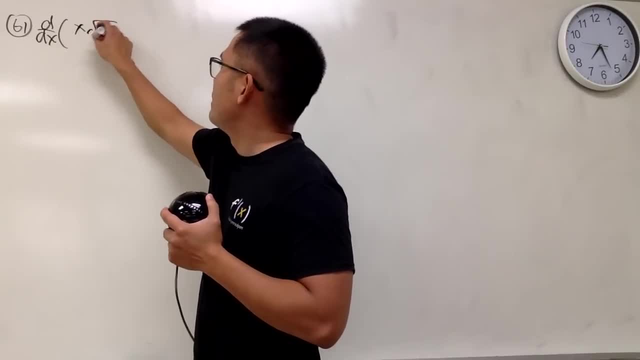 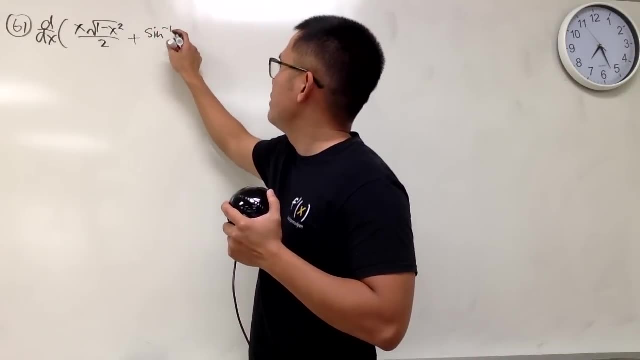 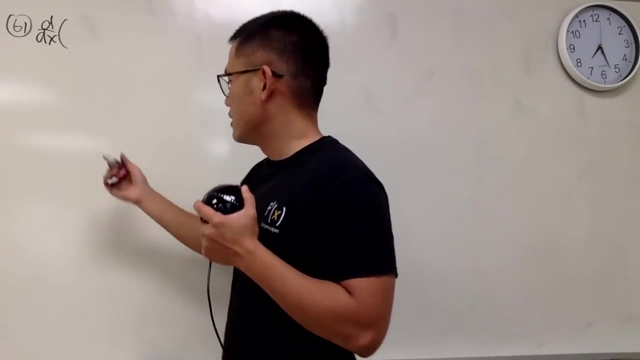 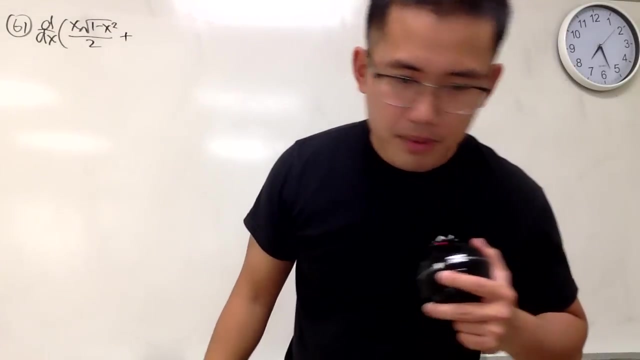 And we have x squared root of 1 minus x squared over 2, and plus inverse sine of x over 2, like that. Let me write down the question better: x squared root of 1 minus x squared over 2.. And plus inverse sine of x over 2,, like this: 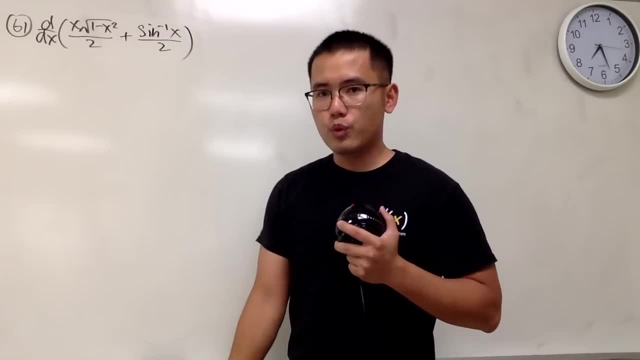 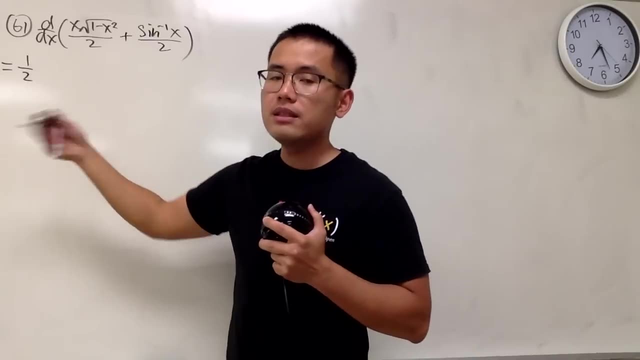 OK, first thing. first, both of them have the over 2.. Do not use quotient rule, though, because over 2 is just a constant multiple. Perhaps it's better if we put a 1 over 2 in the front. That way it doesn't bother us too much. 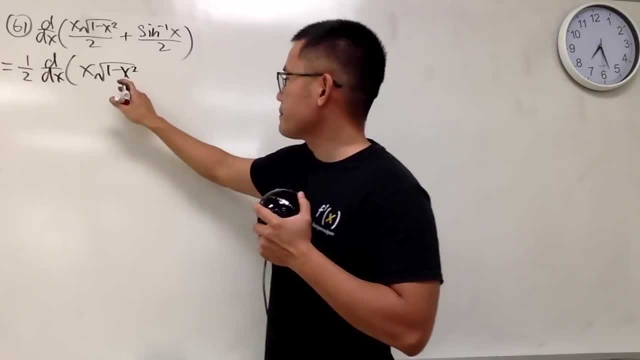 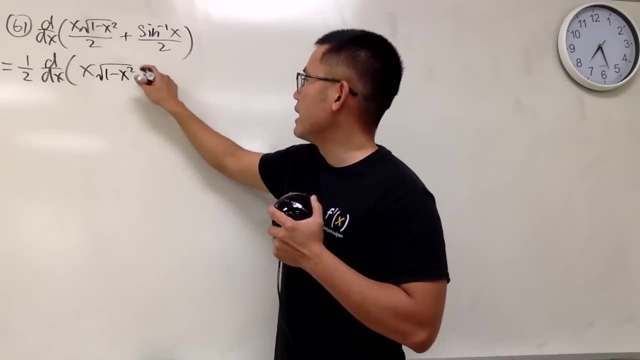 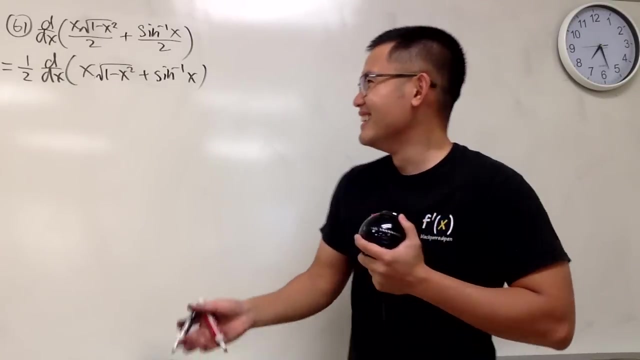 So that we can look at x times square root of 1 minus x squared And then plus inverse sine of x. I think this right here looks slightly more, slightly less intimidating. I don't want you guys to feel like, oh man. 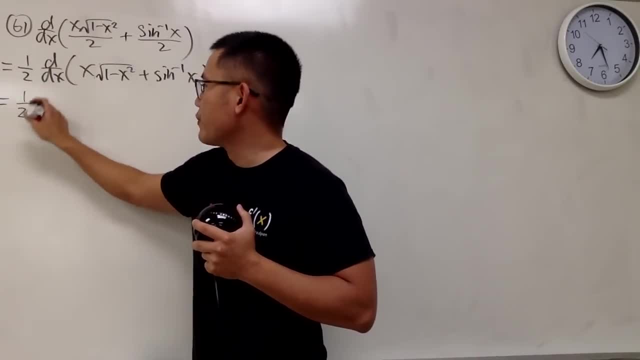 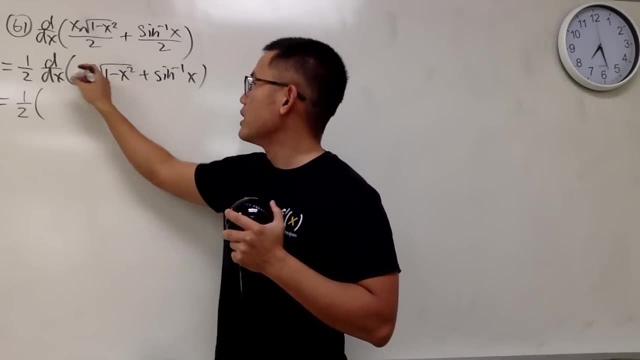 I just made the question worse. Anyway, here we go. Put down the 1 half all the way in the front. Open the parentheses for the result of differentiation. Here is the deal. We have to use the Prada rule. Keep the first function, which is x times the derivative. 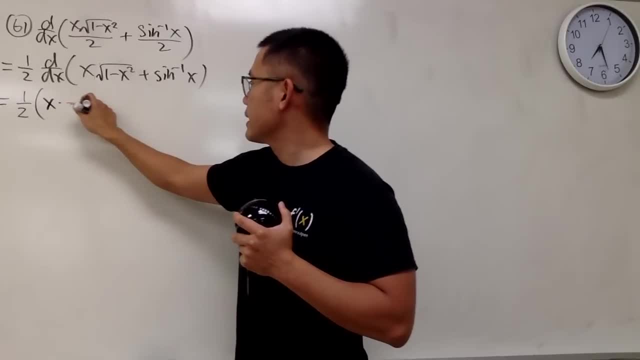 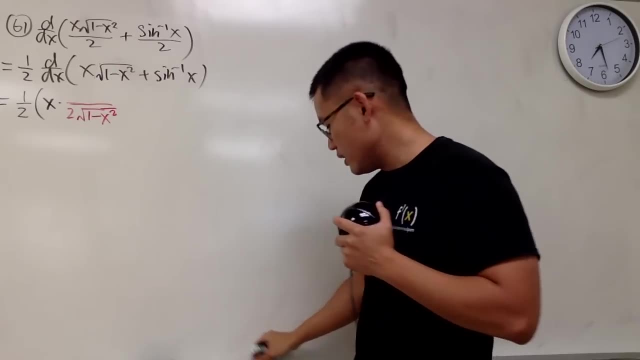 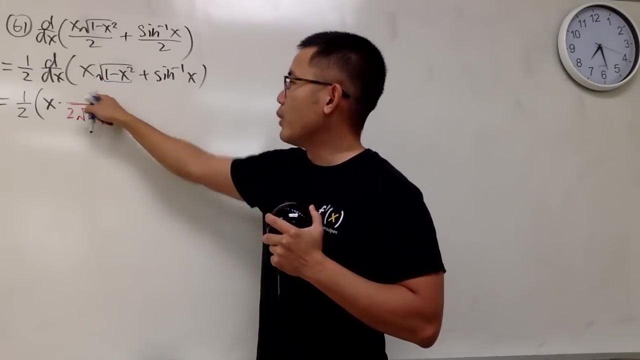 of the second. The derivative of this is 1 over 2 square root of 1 minus x squared. But you guys all know the deal: We have to multiply by the derivative of the inside, which that will give us negative 2x. 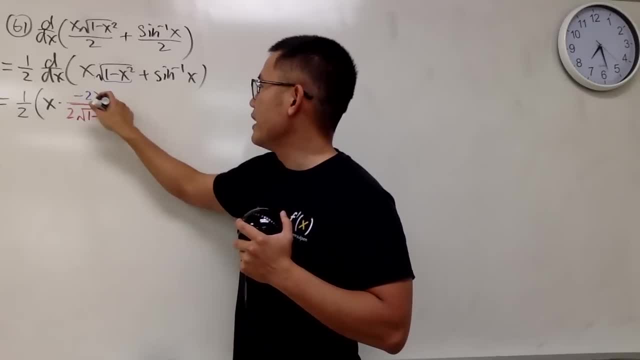 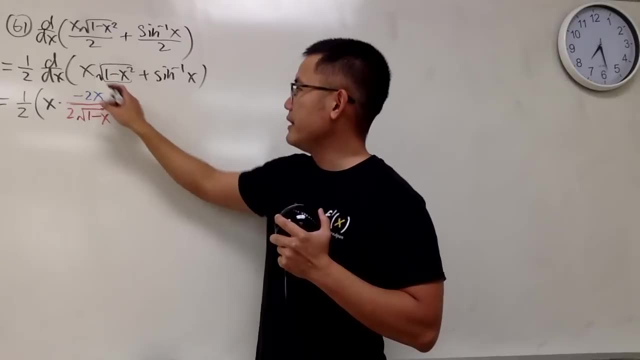 It's 1 times negative 2x. So this time I will just start to put down the negative 2x on the top. Save some space this way. So that's the first part, And then we have to add the second function, which is square root of 1 minus x, squared. 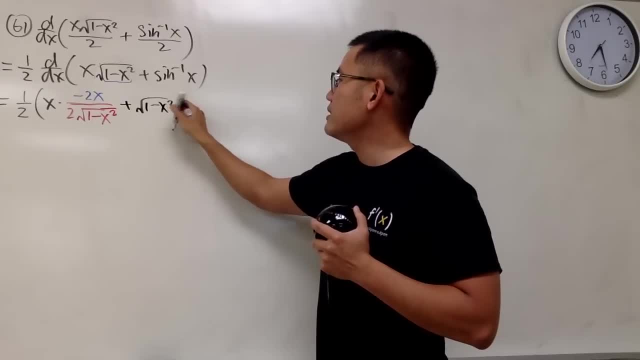 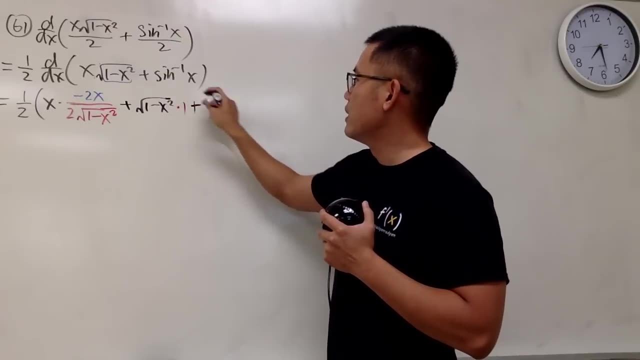 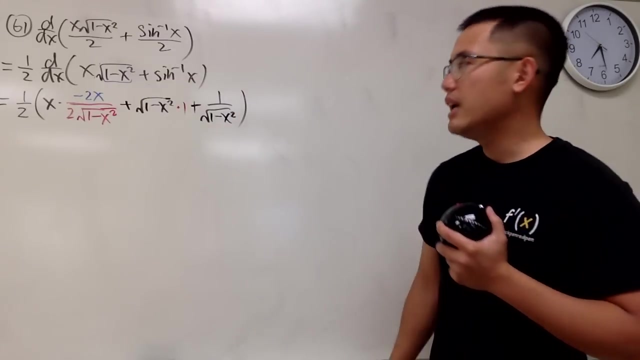 And we multiply by 2.. That's the derivative of the first, which is just going to give us 1, like that. And then this one is just going to give us 1 over square root of 1 minus x squared. That's the derivative of inverse sine x. 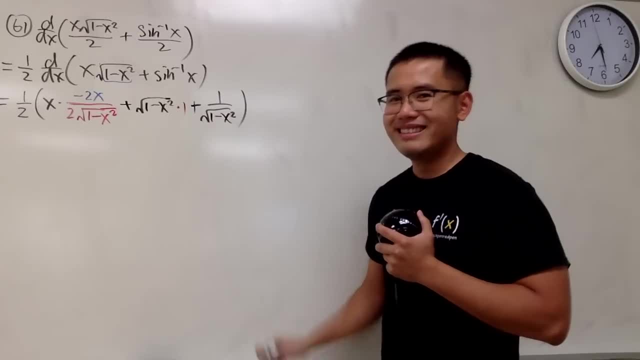 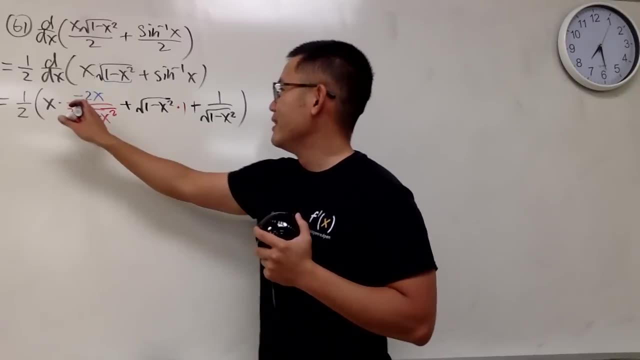 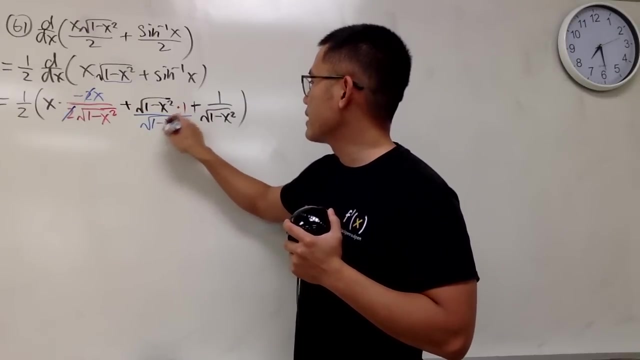 Now the question is now what? It seems that we have to get some common denominator again, So we will get the common denominator, isn't it OK? So cancel this out. first, though, Right here, let's just multiply the bottom and the top by 1 minus x squared. 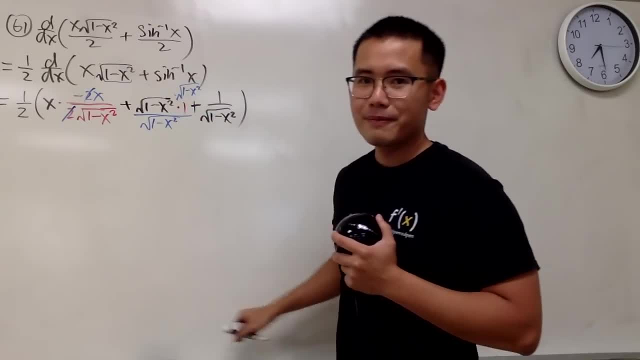 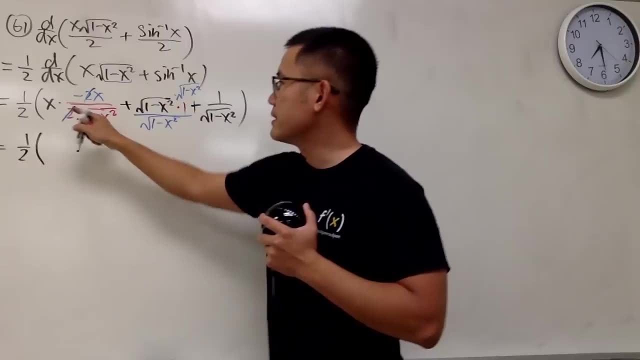 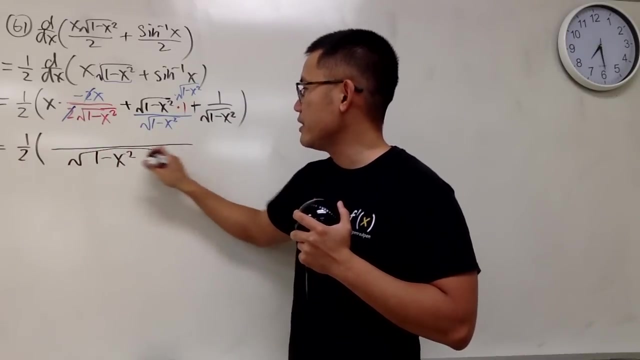 I'll also multiply this right here. OK, So we will see the answer right here is: well, the result is so far 1 over 2 times. Here we have x squared. Well, everybody has a square root of 1 minus x squared for the denominator. 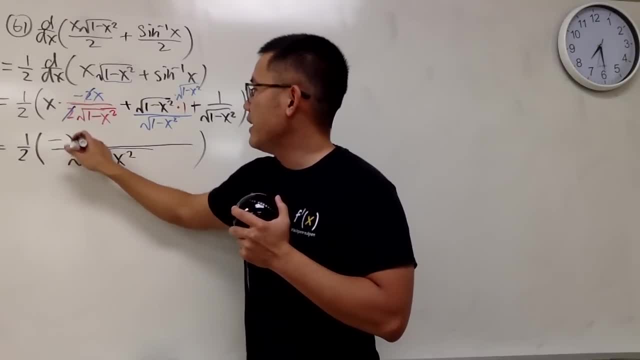 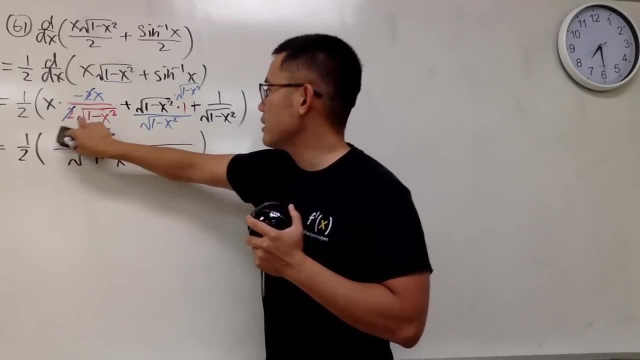 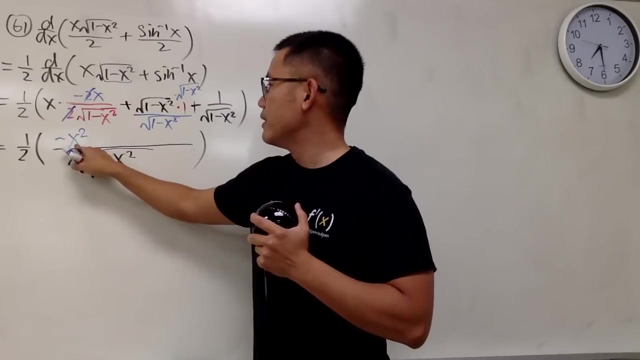 So let's put that down. This guy has negative x squared. This guy we add and just put down. let's just put down: this guy different color, This guy has negative x squared. first guy, Next guy plus. 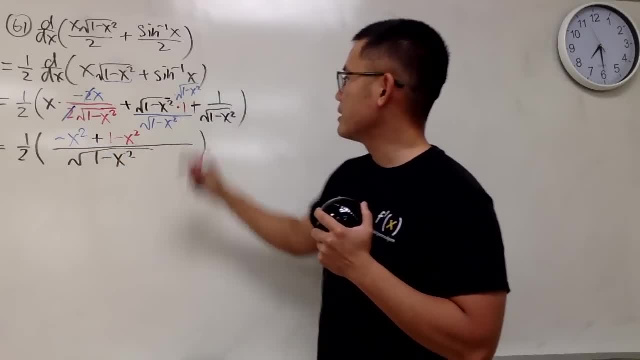 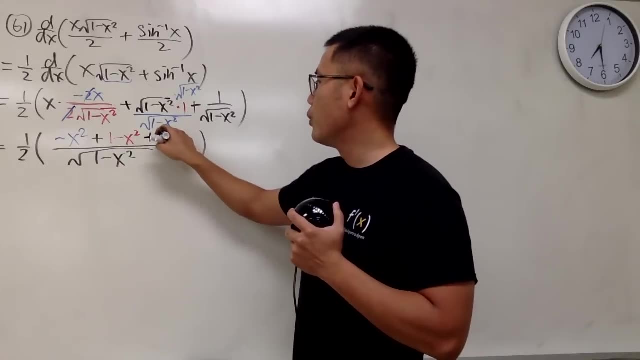 This times that is just 1 minus x squared right. 1 minus x squared. Lastly, we have to add: this guy is just 1.. So we have to add 1.. circles 1,, 2,, 3,, 4,, 5, 6.. 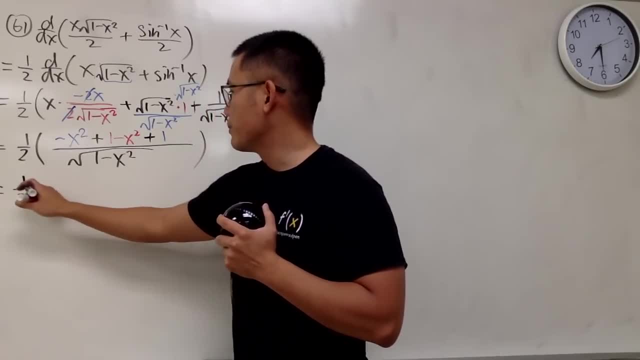 So it's 1.. There's also an Yangtze problem, So we get 1 squared plus 2 multiplied by 0.. This is the last one that we have Here. let's do it again. OK, So let's do it again. 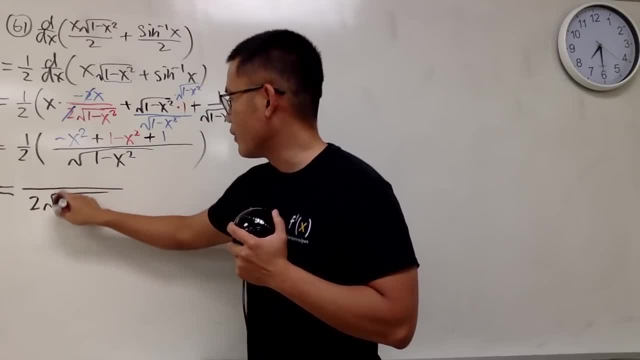 So 1 minus 2 times x, squared 1 plus 1. We have a square root of 2.. This is a square root of 2. And we have two squares. Well, we can put these down together already, So we will. 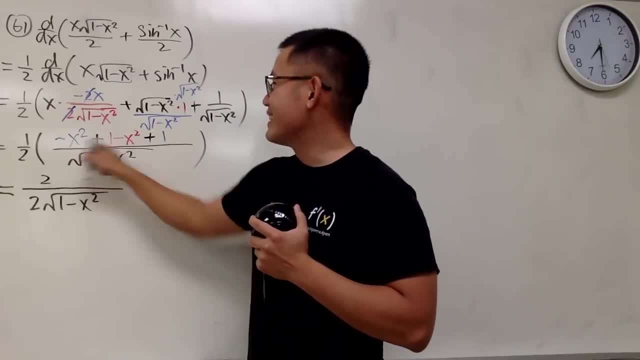 OK, Here's the e-cosine. OK, Here we go Two times. this is 2 times the square root of 1 minus x squared. 1 plus 1 is 2.. This times that is negative 2x squared. 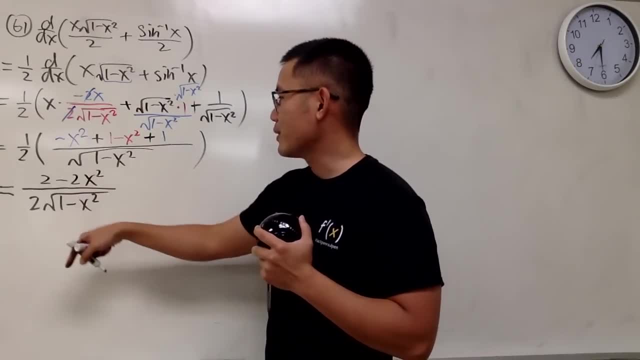 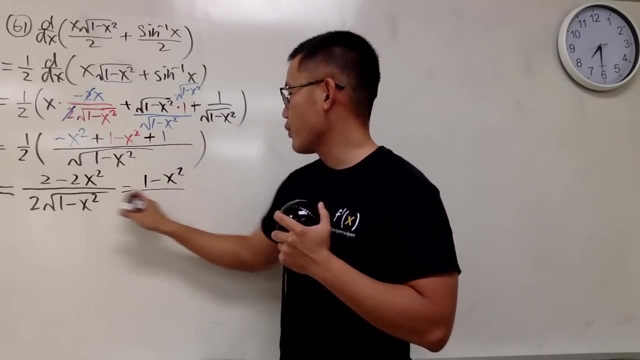 OK, Let's simplify a little bit bit. Of course we can factor out the 2 and all that, So reduce the 2, so we get 1 minus x squared over square root of 1 minus x squared. Just reduce the 2.. Just factor out the 2s. 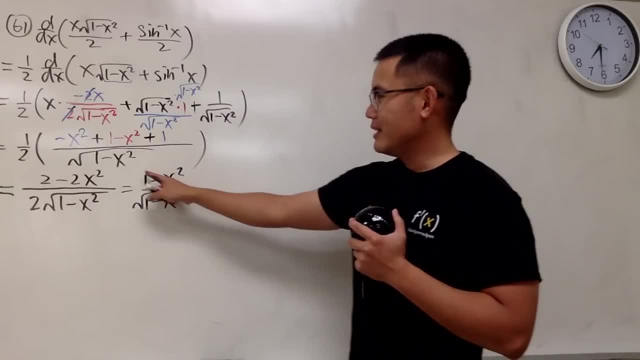 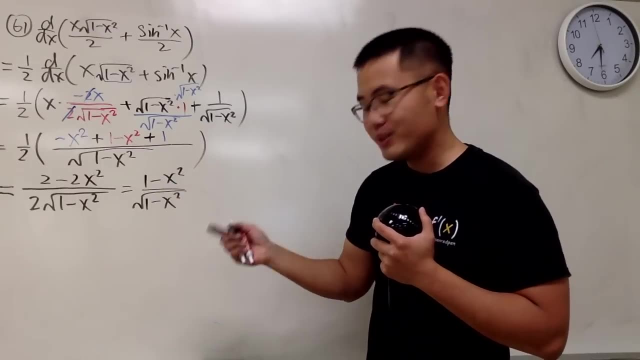 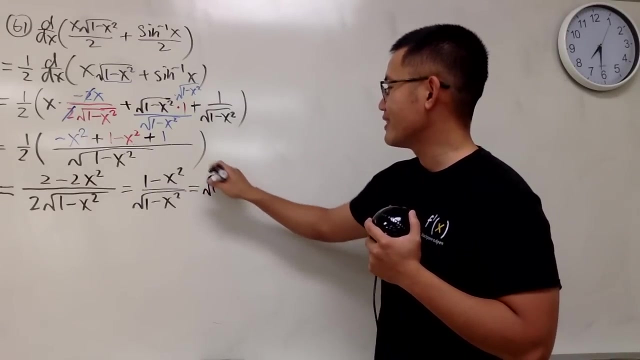 Cancel out. What can we do with this? This and that have the same base. This is to the first power over. this is to the 1 half power. 1 minus 1 half is 1 half Positive though, So you end up with square root of 1 minus x squared. Very good, huh, Yeah, In fact. 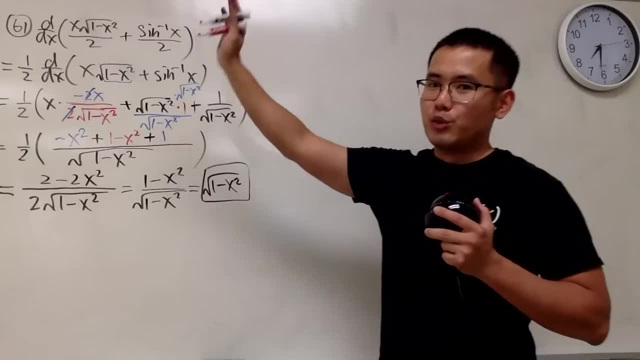 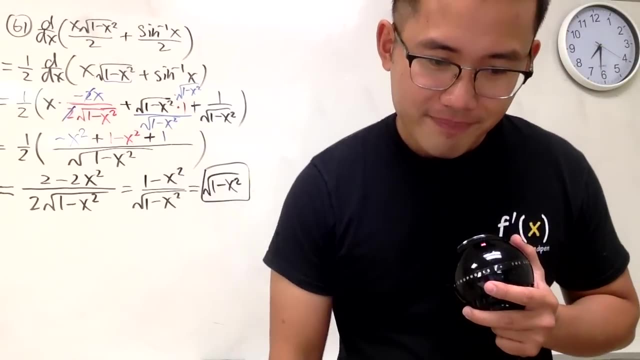 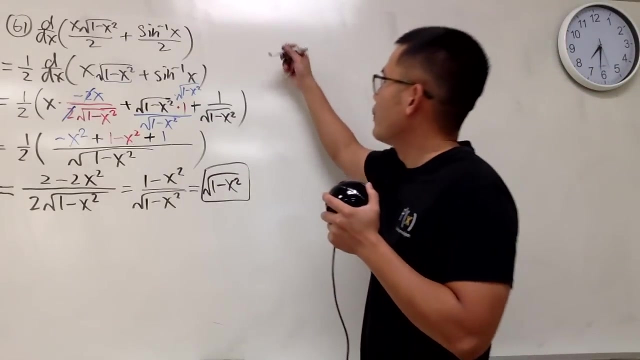 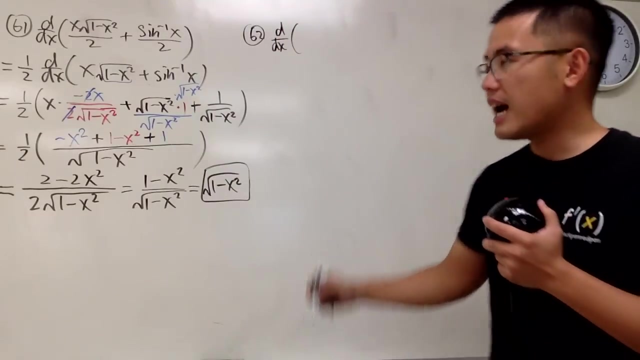 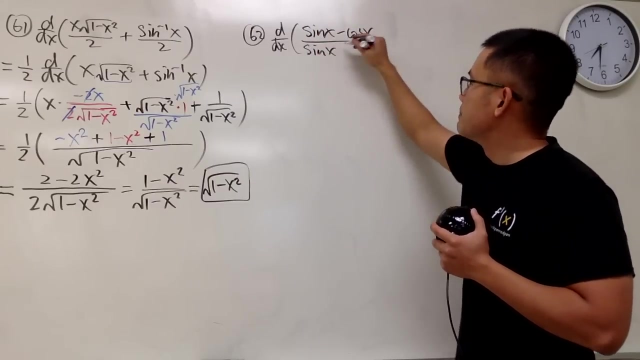 this is another calculus 2 question. Can you find derivative of what function will give you square root of 1 minus x squared as the answer? I'll just do it here: 62.. I want to have more space dx. Here we have sine x minus cosine x over sine x plus cosine x, like this Quotient rule. 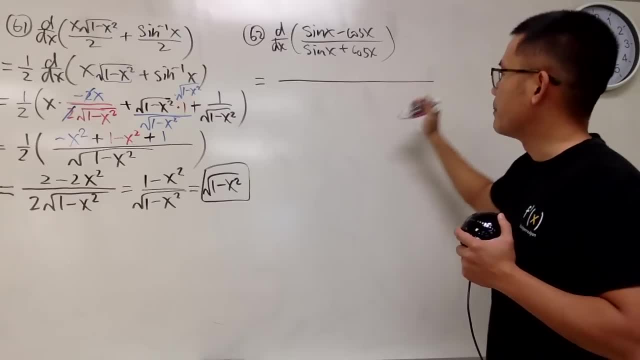 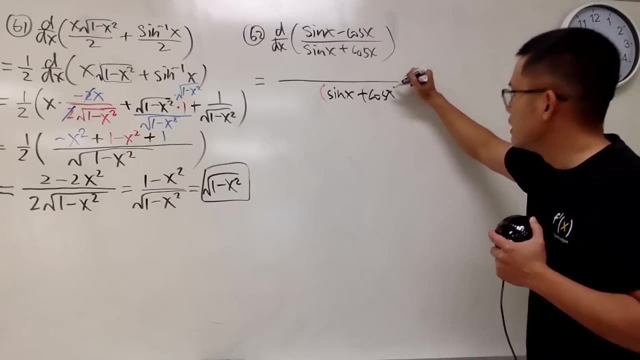 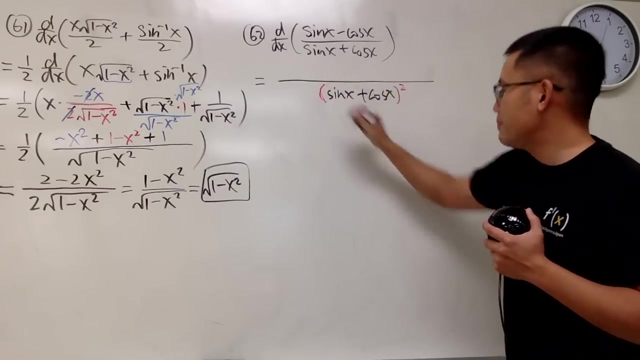 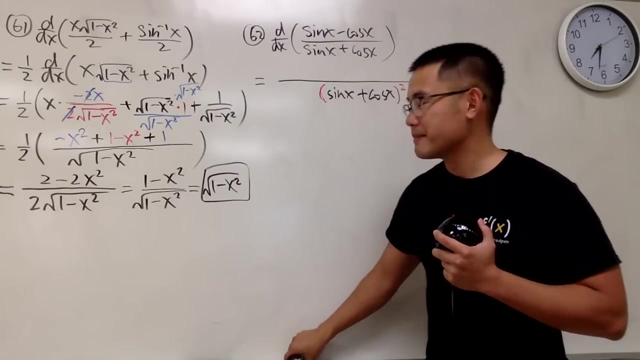 in action. Go ahead and square the denominator. So we will square the denominator Sine x plus cosine x, And here is the square of the denominator. Okay, The red pen is kind of like tired. Okay, So we'll see. Anyway, On the top Put: 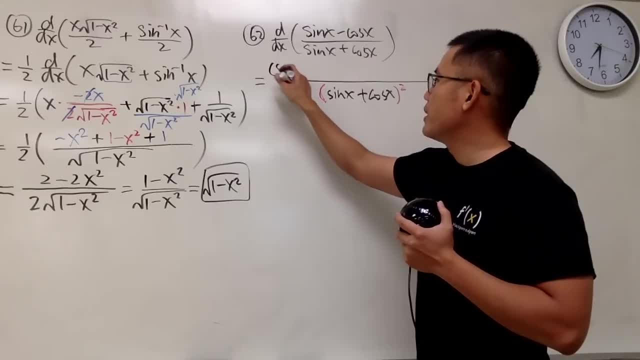 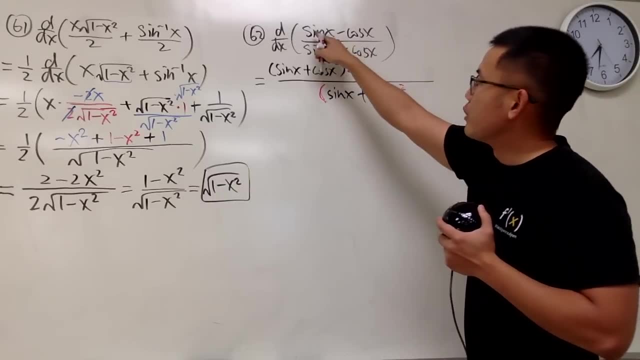 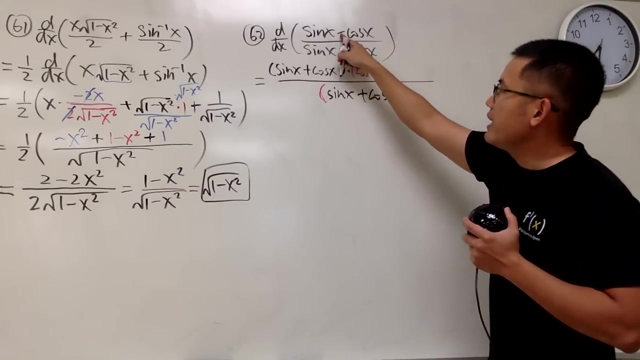 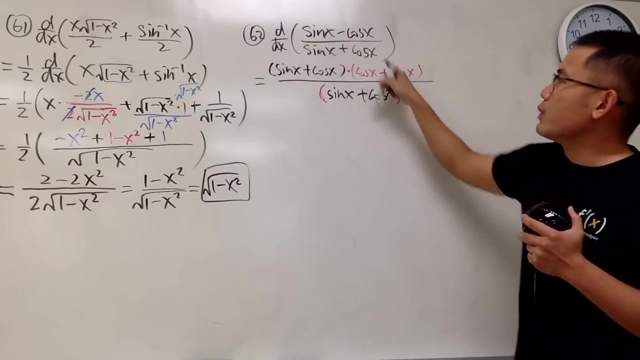 this on the top. So this right here we have parentheses: sine x plus cosine x, And then we have to multiply by the derivative of the top. Derivative of sine is cosine x And the derivative of negative sine x is positive. sine x- Negative cosine- will give you positive. 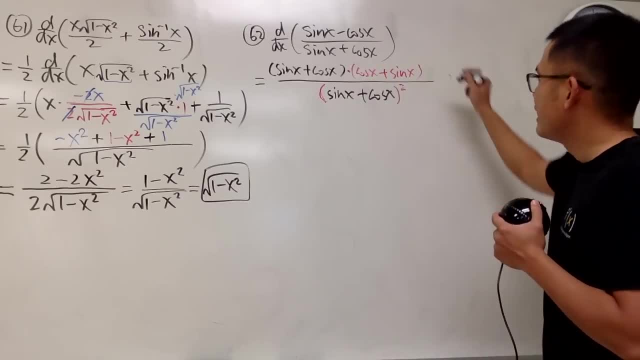 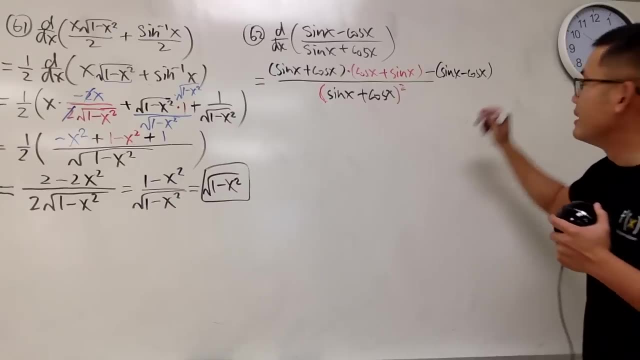 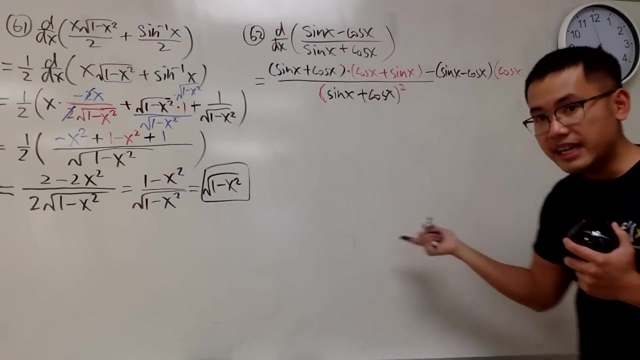 sine. Okay, So this is what we have. Then we minus the top function, which is sine x, minus cosine x. Then times the derivative of the bottom, Derivative of this is cosine, Derivative of this is negative sine. So we have minus sine x. 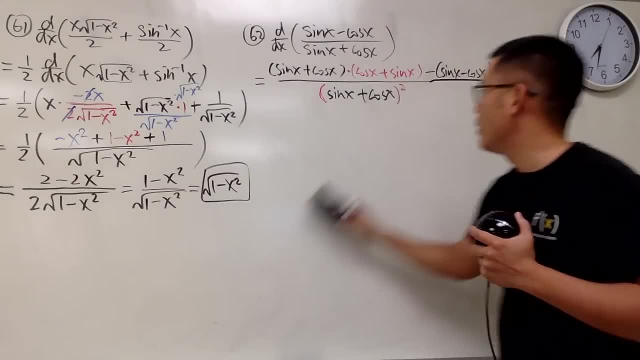 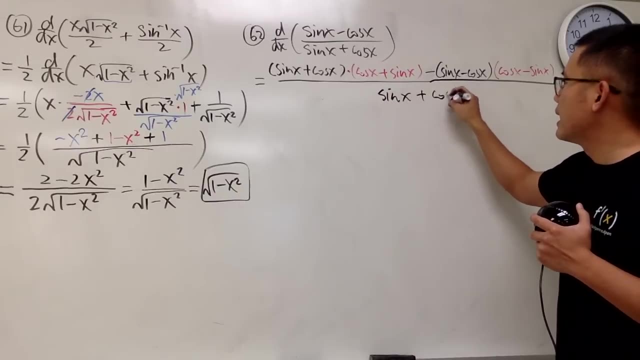 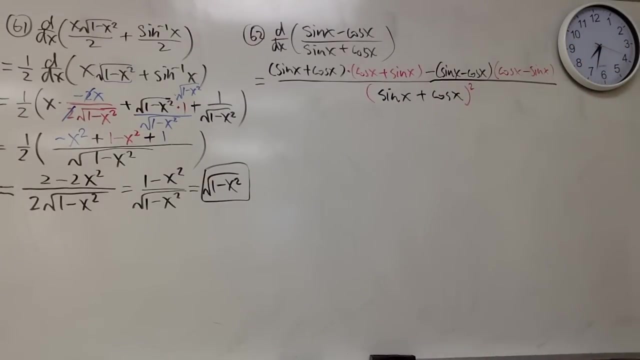 Right here. Wow, Whoa Man, Crazy looking expression. huh, Okay, Let's calm down And we shall be able to. I want to cancel things out. Let me just double check to see how it happened. Of course, you cannot just say I want to cancel things out without Okay, I guess. 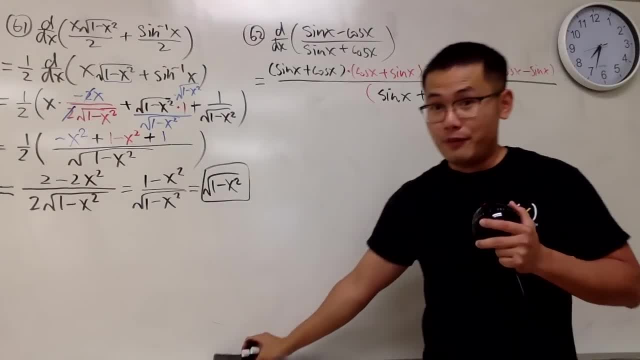 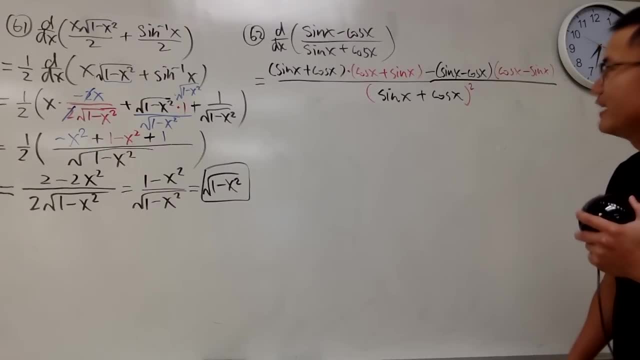 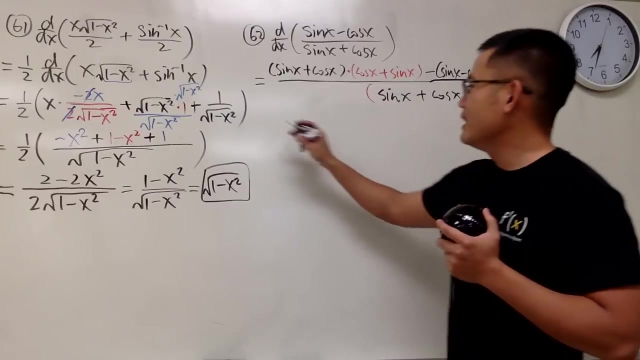 we really have to multiply things out because on the top, unfortunately, we cannot factor anything. If you switch this, it becomes positive. That's not, cannot really factor. I was thinking about To factor with difference of two squares, But you know what? Let's just deal with this. 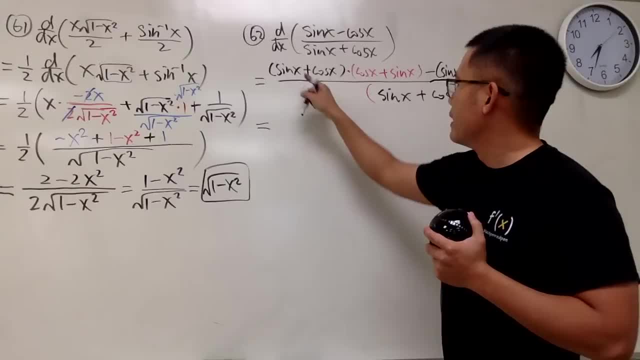 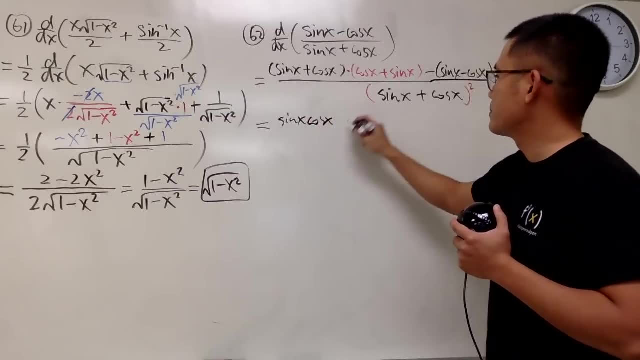 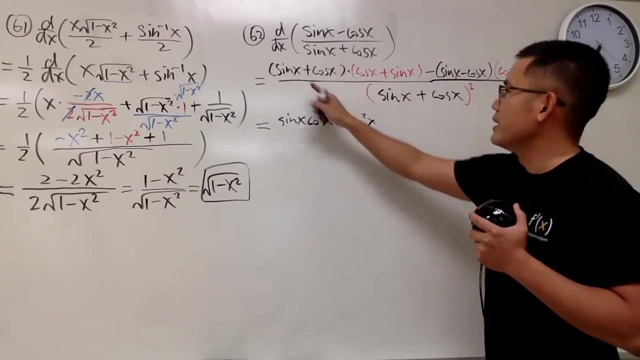 Let's just multiply things out. So so here we go: Sine times cosine right, So sine x, cosine x, and then sine x, so plus. I know this is just sine plus cosine squared. I'm not sure I've done that, but it's too late. And then, this times, this is plus cosine squared. 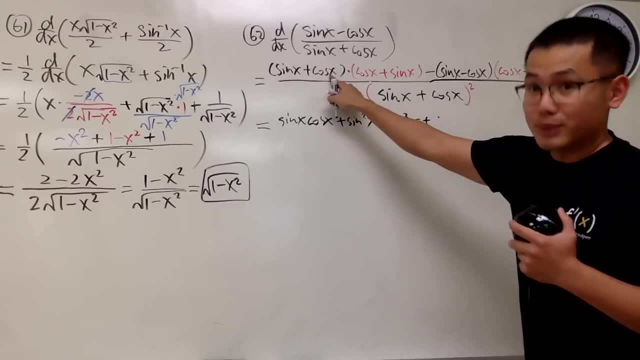 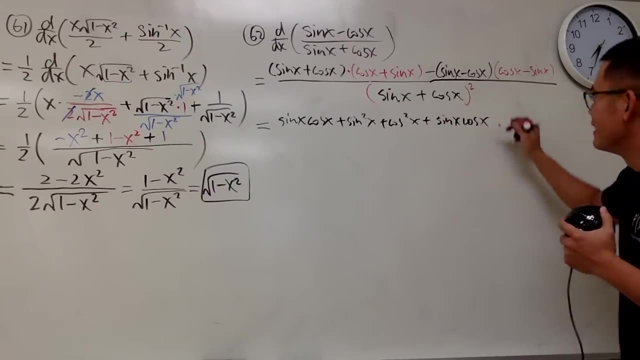 x. and then lastly, plus sine x times cosine x. Yeah, So sin x cosine x. okay, Okay, now minus, multiply this out. we have sin cosine. this times, that is minus sin square x. and then I know I should have just used the binomial theorem. 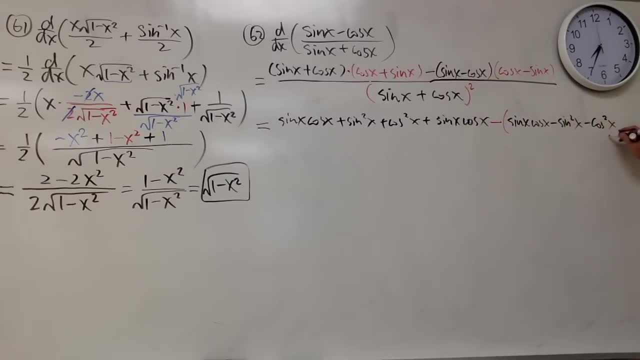 I seriously should have done that, plus sin cosine. yeah, This is sin cosine, Can we see? okay, Yes, Okay. so this is what we have, and all over the denominator, I will just write it down like this: okay. 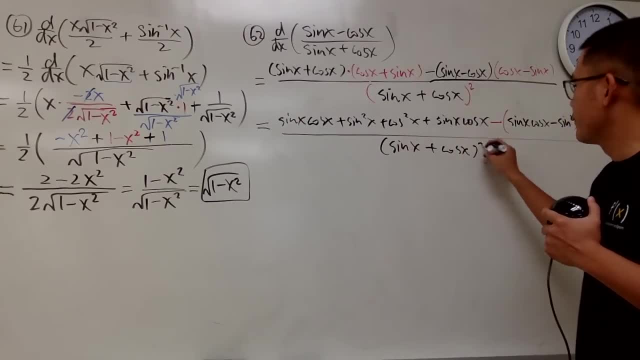 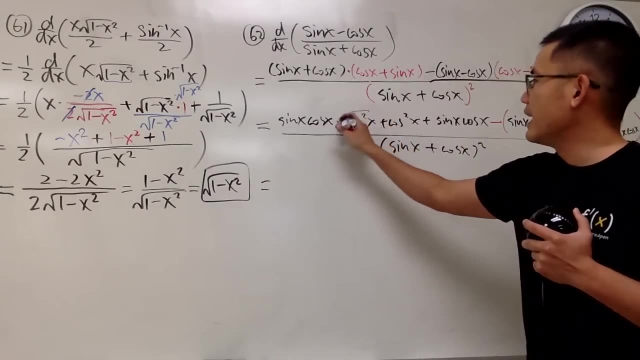 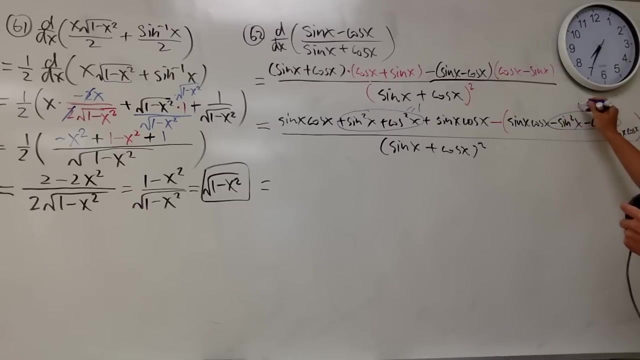 I want to show you guys all the legitimate work. Okay, now have fun to reduce, simplify this guys. This guy is just 1.. Okay, negative, negative. this right here is going to give us negative 1, all right. 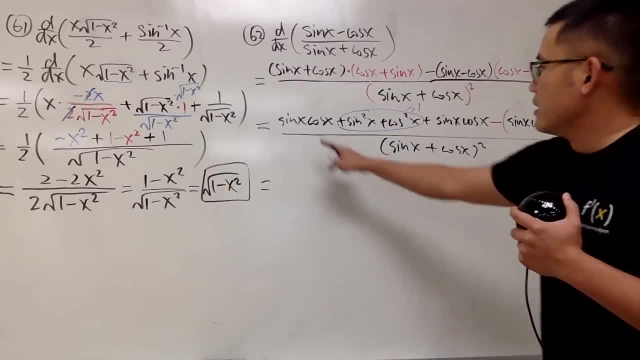 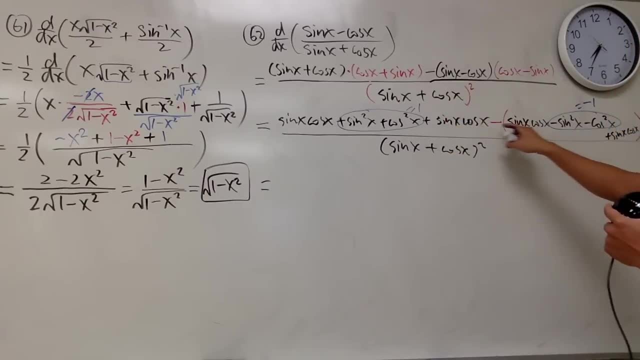 Oh, check this out, check this out, check this out. Sin x, cosine x. so that's 2, 2 of them. Cancel, cancel. Ah, so just imagine, this will cancel with that. this will cancel with that. 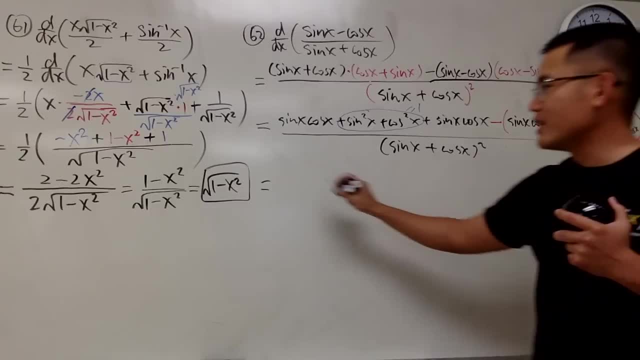 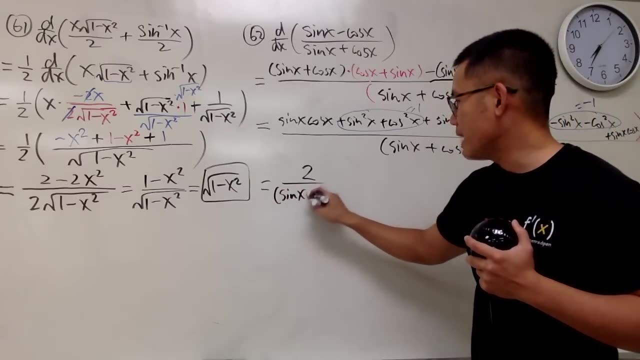 in the end we're just doing 1 plus 1 on the top, so all together we have 2 on the top. Haha, very nice over this guy for the denominator. so I just put it down slightly more compact. 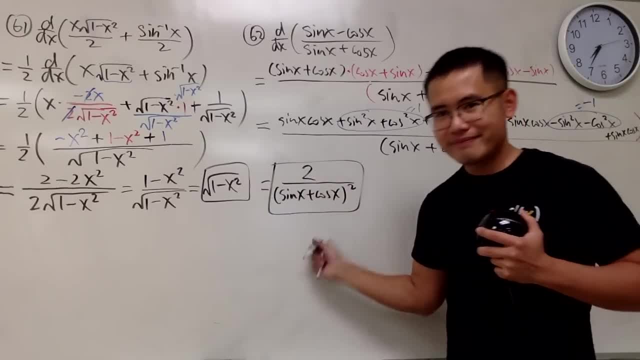 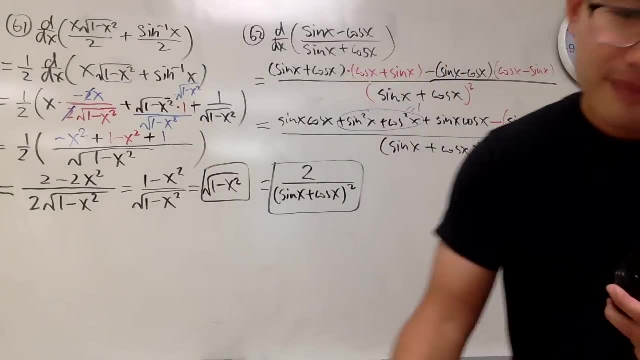 so that it does not look that intimidating. I believe that's the answer and I do have that as the answer choice. That means I did it right. I know the answer, even though I didn't write it down. I know what the answer is. 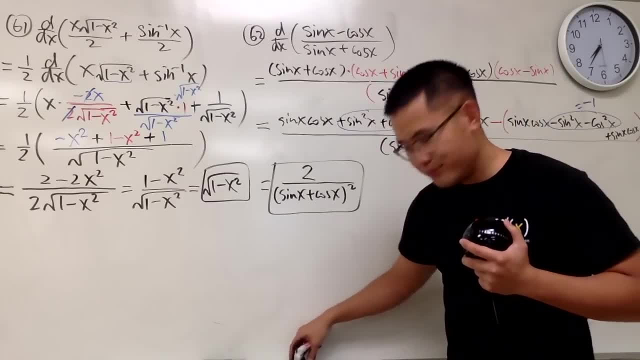 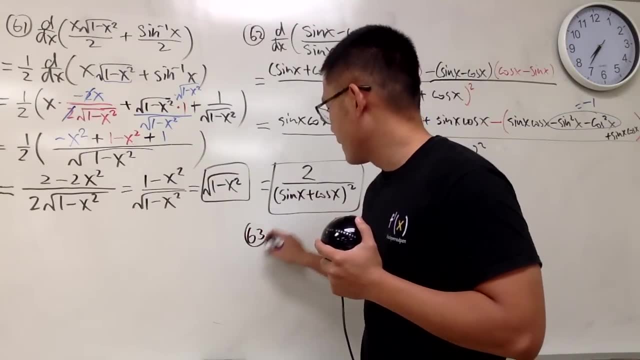 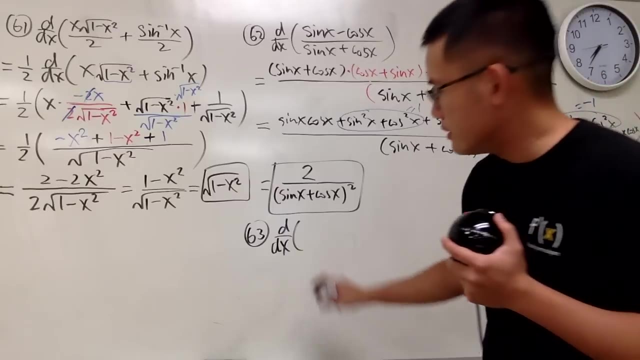 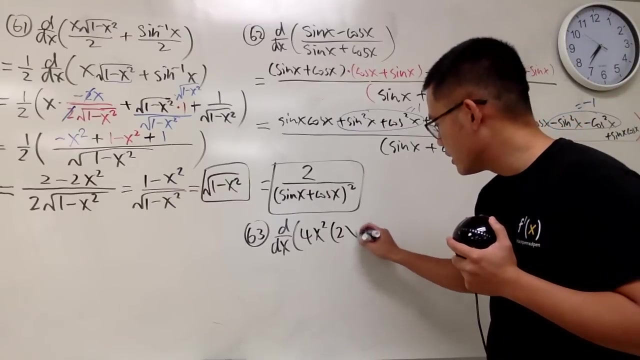 There's a nice pattern. I don't know if you guys figured it out already. You can leave a comment down below and also leave a timestamp, so I know you guys are watching this. part Number 63.. Differentiating 4x squared times 2x third power minus 5x squared. 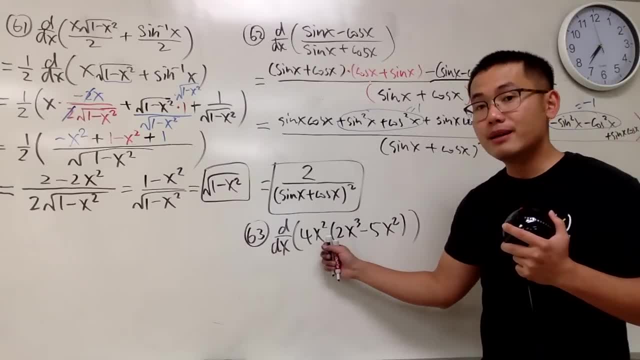 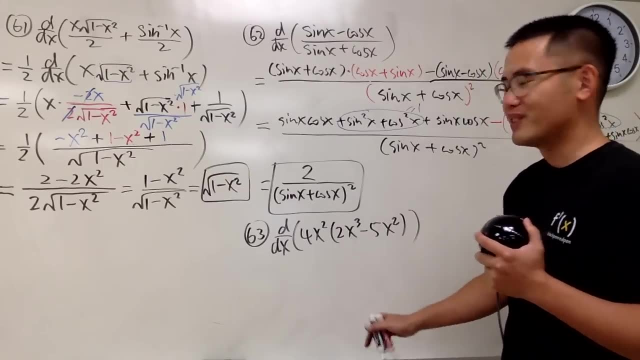 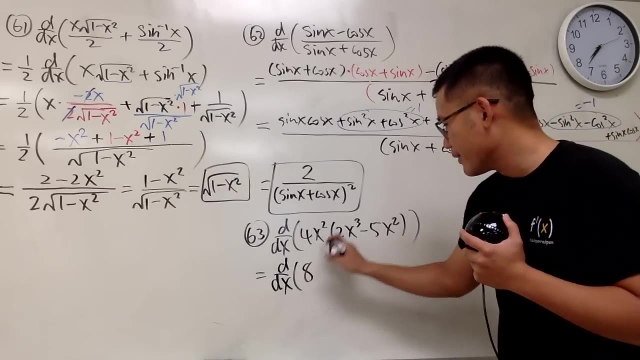 Okay, Ah, it's a product. but should we use product rule? No, because we can do the product in the algebra world first. So let's go ahead, just do the Google things: Distribute. distribute. So 8x squared times x to the third power. 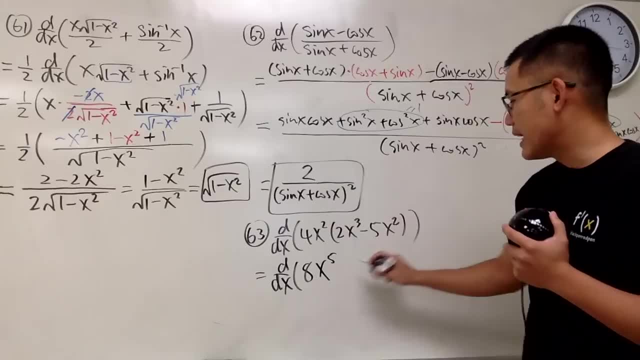 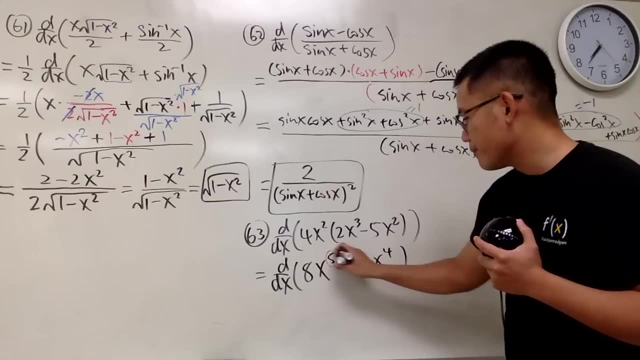 you add the powers, so x to the fifth power- This times that is minus 20, and you add the powers again, so x to the fourth. Now we can just do the power rule Right here Nicely easily. 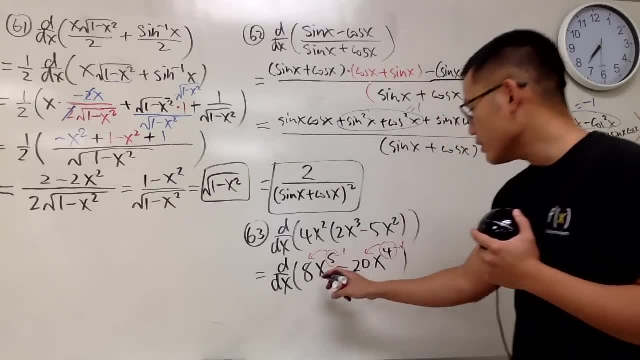 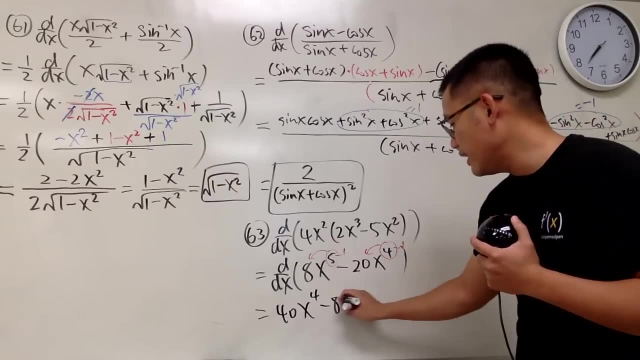 Do not do the power rule right here and right there. Let me show you. You see, this is the right way to do it. And you get 40x to the fourth power. This is negative. 80x to the third power. 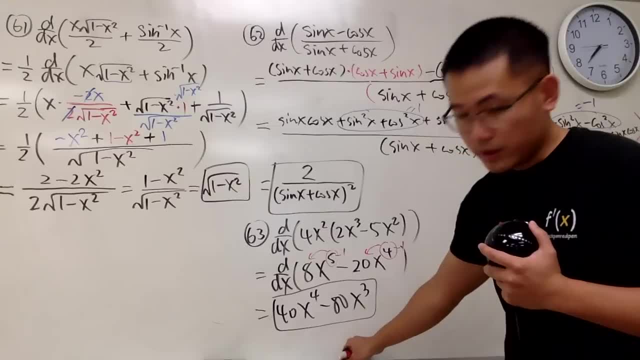 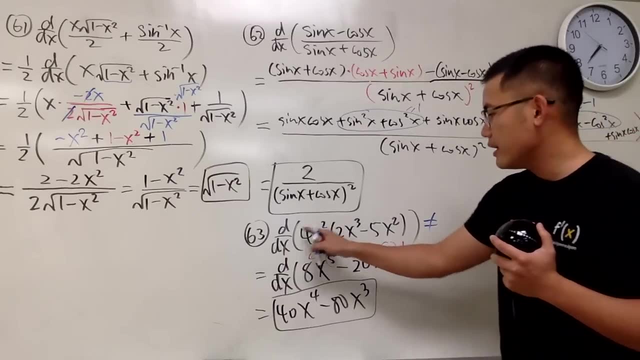 With that you are done. Okay, With this right here, you are done. Do not alright this right here. do not just say, hey, this right here should give you 8x, because that's at the root of this. 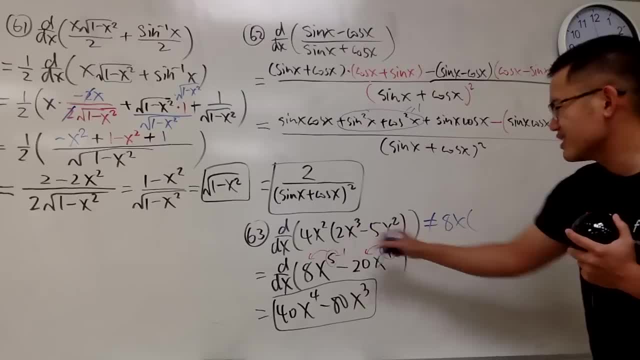 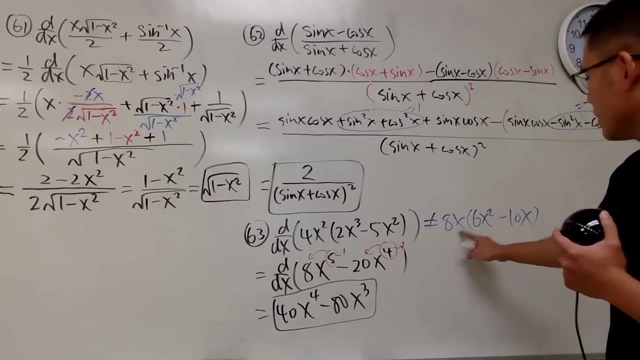 And then say: hey, this right here, the root of this is like 6x squared minus 10x. Don't do this, because you can see that when you multiply this and that, it's not that Right. This is not that. 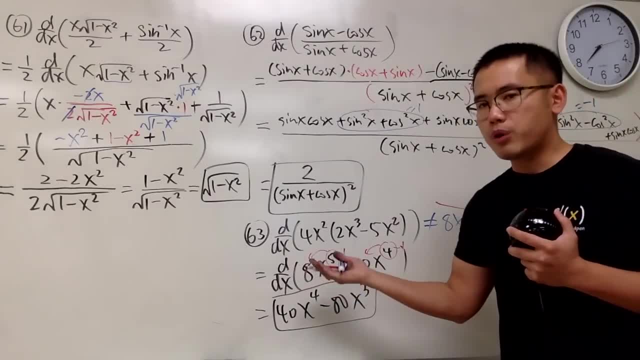 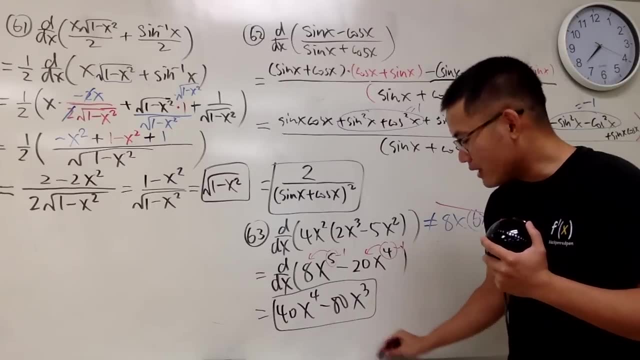 This is not correct. You can also do the product rule, but the product rule is, of course, much harder. It's not needed. It's not like super hard, It's just there's no need for it. Okay, so take a look. 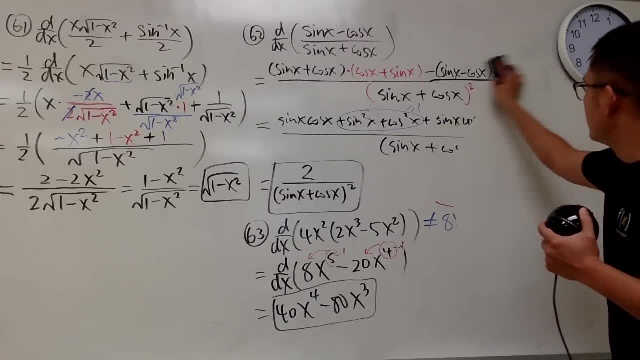 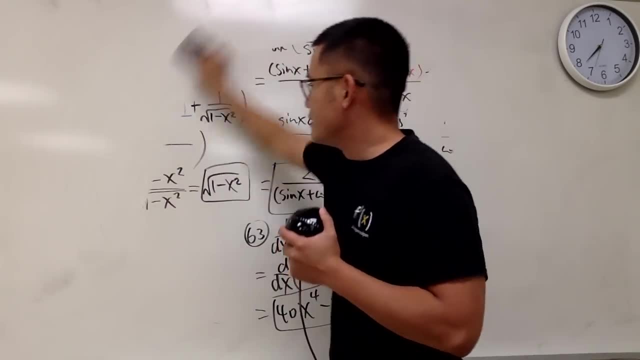 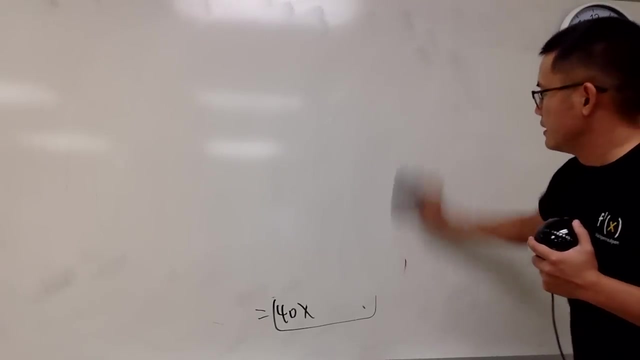 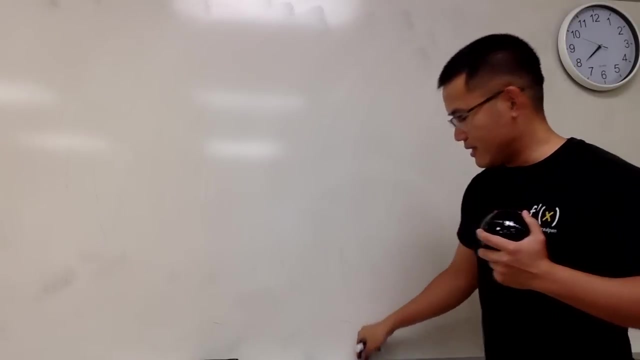 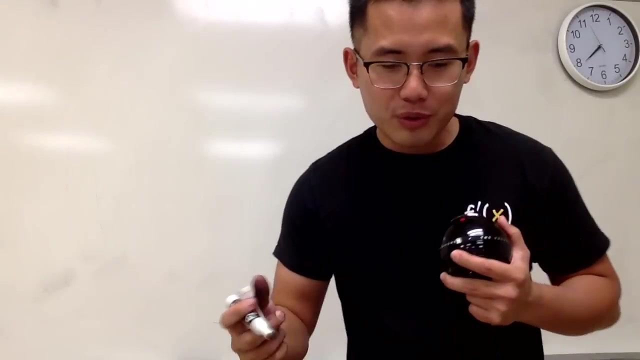 Okay, so take a look. And, as people often say, differentiation is like a mechanical work, right, So it's not hard. You can always just differentiate whatever you want, But the good differentiation are the ones you have to actually come up with. nicely. 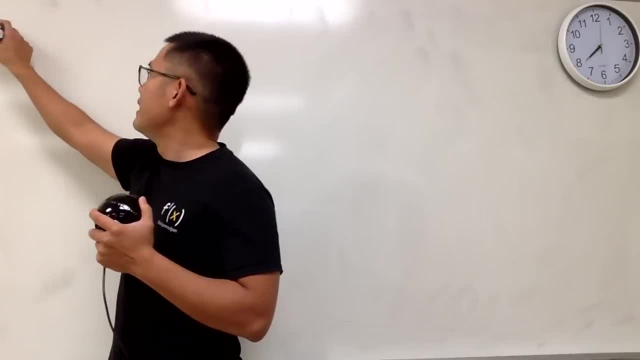 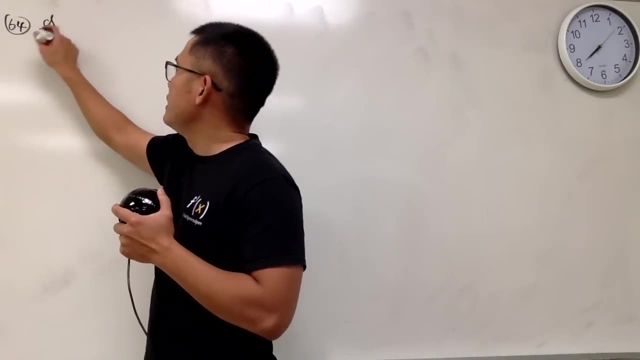 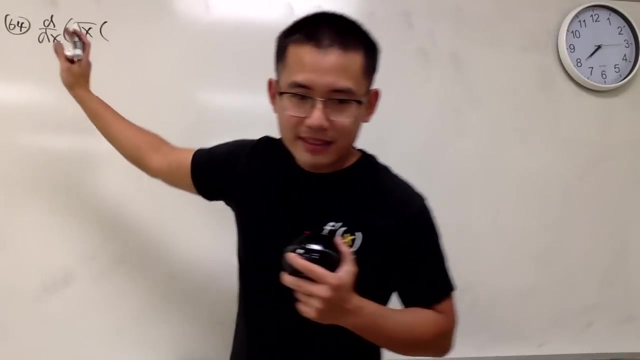 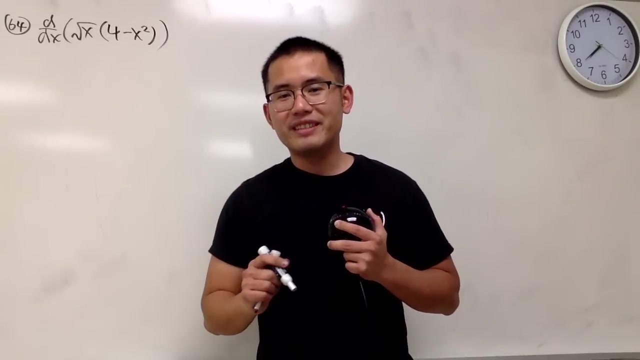 like the ones that are actually simplified and have like some really compact answer, some really nice answer and all that. Anyway, 64d dx. We have square root of, or square root of x times 4 minus x squared. We will do what we just did. 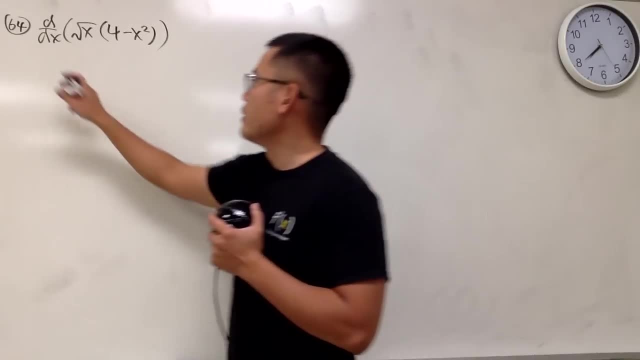 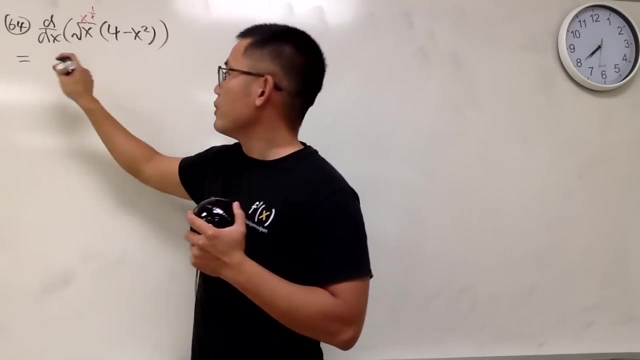 Multiply, multiply and then just use the power rule. Okay, So again, you can look at this right here as x to the 1 half power. So let me just write it down: x to the 1 half power. So we are just multiplying. 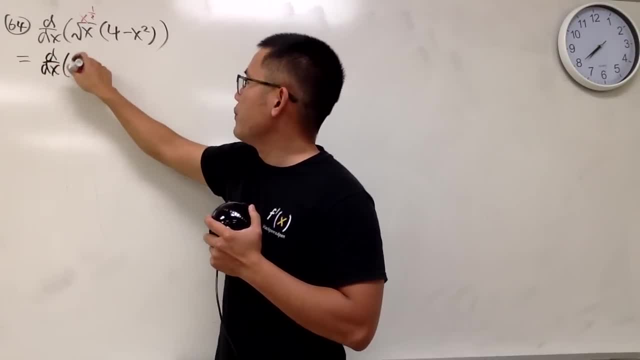 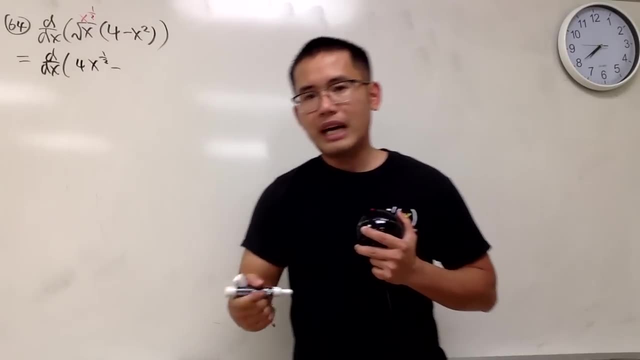 So we still have to keep the d dx, x to the 1 half times. that is just 4x to the 1 half And minus this times that 2 plus 1 half is 5 over 2.. So we have x to the 5 over 2, like this: 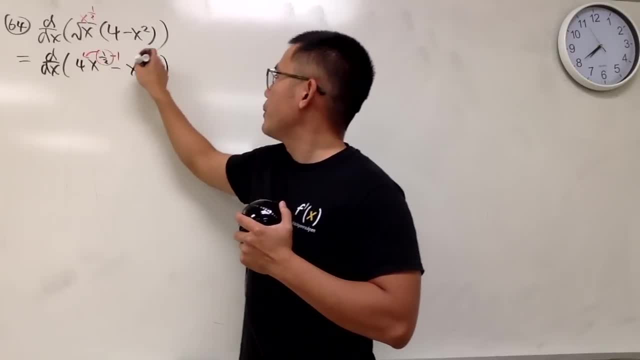 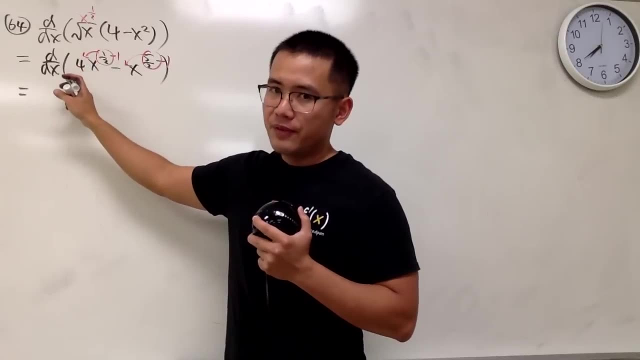 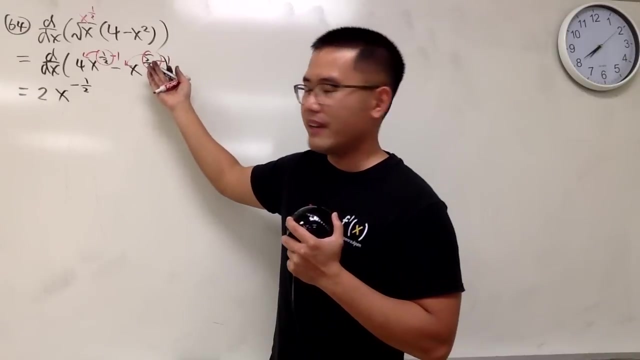 Now power rule, Power rule, The good old power rule. right, Okay, 1 half times 4 is 2.. And then this is x to the negative 1 half. Here. bring the 5 over 2 in the front. 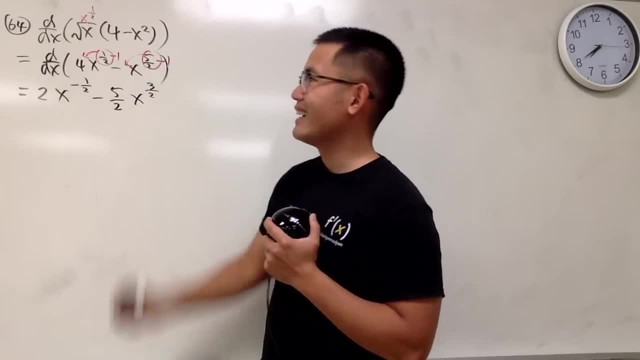 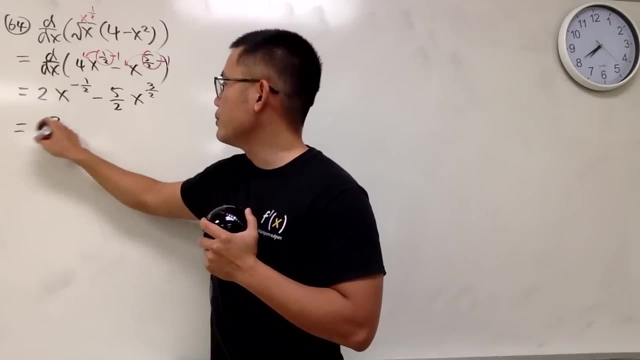 And minus 1, we get x to the positive 3 half like this. Okay, this should go down to the denominator, so we will put it down in the denominator. This is 2 over x to the 1 half power. 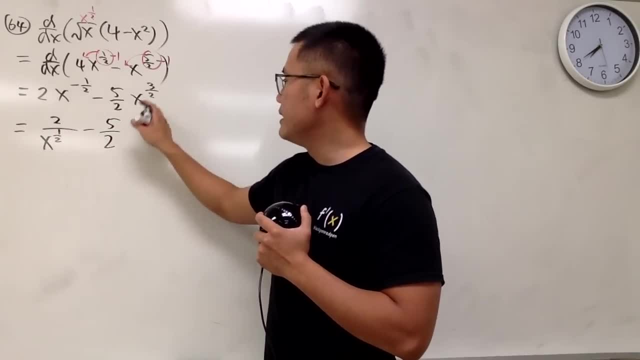 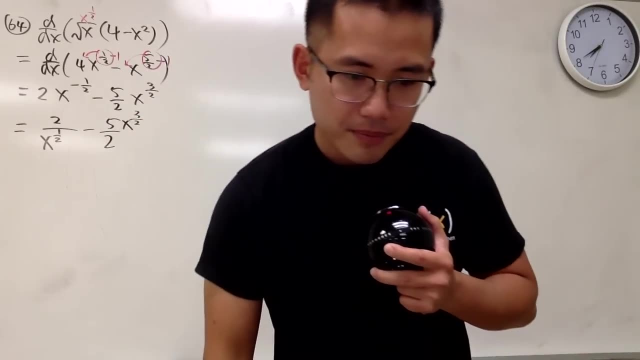 And this is minus 5 over 2.. And this right here is on the top. So x to the 3 half power. Can we get some common denominator right here? And yeah, I combined the fractions again, So let's see. 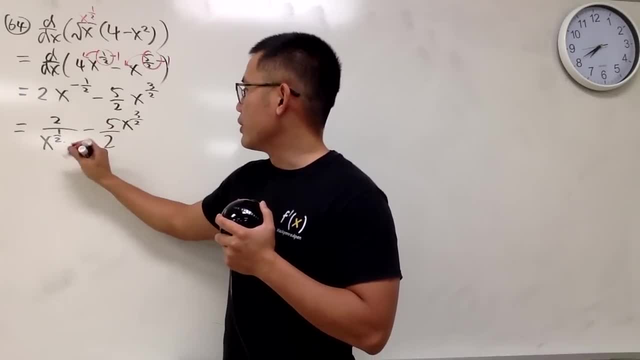 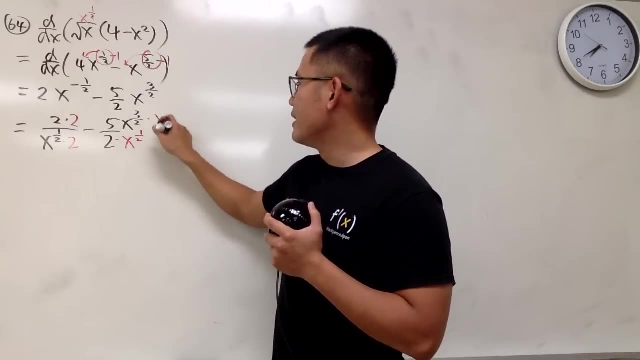 This right here needs this 2.. So multiply the 2 right here and right here. This right here needs the x to the 1 half power. So we multiply this right here: x to the 1 half power, x to the 2.. 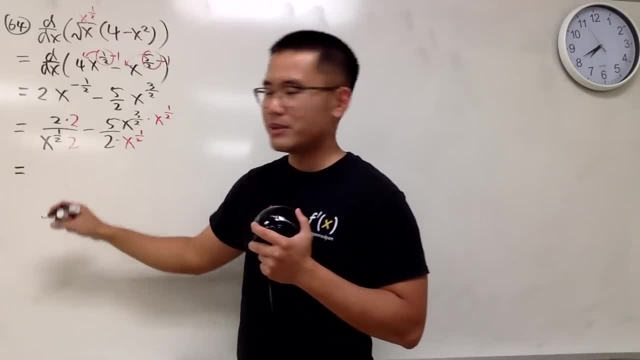 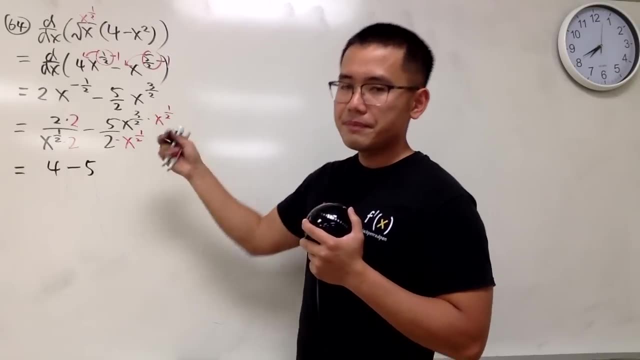 x to the 1 half power, Okay, 2 times 2.. 4 minus 5.. x to the 3 over 2 times x to the 1 half. Multiply you get x to the 4 over 2,. 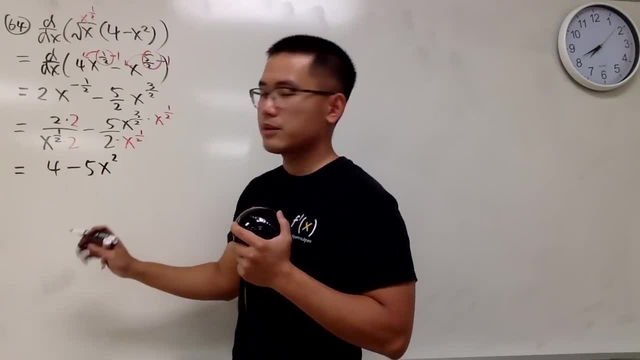 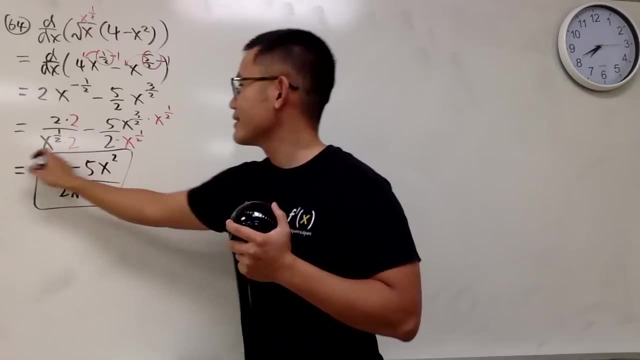 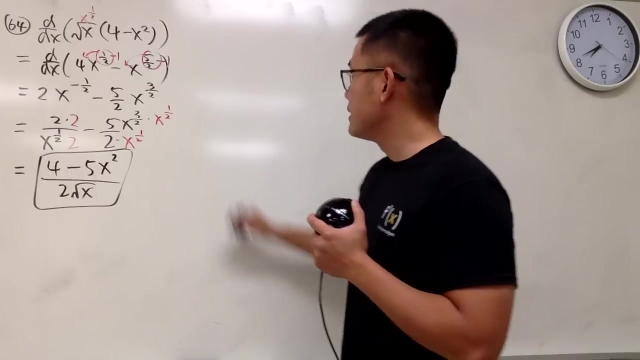 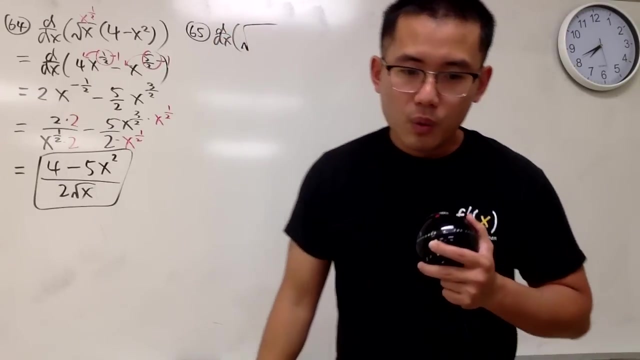 which is just 2, right For the power. x squared Over 2 and x to the 1 half, power is just square root of x, Just like that. That's it Okay. So now we have 165 differentiating square root of 1 plus x over 1 minus x. 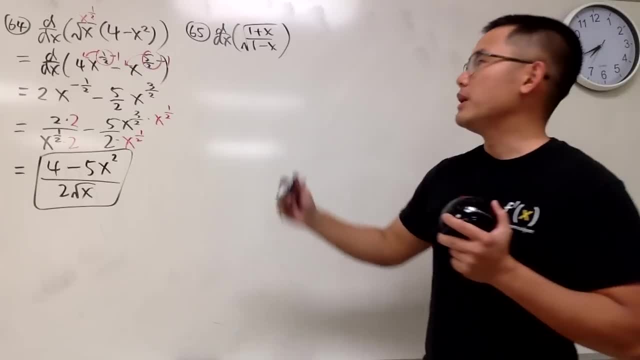 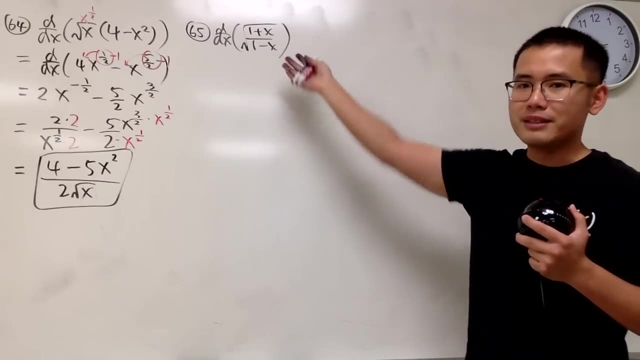 Like this: Okay, Here is the deal. Some people may tell you: hey, you can just call that to be y And then take the natural log on both sides And you can use the natural log property to reduce the right-hand side. 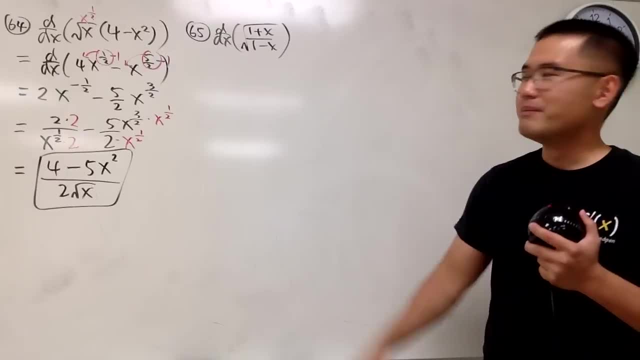 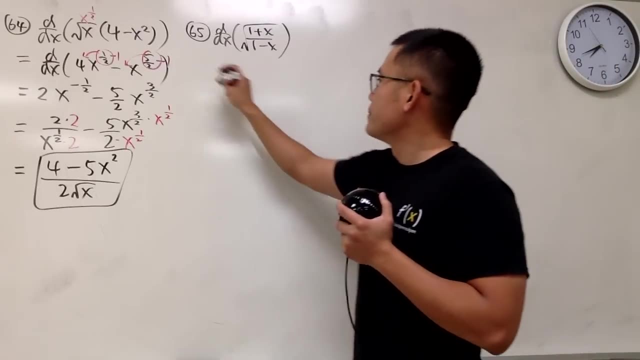 You can do that, That's not that bad. But this is also not that bad. Not that bad if you just do it. So just do it Like thank you, Okay. So here we go To do this. 1 over 2 square root of the inside. 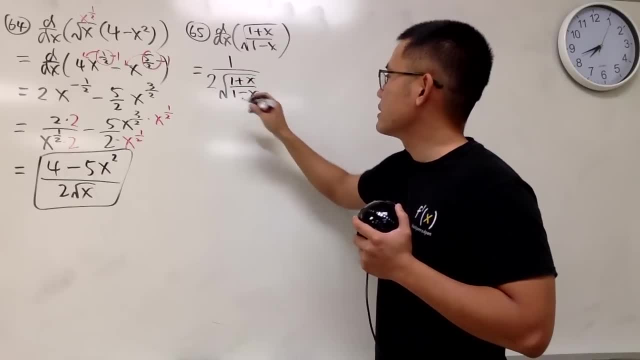 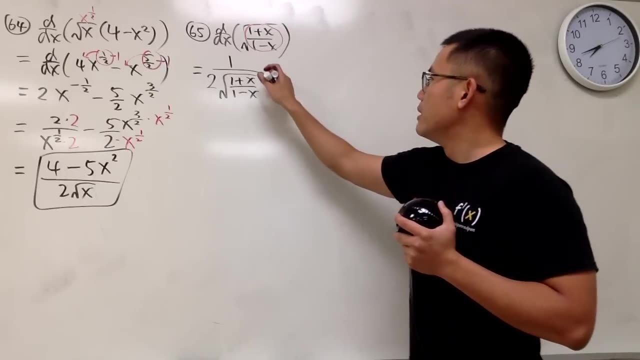 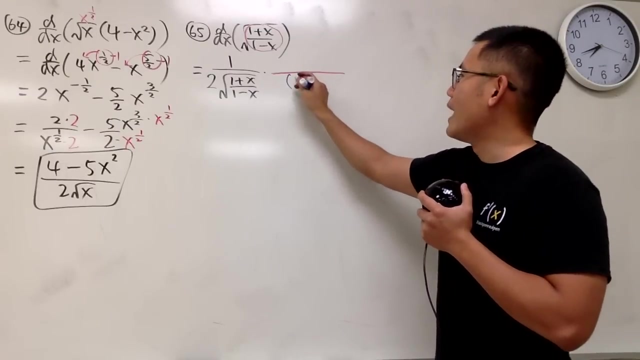 You literally just write it down: 1 plus x over 1 minus x And we have to multiply by the derivative inside, which requires the quotient rule. Multiply by- let's square the bottom, So parentheses: with 1 minus x. With 1 minus x inside. 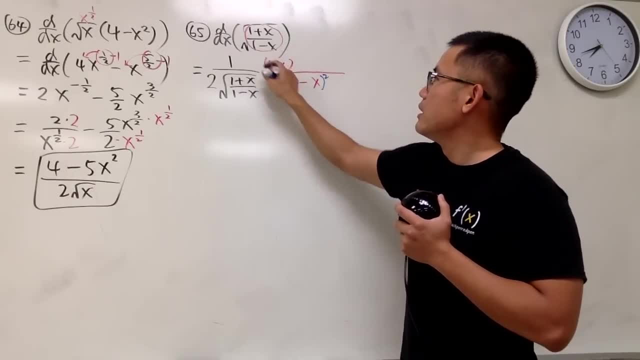 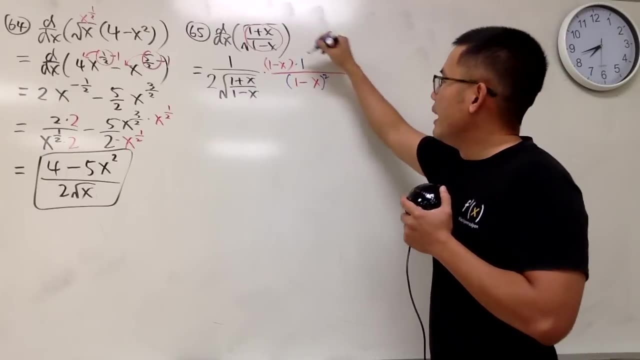 Square. that Bottom function here times the derivative of the top. The derivative of this right here is just 1.. The inside function, wise Okay, And then minus the top function, which is 1 plus x times the derivative of the bottom. 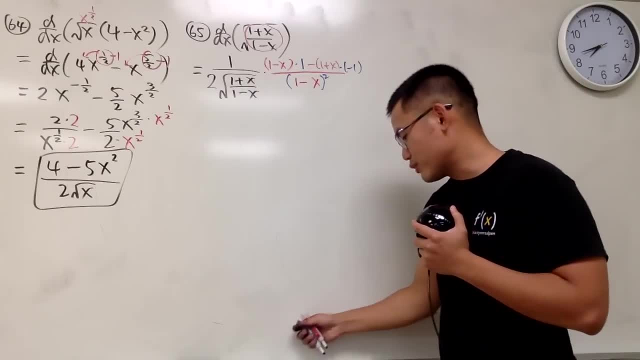 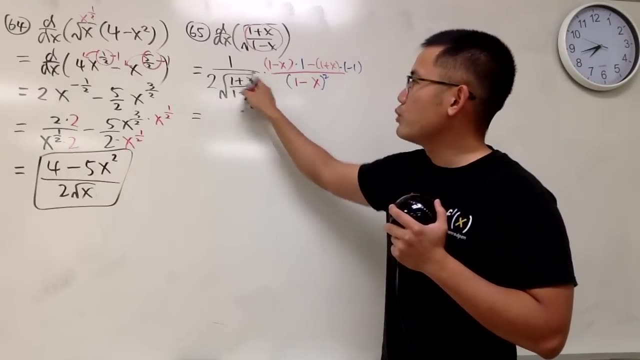 which is negative 1.. Like that Told you, it's not so bad. Now check this out. This is what I will do. This right here. It's the same as saying square root of 1 plus x over square root of 1 minus x. 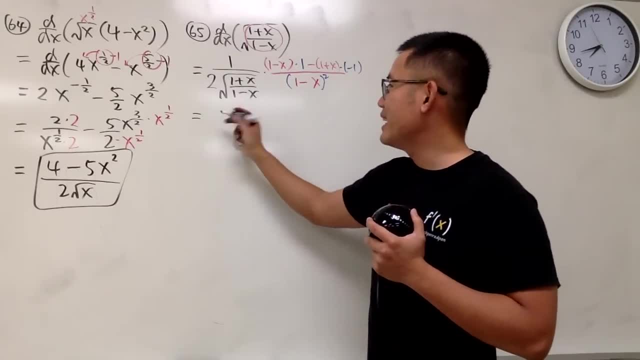 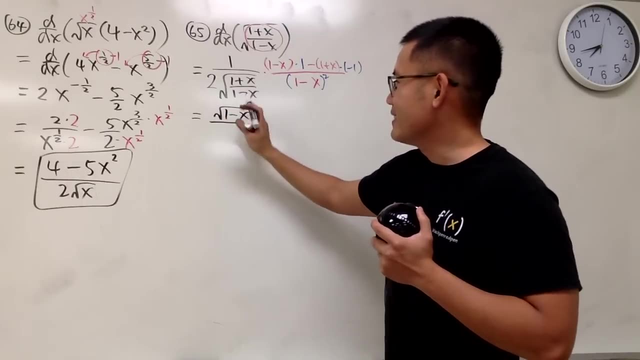 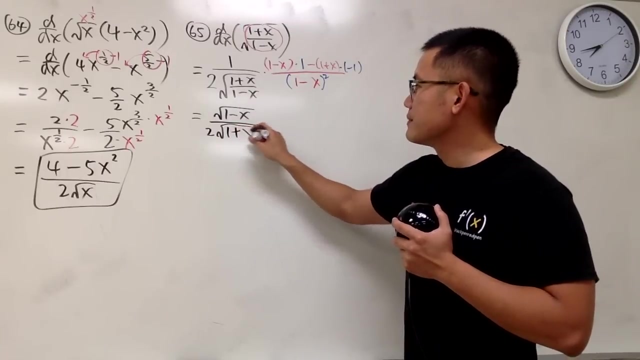 I can bring this up up So we get square root of 1 minus x. Bring this up up Like this, And then, divided by 2, square root of 1 plus x. Okay, And right here let's see how we can simplify this. 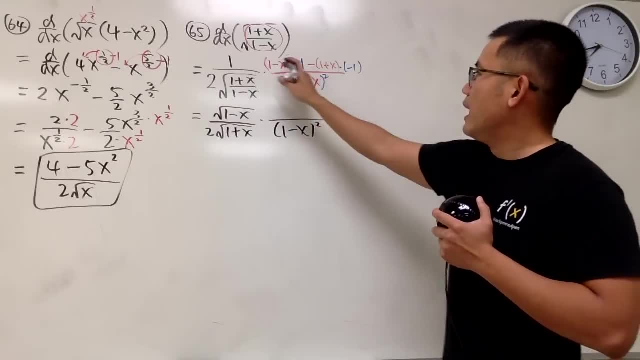 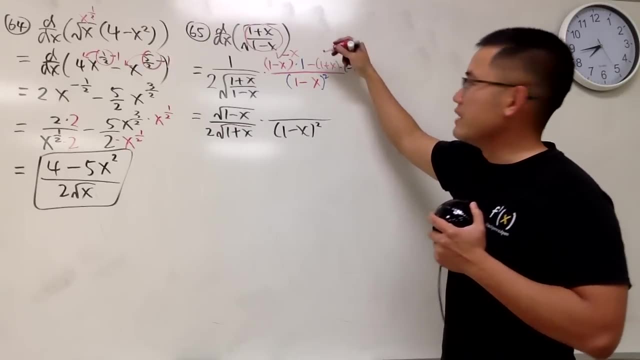 Here we have parentheses: 1 minus x, Square On the top. here, though, This is just 1 minus x, And negative times negative makes it positive, So we have to just add 1. Add x, Negative x, Positive x. 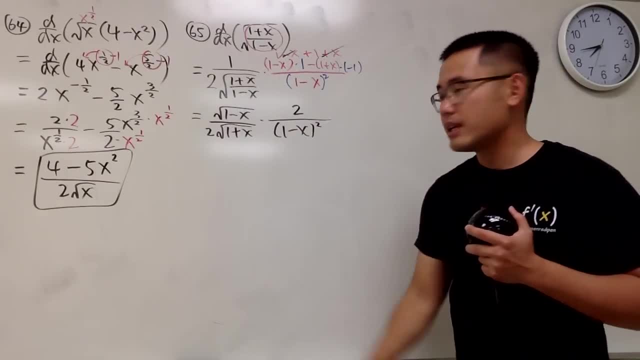 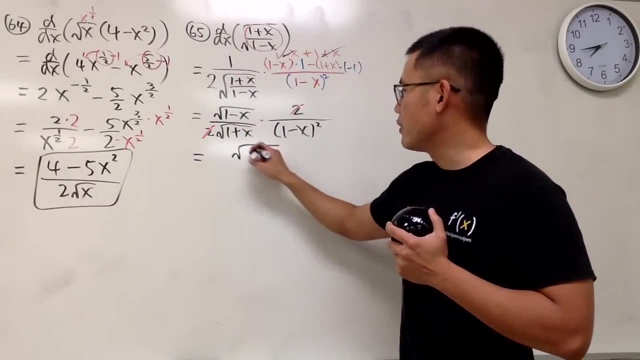 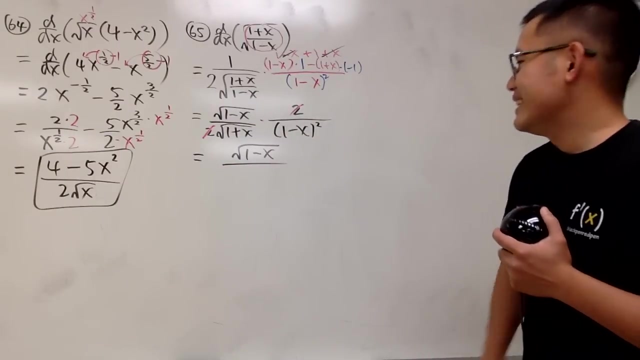 Cancel. 1 plus 1 is 2.. Cancel- Cancel. Finally, we can put this together. On the top we have square root of 1 minus x Over. We can put this down first. You can reduce more, but 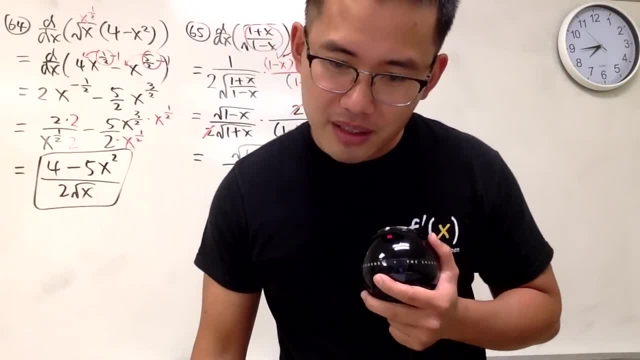 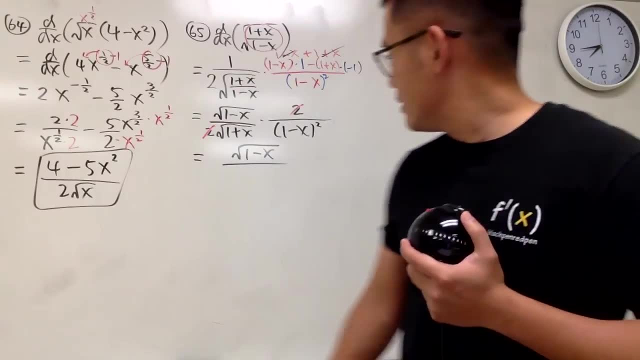 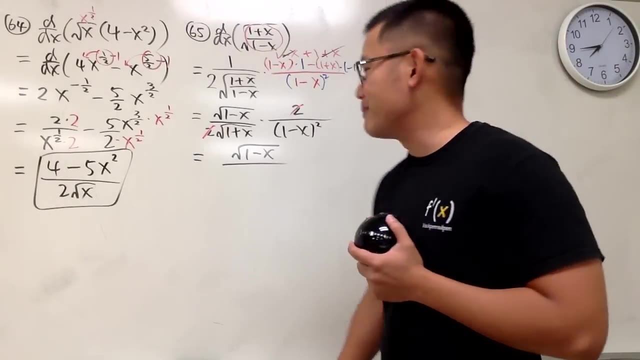 Ah, man, Did I do that? I didn't do it for the answer key. Did I do that? Yeah, I didn't do that, But I could have done that. But like I don't know This and that we can have reduced it more, 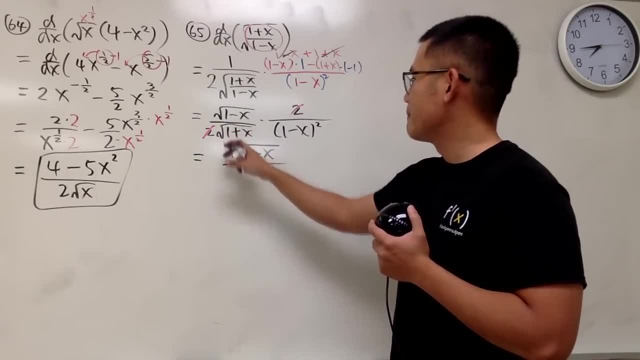 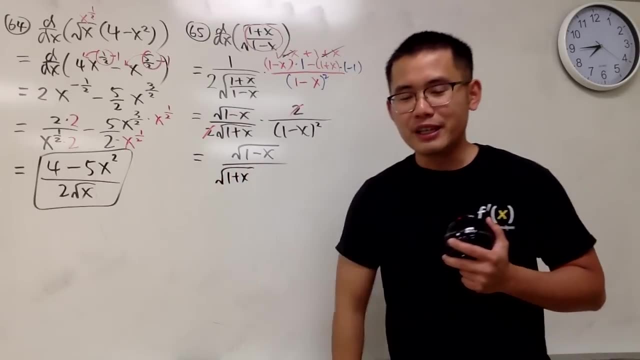 But up to you, Anyway, that's. That's Okay. So 1 over that. So I will have this, And then 1 plus x. I will reduce it and I will change it on my answer key because I feel that's better. 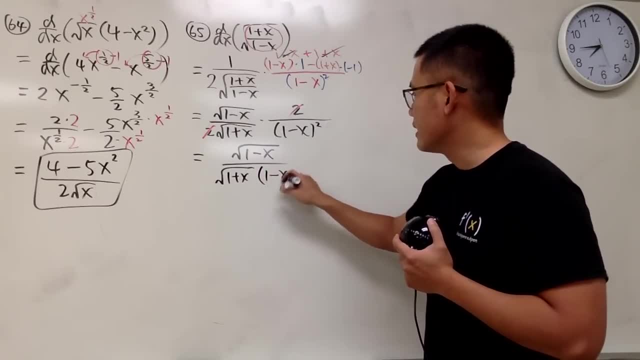 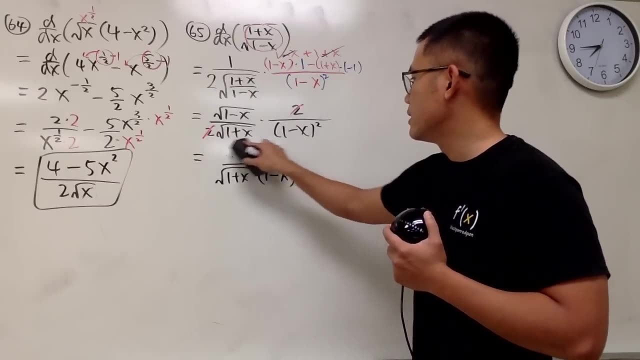 here. Anyway, This is like 1 minus x to the second power, right? But, as I said, we'll reduce this a little bit because they have the same base. Okay, So this right here is the 1 half power. 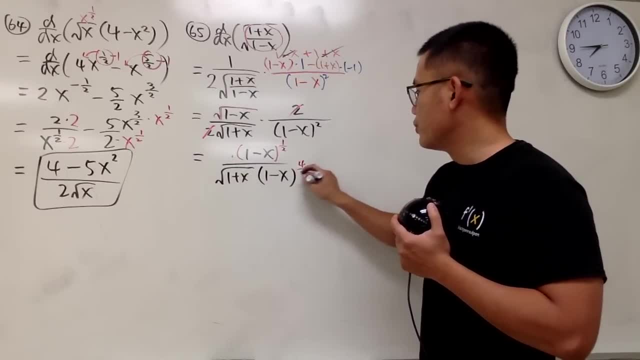 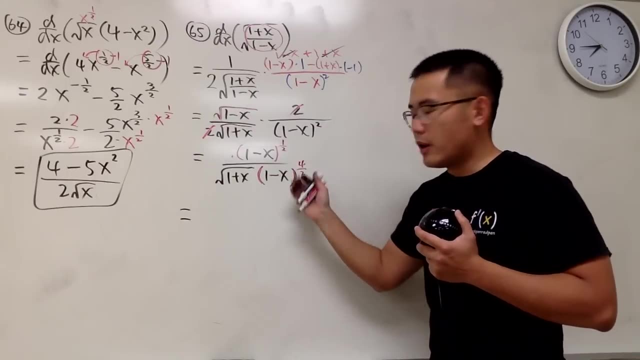 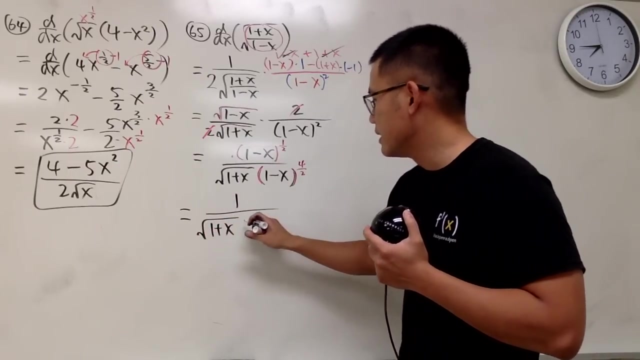 And this is like 4 over 2 power. Okay, So when you reduce, of course, you end up with 3 half power right here on the bottom. So all in all, you have 1 over This. right here is square root of 1 plus x times square root. 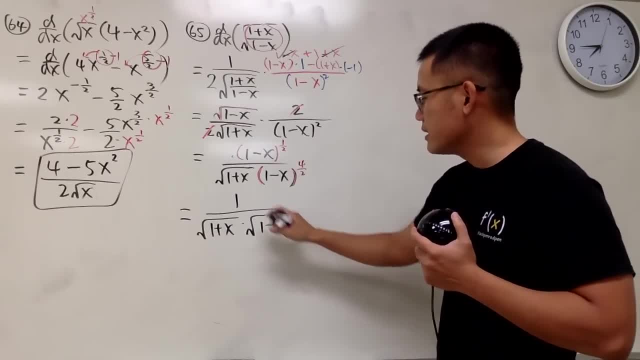 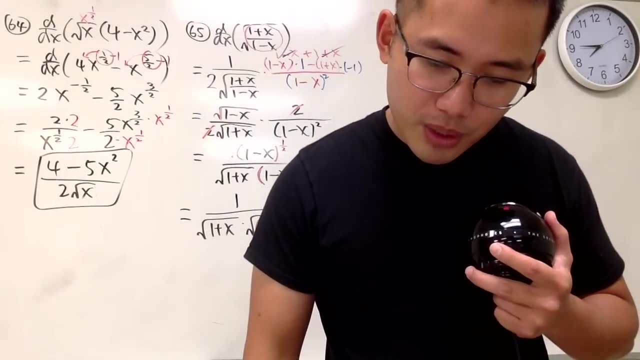 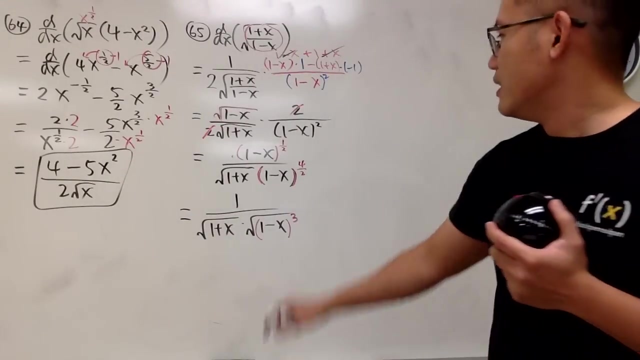 You get 3 half power, So you have 1 minus x in the square root And you raise that to the third power right here. Okay, So I will change that right here. I'll change that On the answer key. I just have this, but I think I should do it like that. 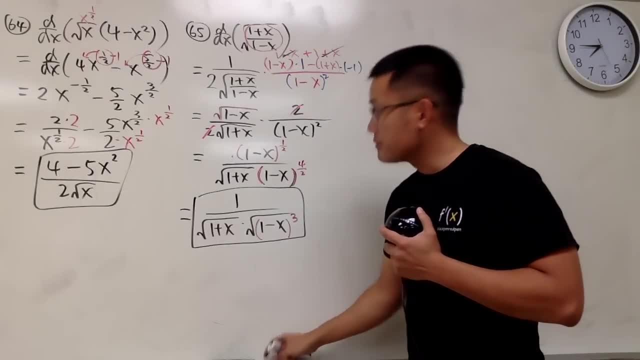 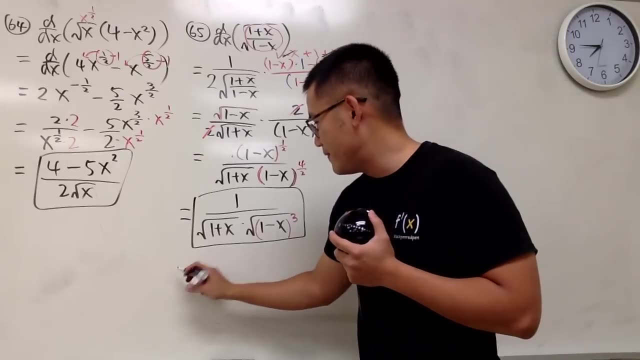 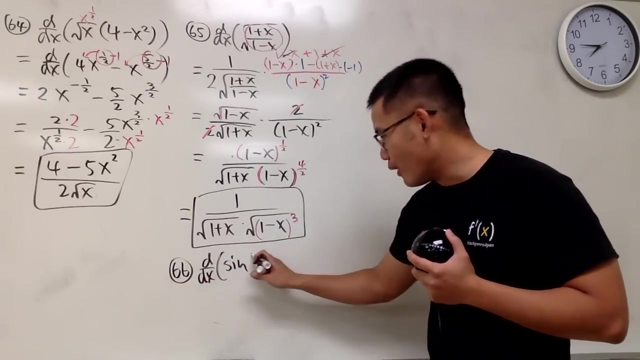 Okay, Same base, Just reduce it All right. Number 66.. This is a really fun one. I will be able to fill in this right here. Number 66.. Differentiating Sine Of Sine Hex. 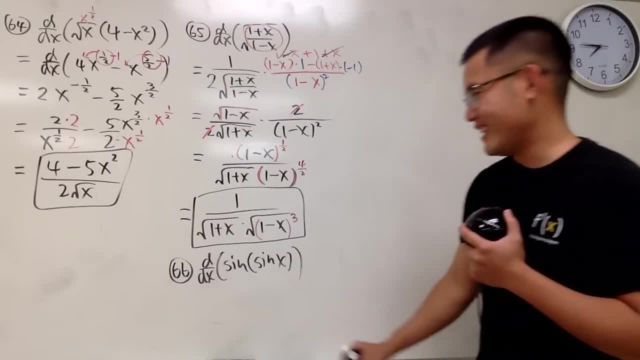 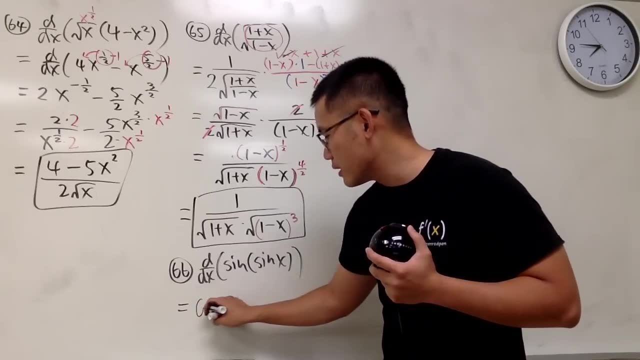 Sometimes you can do a lot of them, but you know two of them is okay. Anyway, here we go. Start from outside. Derivative sine is cosine. Okay, Derivative sine is cosine, And the input you keep it. 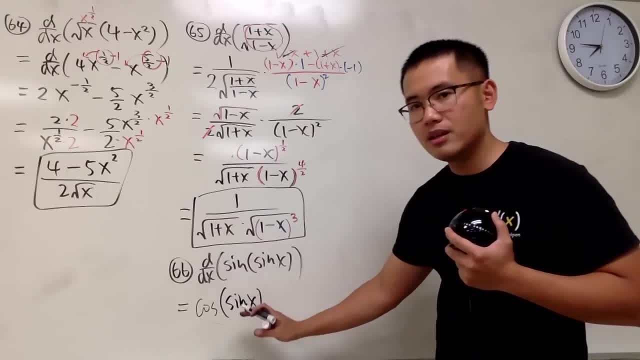 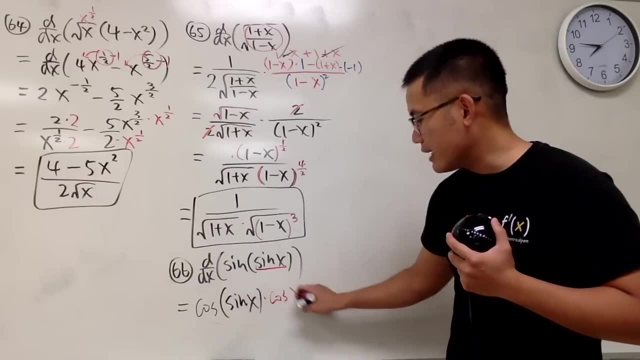 You just keep it. Okay, You keep it. But the channel says you have to multiply by the derivative inside Derivative sine x is cosine, Cosine And you have the x. And if you look at the inside right here, the derivative of x is just 1.. 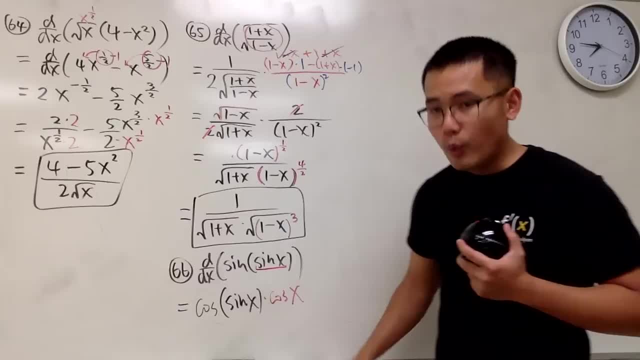 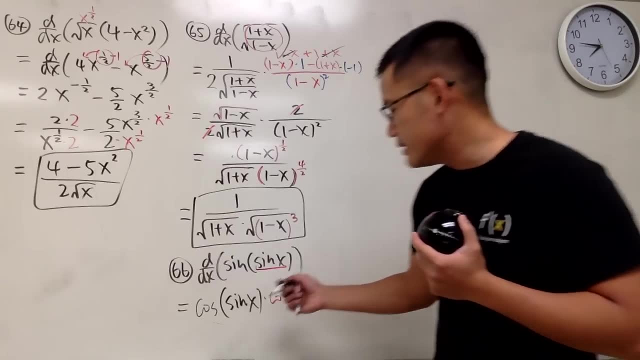 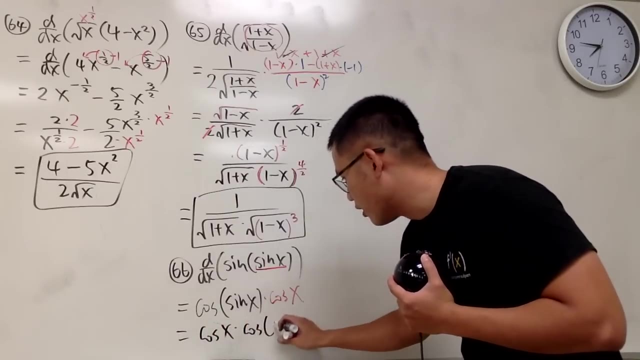 So multiply by 1 doesn't really matter. The truth is you are always using the channel, But sometimes the channel does not matter. And on the answer choice I put down this first: So cosine x times cosine of sine of x. 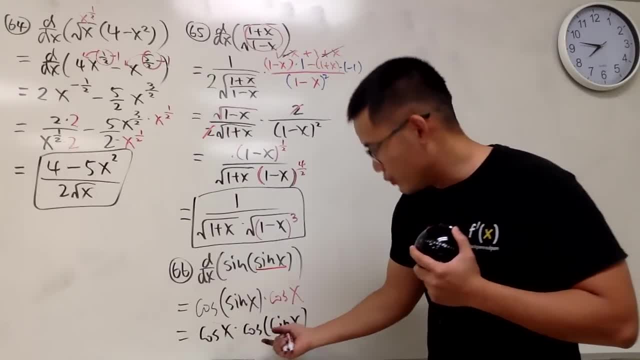 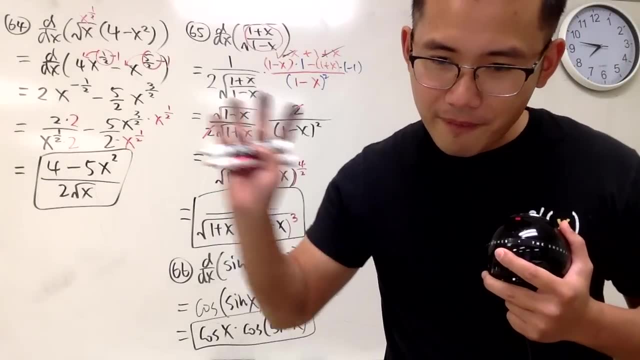 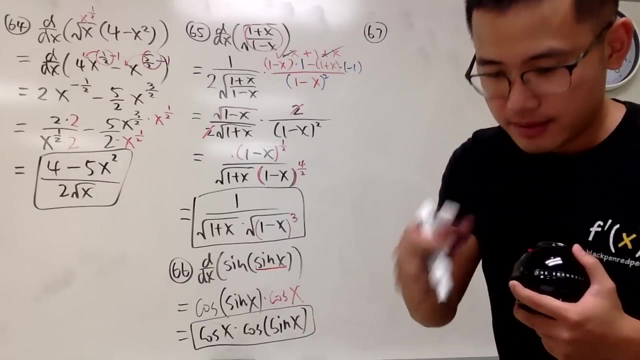 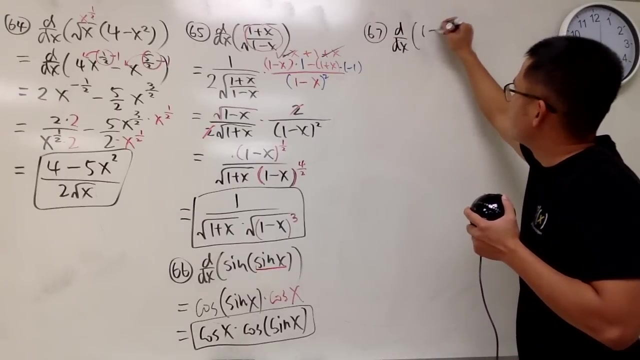 So we put sine in 2 cosine For this part, And then this is just cosine x Multiplying with stem 4 hours. Okay, Number 67.. Okay, The dx 1 plus e to the 2x. 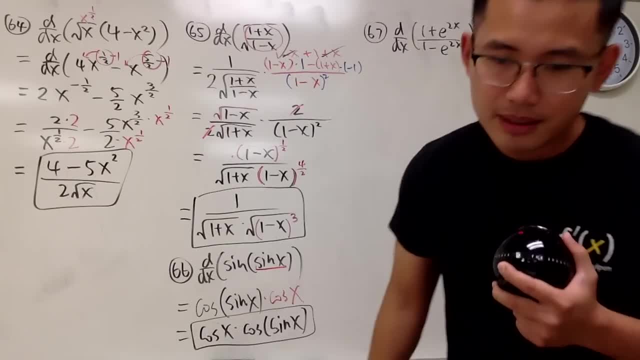 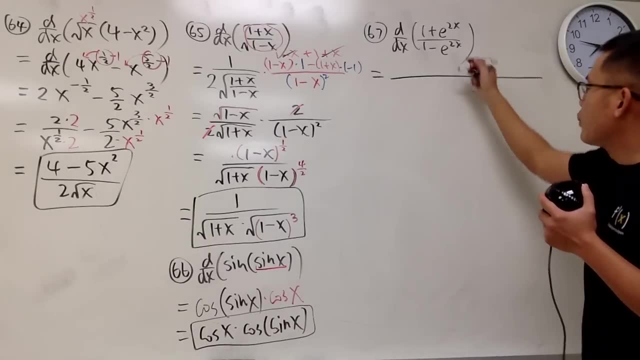 Over 1 minus e to the 2x. Yeah, Okay, Of course, Quotient rule in action. So here we go: Square the denominator before we forget. So 1 minus e to the 2x, Like this: 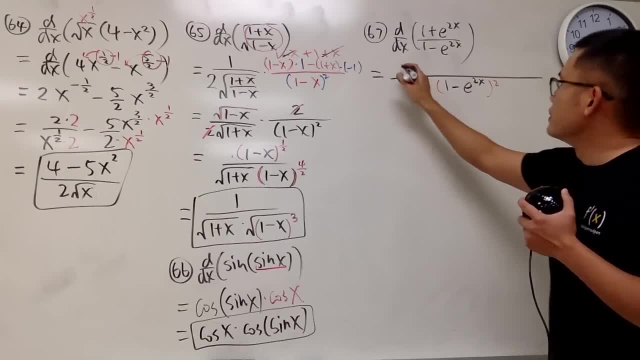 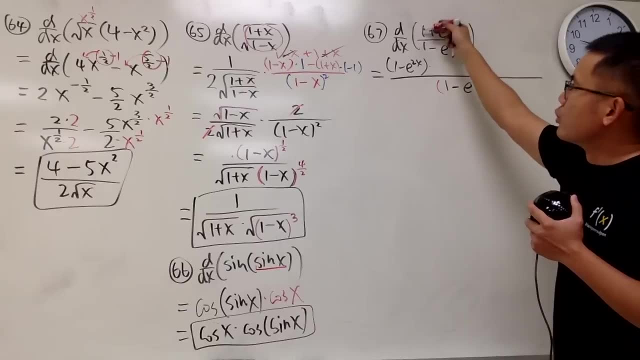 And square that And then we put down the bottom function right here, Which is 1 minus e to the 2x Right. This is the bottom function Times. the derivative of the top Derivative 1 is 0.. Derivative e to the 2x. 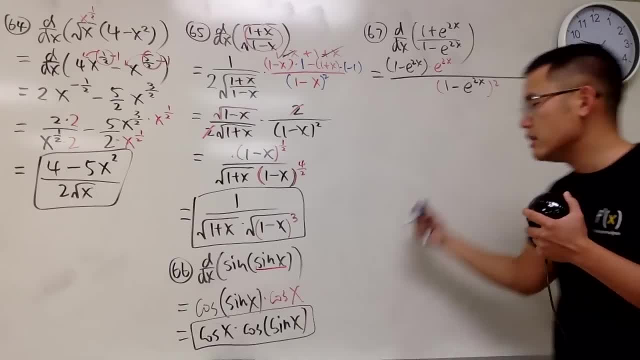 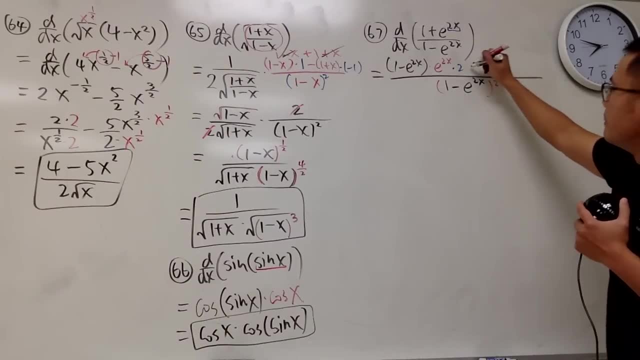 You write down e to the 2x first, But you multiply by the derivative of 2x. Chengdu says so: Multiply by 2.. Then we just minus the top function, Which is 1 plus e to the 2x. 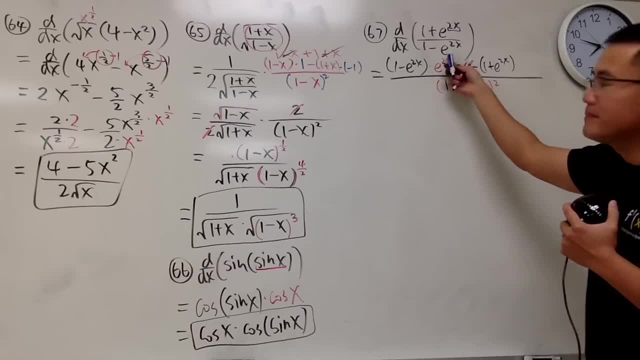 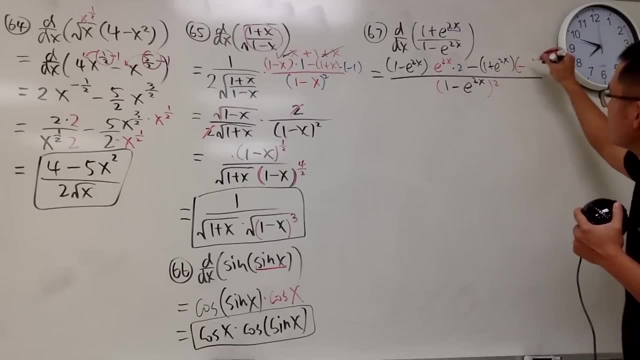 And then multiply by the derivative of the bottom. Derivative of 1 is 0. But derivative negative. So this is still negative And you have e to the 2x. Stays like this And then you multiply by derivative 2x. 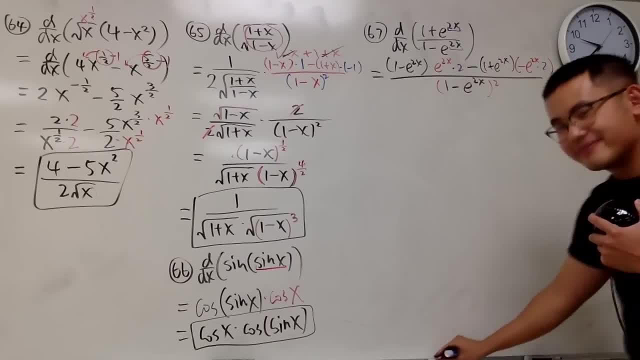 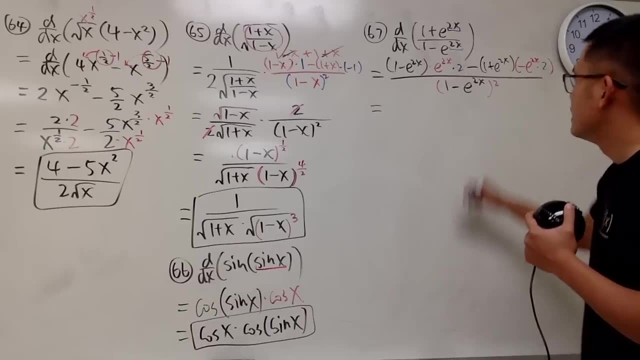 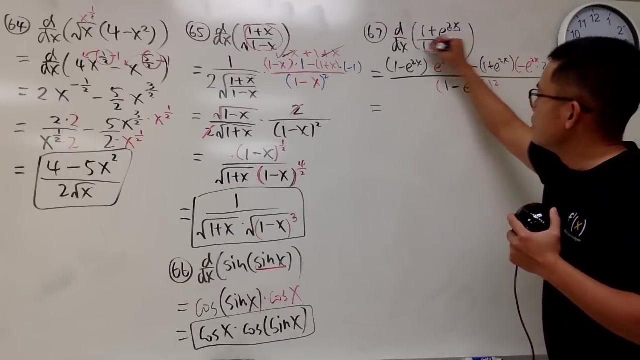 Which is the 2. Like that. Okay, Now let's see if we can simplify this nicely or not. Take 2e to the 2x, Multiply in. Okay, So multiply this into the parentheses, This times that We get 2e to the 2x. 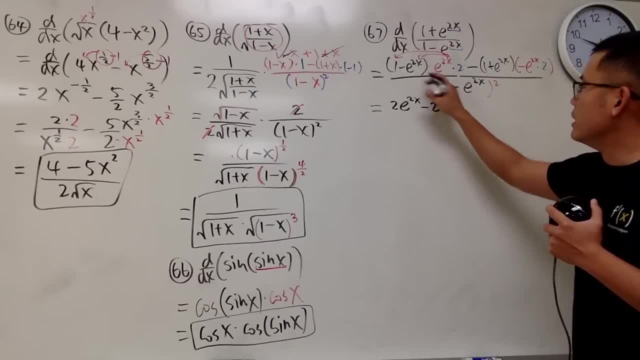 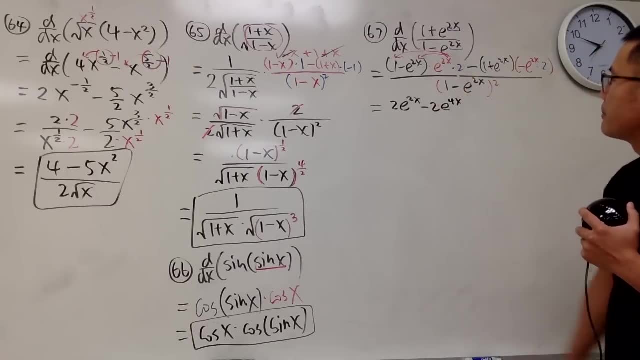 And then this times that is negative, 2e, And you add the exponents, So you have 4x for the exponent. So that's that part. Then negative times: negative is positive, So be careful with it. So we do this. 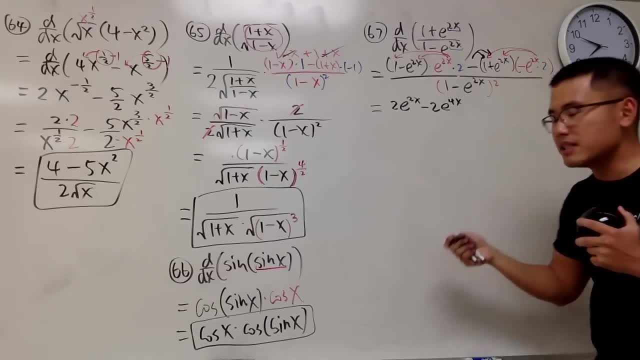 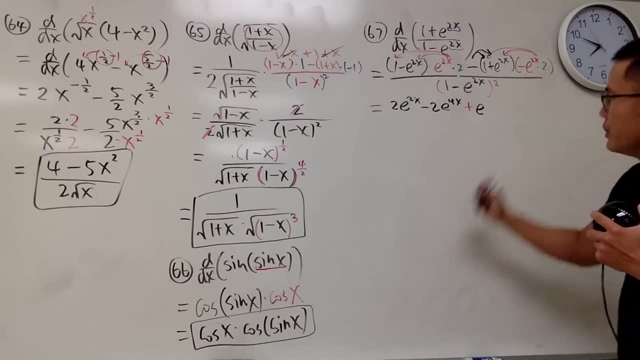 And also in the meantime we do this. So negative together becomes positive. So this is 2e to the 2x times positive 1.. So this is plus Okay, Plus 2e to the 2x, 2e to the 2x. 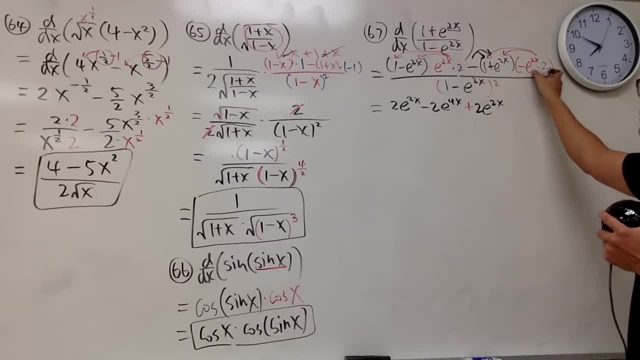 And then Positive times. that is also positive. So you have 2. Plus. This is again plus 2.. e to the 2x times. e to the 2x is e to the 4x. Just a whole video for there. 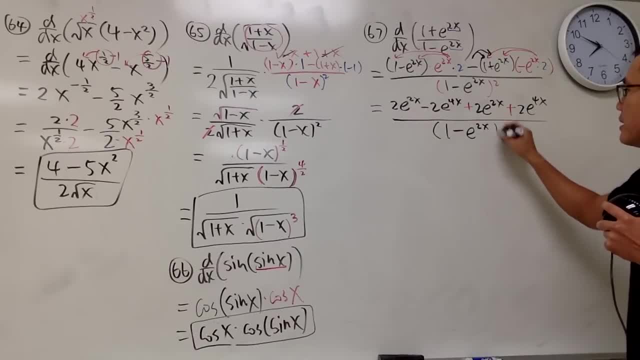 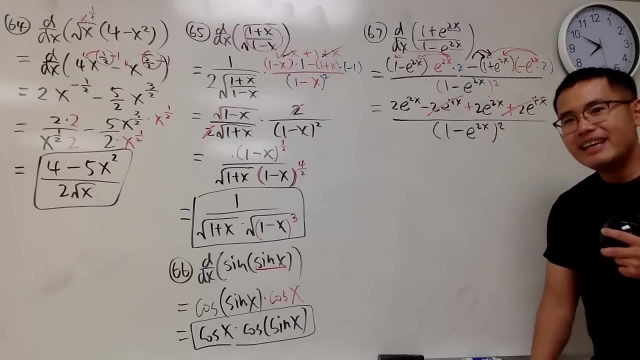 And you have some nice cancellation that's about to happen Right here and here. Cancel them out And we can also combine things right. This and that can be combined in. So, all in all, 4e to the 2x. 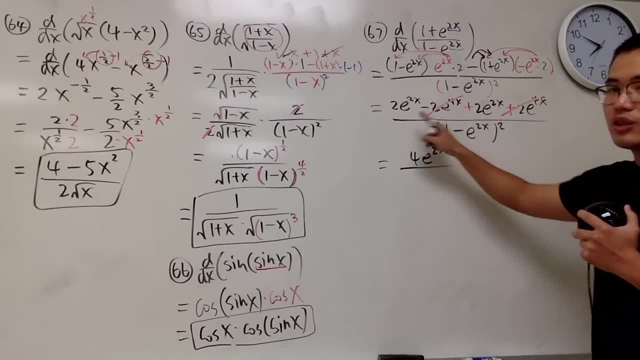 And you're adding. So you keep the e to the 2x term. You just do the coefficient The 2 times 2.. That the 2 plus 2 is 4.. And then the bottom is Parentheses: 1 minus e to the 2x. 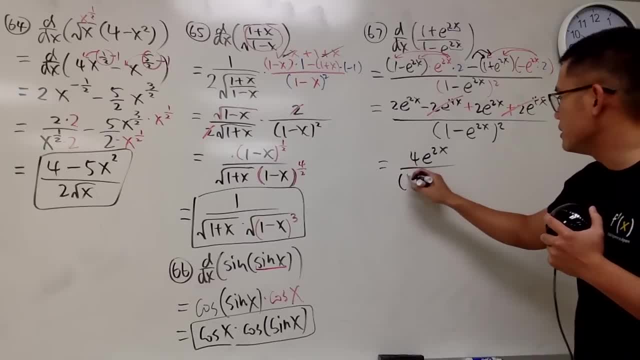 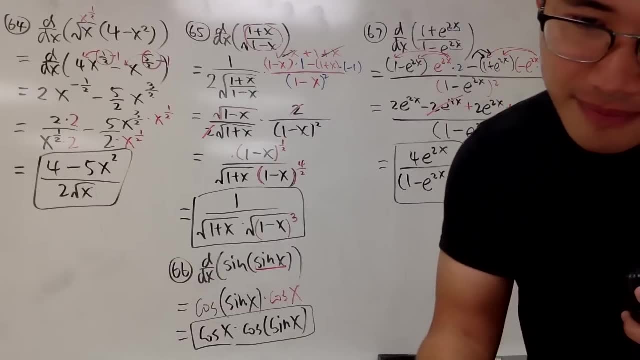 Square And We are done For that one. Okay, I'm going to fit in 68. Right here. And We are done For that one, And We are done For that one, And We are done. 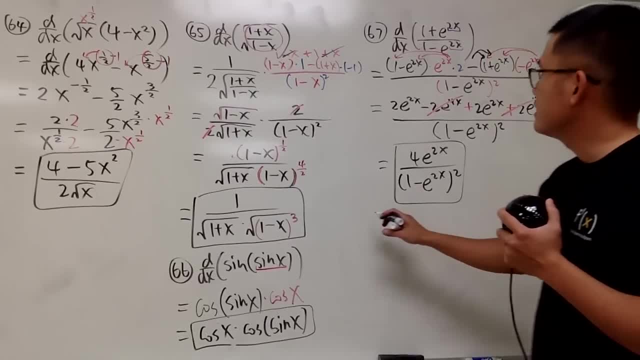 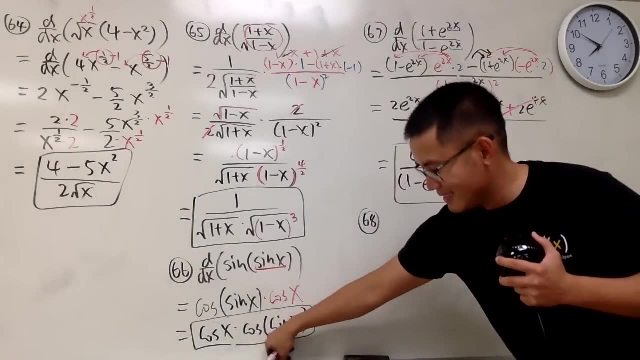 For that one, And We are done, And We are done, We are done. So you're going to fit in 68 right here. Believe it or not, I, I, I believe myself, I, I hope d two them two dash. 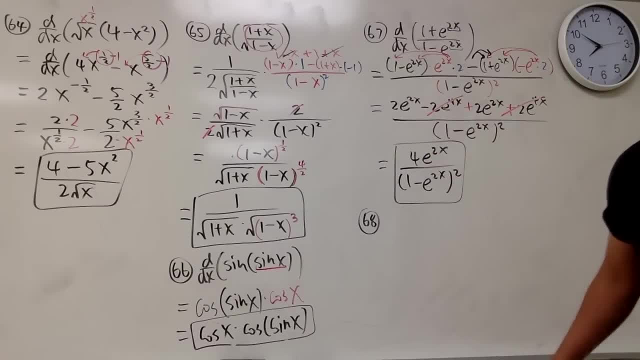 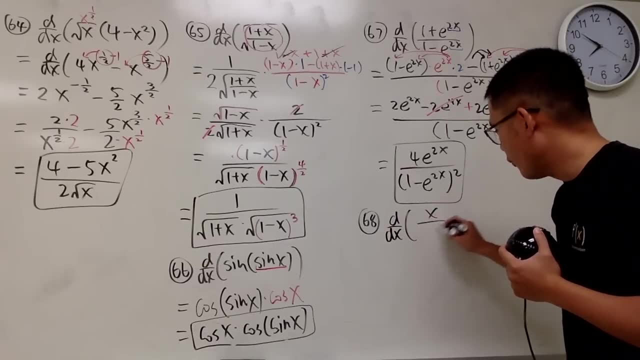 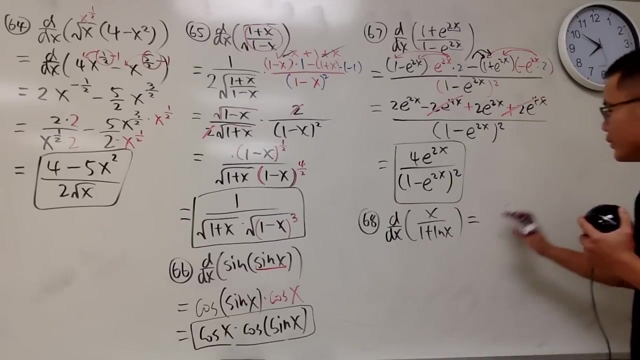 P ignite x Over 1 plus natural log of x. Another quotient rule Example. Okay, I will do it right here. Otherwise space, so square the denominator. so we have 1 plus natural log of x and we square that and we put the bottom function up, which is 1 plus natural log of x. 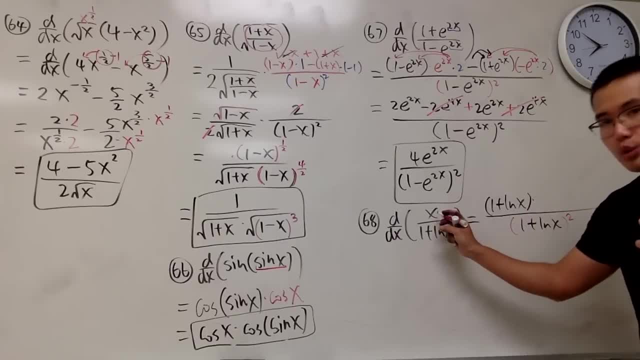 multiplied by the derivative of the top, which is just 1, minus the top function, which is x times the derivative of the bottom, which is just 0, and then plus 1 of x, so it's just 1 of x. like this, this right here is, of course, just minus 1. so you'll see, this right here is just 1 plus natural. 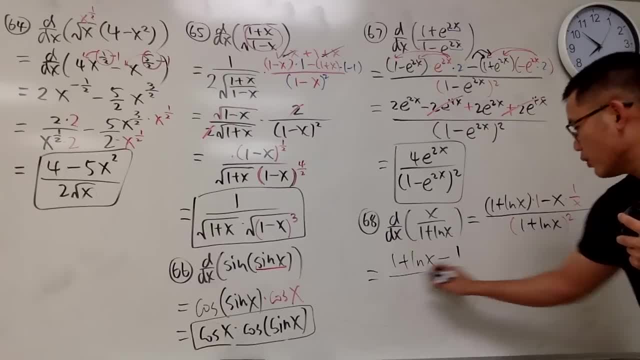 log of x. and then this is again, as i said, minus 1 over this guy. ah, so this is a very nice question, because in the end, 1 minus 1 is 0. we end up with ln x over 1 plus ln x, square like that and with 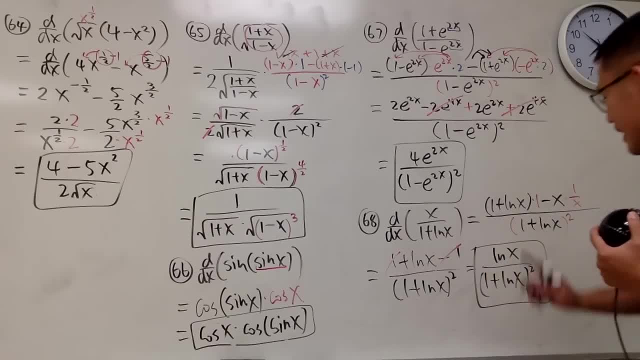 that we are done. i have a question just now: how can i integrate this and get back to that? that's a pretty nice question. maybe do some u substitution. this is a hard one. i will go back to this and then do the derivative right here. okay, so this is, uh, number 69. i mean 68. 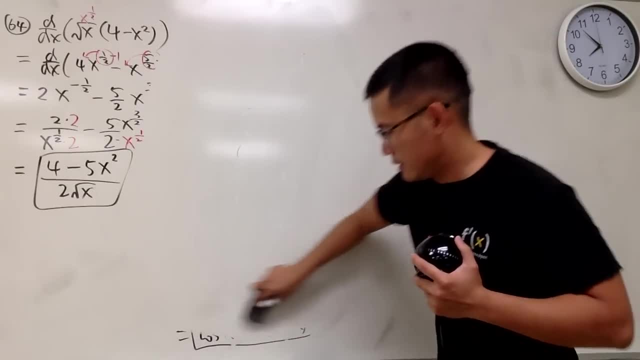 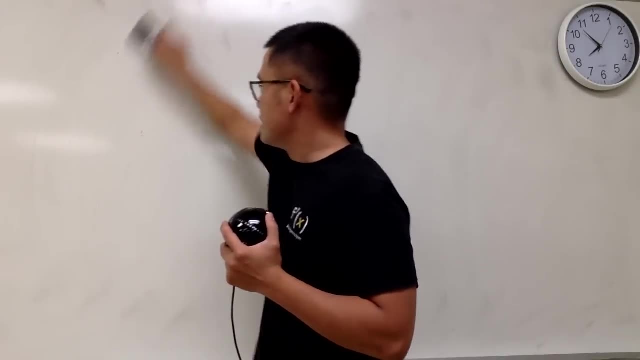 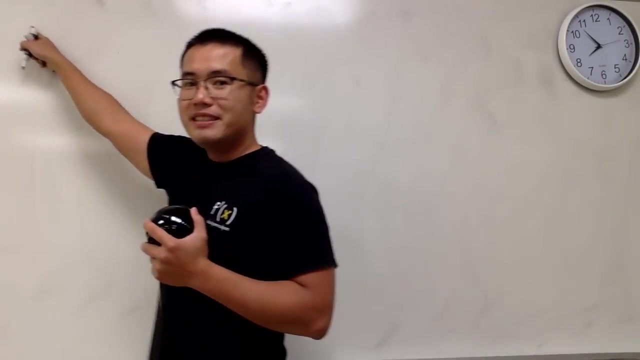 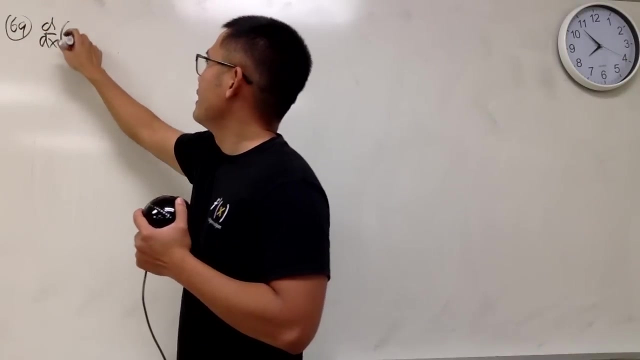 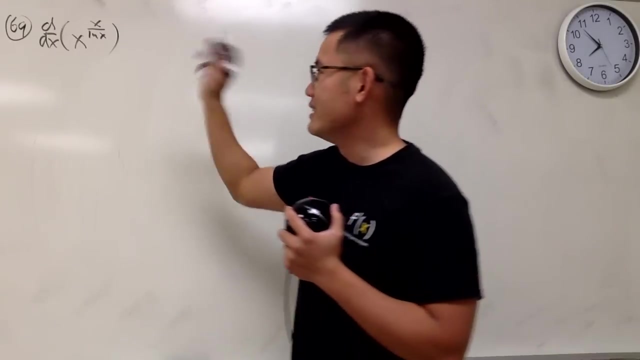 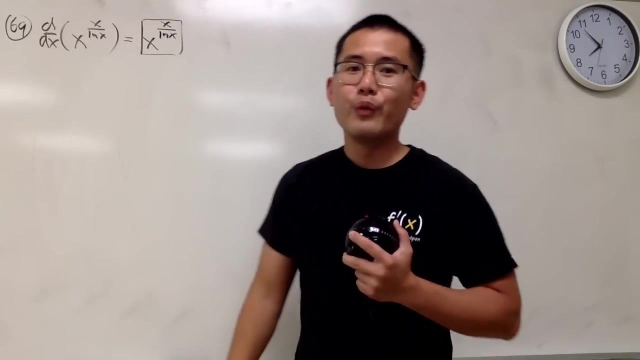 all right, here we go. the next question. all right, this is a extreme fun one, right? not because of the number, but rather the actual question. okay, x raised to the x over natural log of x power, like this. let me tell you: the answer to this right here is x to the x over natural log of x power, and we are 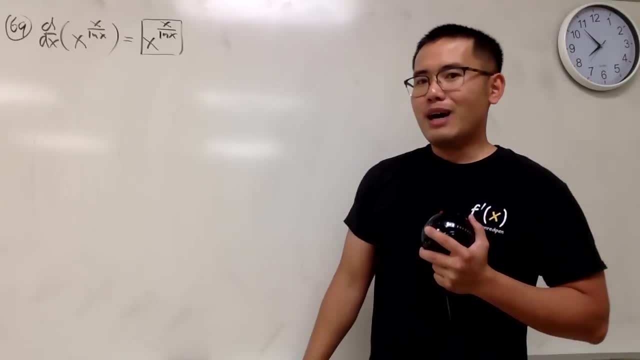 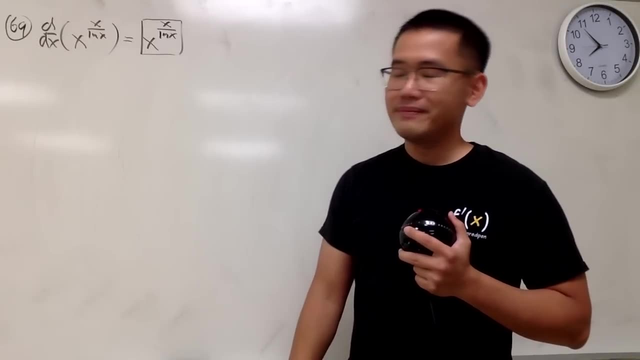 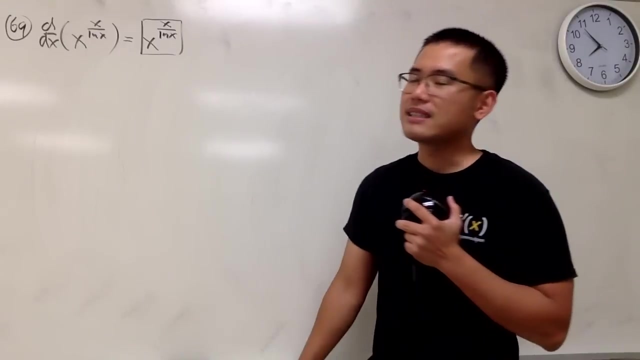 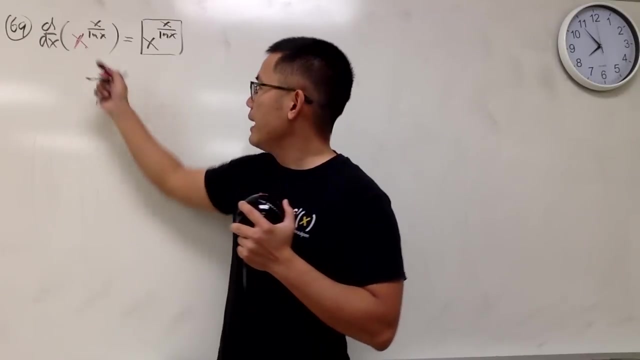 done. wow, what is happening? how can you have the derivative equals to the function itself? there's only one function that can make this happen and, yes, this is e to the x. this is how. look at the base. remember, we have x. this is the function, and this power is also a function, ideally speaking, we want 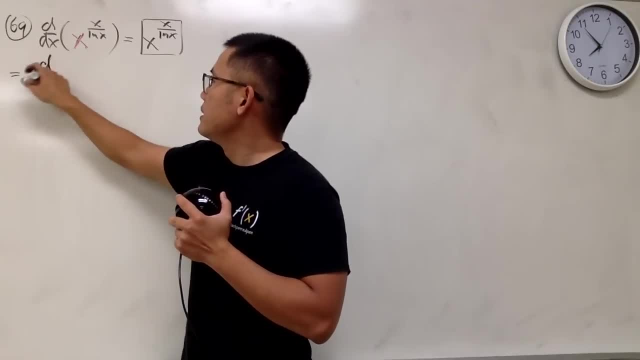 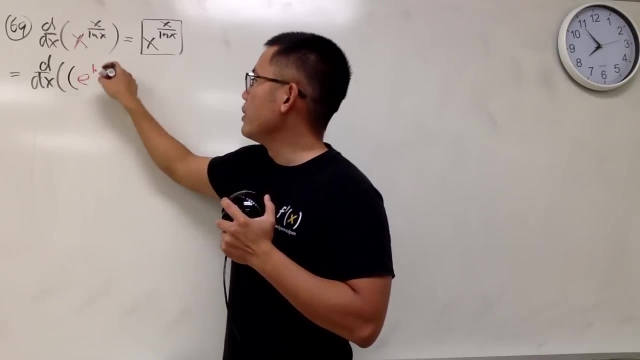 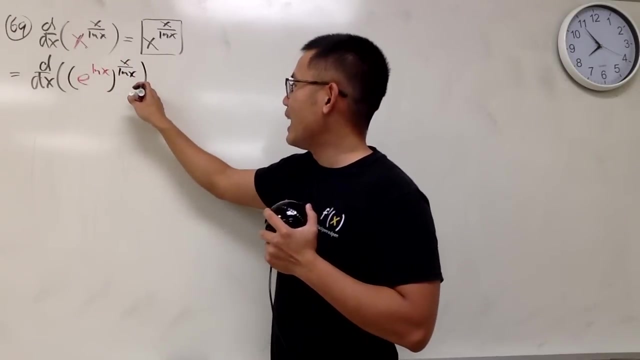 to work with space e. so we do this: this is d, dx, this x, right here, that's right here. e to the natural log of x, right, and then we raise that to the x over. ah, i know, you see it now. huh, right, because now when you multiply the powers, the natural log of x will cancel. so in the end, 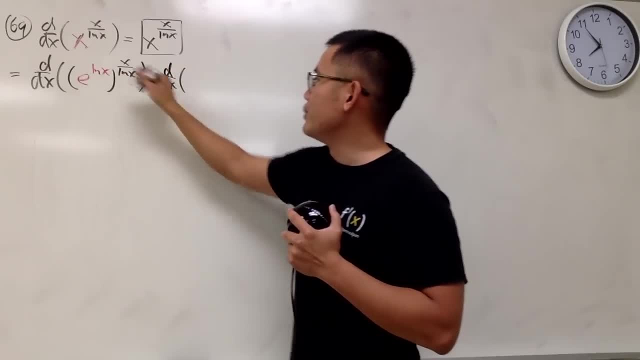 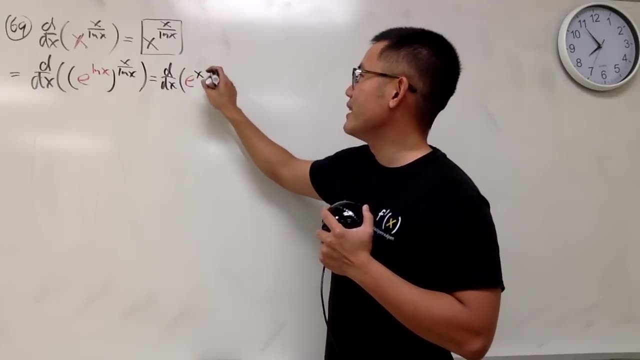 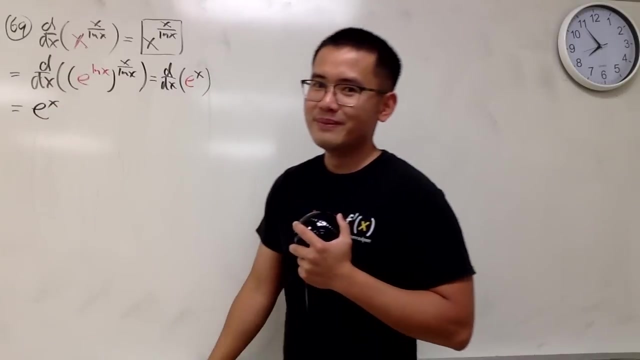 you just have to differentiate e to the x power right, the natural log of x will cancel. we just have to differentiate e to the x and, of course, e to the x will give you e to the x for the derivative and, of course, for this particular question, let me just write it as x to the x. 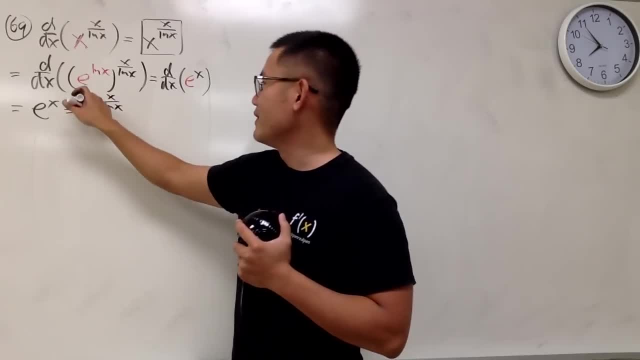 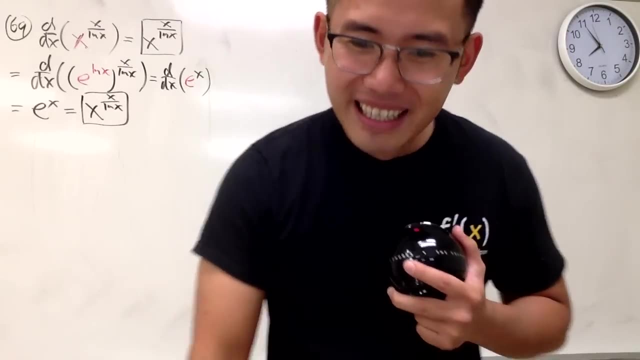 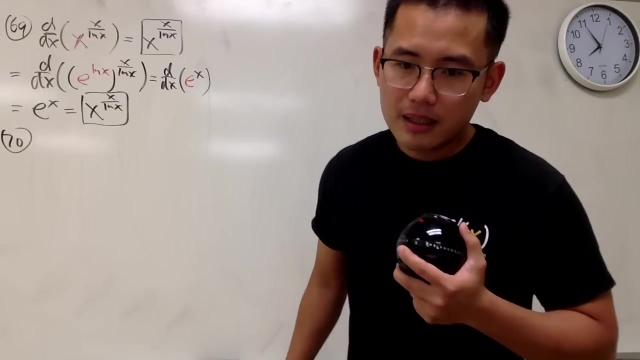 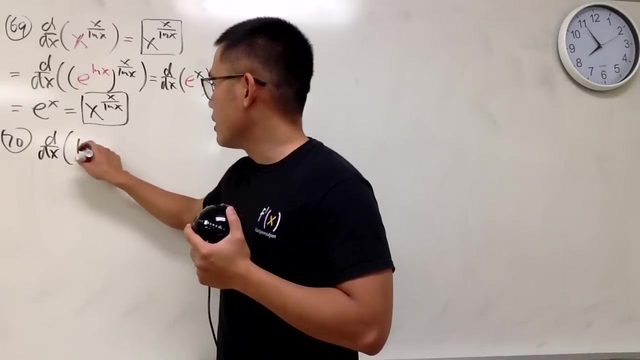 over one x to the x over natural log of x, just for fun for that uh, crazy looking expression. okay, hopefully nobody gets too mad on this one number 70. uh-huh, let's see differentiating natural log and we have a square root right. so this is a natural log and the input is the. 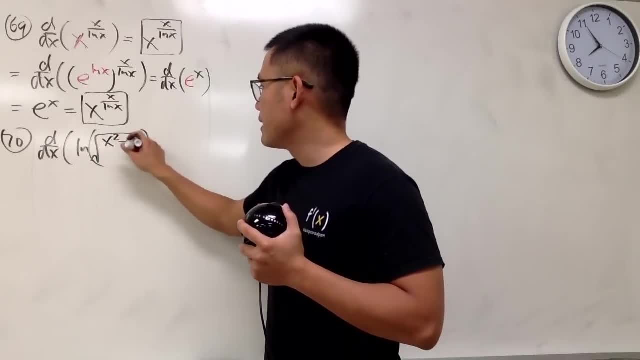 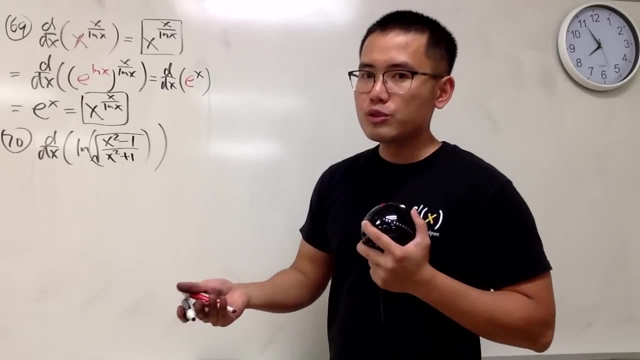 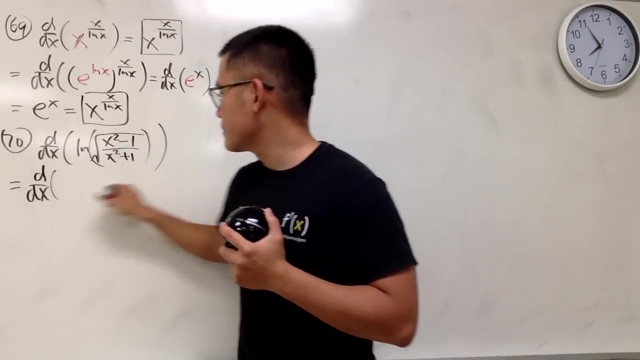 square root and inside here we have x square minus one over x square plus one, like this. All right, Shall we do some algebra first to simplify? Yes, we totally should, so I will do the algebra right here. ddx, As You all know, this right here is the 1 half power, and now this time. 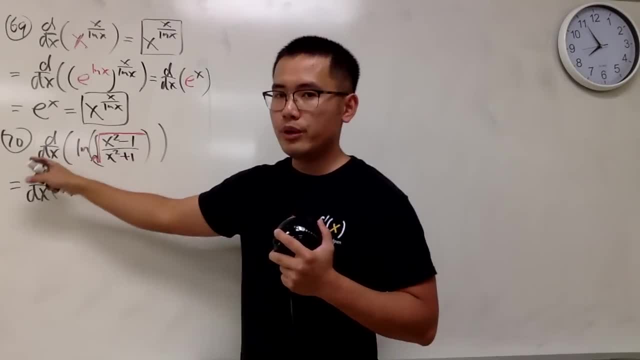 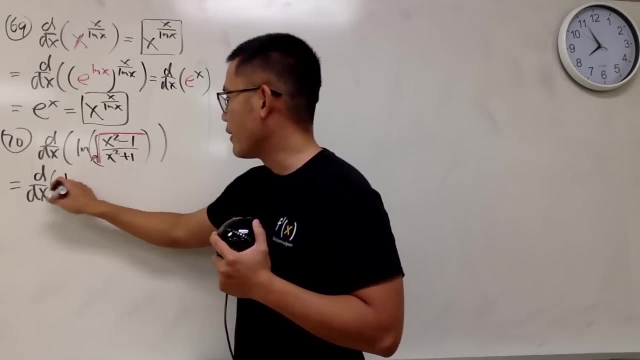 Let's just do a lot of the algebra in your head. okay, 1 half power can be bring to the front and the natural log of a quotient can be split into a subtraction. so First you will have 1 half natural log of this input, x squared minus 1. 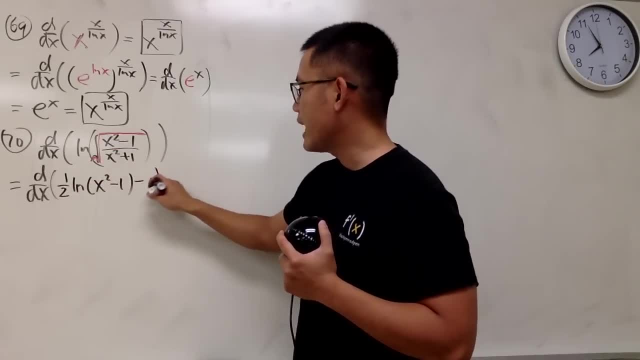 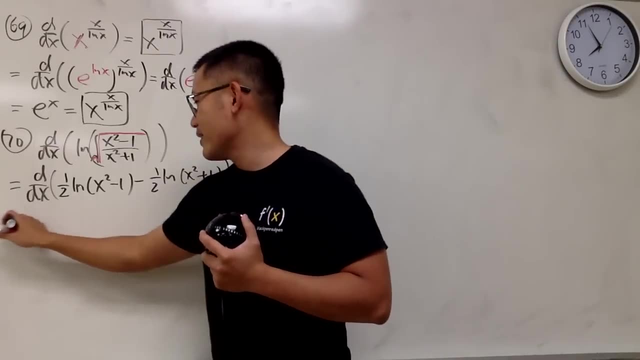 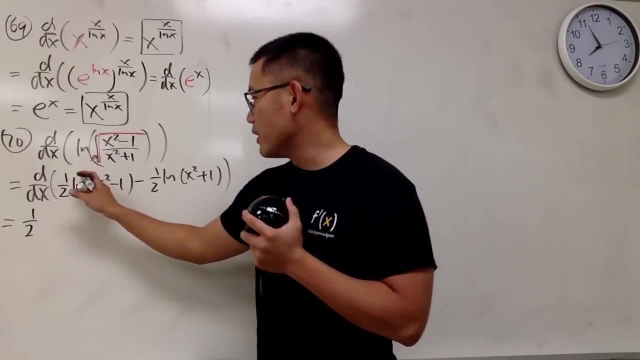 And then 1 half times the other one. so we have minus 1 half natural log of the bottom, Which is x squared plus 1, like this. All right, so Let's just do the derivative now. 1 half is a constant multiple, So just keep it right here. and the derivative of ln of something, It's just 1 over that thing, right. 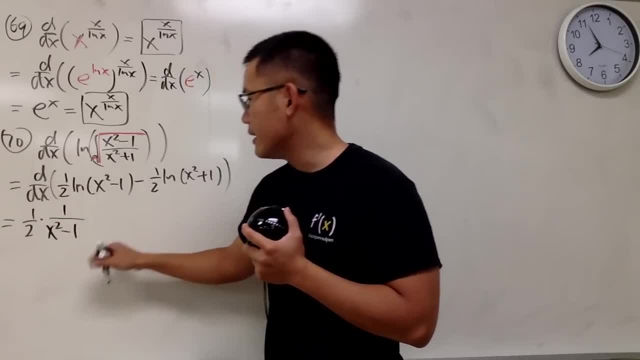 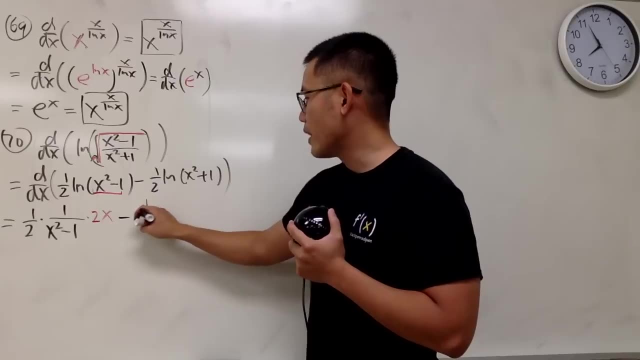 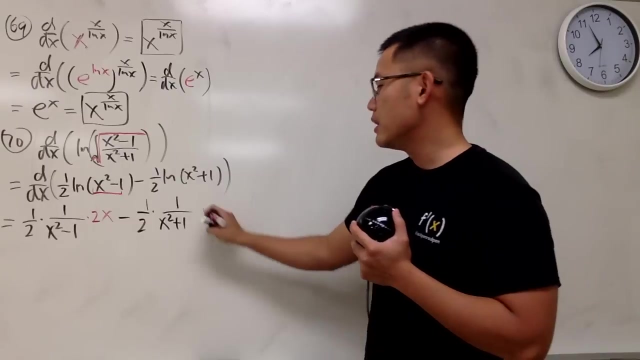 So 1 over x squared minus 1. but We multiply by the derivative inside, which is 2x. the chain to say so, and right here minus 1, half again 1 over the derivative. This is x squared plus 1 in the denominator. Multiply by the derivative inside, which is 2x, like that. 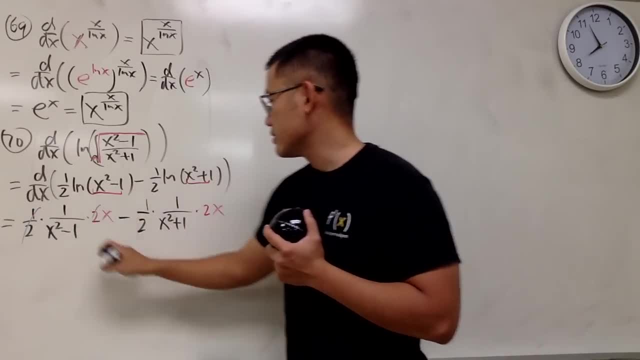 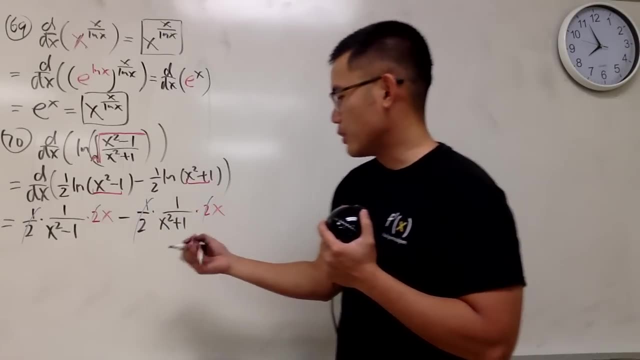 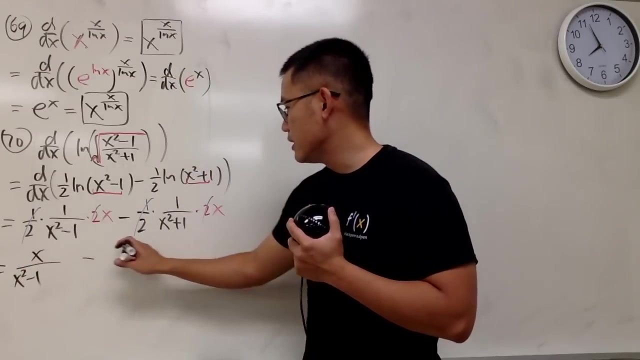 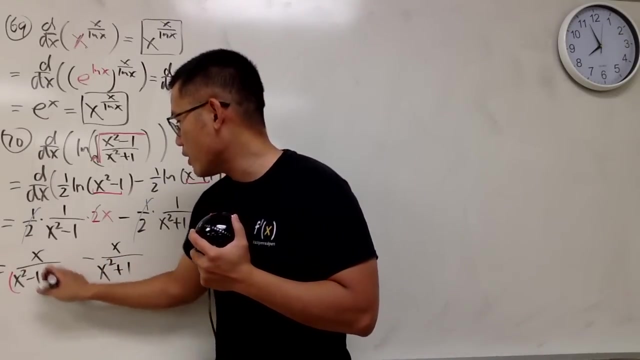 Check this out: This and that cancel, this and that cancel, and we just have this minus that. So I will just write this down for you guys. This right here is x over x squared minus 1 and minus x over x squared plus 1. Well, if you want to combine the fractions, which we will 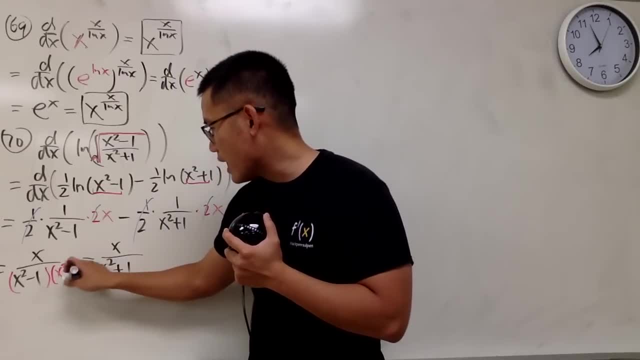 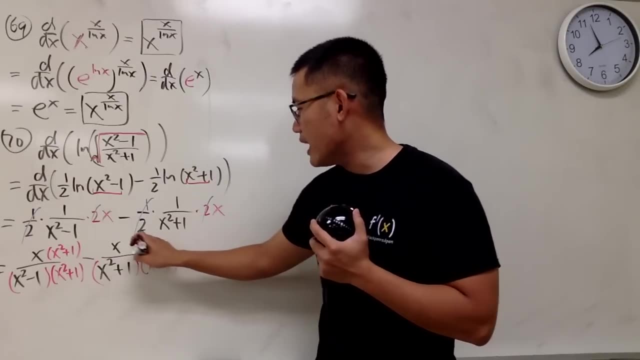 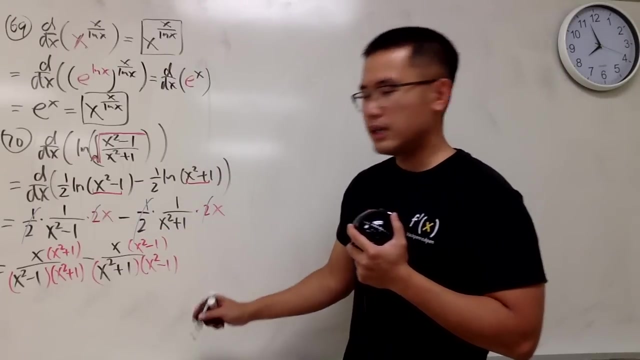 Let's just multiply this one by x, squared plus 1, on the bottom and also on the top, and Multiply this one right here by x, squared minus 1, on the bottom and also on the top. now, Let's see, I will have the space right here. Let's see. 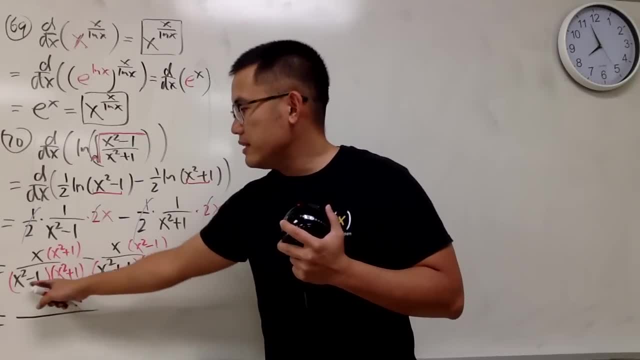 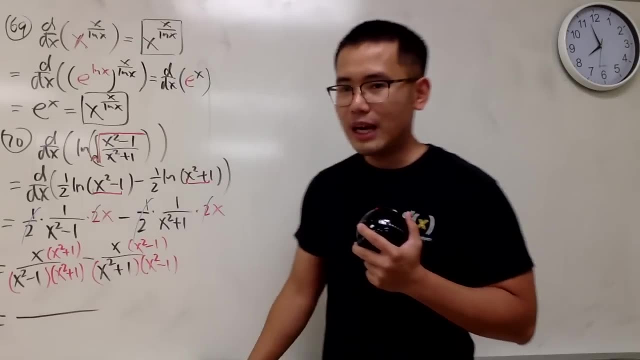 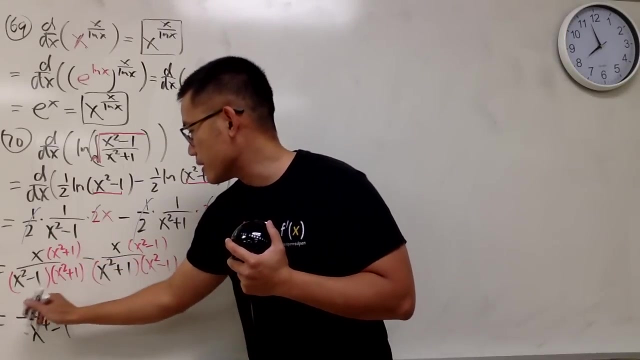 both of them Have the same denominator. This is a. This is a minus B times a plus b, differents of two squares. If you multiply out this and that we end up, it's x to the fourth power minus 1. alright, and The top rise- you see this right here- is x to a third power. 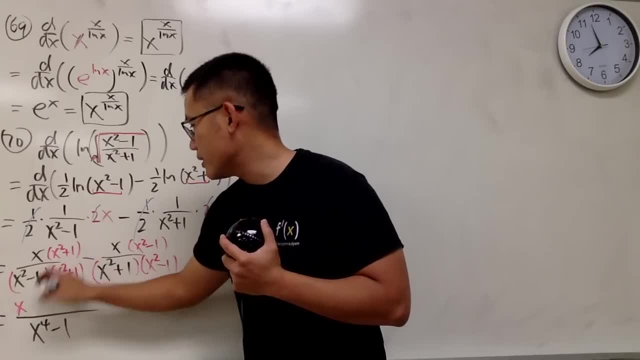 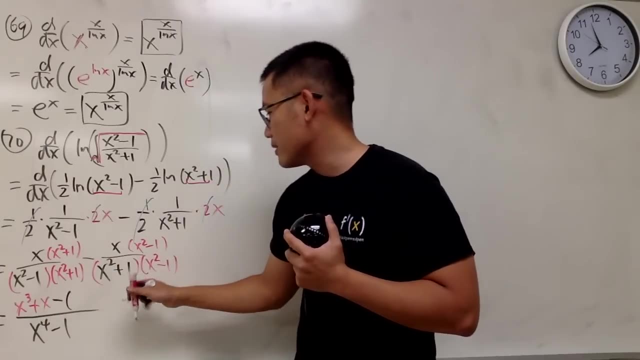 Let's put it down in black that in red x Times x square is extra. third power am: plus x, minus Parentheses this times that Let's just distribute, so it becomes easier. Minus x times that which is negative: x cubed. 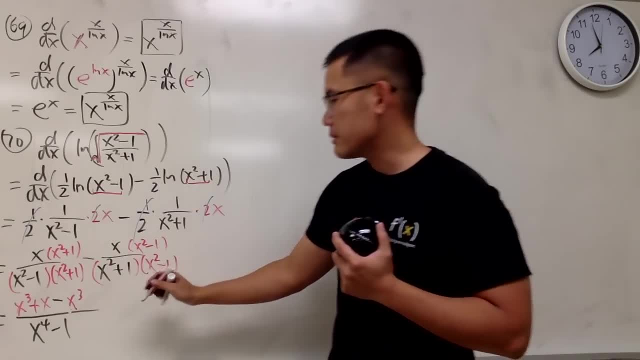 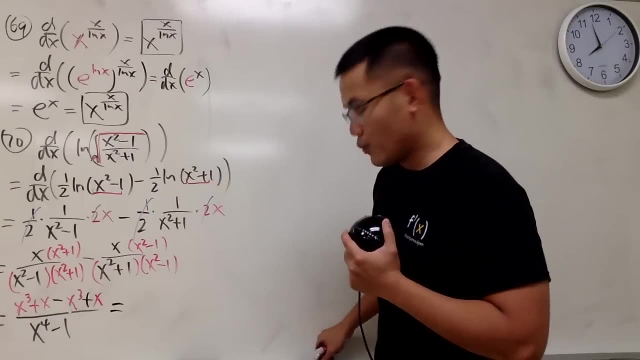 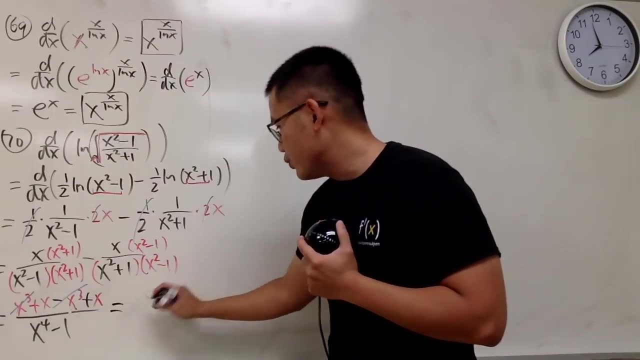 and then minus x times negative, 1 becomes plus x. Yeah, so plus x. In the end, once x to the third power minus x to the third power can be cancelled. x plus x is 2x over x to the fourth power. 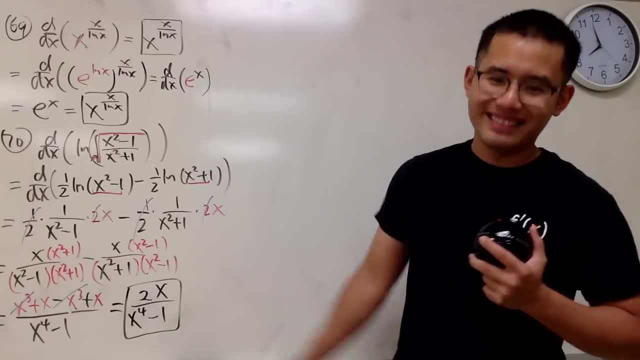 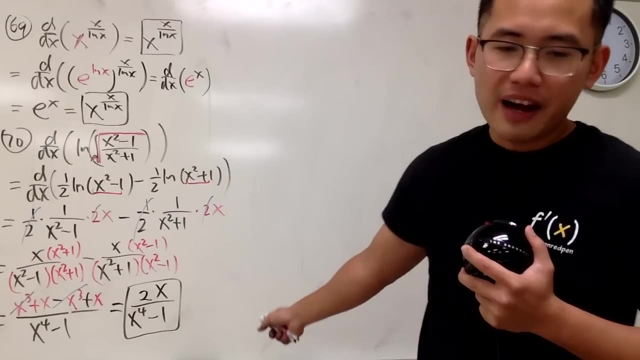 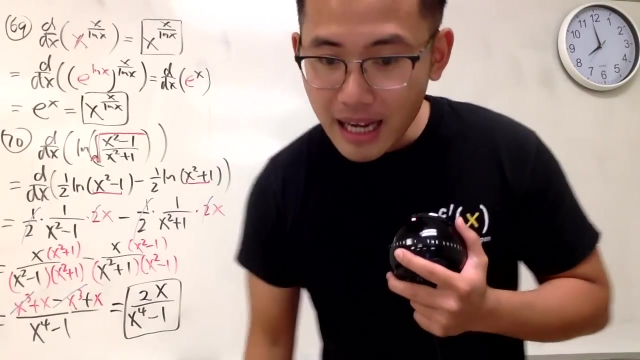 minus 1.. We're done, So it's a very nice one. So it's kind of similar to number 65, but this one you do have the natural log already, so that's what it's meant to be right. Ah, 71.. 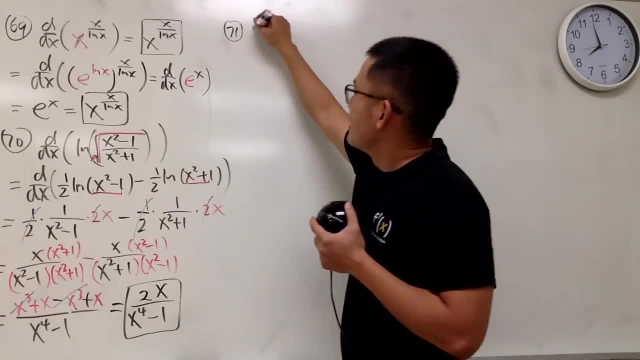 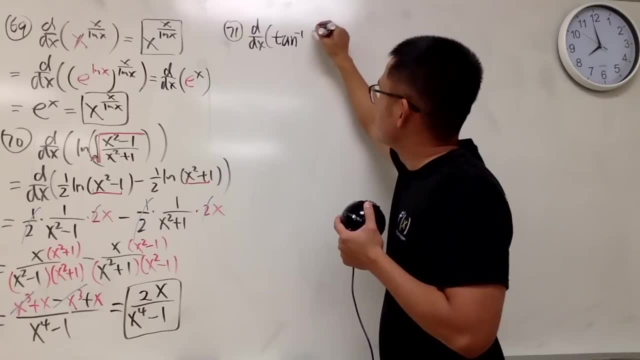 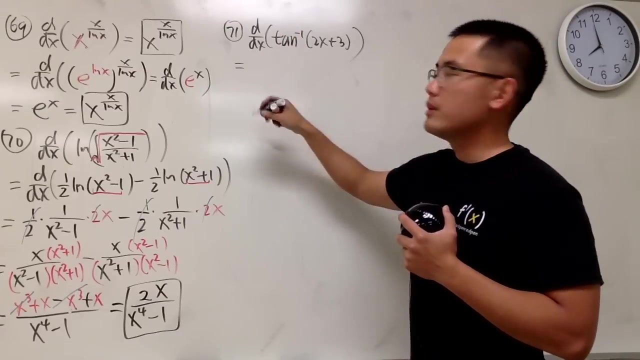 Okay, so this question is not so bad. it's just that I put like some second derivative and also implicit differentiation earlier and I was like: oh man, Anyway, inverse tangent of 2x plus 3.. Here we go, Inverse tangent, you get 1 over 1 plus. 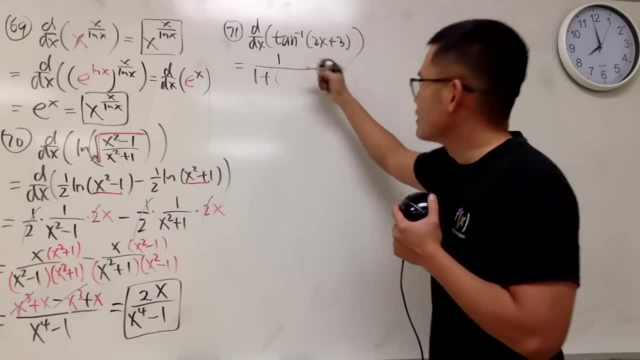 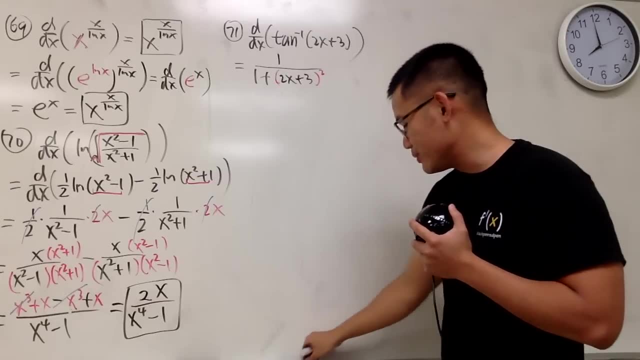 and you have to square the input right here. right? So put down 2x plus 3, and we square that. And what else do we have to do? Yes, Chengdu, Multiply by the derivative of the inside, multiply by these two. 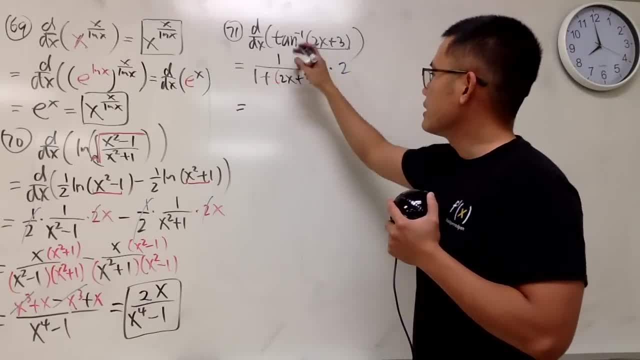 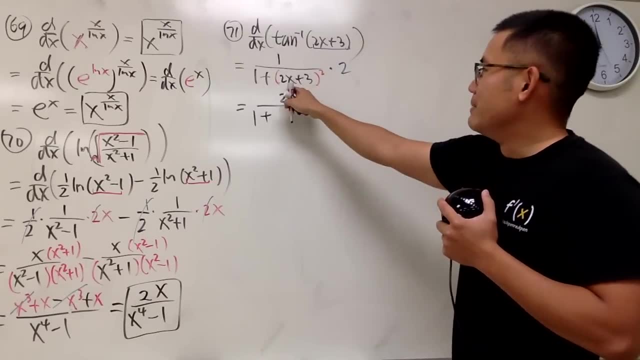 Okay. so now let's see what we get. On the top we have 2,, of course, On the bottom, this is the 1 plus. let's square this out- Binomial, right? So this is 2x squared, so it's 4x squared. 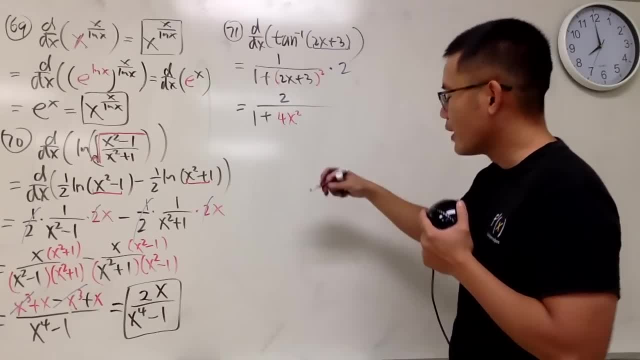 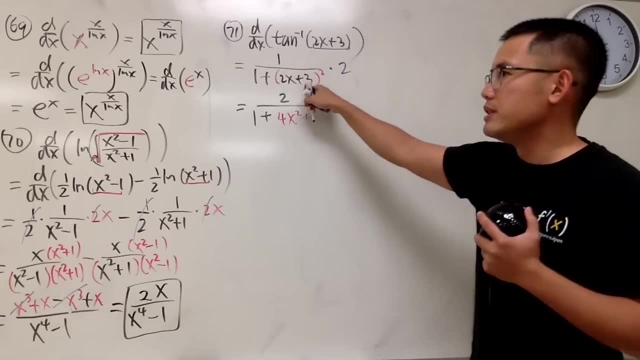 Right, 2x. you square that, You also square the 2, so it's 4x squared. And then the next term is plus 2 times. this times that 2 times 2x is 4x times 3 is plus 12x. 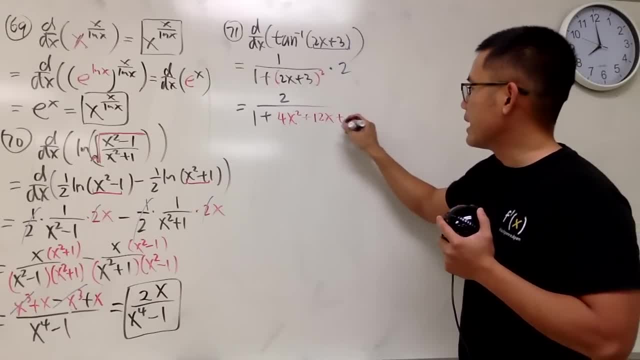 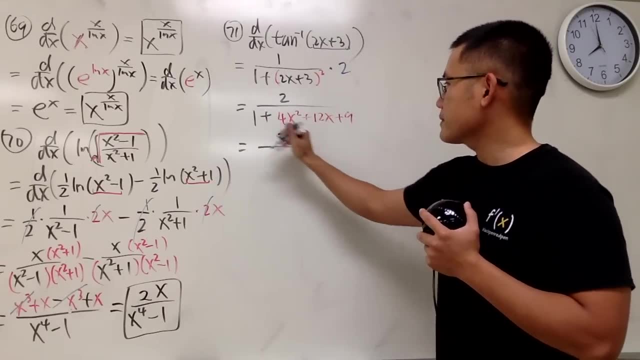 And lastly, you add 3 squared, which is plus 9.. So it's just like that: On the bottom, 1 plus 9, we can do that. So on the top we have 2 over. so again 1 plus 9.. 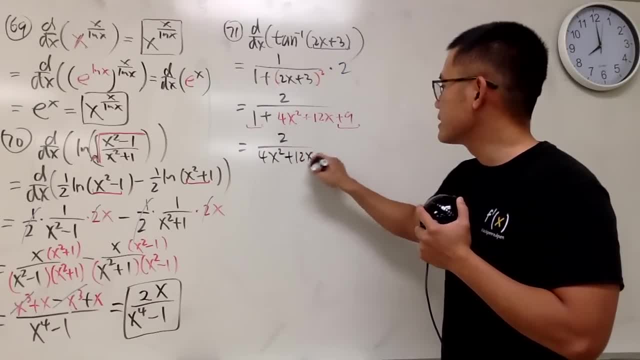 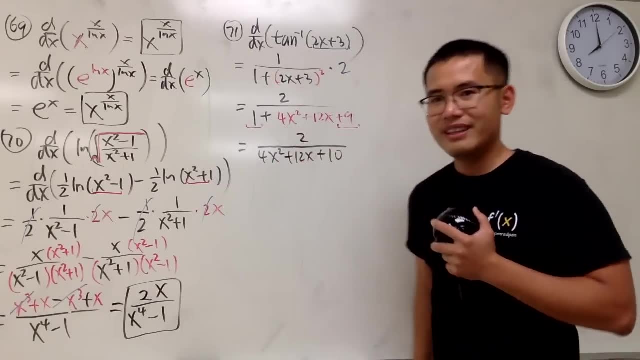 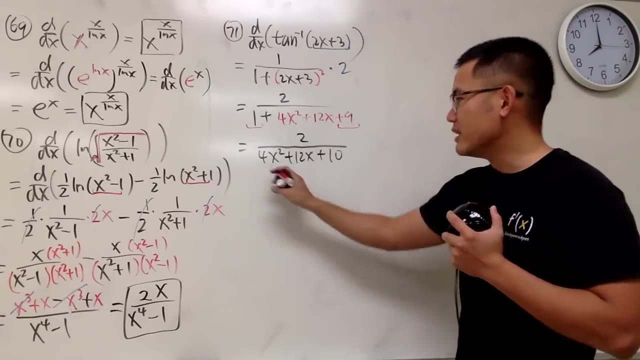 So here we have 4x squared plus 12x plus 10.. Let's put a 2 in the middle. It looks better this way: Reduce, reduce, reduce. We can factor out the 2 and reduce it. So you see, if we factor out the 2, it becomes 2x squared. 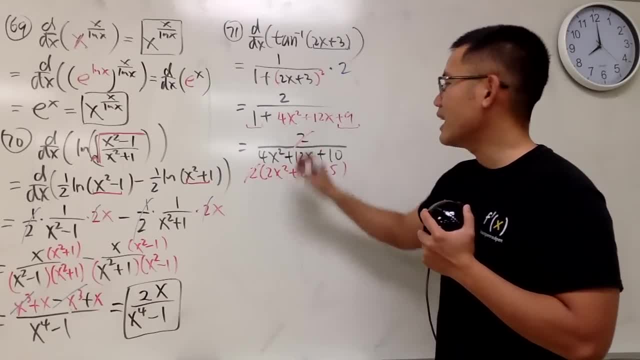 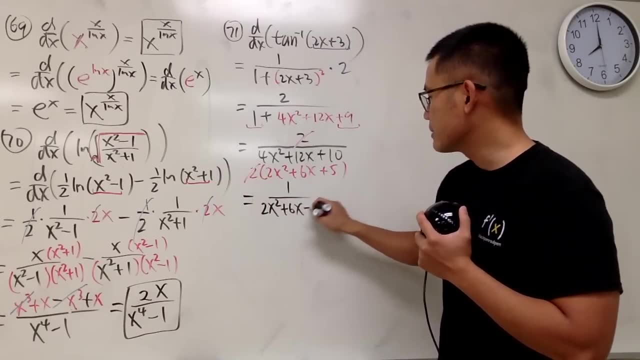 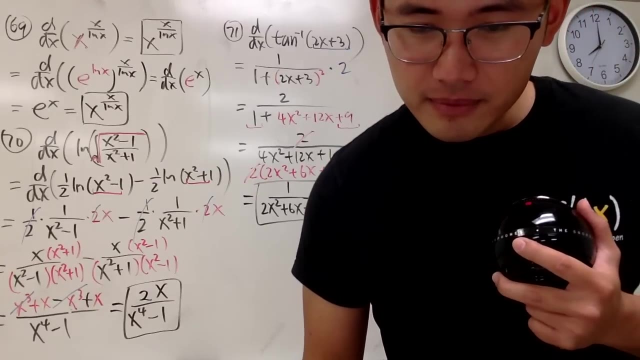 plus 6x plus 5.. And then we can reduce this and that. Very nice. In the end the answer is 1 over 2x squared plus 6x plus 5.. And with that we are done. Okay. cotangent to the force power of 2x. 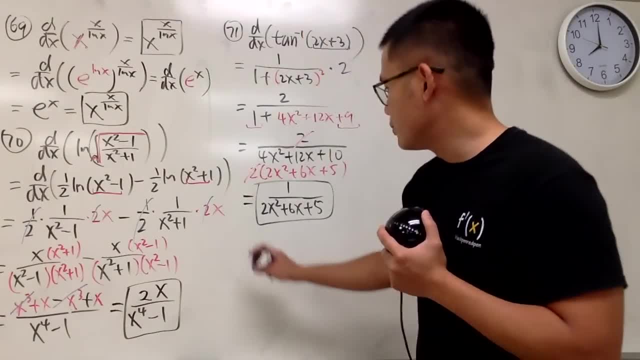 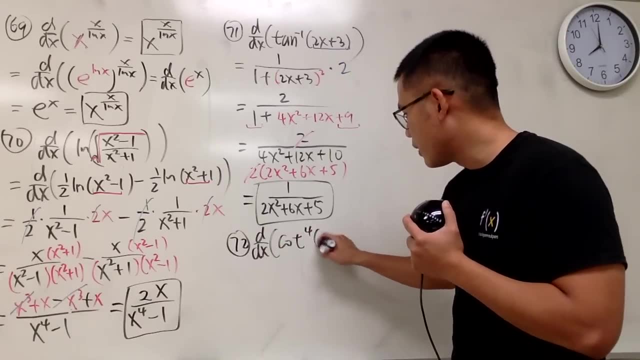 Number 72.. I don't think we need too much, Please, for this one, So number 72.. Differentiating, as I said, it cotangent to the force power of 2x. All right, Okay, here we go. 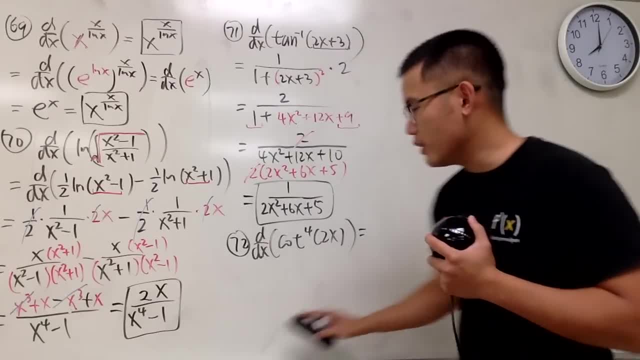 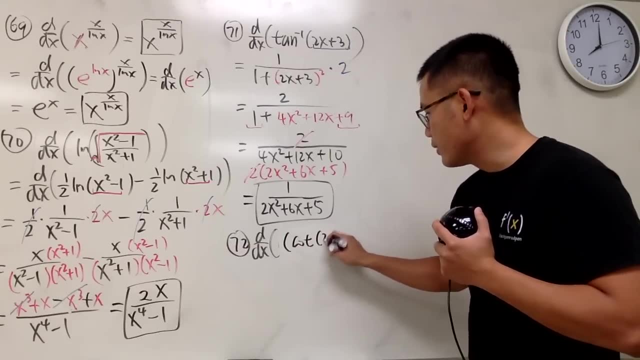 Look at this right here as cotangent of 2x and then to the force power. So perhaps I'll just write it down right here: Cotangent of 2x, like this, And then to the force power. Okay, here we go. 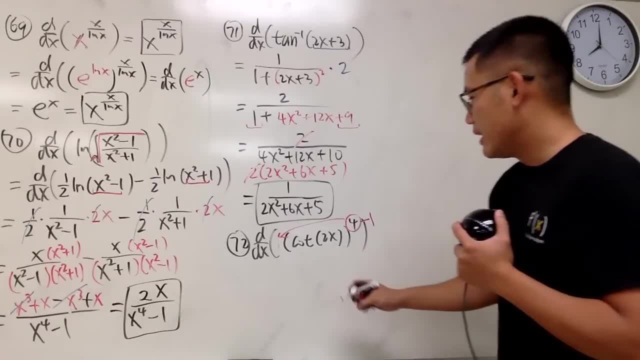 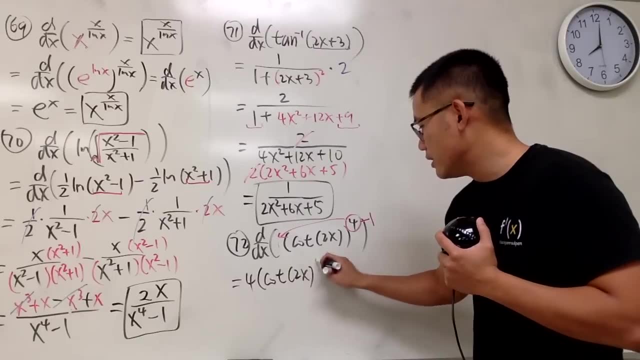 To the power to the front minus 1.. Okay, All right, so we get 4.. And the first part is cotangent of 2x to the third power. And then the Chengdu says: multiply by the derivative of this. 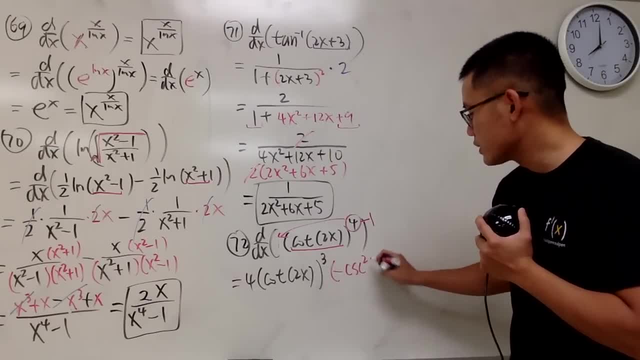 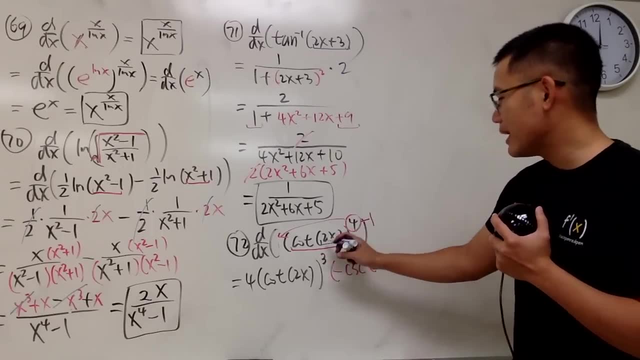 Derivative cotangent is negative, cos secant squared And we keep the same input like that. But the Chengdu of the Chengdu says we have to multiply by the derivative of 2x, which is 2.. Multiply by 2.. 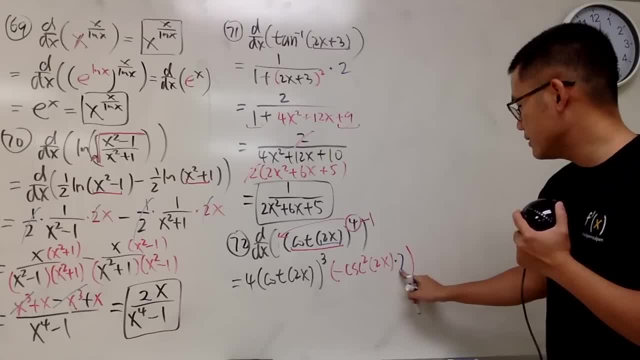 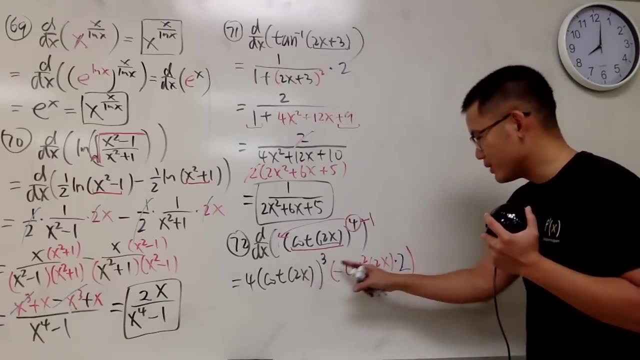 So it's technically like this. if you like, This is a 2. Because this whole thing is at the derivative of the exact. That's why I put the parentheses like that. If you put it right here, it's fine too. 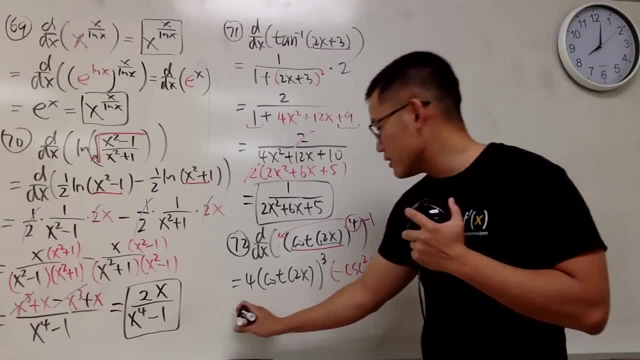 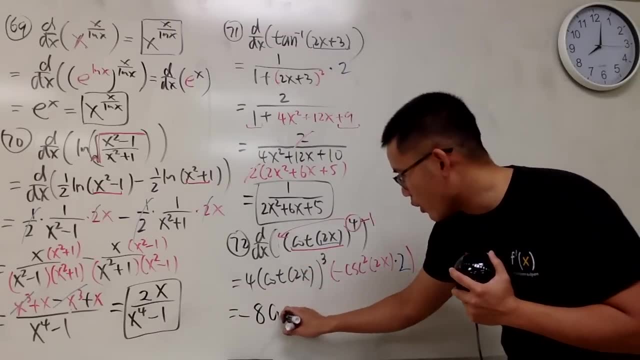 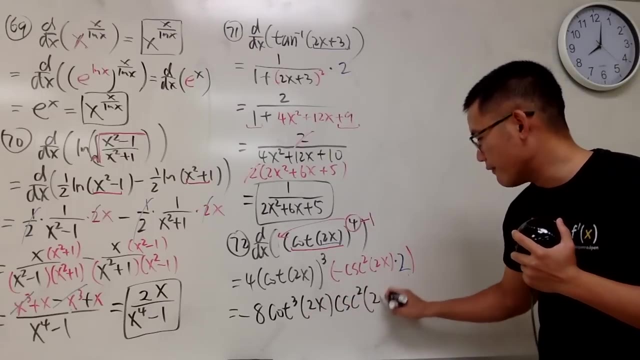 It doesn't really matter that much anyway. Finally, we have the answer 2 times 4, and then that's negative, So we have negative 8.. This right here cotangent third power 2x, And then cos secant squared of 2x. 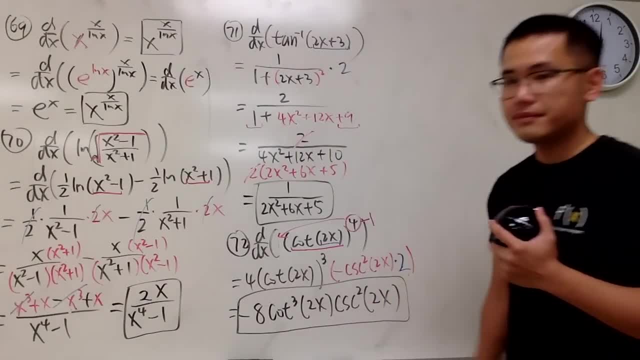 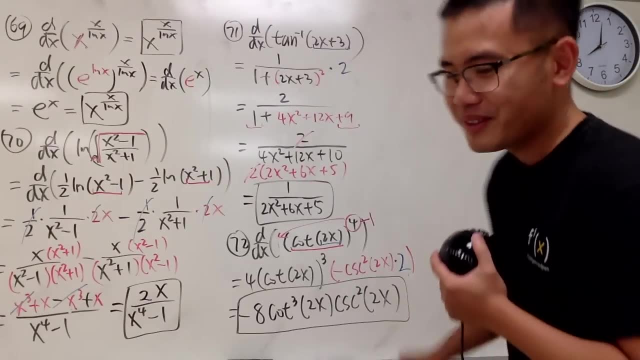 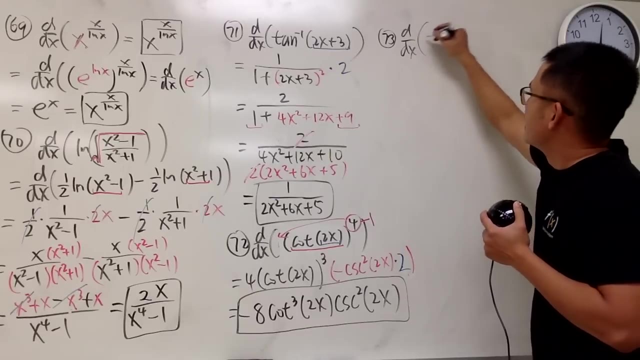 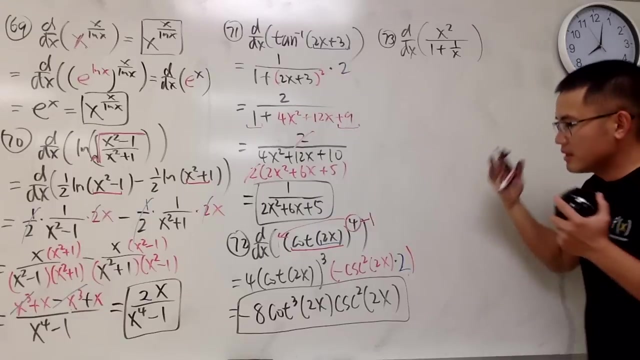 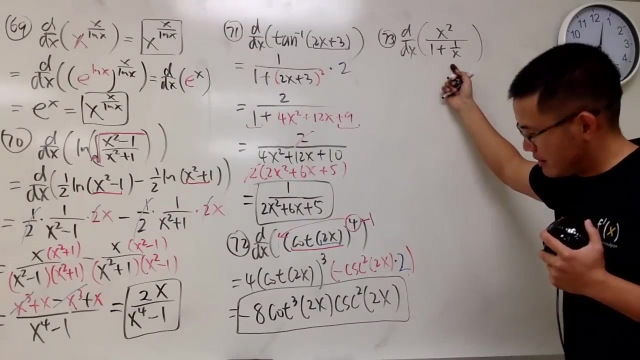 That's it. Ah, complex fraction. Oh my god, complex fraction. Okay, that's 73.. d, dx, And hopefully you should do enough derivative equations so that you can get confidence Like you can differentiate anything This right here. we start off with a complex fraction, but do algebra first. 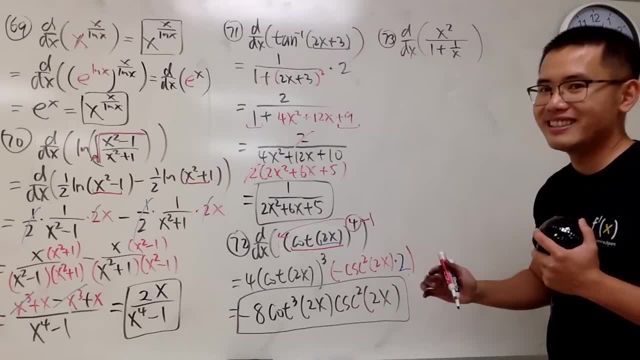 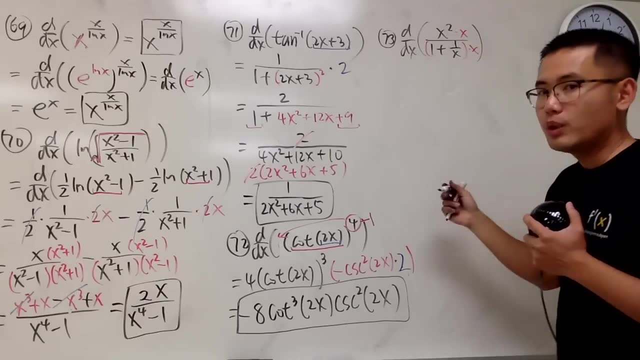 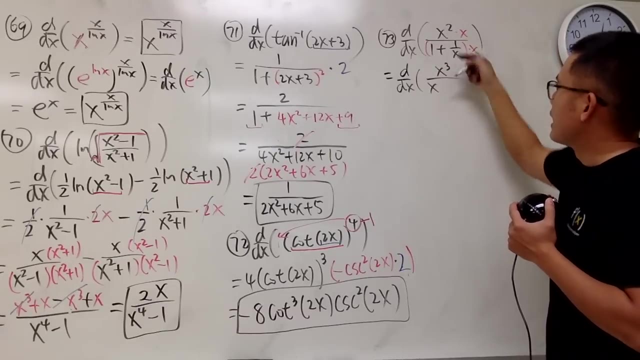 Do algebra first, so that our calculus life will be much easier. So right here let's multiply the top and bottom by x, So that we'll see this. right here is just d dx. On the top is x cubed Over x plus 1.. 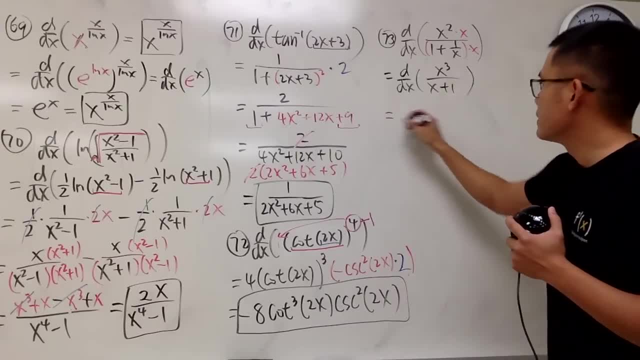 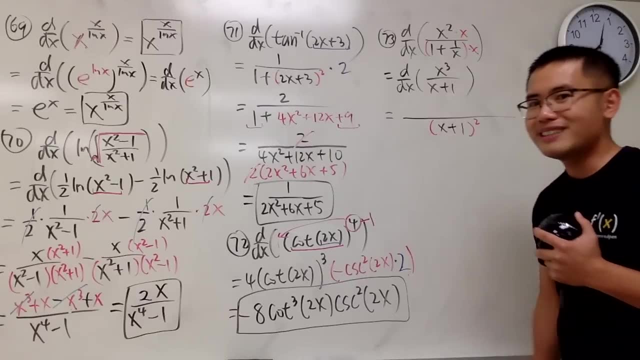 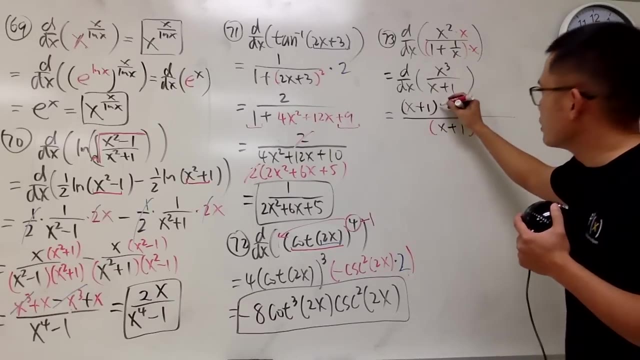 And now this is just a nice quotient rule equation. So square the bottom. Let's put down parentheses with x plus 1.. Let's square that. And then the top, Put down x plus 1.. Times the derivative of the top, which is going to give us 3x squared. 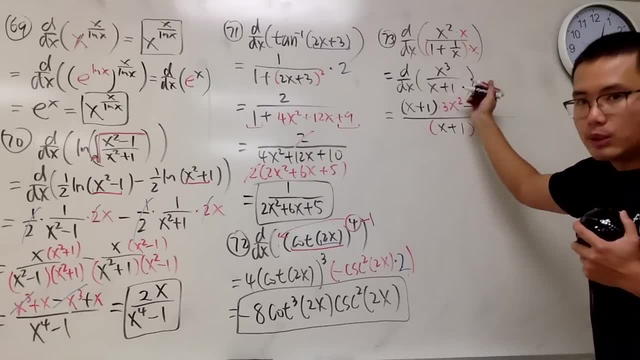 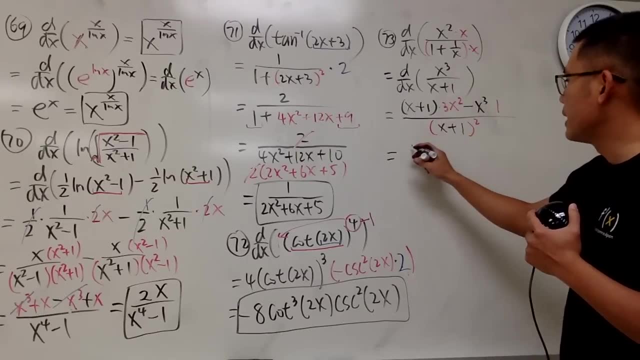 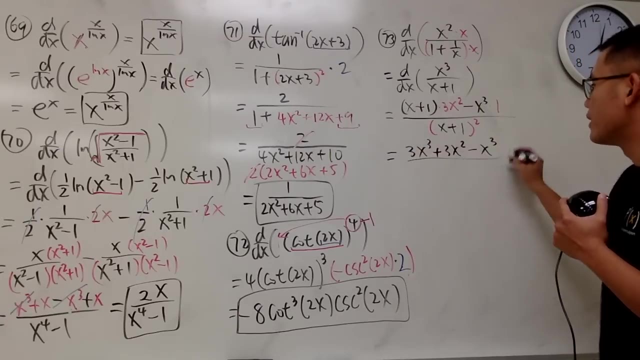 And then minus the top function times the derivative of the bottom Derivative of the bottom is just 1.. So that's what we have, Cleaning things up a little bit. multiply this out: we get 3x cubed plus 3x squared and then minus x cubed over parentheses. x plus 1 to the second. 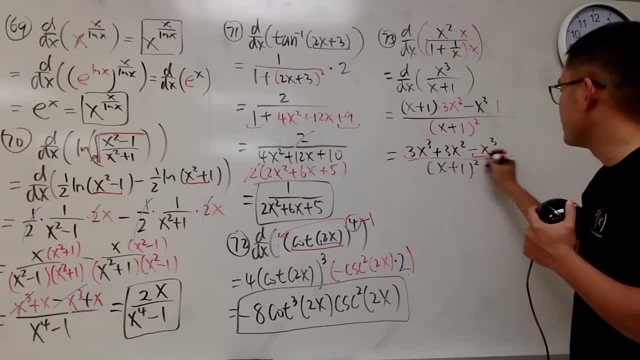 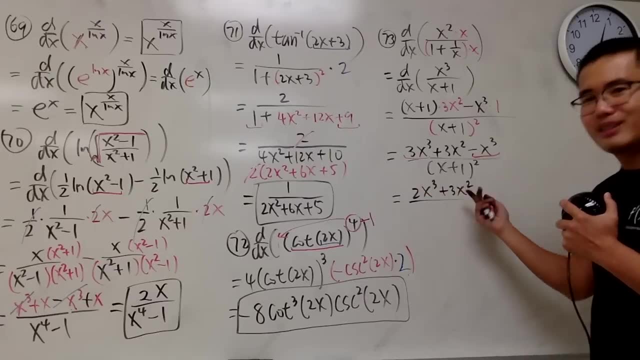 power. This and that can be combined, So we will. this is 2x cubed plus 3x squared. Hey, just to reverse, Cool huh. This right here is x plus 1 to the second power, And with: 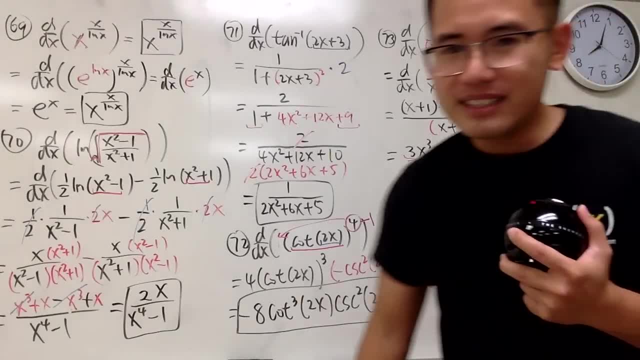 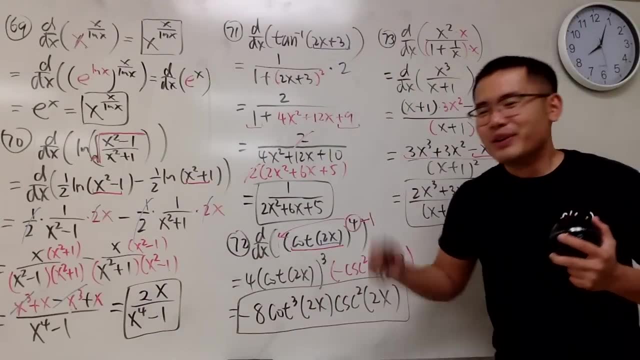 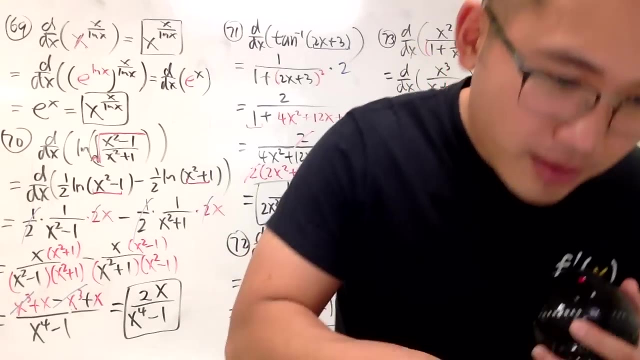 that we are done. Not so bad, not so bad, not so bad. 3 more sheets, 20 something, I don't know, man, 28.. Any questions? I have to look at this carefully, because I just want. 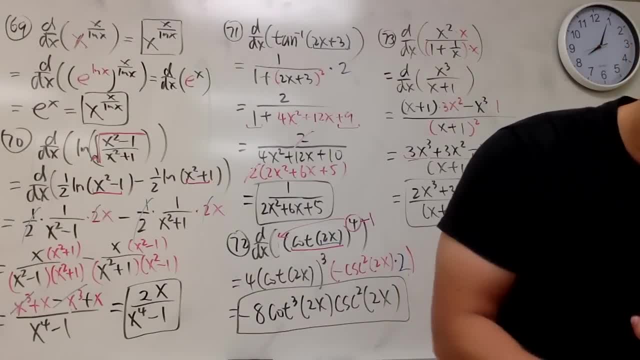 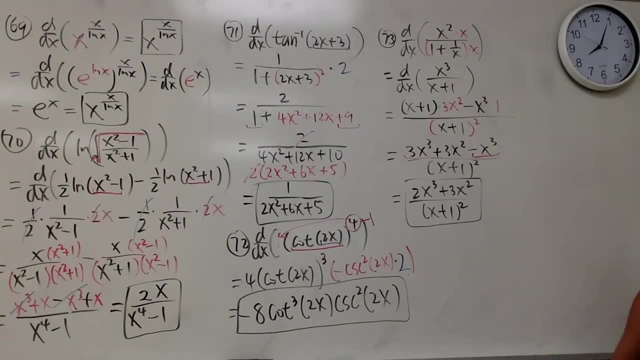 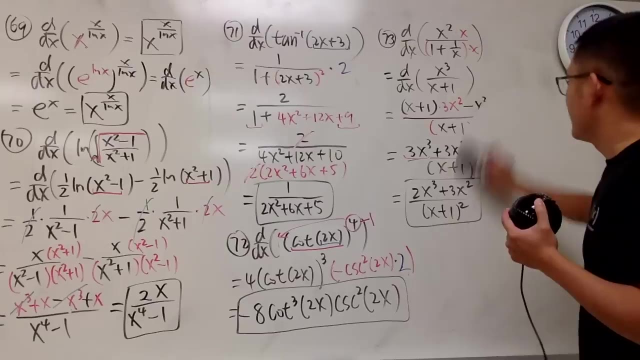 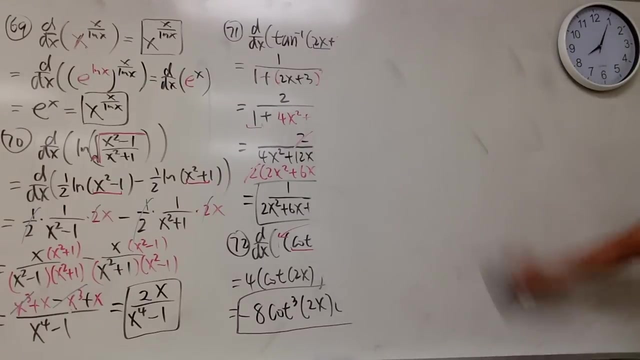 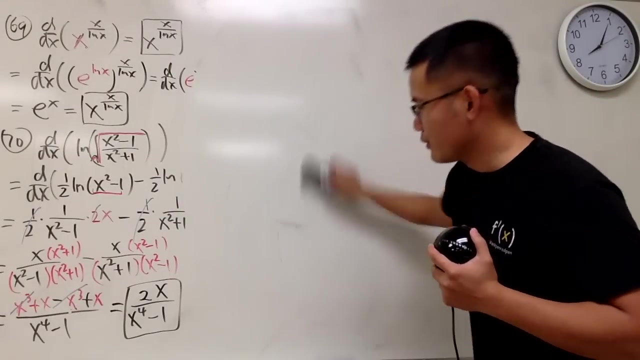 to save paper, so the printout is tiny. So this right here, 70.. I will go on the no, I will just, I will just erase. I will not be lazy. I will erase, I will erase. Uh huh, It's like I will survive, I will survive. Uh huh, Uh huh, I don't. 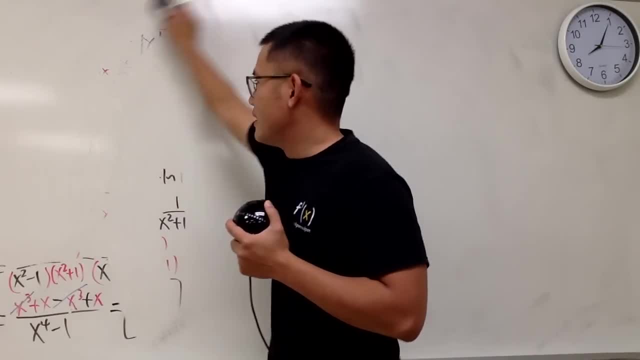 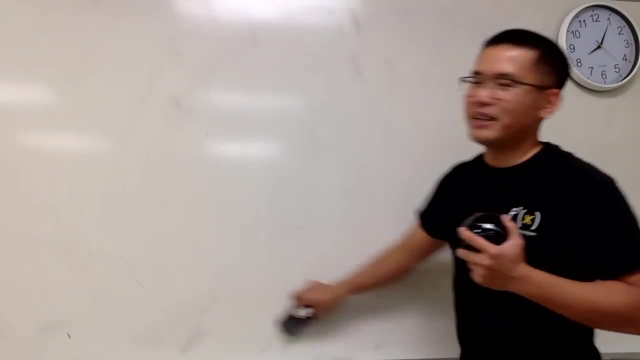 know Man, I remember, uh, I heard that music. it was still just the thing that is happening. I will survive. When I was running mirrors, I was like I will survive, I will survive. I know, even though it's not, it's not meant to be like for like running or so, but like it's, it's, it's. 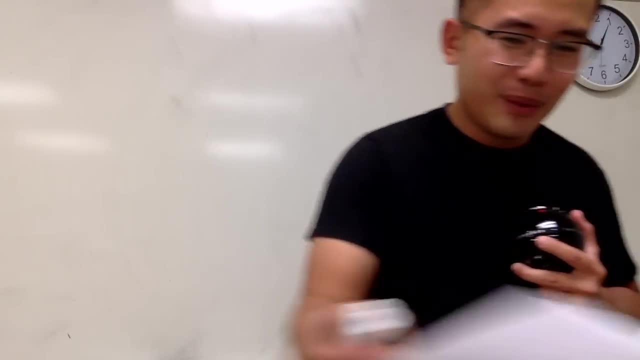 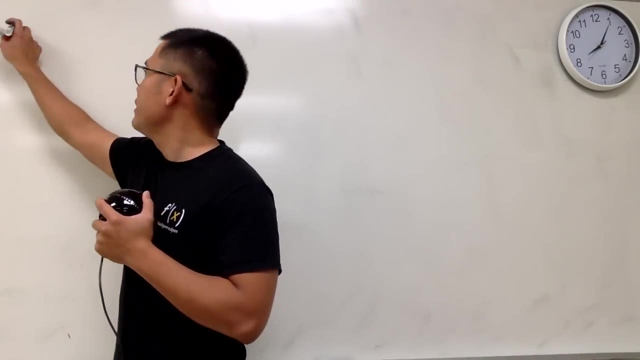 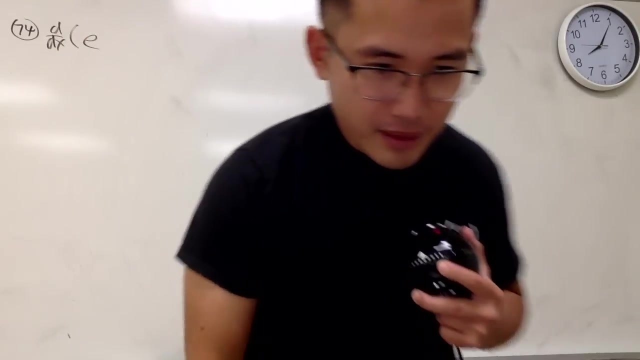 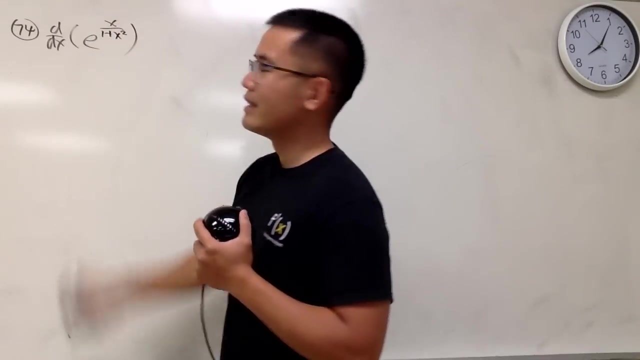 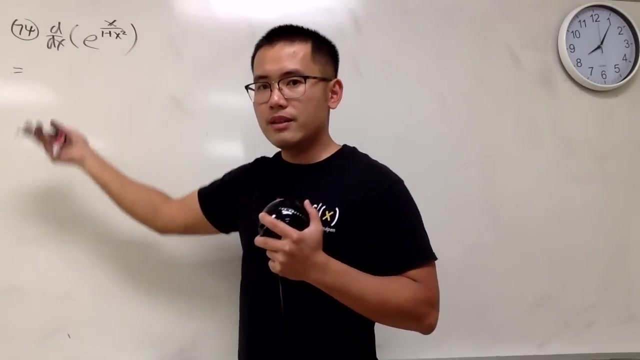 it fits like. let me just say I will survive. I will survive. Number 74, right here, Differentiating d, dx, e is e, e, x to the no x over 1 plus x squared power. So for this one we just have to, you know, do the outside and then like the quotient rule and all that. 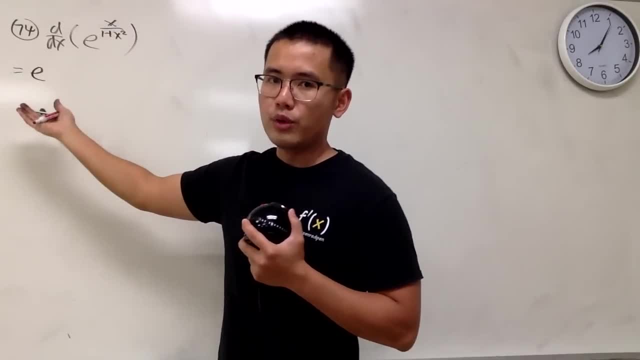 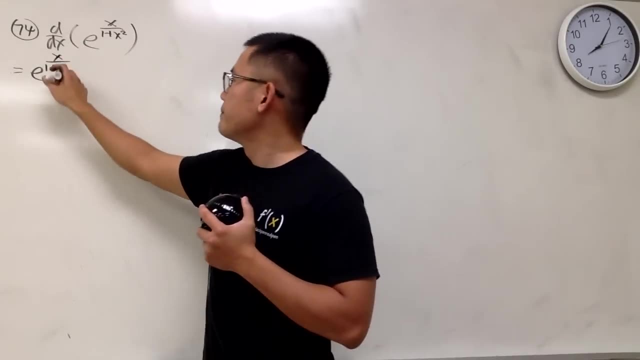 So first e to the power i over the derivative, for that is just e to that power i over. so e to the 1, e to the x over 1 plus x squared. Then what happens? Then what happens? 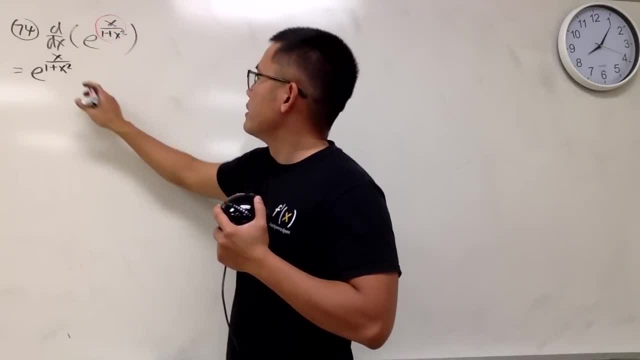 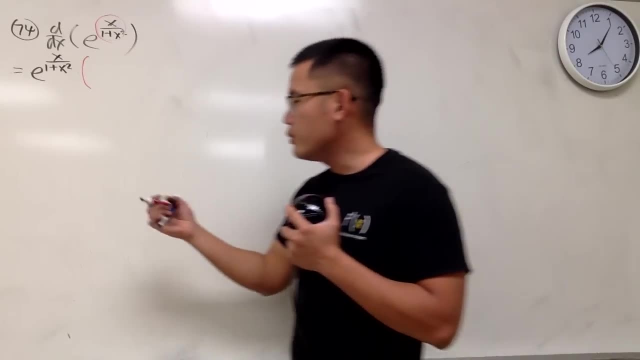 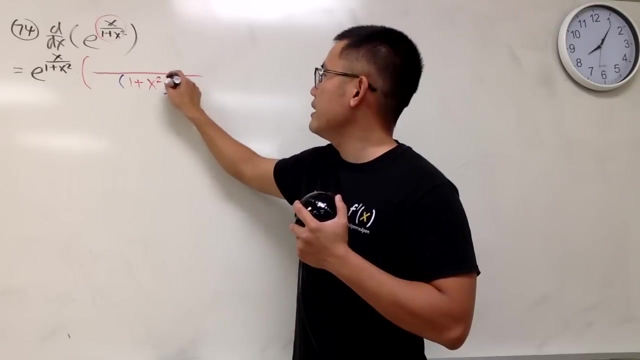 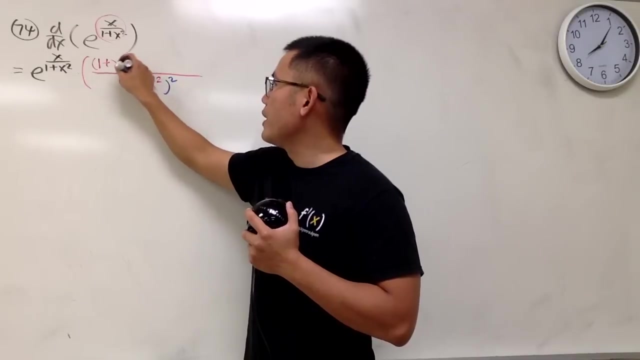 So we multiply by the derivative right here. So multiply by and we have to use the quotient rule. So we see that we have to square the denominator, which is 1 plus x squared, and square that Multiply. well, on top. right now we put on the bottom function: 1 plus x squared. 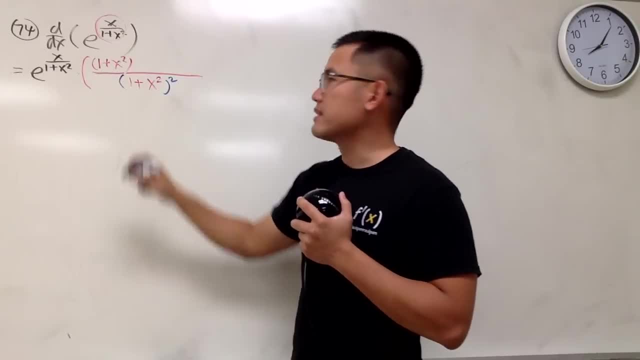 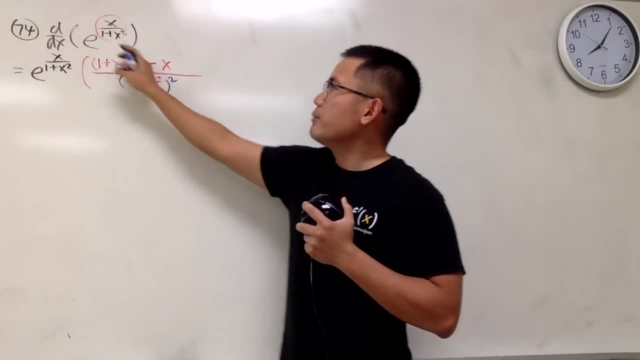 and multiply by the derivative of the top, The derivative x is 1.. So multiply. So we multiply by 1 minus the top function, which is x, And multiply by the derivative of the bottom: The derivative of 1 is 0.. 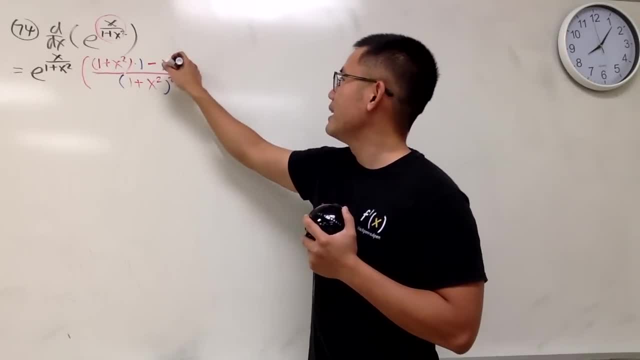 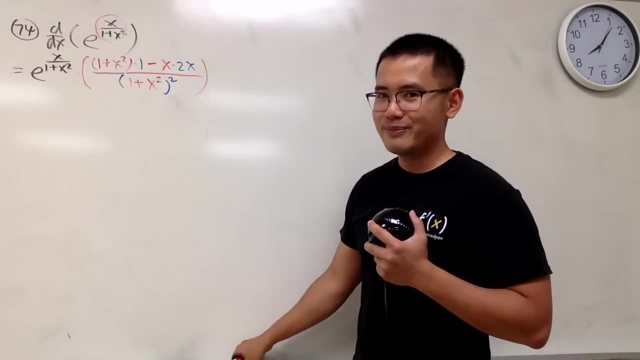 The derivative of x squared is 2x, So we just multiply by 2x, So that's pretty much it. Now we just have to clean things up, like we always do, Just like I will have to clean my hand later on. 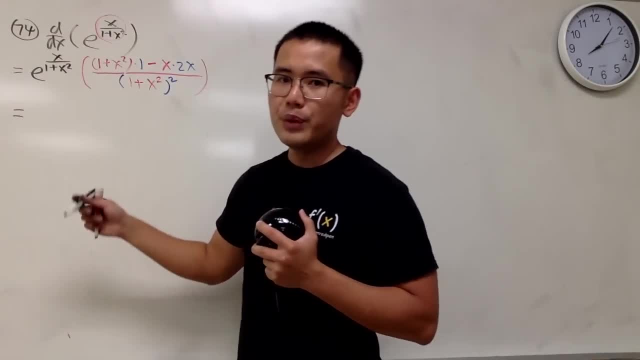 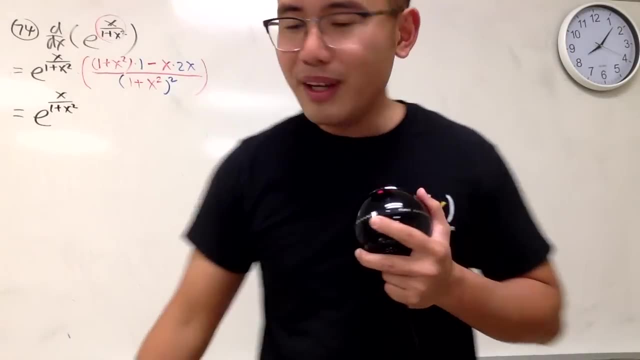 So yeah, Anyway, here we go. This is just e to the x, So this is 1 plus x squared. and how did I write that? Oh, I put that all the way on the top, It's okay. 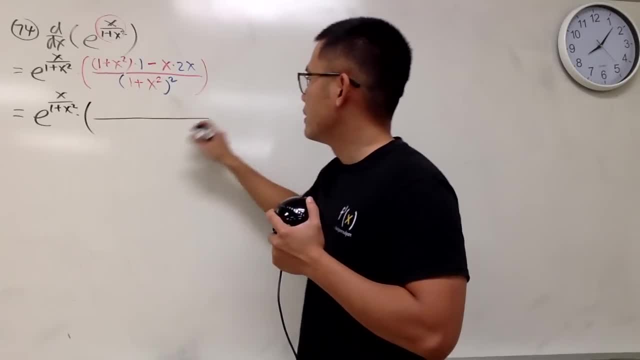 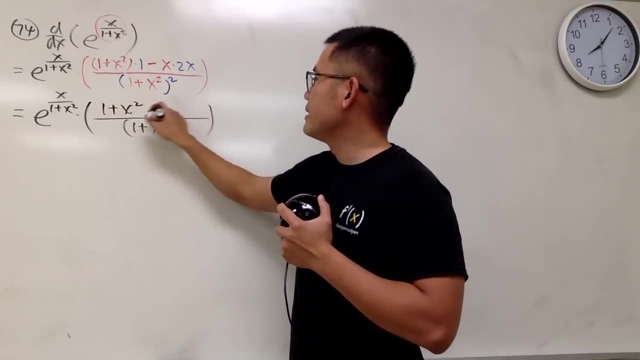 Later, later. Anyway, put it like this right here: So this is 1 plus x squared and square that: This right here is 1 plus x squared, and then minus this and that is 2x squared. So here is the answer. 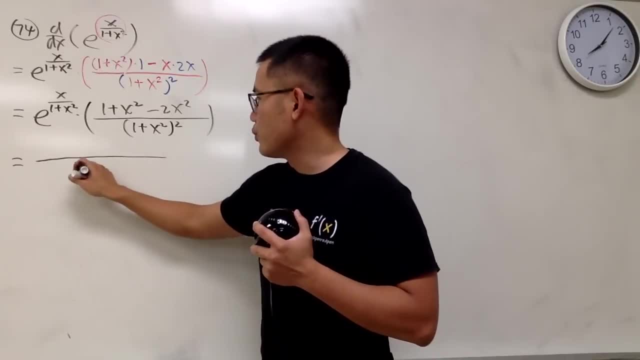 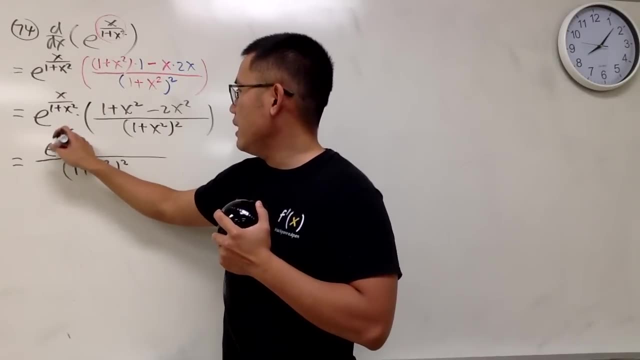 This is how I wrote it. I put this on the bottom only, So 1 plus x squared squared, And I put this on the top, So I actually have this first e to the x over 1 plus x squared. 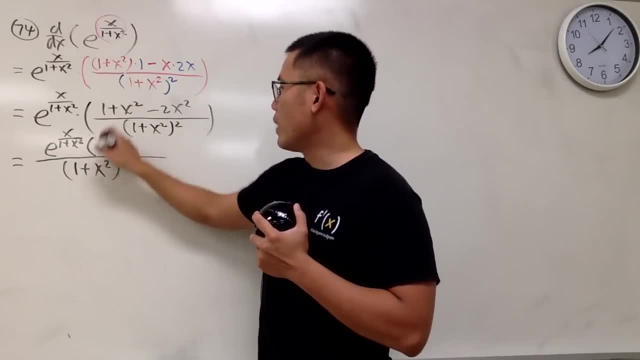 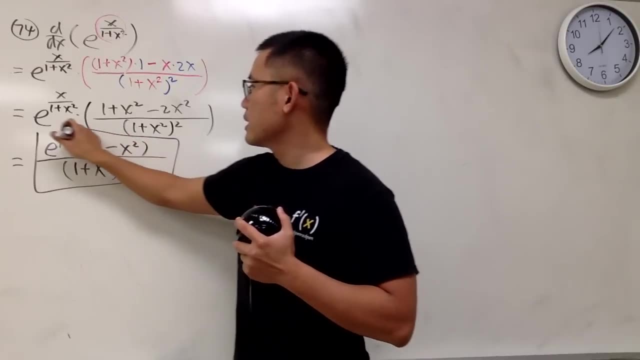 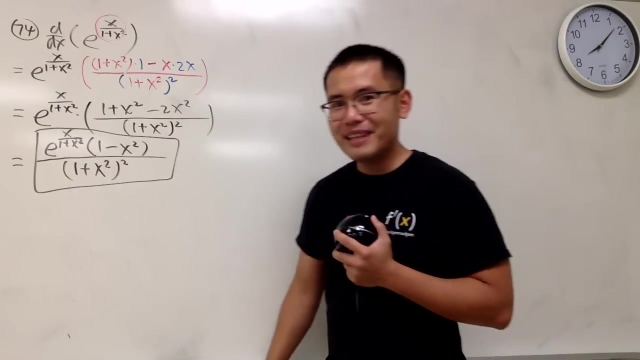 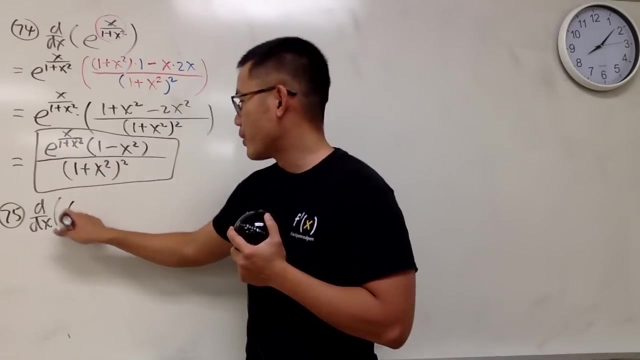 Okay, And then, of course, multiply by 1.. This is going to give us negative x squared, And with that we are done. Okay, Just like that. Next one, Number 75.. dx- Here we have parentheses. 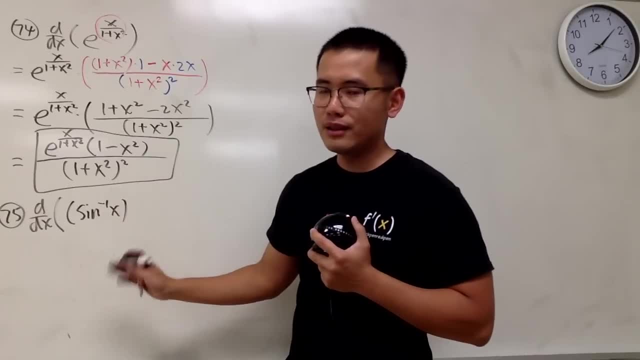 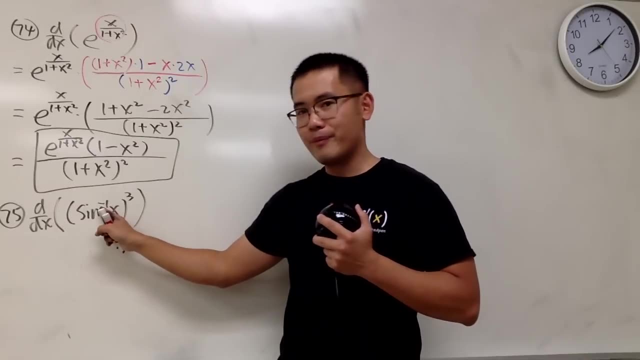 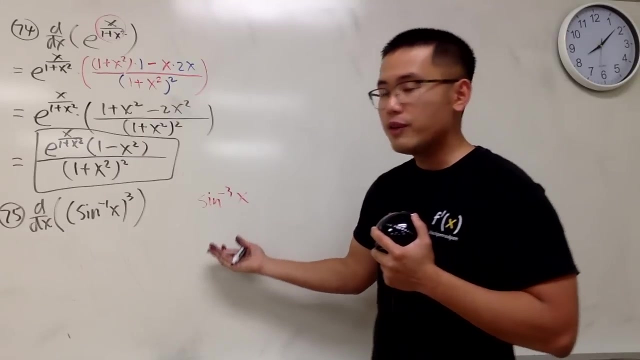 With inverse sine of x inside and then raised to the third power. Please, please, please, do not put down sine with a negative 3 power right here. Okay, If you ever write sine negative 3 power like this- I don't know if you are saying this or are you trying to say sine x to the negative 3.. 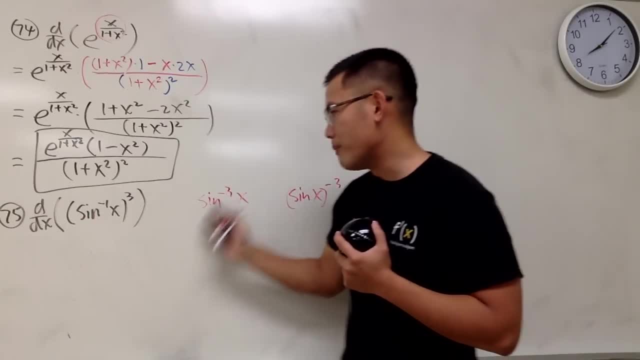 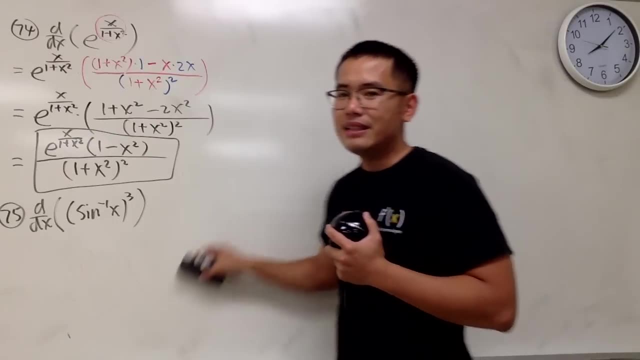 We don't know. Don't do this. This is just so bad. I know this is the The one that's the worst, But just don't do it like that, And for the regular calculus course and whatsoever, when you have this. 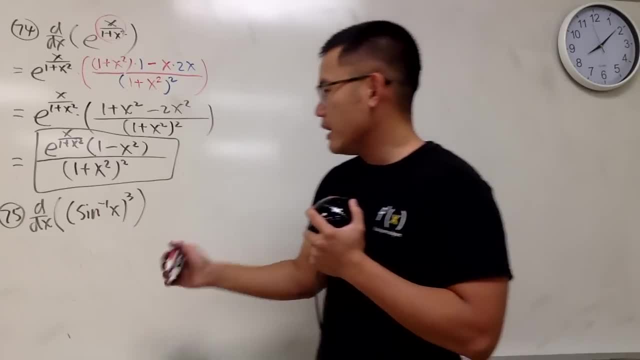 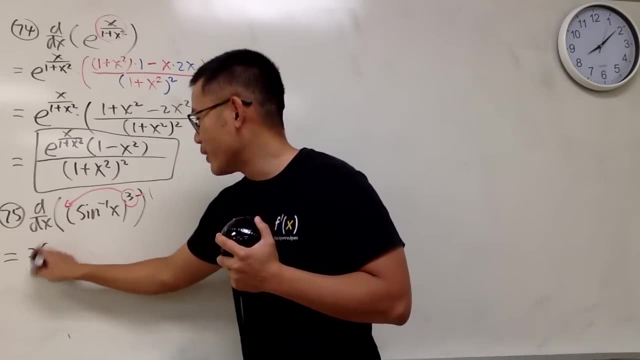 negative 1 right here means the arc sine. Okay, Anyway, here we go. Power rule: first Bring that to the front- Minus 1.. So we have 3, parentheses: inverse sine of x raised to the positive 2.. 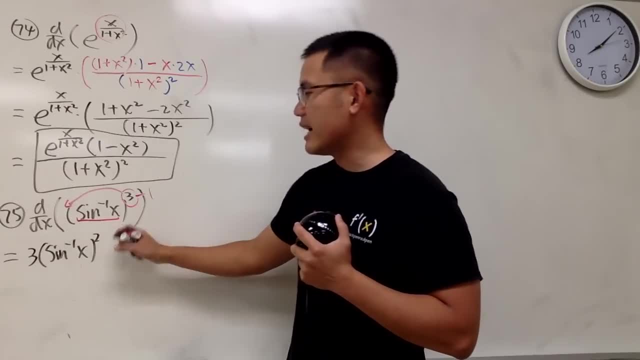 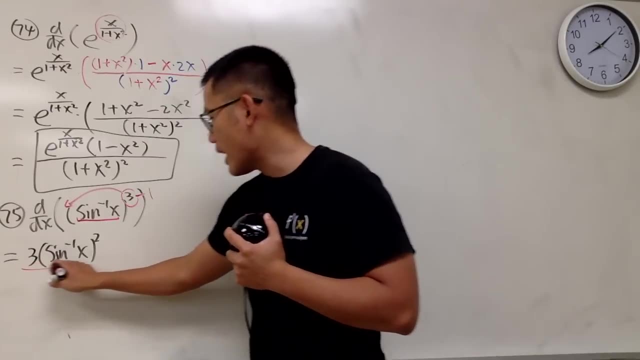 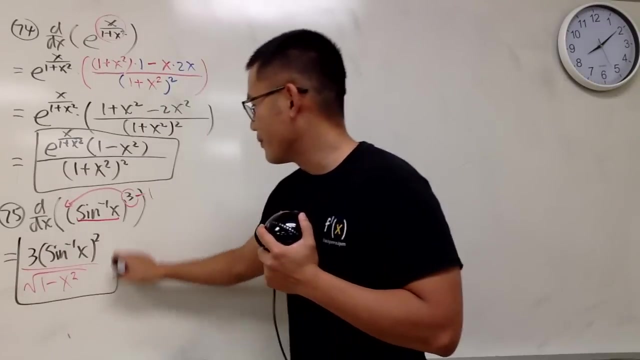 Okay, And then multiply by the derivative inside. The derivative of the inverse sine is 1 over square root of 1 minus x squared. I will just put that right here, Just like that. Okay, So with that we are done. 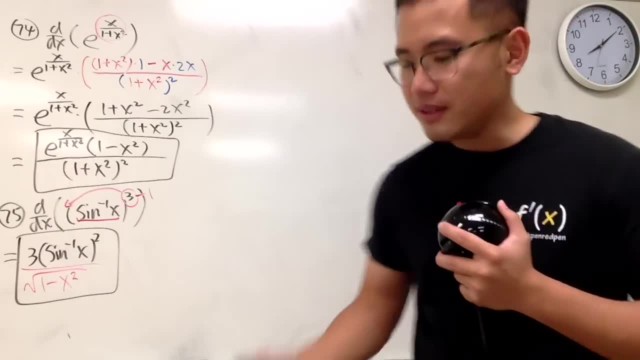 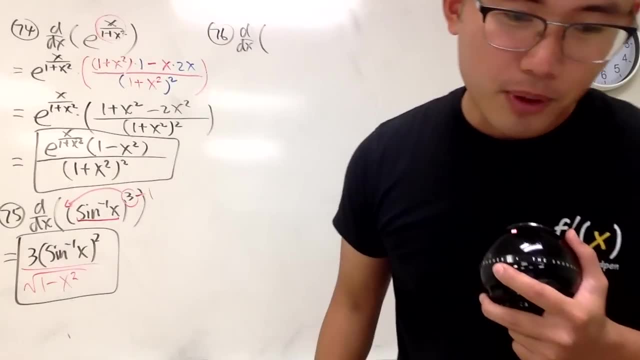 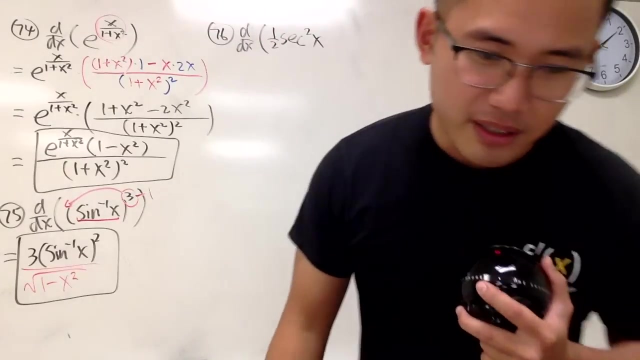 Number 76.. Number 76.. d dx. I should start training for my marathon too. by the way, I haven't started running. I have been going to the gym but haven't been running yet, So my cardio needs to work. 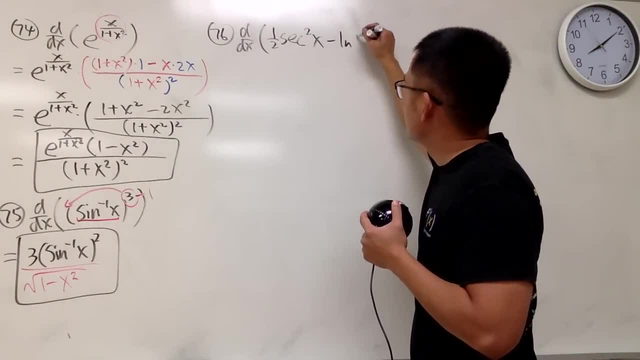 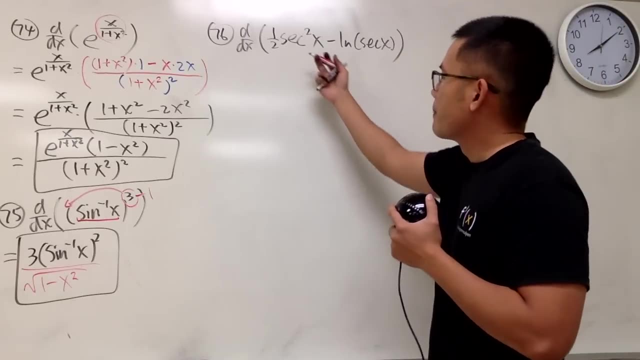 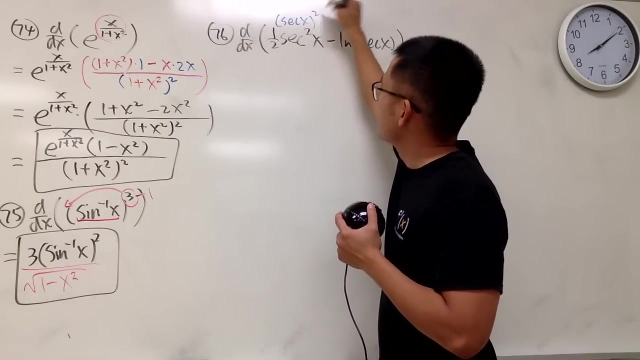 Okay, And this minus natural log of parentheses, secant x Like that Very good. So again, whenever you have the power right here, it's a good idea to write it as secant x and then raise that to the second power. 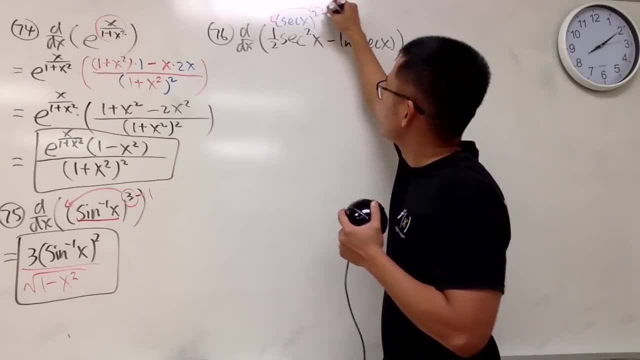 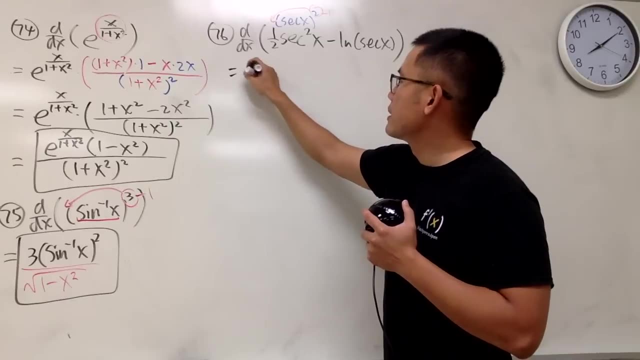 Anyway, here we go. Bring the power to the front Minus 1.. 2 times 1 half is just 1.. So you have just this secant, Okay, This secant x to the first power. So let me just emphasize. 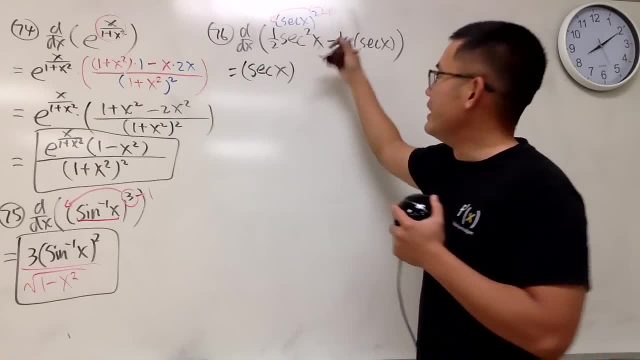 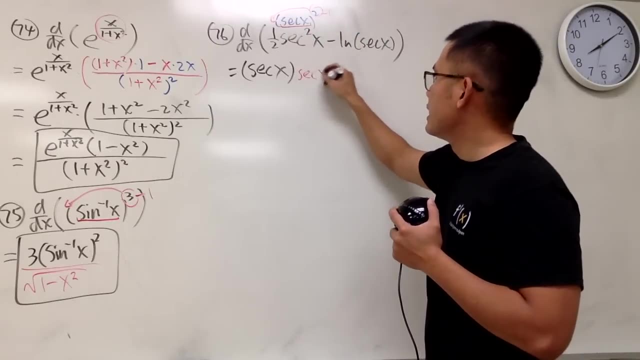 This right here is from here to the first power. And then we multiply by the derivative of the inside. The derivative of secant x is secant x times tangent x. That's the first part. Then we work on this part. 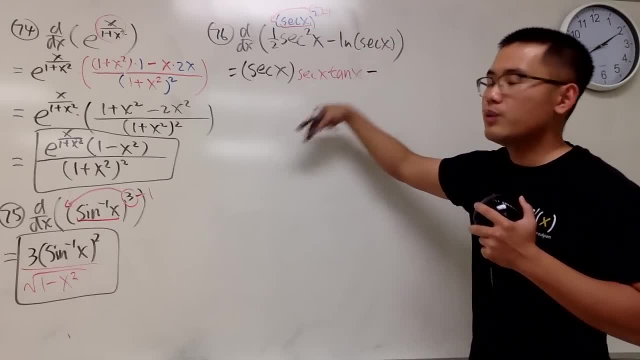 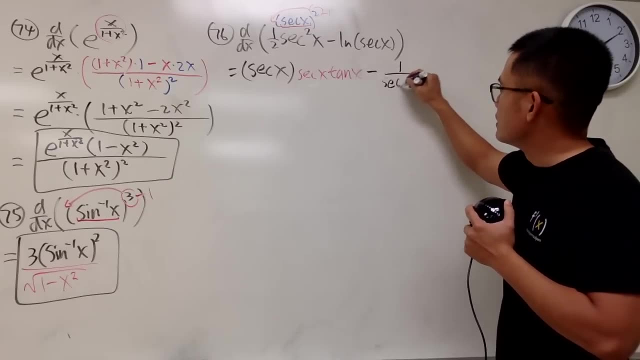 We minus. Okay, We did the derivative of this already. We minus this part. The derivative of natural log of something is just 1 over of the inside, which is secant, x. And again we multiply by the derivative of the inside. 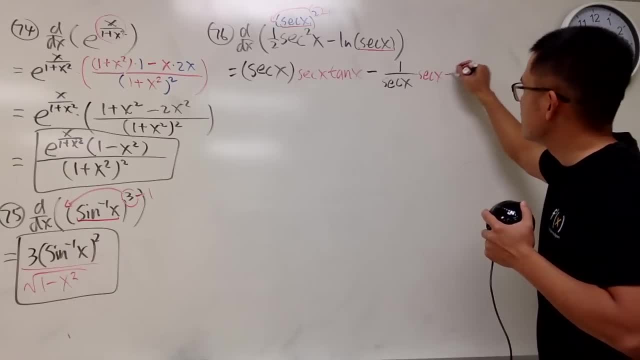 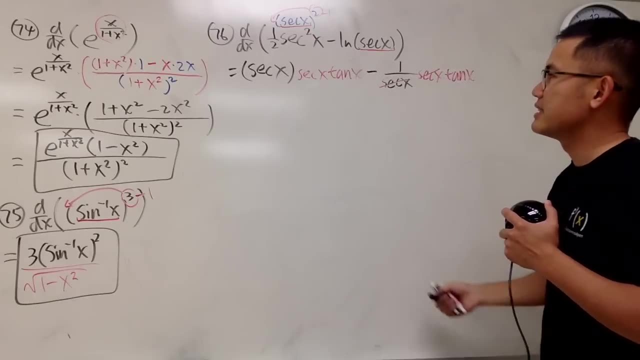 The derivative of secant x is secant x times tangent x. Well, well, What's happening Here? we can cancel the secant x, That's nice. And perhaps right here we can do the following: This right here is, of course, secant x. 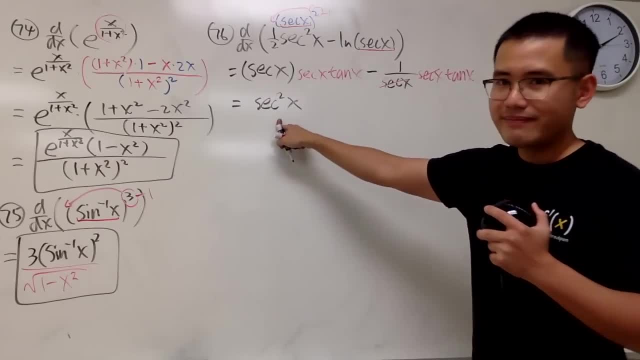 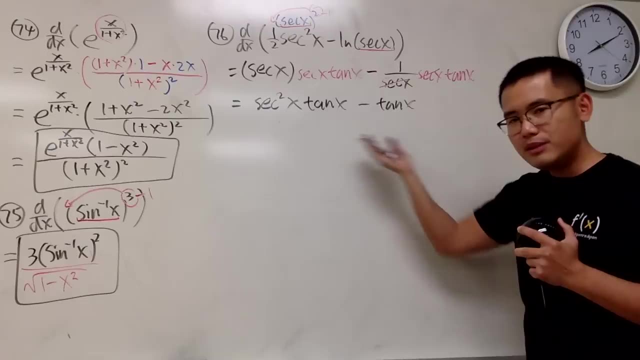 And in the next setting is of course, secant x And we have the tangent x And the minus. This right here is just tangent x. So that's good And you see, both of them have tangent x. 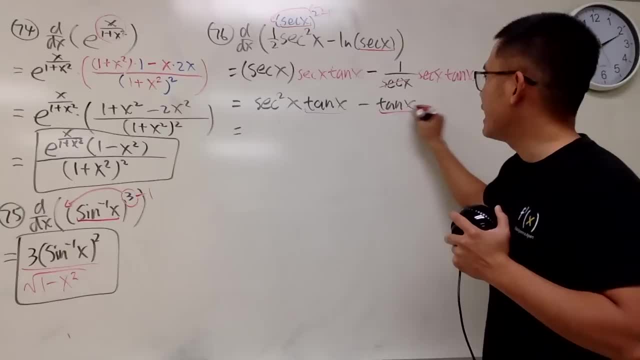 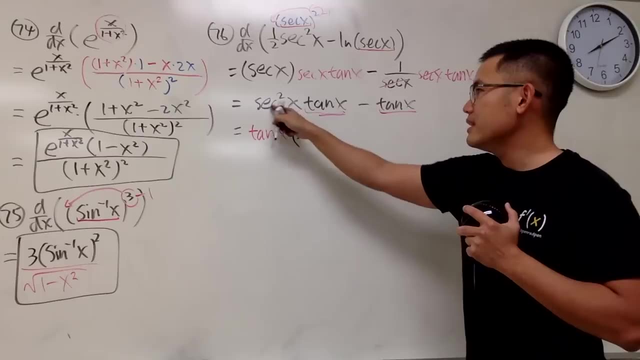 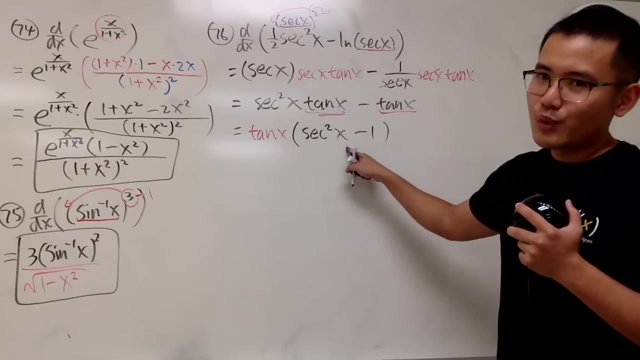 Let's factor it out. So again this and that we are going to factor it out, So that's in the front right here, And then we will end up with secant x and then minus 1.. What's secant squared x minus 1? This right here is nicely equal to tangent. 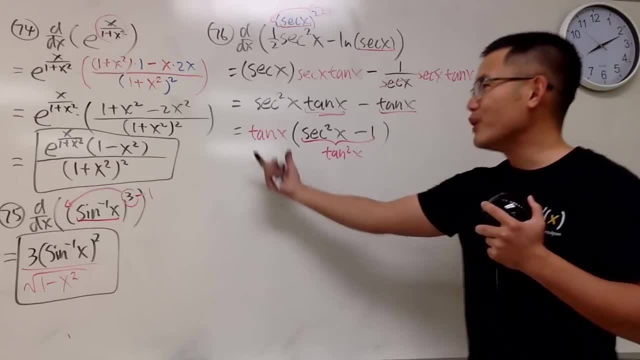 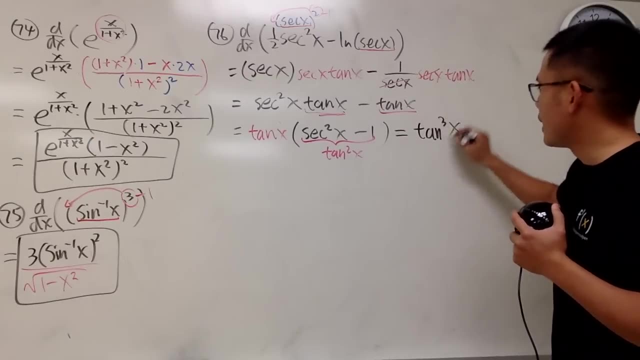 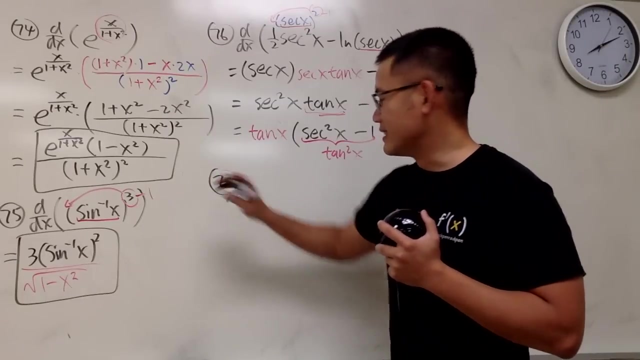 squared x. So all in all, we have tangent to the first power times, tangent to the second power, so we will end up with tangent to the third power, x. Very, very nice, Very, very nice. As I said, I've set up a lot of these questions so that they 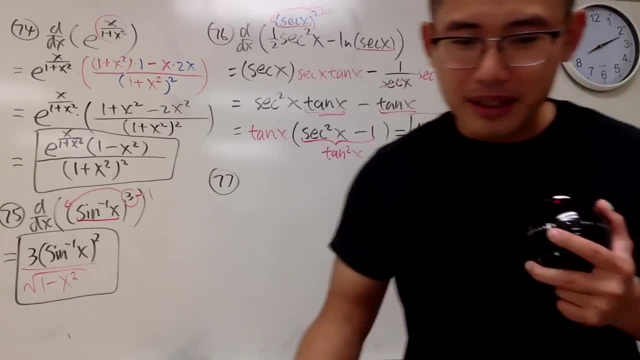 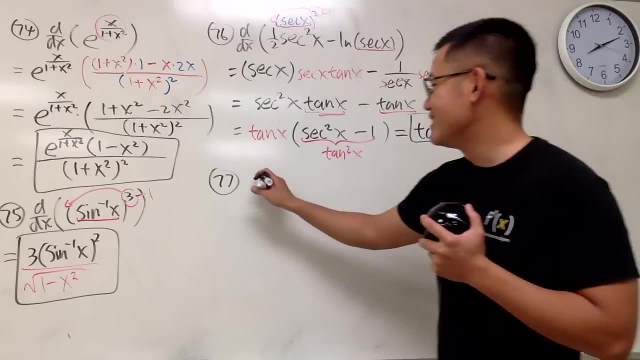 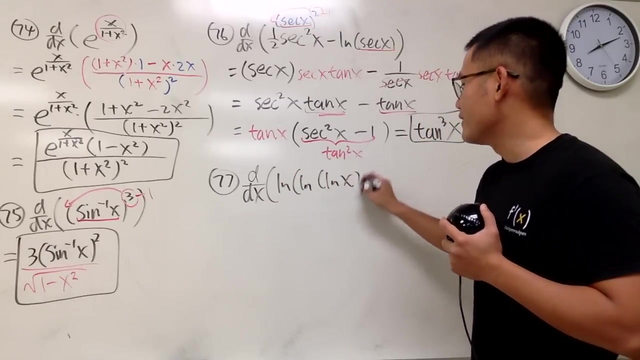 have some really nice simplifications. Otherwise the derivatives: they aren't so much fun. Next one: this is a fun one, It's actually a rather famous one: Natural log of natural log of natural log of x. It's just a lot. 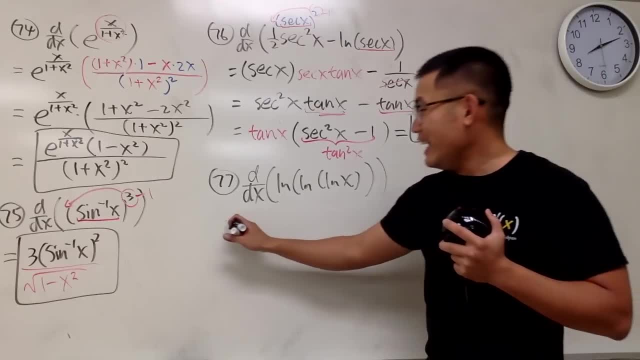 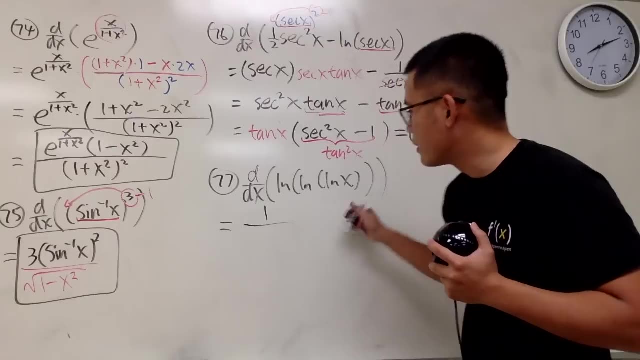 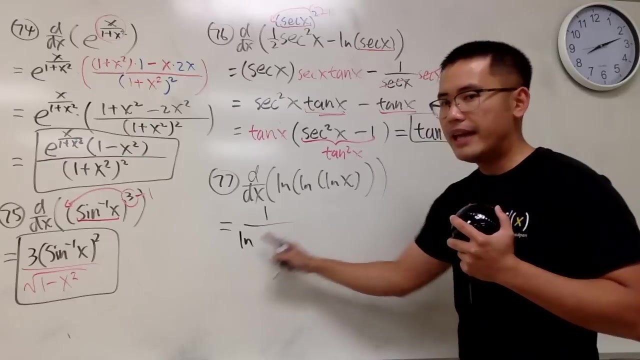 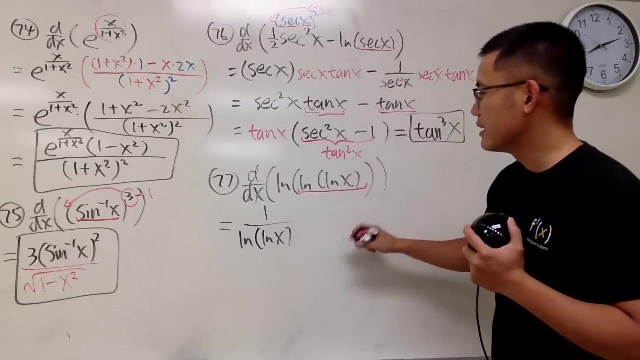 of people will do this kind of derivative equation. Anyway, here we go. First natural log tells you you have to put down 1 over this. This is the inside. You put it down in the denominator, which is natural log, and then natural log of x, Right, And then the channel says: multiply by the derivative of the inside. 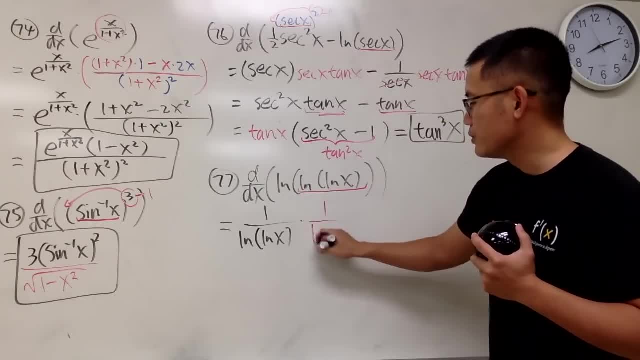 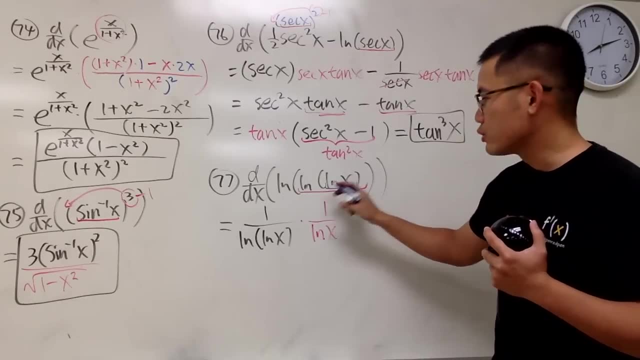 This natural log says you have to do 1 over the inside, which is natural log of x. And then the channel says you have to multiply by the derivative of. this Derivative here of natural log of x tells you you have to put the x in the denominator That was in. 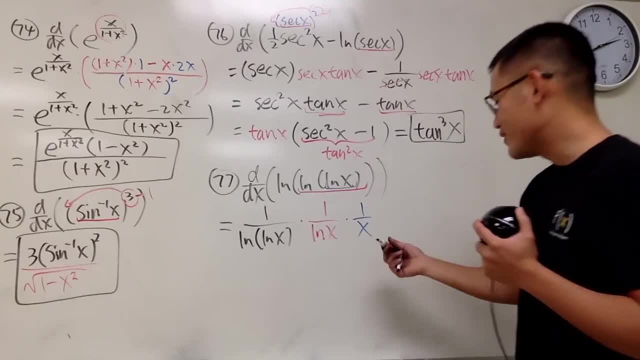 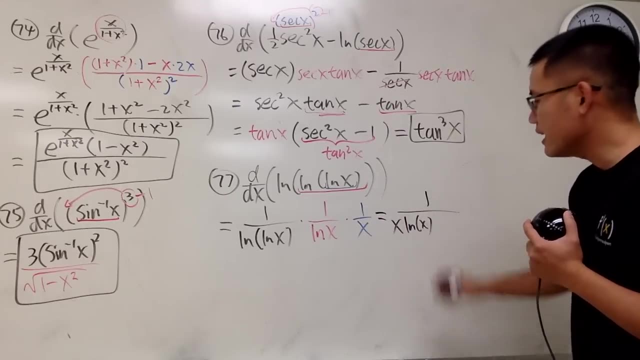 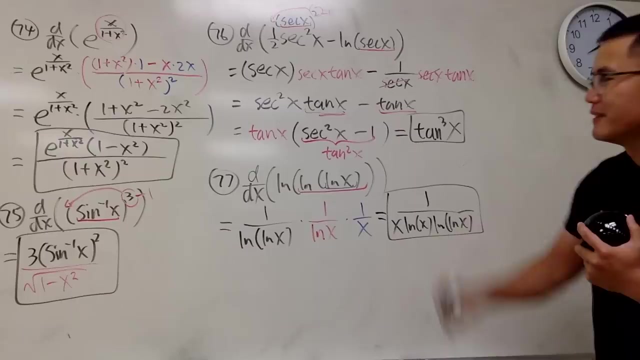 the denominator. So that's pretty much it. In the end. we just write things down nicely: 1 over this x goes first, and then natural log of just x goes next And lastly natural log of natural log of x, Like that. So this is it. Dr Payam also did a video on this. 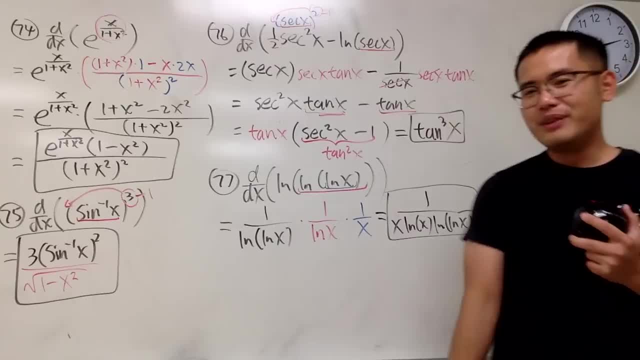 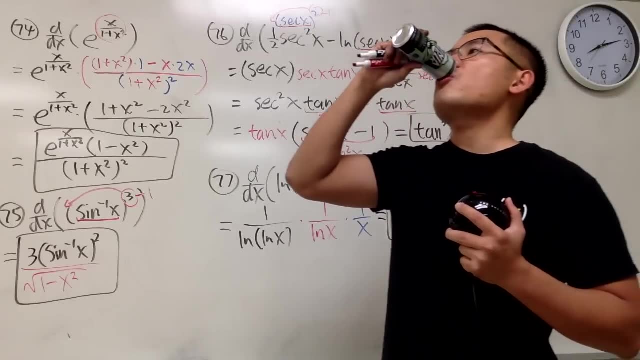 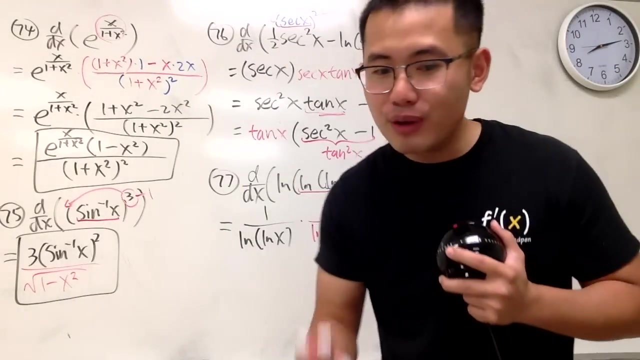 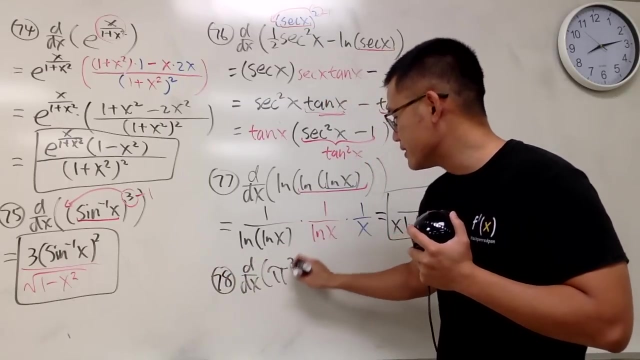 guy. And this is the beginning of the Chengdu. So if you guys haven't seen the video, go check that out. Ninja milk Number 78.. We are going to be differentiating pi to the third power. Please pause the video. 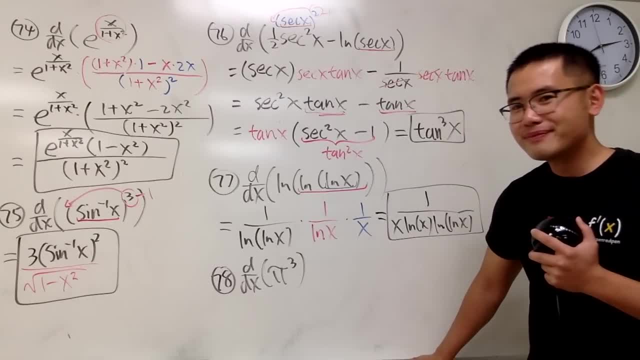 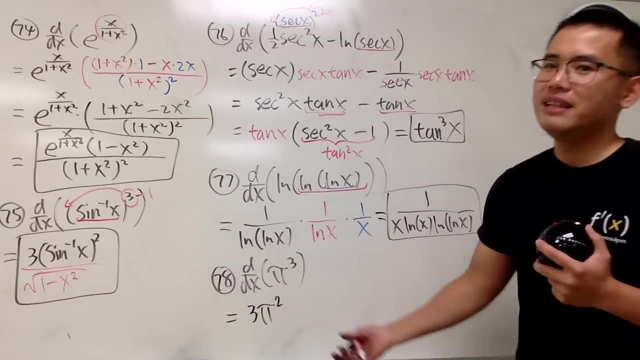 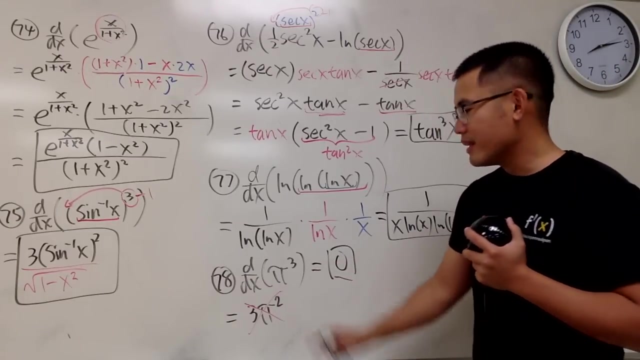 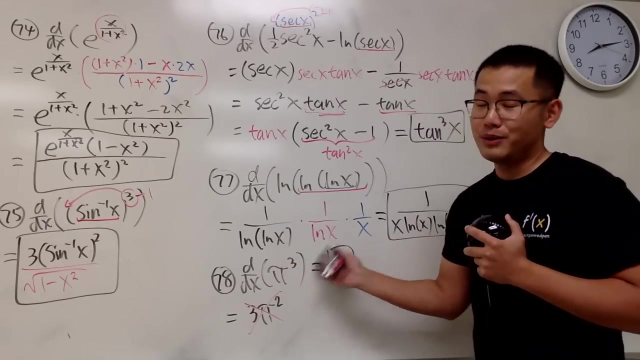 and give this a try first. Okay, Good, The answer is equal to 3 pi squared. Easy, right? No, The answer to this is just equal to 0.. Why? Pi is a constant. When you raise a constant to a third power, it's still a constant. When you do d dx of pi to a third power, you get: 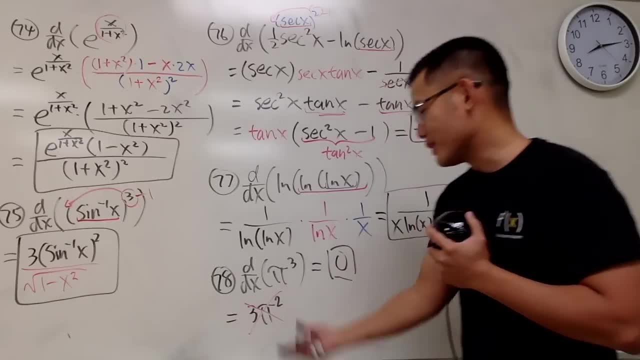 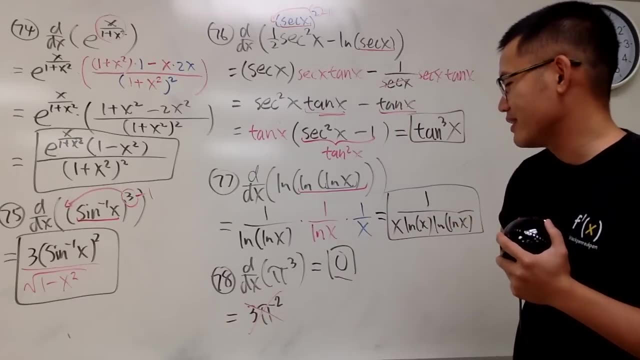 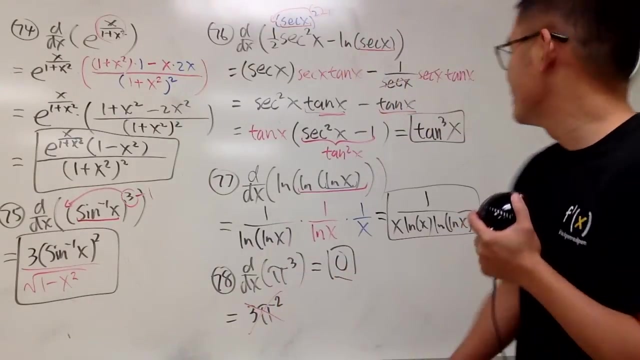 0 for it. That's it. If you do that, then you got tricked And usually this is a pretty tricky question for the AP. I'm not sure about AP test Your AP class. maybe Your AP teacher might do this to you. Yeah, I did this to my students too, So I'm not sure if you guys. 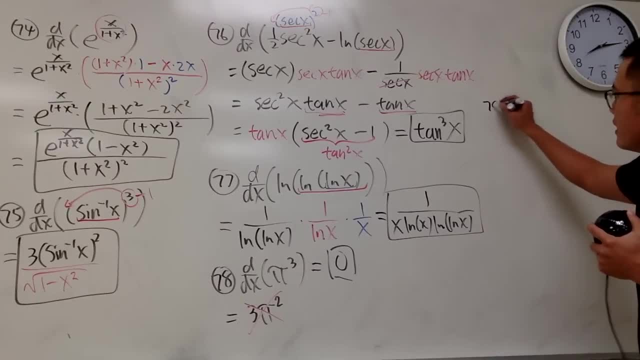 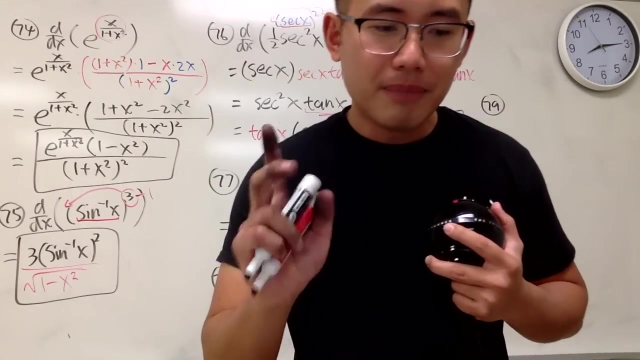 did this to me. I don't blame them. All right, Number 79.. I want to fit this right here, Okay. Oh my god, The ones, I'm scared, they are coming. The hyperbolic: they are not so bad, But the definition, they are coming. 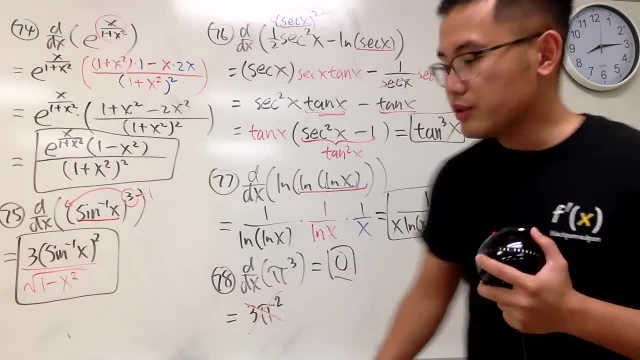 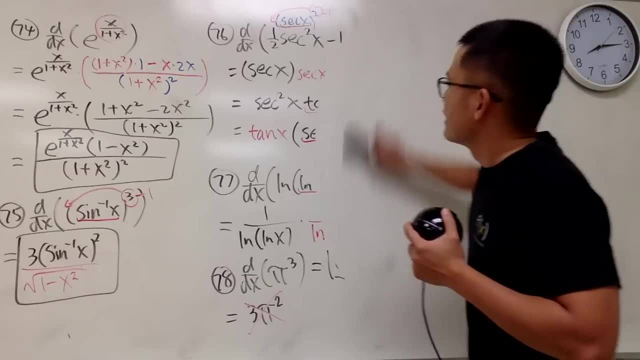 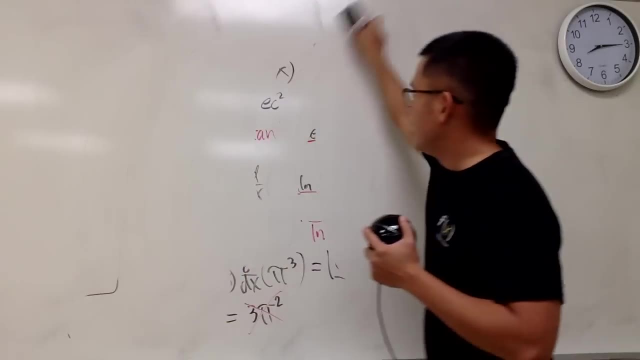 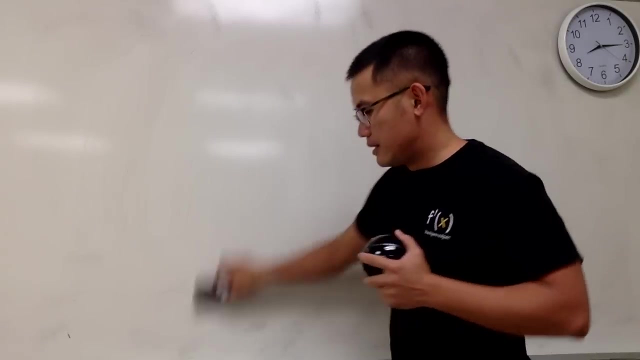 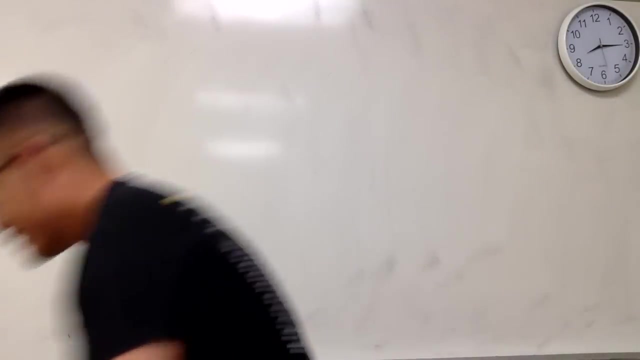 pretty soon, Actually, for this one, I'm going to erase: Okay, Okay, Okay, Okay, Okay, Okay, I'm going to erase, I'm going to erase. Oh, I will erase, I will erase. Okay, Restroom break. I'm going to just clean my head at least one time. Seriously, It's. 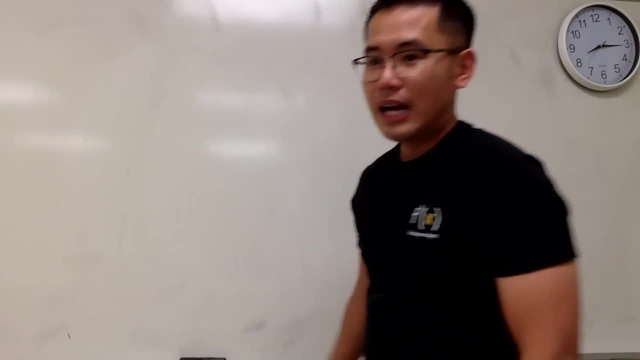 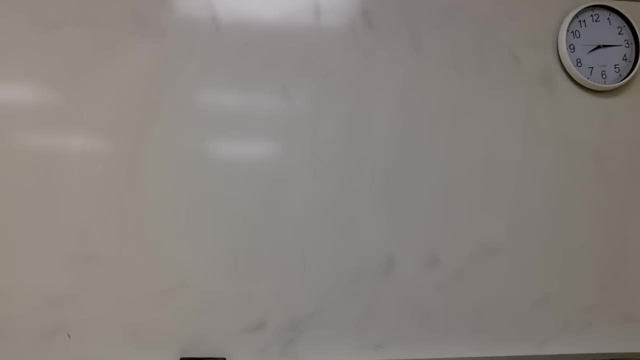 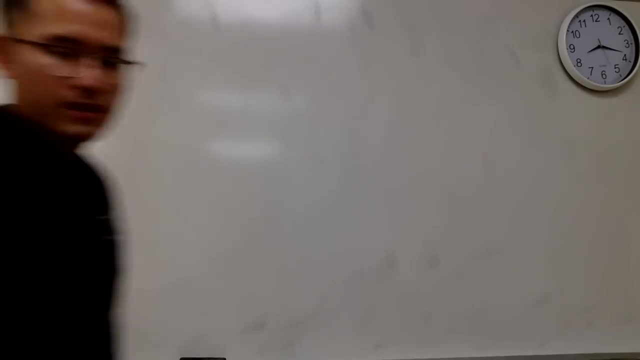 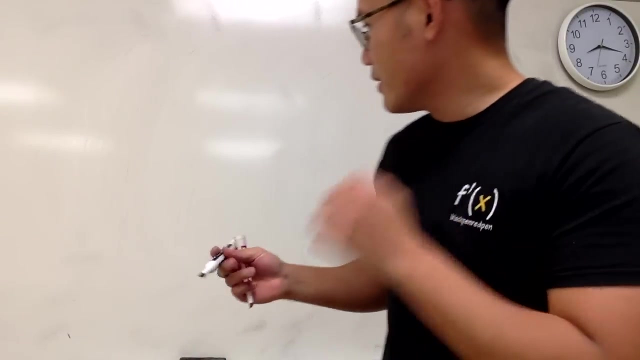 just bad, Just all the markers and all that stuff. So I will be back in a minute. Thank you, Feel much better. I personally prefer chalk. Ten years ago. 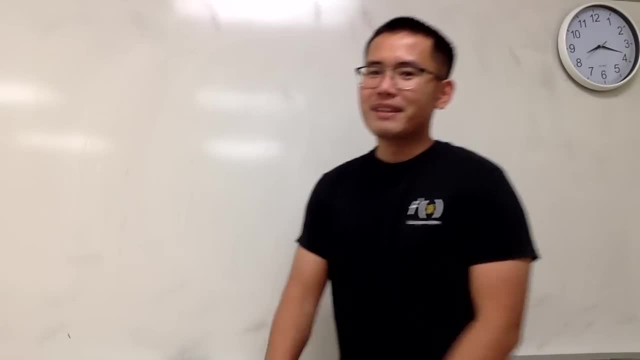 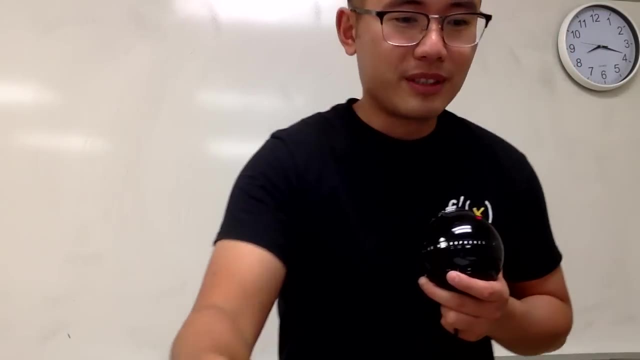 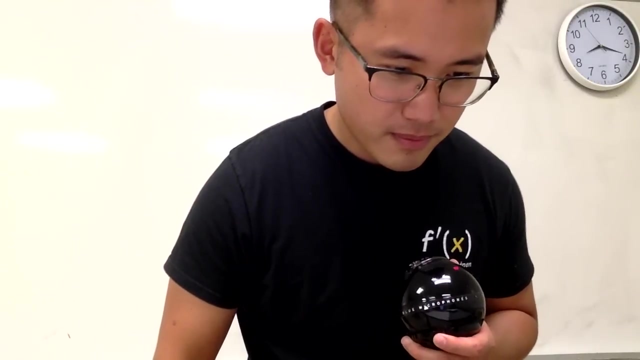 Nowadays, of course I use markers, But the downside is, markers is really dirty. It's dirtier than chalks. If you have a bad one. of course I mean like anyway, Okay, number 79.. 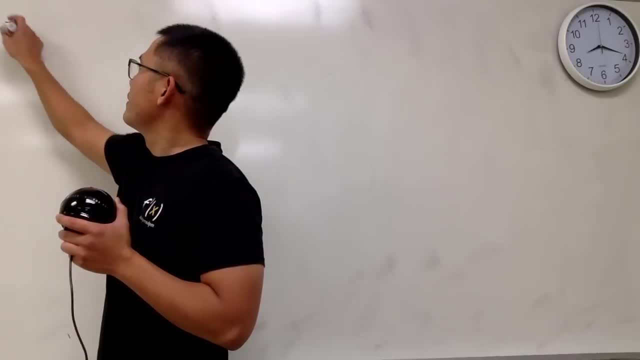 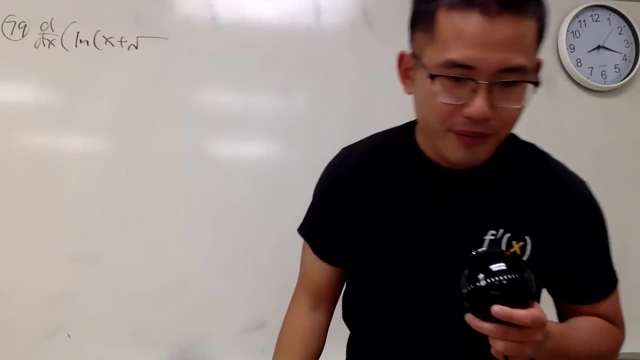 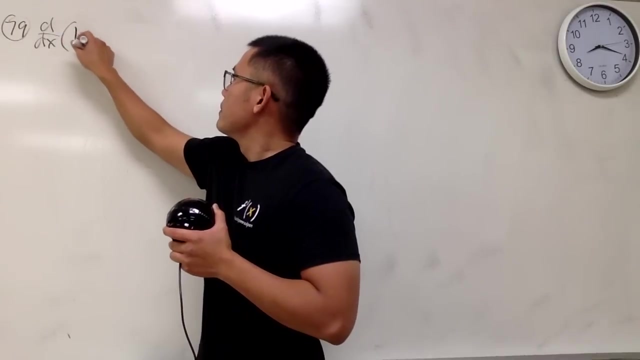 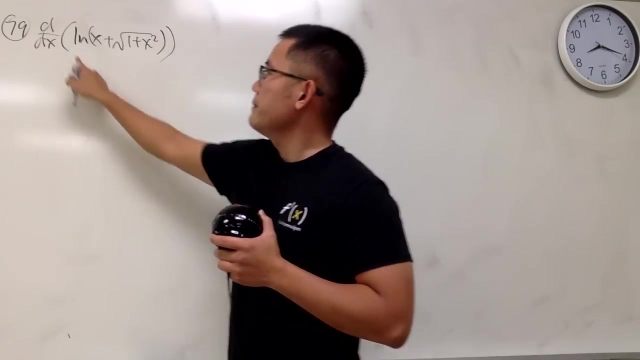 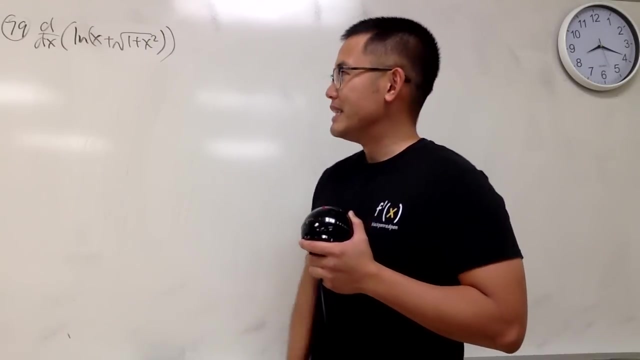 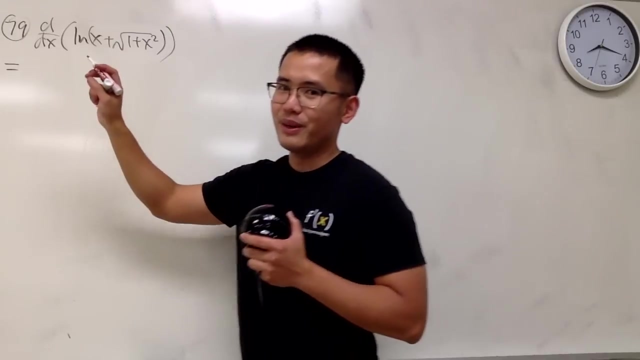 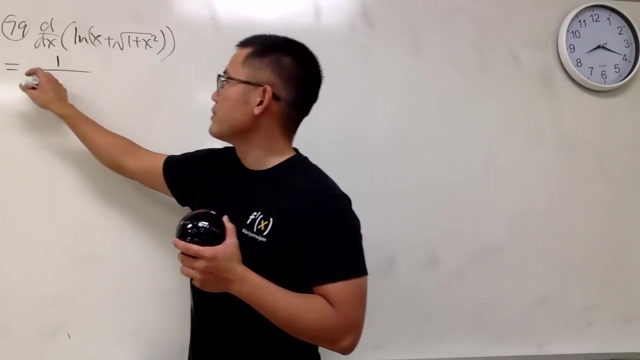 Here we go, Depreciating natural log of x plus square root of 1 plus x square. I'm going to write this down better for you guys. 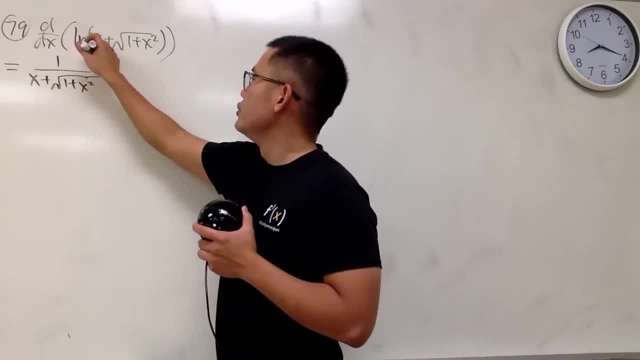 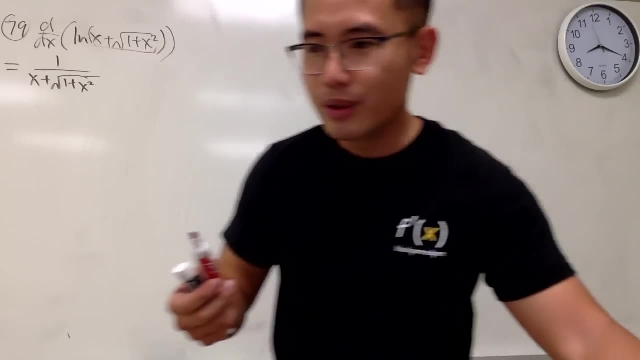 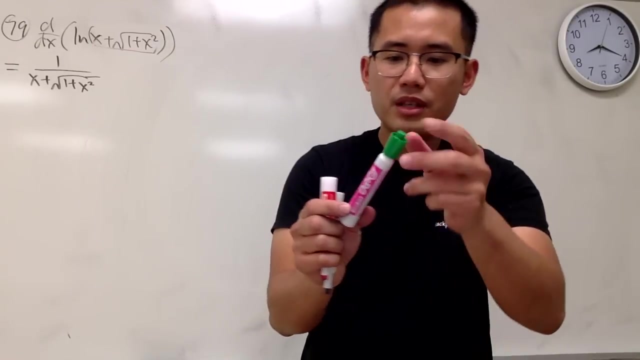 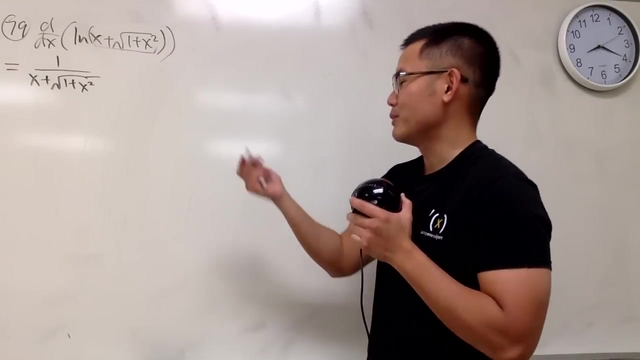 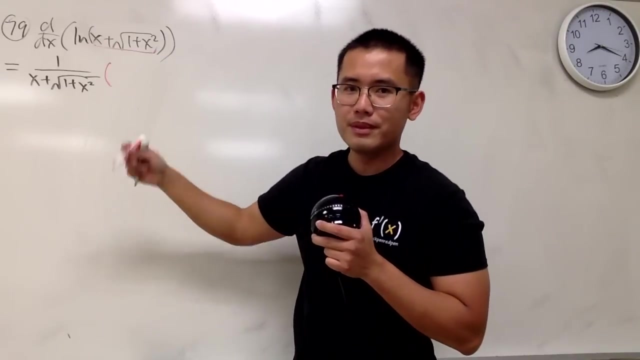 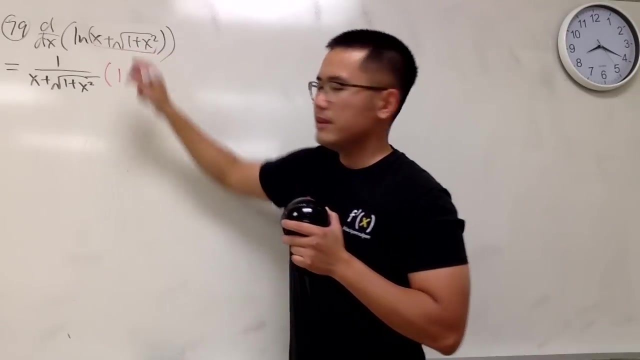 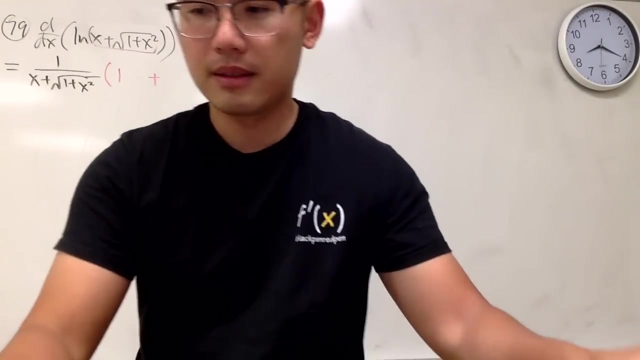 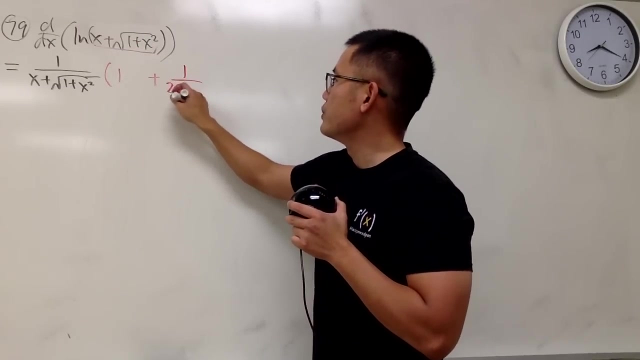 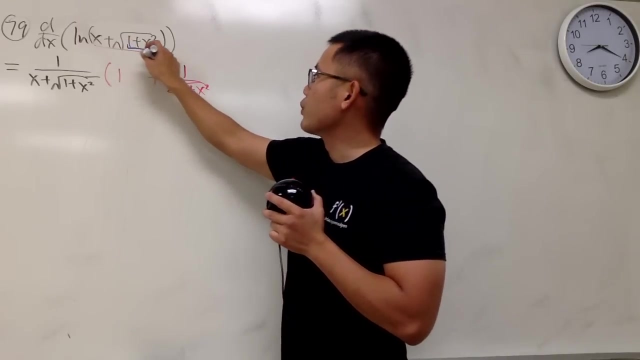 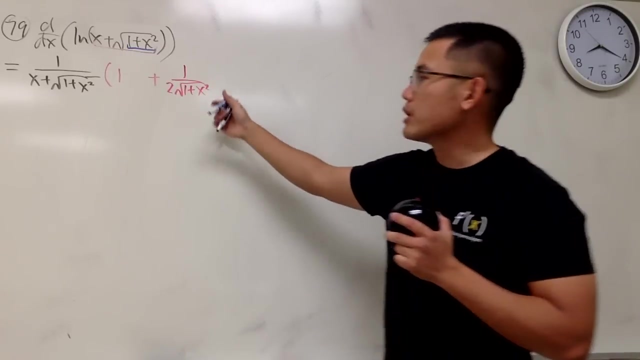 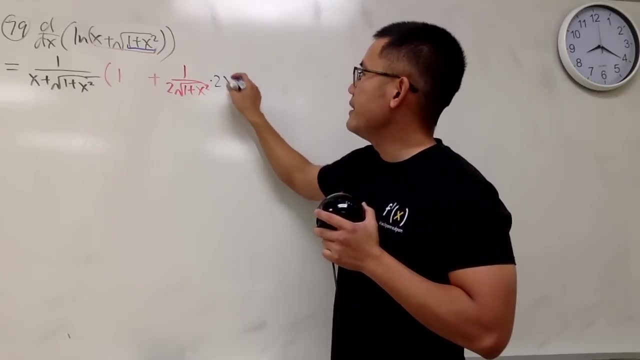 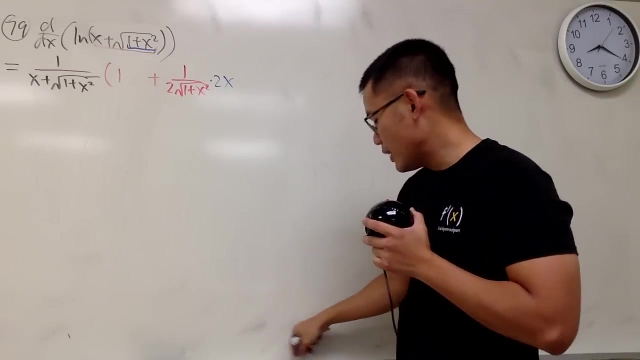 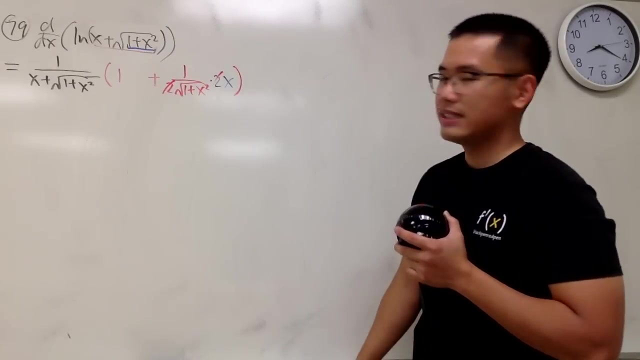 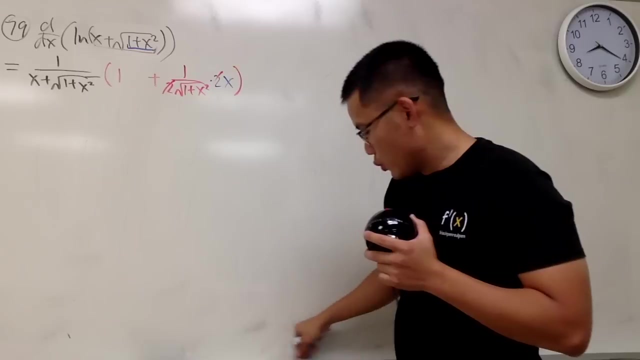 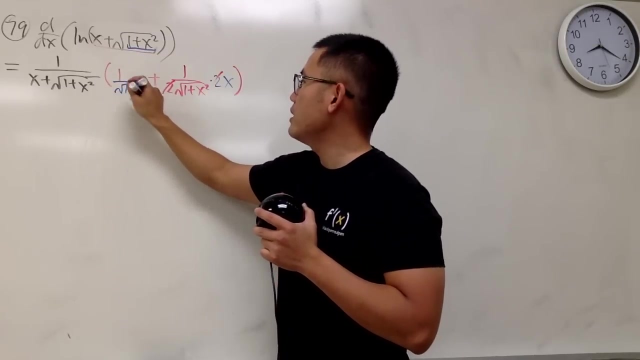 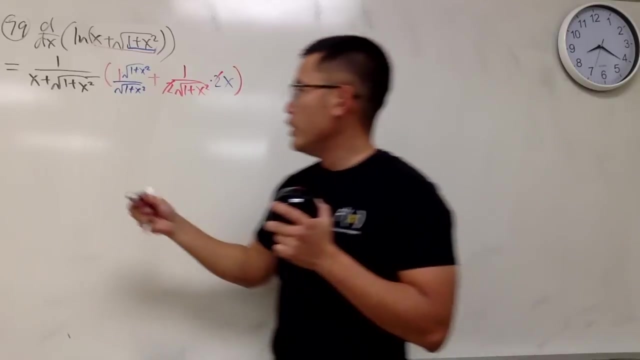 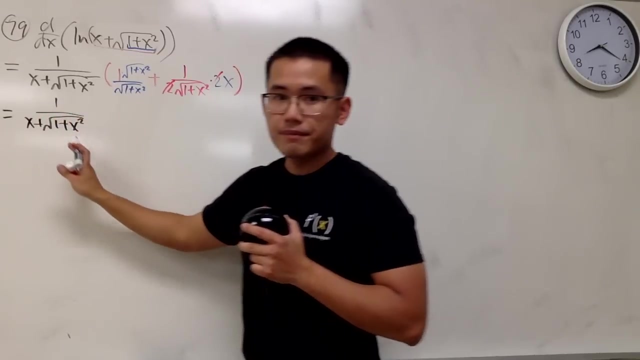 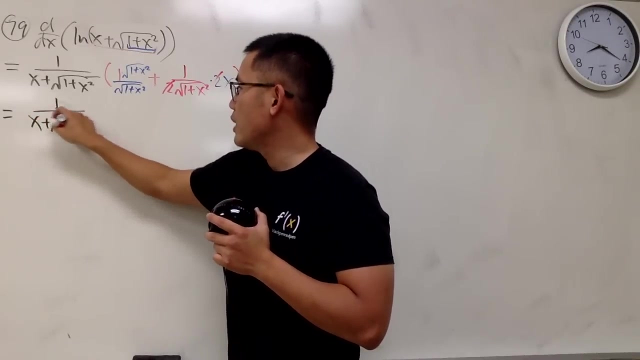 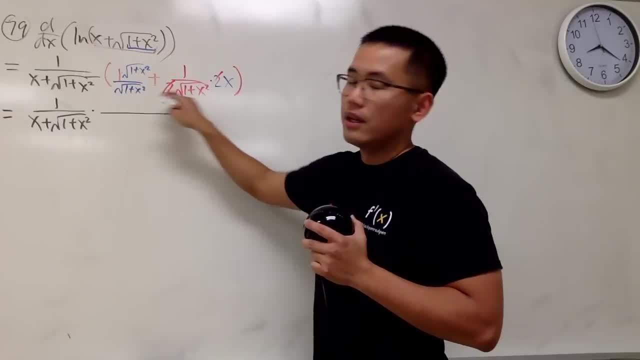 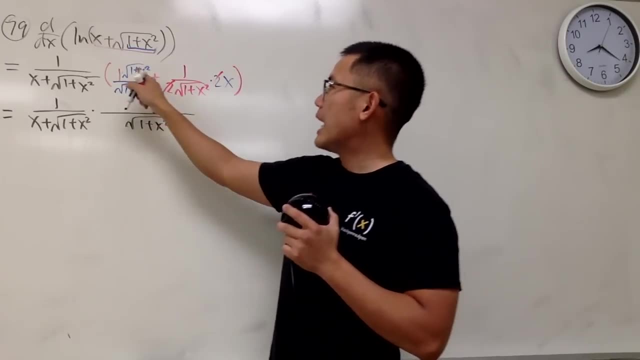 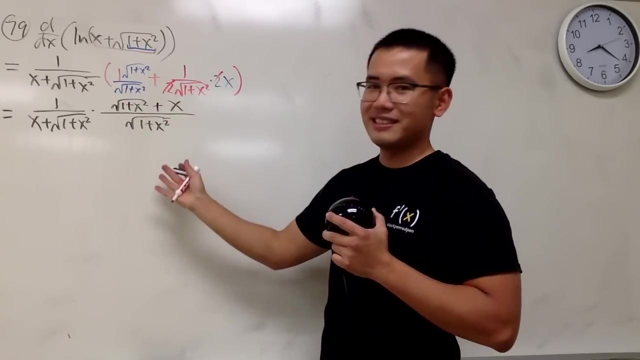 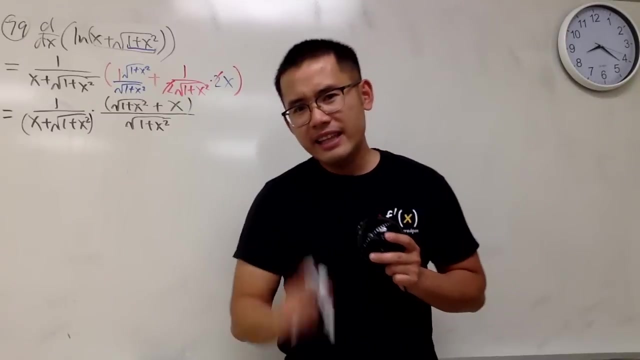 plus, this is just an x, right here, right? So of course you see that this part and this part, they should be in the parentheses, And the nice thing is that they are the same, even though the order. but you know. 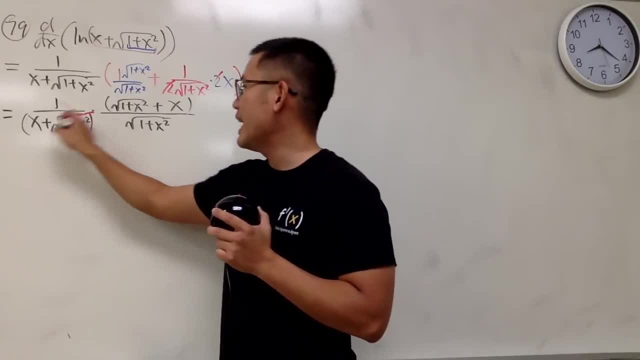 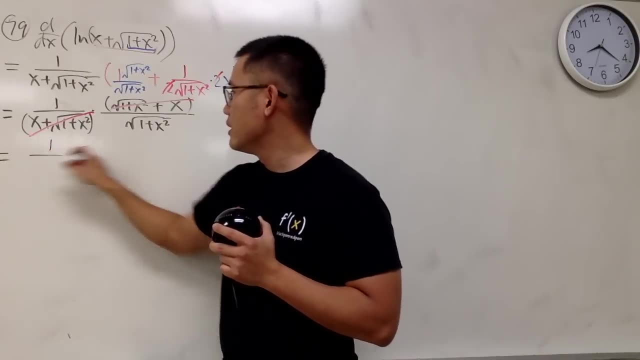 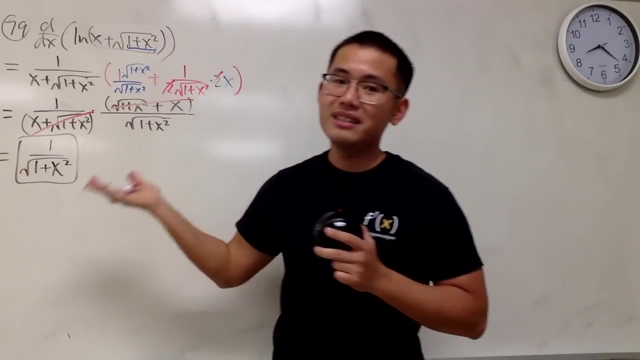 the order of addition does not matter. Therefore we can just cancel them out nicely, And in the end we end up with the third one over square root of one minus Nice. So one plus x squared. This is it. Very nice, isn't it? 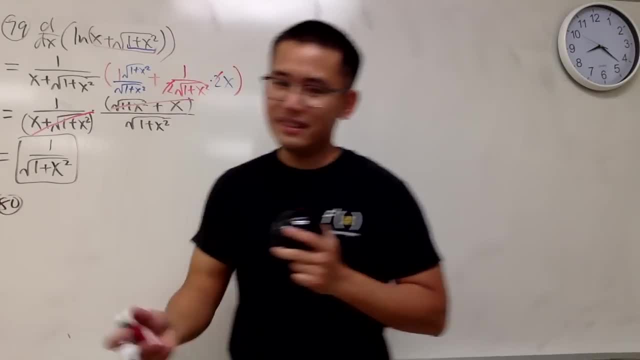 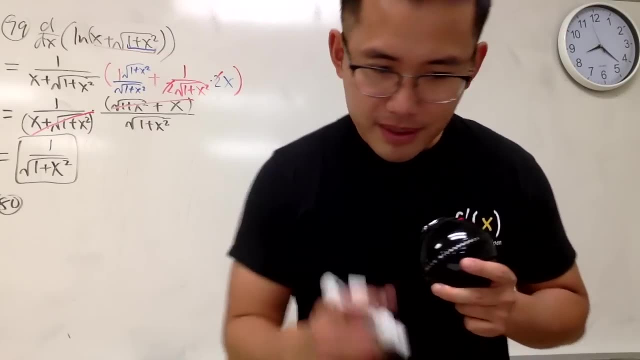 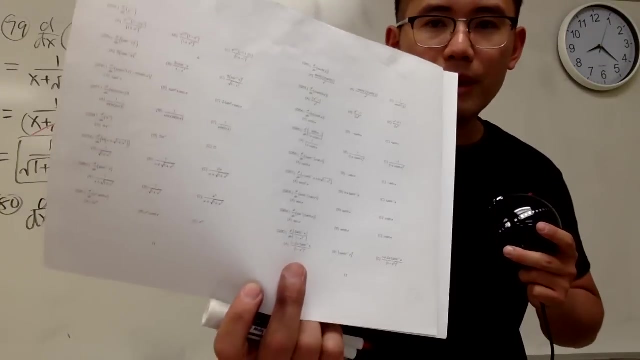 Maybe you see it, maybe you don't, but it's okay. Number 80, this is the time that I will explain it to you guys. Yes, this right here, From number 80 to number 90, it depends if you have covered the hyperbolic functions or not. 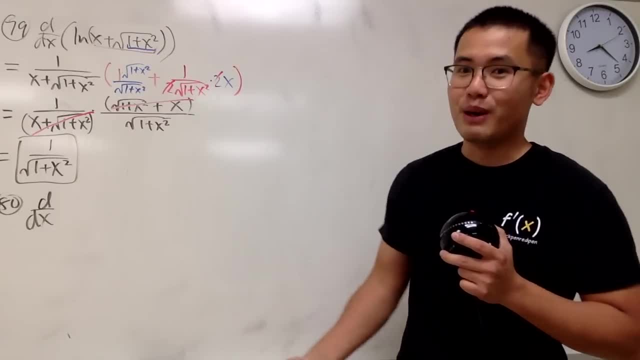 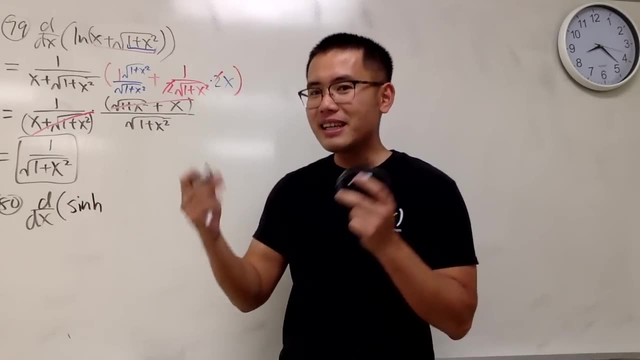 If you haven't, you can skip this part. If you have, you can watch this part, of course. Anyway, differentiating sine with an h next to it. This is not sine and h is a constant. This is called the hyperbolic sine, okay. 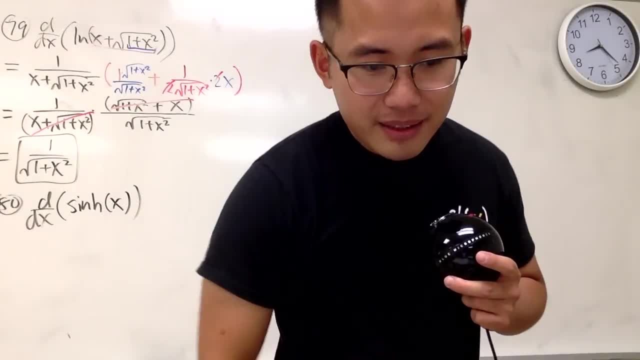 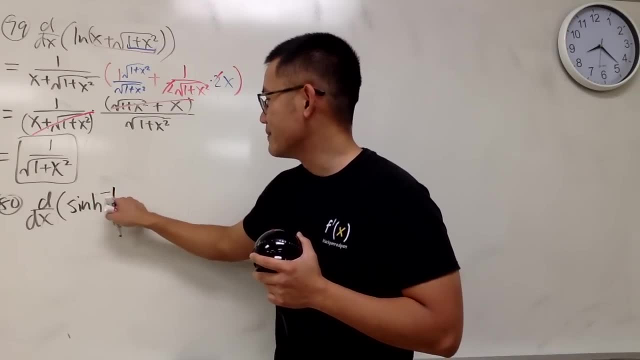 And the input is x. like this, And to make it more fun, let's talk about the inverse hyperbolic sine x. Okay, The inverse hyperbolic sine of x. And again, this right here is the input, this right here is the name. 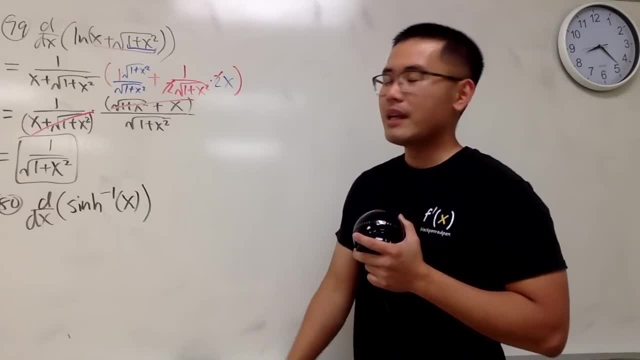 and we want the inverse of it. So it's like that, And I'll tell you guys more about what the inverse in all that stuff is. Well, the truth is this right here. the answer is that, Because you notice this right here. 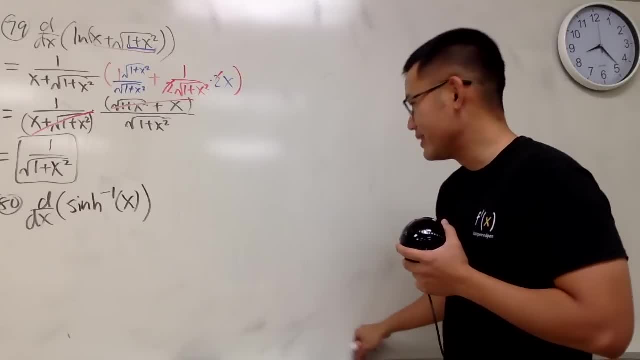 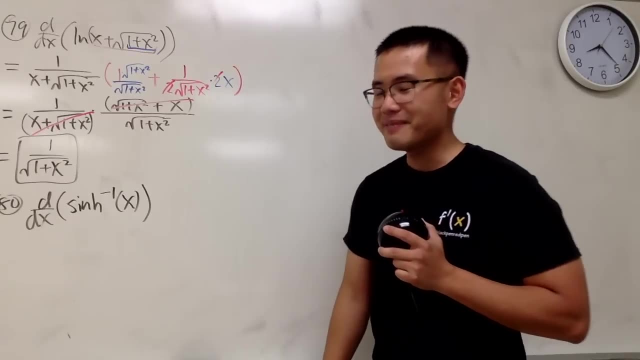 if you have the regular sign, sorry, let me just write it down right here. I'll do it and I'll write it down. Okay, I have no idea what this is. Let me just say it like that. Okay, Well, how can I figure this out? 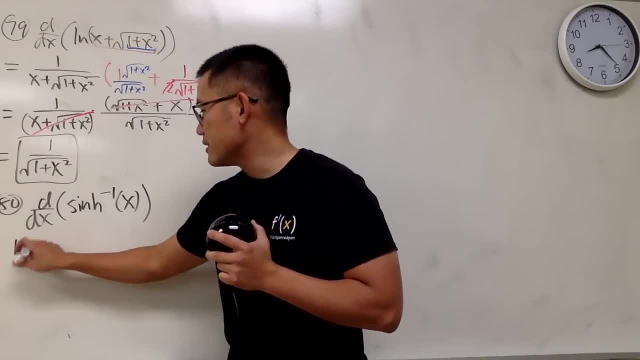 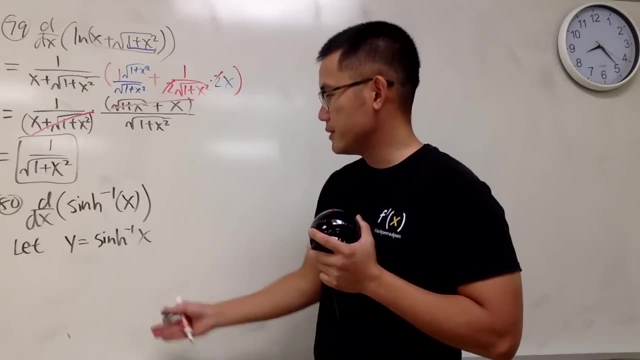 Two ways. First way, I can do the following. I can say that y equal to the inverse hyperbolic sine, x, like that. Okay, And the reason I want to do this is because hopefully we know the regular hyperbolic sine better. 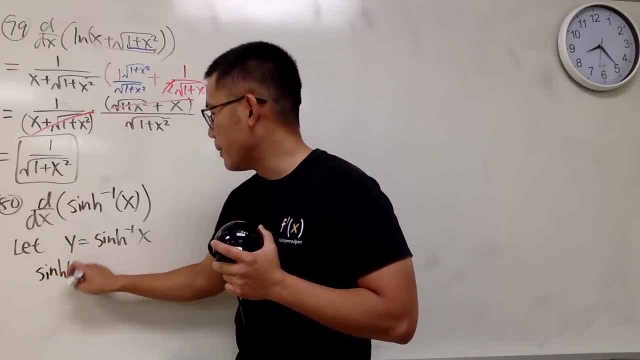 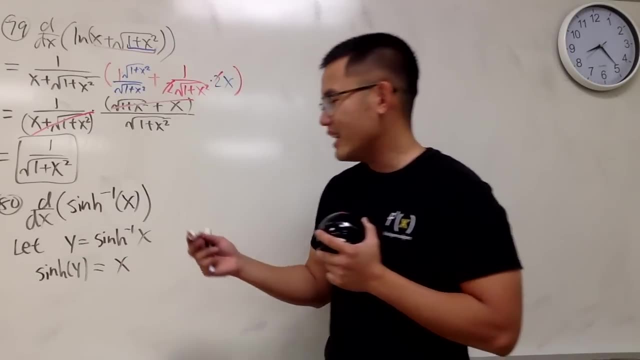 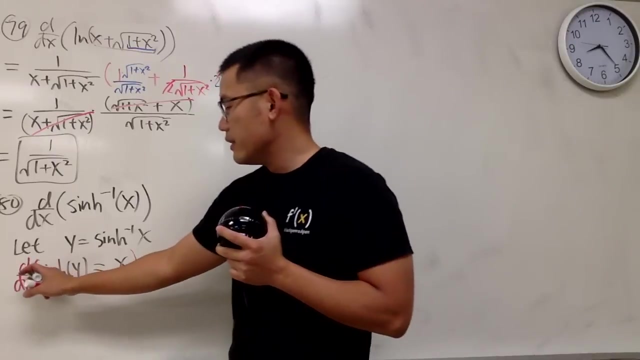 Well, if so, we can just take the regular hyperbolic sine function on both sides and we'll end up with this, And then we can do implicit differentiation. This is how we can figure out the derivative of inverse functions. Okay, when we do that, here is the deal. 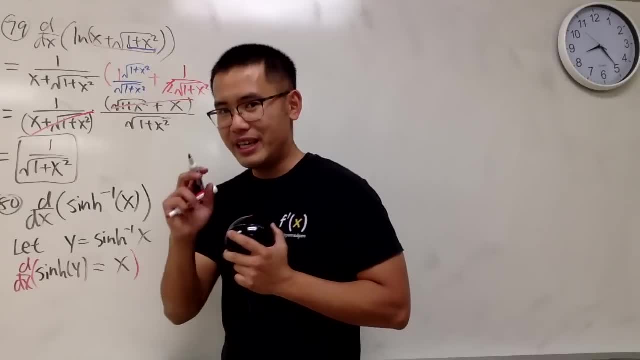 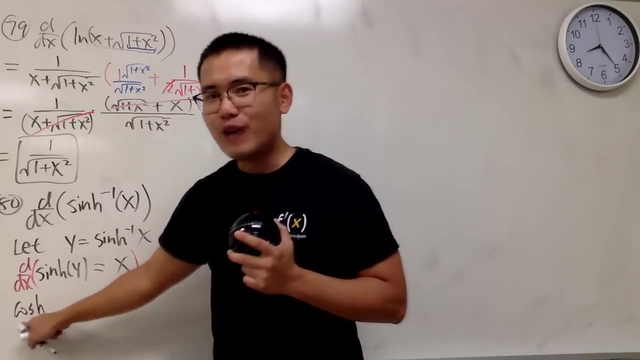 When we differentiate hyperbolic sine, we get hyperbolic cosine. So we have hyperbolic cosine, namely cosh. If you have a friend named Josh, you know that's not cool enough. Cosh is better And, by the way, this is sinh. 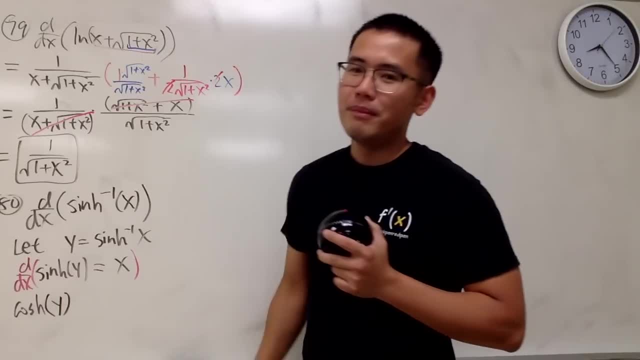 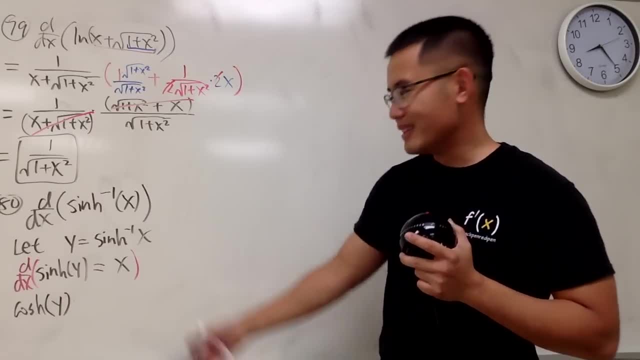 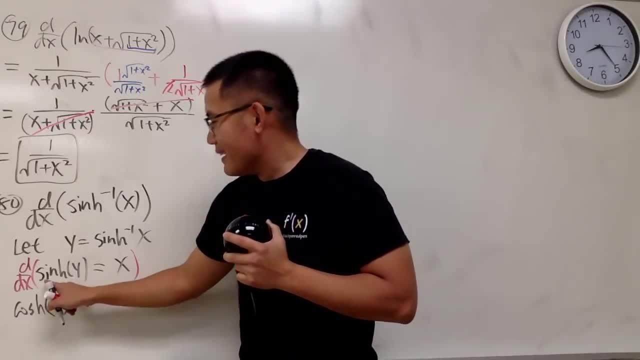 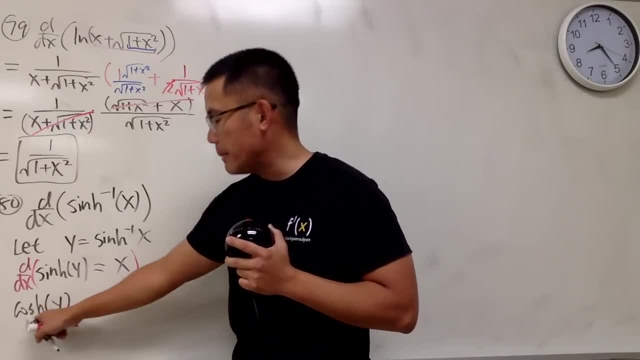 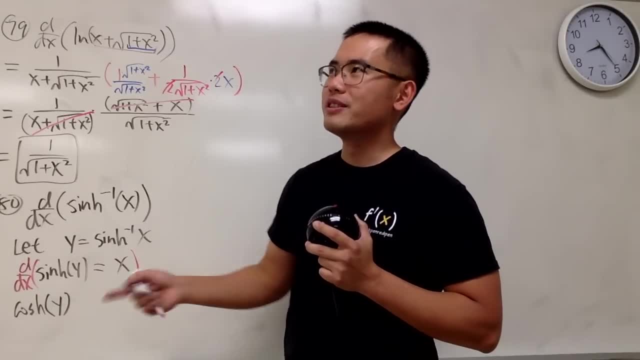 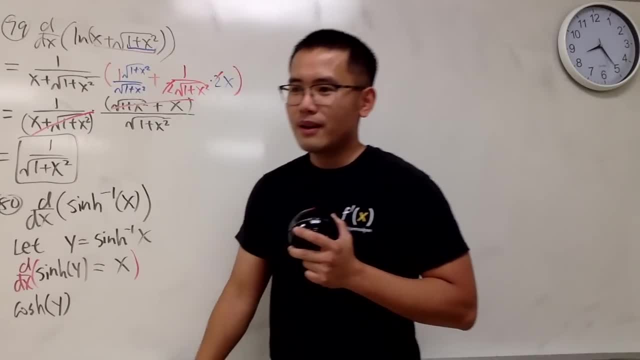 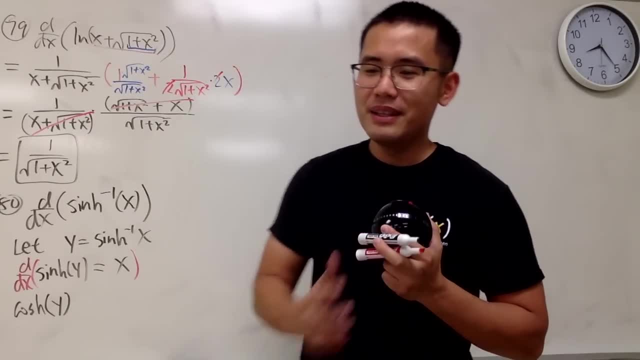 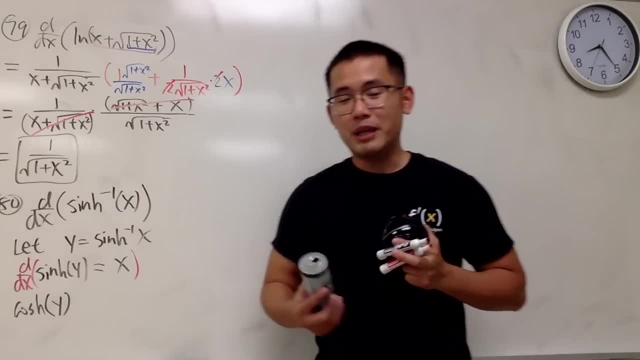 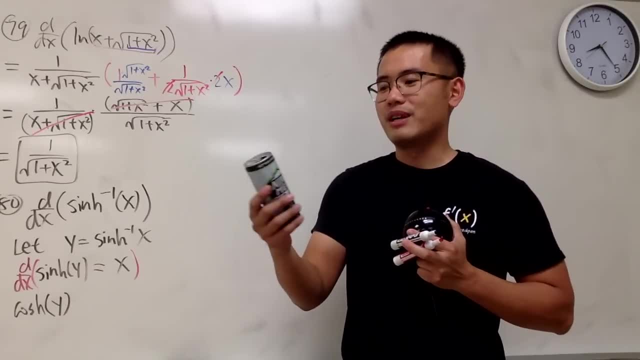 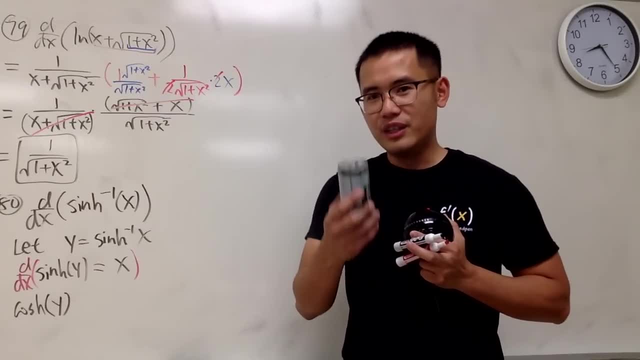 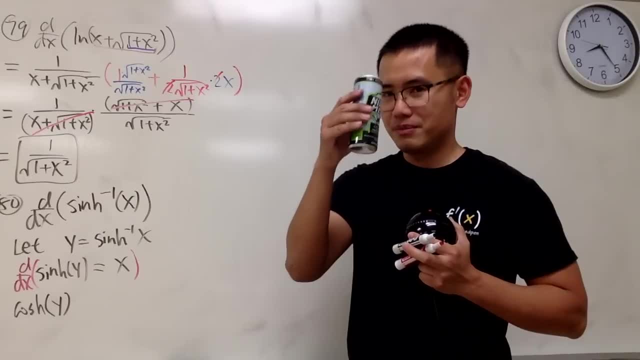 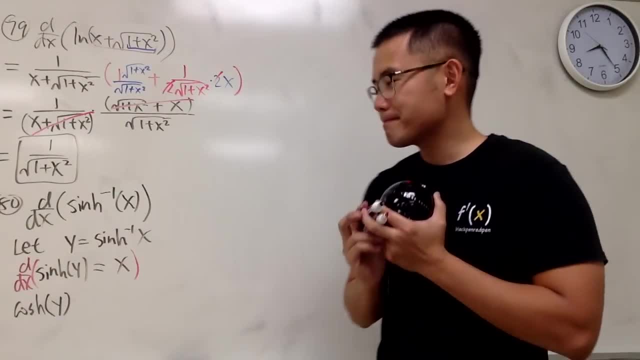 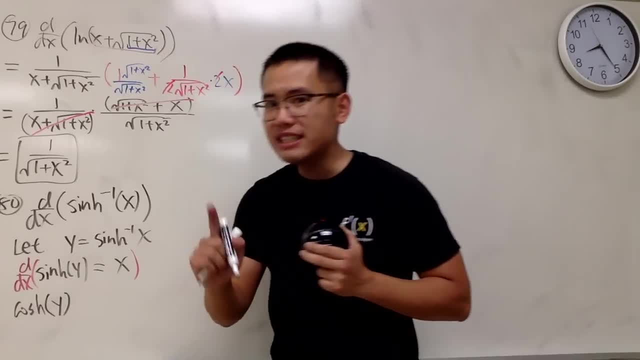 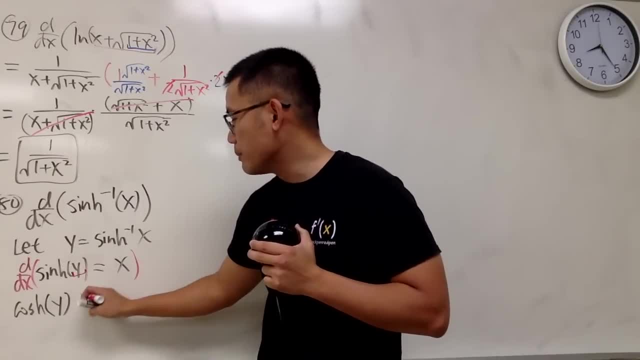 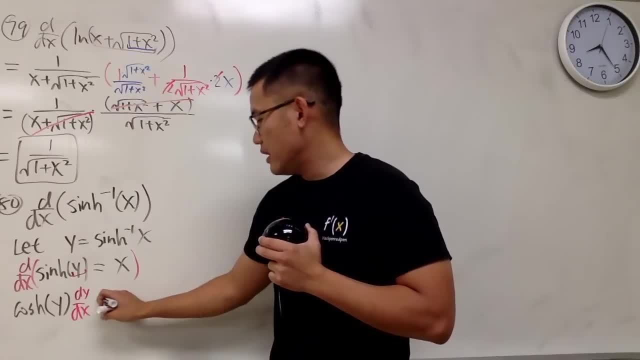 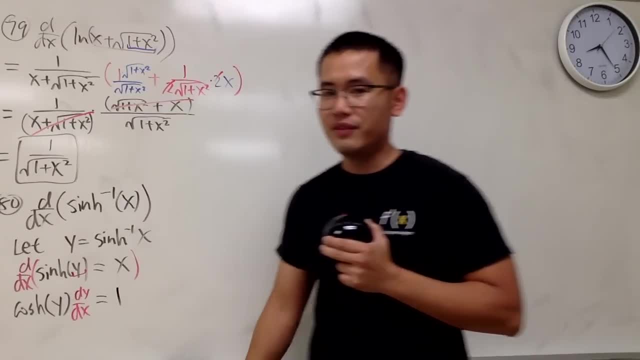 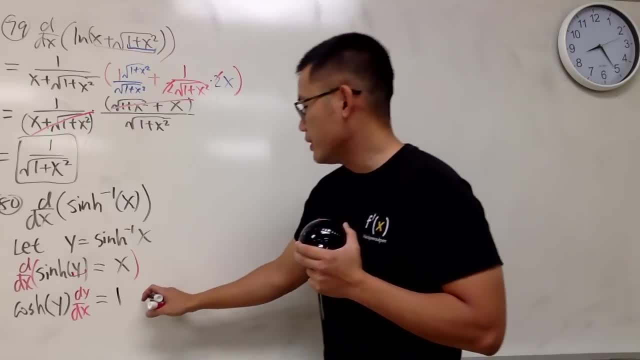 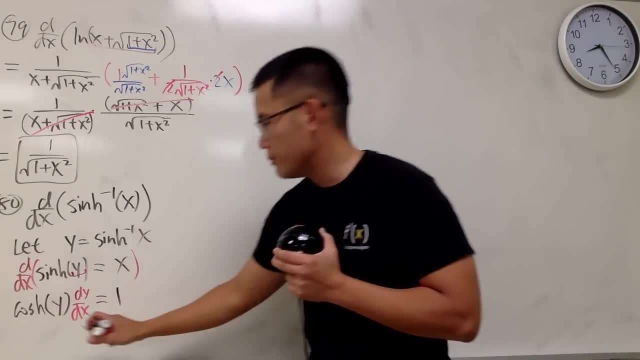 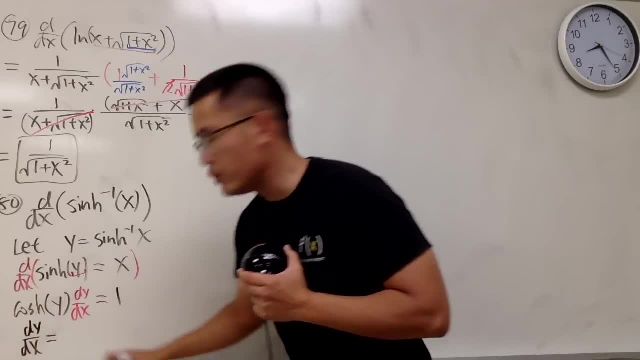 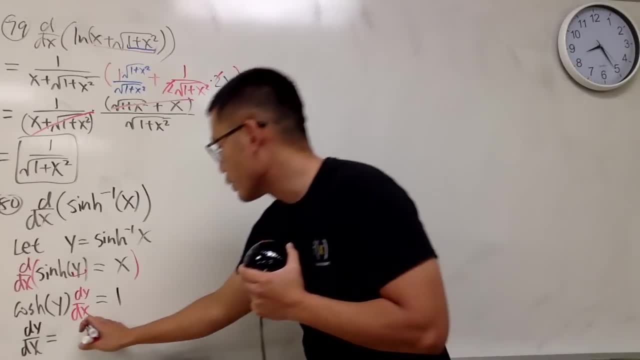 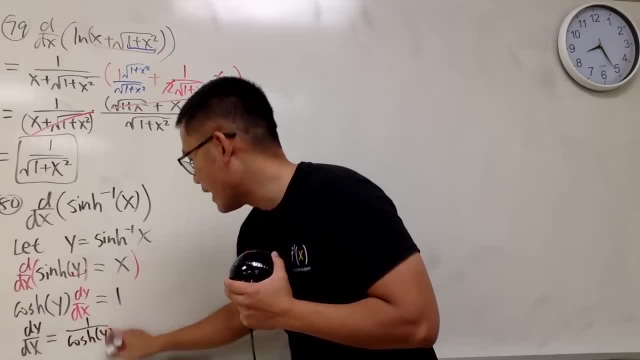 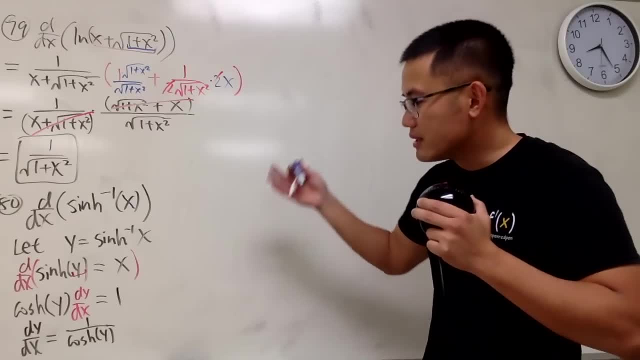 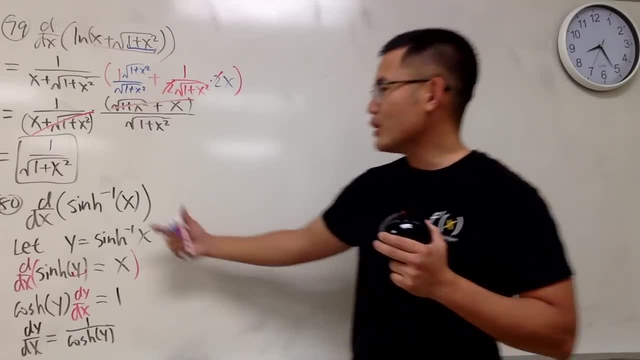 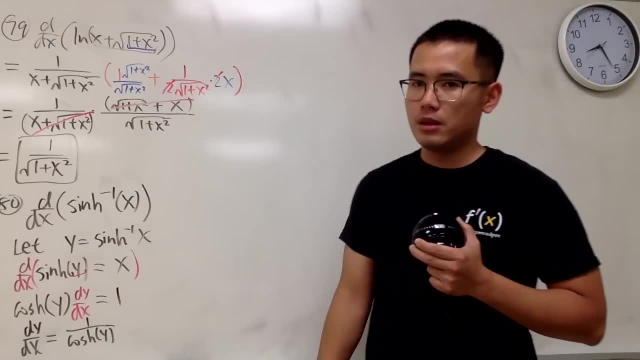 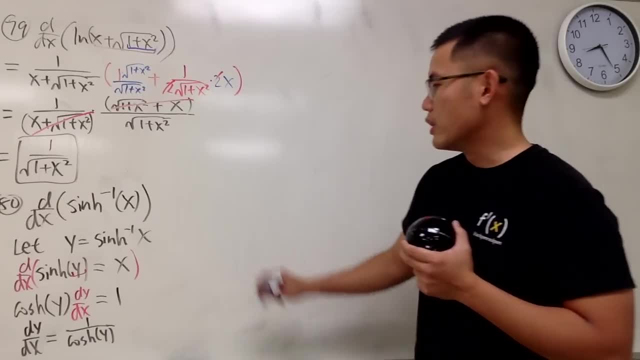 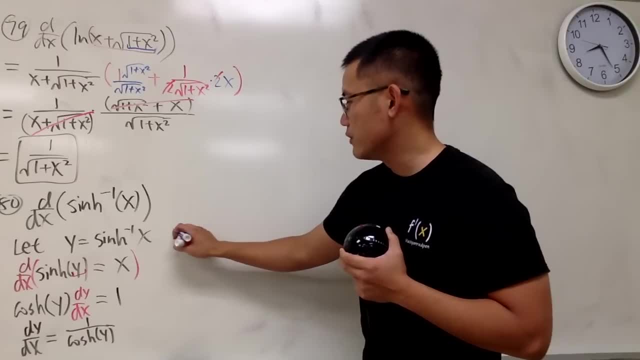 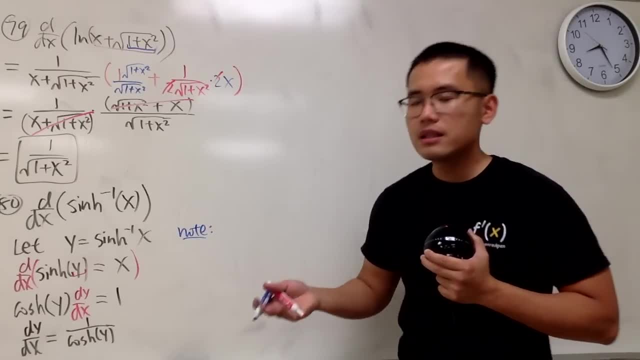 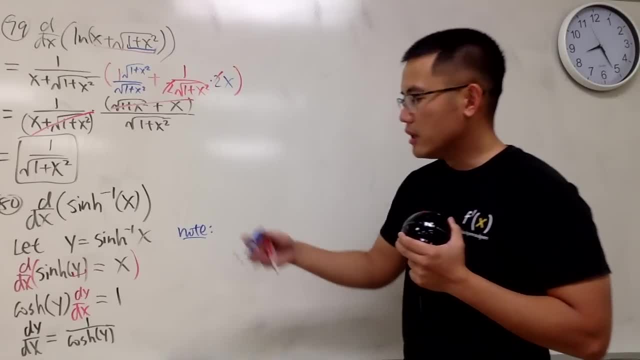 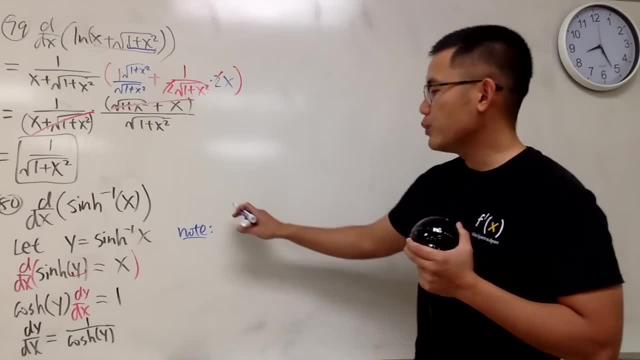 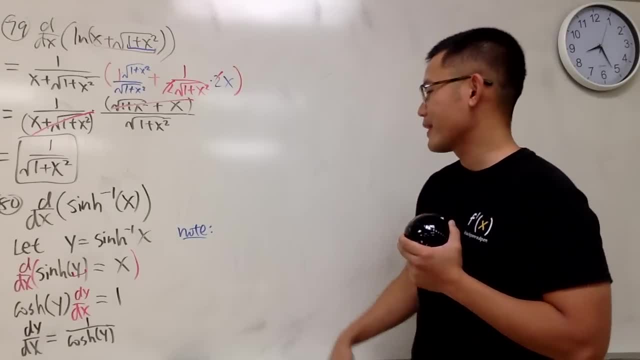 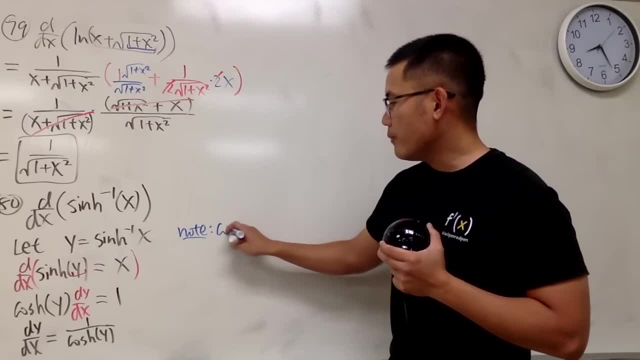 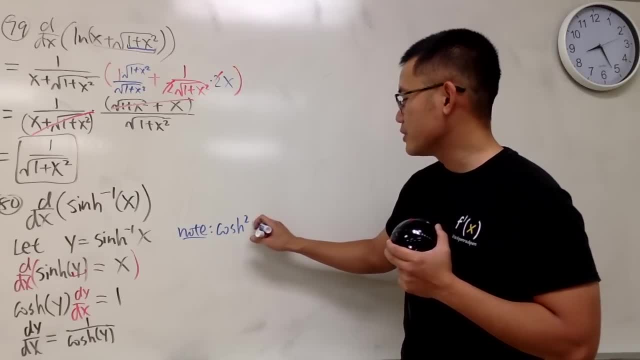 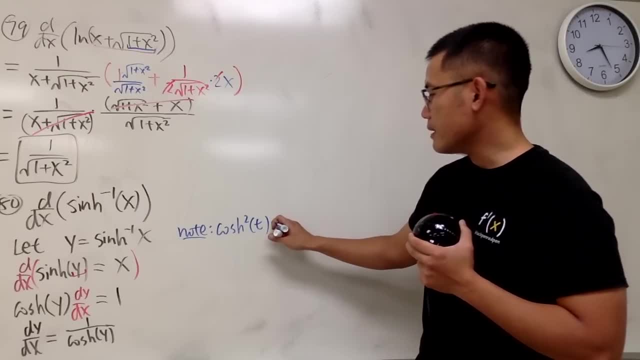 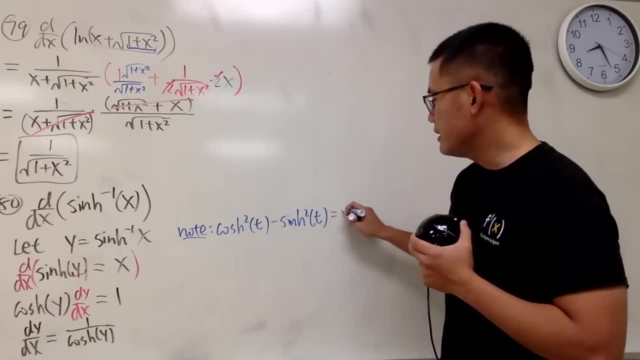 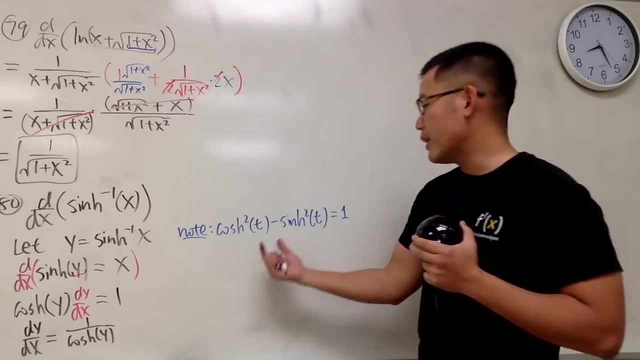 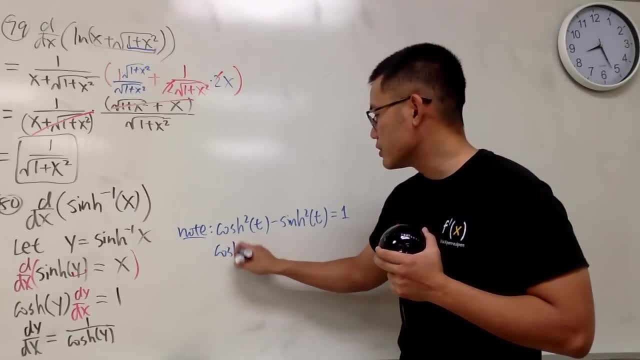 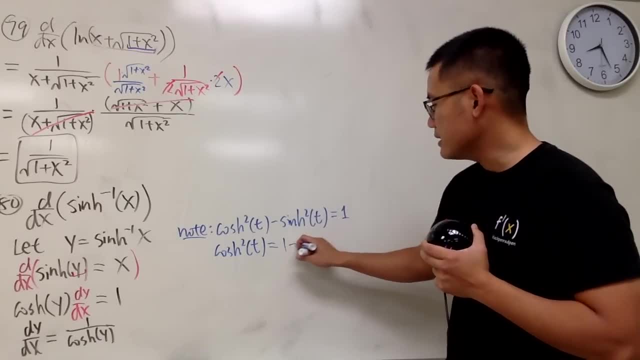 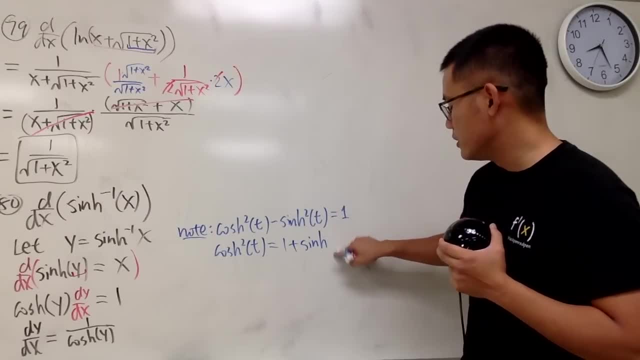 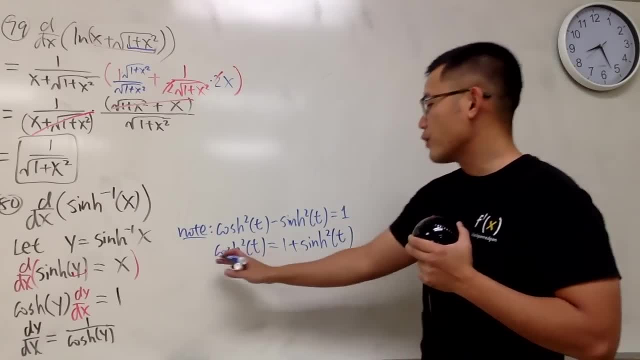 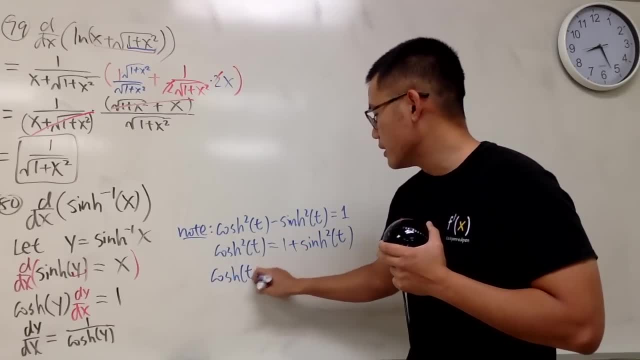 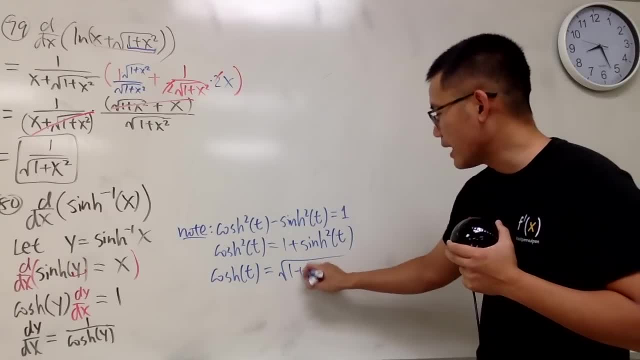 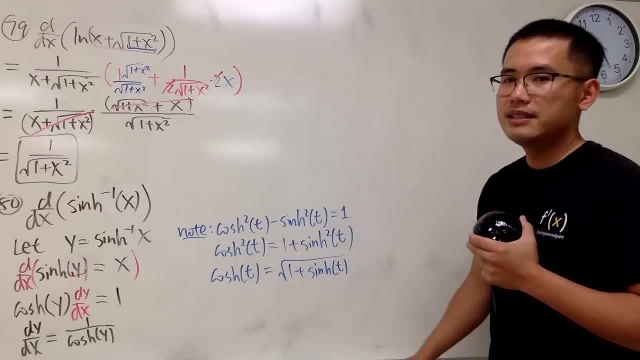 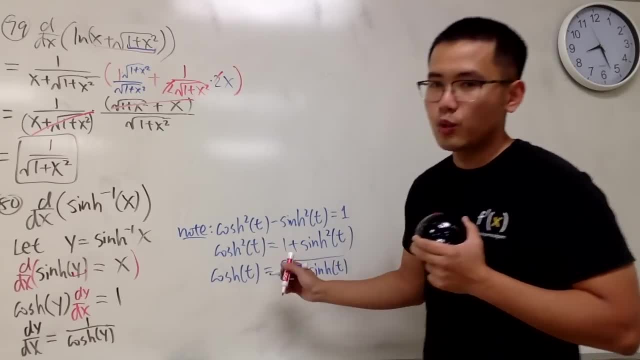 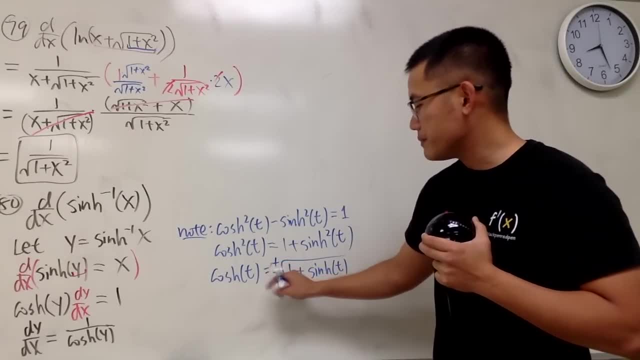 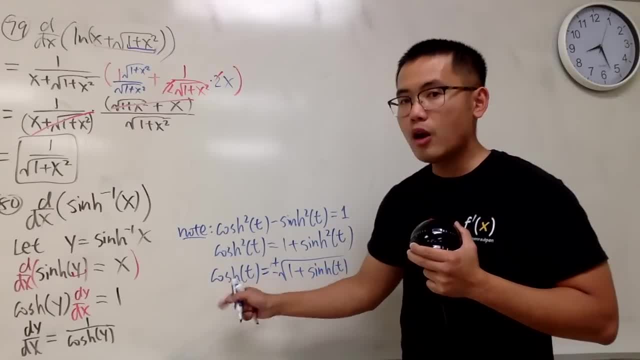 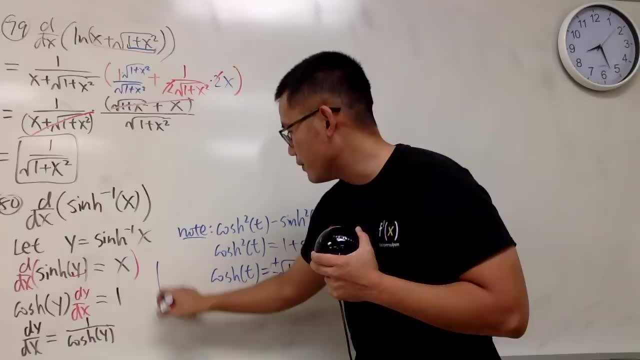 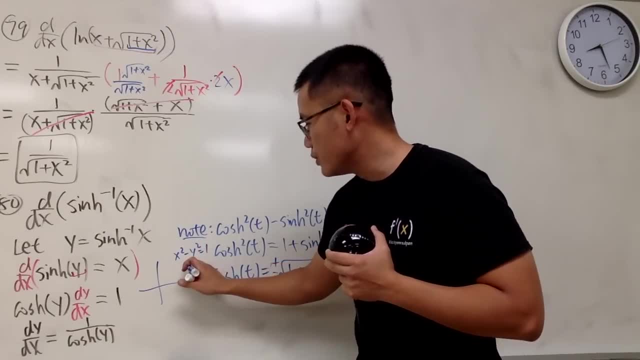 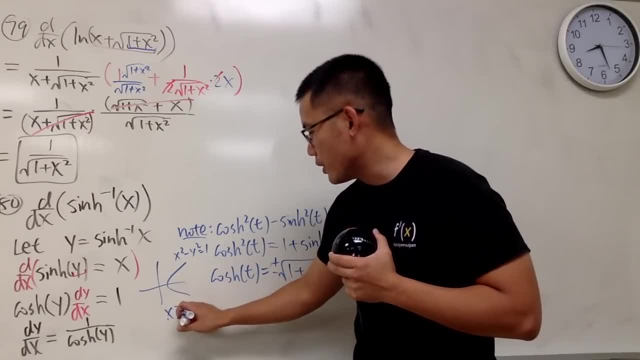 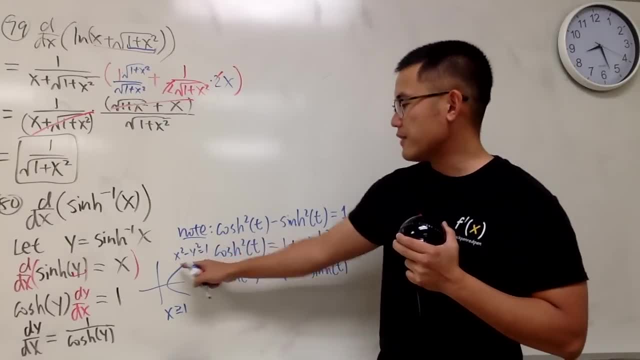 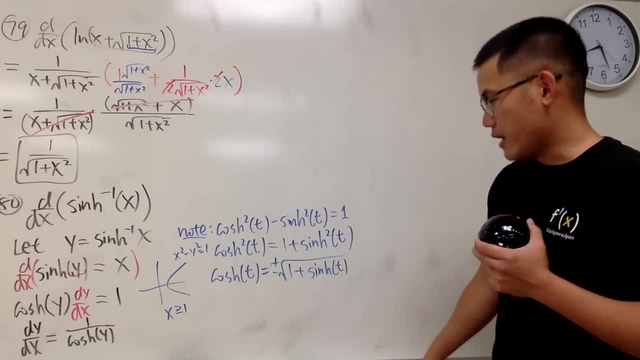 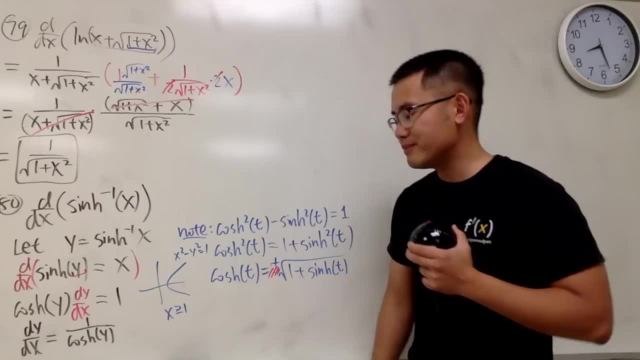 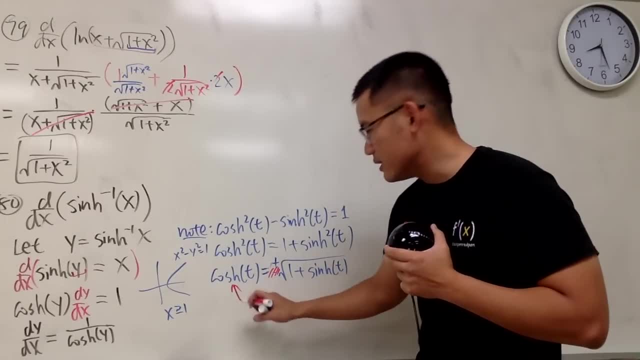 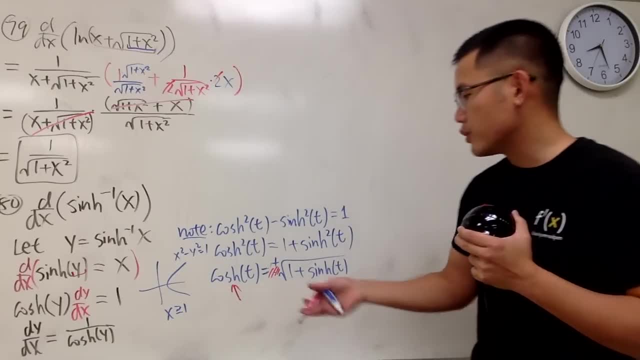 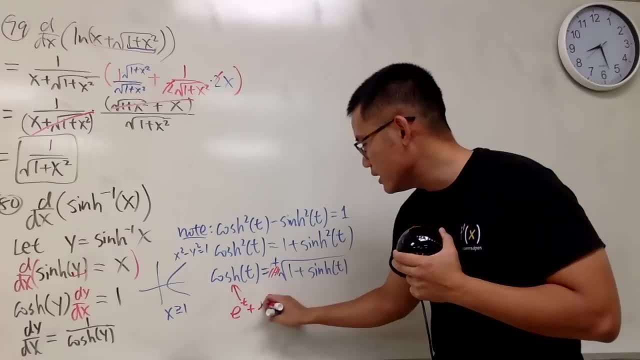 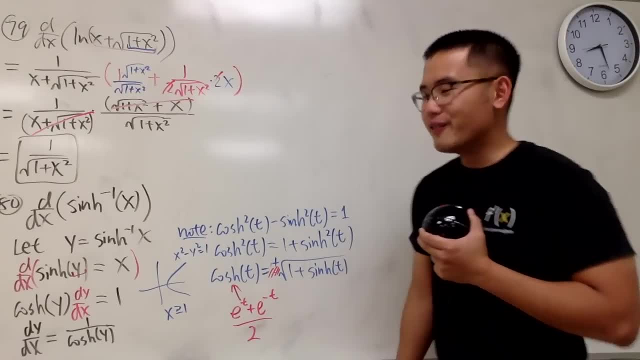 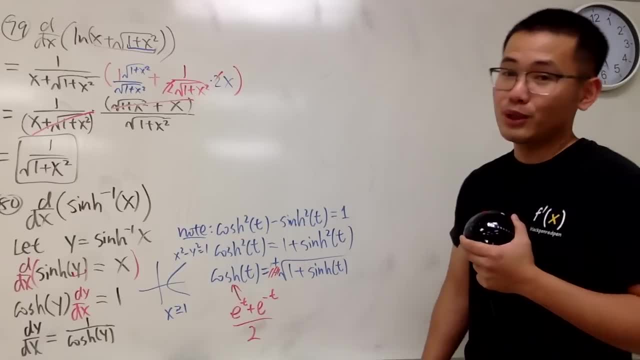 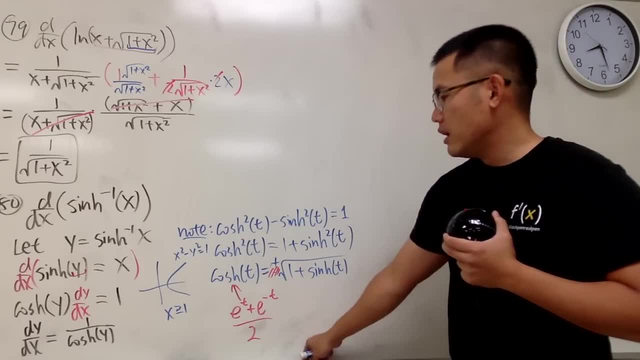 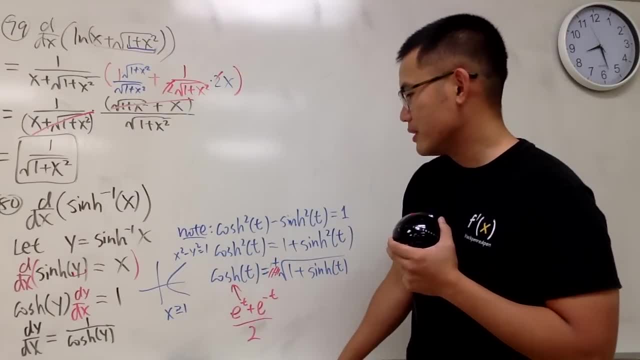 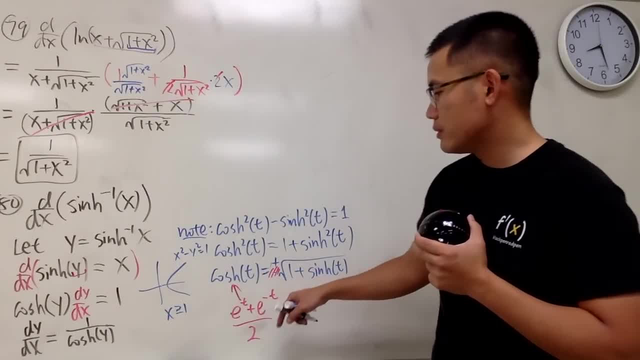 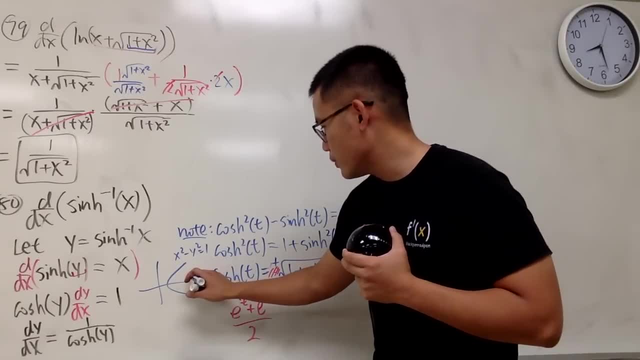 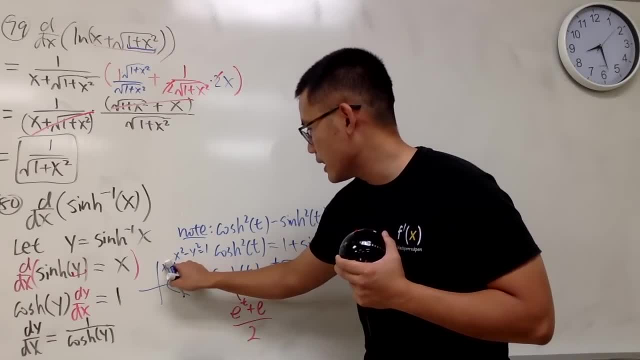 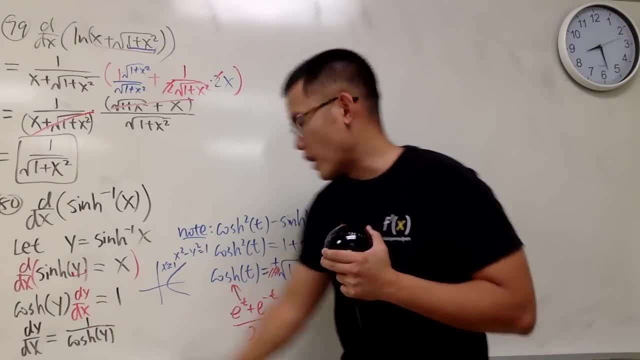 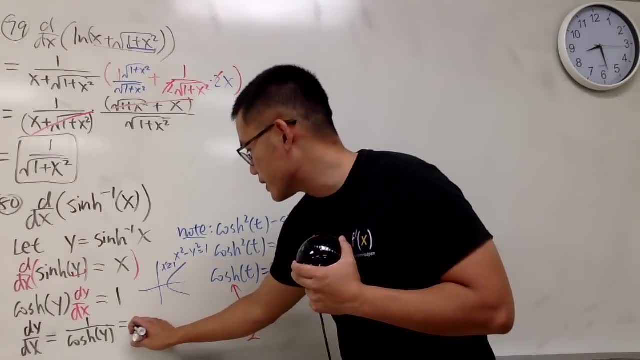 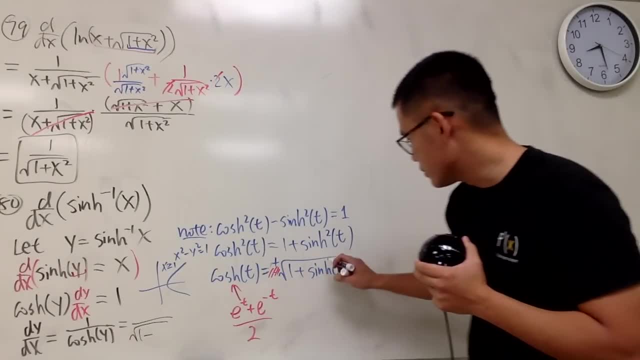 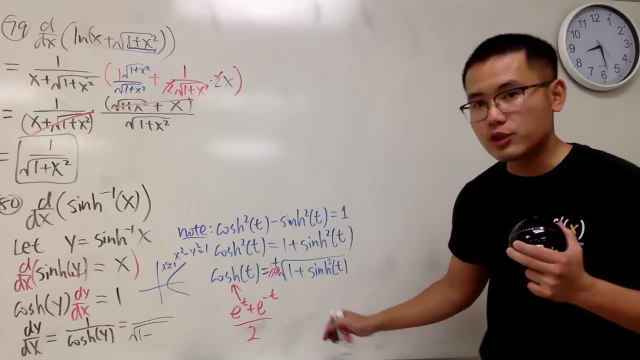 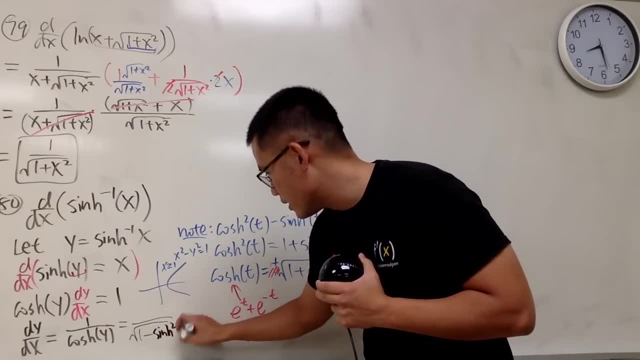 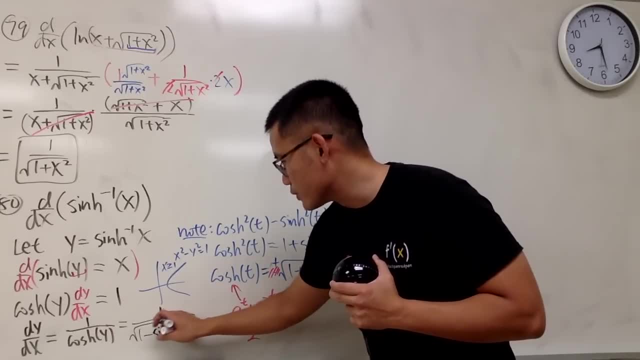 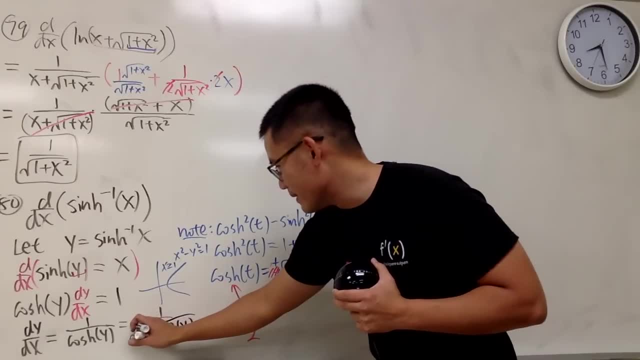 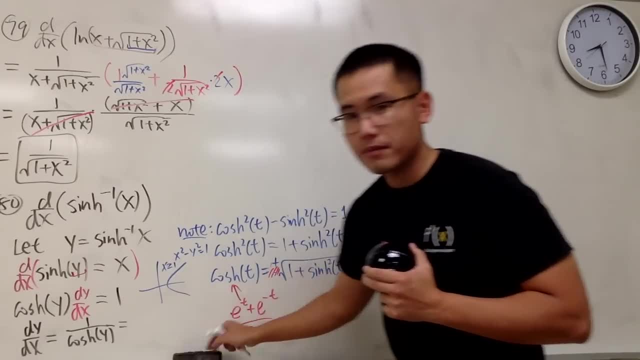 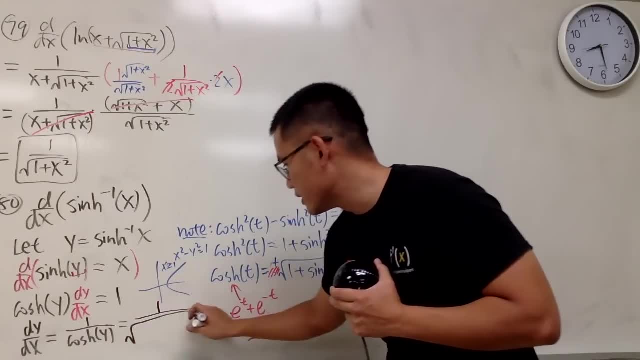 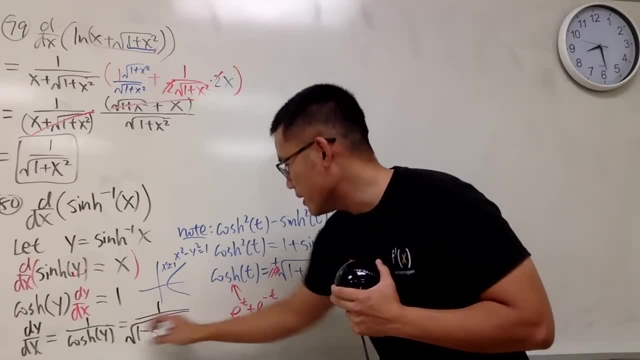 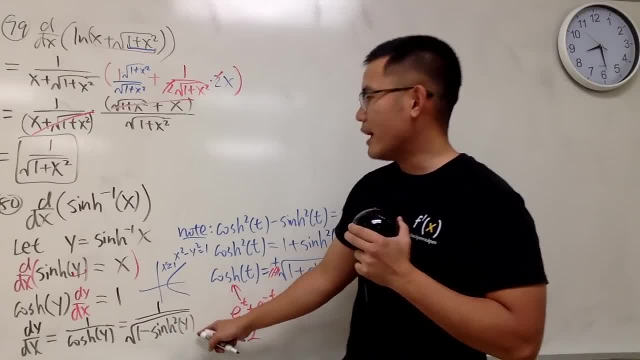 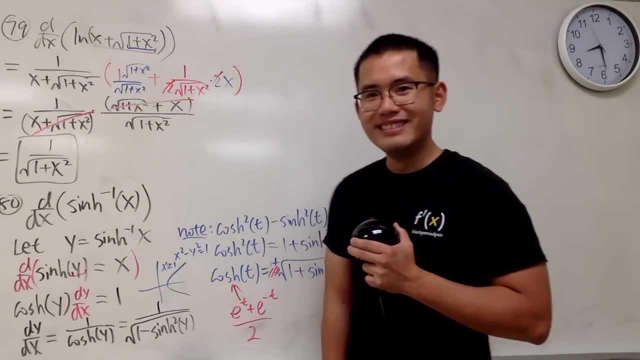 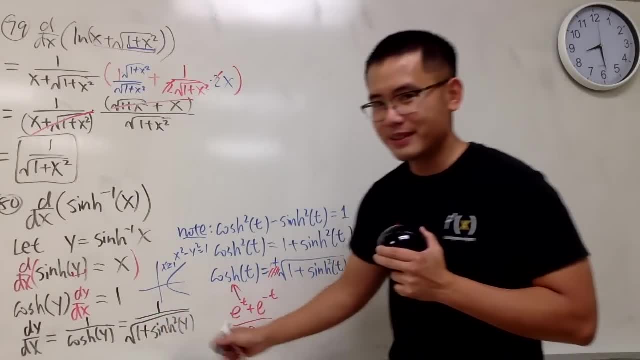 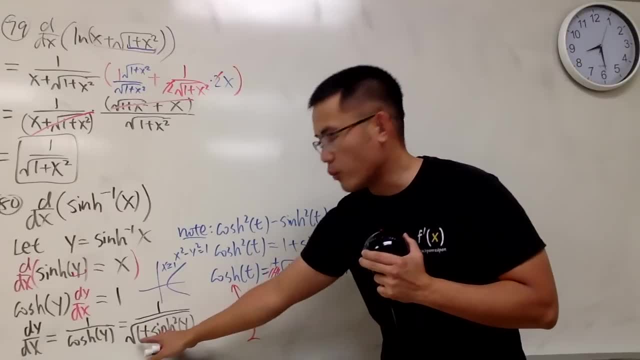 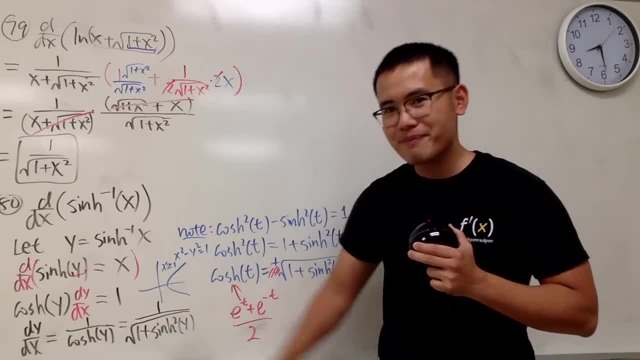 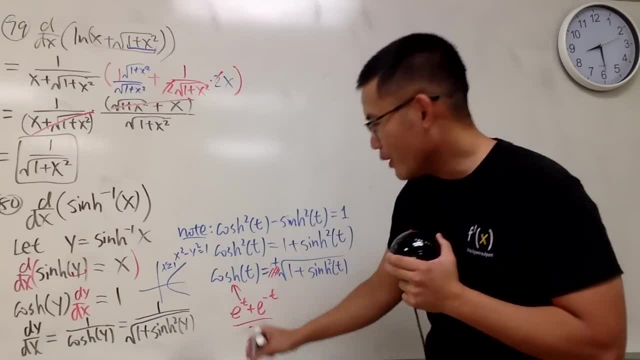 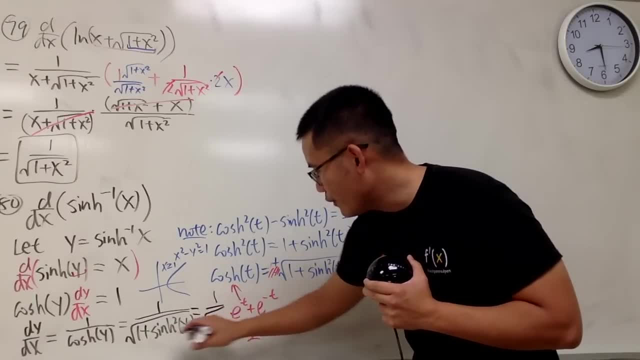 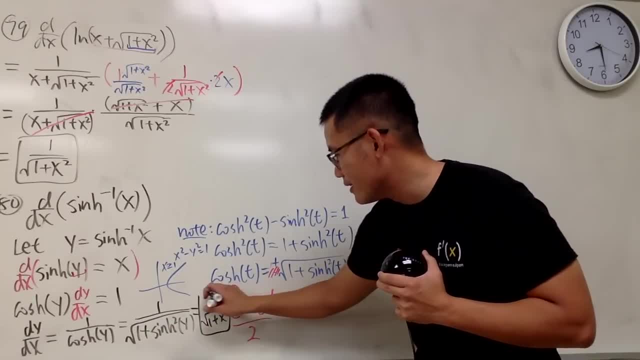 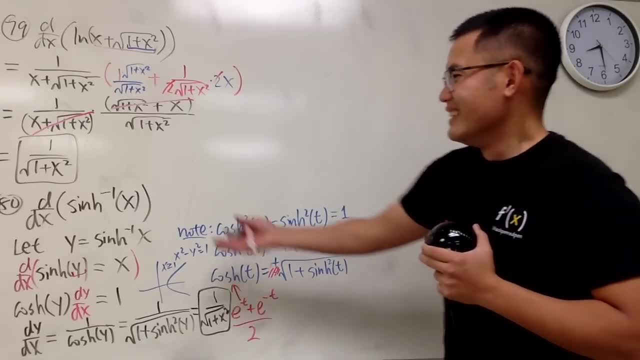 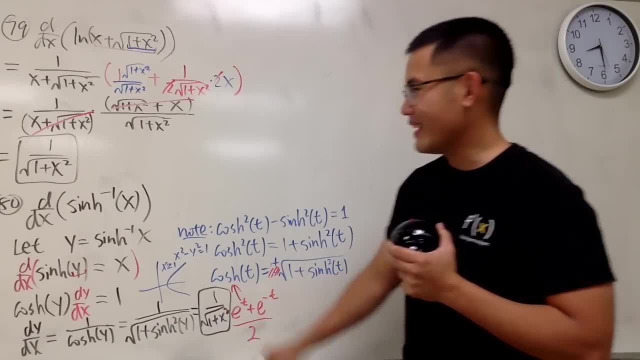 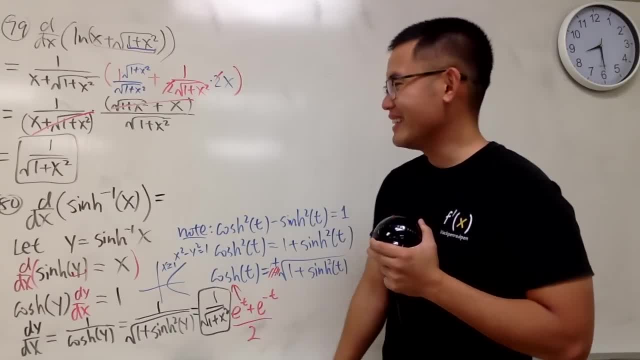 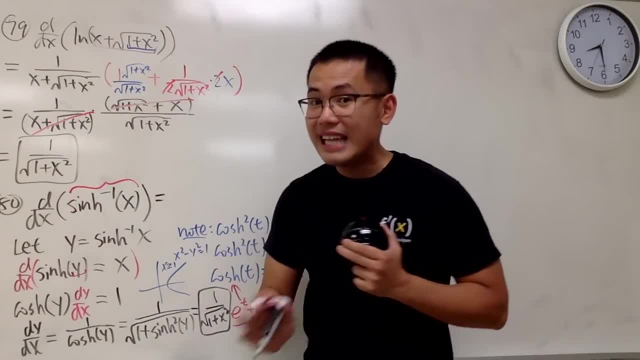 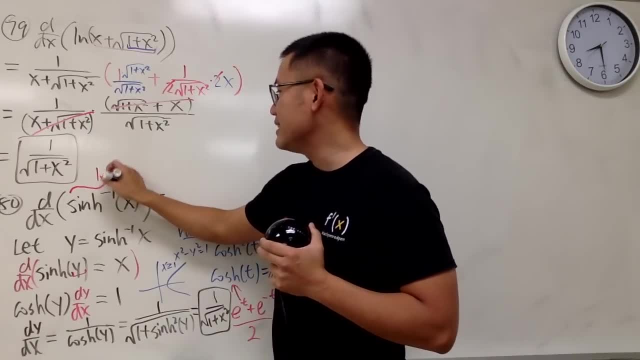 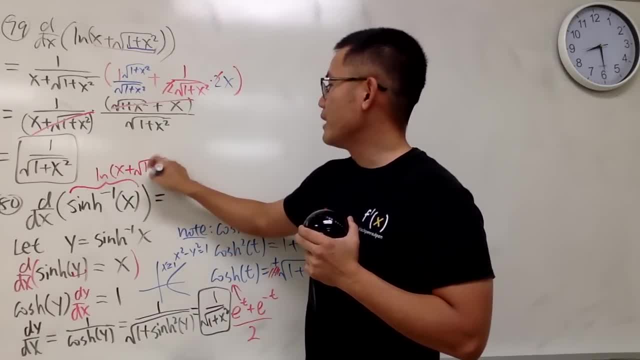 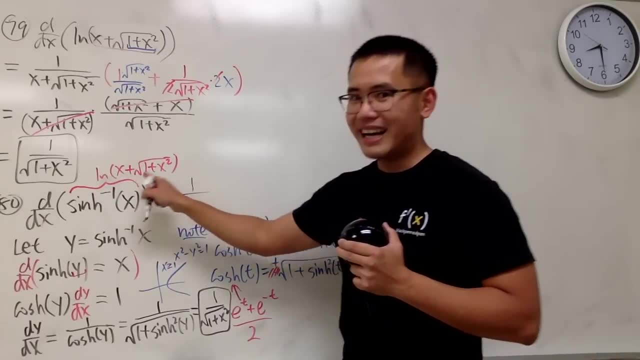 Anyway, this right here is the derivative of the inverse function. Anyway, this right here is the derivative of the inverse function. You can do that by doing some algebra or so, or you can check out my other video for it. But anyway, they are exactly the same. 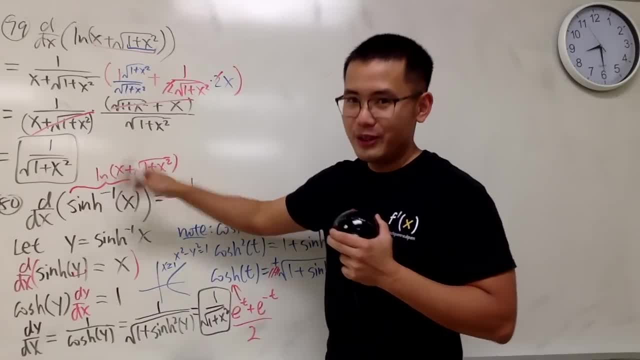 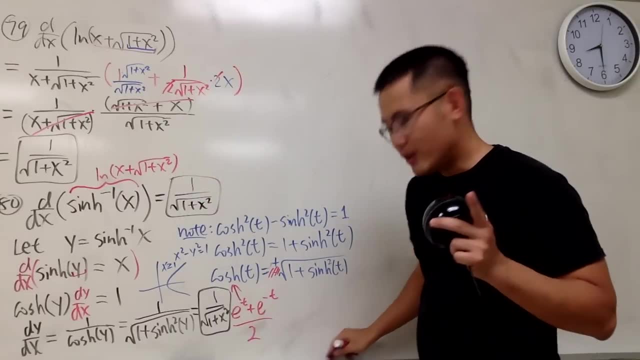 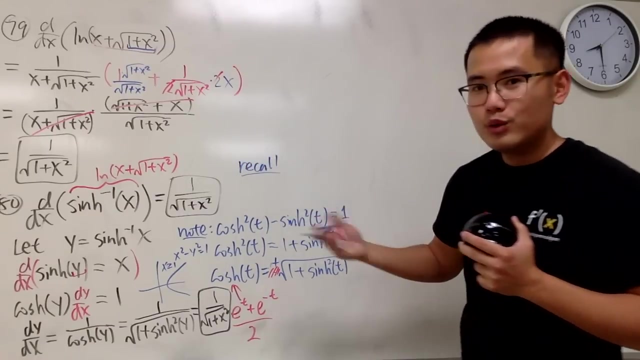 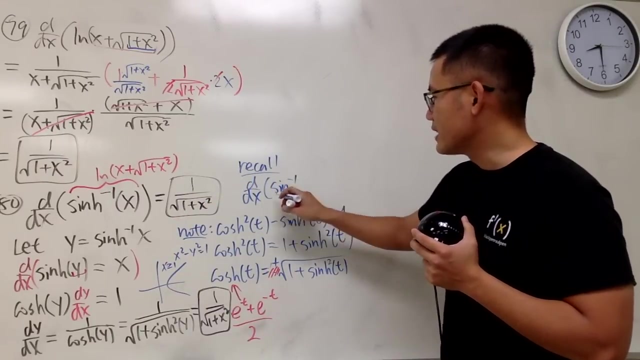 So to differentiate this, if you have this version for it, you can just differentiate that which we did it already. So this is it. And remember, let me just say recall, Remember- the regular version for the inverse sign. if you have the inverse sign, and this is the regular version, not the hyperbolic version, 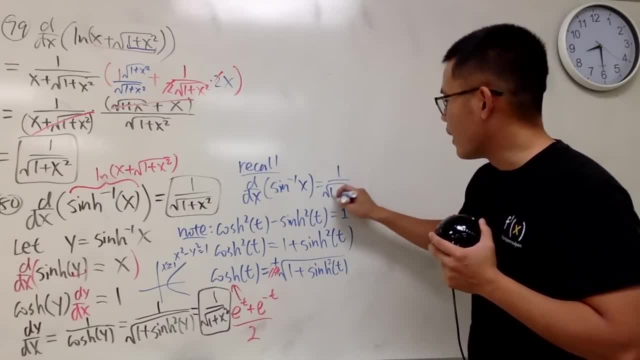 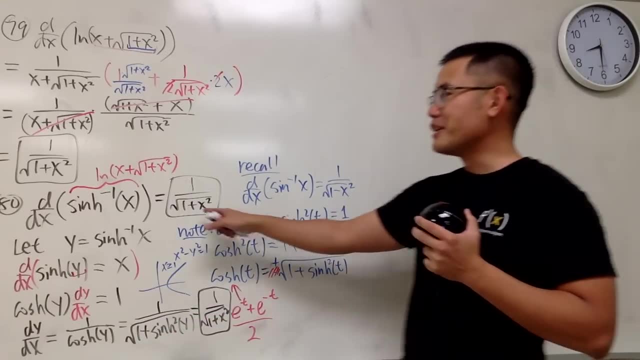 of x for the input. right here you get 1 over square root of 1 minus x squared, And there's no typo. Earlier, it was my bad, but this is it. You see, this is the minus and here you have the plus. 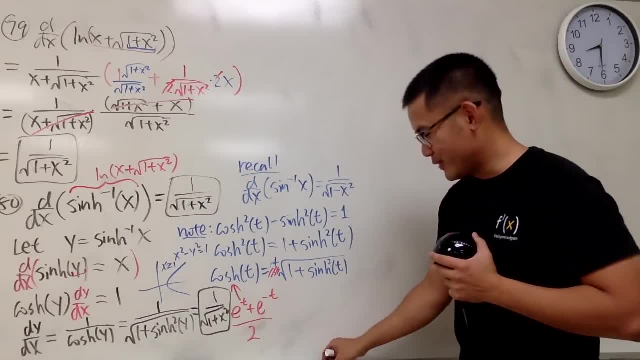 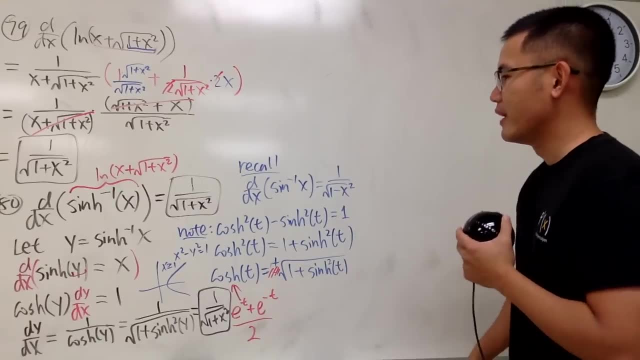 when you have the hyperbolic version of it. Very cool, very cool, very cool. So when I do the 100 trig identities, perhaps I will just include some of the what's that called hyperbolic trig identities as well. 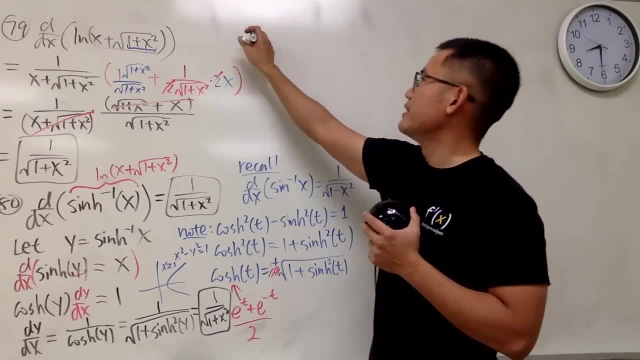 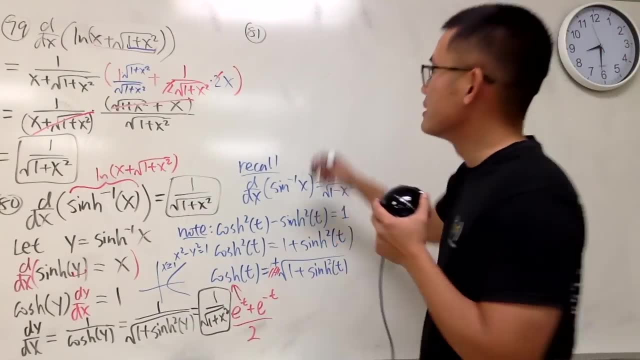 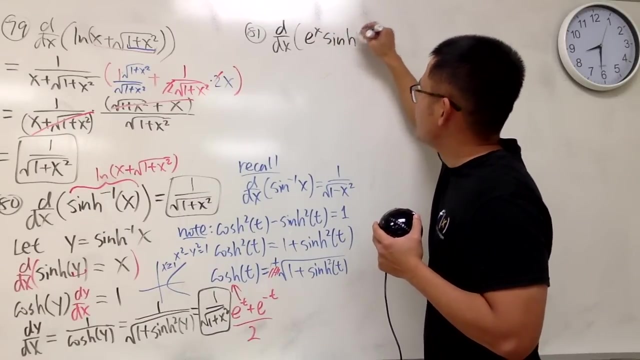 Anyway, number 80.. That's the same as number 79,, technically or secretly, Number 81.. For the rest, I will just kind of show you guys the things that you have to know on a normal way. okay, d, dx, e to the x times sinh x. 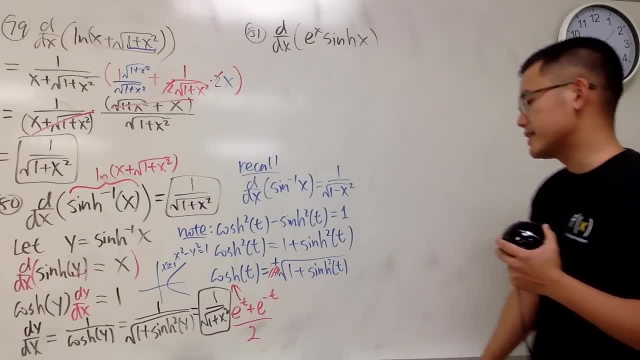 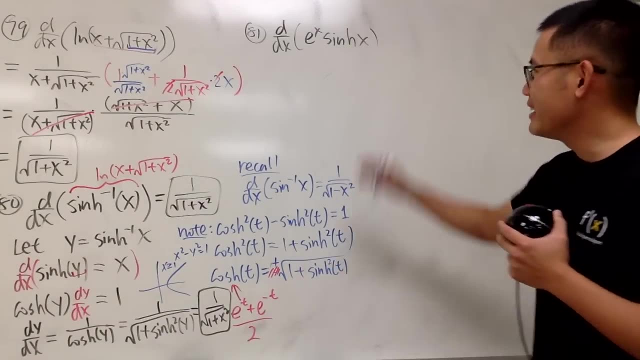 and this is the regular version. okay, sinh of x. Well, cosh is this: sinh is just a minus in between, And then the input is just x instead because we're using x. So to differentiate this right here we can look at: 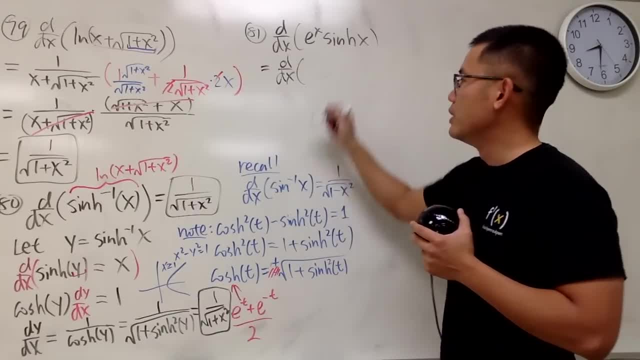 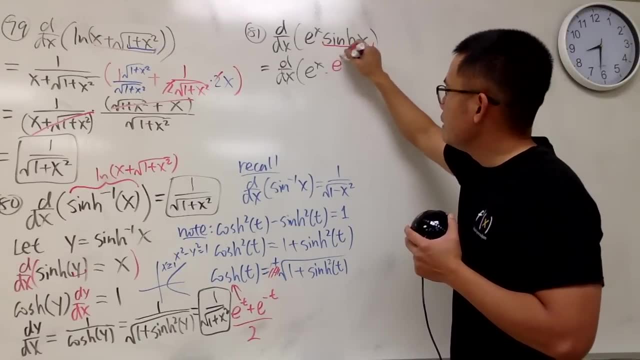 we can, you know, skip the product rule, because this is e to the x and again for sinh of x. this right here is nicely equal to e to the x minus e to the negative, x all over 2.. So of course we can just 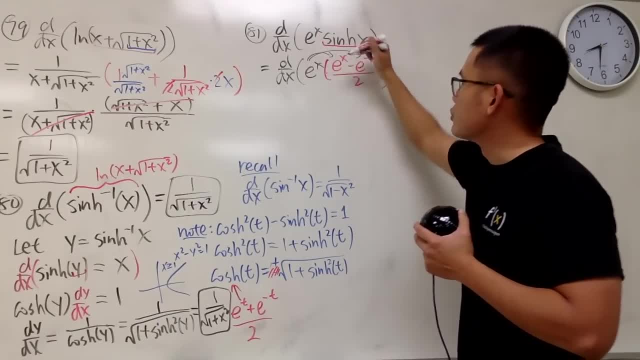 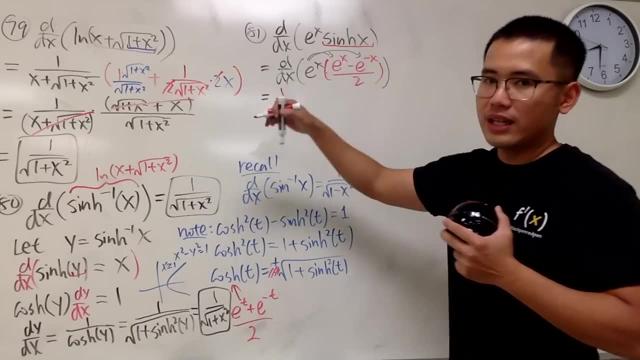 distribute the e to the x first and do the algebra, and then we can just be happy, right? Okay, when we do that, let's put the 1 over 2 all the way in the front, And then we have the differentiation. 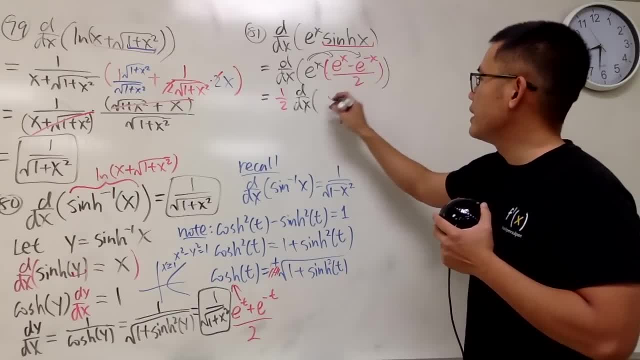 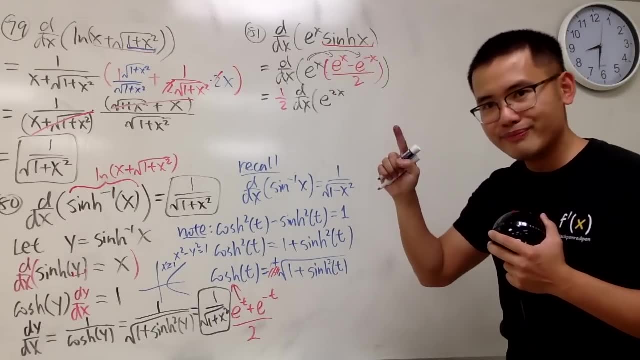 We haven't differentiated yet e to the x. e to the x is e to the 2x, e to the x times e to the negative, x is e to the 0. So it's just minus 1, like that. 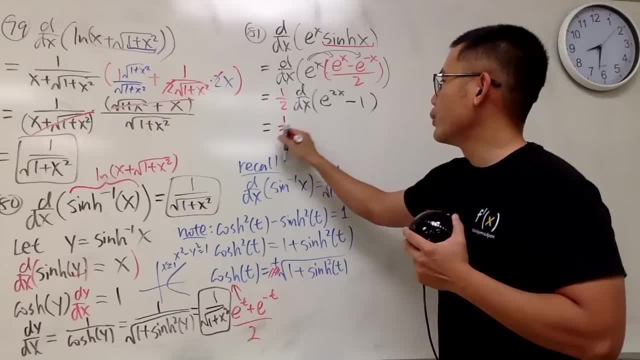 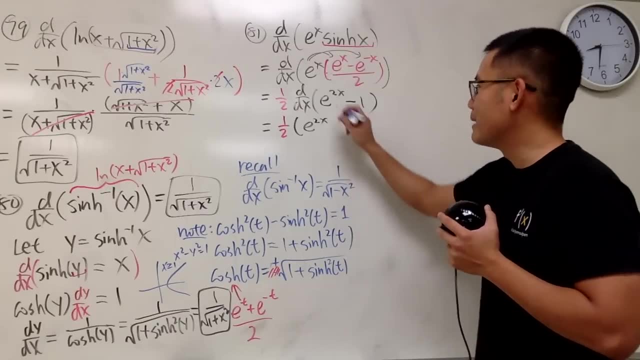 Now for this one: 1 half all the way in the front. Differentiating e to the 2x is e to the 2x. But the Chengdu says we have to multiply by the derivative of 2x, which is 2.. 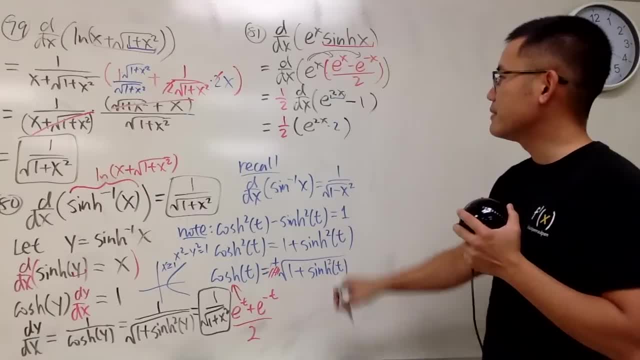 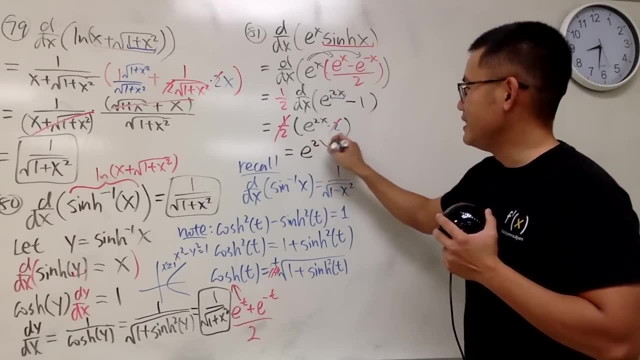 And the derivative of minus 1 is 0, so it doesn't matter. 2 and 1 half cancel each other out. So finally, the answer to this is nicely equal to just e to the 2x. Very good, huh. 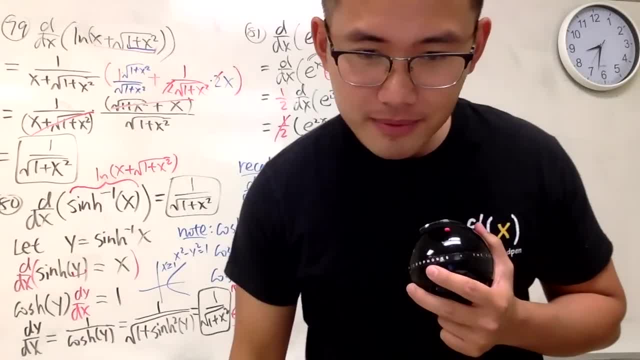 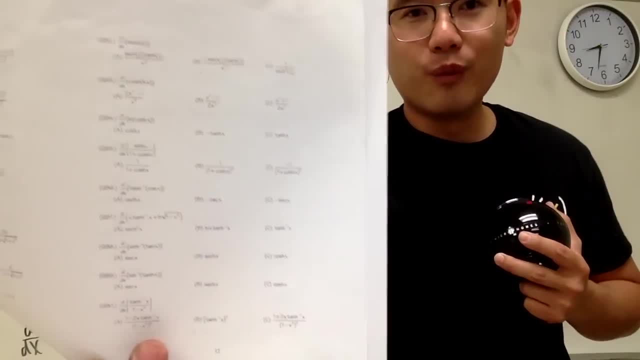 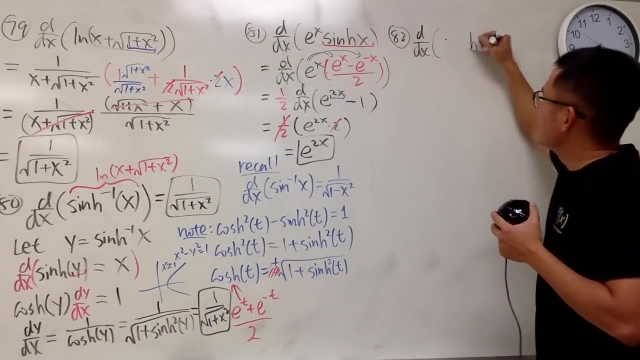 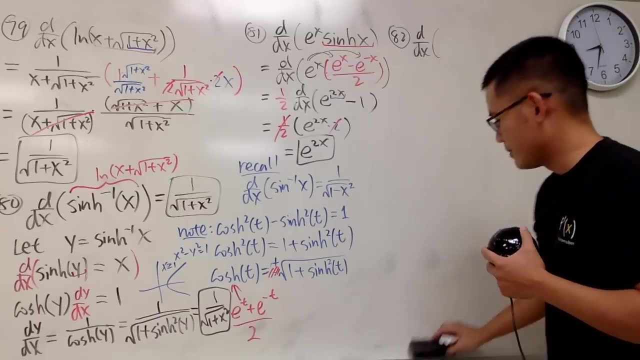 82.. Okay, Hyperbolic secant of 1 over x. Oh my god, Hyperbolic secant. okay of 1 over x. That looks like a- let me just write it down better: Hyperbolic-. 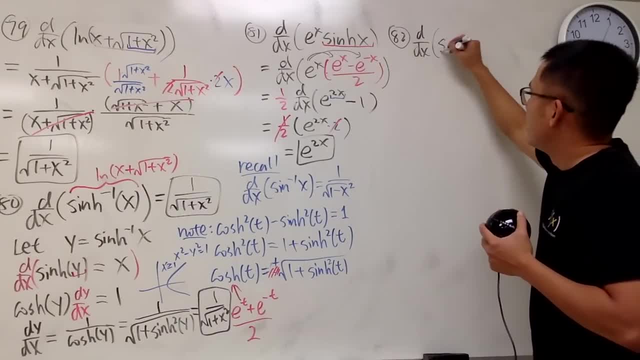 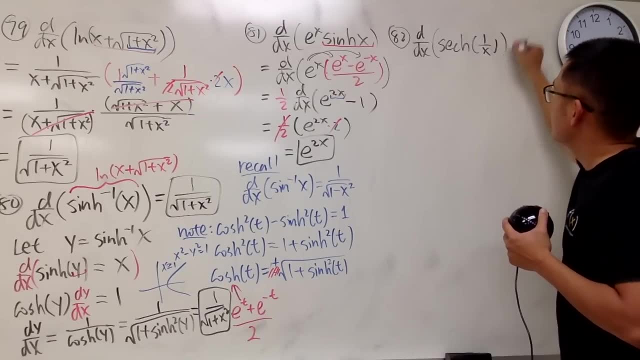 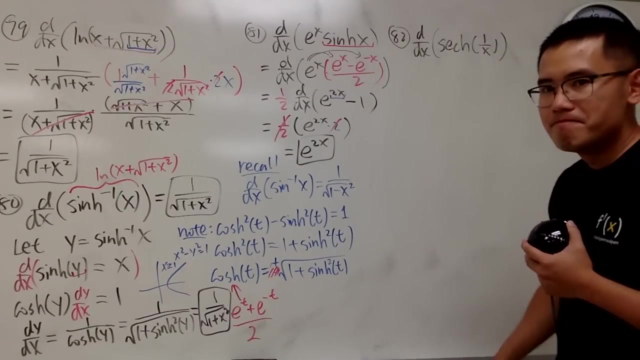 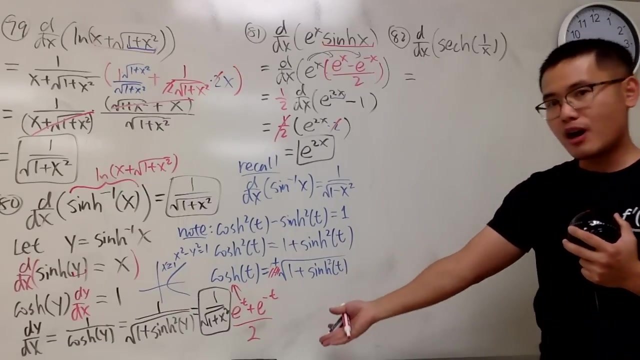 I don't want to have space There we go, There we go Of x. No, no, It's 1 over x. Okay, Like that, Well, well, Well, the truth is, I told you guys about Cauch. 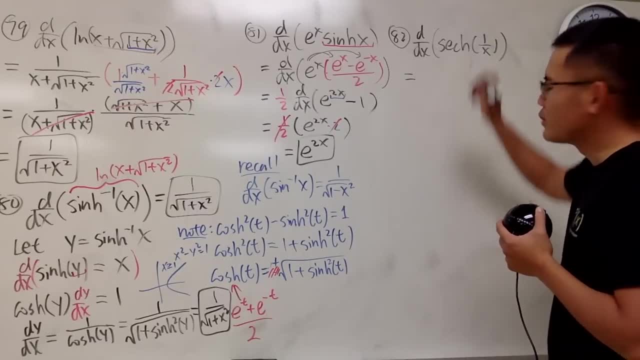 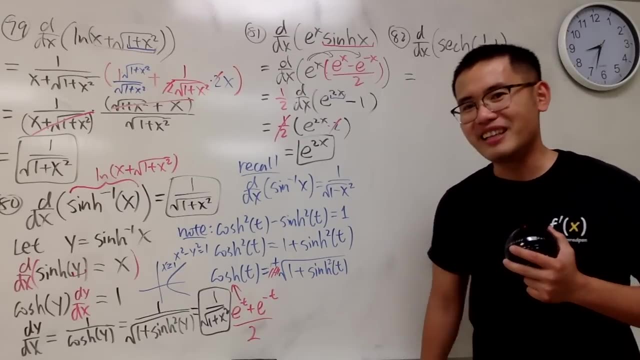 and Zinc. We'll be using them along the way. This right here: yes, you are thinking it's secant h and then tangent h, right Kind of, but you're missing the negative sign. Let me show you This right here. 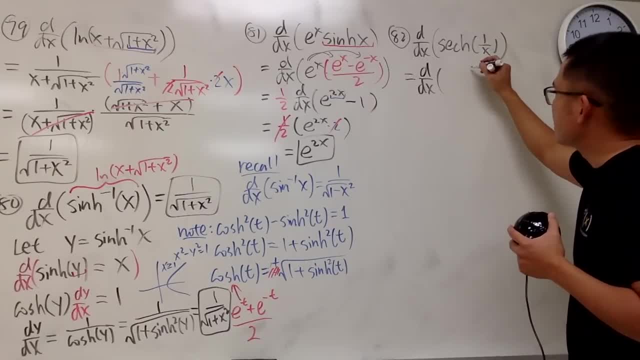 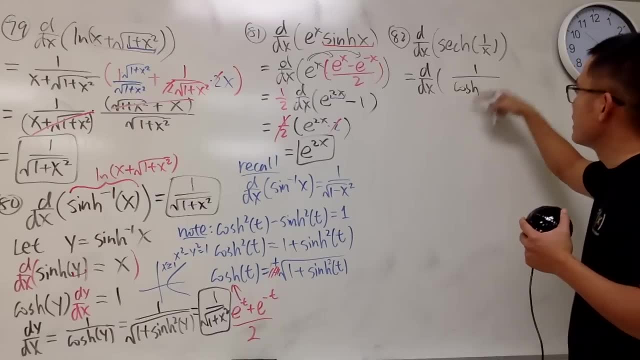 yes, you are thinking what exactly this is. This is exactly the same as 1 over Cauch. Okay, Hyperbolic secant is the same as hyperbolic cosine, 1 over hyperbolic cosine. And then the input stays the same. right here, of course. 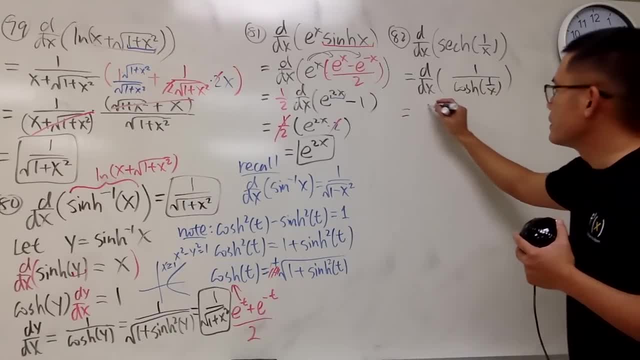 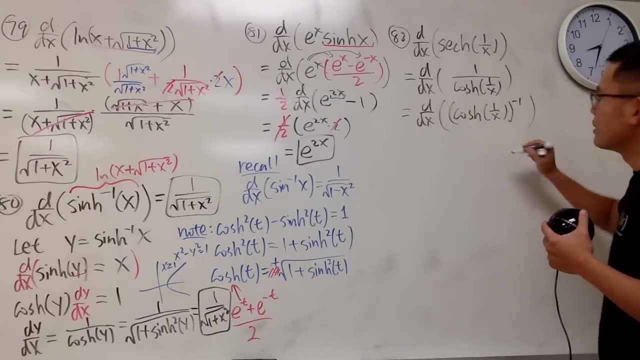 Then we can write this to the negative 1 power. This is d dx Cauch of 1 over x. Then raised to the negative 1 power, This means 1 over. This does not mean the inverse Cauch. 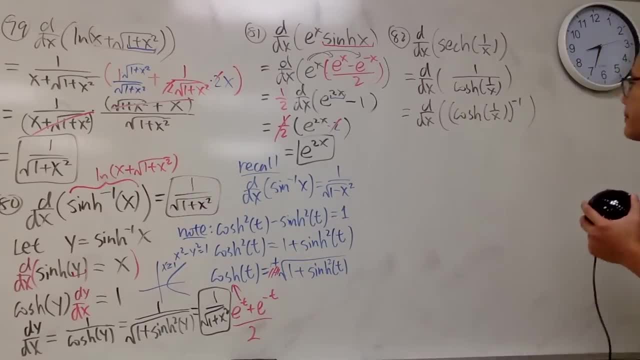 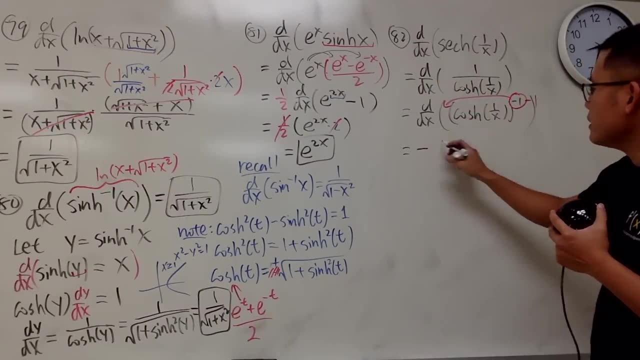 Okay, So again, know your notations. All that, Right. here we can bring the negative 1 to the front, Minus 1.. Good, all that. So we have negative parenthesis. Cauch of 1 over x. 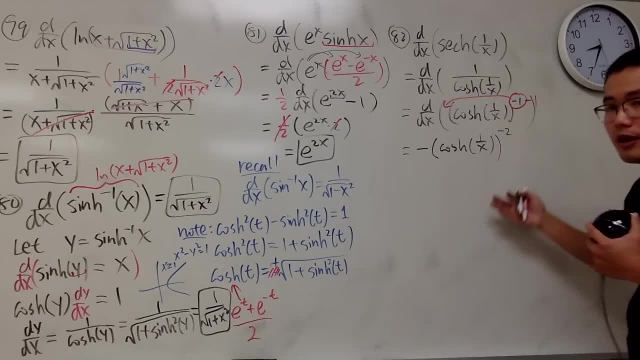 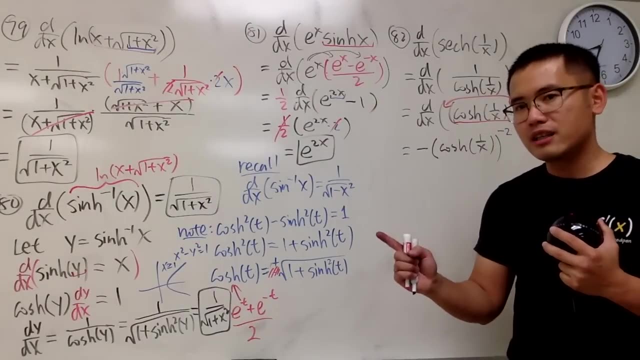 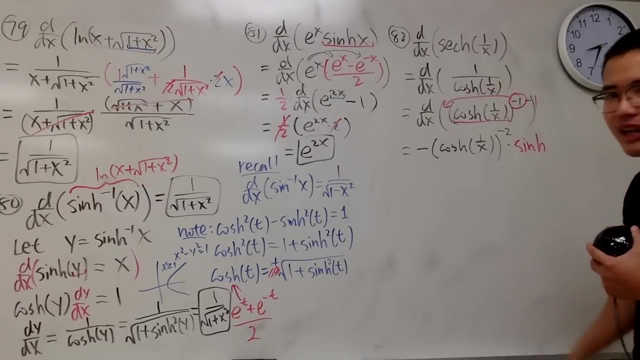 to the negative 2 power right here. And then we have to multiply by the derivative inside. The derivative of cosine is negative sine, But the derivative of Cauch is positive, sinh. Okay, There's no typo. The derivative of Cauch is sinh. 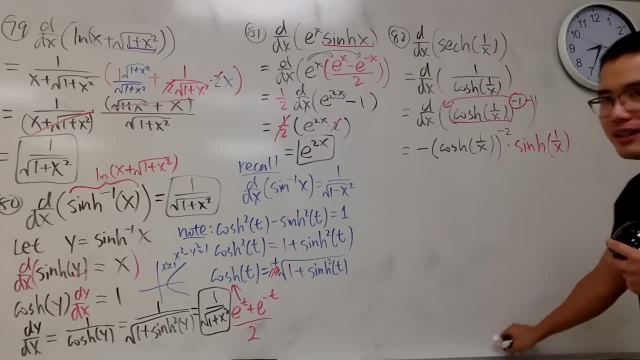 And you still keep the input And, of course, we still have to do the chain loop right here. The derivative of 1 over x is negative: 1 over x squared. This is the one I told you guys. You should know it by heart. 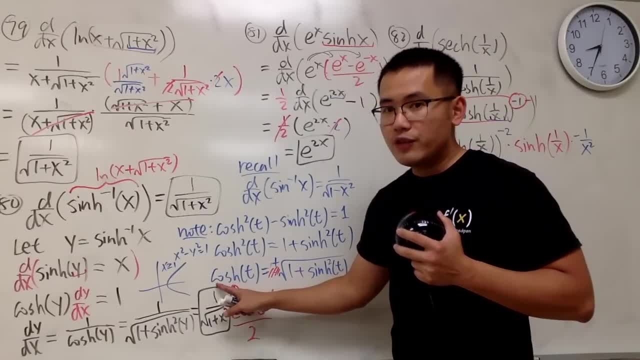 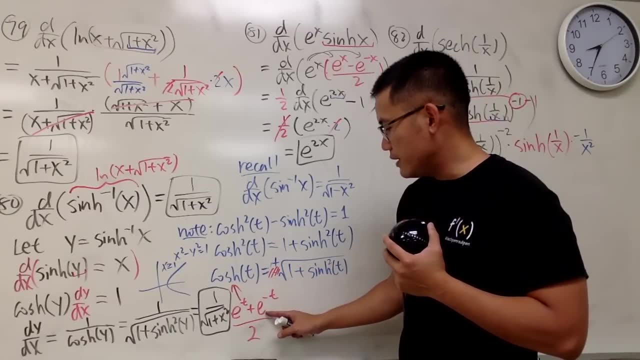 Let me prove it to you guys real quick. When we differentiate Cauch t, you differentiate this e to the t, which still gives you e to the t. Differentiating this, you get negative e to the negative. t over 2 is still over 2.. 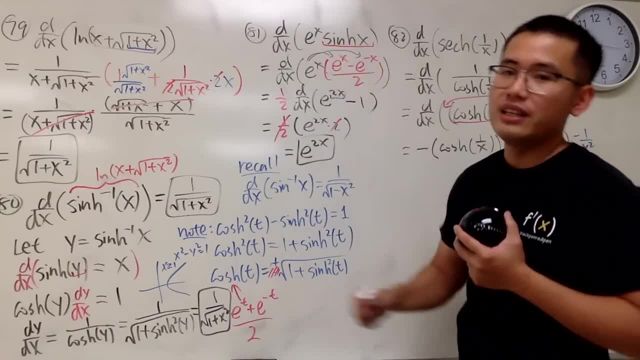 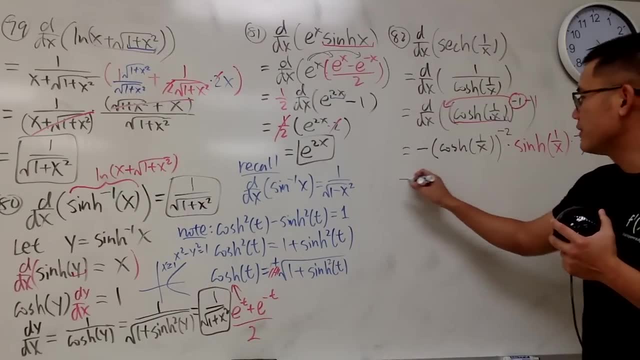 This right here is exactly that, which is exactly just sinh of x, Right? Just if you use a different input, of course. Anyway, this is the idea, But of course we simplify this a little bit. That's positive. 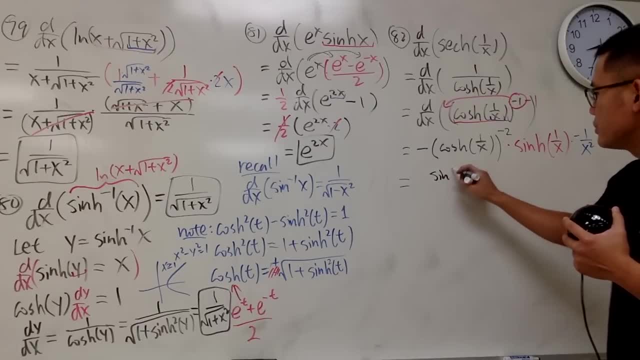 This goes down to the denominator. This stays on the top. So you have sinh of 1 over x, Of 1 over x. This, right here, is the same as saying Cauch of 1 over x. Right, Cauch of 1 over x. 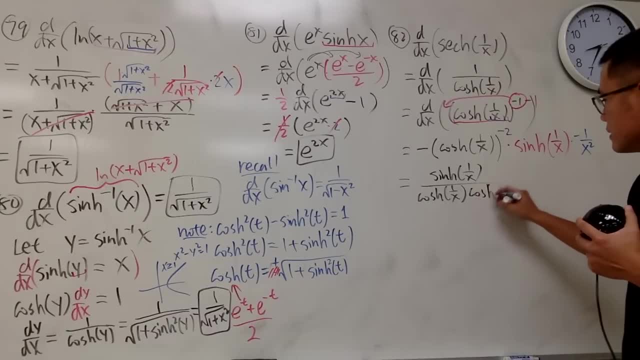 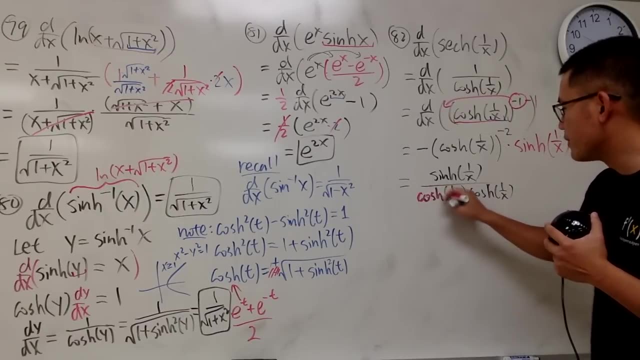 And another Cauch of 1 over x. Yeah, And the reason I want to do that is because, just like the Google days to prove the derivative of secant, you see that right here. This is 1 over that, which is by definition. 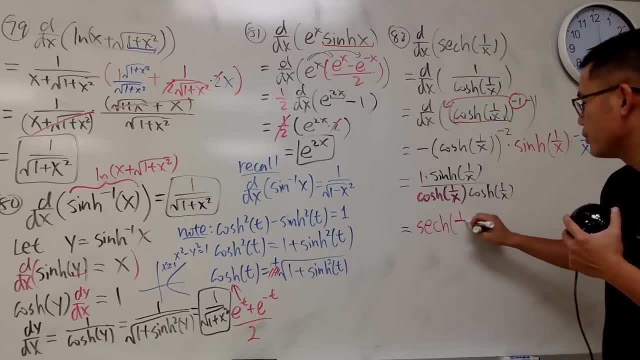 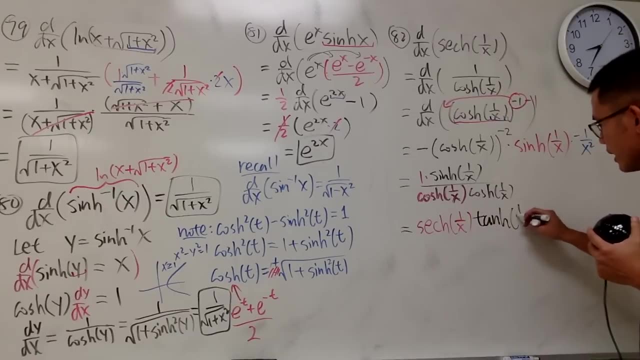 the hyperbolic of the secant and of the input, which is 1 over x. This right here, yes, is the hyperbolic tangent. So you have the tangent and the input is 1 over x, And with that we are done. 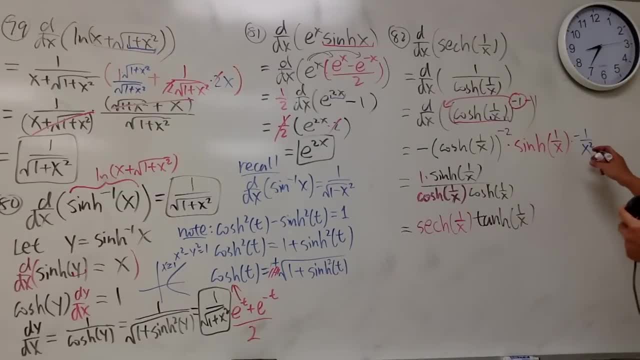 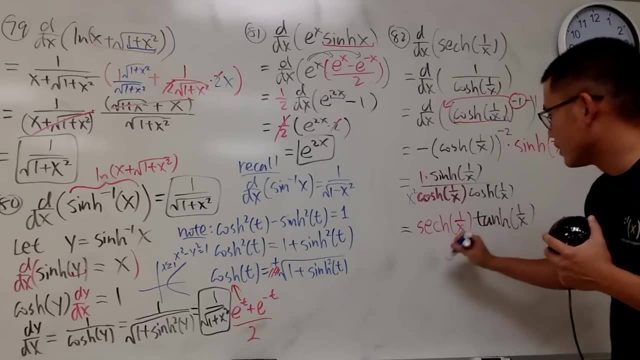 Very, very nice. Oh, I forgot the 1 over x. Oh, I forgot the x squared. I forgot this guy. The x squared Right. I forgot this guy x squared right here. So we have to have the. 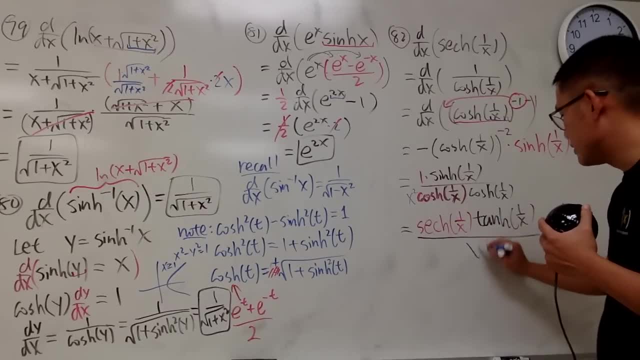 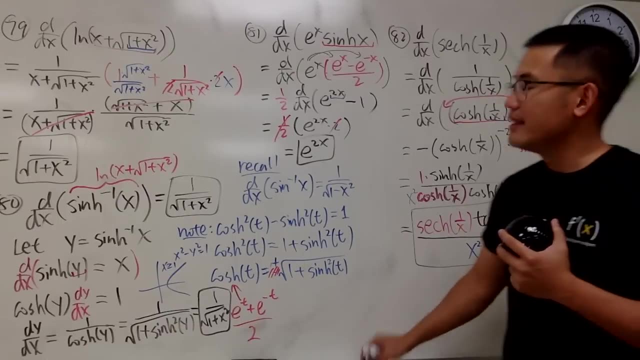 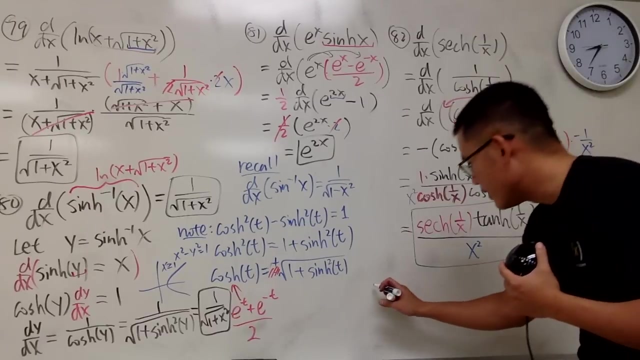 over this. x squared is still in the denominator, And with that we are done For sure. Alright, that's 82.. Now 83.. Let's see, just for fun I want to fit in here 83.. 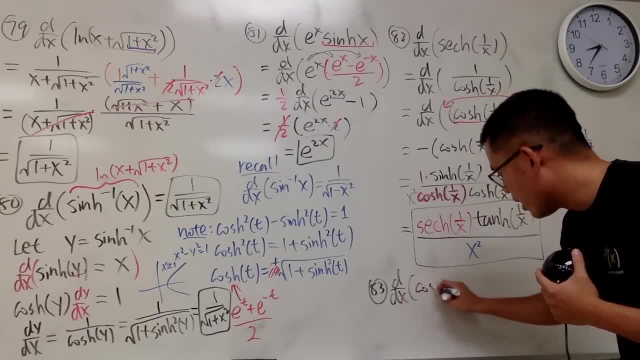 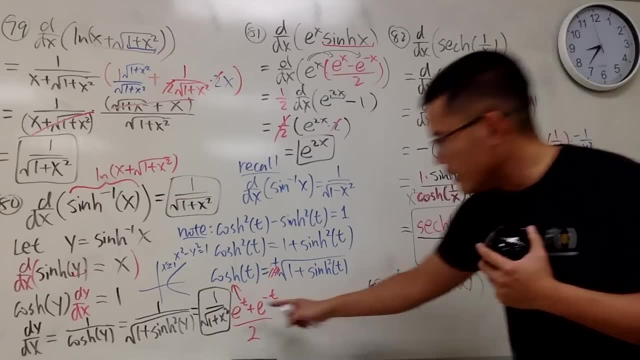 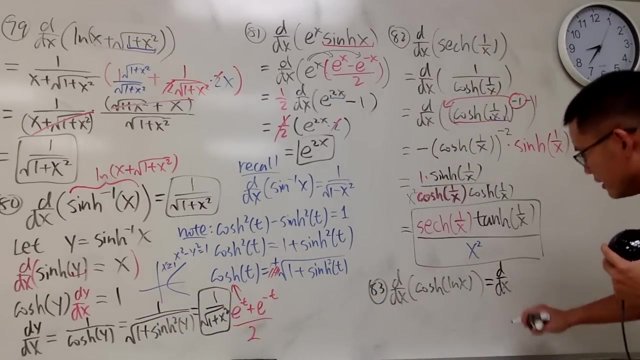 d dx of Cauch of natural log of x. This is not so bad because we can just put the natural log of x in here and in here and we can take care of business. Check this out: Do the algebra d dx, So put the natural log of x. 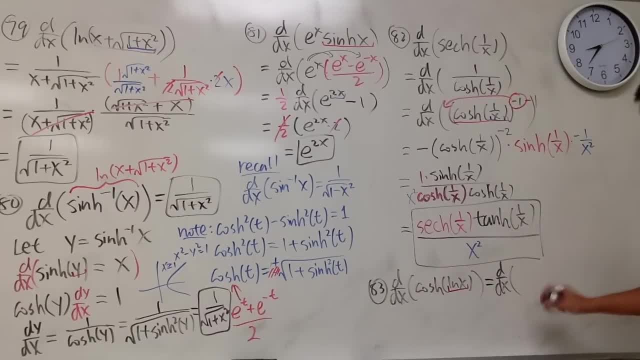 again in here and here. So we end up with over 2 is still over 2 on the bottom, So let's put that down. And we have e to the natural log of x, So e to the natural log of x. 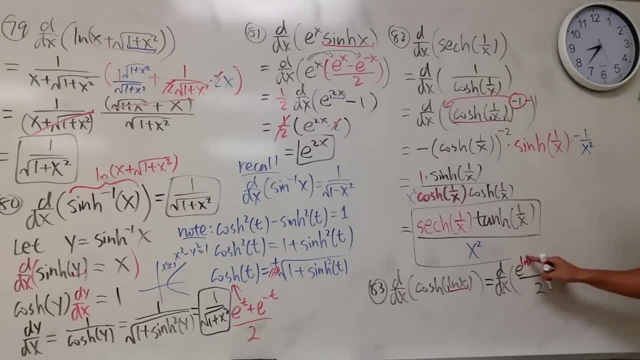 And then for the other part. for the other part, we have the plus e to the negative natural log of x, like this: Well, well, we can simplify this and just have to do it carefully, Because, for example, e to the natural log of x. 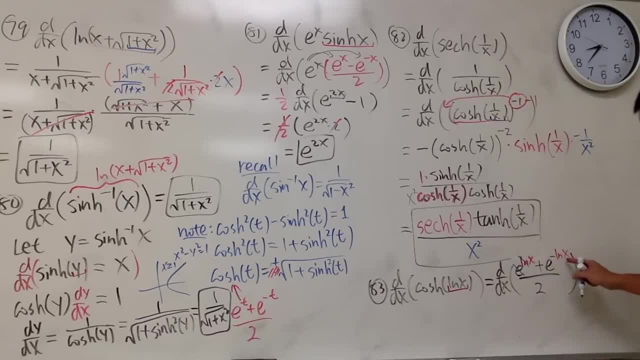 they cancel out nicely, But this and that it does not cancel out nicely yet You have to put the negative right here. So you end up with e to the natural log of x to the negative 1 power and then cancel it out. 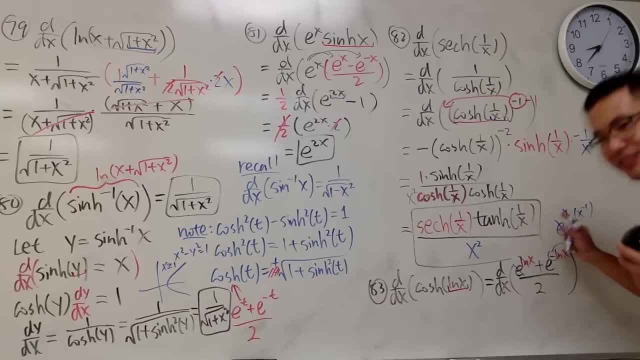 You have to make sure this is right here, is clean. It has to be just a positive 1, technically. So bring that to the front, so you have that, So we see this right here. It's actually just to have the 1 over 2. 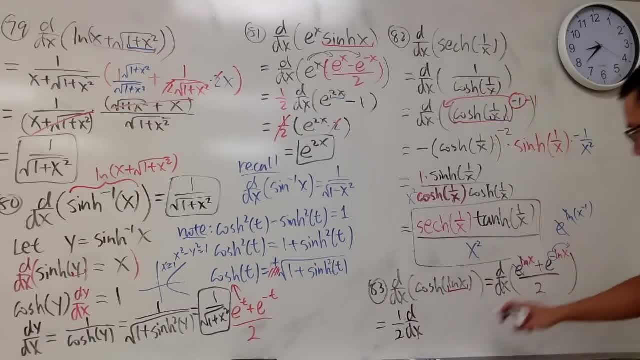 all the way in the front. and then d, dx. First part is we just have to differentiate x. Second part: we have to add it with x to the negative 1 power. So this is all we are differentiating. So here we go. 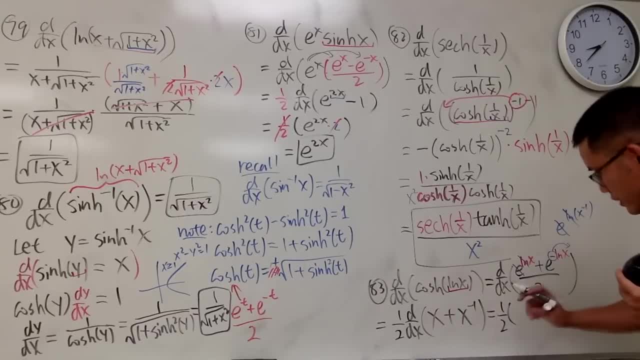 1 half all the way in the front. Put down the parentheses for the result of the derivative. Derivative of x with respect to x is 1.. Derivative of this is negative 1 over x squared And you can just get a. 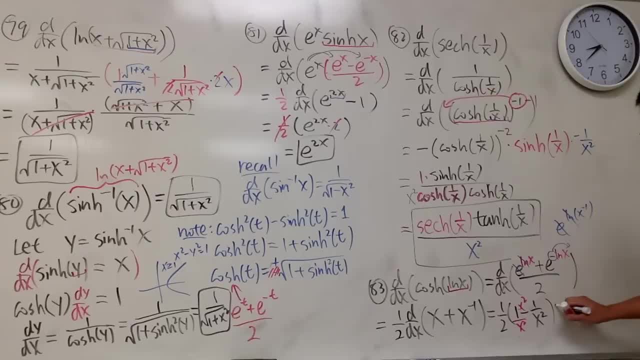 common denominator real quick. In the end we end up. let's see 2x squared on the bottom right And then this is x squared minus 1 times 1 is still x squared minus 1.. Like that, Whoa. 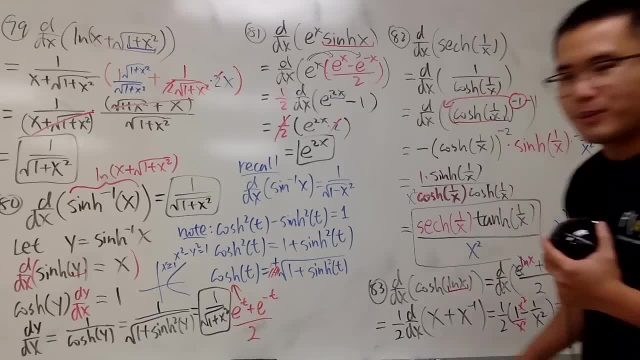 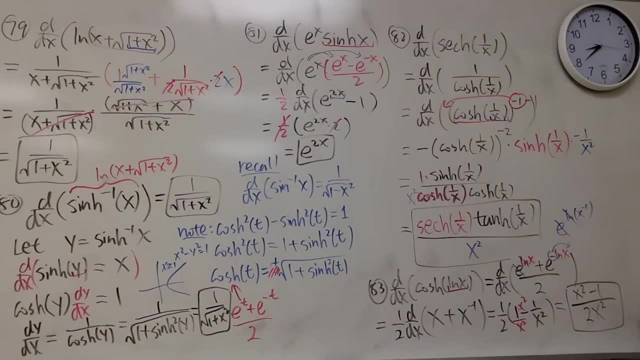 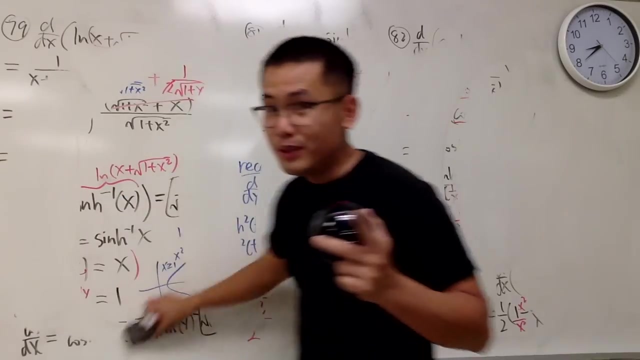 Look at that. I told you this should be able to fit in there. Let's just take a look, take a look, take a look. Okay, Let me know if you guys like the hyperbolic trig function more or the regular trig function. 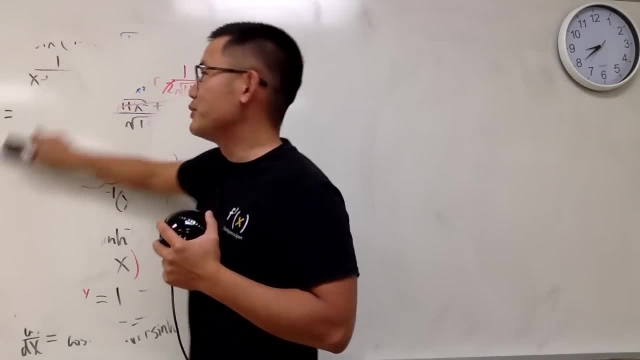 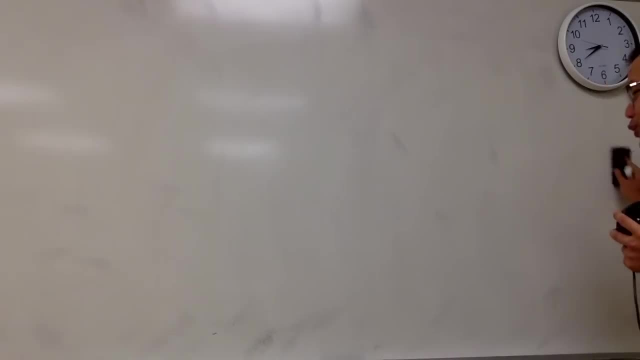 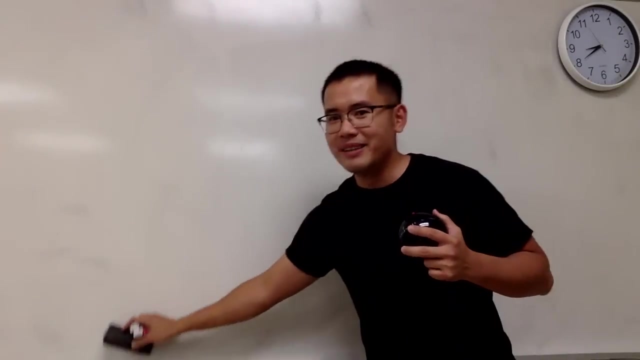 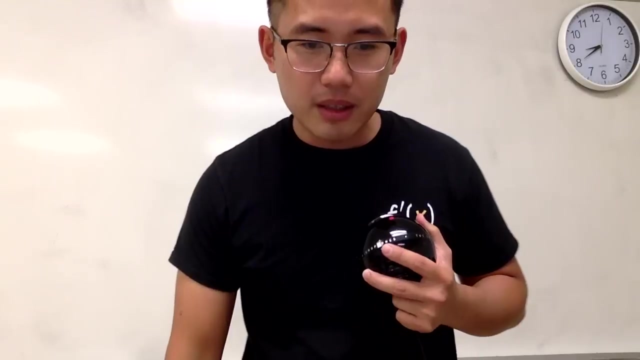 yeah, Yes, I will be doing 100 limits And I have a lot more ideas, but it also takes a lot of preparation and energy and also time And yeah, So I'll try to see if I can do them as soon as possible. 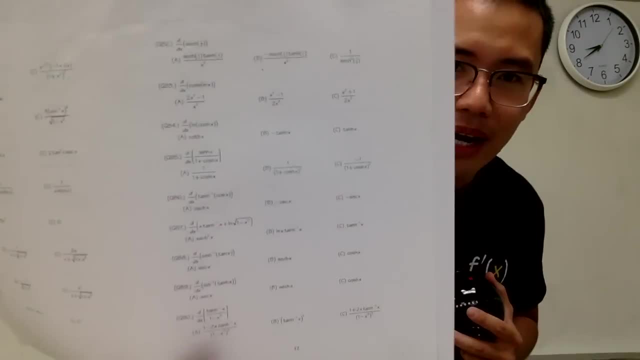 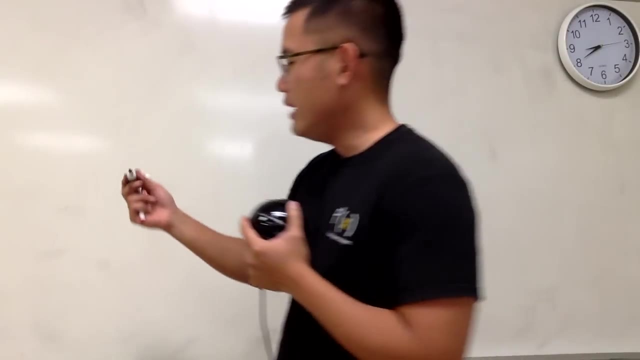 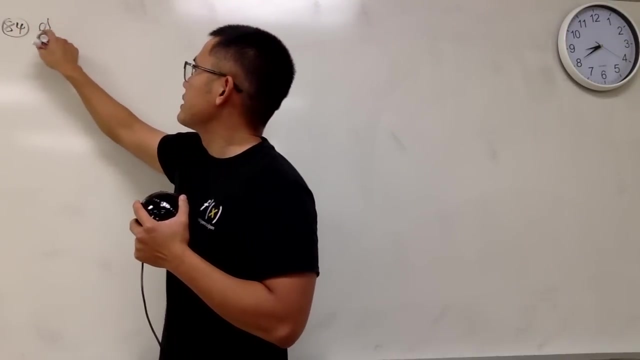 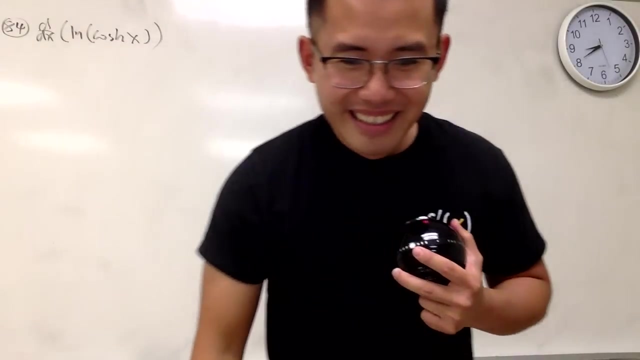 Number 84. I kid you not, I switched the natural log and also the cosh, You can see. okay, Yeah, So 84.. d dx of natural log of cosh of just x. All right, Go, cosh. 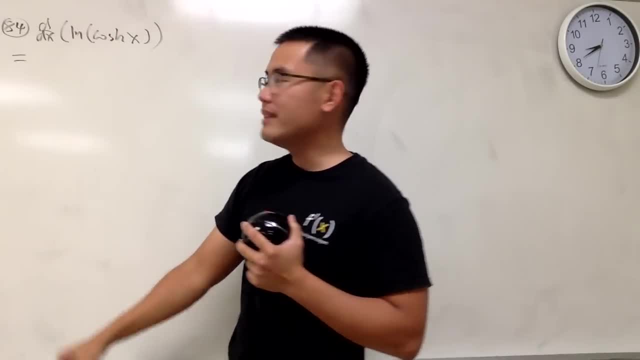 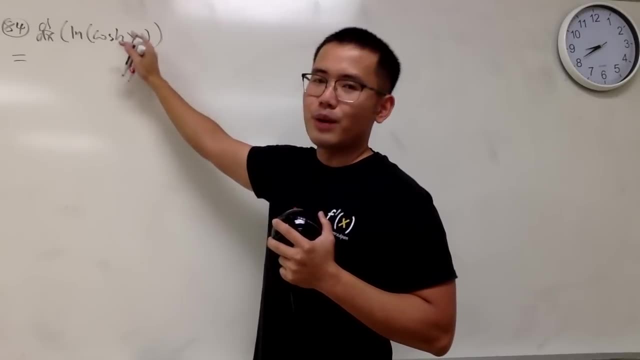 Okay, here we go. Natural log of whatever This one. we cannot do algebra in the sense that do not write it as e to the x plus whatever, whatever. all that Doesn't really help Check this out, though, Because we can actually just answer the. 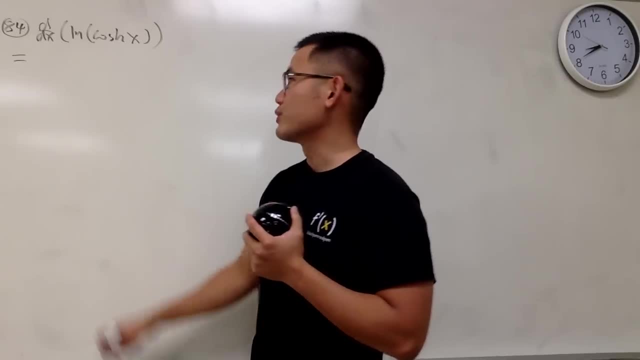 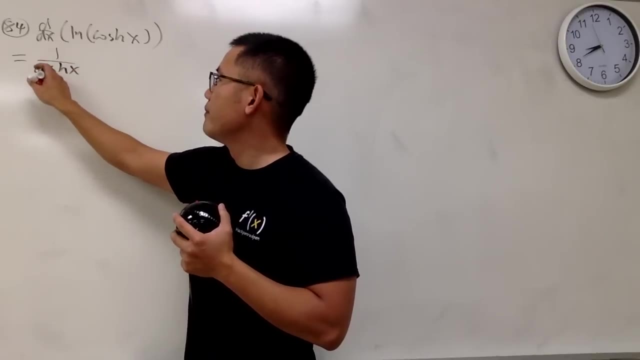 answer the question. in the hyperbolic trig function world Derivative natural of something is just 1 over 5.. But that is so. just write that down. Then take the derivative of the inside. Chengdu says so. Multiply by the derivative. 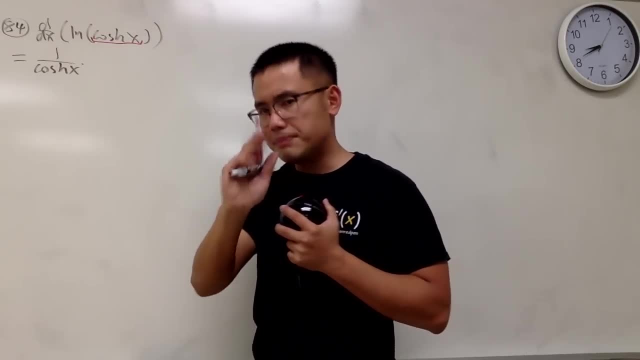 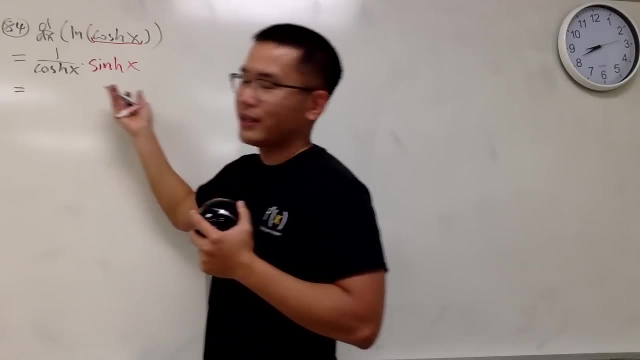 cosh is sinh And it's positive. So just multiply by sinh x. Guess what You're done, Because actually you're not done yet You can write this as sinh over cosh, which is tanh or hyperbolic tangent. 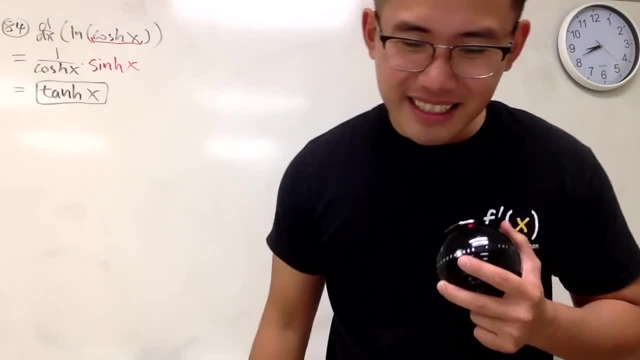 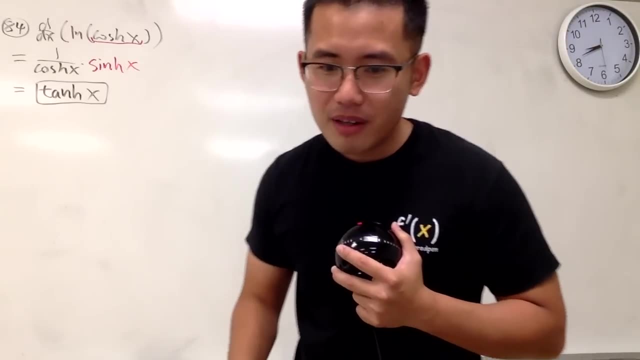 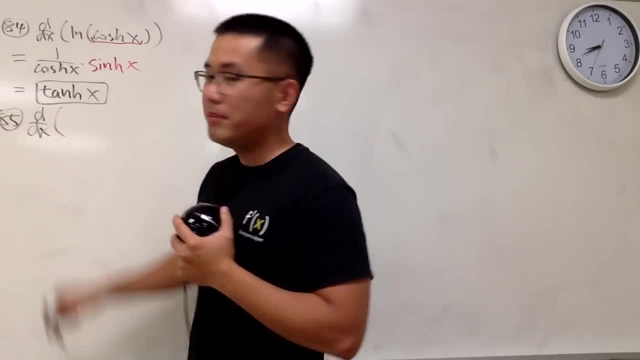 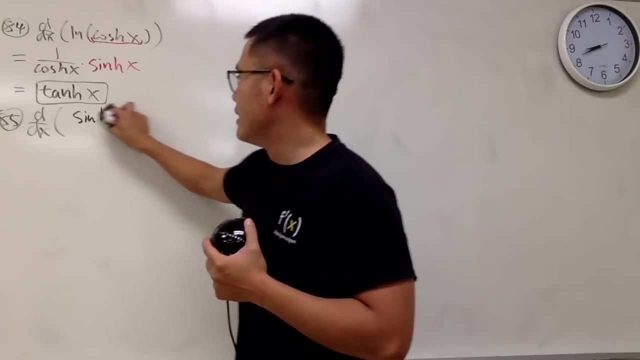 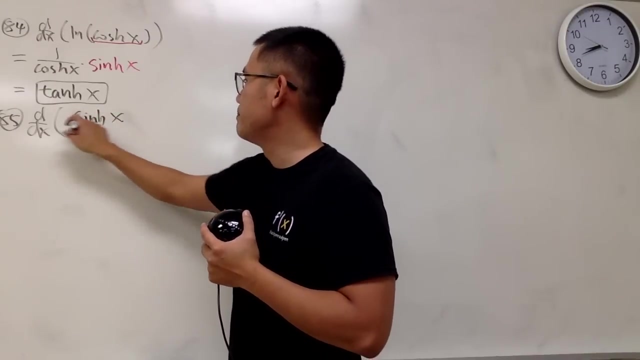 because I know the hard ones are coming. So, yeah, Anyway, sinh, oh man, You have to make sure the h is not too far apart from the sin, Otherwise it looks bad. So yeah, One plus. We did this version. 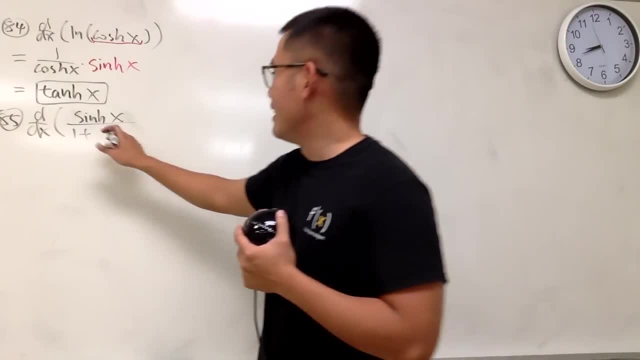 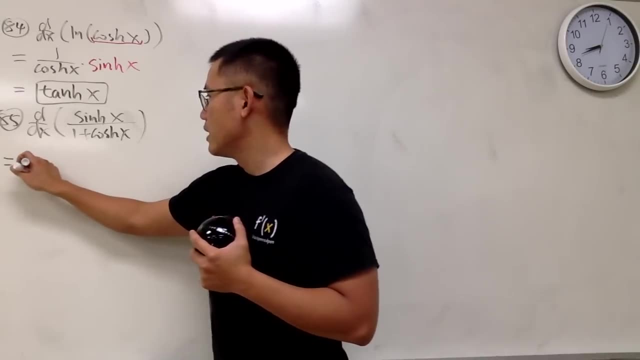 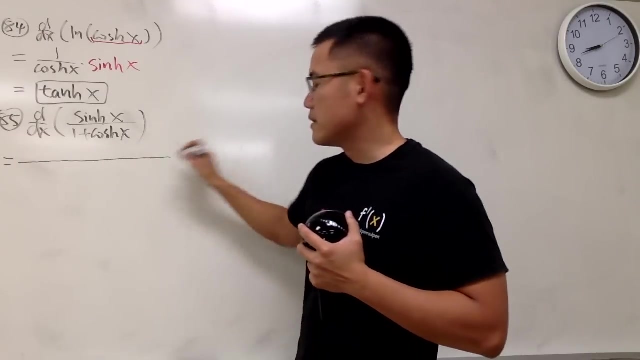 question number two: okay, Long time ago, But this is the hyperbolic version of the question. Here we go, Horrible, sorry. Okay, Here we go. Square the denominator, So put a parentheses and then with one plus. 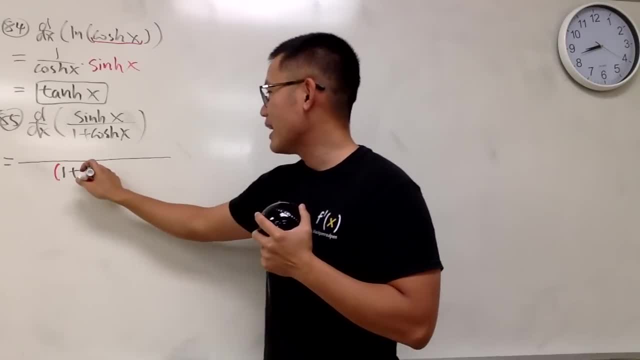 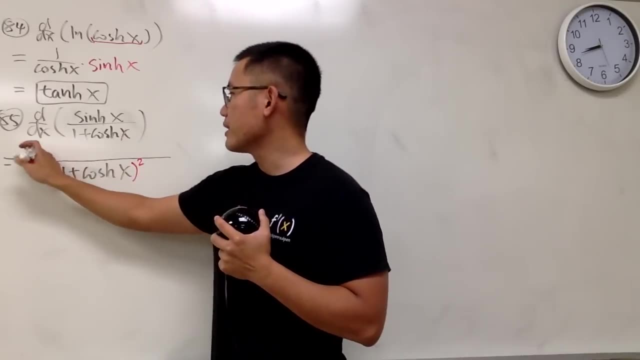 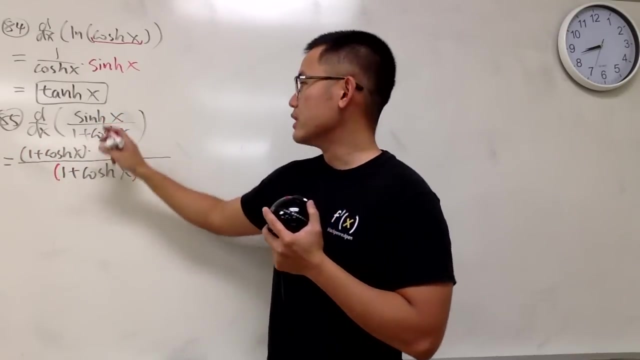 with one plus cosh x inside right Square that. And now on the top, you of course put on the denominator one plus cosh x times the derivative of the top Derivative. sinh x is just cosh x. 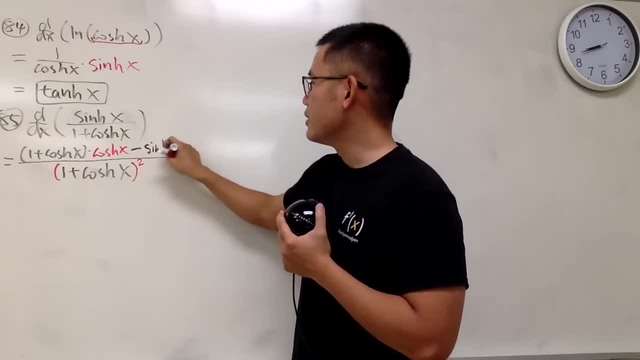 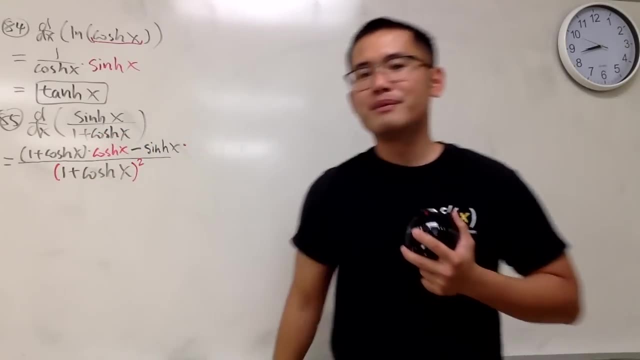 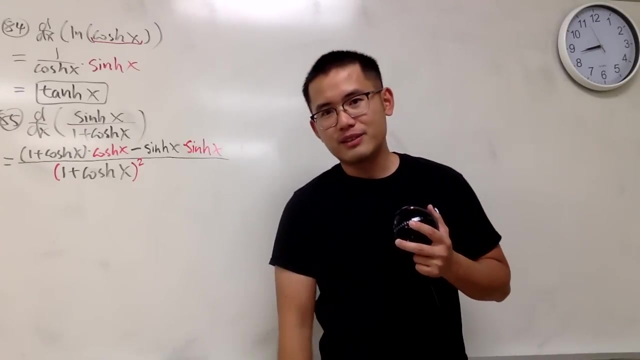 And then minus the top, which is sinh x Times the derivative of the bottom. The derivative of sinh x is positive sinh x. So you just multiply by sinh x. like this Can we expect some kind of cancellations? Well, watch to find out. 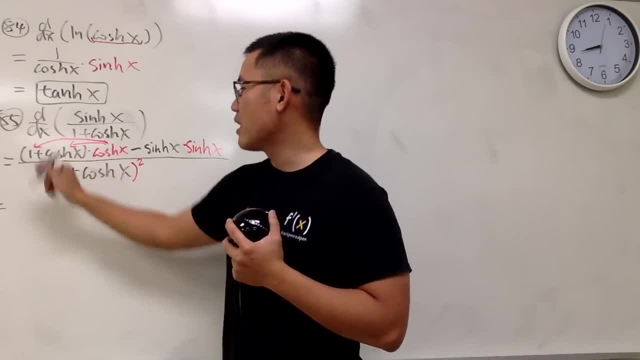 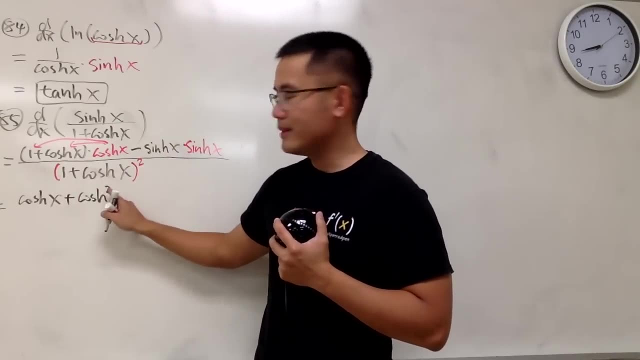 Here we continue, This times, this, this times, that cosh of x, This times that, of course, we write it as cosh square right, just like the trick function. you put a square right here of x. 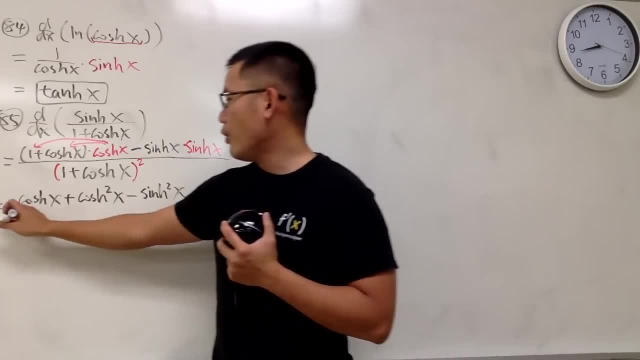 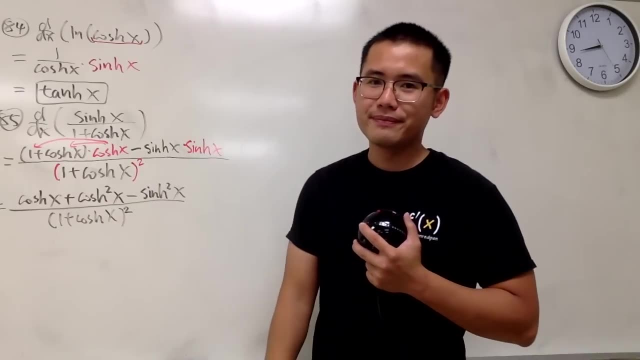 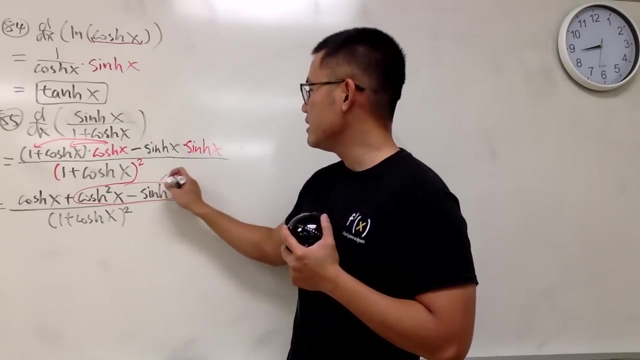 And then minus sinh, square x, all over this right here, parentheses, one plus cosh x and square that. Yes, very good, This right here. as I mentioned earlier, it's nicely equal to one And we just have one in that. 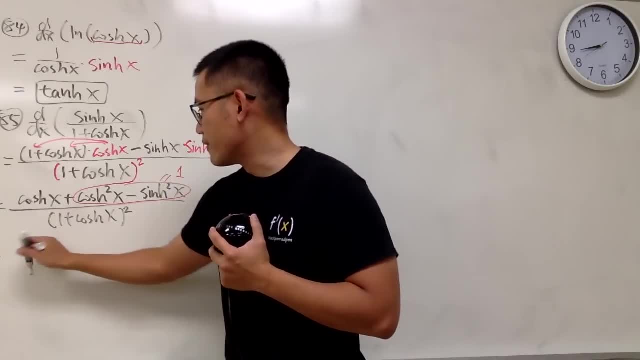 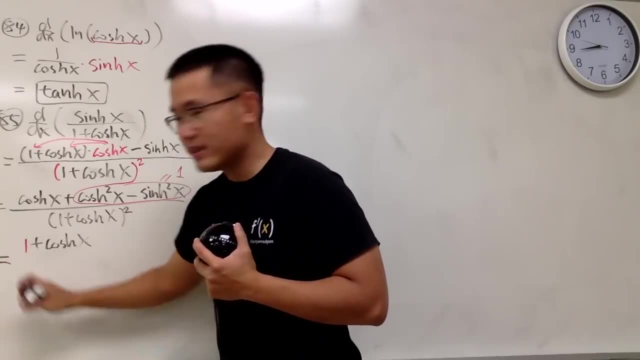 right. So you see, I can put down the one right here first, And this feels like deja vu, but it's not exactly. Anyway, this is equal to okay. this is equal sign you can see now over this guy. 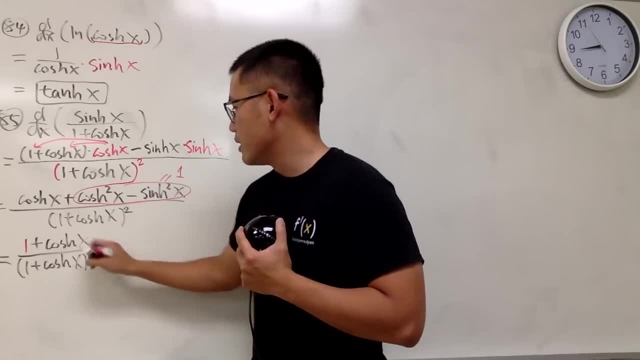 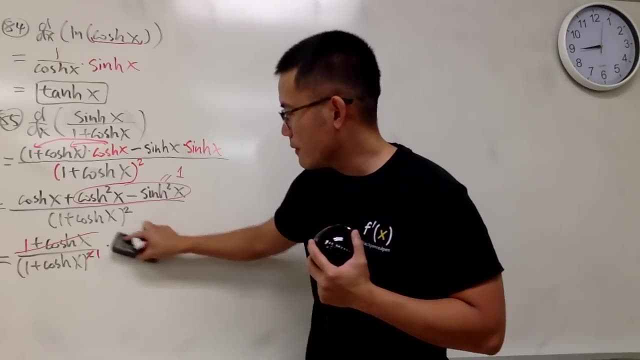 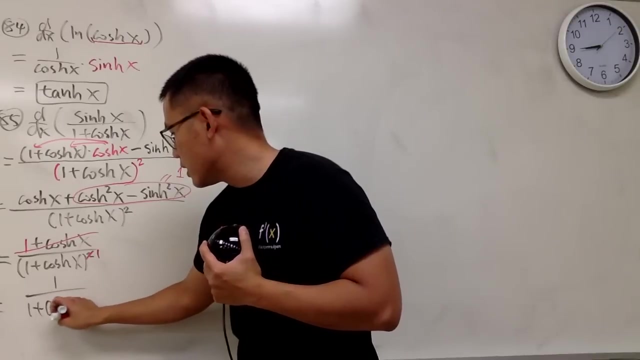 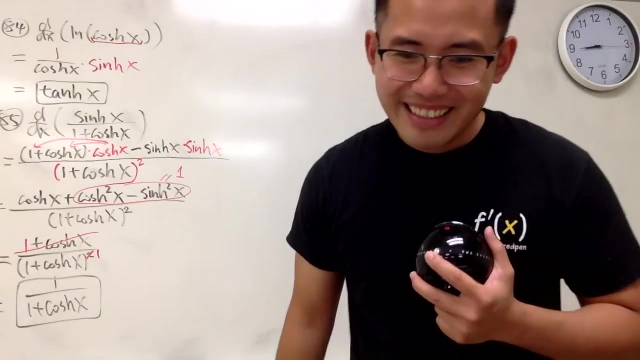 parentheses: one plus cosh x square. Cancel this, cancel one of that. So finally we get one over. finally we end up with just one over one plus cosh x, right here And we are done. Ah, number 86.. 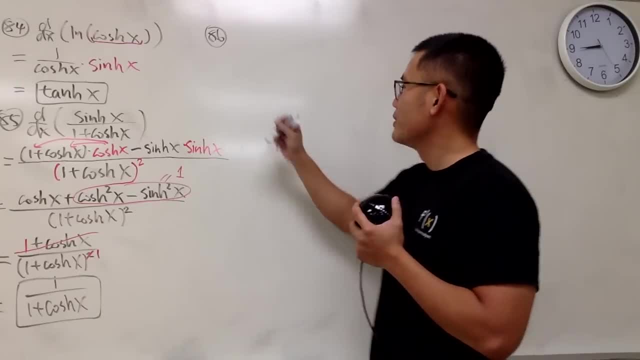 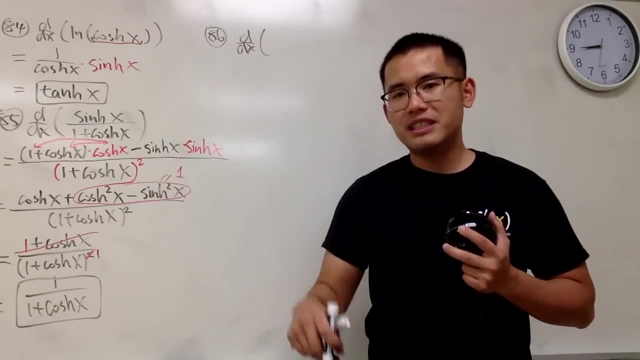 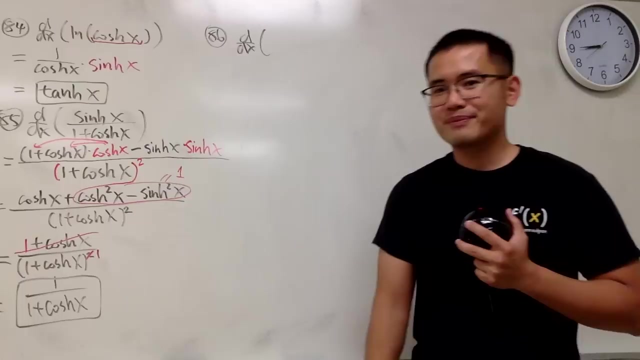 This is one of the my favorite one. So we are going to differentiate. Okay, derivative of secant is secant x times tangent x, But can you give me derivative of what function will give you secant x? In fact, we saw it. 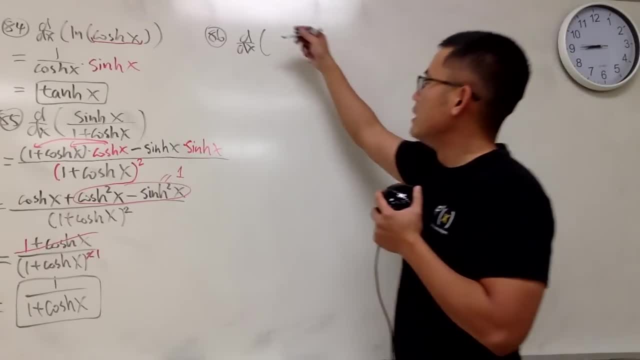 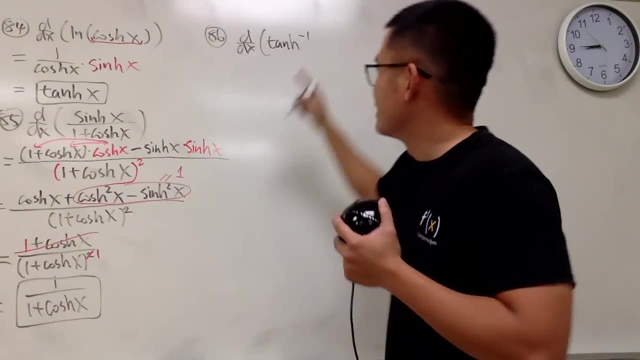 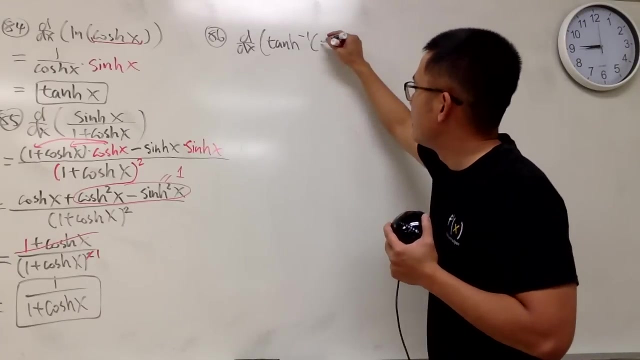 earlier, but we are going to see again right here, Differentiating inverse tangent, sorry, inverse hyperbolic tangent, and this is the inverse hyperbolic tangent of cosine. Okay, In fact I said it wrong. Derivative of cosecant. 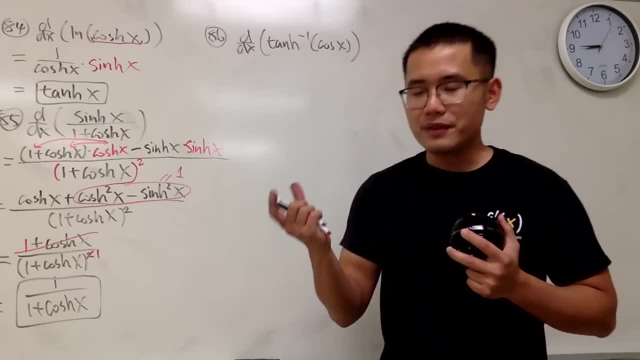 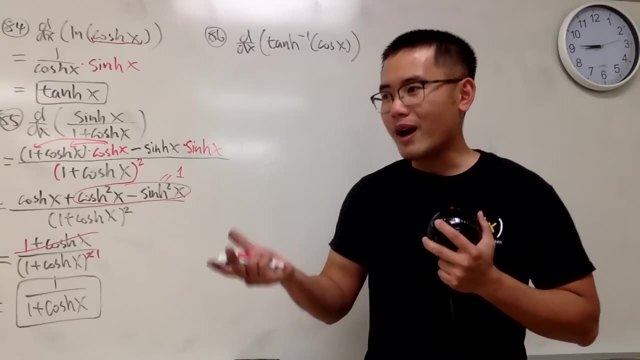 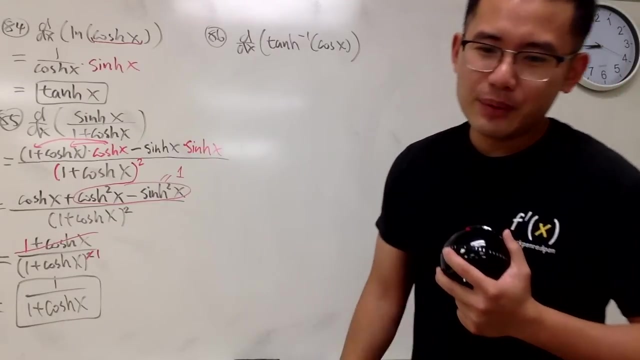 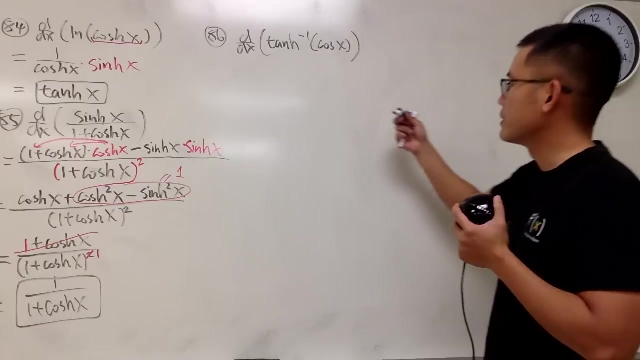 is equal to negative cosecant times, cotangent. But can you tell me derivative of what will give us cosecant, Or maybe a negative version of it? Watch to find out, Anyway, anyway, anyway, anyway. So this right here, I will just tell. 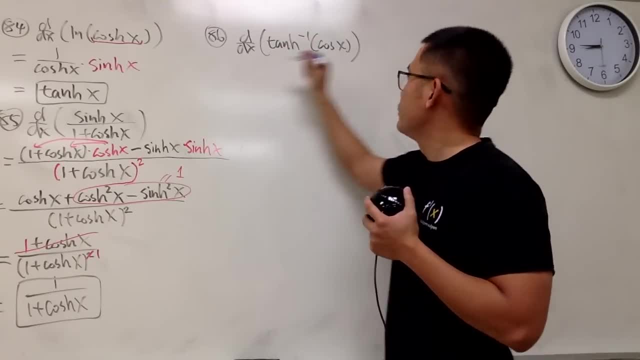 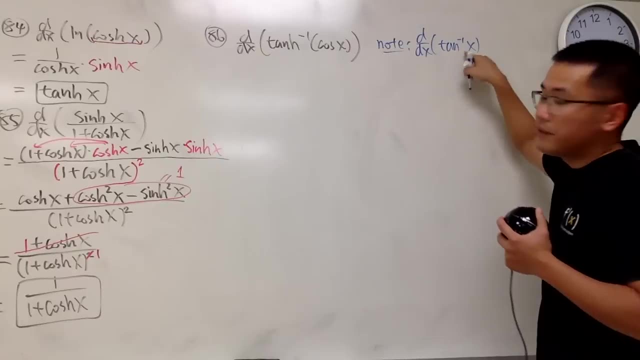 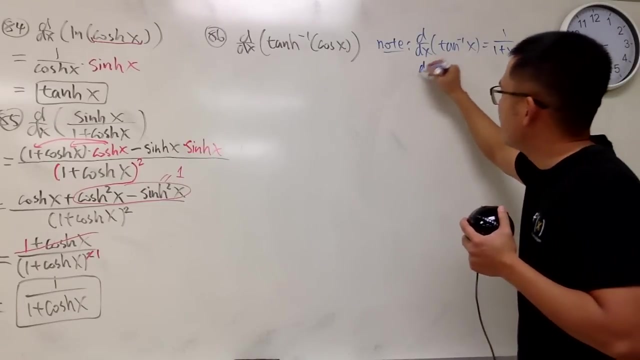 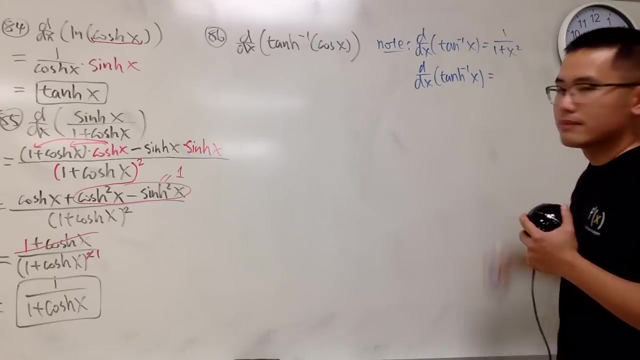 you guys, what the what the deal is? okay, In order to do this, okay, you will have to know the following. So here's some notes. on the side d dx of the Property derivative of the inverse hyperbolic tangent of: 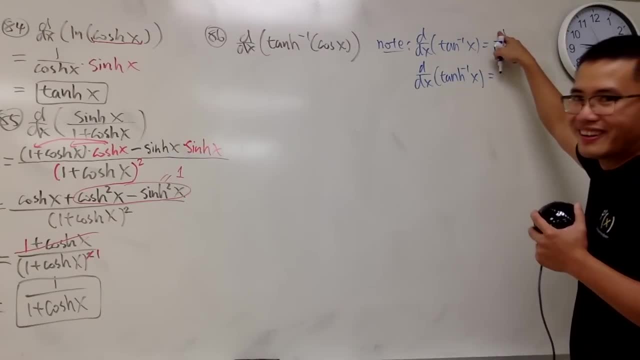 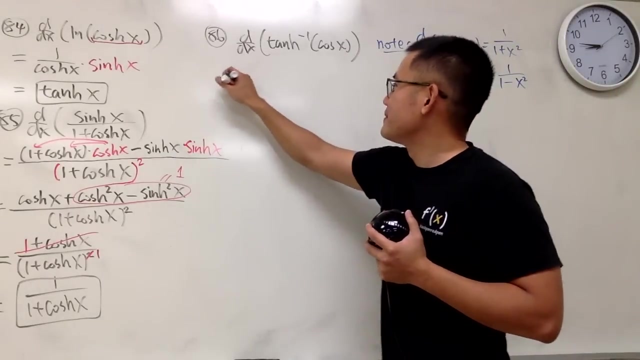 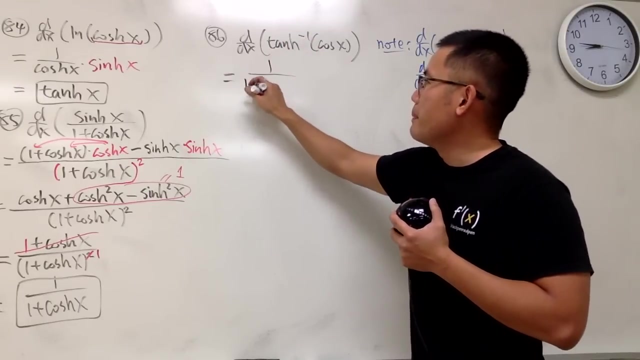 x is. No, It's not a negative sign. right here, That's inverse cotangent. that will do the work. This: right here: we gave 1 over, 1 minus x. squared like that tangent. you have to have 1 over, 1 minus. we will have to square this guy, so I will. 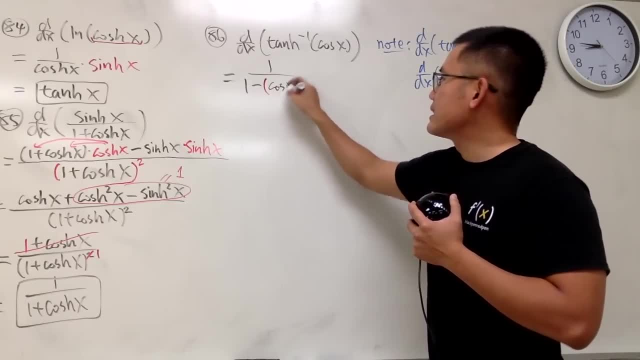 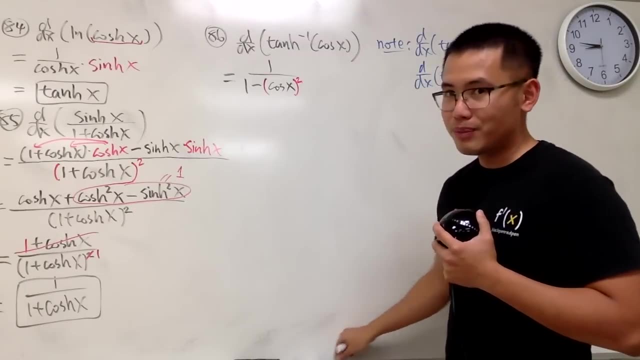 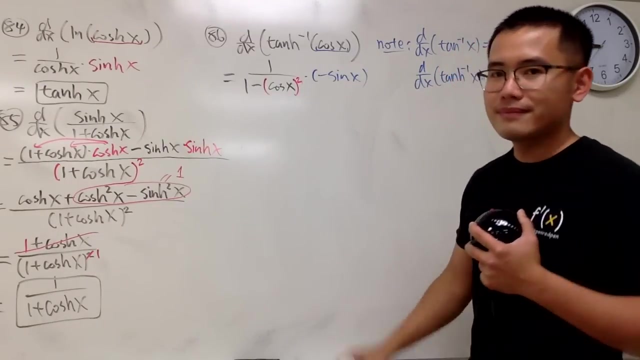 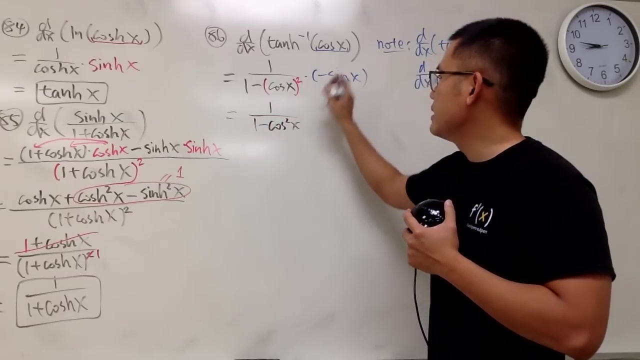 put a parenthesis with cosine x and square that. This is cosine x. okay, And we multiply by the derivative of the inside, which is negative sine x. Now check this out. This is just 1 over. this is 1 minus cosine square x, and perhaps I can put a negative sine x. 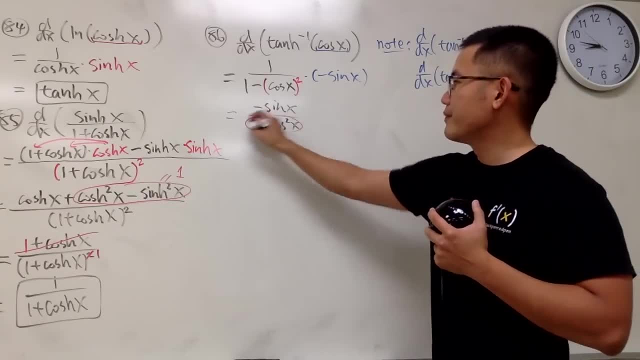 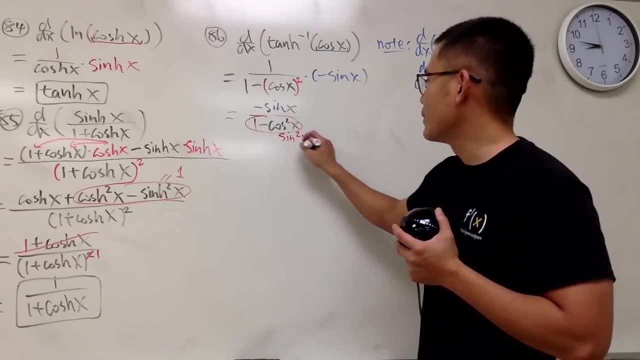 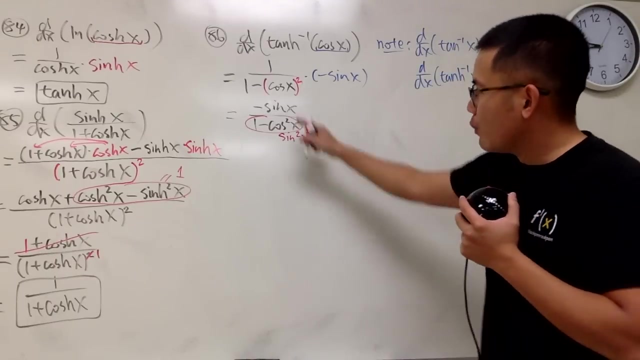 on the top like this: right. But what's this? We saw it earlier. This right here is just nice to equal to sine square x. right, This is just sine square x. 1 minus cosine square is 1.. 1 minus cosine square is sine square. What's on the top? Sine x. So can we just. 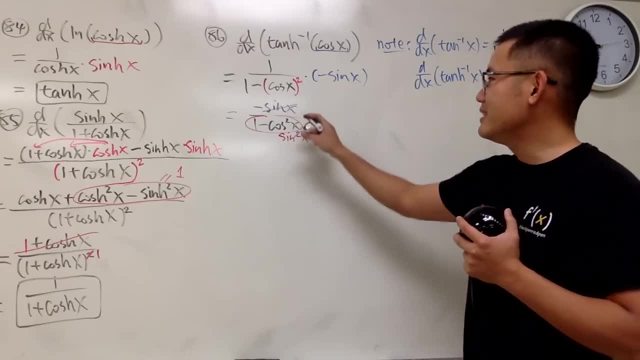 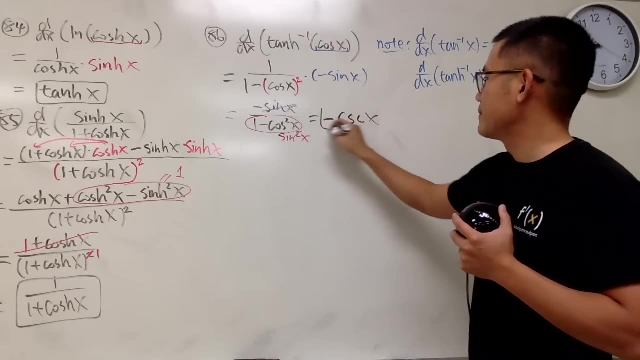 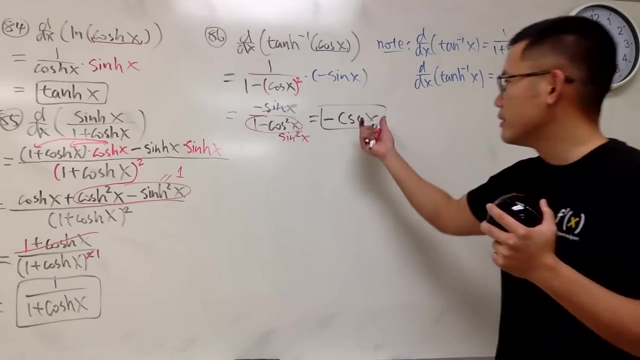 cancel, cancel, Cancel. Yeah, This is going to be negative 1 over sine x. In another word, we get negative cosecant x. So, in fact, if you want to find out the derivative of what will give you cosecant, 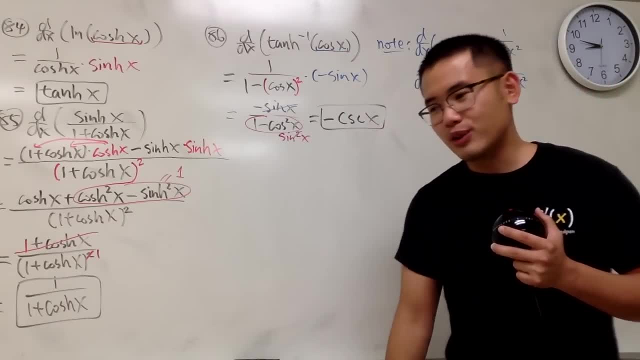 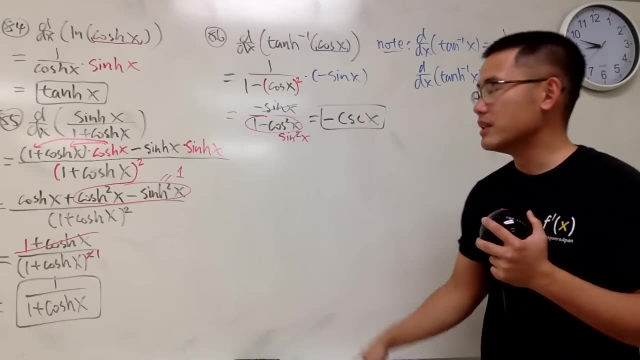 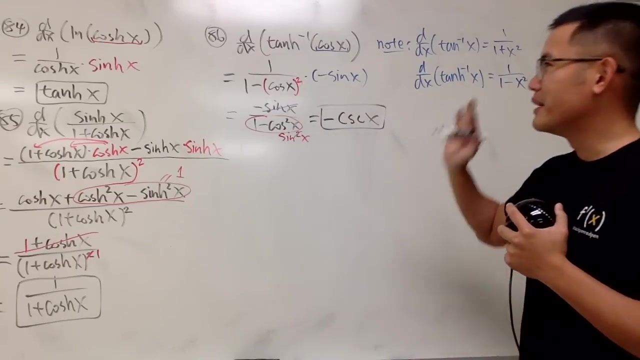 or secant. you can use the inverse hyperbolic tension to help you out. right, You can just have a think about what other things you have to do with this, so you can end up with the derivative. So again, this is just one way, right. You can do this one on the top, As it's a worshipped 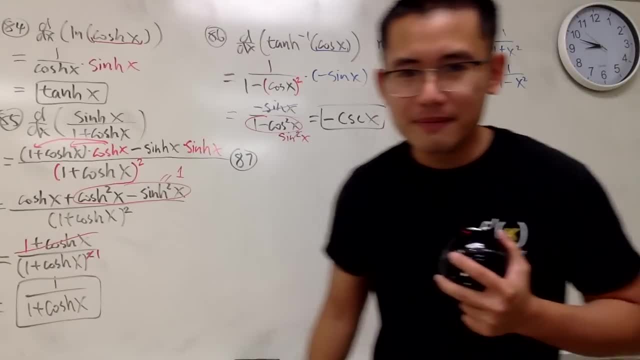 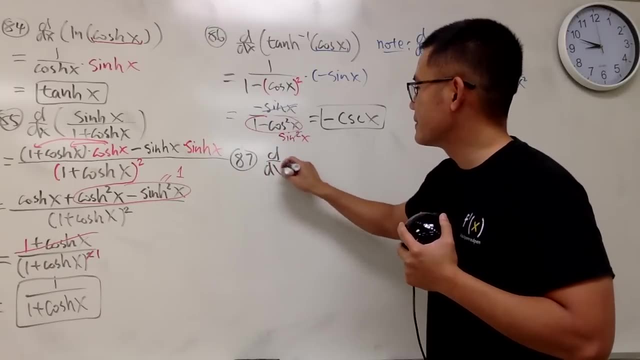 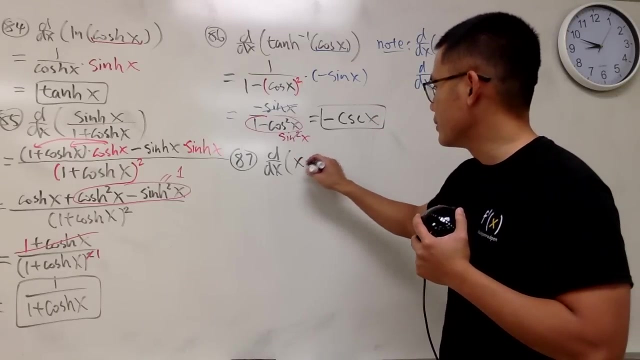 problem whether you use the perfect formula. whatever you use, it helps you out a lot. Okay, And this is the end of the answer. The answer is basically it's going to be a cosecant and maybe a negative version, just multiplied by negative. Anyway, that's the answer for. 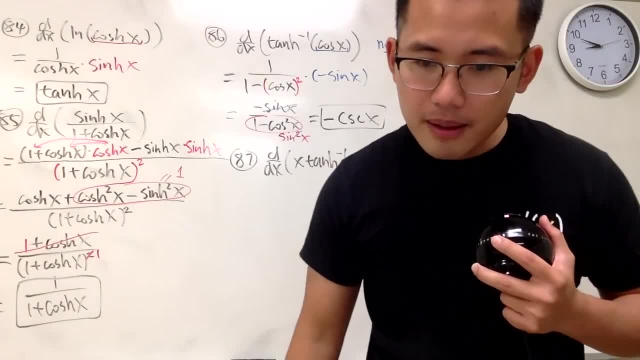 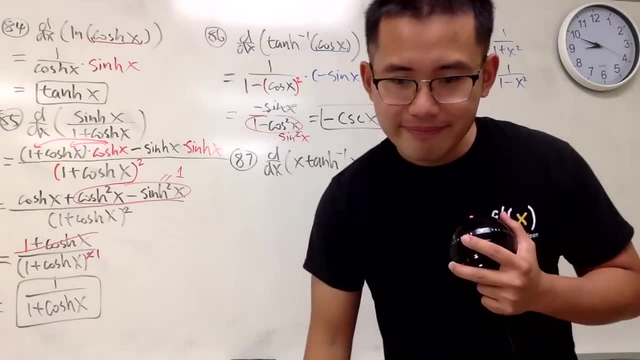 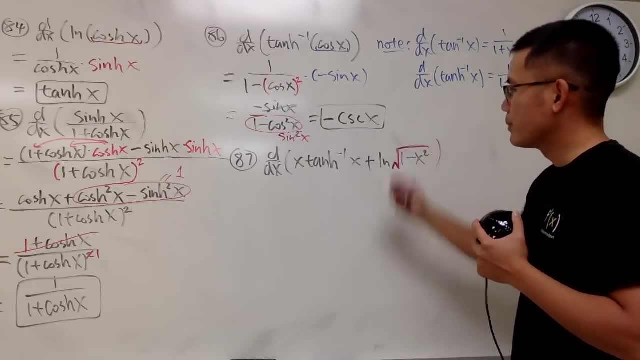 Well, you guys all know the deal. this right here is the 1 half power, so I put that all the way, not all the way, please, right here, right. So I will just change that for you guys. 1 half natural log of this guy. 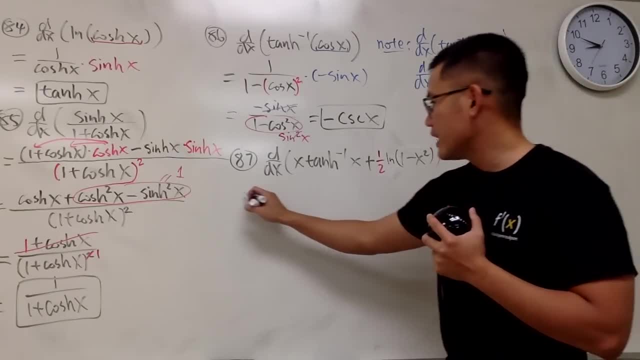 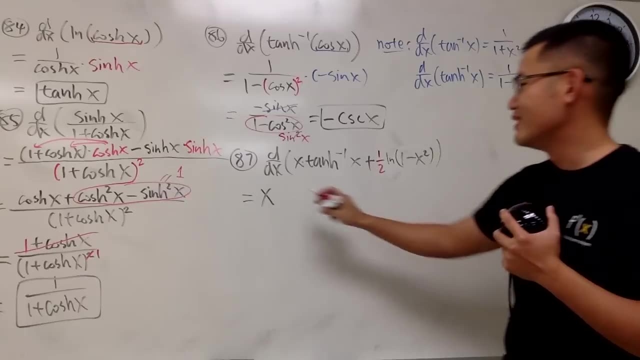 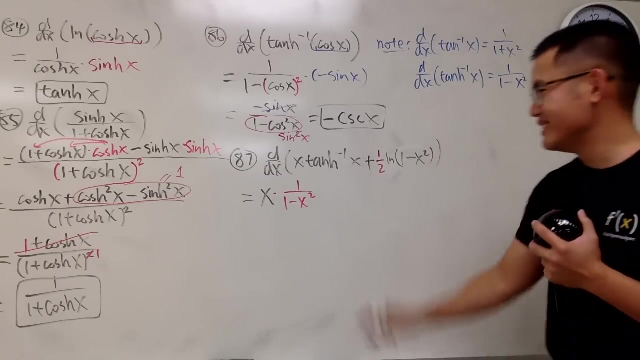 And now let's get to work Here. let's do your product right here: x times the derivative of the second. it's right here. so we multiply by 1 over 1 minus x squared. Chen Lu says you have to multiply by 1, but you know you don't have to. 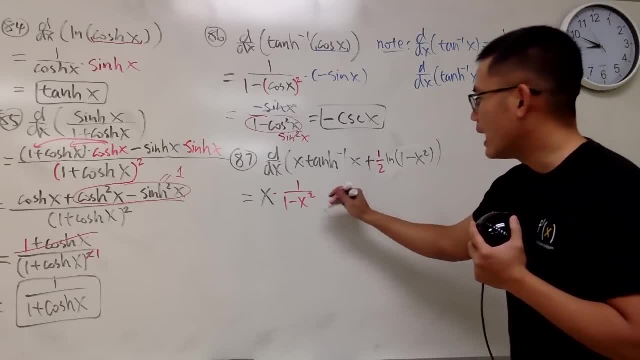 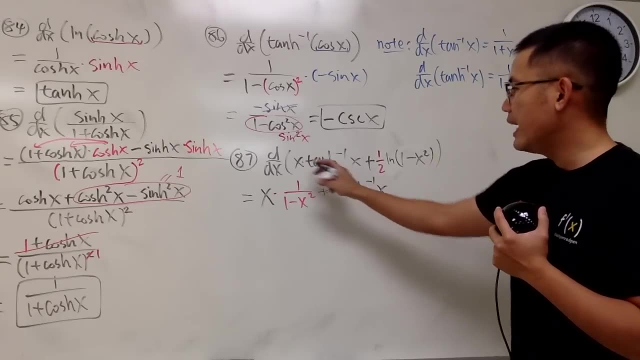 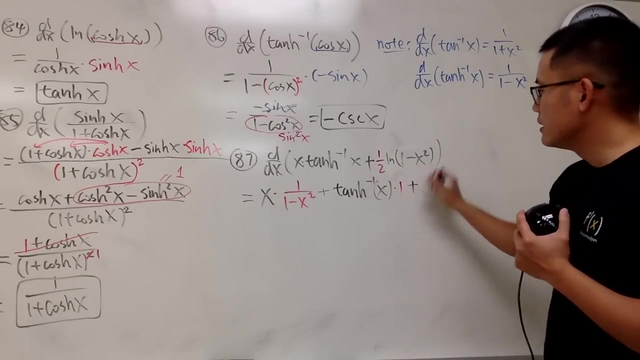 1 multiplied by 1, doesn't matter. And then you add second function, which is inverse hyperbolic tangent of x, and you multiply by the derivative of the first, which is just 1.. So that's what we have Now. we add the derivative of this part. this is just 1 half. 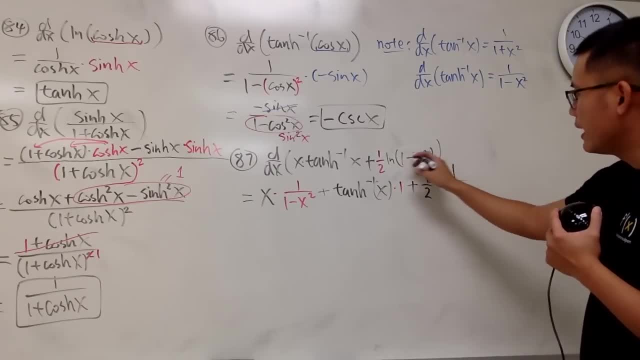 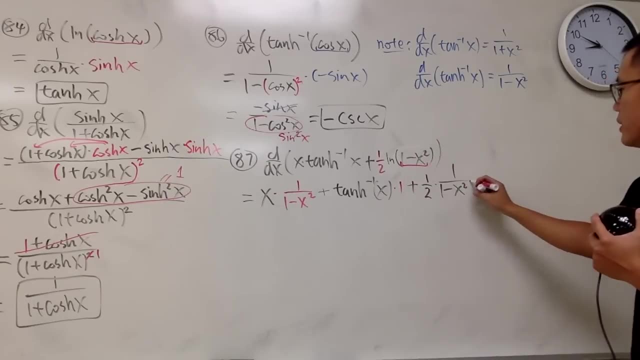 times the natural log will give you 1 over and you put the inside in the denominator and Chen Lu says: multiply by the derivative right here, which is negative 2x. just like that. This and that again cancel out. 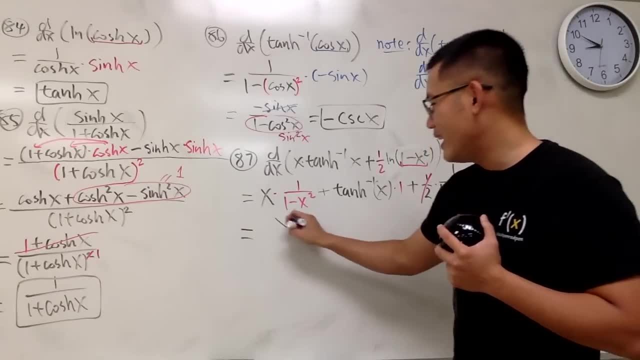 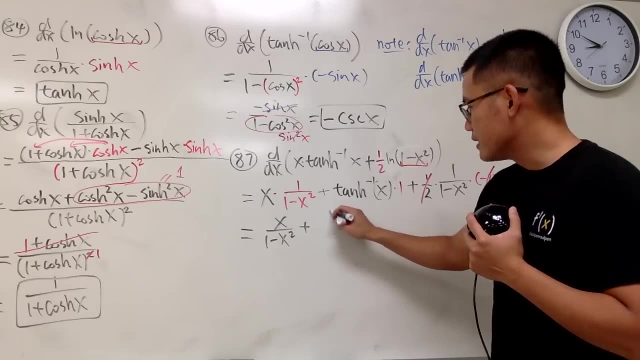 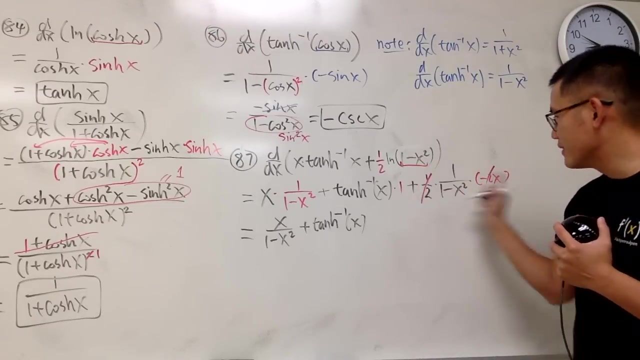 You guys will see why I say again This right here: x over 1, minus x squared. This right here, plus inverse hyperbolic tangent of x, This right here is negative, though Negative okay. So, minus x over 1, minus x squared. 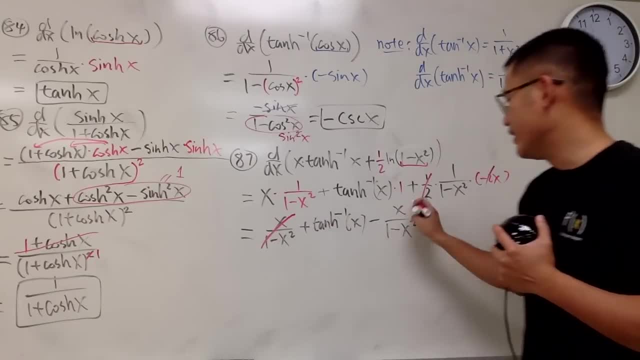 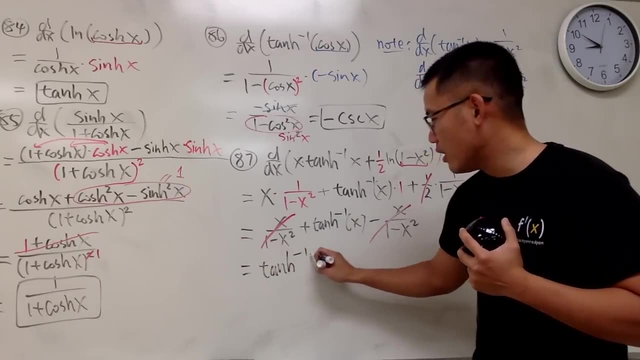 This is positive, This is negative. Of course, they can say bye-bye to each other. Finally, we end up with the inverse hyperbolic tangent of x And this, right here, is your nice x And this, right here, is your nice x. 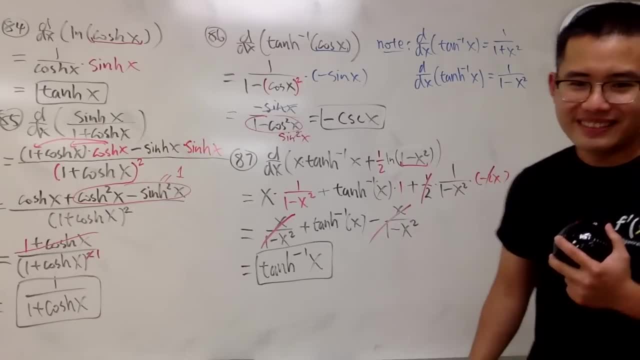 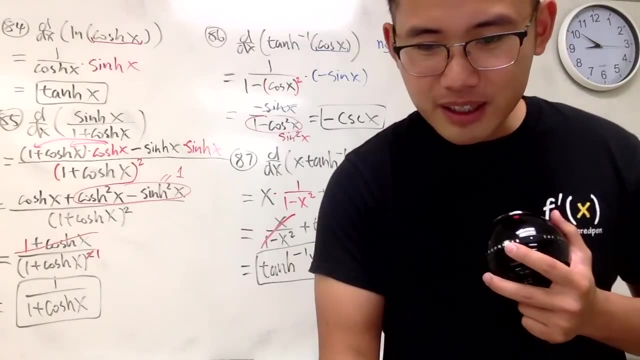 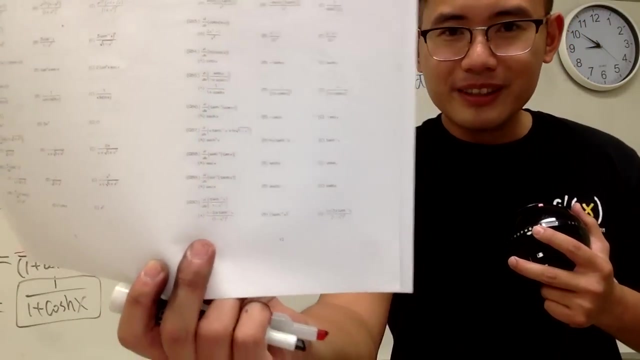 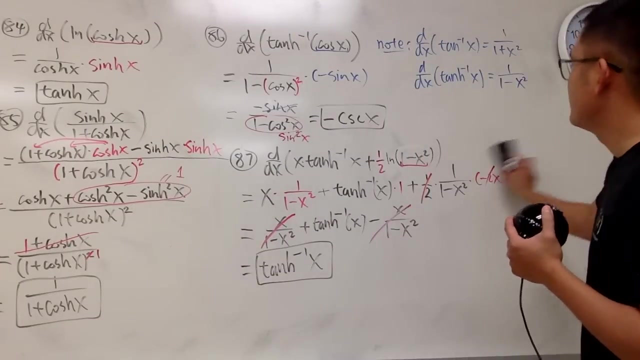 And this right here is your nice x, very, very nice, similar looking than the regular inverse tangent X. we did that earlier as well. okay, I am going to do the next two side-by-side. which one? I'm gonna do the next two side-by-side. so I will have to erase the board and again. 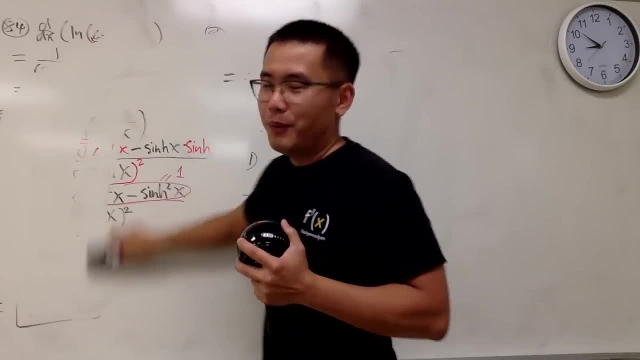 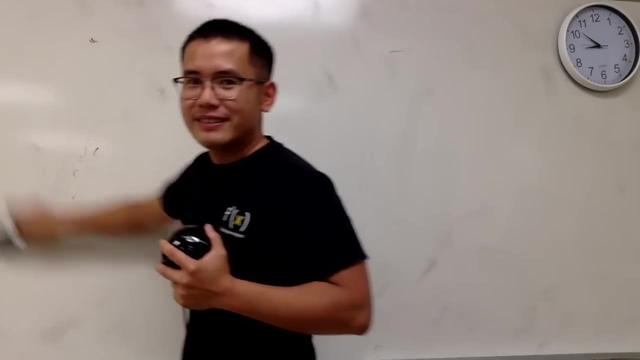 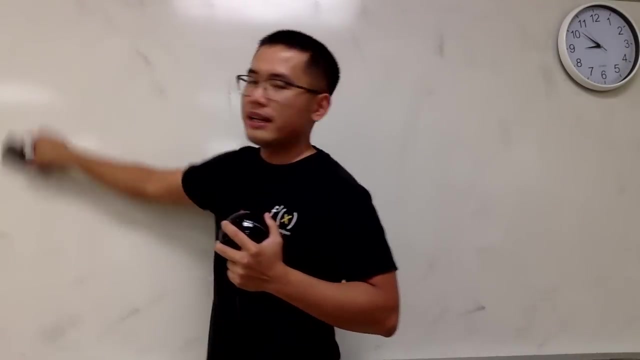 I'm not so happy because, well, I'm kind of happy because it's almost done, but like the hard ones are coming, so I'm not exactly like super, super happy. this is like I don't know whoever decides the course. they put like uphill at the finish line and that that's. that's really mean. okay, I would rather have the. 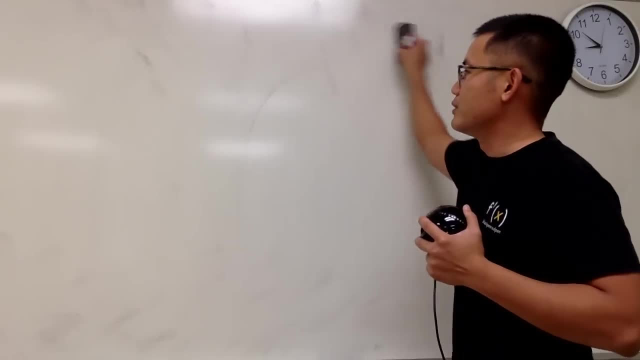 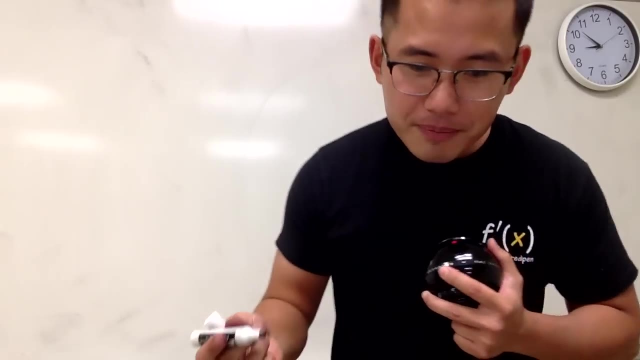 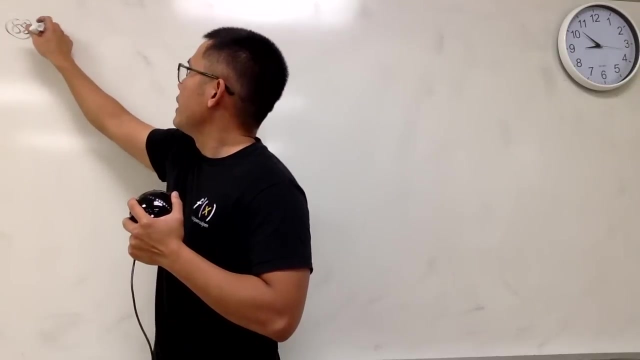 uphill than the first three mile or so and just just have it done with it. yeah, if you run, you know what I'm talking about. anyway, number 88: I'll put it down right here. okay, here we go, the DX. we are going to be differentiating. 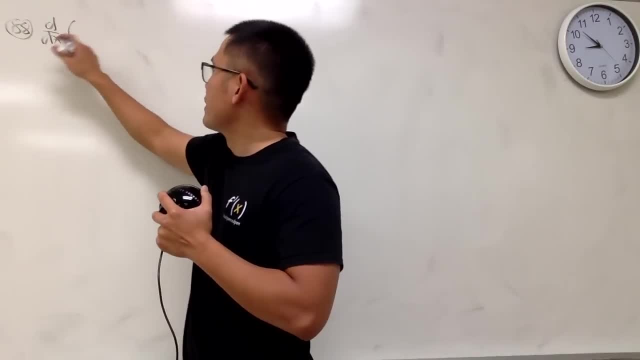 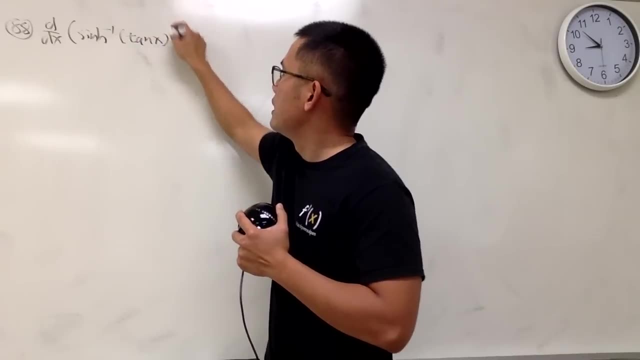 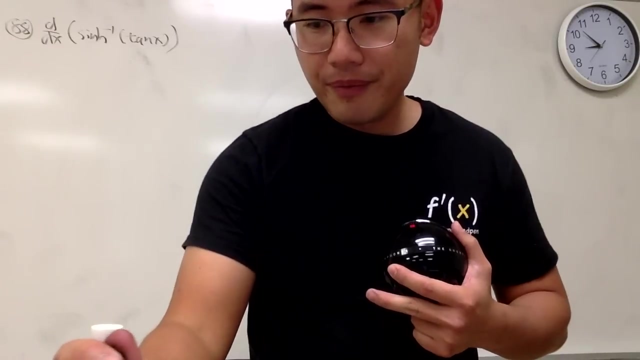 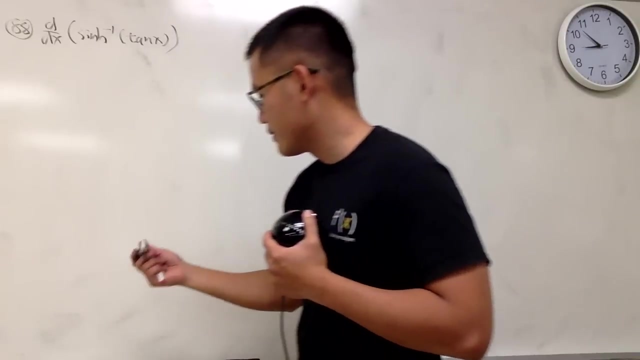 inverse cinch. okay, the first one right here is inverse cinch and the input is tangent X. okay, I am going to just treat myself better. I will have to. I would like to have a better marker right here so I can feel the writing experience is better, so I will use this one much better, okay, so 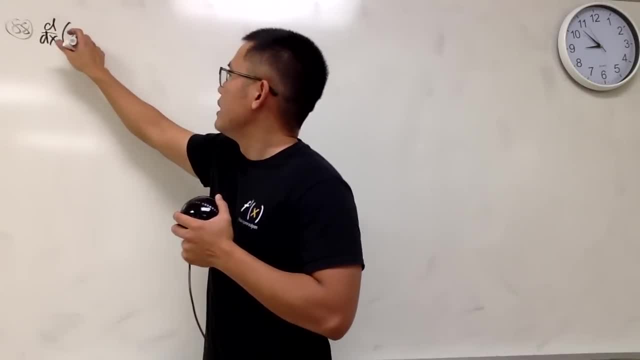 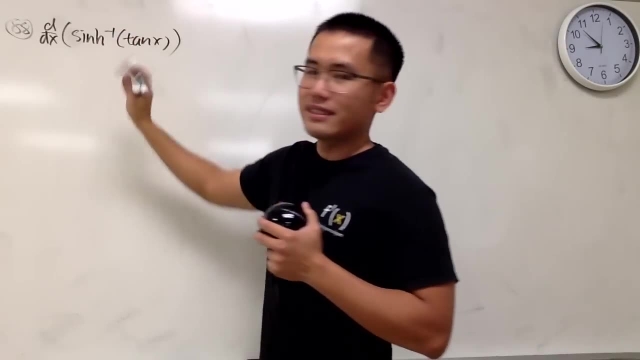 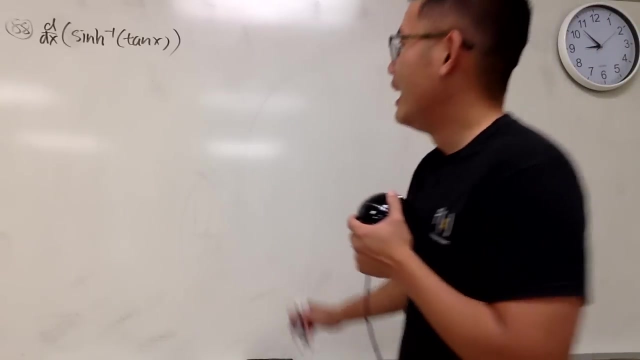 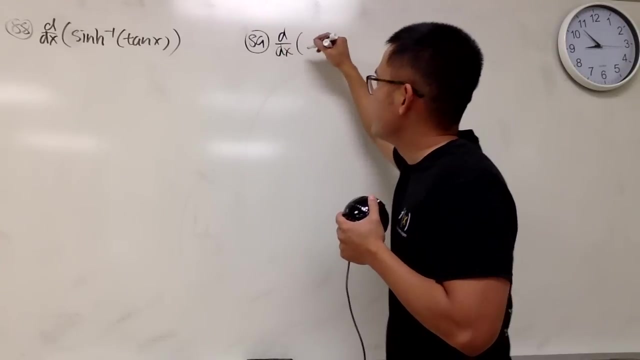 number 88: the DX inverse cinch of regular tangent X like this: yeah, hyperbolic together with the regular. so you are going to see what's going to happen and on the contrary, on the other hand, I'll say number 89. we will differentiate the regular sign of 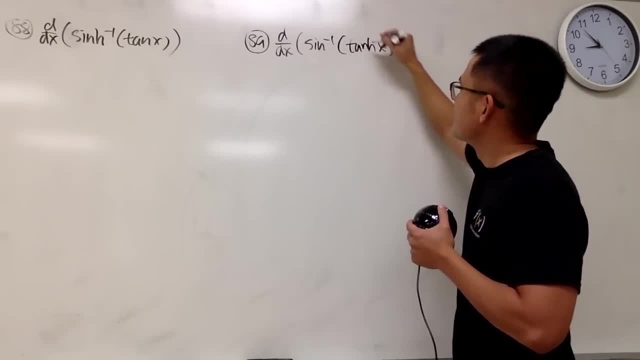 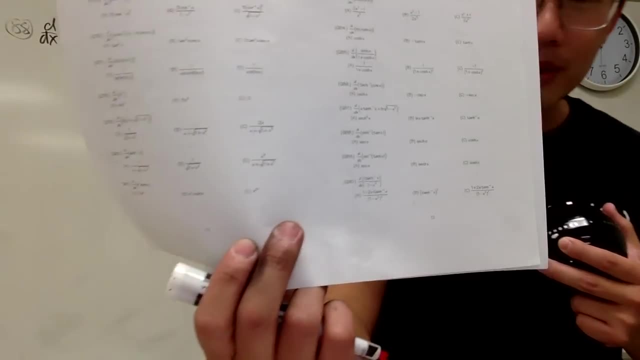 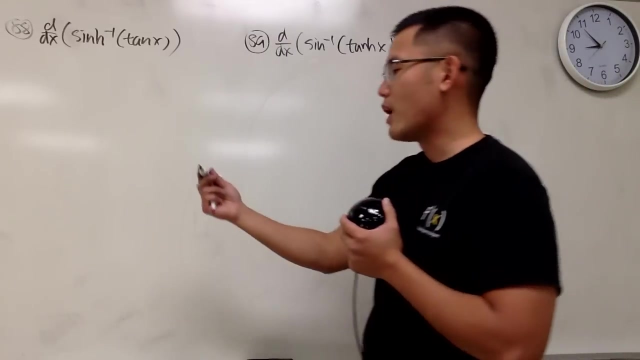 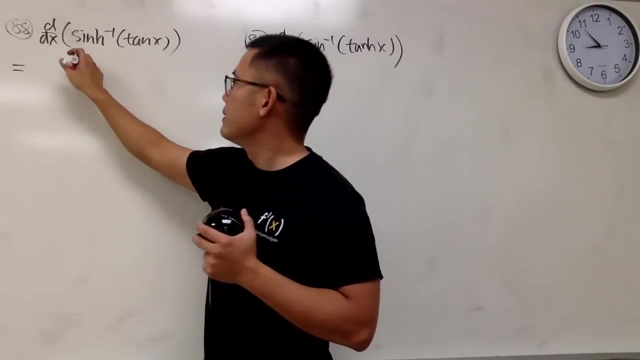 hyperbolic tangent X. whoo, what in the world is happening? huh. so again, I'm just looking at the questions. I just want to make sure that I wrote down the correct question. now start with this one. here we go: inverse cinch is 1 over square root of 1, plus it is plus, okay. and then you put: 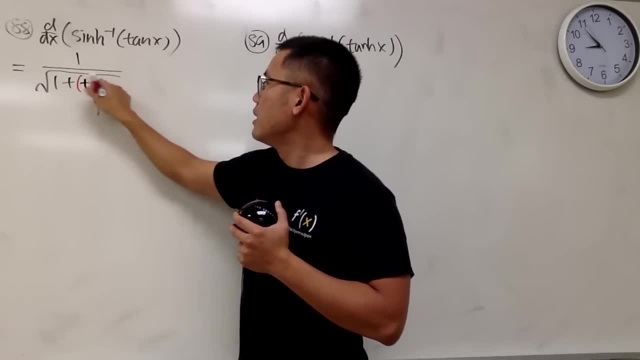 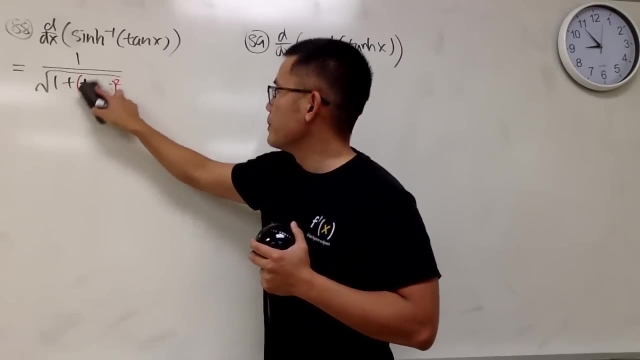 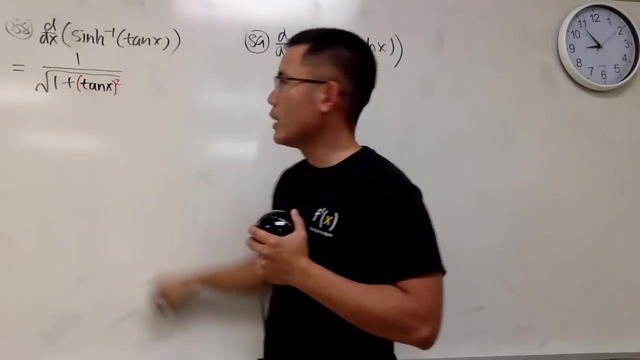 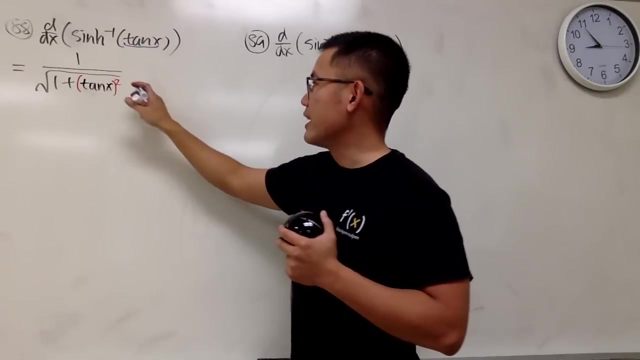 this right here and you square that, so tangent square. and then what else do we do? whether we write it right down, the tangent X better. and what else do we do? we multiply by the derivative of the inside- Chen Du says so- derivative of tangent X. this is a regular tangent X. we get regular. 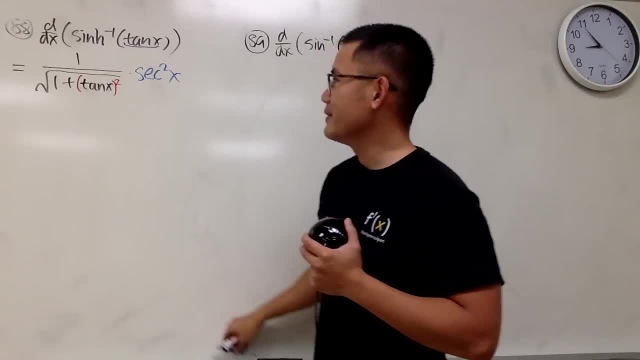 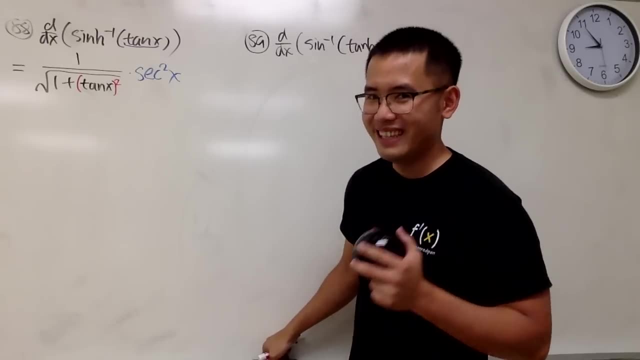 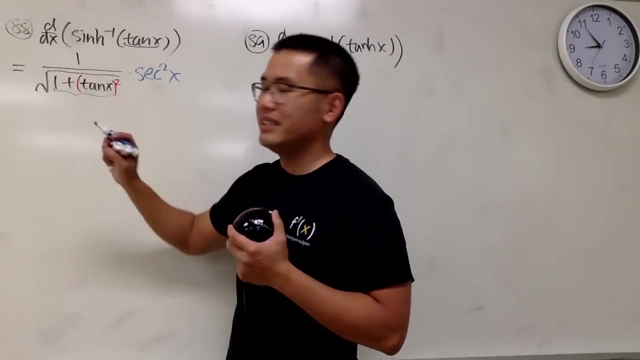 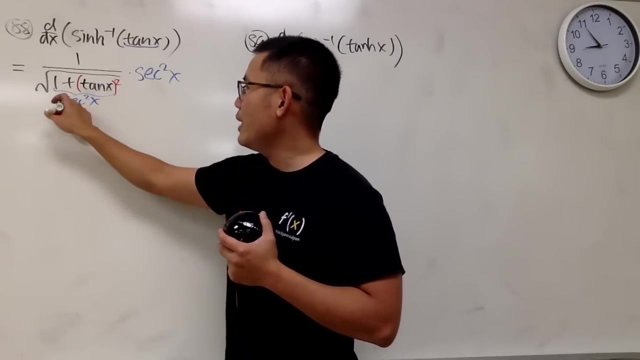 secant square X. okay, so it's just like that. okay, this is good, but is there anything that we can simplify? yes, because 1 plus tangent square- this right here- is nice- the equal to secant square as well. so you are looking at the square root of. 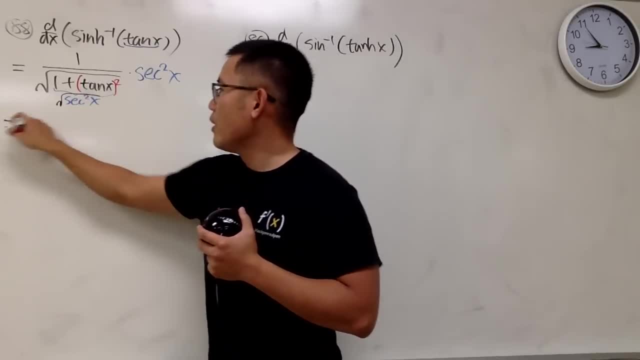 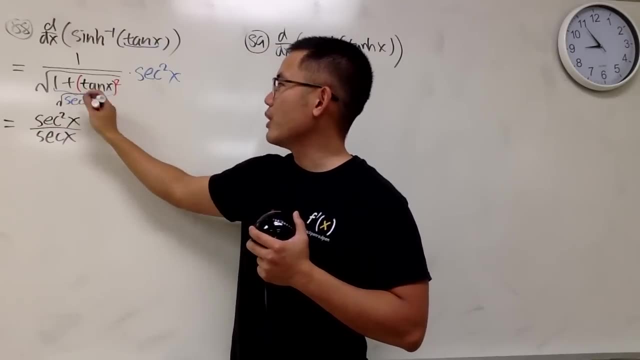 that which is just a secant X in the denominator. on all you just have secant square X over secant to the first pole X right after you take the square root and also this the square, they cancel and of course we just try not to deal with the. 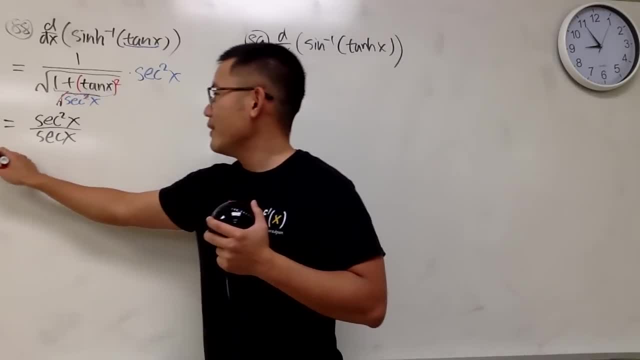 absolute for you, don't worry about it. whenever you do things happen. but now I'm going to show you how to do it. for now, I'm going to show you how to do it. for now I'm going to show you how to do it. 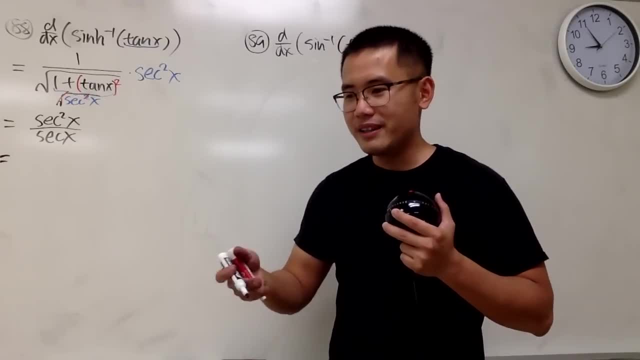 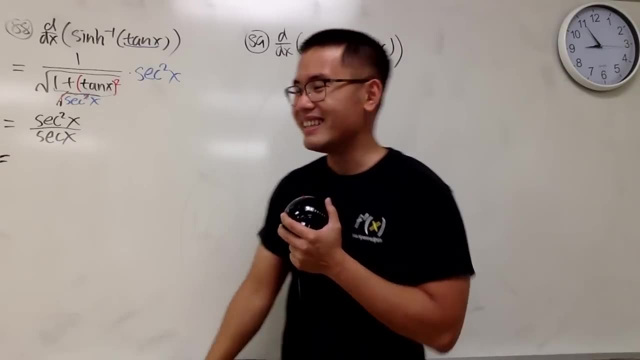 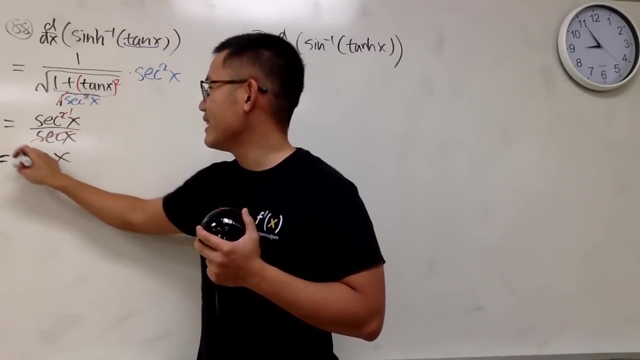 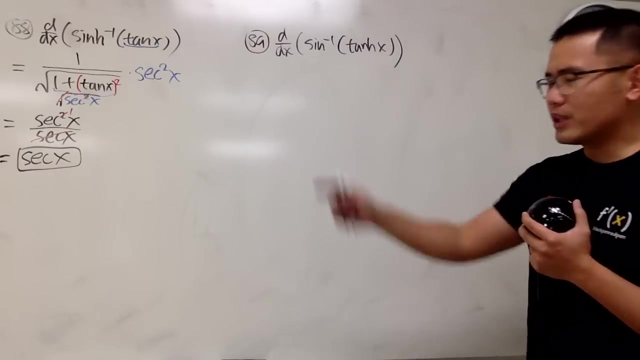 you have found to be more technical. you had to get the actual domain and also the X values that you are talking about on this one anyway, this and that cancel one of them out and you end up with what? secant X. the root of this would actually give you secant X. we have solved, we have seen the root of some function. 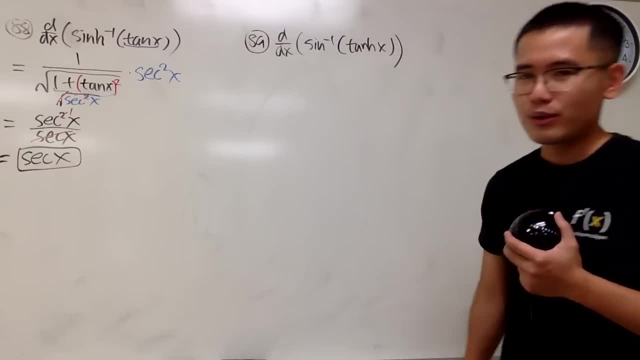 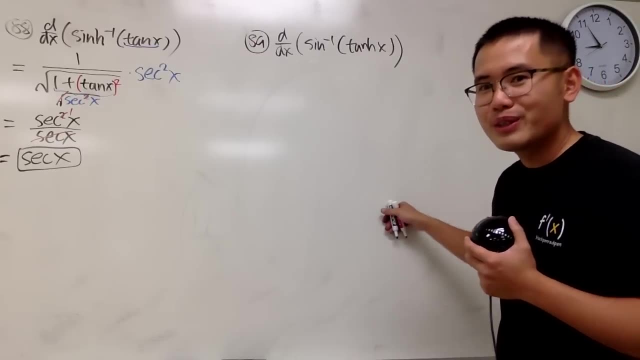 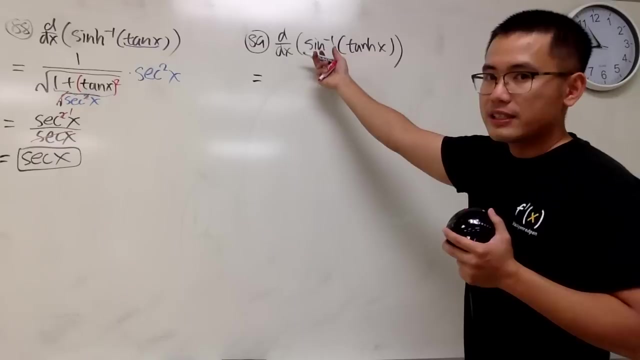 will give us secant X earlier as well, like I don't know how many hours ago, but yeah anyway. let's take a look of number 89. take a guess what the answer is. okay, we'll see. okay, this is the regular inverse sign. so we get 1 over square root. 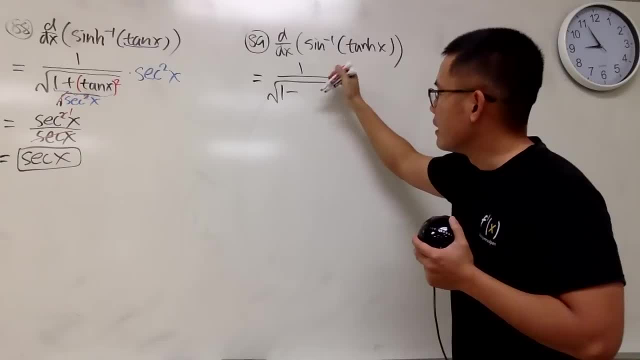 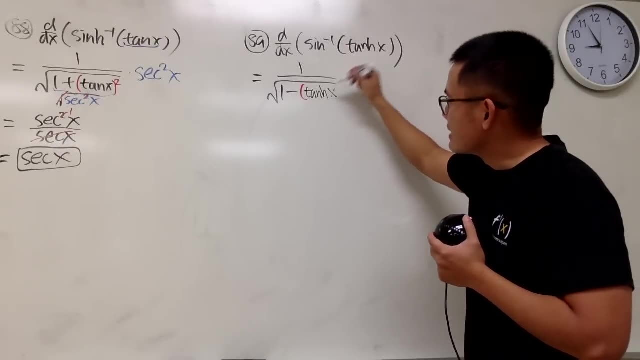 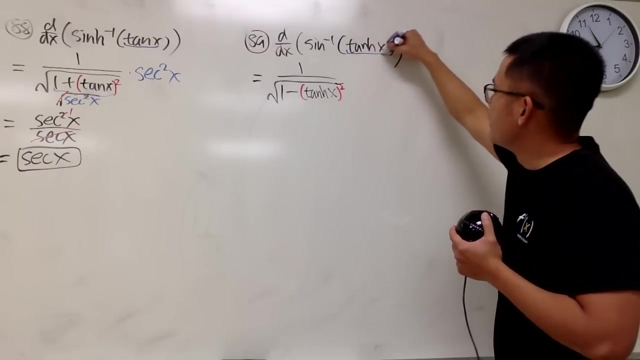 1 minus this. right here we have the parentheses with tangent, with H, so it's a hyperbolic tangent. okay, X, and we square that inside. but instead of dividing by half, we will give the denominator and we multiply by the derivative inside. derivative of the hyperbolic tangent: yes, 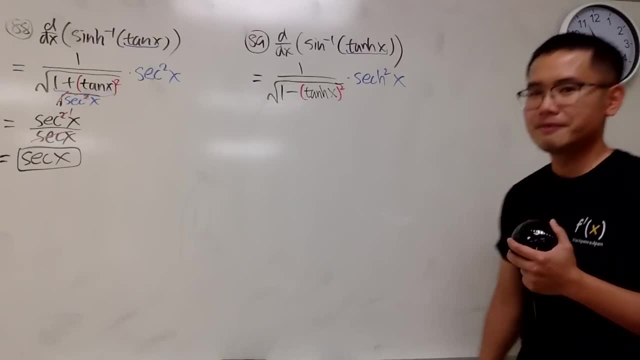 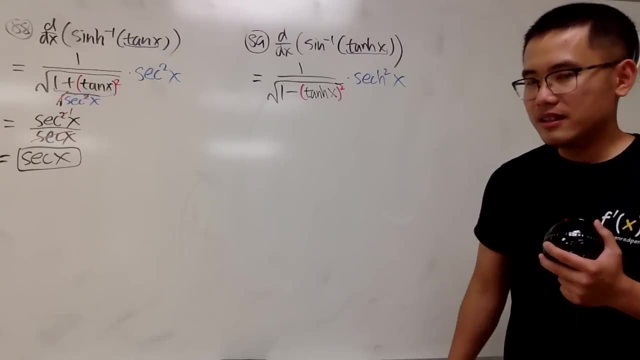 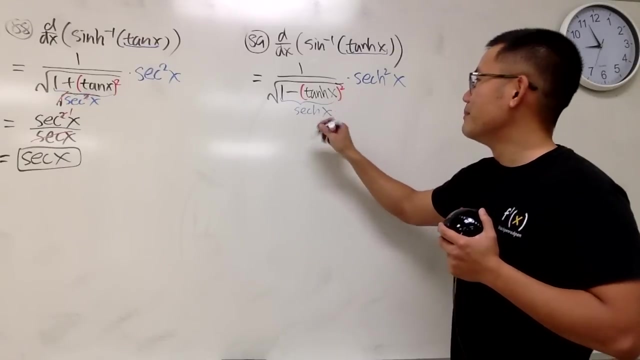 is the hyperbolic secant squared X. that is true, you can prove that with whichever way that you want. but why it's this? yes, identity, yes, this, right here. it's also the same, as You have to make sure, it's a minus 1, minus 10 squared. 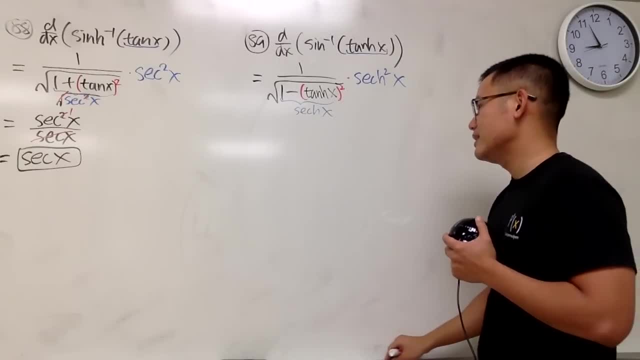 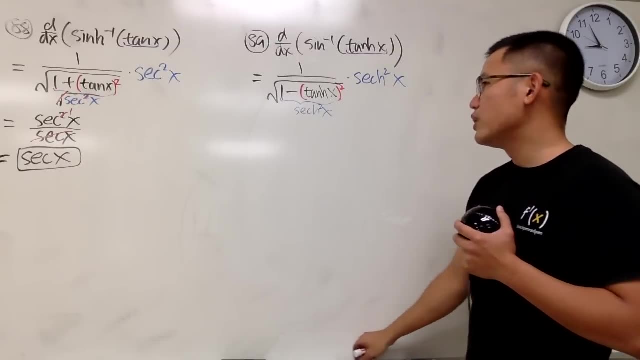 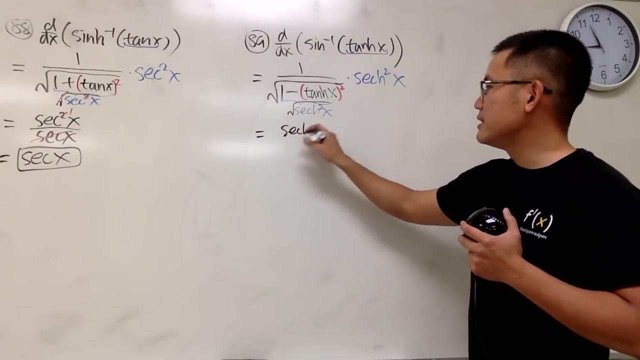 It's actually inverse: hyperbolic secant x squared And just like that you take the square root. So you're looking at on the top, hyperbolic secant squared x Over on the bottom. it's just to the first power. 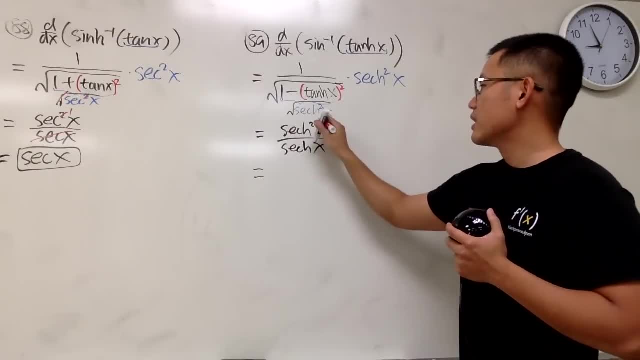 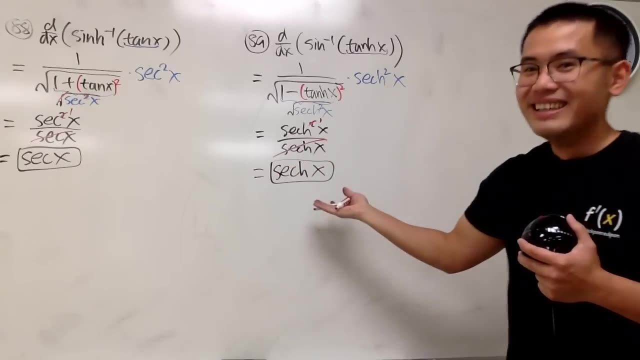 So hyperbolic secant of x, Cancel, cancel. this is 1.. So you have hyperbolic secant of x. So cool, huh. You just put the h somewhere and you can get the h somewhere else too. 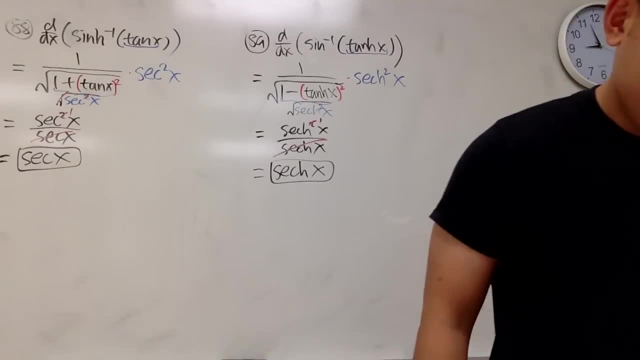 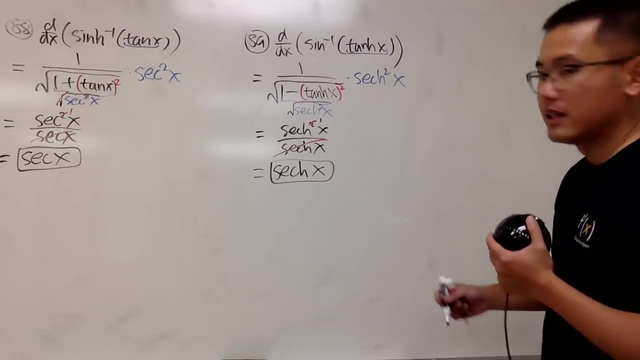 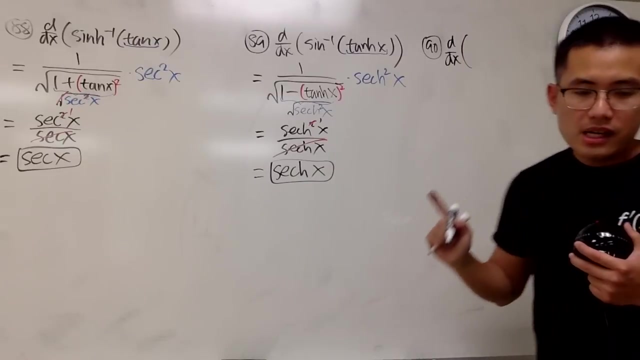 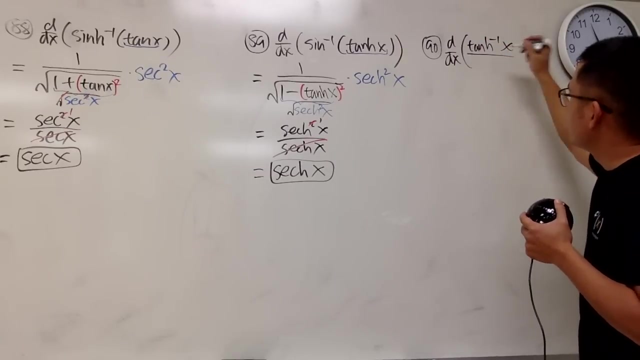 Like that. Very, very, very nice. OK, The last multiple choice question. let's see, I will put it down right here: 90. d dx. Here we have the inverse hyperbolic tangent of x over 1 minus x, squared like that: 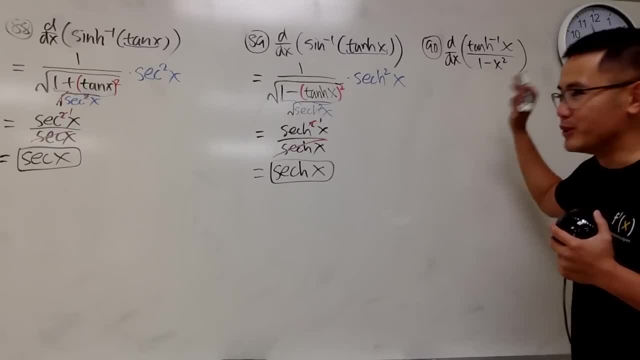 OK, Don't be too excited, We're not doing integral. You don't do your substitution for this, But we'll do quotient rule for this. OK, here we go. Right, here we square the denominator. We square the denominator. 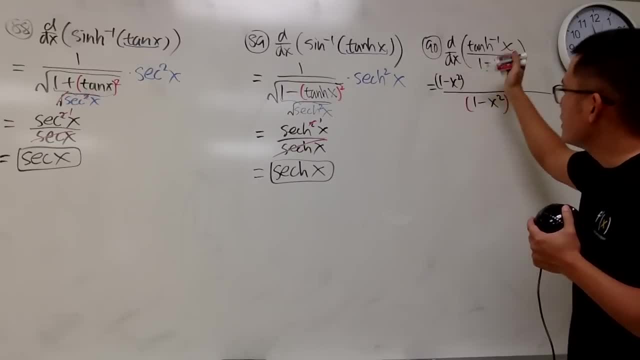 On the top we put 1 minus x squared, the denominator OK Right here, And then multiply by the derivative of the top function, which is 1 over 1 minus x squared like that, And then we minus the top function, which is inverse hyperbolic tangent of x. 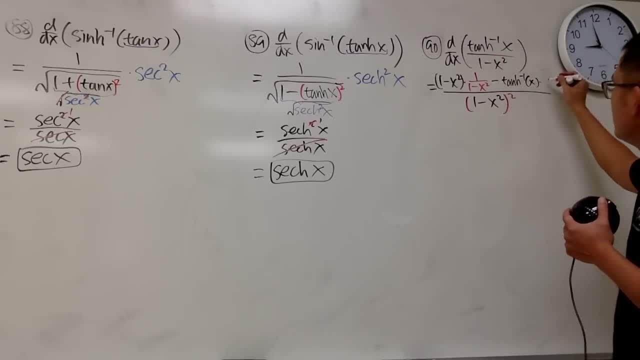 times the derivative of the bottom, which is going to give us negative 2x. OK, And again, this x is the only input for the inverse hyperbolic tangent. Well, well, This and that cancel nicely, So we don't have to worry about the complex fraction situation. 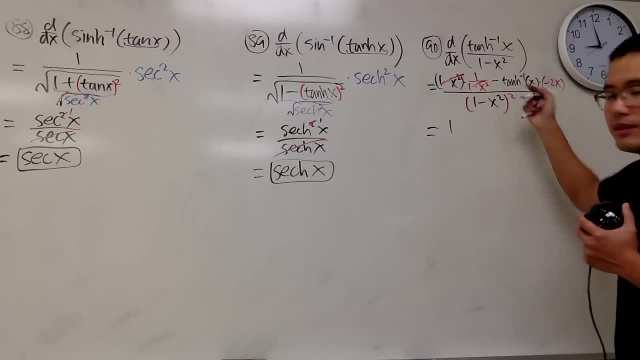 We just have a 1 right here. Negative times, negative, OK, So plus 2x, And this is the hyperbolic inverse, hyperbolic tangent of x. And then on the bottom, here we have this guy which is, parentheses, 1 minus x, squared, squared. 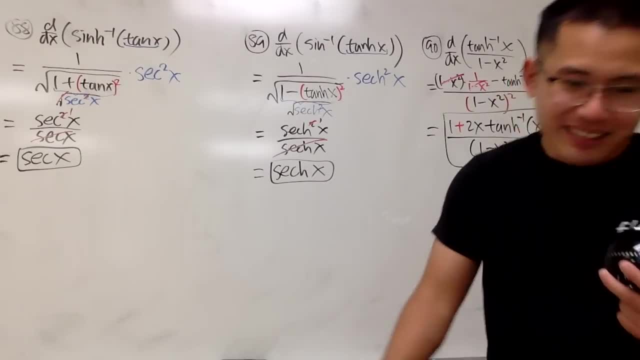 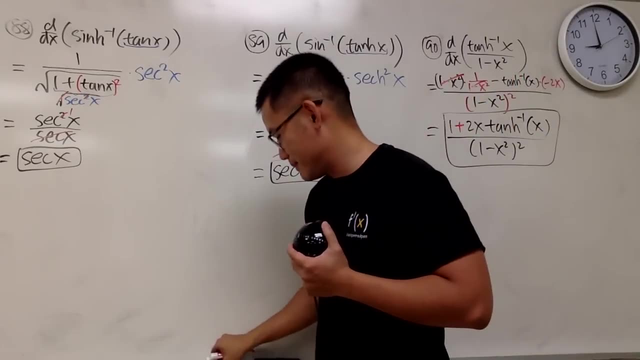 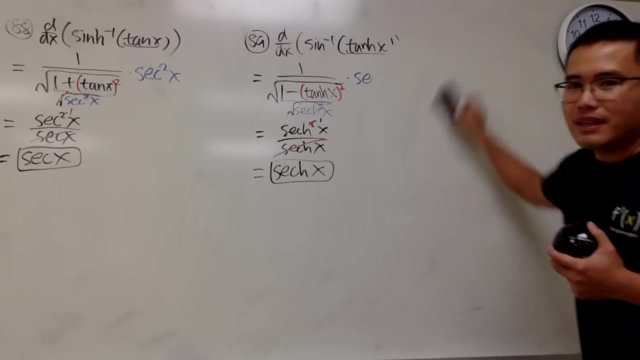 So we can take a big meter And with that we are done. We are done with all the multiple choice questions. I'm not so happy, as I said, Even though I'm almost done, but I know the hard part is coming, so I will have to calm. 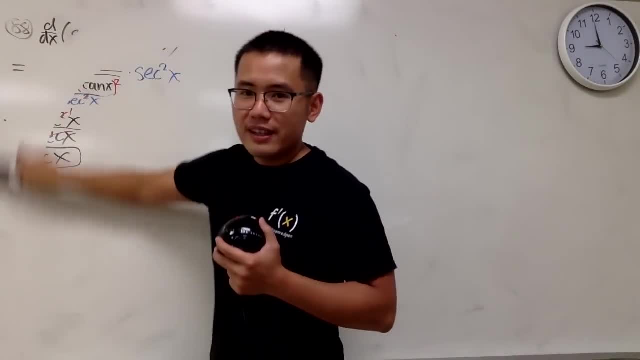 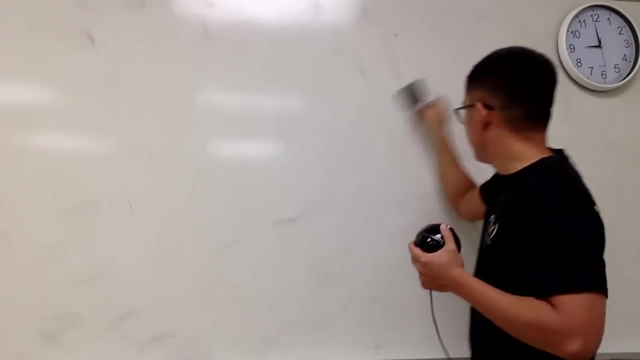 down. I will have to make sure I can get ready for the next 10 questions. I don't know how long it will take. It's 5 hours only. It's not so bad. 5 hours only. 5 hours and 40 minutes. 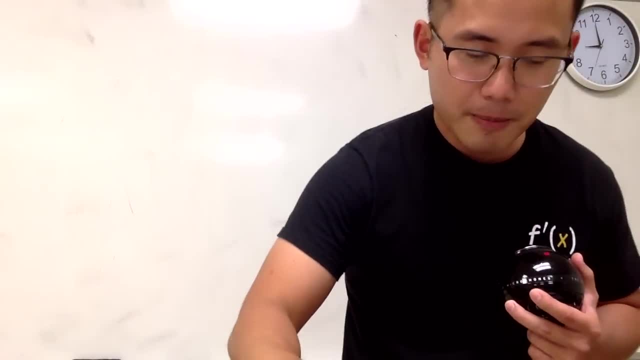 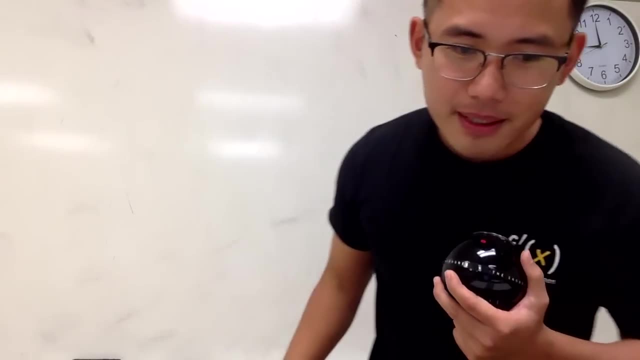 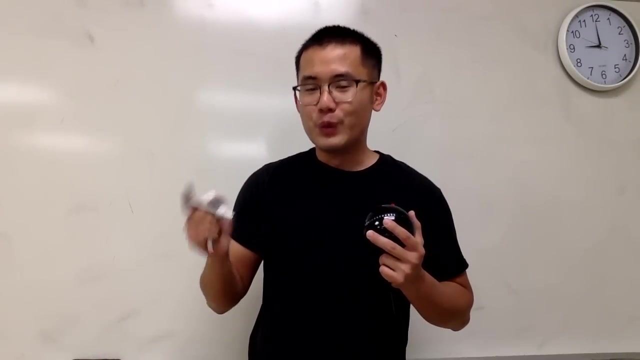 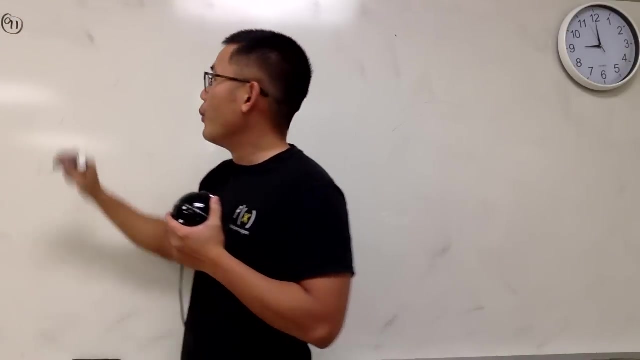 I just saw the timer, But the good news is last page. Okay, Ladies and gentlemen, welcome to take the derivative with definitions. So number 80, sorry, number 91,. right, So we are going to be differentiating d, dx again, x to the third power. 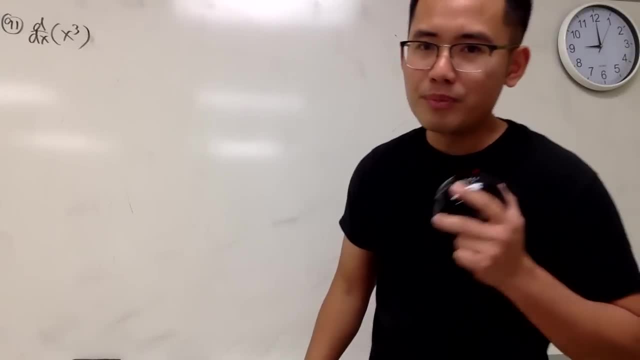 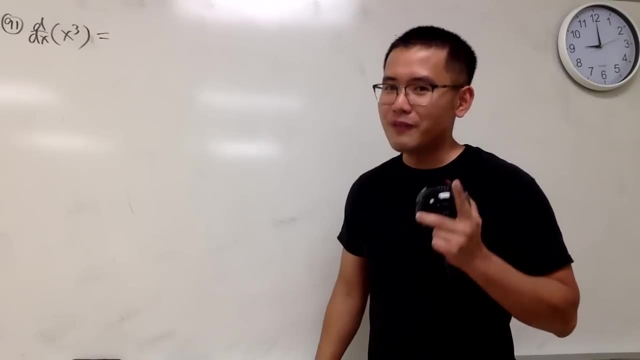 I know the answer. you know the answer, everybody knows the answer, but do you remember how to use the definition for the answer? No, you don't. Then watch out, okay, And you just have to make sure you follow direction. 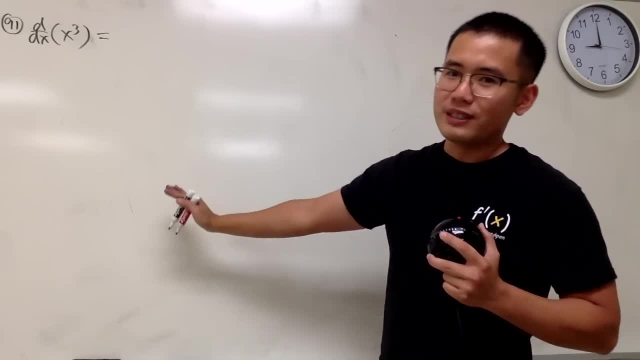 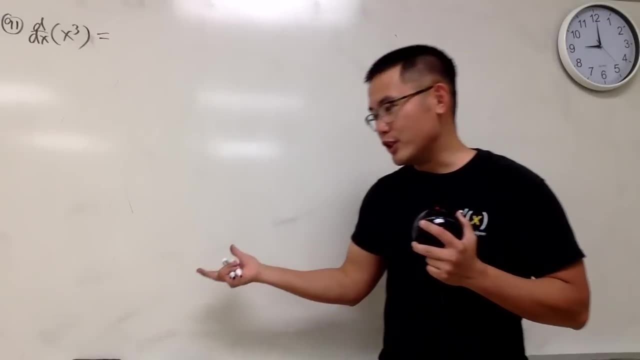 See a lot of students. they lose points for this kind of questions on the exams because they don't follow direction. If the question say use the definition, you have to use the definition, Otherwise you just you're not going to get. 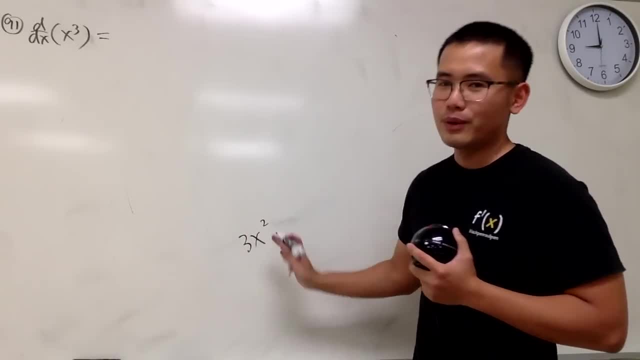 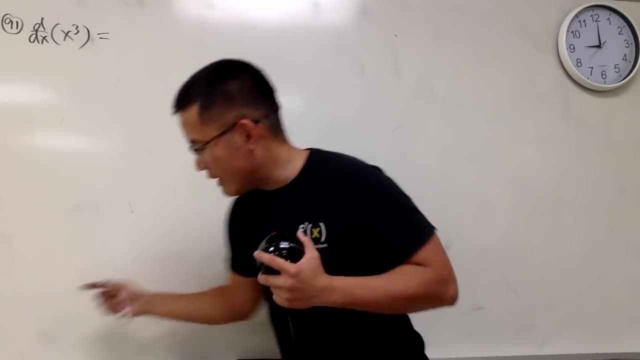 any points. Okay, seriously, Don't be cute and say the answer is 3x to the second power. No, you have to show the work on the exams. So you have to remember, you have to remember. okay, You have to have to know that. 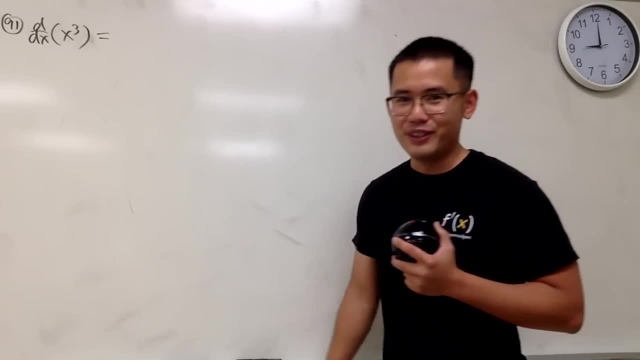 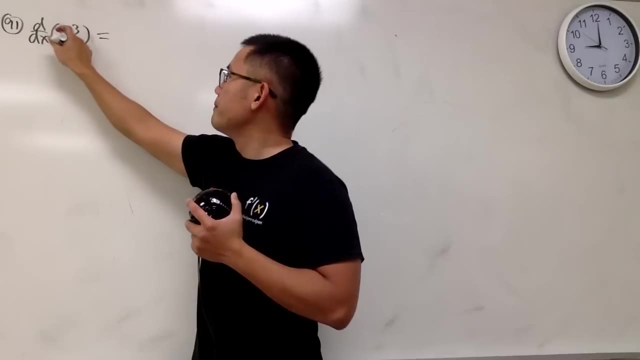 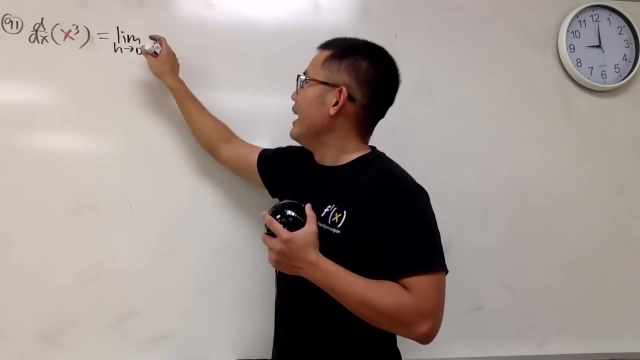 And why do you need to know this? Well, that's how you can prove things with definitions. Anyway, here we go. This is the function, This is the input, the x is the input. Well, you take the limit, as h goes to 0.. 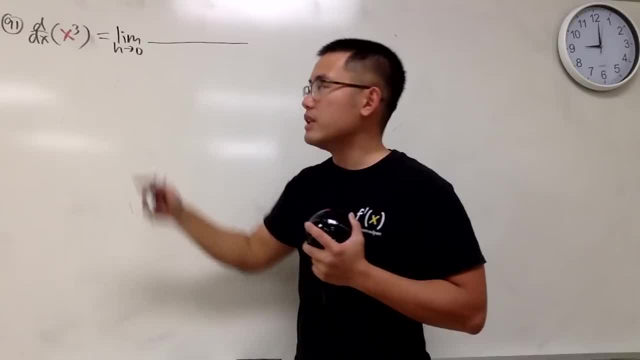 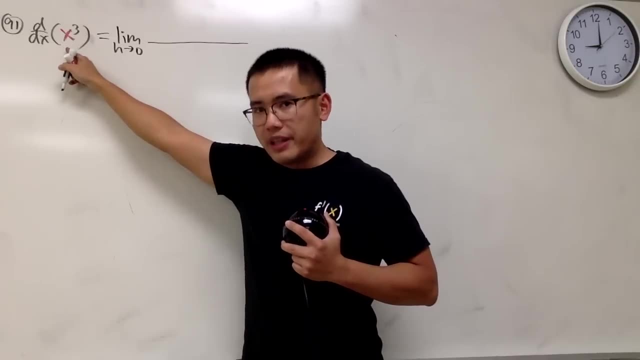 And remember the difference quotient is f of x plus h minus f of x or over h. So you put x plus h into x, right here. So you open the parentheses with x plus h here and you raise that to the third power. 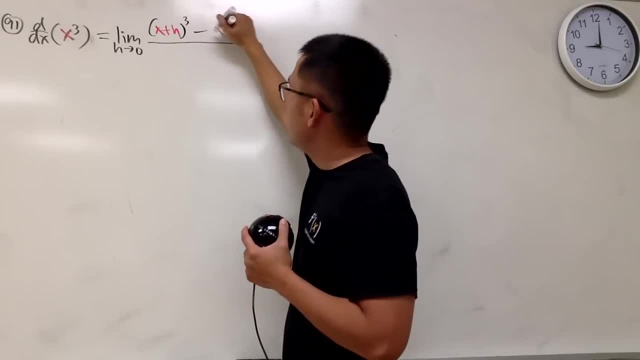 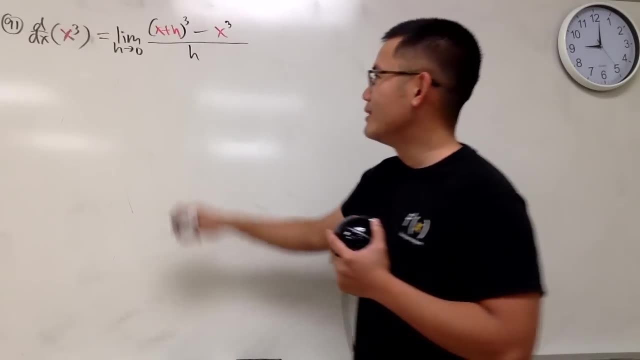 And then you minus this right here, it's just that. So it's x to the third power, And then you divide it by h, like that. Okay, Now you can just do this, You can do this, You can do this. 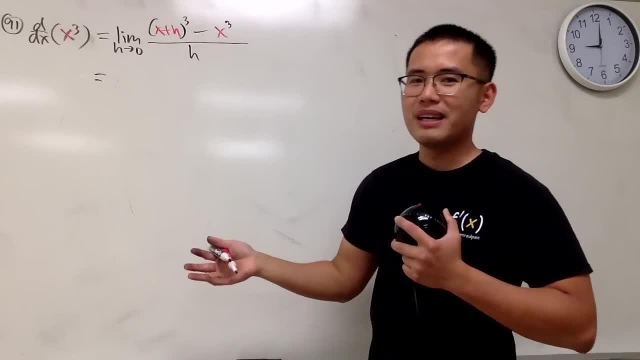 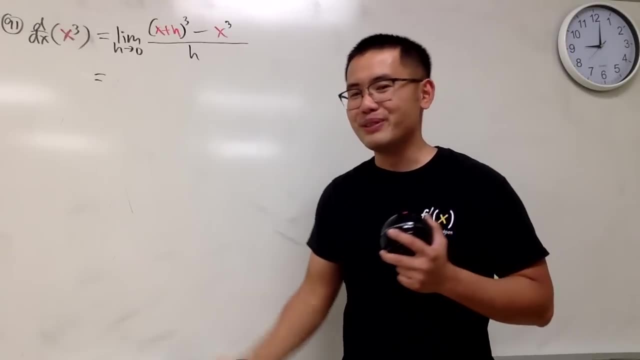 You can just multiply this out. You can also try to factor it, but I think multiply it's easier. for this situation You can actually use the difference of two cubes to factor it, but up to you. Anyway, you have to write down the limit as h approaching 0.. 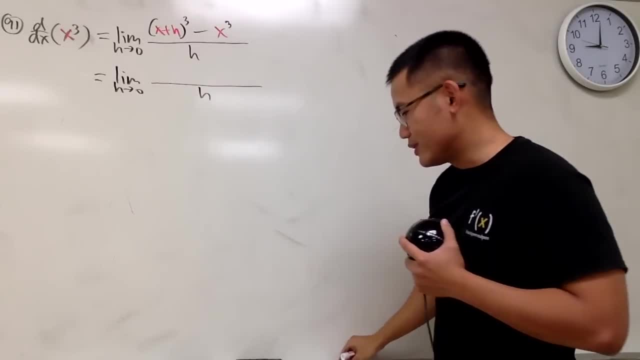 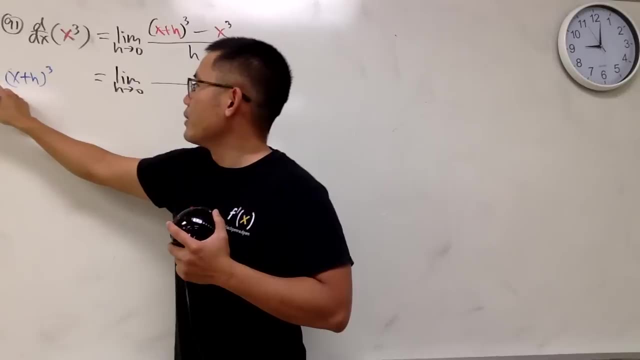 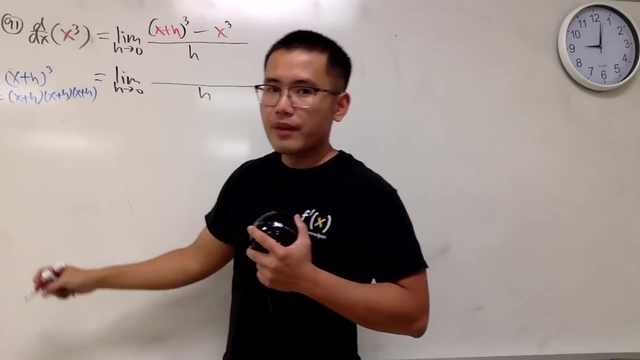 And when you multiply this out, you just do it somewhere. I'll show you, just to make sure that we know what we are doing. okay, x plus h, x plus h, x plus h. So for the first two part, of course, we just multiply this out. 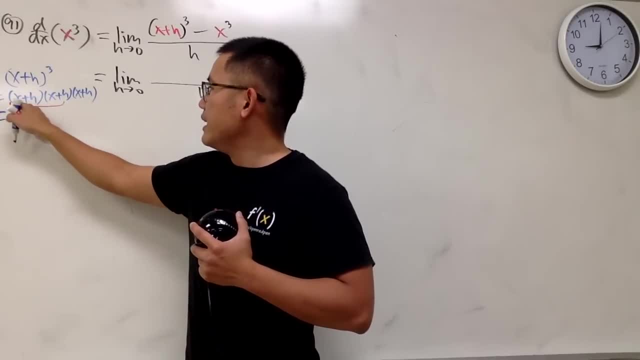 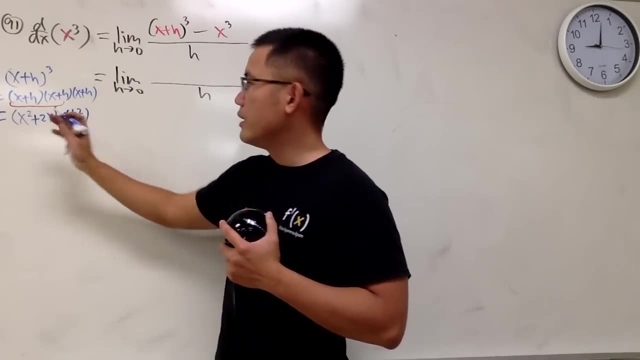 So you end out with x squared, and then you get xh plus another xh, So you have two of them, 2xh, And lastly you have h squared, all right, And you have to multiply it one more time, so x plus h. 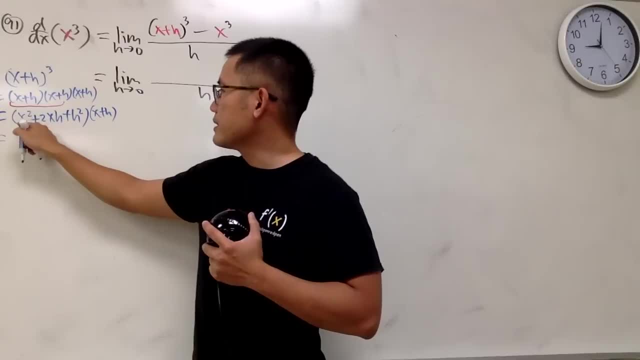 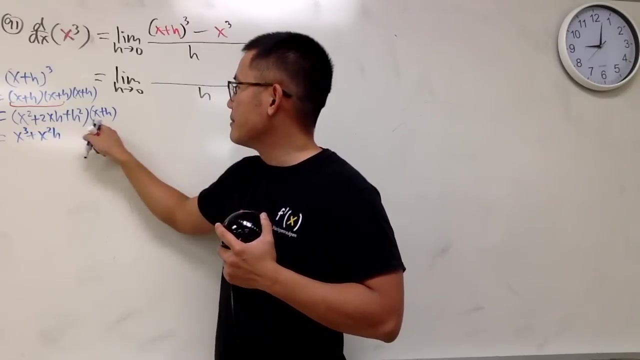 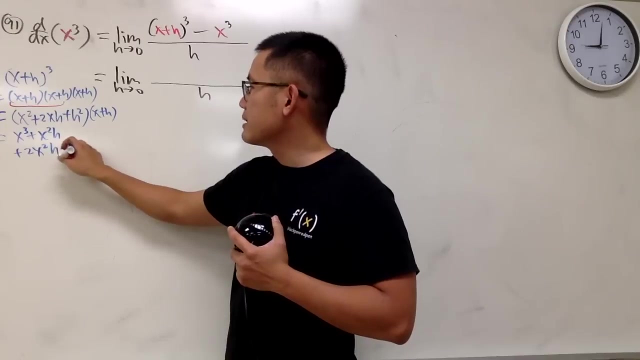 So you do this times that, which is okay. let's do this times that, Which is: is x squared times x, which is x to the third power, and x squared times h, so it's plus x squared h. and then, this times, that is plus 2x squared h, and this times that is plus. 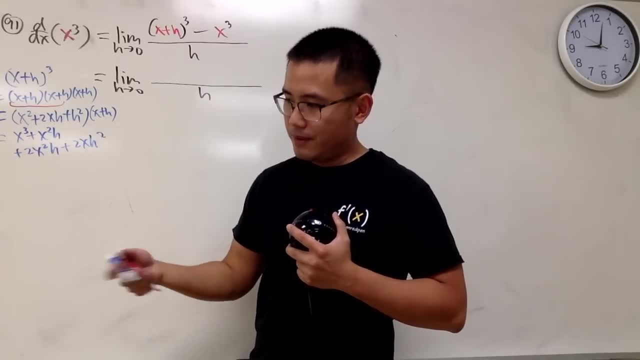 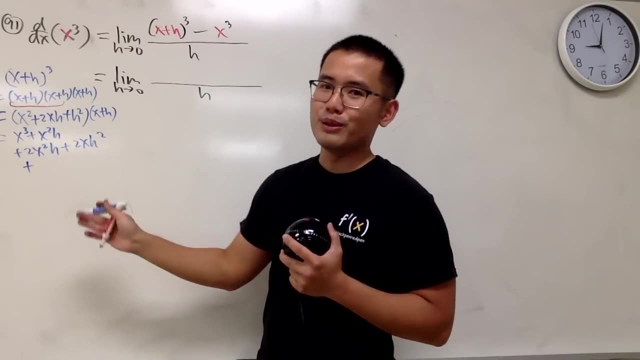 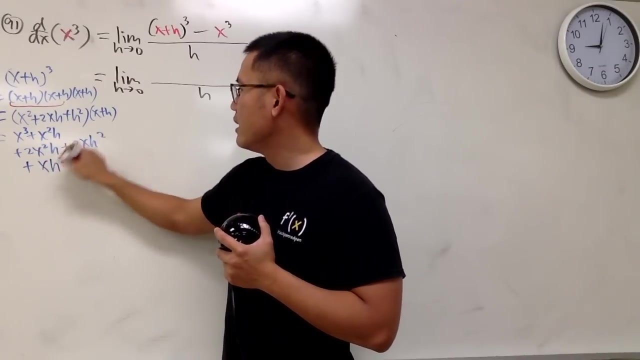 2xh squared. I know the Pascal's triangle, I know the fast way, but I just want to show you guys all the work because I know not all the students know about this. okay, So that's the: this times, that is x times h squared, and then this times, that is plus h to the. 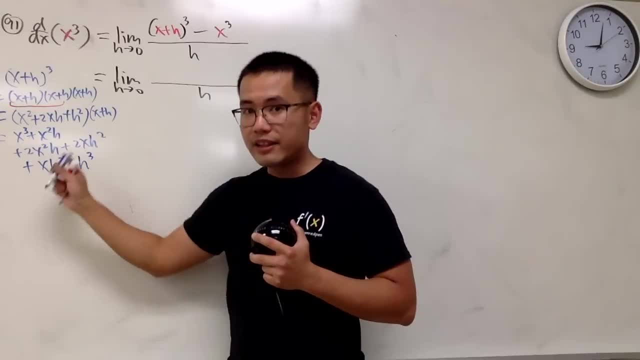 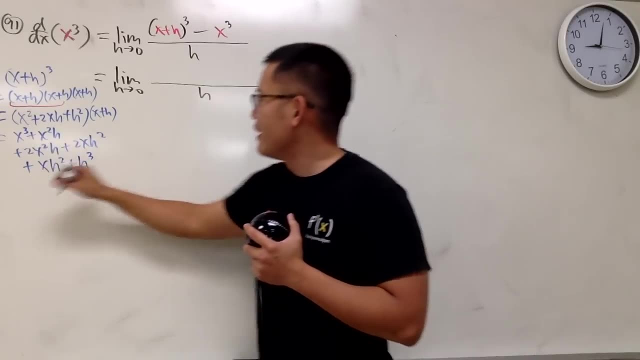 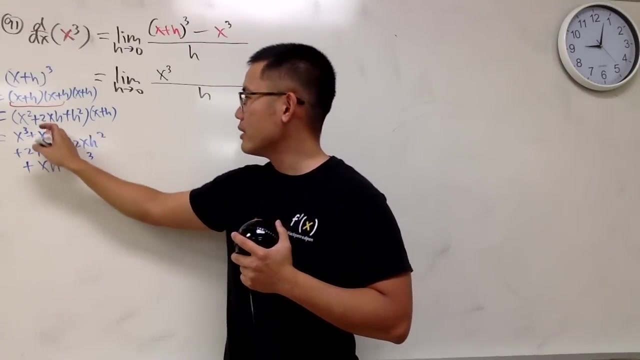 third power. like that, All in all, we can collect like terms and put the result right here. So when we do that, we'll see this right. here is x to the third power and let's see: this is x squared h and we have two more. 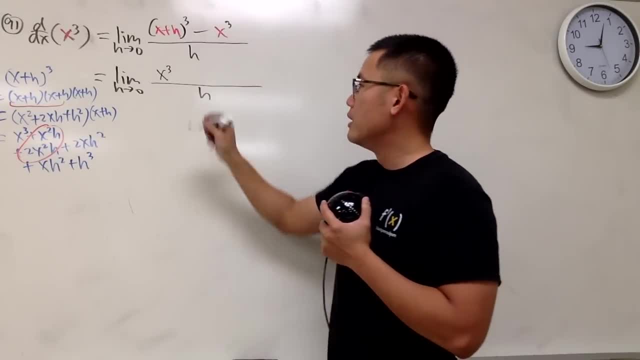 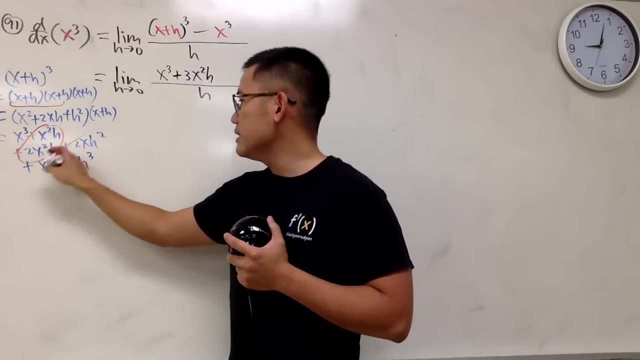 These two things can be combined. So in all we have three of them. So we plus 3x squared h, and we see that this and that are like terms. 2 plus 1 is against 3.. So we 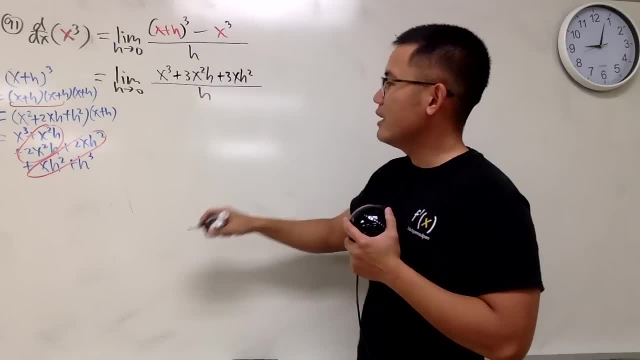 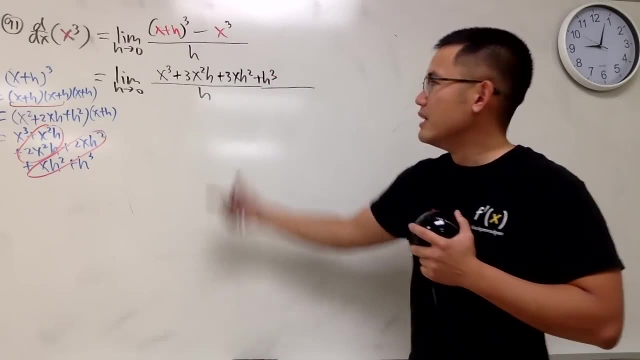 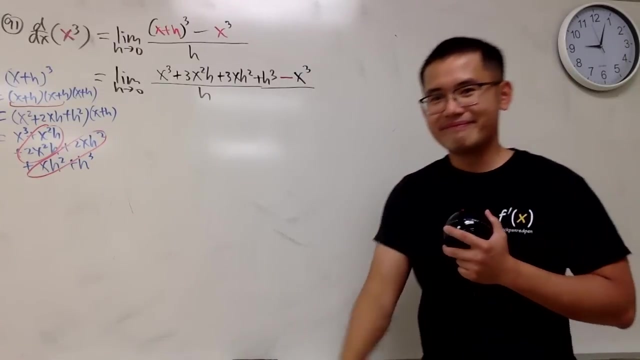 put down plus 3xh squared and lastly we have the plus h squared. no h to the third power, right here. This is the first part, all right. And then we have to just minus x to the third power, And now we'll just literally minus the x to the third power. 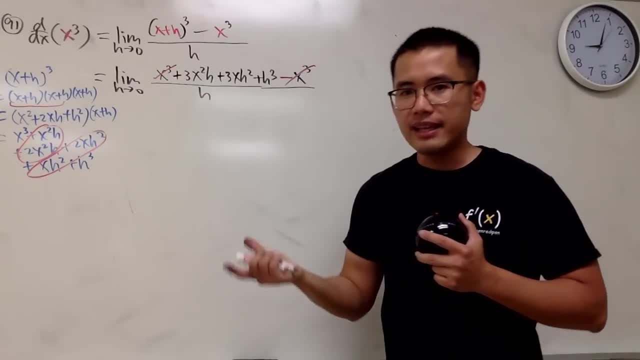 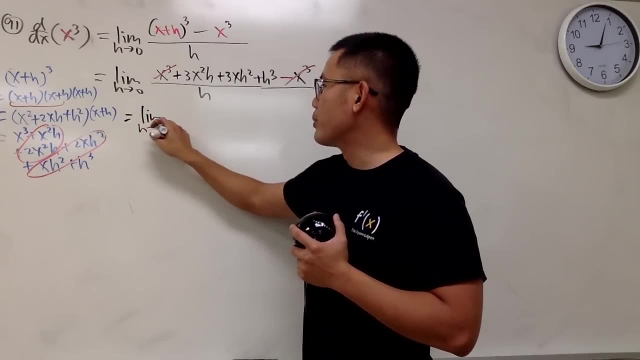 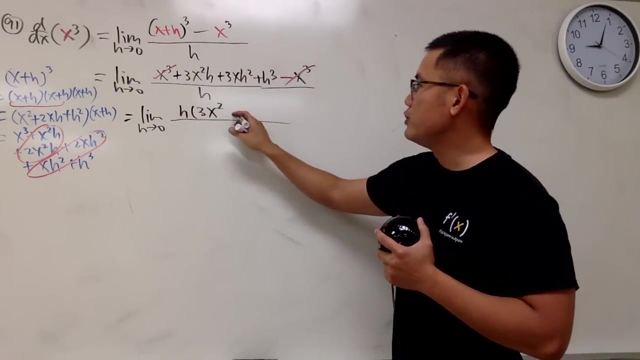 That's good, huh? And, as you can see, everybody on the top has an h, So we can factor it out and good things are about to happen. So check this out. Here we have the limit as h approaching 0.. Factor out the h and we have 3x squared, And then factor out the. 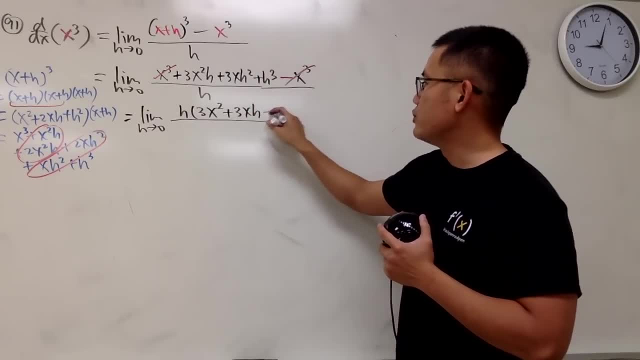 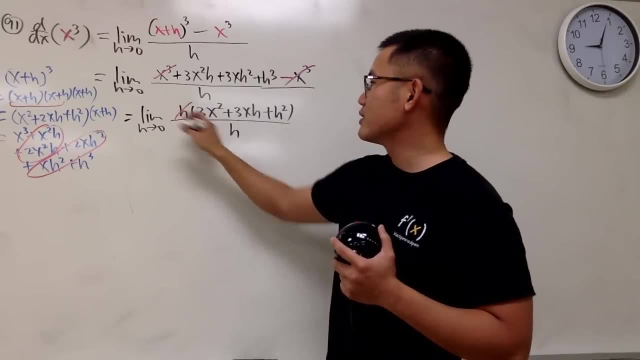 h. we have plus 3xh, And then factor out the h, we have plus 3x squared, And then this is all over h. What can we do with the h's? Cancel them out. Cancel this out. Lastly, 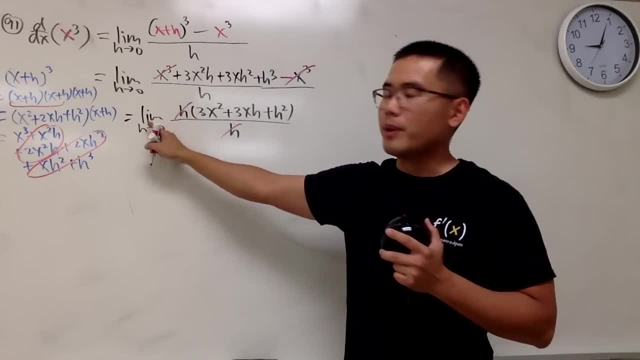 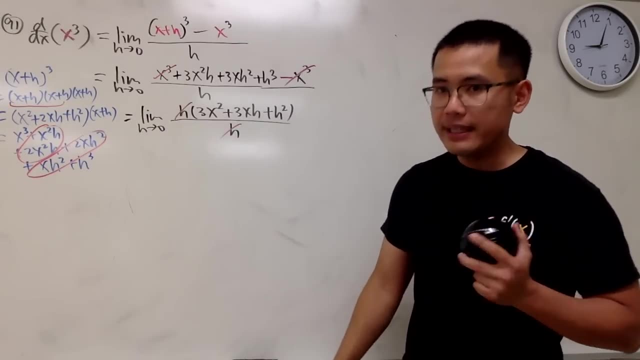 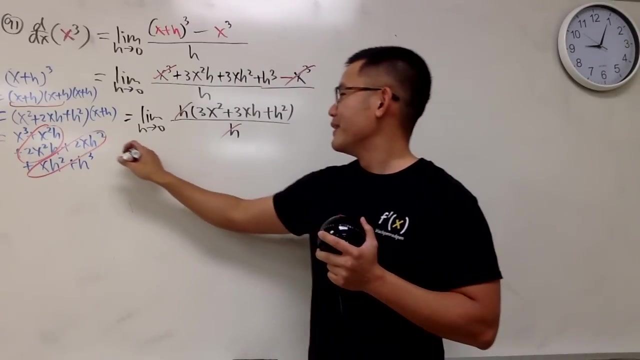 remember x. okay, remember, x is the variable. Remember that we are taking the limit as h going to 0. So we just put 0 into all the h, the remaining h, And you see, when you cancel this h and that h, there's no more 0 over 0. So, no, nothing, okay, No worry. 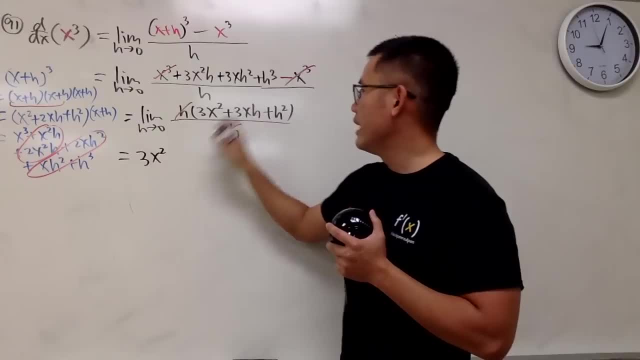 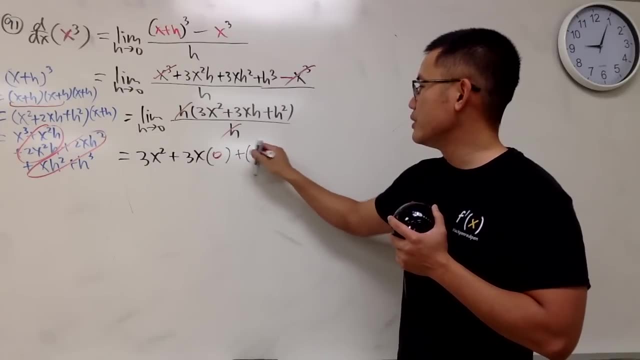 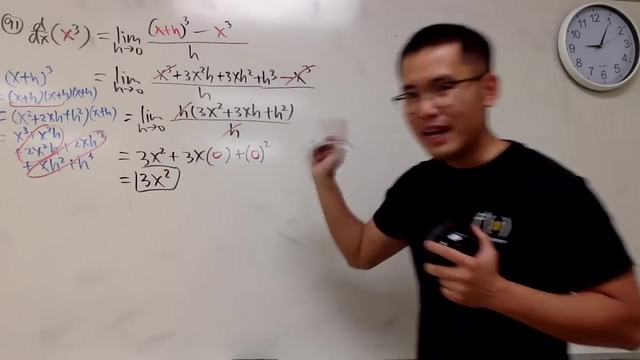 okay, So you have 3x squared and plus 3x times putting 0 in here, and lastly, you put down plus 0 squared. This is 0.0.. Yes, we get 3x squared. okay, And we are done. This is actually. 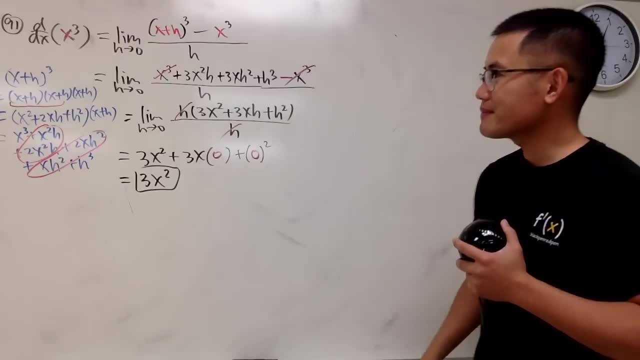 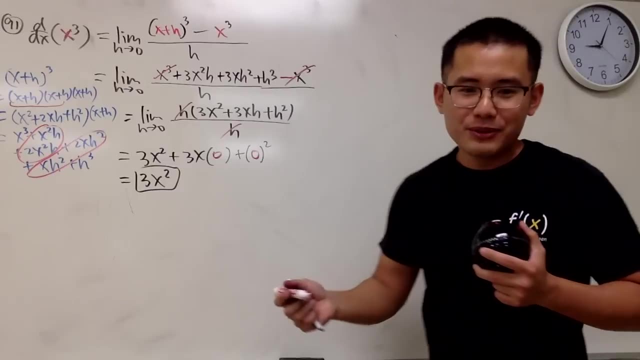 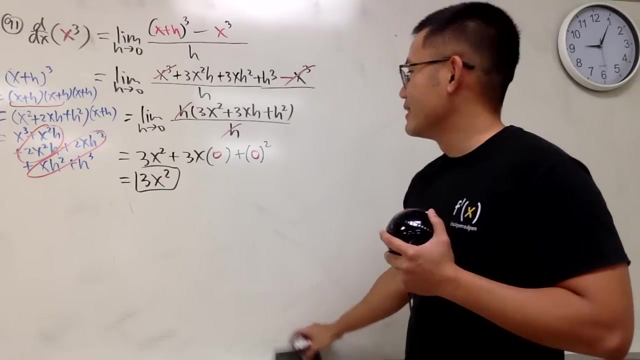 not that bad. I know, Yeah, I wasn't going to do this in the first place. I know I'm sure Some of you guys are going to say, hey, where's the definition of derivative? Yeah, So I have. you know, I have to. So 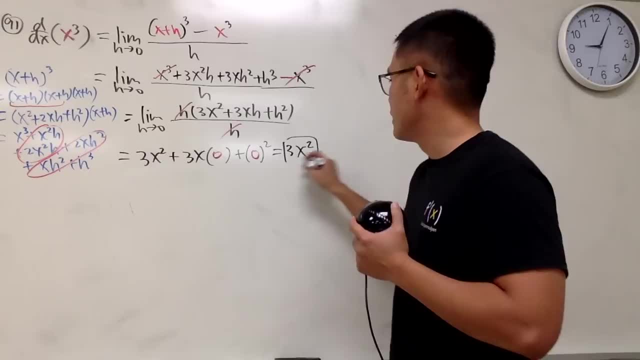 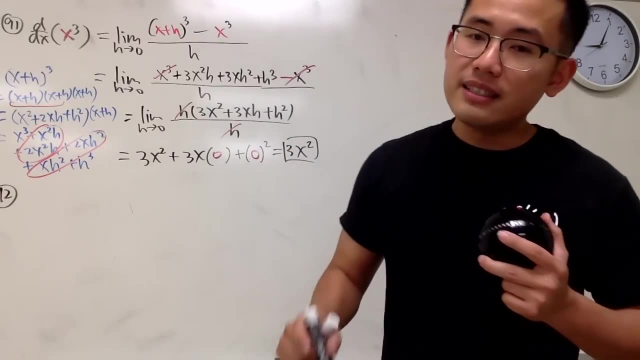 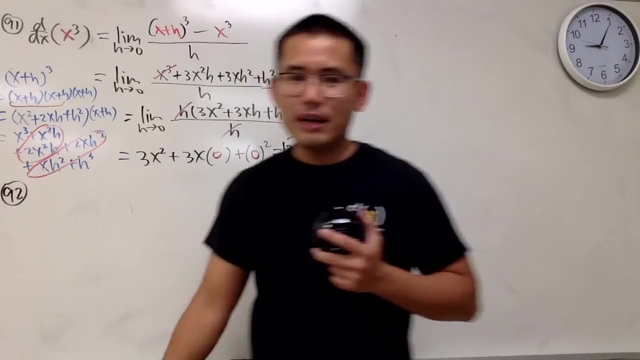 anyway, this right here is 3x squared. Let me see if I can fit in one more right here, Number 92.. I'll give you guys another type of the question. This is another one that we did in the first couple questions. I'm not going to bother to look it up because 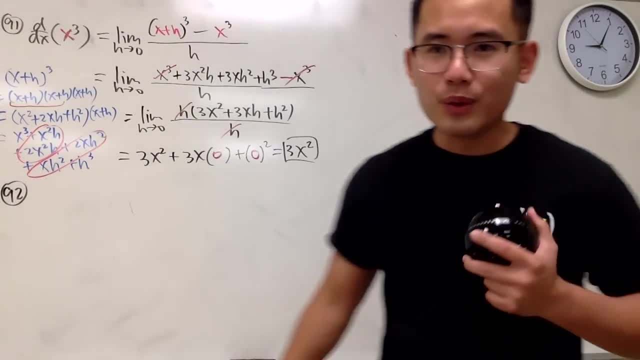 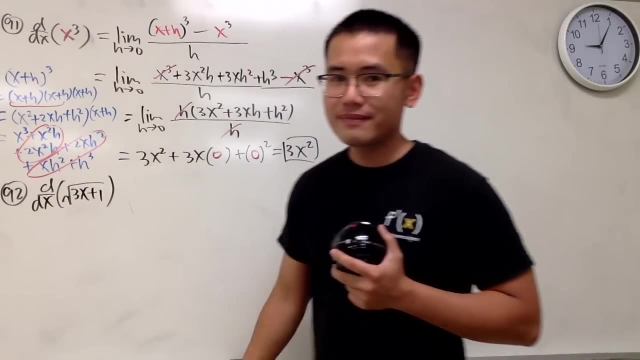 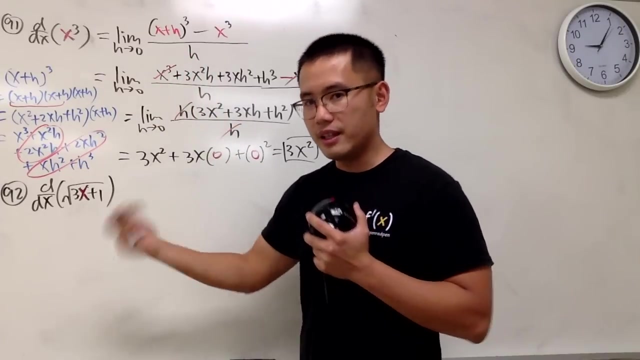 I'm just going to finish this and I want to go home. Anyway, d dx, square root of 3x plus 1.. Here is the input, which is x, right here. So you are going to plug in x plus h in there and then do the rest. 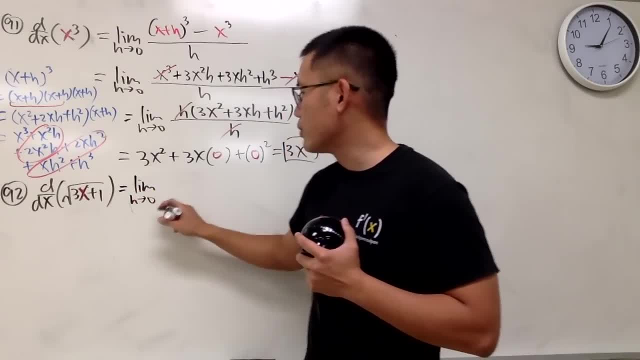 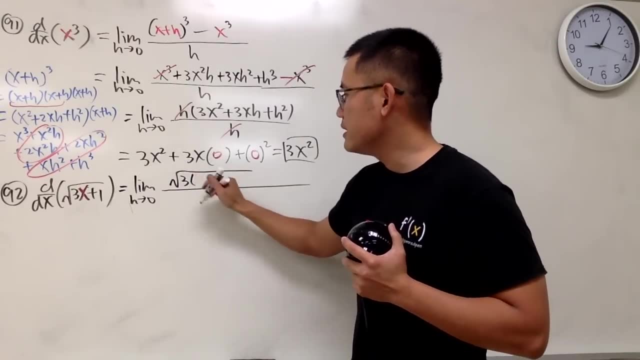 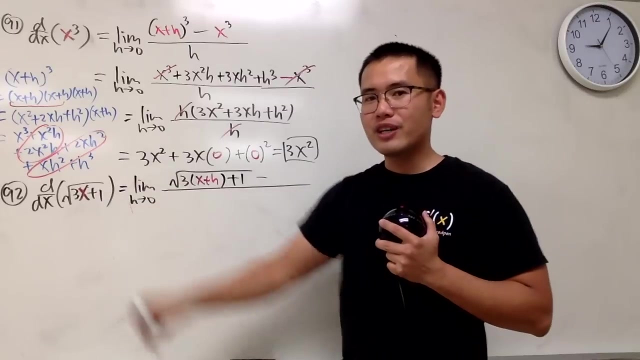 Anyway, take the limit as h going to 0, put in x plus h right here, So we have the square root 3, parentheses x plus h and then plus 1.. And then minus that function, which is just square root of 3x plus 1.. 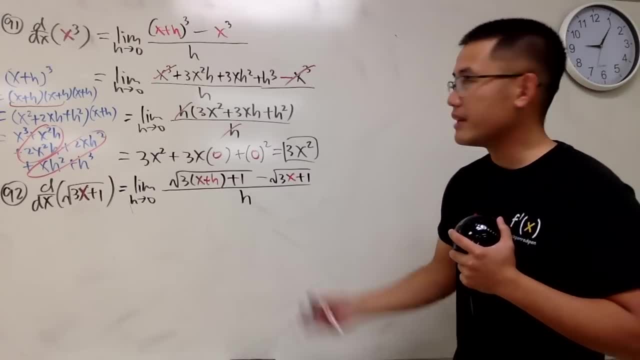 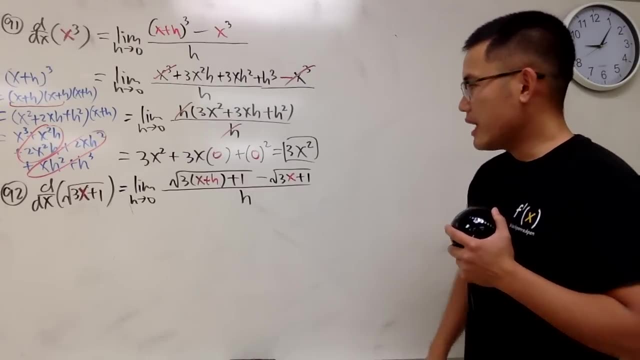 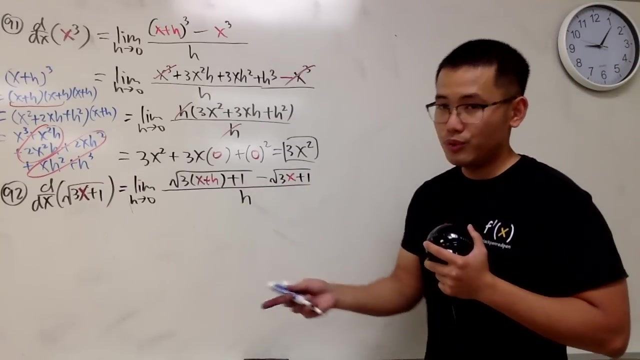 And everybody is divided by h, right here, right? So my h is okay. okay, Yeah, I'm just going to make sure I'm okay. Now we are going to just see how to simplify this kind of limit, To do so when you have square roots, keep in mind. 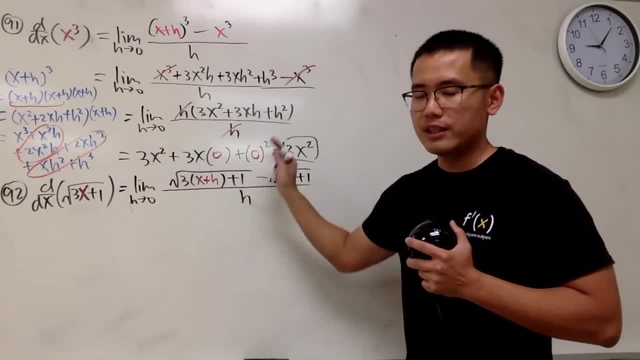 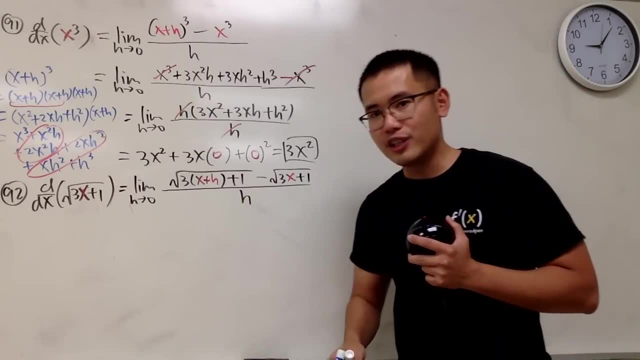 if you plug in x plus h, if you plug in 0 into h, right now you get 0 for 0.. One way to simplify this kind of situation, when we have square root, is to multiply the top and bottom by the conjugate. 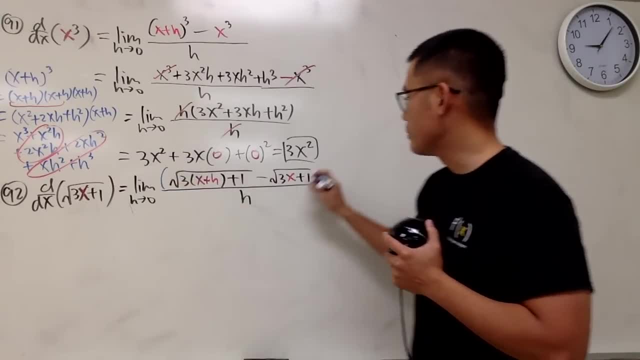 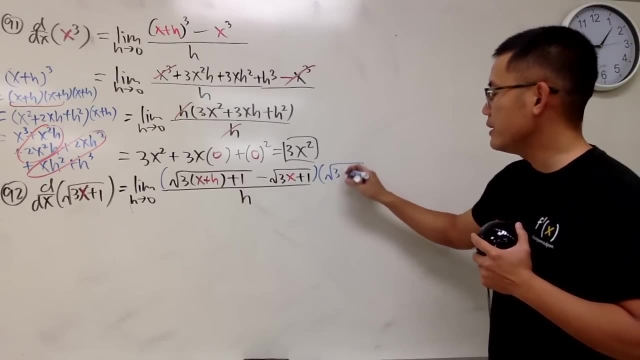 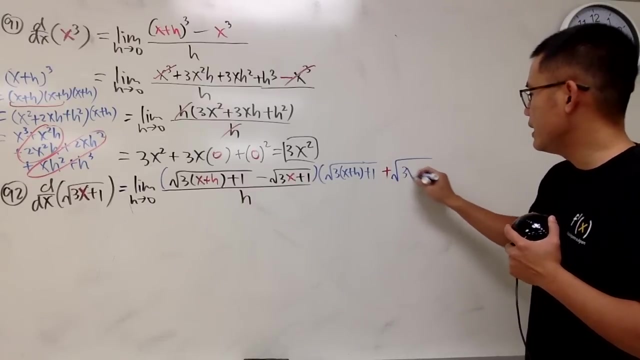 So that's the usual strategy, So we will do so. So multiply the top and bottom by the conjugate, which is just this: plus that square root of 3x plus h plus 1, and then plus square root of 3x plus 1.. 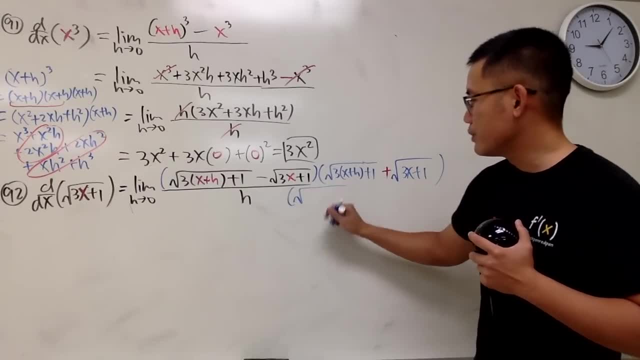 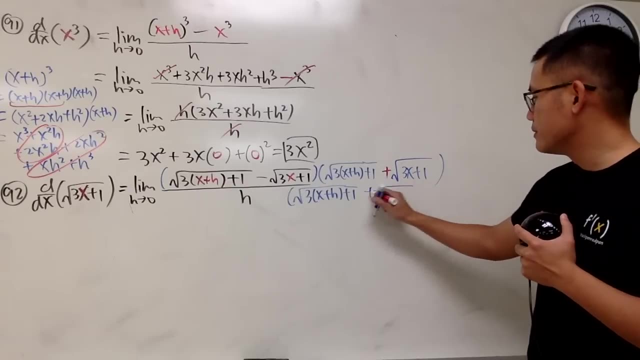 And then, of course, do the same thing on the bottom. So parenthesis: square root of 3x plus h plus 1, plus square root of- I like to keep my color consistent- and then the 3x plus 1,, like that: 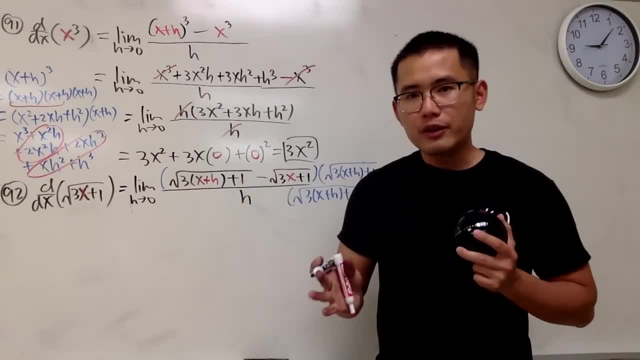 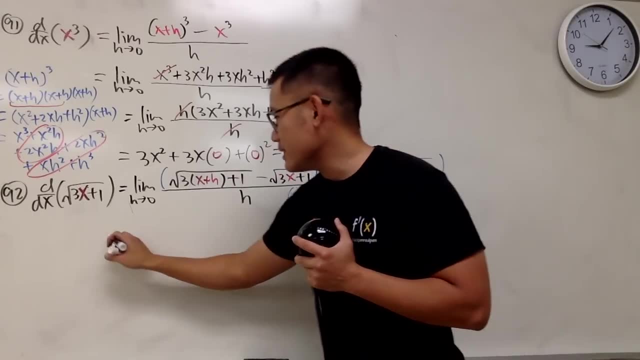 Okay, here is the good news: To multiply out the top, it's not so bad because you are in the form of a minus b times a plus b. So this is going to give us the following: We still have the limit as h approaching 0.. 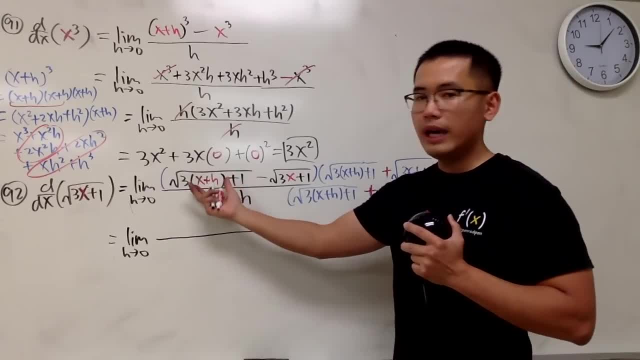 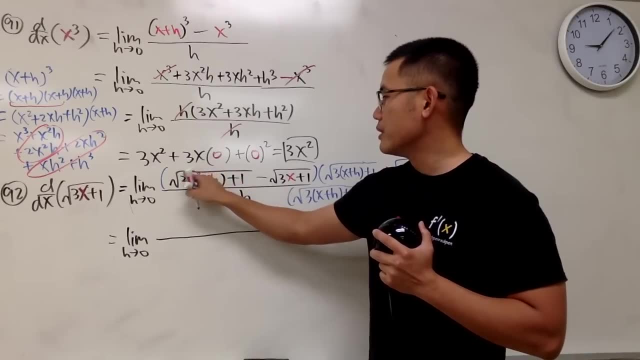 Well, well, on the top, we just have to do a squared minus b squared. a squared is just the inside. Well, in the meantime, let's also distribute that part. How's that Actually? let me just keep it as how it is. 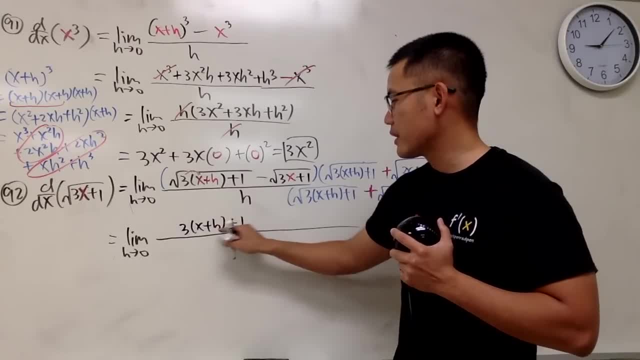 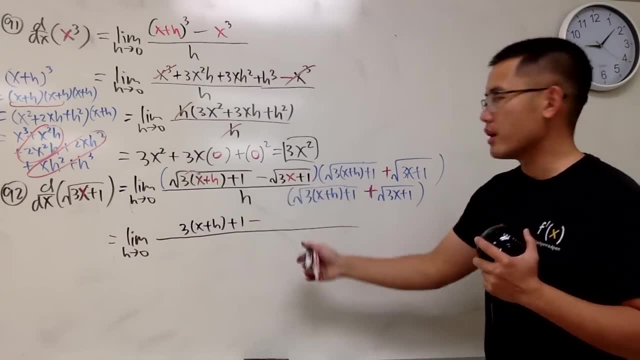 3 parenthesis: x plus h plus 1.. Okay, a squared And then minus b squared. b squared is just this thing squared And that's just going to give us the inside. And let's put a parenthesis because I will have to distribute the negative in a second. 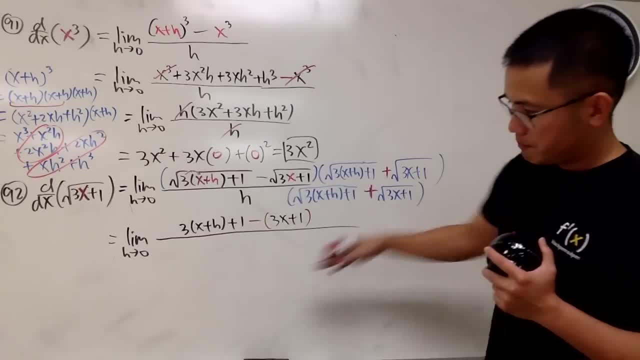 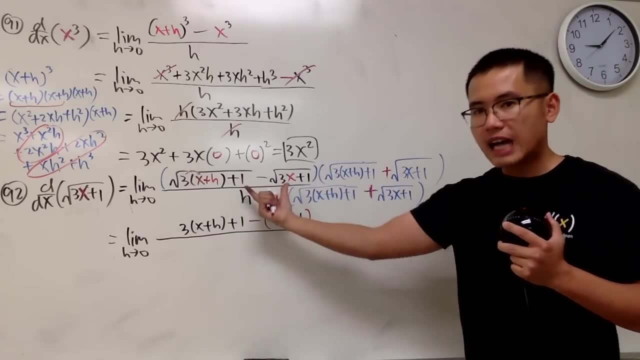 That's what we have right. And for the bottom, just go ahead write it down again, Because, remember, the point of multiplying this conjugate is to fix the top. So just multiply out the top And for the bottom, just leave it like this. 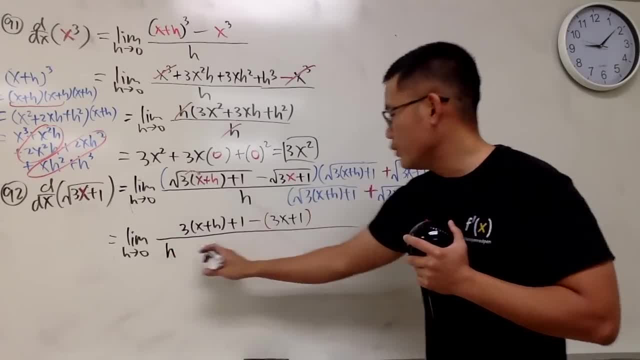 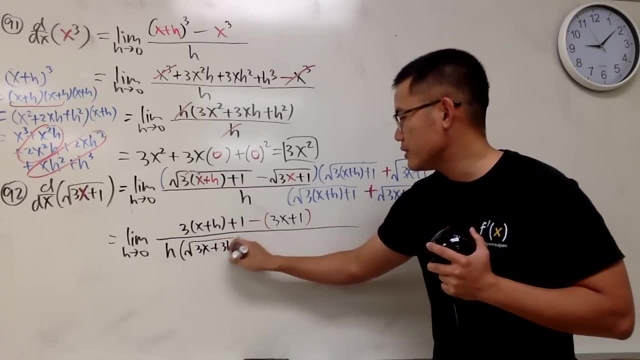 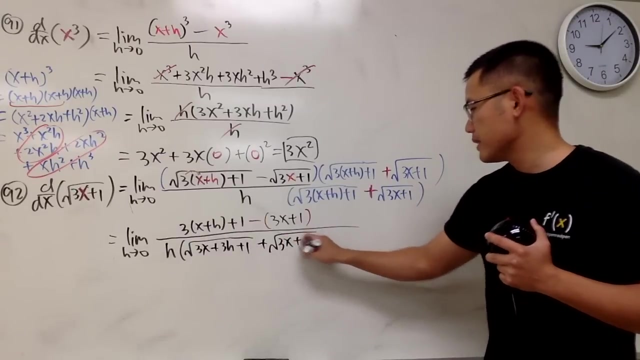 and wait for good things to happen. So you will see, the good things will happen. This right now. let's just multiply it: 3x plus h, 3h, and then plus 1, and then plus square root of 3x plus 1.. 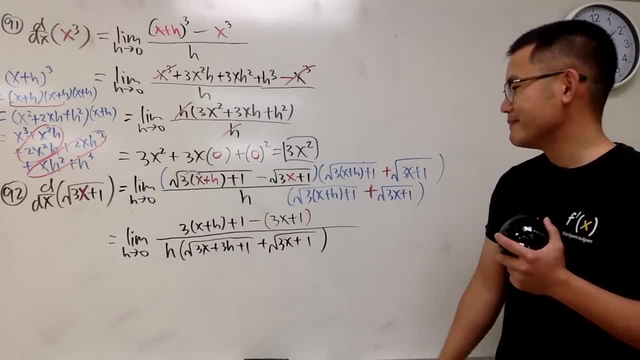 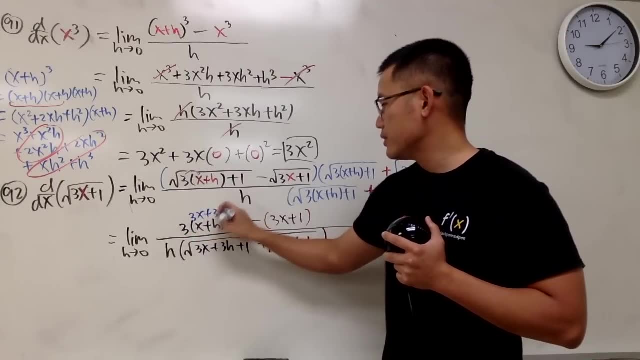 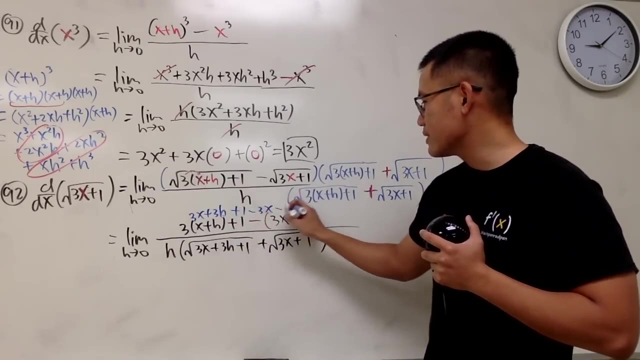 It actually doesn't matter if you multiply it out or not, but whatever. Anyway, right here here we go. This right here is 3x plus 3h plus 1 minus 3x minus 1.. Yeah, Can we reduce? 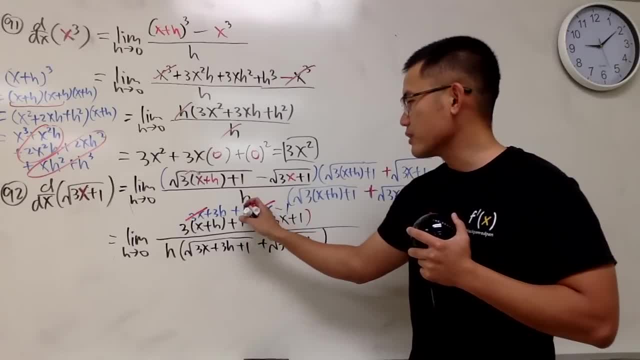 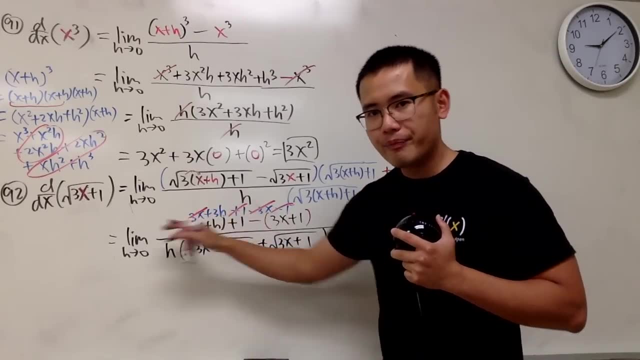 Yes, You literally cancel out the 3x and also the 1 minus 1 is done. Yeah, And now check this out On the top. we have just 3h left over. h times this quantity. This is 3 times h. 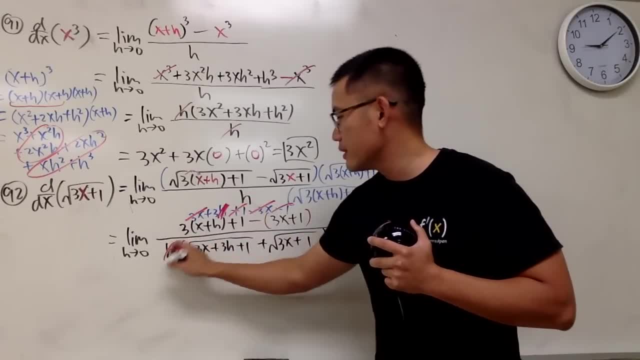 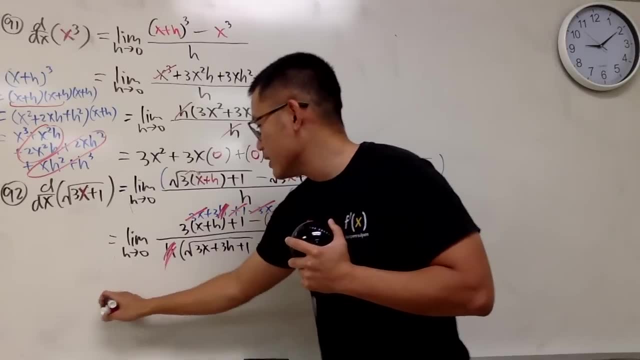 So we can just divide the h out. So we divide this out. Okay, Cool. So no more 0 over 0 situation. We just have that 3 on the top and now we can just put the 0 into the remaining h. 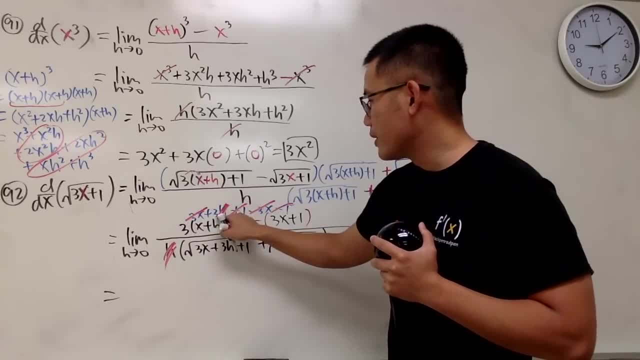 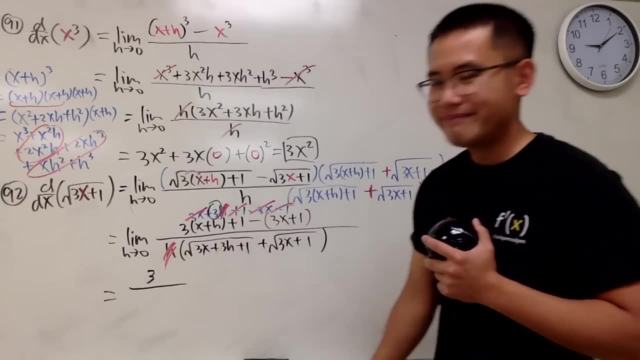 which is only this right here. Keep in mind, we still have this 3 right here, though. Okay, We still have this 3 right here. So this 3, this 3 right here, 3 over. well, I put in 0 into h. 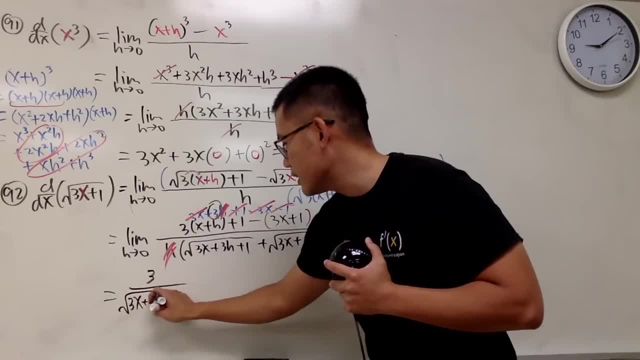 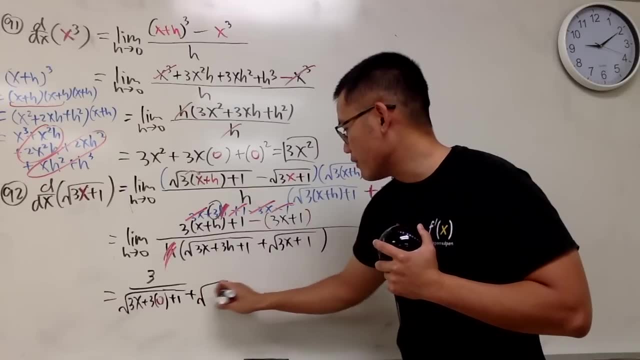 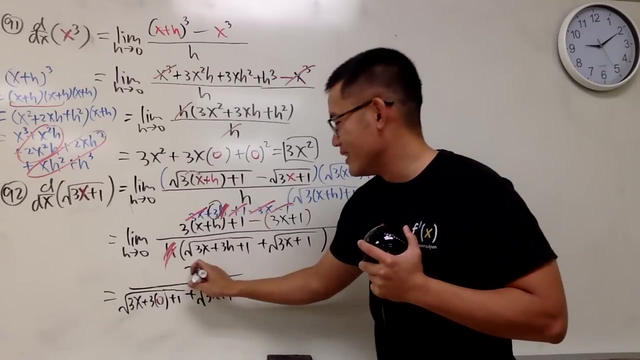 So we have square root of 3x plus 3 times 0 plus 1, and then plus square root of 3x plus 1.. Like this, Don't forget this: 3.. This is how you can show that you need a chain rule. 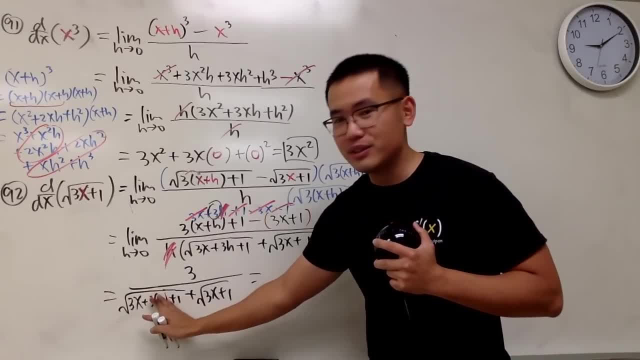 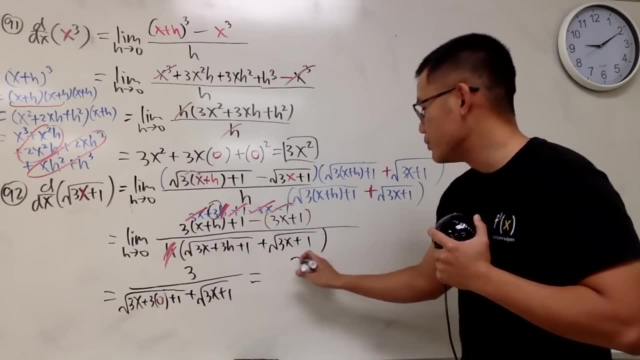 Need a 3.. In the end, of course, this right here is just 0, and you have 3x plus 1 inside here in the square root, and they are the same square root, So we can have 3 over 2 square root of 3x plus 1.. 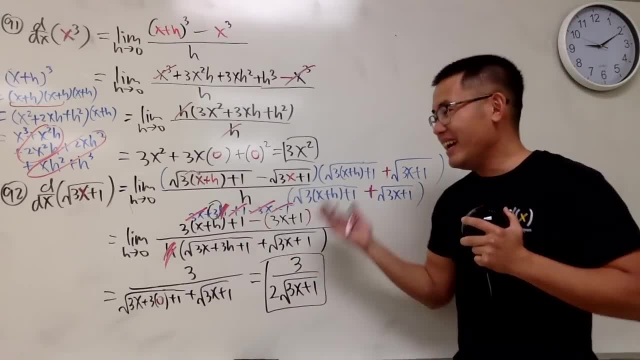 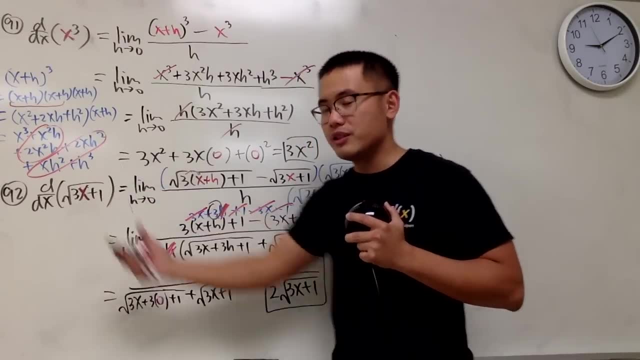 And we are done, Okay. That's why, you see, we need a chain rule. We need to multiply by the derivative of the inside 3x plus 1, which is going to be the 3 right here on the top. 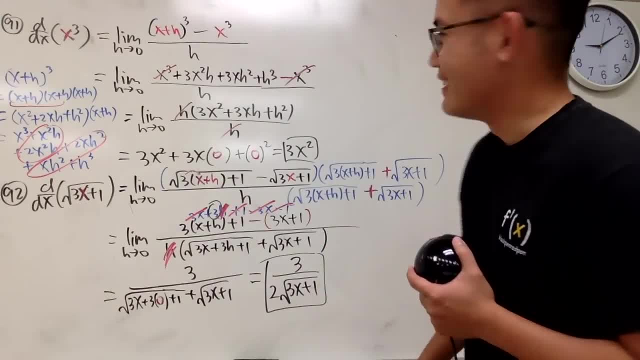 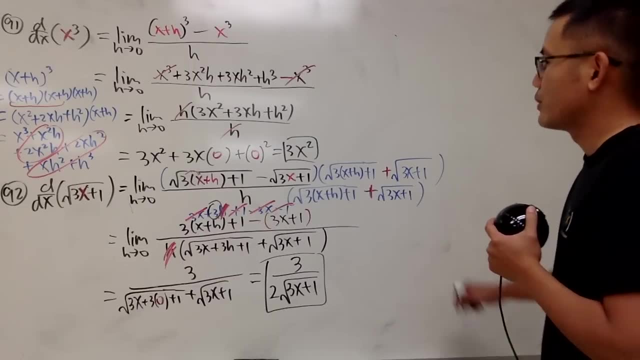 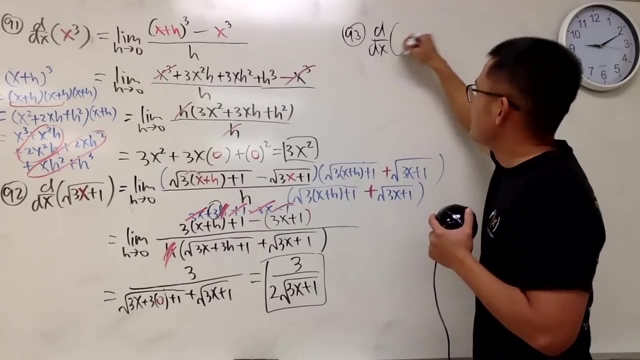 Right Chain rule matters Number 93. I need more space? No, not really. I will see I will try to fit in 93. It's seriously a lot of fun to just try to fit in a lot of like crazy computations and all that things. 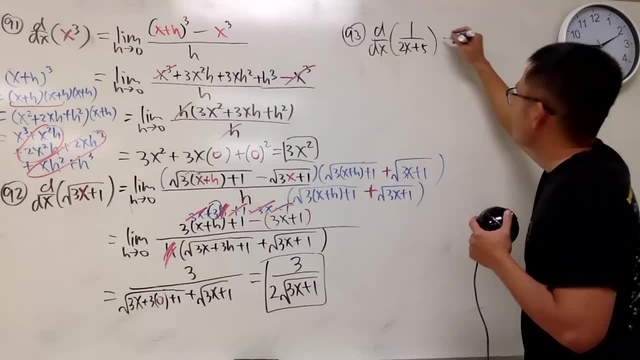 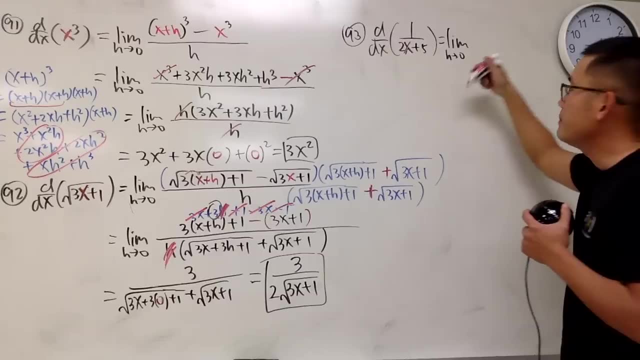 2x plus 5.. In the denominator, Anyway, here we go, Limit as h approaching 0.. Here is the x, So I will put down x plus h in here. So we have 1 over 2, parentheses: x plus h. 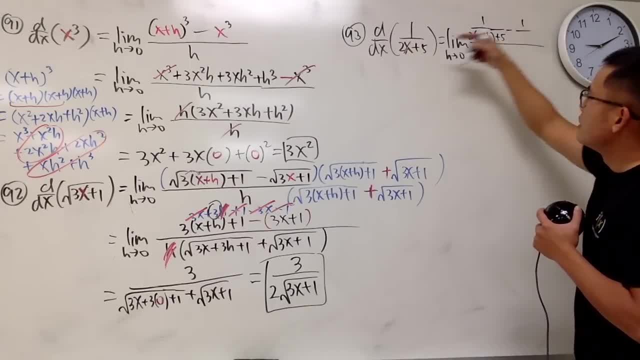 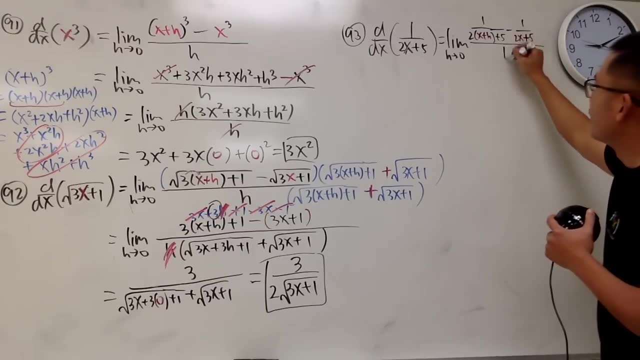 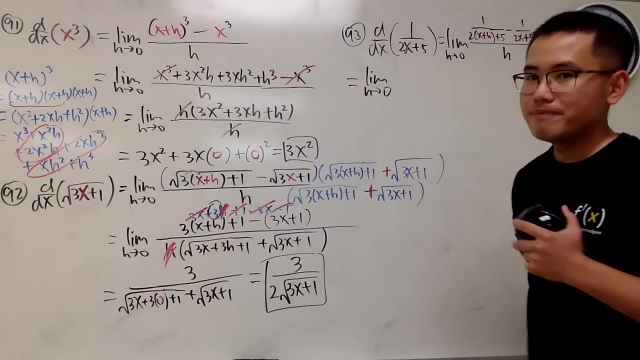 and then plus 5, and then minus 1 over 2,, x plus 5. And all over h, like this. Now take the limit as h approaching 0.. I cannot regret, but I will try to just deal with this. 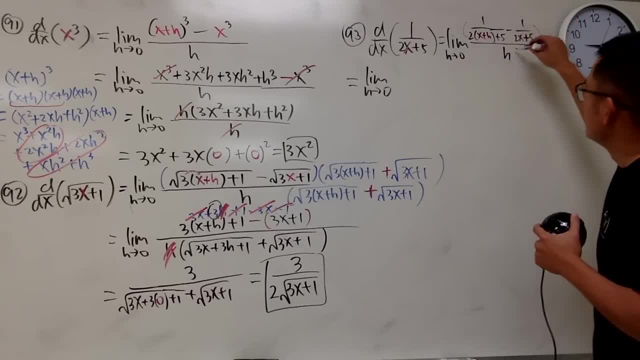 We are going to multiply the top and bottom by the LCD, Okay, So, yeah, I don't know if I have enough space. Okay, We have done a lot of LCD already, so let's not show work on this one, Okay. 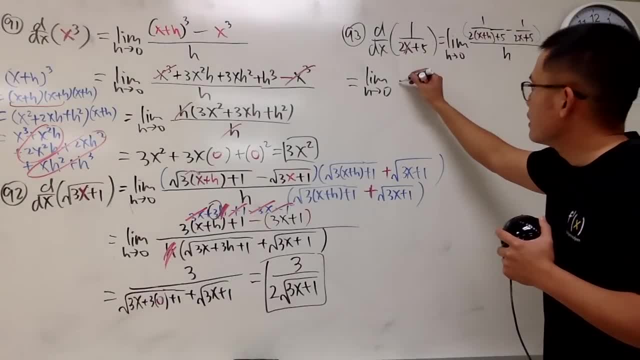 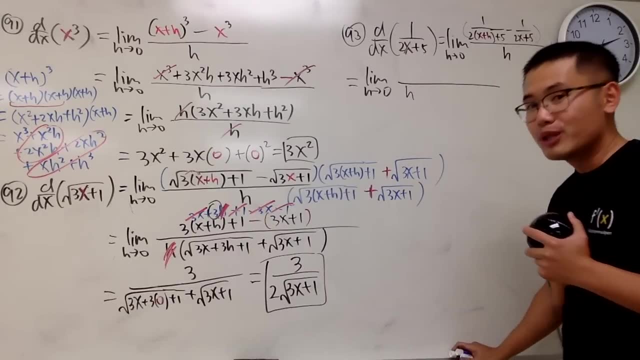 So I will just show you, guys, what we can do. Here is the deal h on the bottom h. You multiply the top and bottom by this and that, namely the LCD, And when you do that, you pretty much have parentheses with this. 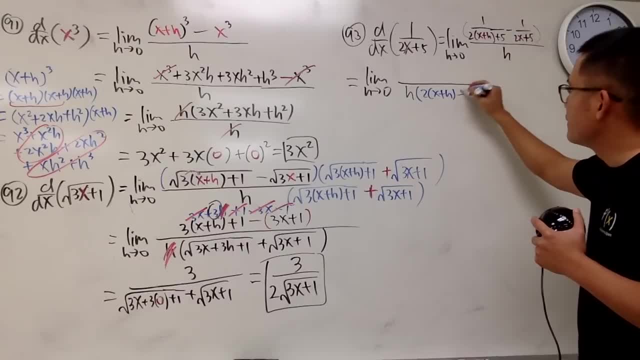 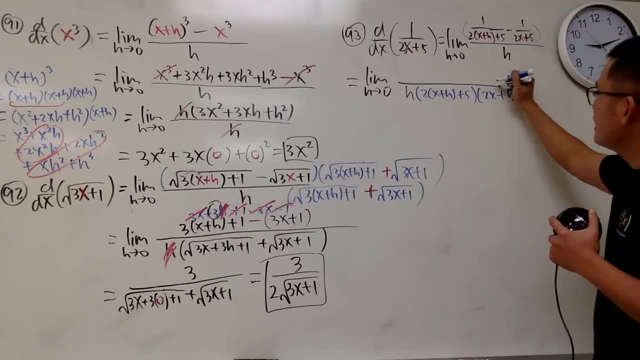 namely 2 parentheses x plus h plus 5.. That's this denominator. And then you multiply by 2x plus 5.. Yeah, And then, remember, we are multiplying this, this and that on the top and bottom. When you have this multiplied with the top, you have this right, here only. 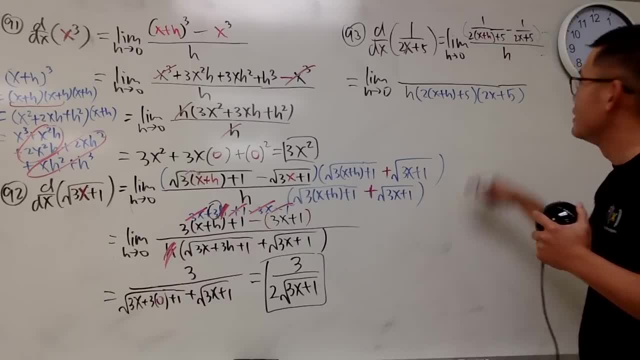 Because this and that will cancel. Just multiply it out. you know You pretty much have 2x plus 5. Right here And then minus. you pretty much have this right here. So just do this and do that. That's the best way to do it. 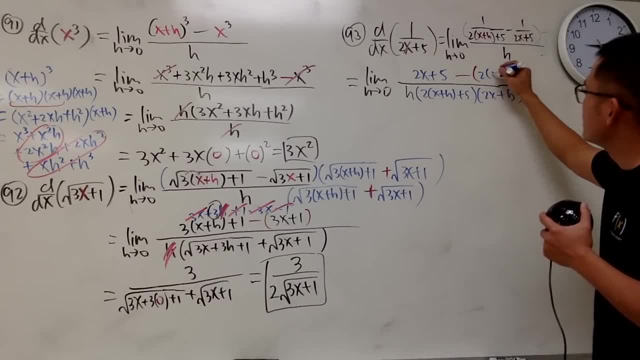 Minus. you pretty much have this right here. So just do this and do that. That's the best way to do it- Minus parentheses, and here you have 2 parentheses: x plus h. Why don't I distribute? I don't know, man. 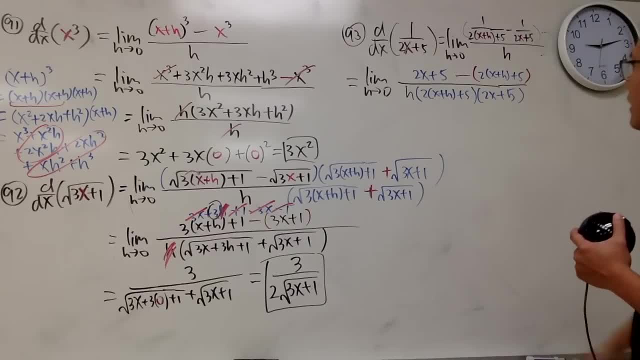 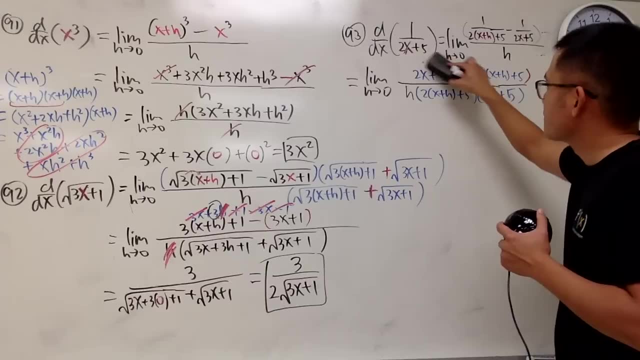 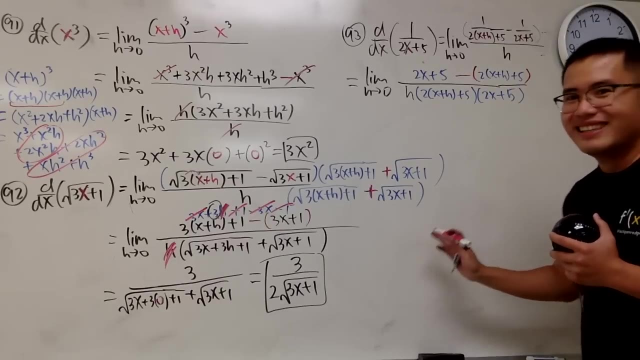 Anyway, this is what we have Now. let's just clean things up. This right here is 2.. See, this is why I don't know, Why don't I distribute, I don't know. Okay, I'm not tired, I can still do this. 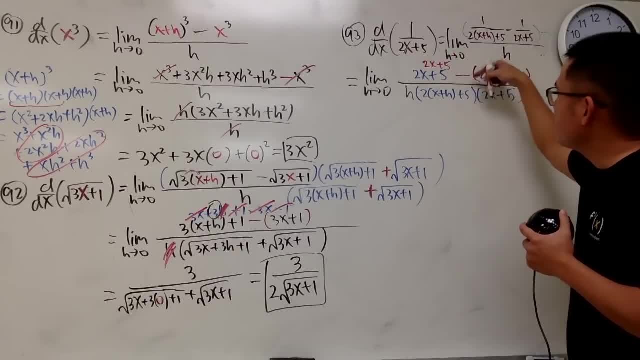 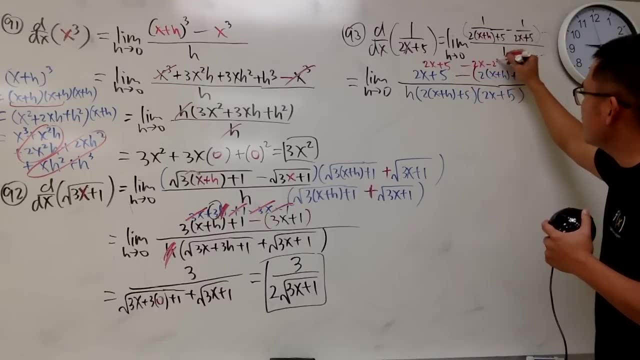 Alright, so here we go: 2x plus 5. And minus, you see, this is 2x Plus 2h, But it's minus, because minus 2x, Minus 2h, yeah, Okay. 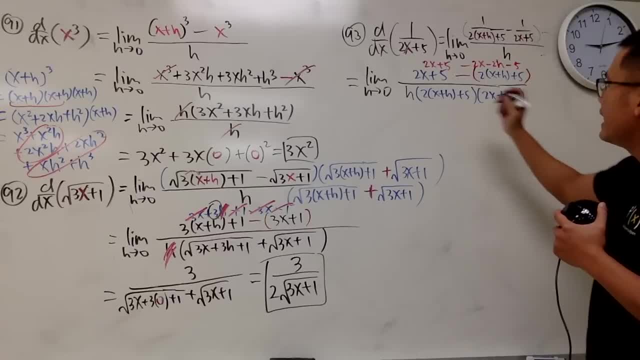 And then minus 5.. Okay, And you see 2x negative, 2x cancel, 5 and negative 5, cancel. You have the negative 2h, You have the negative 2h. This h and that h. 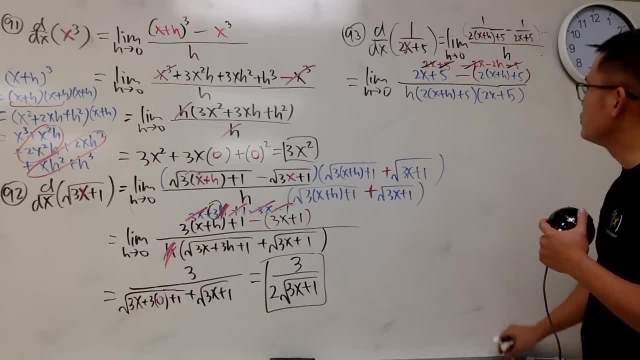 hey, hey, we can cancel that out again, Just like over there. So be sure, You cancel out this right here And you cancel out this right here. It's the idsign. you know: three cancellations And you get the negative 2. 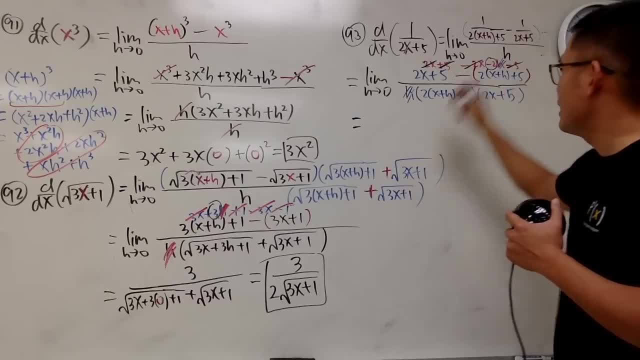 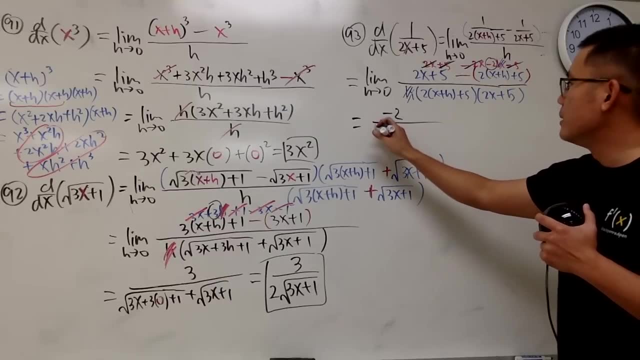 on the top. Don't forget about that. Now on the top we have negative 2 left. On the bottom we're putting 0 for the h right here. That's about all. So we get parentheses 2x plus. 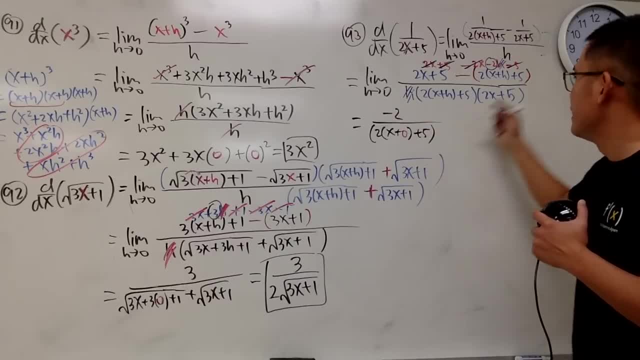 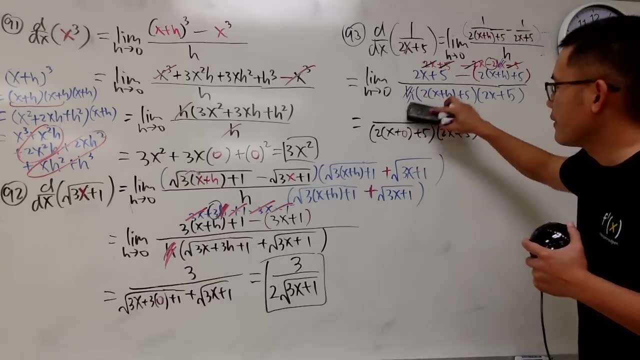 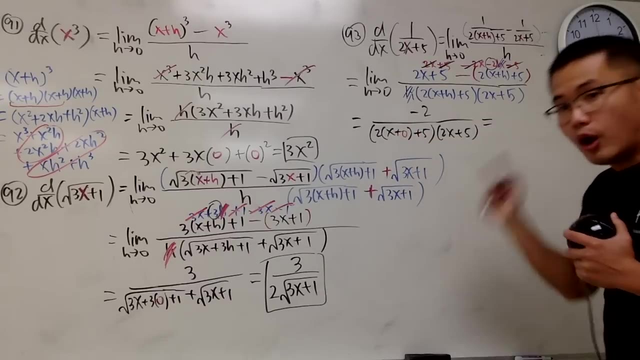 0 and plus 5.. And this right here is another 2x plus 5.. Of course, if you distribute, it's the same thing. at the end, This right here is just 2x plus 5 and 2x plus 5.. 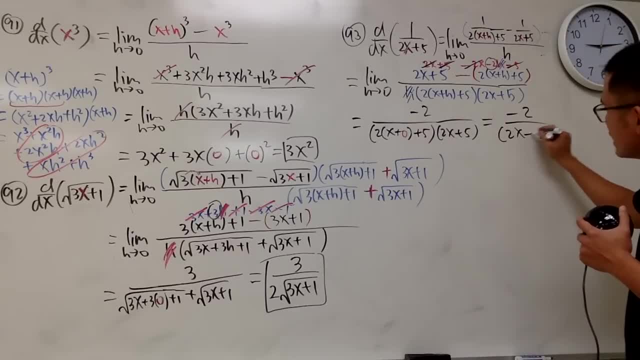 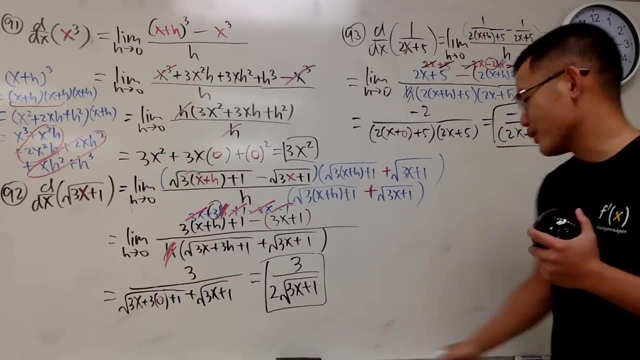 All in all we get negative 2 over parentheses, 2x plus 5 to the second power. Now you can see that this kind of quotient rule or the, if you bring this to the negative 1 power, all that. 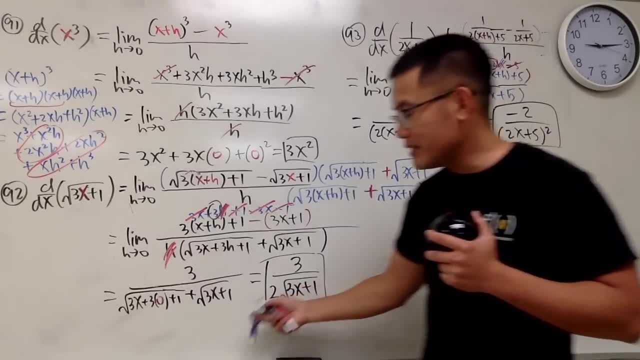 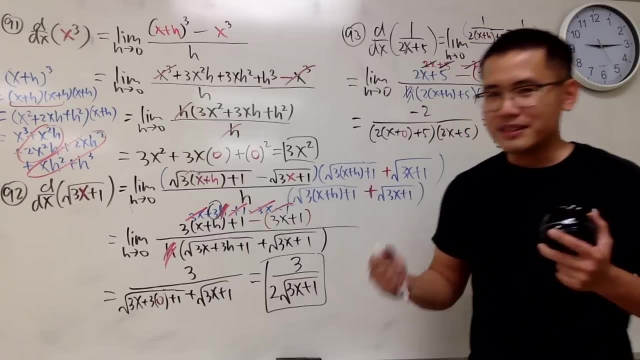 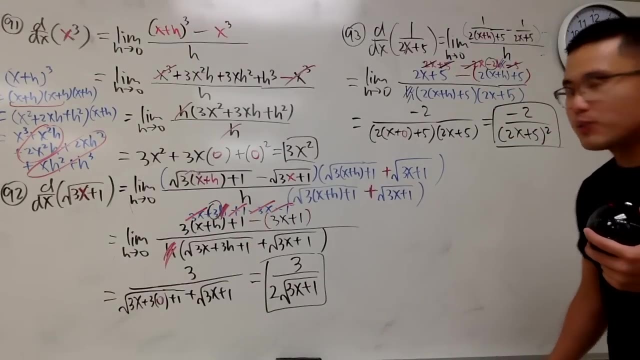 and also the chain rule. they all work legitimately. alright, Don't be afraid of using the definition of derivative. This is, like all the calculus teacher, the things that we want to tell the students. Okay, For the next one, I will have to. 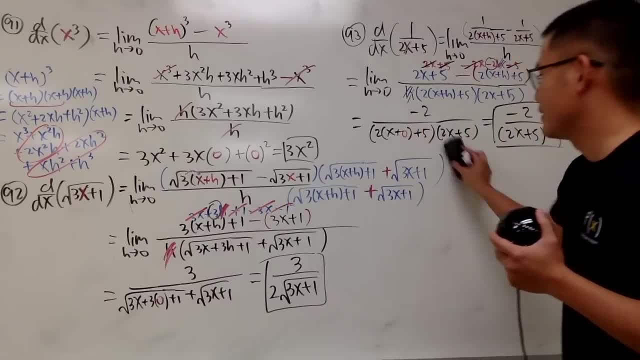 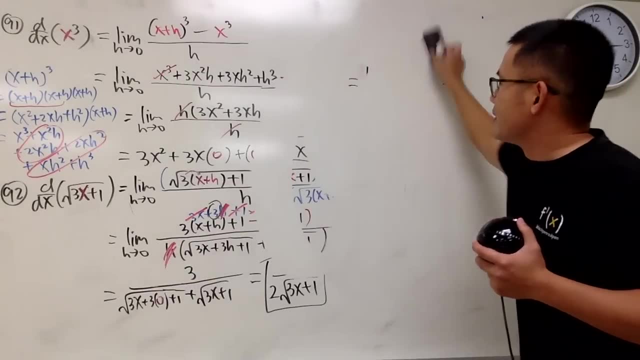 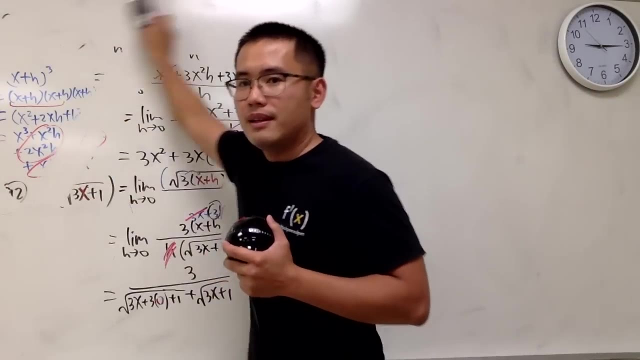 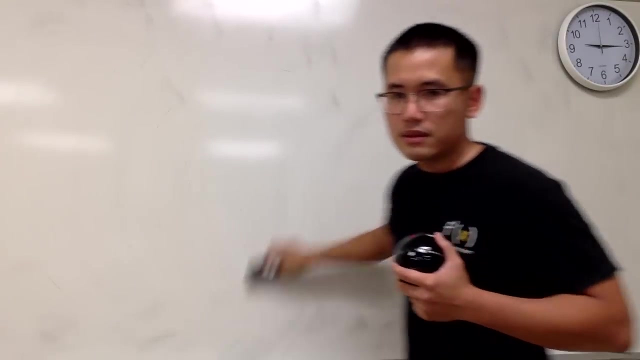 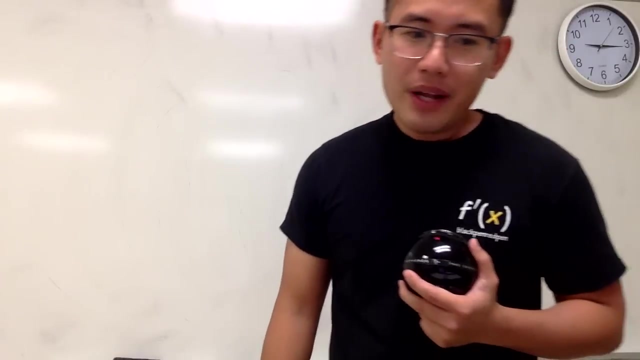 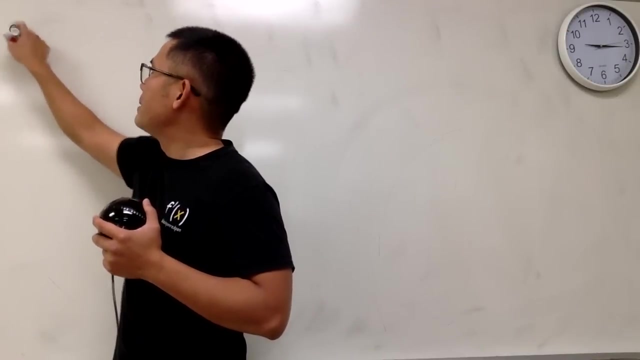 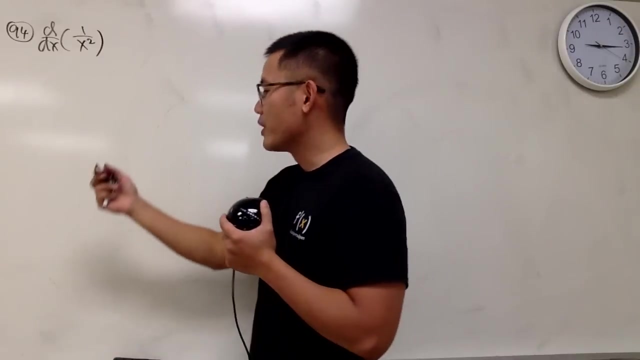 erase the board. This is too long. so yeah, One over x to the second power right, Number 94.. Again, I'm not so happy because the harder ones are coming, But it's okay, We can survive. Here we go. 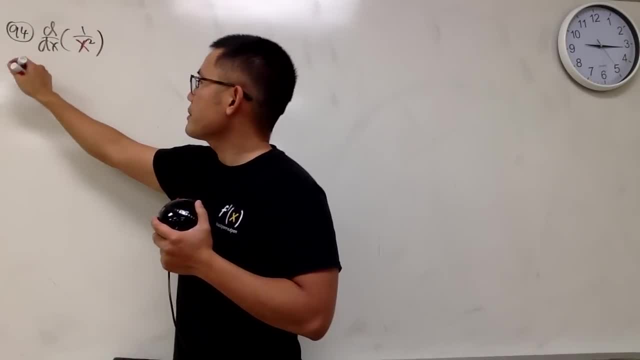 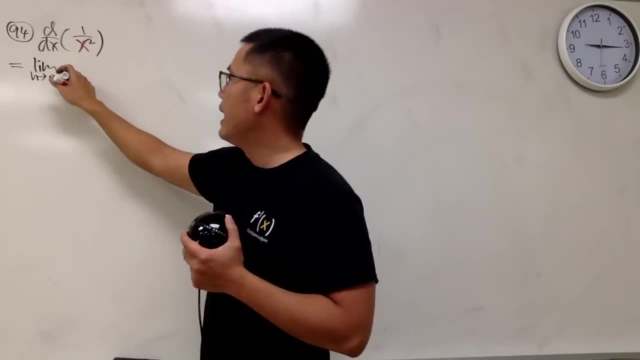 x is right here, so we are going to write it down. I'll put it down right here. Why not? I think it saves some more space. The limit as h approaching 0, and we will just have 1 over parentheses. 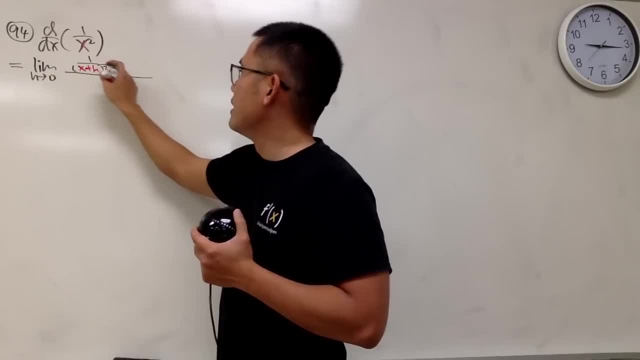 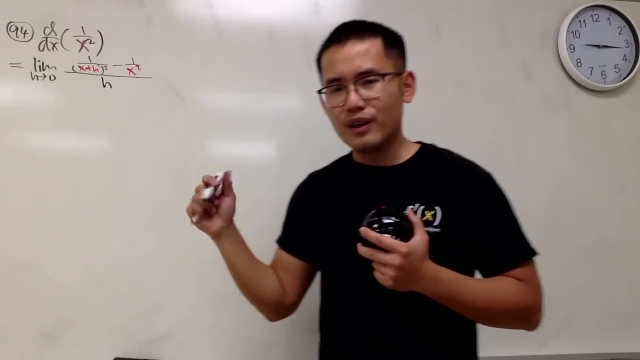 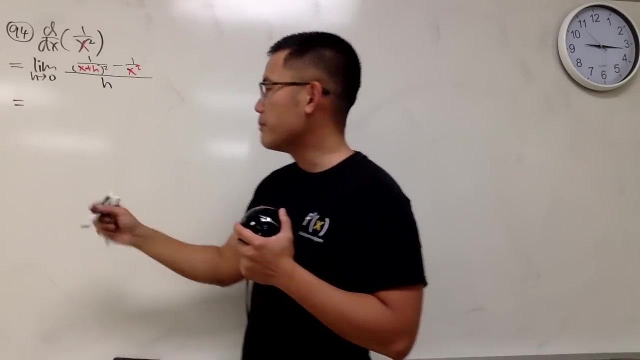 x plus h, square that guy minus 1 over x, squared over h. right here, And let's practice what we did over there. okay, So this, right here: you multiply the top and bottom by this and that, namely this common denominator. 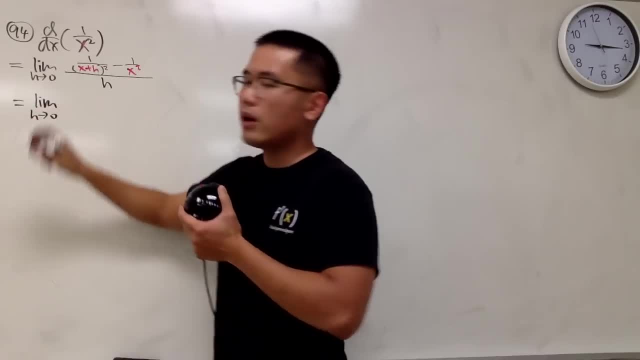 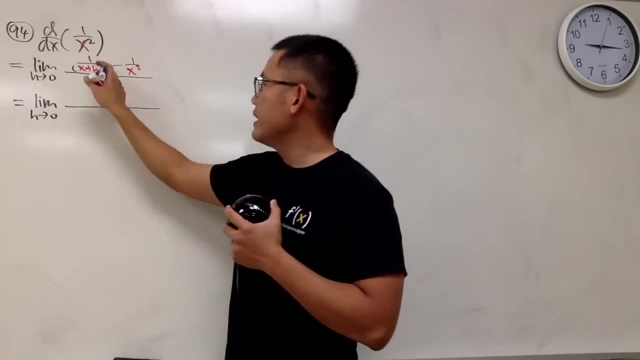 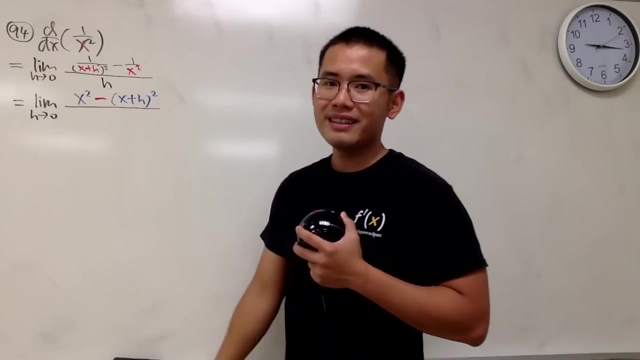 Limit as h approaching 0.. Well, well, you put this right here. you put this right there, So we get x squared minus. you put this right here, so it's parentheses: x plus h squared, okay, And then the bottom is just h. 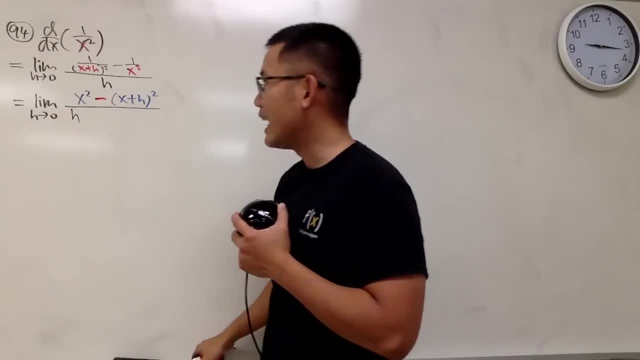 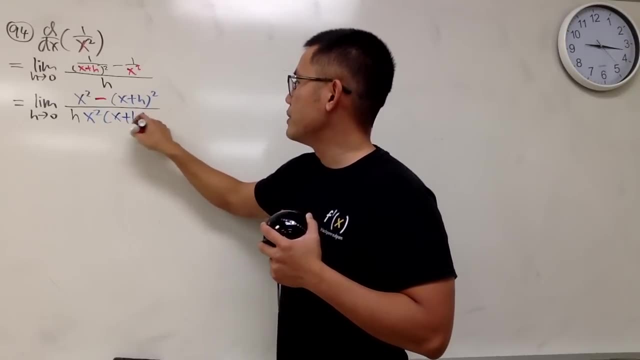 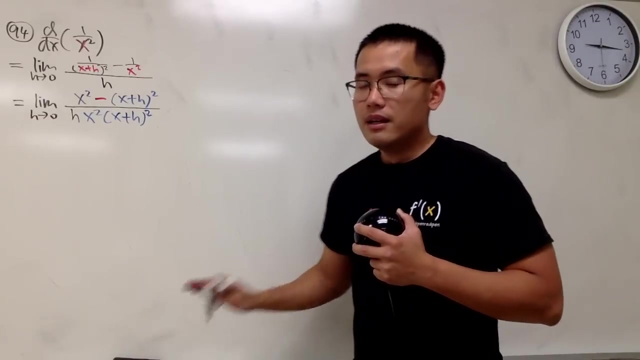 in black times this and that. So I will put down x squared, first parentheses, and we have x plus h squared like that. Okay, Here it's a common mistake Some students, they just like to cancel this out and then cancel this out and 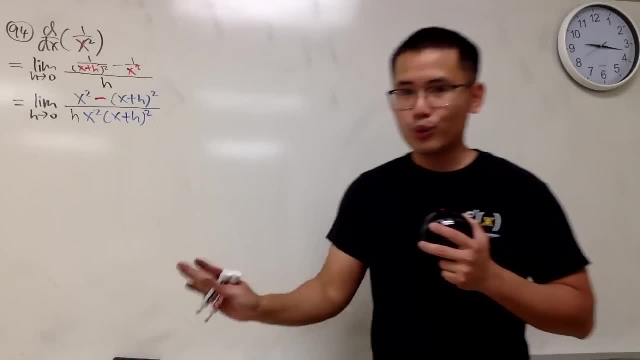 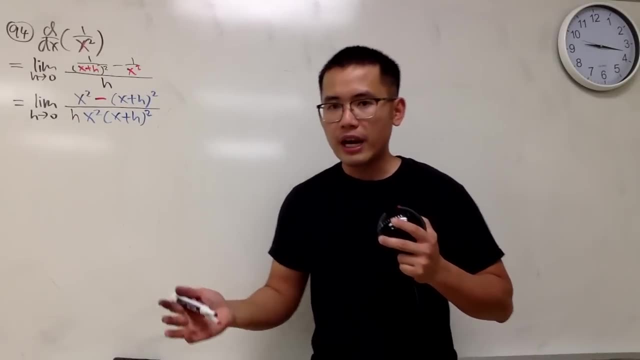 no, you are forgetting the minus sign between. so don't do that, Don't do that. You can do the difference of two squares, you can factor it out and you can simplify it. That's okay, But I find it easier. 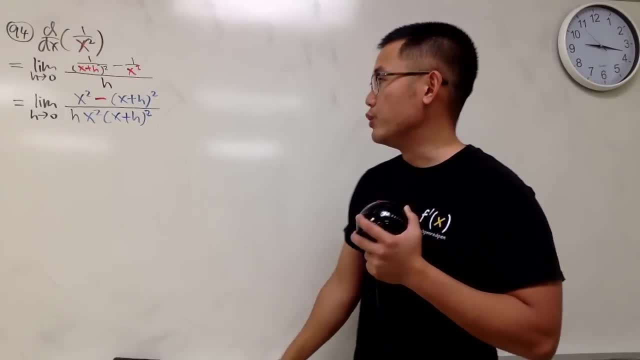 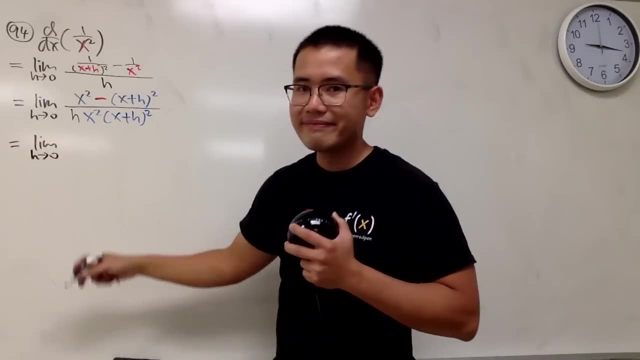 to follow, in the sense that if you just multiply this out and then just reduce, So that's what we will do. So let me just write it down again: This is the limit as h approaching 0, and we have x squared and this is: 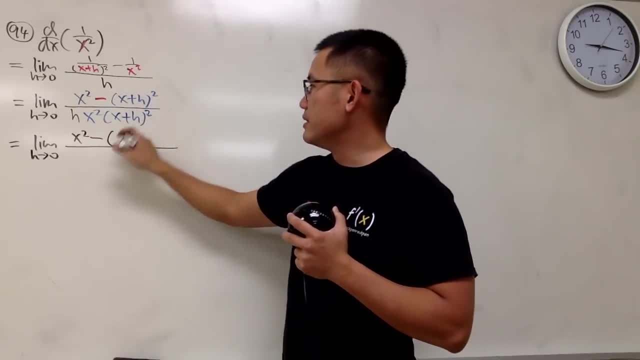 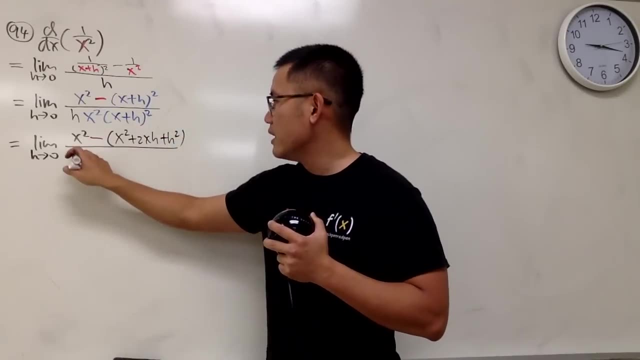 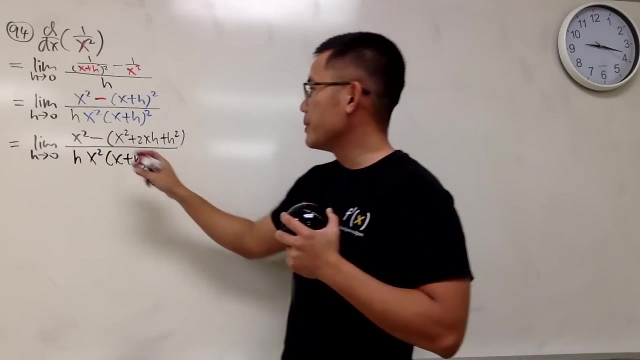 minus. When you multiply this out, this is just going to give you x squared plus 2xh plus h squared, And we have all this, Then the h times x squared, times x plus h squared, like that. Now, be really careful. 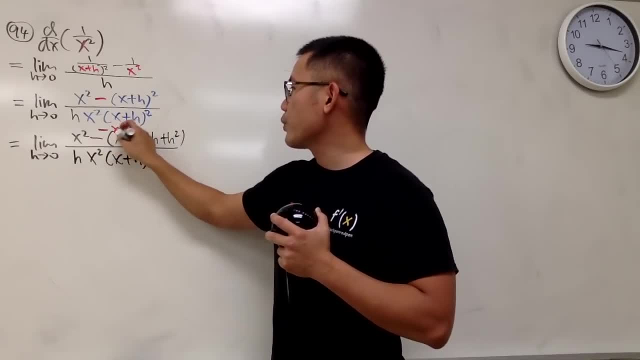 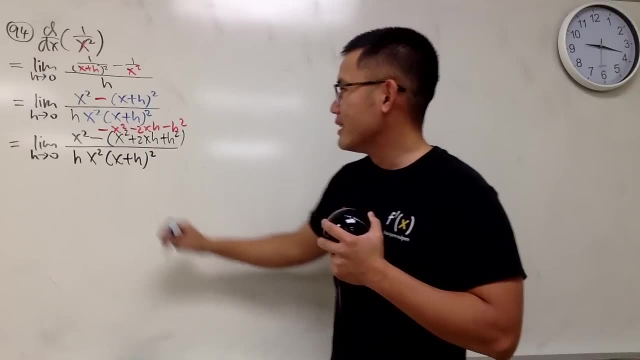 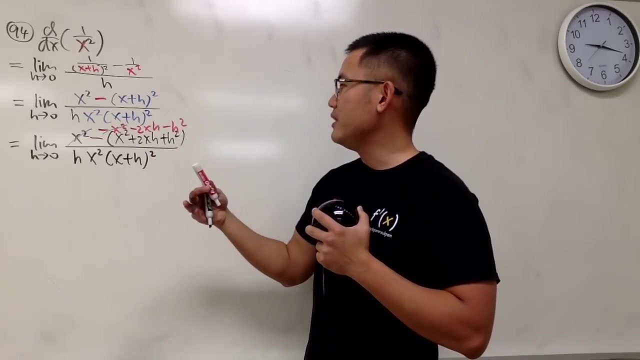 you have to distribute this, so it's actually negative x squared and then negative 2xh and negative h squared. Well, well, this is x squared, this is negative x squared, so they can be canceled. On the top they have the. 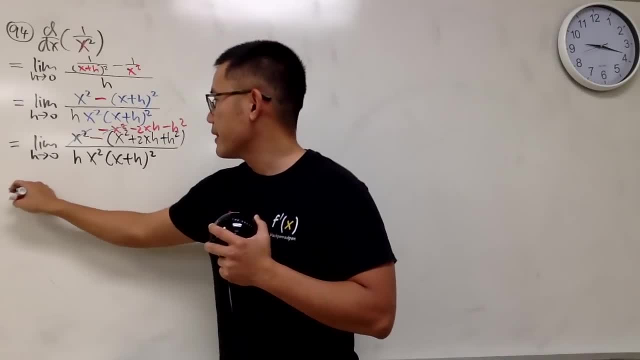 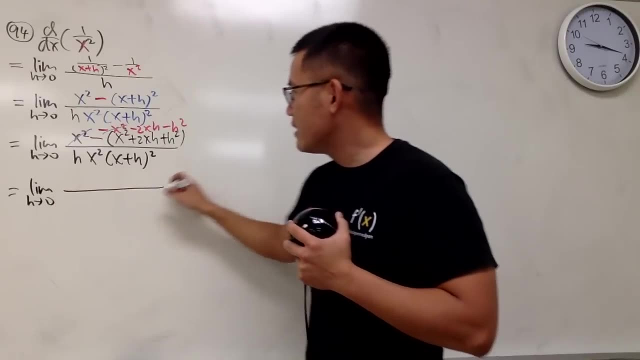 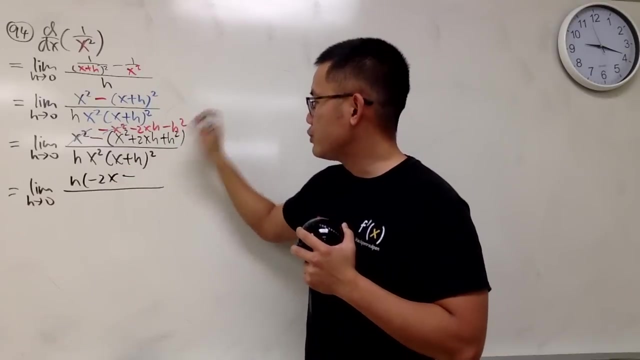 h left so we can factor an h. So let's see this is the limit as h approaching 0.. When we factor out the h, we will have negative 2 x minus h to the first power, like this over this h. 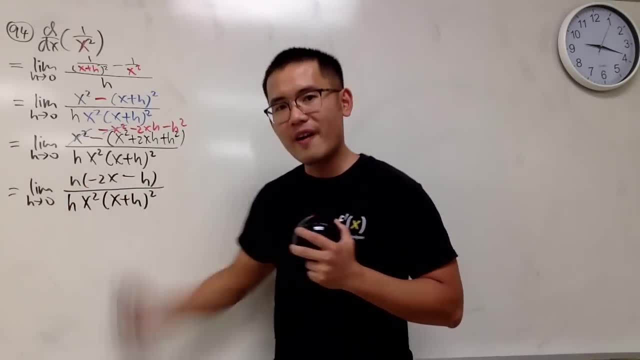 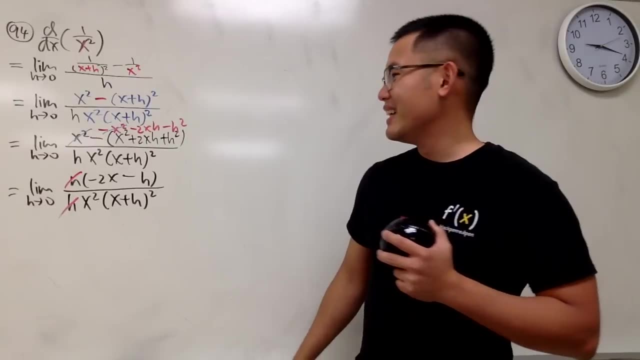 times x squared, times x plus h squared like that. So good. The moment you cancel the h, it's the h. So good, Now we can just put the 0 into the rest of the h and we'll be done, and then just simplify. 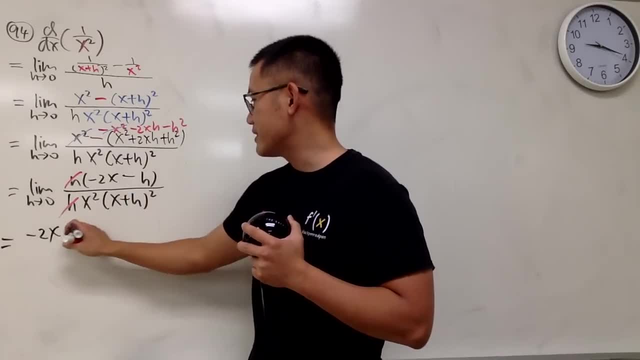 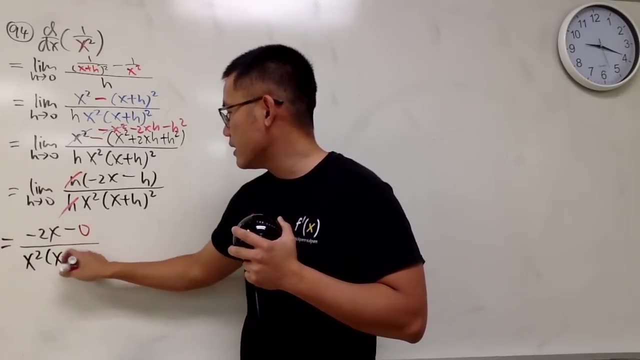 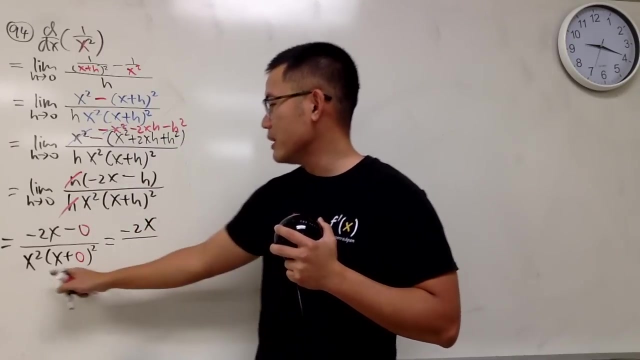 if you need to. On the top it's negative 2x minus 0.. On the bottom, this is x squared times x plus 0 in here and we square that Well. well, On the top it's negative 2x. On the bottom, this is: 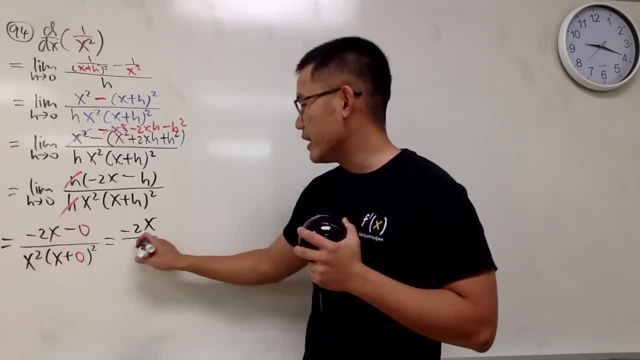 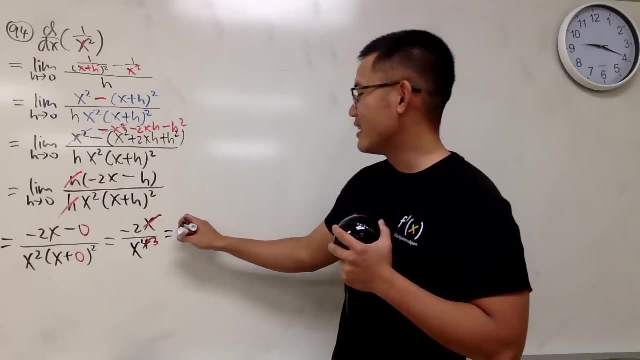 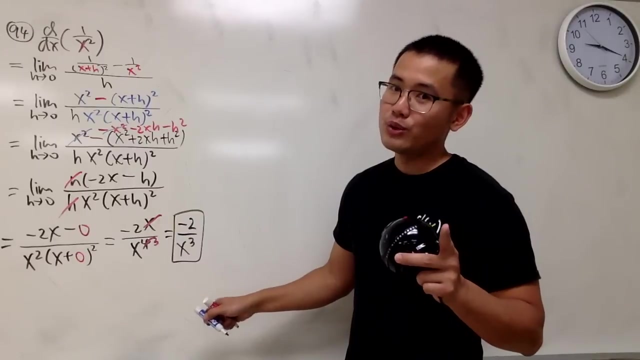 x squared. This is also x squared. Multiply them, we get x to the fourth power. This and that can be canceled. Finally, we get the answer negative: 2 over x to the third power. I know what you guys want me to do. I know. 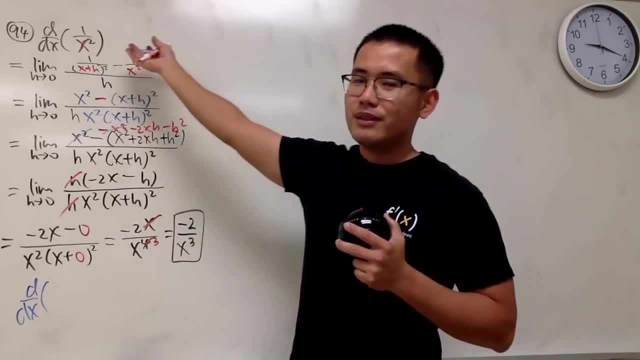 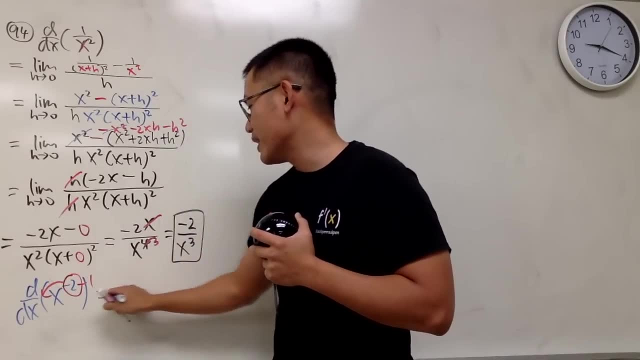 I already do d dx. Hey, this is just x to the negative 2 power, isn't it? Why don't I just do this front minus 1 and we get negative 2, x to the negative 3, which is the same as that. 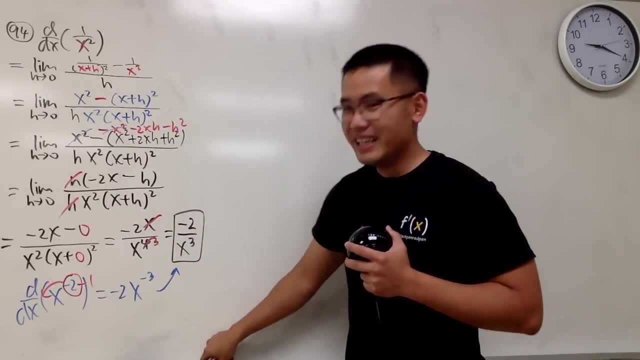 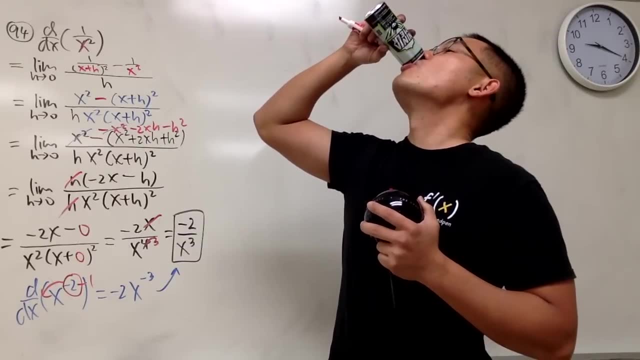 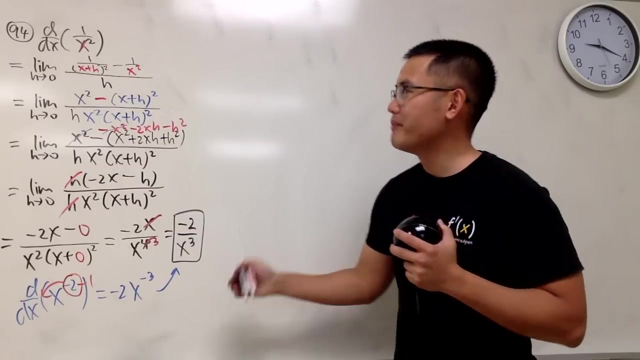 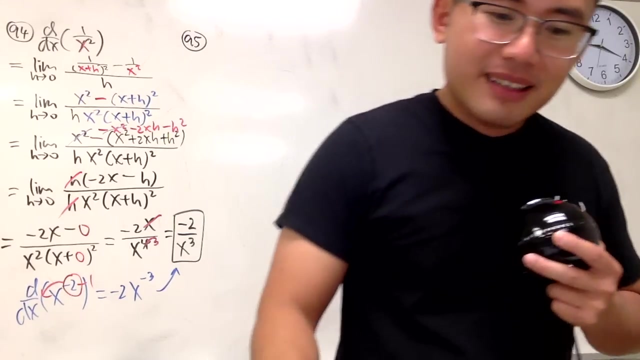 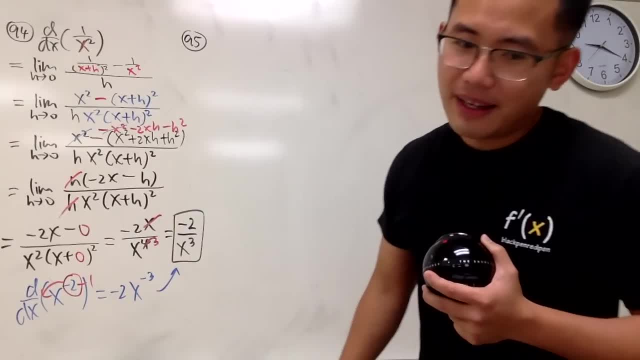 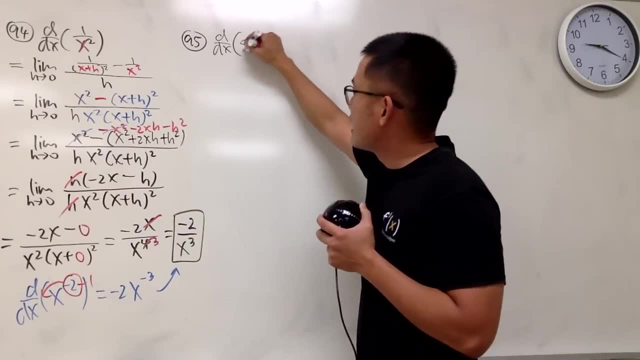 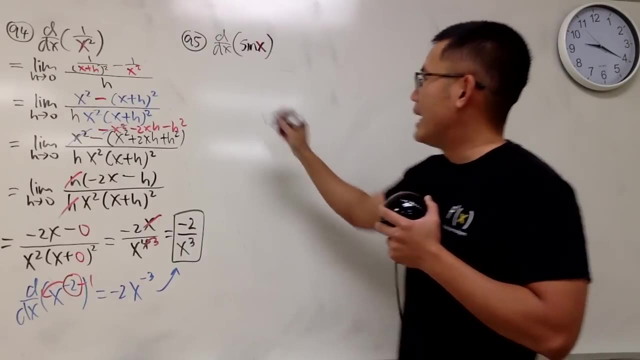 that I'm like I didn't put any easy one. at the end I will just show you Sine x. Okay, Here is the input. Sine of x, They are not so bad, It's just a lot to write Especially. 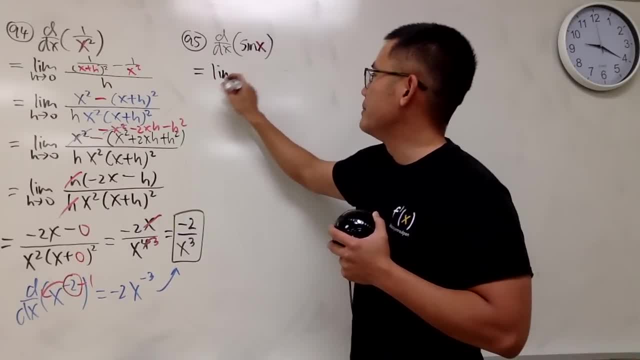 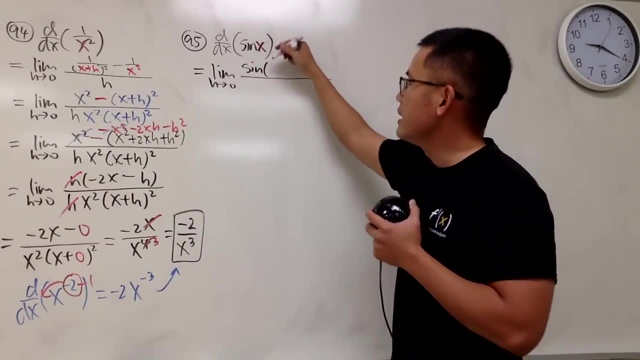 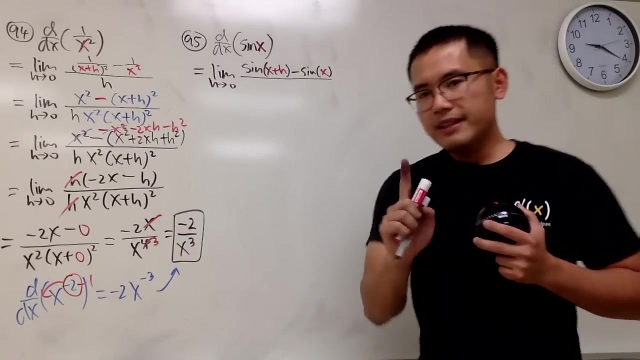 once it's a 90 something question. it's just tiring. Anyway, take the limit as h approaching 0.. On the top we have sine. open the parentheses. here we have x plus h minus sine of x, Like this This time: 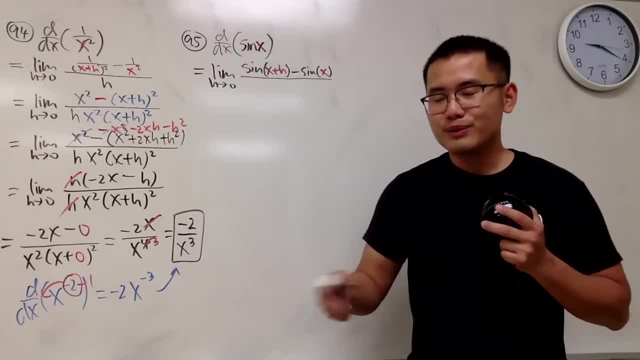 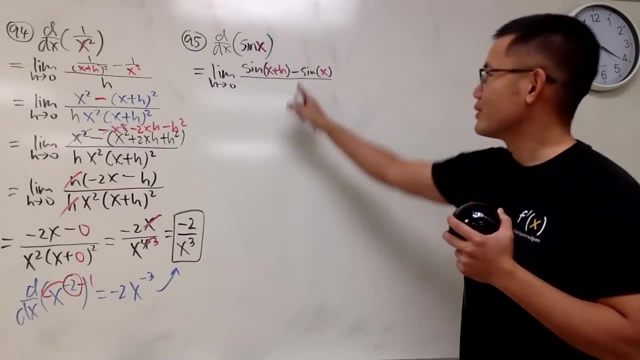 be really careful. We are using h as a variable. It's not sinh, okay, Not yet. No, we don't do definition with sinh, No, no, no, Just regular sine, Okay, Anyway, this is over h. 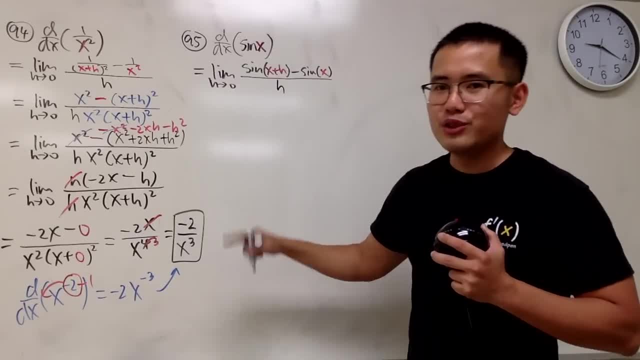 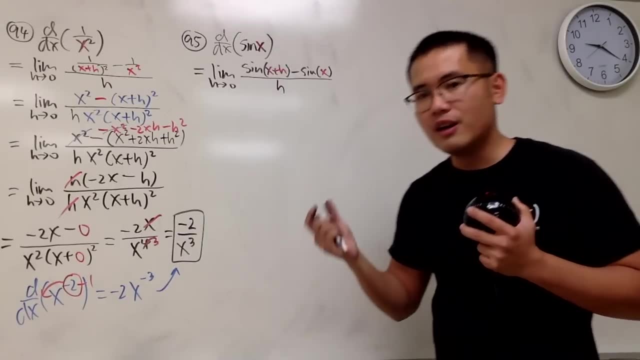 Here is the deal: Do not multiply the conjugate, Do not get whatever. The way we do is look at this: right here We have the angle sum formula for sine. So we do that With that said, this right here is the limit. 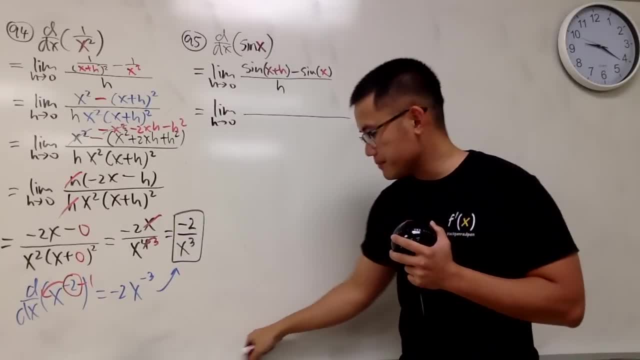 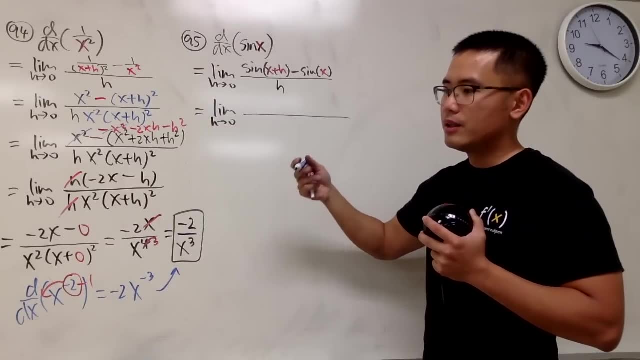 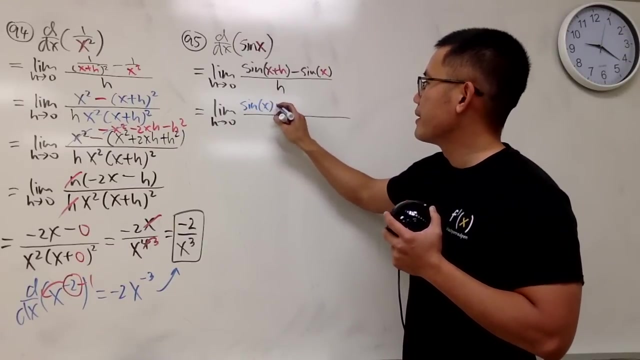 as h approaching 0.. Let me just tell you guys that Sine of a plus b is sine a cosine b plus sine b cosine a. So here, sine of x plus h. let me write it down: We have sine of x times. 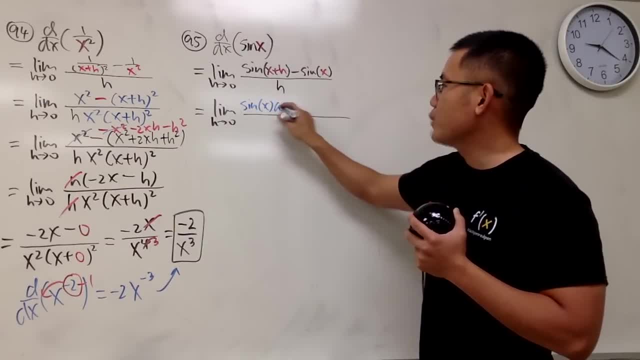 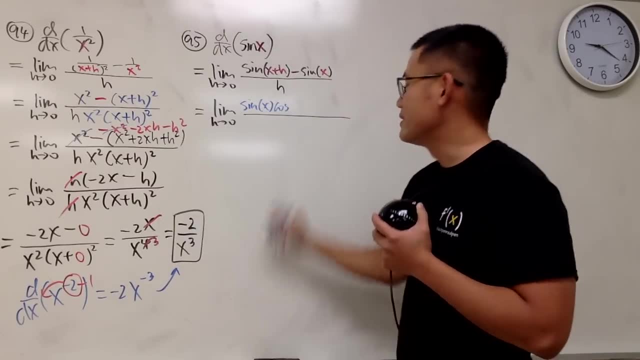 cosine of h. And for this one I really have to put a parentheses just to make sure that you guys know this is not cosh anymore. Cosh left us already. okay, This is not cosh, It's cosine of h. 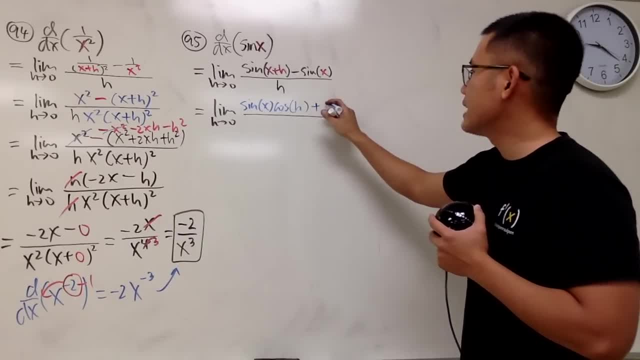 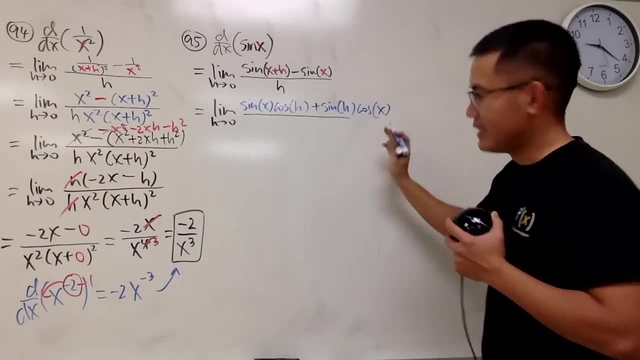 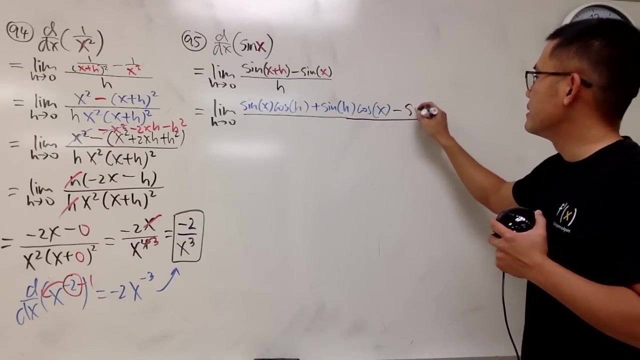 Cosine of h And then plus sine of h, okay, Sine of h times cosine of the first, which is x, Like this: This is the angle sum formula for sine, regular sine, And then minus sine of x, like this: 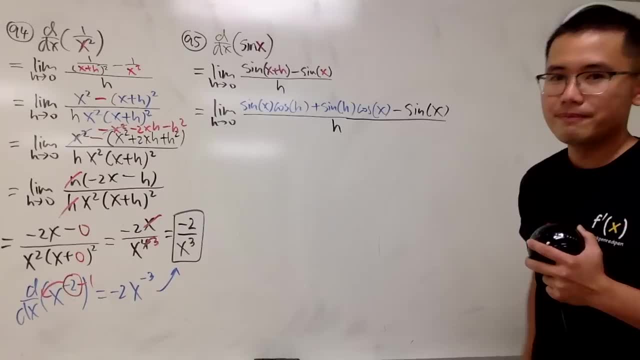 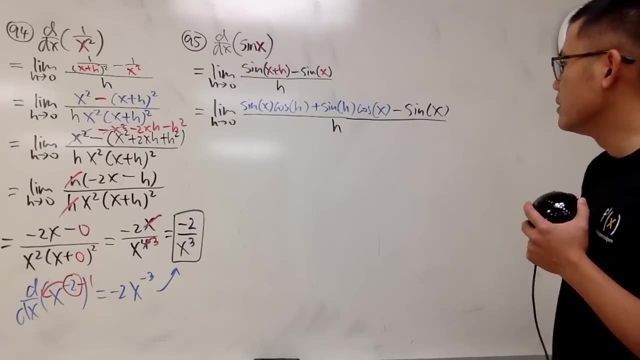 All over h right here. So this is all good. Now here is the deal. If you take a look, hmm, Let's see, This one has sine of x. This one has the minus sine of x as well. This is what we like. 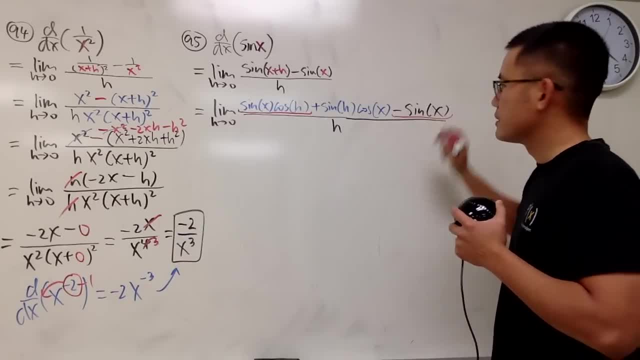 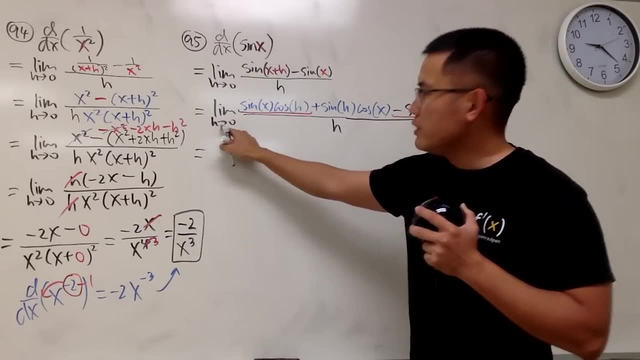 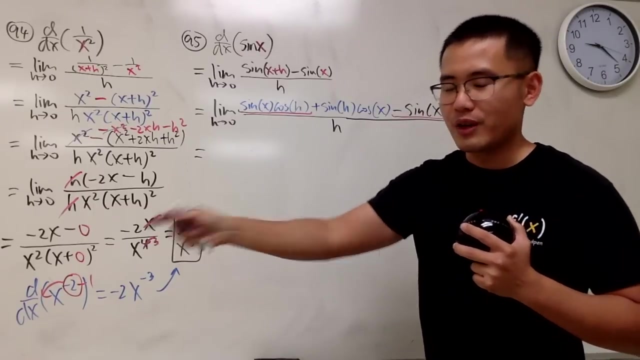 to do. I'm going to pair this up with this, Okay, And you see the following: When you are talking about h is approaching zero, that means in the h world in the limit sense. okay, That means x. it's like you can just bring to the front, It's not. 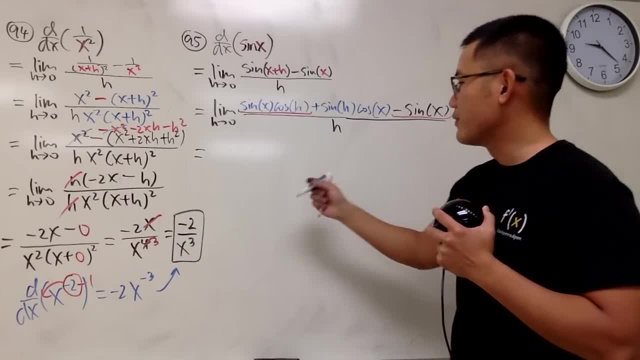 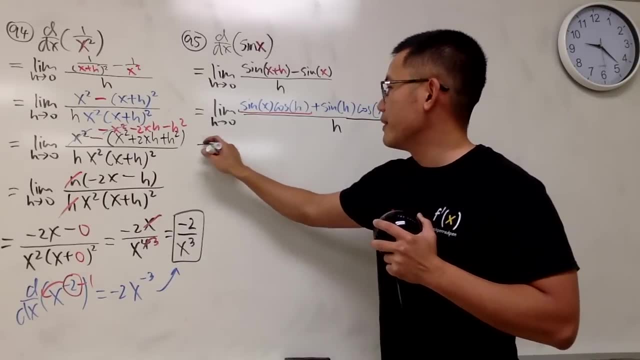 It's not affected by the h, So I would like to write this down for you guys. as I said, It's not hard, It's just a lot to write. Let me write it down. This is the limit as h approaching zero. 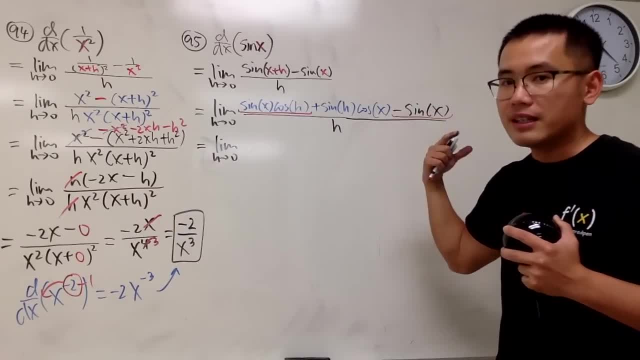 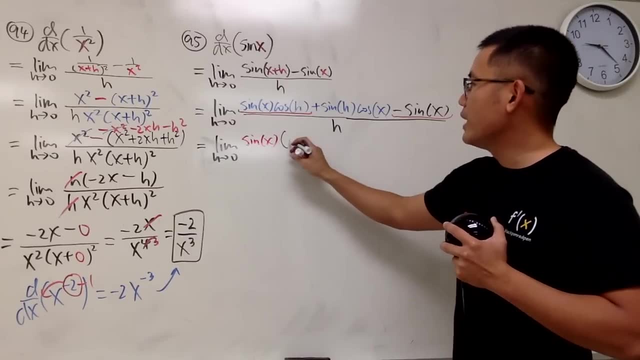 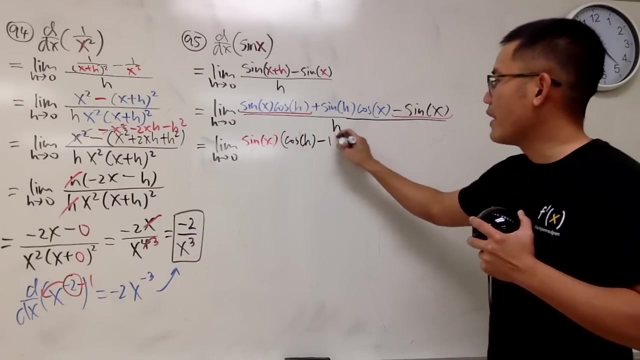 I'm going to put this and that together, but because both of them have the sine, so I can factor out the sine of x, isn't it Okay? And right here we have cosine of h, Cosine of h Minus one after: 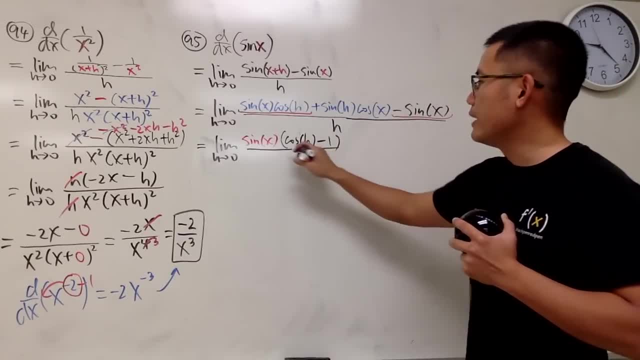 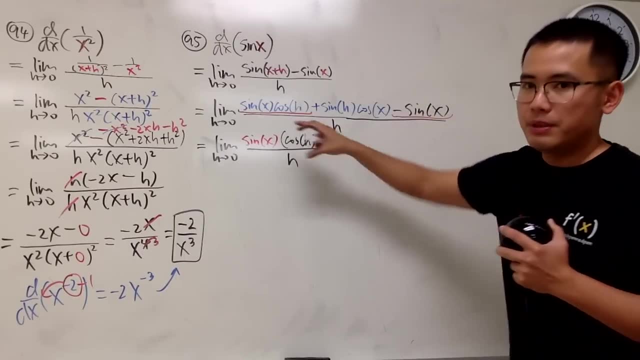 we factor that out And then we have this over h, of course, because the denominator is over h, And then we can say we plus. I'm just splitting the fraction right now. Here we have sine h, cosine x, But let me write down: 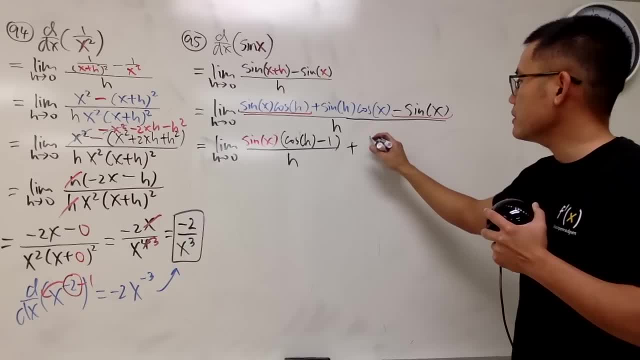 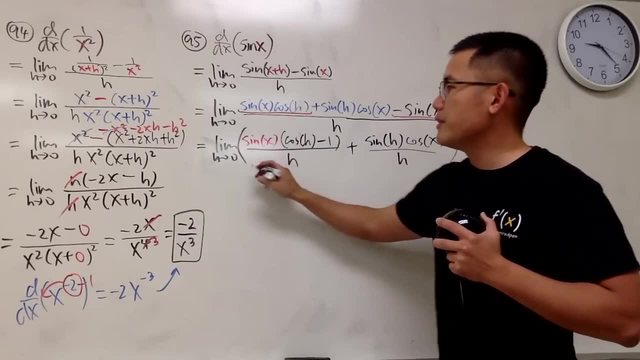 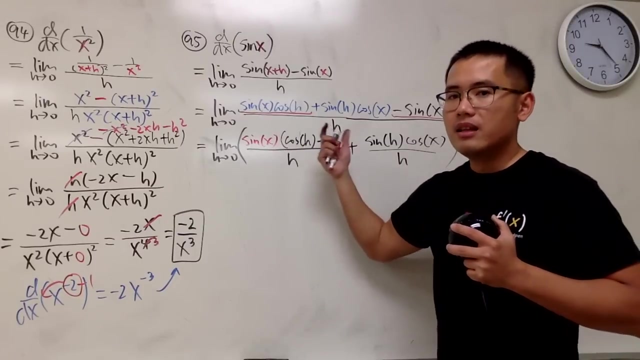 the cosine x right here. Let me just write it down like this: Sine h, cosine x, And this is also over h, And we are taking the limit for this right here, Right Now, by the limit laws. we can say the limit. 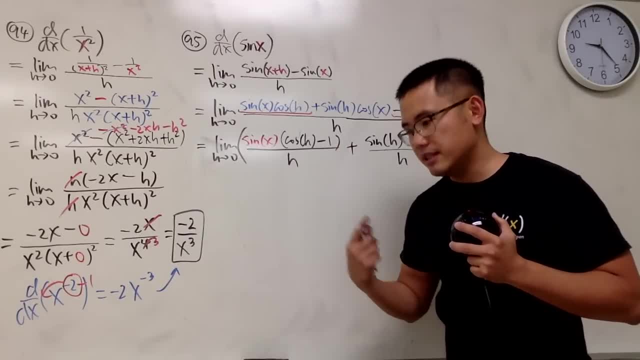 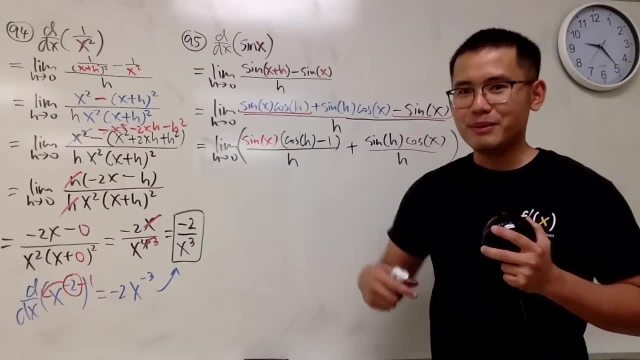 of the sum is the sum of the limits, if both limits exist. And also the limit of the finite product is the finite product of the limits, if the limits exist. Okay, So I did say that, And now I'm going to write it down. 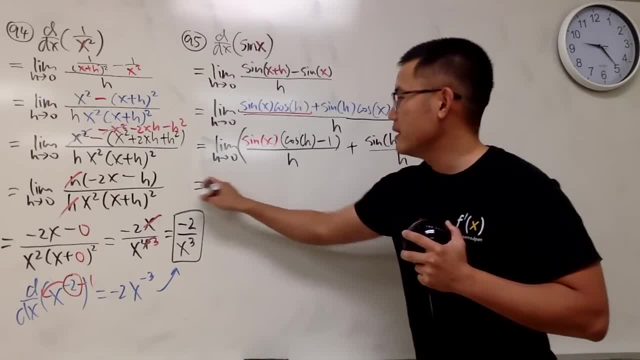 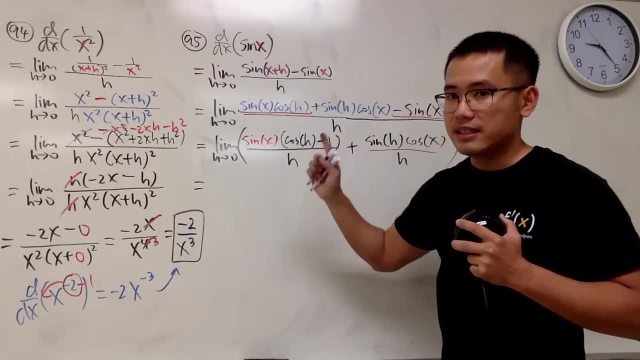 in action. for you guys. What I mean by that is: I can say the limit of this plus the limit of that. Okay, And again, h approaching 0, the x doesn't matter, So I can put the sine x in the front first. 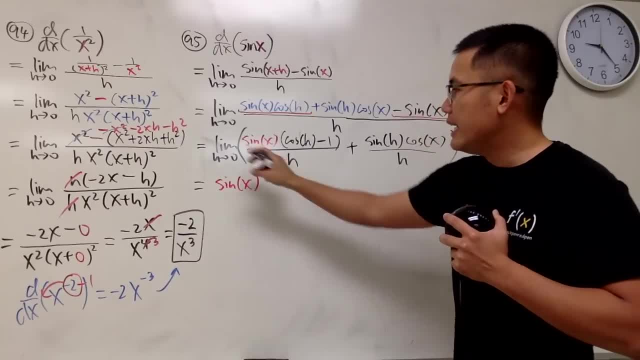 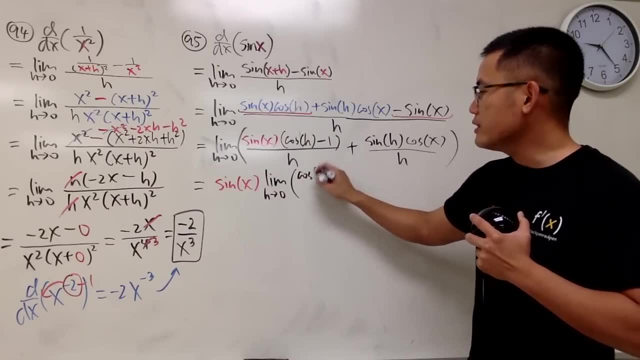 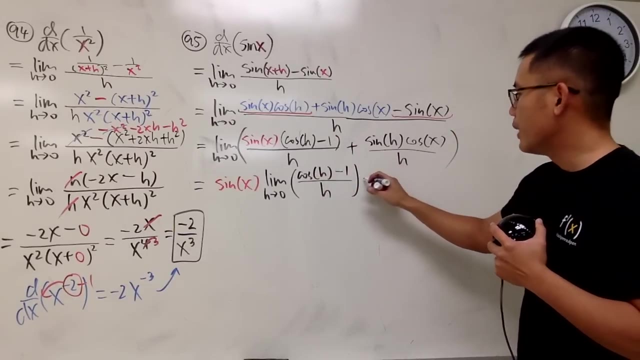 Sine of x Right here, And then I'll just focus on taking the limit as h approaching 0. And we are looking at this part, namely cosine of h minus 1 over h. Okay, And then we are going to add: 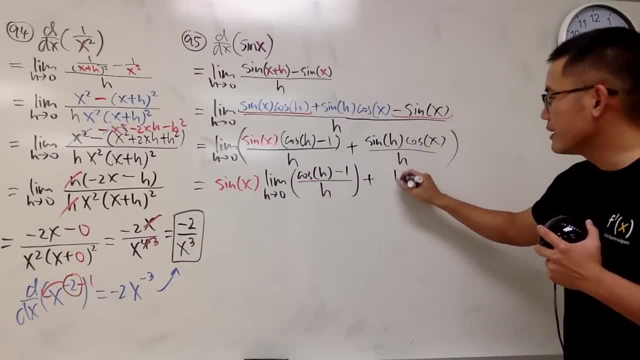 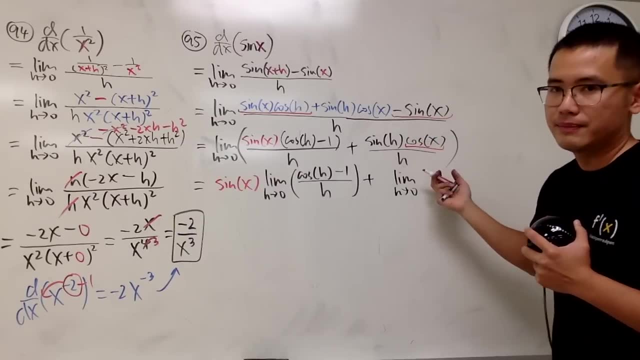 we are taking the limit of this guy. Okay, We are taking the limit of this guy as h approaching 0. But notice, here we have the cosine of x. In the h world, the cosine x doesn't matter, So we can just put that in the front. 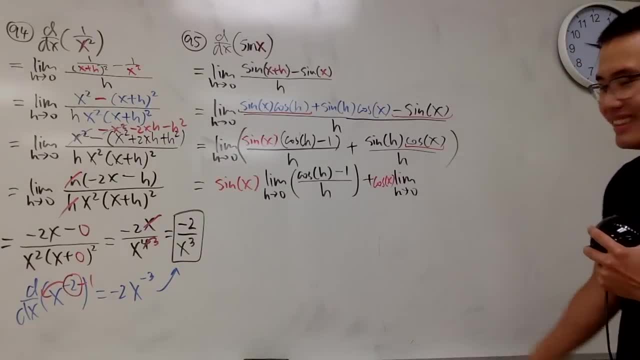 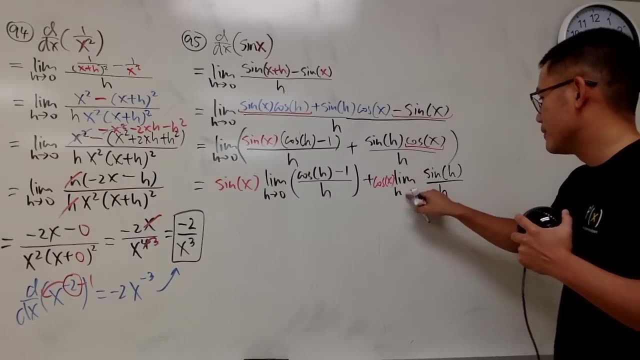 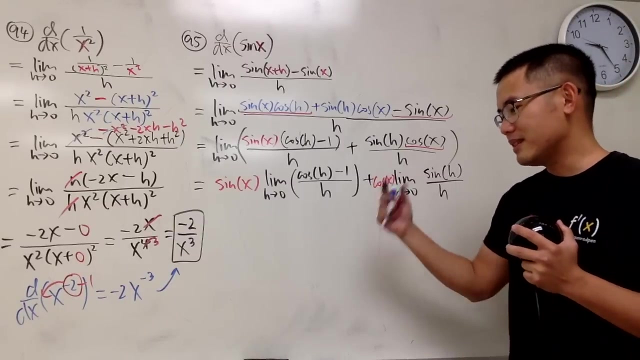 Right, We're not looking at the. there's no h right here, And then the left over right here is sine of h over h, Like that. Alright, Now this is the part that has a lot of the controversy. This is the most. 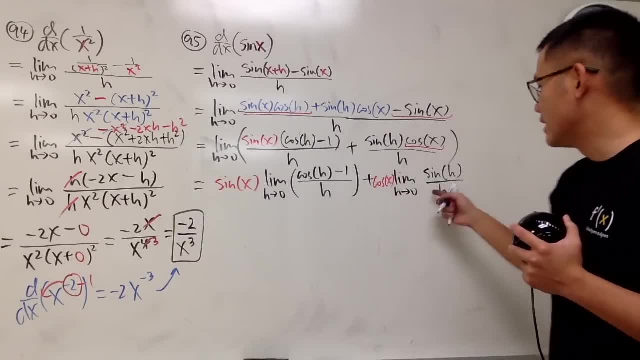 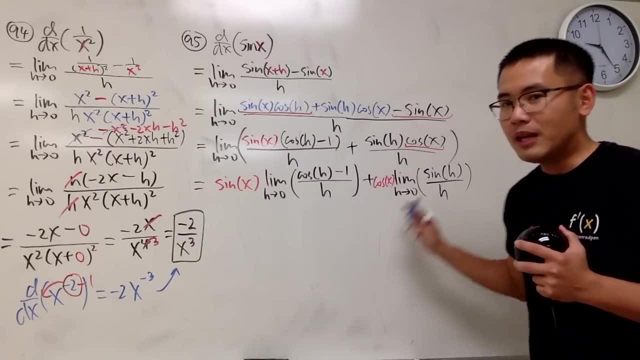 controversial part. What's the limit of this, What's the limit of that, Especially this one? I call this the limit. You don't do Lapito's rule to figure out this limit. You don't do like derivative Taylor series, whatever to do this. 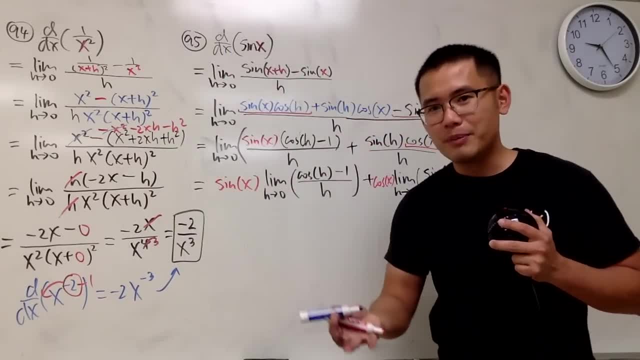 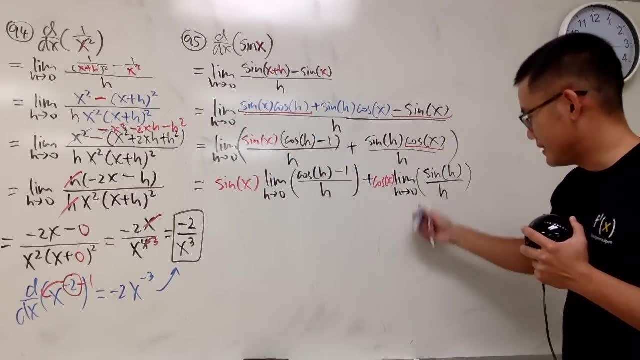 Because we are trying to figure out the derivative sine x. If you only use Lapito's rule, you have to know the derivative sine x in the first place, But we don't. So let me just tell you guys in blue, This limit. 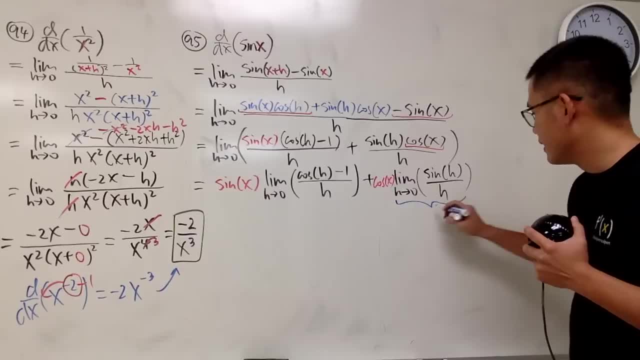 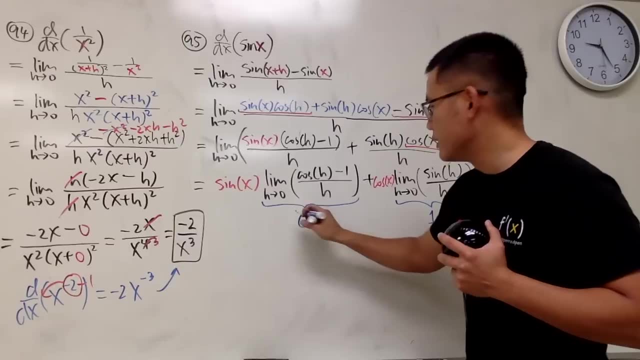 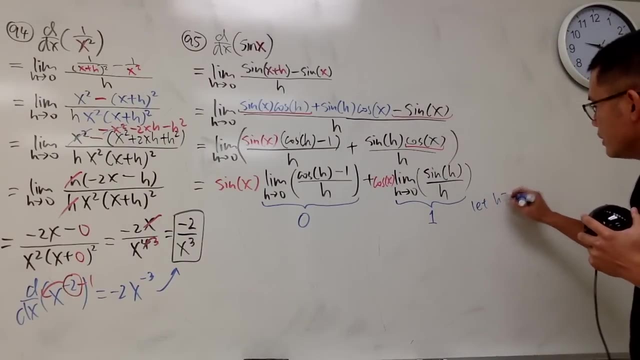 right here. this limit right here is equal to 1.. And this limit right here is equal to 0.. One way you can do it is you can just let, for example, h equals 0.00001 and you put it into here and put it into here. 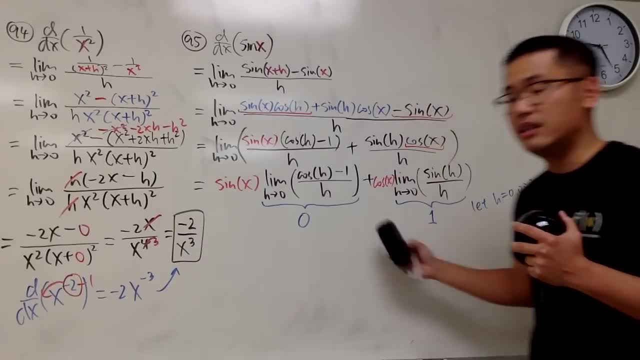 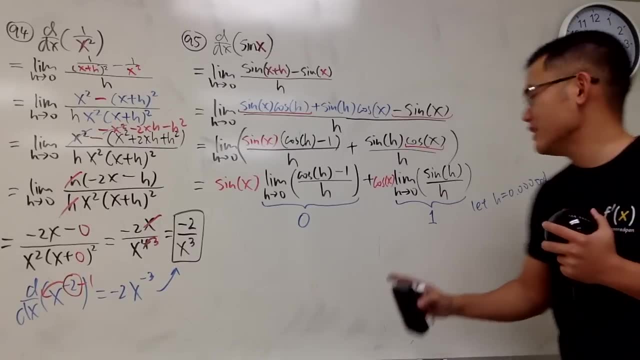 and you'll see the number is approaching 1.. That's the limit. The limit is 1.. Of course, you have to just do even more zeros and you'll see it's approaching 1.. I will be much happier if you do this kind of. 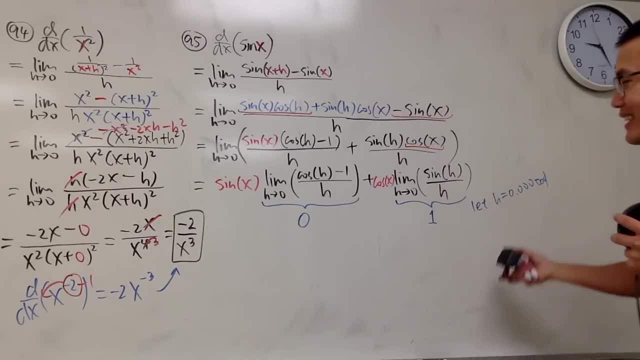 things right here and say the answer is 1 rather than hey, Lapito's rule and all that stuff, No. And keep in mind: h right here has to be in radians. Why I will let you guys know later on. 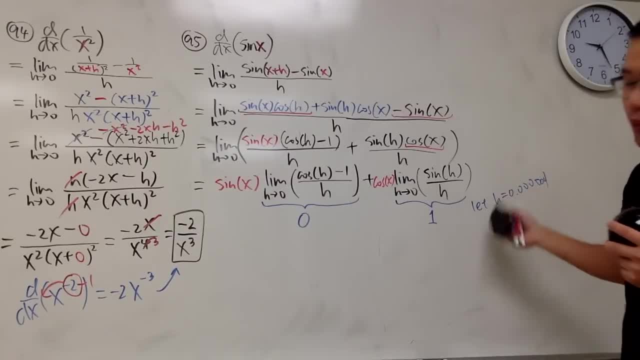 I will do another video for it. So this is one way to do it in the. you know, just use a calculator for it quickly. Or you can also do geometry, okay. Or secondly, I'll just put on one. 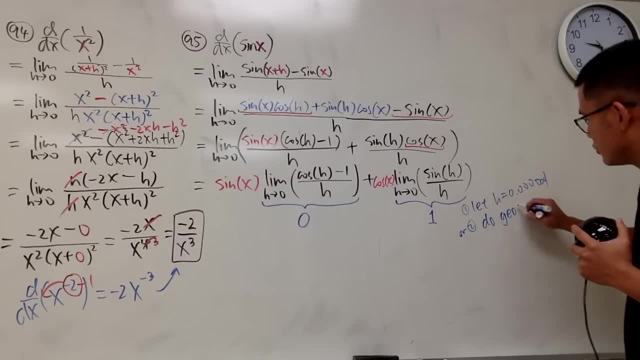 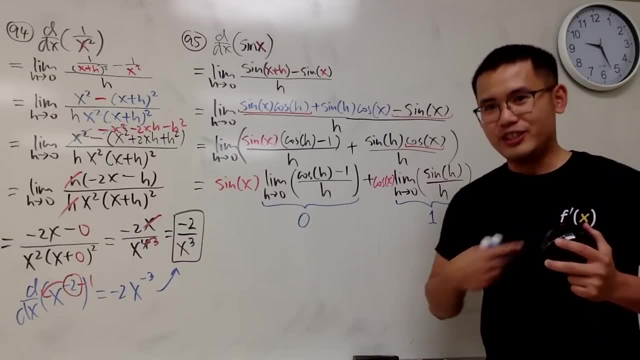 Or do some geometry, Geometry, Okay, And I do have a video on this right here And I do have. I actually have a t-shirt with the geometric picture, the picture that you need. I will have the link in the description. 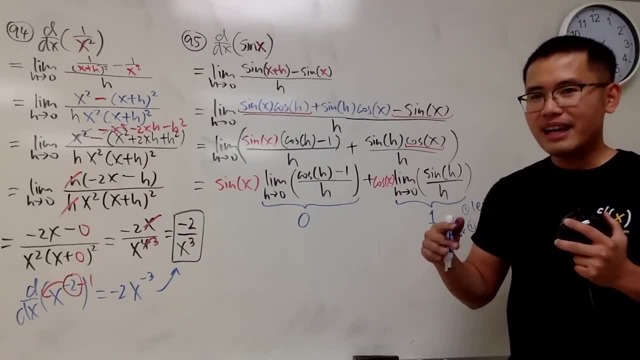 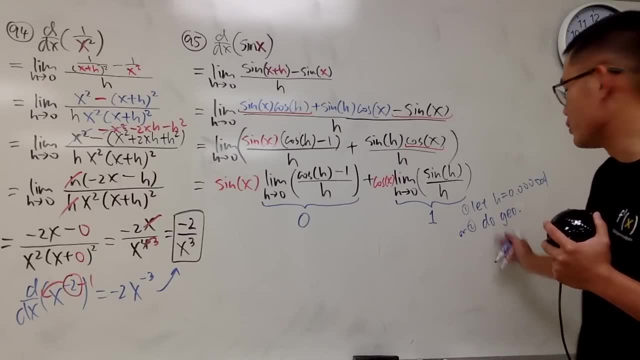 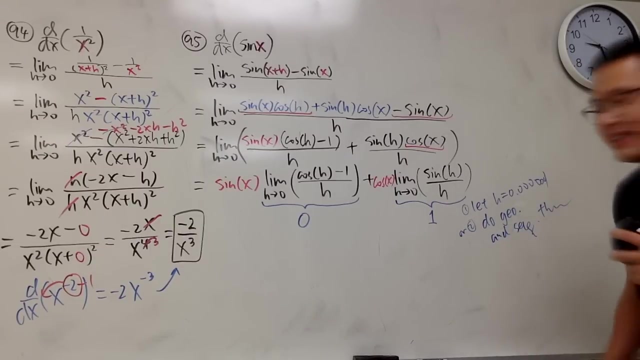 for you guys: The triangles, the sector and the connection between sine theta, theta and tangent theta, all that stuff, And squeeze theorem. Do geometry and squeeze theorem Okay. So hopefully it gets okay with this little explanation and then 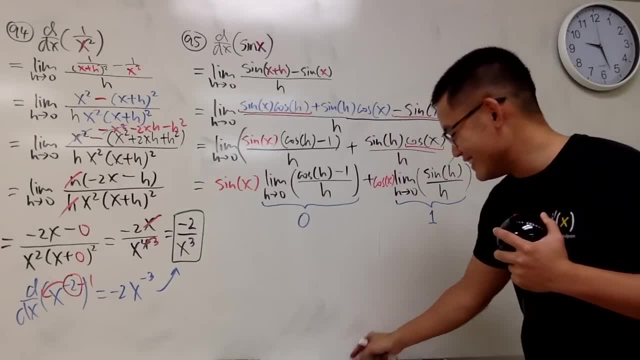 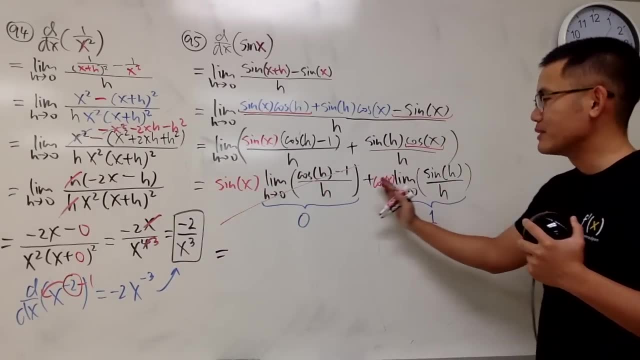 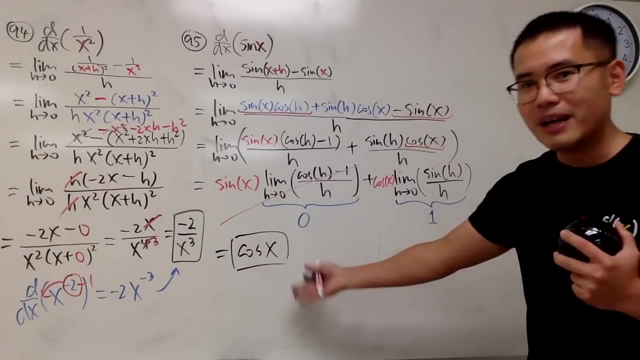 I will just continue to figure out my derivatives. Alright, Alright. Finally, you see that sine of x times 0, this is all gone. 0. 1 times cosine x. Finally, this right here is just cosine x. Ladies and gentlemen. 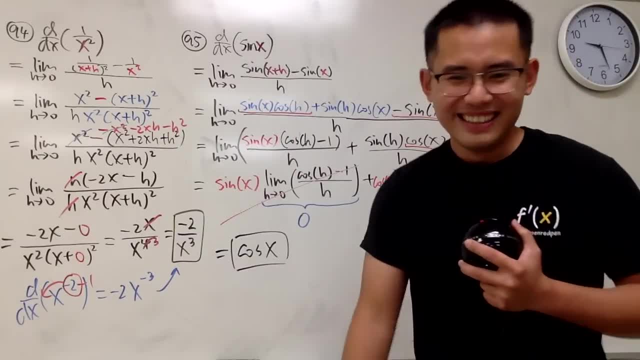 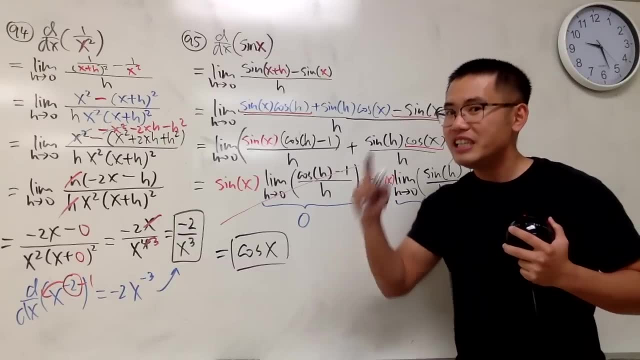 derivative of sine x is cosine x. I know, I know, I know And I. what I'm going to do next is I'll show you guys how to prove the derivative of secant x with the definition. Alright, take a look. 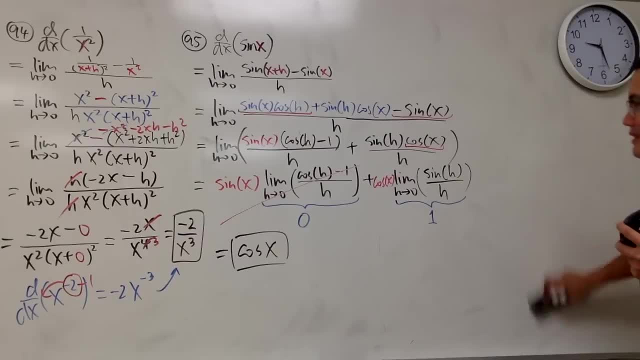 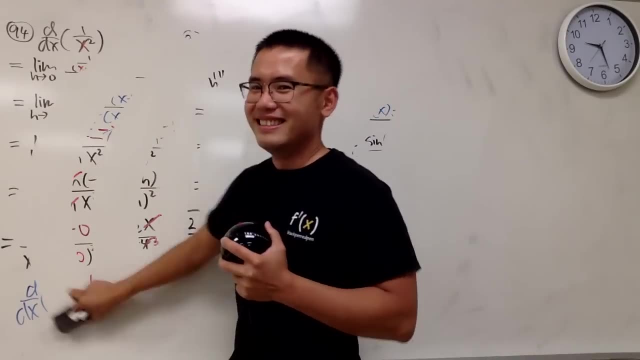 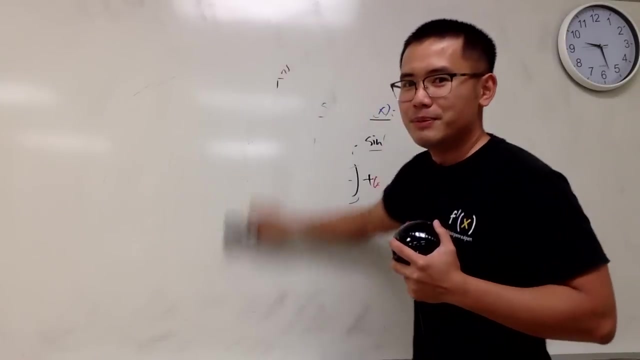 And then remember these two limits. I'm not going to give you guys too many explanations anymore, because I did that already. Alright, Man, That's the part that's like. it's hard to convince people in the- uh, it's called circular reasoning, so it's. 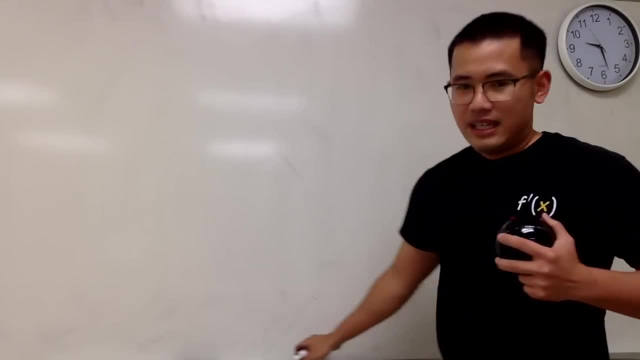 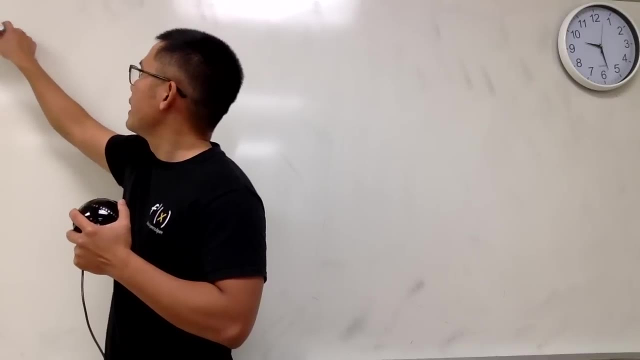 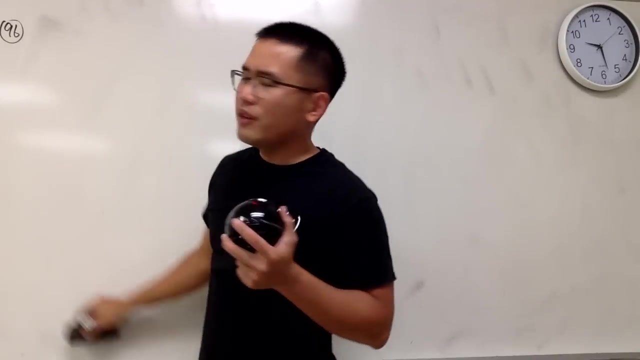 kind of weird. It's, it's, it's, yeah, Okay, Number 96, secant x- Okay, Number differentiating, Because I've been using derivative of secant x a lot. I don't know if I have. 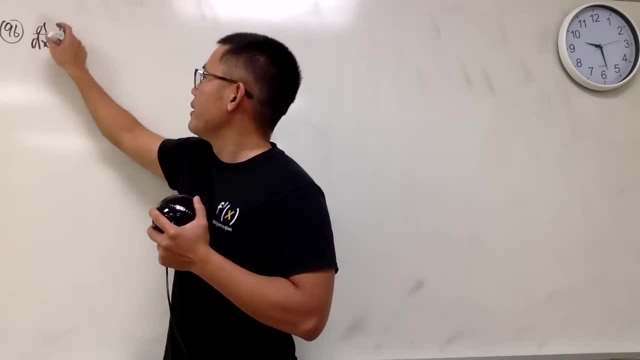 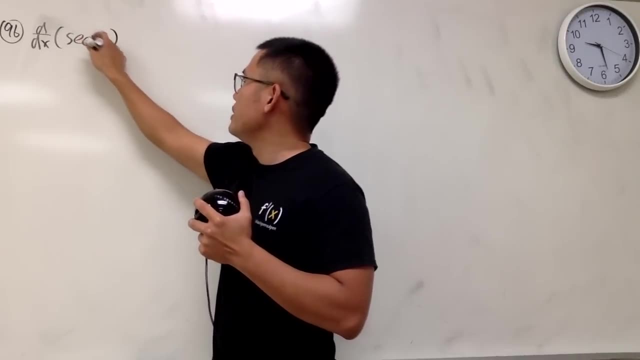 been doing it right or not. Maybe I should go back to redo the whole thing. if derivative of secant x happens to be, like I don't know, tension to the fifth power, I don't know, We'll see. Anyway, here we. 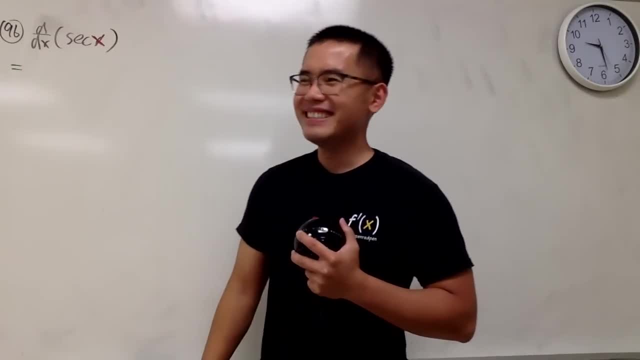 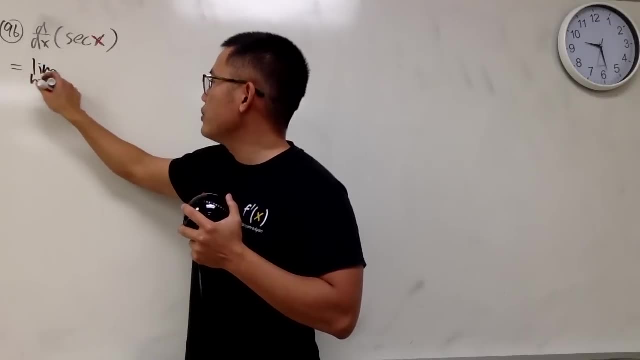 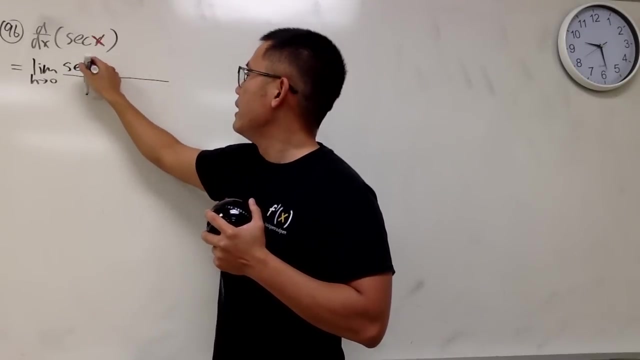 go The first. Here we go The definition of derivative. We take the limit as h approaching 0, and, as you can see, this right here is our uh input. So we have secant of x plus h and then minus secant of. 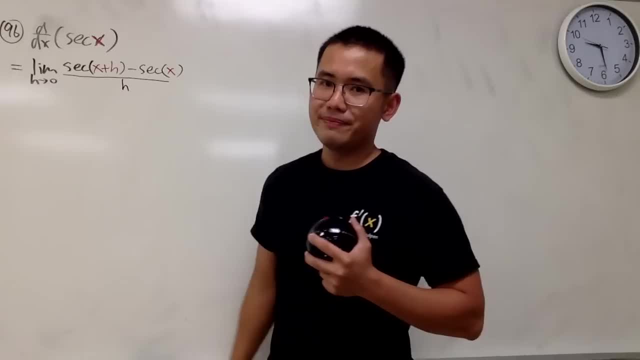 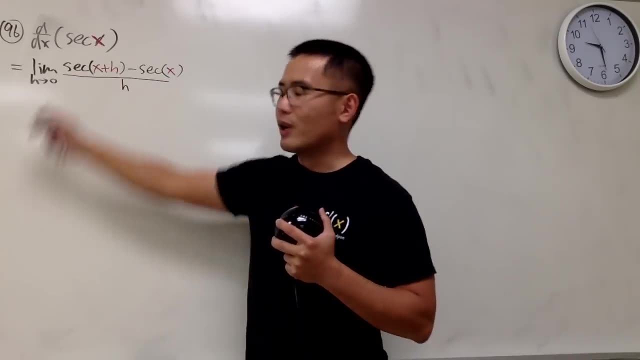 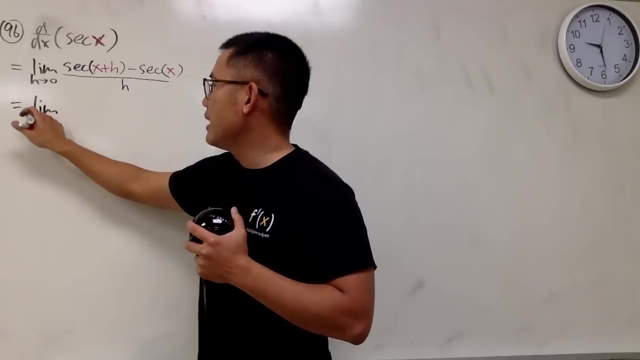 x over h, Right? Well, we don't really have a nice formula for the angle sum for secant, because we usually look at secant as 1 over cosine. so we'll do that. That's the deal. So here this is the limit as h. 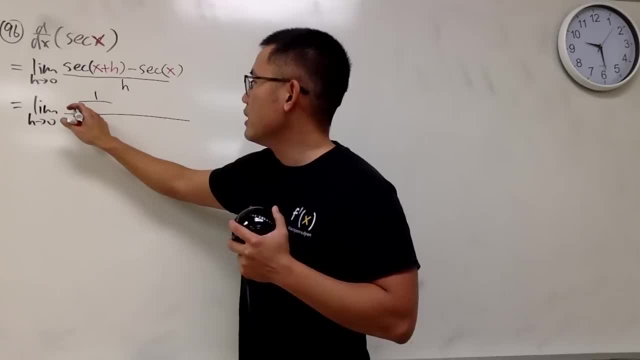 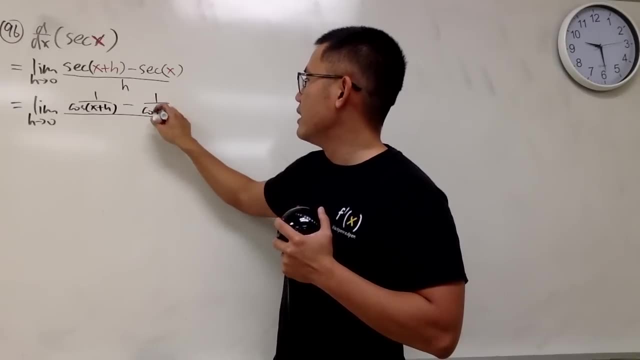 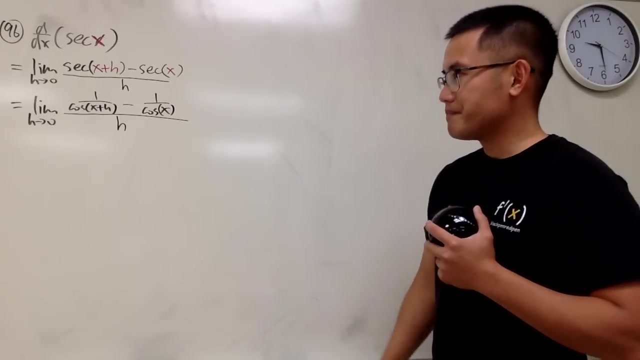 approaching 0.. This, right here, is 1 over cosine of x plus h minus. this is, of course, 1 over cosine x, And this is why I didn't do cosine, because we are seeing cosine right here as well. Now. 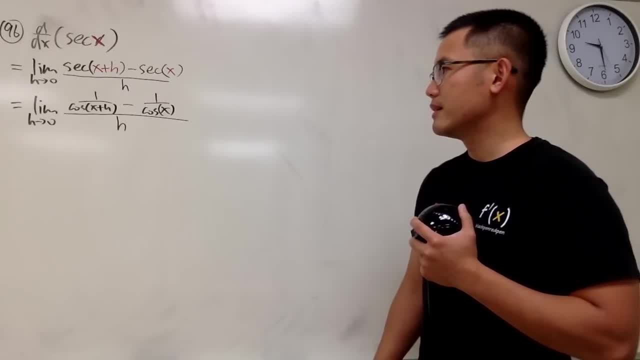 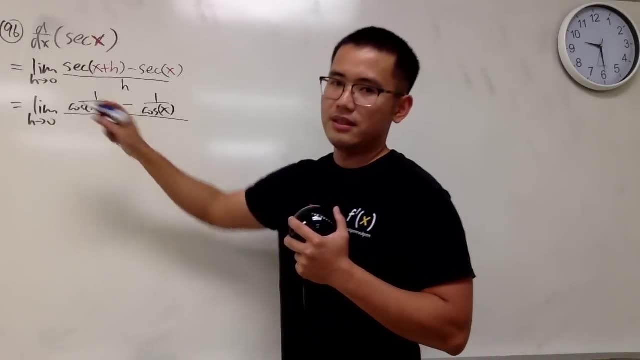 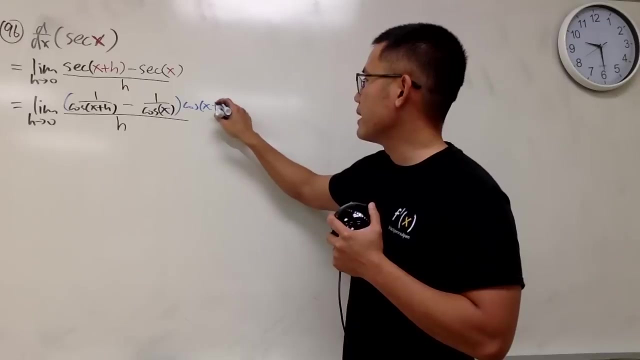 let's do the following: I'm just going to multiply the common denominator and then I'll tell you guys how to expand this in the meantime too. okay, So multiply the common denominator. So this time I will really just put this down for you. Cosine of x plus h. 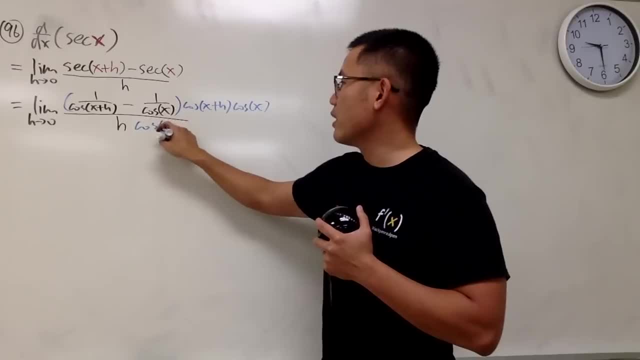 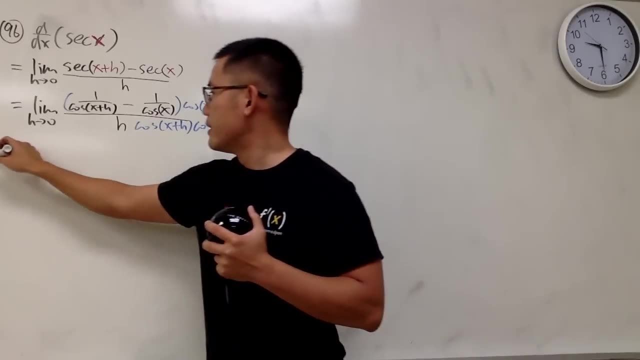 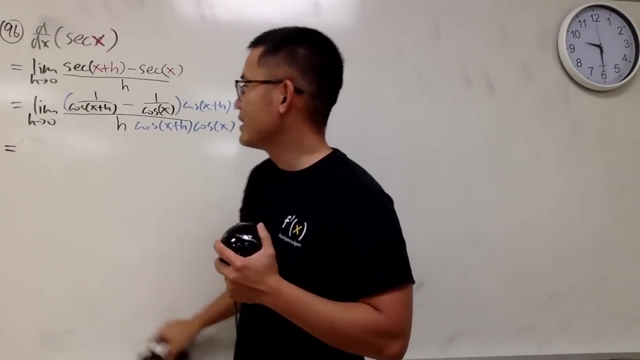 times cosine of x And here cosine of x plus h cosine of x. right Here we have the limit as h approaching 0.. Man, my limit is like getting worse. sorry, The limit as h approaching 0.. 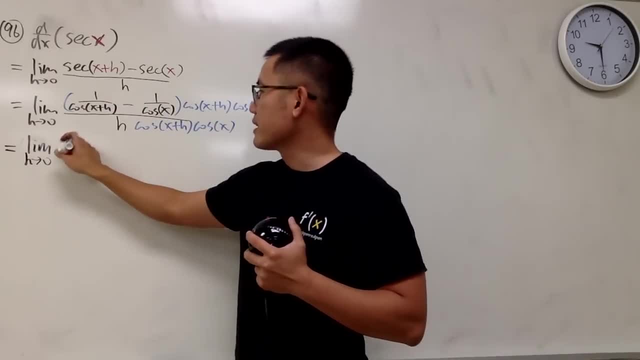 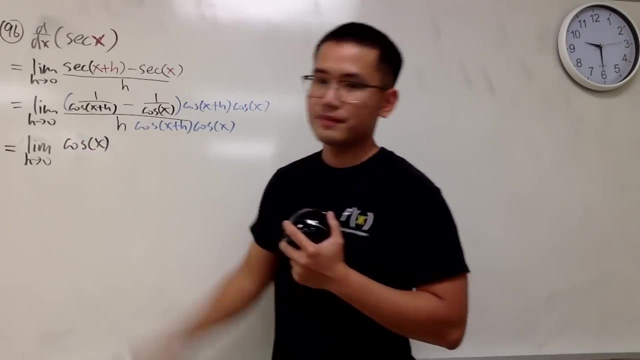 This times that of course we just have the cosine of x on the top, and that's what I told you guys earlier for the complex fractions situations. Now, when we have this times that of course the cosine of x cancel, we have. 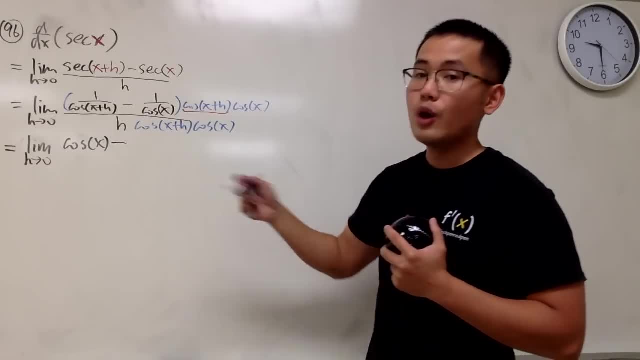 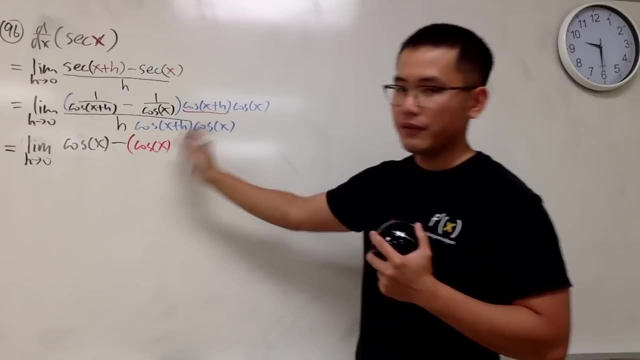 minus. and let me just tell you for this part, right here, we can expand it and the way to do it is: we get cosine of the first angle, which is cosine of x times, cosine of h, cosine of the second angle, and then 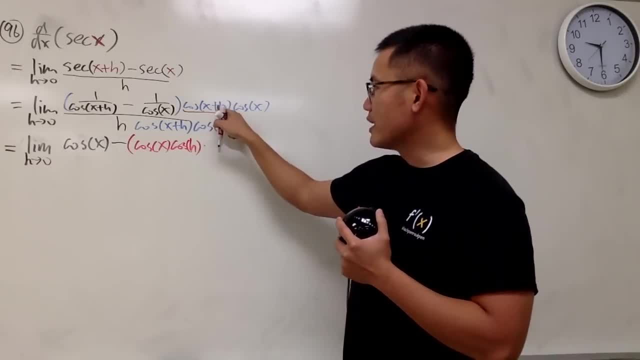 if it's a plus, it's weird, right? If this right here is plus, in fact here it's minus. You have to just remember that, Okay, Or you can see the proof for it. you will have a video for that as well. 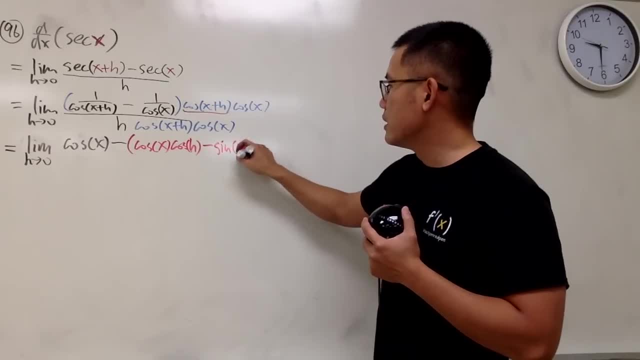 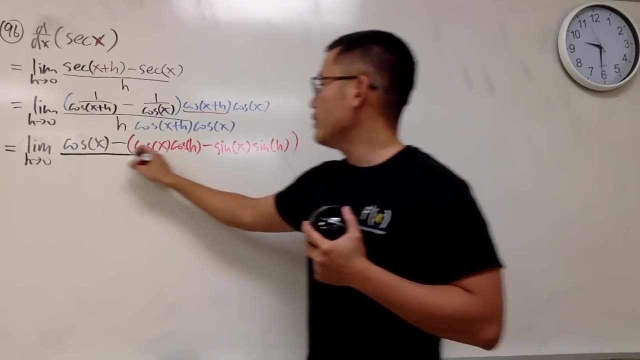 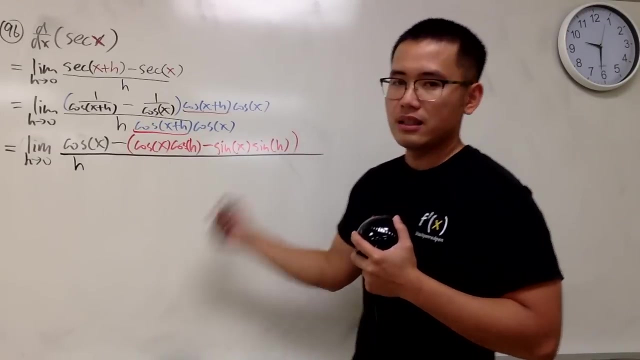 And then, secondly, you do sine of the first and the sine of the second. Yeah, so just like this. Okay, So all over. this is the h, all the way in the front, and we have this part again. so you just write it down again. 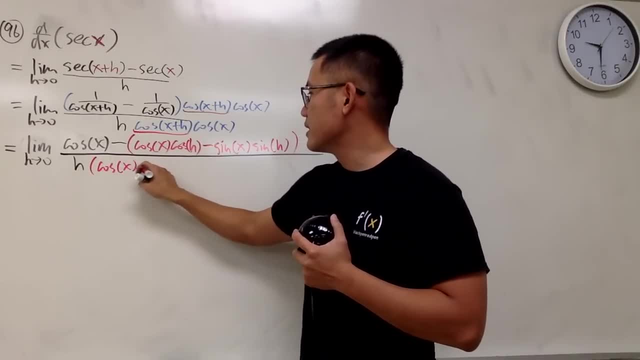 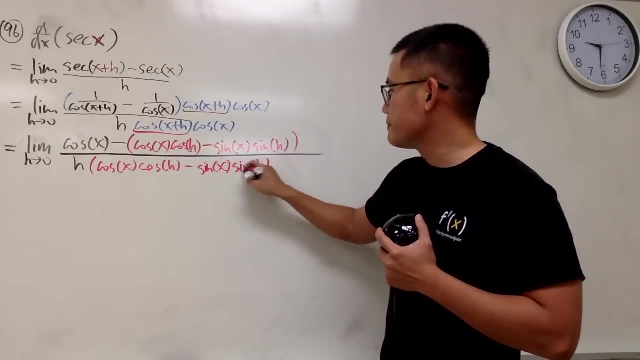 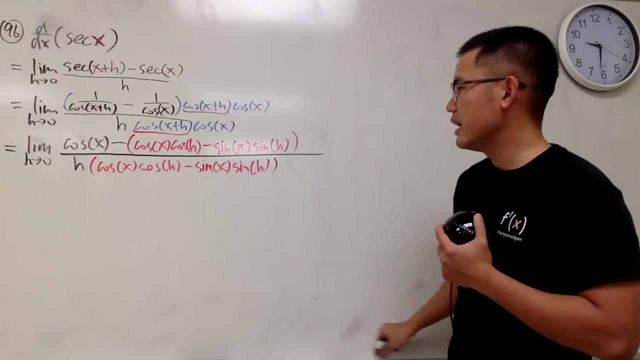 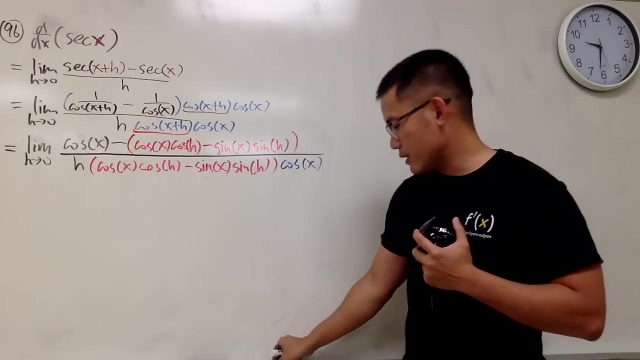 Man, it's a lot, I know Cosine x, cosine h, minus sine x, sine h. So that's that part, and then of course, we still have the cosine x right here, Right? So hopefully you guys are okay with all this. 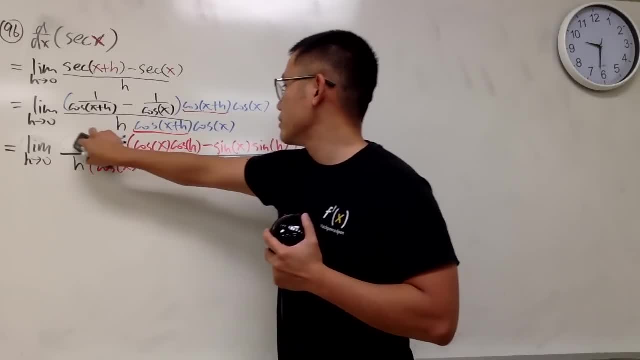 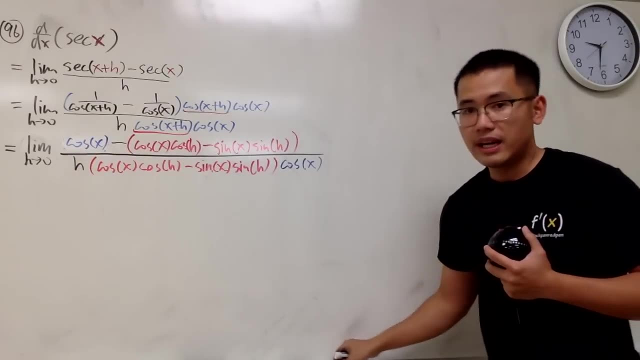 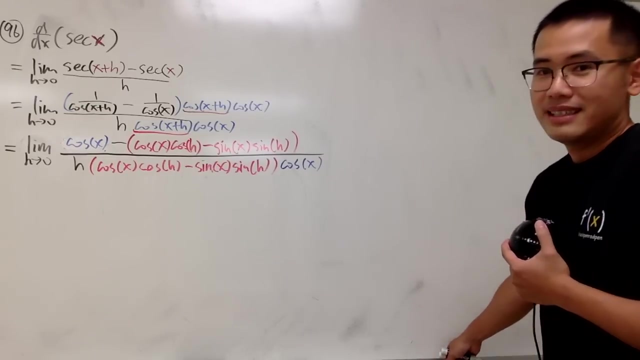 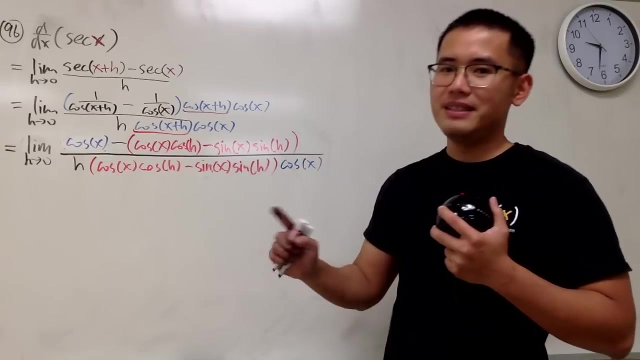 And maybe I will just might as well change the cosine x in blue. So this is just some of the prep work for that. Now we have to just kind of play around with all this. Yeah, Here is the deal We are gonna split. 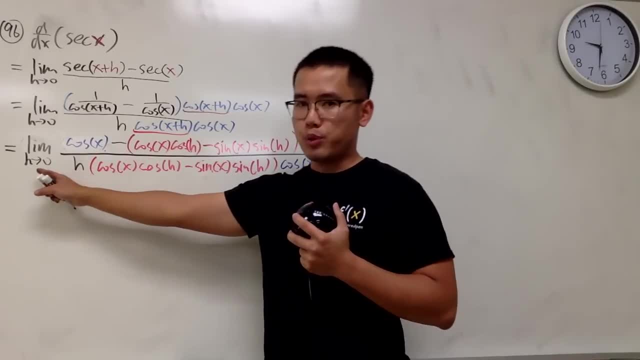 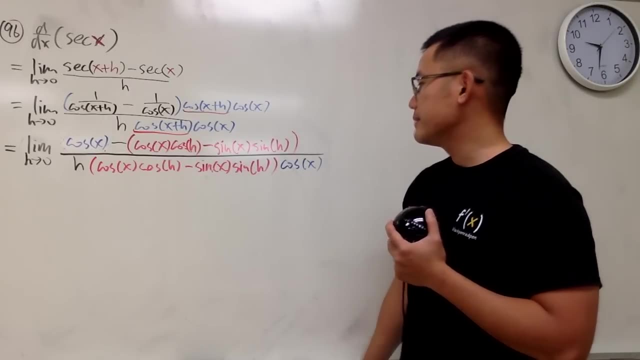 things up right And you see, when h is approaching 0, in fact, you still end up with 0 over 0 situation. if you're just plugging 0 into all the h And again, just to hold you earlier, we can take out the parts. 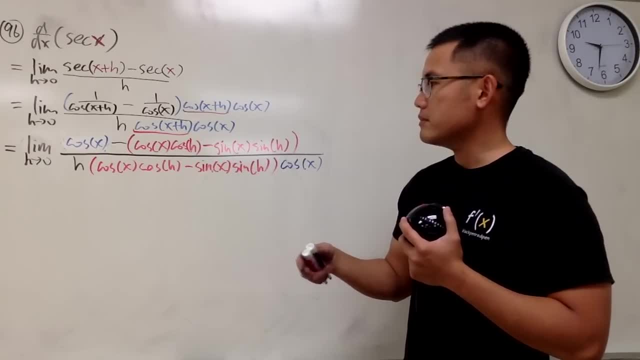 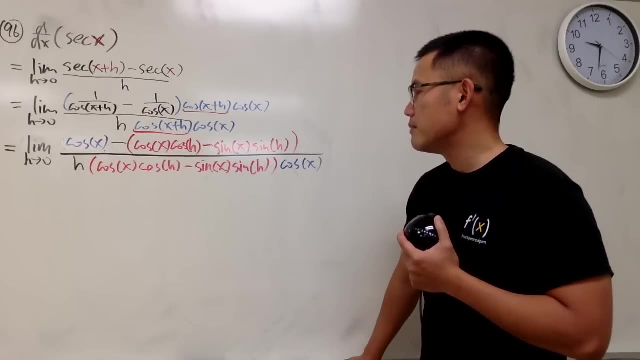 that has nothing to do with the. what's that? the x with the h? you know all that stuff, okay. So How should I split this in a nicer way? Let's see. 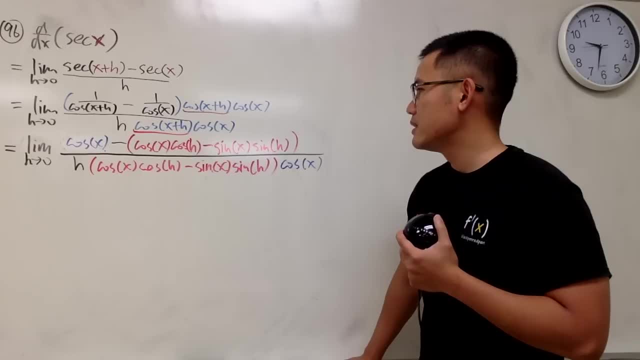 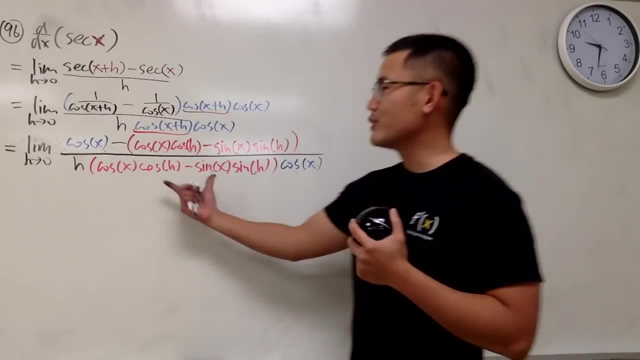 Okay, Man, as I told you, this is just a lot to write, So unfortunately, this has to stay inside of the limit. so it's that, but this can go out. But here is how I will split this, okay. 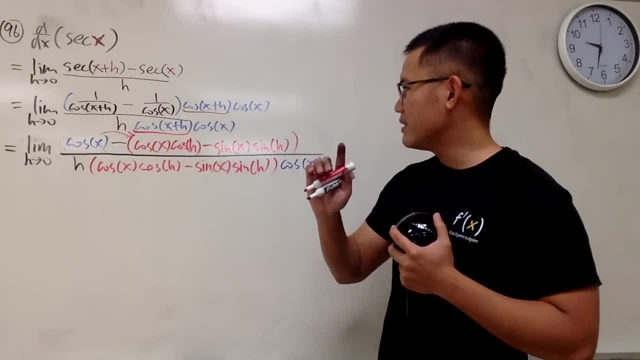 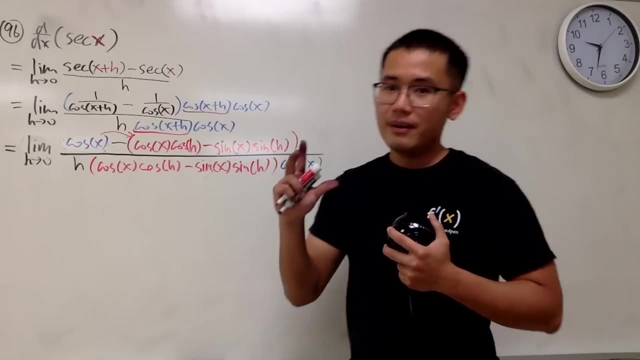 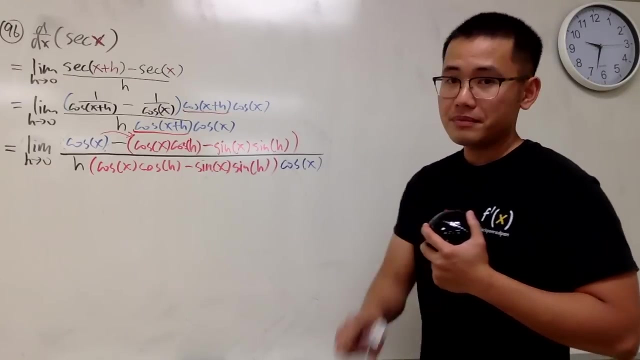 So multiply this in and, uh, check this out, I have the cos x, cos x, so we can factor that out and then we can pair things up. The hard part is to pair things up the right way, Um. 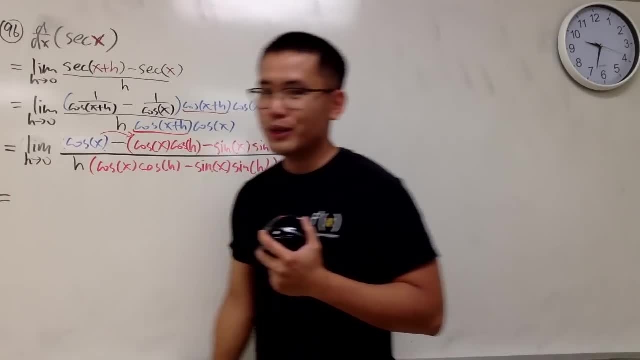 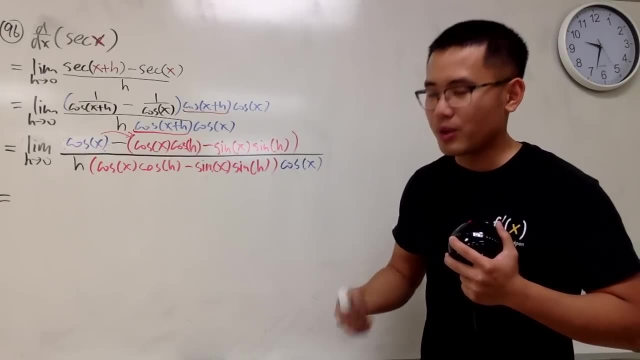 Okay, This is like the limit law to the finest: The limit of the product, the finite amount of product. it's the finite amount of product of the limit. So here's the deal. I'm not going to touch the h. 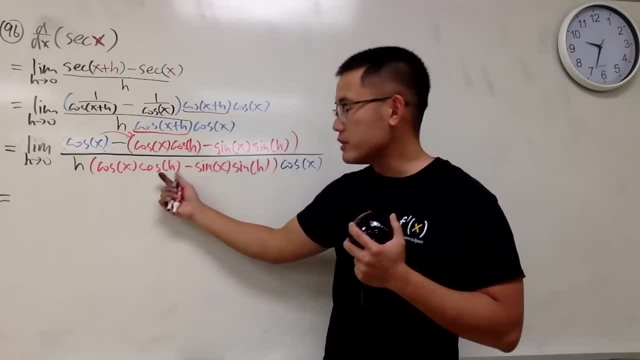 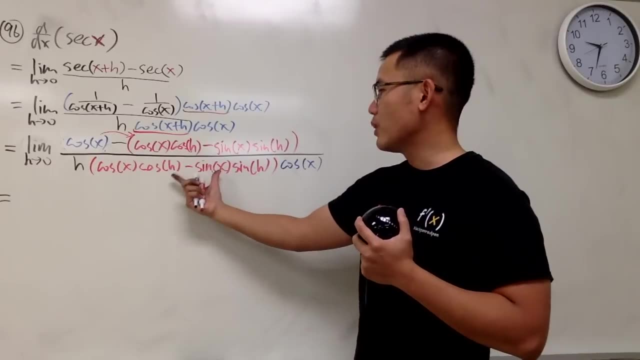 I'm going to split this. In fact, if we have h equal to 0, approaching 0,, right here, this is just cos x. Likewise, this is just going to be 0, so this is good. So this is one part that I can do. 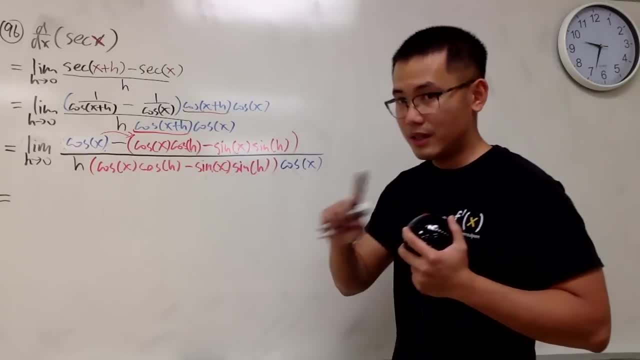 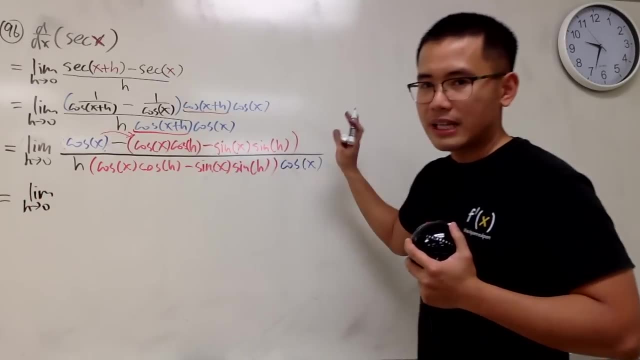 So I would like to just take the limit of this part. I will show you As h approaching 0, and let me just forget about the top for now, okay, and also the h. Just don't do that for now. So 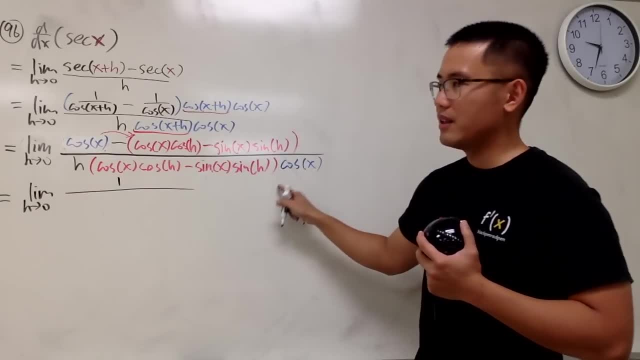 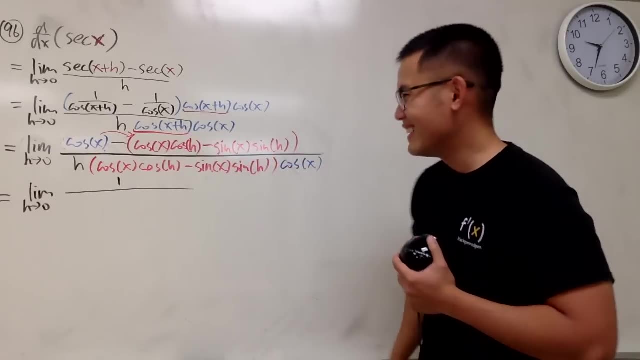 I would like to look at this one over. this whole thing here, This whole thing here, Man, perhaps I should have just written it like that: huh, Ah, man, let's see if I should do that. I should totally do that, Man, I should. 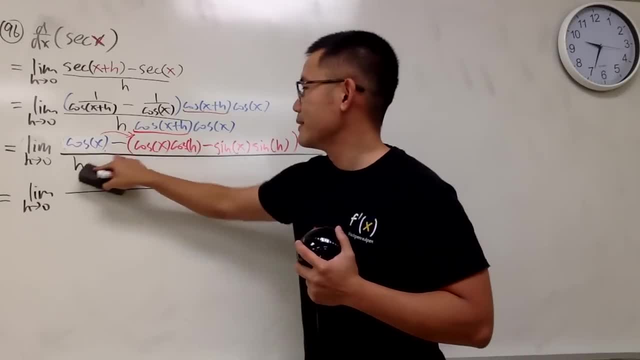 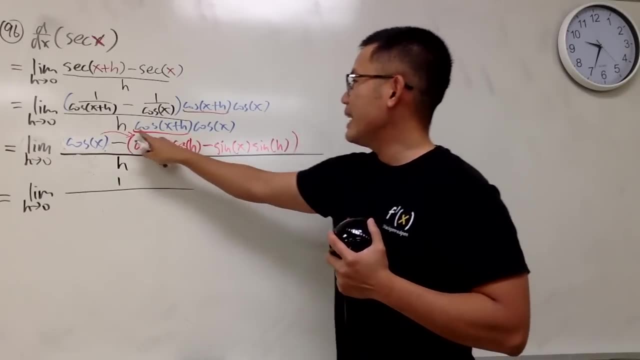 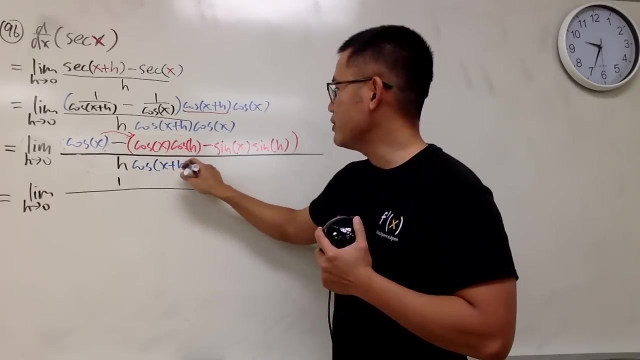 totally do that. Ah. So, man, I'm mad at myself. h. I am going to just keep this right here. You'll see why. So h cos and this is cos. So what I will do is I'm just going to put down this right here first. 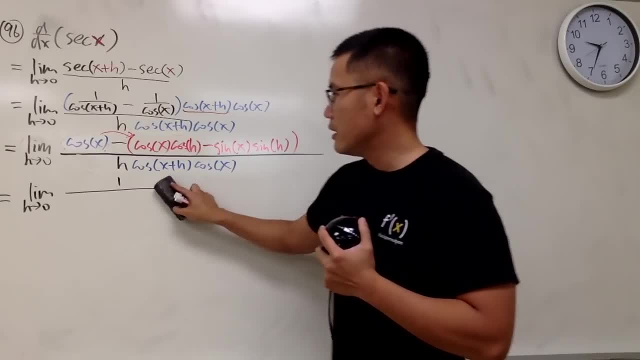 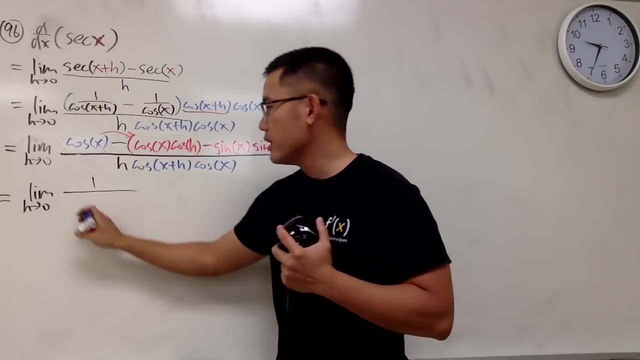 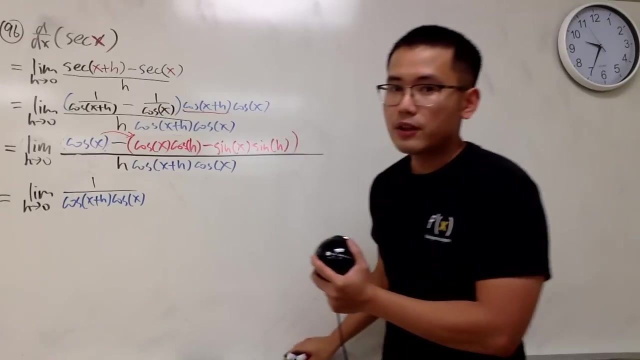 Okay, So we have 1.. We have 1 over. I just want to put this down right here. okay, So this is cos, cos. So that's the first part. I want to just keep it as how it is And I will have to. 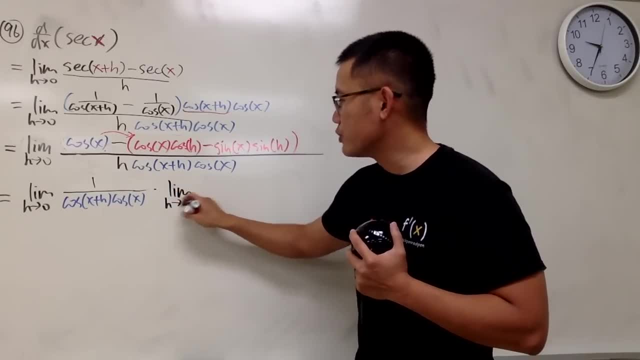 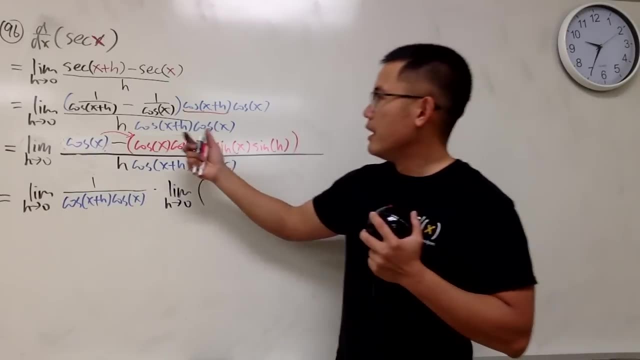 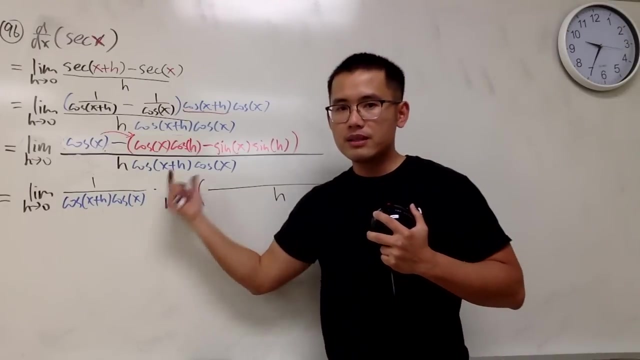 multiply by the following The limit as h approaching 0 and we will see the rest. So you see, I am putting down this part right here. So this right here is just the one that was h in the denominator. I put down these two. 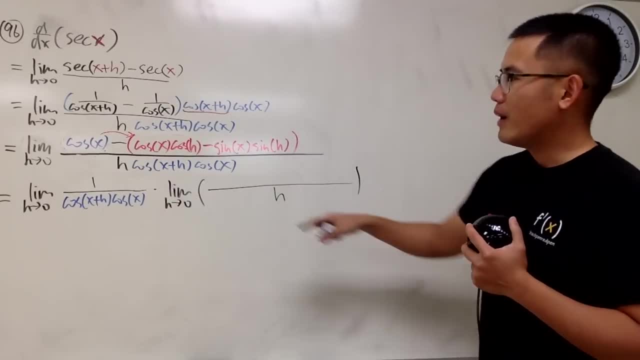 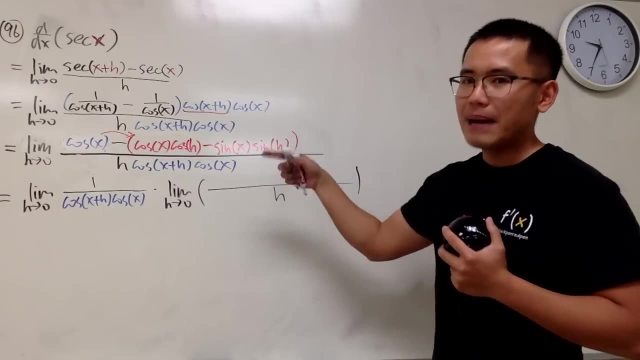 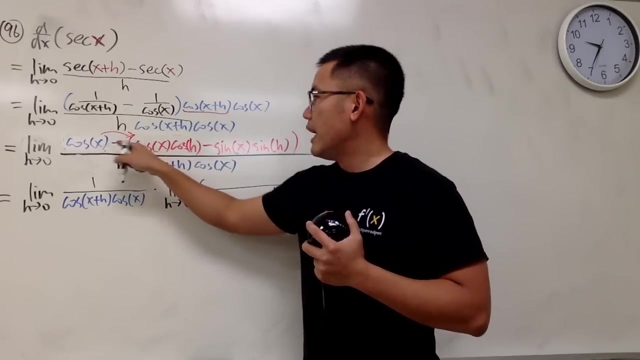 in the front already, And that's going to be nice. Now I will have to just pair the the top on the top. I just have to pair the top nicely on the top Here. cos minus, cos, cos right. I will just factor the cos right here. 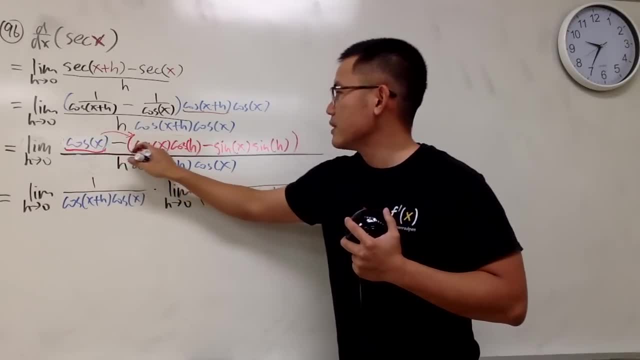 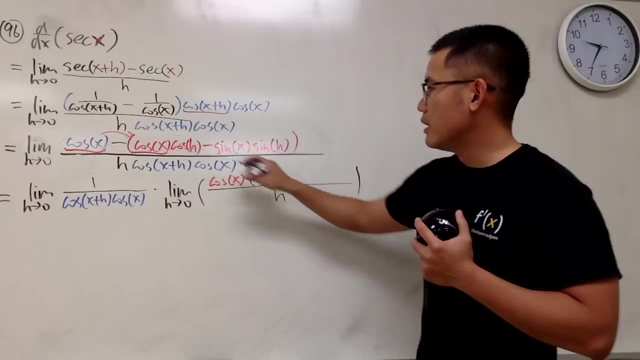 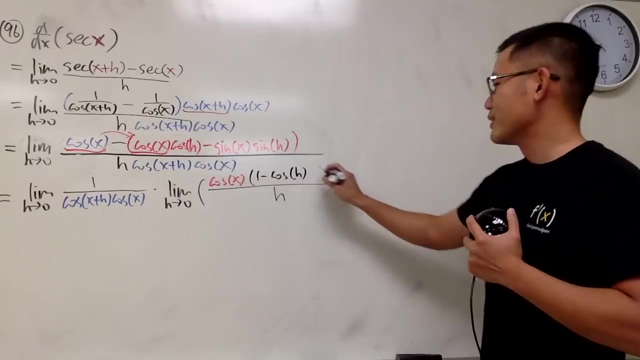 So I will put down cos and this is the cos, cos and then parentheses. this will be a 1 minus cos. Good, huh, Yeah, of course it is Good. Then this is negative and this is negative. so I should have. 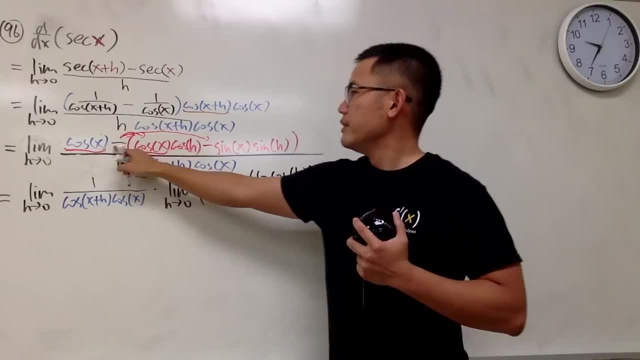 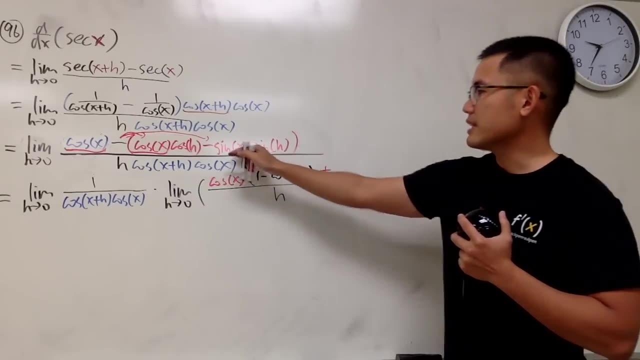 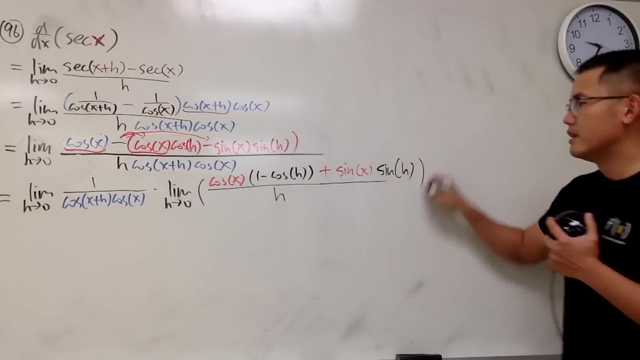 done this like this: Negative times negative becomes plus. So we have- let me just write it down again- Plus and you have the sin right here. times sin, and I think you guys know where I am going. Yeah, that's pretty much the idea, right? 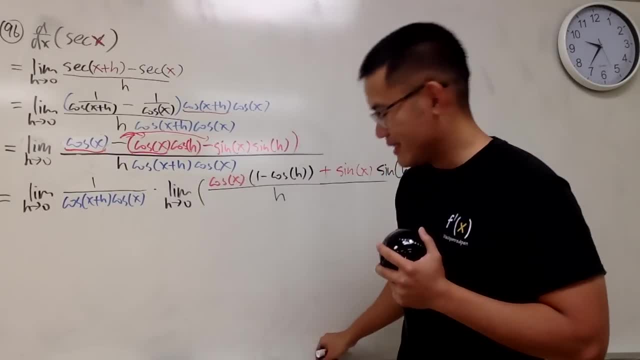 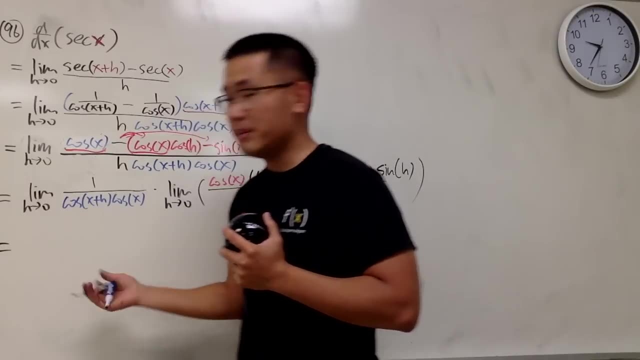 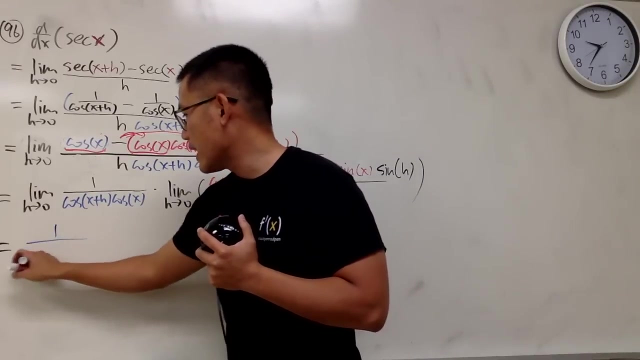 So for this part, in fact, as I said, if you can figure out the limit, go ahead and do it, and that's pretty much the limit law. Putting 0 into the h, we will end up 1 over cos x plus. 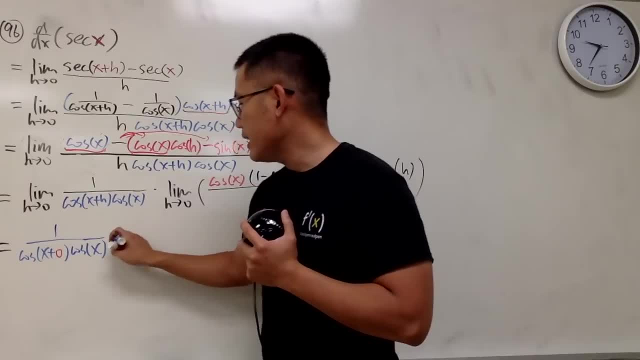 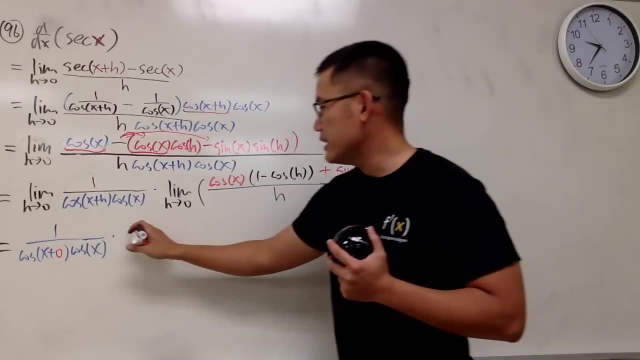 0 cos and that's it. This is the first part of the limit. Let's just ignore that for now And now, if you look at this part, of course, let's just do it like this: okay, Save some space, save some time. 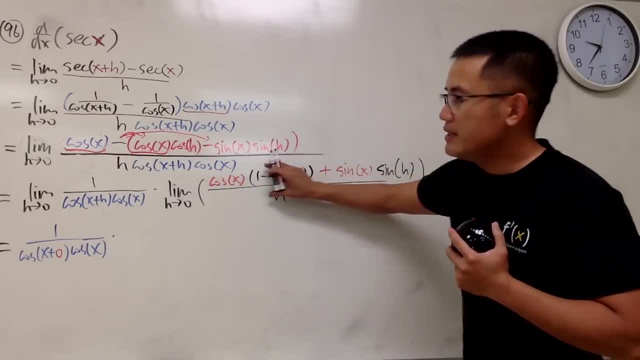 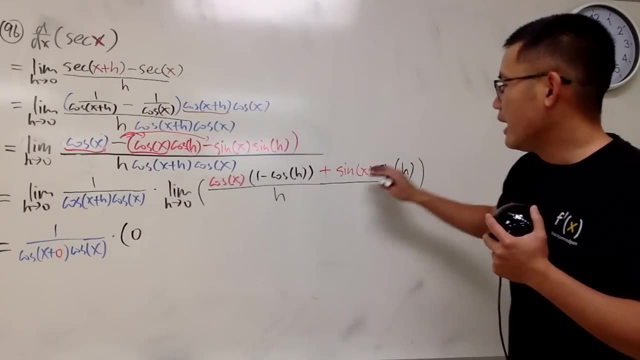 Just like what we did earlier. The limit as h approaching 0, this is going to give you 0. So this is nothing here. So multiply by 0. And this is going to give you 1.. So we end up with just sin x. 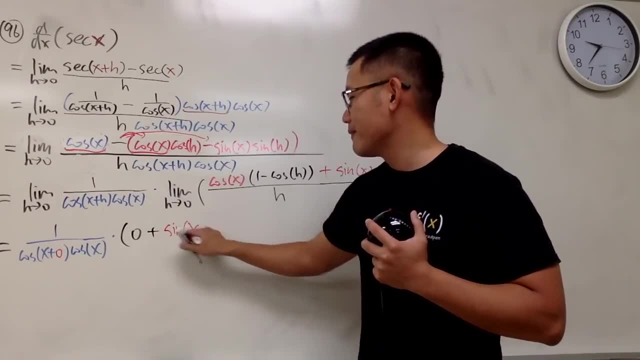 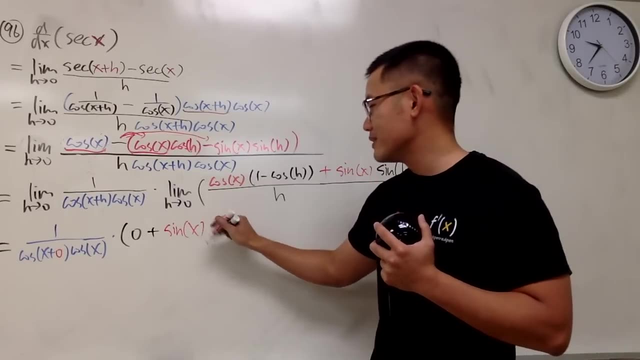 right here. So it's plus sin x. Okay, Sin h over h. the limit of that will be 1.. So it's just sin x remaining. So it's like this. Now we see that all in all, we just have sin x. 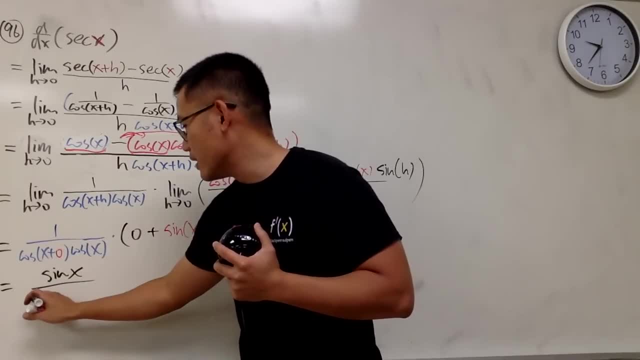 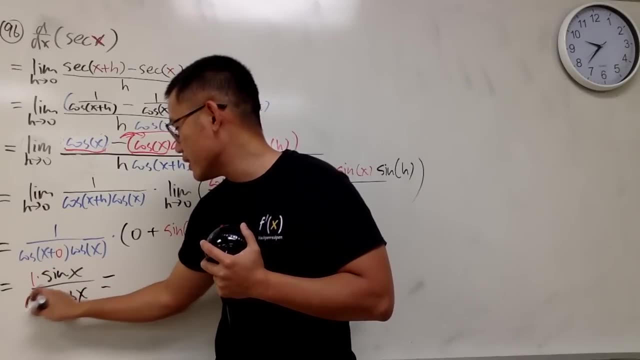 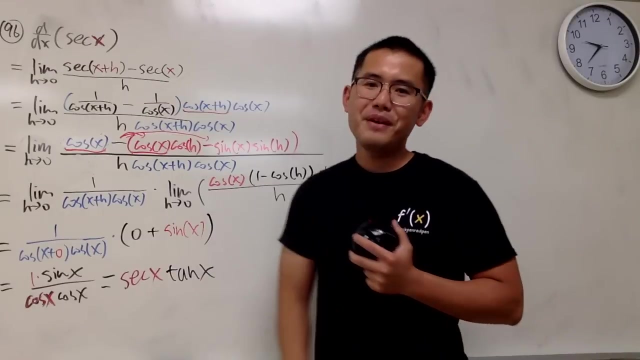 on the top over. this is, of course, cos x, and this is another cos x, and this is 1 times that, which is, we can pair this up as sec x. Pair them up, we get tan x. Very nice, Right, Very nice. 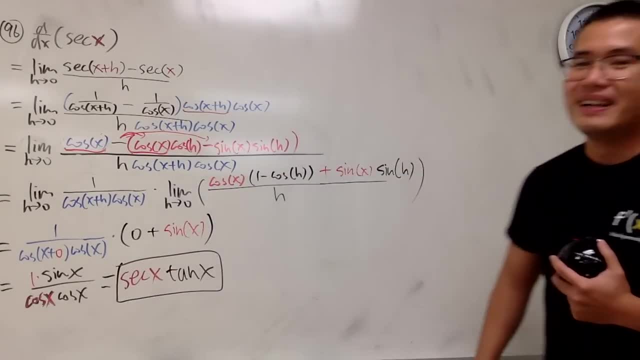 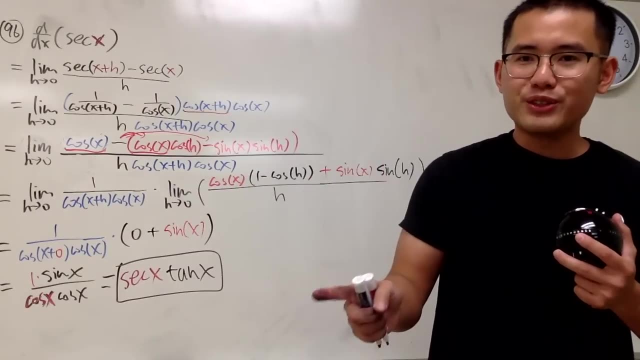 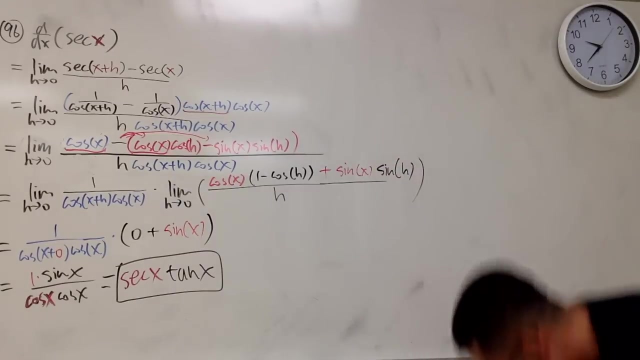 Very nice. So that's it, The derivative of sec x by the definition. I'm not going to do the derivative tangent by definition, because I'll give you guys something better. Anyway, number 97.. I will have to erase all this. 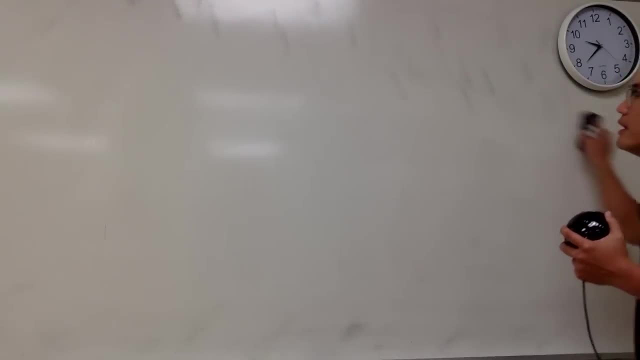 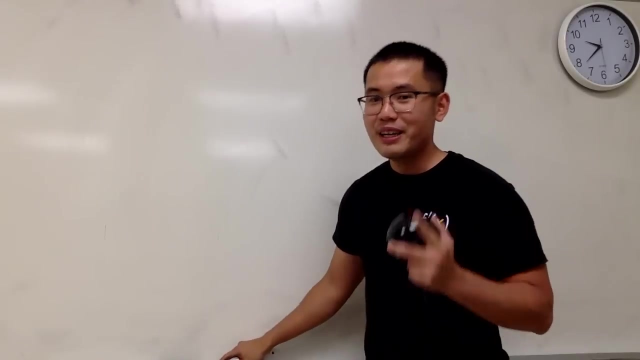 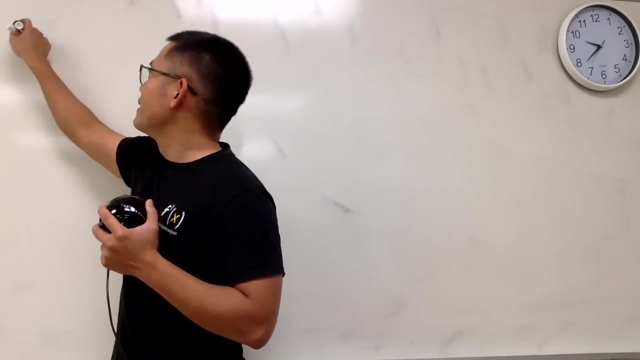 How are you guys doing? Are you guys still watching? Are you guys still doing? good, Let me know. Alright, Now number 97, right here, No kidding, I will show you guys for the first time on my channel how to. 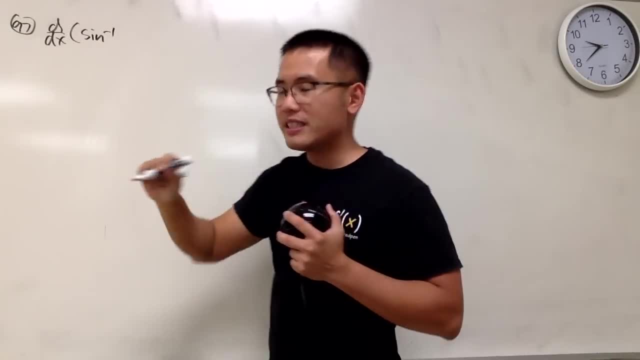 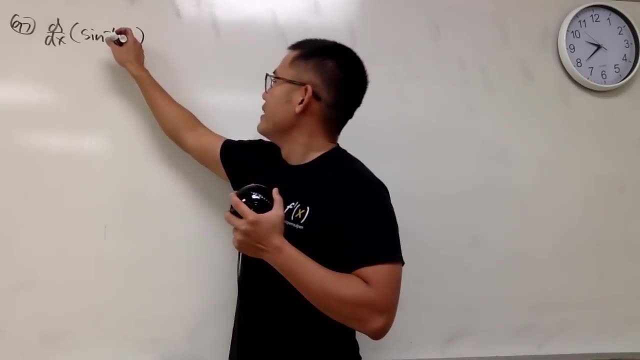 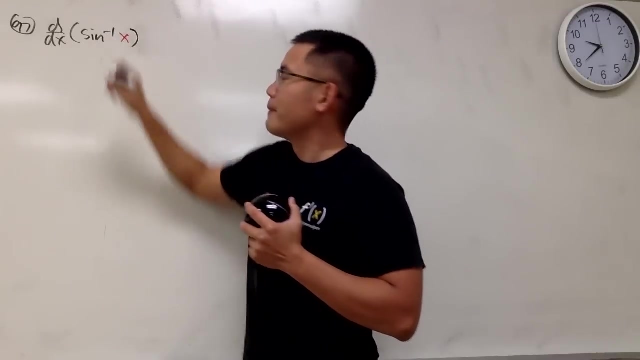 differentiate how to find the derivative of the inverse sine of x. with the definition of the derivative, Here we go. This right here is x. Sorry, that's a bad one. Here we go. By definition, we take the limit as h approaching 0, and now? 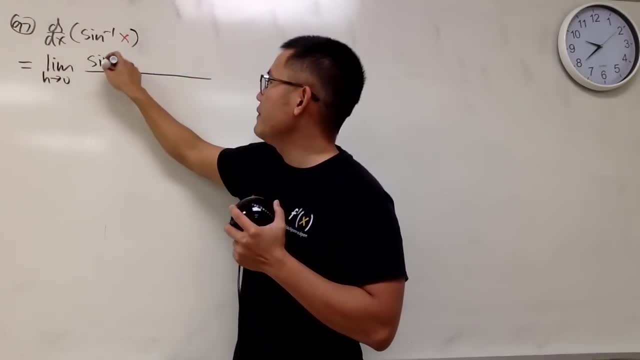 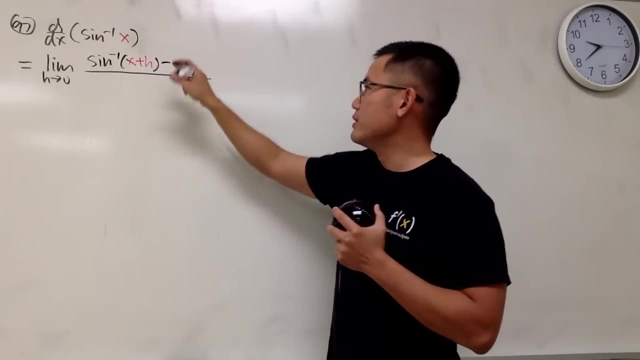 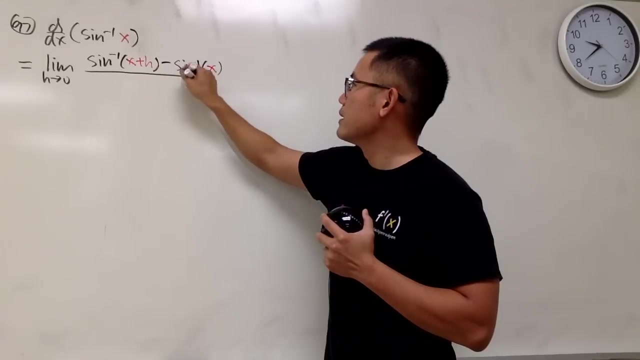 this right here is the inverse sine. so we have the inverse and this inside is x plus h and then we minus, of course, the original function, which is the inverse sine of x. Like that You don't put a plus h And then all over h. 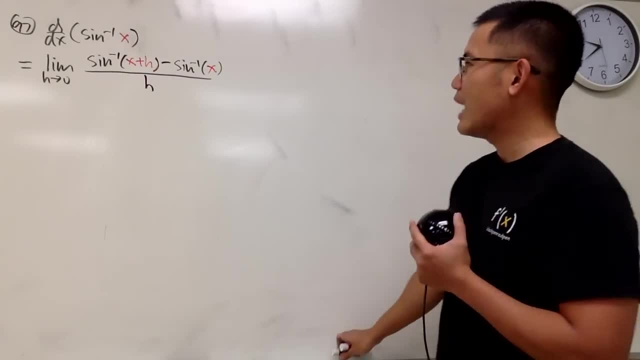 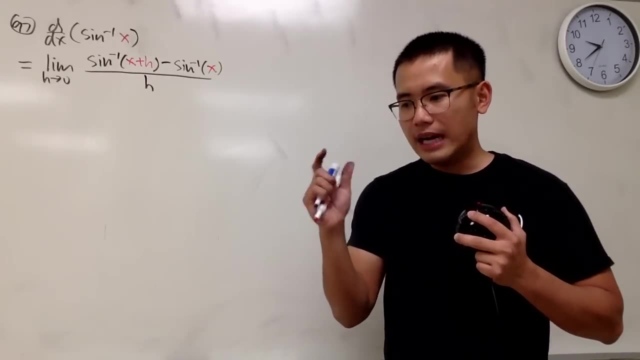 Alright, Here is the hardest part. It's like how in the world can we simplify the top? Well, we just have to do the angle addition identity kind of like backwards. I will show you what I mean by that. So let me just make a. 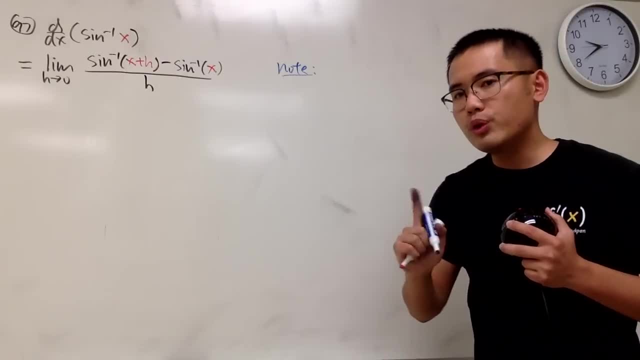 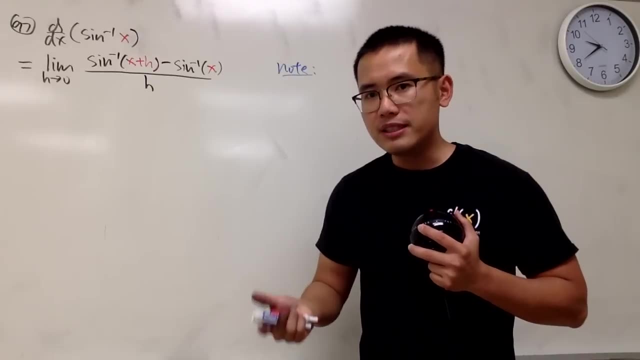 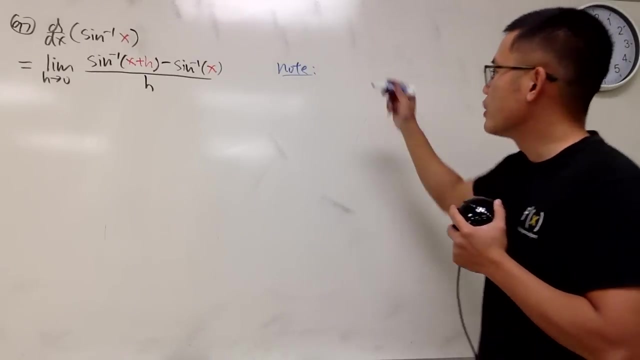 note right here. This time, though, we want to look at the angle difference formula, because whenever we are taking the inverse trig function, it represents an angle, right? So you see, we have the first angle minus the second angle. That's what we have to look at. So, in fact, 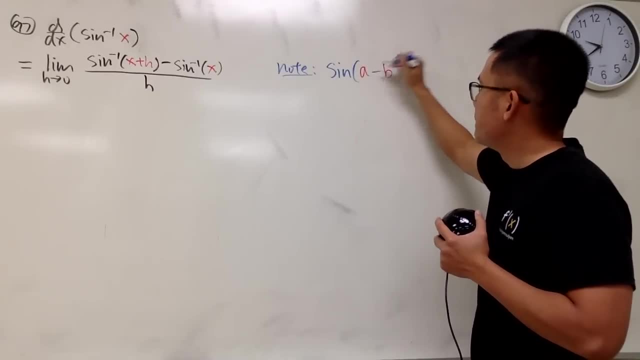 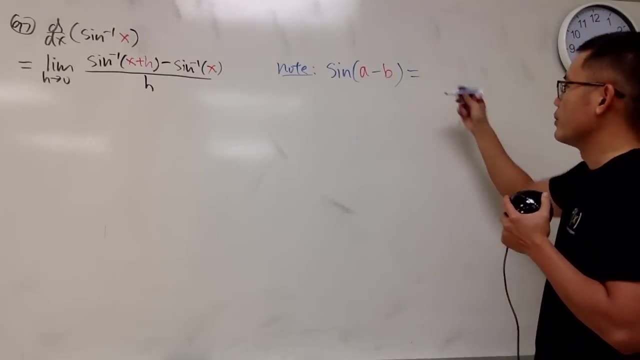 I will have to look at sine of a minus b. These two angles are being subtracted. Okay, So that's the key. Well, if you look at this one right here, let me tell you: the identity right here is sine a. 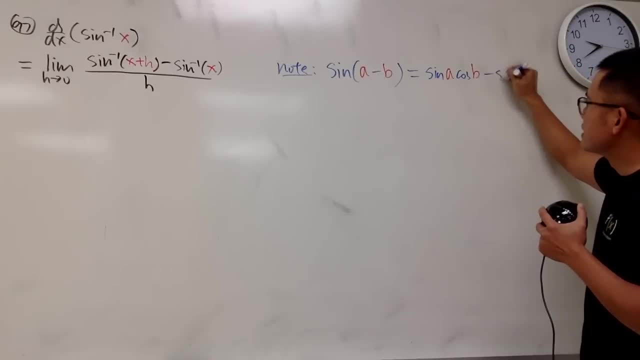 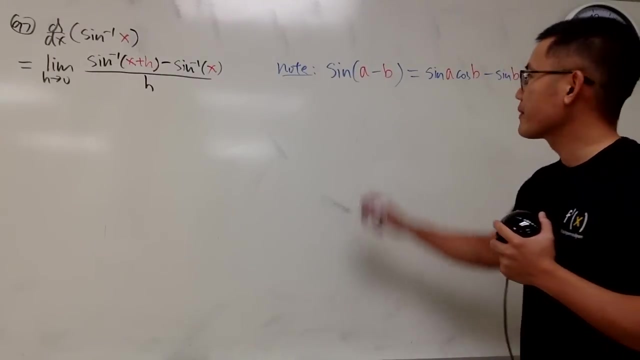 cosine b and you minus sine b, cosine sine a, And usually I use the alpha-beta, but you know why so serious about like this. right here It's 97 already. Okay, Here is the DO This. right here it's the angle I will put. 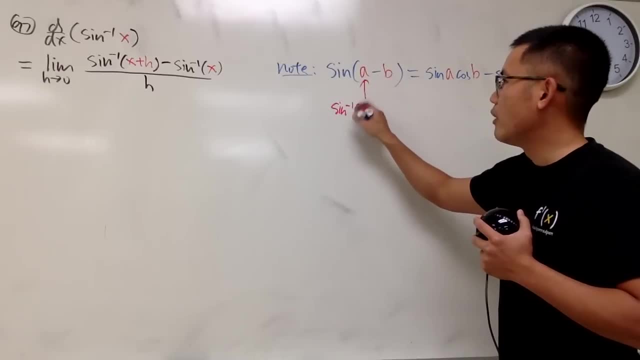 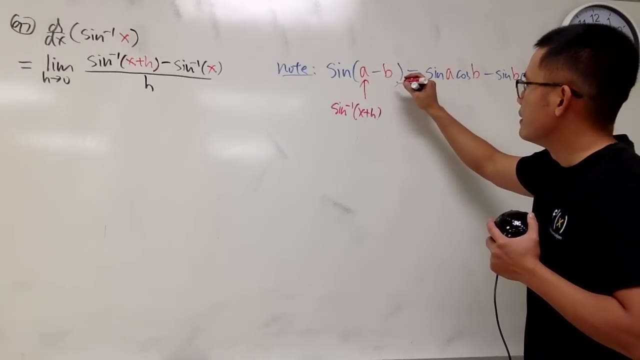 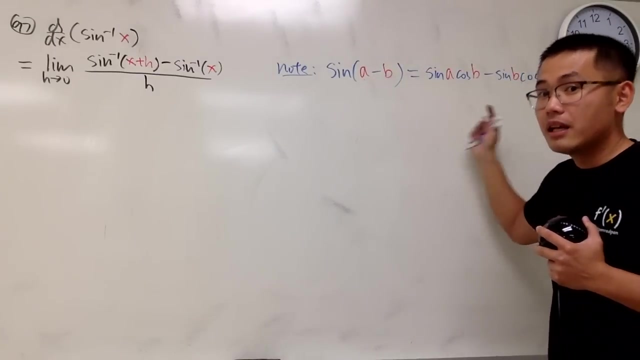 it to be the inverse sine of x plus h. Hold on, Let's do this right here, Let's do this right here. So we're good with this identity, right? And now you see, this right here is sine of a minus b. 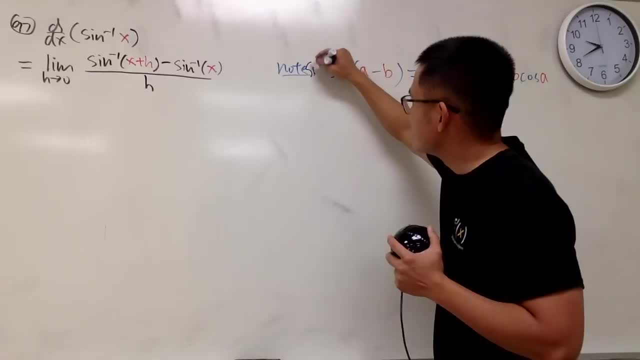 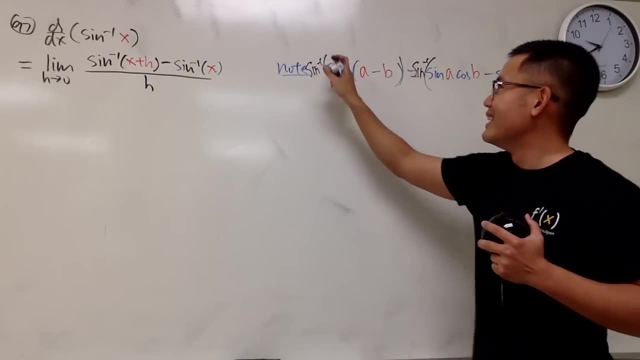 So we are just going to take the inverse sine on both sides, Take the inverse sine here and take the inverse sine right here, So that this and that will cancel out And don't worry about the domain, because right here everything is small. right here, right. 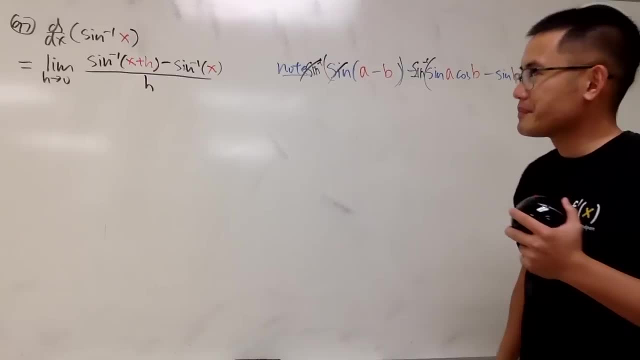 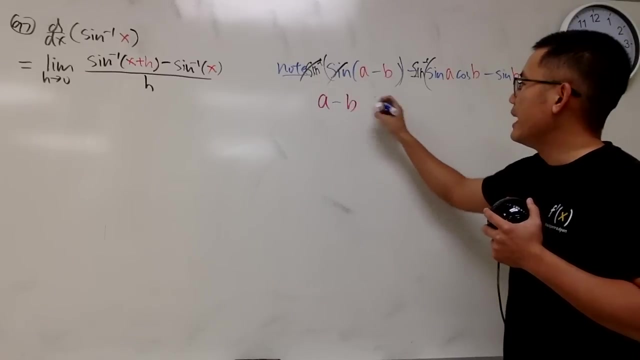 You see x plus h And we can, yeah, just negative pi over 2 to pi. That's good Anyway. so this is good And you will see that right here we can come up with a minus b And this right. 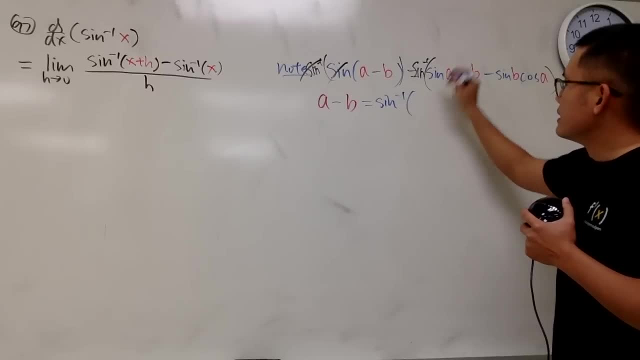 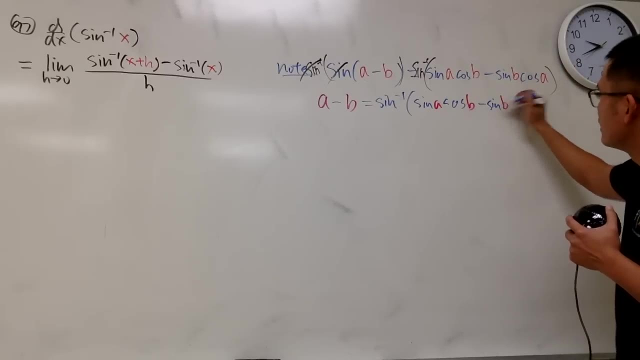 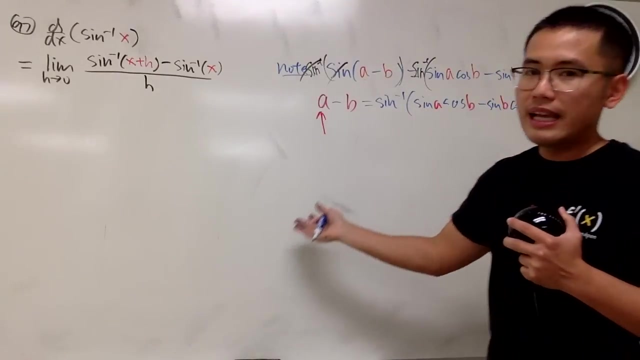 here. it's going to give us inverse sine of sine a cosine b, okay, And then minus sine b cosine a. So I think this is believable. Now what I'm going to do is I'm going to let a equal to inverse sine. 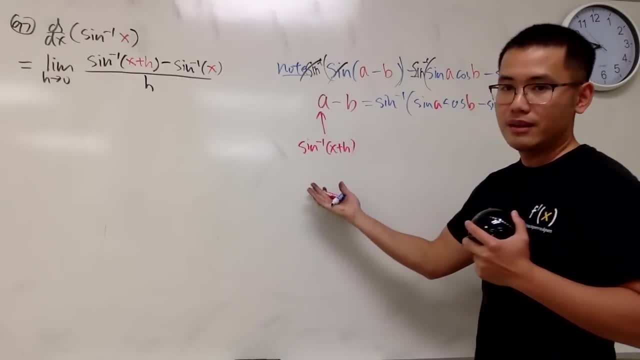 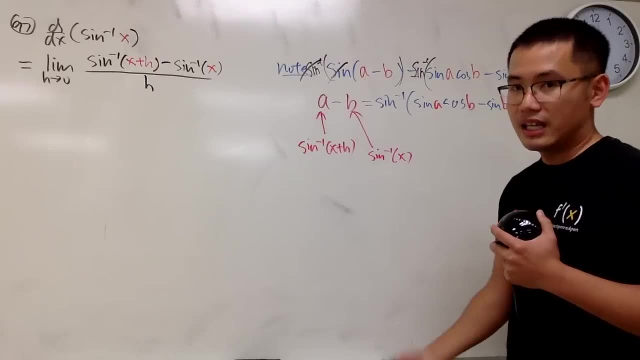 again, this is meant to be an angle Right here, Inverse sine of x plus h And of course b will just be inverse sine of x. And guess what I'm going to do? Of course, I will just put all the a's right here. 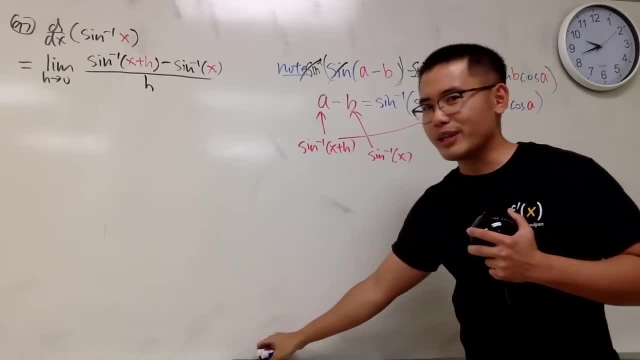 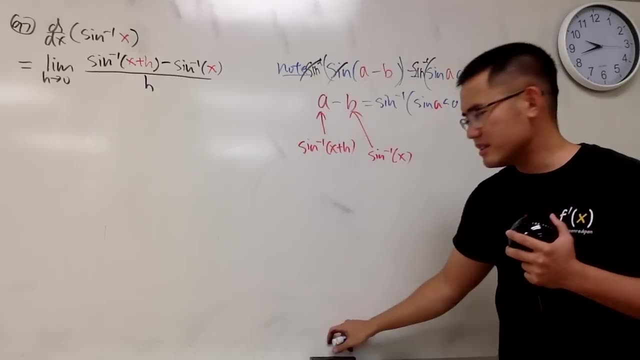 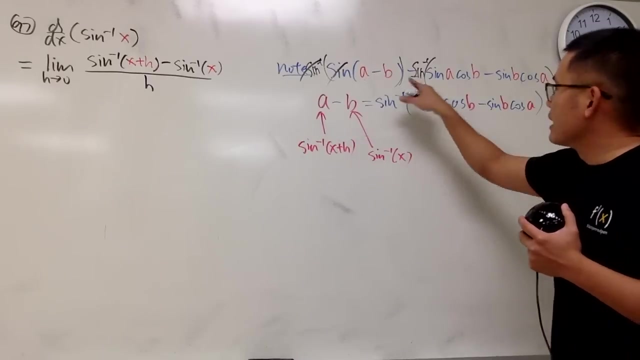 Yeah, it's too many arrows, though. I think I'm not going to draw the arrows, otherwise it's too confusing, Right? But here is the trouble, If I put inverse sine of this in here. yes, it's easy. they can just cancel out like this. 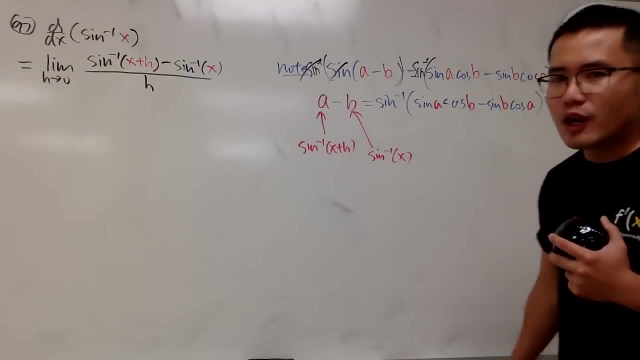 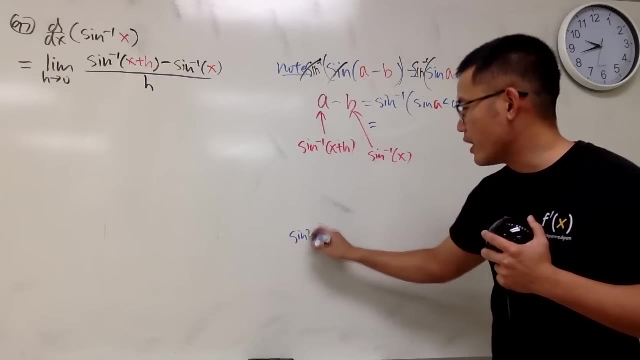 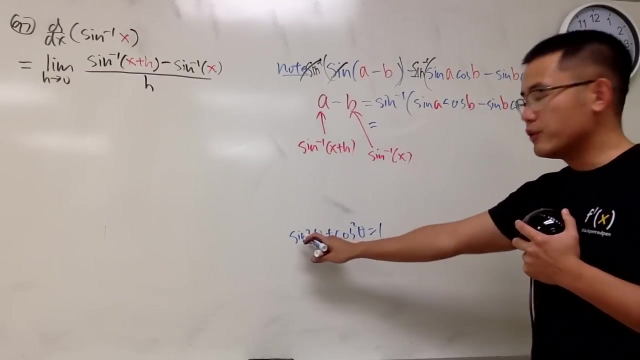 But for the cosine it does not cancel out nicely. It's okay, though. this is what we can do. Of course, we all know sine square of theta plus cosine square theta is equal to one. Well, we can move this to the other side, And 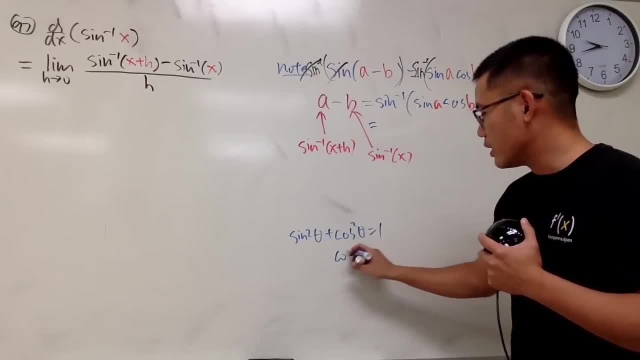 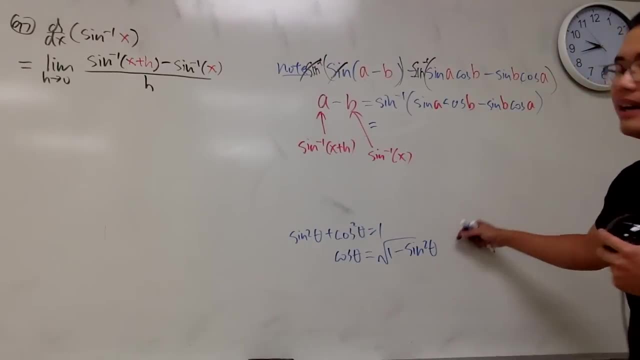 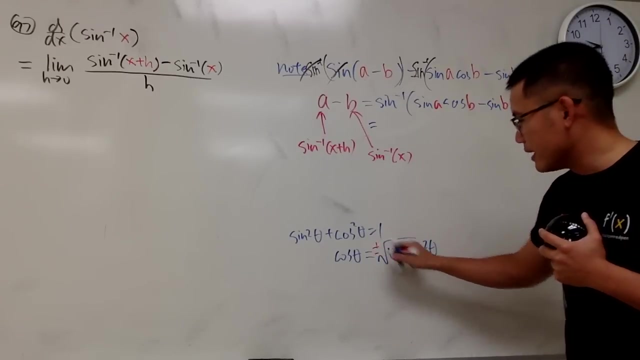 we can just take the square root. So in other words, cosine theta is equal to square root of one, minus sine square theta. Right, Okay, so you might be wondering, should we put down the plus minus? Um, technically we do. 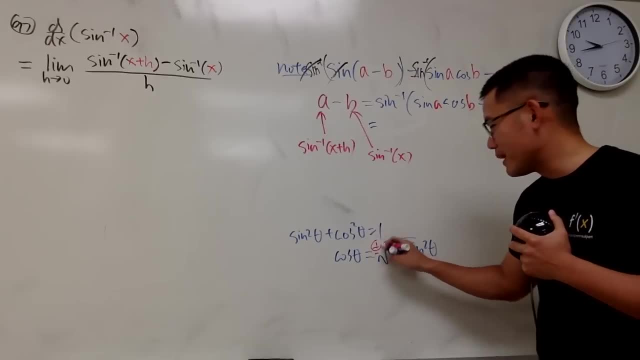 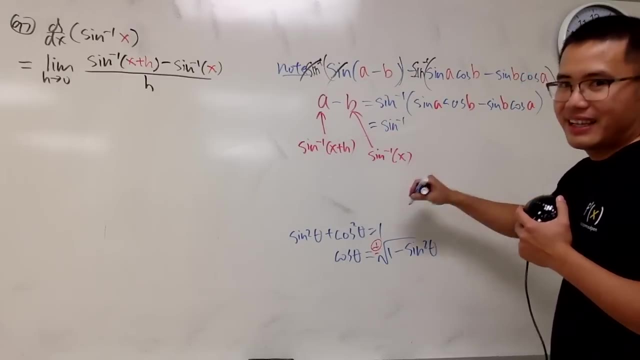 But let's just do the positive version first, okay, Anyway. so what I'm going to do is right here. what I'm going to do right here is inverse sine, and this right here is the same as saying sine a and instead of cosine b. we can look at this. 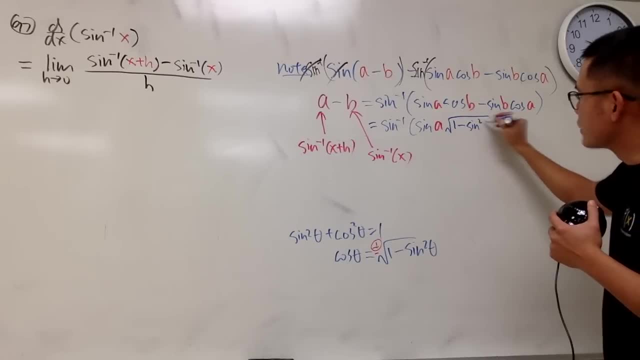 as the square root of one minus sine square b Right, Just like this. And again, let's just deal with the positive version first, And the way you can do it is that you can just say that x equal to that, x approaching zero plus. 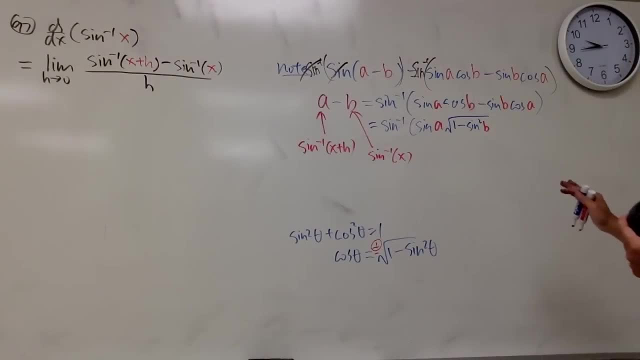 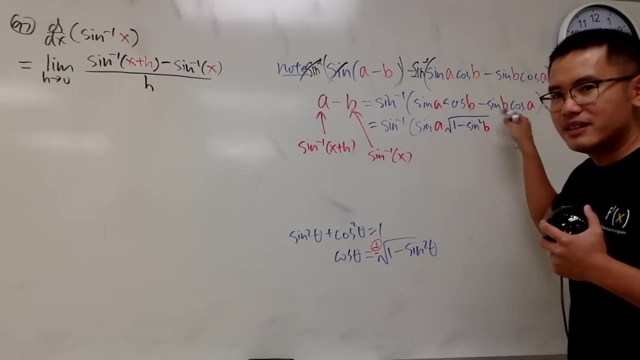 and you can say that's positive or positive. I think that's how you can do it. Or you can just restrict the domain And then the other one. it should be symmetrical. It's minus- minus and you can be able to factor. 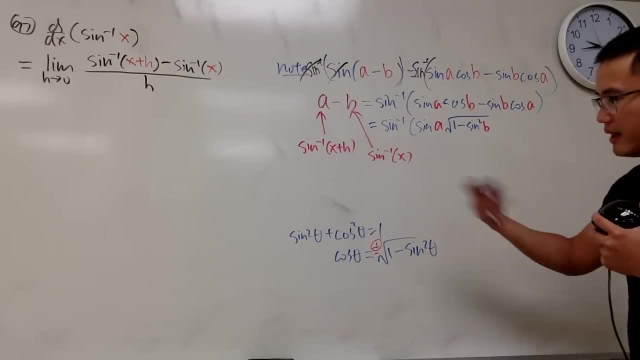 all the stuff. I think that should be it. So let's just do this part and then the other part. you guys do it. Anyway, for the other one, minus sine b, and this is cosine a We don't like. 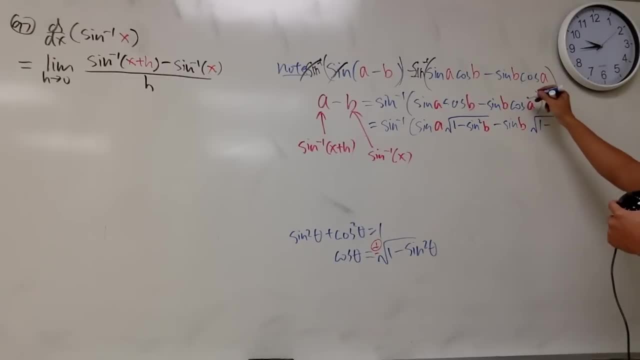 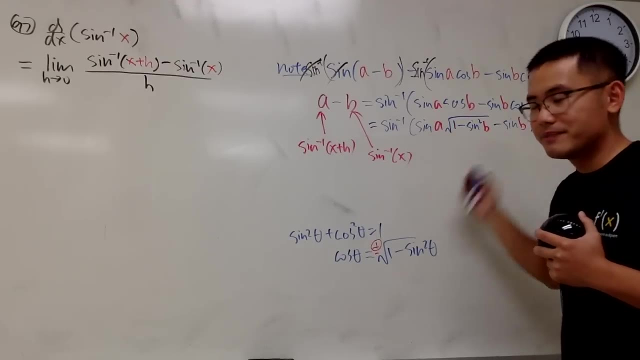 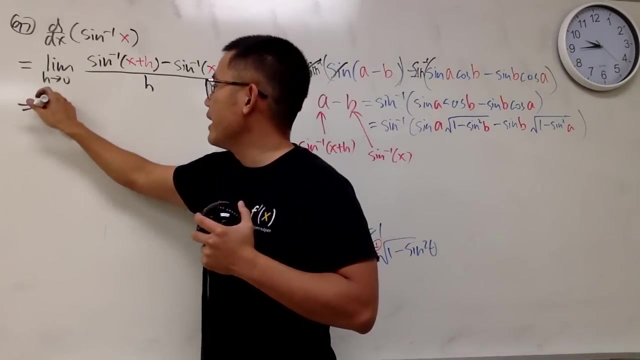 that We write here as square root of one minus sine square a. So this is the version that I'm going to use Now. let's do this right here. Come back here and we take the limit as h approaching zero. Let's see. 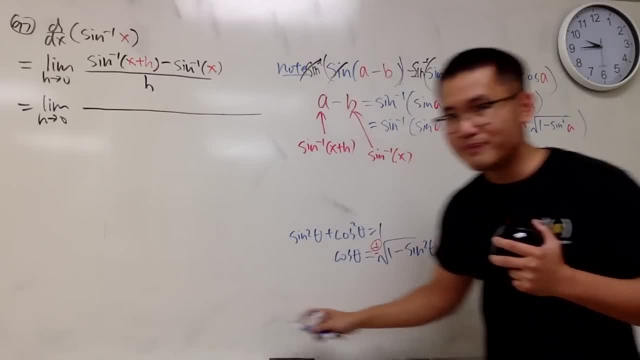 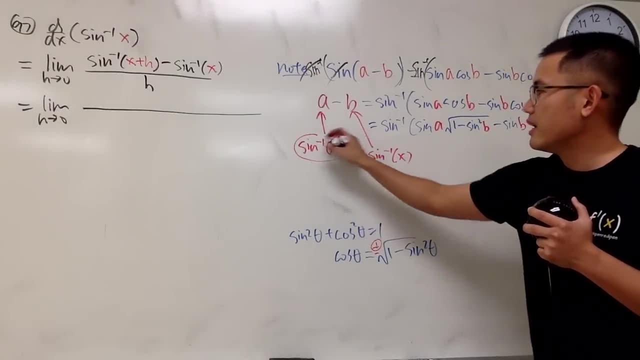 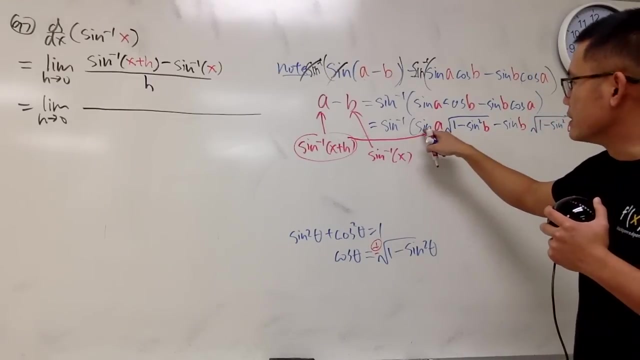 what we have right here. Well, well, I am going to put this right here as the a Put it in here. So I will just do it one by one for you guys. I put it right here When we do that, you see sine. 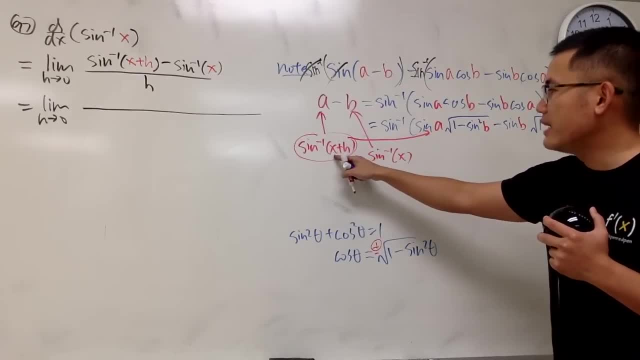 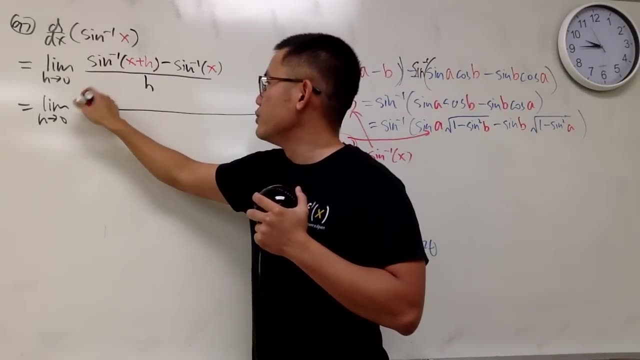 and inverse will cancel. That means we just have x plus h left right here first. And don't forget, we still have the inverse sine right here, So I will write it down for you guys. We still have the big inverse sine right here in the front. 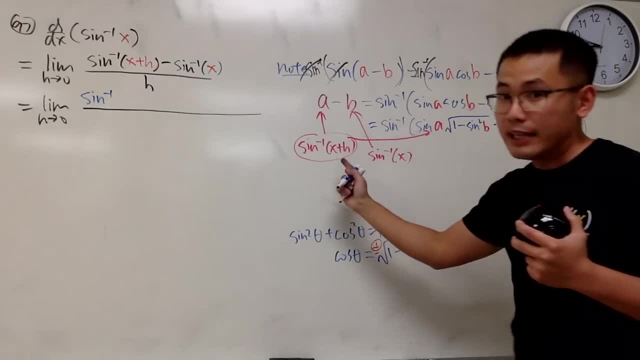 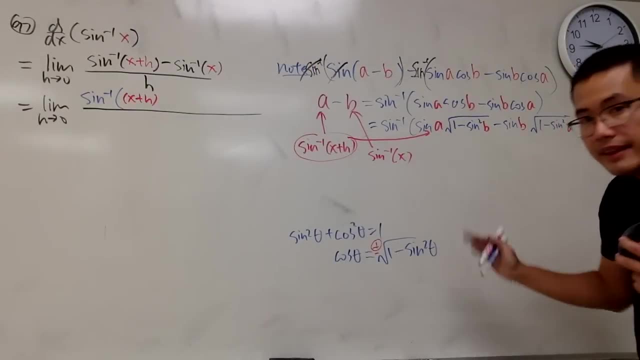 And the first thing that we get right here is x plus h only. So I will just put in x plus h, Right, And then we will do this. Put it here, This is the b. Put it here, And we have the square root. 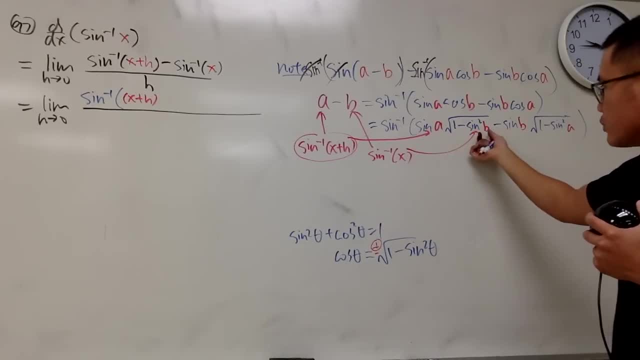 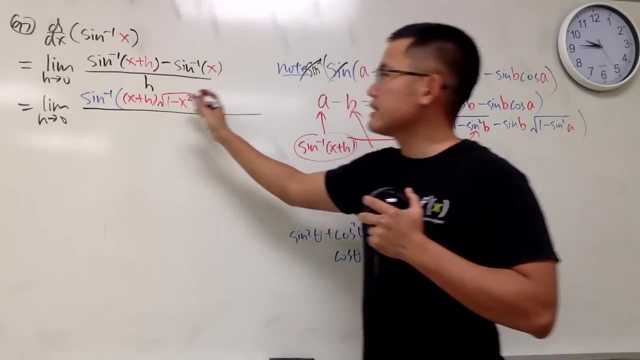 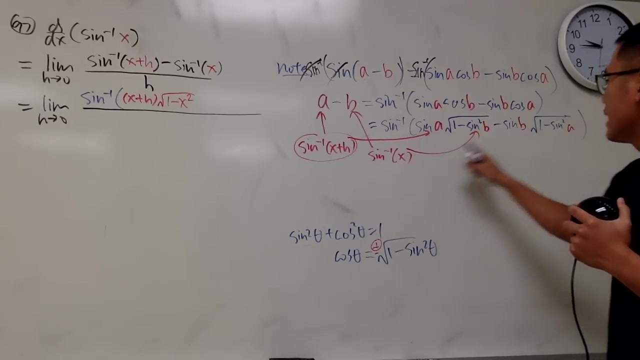 Sine and inverse sine will cancel. So you end up with just x right here And to the second power. So you multiply this by 1 minus x, squared Like that Right, And then continue When you do the same thing this time. 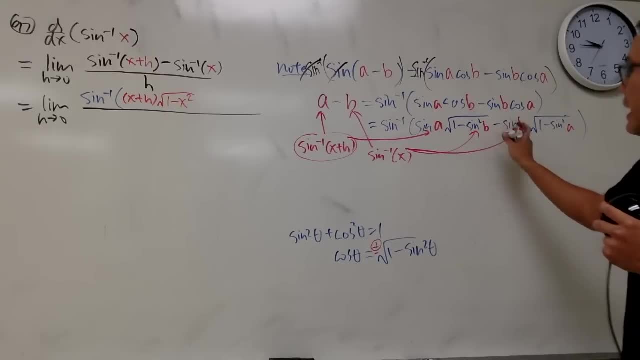 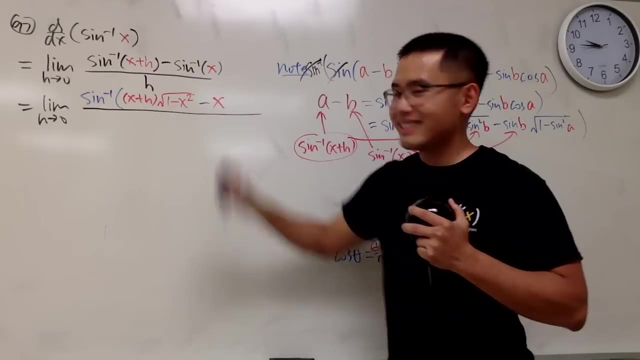 this right here. Put it here: It's just x, because sine and inverse sine cancel, So it's just x. So that's a minus, by the way. So we have minus, just x. And then, lastly, we put this in here and: 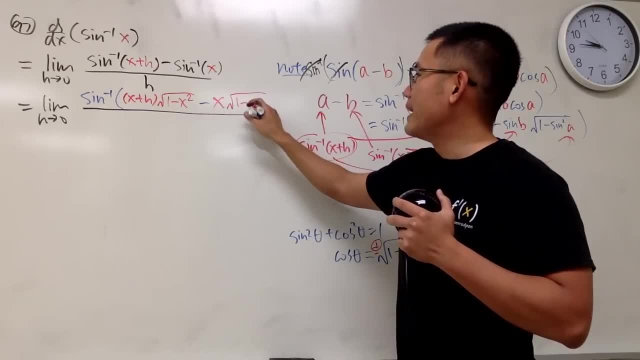 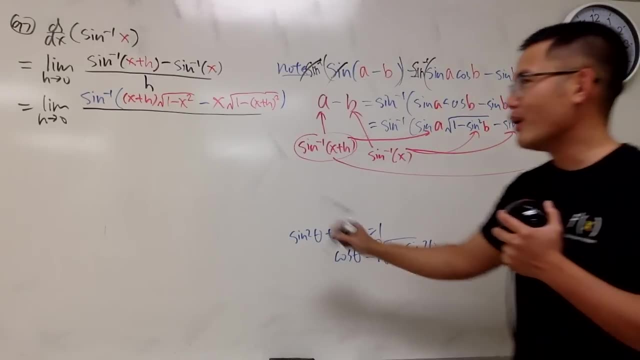 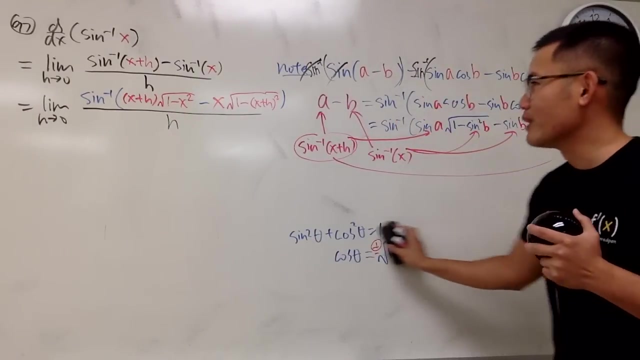 it's pretty much the same speech. We get square root of 1 minus parentheses, x plus h squared Like that. Okay, And then this is still all over h. So this is how you play around with the angle difference formula, Right. 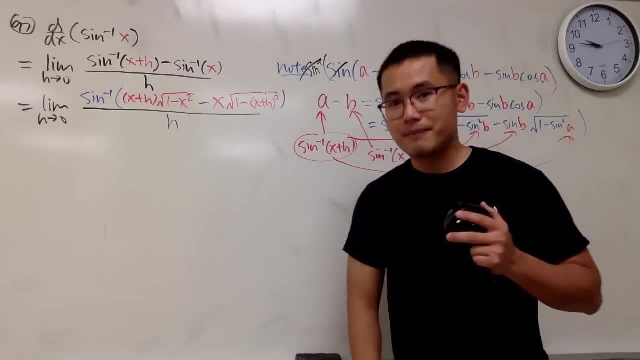 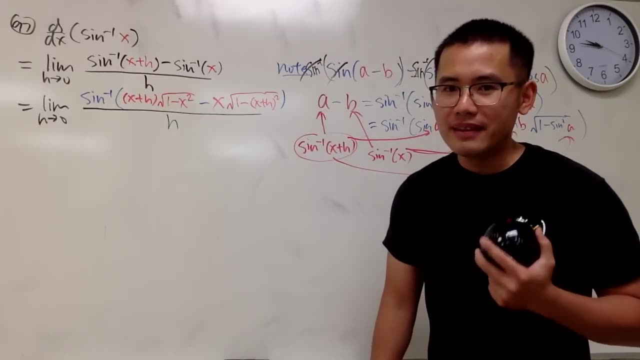 So check this out. We still have the inverse sine and all that stuff. Right, Are we good? Hopefully, Hopefully. right now we are all good, But the next one- I know a lot of you guys will not be so happy about it. 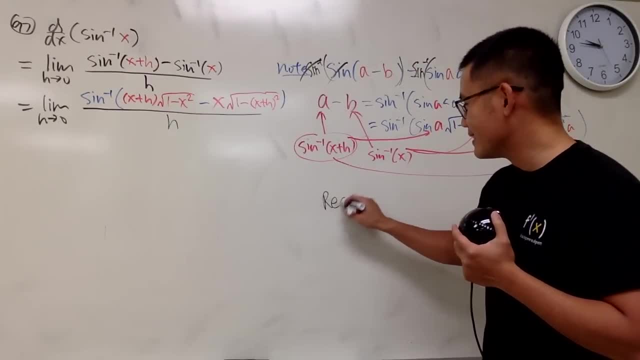 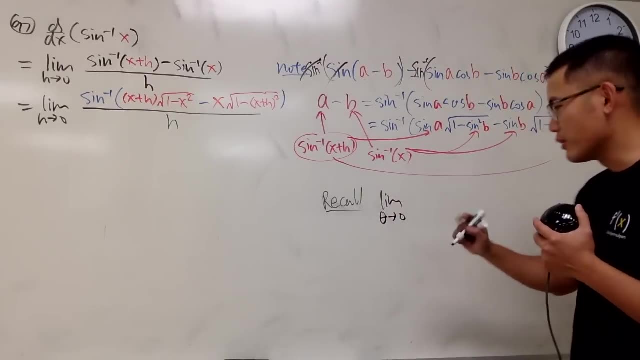 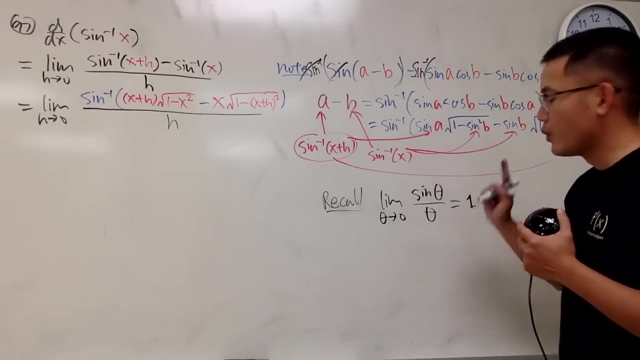 But I'm going to do it anyway. Recall: recall the limit as any angle theta. Okay, It can be h, but let me just use any angle theta, Sine, theta over theta. This right here is equal to 1. Okay. 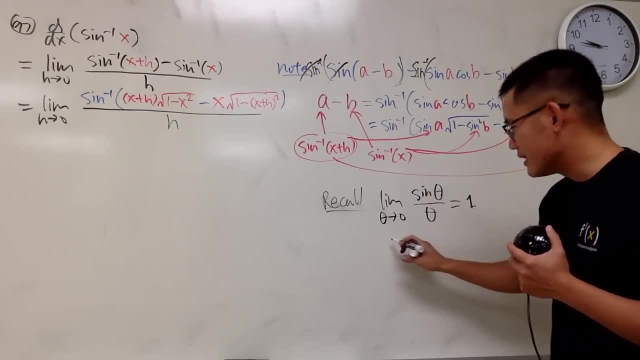 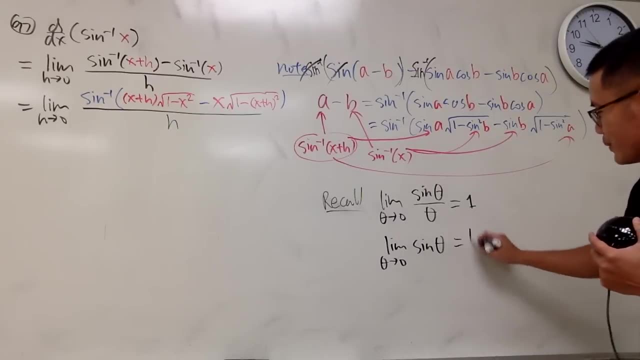 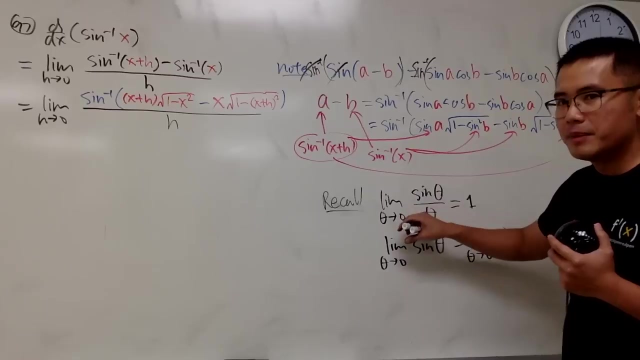 Here is the deal. If you would like, you can look at this as the limit as theta approaching zero of sine theta, This being equal to the limit as theta approaching zero of just theta. You can look at this as the limit of the top over the limit of the bottom. 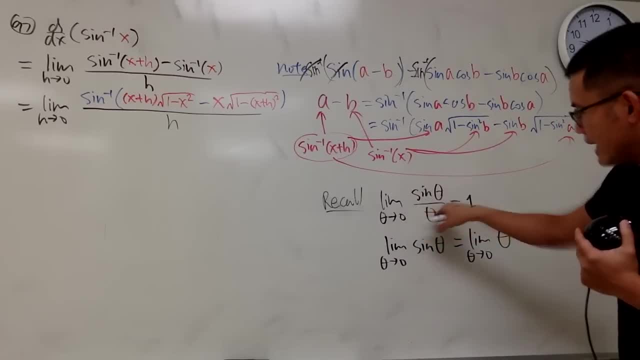 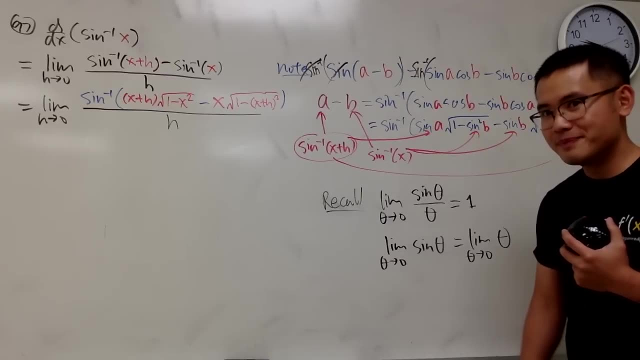 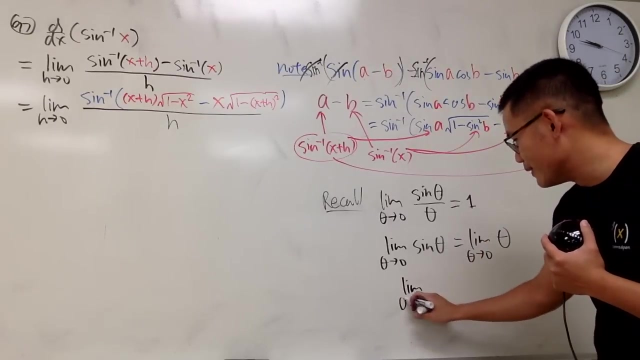 And then multiply limit of that on both sides. It defines the same thing, Okay, Yeah. Lastly, what I'm going to do is based on this. I will tell you the limit of theta approaching zero. I'm going to take the inverse sine on both sides. 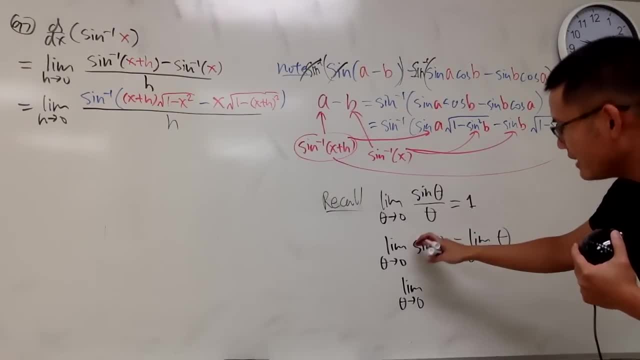 And of course they are continuous. so we can do that. And when we take the inverse sine on both sides, that means the limit as theta approaching zero of theta. this right here is equal to the limit as theta approaching zero of inverse sine theta, like this: 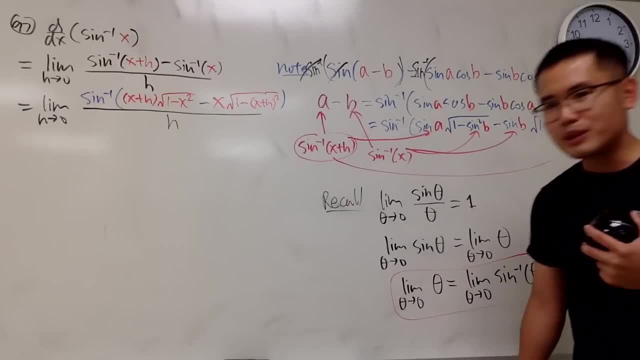 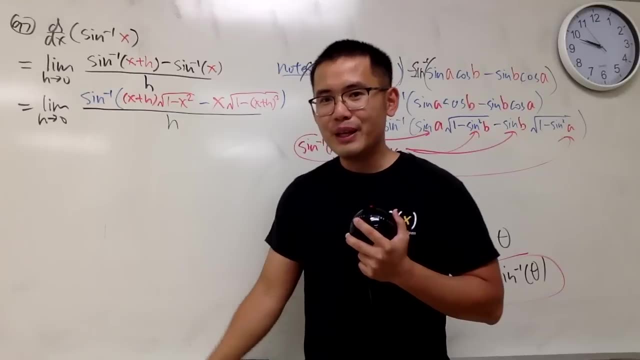 So what am I doing? Well, look at this one and look at it backwards. What it's saying is that, hey, if the inside right here is small, even though you're inside of the inverse sine, you can just forget about it. 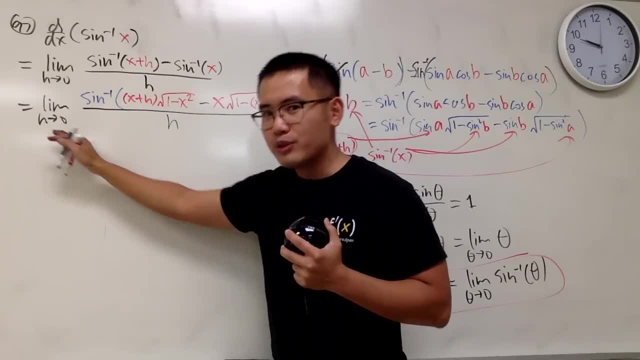 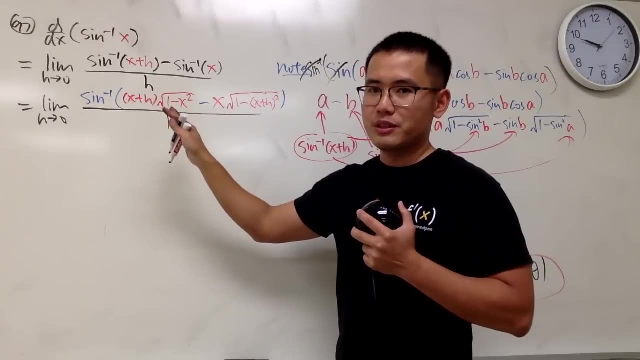 Check this out: h approaching zero. if you're putting h approaching zero here, you're putting zero. this is just actually the same as theta, so inside is actually approaching zero as well. So this is legitimate. Let me put this down. 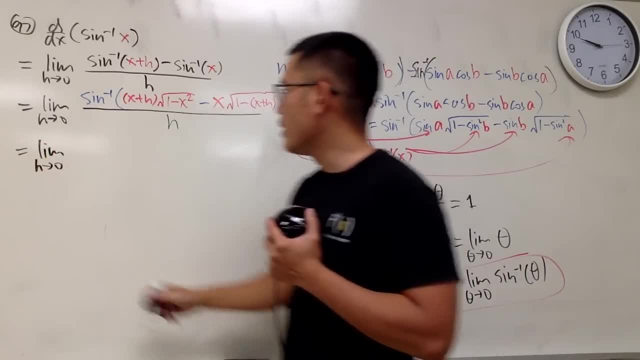 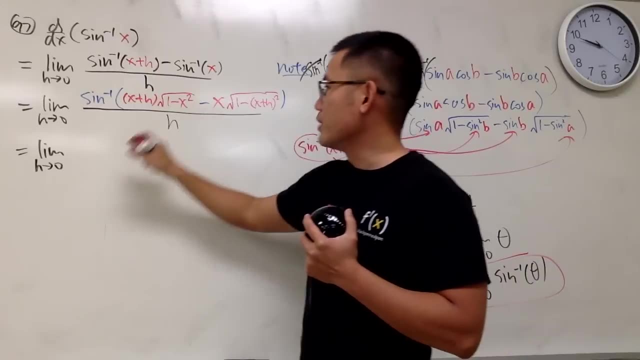 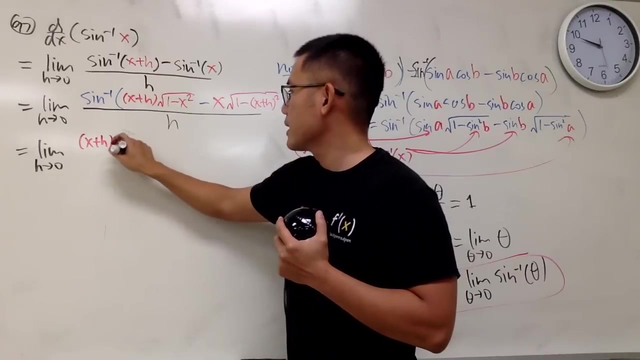 This right here is the limit. as h approaching zero, You can just drop the inverse sine, because again we have the inside: it's approaching zero. So we can just put this down: x plus h square root of one, minus x squared, And then this is minus x square root. 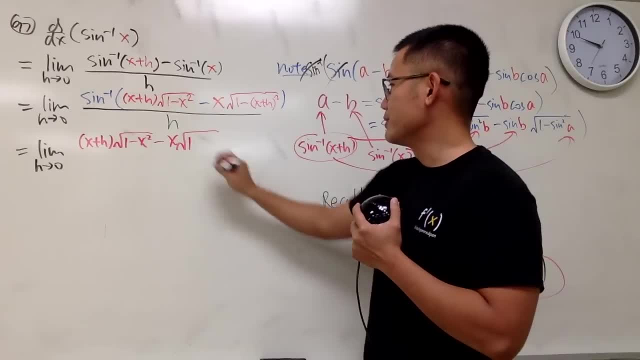 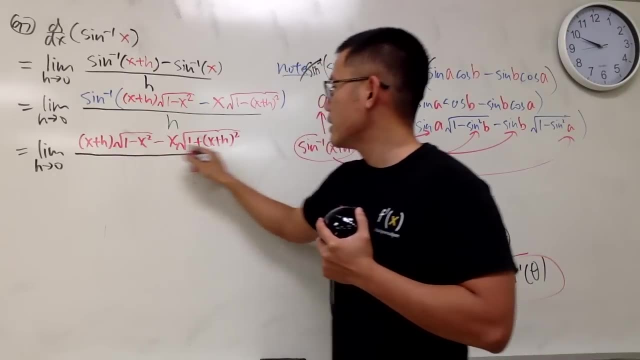 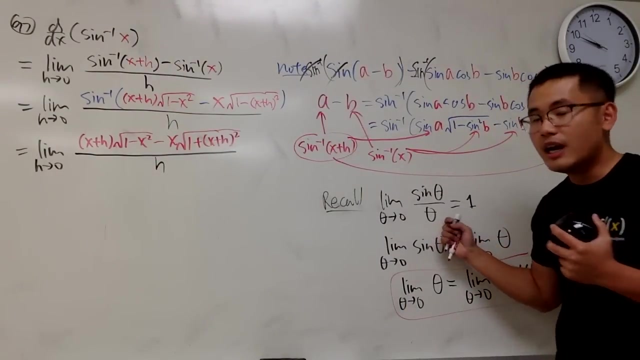 of one minus- excuse me, because it's being so many hours, and then this is all over h. So again that. And now, seriously, you don't have to do, you should not do L'Hospital's rule on this. You should do geometry for this. 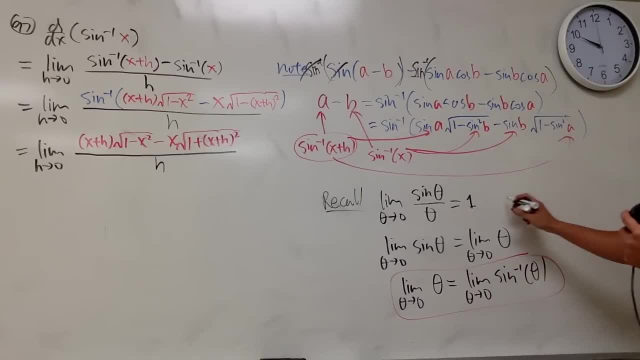 And then, based on that, you can come with all this And the picture is like this: okay, This is the picture, So you get this right here. you can get a triangle and you can get the arc, and you can get a. 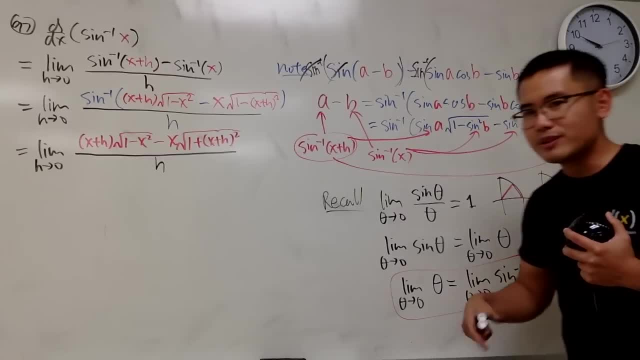 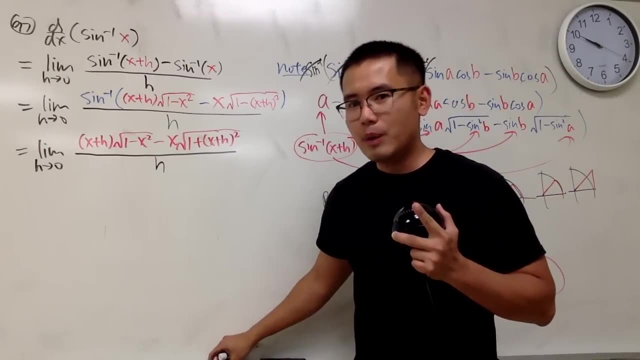 tangent And you can, you know, do some series theorem to figure it out: 100 limit. I'll promise you I'll do that In my 100 limit video, But not now. So hopefully this is legit okay. 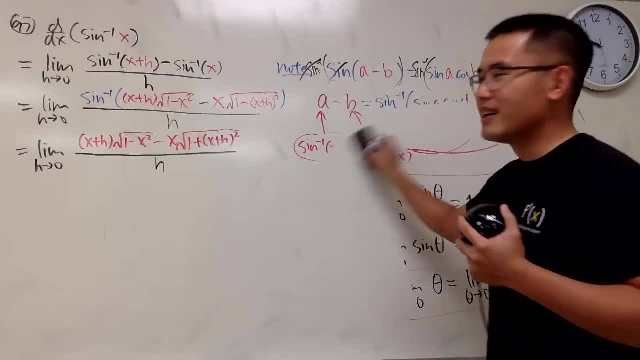 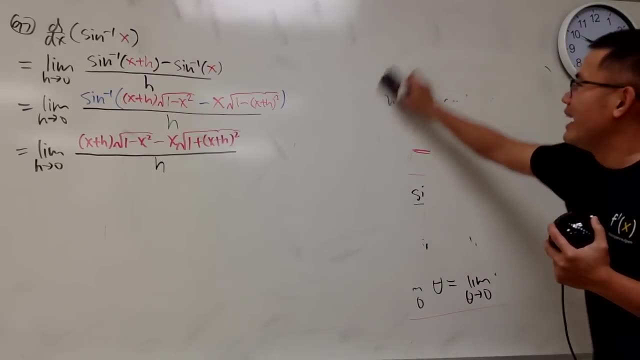 Okay, This is pretty good because this is pretty algebraic. There's no more like inverse sign or regular sign whatsoever, And the good thing is, if this is algebraic enough, we can just do the usual thing right. 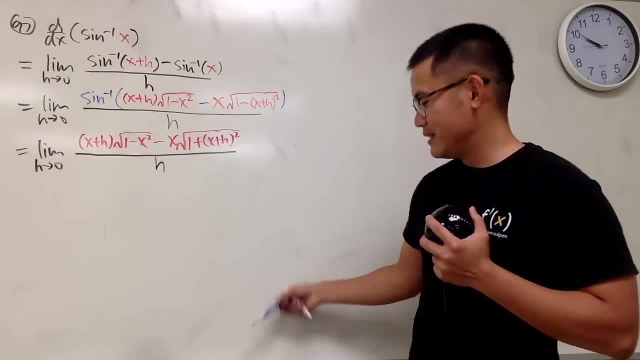 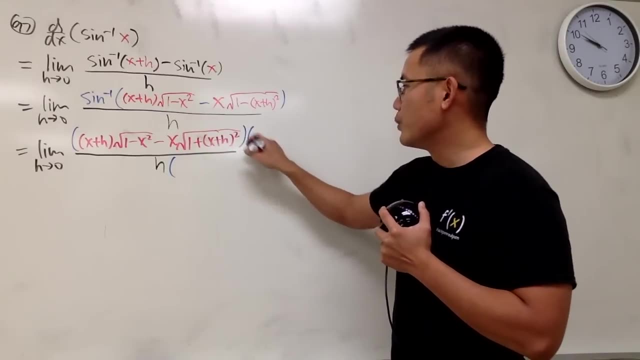 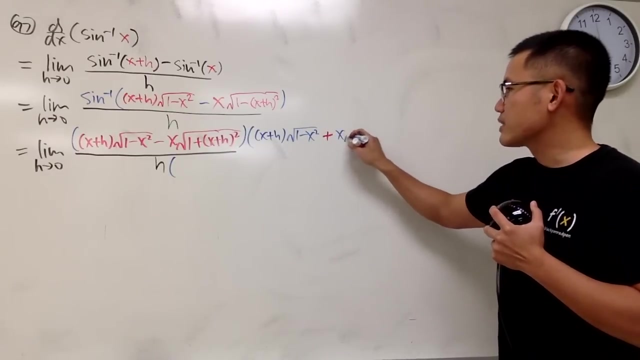 Do the count you get. So multiply this right here, which is about the count you get. Namely, we just do x plus h times square root of 1 minus x squared plus x. squared root of 1 plus x plus h. 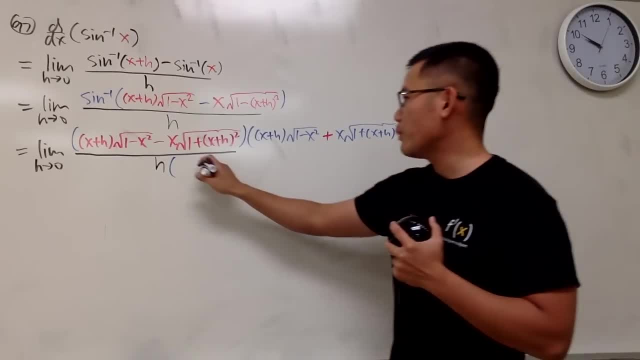 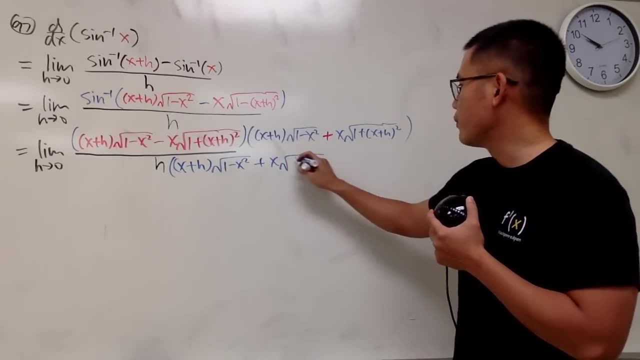 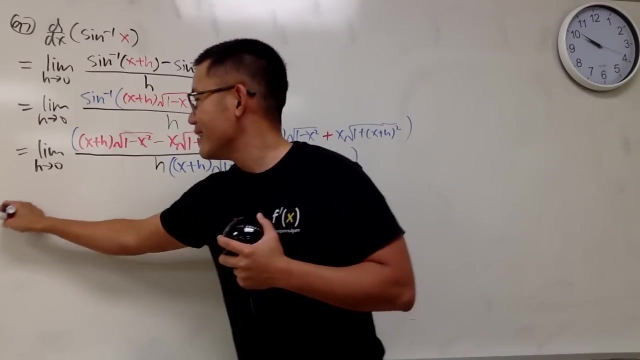 squared This right here And also put that one on the bottom right here: Square root of 1 minus x. squared plus x. squared root of 1 plus parentheses, x plus h. squared like that. Man, This is life On the top. 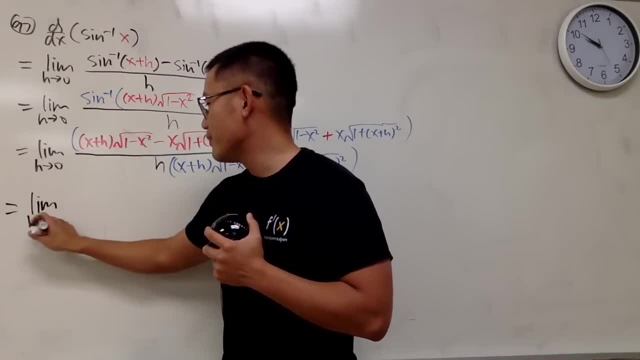 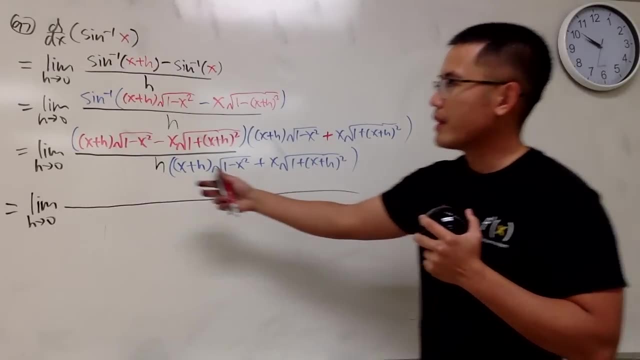 this is actually not that bad to multiply the L, because it's in the form of a minus b times a plus b. You guys should know that, right. So here we go. So we will just have this being squared Namely: 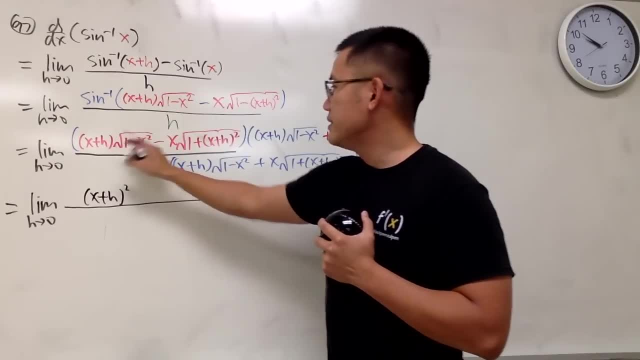 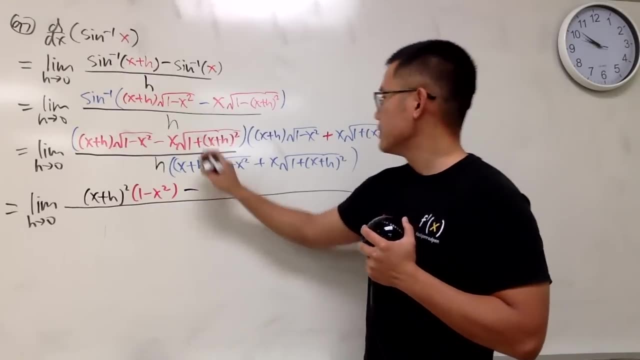 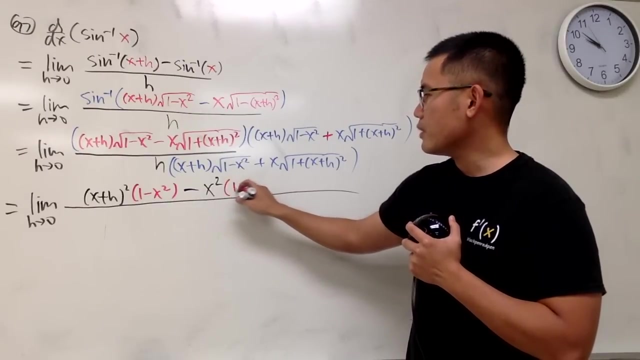 x plus h being squared And this thing squared, which is just the 1 minus x squared, okay, And then minus this and that, so you pretty much just have x being squared and this right here being squared by itself, which is 1. 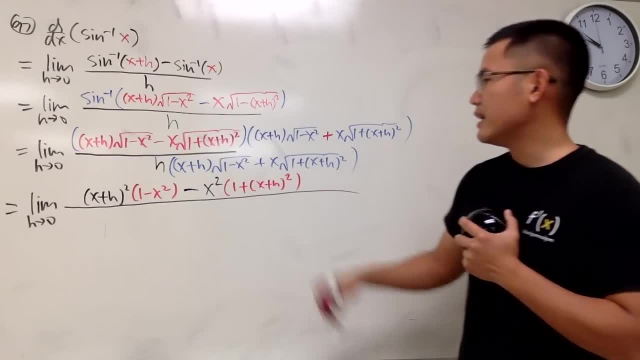 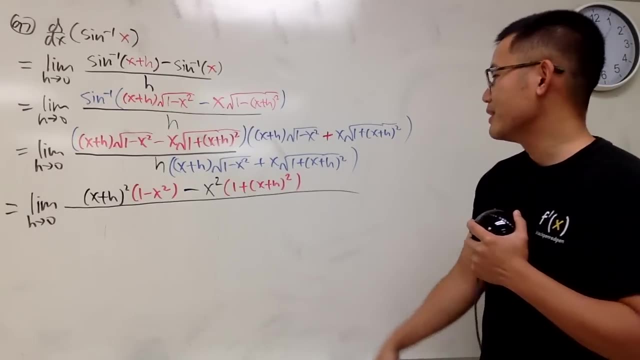 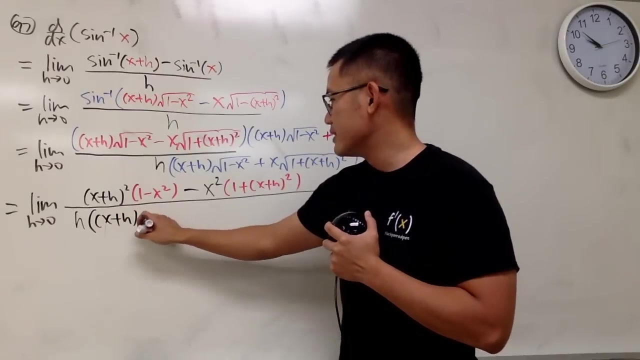 plus parentheses, x plus h, squared like that. And, uh, multiply out the bottom, okay. So here we have No, don't multiply out the bottom. And then just, I mean rewrite the bottom: x plus h and square root. 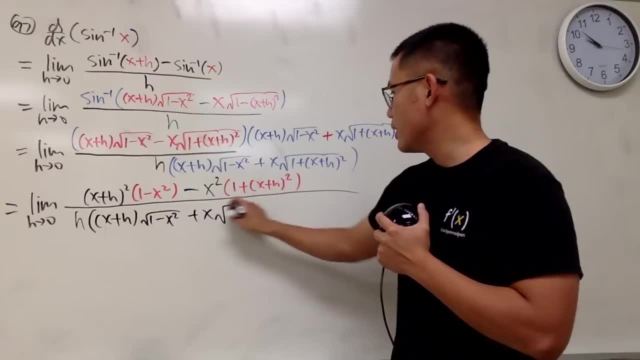 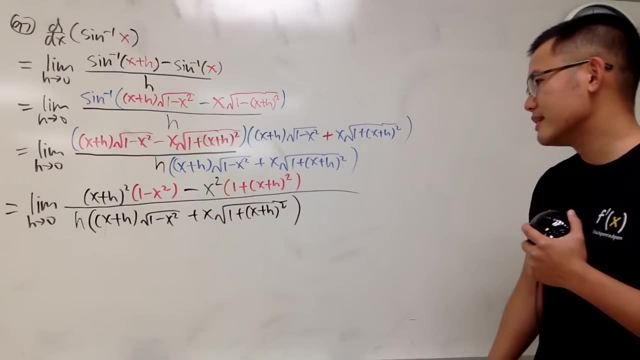 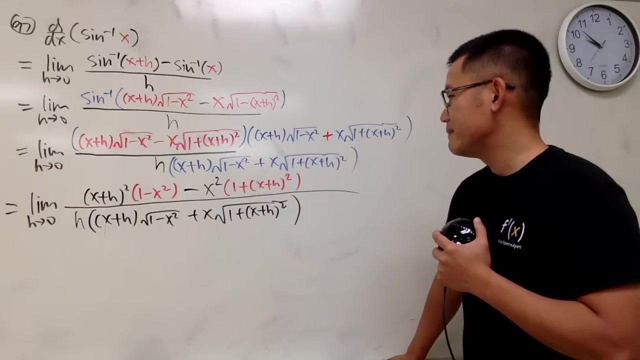 of 1 minus x squared. plus x squared. root of 1 plus x plus h squared. Yeah Man, why is this so? Let's see, Is there any fast way to cancel this guy out? I feel this should be a fast way. 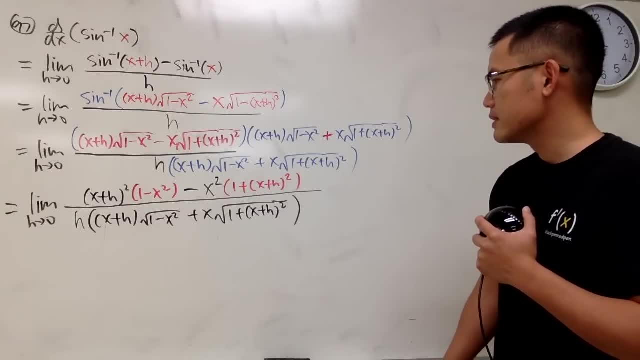 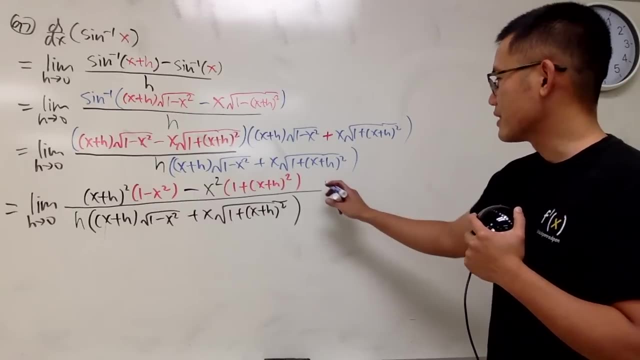 to cancel out the top. Let's see, There, I think it is Alright. so just the top. okay, Just the top, Just the top, Just the top, Because I don't want to write this guy down again. So 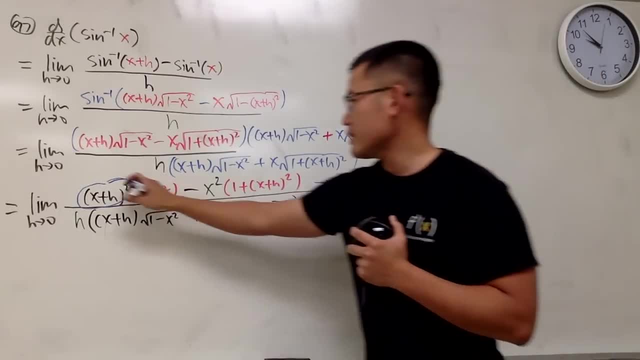 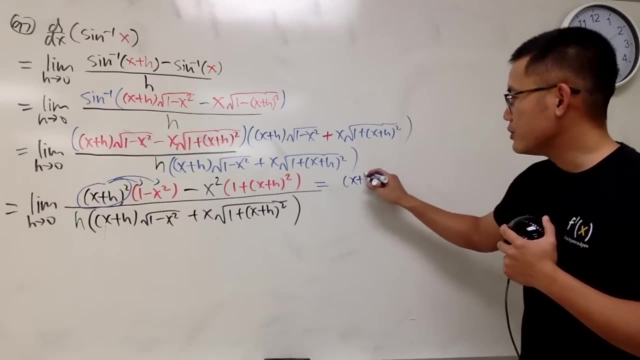 if you take this guy and then distribute it, okay. So let's see what we get. We should get just the top, okay, Equal sign, just algebra. So x plus h squared yeah, And then minus x squared times that guy. 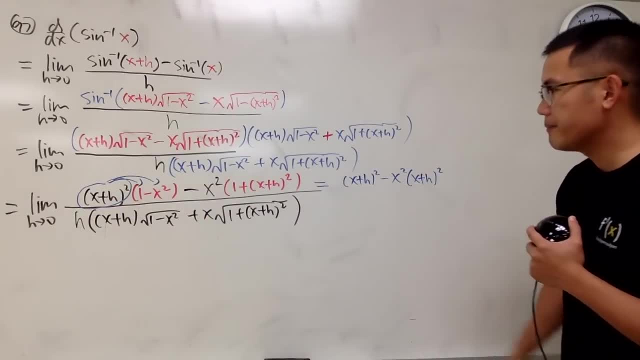 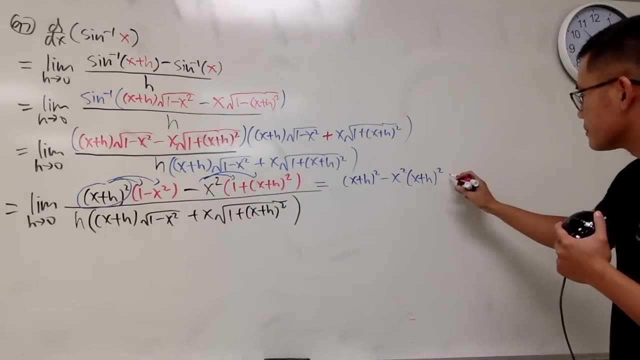 So x squared times x plus h squared. yeah, Next we take this guy, distribute, distribute So we have negative x squared And then minus x squared. Ah, yes, yes, yes, I see this guy now. Okay, okay, okay, okay. 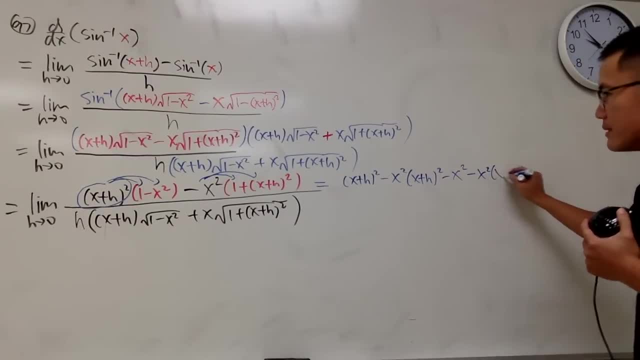 We're good. we're good, we're good. x squared times that guy. So x squared times, x plus h squared like that. Okay, You're kidding me, This is minus. Wait, they don't cancel out nicely. 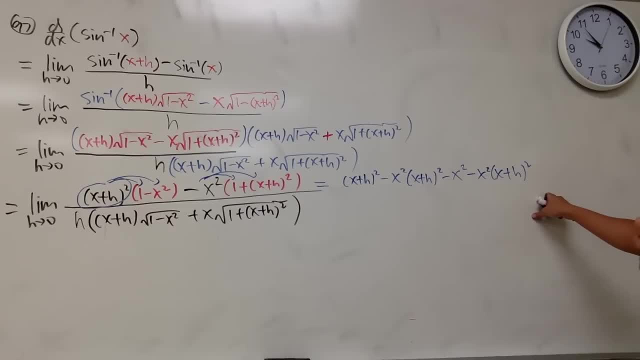 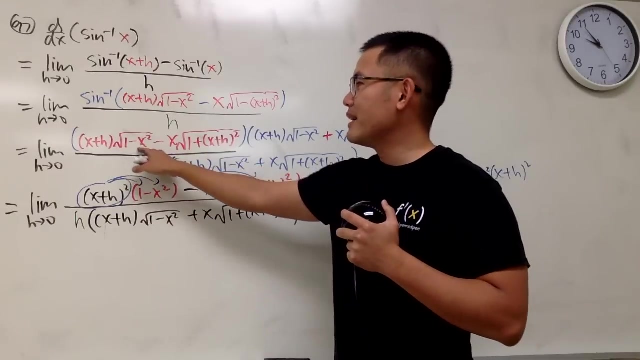 Let's see, let's see, let's see. Did I make a mistake somewhere? Hopefully not, I am afraid. so I didn't make a mistake. Okay, 1 minus x. squared This right here have been a 1 minus. 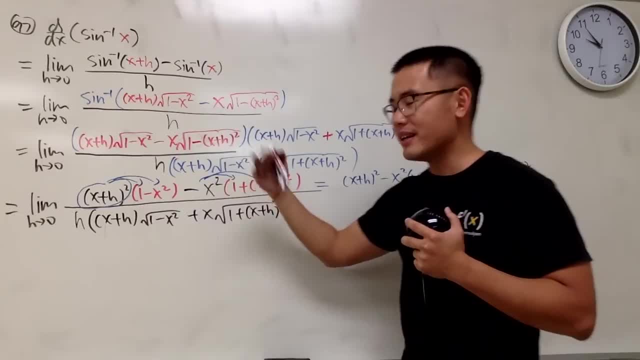 1 minus. okay, 1 minus, Because remember it's 1 minus cosine squared and that you take cosine to be the inverse, all that stuff, right? Sorry, 1 minus sine squared, So that should have been a minus. 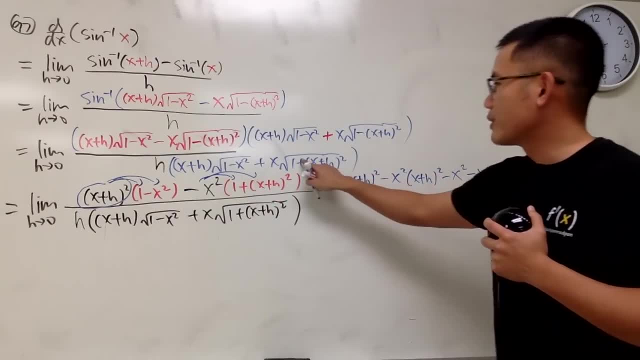 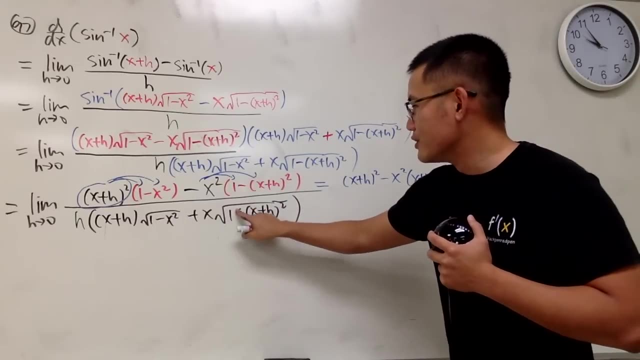 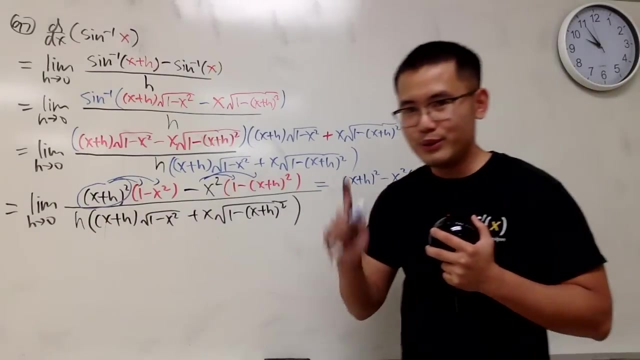 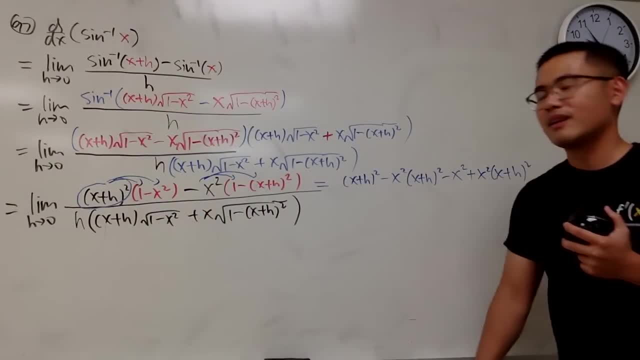 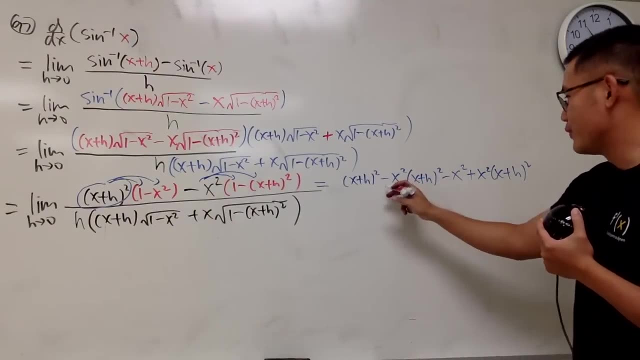 this guy, it becomes a plus. Thank all my subscribers, Alright, so okay, hopefully you guys are okay. okay, If you want to watch how to do this, of course you should be able to do all that. Anyway, this and. 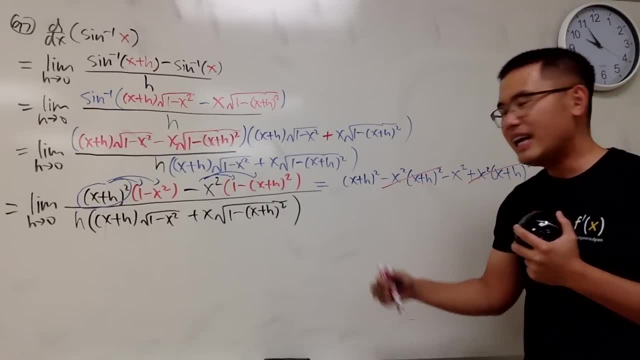 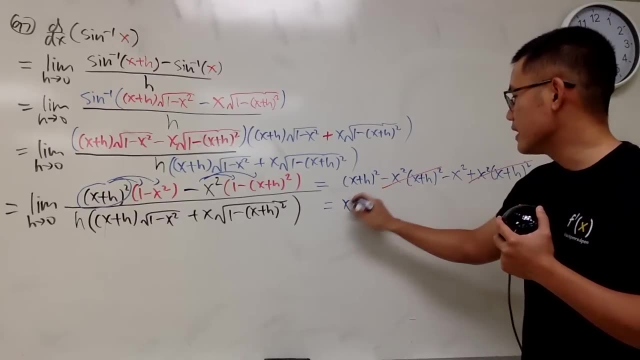 that cancel each other on 9th D, And it happened when we did this, So let me not do anything fancy and just multiply this out: This is x squared plus 2x, h plus h squared, and this is minus x squared, So this: 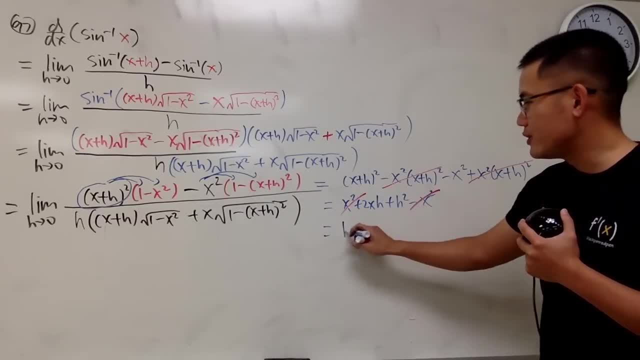 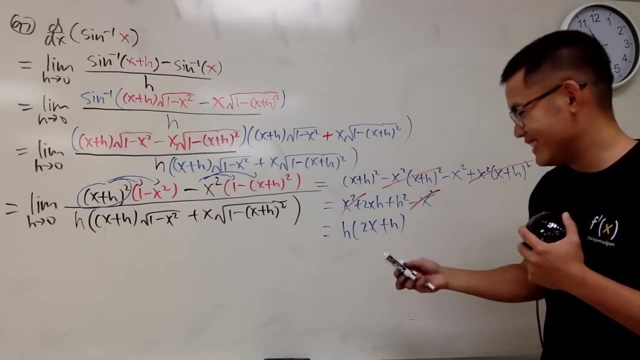 and that cancel again And you see I can factor the h, So we get 2x plus h, Like that. This is what's happened on the top. Alright, so I will just do this one legitimately, okay. This right here is the. 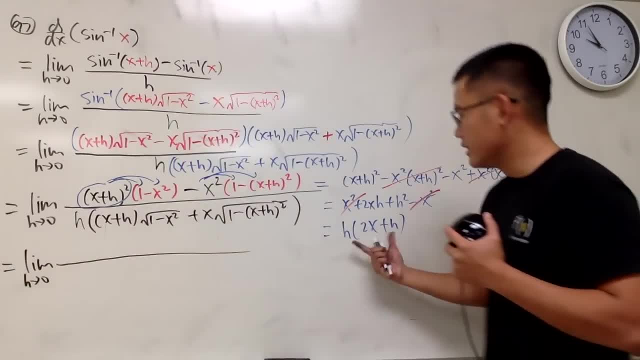 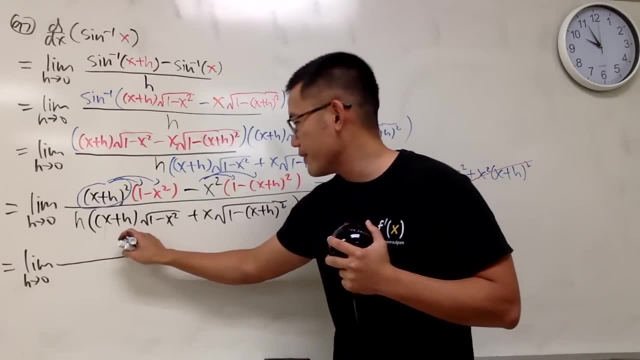 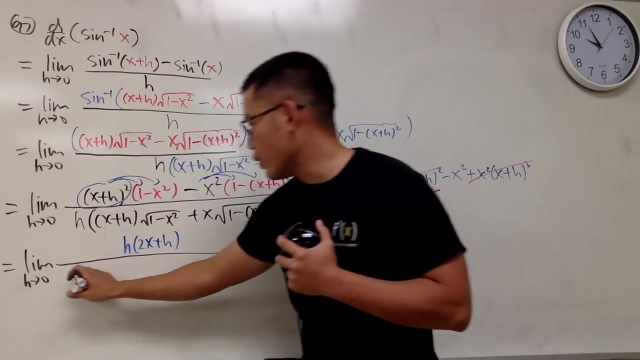 limit as h approaching 0.. This is on the top, alright. So we have h times 2x plus h. Okay, And we have the h all the way in the front. Okay, here we go: x plus h, And then this is the square root. 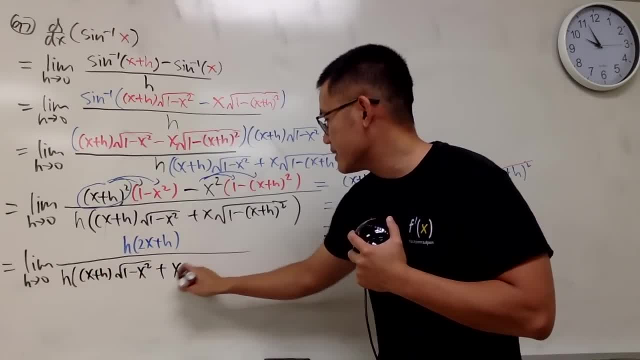 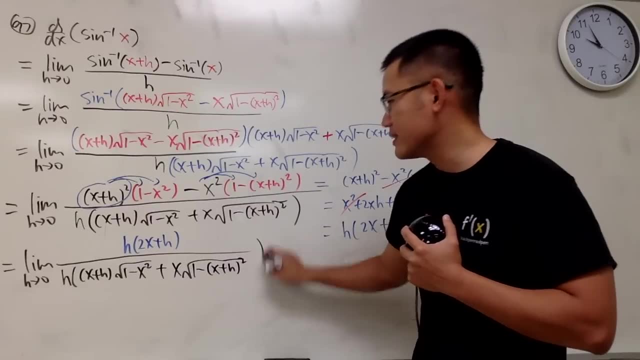 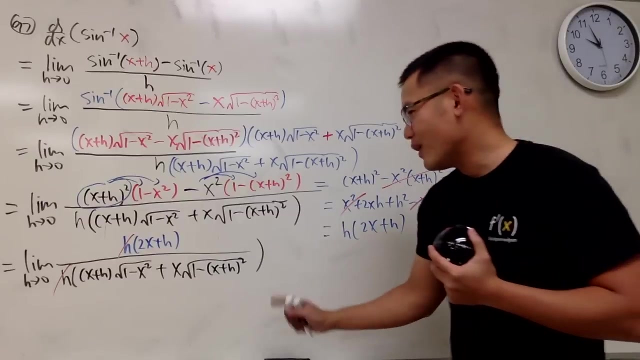 of 1 minus x, squared And plus x 1, the square root of 1.. Man, this is minus, And then x plus h, squared like this: Oh my god, Cancel out this h. Oh, cool, And now, of course. 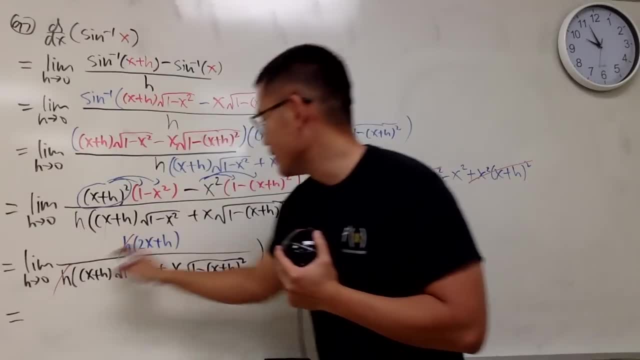 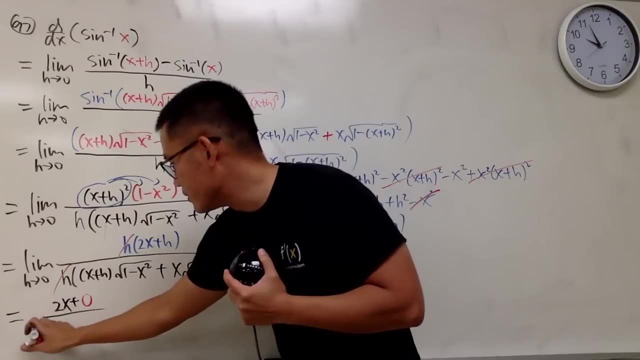 we just have to plug this 0 into all the h, So putting 0 in here, we get 2x plus 0 over. Okay, don't panic. This right here is just x plus 0.. This right here is square root of 1 minus. 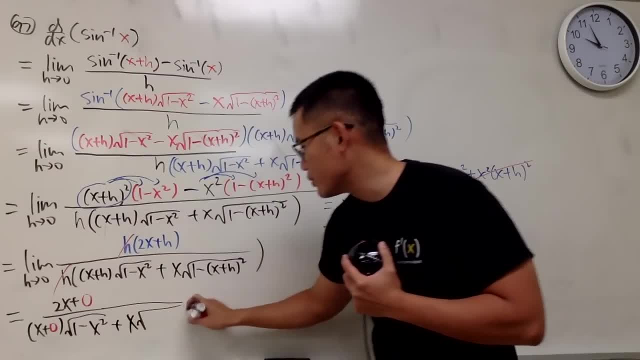 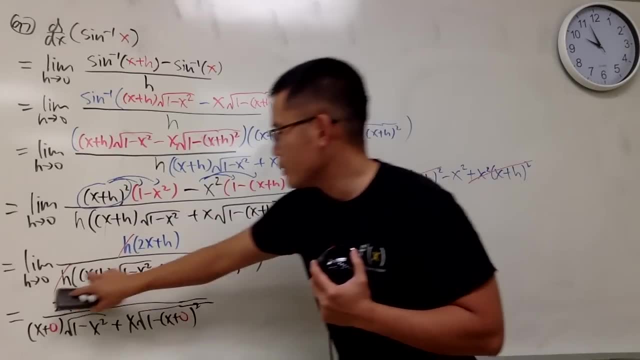 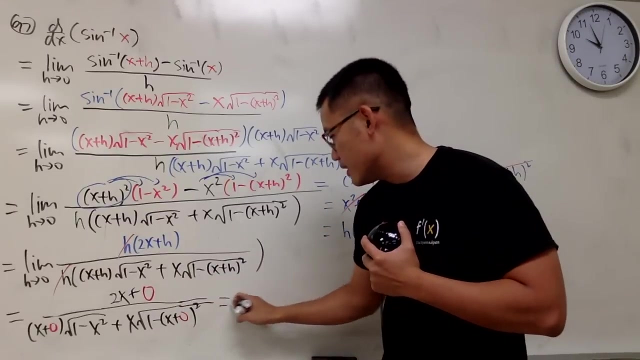 x squared, And then we add x times square root of 1 minus parentheses, x plus 0 squared. Yeah, Man, I also want. I just want to put up 2x plus 0.. Finally, we see on the top it's just 2x. 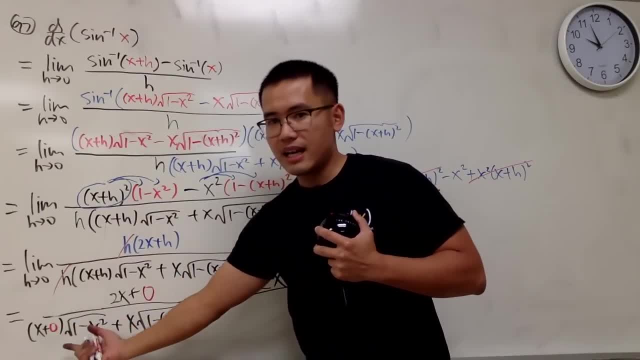 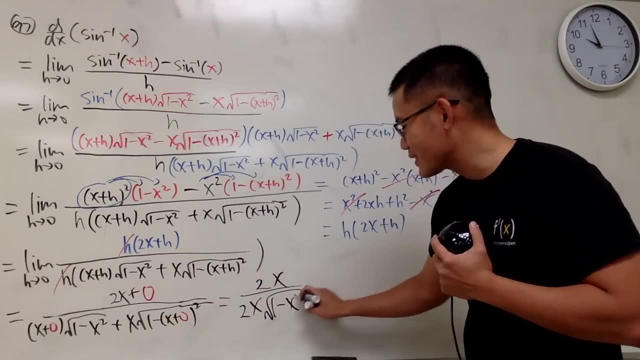 On the bottom. check this out. This right here is x times that x times the same thing. So you have two of them, Namely, you have 2x times what Square root of 1 minus x squared. And what happened with the 2x? 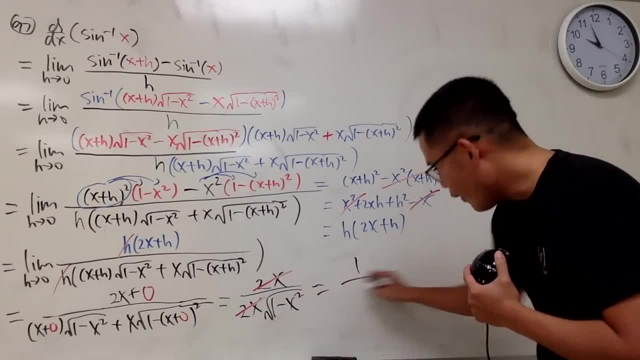 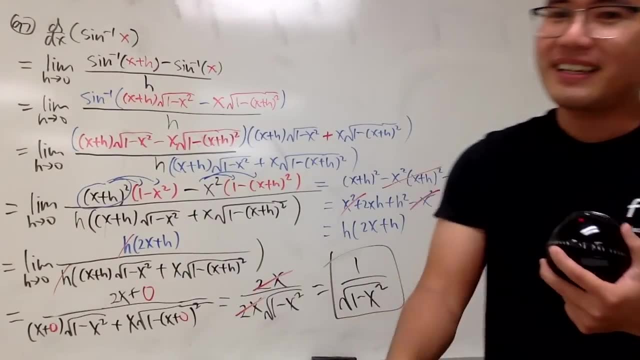 Bye-bye, Bye-bye. We get 1 over square root of 1 minus x squared. Oh my goodness, How long did this take me? Oh my god, man. So, as I told you, this is why I said: oh man, I don't know if I 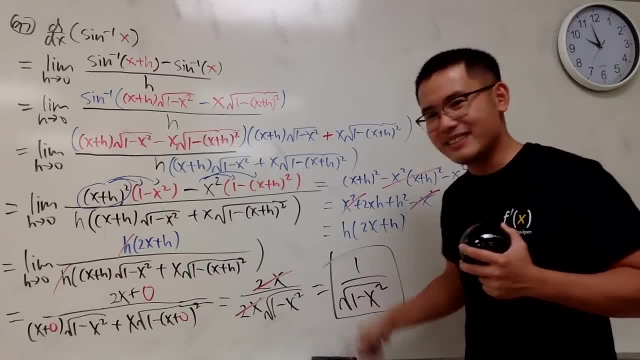 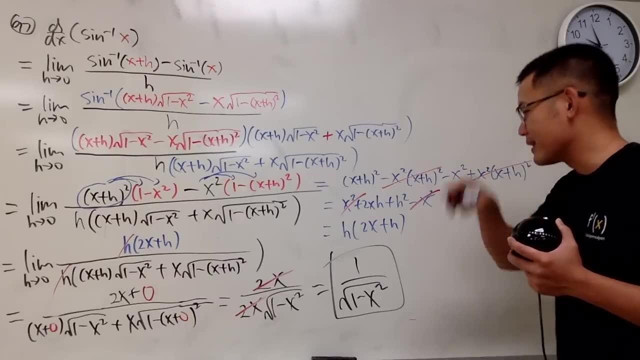 was ready for this or not. but this is it. This is it okay. This is hopefully from here to here. you guys are feeling okay, You guys think this is really legit and all that right. So good, 10 o'clock already, Man. 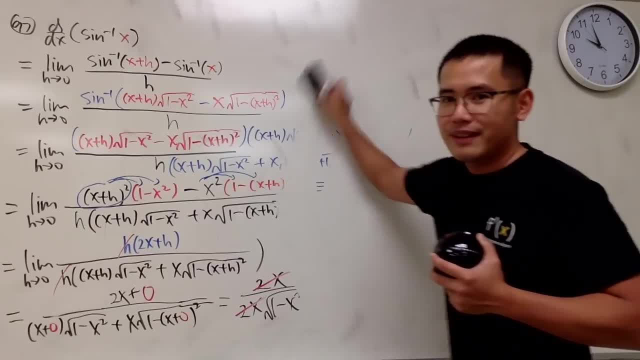 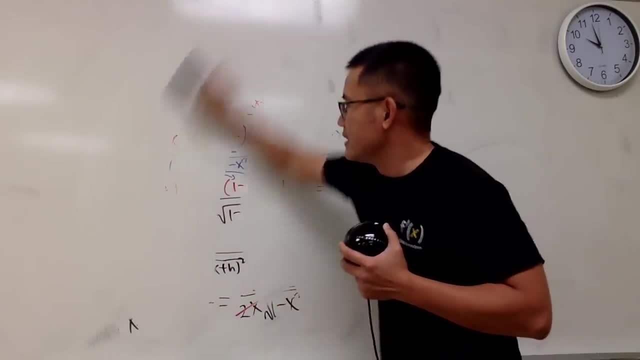 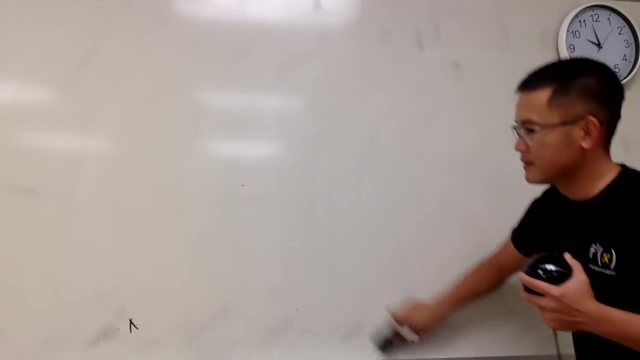 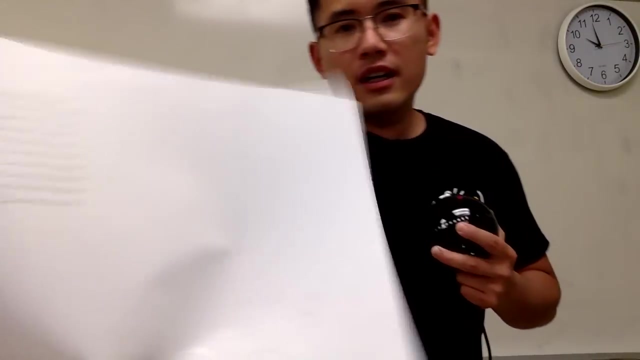 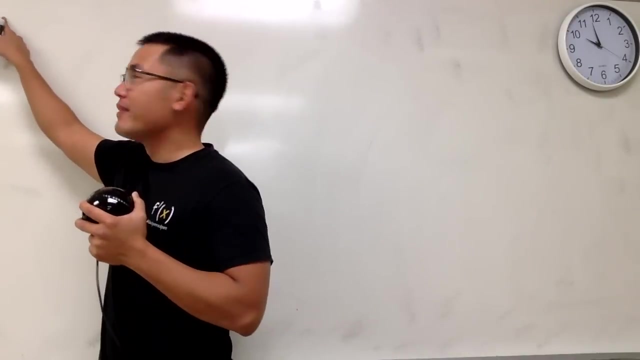 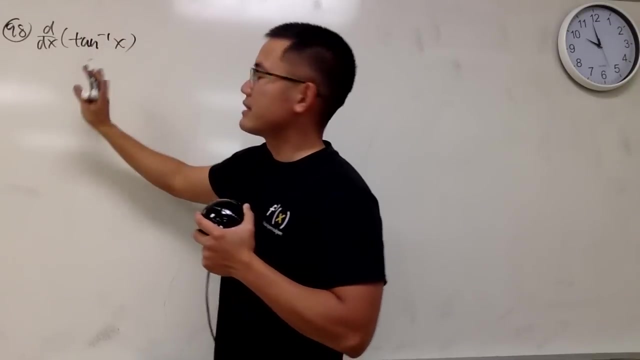 Alright. Number 97.. Ugh- Inforstention of X flows. the definition Alright, So, Without wasting any time, Number 98.. D'x- inverse tangent of x, Right. 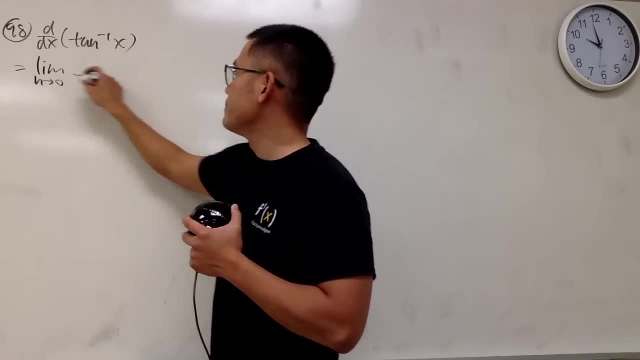 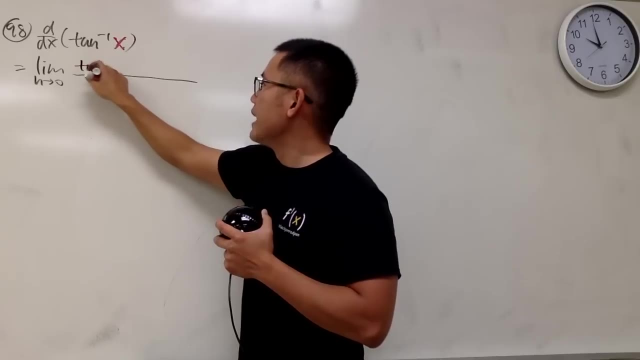 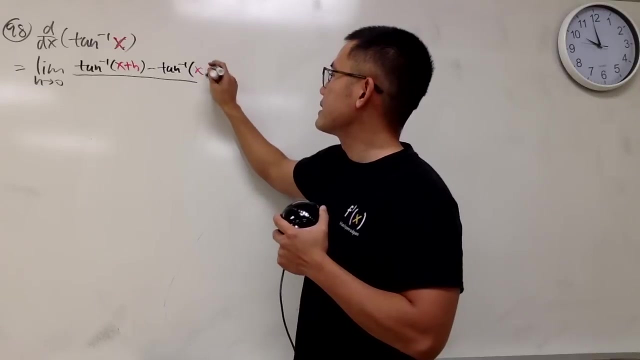 So here we go. Take the limit as h approaching 0, and again this right here is h. so this is, this is x. This right here is going to be the inverse tangent of x plus h, and then minus inverse tangent of x, and then this is all over h. So what do we do? 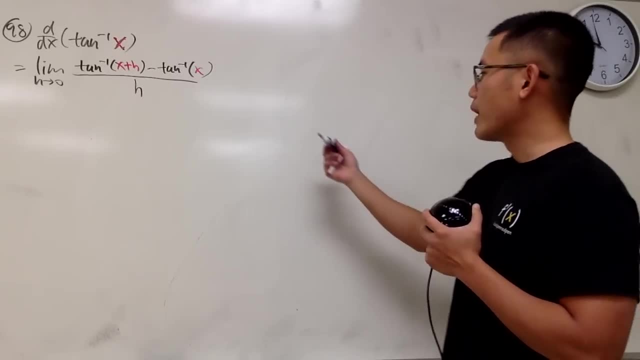 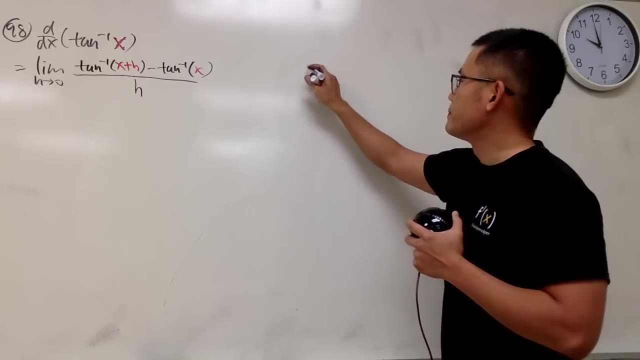 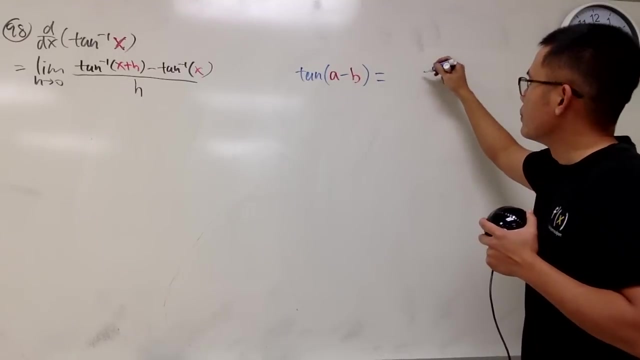 We do the same thing as what we did earlier. Therefore, right here we will just do the tangent situation and again I want the tangent subtract, the angle subtraction formula. So you look at, tangent of a minus b, This right here, is equal to. let me just tell you guys what the answer is. okay, This right here is equal to. 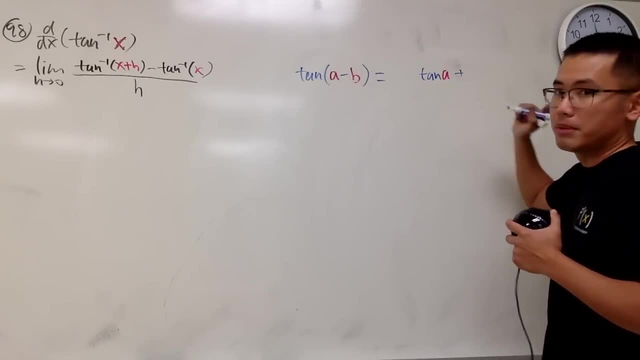 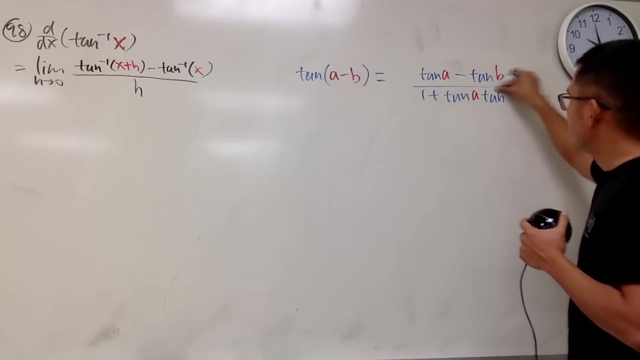 tangent of a plus. okay, this right here should be a plus, sorry. tangent of a minus minus, right, minus. tangent of b over 1h. Here's the plus Tangent a times tangent b. okay, And you know the deal. What we do is we'll just take the inverse tangent. 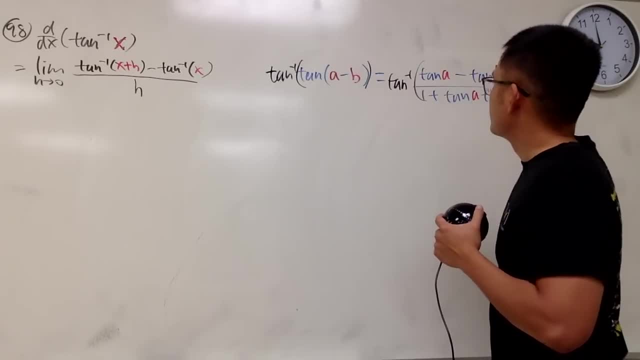 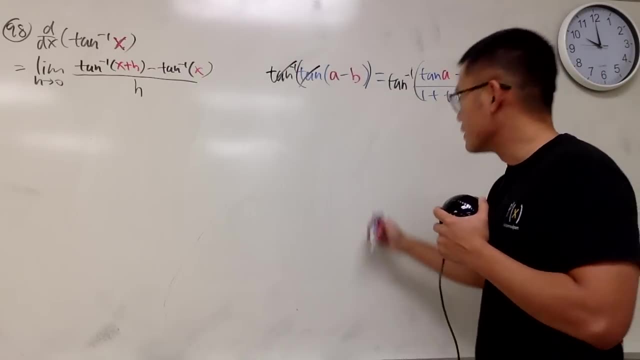 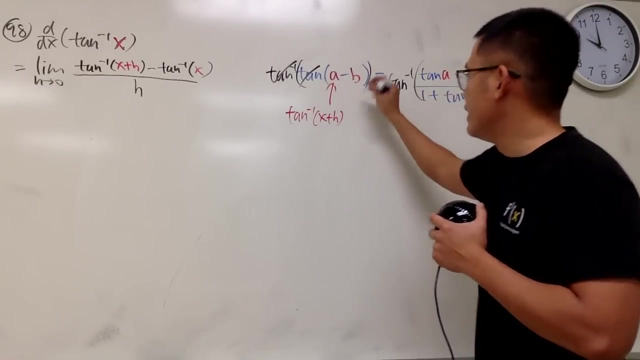 on both sides. Okay, Take the inverse tangent on both sides, so they will be gone. and then, of course, for this a, we'll just make it to equal to inverse tangent of x plus h, and then for the b, we'll just make it equal to inverse tangent of x. 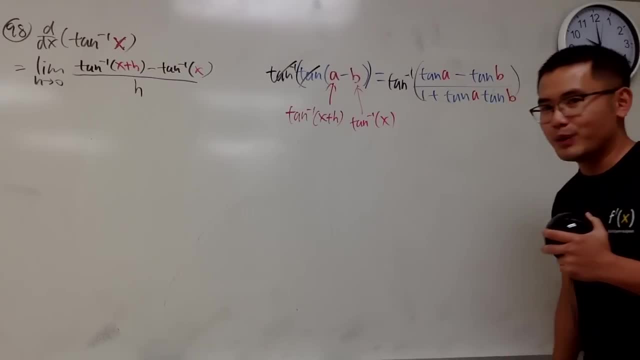 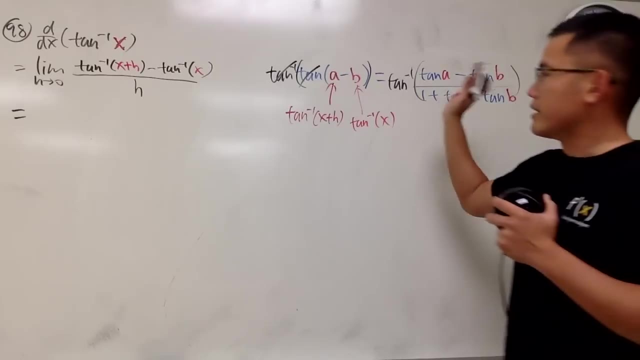 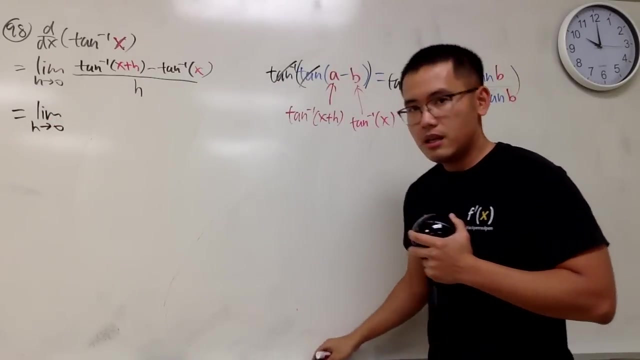 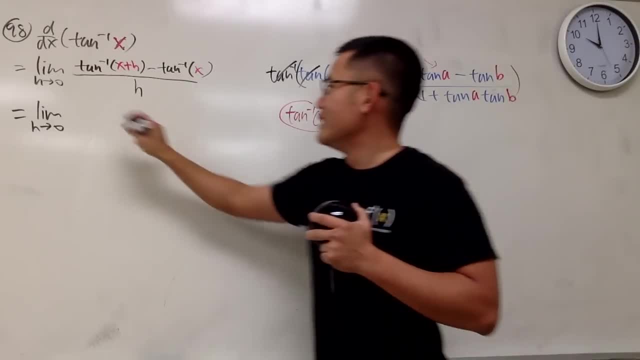 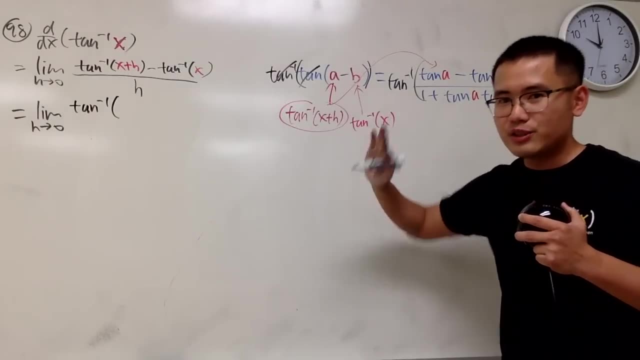 Don't forget, we still have the inverse tangent, but you'll know what we are going to do. Yes, That's later though. Inverse tangent, Tangent a. if a, is this of course tangent and inverse tangent. they cancel Namely, we just get x plus h. 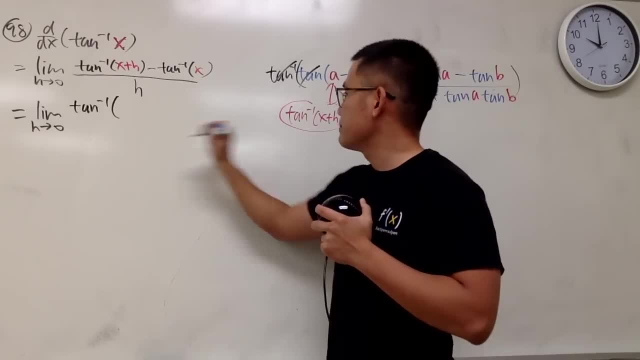 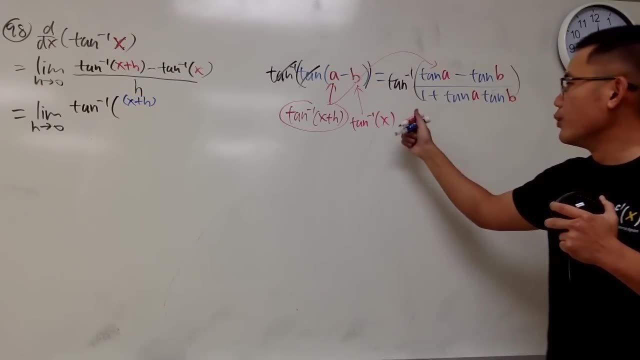 So on the top here we get x plus h- I'll put it down in blue: x plus h. And then we have the minus, and of course we put this right here for that. So we have minus, So we have minus, So we have minus. 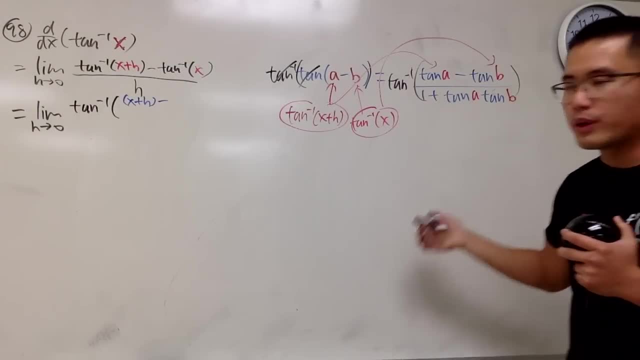 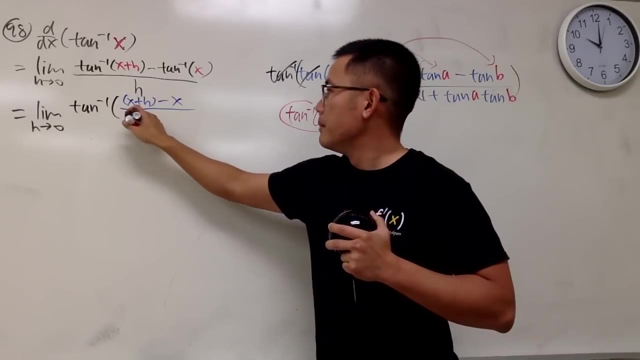 And this in here, tangent, inverse tangent- will cancel. We'll just have minus x over same thing, So it's just going to be 1 plus this right here will give us just x plus h And, lastly, this part will just give us x. 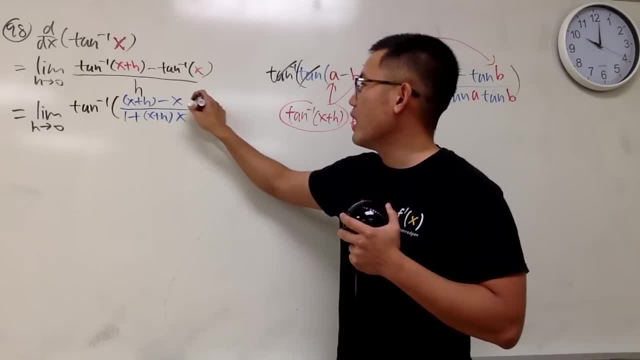 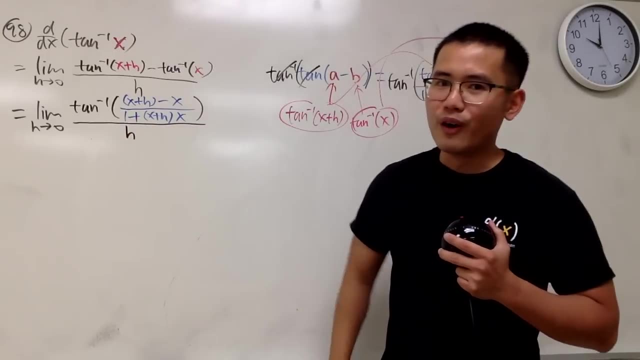 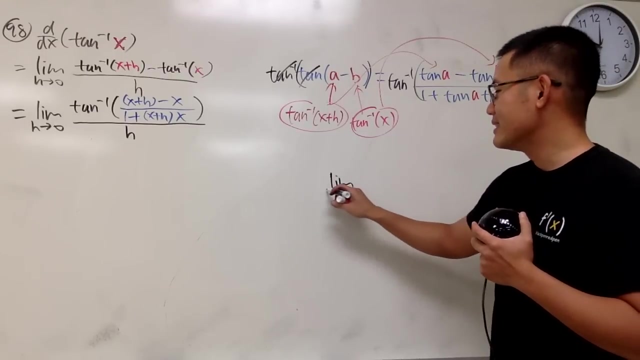 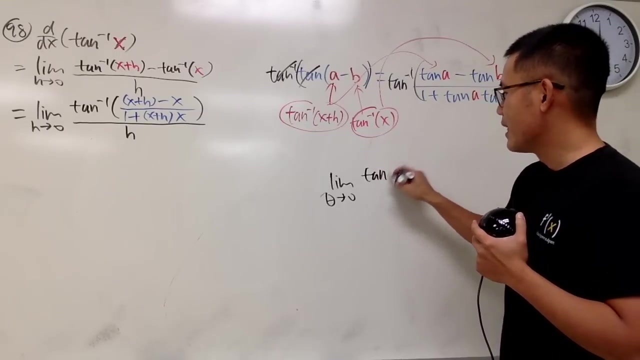 So that's the beauty, And I think you guys can see what is going on already, right, And this right here is all over h. This right here is all over h. Yes, I'll tell you The limit as angle theta goes to 0 of tangent theta over theta. 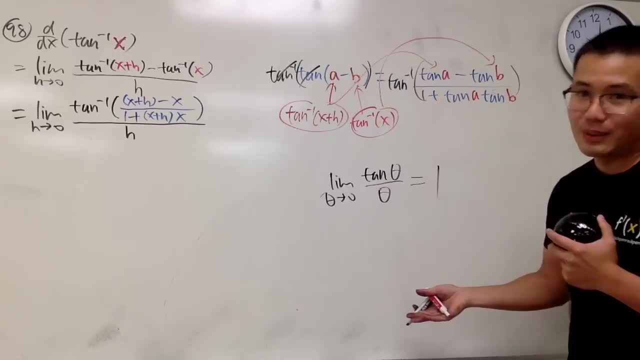 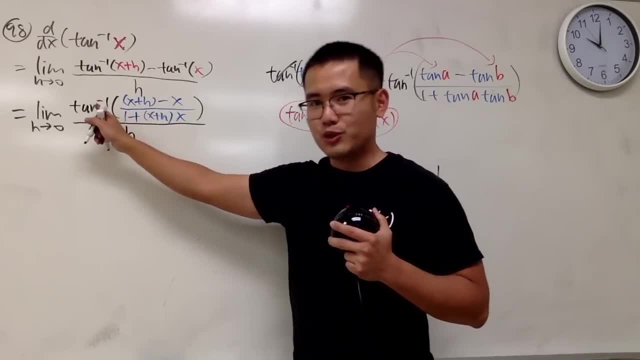 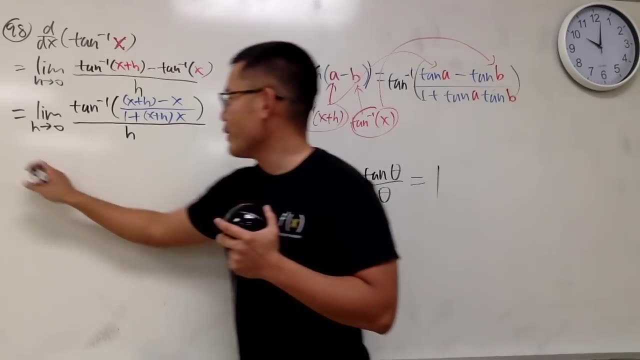 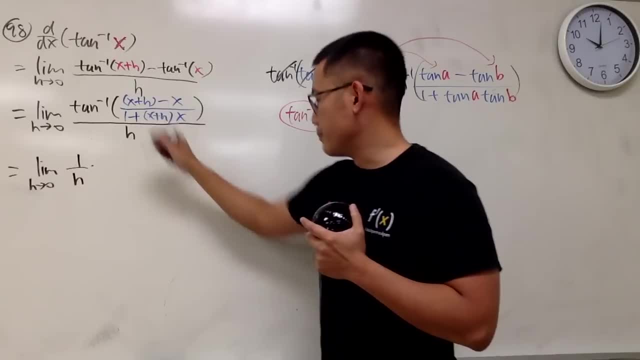 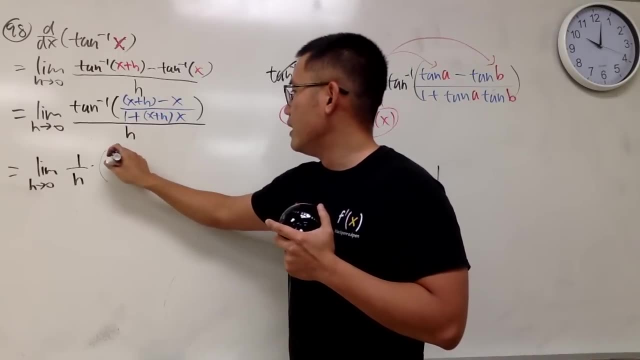 but perhaps let me just write the 1 over h, like this times the blue part right here. so no more inverse tangent because of this, right here. okay, So here we have x plus h. oh, you can just cancel them out, so we just have h, right here. 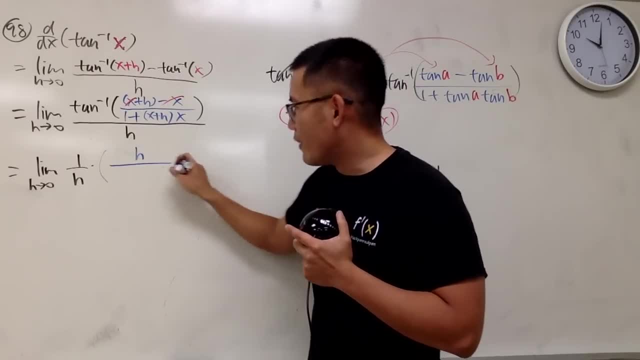 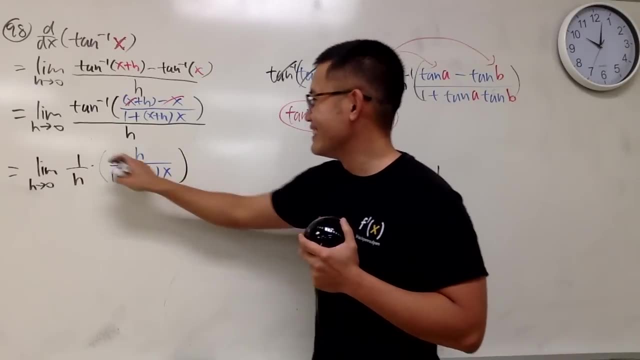 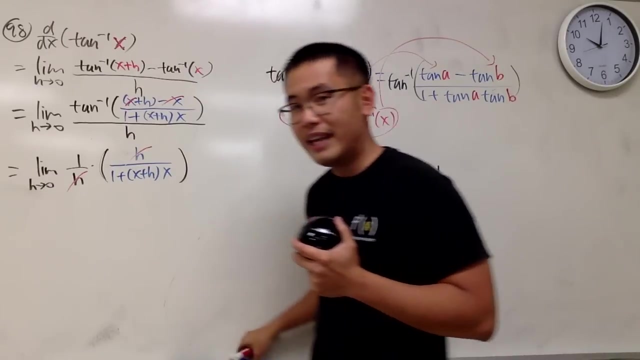 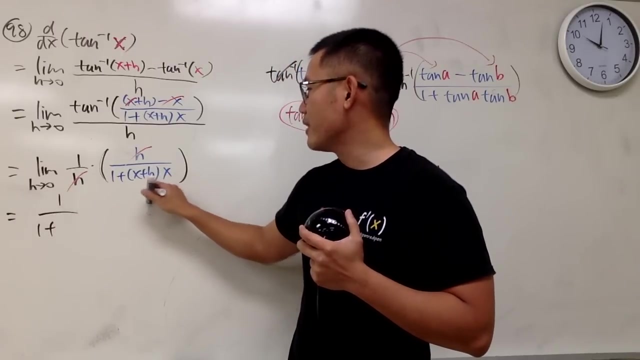 so just the blue part here, so just the h over 1, plus parentheses x, plus h times x, Yes, yes, h, h, cancel out, and then you put the 0 in here. So, ladies and gentlemen, in the end we get 1 over 1 plus this, right here. if you put 0 here, you just get 0,. 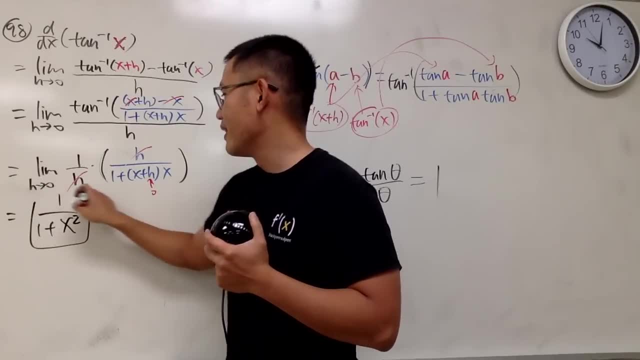 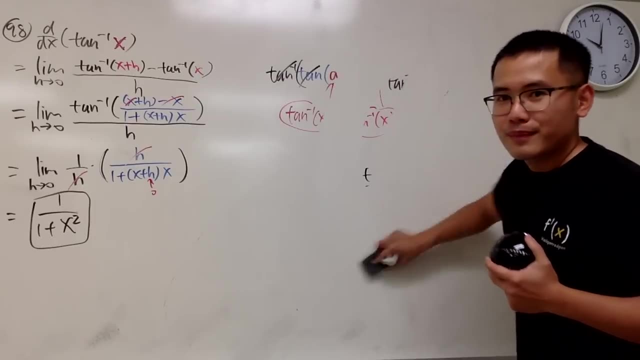 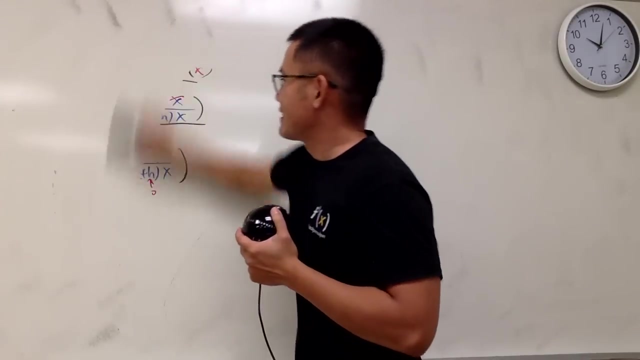 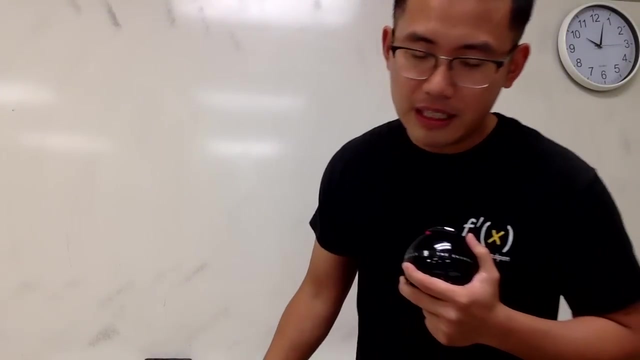 you just get x times 0.. the other x, you get x square. Well, much better, right? All right, Couple more questions and we'll be done. Of course you guys can see I haven't eaten anything yet, but yeah. 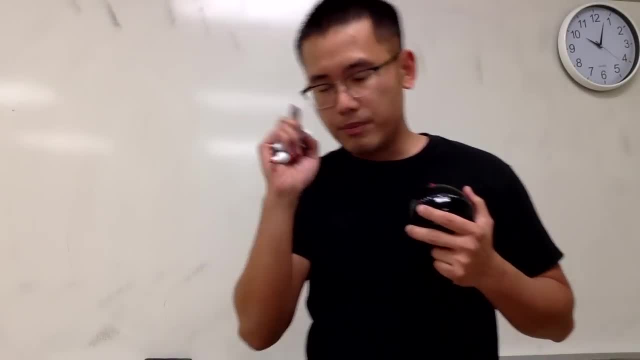 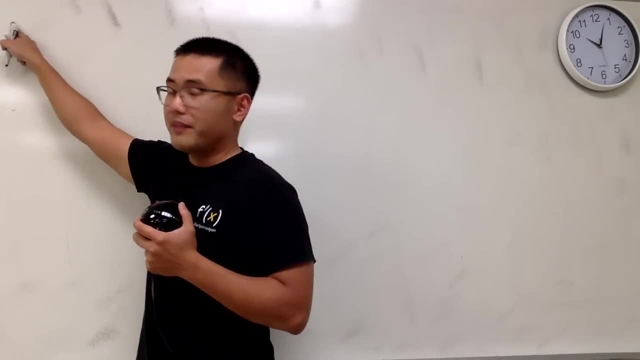 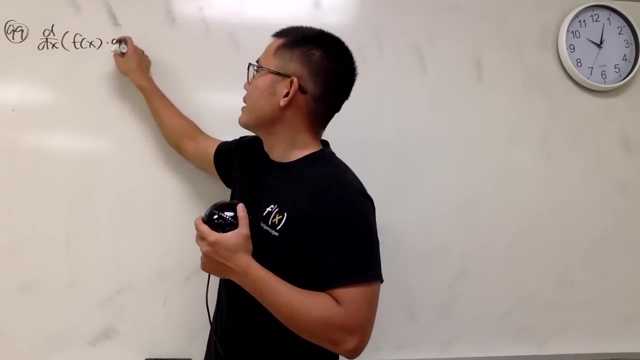 All right, so the last two. we are going to prove the product rule and also the quotient rule. So here we go. By definition, of course, 99.. d dx, just two: random generate like not random generating function. 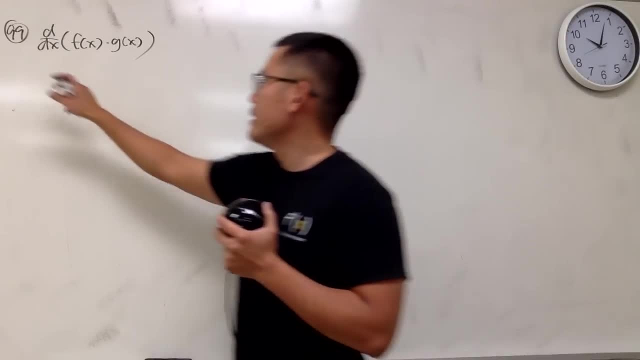 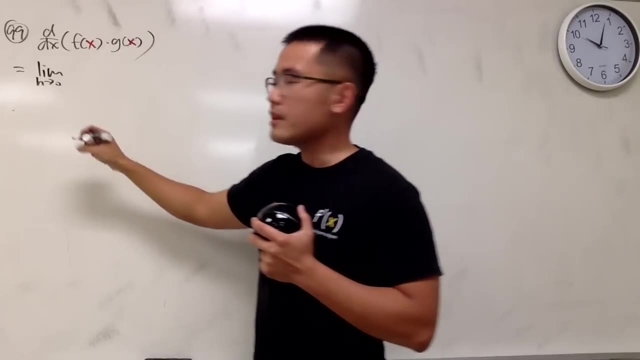 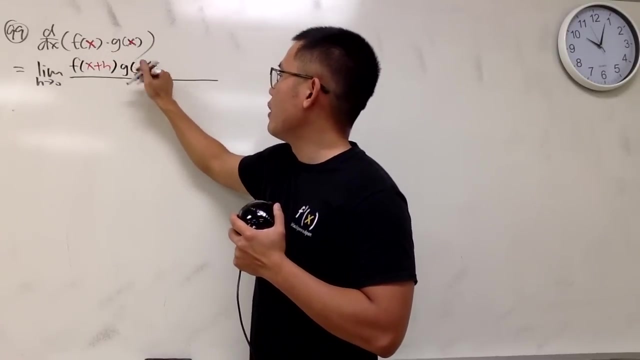 general functions. I have two general functions. I don't know what they are. Anyway, enough talking. here is the deal Limit as h approaching 0, this is x. They are the input. So first part, we have f of x plus h times g of x plus h, right. 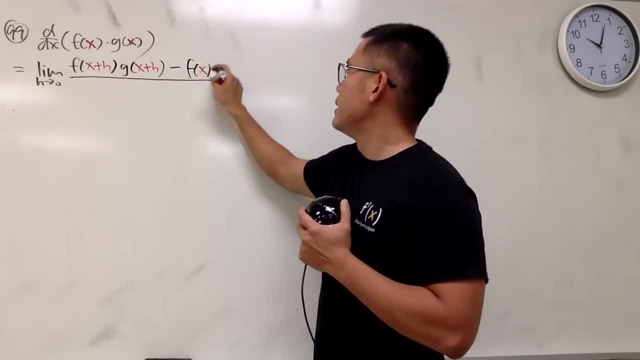 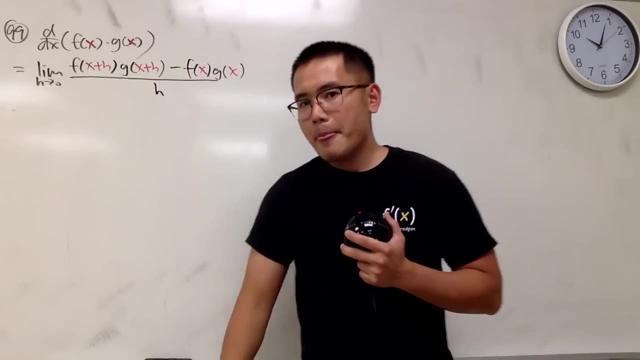 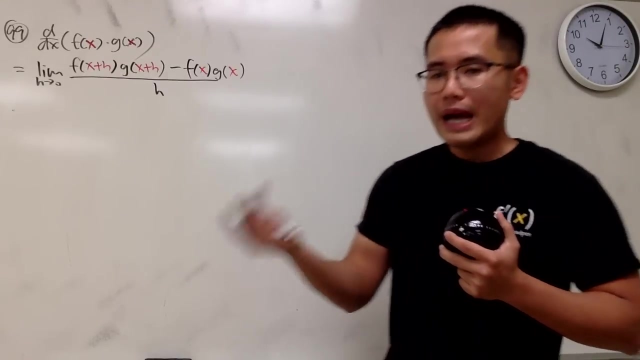 And then minus f of x, times g of x, all over h. Huh, how in the world can we prove this guy? Well, this is one of the example that you have to add something and then subtract something. Well, this is one of the example that you have to add something. 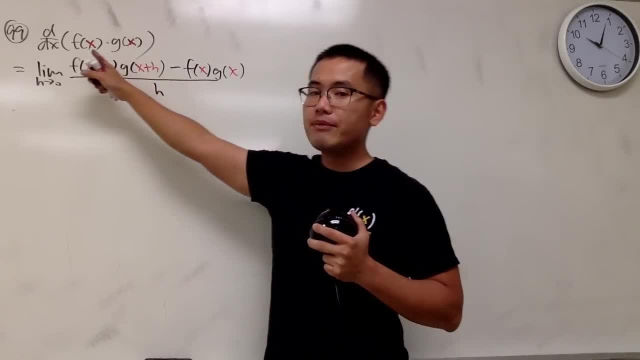 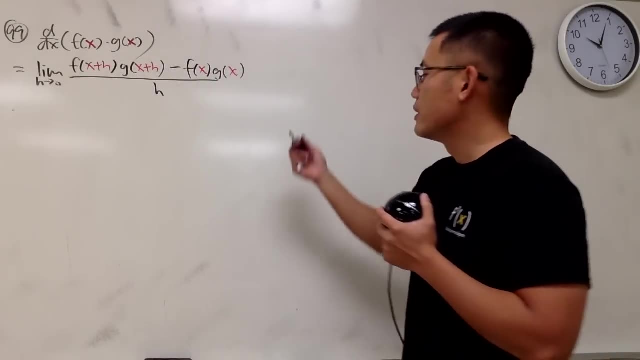 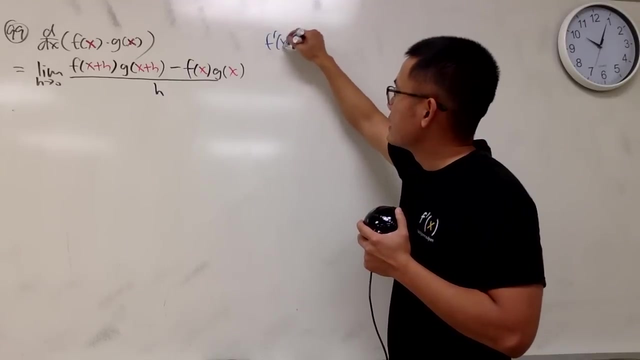 to make things work. Let me show you. Of course, we have to know the derivative of f and g, that they do have to exist. Remember what does it mean to have a derivative? The derivative, the definition of derivative. f. prime of x. 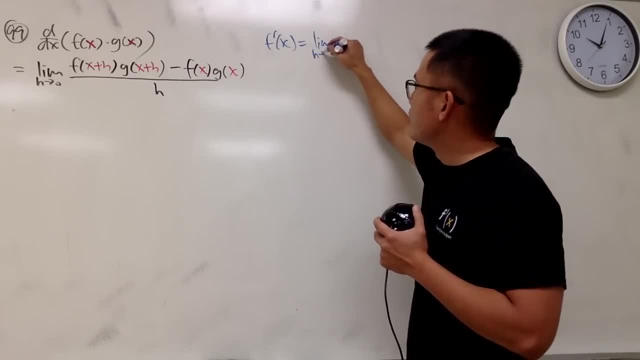 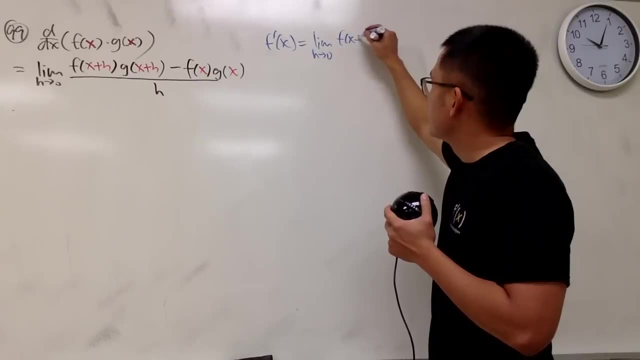 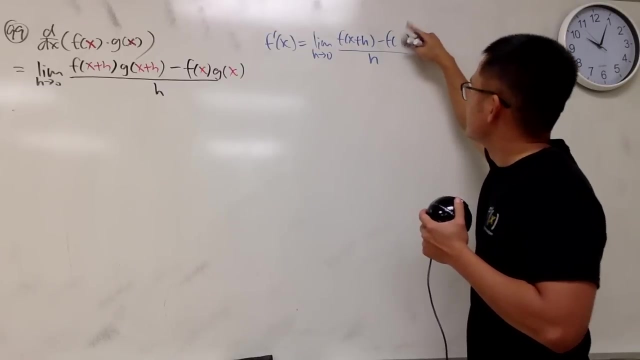 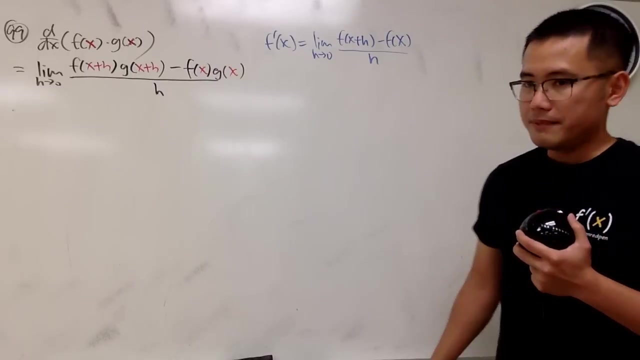 this right here is the limit as h approaching 0, f of x plus h, f of x plus h minus f of x all over h like that. yeah, That's the definition of f prime of x, And that's the one we have been doing already. 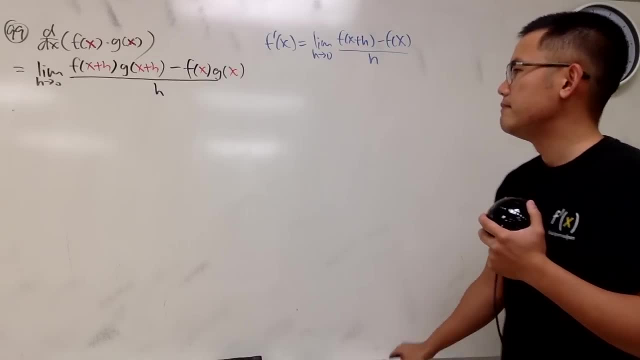 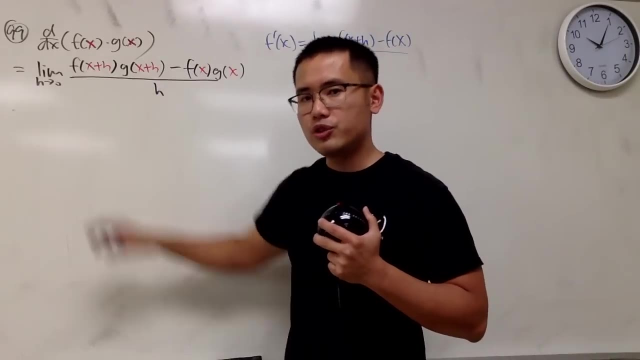 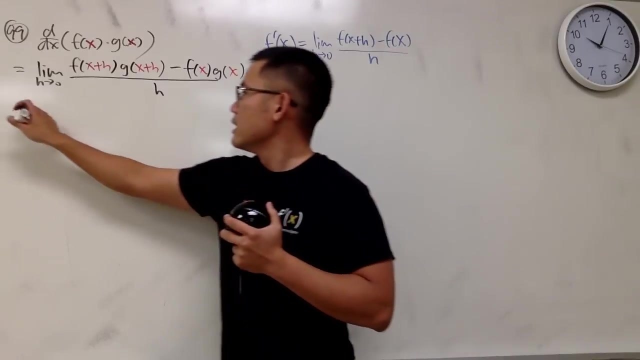 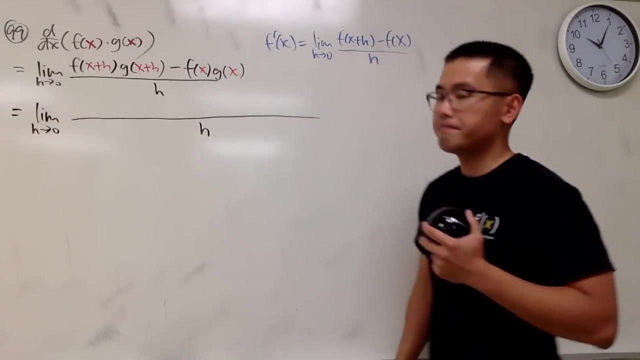 Well, I somehow see that we have the f of x plus h. Let's see if we can do the following to make this work out nicely. Well, not. This right here is the limit as x approaching 0.. We have the h right here. 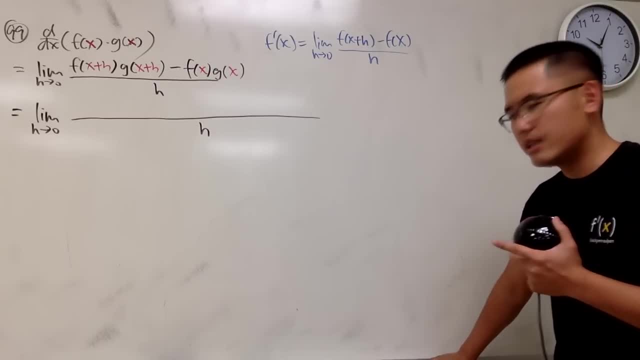 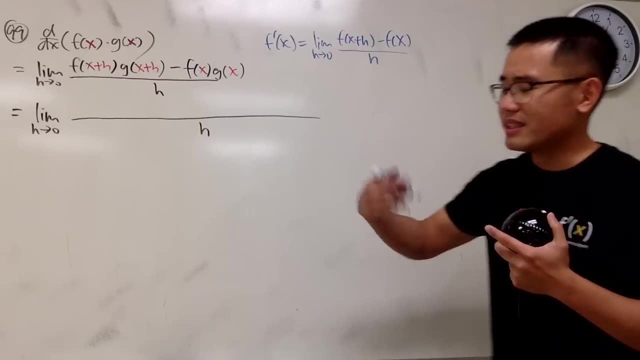 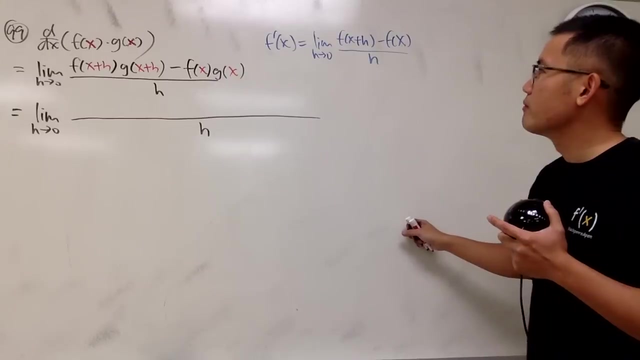 This right here. it's kind of similar to the idea when we're doing the derivative of sine. You want to kind of factor out the ones, the function part that doesn't have the h. This right here has the f of x, Hm. 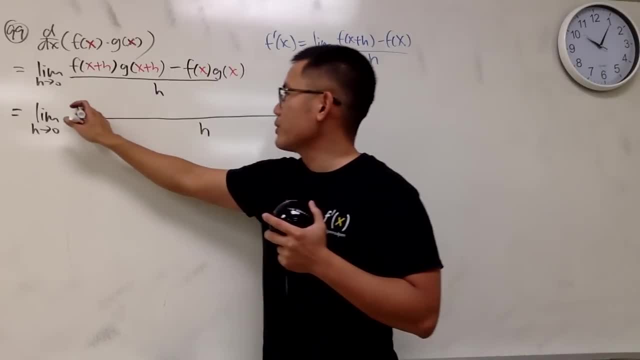 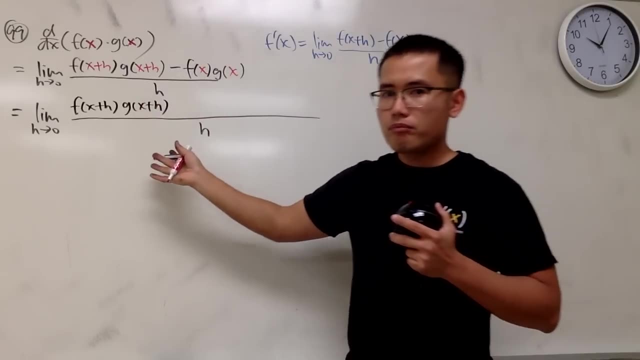 And I also want to have the f of x. I want to have the g to be involved. This is what we are going to do. Perhaps I will have f of x plus h times g of x plus h. okay, This right now looks pretty symmetric. 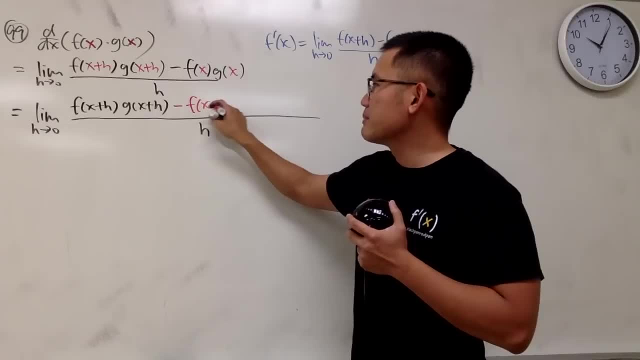 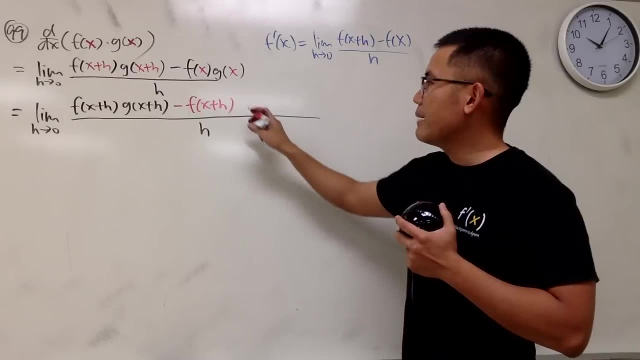 but what I would like to do is, perhaps let me minus f of x, plus h, And you see, when you do that, you can be able to factor this out. Well, in the meantime, though, I would like to just multiply by g of x. 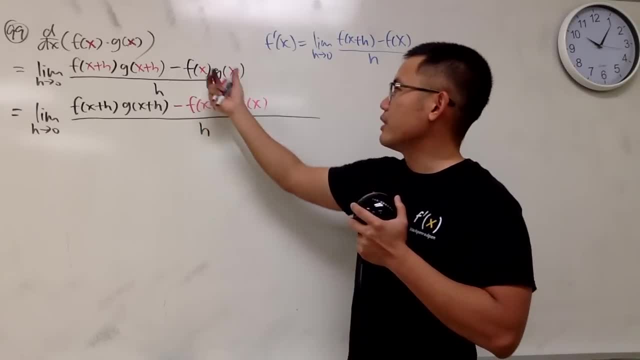 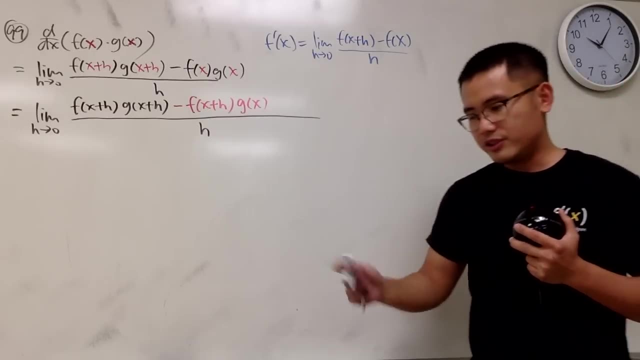 without the h, And the idea is kind of like you can just pick this with that, this with that, And there's also a geometric proof that you can check that out. You can check out Dr Pan's video for that, But it's been 6 hours and 20-something minutes. 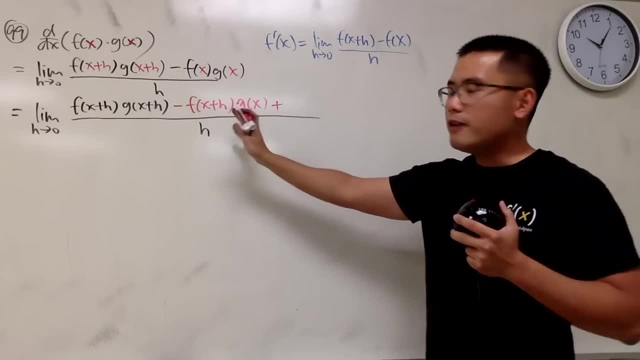 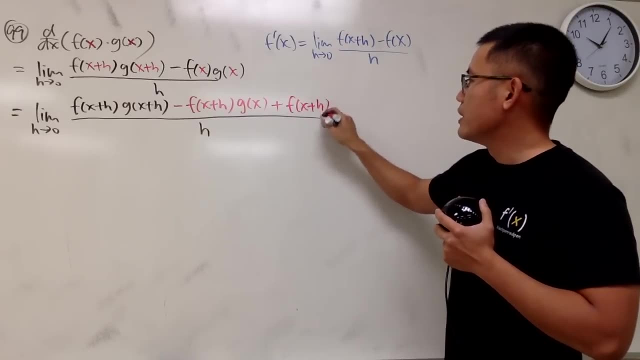 so let me just finish this so I can go home. Thank you, okay, Right here, you cannot just subtract something, You also have to add it back. So you add it with f of x plus h times g of x, So this is the equivalent than the original. 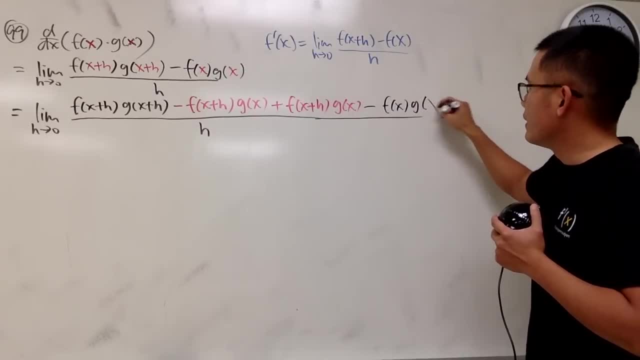 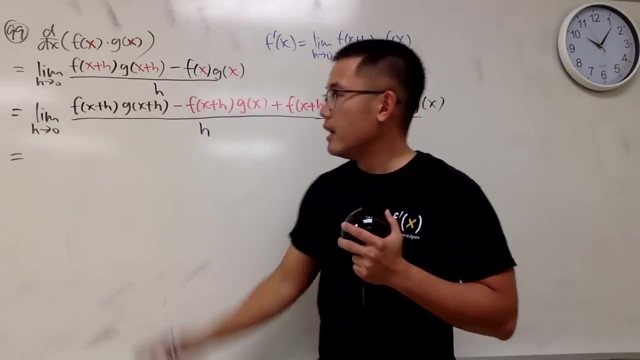 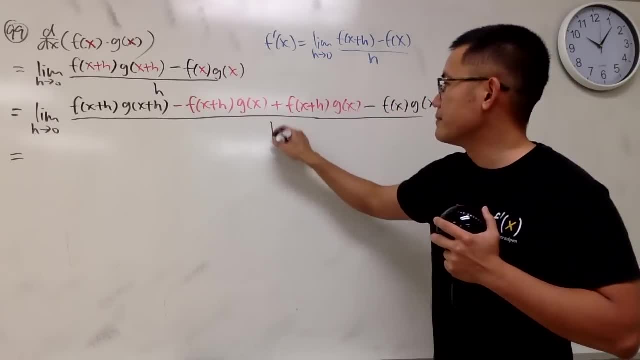 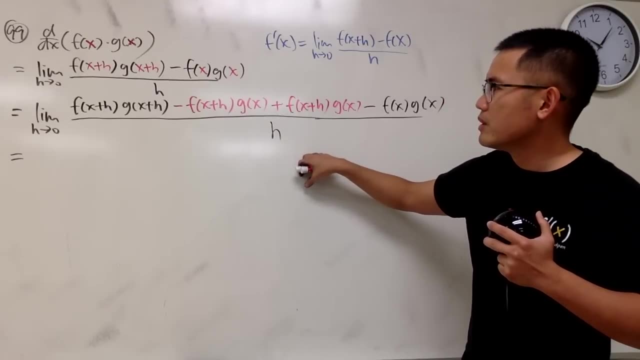 And keep in mind these guys. they all have the h in the denominator. So look at this guy with the h And is there anything that we can do? Well? well, let's see. Both of them have the f of x plus h. 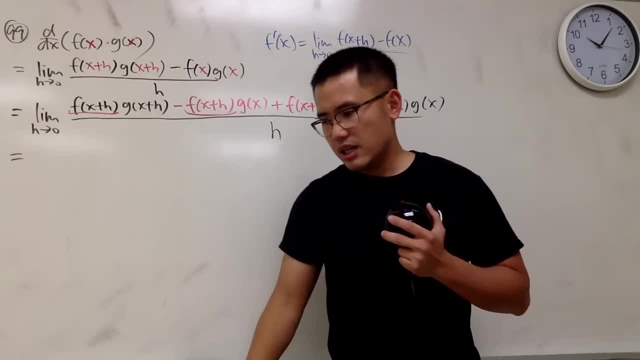 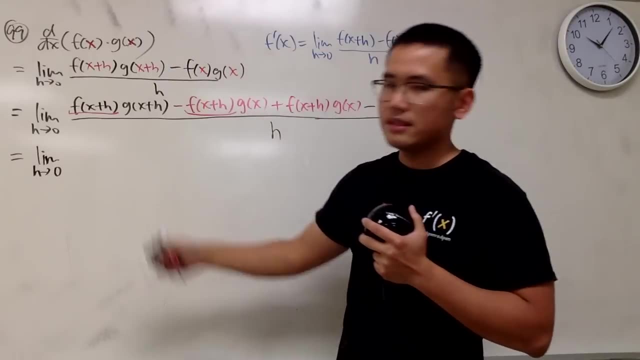 I'm going to factor it out, but I cannot take it out to the, to the limit, So I could just, you know, stick with it. The limit as h approaching the limit as h approaching 0.. Let me just factor this guy out, which is f of x plus h. 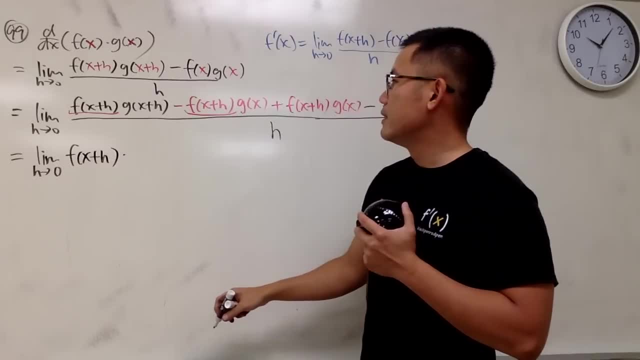 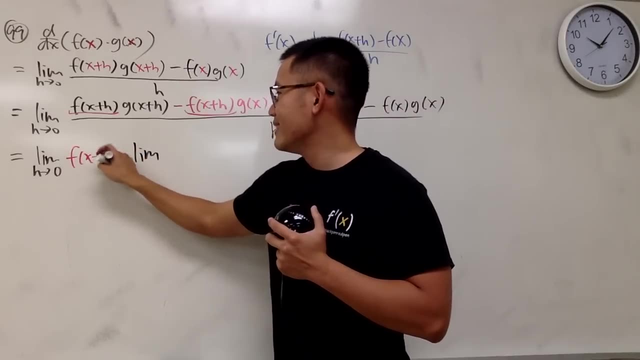 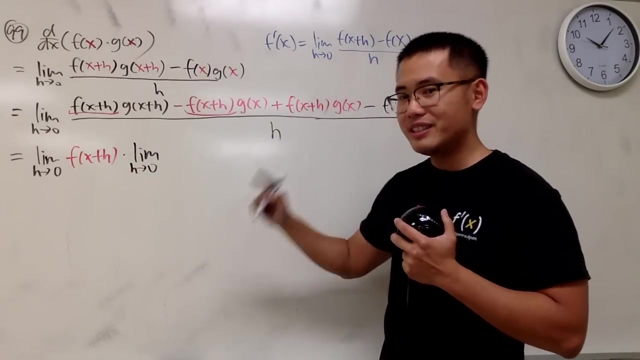 And that's it times the limit. Perhaps I'll put this down in red. I still care about the color, The limit as h approaching 0.. I will do this, minus that Over that, And you see, that will be the g prime if you just change over the f to g from here. 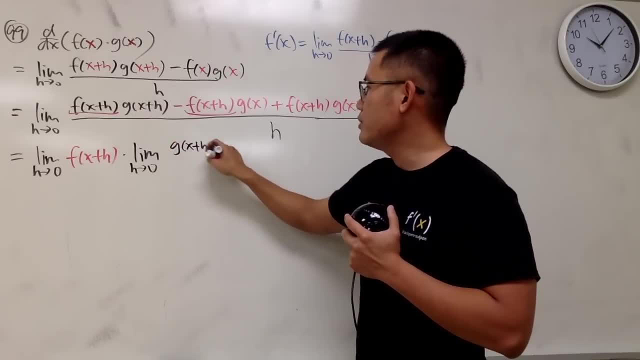 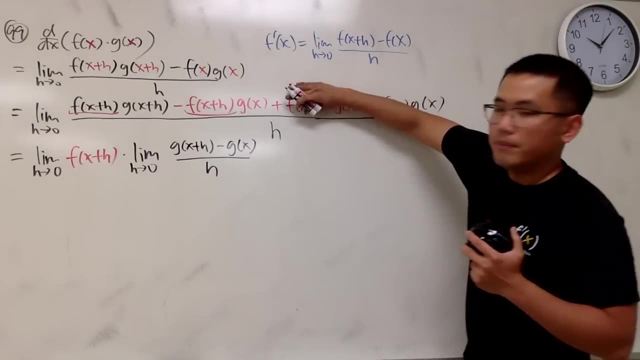 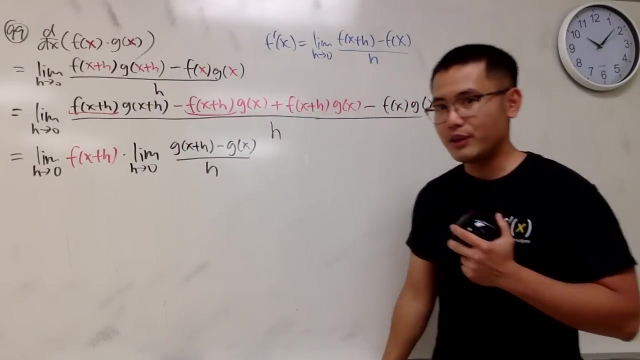 That's very nice. So let me put down g of x plus h minus g of x over h. So if you just ignore this part, just factor this out and then write this down. That's the first part. That's very good. 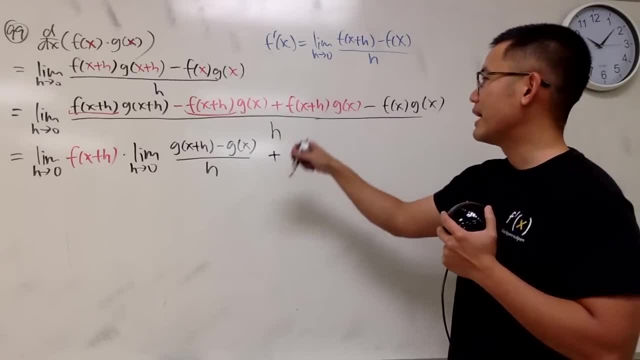 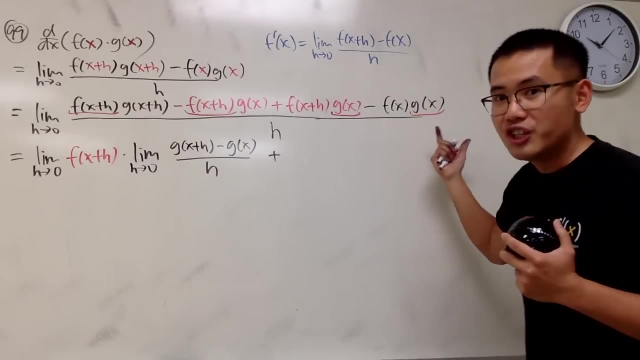 Now we add to do the same limit, But for this one we can factor out. Okay, We can factor out the g of x And this one right here. you don't have to do this because it's just g of x. 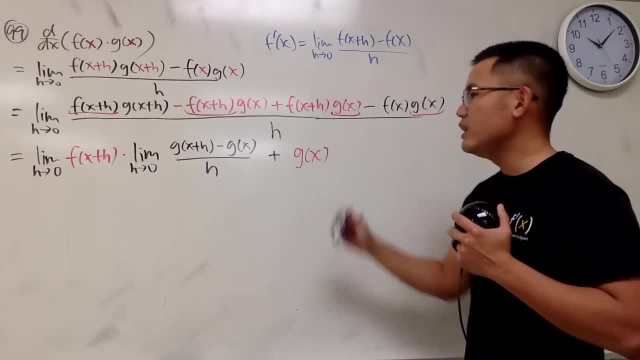 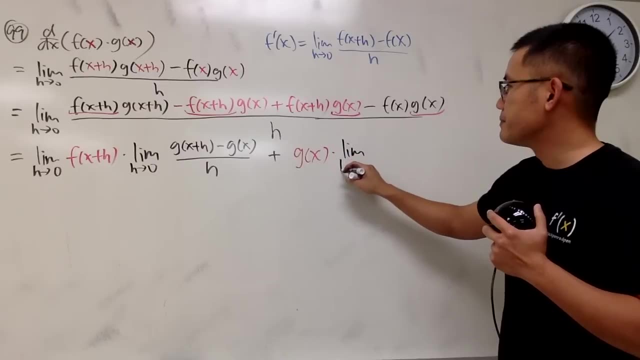 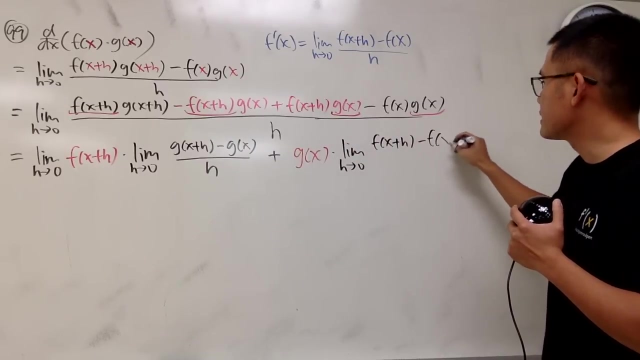 You can put it outside of the limit without any worry. And then the left over is exactly what we have right here. So we multiply by the limit as h approaching 0. And this minus that. so f of x plus h minus f of x all over h. 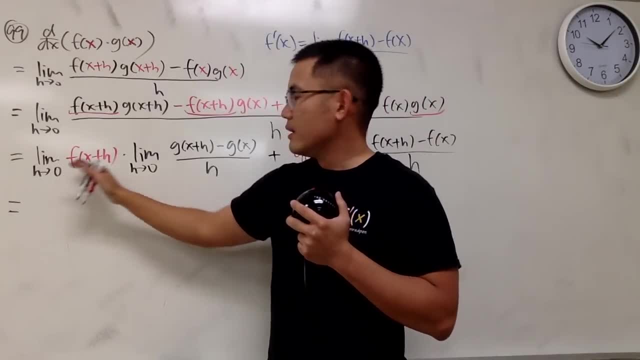 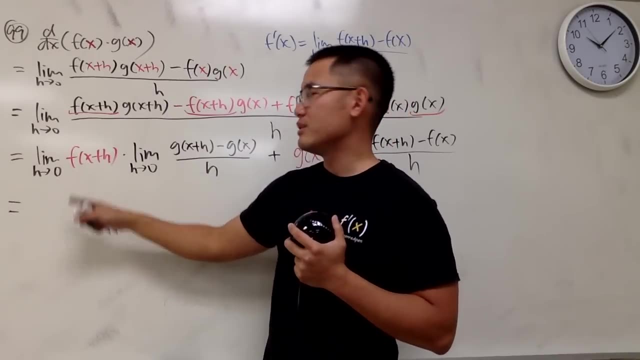 Now this right here. Okay, F has to be continuous, Otherwise you cannot have limits, right. So you can just put a 0 right here, nicely, and just f of x plus 0. It's just f of x, actually. 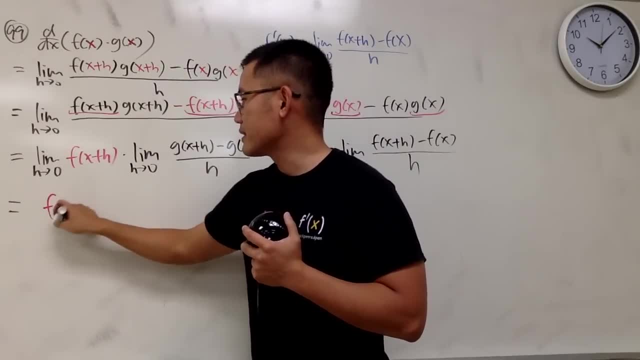 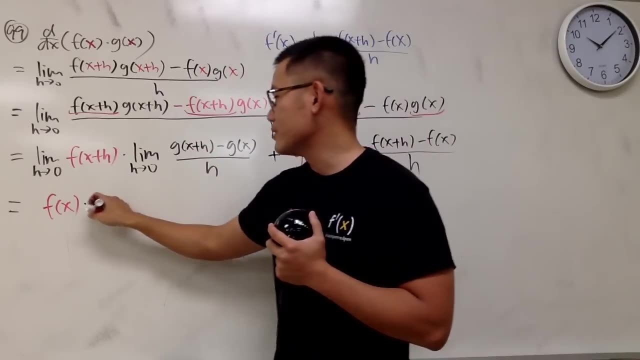 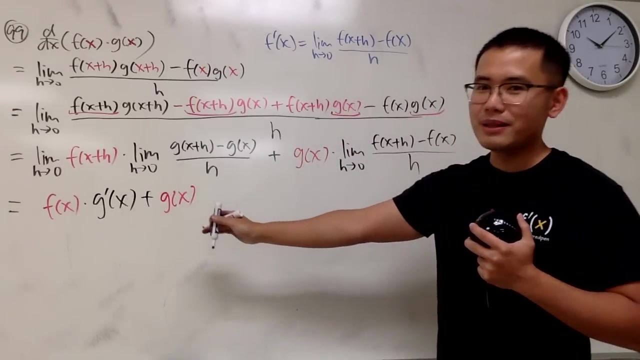 Yeah, so it's all good. This right here is just f of x, Namely the original function times. this right here is the definition of g prime, So it's just g prime of x- This right here, plus g prime of no. this right here is just g prime. 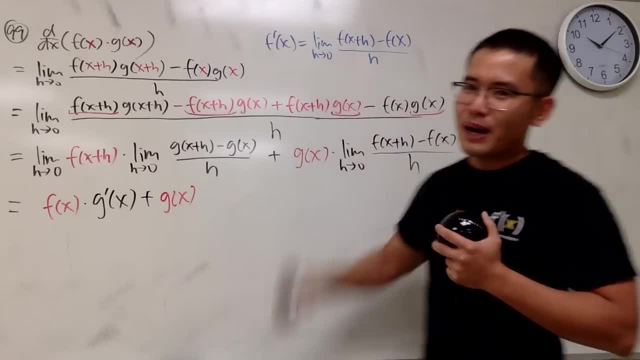 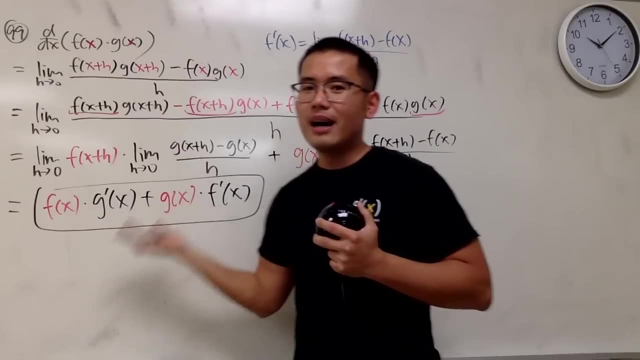 This, right here, is just g of x. This right here, you know, is f prime of x. So we multiply by f prime of x And guess what We are done, Ladies and gentlemen? the product, product rule, okay. 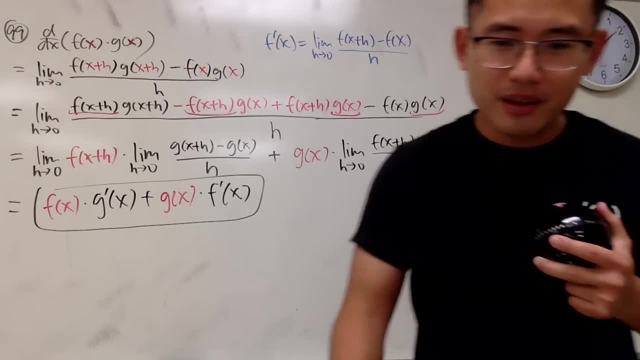 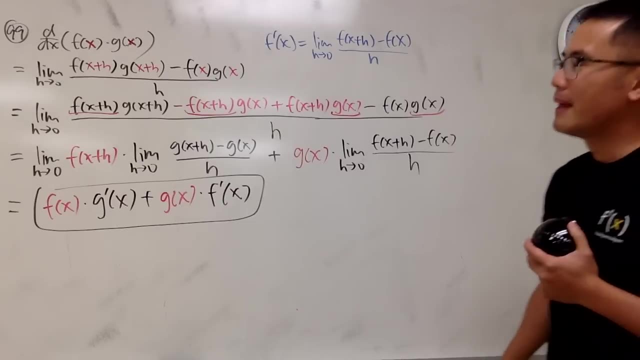 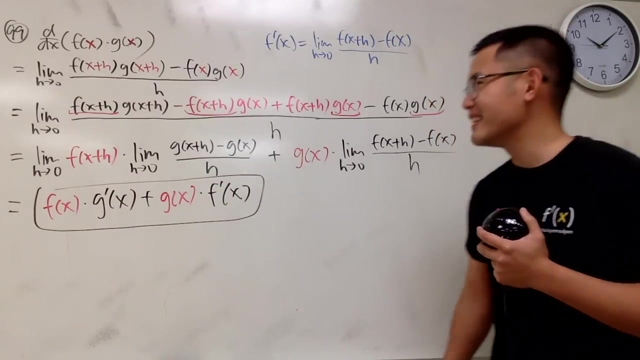 The product rule Man. I've been saying product rule for the whole video. I feel so bad now I am wondering if I should do the next one or not, which is the quotient rule. What should we just do it, Okay. 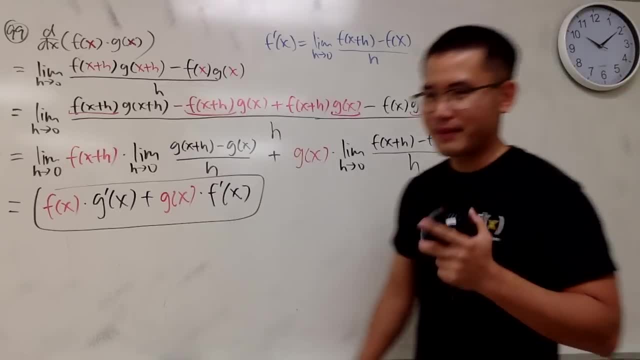 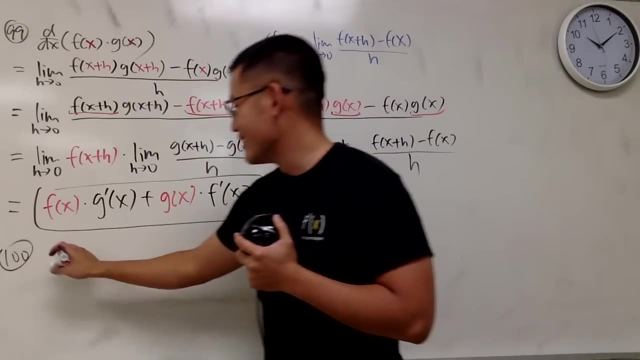 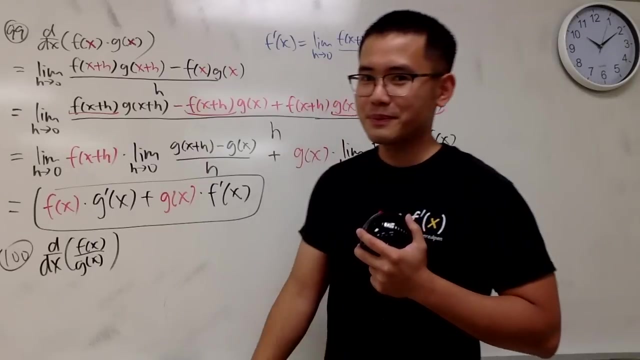 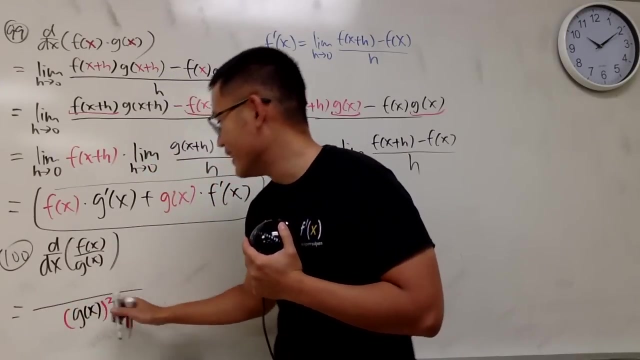 I will do this. I will do this. Okay, Number 100.. d, dx, f of x over g of x. You guys do it. This right here will be the bottom one squared and then the bottom one times d derivative of the top one, which is f prime of x. 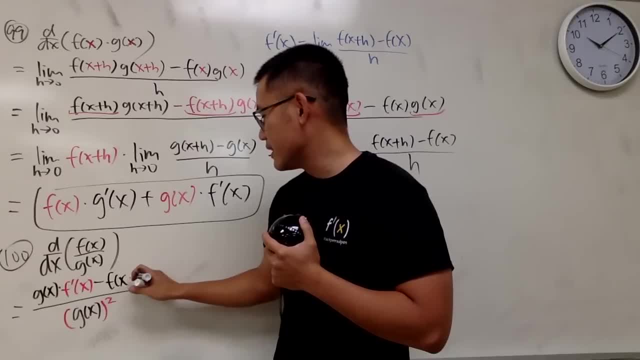 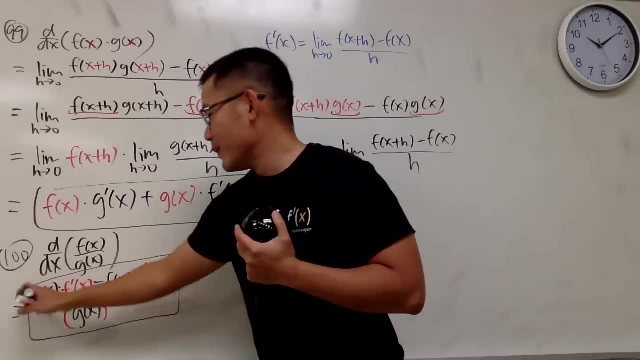 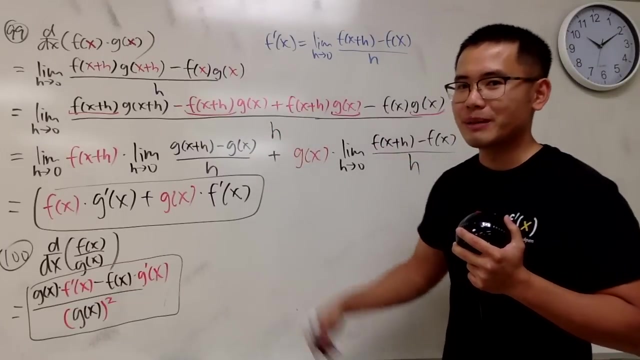 Okay, And then minus the top one, which is f of x times the derivative of the bottom one. This right here is it. Well, the hard part is you have to figure out what to add, what to subtract. And well, just study up. 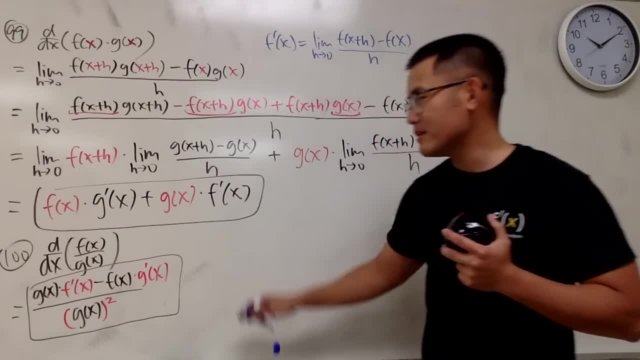 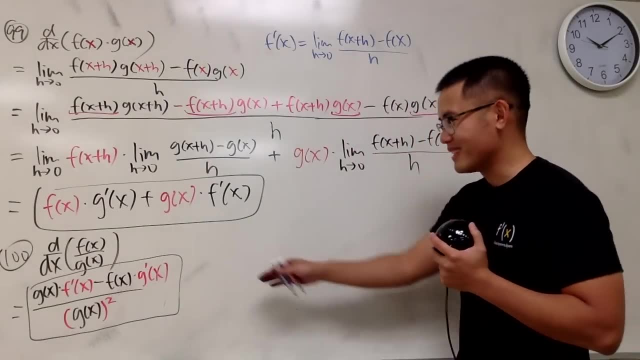 You guys can do it: Get a common denominator. Just multiply the top and bottom by the common denominator. You end up with a complex fraction. I hope you guys are not so mad because I am not doing that one. I don't know. 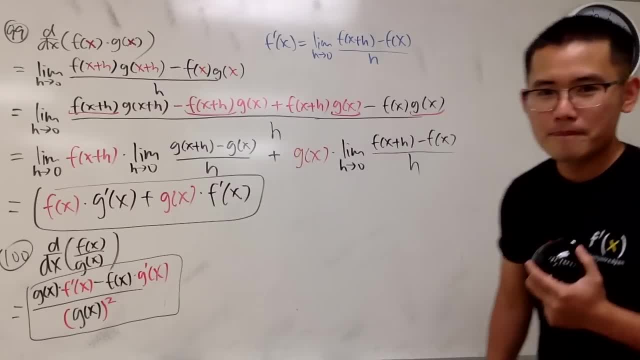 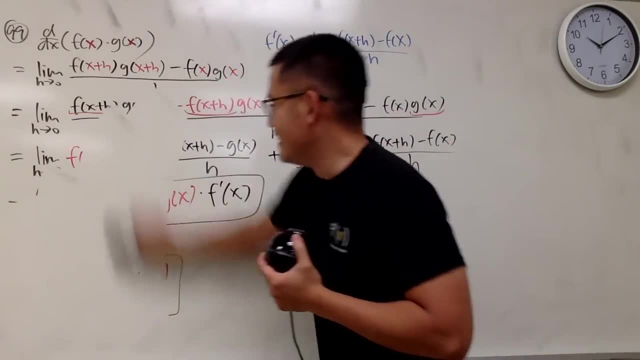 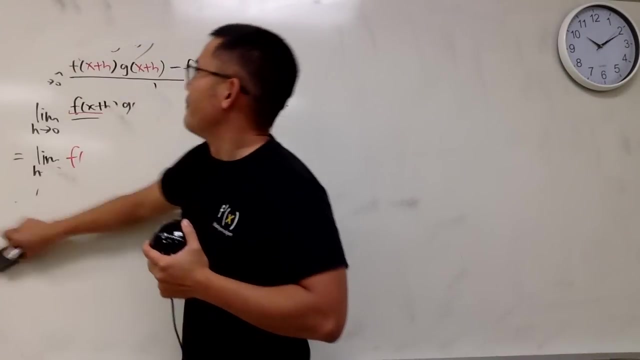 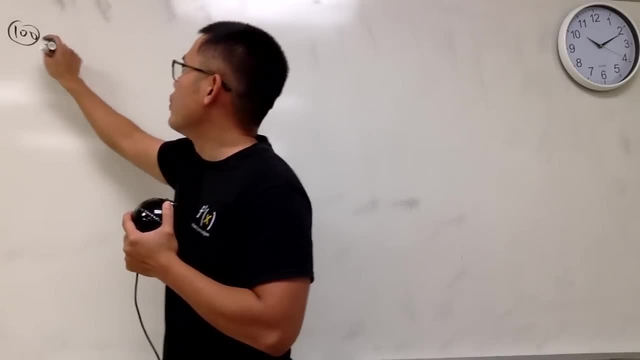 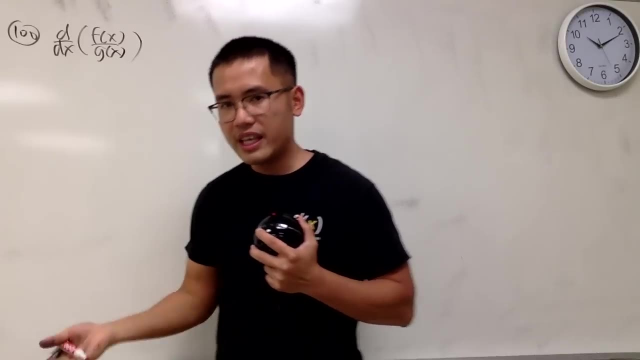 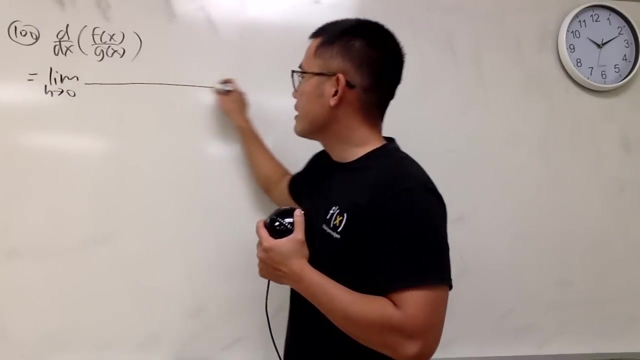 Right, here We are going to be proving the quotient rule d, dx, f of x, g of x And dividing. Here we go, Go ahead, Write down the limit as h approaching 0.. And on the top here we have f of you see, the input is x and x here. 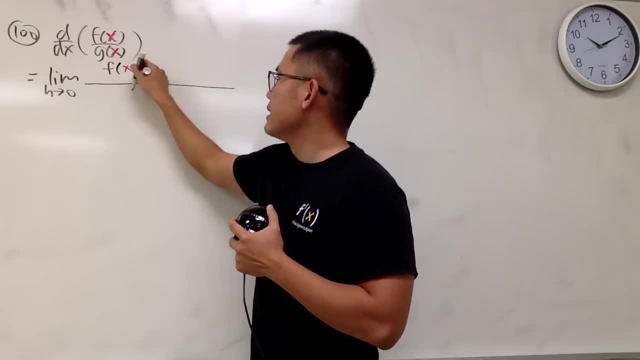 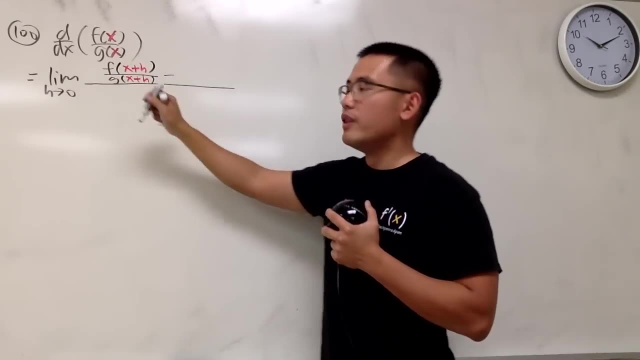 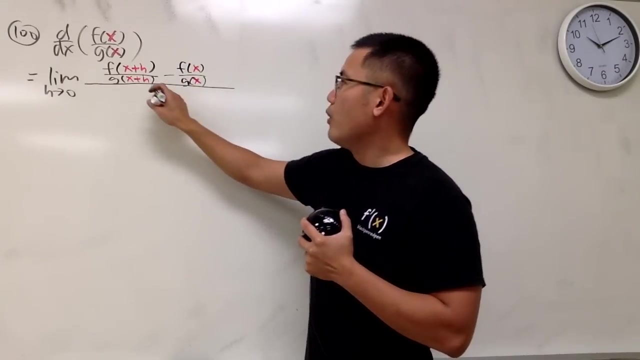 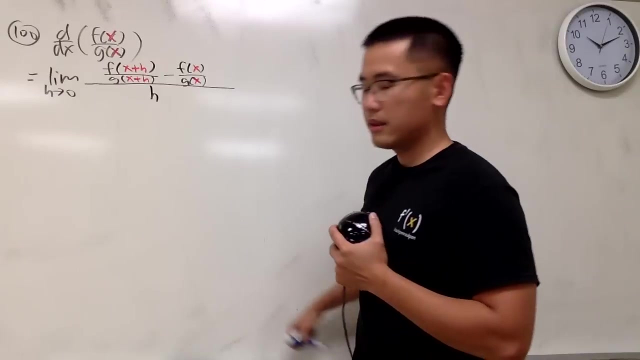 So that means we have f of x plus h over g of x plus h And then minus the original, namely f of x over g of x or over h, like that. Well, well, Let's just multiply, Let's just fix the what's that called the complex fraction situation first. 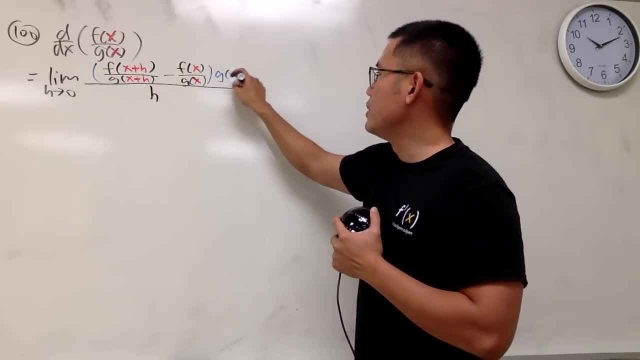 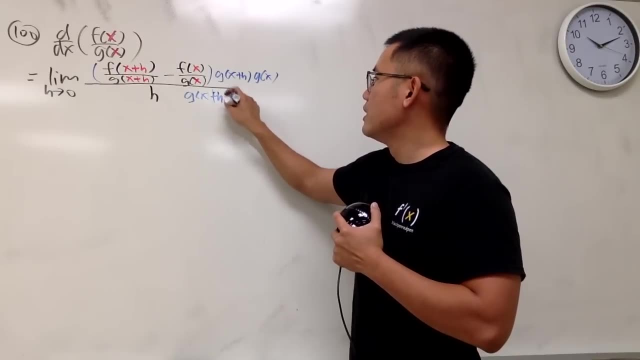 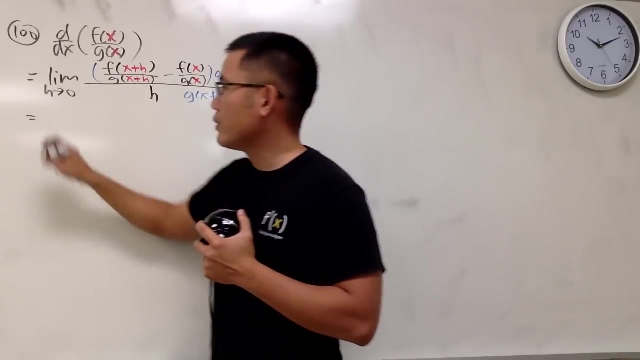 So multiply the top and bottom by the denominator, which is g of x plus h, g of x and g of x, So you guys can see this is rather similar to the secant right. So that's why I've been putting down, organizing all the worksheets right here. 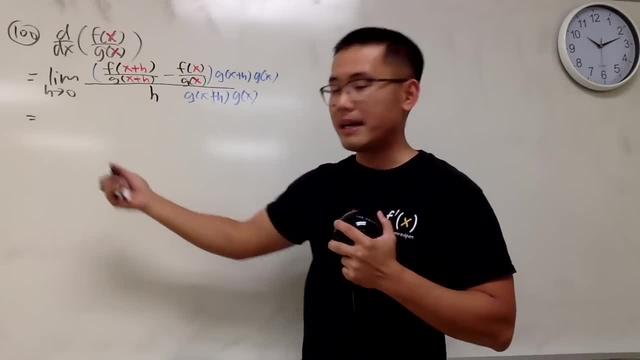 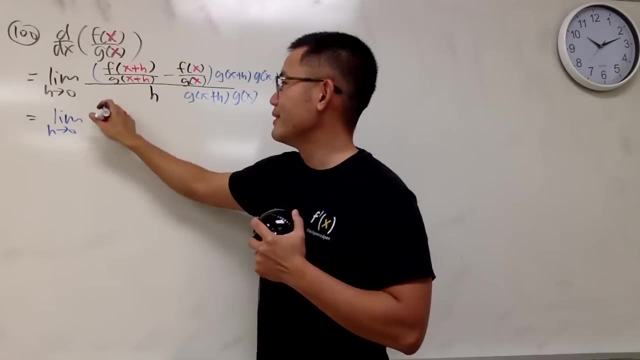 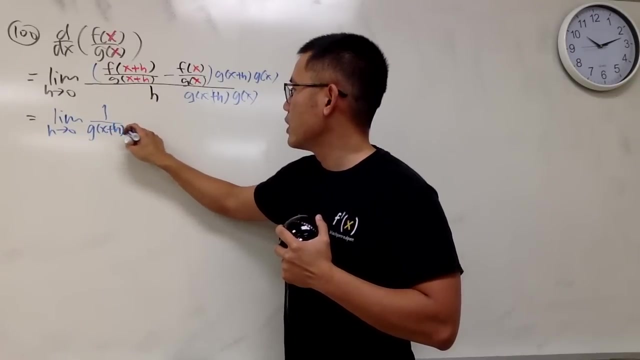 So this time I'm going to just put that as a limit by itself for the denominator right here, because you guys have seen the secant situation right, hopefully. So one over this and that. okay, just the blue portion g of x like this: 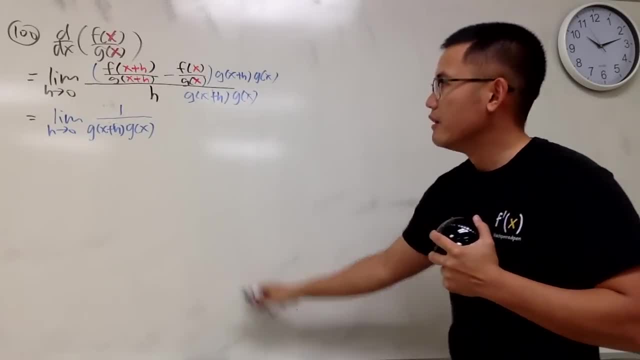 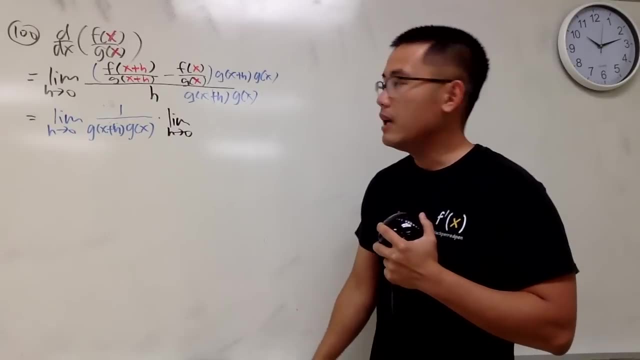 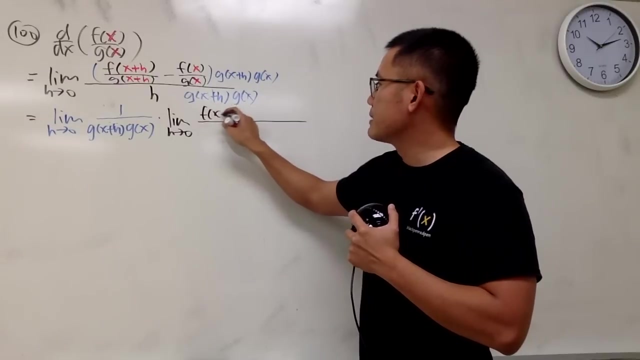 One over. all right. Now for the part for the left over. this is the limit as h approaching 0.. Okay, when you multiply this and that, this and that will cancel. so you have this following: F of x plus g of x. 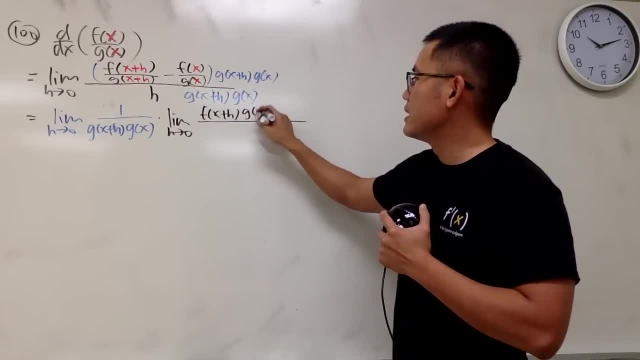 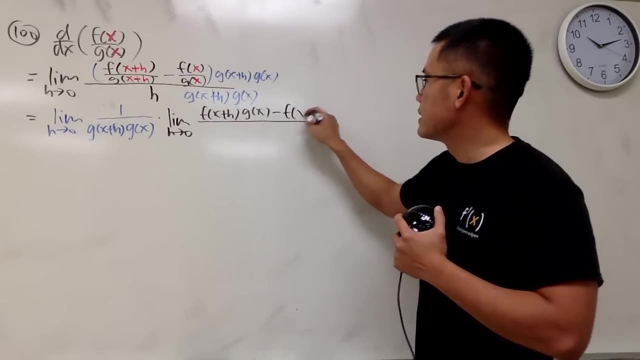 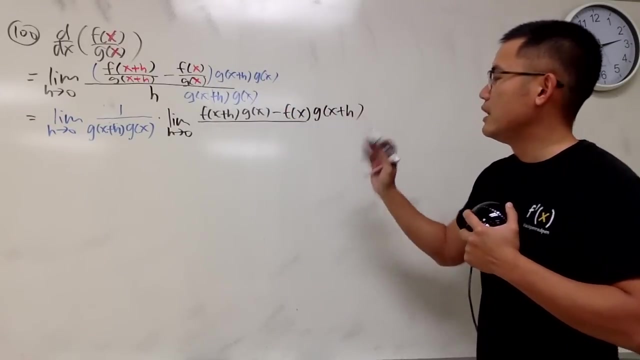 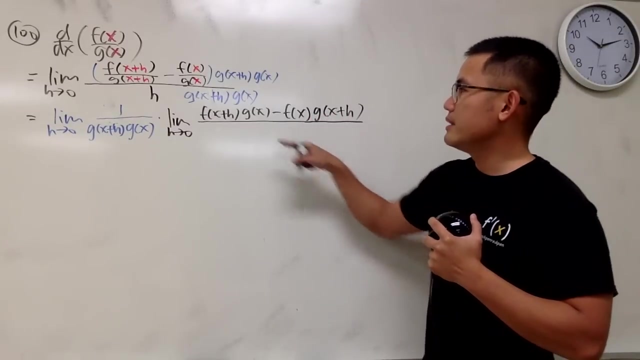 F plus h times g of x. yeah, this times that and then minus f of x and times this, which is g of x plus h, like this: Let's see if this is correct. It is correct And all over h right. 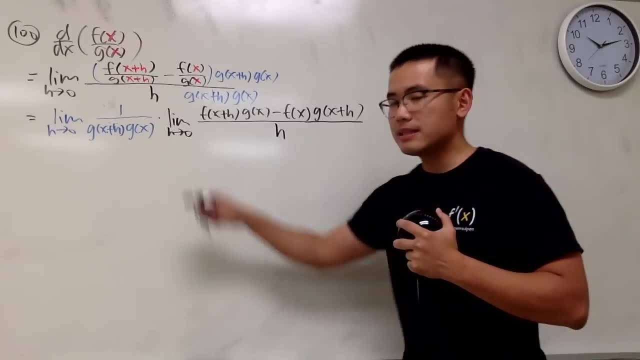 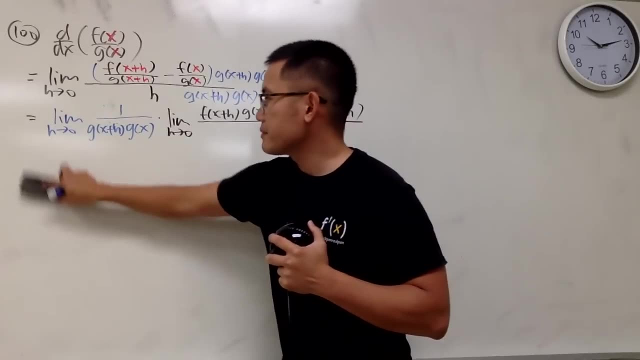 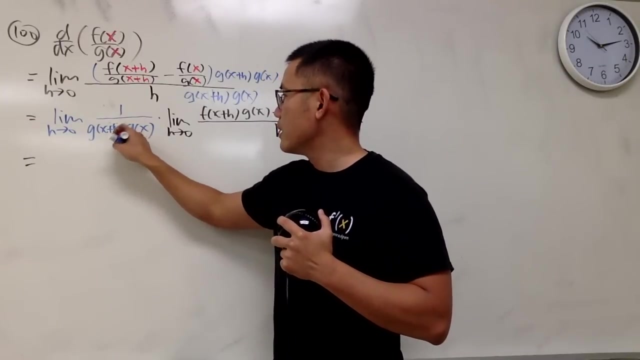 So that's the one that we have, And now perhaps that's, Let's take care of this part first. Right here you can see that if we put 0 into h, what do we get? This will give us 0 here. 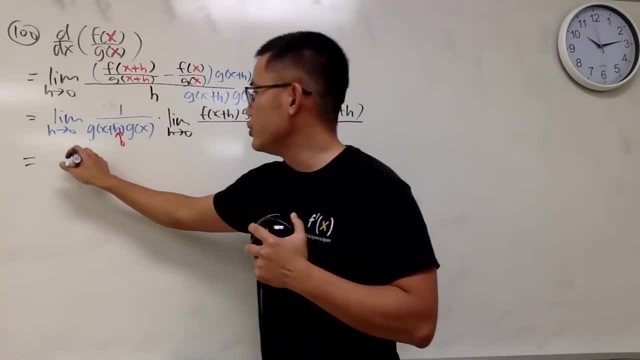 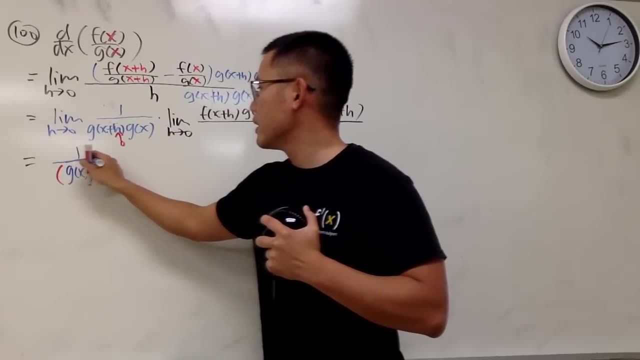 So we end up with g of x times g of x, namely we get 1 over g squared, namely the bottom one, and you square right. So that's that part, And now for this one. Of course you know what's coming. 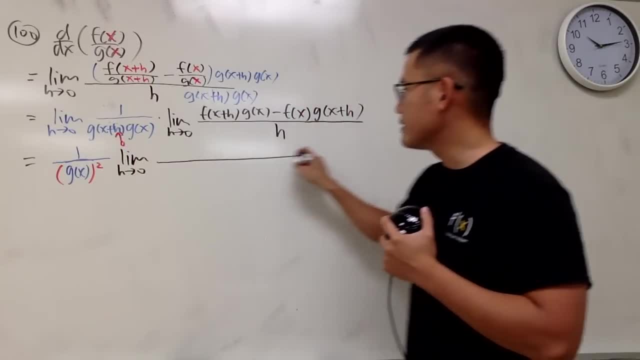 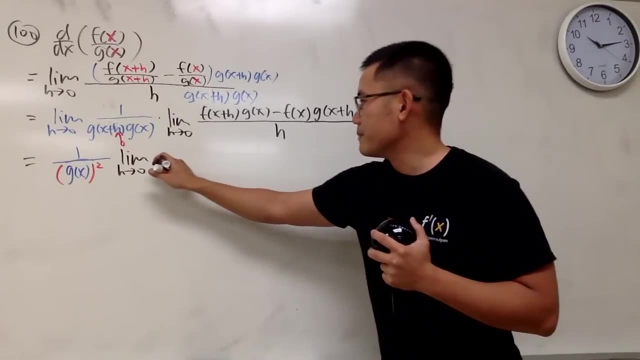 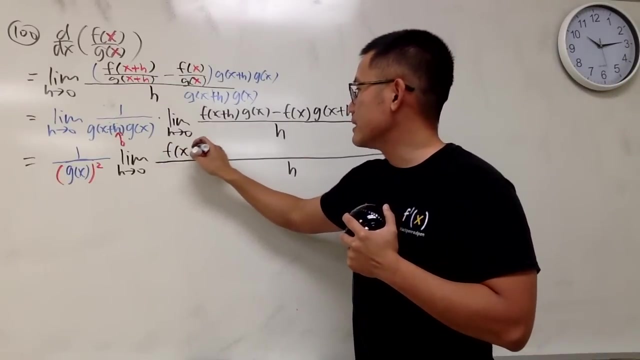 You are going to take the limit as h approaching 0, and you are going to find something to add and find something to subtract. The same thing to subtract. Okay, so h right here. hopefully this should be enough space, This right here. f of x plus h and g of x, right. 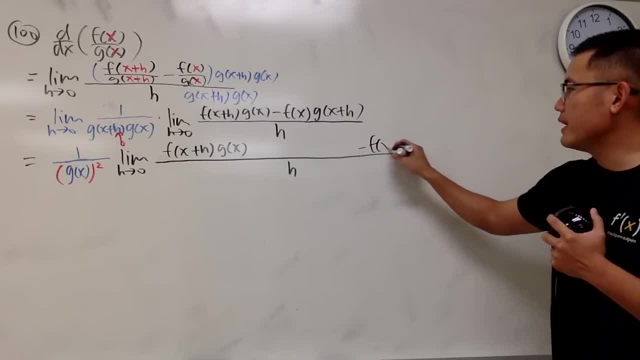 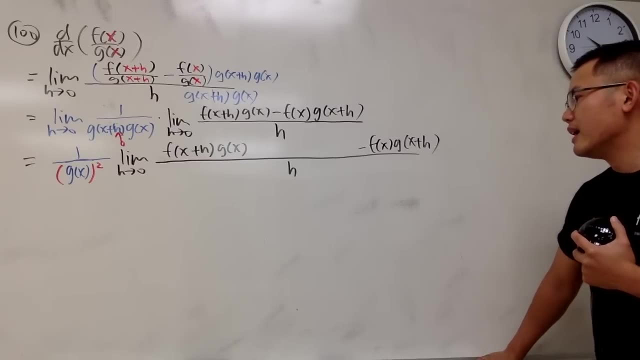 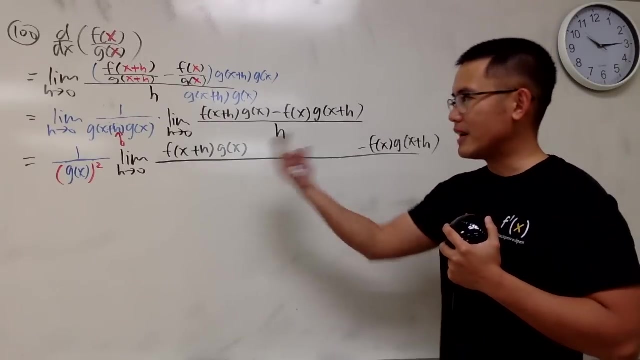 And this right here is minus f of x, g of x. Right, Okay, So f of x plus h. Yeah, Now I want to have the derivative come up to help us out, right? So remember, you should be able to factor things out, and all that. 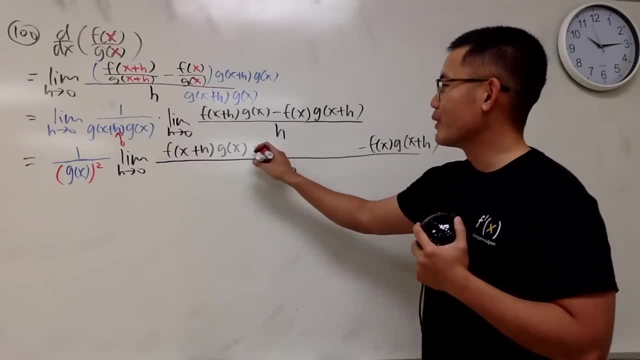 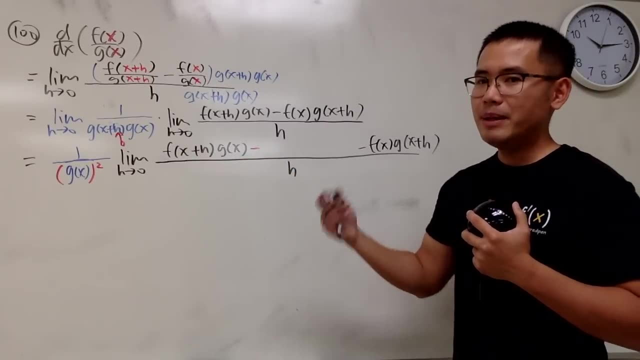 Hmm, What should we do Here? we are going to minus. You may want to try to factor out the g of x first, So I want the g of x. In the meantime, if you want to have the derivative form, you want to have f of x plus h minus. 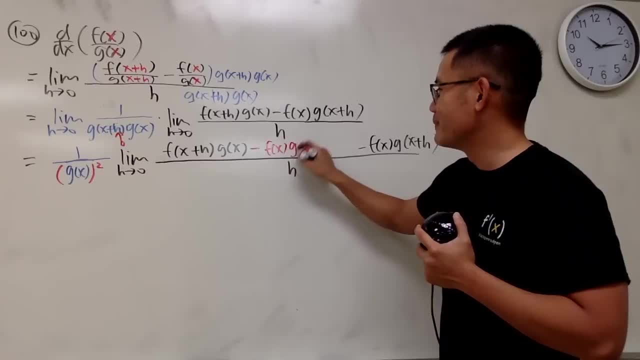 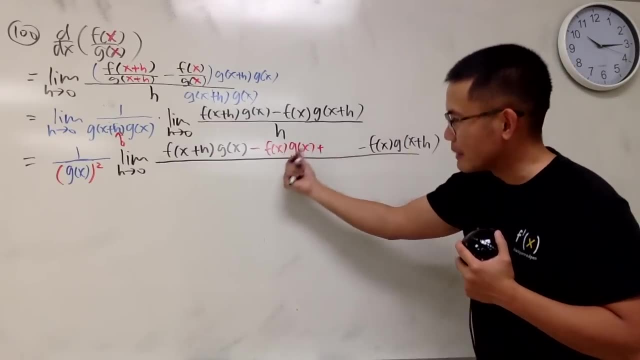 f of x Times g of x. So this way you can factor the g of x, Don't just add, Don't forget to, I mean, don't just subtract, Don't forget to add it back. So f of x, g of x. 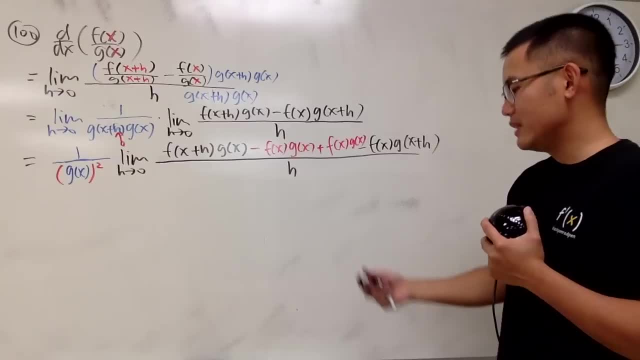 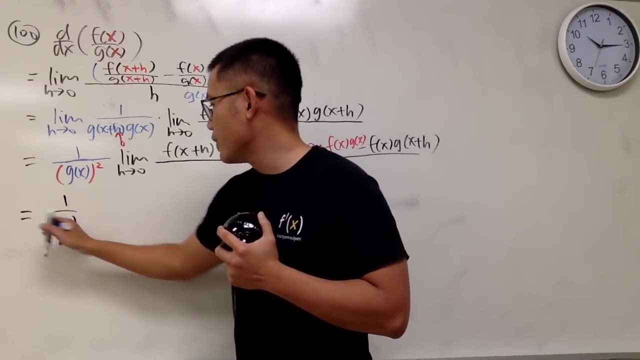 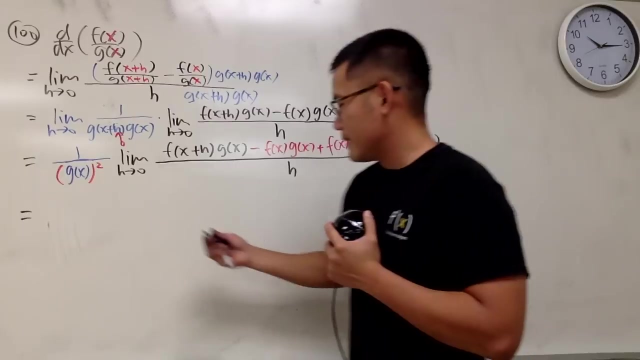 This is what you have to do Now. it's just how we write it down nicely. This right here is 1 over g of x, And we are going to square that, So perhaps I should still keep this in mind. I should keep this in blue, why not? 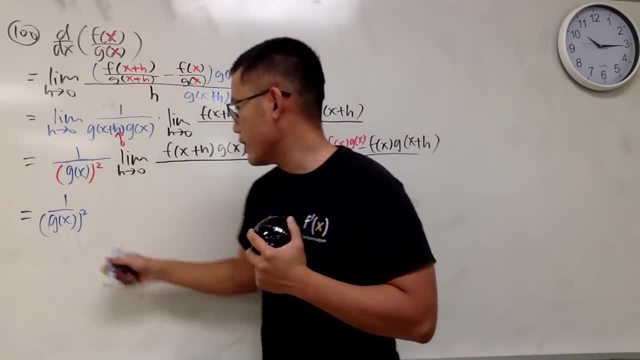 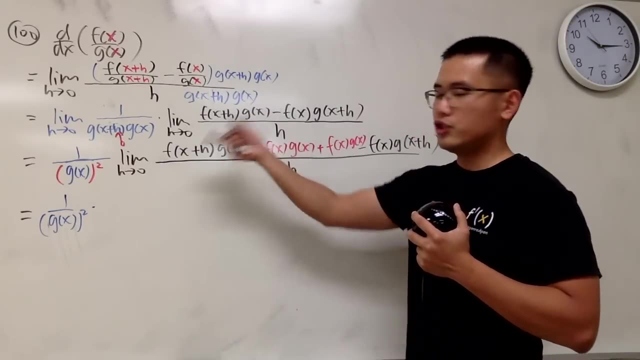 1 over g of x squared. Okay, So we'll do this, Not in our head, but I'll just write it down. I will factor out the g of x. All right, So this is the parentheses. We factor out the g of x. 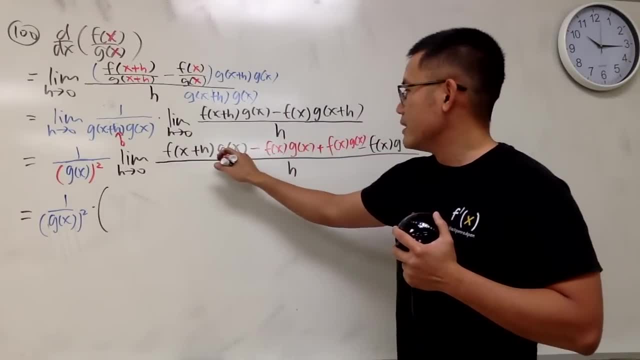 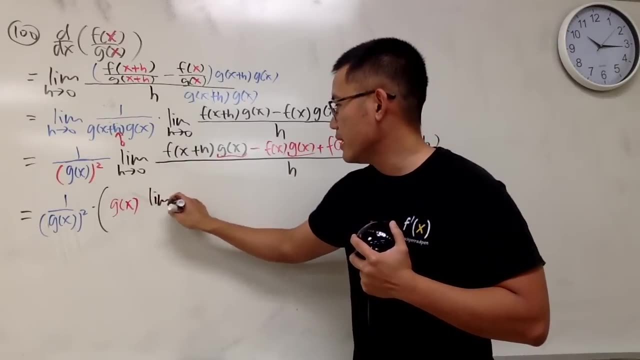 Let's just write it in red man. This times that Write it down, It's g of x. Take the limit of the remaining, which is the limit as h minus f of x, plus h minus f of x Approaching zero. 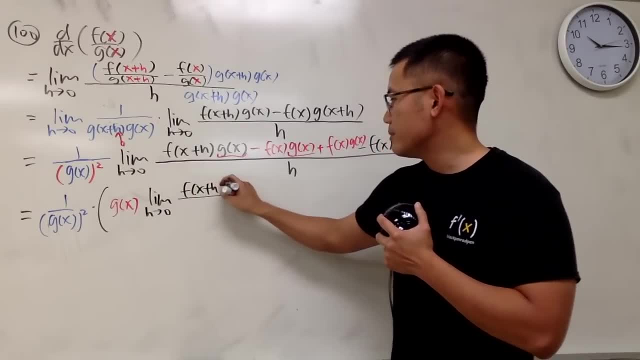 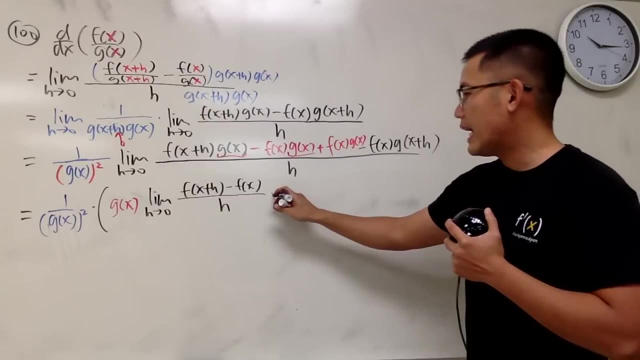 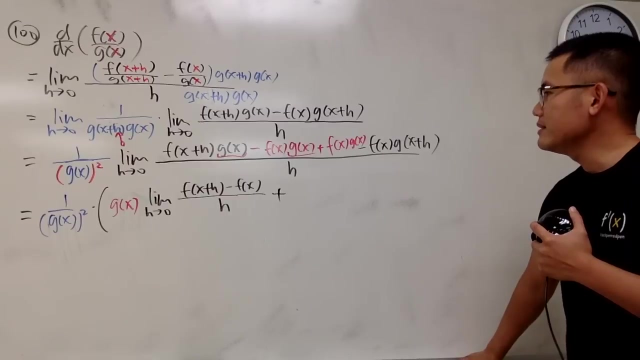 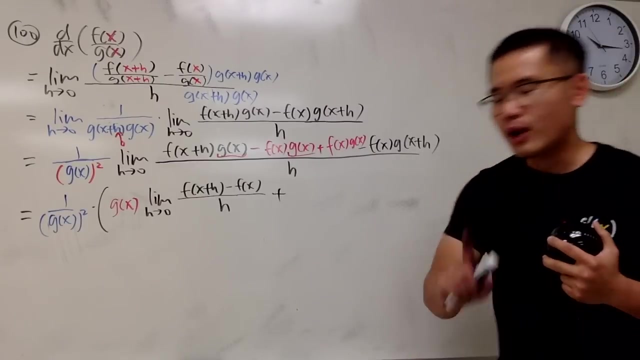 Approaching zero And we have f of x plus h minus f of x all over h. All right, Next part, we add: Why is this adding? why is this adding? uh-oh, f of x. oh, don't worry, I almost had a heart attack, okay. 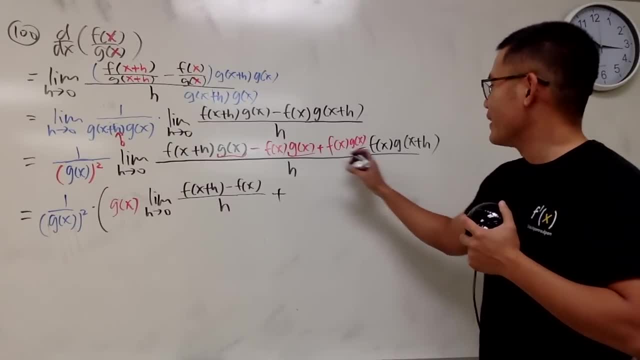 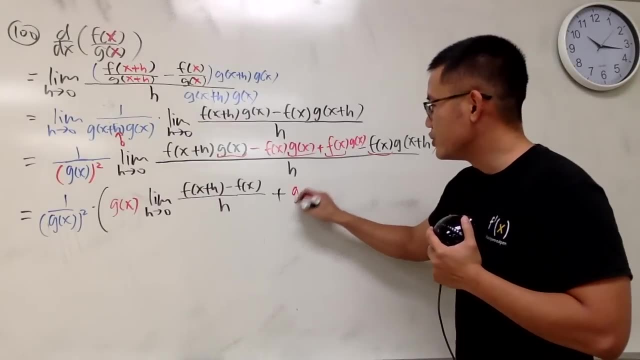 okay, okay, we're good, we're good, we're good. okay, right here, f of x and f of x. we can factor out, so we still add. okay, for now, still add this: right here is g: 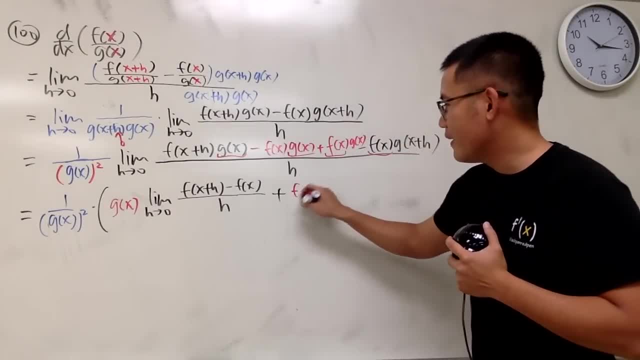 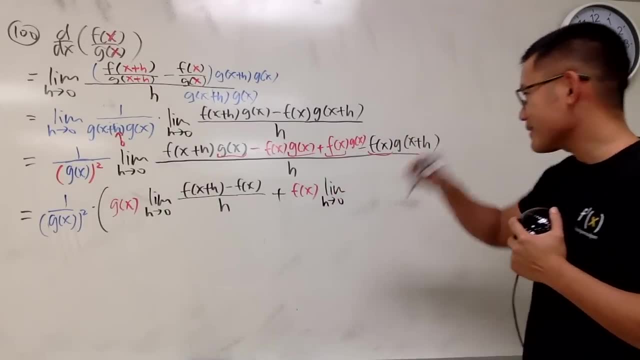 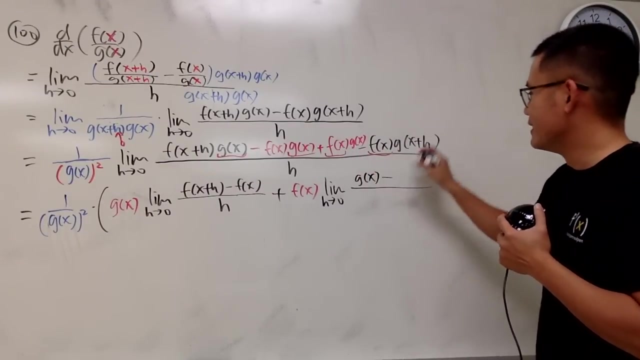 no, this, right here, is f of x, f of x, right here. okay, factor it out. and then we have the limit as h approaching 0,. now this is g of x minus g of x plus h. did you see something? 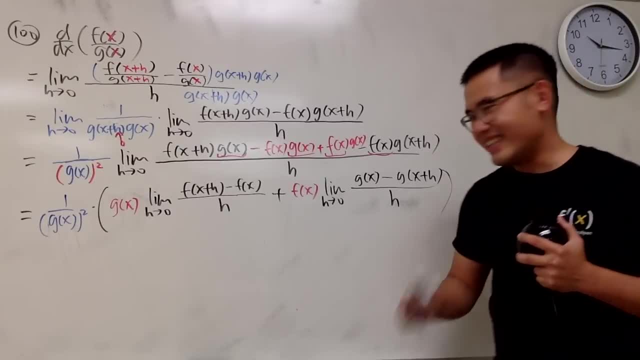 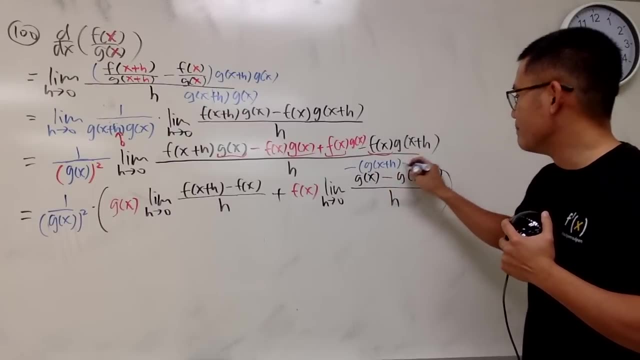 kind of weird. Yes, okay, this right here is not what we preferred. it's okay, just factor out a negative so we can get g of x plus h minus g of x. this negative man scared me all right. 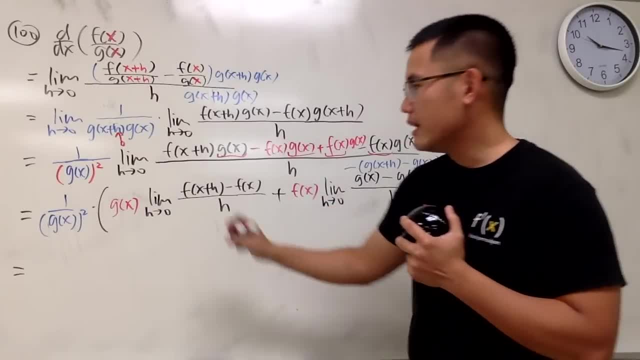 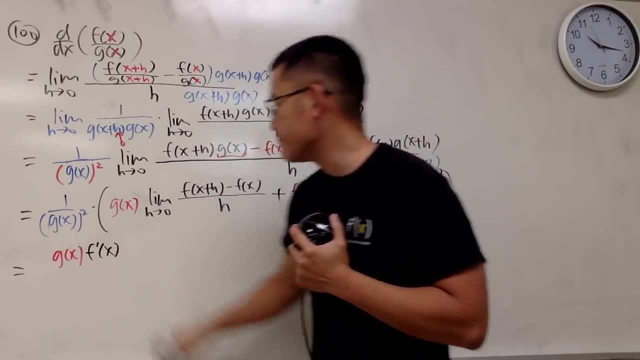 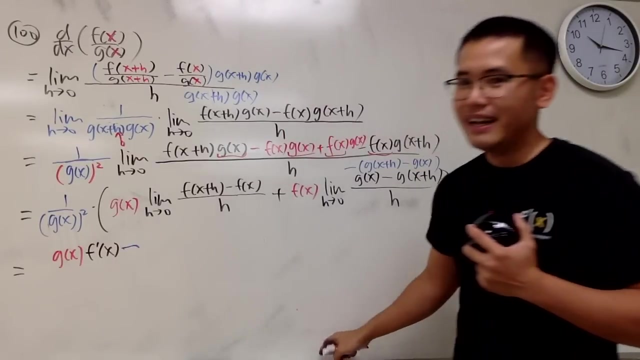 all in all, let's write down the top right here: right, so we have g of x times this right here is the derivative right, so derivative of the top. and then this right here: right, it's a minus right plus times minus, so it's a minus, and we have the function f of x. 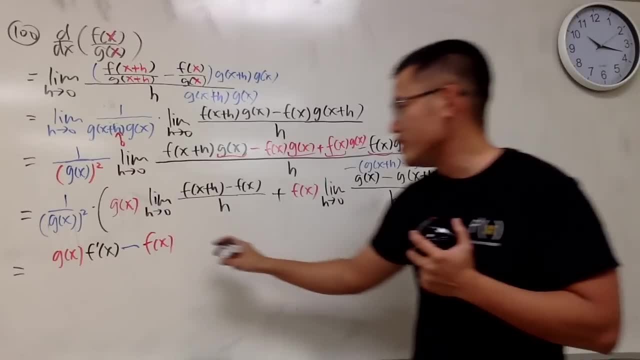 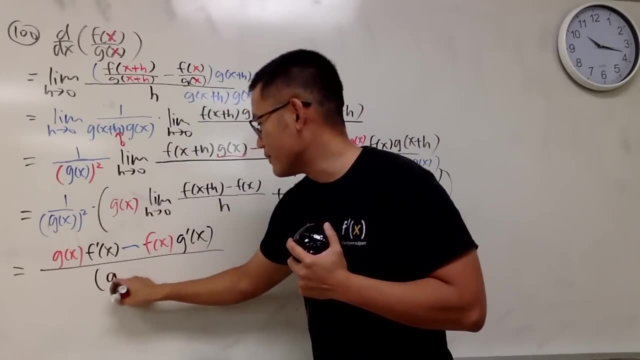 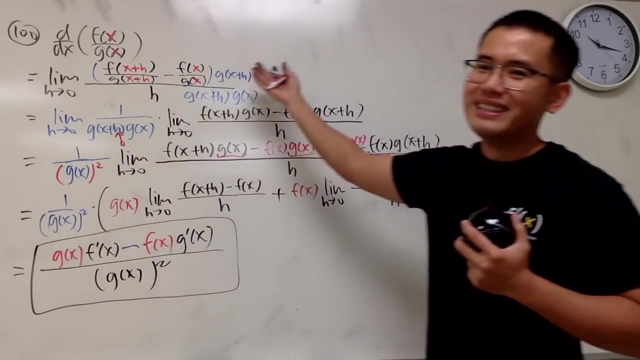 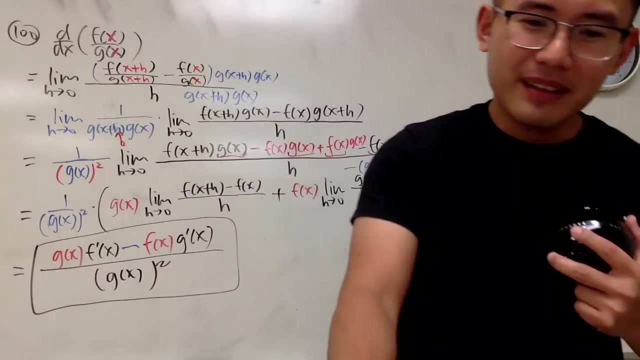 and this part right here is g, prime of x, all in all divided by the bottom function squared, and we are done. this is 100 derivatives. but you guys know I have another one for you guys. this right here, it's the adult power rule. I will try to fit in here, right. 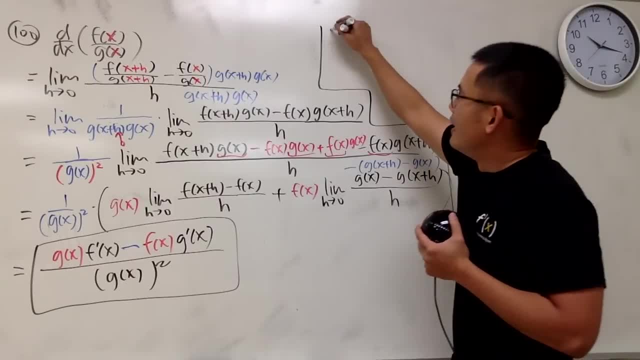 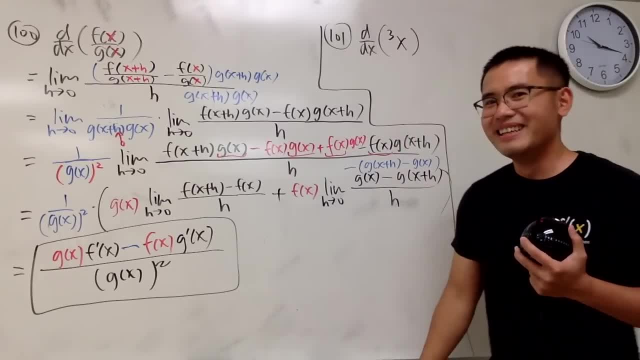 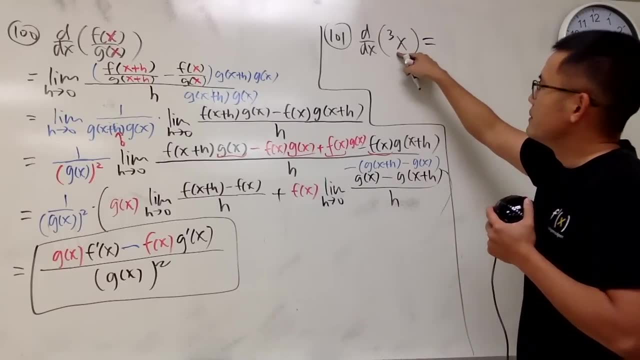 meaning that you put a 3 right here: titration okay, titration okay, don't worry. what does this mean? I will tell you. this means okay, if you have the 3 right here. it means x times, x times. 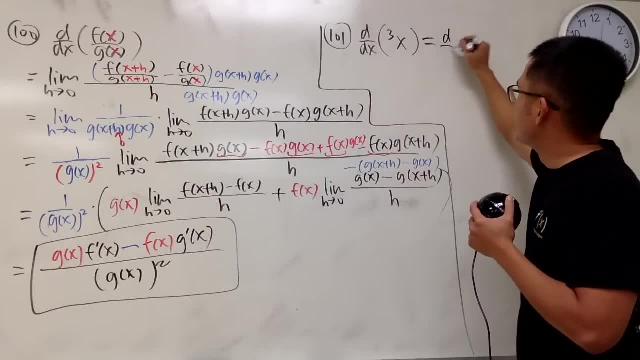 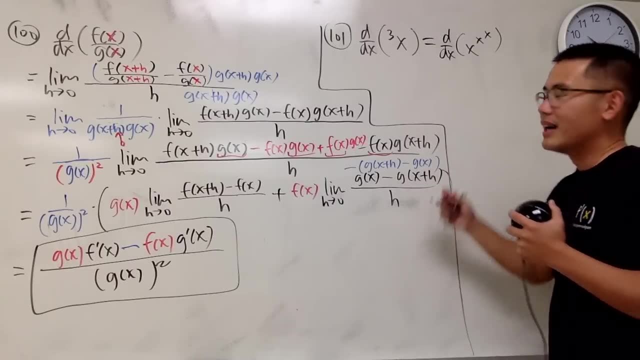 x. but when you have this 3 right here, this means we differentiate x to the x to the x power, like that right? well, again we have, the base is x. we don't like that, so we are going to look. 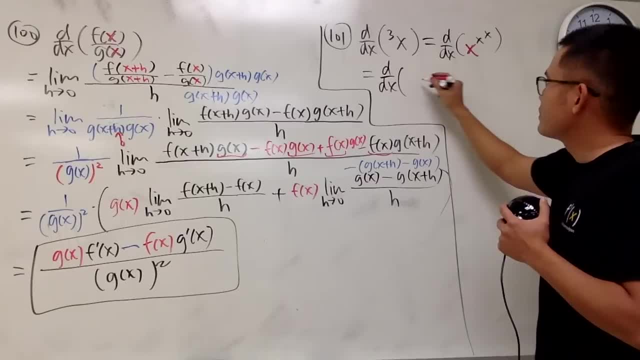 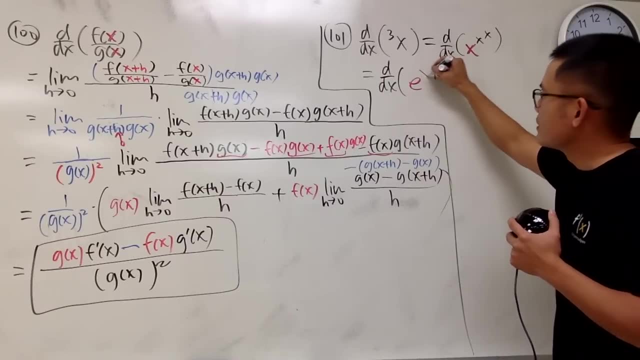 at the derivative. well, this right here is just e to the natural log of x, raised to the x to the x power, but we can put that in the front. so it's just x to x right here, like this, and now. 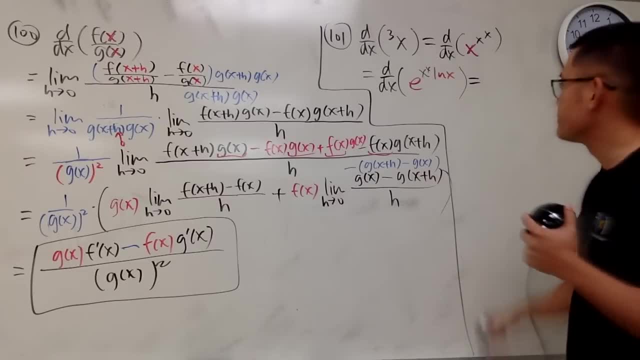 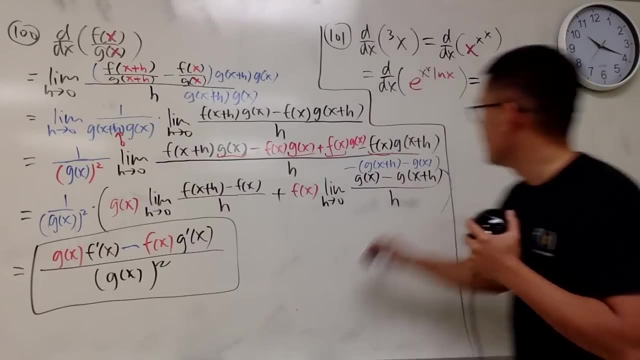 I will write this down for you. we can differentiate this guy already. perhaps I will just. I will just do it here. that's. I think I should be okay. why did I write it so big? all right again. 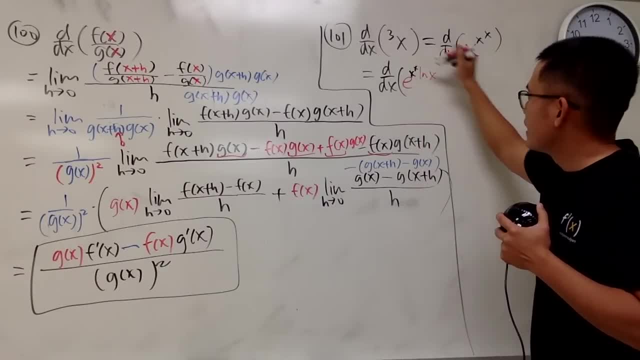 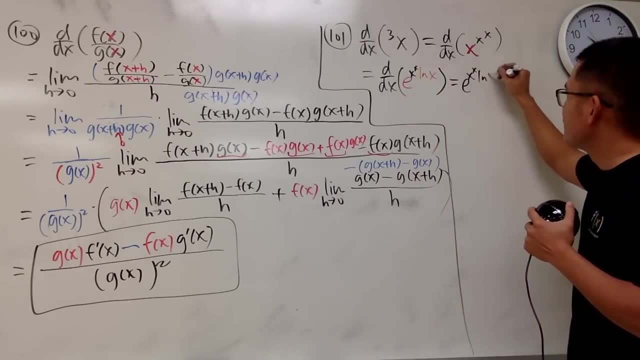 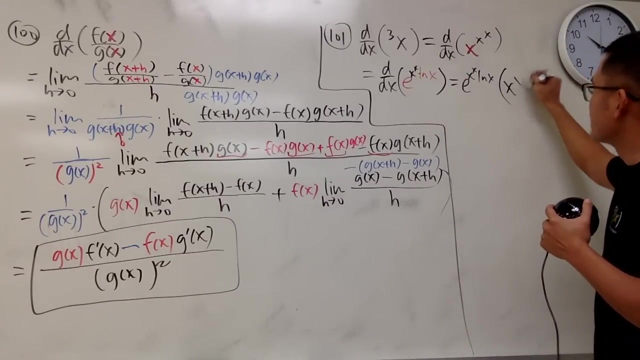 this is e to the natural log of x, and then this is x to the x. right, okay, here we go. e to the whatever, we just get the same thing right. e to the that whatever times. well, product rule in action. first one, we have x to the x, that's the first function and we multiply. 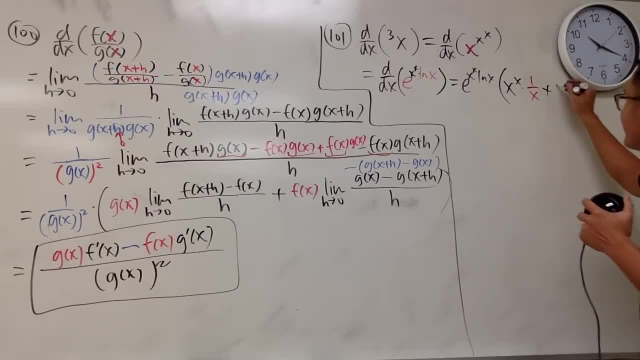 by x. and then we add the second function, which is natural log of x. but do you guys remember what's the derivative of x to the x? maybe you have to go back to watch the video. huh, I will tell you. 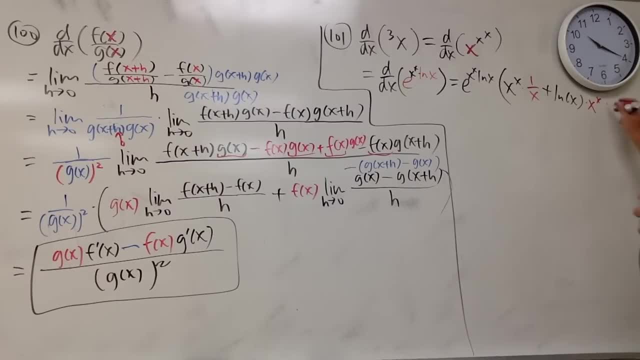 is x to the x. but this is kind of weird. it's like going down like this times that means that was e, it's 1 plus natural log of x like this. all right, so no kidding. now this right here is what. 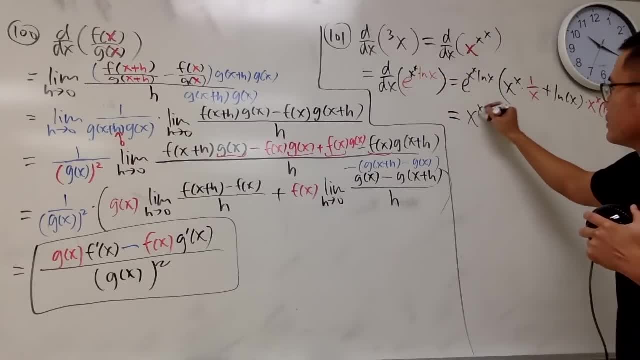 well, if you look back, it's just x to the x to the x. so this is x to the x to the x, x to the x to the x, and notice, this guy has x to the x and this guy also has x to the x. so I'm going to factor that out right here as well. 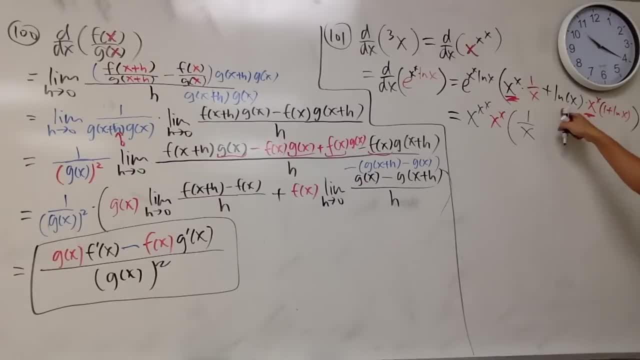 okay, right here I have 1 over x. right here I have natural log of x. perhaps I want to distribute this in so we get plus natural log of x, right, and then plus natural log of x times natural log of x. ladies and gentlemen, natural log of x, squared done. 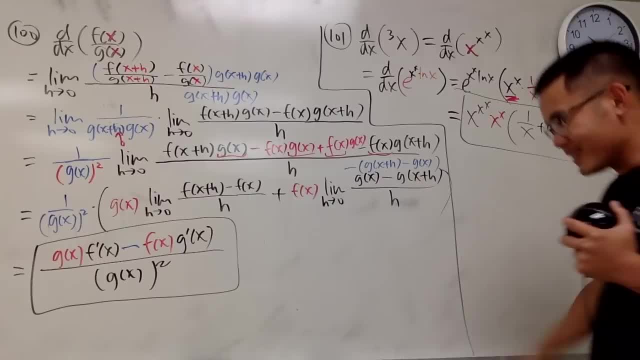 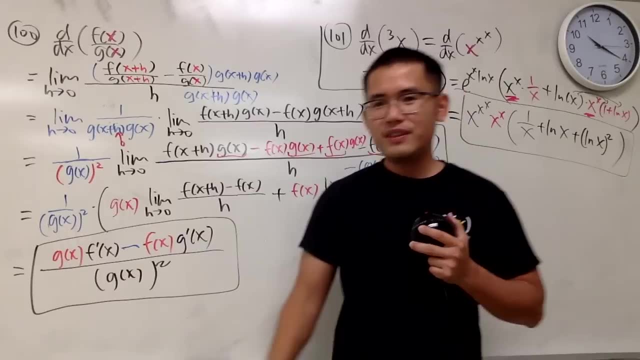 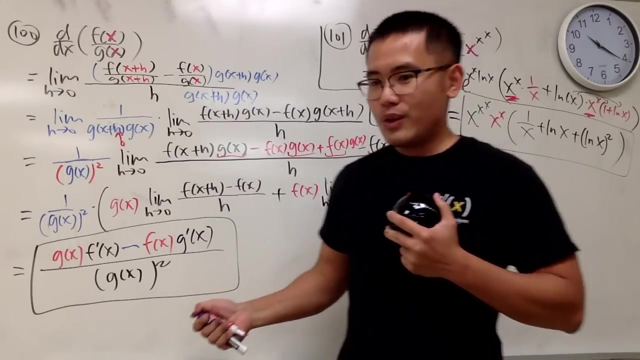 Oh my god, take a look, take a look, take a look. oh my god, I did 101 derivative. this is 6 hours and 30 minutes, the longest video I have done so far. this is man. whoa whoa. 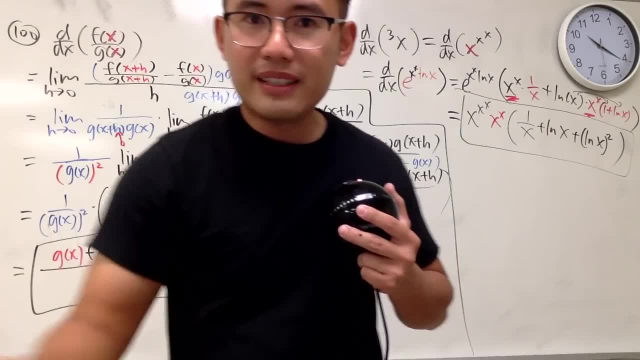 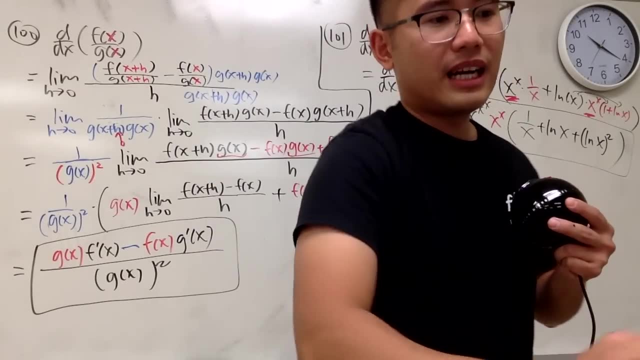 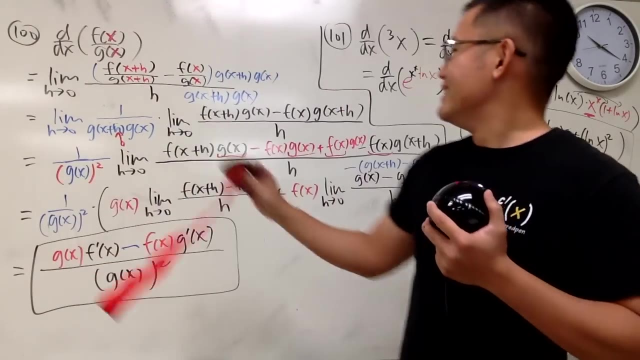 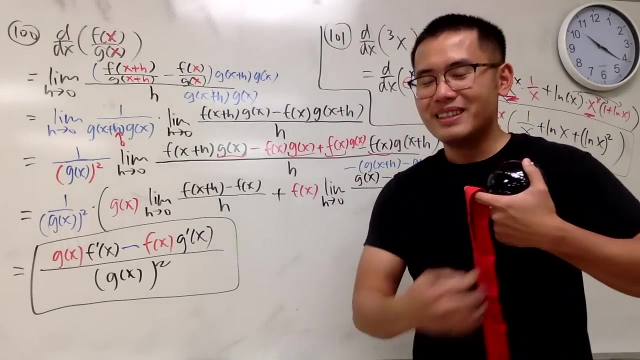 whoa, all right, thank you guys so much for watching and again download the file and I have the other file for you guys as well and of course I'm going to put down my Marisol Meadow for the 100 derivatives. so funny, this right here I was. I PR did this. 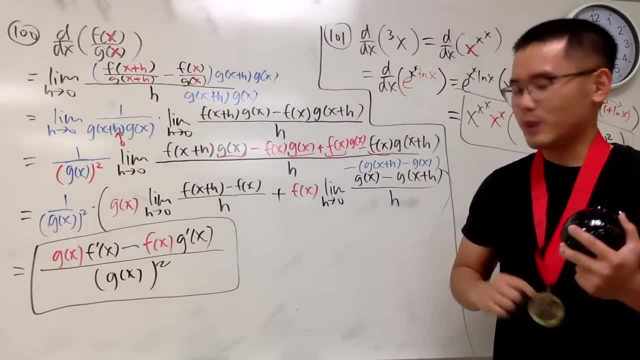 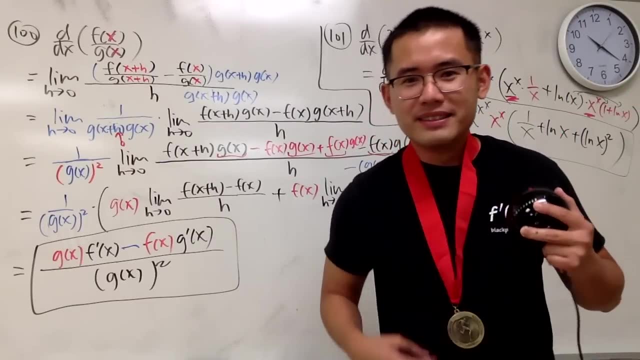 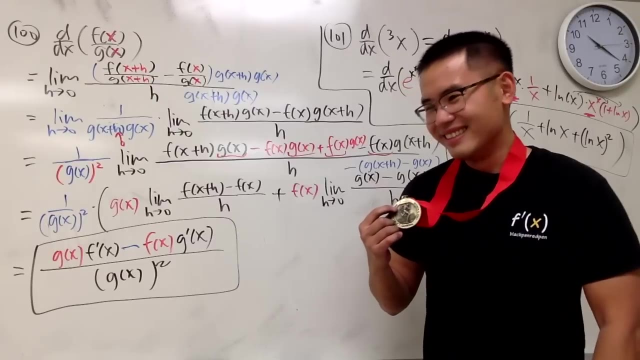 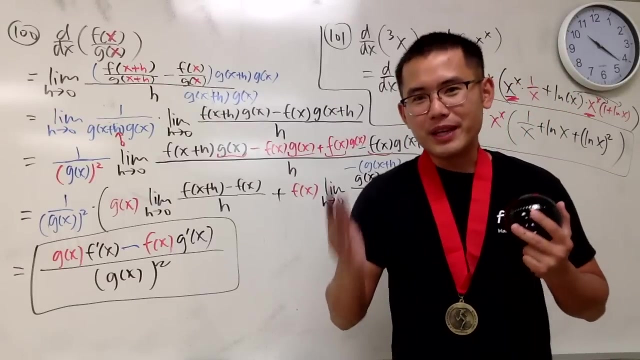 4 hours and 22 minutes or so. yeah, that was when I was much younger, and this right here. I also PR did this right here. 4 hours, I mean 6 hours and 37 minutes. Oh my god, this is just amazing. all right, so hopefully you guys all find this video to be.